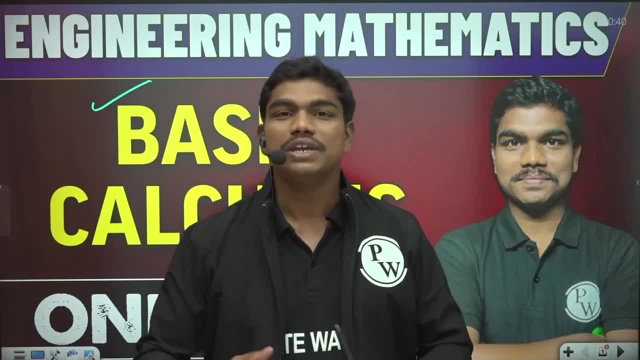 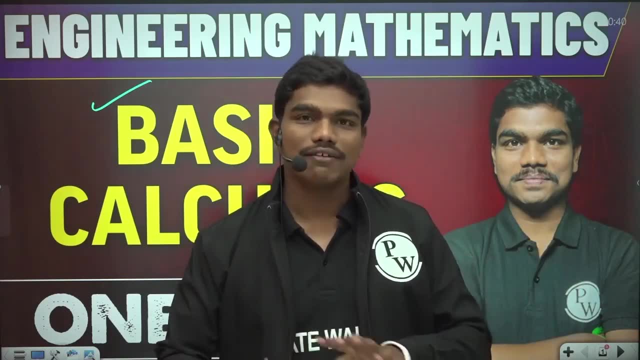 Yes, we are going to cover the complete syllabus of engineering mathematics. You are going to get every module like this, in single shot so that after some eight to nine- you know lectures from us definitely- you will have complete command over the syllabus. Okay, so this basic calculus, if you 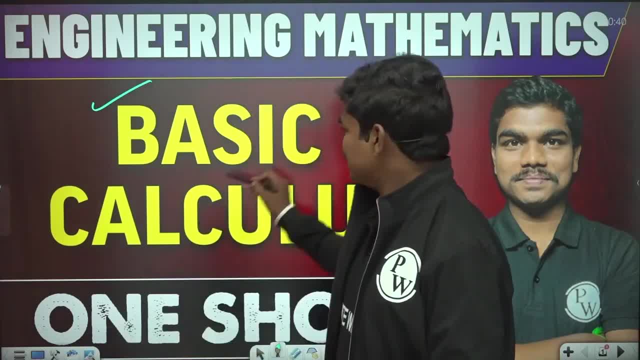 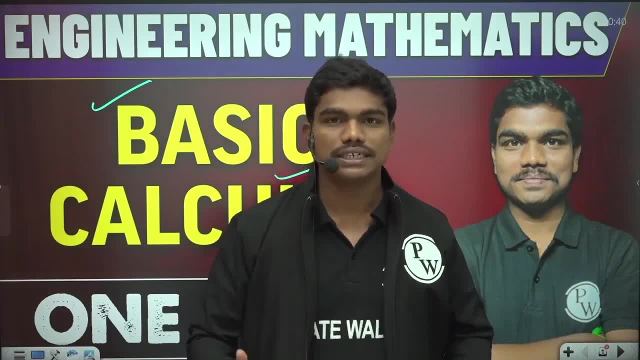 see one of my favorite chapters, actually and definitely. if you see, this basic calculus is a strong foundation for many of the technical subjects that we deal with. Okay, for example, you take any of your core subjects, you have differentiations, integrations, then after 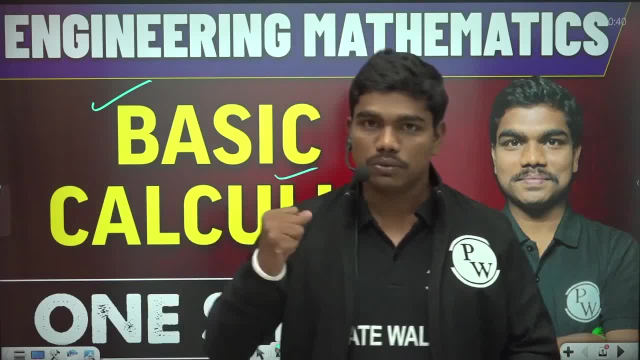 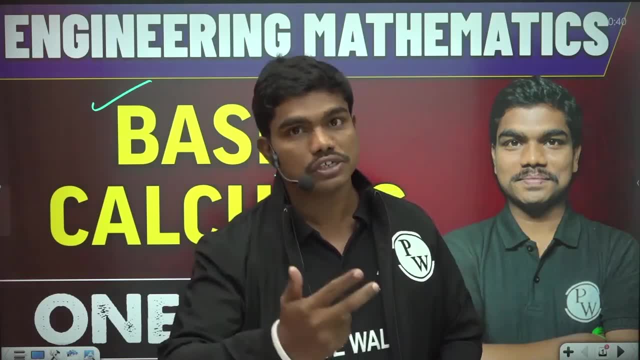 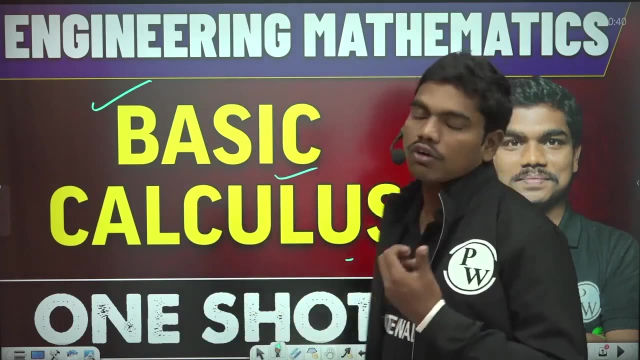 solving differential equations and this basic calculus is a strong foundation for many of the is one very basic chapter and very strong foundation for the upcoming chapters, like differential equations, vector calculus, or you say, complex calculus, or some integrations in probability, all these things. okay, so that's how this basic calculus is basically, you know. 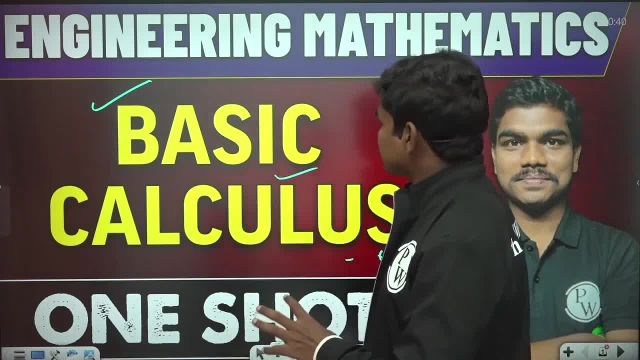 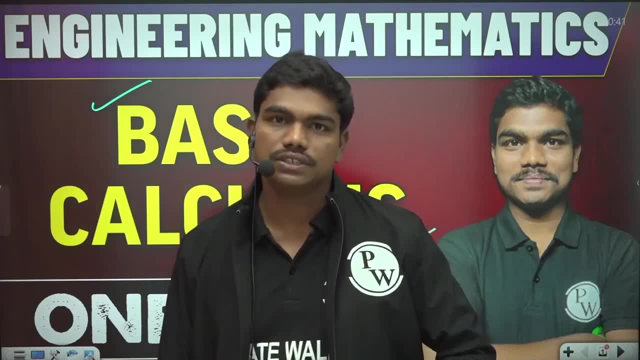 majority. it's developed by isaac newton and this basic calculus involves, you know, some of the very inceptional, i mean the fundamental themes of you know the general physics. okay, so, without any delay, let us start this module. so, before starting this module, i would like to give you some quick 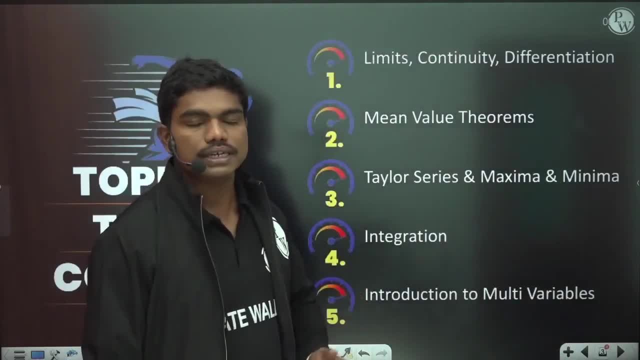 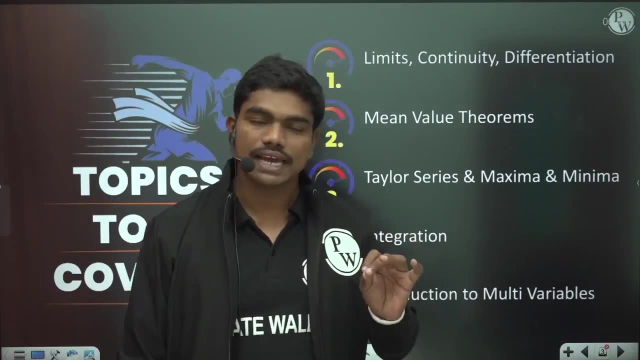 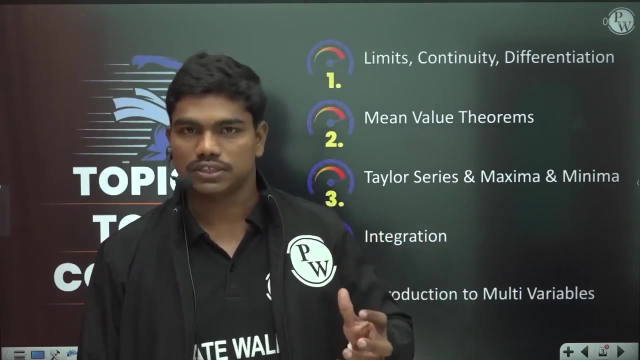 review of the topics that i'm going to cover. so basically, anyhow, i'm going to divide this lecture basically into three parts. first part, differential equations- i mean sorry, differential calculus of single variable. then integral calculus of single variable and finally i'm going to review of some multi-variable calculus also okay, like limits, uh, you know, uh, maximum in my concepts, in. 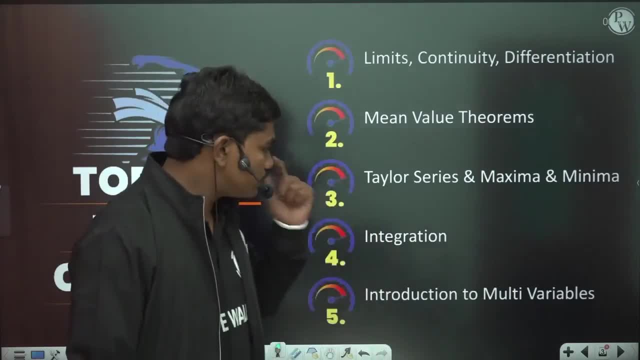 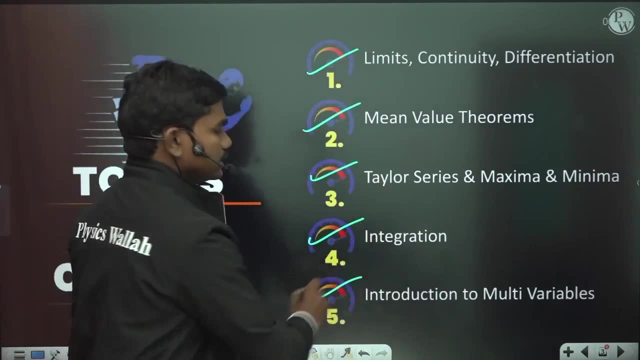 two variables, three variables will deal all these things. okay, so once we are done with that, until the end of the video, i will see you in the next video. okay, bye, bye. basically that i'm going to cover in differential calculus and this is basically integral calculus and this is i'll talk about some multi-variables, uh calculus in this video. okay, so without any. 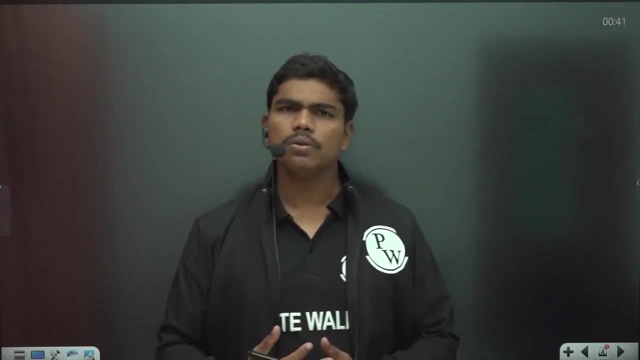 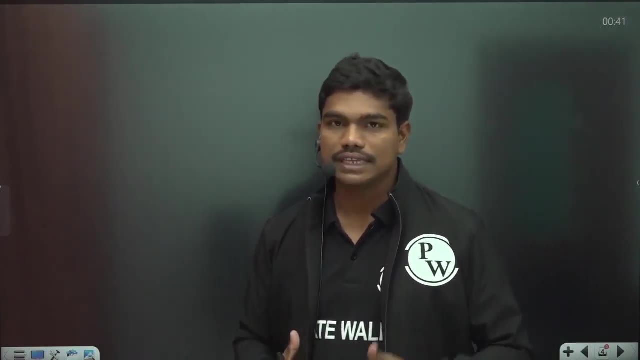 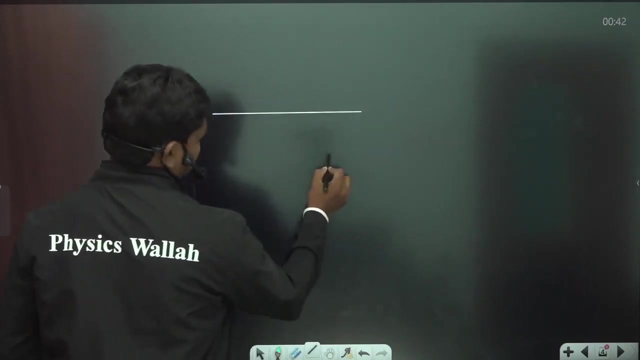 delay, let us start the sessions. so first, why we need to build these fundamentals? because we have seen it's quite often that we deal with differential equations correct in our day-to-day physics. as i told you in the first. uh, generally i say: if you see, let us suppose. if you have any block, for example, 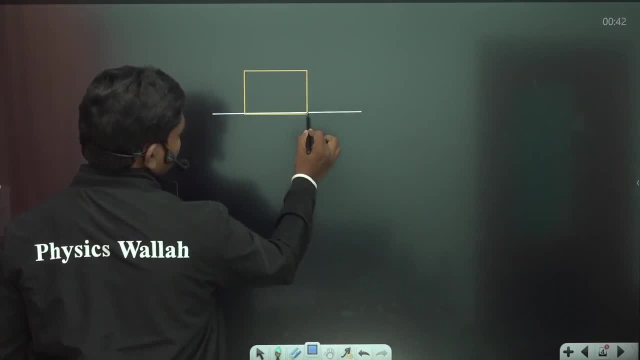 okay, let us suppose i'm giving some simple class 12 level example, class 11 level. so let us suppose if this is a block, on this block you are applying some force f. okay, so you have applied a force f on this block m, for example. then what happens? obviously the physics that we can understand is: 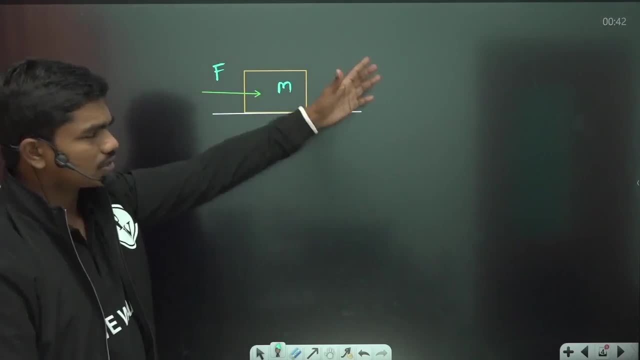 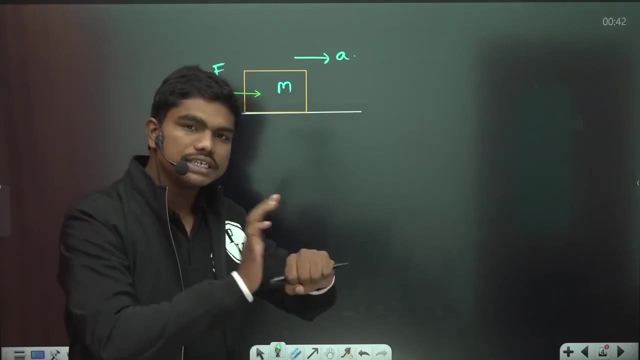 when you apply certain force on a mass m, this mass will accelerate, correct? so this block will try to move with certain acceleration. so this is the physics that's happening. so there is a block, you are pushing it, the block is moving. now, if you want to understand, or if i ask you this question, 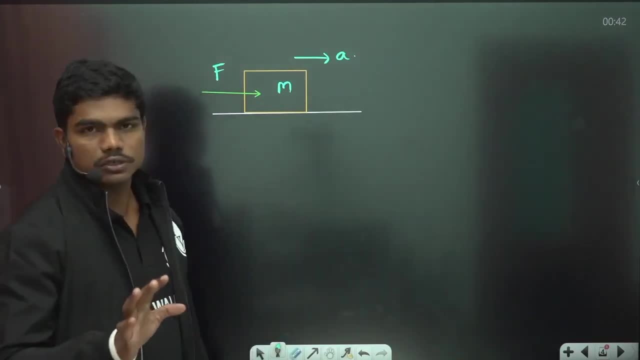 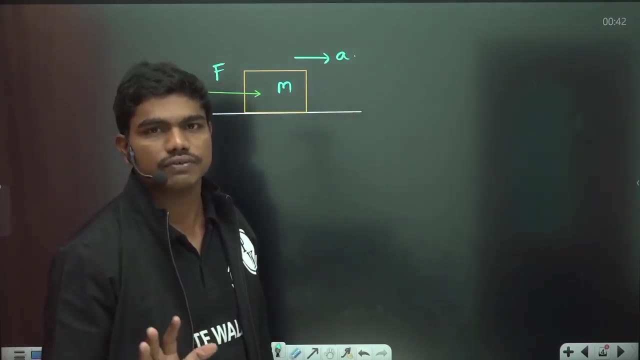 let us suppose initially, at time t equal to zero means initially, this block is at rest. then after what time this block will have a velocity of two meters per second, if i ask you this question, for example. okay, you know that this block starts from west and it accelerates. now if i ask you this, 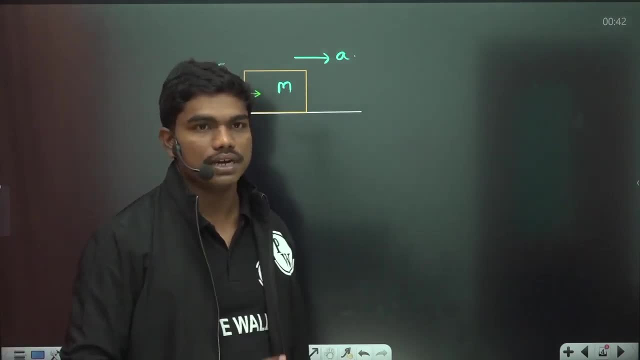 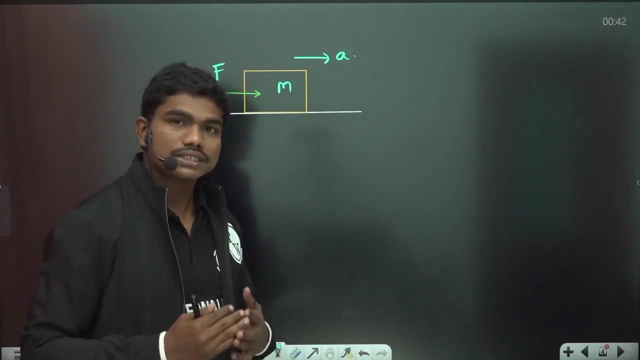 question after what time this block will have two meters per second, for example? let us say so now. just by looking at this physics, you cannot answer this question correct. you need to do some mathematical calculations. so basically, every physical phenomena has to be converted to some mathematical equations. 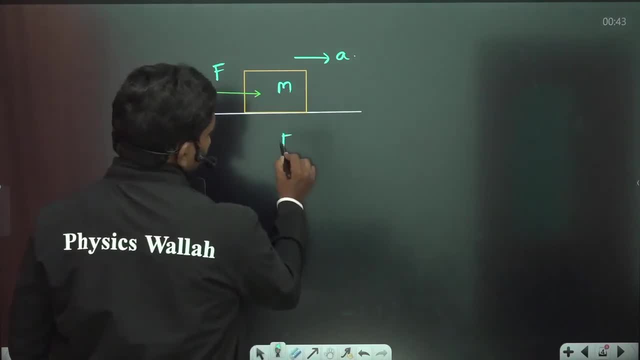 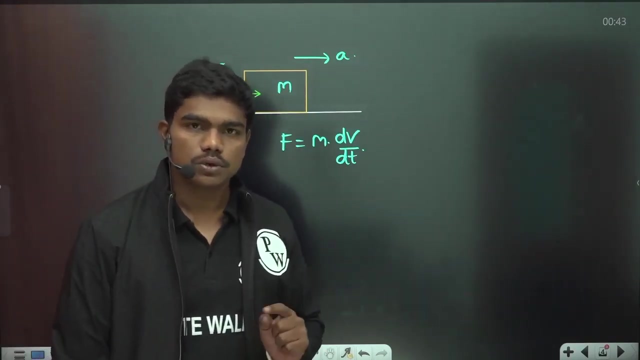 for our understanding. so, similarly, we will come to know that f is equal to m into dv, by dt, so mass into acceleration, and you know acceleration is nothing but a rate of change of velocity. so now, if you see, you will come to know that this is a differential equation, correct? so not only this, like this in many 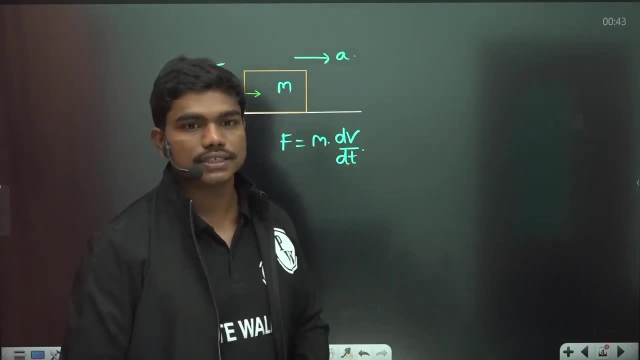 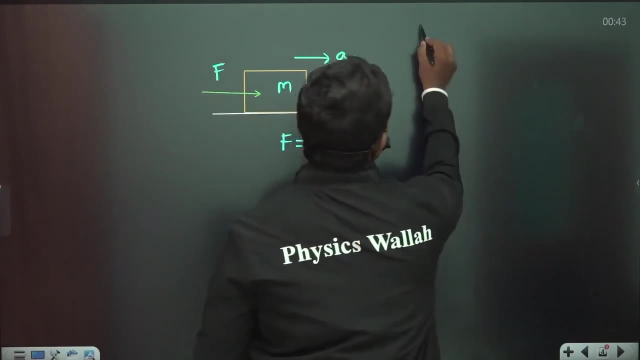 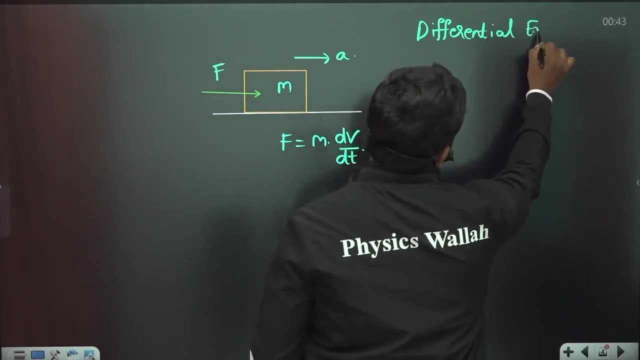 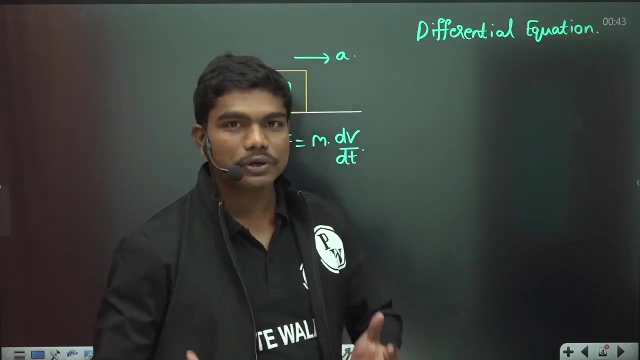 situations we generally come across. many parts of calculus actually, and differential equations is one very important domain of calculus actually. okay, now to solve differential equations. let us end it up with a differential equation, for example, differential equation. okay, so to solve this differential equation, definitely you should know integration correct, because if you can, if you want, 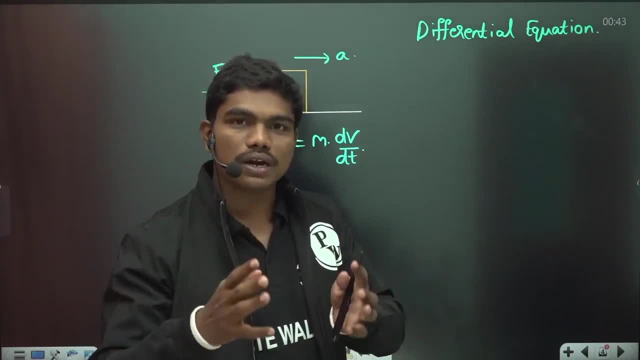 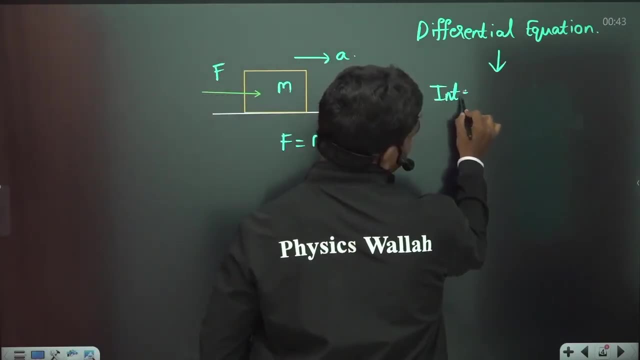 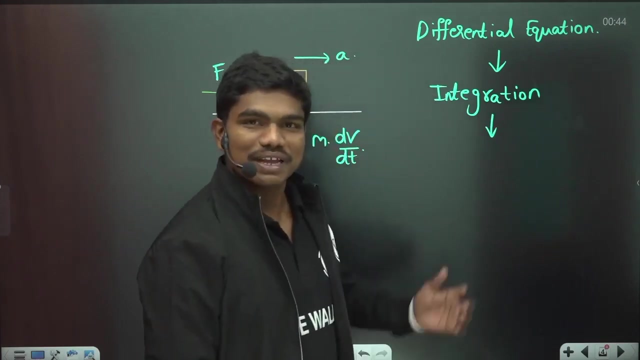 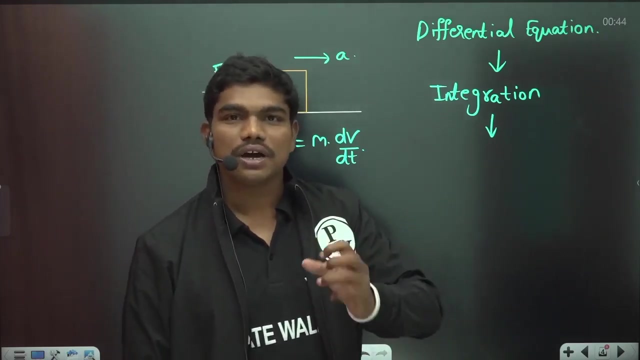 to do solve some differential equations, then definitely you should know what are the integrals of some functions. okay, so to solve differential equations we have to know something on this integration, integration- if you want to talk something about integration, then definitely should know what is differentiation correct, because if i ask you what is integral of sine x, your answer is minus cos x, because you know. 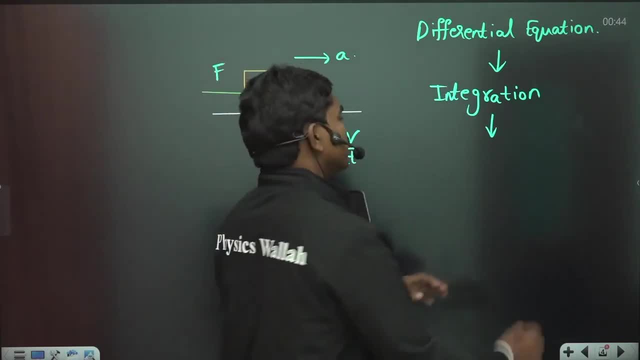 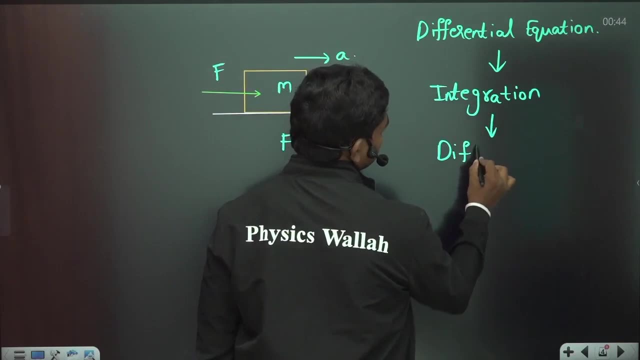 that differentiation of cos x is minus sine x, correct. so that's why, anyhow, we'll see how those things are coming. so in integration, if you want to talk about integration, you need to know what is differentiation means. basically, you should know what is a derivative. so once you know, 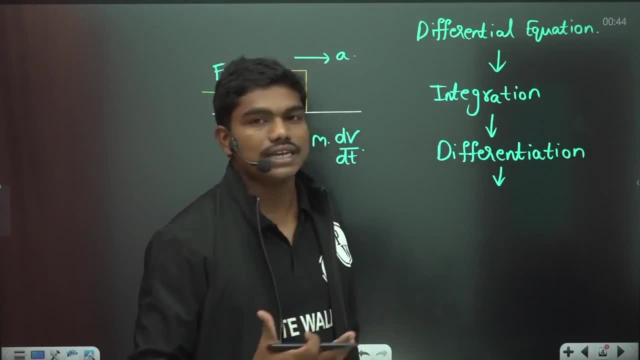 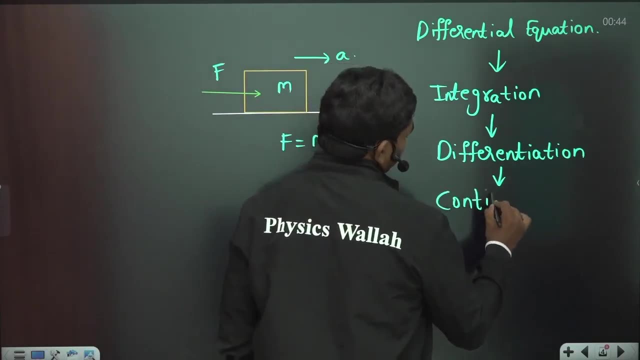 what is differentiation means? basically, if you want to know what is differentiation, actually, you need to know where two very important concepts which are called continuity and limits. continuity and, of course, for knowing continuity, you should know what is a limit. now, to know what is a limit, basically, okay, we need to know one very, very important concept, which is called neighborhood. 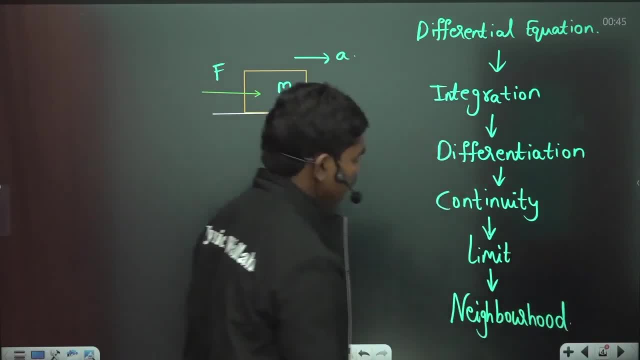 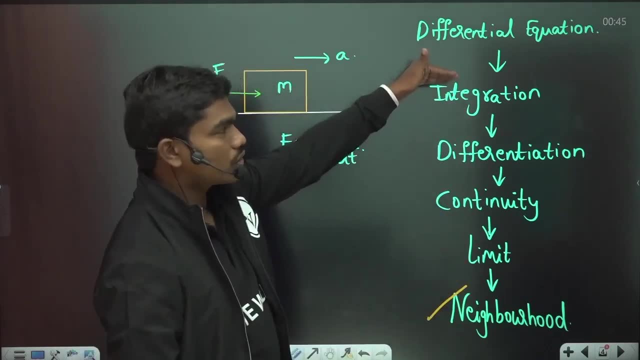 neighborhood, okay. so we will start our discussion from this point: neighborhood, okay. so eventually we'll go till this part in this module and we'll have a separate module for differential equations, because that's quite a big, uh, you know- domain in mathematics. so that's why, if you see, we'll take the uh, this in. 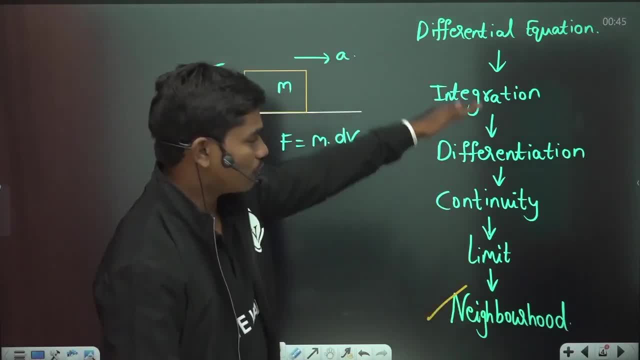 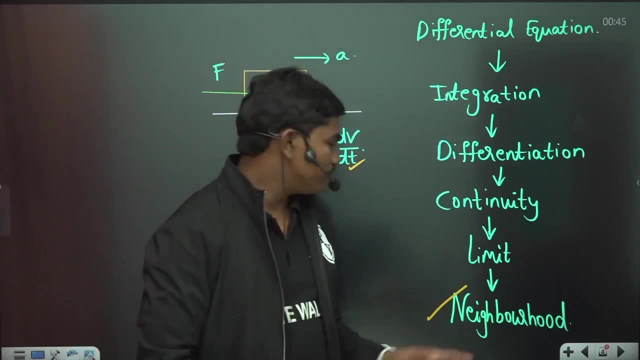 this module we'll take here so that, once acquiring knowledge of all these five or six- you can say- subtopics, we will get to know how to solve this differential equation. okay, so basically, we'll start, start this differential- uh, start this module by understanding what is a neighborhood. okay, now, 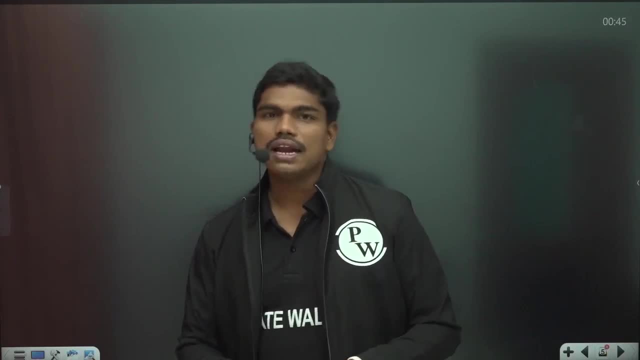 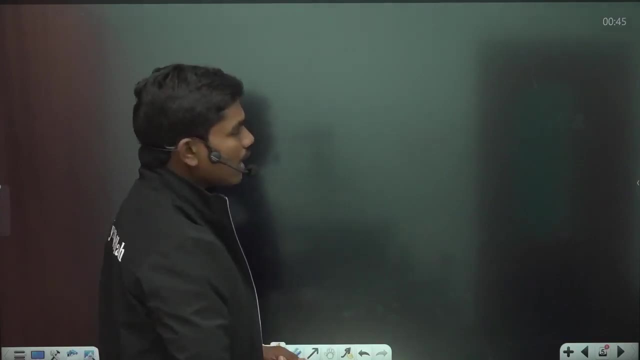 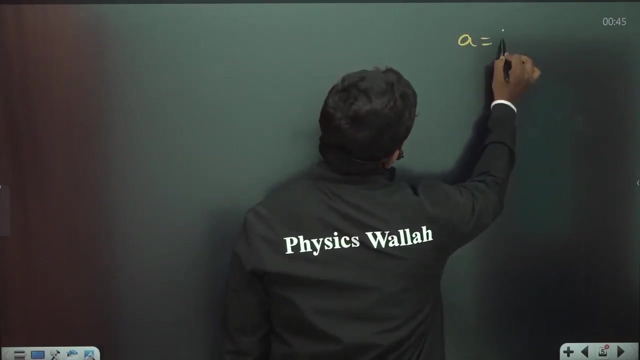 before i speak something about neighborhood, i'll ask you something. look, let us suppose i'm writing some two thick- uh you know four or five steps here, basically, and i'll ask you to identify what is the wrong step. okay, you can pause the video and you can try to attempt. look, for example: let a is equal. 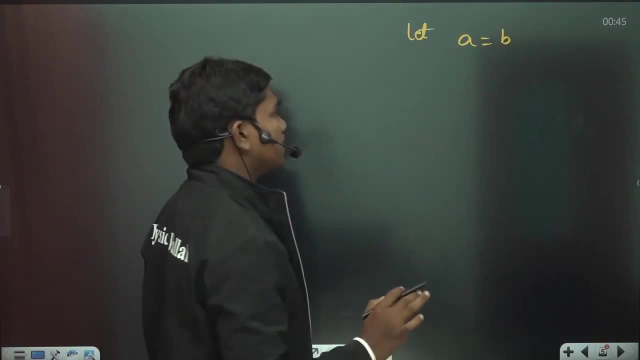 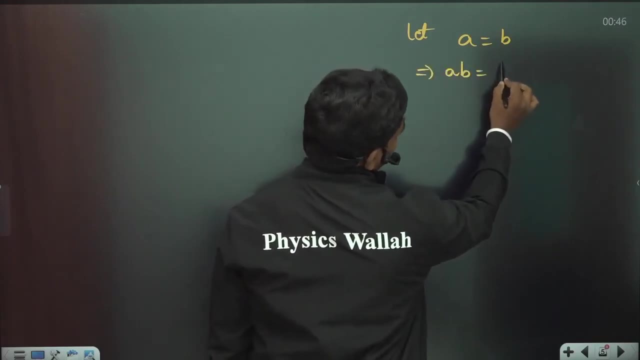 to b. okay, let us suppose i'm writing that let a is equal to b, for example, there are two numbers. i'm taking them equal, so whenever they are equal, i can write a, b is equal to b square. i can write this: if a- b is equal to b square, i can write: a square minus a. b is equal to a square minus b square. 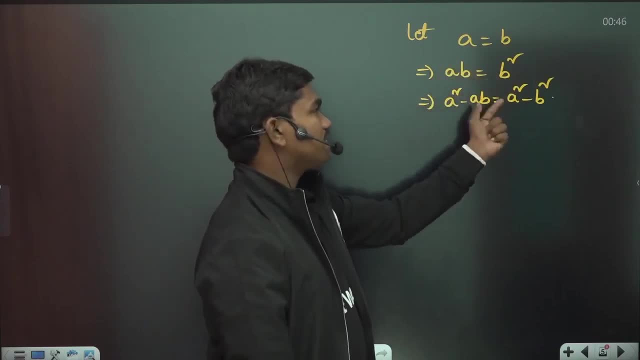 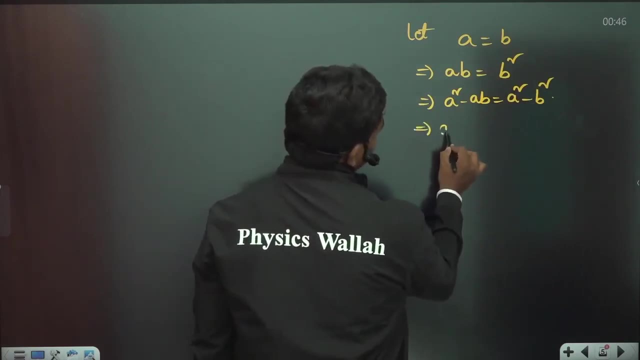 correct. i can write, because if a, b and b square, both are same. then if i subtract a, b from a square, or if i subtract b square from a square, both are same, correct. so now let us suppose i am taking a common and write a minus b. here also i am factorizing a. 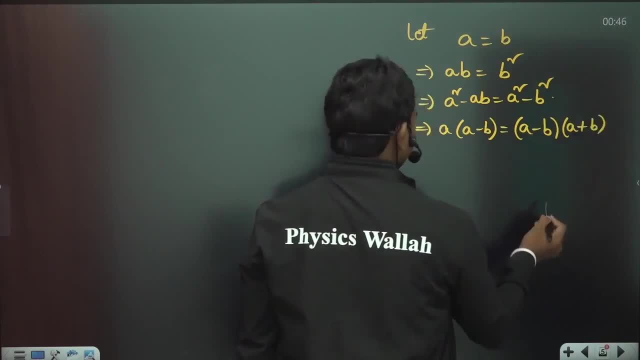 minus b into a plus b. okay, so now, if you see, i'm cancelling the common factor a minus b, so a is equal to a plus b. this is what we have. okay, now, since a is equal to b, i'm substituting this b, uh, as a. basically, okay, so a is equal to a plus. since b is same as a, i'm replacing this. 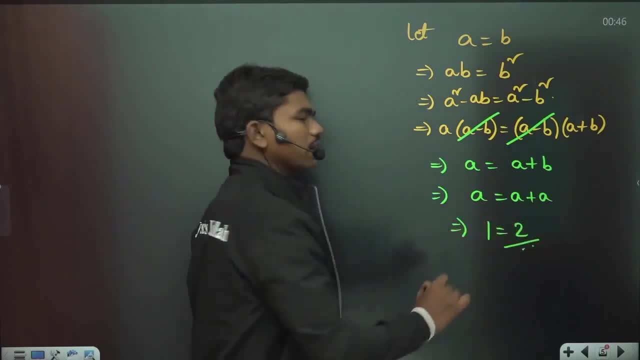 so you will get: 1 is equal to 2, basically okay, but of course you know this result is pretty much wrong, so definitely i might have considered- or maybe you might not have considered that. you know this result is pretty much wrong, so definitely i might have considered. 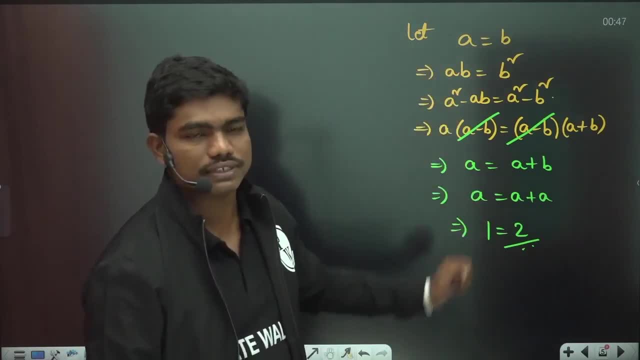 I might have committed one mistake in out of this, six steps, six to seven steps, okay, So what is the mistake that they have committed? Okay, so I request you to pause the video for a while and answer this question. Okay, Now, if you see, the mistake that I have committed here is: 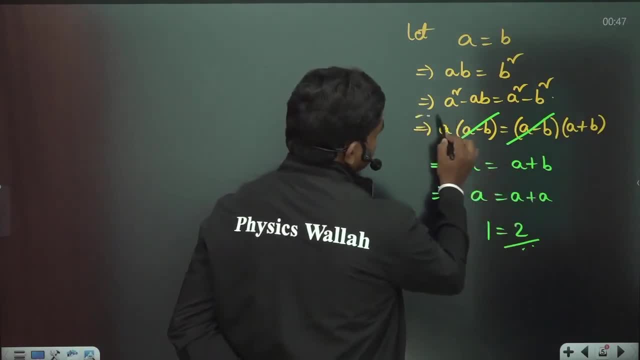 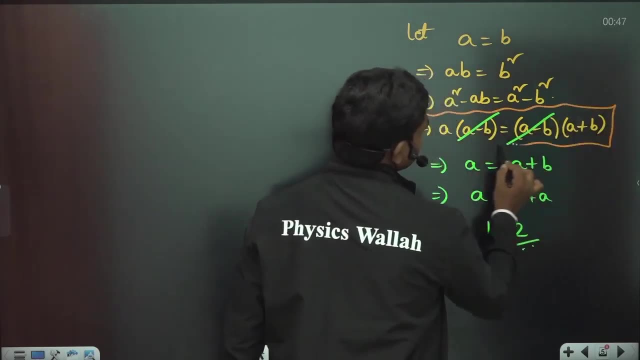 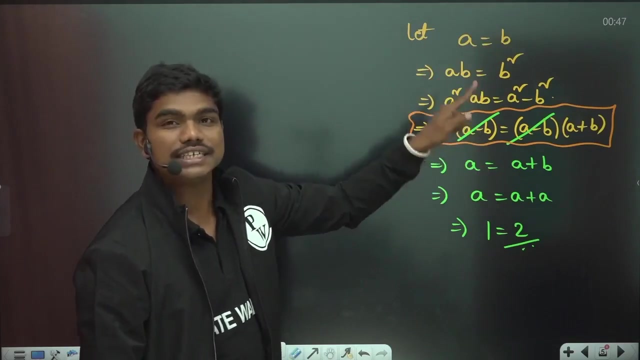 Look, the mistake that I have compared here is: this is basically in this system. The mistake that I have committed is basically in this step. So what is the mistake I have committed? look: whenever a is exactly equal to b, a minus b is actually zero. okay, so i cannot cancel two zeros. 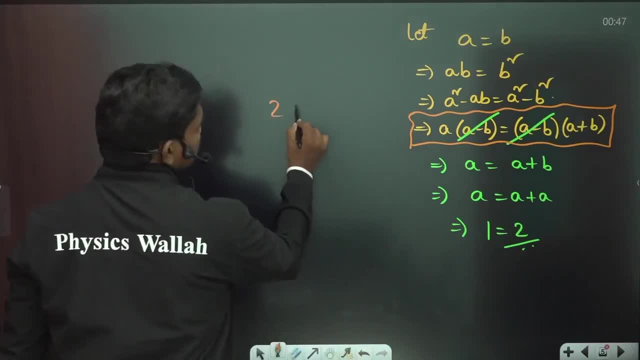 correct, because what happens if i cancel two zeros? i can write two into zero is equal to three into zero, and i can cancel zero and zero. i can write two is equal to three. but this is wrong, actually correct, you know. so that's the reason: two zeros cannot be cancelled, but actually i have cancelled. 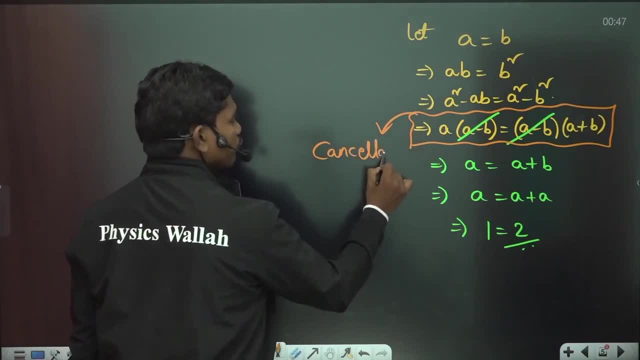 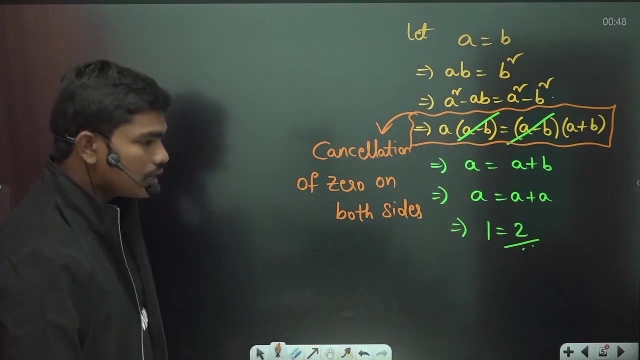 two zeros here. cancellation of zero on both sides. cancellation of zero on both sides actually gave me this result, which is not we are certain to see in mathematics. but i will tell you something you all have done: this example that, let us suppose, if i write this, x tends to 2, x square minus 4. 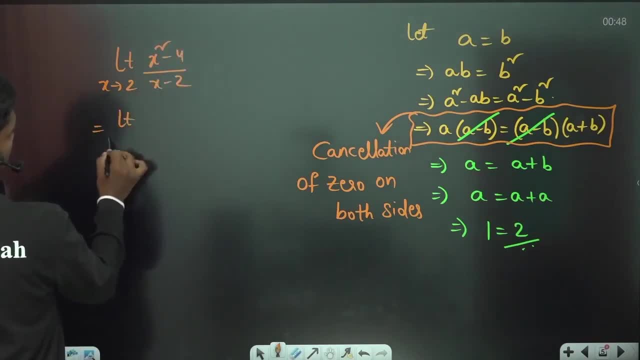 by x minus 2. let us suppose if i write this limit, x tends to 2, you will find that i will be able to find the state of this problem. so let us try to solve it and we will see what we are going to do next. so let us start with this. 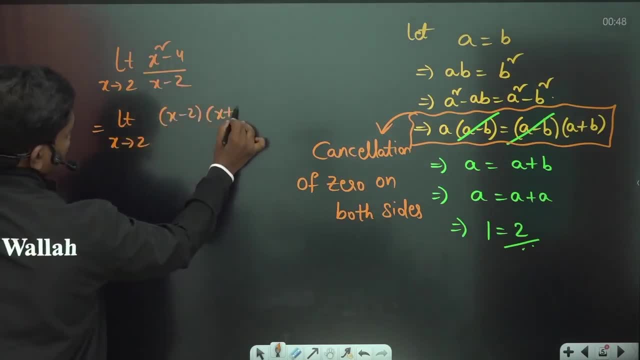 factorize this as x minus 2 into x plus 2 divided by x minus 2. now what you will do? you will cancel this x minus 2 and x minus 2. then you will get this result: limit x tends to 2, x plus 2, which. 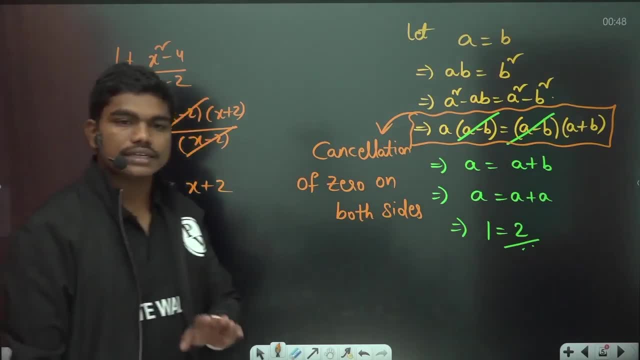 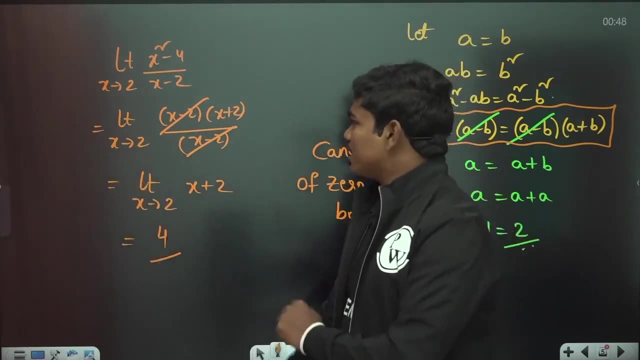 you will write as 4, correct. you have done this calculation. of course, i will tell you why this is coming and all don't worry if you, some of you- are from plus 1 or 10th class level, don't worry, i'll tell you what is this? okay now, first thing, one thing is very clear: that two zeros cannot be. 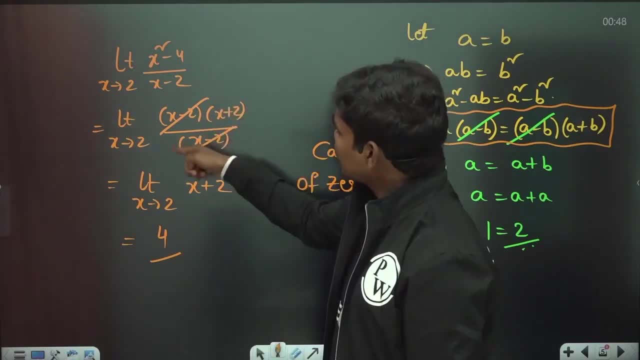 canceled. okay, two zeros cannot be canceled, so you have canceled these two. which means one thing is very clear: when two zeros cannot be canceled, but still you are canceling these two, that means x minus 2 is not equal to 0. this much you know now. this means x is not equal to 2. okay, fine, x is not. 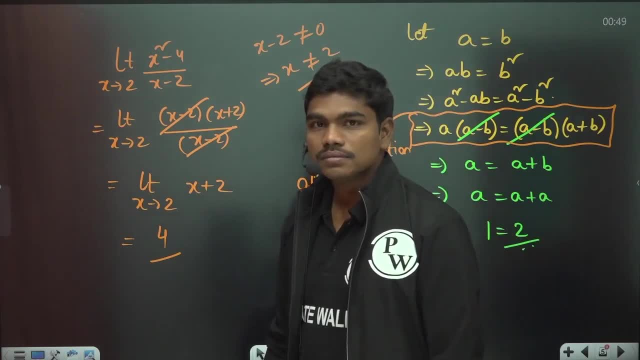 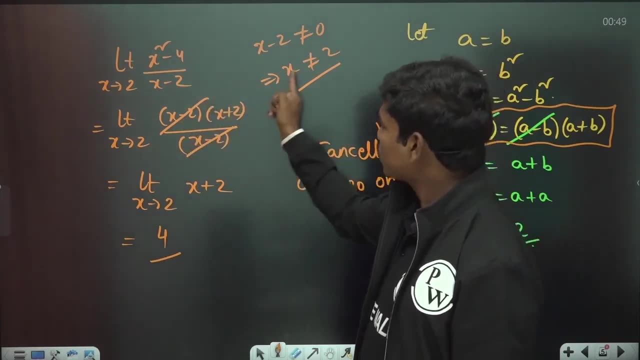 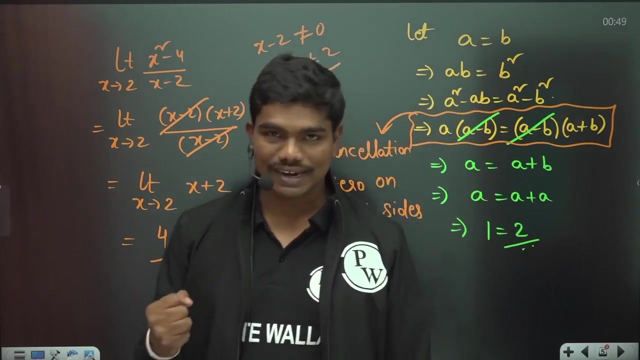 equal to 2, then why are you substituting x equal to 2 again here? tell me, here, tell this step. you clear that this x is not equal to 2. good, then why you are substituting again x equal to 2. so this is why you should know the concept of neighborhood, actually, and the definition of limit. okay, so here. 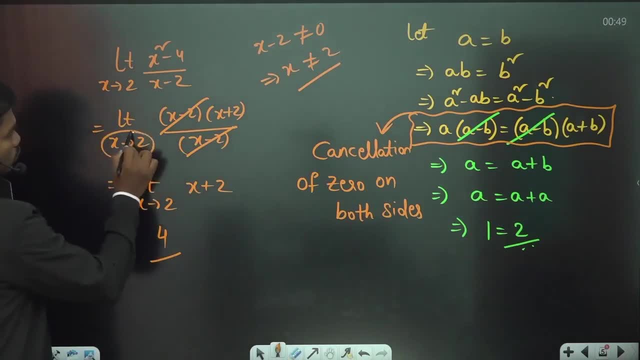 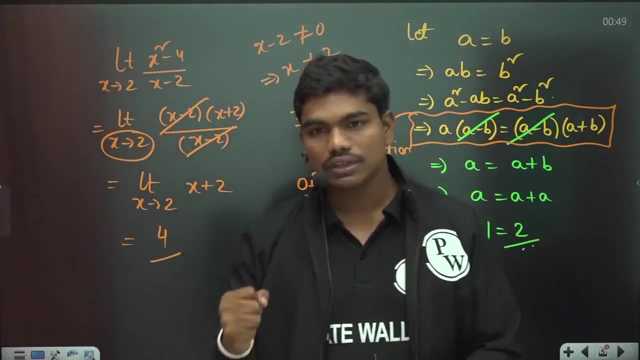 there is very much difference between x tends to 2 and x equal to 2, okay, so both are not same actually here. so that's why, if you see, we have to study the concept of neighborhood and in neighborhood we will come to know what is this meaning of x tends to 2, okay. 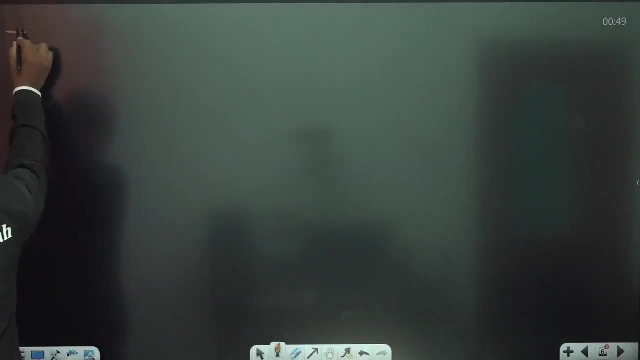 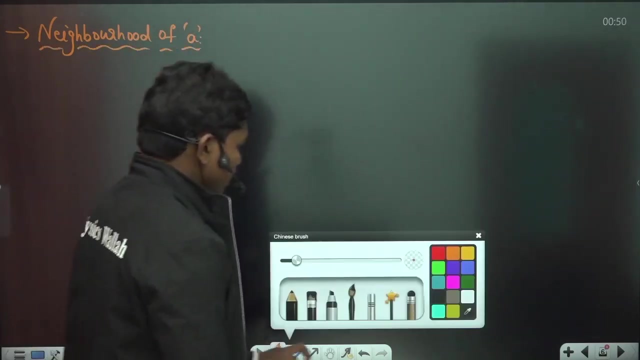 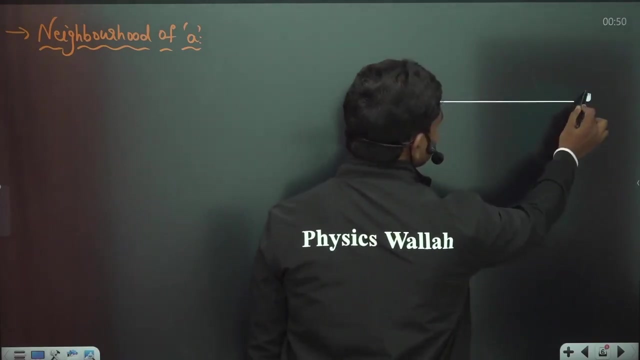 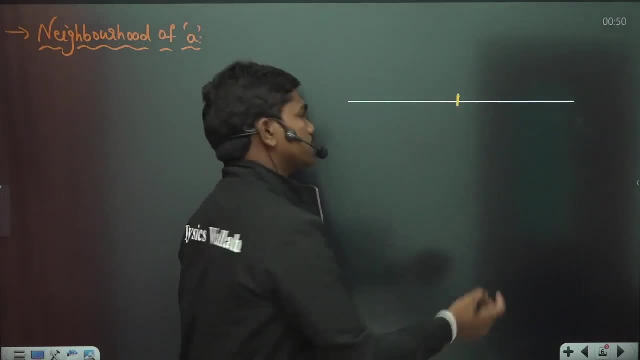 example. okay, this is your home. for example, my name is venice, so let us call v, so this is your home. so then what happens? the people who are immediately next to us are called neighbors of us, correct? similarly, someone who is here is also neighbors, but someone who is very far away, he is not a neighbor. you know this correct? now let us. 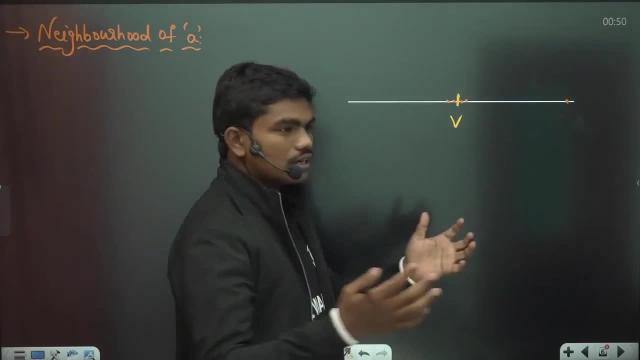 suppose you have some function in your home, then what you will do, you will call certain people as neighbors, depending upon your closeness with them or depending upon the budget for the function. so, depending on certain parameters, you decide some limit, some range up to which you should call them. 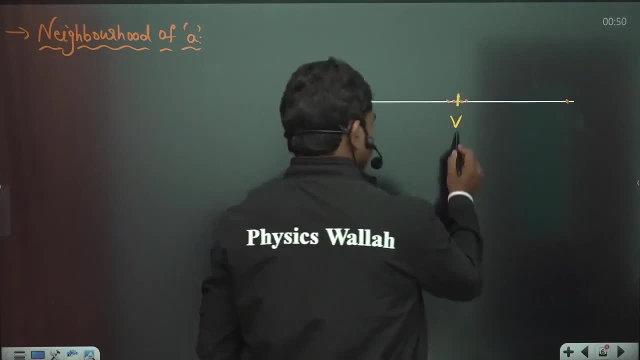 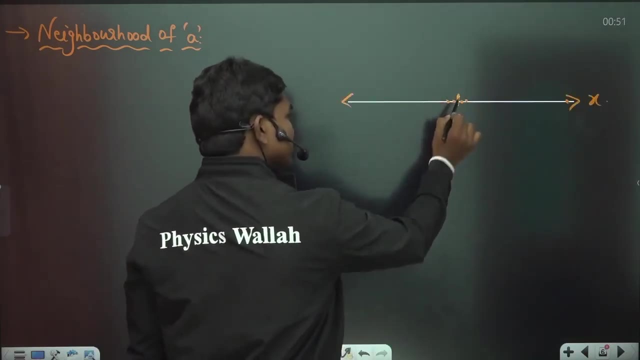 for the function correct. similarly, if this is my x-axis, let us say then if you have a real number a, then definitely there could be some real numbers which are very close to a correct. a minus one will be here somewhere very far away. a minus one is not a neighbor of a, because you know between any 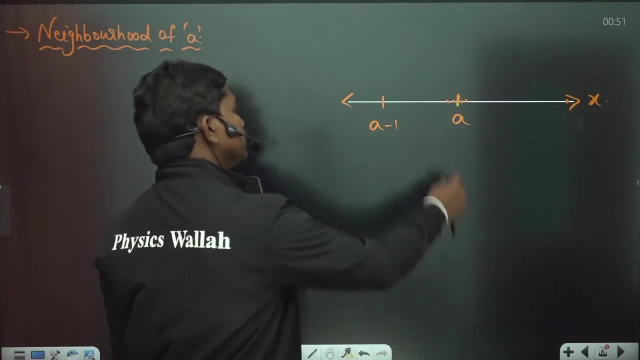 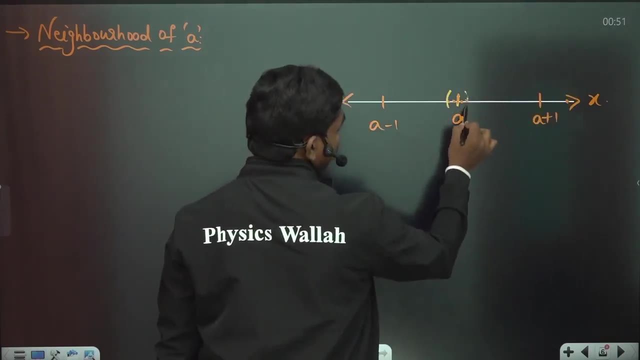 two real numbers. there are infinitely many real numbers, so that's why these two are the real numbers, are very far away. similarly, a plus one is also somewhere far away, but there are some real numbers which are very close to this, a correct. so let us suppose, if i divide this, if i write this value of x: 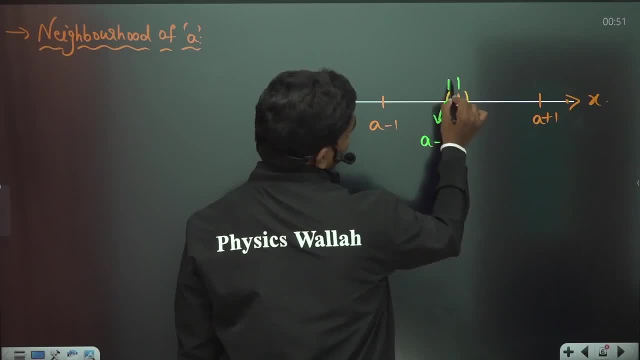 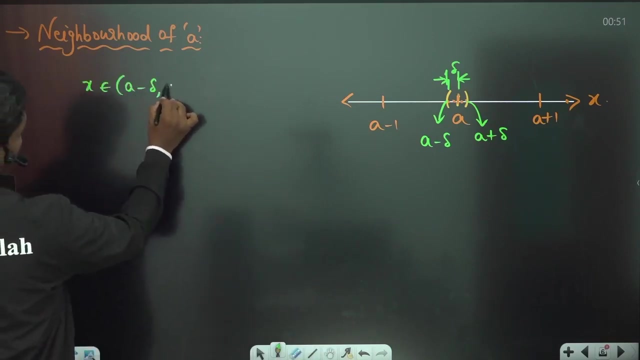 as a minus delta means assuming this: this space is delta, this space is delta, and similarly this value as a plus delta. then you can observe one thing: if i write x belongs to a minus delta comma. a plus delta where delta is some positive number, but very small, okay. where delta is greater than zero, but delta is very small, okay, very, very small. so where? 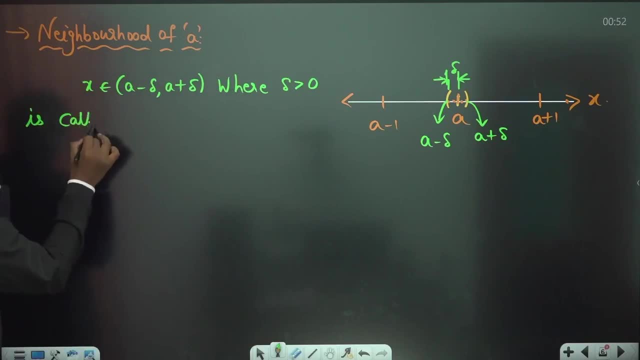 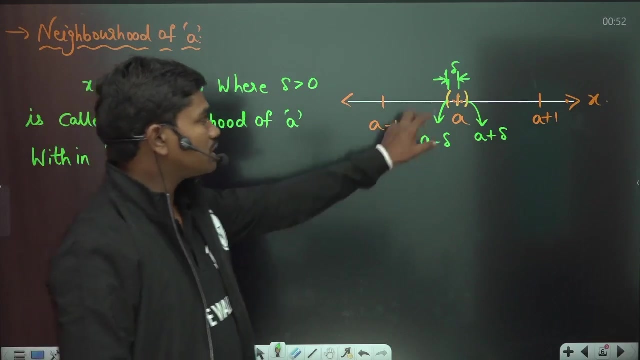 delta greater than zero is called neighborhood of a, neighborhood of a within delta limits. within delta limits. within delta limits. okay. so why i am writing delta limits? because if i change this length of delta or if i change the value of delta, then definitely the interval link increases, or? 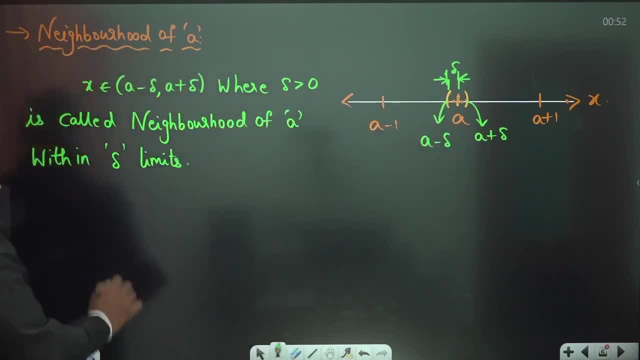 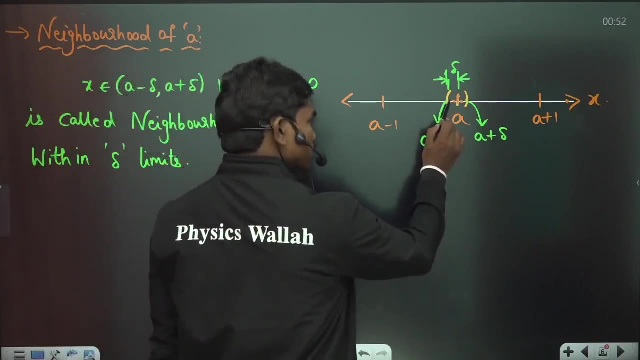 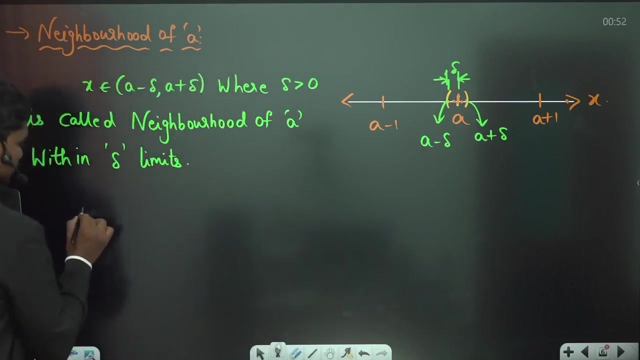 decreases depending upon the variation of delta. okay, so this is called neighborhood of delta. so when i write x tends to a, the meaning is x is in the neighborhood of a and it is moving towards. that is the meaning of this. okay, so when i say, if i say x tends to a, 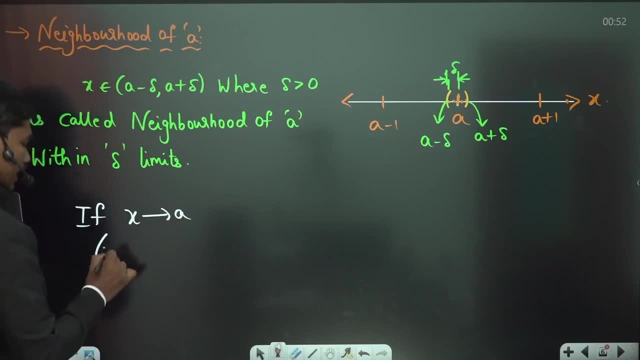 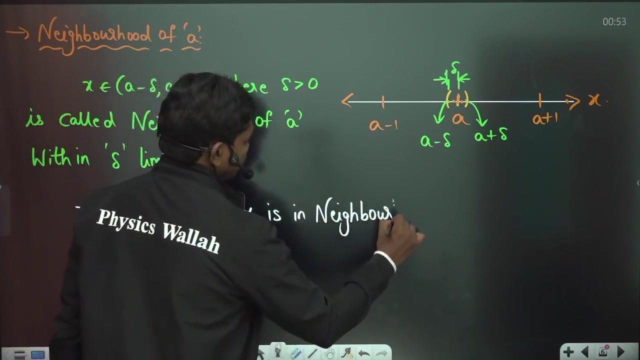 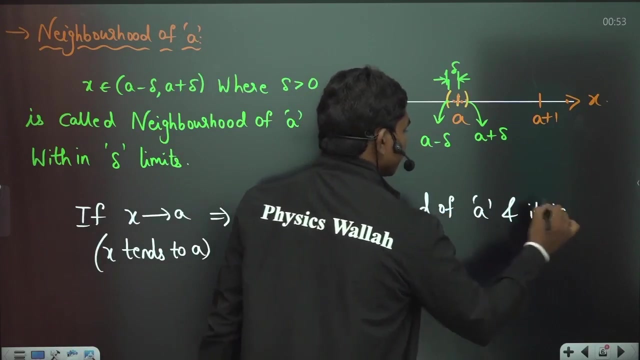 if we x tends to a, this is read as x tends to a. basically okay, so x tends to a. then this implies x is in neighborhood of a, x is in neighborhood of a, x is in neighborhood of a and it is moving towards a and it is moving towards. 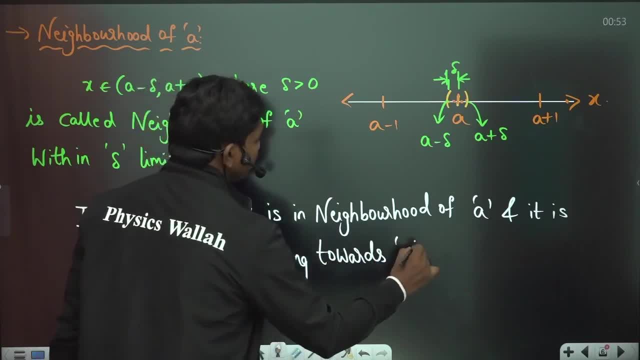 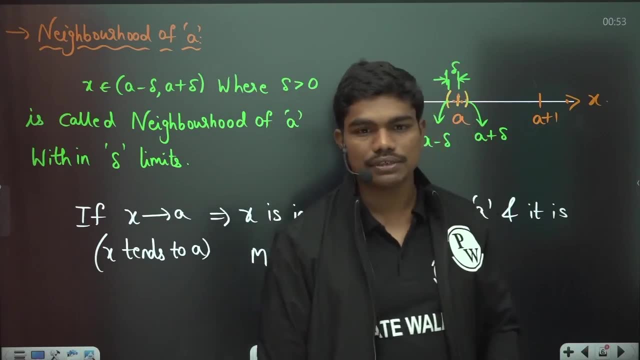 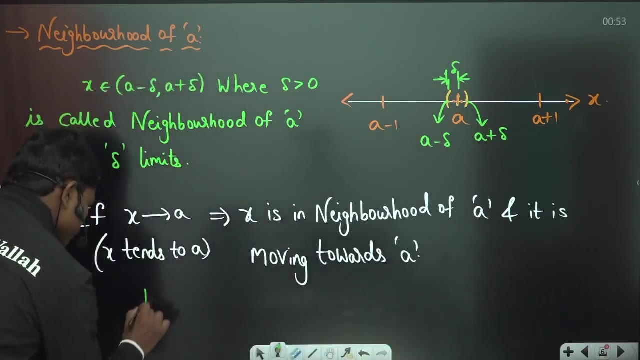 it is moving towards a. this is the meaning of neighborhood, basically okay. or x tends to a. basically now there is something called deleted neighborhood, okay. so what is this deleted neighborhood? so deleted neighborhood. if i write in a simple sentence: deleted neighborhood is nothing but deleted neighborhood. neighborhood is nothing but x belongs to. 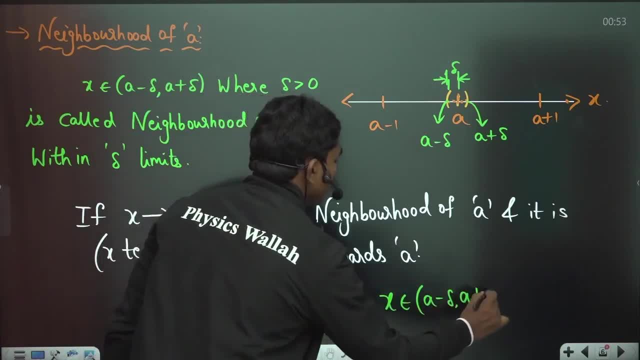 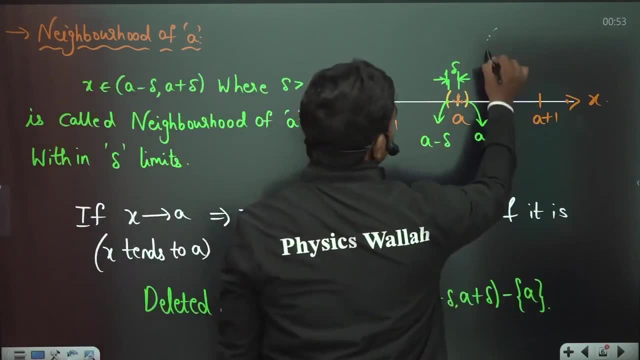 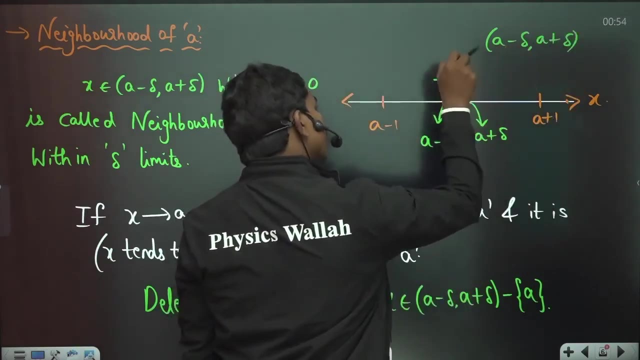 a minus delta comma, a plus delta minus a. so from this interval, when i write this interval, a minus delta to a plus delta, then definitely you know there are infinitely real number, infinitely many real numbers in between these two values. and also a is also coming in between this interval. 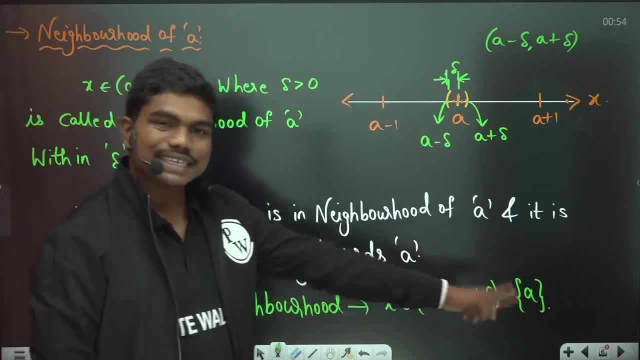 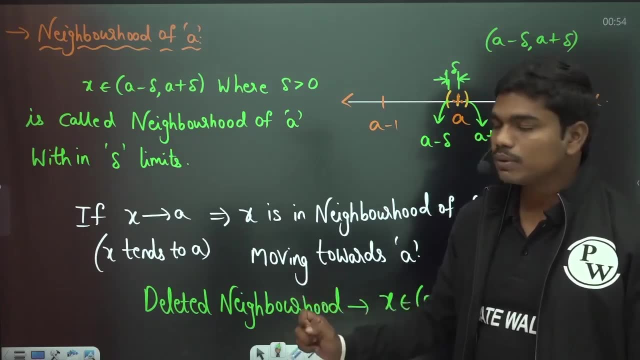 but when i say deleted, a is actually skipped out of the interval. okay, so a is not there in the interval and limits are defined on deleted neighborhood. actually, okay. that's why you'll never substitute means basically you never mean that x is actually equal to a, but x 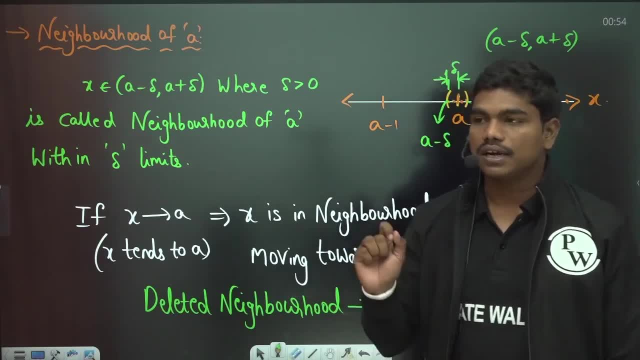 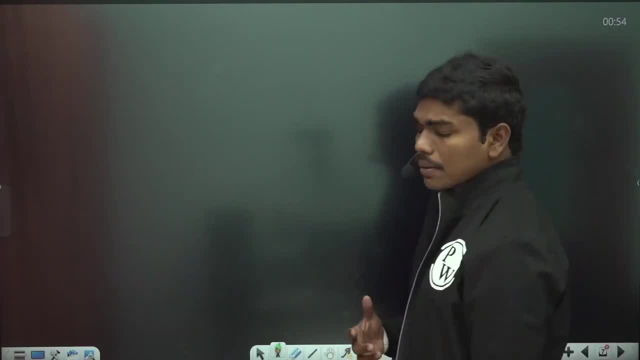 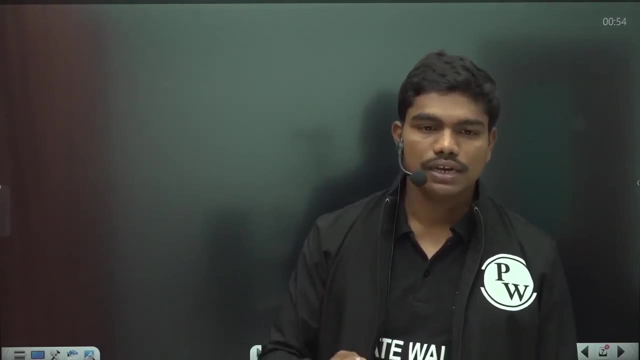 is lying somewhere in between a minus delta to a plus delta. okay, now let us see the definition of limit. what is a limit actually? okay, look, for example. many of you might be doing this. uh, you know simple things like sfds, bmds, for example. you take strength of materials, for example. okay, 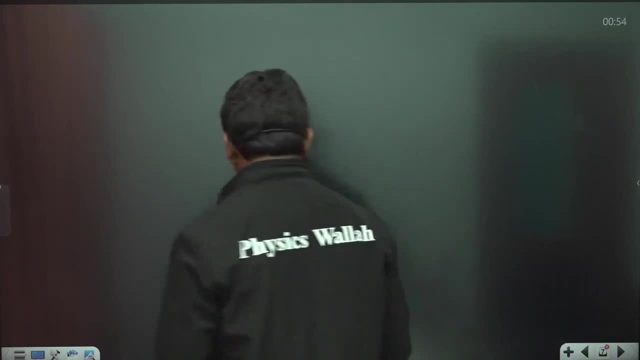 uh, some of you know could understand this. look, i'll tell you. let us suppose i have a beam, for example. i have a beam. i have a beam like this, for example. okay, i have a beam like this, it is fixed. let us suppose it is fixed now. let us suppose i'm putting some loads on this, for example, for fun. 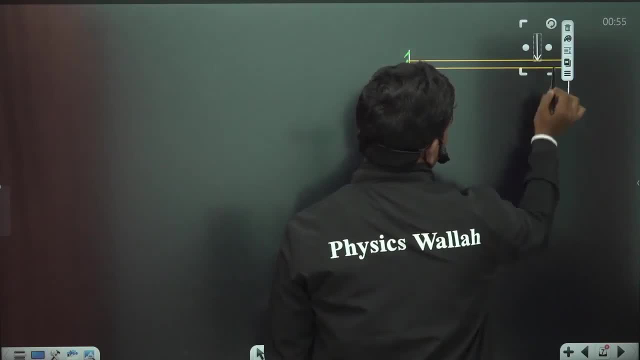 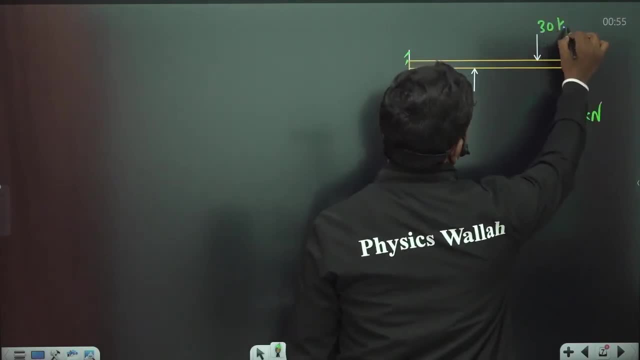 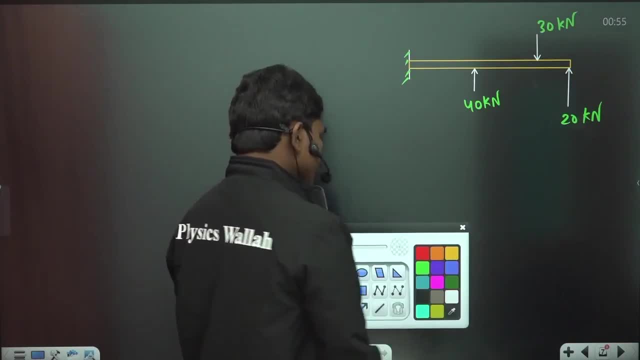 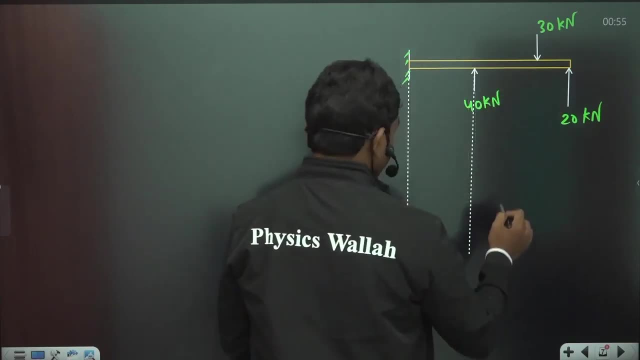 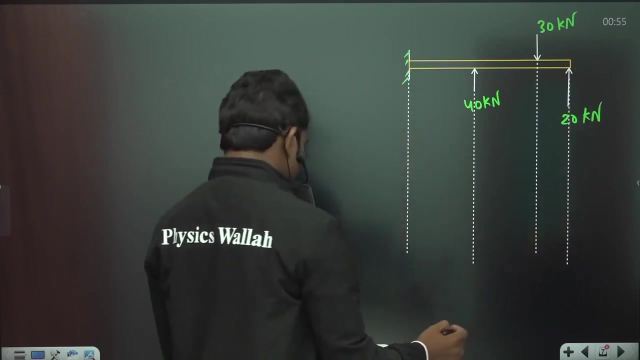 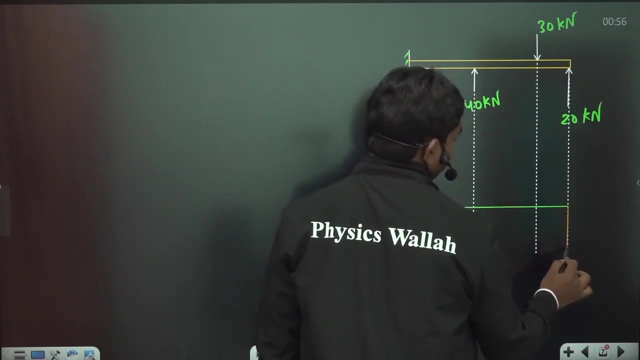 the sfd of this beam: shear force diagram. basically. okay, so if i draw the sfd of this beam, how does it look like? it looks fit like this. okay, now let us suppose if this is your zero shear axis, so this is a zero shear axis, for example. now, if i draw the sfd, it looks something like this: 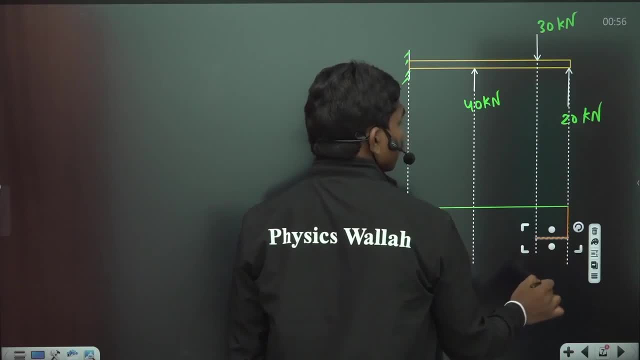 so basically you have 20, so 20. let us say this is 20. now here to here, no load, so no load. so now you have 30, so this goes to plus 10, so then it has plus 10 and then it came to 40. actually, 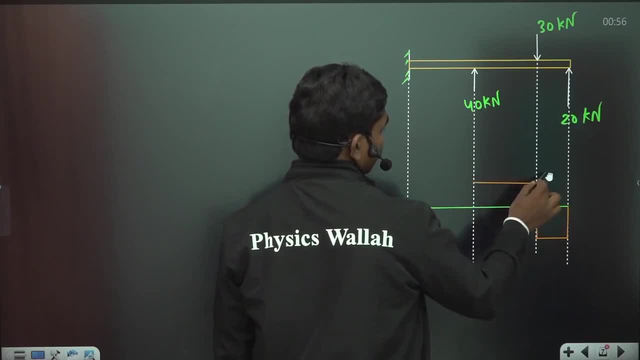 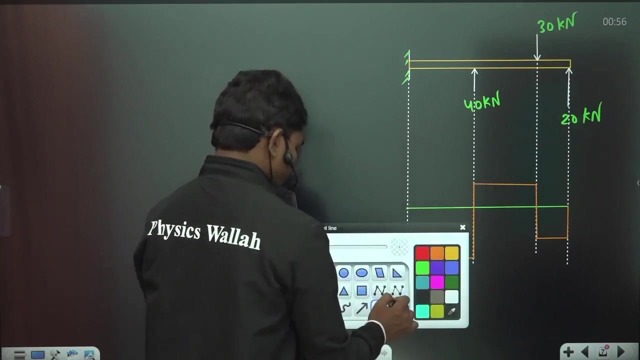 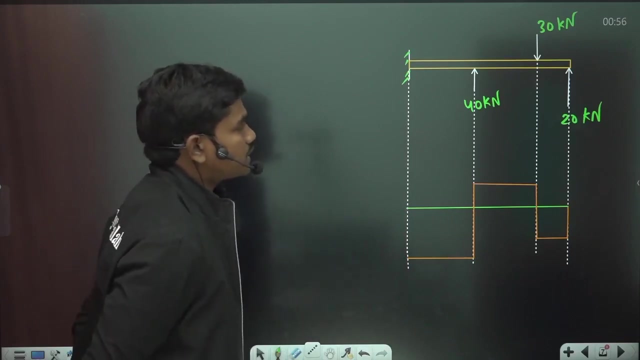 means here you have some minus 30. okay, so some minus 30 it came out and finally no load. so if you see, this continues like this, okay, so this continues. this continues like this, right? so if you see, this is the shear force diagram basically here. so 40 increase again 30 degrees, again 20. 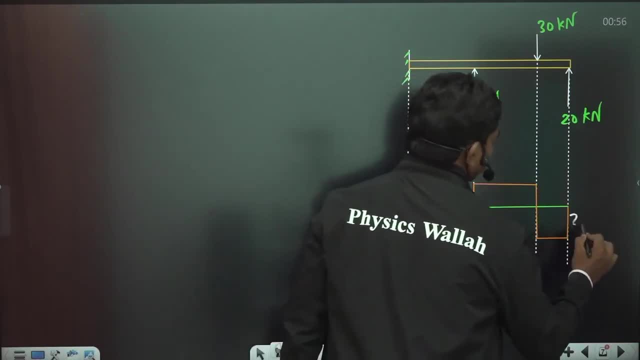 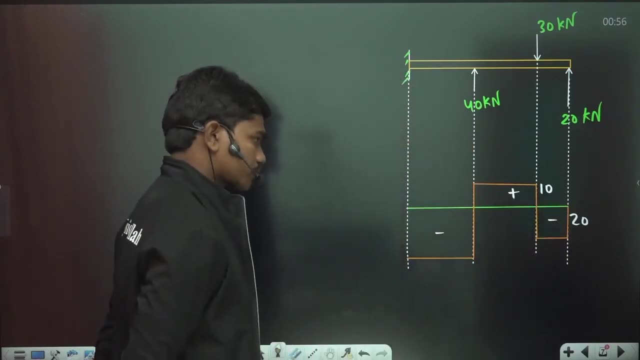 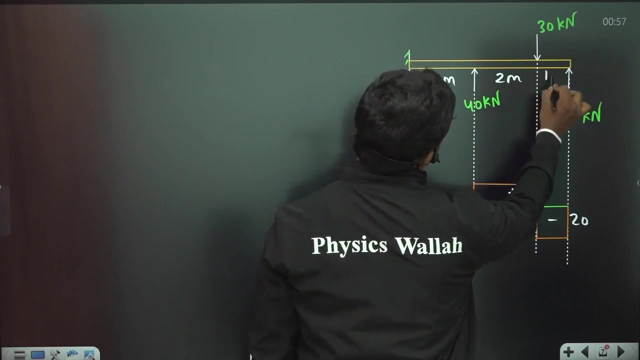 increase. okay, so if you see these values, for example, this is 20, this is plus 10, actually plus 10, of course minus and negative. so now if i ask you, for example, if i ask you, let us suppose, if this length is 2 meters, this is also 2 meters, this is 1 meter, for example. now, if i ask you, 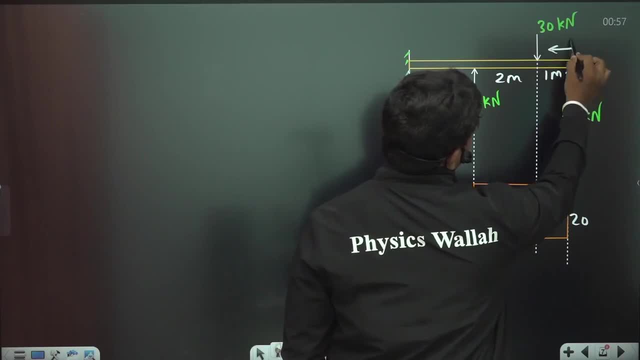 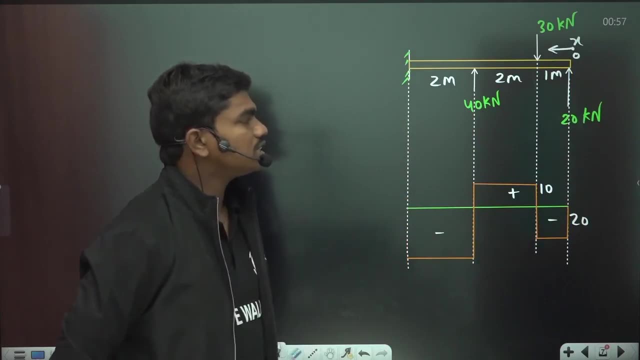 let us suppose i am starting my x here and my x is going like this: this is origin. okay, this is origin. let us suppose i have started here and my x is going like this: now, let us suppose, if i ask you, what is the shear force diagram here? and what is the shear force diagram here and what is the? 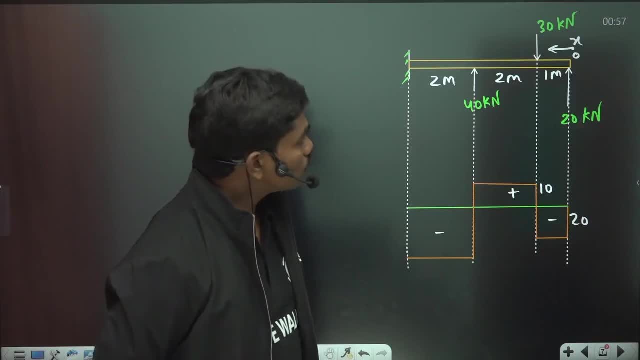 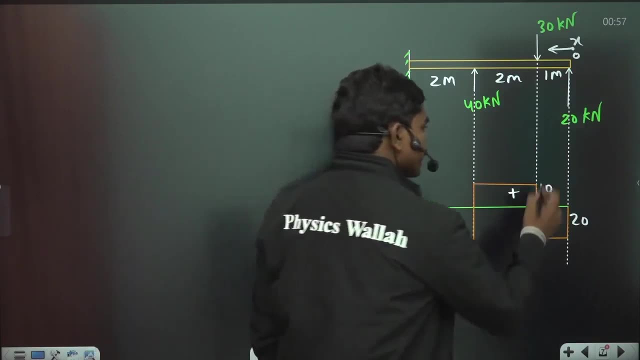 force value at x equal to 1 meter, for example. okay, so at x is equal to 1 meter, what is the shear force value? if i ask you this question, actually speaking, if you see, at exactly x equal to 1, at this point it is 10. at this point it is minus 20. so you have two values to tell me. so 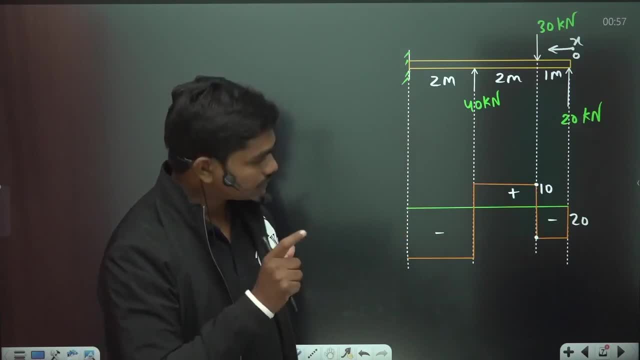 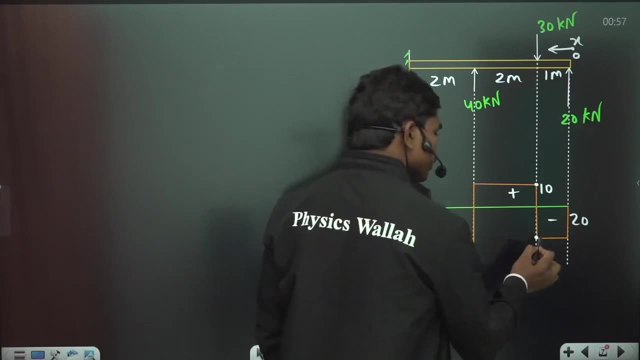 which value you will tell me actually. so that's why, if you see there is some ambiguity here, for example, if i ask you what is the value of shear force at x equal to 0.99 meters, you will definitely say minus 20, because you know. here comes the point. and similarly, if i ask you what is the 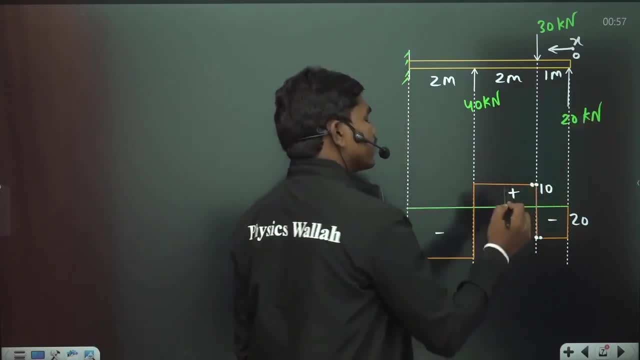 shear force. at x equal to 1.01, something like that, you will say definitely 10. but if i ask you exactly: at x equal to 1, what is the shear force? then definitely there is some dilemma for you, because here it is plus 10 and here it is minus 20. so that's why, if you see in some standard books and 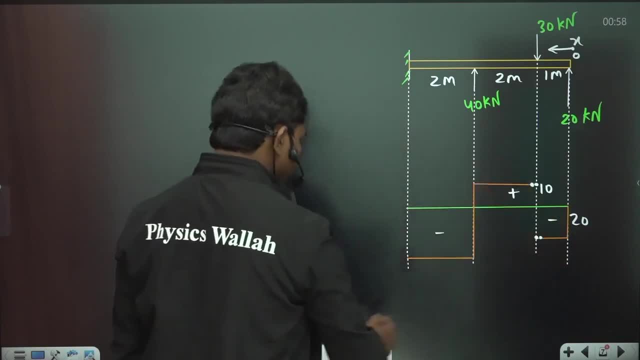 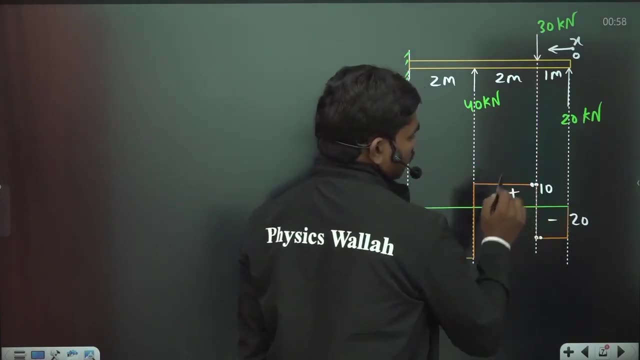 all this line is not represented by solid line. it is represented actually by some dotted line, actually like this. okay, because there is some discontinuity at the points of application. okay now, anyhow, this is just a one example which i'm quoting so that few people can relate, because i'm also from mechanical you. 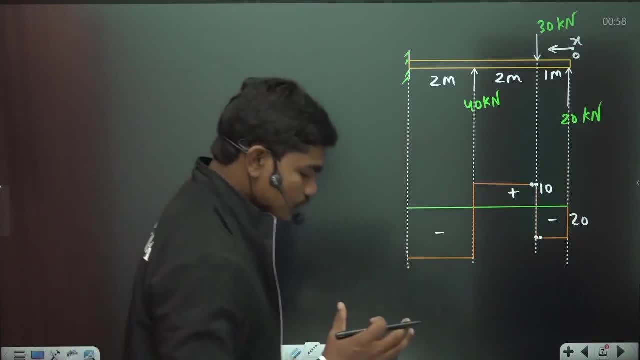 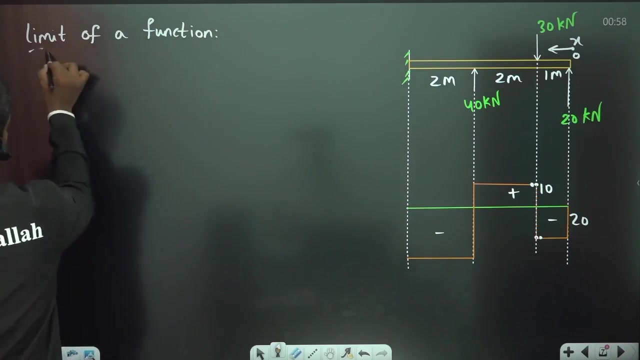 know i have some idea on that, but anyhow, let us try to understand. what is a limit actually? okay, so limit of a function, limit of a function, limit of a function. i'll define in the simple terms, let me not make the things complicated: a value. or you can say: 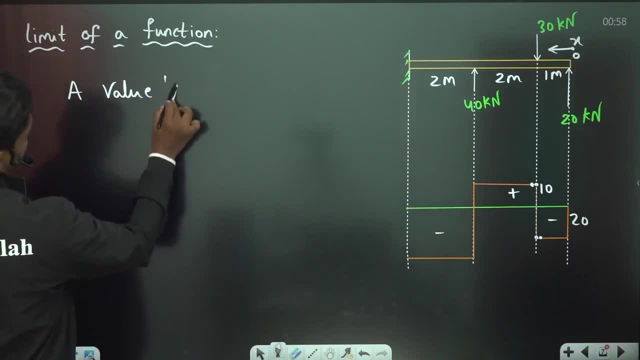 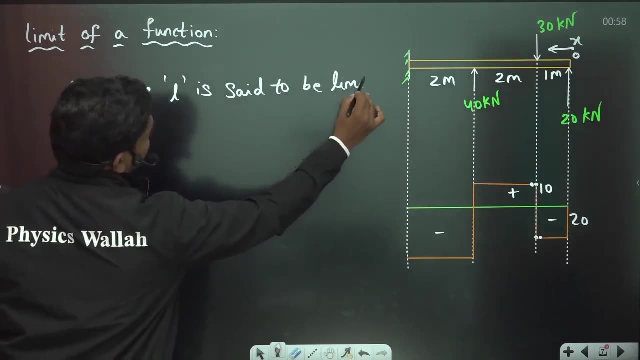 okay, it can be complex. also. sometimes a value l is said to be, is said to be, limit of a function, limit of a function. f of x at x is equal to a if f of x tends to l as X tends to a, if f of x tends to x, ya means that if it depends on the value client is constant in the trial. the section just salient value of f guidelines is not satisfied. thats one of missing tremor of a function limit. the property of other function at x is equal to a. lets say let's write a function as x. their function is equal to a and one next to that. let us try to knocks on table a value's. 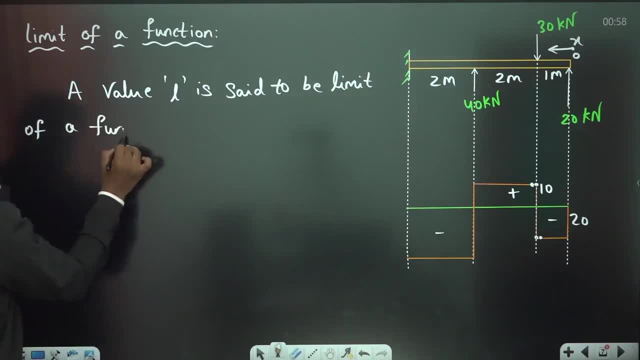 well, let's write the term limit of function. it would be aört. and then part 1, limit limit of that line is equal to lambda. l comes in curve to l and k, kx is equal to l. the a x left x is equal to a, just simply comes together the formula here: 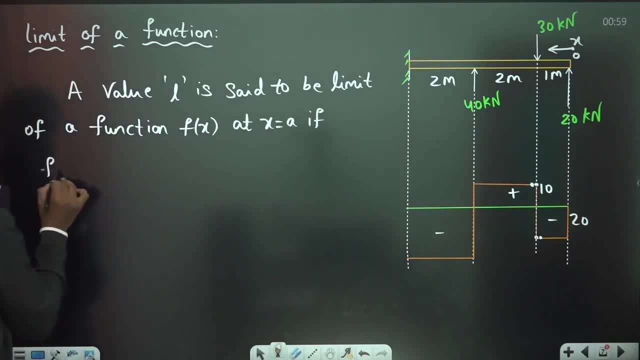 you to love it. you so what it is: X tends to L as X tends to A. What is the meaning of this? Look, I'll tell you. For example, let us suppose you have some graph: This is y-axis and this is your x-axis, x, y horizon. Now let us 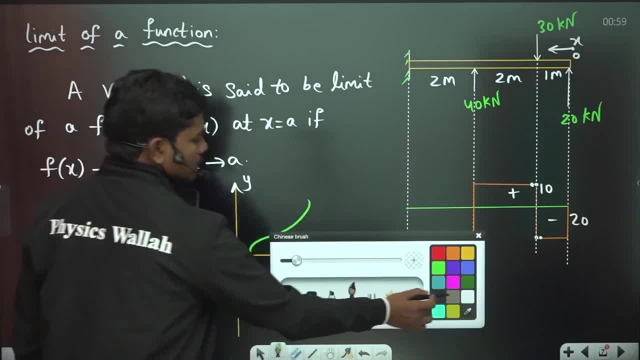 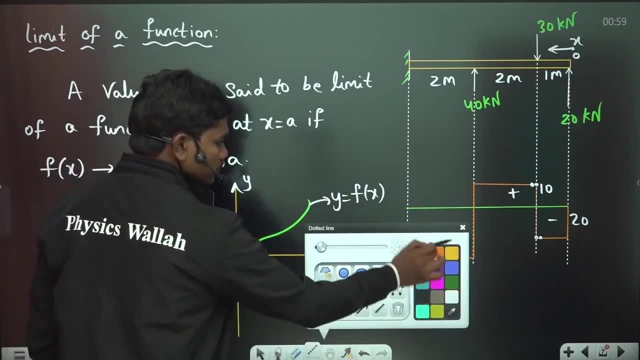 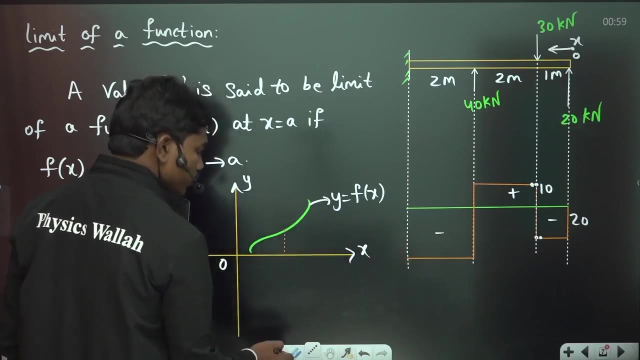 suppose there is some function like this, For example, this is some function: y is equal to f of x. Now let us assume this point is x is equal to A, for example. So let us suppose this is the point: x is equal to A. Now try to understand one thing. Let us suppose this: 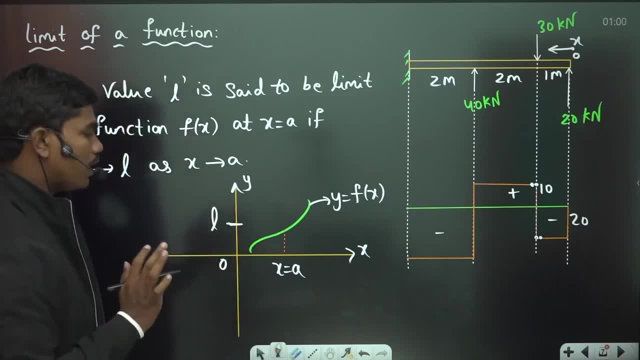 value is L. This value is L and I'm telling you this L doesn't have any connection with this function. This L is just a number On y-axis. that's it Basically. I'm telling you this L doesn't have any connection with. 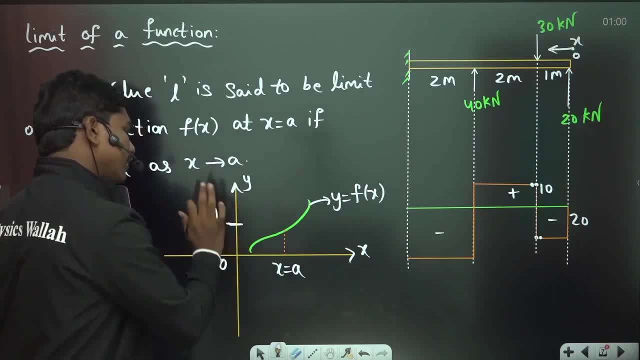 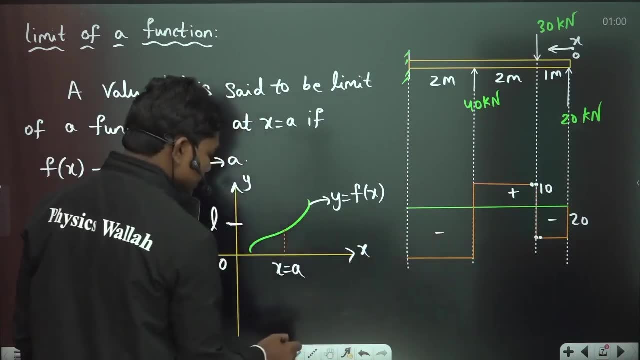 this f of x or A, This L is just a value on y-axis, Now, initially, as I told you, as x is tending to A, So let us suppose x is initially in this neighborhood. So let us suppose x is initially in this neighborhood. When x is in this neighborhood, you can understand. 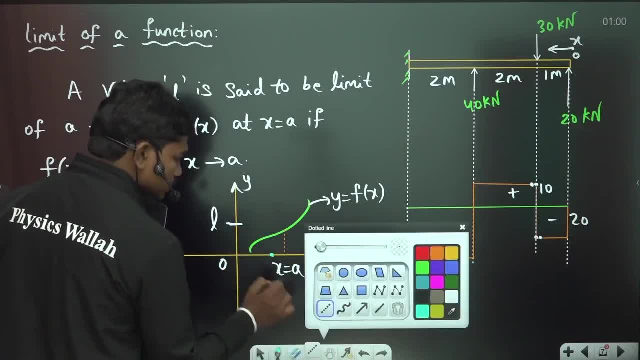 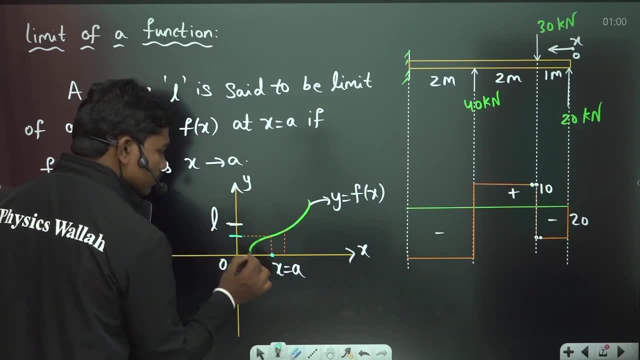 one thing: When x is in this neighborhood, you can get this. This is your x, This is your f of x value, correct? This is your f of x value. Now, let us suppose, as x is moving towards A, So from this point it came here, for example, because I'm telling you x is. 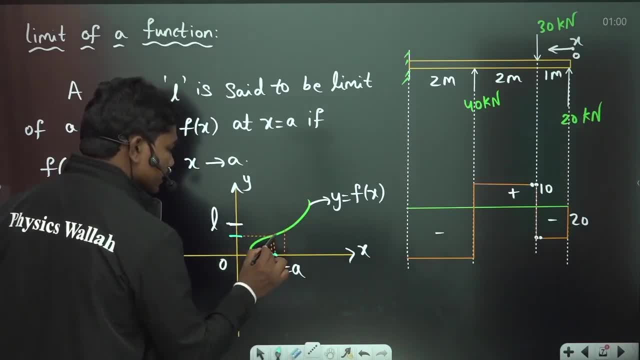 moving towards A. So this point gives you something like this: that this is your f of x value correct. Now let us suppose x still moved towards A. Then definitely you can understand: this is your f of x value correct. So here you can understand one thing: When 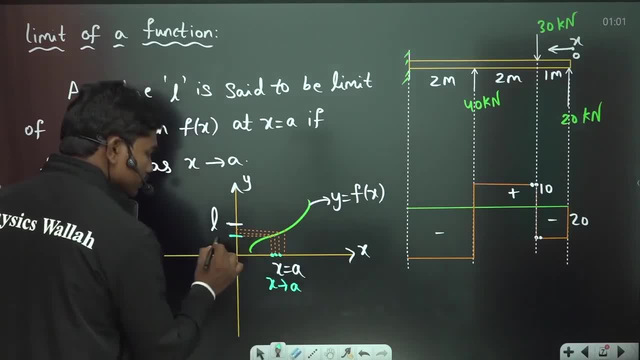 x is moving towards this A. if this value is your f of x, you can understand. this f of x value is moving towards your L, correct? Now x tends to A. This means, I told you, x is in the neighborhood of A and x is moving towards A Now, whenever x is in the neighborhood. 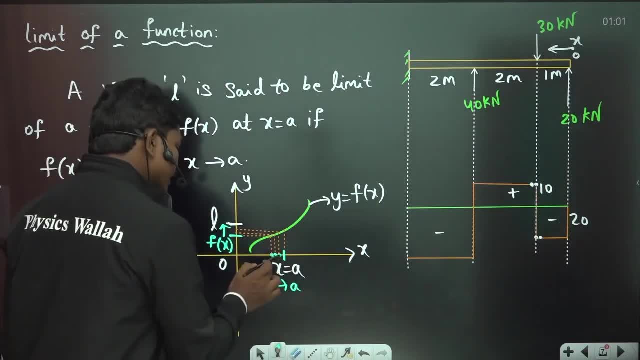 of A. whenever this point is, x is equal to A. x can be on the left side means in the left neighborhood, or it can also be on the right side, So it can be on the right neighborhood also. So let us suppose if I take the right neighborhood, let us see what's happening. 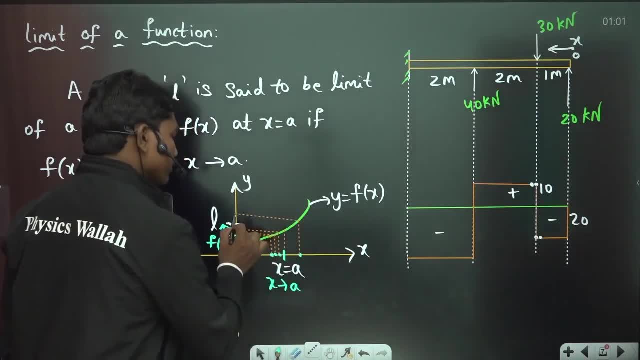 So let us suppose at this location, if this is the f of x value, then let us suppose, if x is moving towards A, then what happens? This function will come something like this: S on, So in this case also, you can observe, as x is moving towards A, this f of x value. 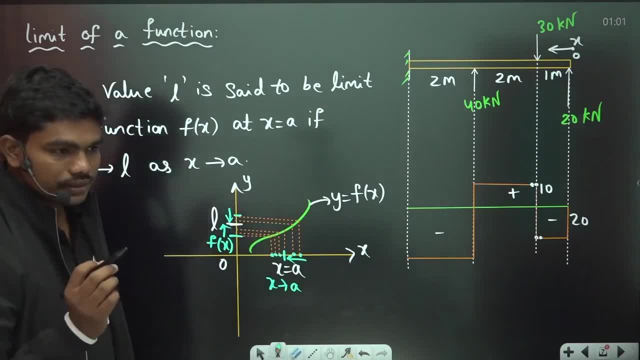 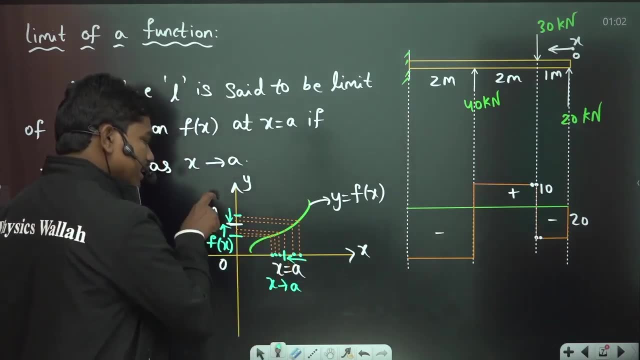 is moving towards L. So this means basically there exists some value L such that whenever we are moving your x close to a particular real number, immediately f of x gets adjusted to move to some number. So this is the f of x value. So this is the f of x value. So 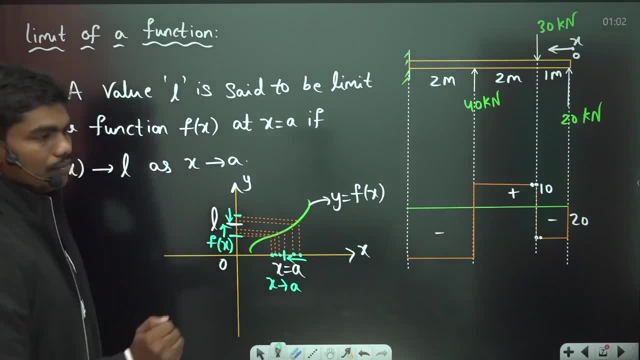 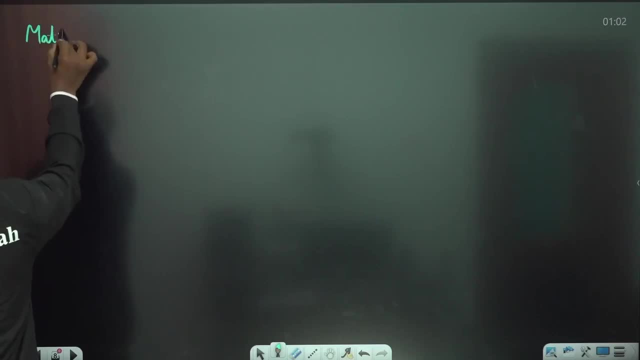 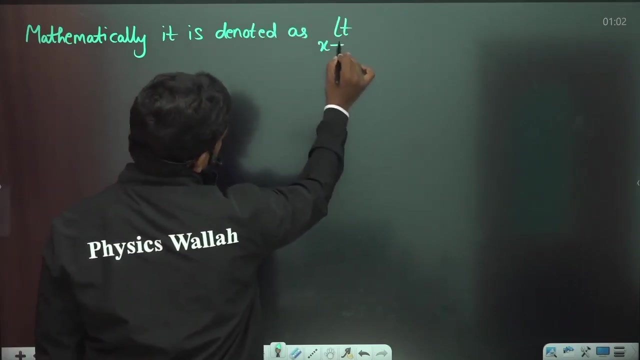 that's why we call this L as the limit. Now, fantastically, I will tell you one thing: Normally, mathematically, it is denoted as: mathematically, mathematically, it is denoted as: mathematically, it is denoted as limit. x tends to A, f of x is equal to L. Look I. 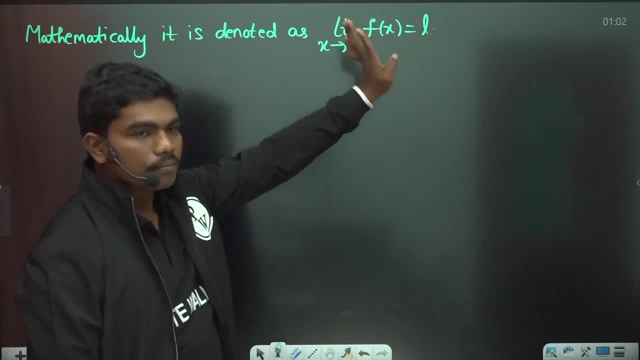 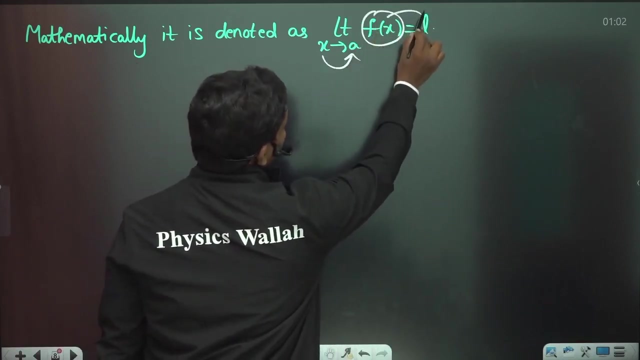 am telling you again: f of x is never equal to l. okay, but because of this symbol limit, we write this in this notation, that limit x tends to, f of x is equal to l. the meaning of this equation is: as x is moving towards a, this f of x is moving towards l. this is the meaning of that. okay, now there is concept of. 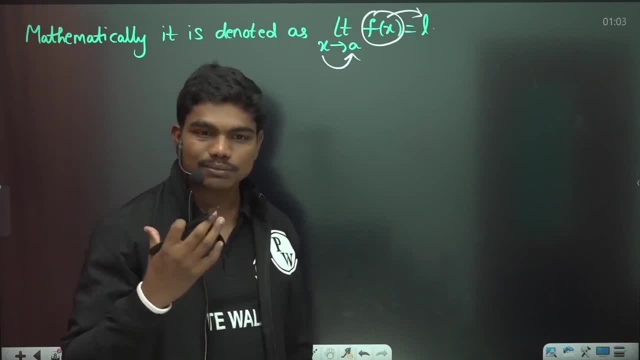 left hand limit and right hand limit, because whenever i'm telling x is moving towards a, i'm not mentioning the direction. so whatever direction you take, definitely f of x should move towards. l understood, even if i take that x is in the left side of a and moving towards right, or if i take 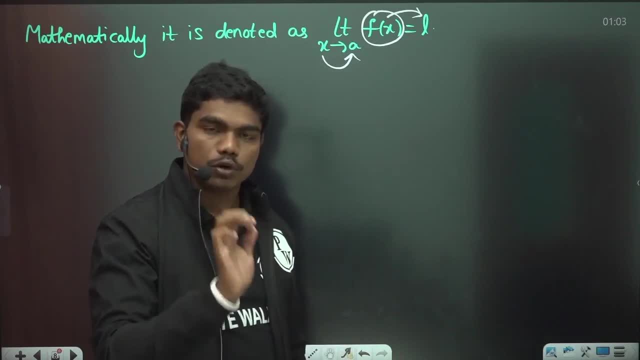 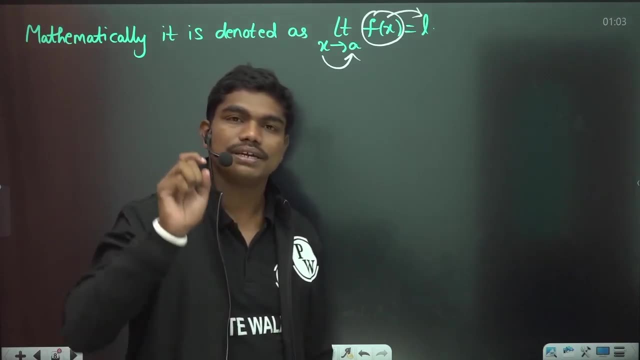 x is in the right side of a and moving towards left, then in both the cases my f of x should move to l. that's the reason why if our limit to exist- left hand limit and right hand limit- both should be same, because in the definition of limit they didn't specify the direction. 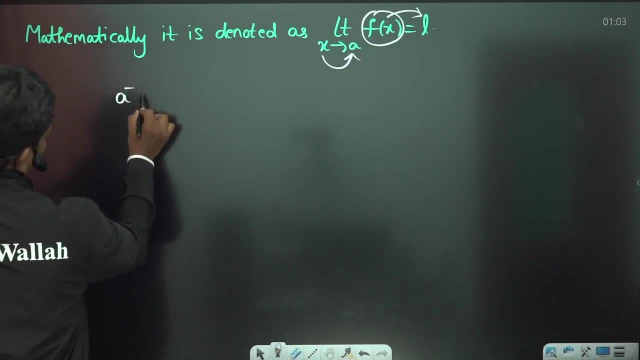 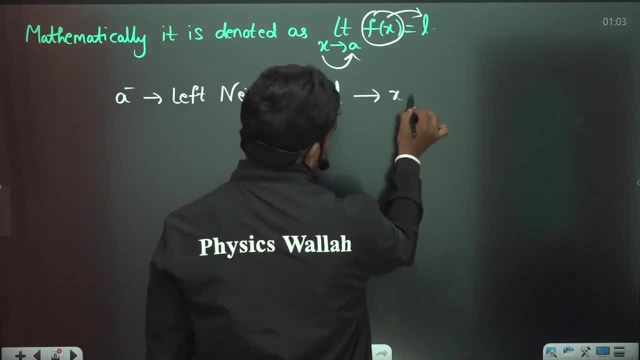 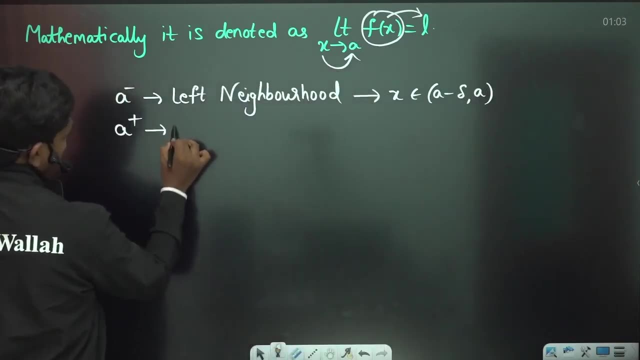 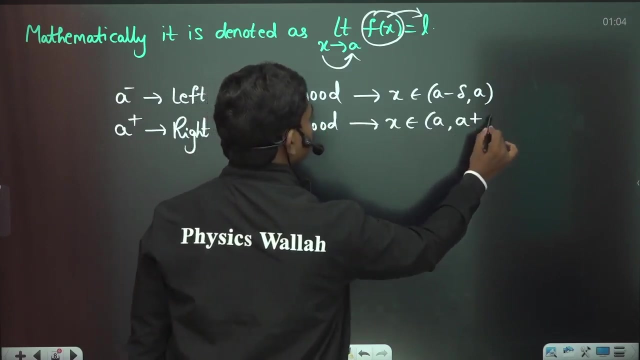 left neighborhood, basically, and this implies x belongs to a minus delta comma, a. similarly, a plus denotes right neighborhood, right neighborhood, right neighborhood, and this tells you that x belongs to a comma a plus delta. because, if you see, if you take the total neighborhood, a minus delta to a plus delta, a minus delta to a is the values of a are. 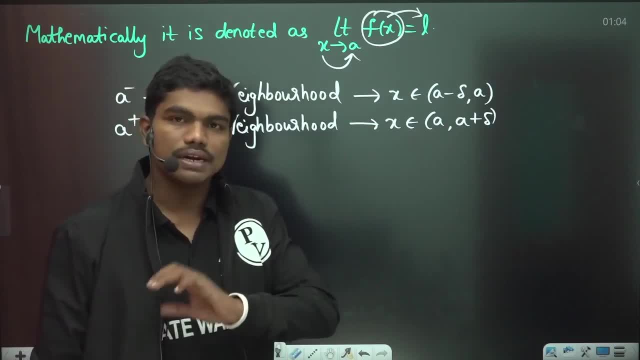 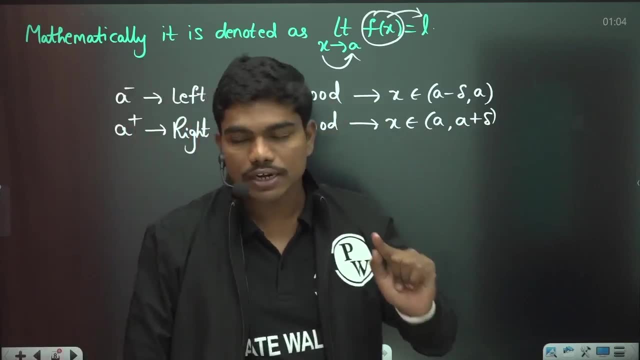 the values of x, which lies to the left side of a, on a number line. similarly, this belongs to the right side of the a, so that's why they're called left neighborhood and right neighborhood. one point i'd like to tell here. many students, even in previously, in my offline classes and all they 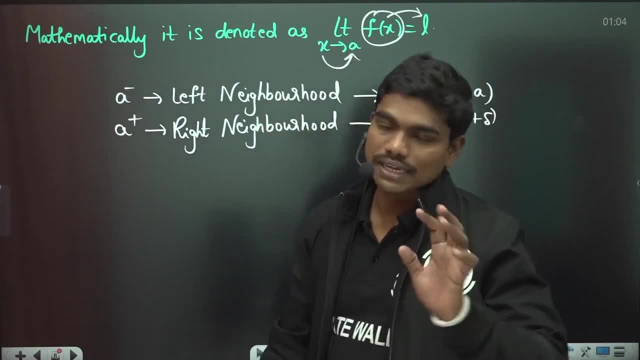 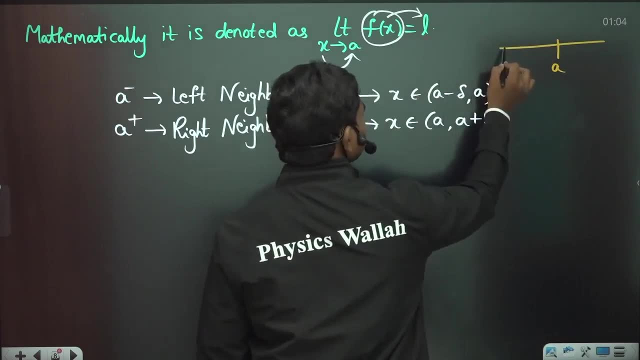 used to commit this mistake. a minus is different from minus a. okay, so look, whenever this is a number line, if this value is a, then minus a will be somewhere. you know five. actually minus a will be somewhere here because zero is in between. there are many real numbers, but a minus are the values. 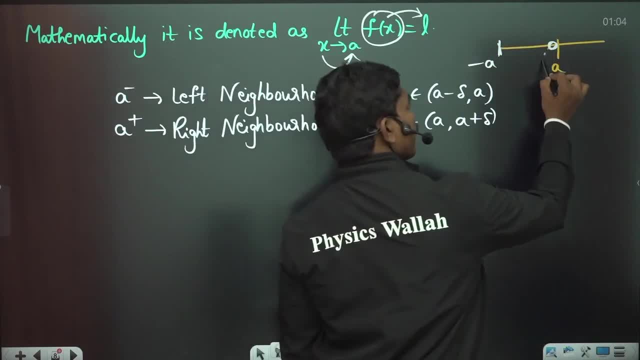 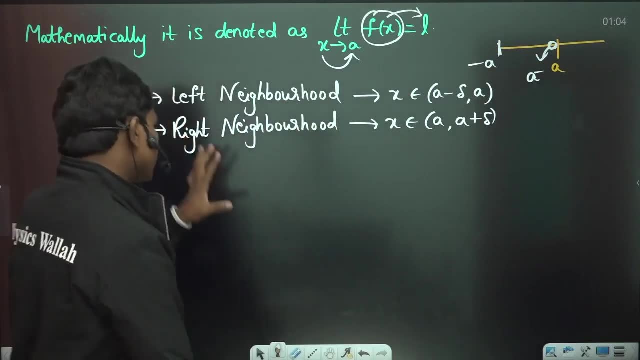 which are here. okay, so a, this is a minus and this is minus a somewhere five. okay, so that's called left neighborhood, actually clear, so that's why you generally write this. as for limit to exist for limit of a function: f of x, for limit of a function f of x to exist to exist limit extends to a minus f of x. this should be. 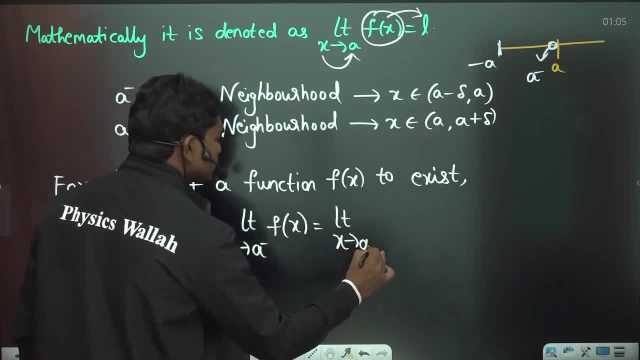 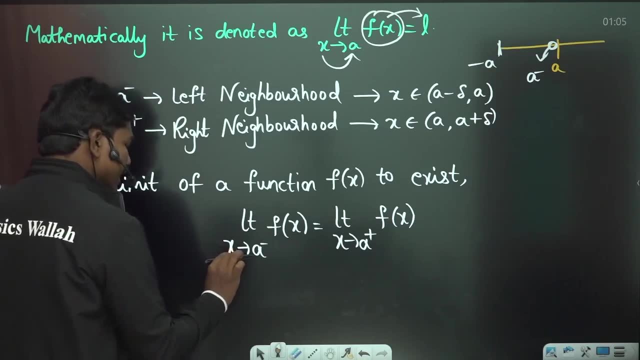 same as limit extends to a plus f of x. okay, the meaning of this equation is if your x is on the left side of a and moving towards a, then this limit value should be same as if x is in the right side and moving towards. x is equal to a. okay, so that's the 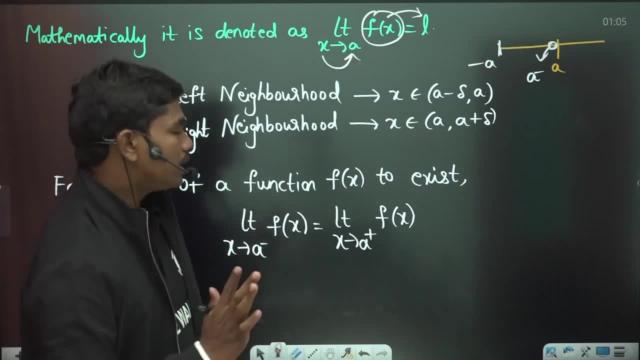 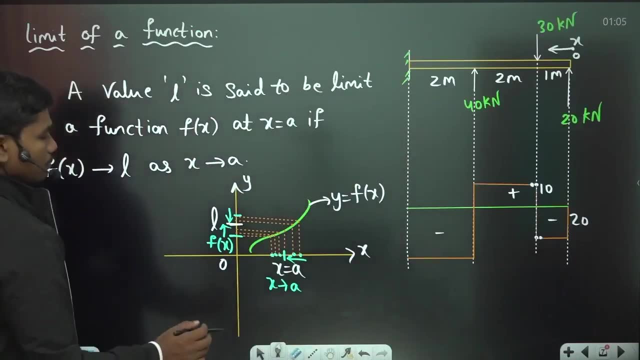 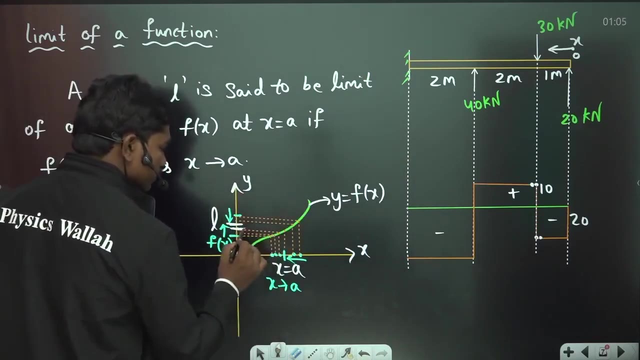 meaning of left hand limit and a right hand limit, for example. okay, now, why you are substituting x is equal to a is because you take this equation. you know, for example, at this location: at this location, you know that this value, if the function is continuous, of course you can understand this. 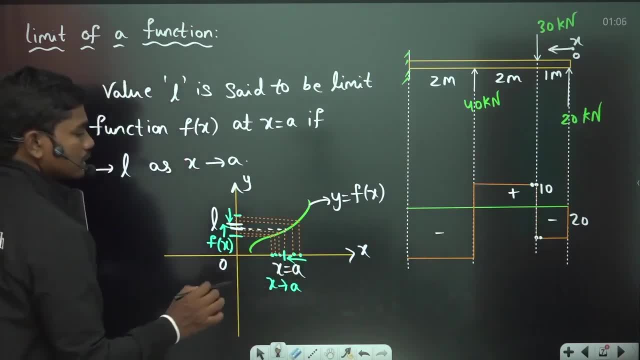 l value is nothing but almost equal to this f of a value, correct? so when a function is continuous, of course you can understand this. l value is nothing, but almost whenever x is almost zero, it's almost touching a. this f of x is almost touching l. so whenever 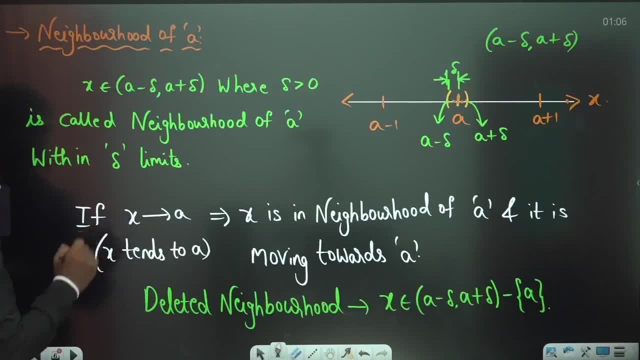 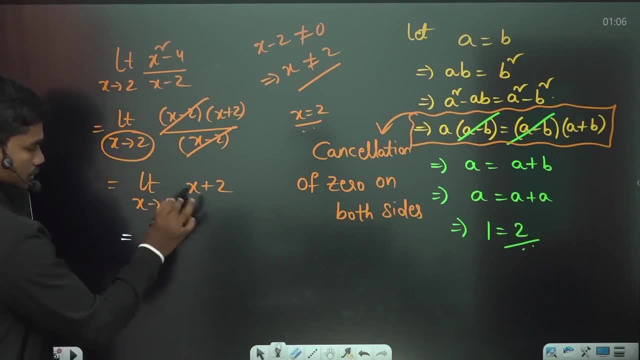 actually in that calculation, what i have shown you in this calculation. in this calculation, what you should actually do is look. what you're actually doing is you are not actually substituting two when x is tending to two, you are substituting 1.9999 plus two, so this is giving you 3.9999. 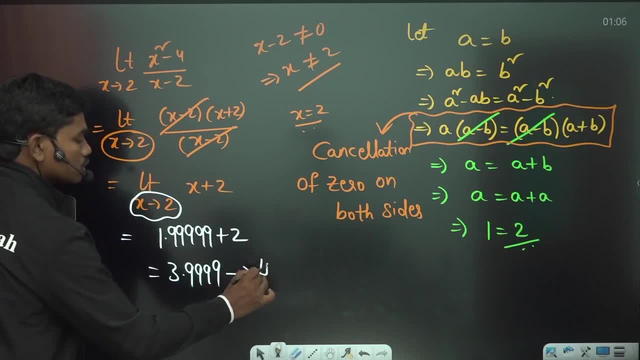 and all, but this value is nothing but very close to four. that's why you are actually substituting two and writing it as four because of this symbol here. okay, if this symbol, lt, is not here, you are not supposed to substitute. x is equal to two. okay, you actually need to substitute whenever x is tending to two. you. 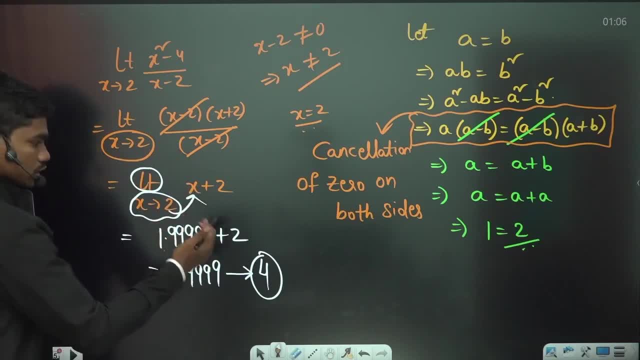 should write only 1.9999 or 2.00001 plus 2 and you should take four. but since this limit definition is there, this lt is there on the top. that's why you are actually substituting two. okay, so i hope you'll take 4.. 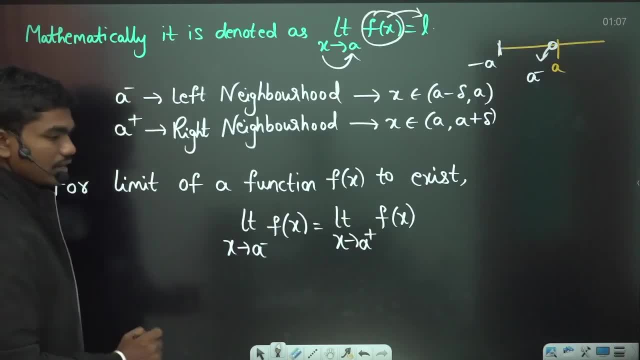 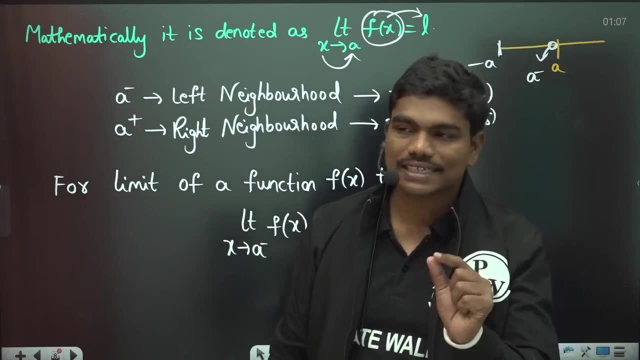 okay, so i hope you'll take 4.. understood this? so this is basically the meaning of limit whenever you're having any function. if yes, as x is tending to a particular number on x axis, if f of x is tending to one particular number. 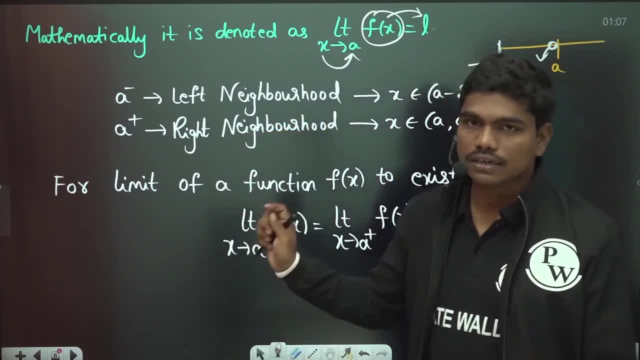 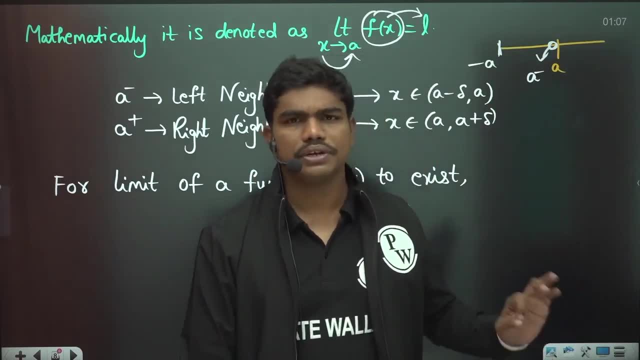 on y axis, then we say that limit exists for that. you know, function at that value of x, okay, so this is the basic definition of limit and before going further, for continuity, all these things, i would like to give you some, uh, you know, most popular or you say, most frequently used graphs. actually, okay, 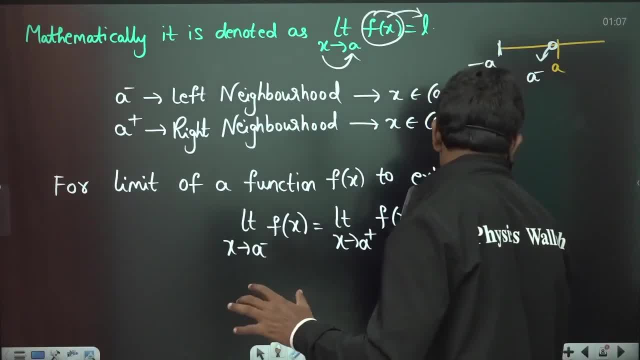 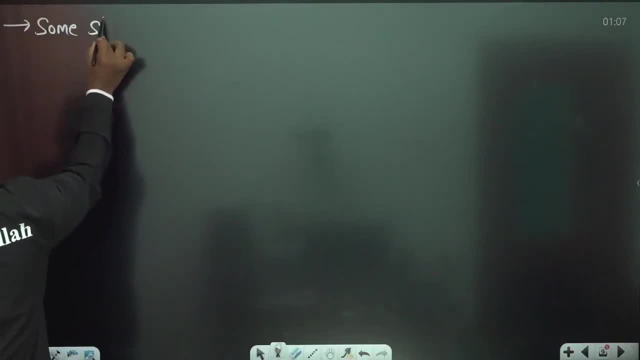 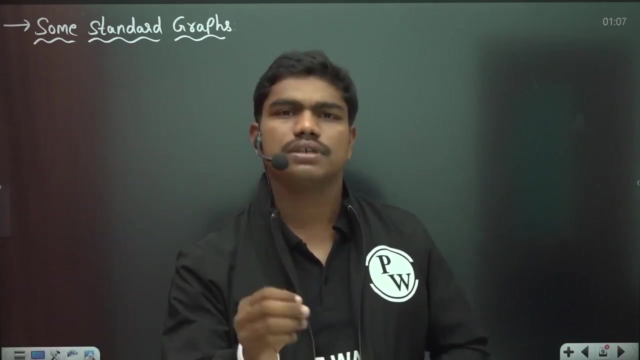 let us see some graphs which are very important for you in the applications of differentiation and all. so some standard graphs. let me give you some standard graphs, some standard graphs let me give you. so, first of all, to draw any function. let us suppose if i give you some random function, if i talk about sine x, cos x and all you know how to draw. but let us suppose, 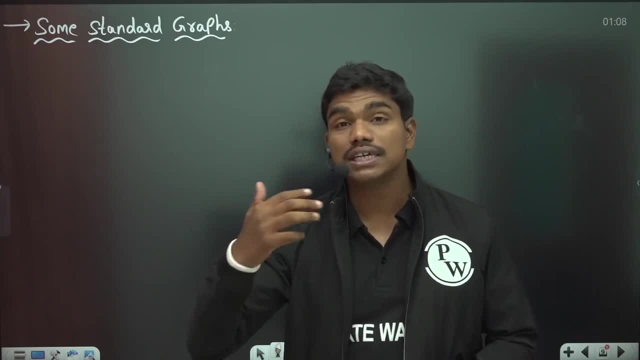 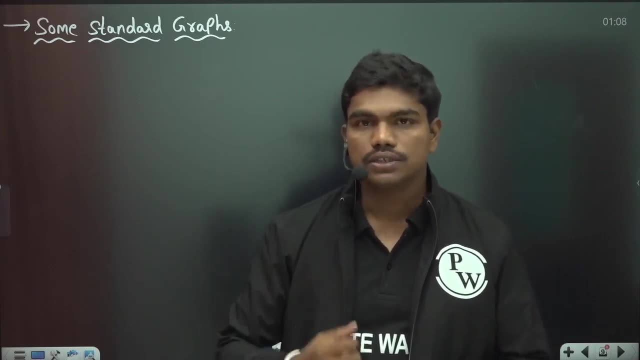 i give you some random function like x into sine x, sine x by x, such kind of graphs. if i give you, what is the how to basically proceed? okay, what is the common procedure to draw any graph? okay, so let us see here that i'll explain you with one example. first let us deal with 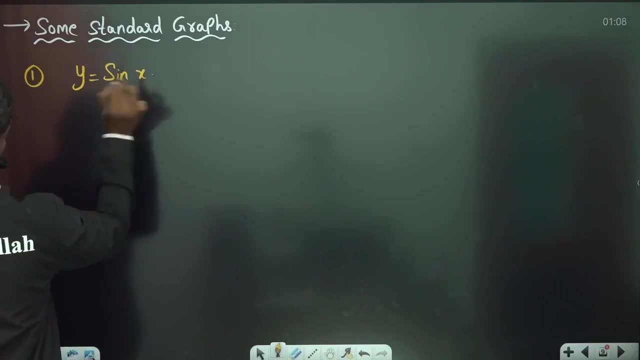 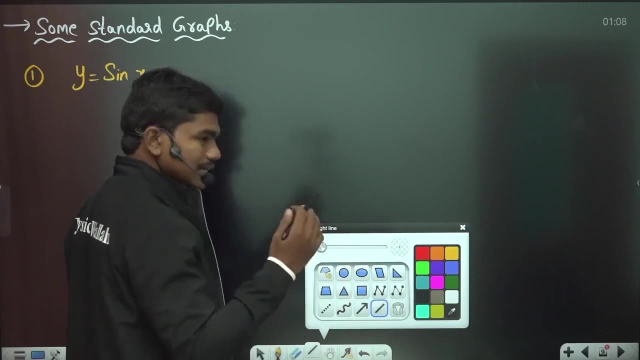 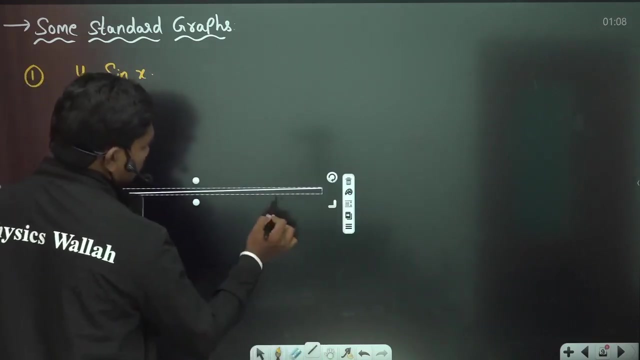 the sinusoidal function y is equal to sine x. okay, so when y is equal to sine x, so of course you know, you all know, that it's a wave shift. but let me tell you in a step by step manner how actually you can draw the graph. so see here. first of all, first step is establish the coordinate system. 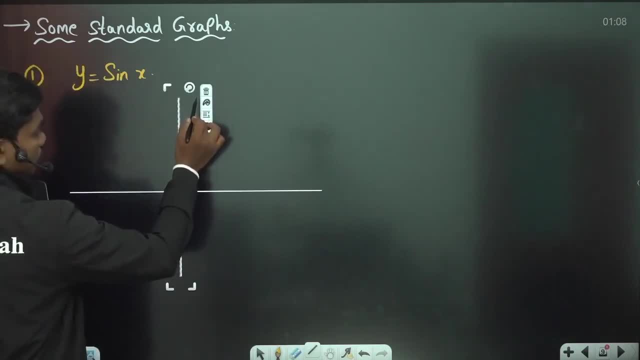 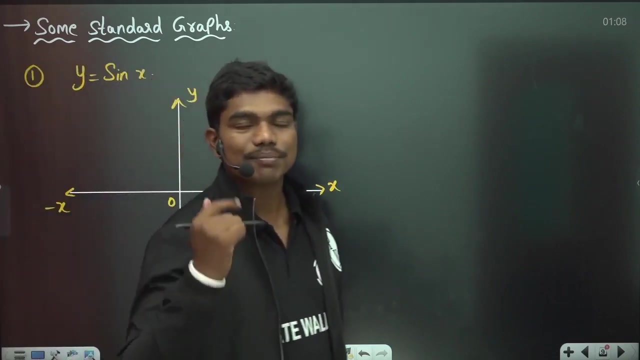 establish the coordinate system. establish the coordinate system, or isn't? you can say x axis minus x, axis y and minus y. now, after establishing coordinate system, you should check for the maximum and minimum values of the function. if it has some maximum, okay good. if you don't have, also, it's good. you can draw the graph till infinity. 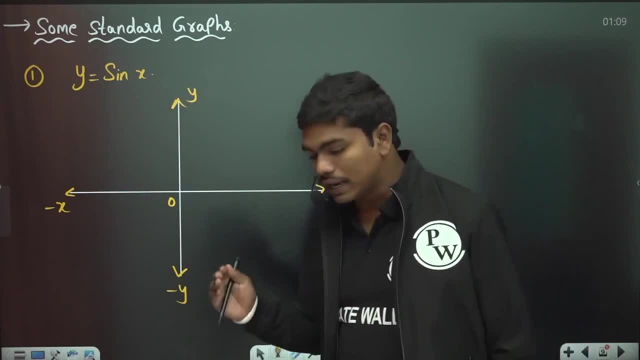 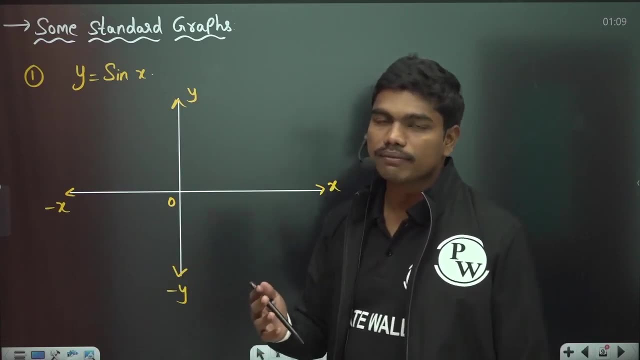 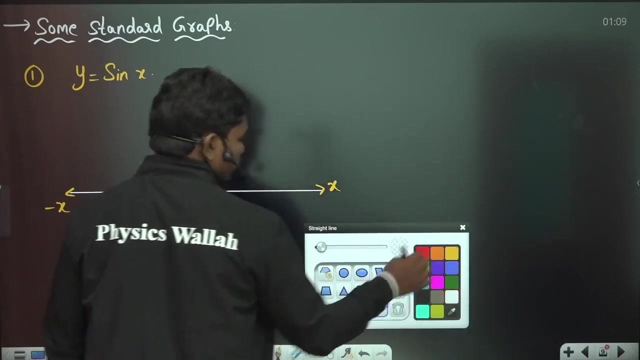 okay, so now, if you see, we try to identify what are the maximum and minimum values of this function, sine x. okay, so we all know generally that sine x has the maximum value of y equal to 1 and minimum y is equal to minus 1. correct, so now let us see it. we know that it has maximum value that x is equal. 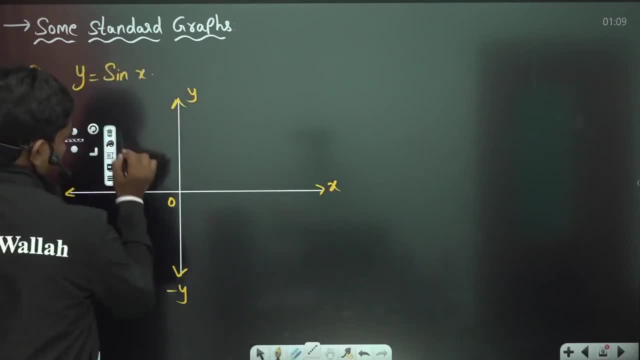 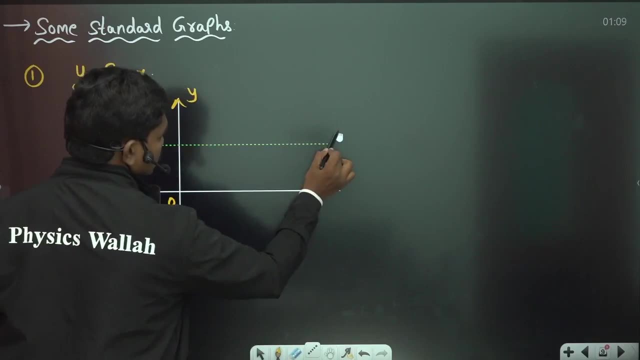 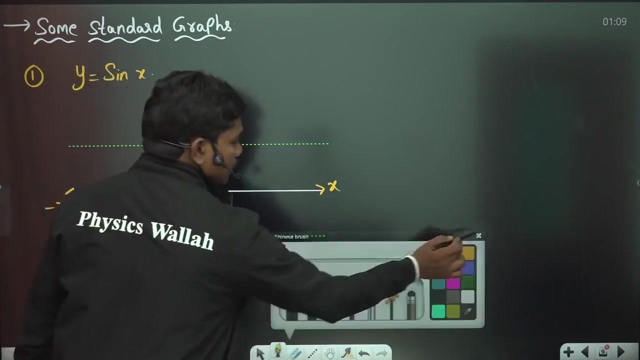 to 1. so let us draw the maximum value. we will draw the maximum value that y is equal to 1, so this is some maximum value, and we'll also draw y is equal to minus 1, like this. okay, so now, if you see, this is y is equal to 1. 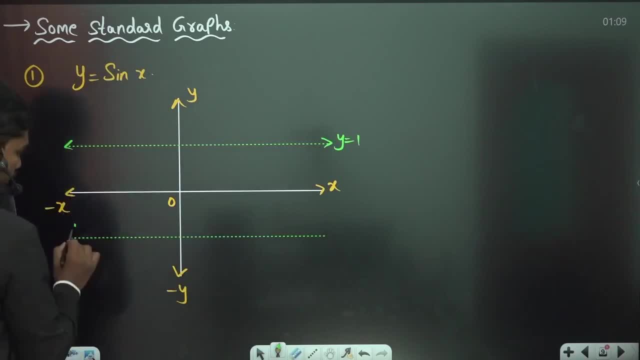 and this is y, is equal to minus 1. now you know one thing: whatever you draw, you should draw in between these two lines, correct? definitely, there is no nothing which is going to go above this line and also there is no graph which is going to come below this line, because these are the maximum and 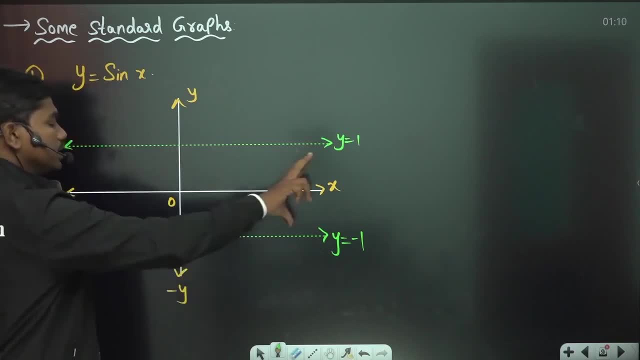 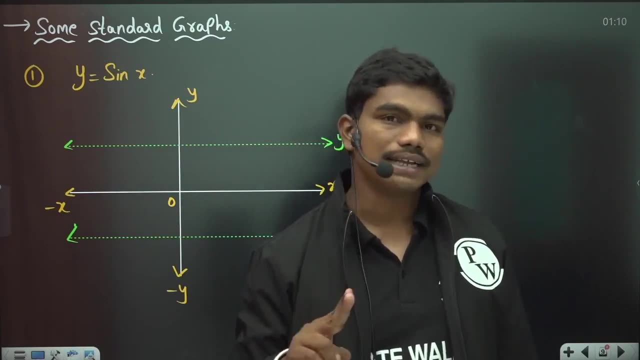 minimum values. so definitely the graph should lie in between these two lines. so that's what you know now. so first point: establish the coordinate system, draw the coordinate system. second point: identify the maxima and minimum values. now, third point: check if the function has any periodicity means. 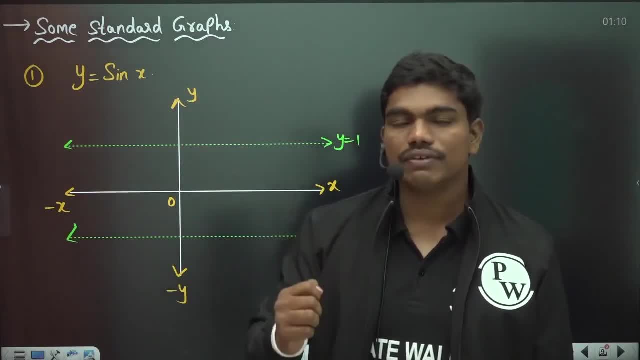 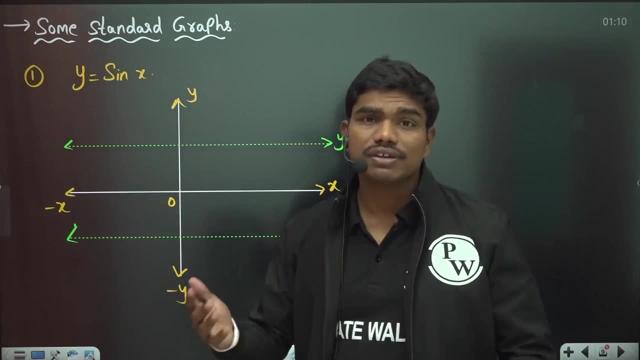 is. is it of any repeating in nature? okay, so you should check for that. for example, you know sin x is such function which is repeating after every two pi intervals. okay, now there could be some other function which is repeating after pi intervals only. okay, so we should check the. 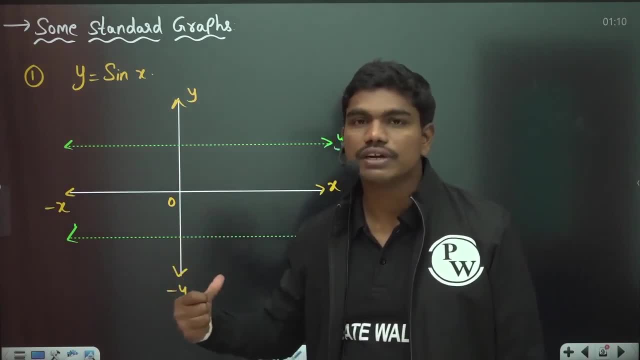 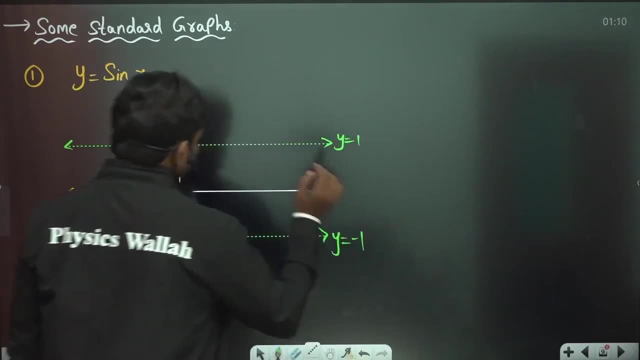 third point is to check for the, the repeating or periodicity of the function. okay, so for example, sin x, you know 2 pi is the interval. so let us split this into intervals of 2 pi. so let us suppose this is 2 pi interval, then this is one. 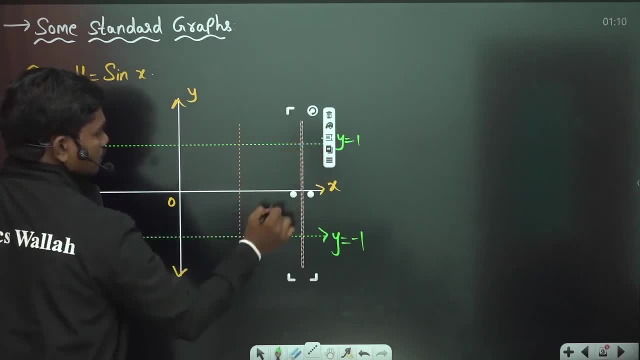 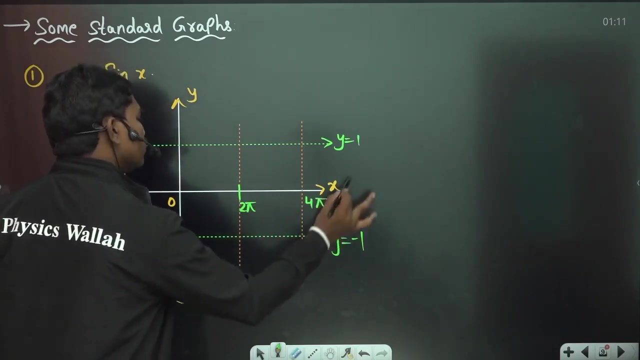 more 2 pi. interval like this: basically: similarly here, 2 pi, one more 2 pi. similarly here, you can say: lastly, one more 2 pi. like this: so you understood that there is some repeating in pattern. so in this part let us suppose: if this is, x is equal to 2 pi. for example, x is equal to 2 pi, 4 pi. similarly it goes: 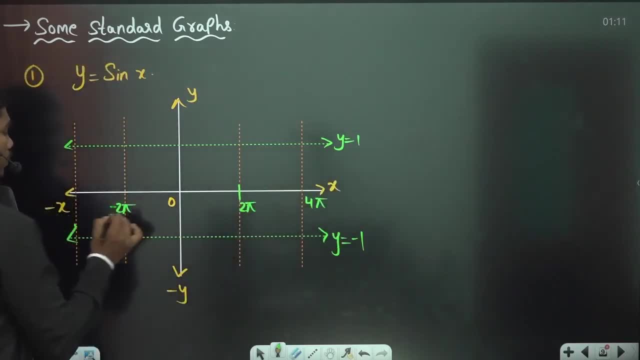 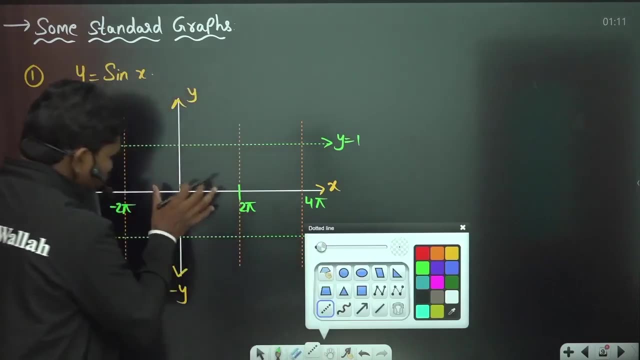 like that: okay, 0. so minus 2 pi, minus 4 pi. like this: okay. now what is the shape of the graph from 0 to 2 pi? you know, in 0 to 2 pi we focus because once you know what is the shape in 0 to 2 pi, same loop. 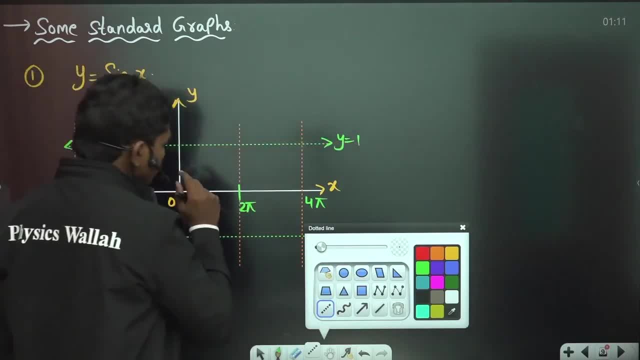 will continue. same loop will also reflect to the left hand side. now what is the shape of the graph from 0 to 2 pi? this is what you need to check. so now let us see what is the shape of the graph from 0 to 2 pi. this is what you need to check. 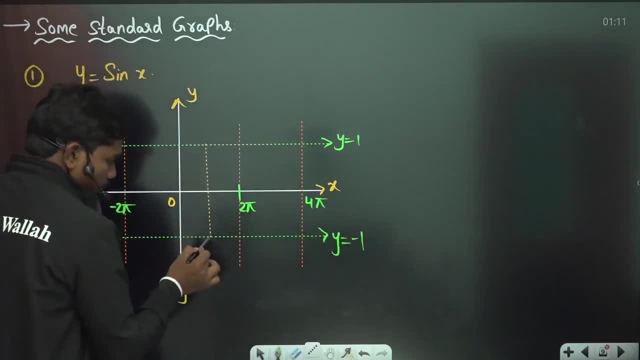 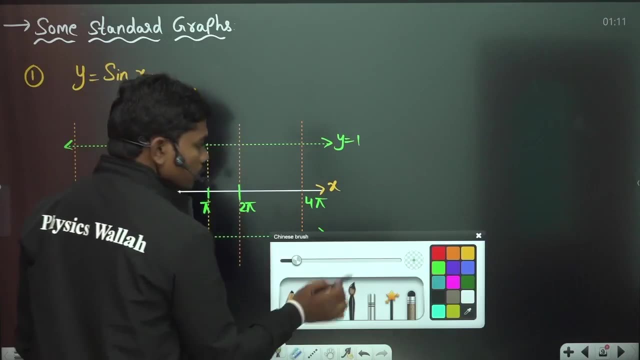 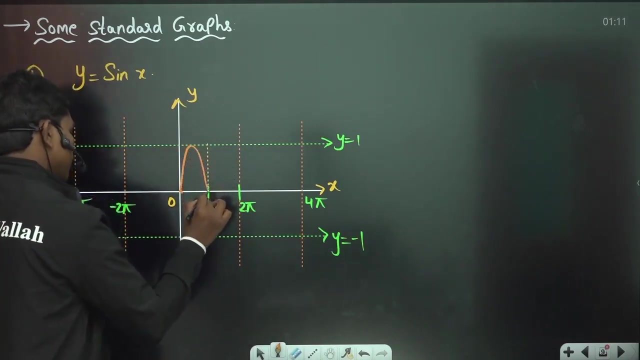 okay. so once you check this, you know at x is equal to pi, this value is 0, so let us suppose if this is, x is equal to pi, for example. okay, so you know in this, if you draw the graph, you will get your graph like this: you know it starts at 0, reaches maximum at pi by 2, then again comes to: 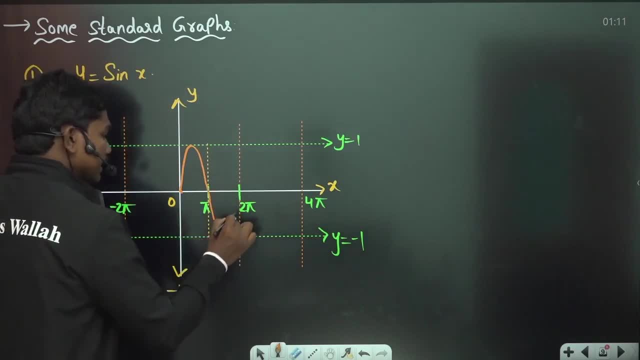 0 at pi, then it goes to minimum at 3 pi by 2 and again it touches 0. so you know that this is the graph from 0 to 2 pi. so once you know, then just copy this, that's it okay. so if you copy this, 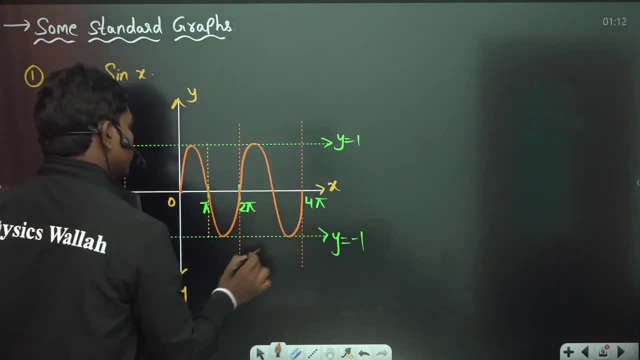 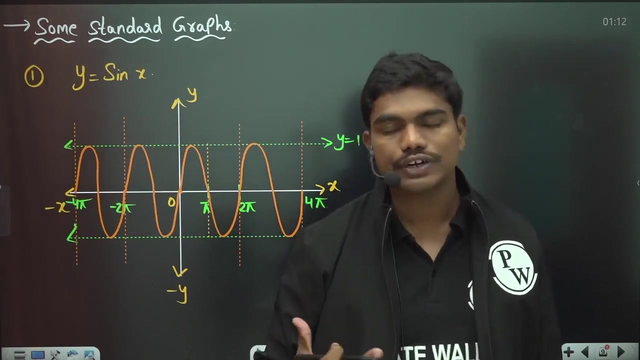 like this: similarly. if you copy this again, you will get something like this: like this similarly, and many things like this. okay, so this is how you generate the graph of sine x. okay, of course, i know that it's a very simple graph- you all can draw in a single go, but this is the general procedure for drawing any. 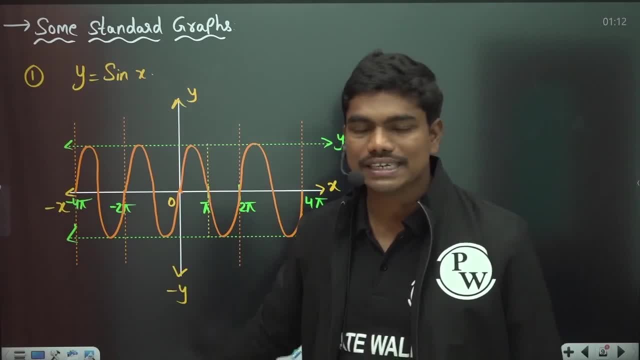 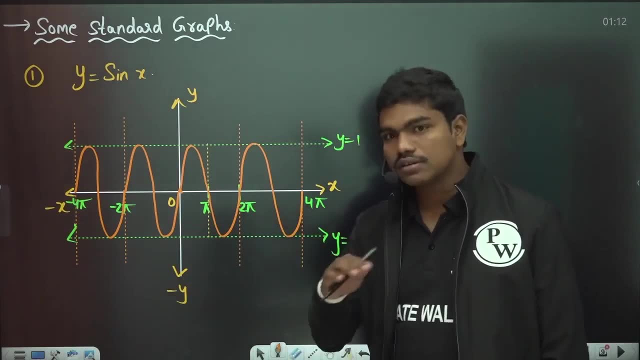 graph complex functions also. right now you know sine x, so that's why you'll draw very easily. but let us suppose if i ask you some complicated function then you will be in trouble. okay, so that's why these are the steps: first, identify first dollars coordinate system. second, identify the maximum minimum values. third, check. 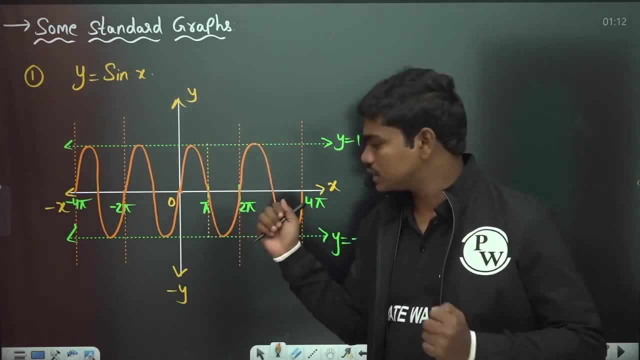 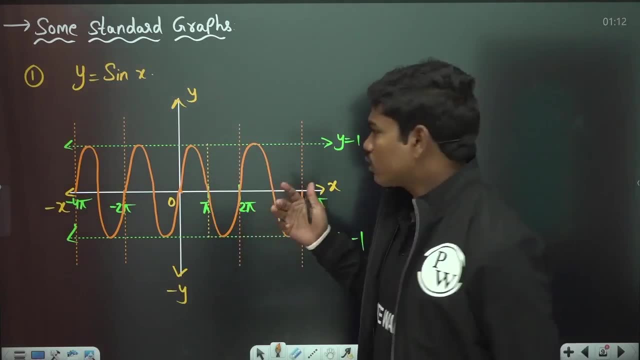 for any repetiveness of the function means. is there any periodicity of the function? check for that. and fourth point: try to plot the graph in that one particular box so that you can just replicate it. okay, now, cos x, so cos x. i'm not elaborating much since, uh, you know you might be. 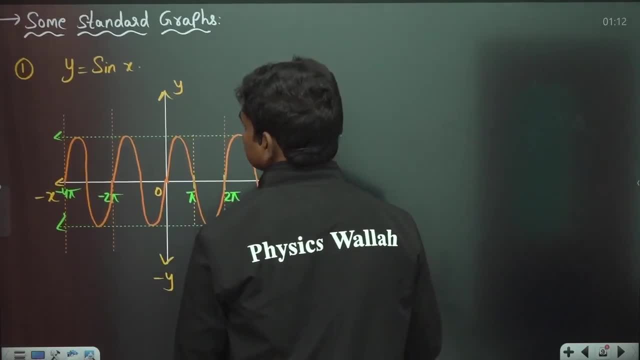 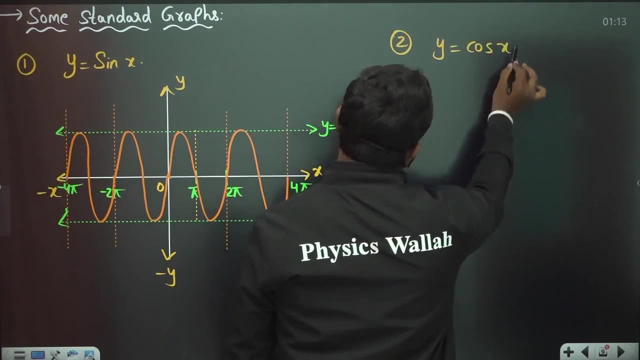 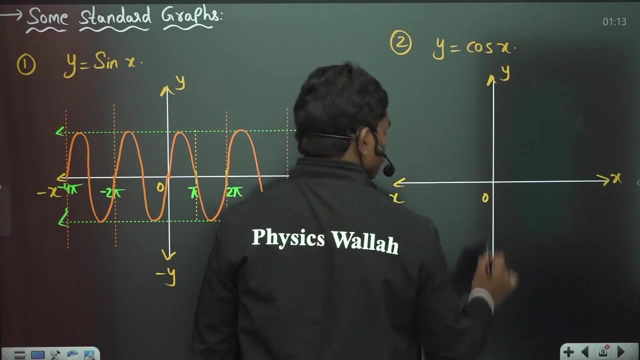 very clear of this. so cos x, y is equal to cos x, y is equal to cos x. again same graph, same graph here: x 0 minus x, y minus y. then you have your maximum and minimum limits. so maximum is y is equal to 1, let us say, and y. 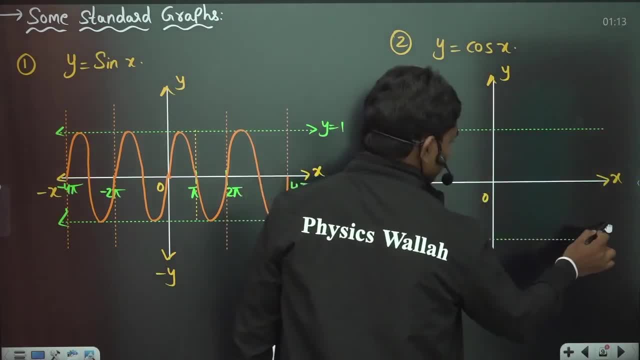 is equal to minus 1 is the minimum. so if this is y is equal to 1, and if this is y is equal to minus 1, then again you can identify certain periodicity for this also: 2 pi intervals, so 0 to 2 pi, then again 4 pi. 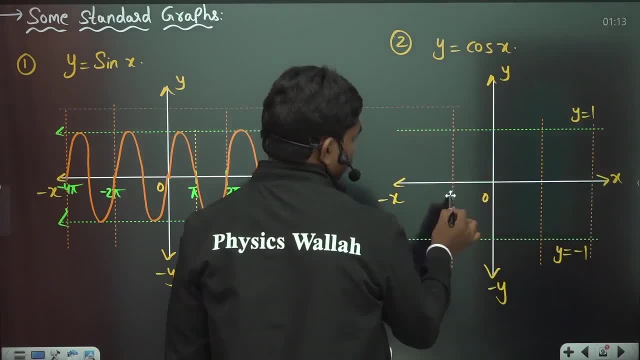 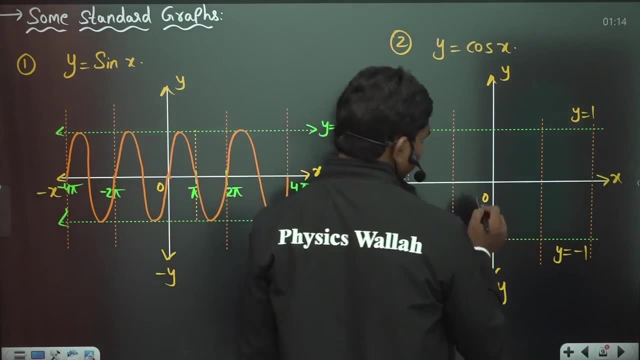 minus 2 pi. minus 2 pi and minus 4 pi, something like this. okay, so this is minus 4 pi. now, if you draw the graph in between this, then definitely you know at cos 0 this is 1, and also if this is 2 pi, for example, 4 pi, now you know cos 2 pi is also 1. so if you go for the graph, 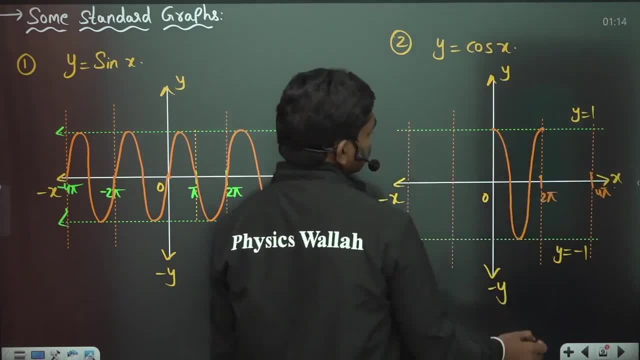 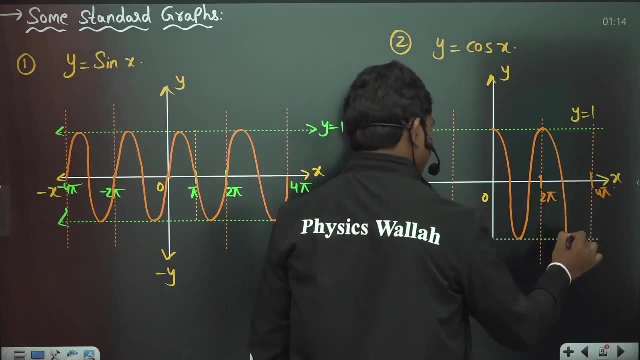 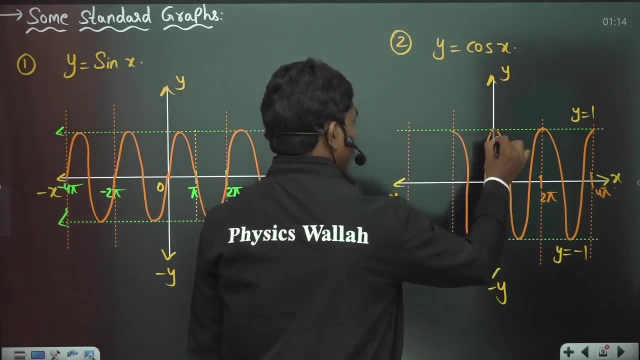 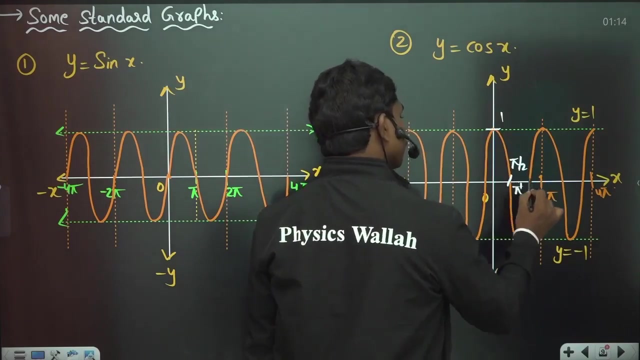 it goes something like this, correct. so similarly you can. you can connect similarly here, similarly here. so if you draw the graph of cos x is something like this, such that the cos 0 value is 1 cos pi by 2, 90 cos pi minus 1, cos 3 pi by 2, again 0, cos 2 pi again 1. so this basically goes. 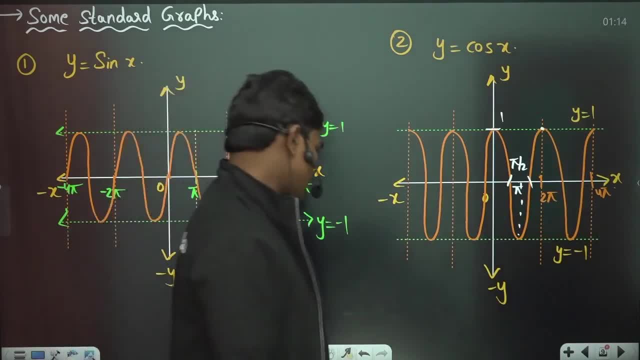 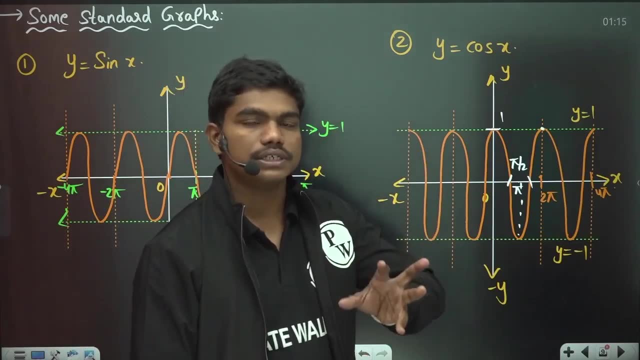 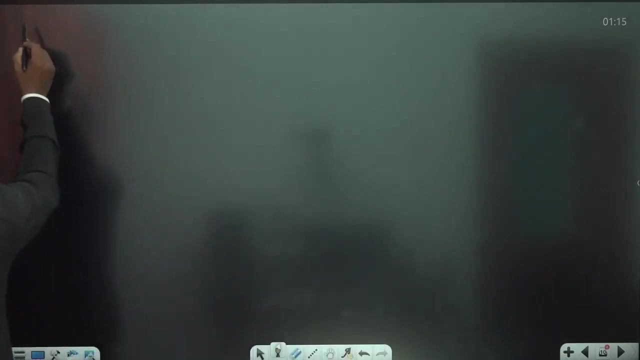 on. okay, so this is how you need to generate the graphs. okay, so now, and as i told you in linear algebra class, also, whenever you want to identify how a graph looks in general, for your interest, this must is one very good graphing calculator. okay, now, third graph which i would like to give you is tan x. 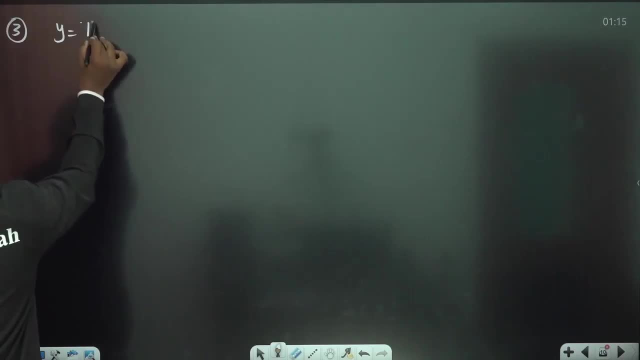 one very important limit i'll give you at this graph: y is equal to tan x is. look, i'll tell you, tan x is also something like this: sin x by cos x. so you know, or is in x minus x, y and minus y. now you have down the coordinate system. now you know if 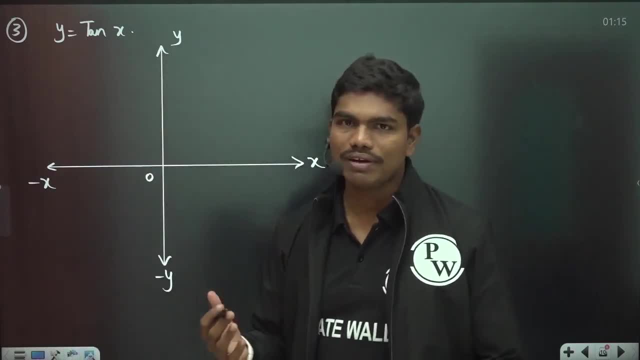 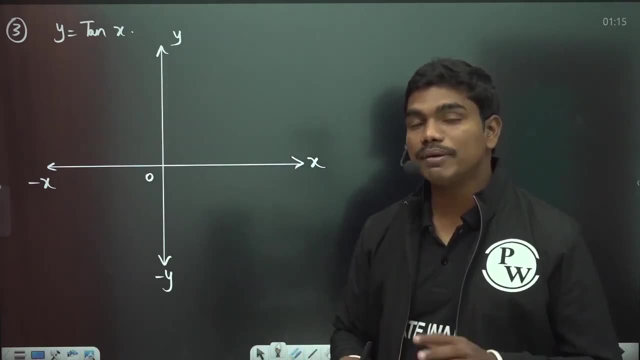 you ask for minimum and maximum values of tan x. you, you don't have any finite values, correct? in case of sin x and cos x, you have plus 1 and minus 1, but in case of tan x, you don't have any maximum or minimum values. so we don't have any limitations. okay, leave now. 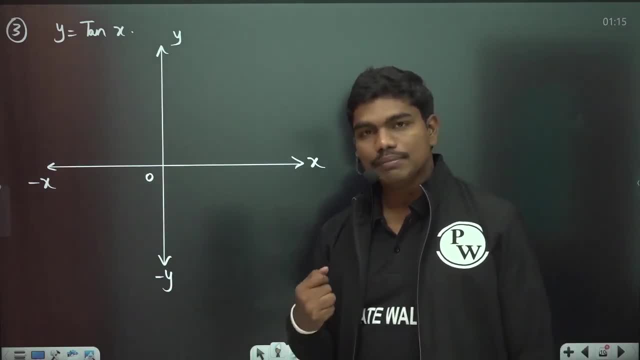 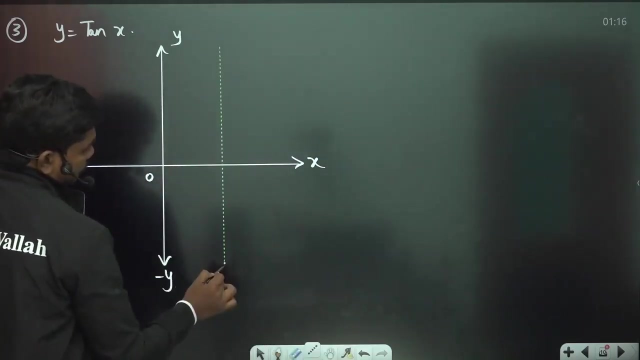 do tan x graph have any periodicity? okay, this is what you need to check. means: is tan x graph repeating in nature? yes, it is repeating, and the period is pi means: after every pi intervals, the graph repeats. okay, so let us check here. so, if you check this, this is pi. 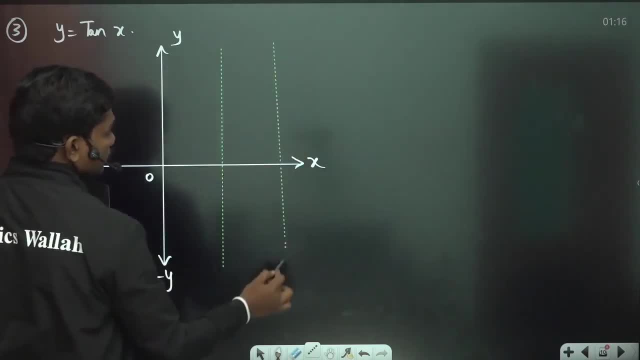 then this is 2 pi. this is 2 pi. similarly, this is minus pi. this is minus 2 pi. okay, so this is minus 2 pi. now if you see what is the shape of the graph: from 0 to pi, 0 to pi, 0 to 2 pi. so again to observe, from 0 to pi, let us take 0 to pi by 2, also pi by. 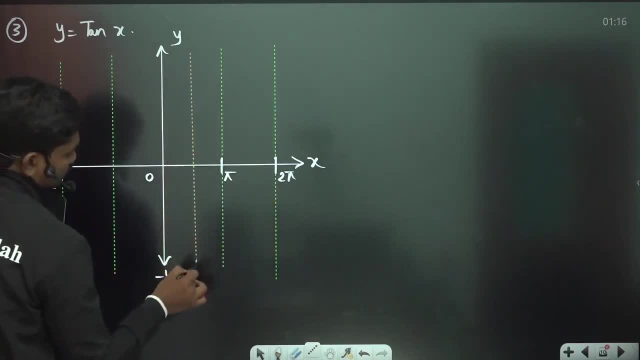 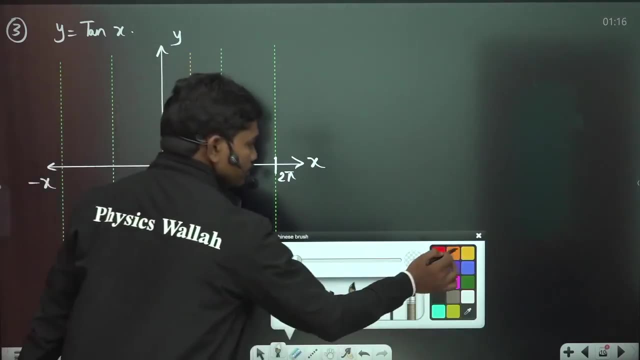 2. also, let us take one value, so pi by 2. let us suppose you are splitting this at pi by 2, for example, for easiness. that's it okay. so if this is for pi by 2, then you know from 0 to pi by 2. 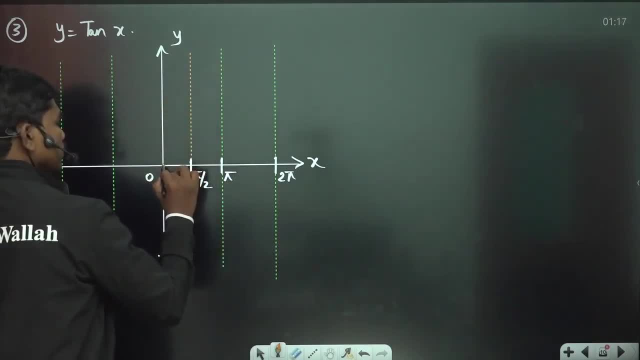 the graph changes from 0 to, because tan 0 is 0 for it changes from 0 to infinity. similarly, from minus pi by 2 to pi by pi. it turns out like this: okay, so this again continues similarly. this again continues like this, okay, so let me draw some neat sketch. so if you see, 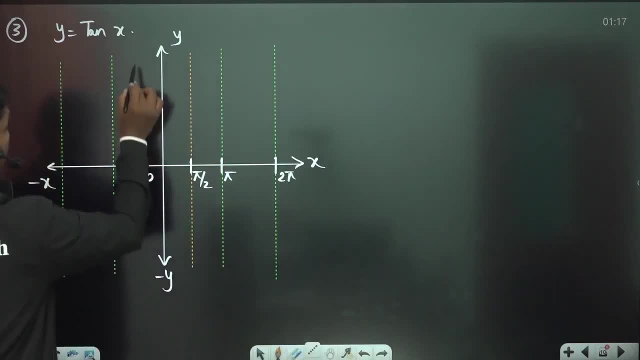 if you see, if you have some minus pi by 2 here, minus pi by 2, let us say, then the graph is something like this: it changes very steeply after pi by 4. actually. similarly, if you have some one more interval here, so then you will have: 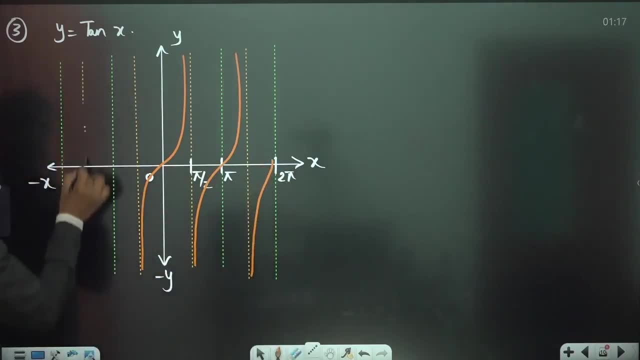 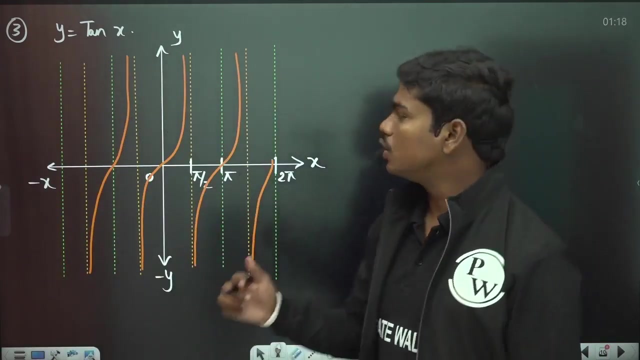 similarly, if you write one more interval like this, then the graph is something like this: yeah, it starts here, basically, and okay, so this is how the graph of y equal to tan x looks like, actually. okay. now here i would like to tell you one very important limit actually in this context. look, if i ask you what is the? 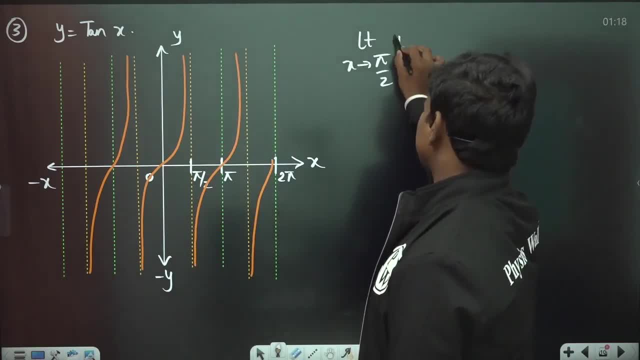 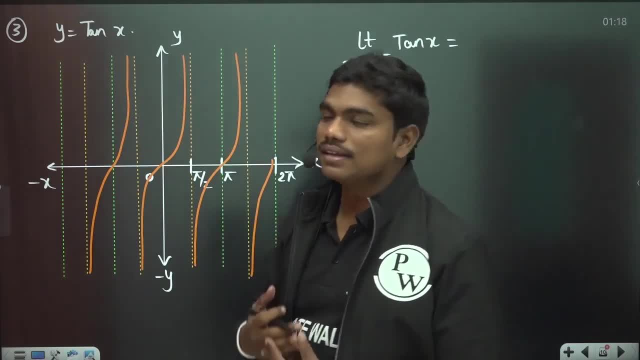 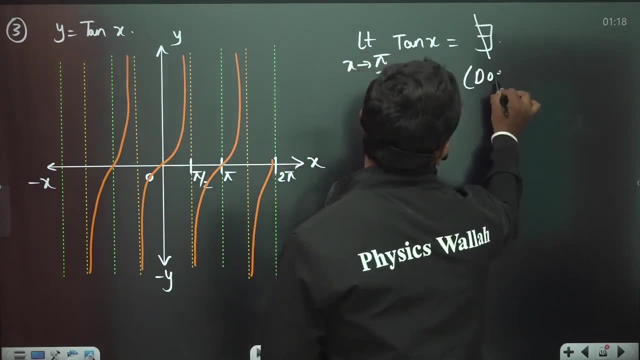 you substitute x equal to pi by 2, tan pi by 2 is infinity, but this limit actually does not exist, okay, so this limit does not exist. okay, this is the symbol for does not exist. okay, normally these are called quantifiers and this is doesn't exist. now why this limit? 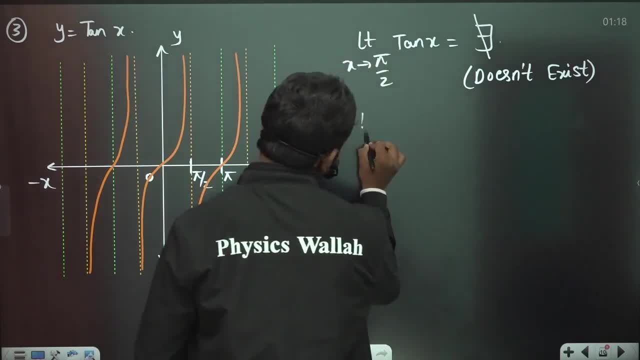 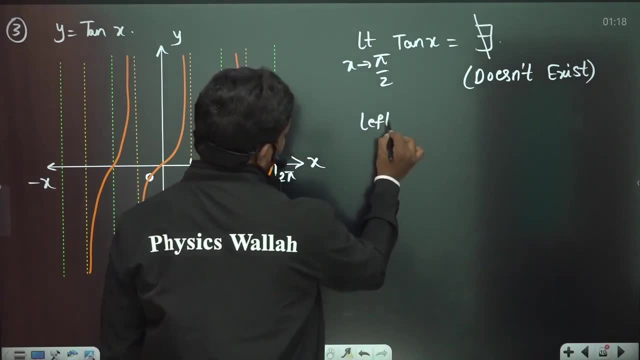 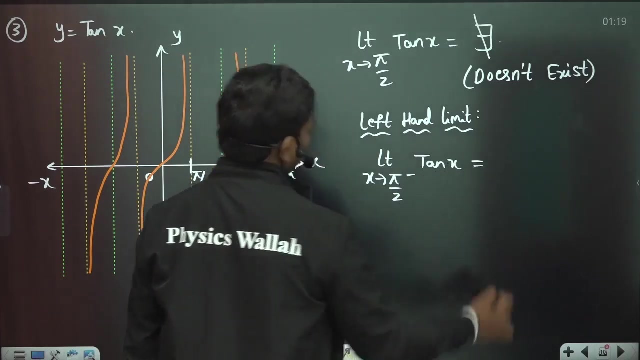 doesn't exist, i'll tell you. look, let us suppose, if you calculate left hand limit, okay, if you calculate left hand limit, left hand limit, let me write completely: so if you calculate left hand limit, if you calculate left hand limit, then limit extends to pi by 2 minus tan x. so if you see this value now, 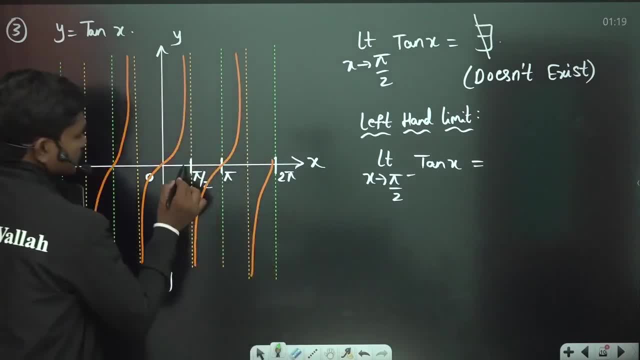 what is pi by 2 minus this interval? basically, okay, so this interval, this is pi by 2, so pi by 2 minus is slightly less. so we can understand one thing: as x is moving to pi by 2 in this direction, as x is moving to pi by 2 in this direction, 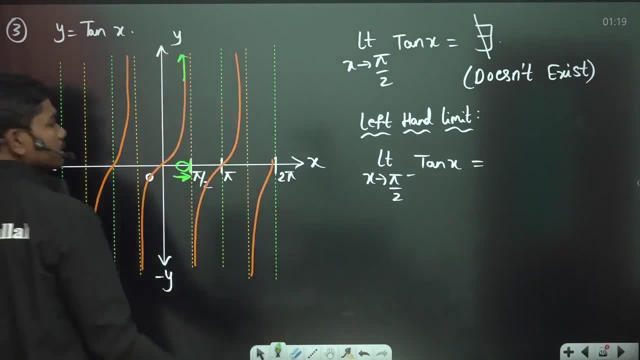 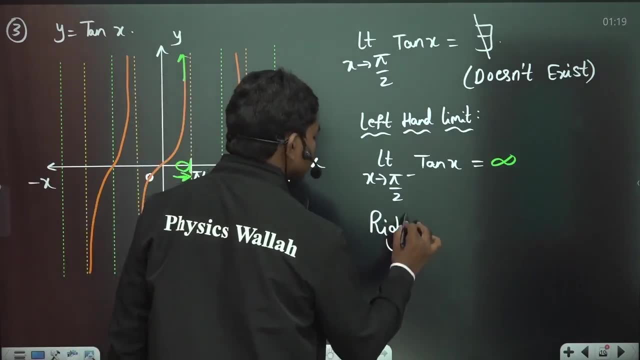 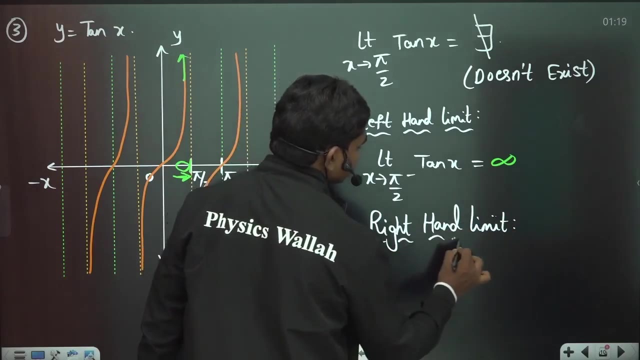 this f of x will move towards plus infinity. that, so that's why this value is infinity. now coming to right hand limit. if you take a right hand limit, if you take a right hand limit, if you take a right hand limit, then in that case you can understand one thing if i write: 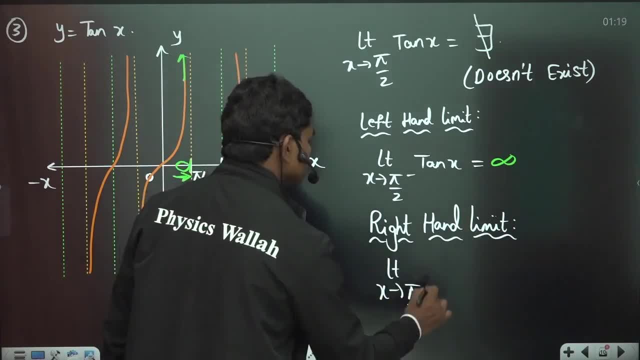 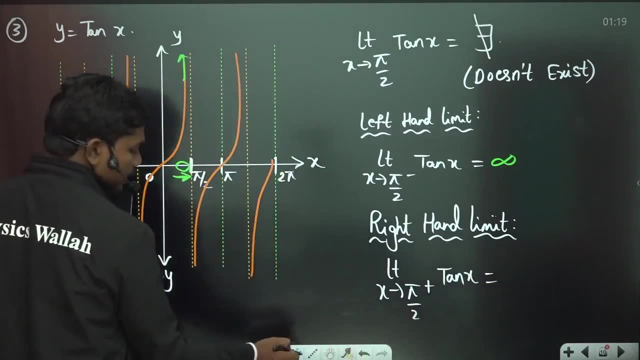 limit: x tends to pi by 2 plus tan x. okay, so let us suppose i'm writing x tends to pi by 2 plus tan x. now pi by 2 is here. so as x is tending to pi by 2 plus, that means x is somewhere here. and 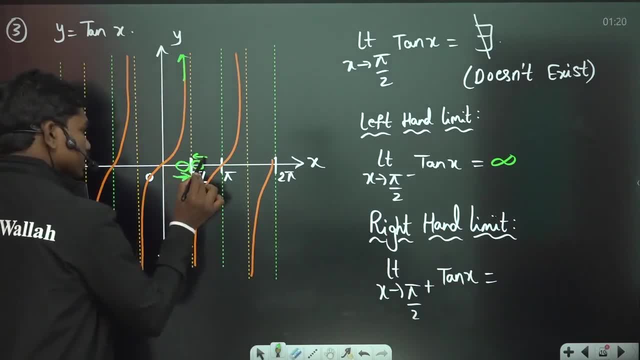 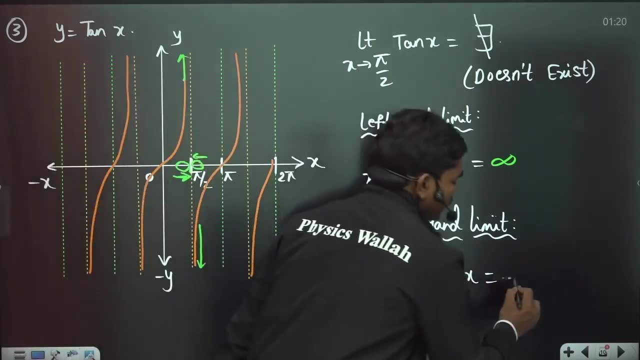 it's moving towards this direction. so you can understand. as x is moving in this direction, this f of x curve is moving towards minus infinity, correct? so this value is minus infinity. so one value is plus infinity and another value is minus infinity, and you can see clearly. 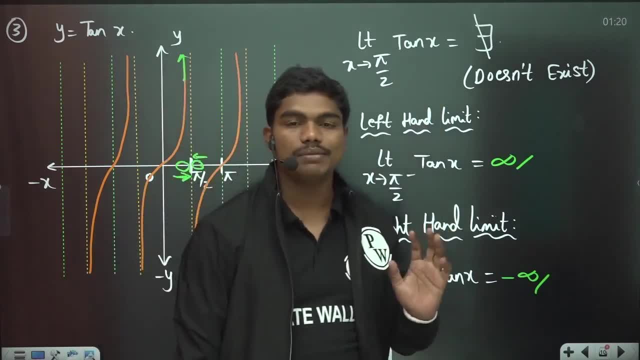 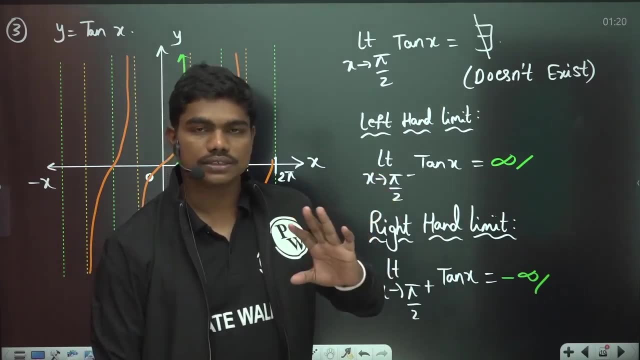 these two are not same and of course this that's the reason why limit extends to pi by 2: tan x does not exist. okay, it's not like blindly you substitute x equal to pi by 2 and you feel infinity. no, that's the wrong way of answering. but actually, if you see clearly, 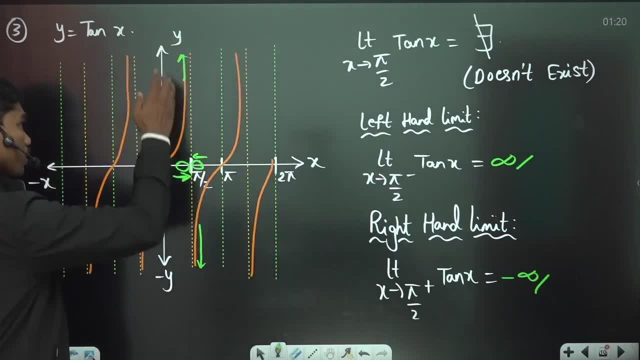 visually, if you see x tends to pi by 2 plus and x tends to pi by 2 minus. if in one case it is minus infinity, i mean sorry, in one case it is plus infinity and in another case it is minus infinity. so that's why this limit is one very important limit. many times they 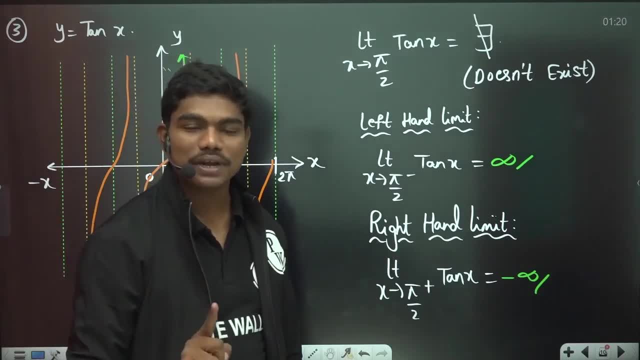 ask you in exams with the first option as infinity okay. so never fall in the trap of that substitution. substituting x equal to pi by 2, and you know writing infinity okay, limit extends to pi by 2. tan x does not exist, okay. so please keep this in mind. clear now. 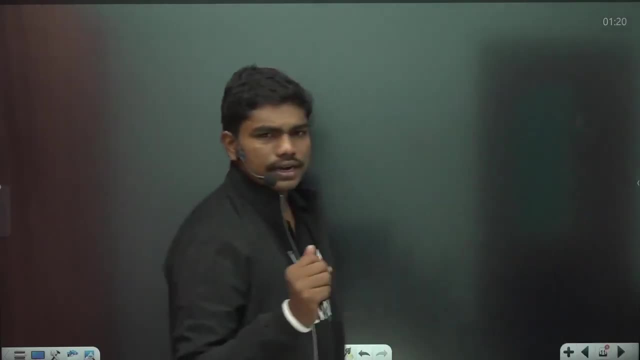 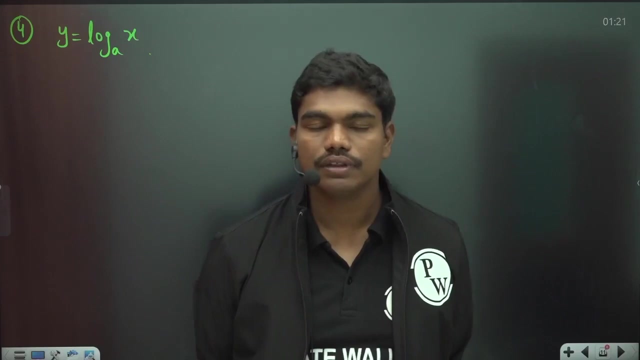 we have seen sine x, cos x, tan x. then let us see some normal functions also. for y is equal to log x to the base a. let us suppose okay if i write log x to the base a. actually okay now if i, because this is one very important graph that people ask you to draw in interviews. 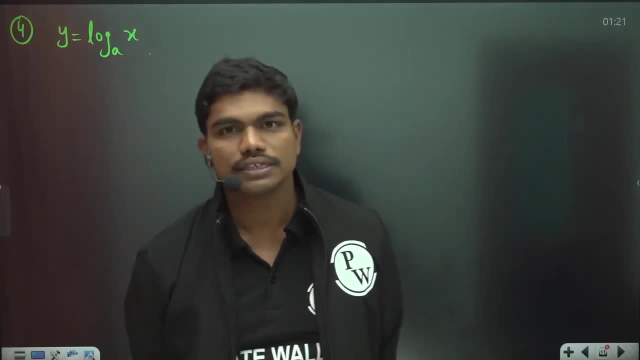 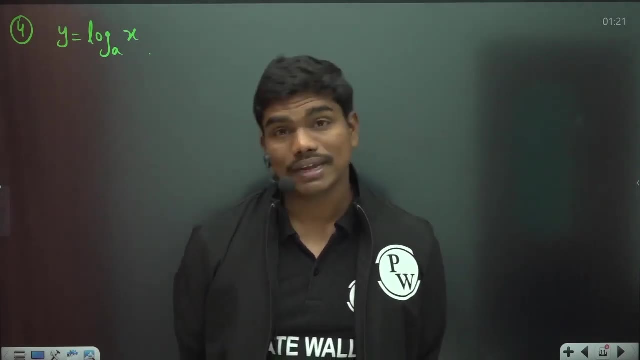 actually okay, because even in my barc interview also there are few people with one of the person. i mean, there is one person for mathematics and generally if you go for iit interviews or you know, sometimes psu interviews also, like i mean not hbcl and all but research oriented. 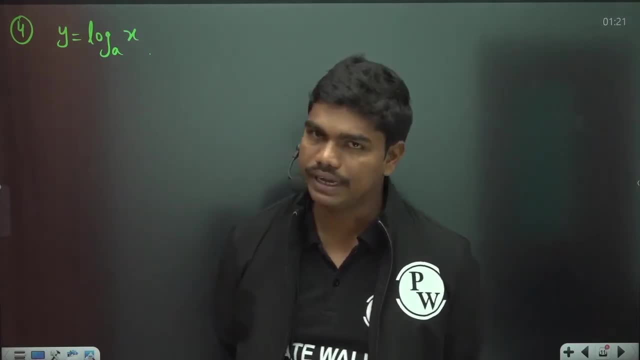 drdo or isro- maybe you know brc, all these things. then definitely they'll be doing research. they'll be having very strong fun. you know knowledge on mathematics, okay, so let us suppose if they ask you some mathematical questions, you should be able to answer them. okay, so? 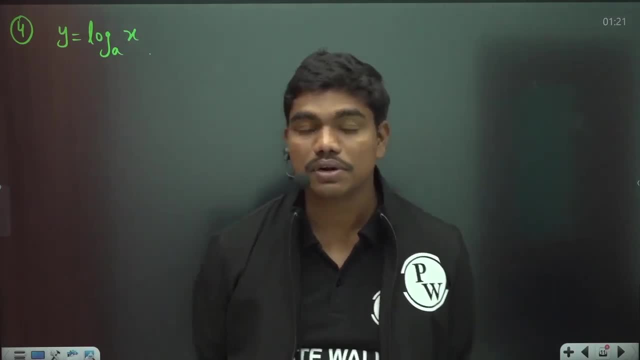 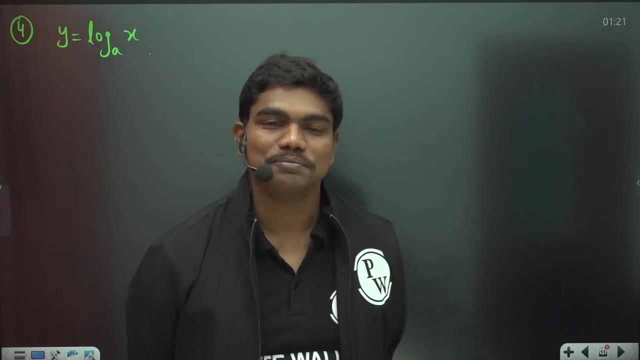 this graph is one very famous graph that's asked in interviews: y equal to log, x to the base a. now, as soon as they ask you this question, log x to the base a. if you slightly start drawing something, they understand that you don't know anything. okay, why? because this: 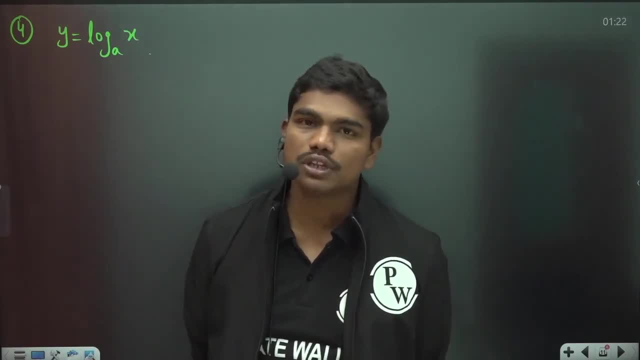 graph the shape of this. i mean shape is same, but depending upon the, you know, quadrants. actually the value of a depends. okay means basically, if i give you, until and unless i give you the value of a, you cannot draw the graph. okay, why? because it has two different. 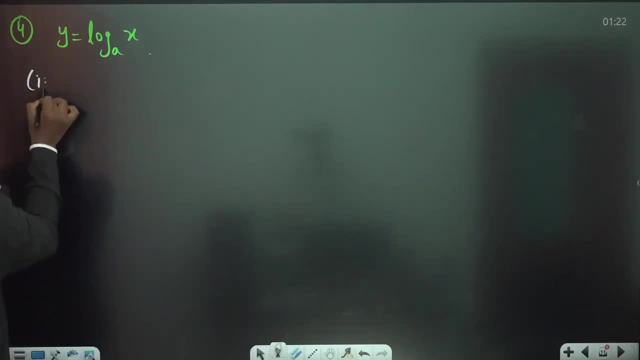 curves. look, i'll tell you. first, if zero less than a less than one, second a greater than one. so these are the two things. now let us see how they look like. so let us suppose. so why am i writing? so this is the real way i will calculate. so i am not considering negative. 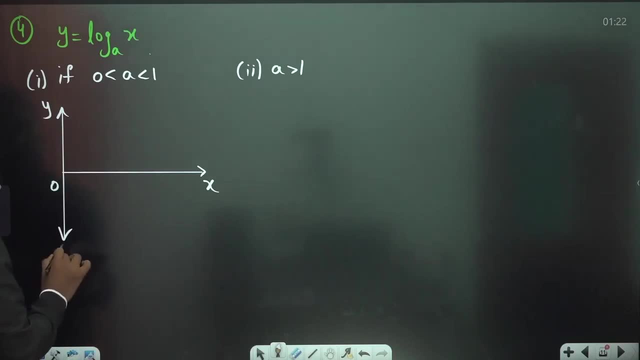 axis for log. okay, y and minus y. so if this is the case, similarly, here also let me draw out the graph: y for y. okay, this is simply: i have x, i have y and y, and all of them areouguh armies. so 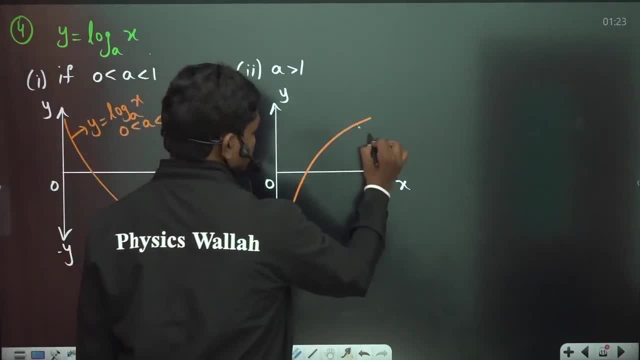 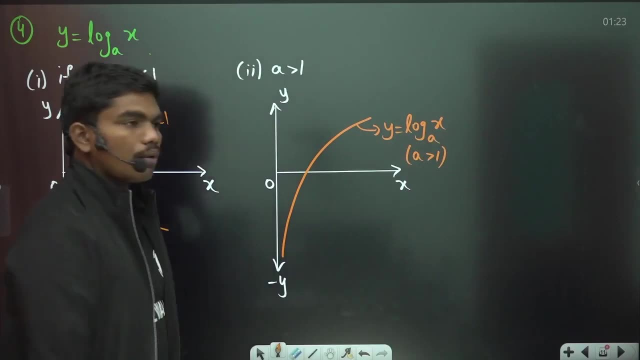 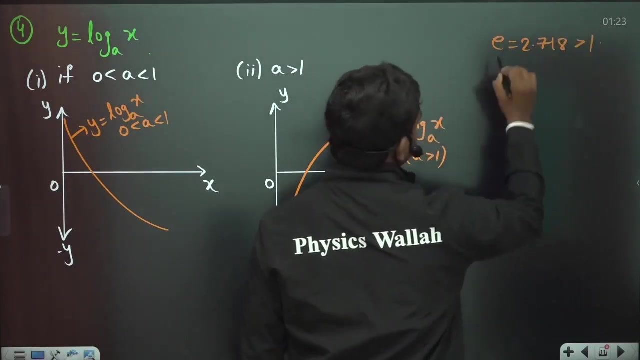 this is then. y is equal to log x to the base a and, of course, when a is greater than 1, so you know normally this natural exponent, okay, so e, for example, e value is around 2.718, which is actually greater than 1. that's why, log x to the base e. you will find the graph in this shape, because a is less. 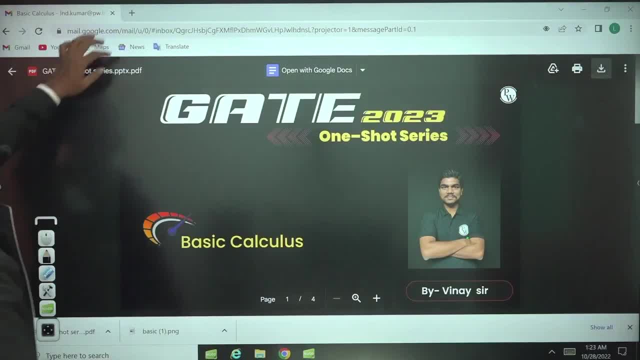 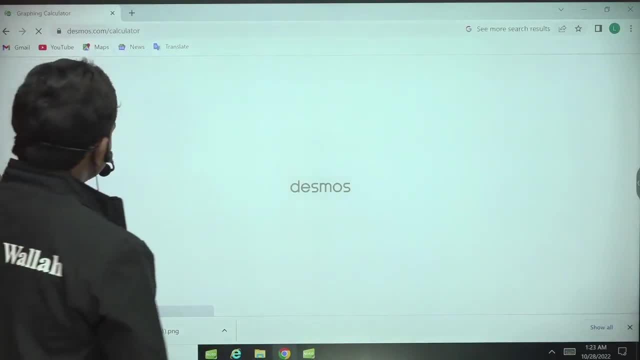 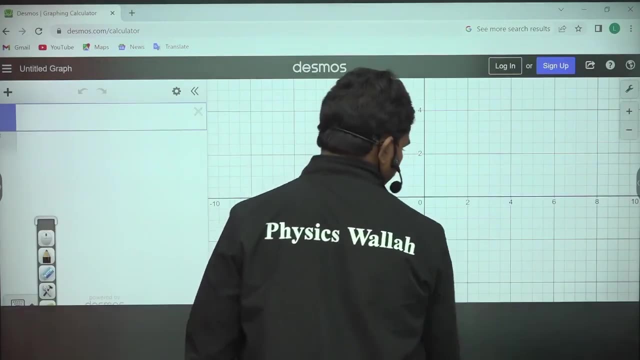 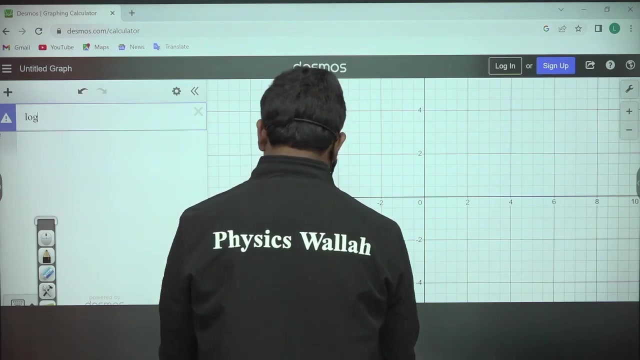 than 1. okay, look, for example, i can show you because we'll use some decimals plotting, you know so decimals graphing calculator, so let us plot both on this graph, okay, so first we'll plot something. i think: yeah, here we have. so see here log. you know, we'll write to the log, to the base. 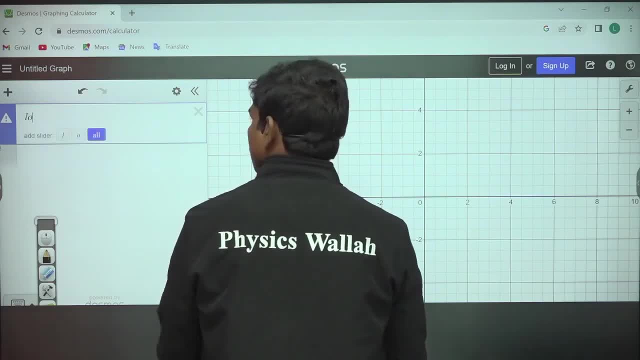 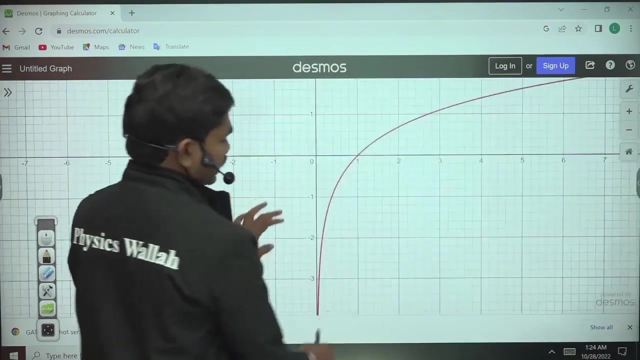 let us write base log to the base. we can write as shift underscore: log to the base. we can write as shift underscore: yes, log. so, for example, let us write e, for example, okay, and then let us write x here, for example. so log e to the base x, x. you can see log e to the base x. the graph is something like this: okay. 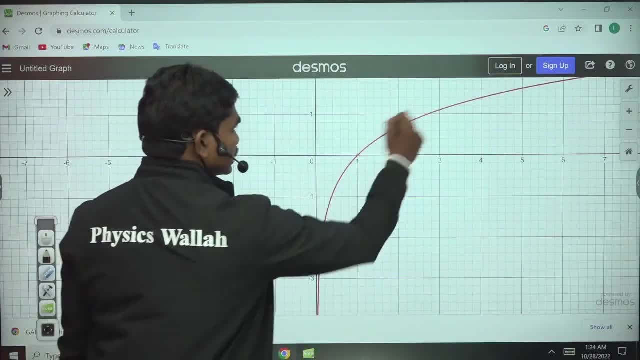 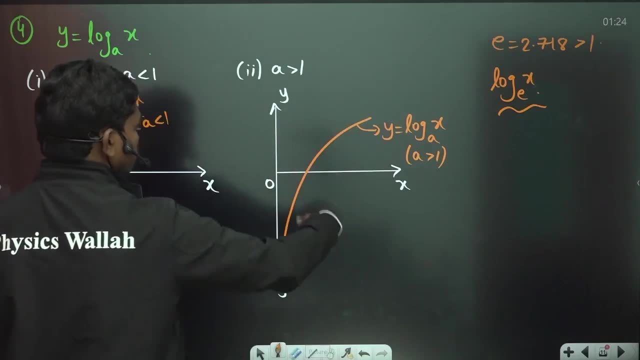 so, basically, this is your x axis, which i have shown, and this is the graph of y- is equal to log x, like the shape, what i have shown you. of course this will be slightly steeper like this, but i have my intention is to just show you the graph. but let us suppose, in case of e, if i have substituted, 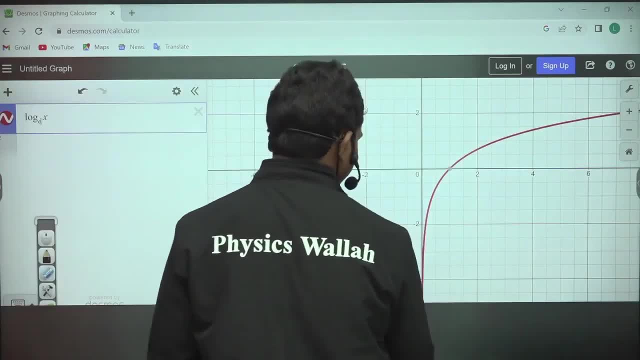 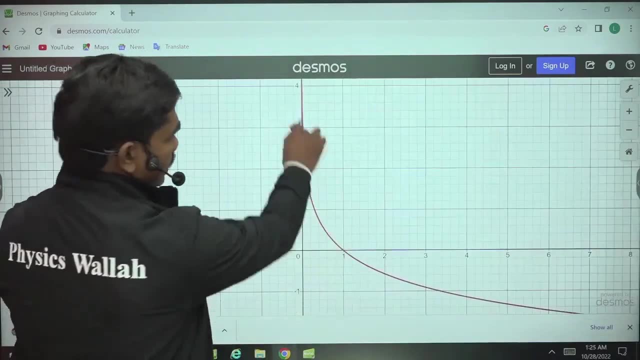 some different value, say uh, for example, 0.3, something like that, 0.3, for example- then you can see immediately the shape of the graph got changed. it's it's now in the different turn, okay. so that's why i have given you two different graphs whenever a value changes, basically the 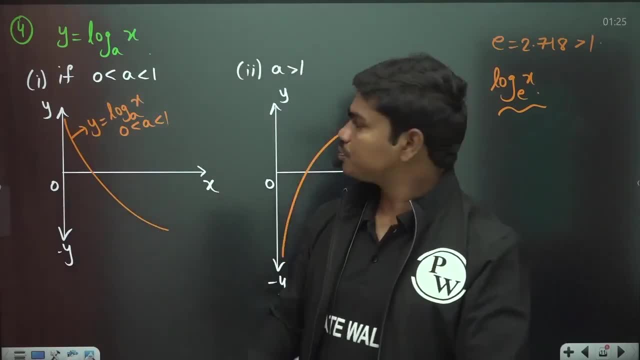 shape of the graph changes. okay. so in interviews if someone asks you what is the shape of that function means if they ask you to draw immediately you will get the shape of the graph and then you can use the shape of the graph to draw out the graph, which is exactly the first question you should. 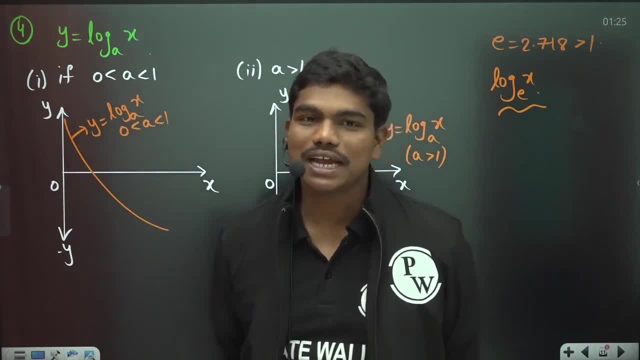 ask them is so what is the value of a? okay, then let us suppose if they tell, a is equal to one, because i have given you for zero, less than e, less than one, and also a greater than one, but exactly at equal to one. you don't have any logarithms. okay, log to the base one. 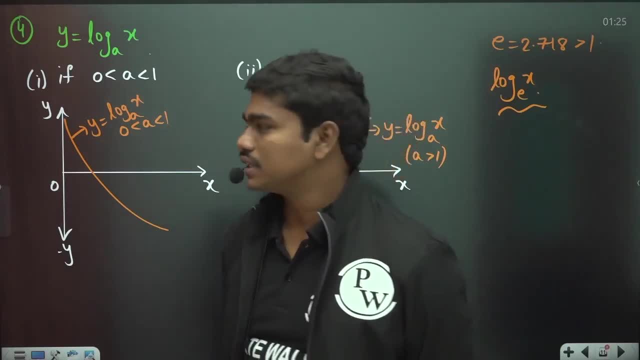 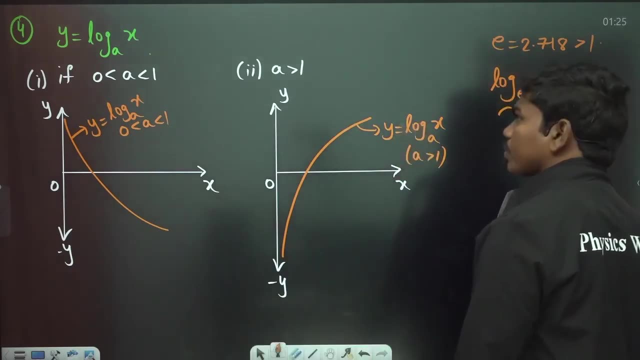 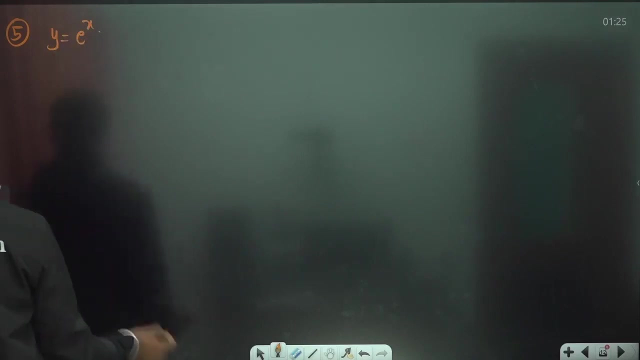 does not exist because that's not unique, actually. okay, so that's the reason. so anyhow, if you see, this is 4 and this function is continuous. anyhow, we'll see what is continuous and all. now, fifth, fifth, y is equal to e power x. e power x. if you take, then definitely you know e power x graph is something like this: 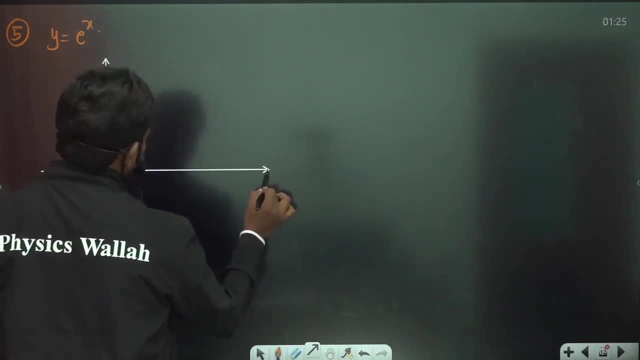 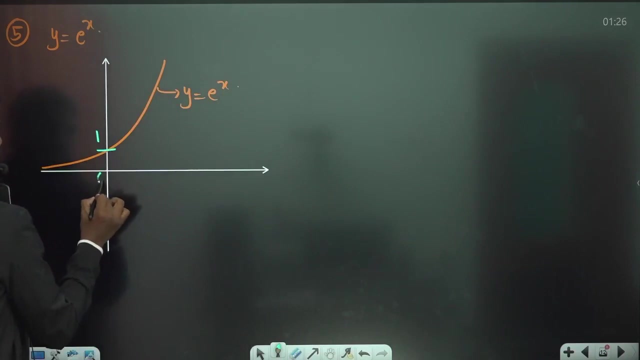 so you know, exponential functions are not negative means basically, at least when the base e. so if you draw the graph of y is equal to e power x. it goes like this: okay, so this is y is equal to e power x. and you know, at x is equal to 0, this value is 1. okay, so this value is 1 and this is 0. 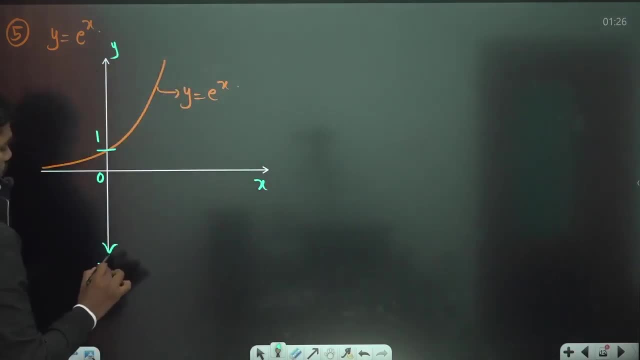 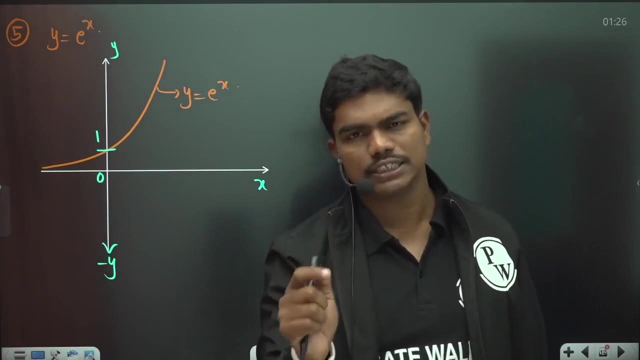 okay. so x, uh y and minus y. okay, so this is: y is equal to e points. why i am drawing all these curves? because we, after some time, we'll you know, uh, we'll deal with something called multiple integrals, or uh, you, you, you deal with, uh, area under the curves, all these things. so that's the reason why i am. 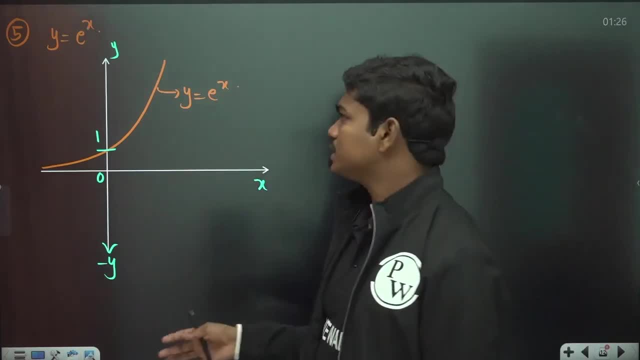 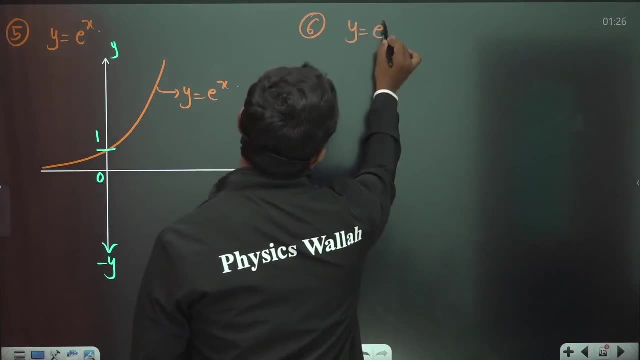 giving you this. okay, you will find length of the curves, okay. so all these things we'll discuss in detail. okay, so sixth, y is equal to e power minus x. this is very simple now, okay, because you see, whatever the values of y that are coming for positive values of x, same values will come here but for negative. 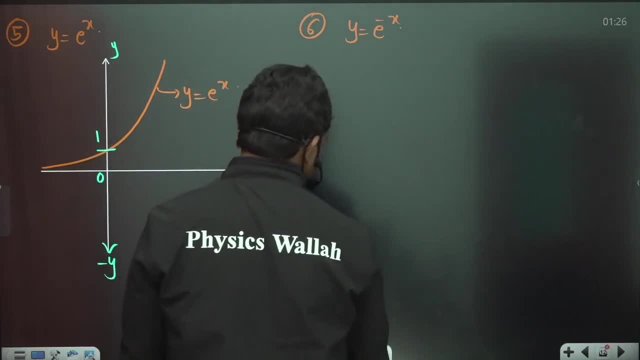 values of x. okay means this gets a worst, actually, okay. so if you draw the graph, it looks something like this: let us move here: 0, x minus x, y minus y. okay. now, if you see, the graph is something like this: if you draw it comes out to be something like this: okay, so this is y is equal to. 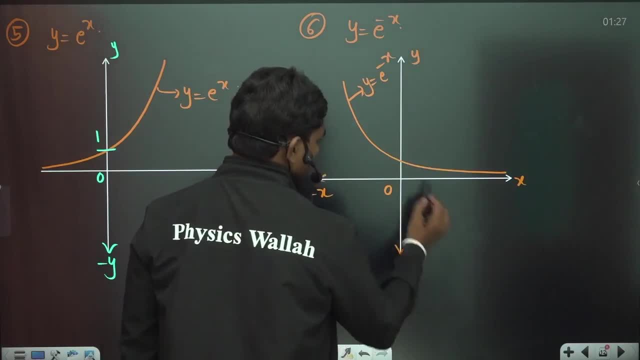 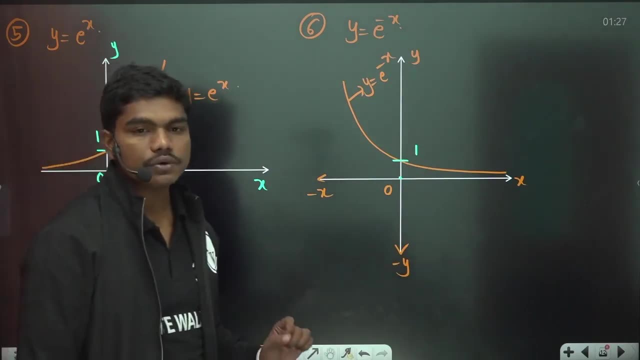 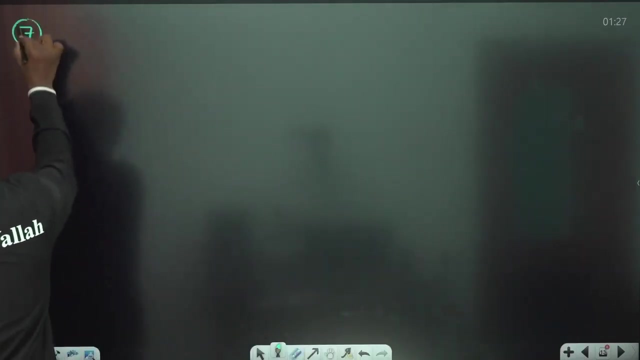 e power minus x. and again, of course, when you put x is equal to 0, this value is going to be 1 at this location of x is equal to 0. so this is the graph of y equal to e power x and y equal to e to the power minus x. next, i would like to give you graph of some mod function. y is equal to: 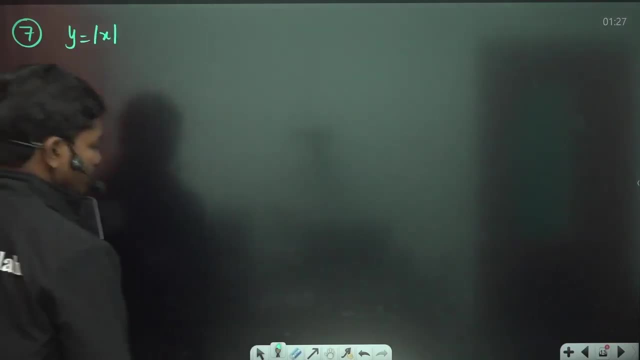 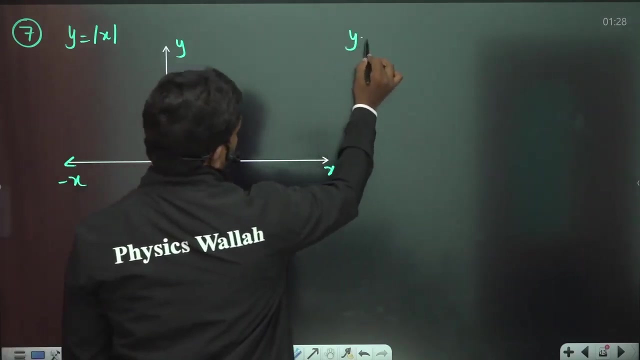 modulus of x. okay, so y is equal to modulus of x. so you know it's very easy. so, horizon: x minus x, y minus y. okay now, basically this function, y is equal to mod. x is actually defined like this. also, x when x is greater than 0. 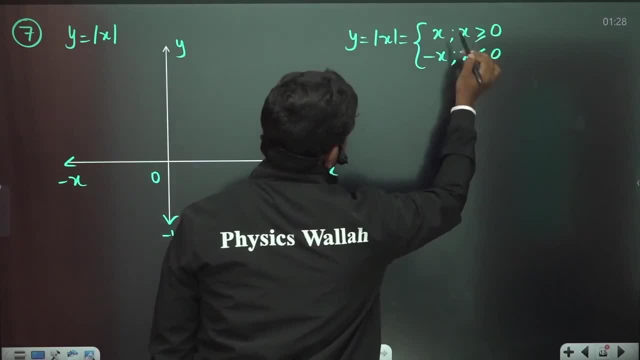 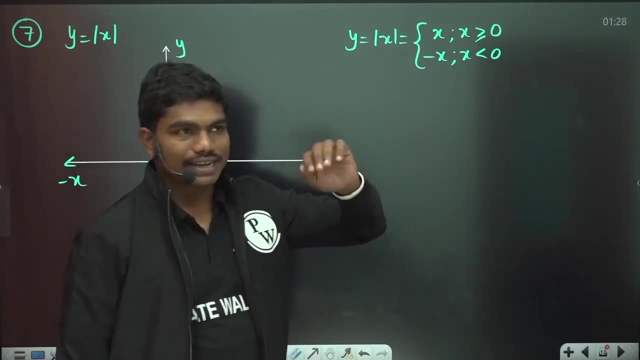 minus x. when x is less than 0, okay, you can put equal to at any place, maybe on the first part or second part. so the meaning of this is: whenever you know mod x function is always positive. means if i take even modulus of negative values, i'll get the absolute value. means basically, if i get 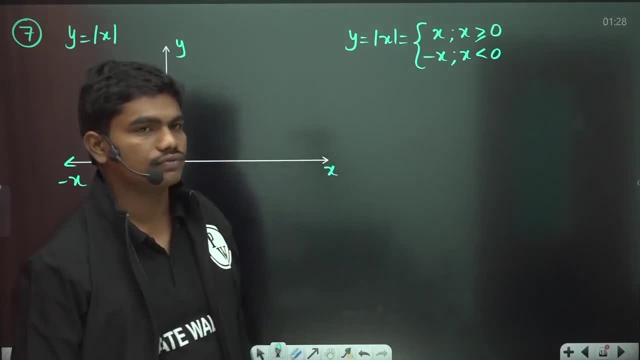 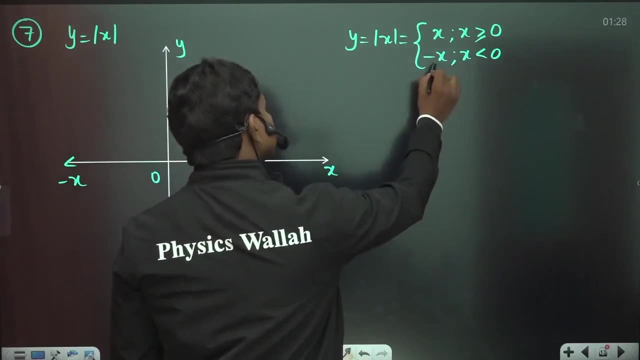 mod of minus 4 or minus 5, something again, i'll get 5 or 4. that's the reason. okay, so y is equal to mod x. now you can understand one thing: if x is negative, then minus x is positive, and if x is positive directly, it is x. now, whenever x is greater than 0 means, let us suppose, x is greater. 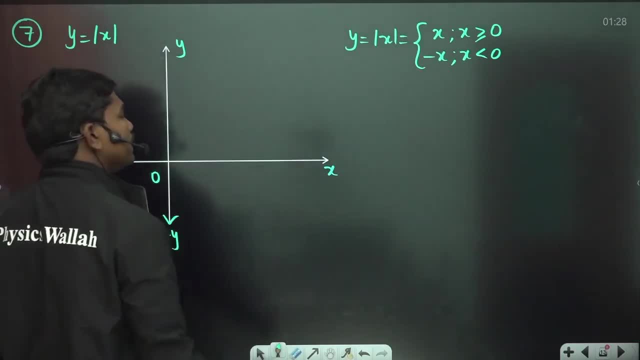 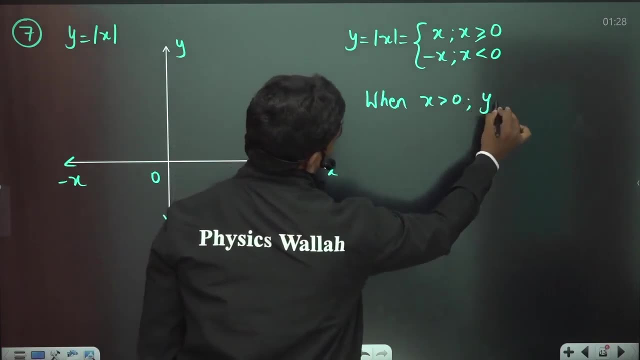 than 0 is to the right side of this y axis. okay, so that's of the form. y is equal to x, actually. okay, so n x is greater than 0. when x is greater than 0, the equation is: y is equal to x, or maybe you can put equal to sign. also, when x is less than 0, this y is equal to. 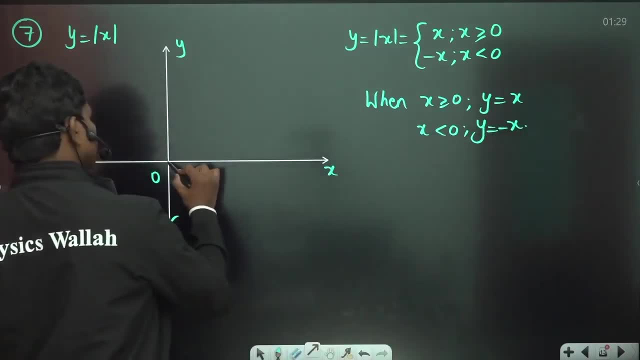 minus x. okay, so first, y is equal to x line. how does it goes on 0, something like this: okay, so this is: y is equal to x, y is equal to x. when x is less than 0, this becomes y is equal to minus x. okay, so something like this: okay, so y is equal to minus x, y is 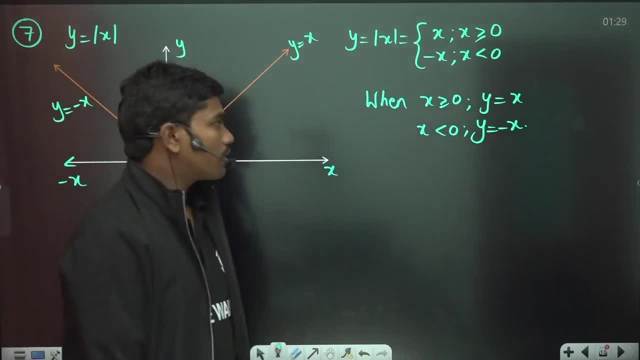 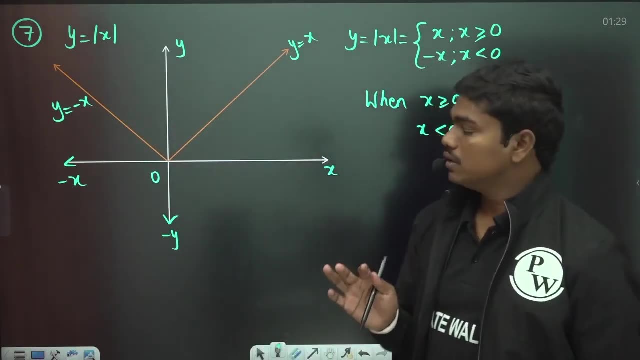 equal to minus x. that's the reason you have. okay, now try to understand one thing before. okay, i'll define what is continuity and all, how to check this mathematically, and all. but right now i'll ask you one thing: from minus infinity to infinity, is there any breaking of this function? did this? 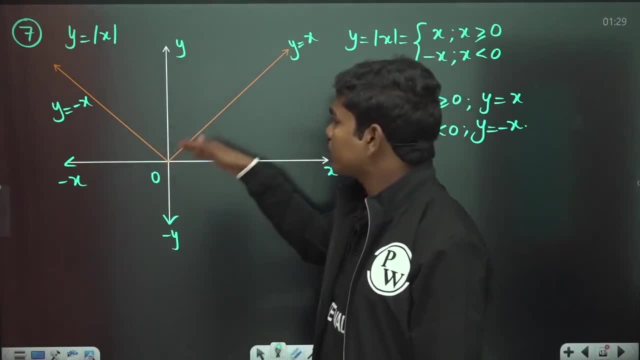 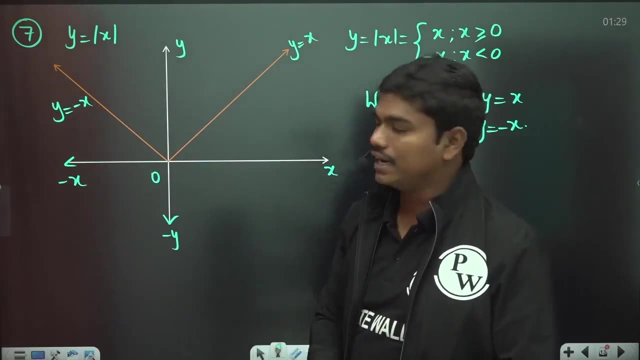 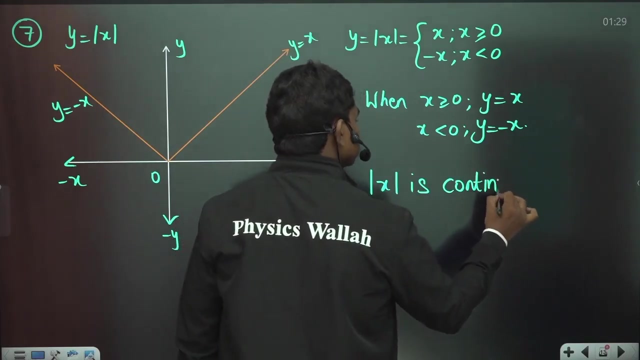 function i broke anywhere. no, it's a continuous graph. okay, you can see, there is a continuous function. there is no, uh, you know, any discontinuity means there is no breaking of this function anywhere. so that's why mod x is continuous. mod x is continuous for all real numbers. okay, there is. 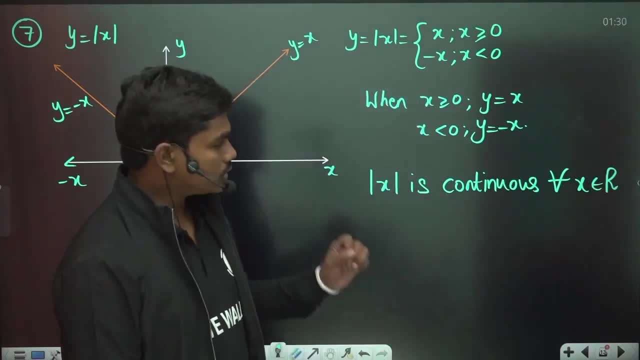 no, nothing like mod x is not continuous. mod x is continuous for all real numbers- okay. there is no, nothing like mod x is not continuous. mod x is continuous for all real numbers- okay. there is no, nothing like mod x is not continuous. mod x is continuous for. 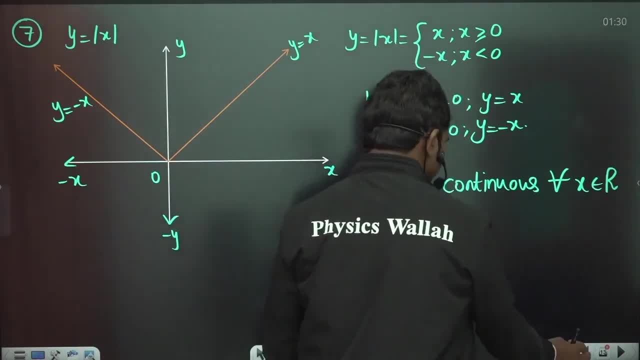 all the real numbers. okay, so, anyhow, this is the mod x function next. uh, i have given you seven, all the real numbers. okay, so, anyhow, this is the mod x function next, uh, i have given you seven- all the real numbers. okay, so, anyhow, this is the mod x function next. uh, i have given you seven graphs. okay, fine, so next, eighth graph. 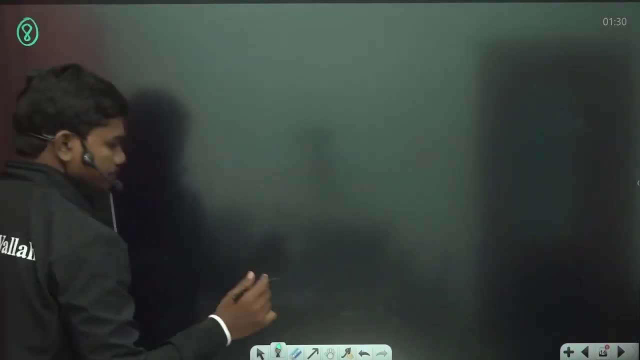 graphs. okay fine, so next eighth graph: graphs. okay fine, so next eighth graph: i would like to give you eight one, so we, i would like to give you eight one, so we, i would like to give you eight one. so we have talked about, have talked about, have talked about technometric functions: exponential. 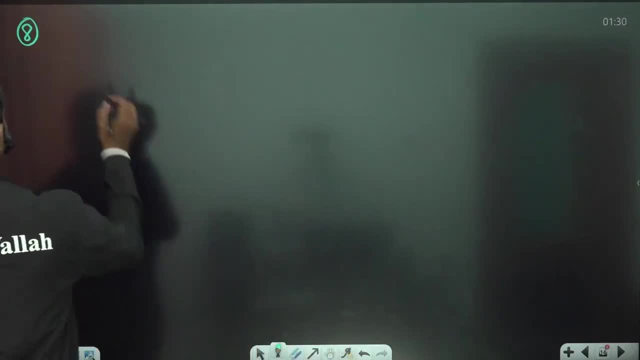 technometric functions. exponential technometric functions. exponential logarithmic algebraic functions. let us logarithmic algebraic functions. let us logarithmic algebraic functions. let us talk about: okay. so you know y square is talk about. okay, so you know y square is talk about. okay, so you know y square is equal to four, a, x, for example. 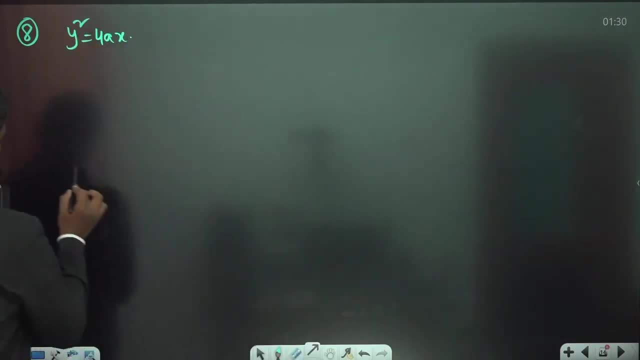 equal to four a x, for example. equal to four a x. for example, y square is equal to four x. so from this, y square is equal to four x. so from this, y square is equal to four x. so from this you can understand one thing whatever. you can understand one thing whatever. 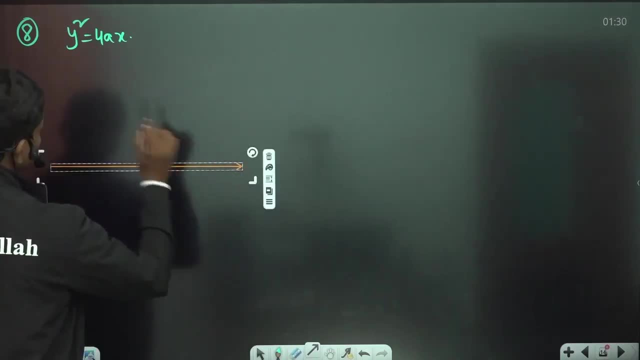 you can understand one thing: whatever the value of y x is always positive. the value of y? x is always positive. the value of y? x is always positive. correct means this function is not correct. means this function is not correct means this function is not defined for negative values of. 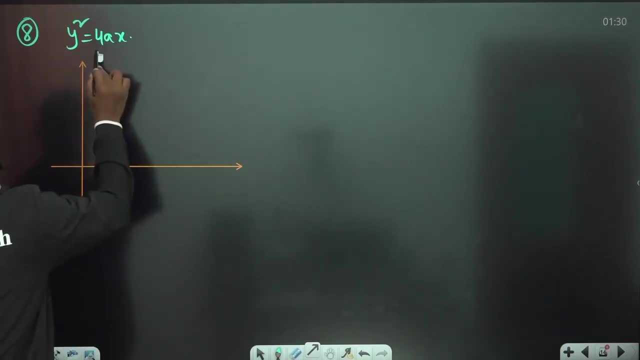 defined for negative values of. defined for negative values of y. i mean negative values of x actually y. i mean negative values of x actually y. i mean negative values of x actually okay. so if you see negative values of x, okay. so if you see negative values of x. 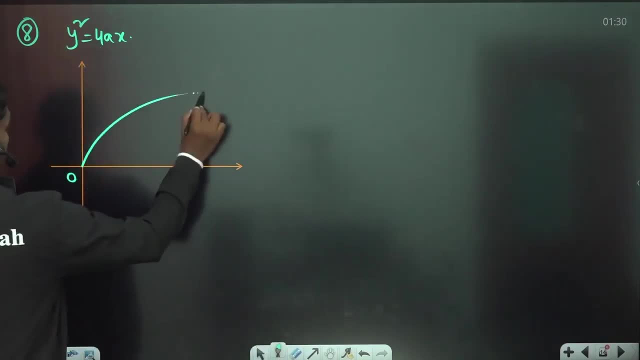 okay. so if you see negative values, of x has not defined, so this is zero. your has not defined, so this is zero. your has not defined, so this is zero. your graph looks something like this graph looks something like this graph looks something like this: okay, symmetric, of course. 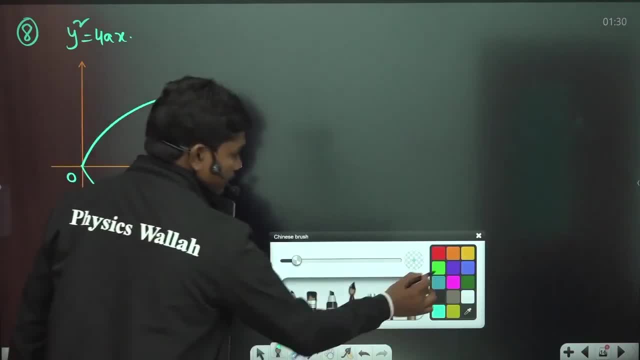 okay, symmetric, of course, okay, symmetric, of course. symmetric, okay, so symmetric. so this is y. symmetric, okay, so symmetric. so this is y. symmetric, okay, so symmetric. so this is: y square is equal to four. x square is equal to four. x square is equal to four x. y square is equal to four x. similarly, if 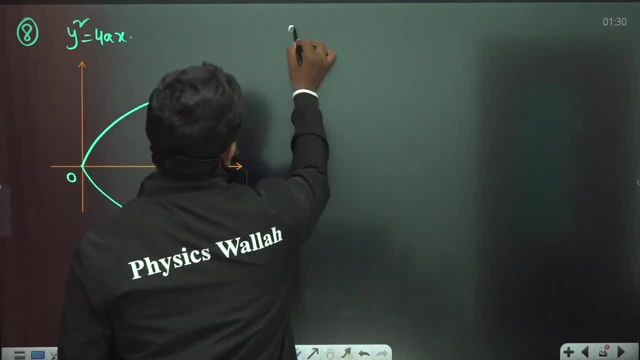 y square is equal to four x. similarly, if y square is equal to four x. similarly, if you write x square is equal to four a y. you write x square is equal to four a y. you write x square is equal to four a y. nine, nine nine, x square is equal to four a y. okay, so. 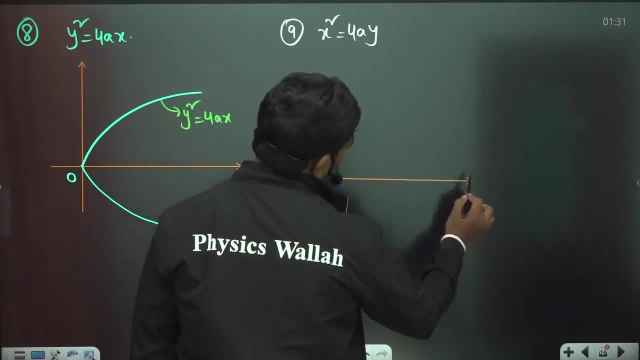 x square is equal to four a y. okay. so x square is equal to four a y. okay. so if you see now we can again plot that. if you see now we can again plot that, if you see now we can again plot that, you can again identify that y is never. 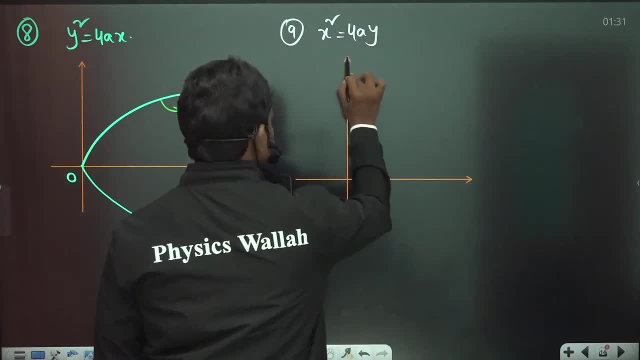 you can again identify that y is never. you can again identify that y is never going to be negative. so that's why, if going to be negative, so that's why, if going to be negative, so that's why, if you see, you see, you see the graph like this: 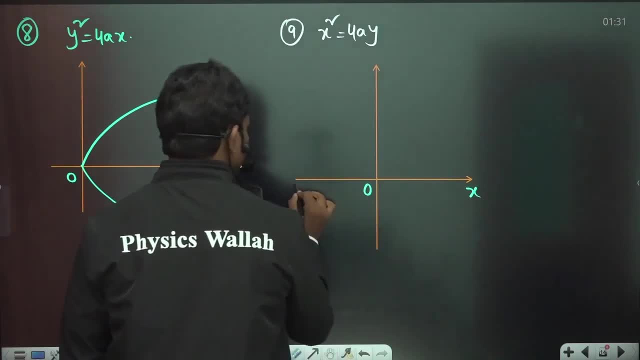 if this is horizon x, if this is horizon x, if this is horizon x minus x, y minus x, y minus x, y minus y, then the graph looks something minus y. then the graph looks something minus y. then the graph looks something like this, like this, like this: okay, so this is x. square is equal to. 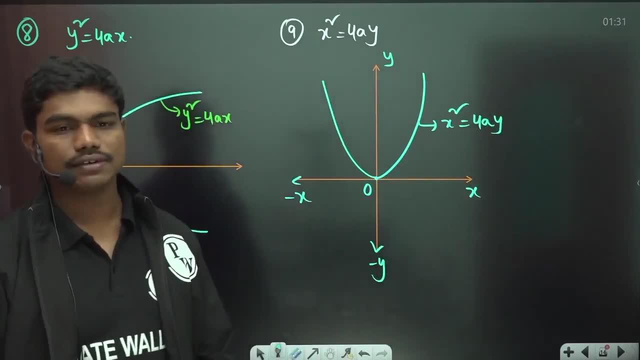 okay, so this is x square is equal to: okay. so this is x square is equal to four a y, basically. okay, so this is how four a y, basically okay. so this is how four a y. basically okay. so this is how you have different graphs. okay, you have different graphs, okay. so now let me, before concluding this, okay, i. so now, let me, before concluding this, okay, i so now let me, before concluding this, okay, i have given you some eight to nine, have given you some eight to nine, have given you some eight to nine graphs which are useful now before. graphs which are useful now before. 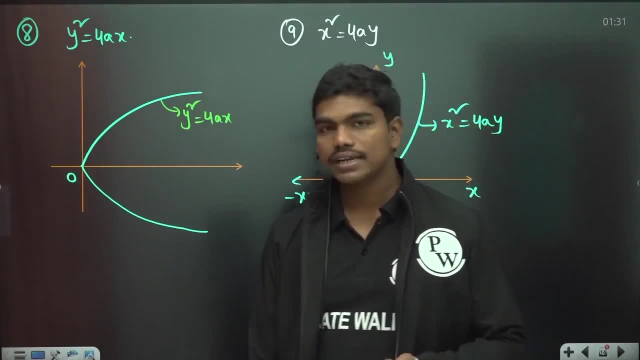 graphs which are useful. now, before concluding, i would like to give you two concluding. i would like to give you two concluding. i would like to give you two important graphs actually x into sine x. important graphs actually x into sine x. important graphs actually x into sine x and x sine x by x. actually okay, y sine x. and x sine x by x, actually okay, y sine x. and x sine x by x. actually okay, y sine x by x. i'm giving you will come to know by x. i'm giving you will come to know by x. i'm giving you will come to know when i teach you the concepts of maxima. 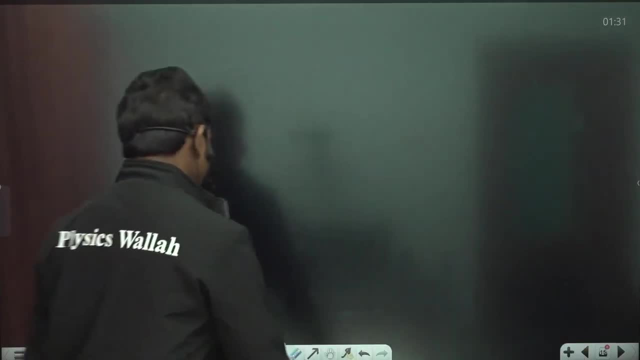 when i teach you the concepts of maxima, when i teach you the concepts of maxima and minima, okay, anyhow, let us see for and minima. okay, anyhow, let us see for and minima. okay, anyhow, let us see for now. so first, i hope it's tenth one, right? yes, tenth, so. 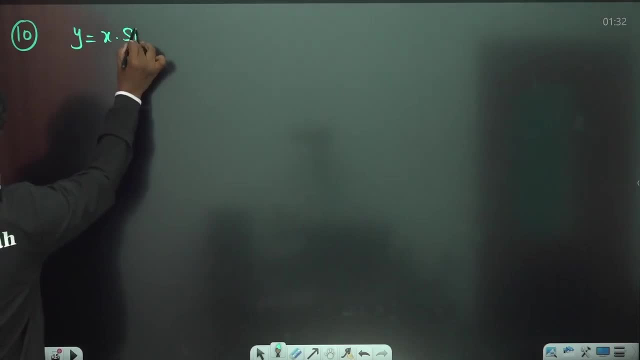 i hope it's tenth one, right? yes, tenth. so i hope it's tenth one, right? yes, tenth. so y is equal to x into sine x, y is equal to x into sine x, y is equal to x into sine x, x into sine x. now it's now, till now, almost. 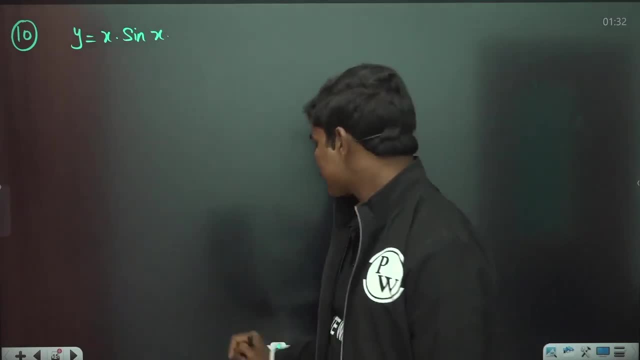 x into sine x. now, it's now till now, almost x into sine x. now, it's now till now, almost all the graphs, what i have done. you know all the graphs what i have done. you know all the graphs what i have done. you know right now how to draw this graph, okay, so 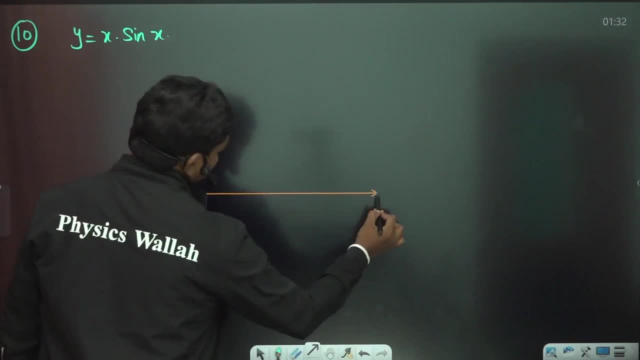 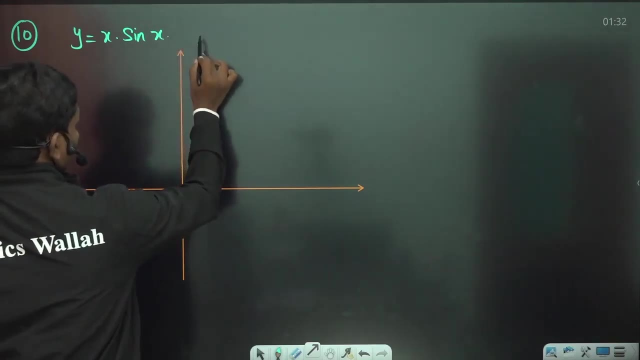 right now how to draw this graph. okay, so right now how to draw this graph. okay, so first, set up the coordinate system as first. set up the coordinate system as first. set up the coordinate system as usual. set up the coordinate system. set up the coordinate system. or is in x. 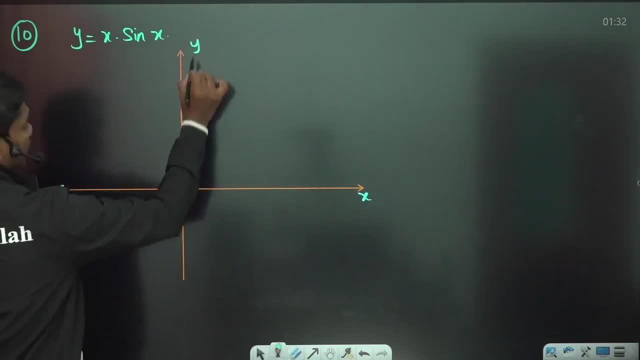 set up the coordinate system. or is in x set up the coordinate system? or is in x minus x, minus x, minus x, y minus y, y minus y. okay, now x into sine x. so you minus y. okay, now x into sine x. so you minus y. okay, now x into sine x. so you know, minus one less than or equal to. 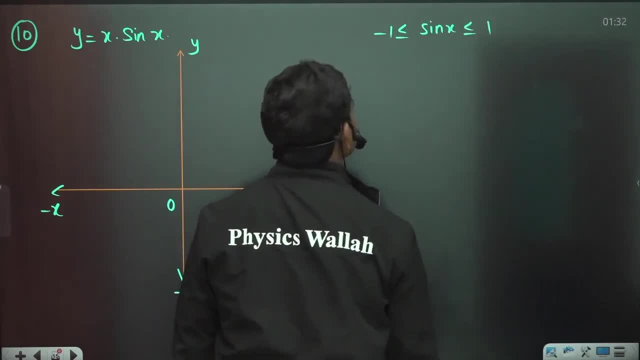 know minus one, less than or equal to know minus one, less than or equal to sine x, less than or equal to sine x, less than or equal to sine x, less than or equal to one, correct? so if you multiply x on all one, correct? so if you multiply x on all, 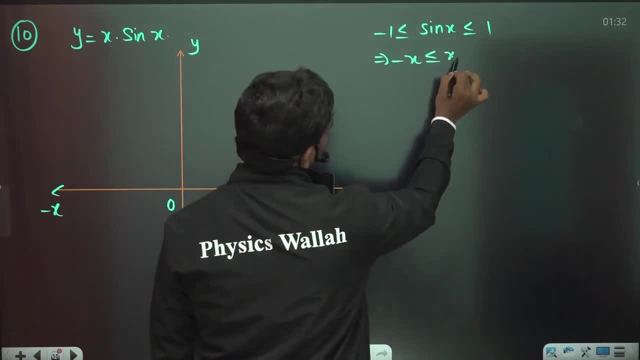 one correct. so if you multiply x on all the sides of this inequality minus x, the sides of this inequality minus x, the sides of this inequality minus x less than or equal to x. into sine x less than or equal to x. into sine x less than or equal to x. into sine x less than or equal to x. so which means one? 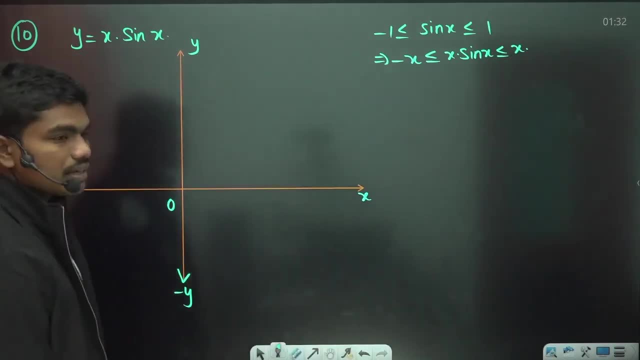 less than or equal to x. so which means one less than or equal to x. so which means one thing is very clear: this x into sine x thing is very clear. this x into sine x thing is very clear. this x into sine x function lies in between the lines y. 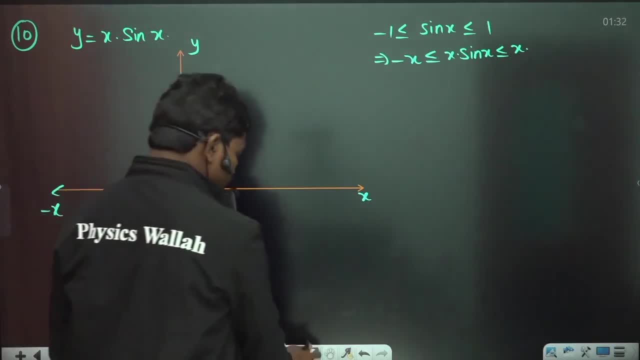 function lies in between the lines: y function lies in between the lines y, equal to minus x, and y is equal to x, so equal to minus x, and y is equal to x, so equal to minus x and y is equal to x. so let us draw them. first of all, y is equal. 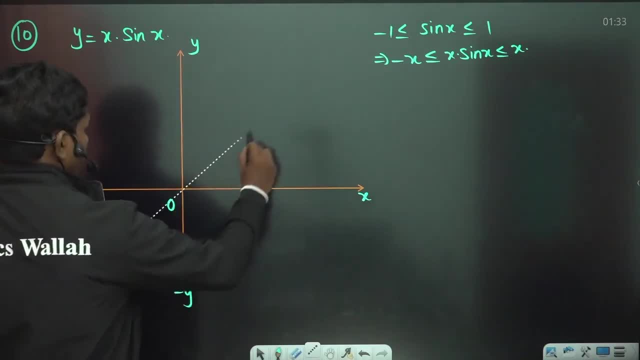 let us draw them first of all. y is equal. let us draw them first of all: y is equal to x. if you draw, y is equal to x to x. if you draw, y is equal to x to x. if you draw y is equal to x, the y is equal to x. function looks. 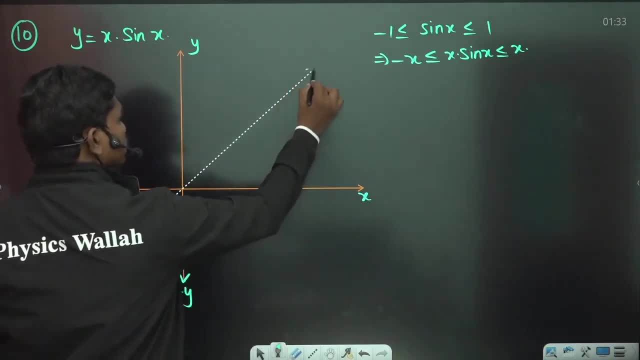 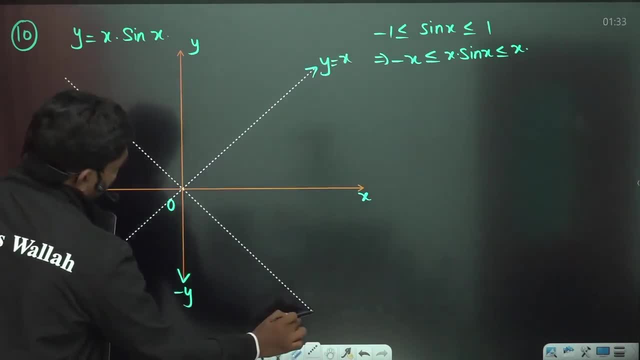 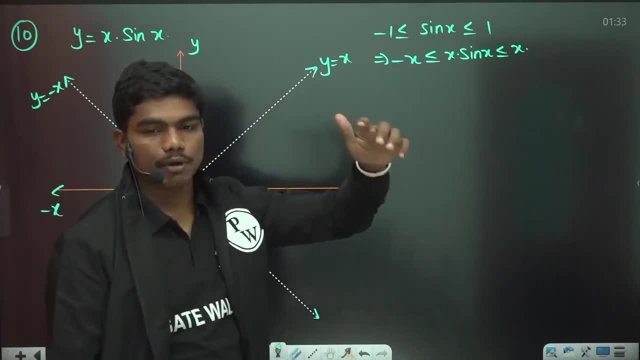 y is equal to minus x. so you can see the y is equal to minus x. so you can see the magnitude of this function is controlled. magnitude of this function is controlled. magnitude of this function is controlled by these two functions, but the shape of by these two functions. but the shape of 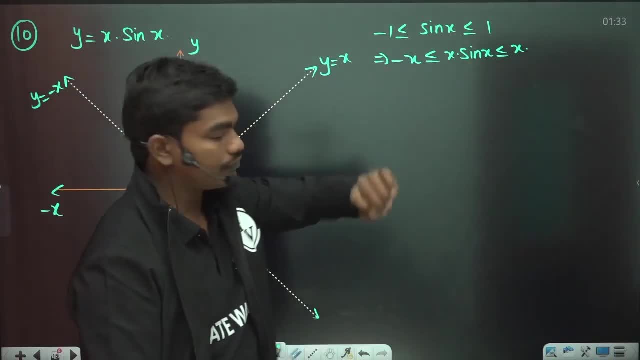 by these two functions. but the shape of this function is actually controlled by this function, is actually controlled by this function, is actually controlled by this. sine x okay means basically, if you this sine x okay means basically, if you this sine x okay means basically, if you see. 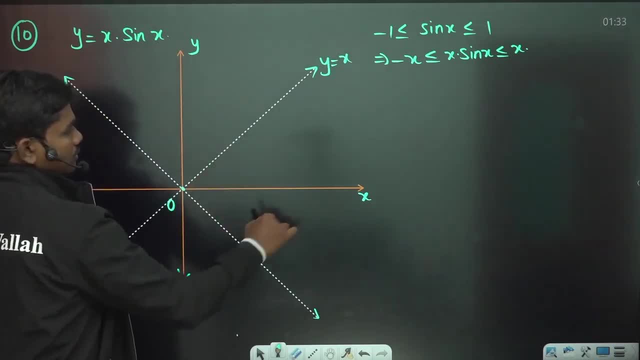 see. see: at x is equal to 0, this function is 0. at x is equal to 0, this function is 0. at x is equal to 0. this function is 0. but after that also the graph is having, but after that also the graph is having. 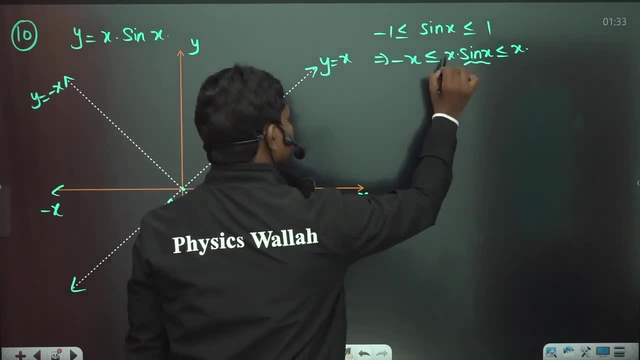 but after that also the graph is having same shape like sine x, because of this same shape like sine x, because of this same shape like sine x, because of this function in multiplication, but the function in multiplication, but the function in multiplication, but the magnitude means basically amplitude of. 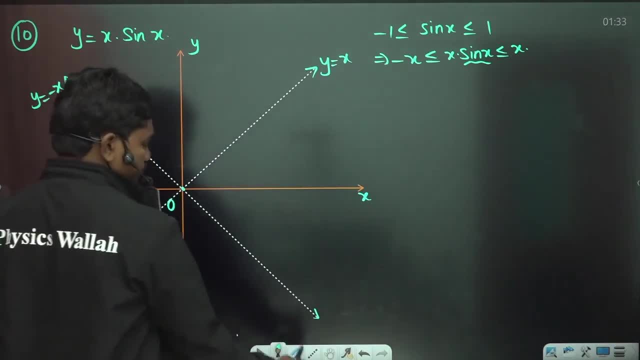 magnitude means basically amplitude of magnitude means basically amplitude of this function will keep on engaging this. this function will keep on engaging this. this function will keep on engaging this is x. so if you see the function means is x. so if you see the function means is x. so if you see the function means, you know, at x is equal to pi. 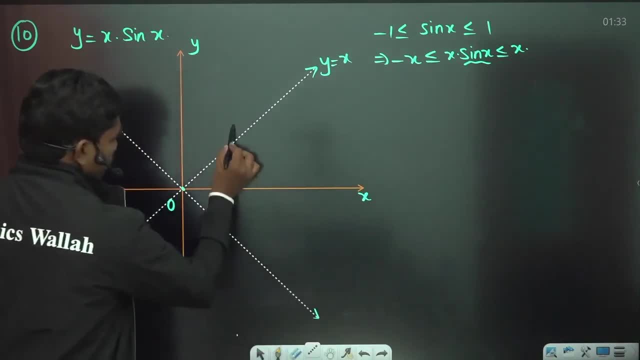 you know at x is equal to pi. you know at x is equal to pi. oh, sorry, at x is equal to oh. sorry, at x is equal to, oh, sorry, at x is equal to pi. okay, at x is equal to pi, for example. pi. okay, at x is equal to pi, for example. 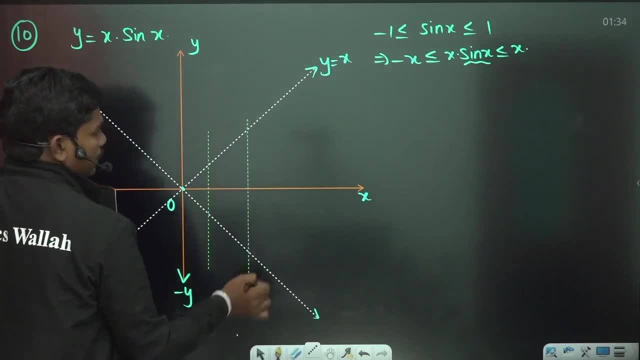 pi, okay, at x is equal to pi. for example, pi is somewhere here at x is equal to 2. pi is somewhere here at x is equal to 2. pi is somewhere here at x is equal to 2 pi. pi pi then at x is equal to 3 pi at all these. 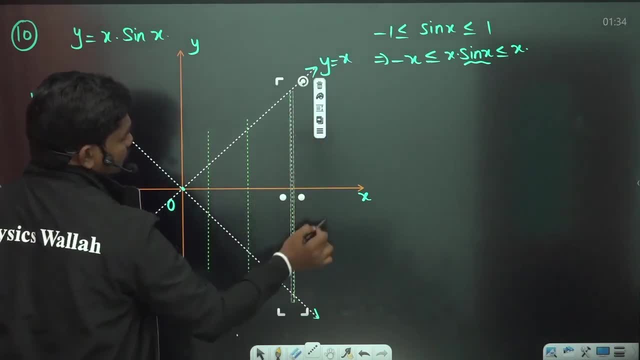 then at x is equal to 3 pi at all these, then at x is equal to 3 pi at all these places, places, places. this function is again going to be zero. this function is again going to be zero. this function is again going to be zero, correct? so, similarly, at x is equal to: 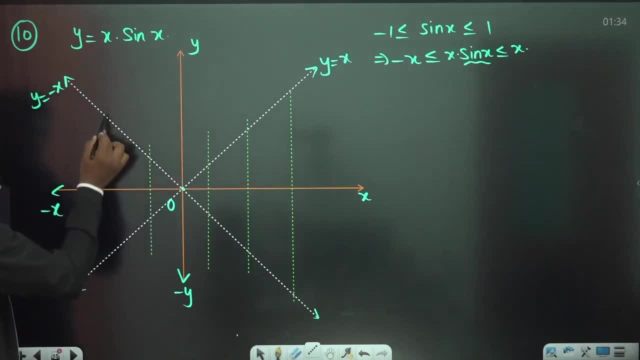 correct. so similarly, at x is equal to correct. so similarly, at x is equal to minus pi. x is equal to minus 2 pi. like this: x is equal to minus 2 pi. like this, x is equal to minus 2 pi like this. so if you see, now you just need to plot. 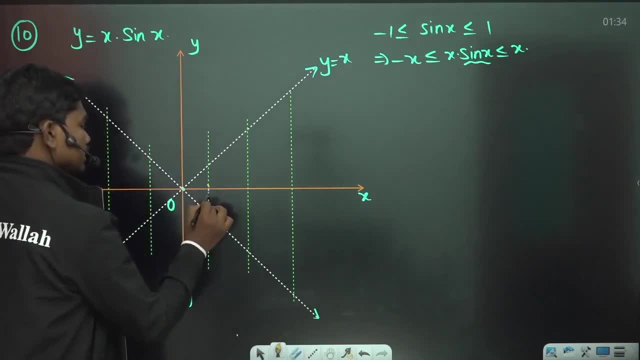 so if you see, now you just need to plot, so if you see, now you just need to plot the graph in between, okay, so the graph in between, okay. so the graph in between, okay. so it starts at zero again at x is equal to. it starts at zero again at x is equal to. 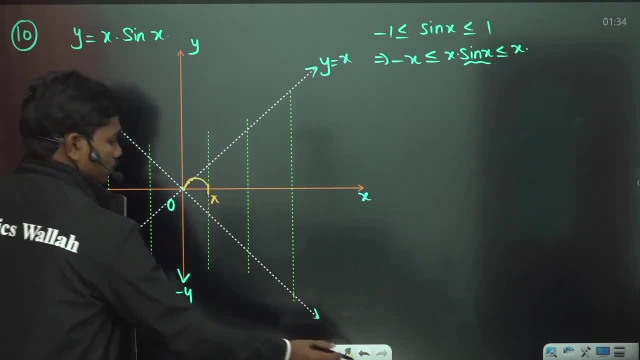 it starts at zero, again at x, is equal to pi. it touches here. so if you see the pi, it touches here. so if you see the pi, it touches here. so if you see the graph comes out, you know graph comes out. you know graph comes out. you know it can't exceed, but it will be almost. 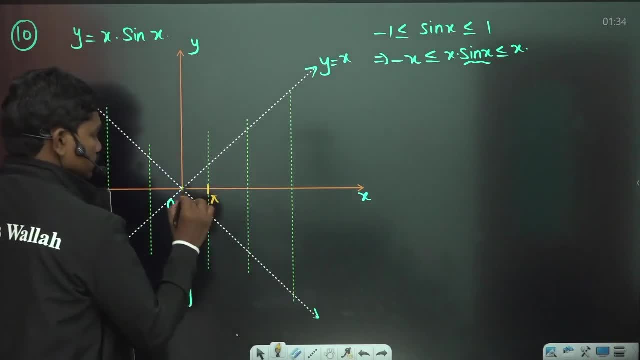 it can't exceed, but it will be almost it can't exceed, but it will be almost the same. okay, so the same. okay, so the same, okay. so this graph will be almost similar to x. this graph will be almost similar to x. this graph will be almost similar to x square graph here. so if you see it comes, 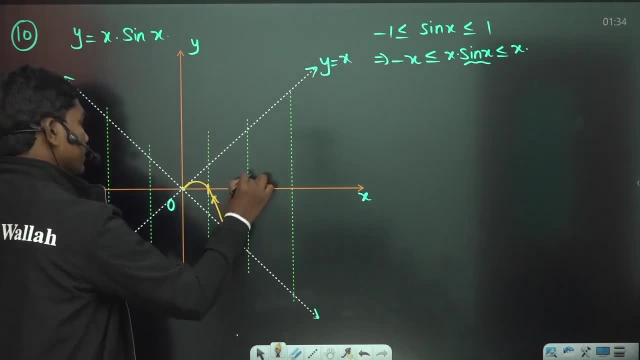 square graph here. so if you see it comes square graph here. so if you see it comes like this, then again it goes like this, then again it goes like this, then again it goes. it comes like this, then again it falls. it comes like this, then again it falls. 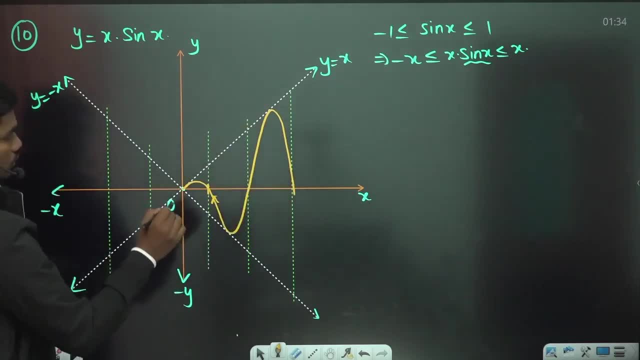 it comes like this, then again it falls like this, and obviously that amplitude like this, and obviously that amplitude like this, and obviously that amplitude keep on increasing similarly here also, keep on increasing similarly here also, keep on increasing similarly here also. if you see, let me, let me. 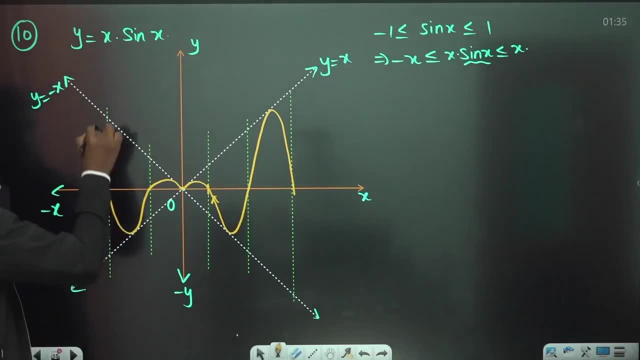 let me, so like this. okay, so it engages basically like this. okay, so it engages basically like this. okay, so it engages basically it is symmetric about. this is pi which i have written. let me, this is pi which i have written. let me, this is pi which i have written. let me draw a different ink. so this is pi. 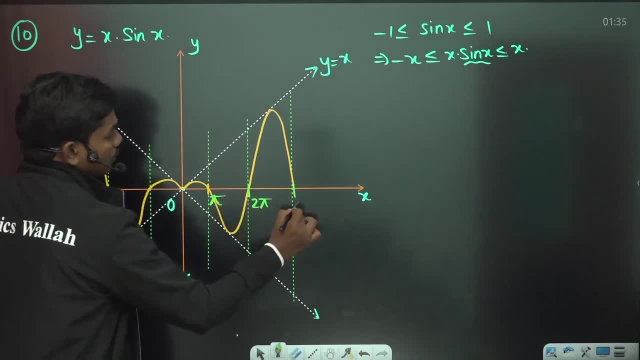 draw a different ink, so this is pi. draw a different ink, so this is pi. actually, this is 2 pi. this is 3 pi. actually, this is 2 pi. this is 3 pi. actually, this is 2 pi. this is 3 pi, and so on. okay, similarly, here, this is: 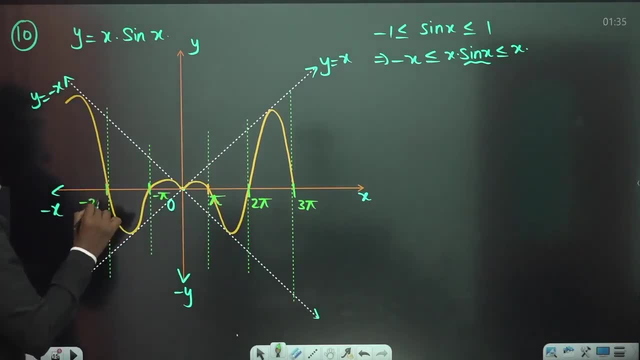 and so on. okay, similarly here this is: and so on. okay, similarly here, this is minus pi, minus pi, minus pi, minus 2 pi, and so on. so if you see this minus 2 pi, and so on, so if you see this minus 2 pi, and so on. so if you see this amplitude keeps on increasing, okay. so if 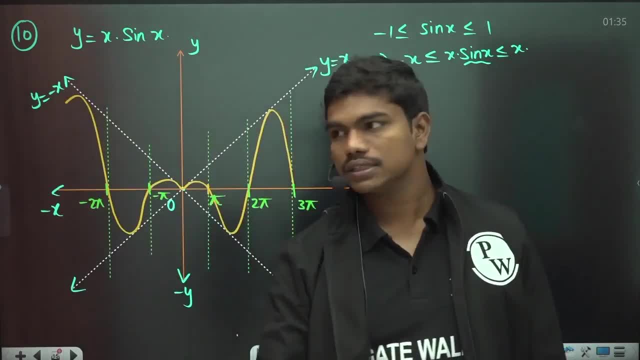 amplitude keeps on increasing, okay. so if amplitude keeps on increasing, okay. so if you see like, for example, under damper, you see like, for example, under damper, you see like, for example, under damper systems, and all in that cases what systems, and all in that cases, what? 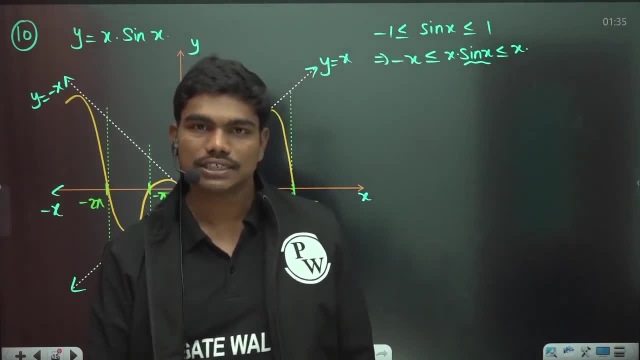 systems and all in that cases, what happens? the amplitude of the vibration happens, the amplitude of the vibration happens. the amplitude of the vibration keep on increasing okay, even in signals. keep on increasing okay, even in signals, keep on increasing okay, even in signals and systems, when noise becomes very high. and systems when noise becomes very high and systems when noise becomes very high, the amplitude of the noise, you know, the amplitude of the noise, you know. the amplitude of the noise, you know, keeps on increasing. so that's how we'll keeps on increasing, so that's how we'll. 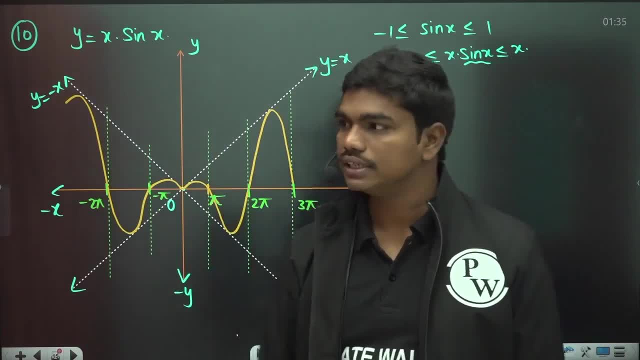 keeps on increasing. so that's how we'll take this function y equal to x into, take this function y equal to x into, take this function y equal to x into sine x. one very important function in sine x, one very important function in sine x, one very important function in general, and of course it don't have any. 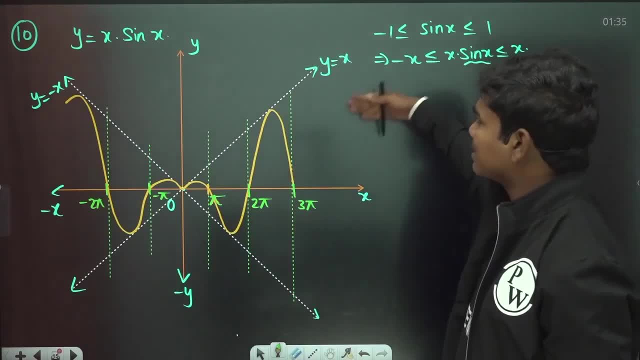 general, and of course it don't have any general and of course it don't have any maximum value. because if you see, as you, maximum value, because if you see, as you, maximum value, because if you see, as you go on it, the amplitude of the function, go on it, the amplitude of the function, 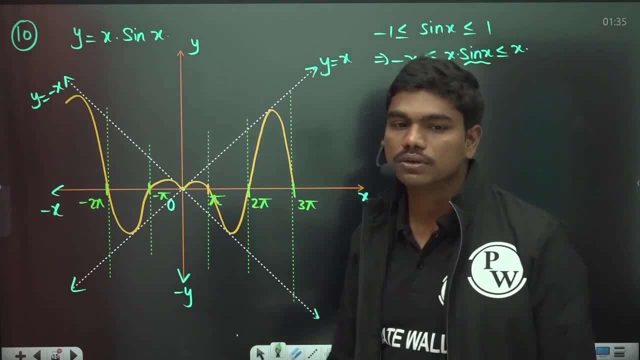 go on it. the amplitude of the function keeps on increasing, okay, so that's why y keeps on increasing. okay, so that's why y keeps on increasing. okay, so that's why y is equal to x into sine X, looks like. is equal to x into sine X, looks like. 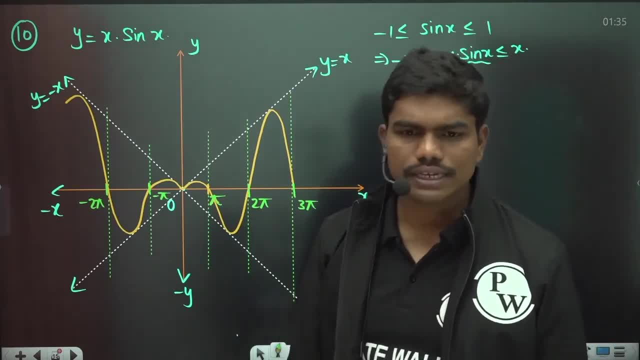 is equal to x into sine X looks like this. okay, here, I would like to give you this. okay here, I would like to give you this. okay, here, I would like to give you one way I say important point or thumb. one way I say important point or thumb. 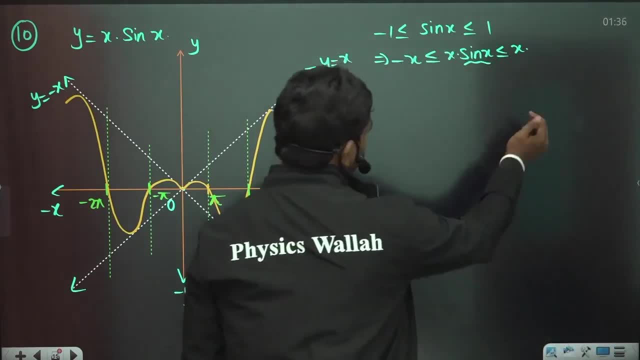 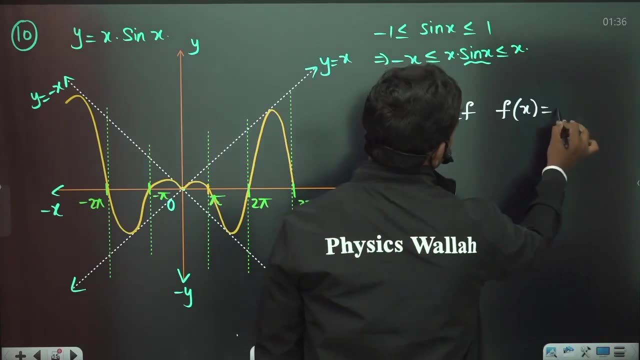 one way I say important point or thumb point, actually that. look, I'll tell you point, actually that. look, I'll tell you point, actually that, look, I'll tell you. if y is equal to, means basically you. if y is equal to, means basically you. if y is equal to, means basically you know, if f of X is equal to minus f, if f 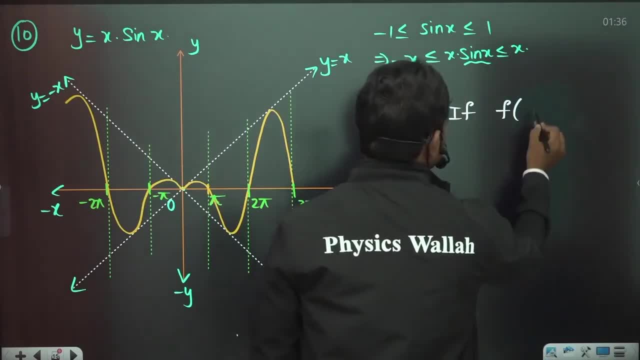 know if f of X is equal to minus f, if f. know if f of X is equal to minus f. if f of X is equal to, or if f of minus X, let of X is equal to, or if f of minus X, let of X is equal to, or if f of minus X, let us say, is equal to f of X. if f of minus. 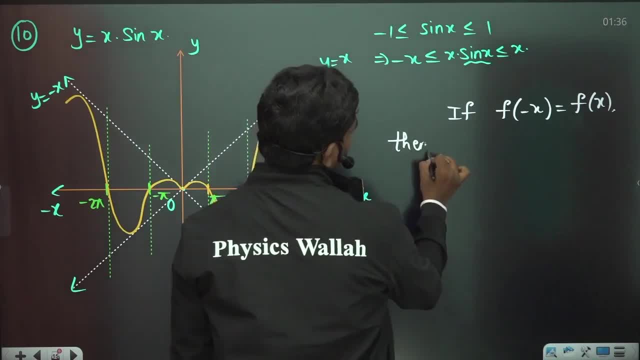 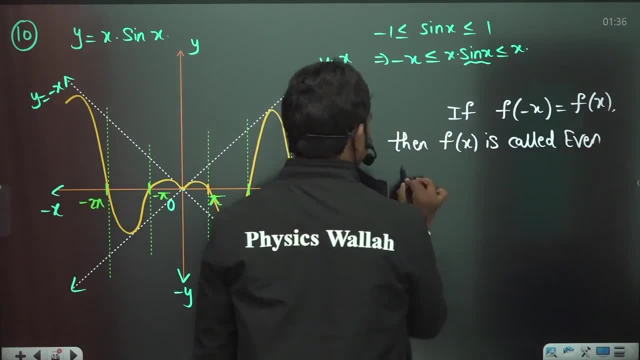 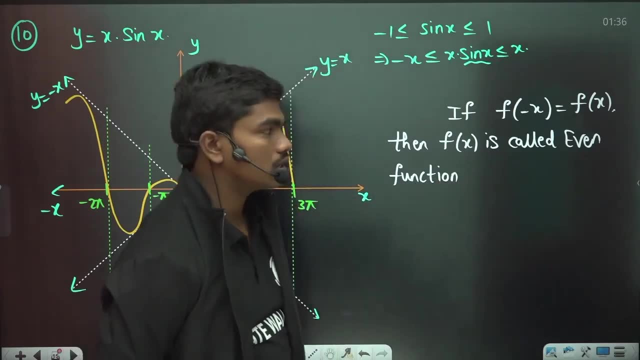 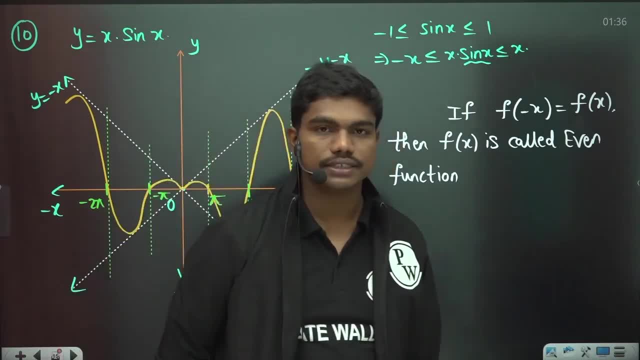 meaning of this even function. look, if you write the series expansion which we, you write the series expansion which we, you write the series expansion which we will see later in Taylor series, after will see later in Taylor series, after will see later in Taylor series after some one hour time. so if you see what 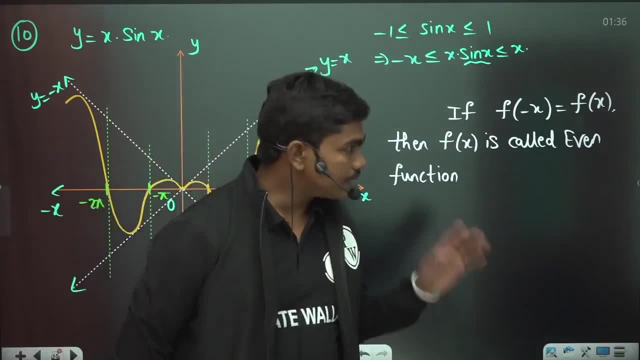 some one hour time. so if you see what, some one hour time. so if you see what, why this is called even function, why this is called even function, why this is called even function, actually, if you write the expansion of, actually, if you write the expansion of, actually, if you write the expansion of this X into sine X, every term will have. 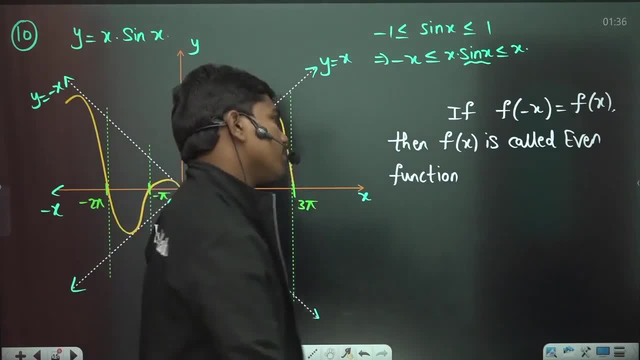 this X into sine X. every term will have this X into sine X. every term will have a even degree. okay, why I will tell you a even degree. okay, why I will tell you a even degree. okay, why I will tell you. look, for example, I am telling you X into. 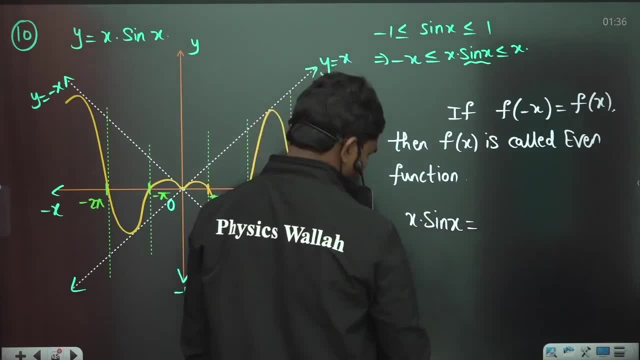 look, for example, I am telling you X into. look, for example, I am telling you X into sine X. is something like this: actually X sine X is something like this: actually X sine X is something like this: actually X into sine X is equal to X times of X. 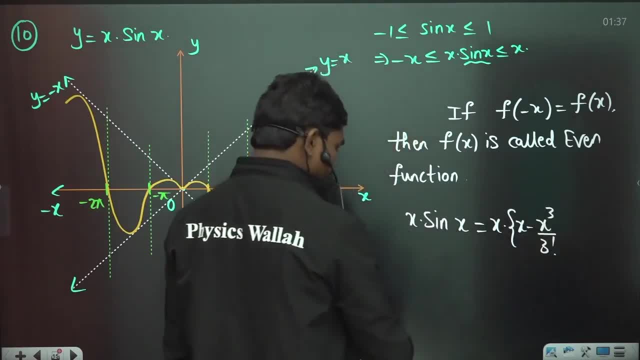 into sine X is equal to X times of X. into sine X is equal to X times of X minus X cubed by 3 factorial. why this minus X cubed by 3 factorial? why this minus X cubed by 3 factorial? why this expression is coming, I will tell you in. 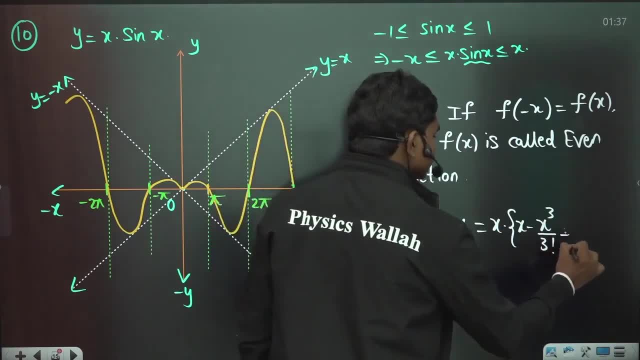 expression is coming, I will tell you in. expression is coming, I will tell you in Taylor series. okay, so, right now, sine X Taylor series. okay, so, right now, sine X Taylor series. okay, so, right now, sine X. expansion: is this X power 5 by 5. expansion: is this X power 5 by 5? 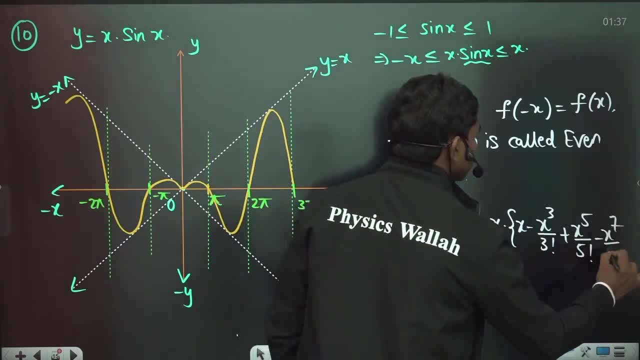 expansion is this: X power 5 by 5 factorial minus X power, 7 by 7 factorial minus X power, 7 by 7 factorial minus X power, 7 by 7 factorial plus, and so on. this goes on till factorial plus, and so on. this goes on till. 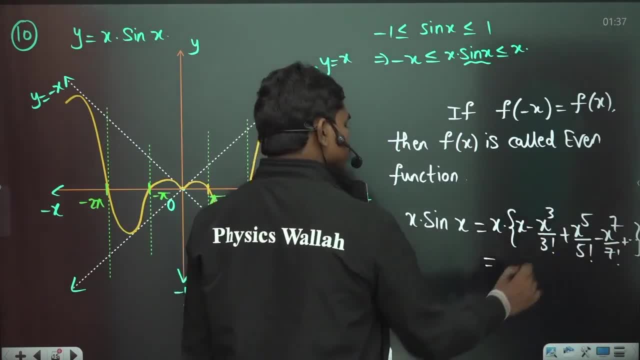 factorial plus and so on. this goes on till infinity. okay. so, if you see when you infinity, okay. so if you see when you infinity, okay. so if you see when you multiply X with all these terms, all these multiply X with all these terms, all these multiply X with all these terms, all these terms will have some even powers, okay. 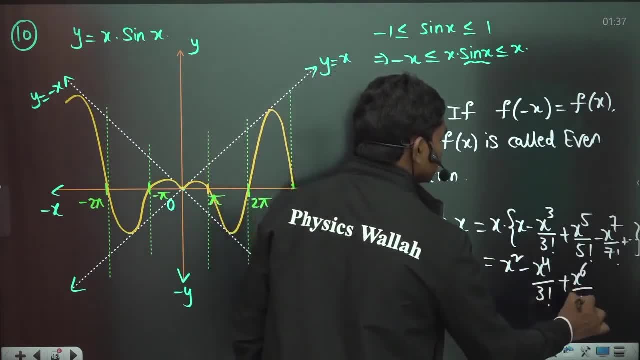 terms will have some even powers. okay, terms will have some even powers, okay. so plus X power 6 by 5 factorial plus, and so plus X power 6 by 5 factorial plus, and so plus X power 6 by 5 factorial plus, and so or minus, you can say minus X power 8. 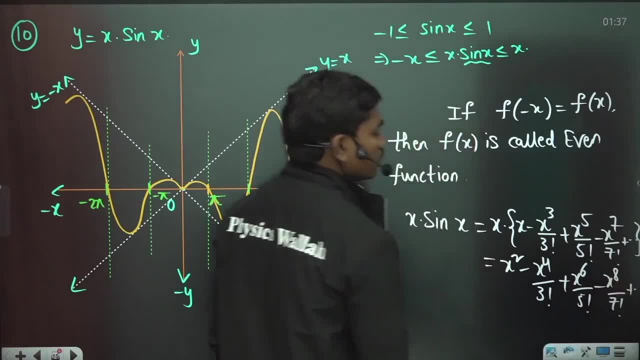 so or minus. you can say minus X power 8 so or minus. you can say minus X power 8 by 7 factorial, and so on. this goes on by 7 factorial, and so on. this goes on by 7 factorial, and so on. this goes on. actually okay, so if you see every term, actually okay. so if you see every term actually okay. so if you see every term have a even power, okay, so that's the have a even power okay. so that's the have a even power okay. so that's the only reason it's called an even function. 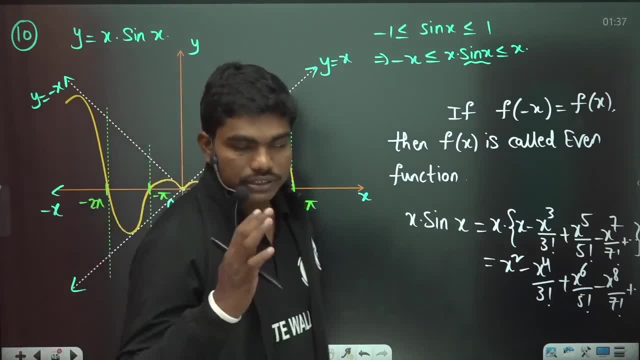 only reason it's called an even function, only reason it's called an even function. and you will observe one thing if this, and you will observe one thing if this, and you will observe one thing if this means: if you plot this, the even means, if you plot this, the even. 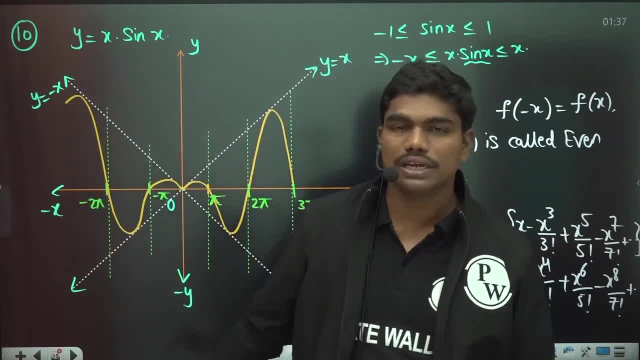 means, if you plot this, the even functions on XY coordinate system, like functions on XY coordinate system, like functions on XY coordinate system like, for example, this function is also a. for example, this function is also a. for example, this function is also a even function. okay, because if I calculate f, 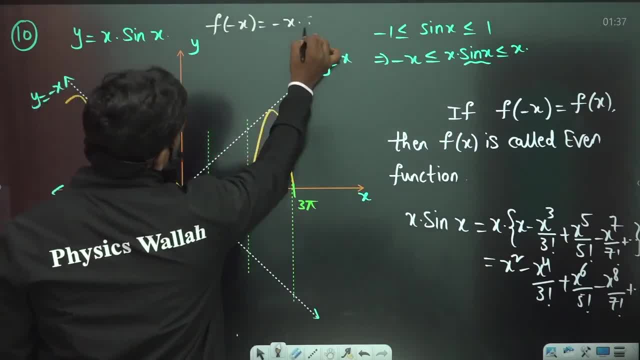 even function. okay, because if I calculate f, even function. okay, because if I calculate f of minus X, this gives me minus X into of minus X, this gives me minus X into of minus X, this gives me minus X into sine of minus X. and you know my sign of. 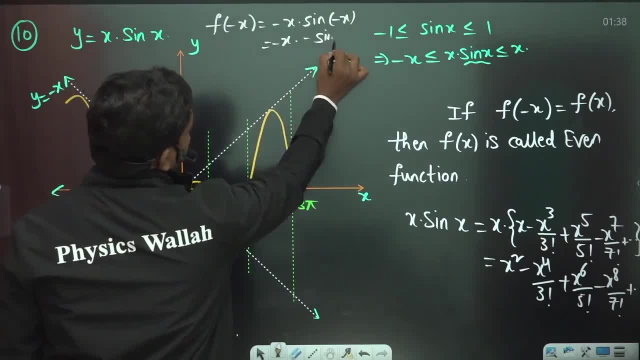 sine of minus X. and you know my sign of sine of minus X and you know my sign of minus X is nothing but minus sine X. so minus X is nothing but minus sine X. so minus X is nothing but minus sine X. so minus X into. minus sine X, so minus into. 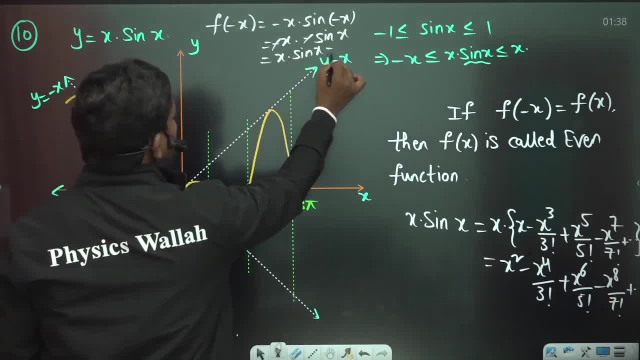 minus X into minus sine X, so minus into minus X into minus sine X, so minus into minus. gets plus again. so this is again minus. gets plus again. so this is again minus. gets plus again. so this is again X into sine X. so if you see, this is same. 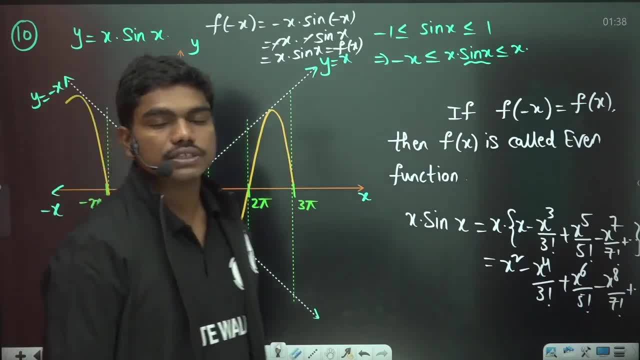 X into sine X. so if you see this is same X into sine X. so if you see this is same as your f of X, okay, so that's why this as your f of X, okay, so that's why this as your f of X, okay. so that's why this function is even function and whenever 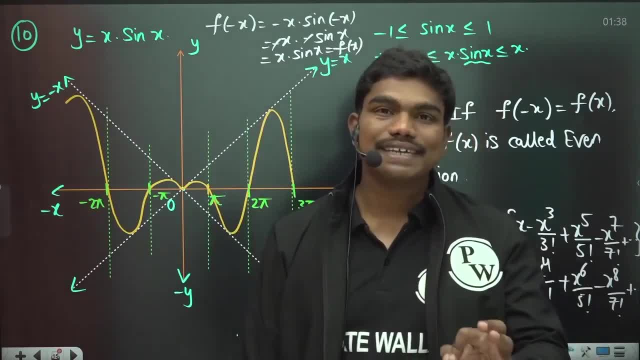 function is even function, and whenever function is even function, and whenever you plot any even function, these, even, you plot any even function. these, even you plot any even function. these even functions are symmetric about y-axis. functions are symmetric about y-axis. functions are symmetric about y-axis. okay, so I'm repeating: whenever you plot, 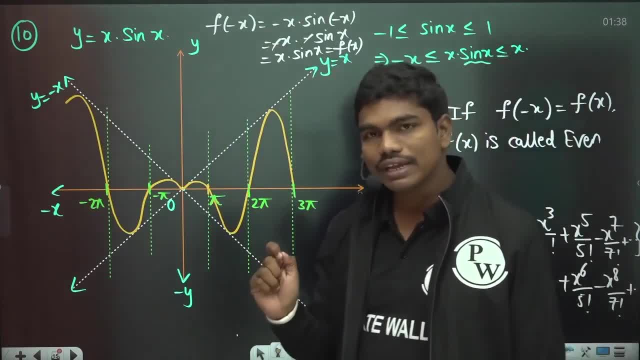 okay, so I'm repeating: whenever you plot: okay, so I'm repeating: whenever you plot about you, whenever you take even about you, whenever you take even about you, whenever you take even functions, the graphs of the even functions, the graphs of the even functions, the graphs of the even functions will be symmetric about y axis. 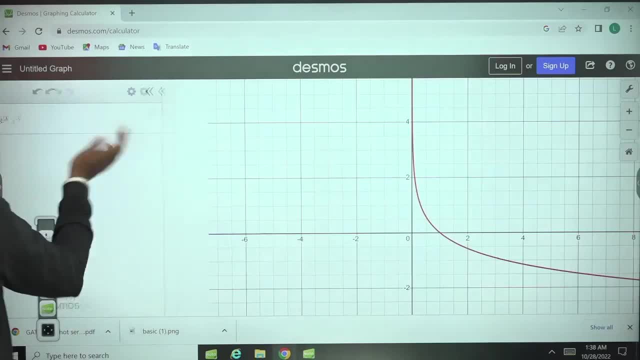 functions will be symmetric about y axis. functions will be symmetric about y axis. okay, so let me show you the actual graph. okay, so, let me show you the actual graph. okay, so let me show you the actual graph. how it looks like. so, anyhow, we have the. how it looks like. so, anyhow, we have the. 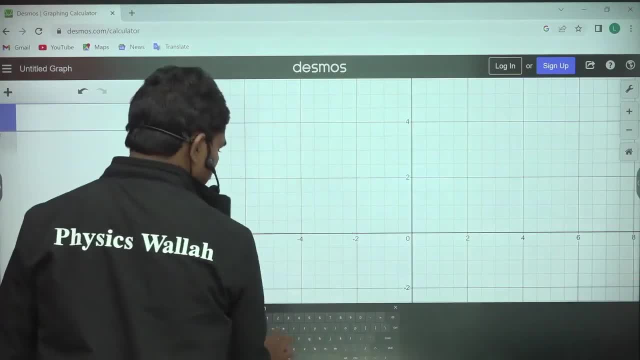 how it looks like. so anyhow, we have the decimals here, so see here: X into sine X. decimals here. so see here: X into sine X. decimals here. so see here: X into sine X. X into. where is this into? yeah, here X. X into. where is this into? yeah, here X. 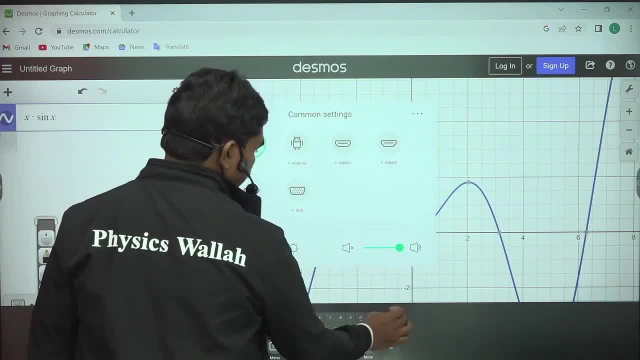 X into. where is this into? yeah here, X into sine X. okay. so if you see the graph into sine X, okay. so if you see the graph into sine X, okay. so if you see the graph is something like this, is something like this, is something like this: 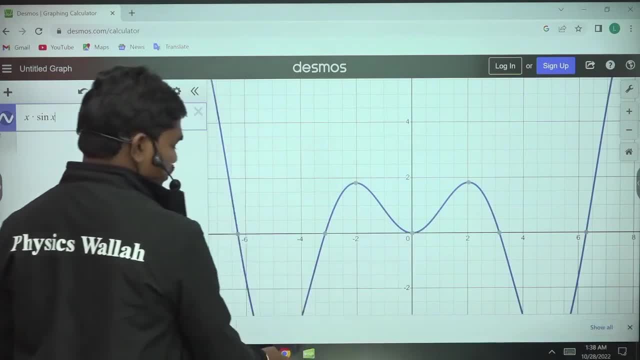 so the graph is something like this: okay, so the graph is something like this: okay, okay, so the graph is something like this: okay, which we have try to draw now, so, if which we have try to draw now, so if which we have try to draw now. so if you see, from 0 they increases again they. 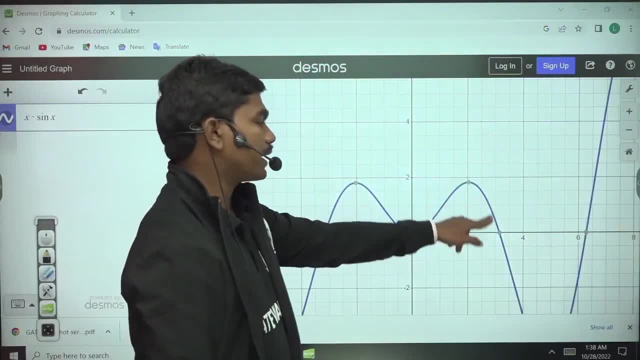 you see, from 0 they increases, again they. you see, from 0 they increases, again they fall and again they go. okay. so from 0 fall and again they go. okay. so from 0 fall and again they go. okay. so from 0 they increases and again they fall. and 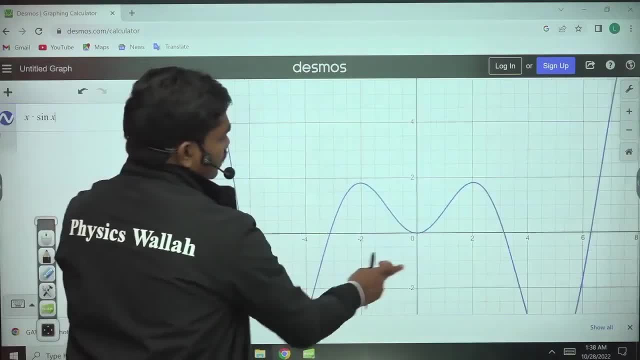 they increases and again they fall, and they increases and again they fall and again they in cases. okay. so this is the again they in cases, okay. so this is the again they in cases, okay. so this is the graph basically, and if you try to saying graph basically, and if you try to saying 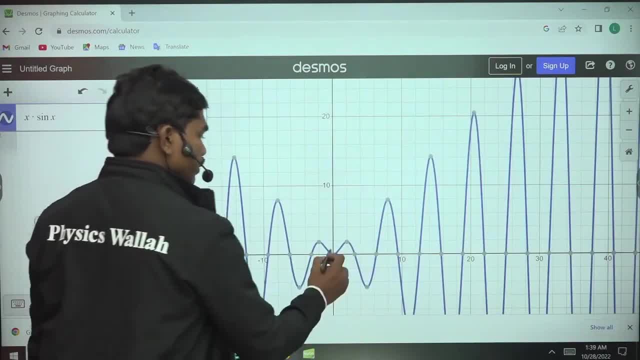 graph, basically, and if you try to saying this, this is how you can see clearly this. this is how you can see clearly this, this is how you can see clearly it's increasing, okay so, and if you it's increasing, okay so, and if you it's increasing, okay so, and if you connect all these points, it is 0 comma 0. 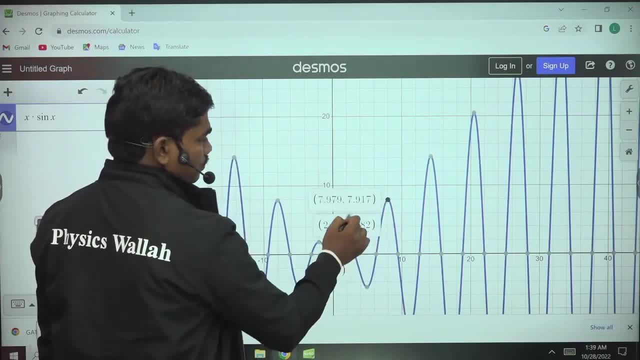 connect all these points. it is 0 comma 0. connect all these points. it is 0 comma 0. this is: you know almost Y is equal to it. this is: you know almost Y is equal to it. this is: you know almost Y is equal to it is controlled by sine X. okay, so all. 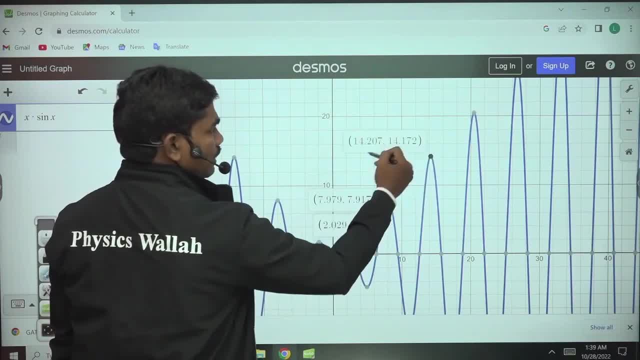 is controlled by sine X. okay. so all is controlled by sine X. okay. so all these points, they have X and Y. these points, they have X and Y. these points, they have X and Y. coordinates equal- okay, all the poles have. coordinates equal, okay, all the poles have. 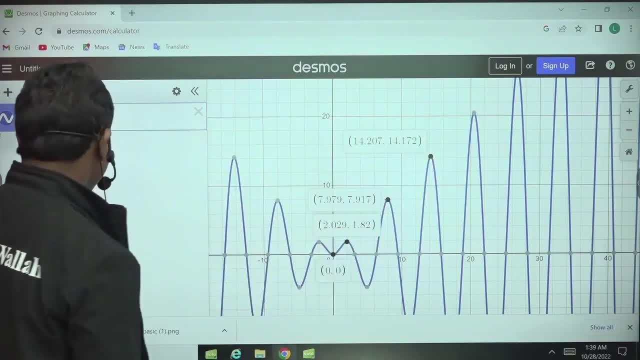 coordinates equal. okay, all the poles have X and Y coordinates almost same. I think X and Y coordinates almost same. I think X and Y coordinates almost same. I think this is rounded off to something. but this is rounded off to something. but this is rounded off to something. but normally, if you see, they are controlled. 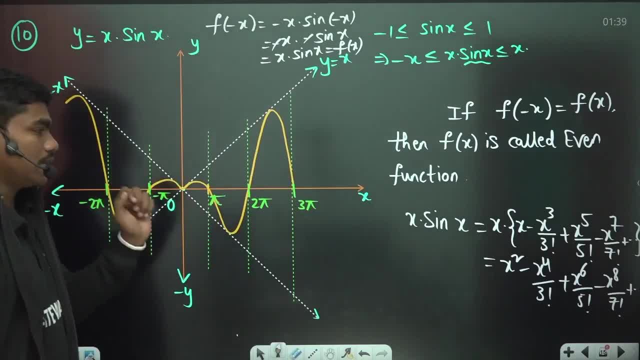 normally, if you see they are controlled normally, if you see they are controlled by this line: Y equal to X and Y is. by this line, Y equal to X and Y is. by this line, Y equal to X and Y is equal to minus X. actually, okay, and this. 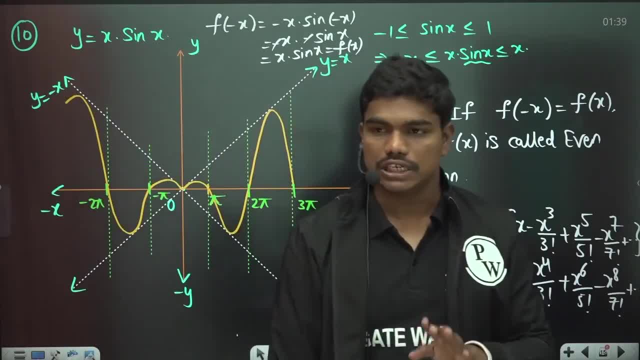 equal to minus X, actually okay. and this equal to minus X, actually okay. and this graph is symmetric about y-axis. because graph is symmetric about y-axis, because graph is symmetric about y-axis, because it is an even function, clear. I hope it's. it is an even function, clear. I hope it's. 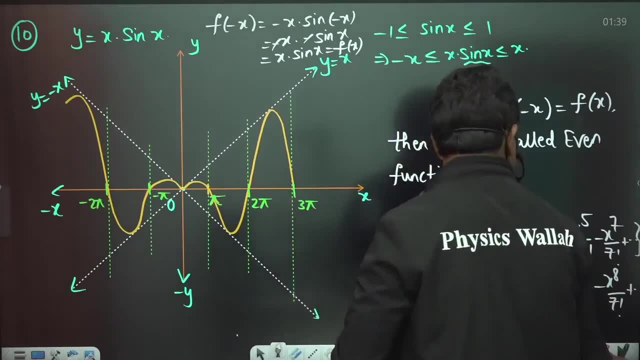 it is an even function. clear, I hope it's clear to you. okay, now, let us go for one. clear to you. okay, now, let us go for one. clear to you. okay, now, let us go for one, last of which is again some important, last of which is again some important. 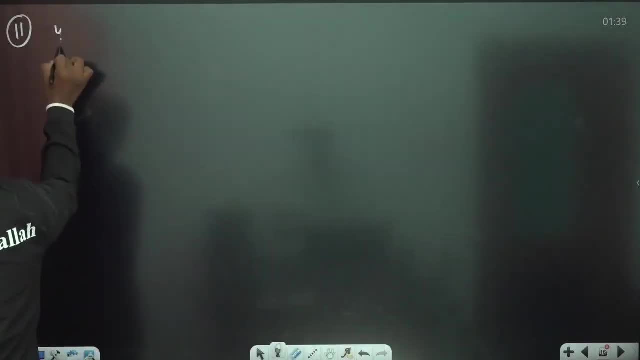 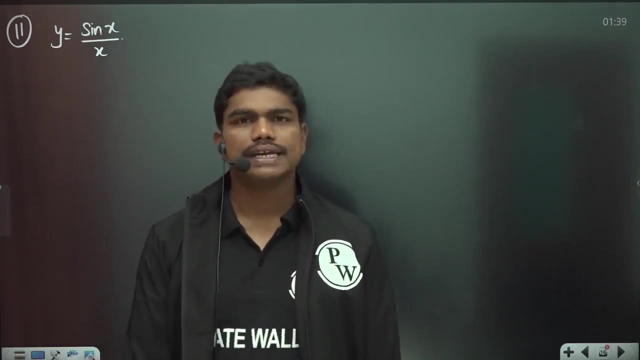 last of which is again some important. graph Y is equal to sine X, Y, X, Y equal to graph. Y is equal to sine X, Y, X. Y equal to graph. Y is equal to sine X, Y, X, Y equal to sine X, Y, X. okay, so Y is equal to sine X by. 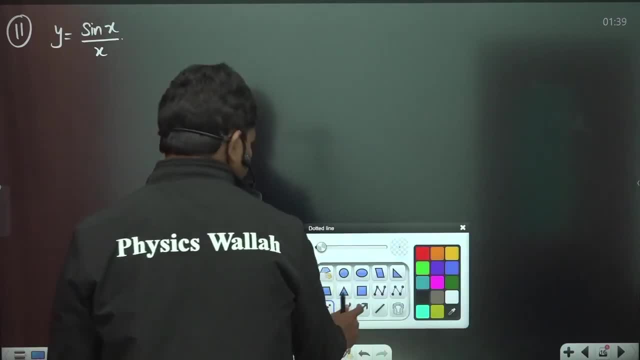 sine X, Y, X. okay, so Y is equal to sine X by sine X, Y X. okay, so Y is equal to sine X by X. if you plot this, this is again one X. if you plot this, this is again one X. if you plot this, this is again one very important graph. if you plot this: 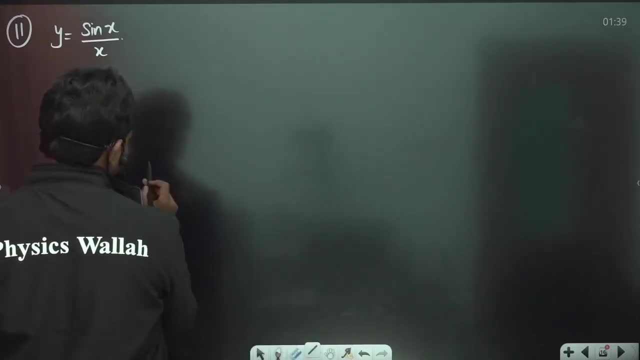 very important graph. if you plot this very important graph, if you plot this, look the graph comes out like this. this look the graph comes out like this. this look the graph comes out like this: this is also even function. so is also even function. so is also even function. so. 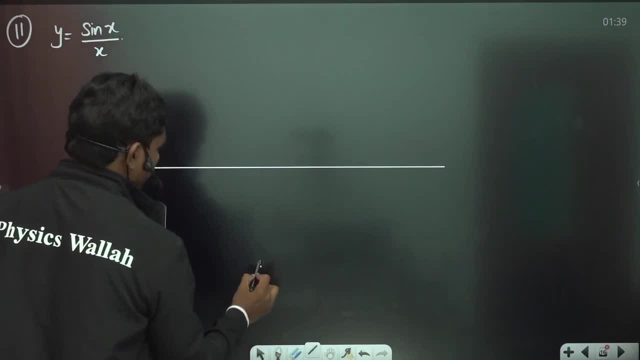 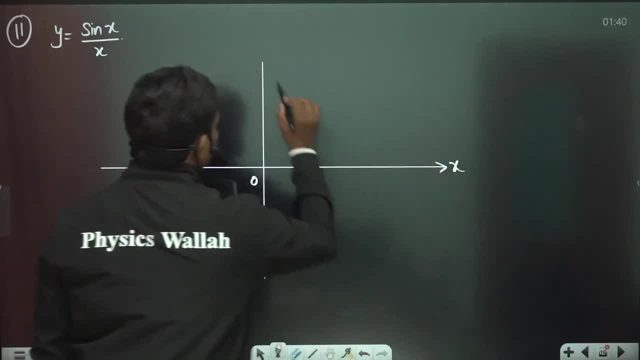 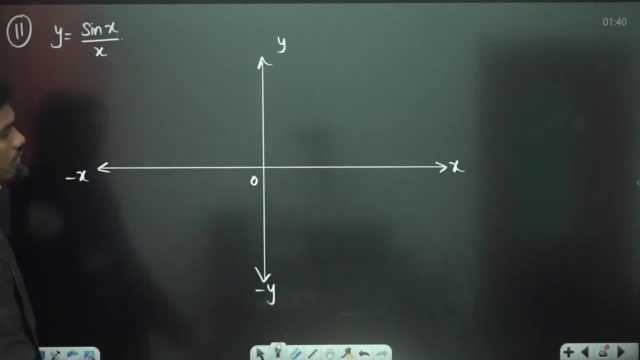 so 0 okay, 0, X okay, 0, X okay, 0 X, Y, Y, Y minus X, minus X, minus X minus Y. now try to understand something minus Y. now try to understand something minus Y. now try to understand something again. you know, minus 1, less than or. 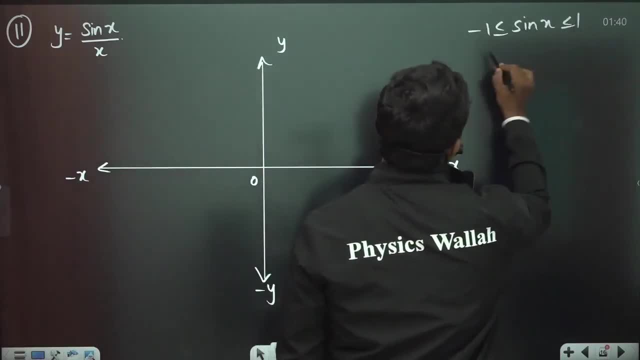 again, you know minus 1, less than. or again you know minus 1, less than or equal to sine X, less than or equal to 1, equal to sine X, less than or equal to 1, equal to sine X, less than or equal to 1. so if you divide with 0, I mean sorry, if 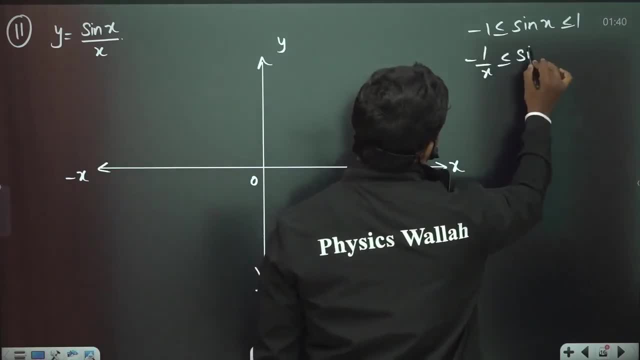 so if you divide with 0, I mean sorry. if so, if you divide with 0, I mean sorry. if you divide with X minus 1 by X less than, or you minus 1 by X less than or equal to sine X by X less than or equal to 1 by. 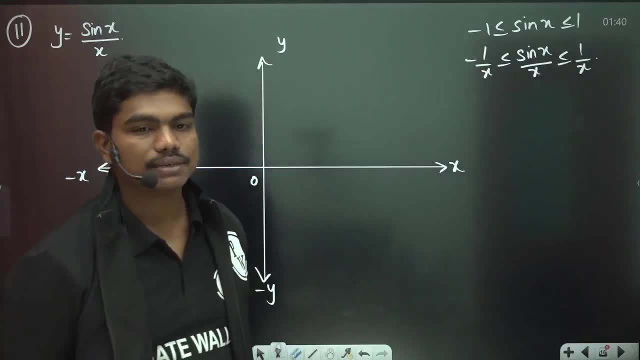 X minus 1 by X, less than or equal to 1 by X, minus 1 by X, less than or equal to 1 by X. okay, so, first of all, you know one X. okay, so, first of all, you know one X. okay, so, first of all, you know one thing: this sine X by X lies in between 1. 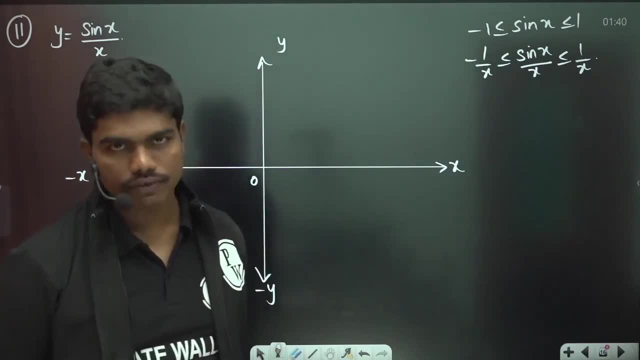 thing. this sine X by X lies in between 1 thing. this sine X by X lies in between 1 by X and minus 1 by X. so how does the by X and minus 1 by X? so how does the by X and minus 1 by X? so how does the graphs of y equal to 1 by X and y equal? 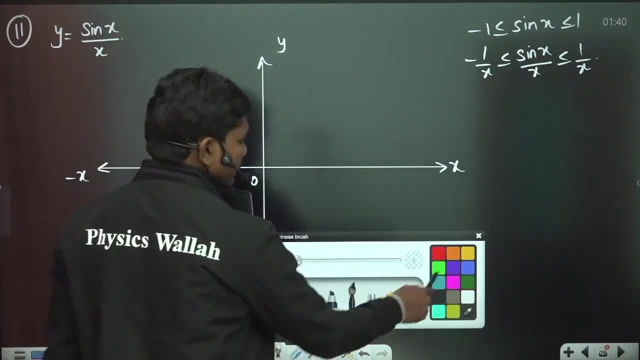 graphs of y equal to 1 by X and y equal. graphs of y equal to 1 by X and y equal to minus 1 by X. look like look y is to minus 1 by X. look like look y is to minus 1 by X. look like look y is equal to 1 by X. will take this form you. 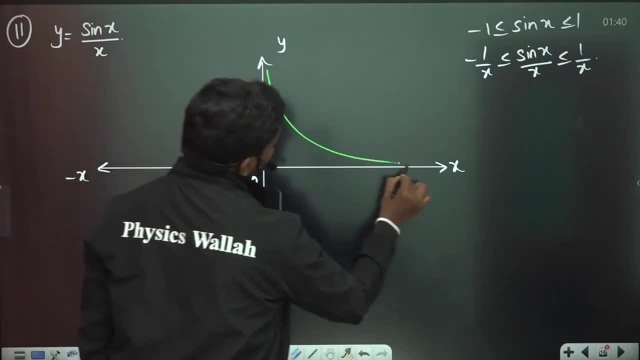 equal to 1 by X, will take this form. you, equal to 1 by X, will take this form. you know rectangular hyperbolas. know rectangular hyperbolas. know rectangular hyperbolas. y is equal to 1 by X. will take this shape. y is equal to 1 by X. will take this shape. 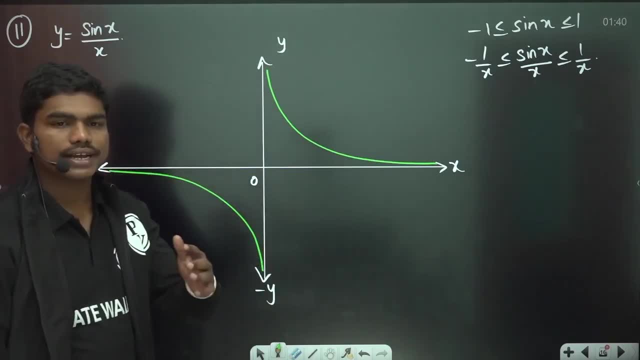 y is equal to 1 by X will take this shape: okay, of course you won't deal with. okay, of course you won't deal with. okay, of course you won't deal with negatives, but many of you in negatives, but many of you in negatives, but many of you in thermodynamics or something in your plus. 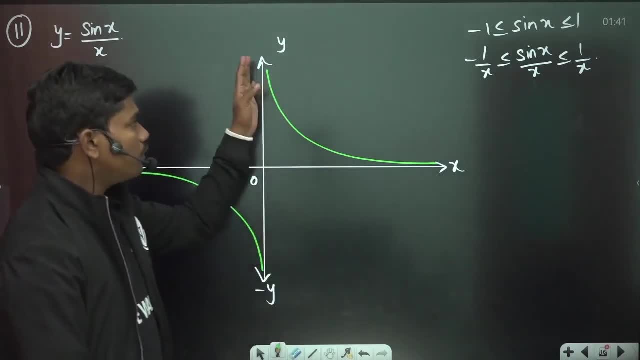 thermodynamics, or something in your plus thermodynamics, or something in your plus one level at least, or in mechanical one level at least, or in mechanical one level at least, or in mechanical. it's quite often so if you plot a PV. it's quite often so if you plot a PV. 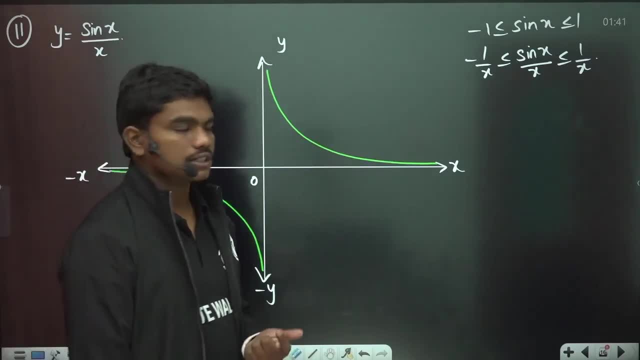 it's quite often so. if you plot a PV diagram for isothermal process, okay so diagram for isothermal process, okay. so diagram for isothermal process, okay. so in isothermal process, you all know this. in isothermal process, you all know this. in isothermal process, you all know this. PV equal to MRT, PV is equal to MRT, so of. 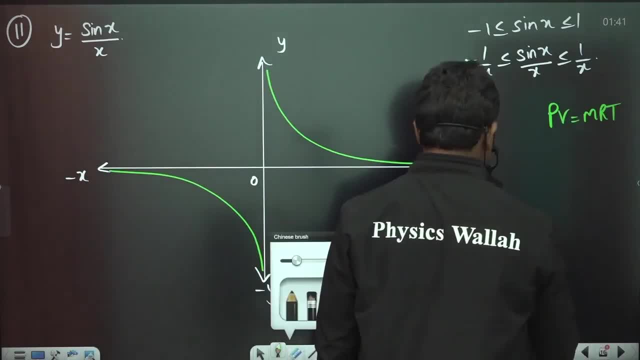 PV equal to MRT, PV is equal to MRT. so of PV equal to MRT, PV is equal to MRT. so, of course, if I close system executing course, if I close system executing course, if I close system executing isothermal process, if you see this term, 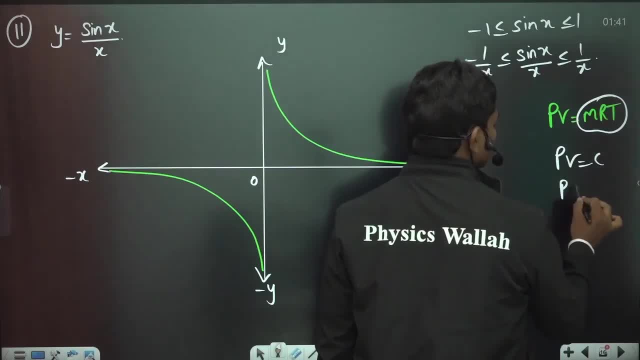 isothermal process, if you see this term, isothermal process, if you see this term is a constant, so PV is equal to some is a constant. so PV is equal to some is a constant, so PV is equal to some constant, so you'll get: pressure is equal. constant, so you'll get: pressure is equal. constant, so you'll get pressure is equal to some constant wave volume. so there to some constant wave volume, so there to some constant wave volume. so there you will have, you will draw a tangler. you will have, you will draw a tangler. 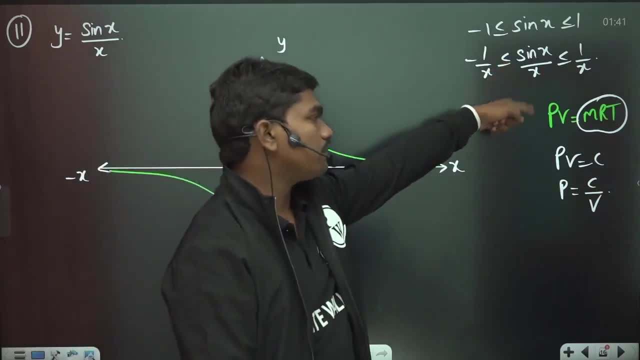 you will have, you will draw a tangler: hyperbolas, actually, because that is hyperbolas, actually, because that is hyperbolas, actually, because that is again same as this function. Y is equal, again same as this function. Y is equal, again same as this function. Y is equal to some 1, by, of course, if I take this Y. 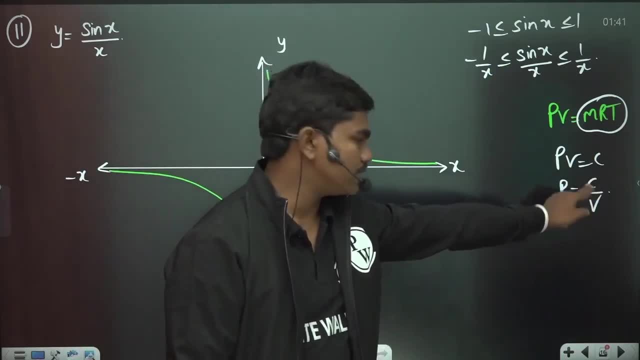 to some: 1 by, of course, if I take this Y to some, 1 by of course. if I take this Y, and if this is X, Y is equal to some, and if this is X, Y is equal to some, and if this is X, Y is equal to some. constant Y, X. okay, this constant value, we. 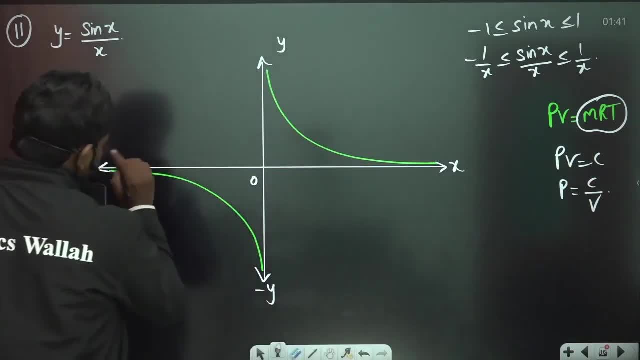 constant Y X. okay, this constant value. we constant Y X. okay, this constant value. we are taking 1 in this case, that's it okay. are taking 1 in this case, that's it okay. are taking 1 in this case, that's it okay. now, similarly, y equal to minus 1 by X. how? 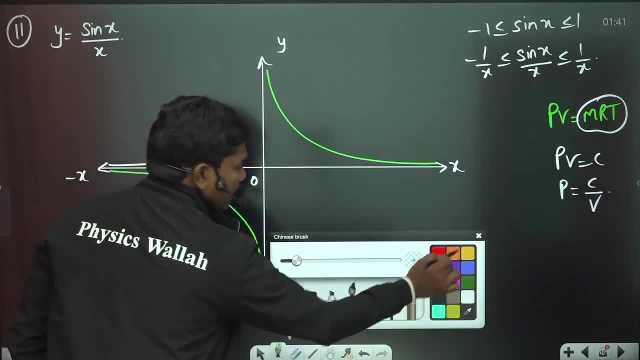 now, similarly, y equal to minus 1 by X. how now, similarly, y equal to minus 1 by X? how does it look like y equal to minus 1? does it look like y equal to minus 1? does it look like y equal to minus 1 by X? y equal to minus 1 by X. look like: 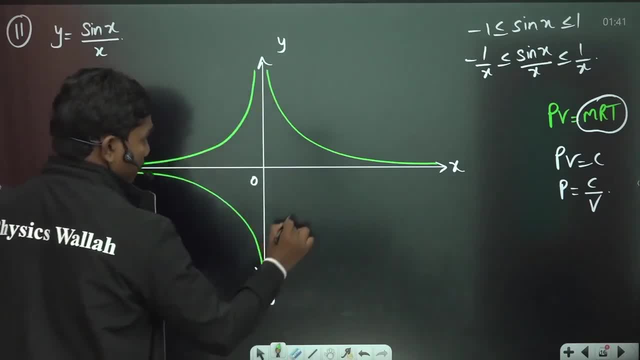 by X: y equal to minus 1 by X. look like by X: y equal to minus 1 by X. look like this: this: this y equal to minus 1 by X. okay now, if you. y equal to minus 1 by X. okay now, if you. 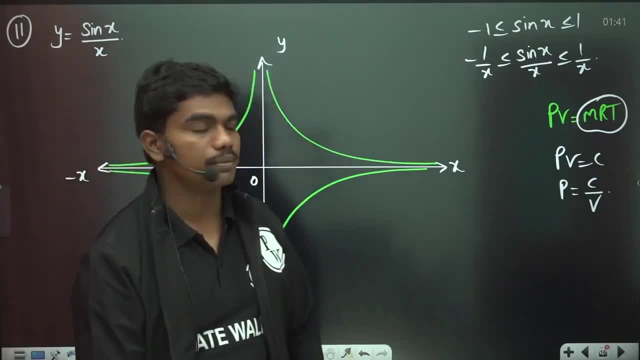 y equal to minus 1 by X. okay, now, if you draw the graph again, is there any? draw the graph again, is there any? draw the graph again. is there any periodicity? yes, there is periodicity periodicity. yes, there is periodicity periodicity. yes, there is periodicity, because at X equal to pi, 2, pi 3, pi all. 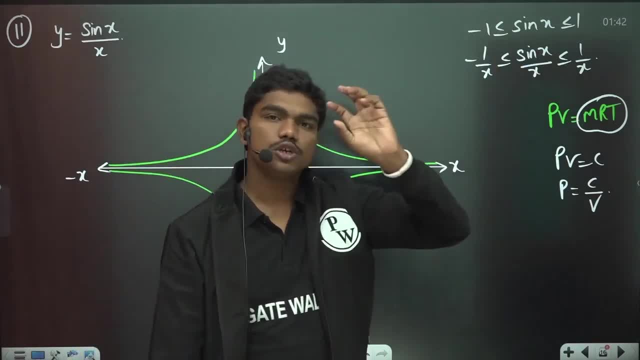 because at X equal to pi 2 pi, 3, pi all. because at X equal to pi 2, pi 3, pi. all these values: this sine X becomes 0 so 0. these values: this sine X becomes 0 so 0. these values: this sine X becomes 0 so 0 by 2 pi 0. 0 by 3 pi 0. okay, so that's how. by 2 pi 0 0, 0 by 3 pi 0. okay, so that's how. by 2 pi 0 0, 0 by 3 pi 0. okay, so that's how. at all the pi multiples, this sine X, at all the pi multiples, this sine X. 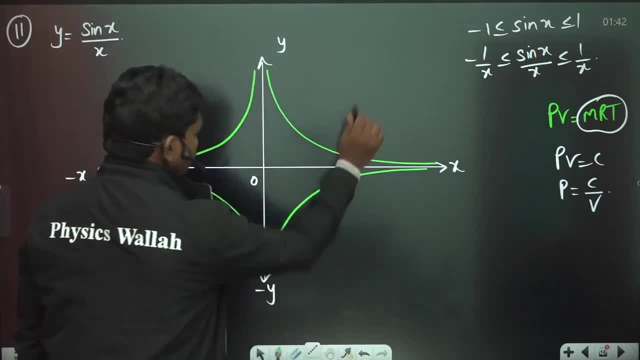 at all. the pi multiples this sine X becomes 0. so if you take some values becomes 0. so if you take some values becomes 0. so if you take some values here pi you can say: for example: then 2, here pi you can say, for example: then 2. 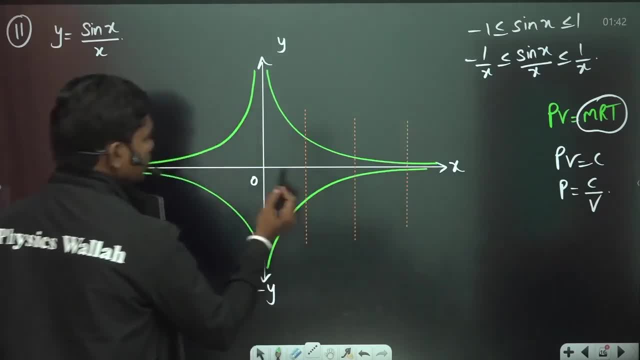 here pi. you can say, for example: then 2 pi, then 3 pi. similarly, if you have minus pi, then 3 pi. similarly, if you have minus pi, then 3 pi. similarly, if you have minus pi, pi, pi minus pi. if you have minus pi minus 2 pi. 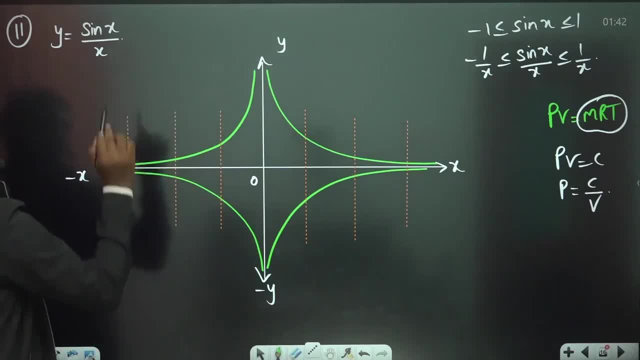 then minus 3 pi. if you have like this, then minus 3 pi. if you have like this, then minus 3 pi. if you have like this, minus 3 pi. so see here: minus 3 pi. so see here: minus 3 pi. so see here 0. 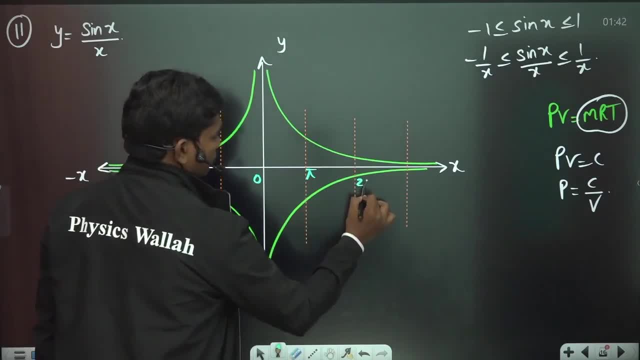 0, 0 by 2 pi, of course 3 pi, and all 0 by 2 pi, of course 3 pi. and all 0 by 2 pi, of course 3 pi. and all similarly minus pi, you can write minus. similarly minus pi, you can write minus. 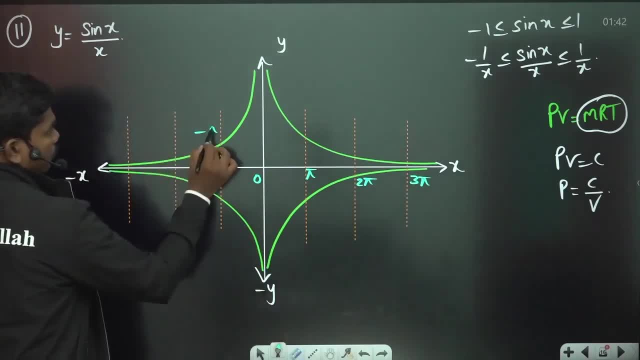 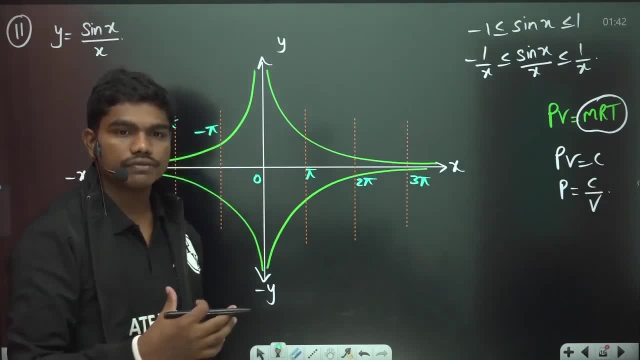 minus 3 pi and all. why I am minus 3 pi and all why I am spending so much time on this graph is spending so much time on this graph is spending so much time on this graph is because they are very much important for. because they are very much important for. 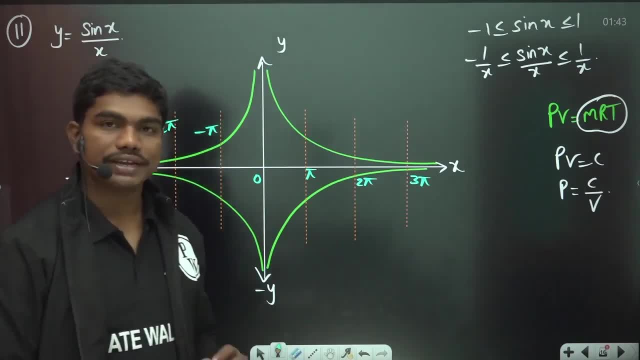 because they are very much important for you in coming topics. okay whenever they you in coming topics. okay whenever they you in coming topics. okay whenever they are talking about area between the curves, are talking about area between the curves, are talking about area between the curves, or double integrals especially, or. 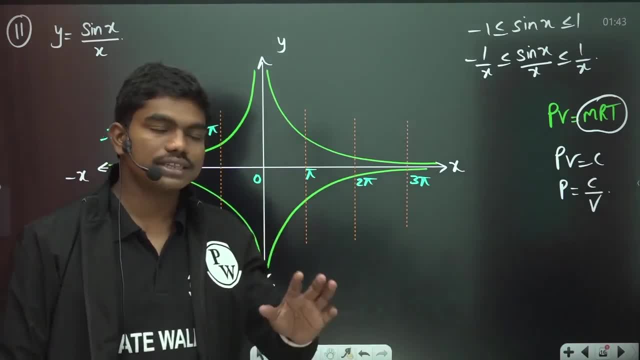 or double integrals especially, or or double integrals especially, or multiple integrals. you can say: when you multiple integrals. you can say when you multiple integrals. you can say: when you are talking about multiple integrals, are talking about multiple integrals, are talking about multiple integrals. plotting these graphs is really important. 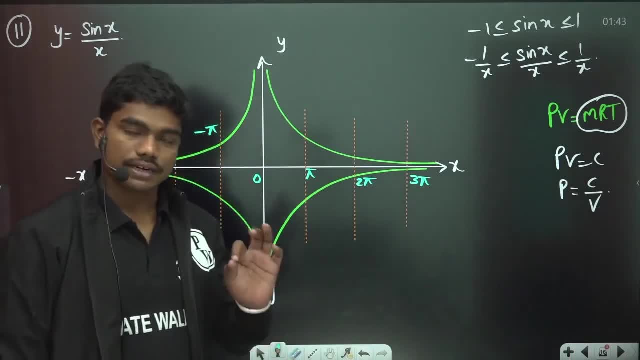 plotting these graphs is really important. plotting these graphs is really important for you, okay? so that's why I'm giving for you, okay, so that's why I'm giving for you, okay, so that's why I'm giving you all this, and also in vector calculus. you all this and also in vector calculus. 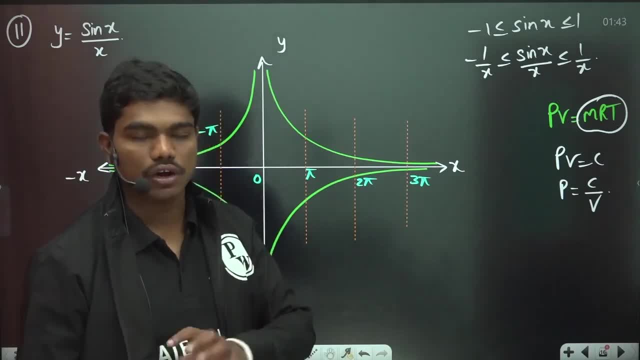 you all this and also in vector calculus, of course, in vector calculus also. when, of course, in vector calculus also, when, of course, in vector calculus also, when you are talking about gain stem and all you are talking about gain stem and all you are talking about gain stem and all you will talk about multiple integrals. 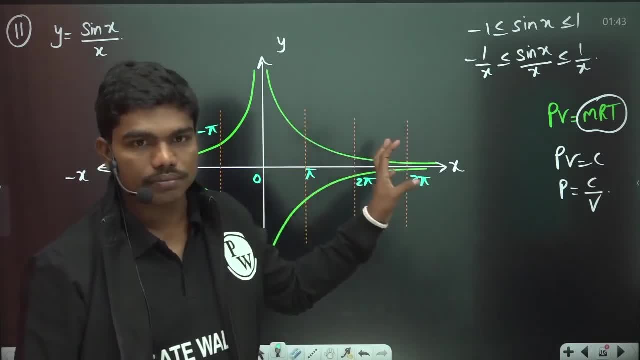 you will talk about multiple integrals. you will talk about multiple integrals and those multiple integrals are very, and those multiple integrals are very and those multiple integrals are very much important. you know, and actually much important. you know, and actually much important. you know, and actually knowing these graphs is very much. 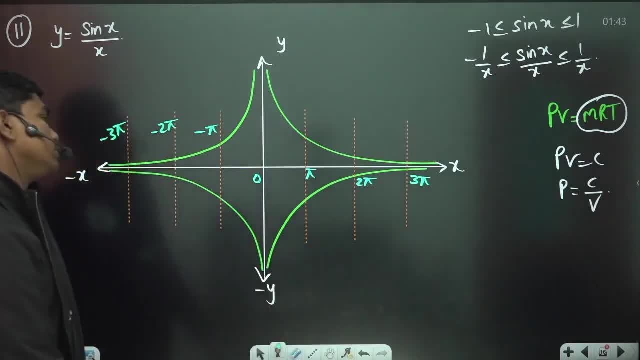 knowing these graphs is very much. knowing these graphs is very much important for you to draw the multiple, important for you to draw the multiple, important for you to draw the multiple. integrals, then okay, so see here. so now I. integrals, then okay, so see here, so now I. 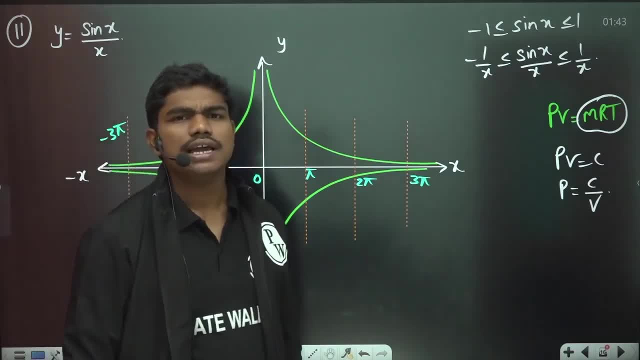 integrals, then okay, so see here. so now I would like to tell one point here. let us would like to tell one point here. let us would like to tell one point here. let us suppose exactly at X is equal to 0. suppose exactly at X is equal to 0. 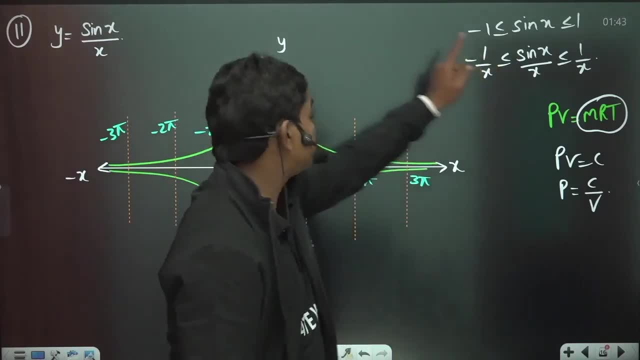 suppose, exactly at X is equal to 0, exactly at X is equal to 0. is this exactly at X is equal to 0, is this exactly at X is equal to 0? is this division possible? means basically: is division possible, means basically: is division possible, means basically: is this function, you know, having any value? 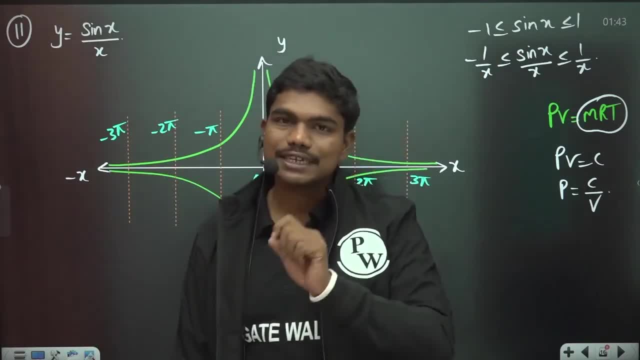 this function you know having any value. this function, you know having any value. you will if you put exact exactly X. you will if you put exact exactly X. you will if you put exact exactly X. equal to 0 sine, 0 by 0, 0 by 0 division is: equal to 0 sine 0 by 0. 0 by 0 division is equal to 0 sine 0 by 0. 0 by 0 division is not defined. so that's why exactly at X, not defined. so that's why exactly at X. 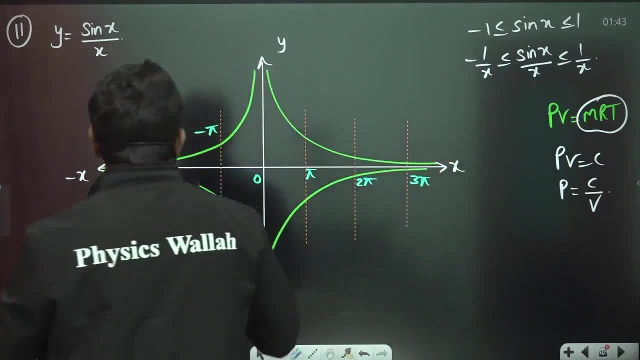 not defined. so that's why, exactly at X equal to 0, you don't have any value here. equal to 0, you don't have any value here. equal to 0, you don't have any value here. okay, but apart from X tends to you know. 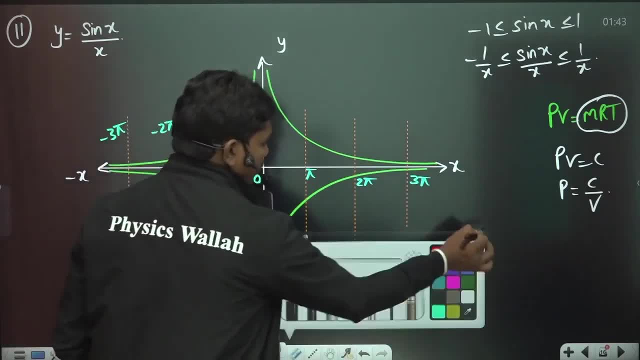 okay, but apart from X tends to you know. okay, but apart from X tends to you know, apart from X is equal to 0, the function apart from X is equal to 0. the function apart from X is equal to 0. the function has a very great shape like this for: 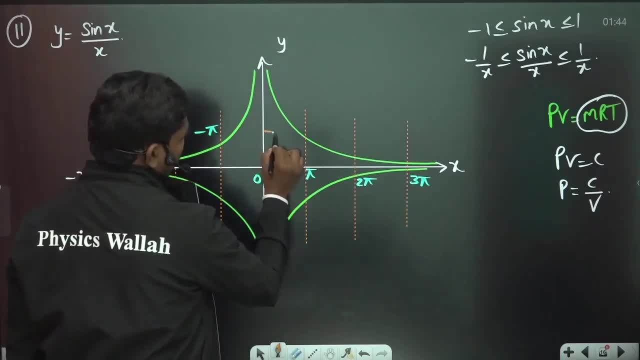 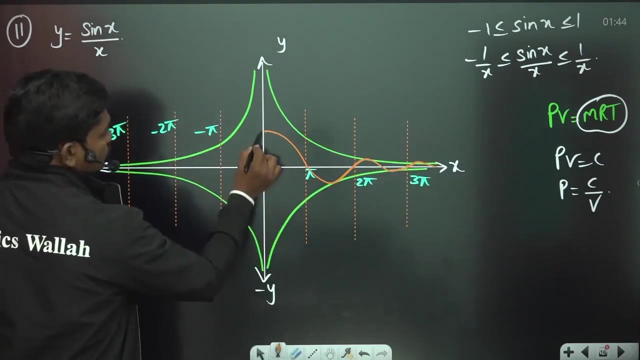 has a very great shape like this, for has a very great shape like this, for example, you can say: it should pass you, it should pass you, it should pass you like this, okay. similarly, if you see: like this, okay. similarly, if you see: like this: okay. similarly, if you see: 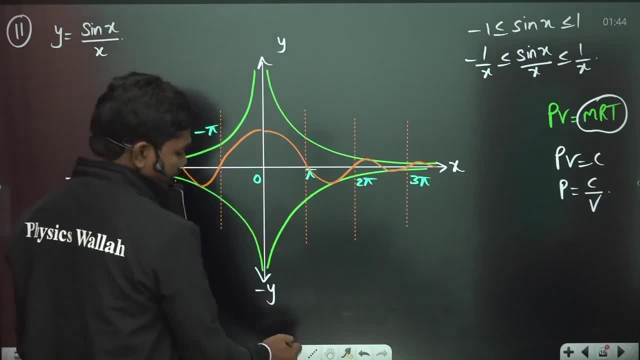 all this it pass okay. now, if you see, intentionally i did not touch this function to y-axis, okay, because exactly at, x is equal to zero. this function has not defined okay, but what is this value means, to which value this function is going, actually, okay, so this value which i'm highlighting here is actually: 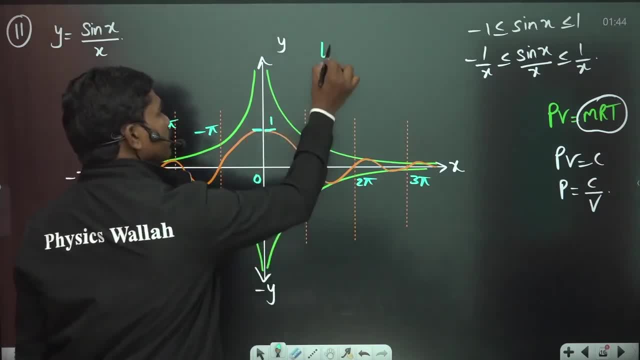 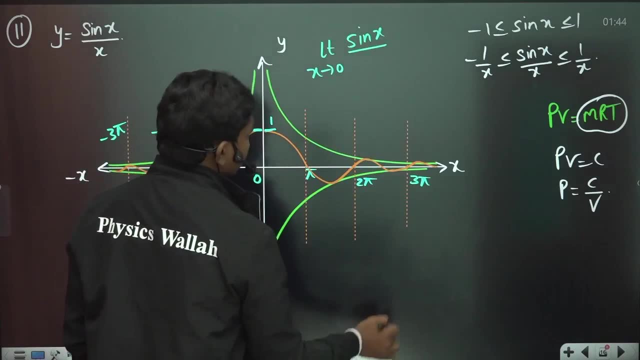 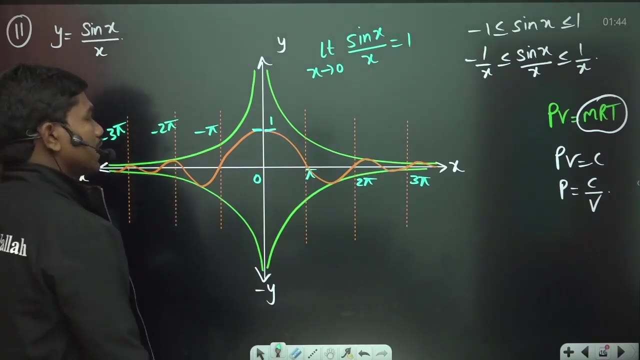 one on y-axis, because you all know one limit limit: x tends to zero, sine x by x, which is one. how this is one, i'll again tell you with the help of taylor series, but right now you believe me. so limit extends to zero sine x by x is equal to one, actually, so that's why you can. 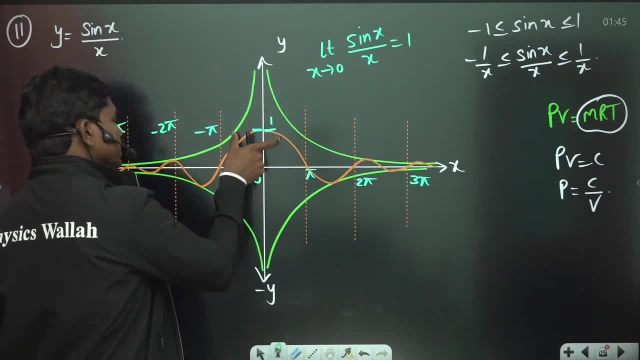 understand one thing: whenever x is coming very close to zero, this function, sine x by x, comes very close to one on y-axis. okay, so that's how i know that this is one here. at this point, i would like to tell you one very important point: what is the maximum value of sine x by x? okay, so maximum. 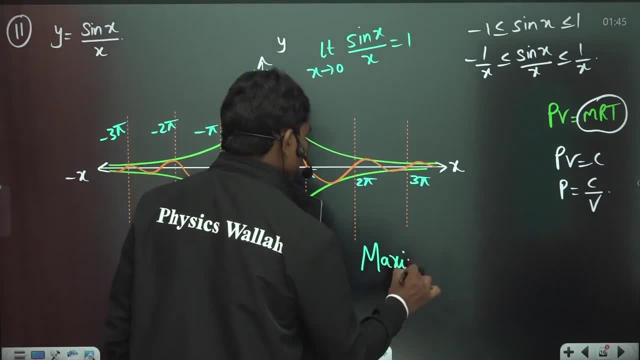 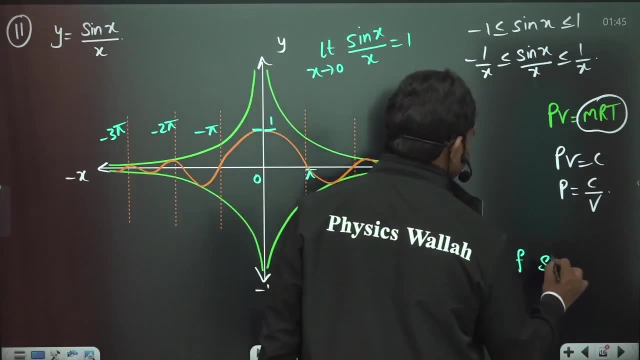 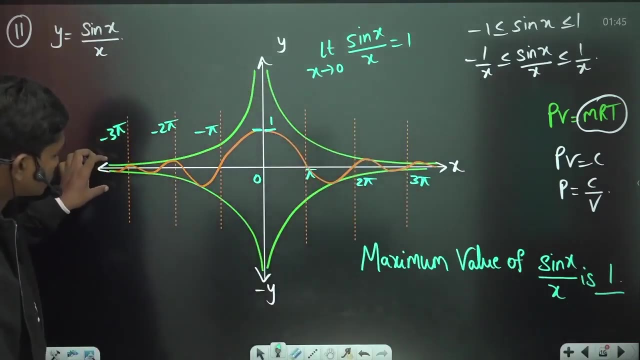 value of sine x by x is one okay, so that's how i know that this is one here. at this point i would: maximum value of sine x by x is one okay, because you can see clearly from the graph that as you go, this graph keep on increasing and this function value keep on increasing. so this is one, and at 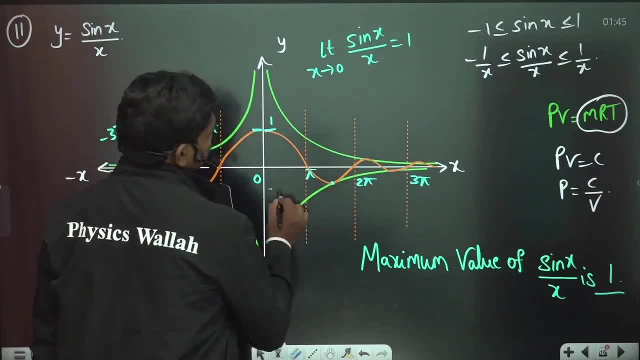 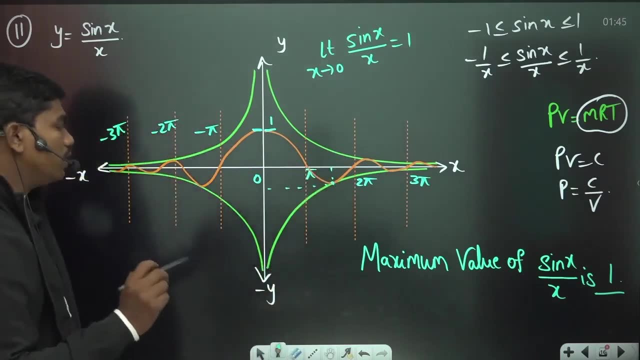 the same time minimum value. if you talk, here comes the minimum value. so this minimum value is basically: at x is equal to three pi by two. okay, so this is one, and at the same time, minimum value at x is equal to three pi by two. this function has the minimum value of y, okay, and actually, if 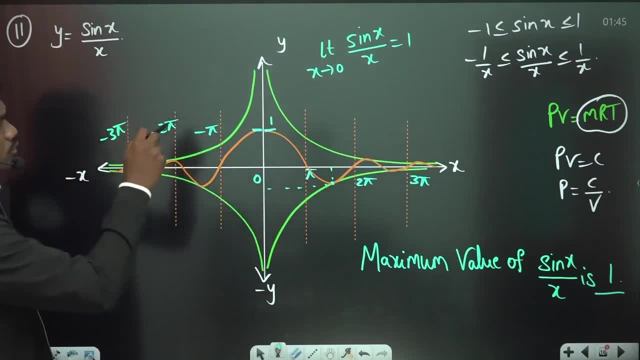 you see, this is uh, sine three pi by two, by three, pi by two. you can write: or: here you can write, basically here: if you, if x is not positive, if they give you x is negative or positive, then this is the value. but if they give you x is only positive, then this is the value. only sign changes. okay. 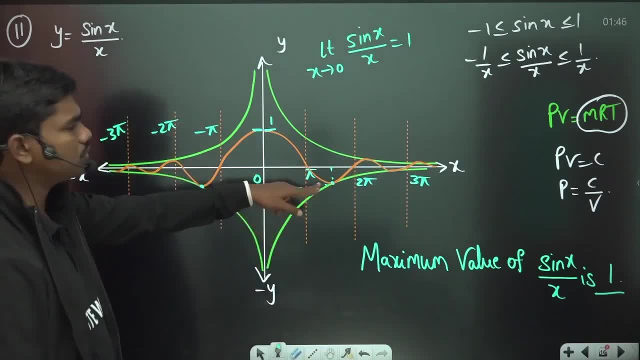 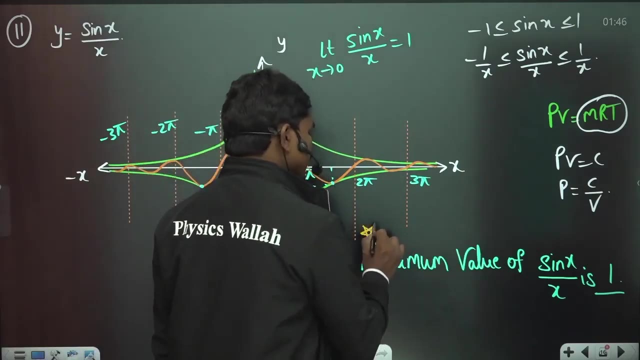 because if you see here, this gives you some positive value. basically, sine three pi by two, divided by three pi by two, that gives you some positive sense actually. but right now, if you see for the whole plane, this is the minimum value. okay, but anyhow, keeping in touch this maximum value, identifying this maximum value, is one very good. 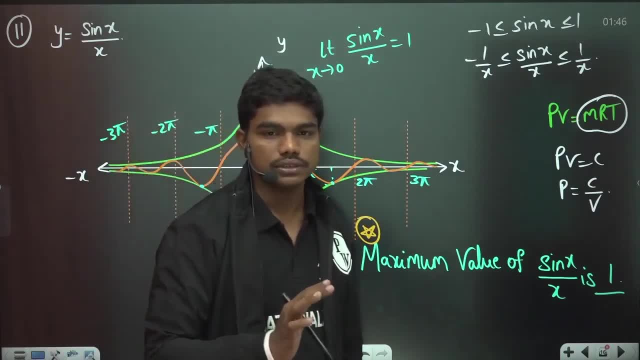 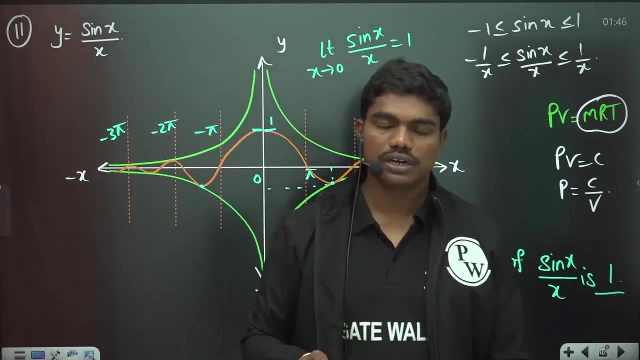 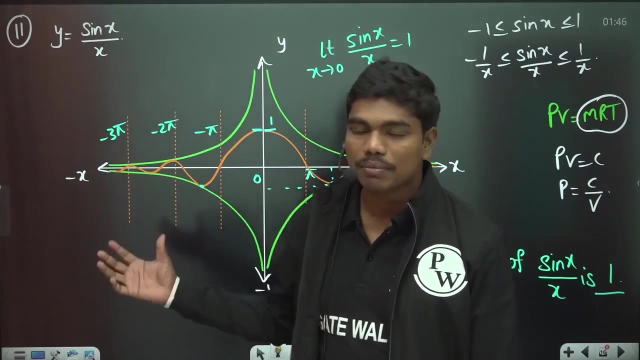 very important thing for sine x by x function clear. so this is where, basically, we finish all the graphs actually. so these graphs are very much important for you to understand in, uh, the real, you know, area under the curve. so some applications: basically, if you talk about applications of differential calculus, then this is the minimum value. okay, so this is the minimum value. 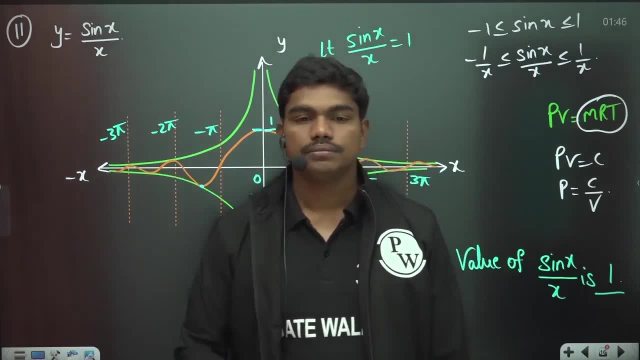 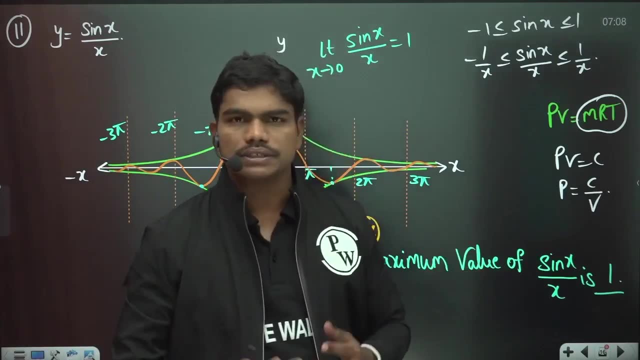 these curves are very important, clear, so so till here we will take part one. we will join the other video. okay, so let us continue. so, basically, we have seen this graph, some standardized graphs actually in calculus, which could help you at the later topics. okay, so now let us talk about. 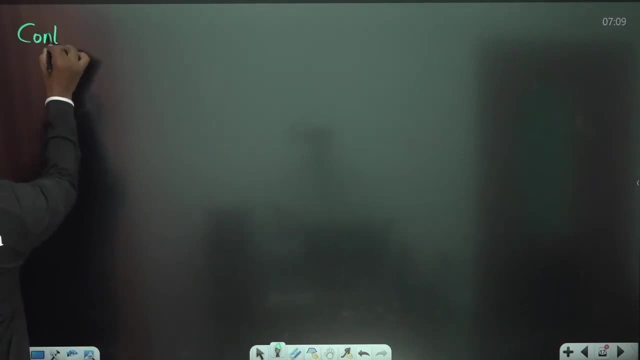 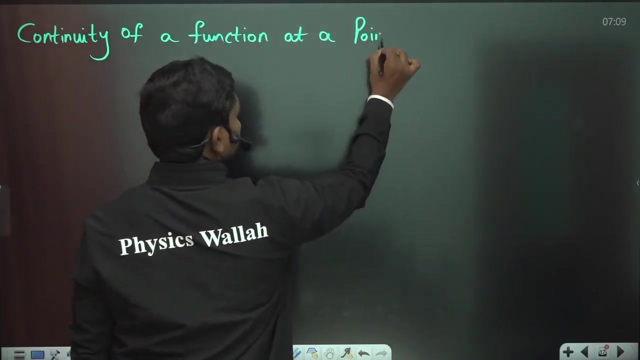 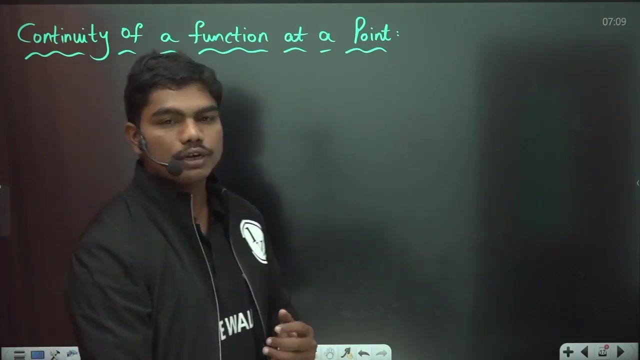 one very important thing, which is continuity of a function at a point. continuity of a function, continuity of a function, continuity of a function at a point, at a point. so what is continuity of a function at a point? so basically, from the meaning of continuity, you mean to say that the function don't have any break. actually, at 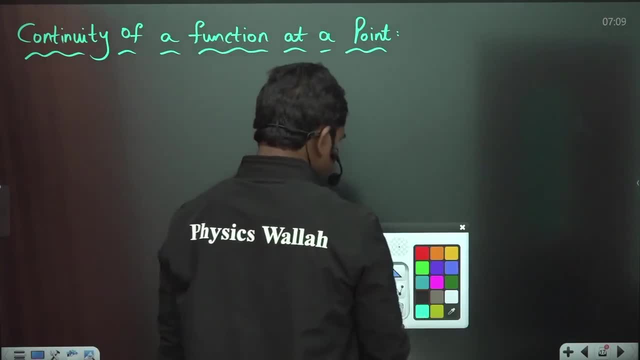 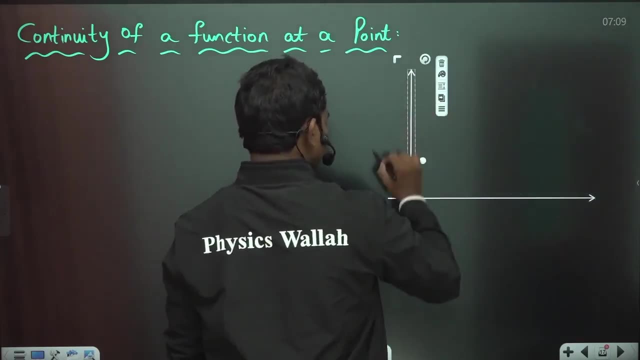 any point. okay means, let us suppose, if you take a function, for example, say something like this: if this is your x-axis and if this is your y-axis, for example, let us say then, if this is your horizon, x, y, which is basically some function of x. so 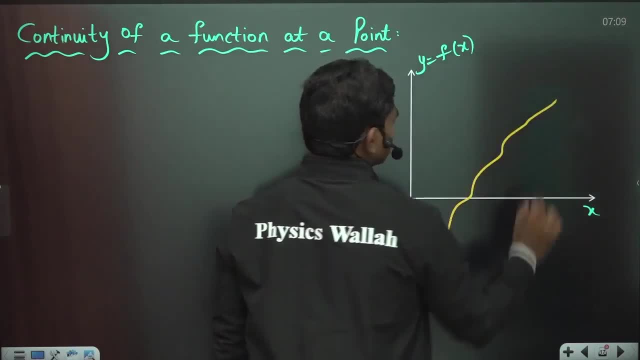 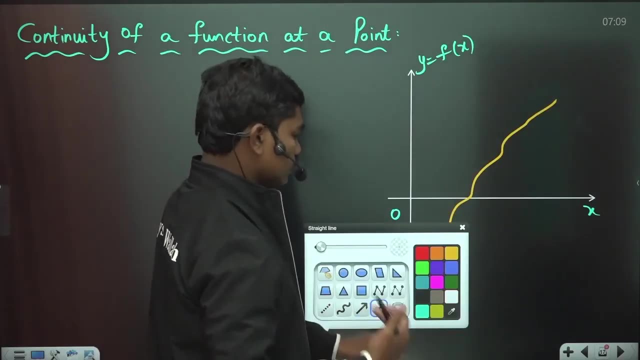 if you see, if I draw a function, this function has to be continuous like this: okay, there should not be any breaking in between. then we say that the function is continuous And of course, limit continuity. all these are talked at a particular point. So if you take, for example, x is equal to 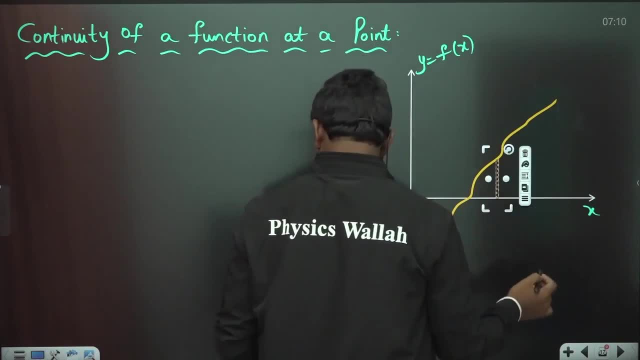 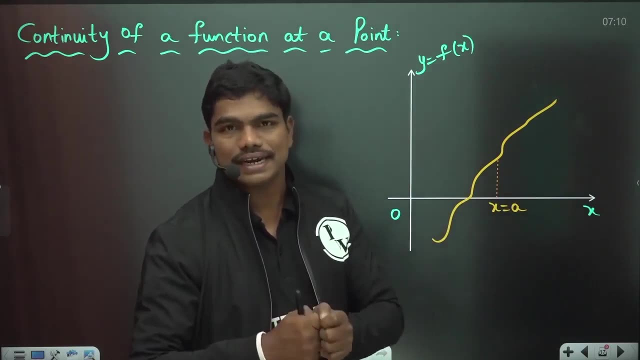 a. something like this: x is equal to a, x is equal to a, then that x is equal to a. if the function has to be continuous, the function should not break at x is equal to a, basically okay. So, mathematically, how do we check whether the function is actually continuous or not? Okay, 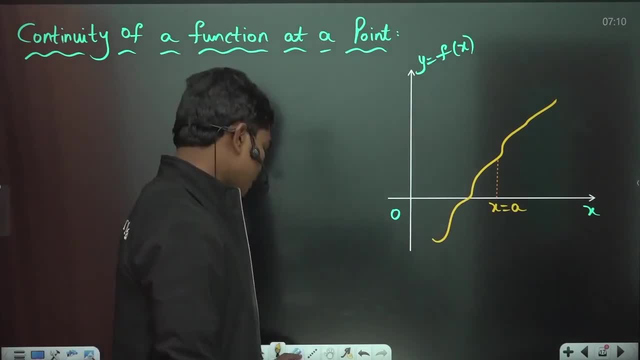 so for checking mathematically. first of all, let me explain you one thing. Look, let us suppose the function is discontinuous here, for example. okay, let us suppose the function is discontinuous here, And many times you might have seen functions like this: f of x is. 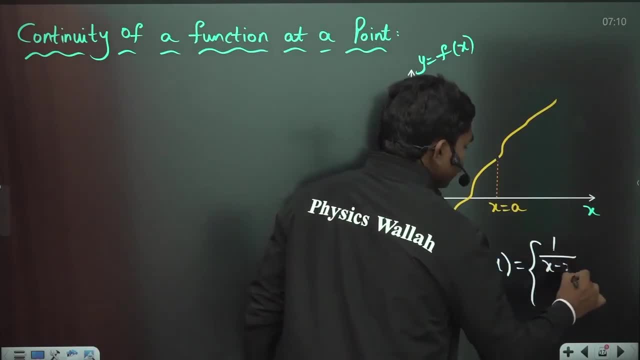 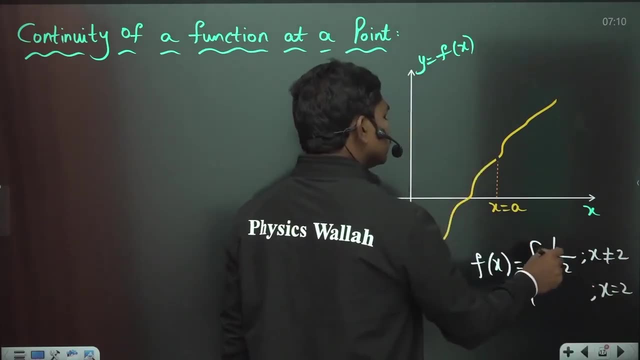 equal to 1 by x minus 2,. when x is not equal to 2, then at x is equal to 2,. since this function is not existing because you with 0 is not defined, so they will define some values, for example say pi by 4, something like. 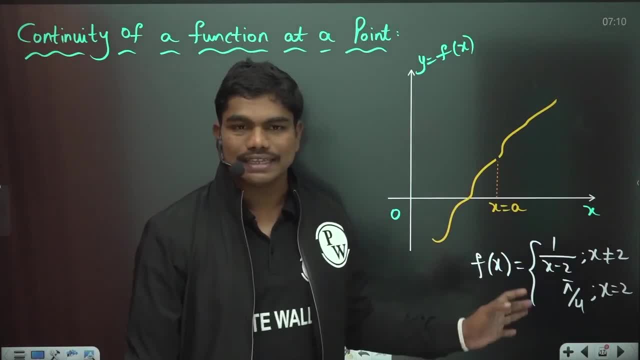 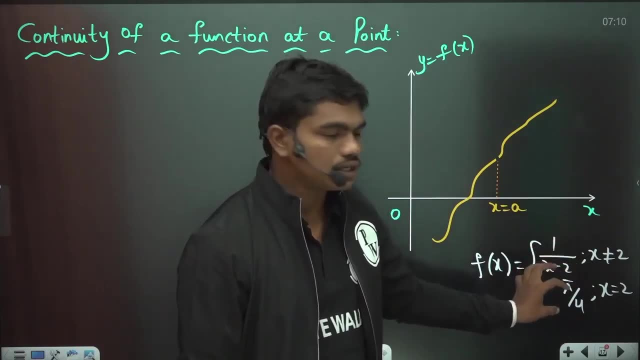 this: okay, they will define some value. so these kind of functions you have seen, and these functions are called split functions. okay means because at x equal to 2 there is some discontinuity for this function, this function is not defined. basically because division with 0 is not defined, they give 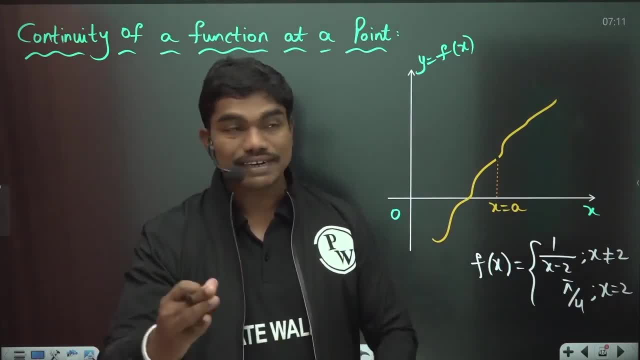 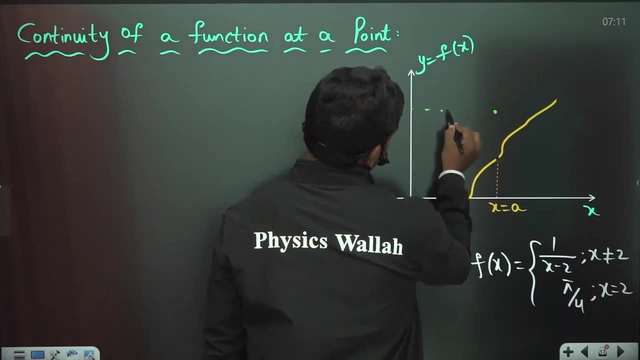 you some other value of y? okay, so these functions are called split functions. okay, so now let us suppose this is defined somewhere here. so f of a is defined somewhere here, for example: okay, this is your f of a at x is equal to. f of a is defined somewhere here and at other parts. the 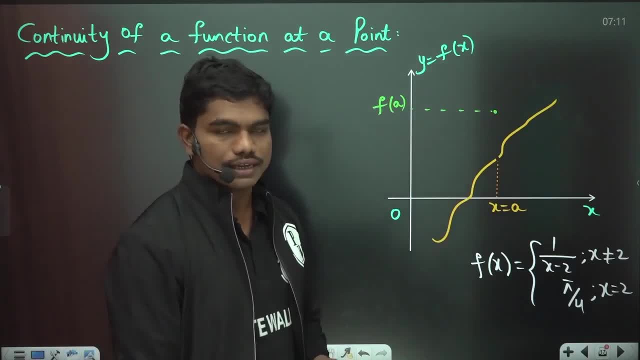 function is continuous. now i want to tell you one very important thing here for the function: even if the function is discontinuous, still limit can exist. how look here? i will tell you. let us suppose if this value is l, for example. okay, if this value is l, then you can understand. 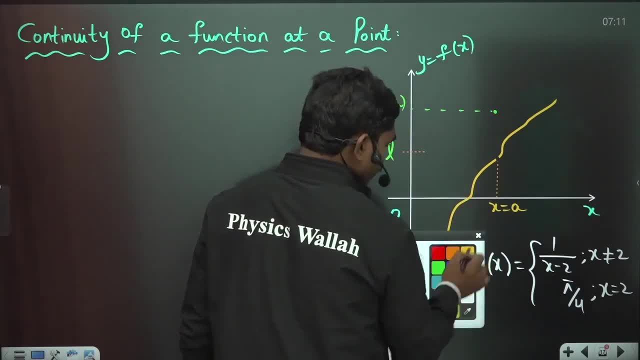 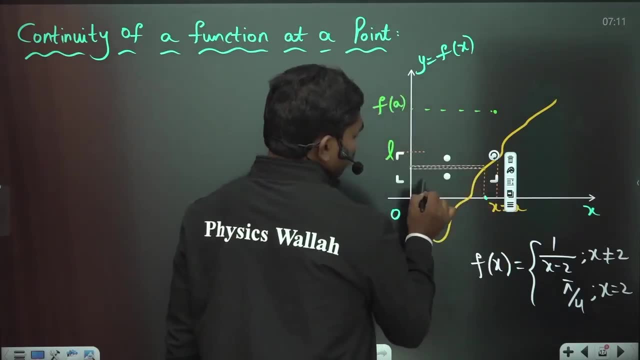 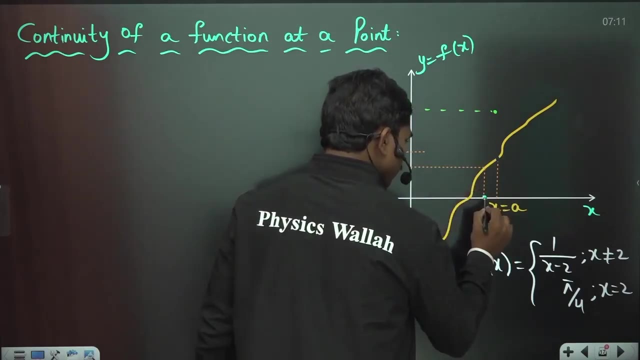 one thing. let us suppose if x is here. if x is here means in the left neighborhood. so then if you see, this is your f of x value, correct, this is your f of x value here. this value is your f of x. now let us suppose if x is moving towards a. let us suppose from this point it moved somewhere here. so as it's. 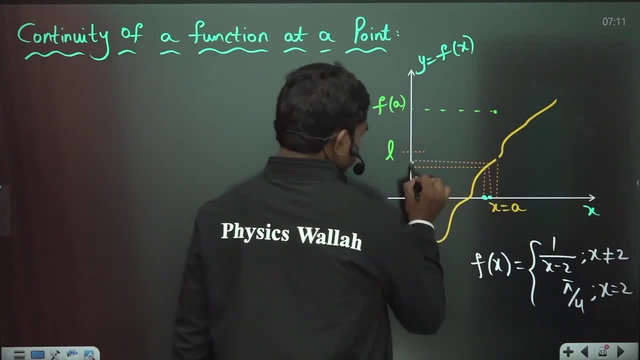 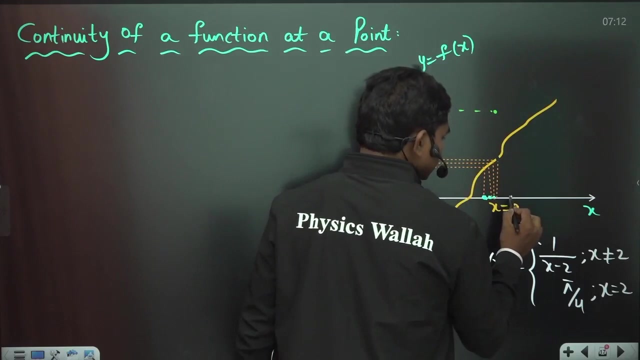 moving towards x is towards a. your f of x is moving towards l. okay, so, similarly, if you take one more point here, somewhere here here, if you take, yes, so somewhere here slightly, if you take, then you will again observe this f of x is basically moving towards l. similarly, in the right side case also, if x is initially at this location, then if 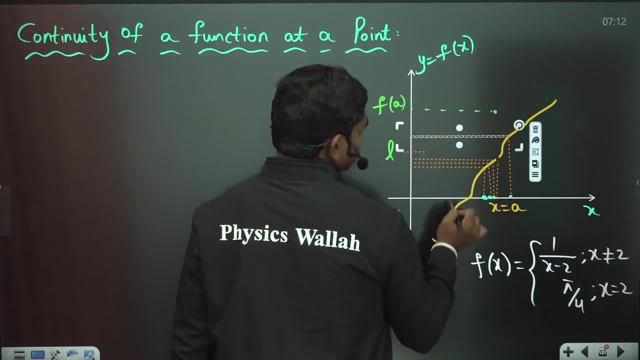 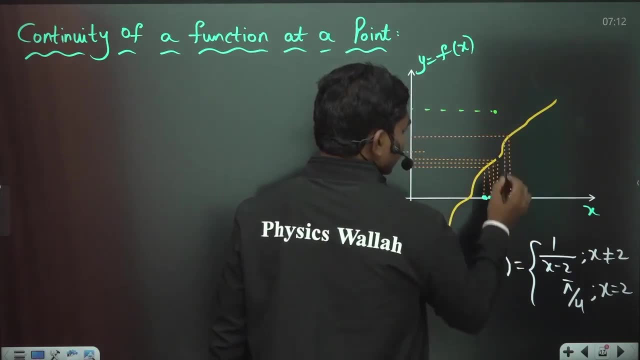 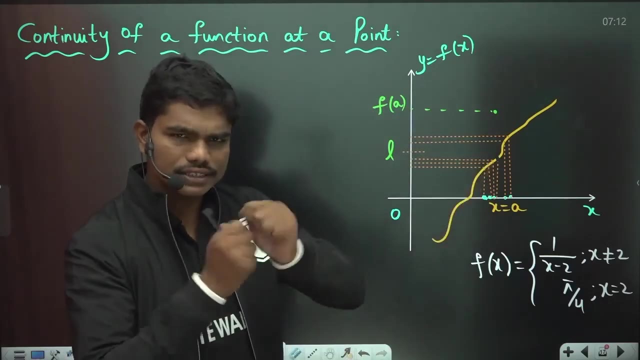 you see, your f of x value is somewhere here. then when x is moving towards a- let us suppose it got slightly moved here- then your f of x value is again tending towards l. so basically you can see one thing: this function is not continuous and x is equal to a. there is clearly, you can see, there is a breaking. 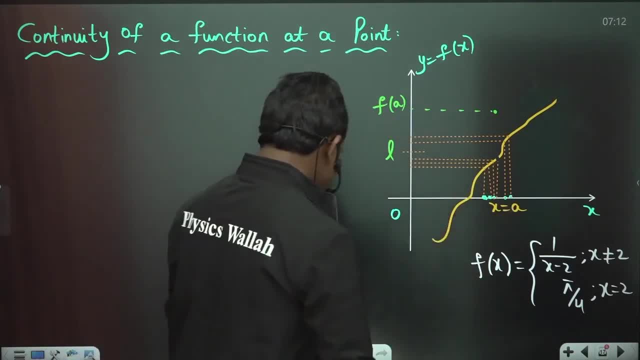 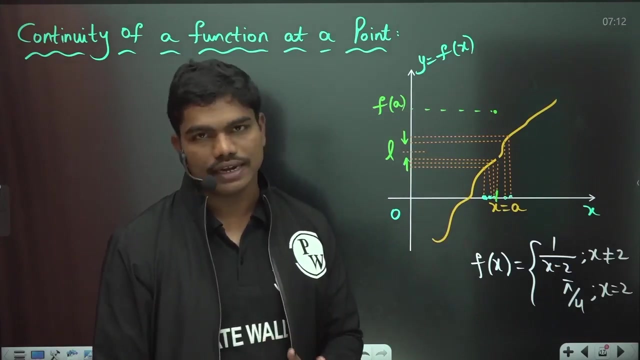 or at that point, but still, as x tends to a means, if this point is a and if this point is a, as x is moving to a from both sides, this f of x values are moving towards l. okay, so you can observe one thing: even though the function is discontinuous, limit of the function still can exist, okay, so 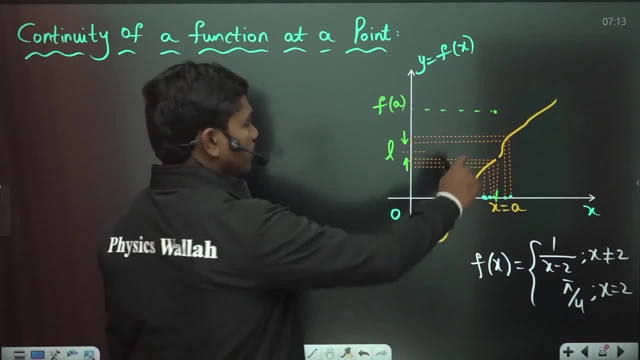 that's how. so basically now i am talking about this function being discontinuous because there is a breaking here now, what I am going to, Kraplik, what i am essentially going to visiting the four a, because there is a breaking here now. let us just judge your third example. 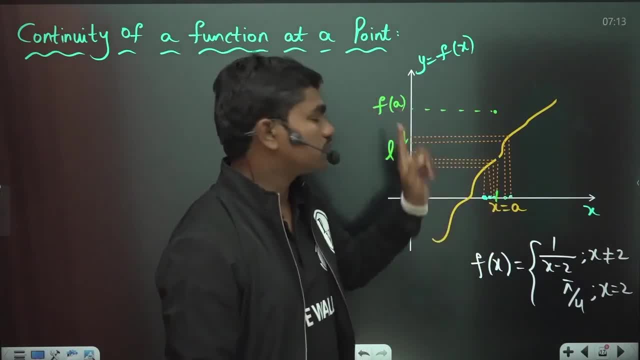 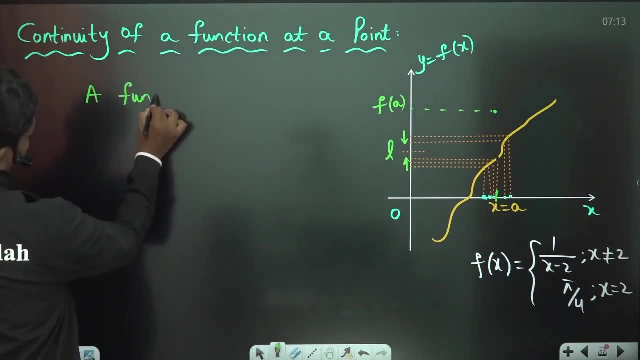 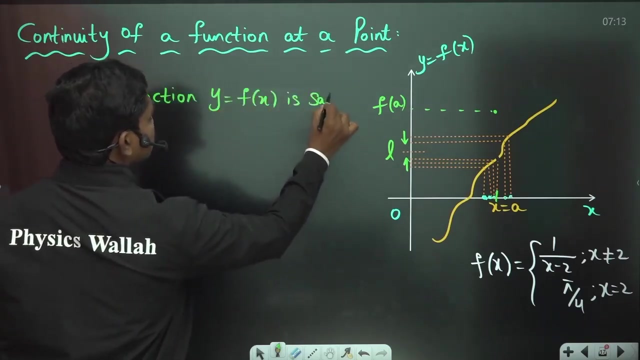 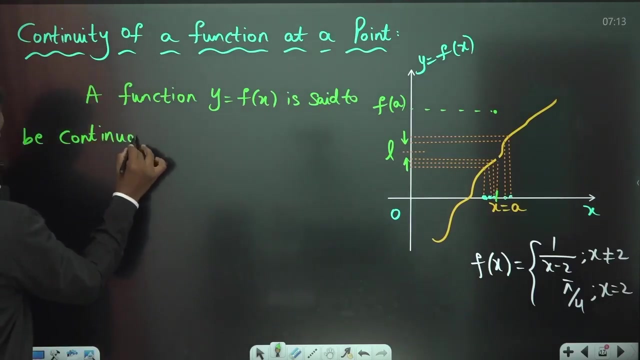 how do we check mathematically at a particular point whether this function is continuous or not? okay, how do we check that? look a function, a function. y is equal to f of x, is said to be. is said to be continuous, is said to be continuous at x is equal to a. 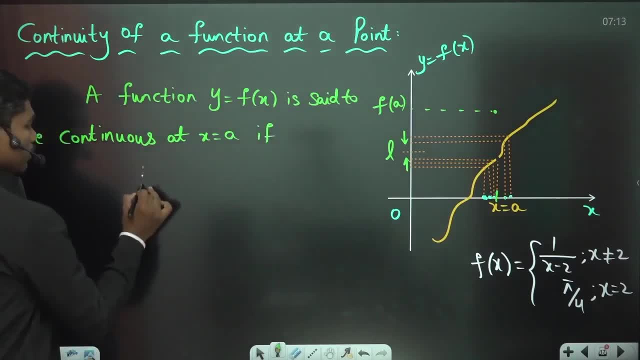 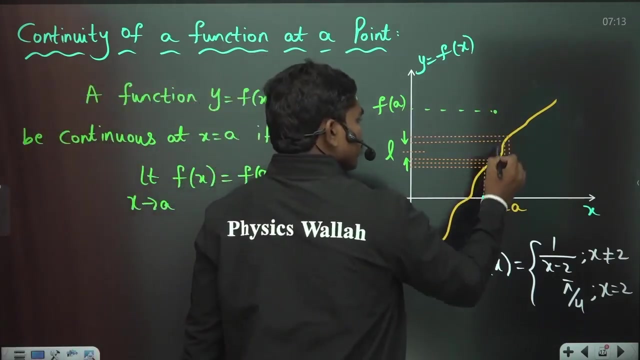 if limit extends to a, f of x is basically is equal to f of a. what is the meaning of this? look, how did this equation come? see here? i'll tell you. look, let us suppose if this point comes here, for example: okay, this point, we have slowly dragged and kept it here, so this point is now. 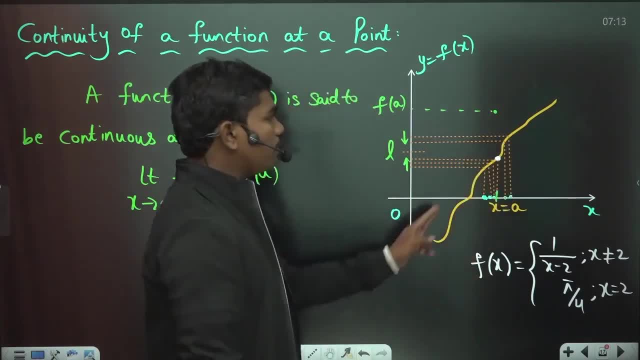 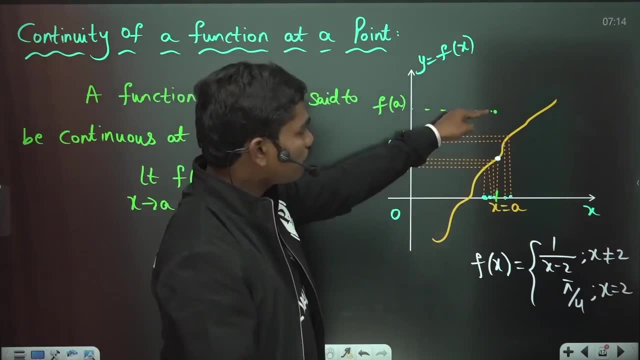 acting as a bridge for these two parts and it is connecting the curve. okay, now, whenever this point comes and sits in this gap, then definitely it is acting as a bridge for this two parts. definitely this function becomes continuous, correct? what is the mathematical meaning of this point? physically coming here, this f of a coming to l, correct? so if this f of a is coming, 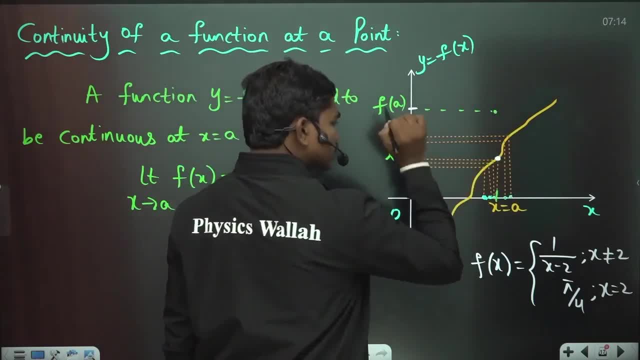 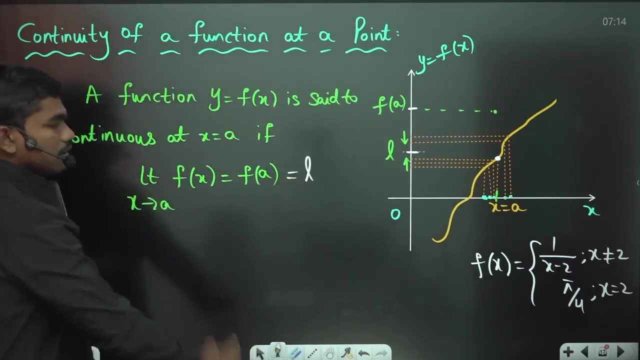 equal to l. that means this point is actually coming and sitting here and making the function continuous, correct. so means basically, this f of a should be equal to l and l is nothing but limit extends to a f of x. so that's how, if a function has to be continuous, it's limited. that particular 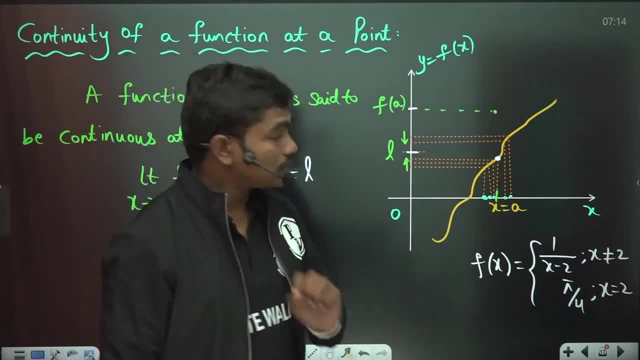 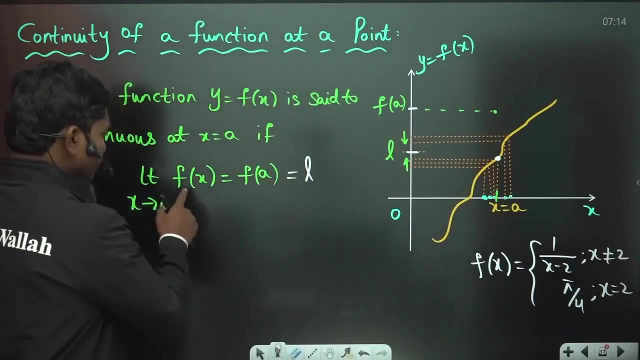 point should be equal to the functional value. okay, look, as i told you, even if a function is discontinuous, still limit can exist. but if the function has to be continuous, definitely this limit has to be equal to the functional value. clear, so we'll write a note here. note if limit. 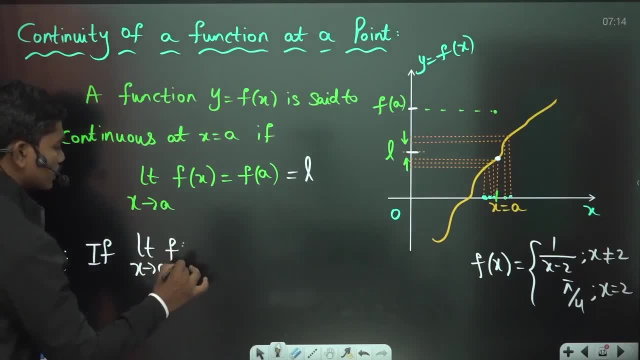 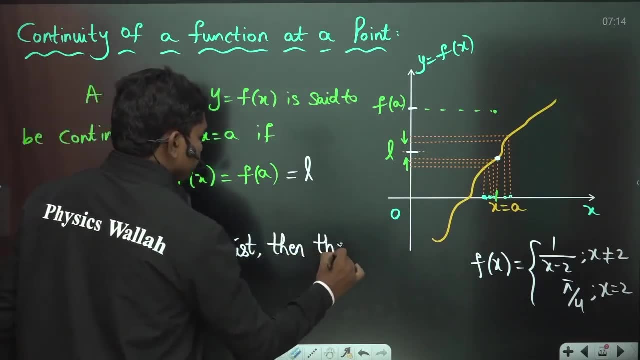 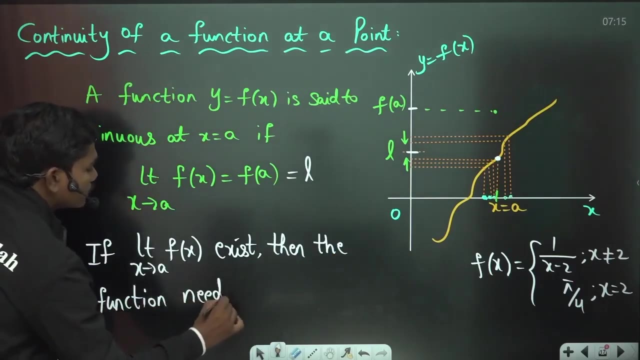 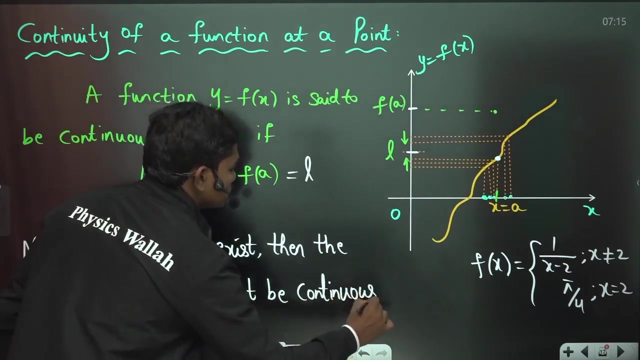 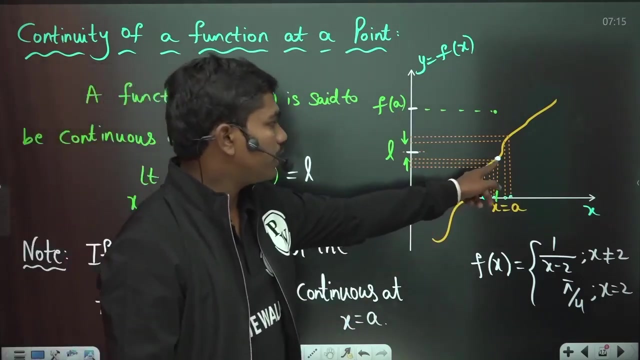 extends to a f of x exist, then the function is continuous. need not be continuous. at x is equal to a. need not be continuous. need not be continuous. at x is equal to a. okay, so at x is equal to a, because you have clearly seen at this point previously the 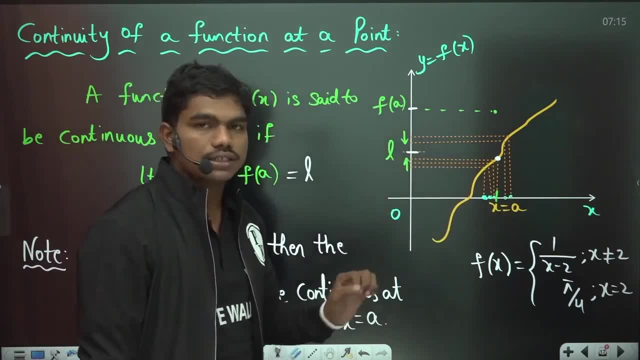 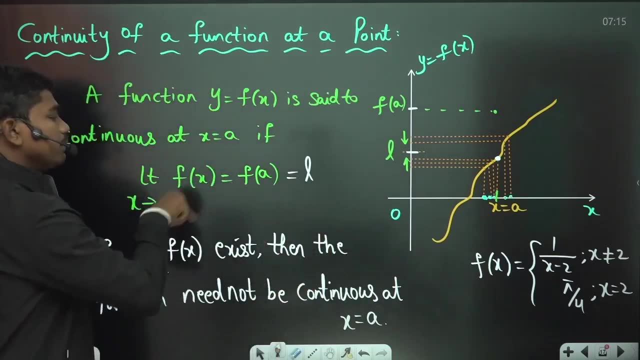 function was discontinuous, but still the limit got existing. okay, so that's how. if function has to be continuous, limit should be equal to the functional value. okay, if these two are not equal, even though this exists independently, but still the function cannot be continuous. okay, so that's how. this property is actually very important. okay, if limit exists. 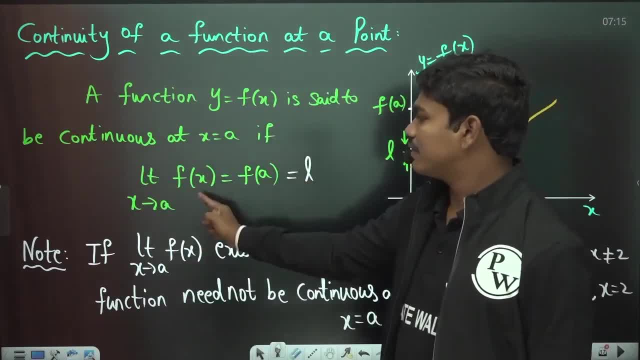 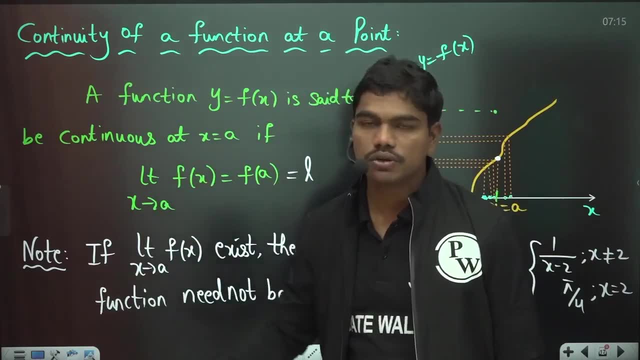 function need not be continuous. but if function is continuous, then definitely limit is existing. okay, because if we want to show this, equality definitely should have some value here. so this limit should definitely exist, okay. so that's how we will talk about continuity. then we move on to 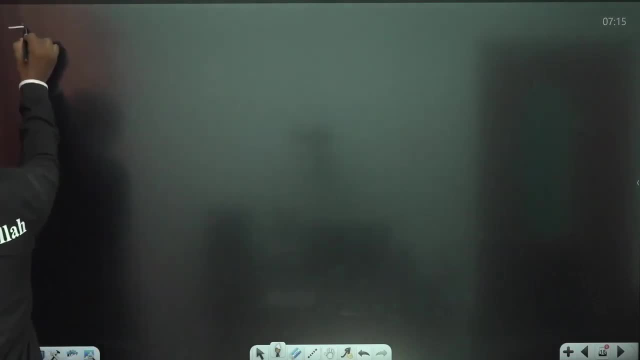 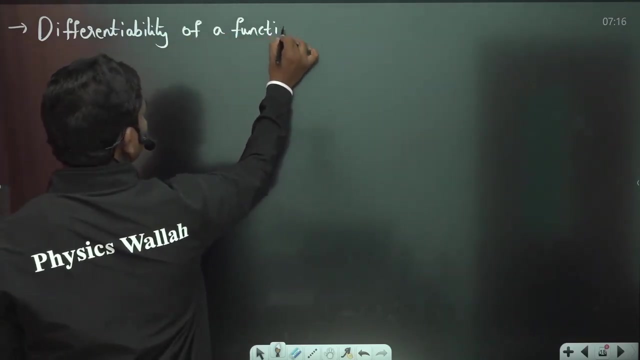 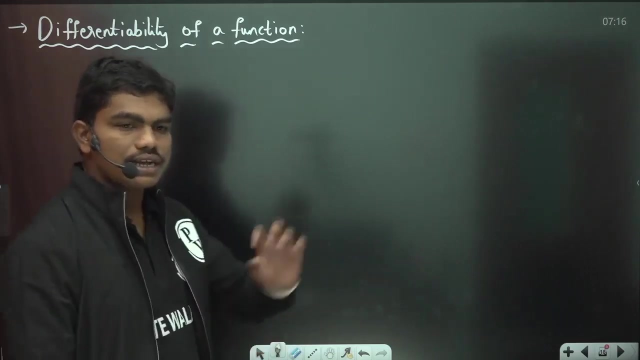 one very drastic application. i would say: differentiation or differentiability of a function. differentiability of a function, differentiability of a function. now see here what is this? differentiability of a function means basically, when you say a function is differentiable at any point, for example: okay, so we'll write it this way: a function, a function y is equal to f of x. 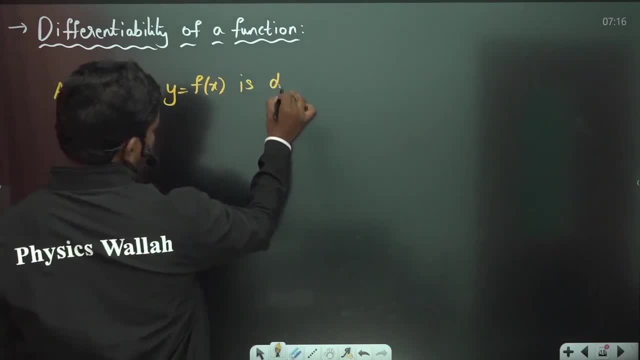 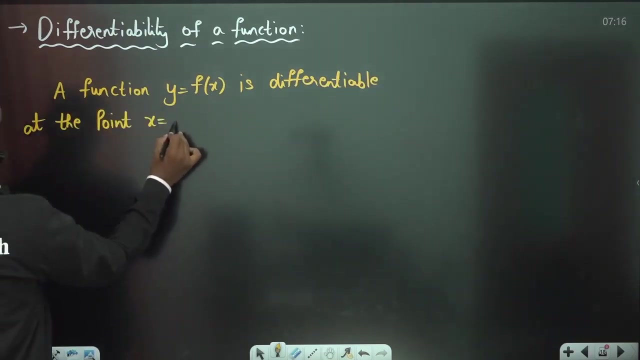 is differentiable at the point. is differentiable is a differentiable at the point. x is equal to a. is differentiable at the point. x is equal to a. if limit extends to a f of x minus f of a divided by x minus a, this limit exists. this limit exists. now, what is this? 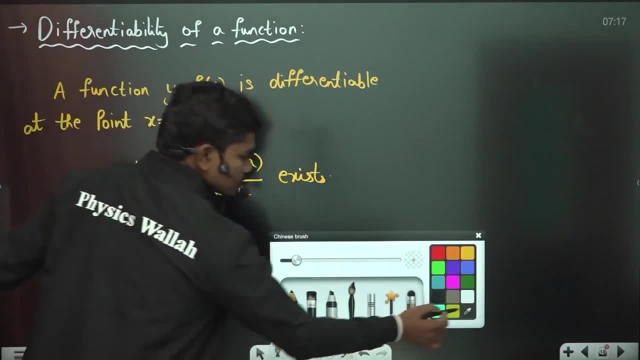 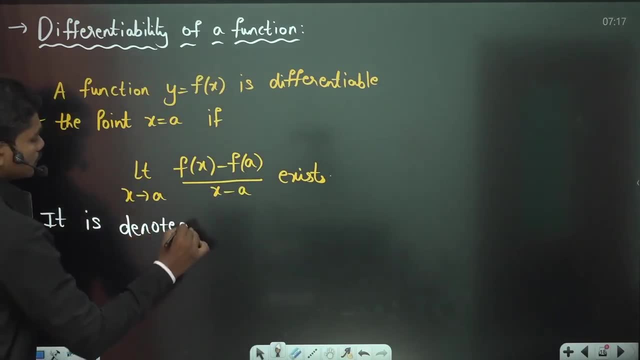 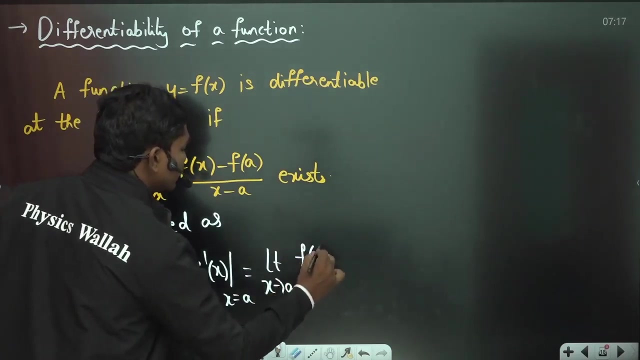 limit, basically, and what, how do you write this? okay, this is written as it is denoted, as it is denoted as it is denoted as f dash of a, which means basically, f dash of x at x is equal to a. this is equal to limit extends to a f of x minus f of a divided by x minus a actually here. okay, so, 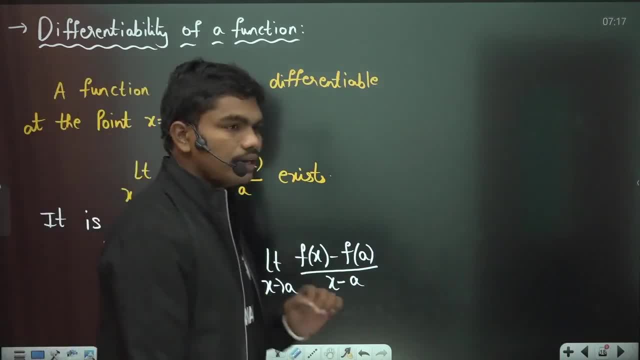 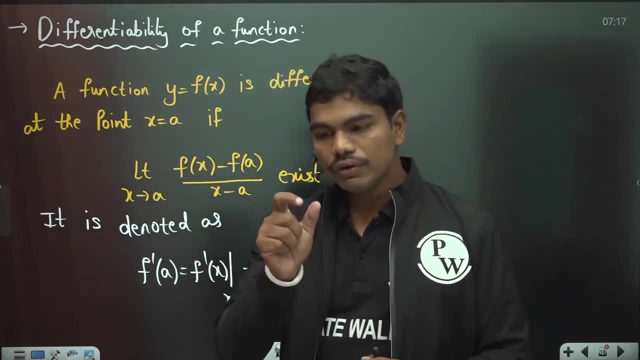 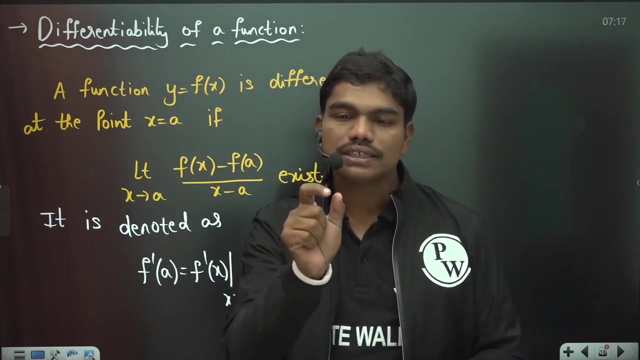 this is how we denote this and who gave this formula? basically, y, f of x minus f of a. you know, derivative is nothing but dy by dx, correct? what dy by dx tells you actually? look, if you add dy by dx that value talks about, when you change a small quantity in x, which is dx, what is the change in y? 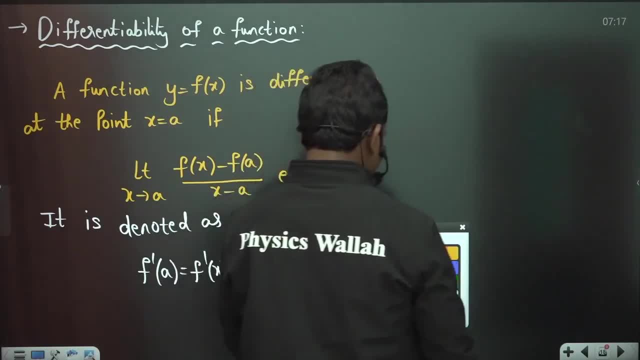 that's what dy by dx talks about. okay, so look here, let me explain you graphically also. let us suppose this is some x axis and y axis, for example. then you have horizon x, y, like this. now let us suppose you have some function, basically okay, so you have. 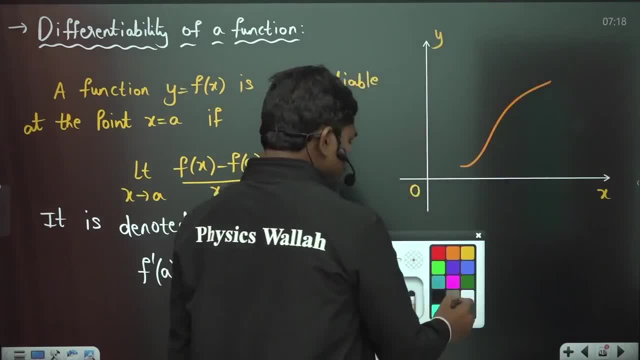 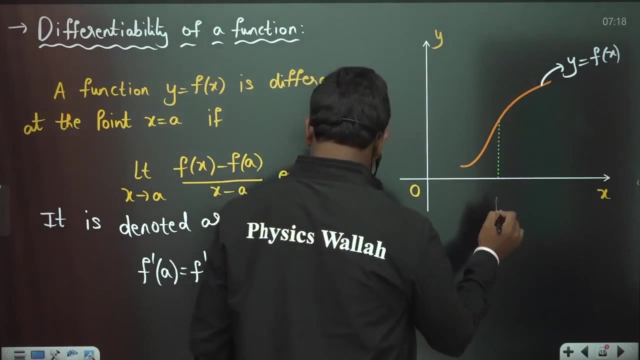 some function like this: now, if this is, y is equal to f of x. and now let us understand one thing. let us suppose this point is x or a, x is equal to a, for example. okay, this is a, x is equal to a, and this point, which is here: 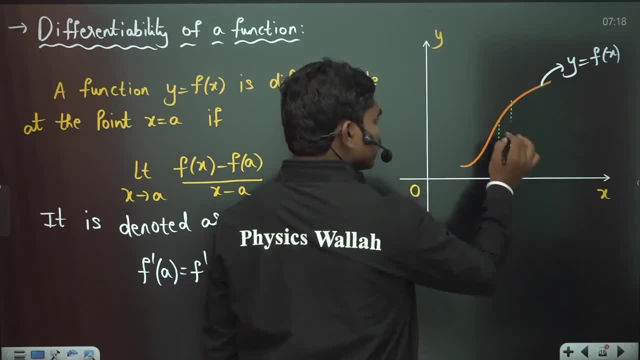 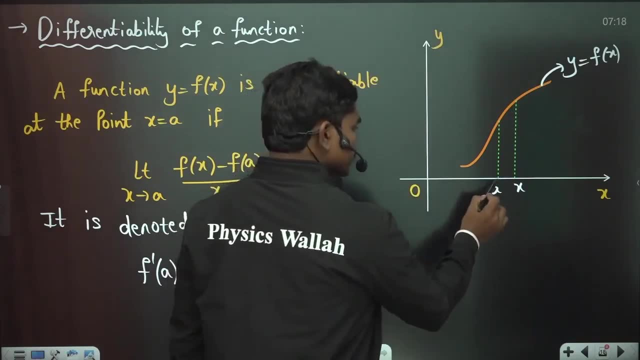 slightly okay. actually, the points f of x is equal to a and this point, which is here slightly okay. actually, the points x and y are very close, but since to make things clear, i am putting them apart. so this is x. now tell me one thing: if this is x is equal to a, then definitely this value is. 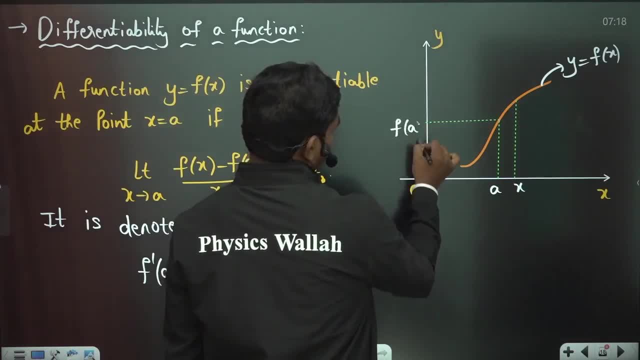 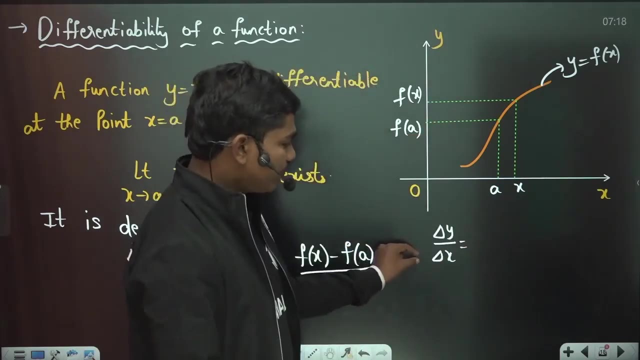 nothing but f of a. correct. and similarly, this value is f of x, f of x. now, if i want to calculate delta y by delta x means, let us suppose if i am interested in finding if i give a small change to x at this location. means initially my x is at a. now let us suppose if i am changing this x by a. 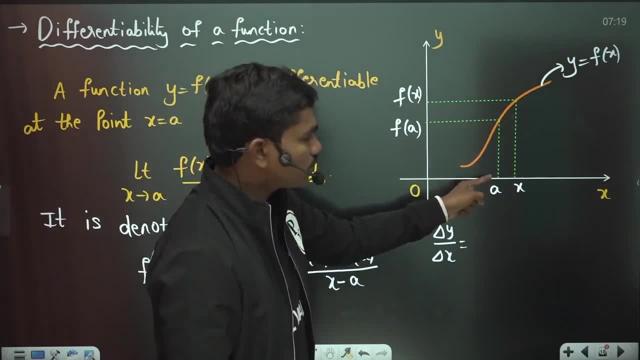 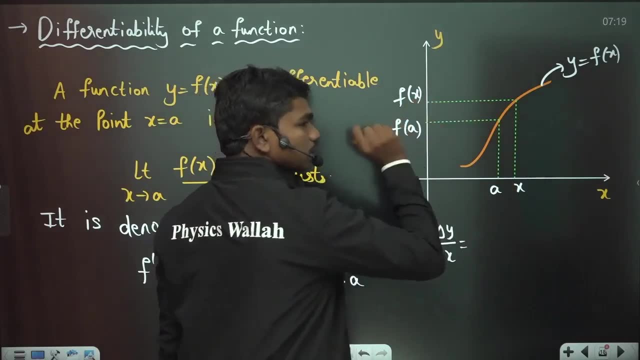 small amount. if initially x is here at this point a, so slightly i have given change. so when i slightly change the value of x, what is the corresponding change in y? okay, that's what i am interested in. okay, so look what is the change in x. i am giving x minus a. this is the change i. 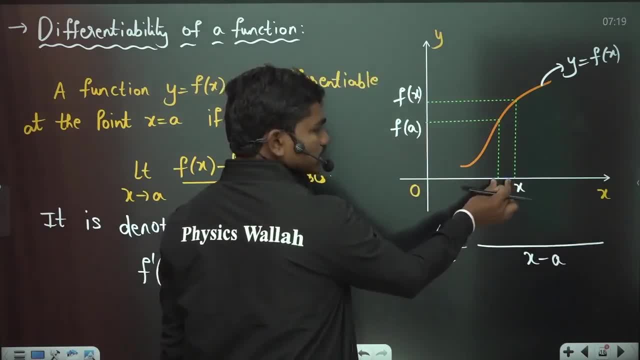 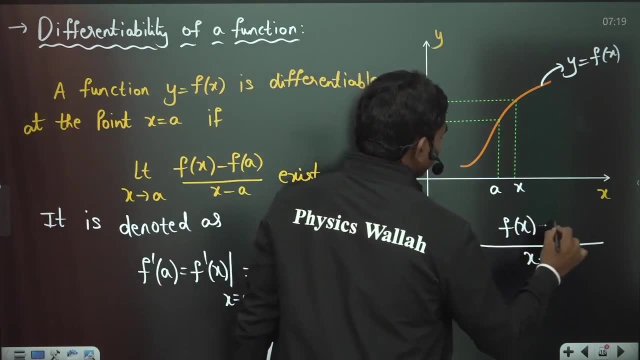 am giving correct, because this x minus a is the difference. so this is the change in x. so this change in x is bringing a change of f of x minus f of a. f of x minus f of a is the change in y. but since limit continuity, 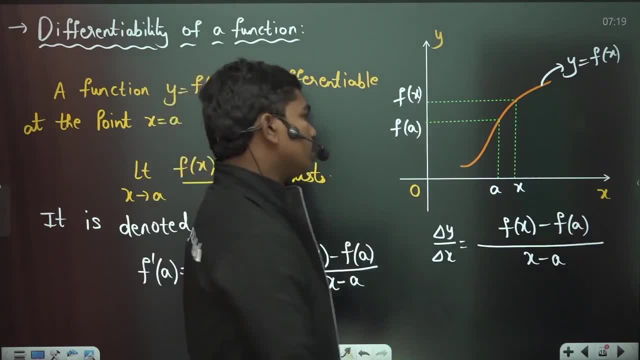 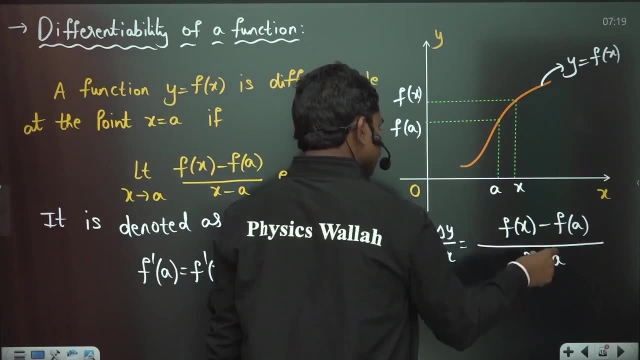 differentiability. all these are defined at a particular point. so if this length has to be some point, actually of very small length actually, then this x minus a distance or this length has to be very small, which means almost zero. if x minus a tends to zero means if x minus a. 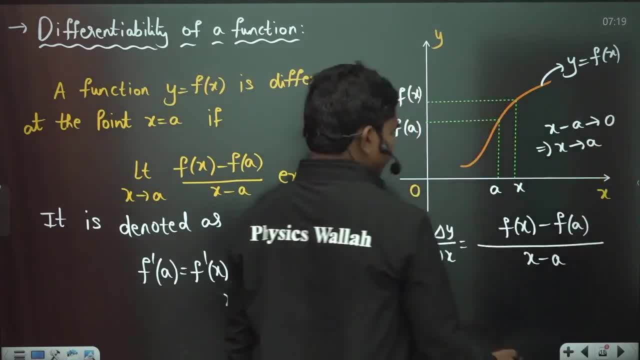 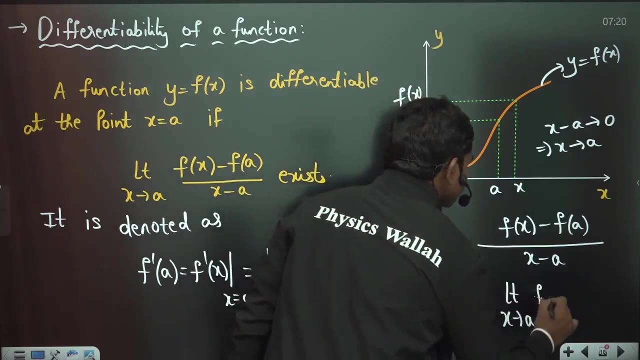 is going to be very small. that means x is going to be very close to a. so that's what we write. limit: this implies dy by dx. at this location, of course, we are talking at the point x is equal to a is nothing but limit. x tends to a f of x minus f of a divided by x minus a. okay so, and of course this: 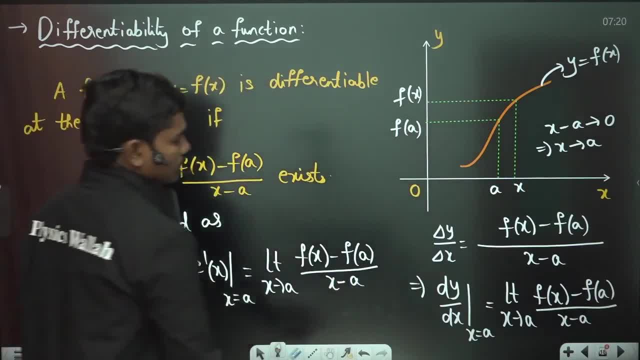 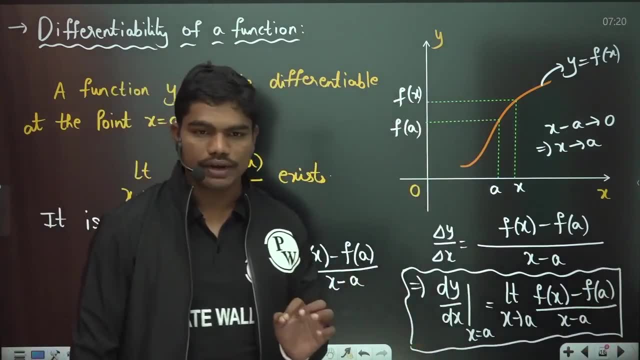 is denoted as f dash of a, which we have written here: f dash of a. so this is how we have got the result okay, so this is how we have got the result. okay, so this is how we have got the result, okay. so now, basically, this is the condition to check whether, at a particular point, limit exists or not. 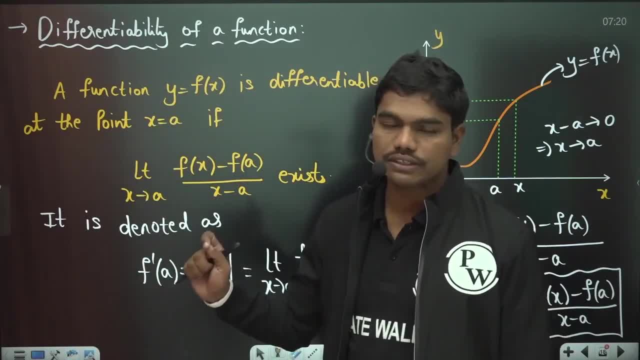 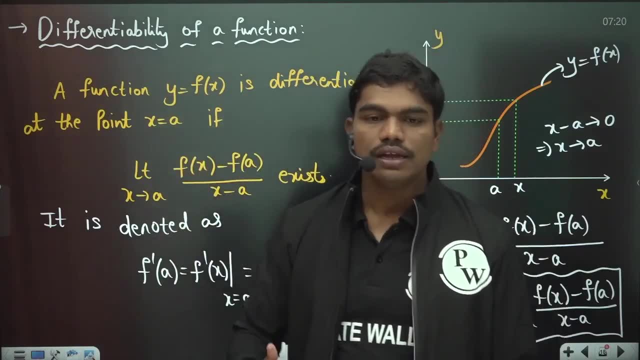 okay, so if this limit is existing, then definitely the function is differentiable and the value of the differentiation is the value of this limit. okay, if this limit does not exist, then the function is not differentiable. okay, so this is the simple way to identify what. what is a derivative? 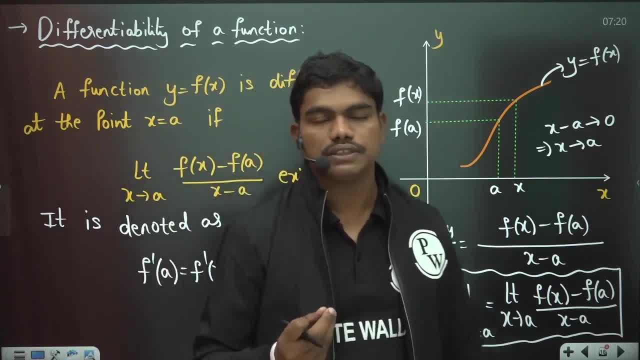 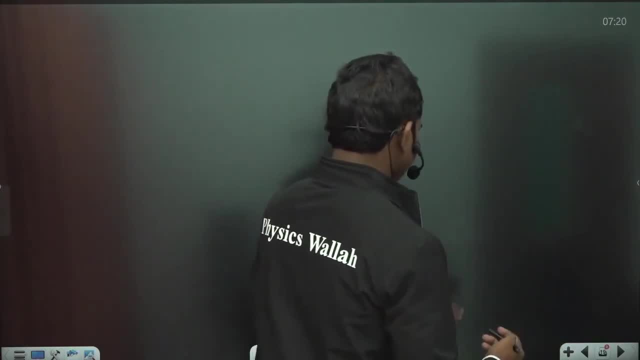 okay, but before this there is again one principle, which is called the first principle of differentiation. okay, so what is the first principle of differentiation? look, same thing. let us suppose this is your x axis and this is your y axis, for example. so this is your origin, x, y. so 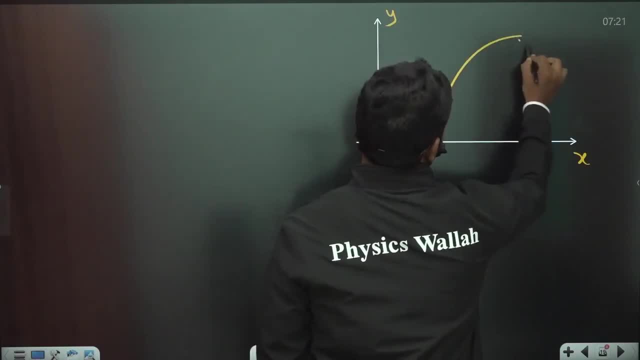 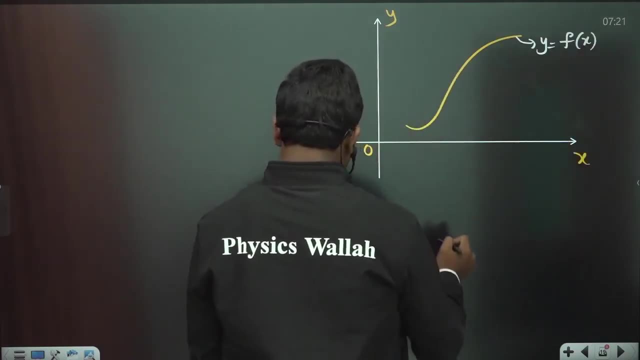 this is: y is equal to f of x again, so y is equal to f of x. okay, so if y is equal to f of x, then then this is the value of x. let us say then, obviously, let us suppose this corresponding value is X plus H. H is some, you know some constant such that 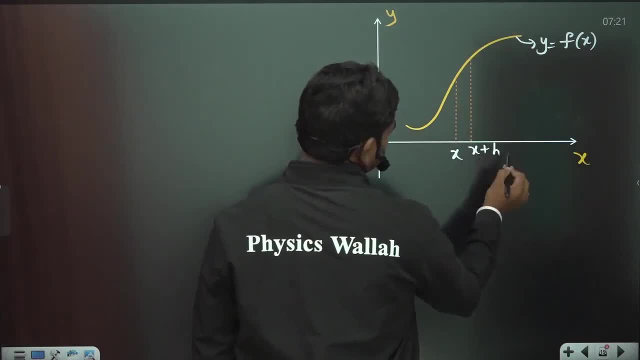 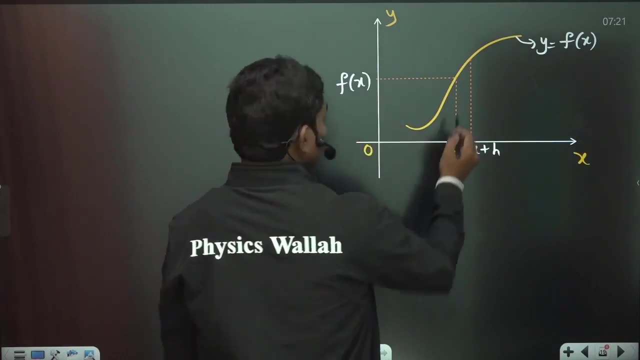 we have given some small increase to X, So this is X plus H. So, correspondingly, what happens? this value will be f of X and this value corresponding here will be f of X plus H. okay, So this value is f of X plus H. So now, if you calculate delta y by delta x, 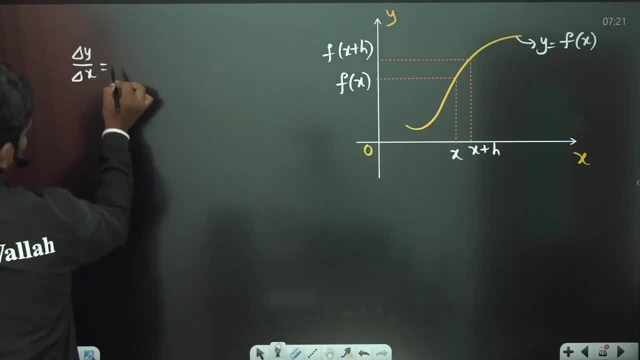 delta y by delta x is actually equal to now. we did not take any particular point here or something. We have taken some random value on X axis. okay, So delta X is basically X plus H minus X, and f of this is f of X plus H minus f of X. okay, So this is delta y by delta X. So 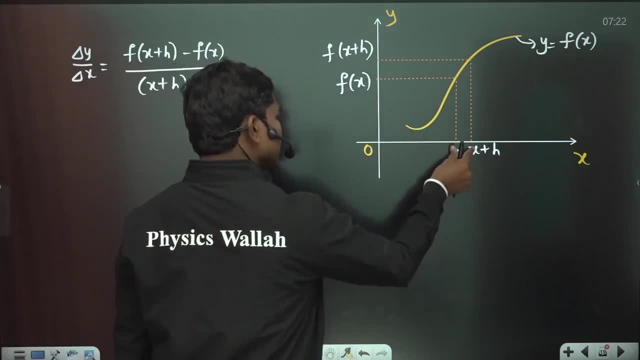 when, if you want to calculate at any particular value of X, this length has to be a point actually. So that means this: X plus H minus X, this is f of X plus H minus X. So this is f of X plus H minus X. So this is f of X plus H minus X. 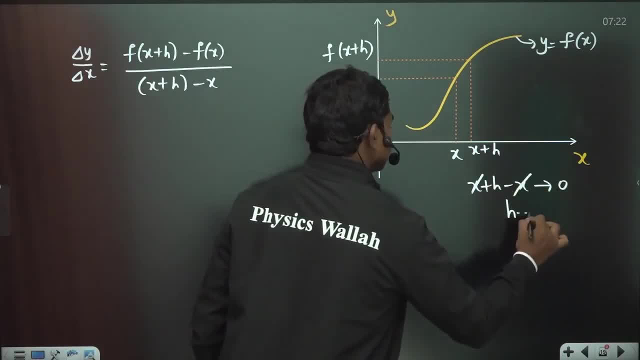 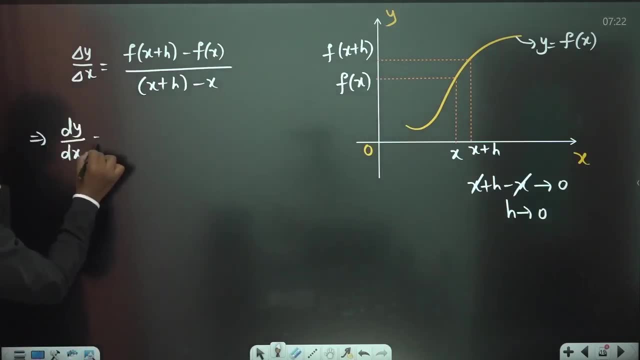 This difference should tend to 0, which means, if you simplify, H tends to 0.. So that's why, if you see, if you want to write this expression in terms of small differences- dy by dx, this is actually delta y by delta x is some big change, okay. So if that has to be a point instantaneous, we will. 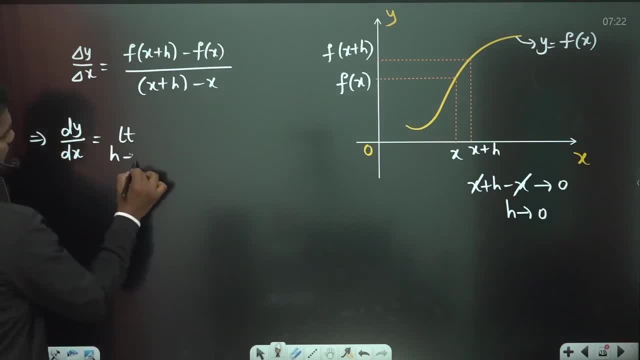 write dy by dx. So this is limit. H tends to 0, f of X plus H, minus f of X divided by H, actually, because X, X gets cancelled. So this is H and this formula you have seen at many locations. 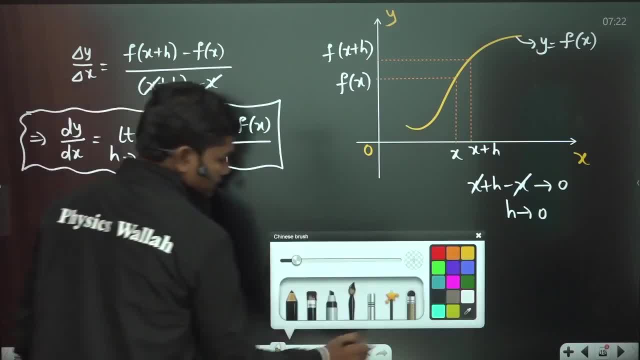 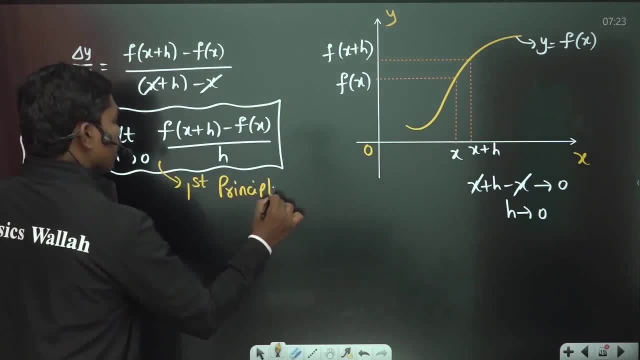 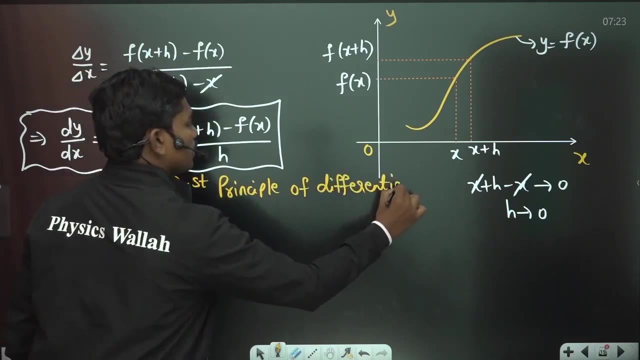 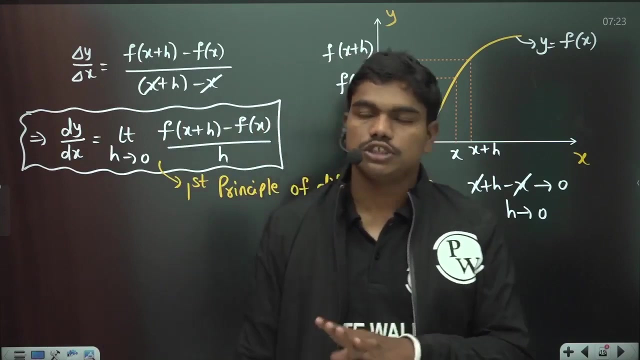 Okay, And this is called the first principle of differentiation. Okay, So this is called first principle, first principle of differentiation. Okay, So this is called first principle of differentiation, differentiation. Now, using this first principle of differentiation, you can calculate limit of any function. Okay, Of course, the function should be continuous. 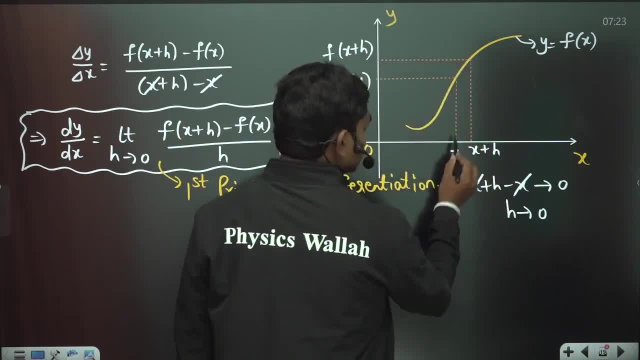 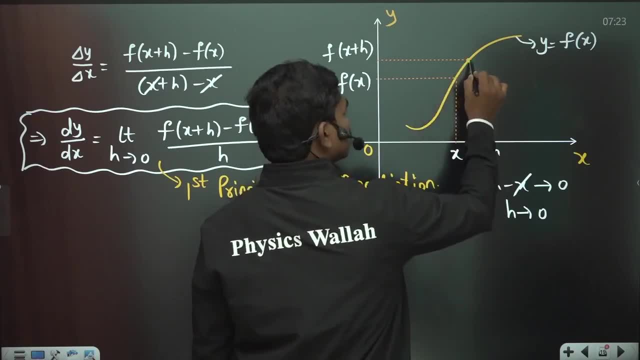 So if you see, because when I am talking about X plus H tends to X, this point should this point should come to this point very smoothly, Okay, There should not be any breakings here in between, because this X plus H is coming towards X, then definitely this point. 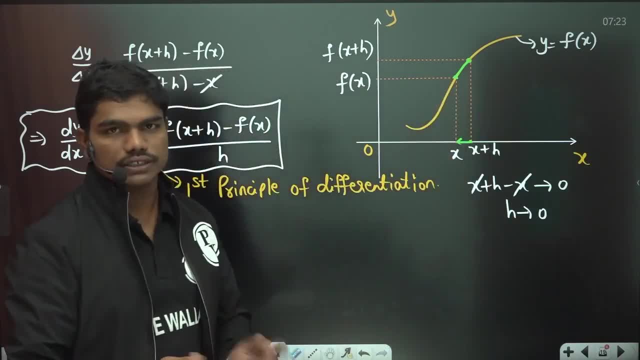 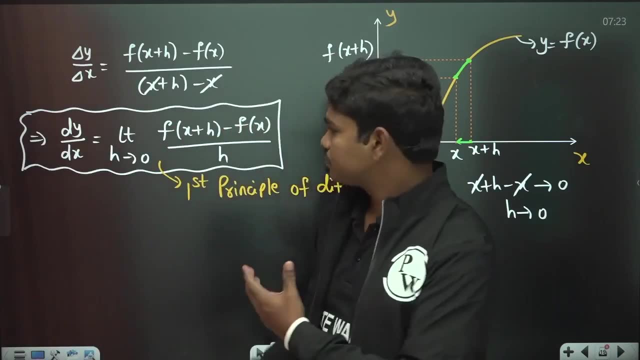 should come to this point smoothly, So there should not be any breaking of the function in between. So that's why, if you see, this is this is the way how you get it actually Okay. So this function is actually. this is basically denoted as f dash of X also, So this is also. 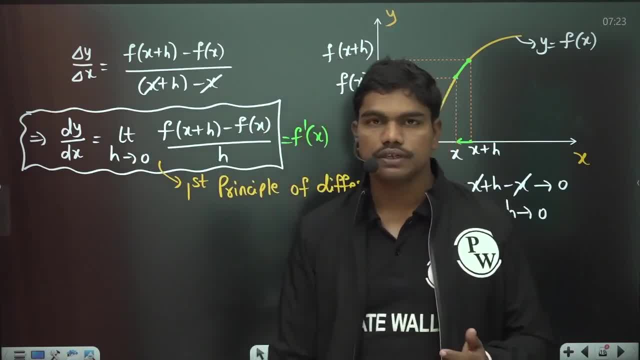 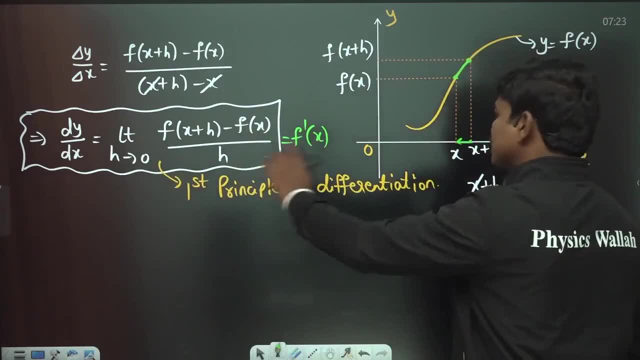 called f, dash of X. So if I give you some function, some continuous function, f of x, then you will calculate this limit And if this limit exists you will say the function is differentiable. Okay, This is in general at any location. this is in particular at a location. 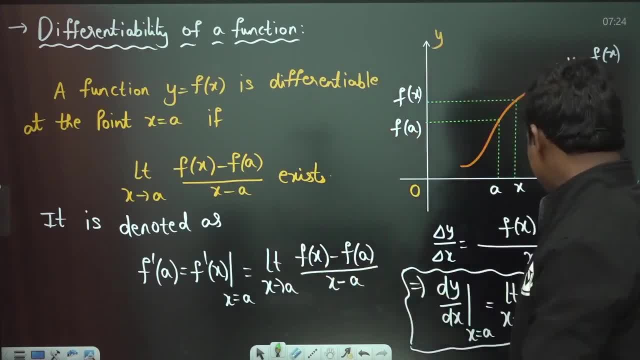 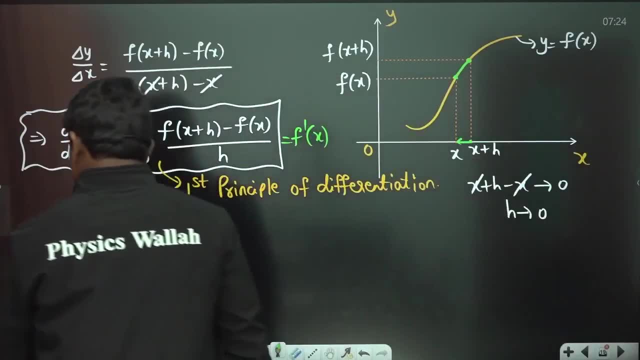 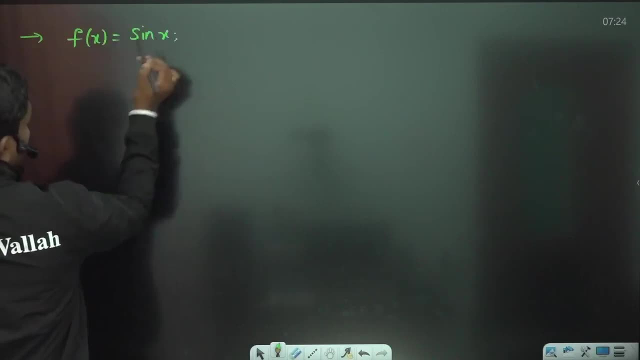 X is equal to A. Okay, Both are identical. You can see in the expressions. we have observed that, And here I would like to add one point. Look, for example. let us suppose I have given you some function. f of X is sine X. Now if I ask you, what is f dash of? for example say: 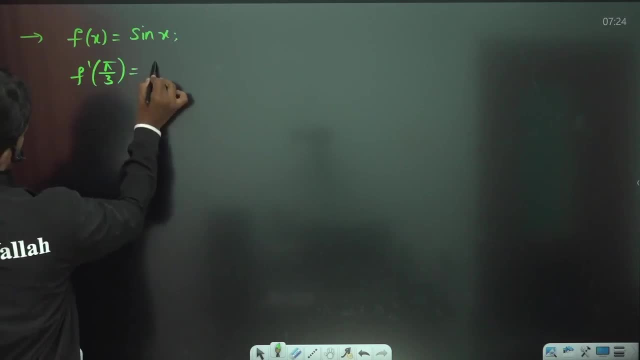 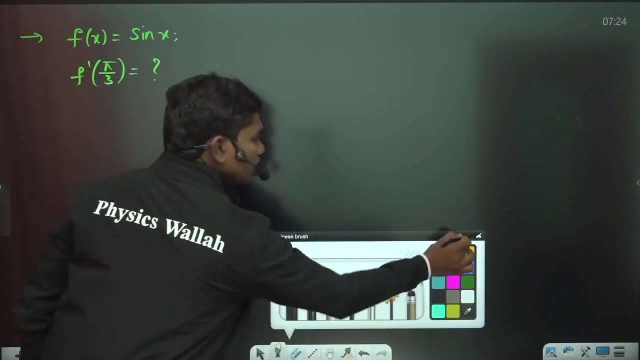 pi by 3, 60,, for example. Okay, Let us suppose if I ask you, what is this value, f dash of pi by 3, basically, Okay, Now you will calculate how you will calculate. first of all, you will calculate. 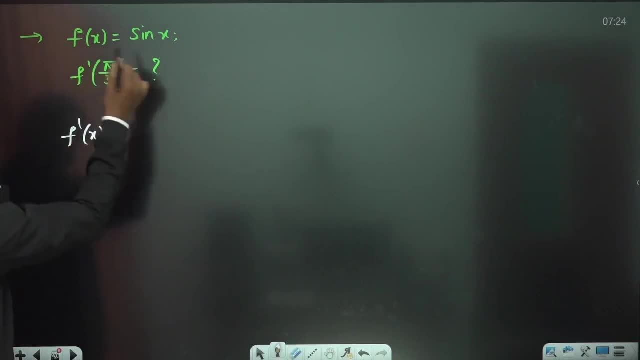 f dash of X. f dash of X is equal to: if f of X is sine X, derivative of that is cos X, then you will substitute this value. f dash of pi by 3 is equal to minus. sorry, minus is not there, So 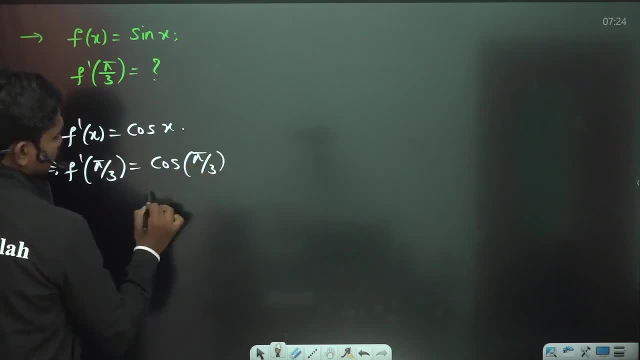 cos pi by 3.. So cos 60 is basically 1 by 2.. So what is the meaning of this 1 by 2?? Okay, Honestly, if I give you any function and if I give you some point, you will get some number. 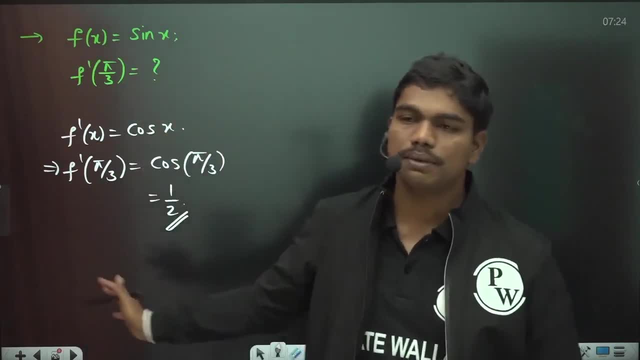 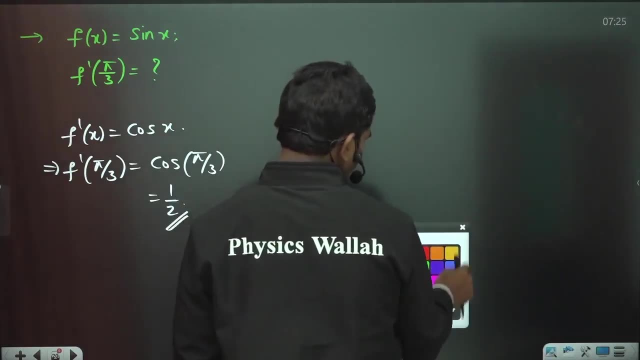 You will differentiate the function. substitute X is equal to something, then you will get some number. But what is this number telling you actually? Okay, So this number is actually telling you this value. Look, let us suppose, if this is your X axis, if this is your Y, 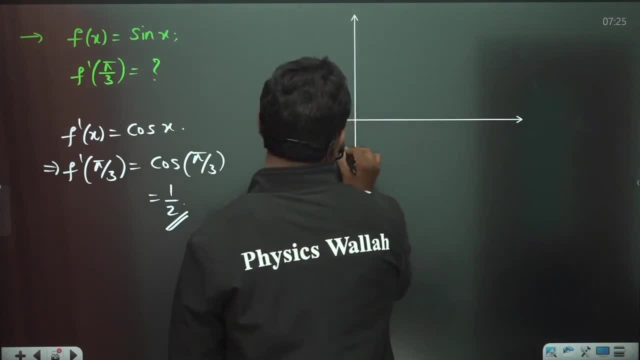 axis. so horizon, X, Y. Now, if you take the function sine X, let me draw. So horizon, this is the line Y is equal to 1,. for example, say like this: This is the line Y is equal to 1.. 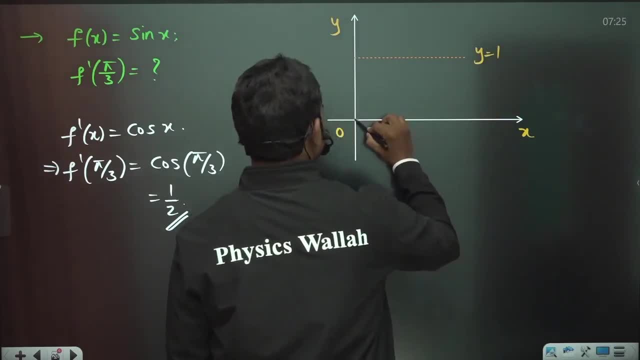 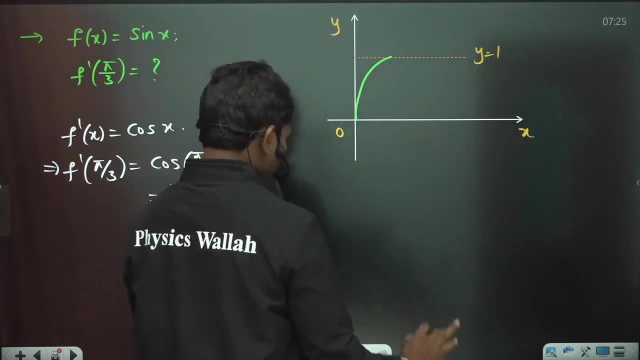 So sine X graph. if you plot the sine X graph, it comes out like this: So it starts from 0 and goes to pi by 2, like this: So, and afterwards it again falls to pi. But I have, of course, I am. 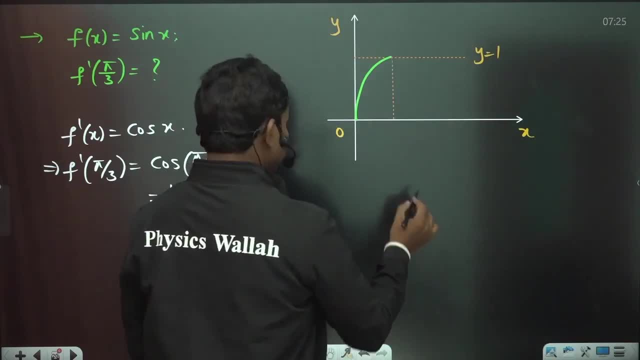 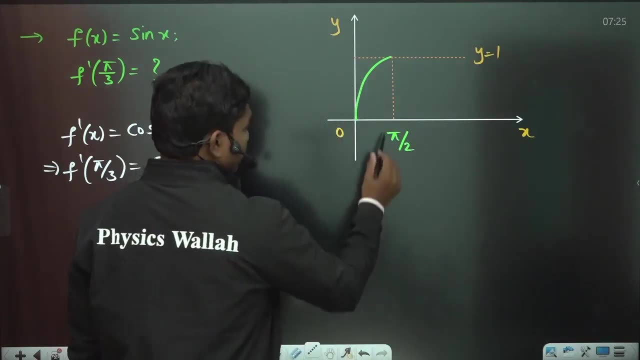 taking only till pi by 2.. Okay, So I am taking only till this pi by 2.. So if this is pi by 2, then what this 1 by 2 is telling you? if you take this point, X is equal to pi by 6, somewhere here. 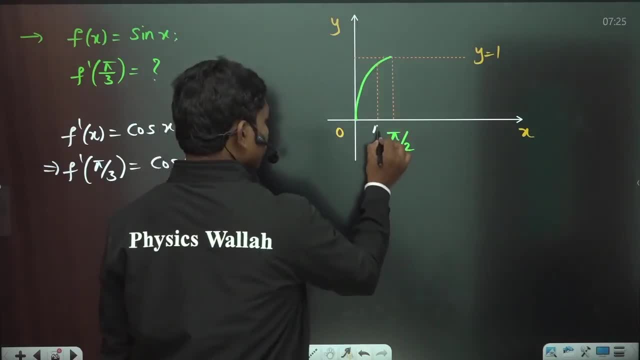 for example, if you take this point, X is equal to pi by 6.. Okay, pi by 3,. I have taken. Okay, so X is equal to pi by 3.. For example, if this point is, you know, pi by 3, X is equal to pi by. 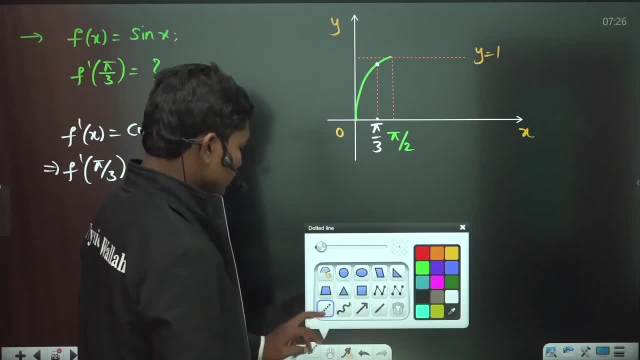 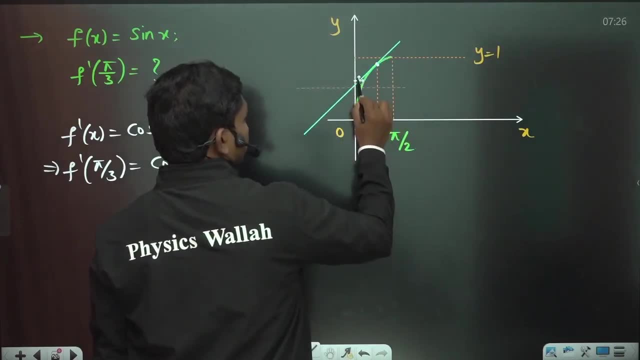 3, then this is the point on the curve. So what this function tells you is: if you draw a tangent to this function at this point, X is equal to pi by 3.. Okay, So let us suppose I am taking some. 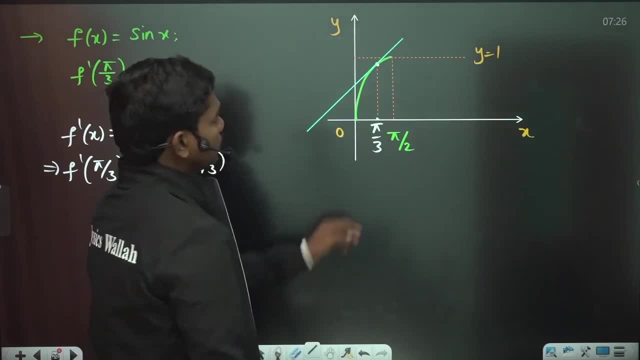 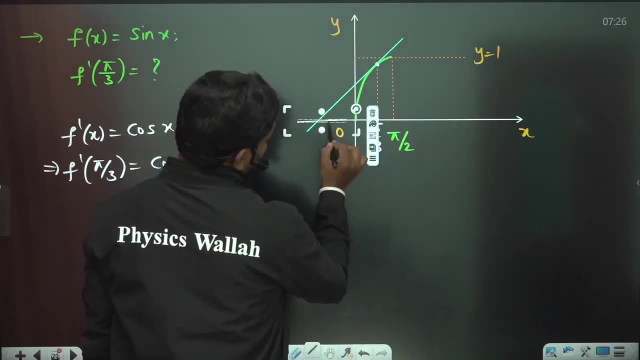 tangent to this function. at X is equal to pi by 3.. Okay So, at X is equal to pi by 3, if I take a tangent, then this tangent, then this tangent will make some angle with the X axis. Okay So. 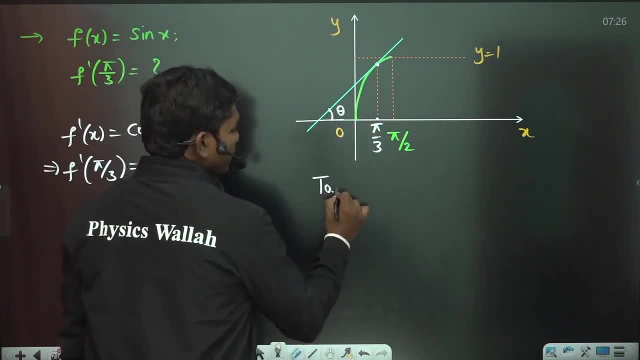 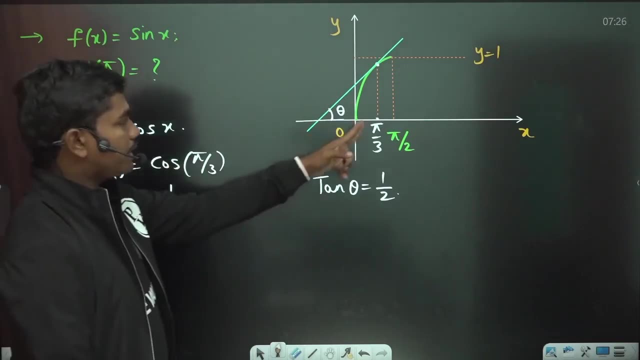 this angle is theta, So tan. theta value is equal to 1 by 2.. This is what we mean. Okay, So geometrically, this value 1 by 2 tells you that at X is equal to pi by 3, if you draw a tangent. 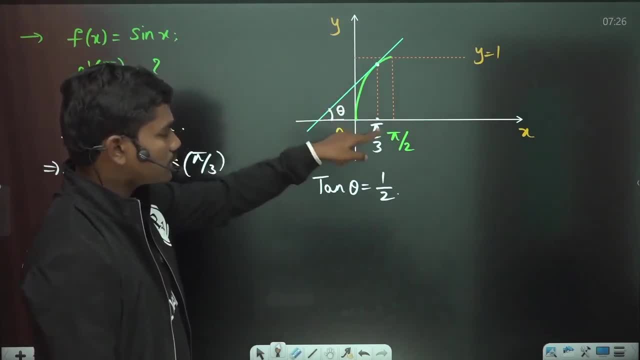 to this curve, then the angle made by the tangent to this X axis is theta. then tan theta value is equal to 1 by 2.. Now it is very clear: if we change the point, this value changes. Similarly, let us suppose instead of pi by 3, if I draw some tangent here, 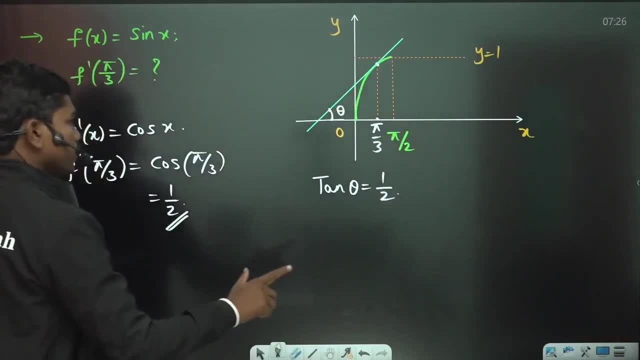 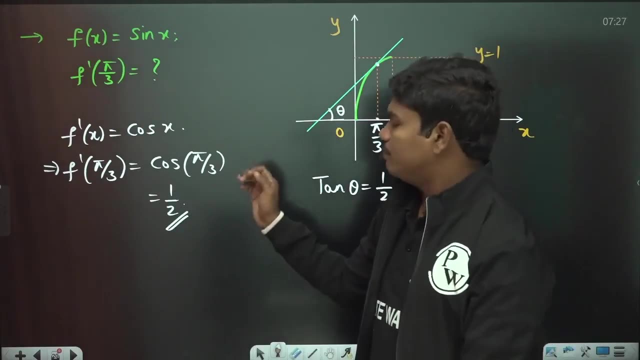 that tangent will make some different theta, but the theta will be in such a way that tan theta value will be equal to F dash of that function at that particular point. Okay, So F dash of A practically means the slope of tangent to the curve at the point X is equal to, and you know. 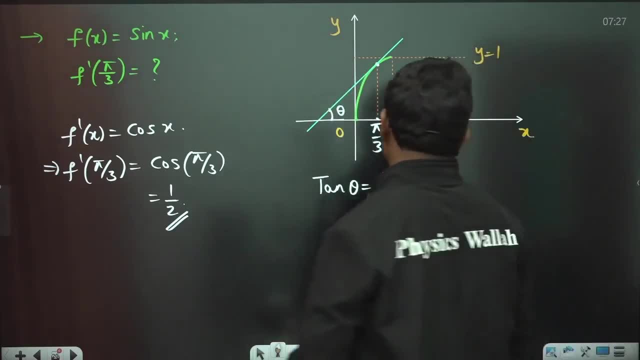 slope is nothing but tan theta for a straight line. we have seen basically, Okay, So if two points are connected by a line segment, then slope is given by tan theta, which is Y2 minus Y1 by X2 minus X1.. Okay, And if you clearly observe, this is nothing but difference in Y divided by difference. 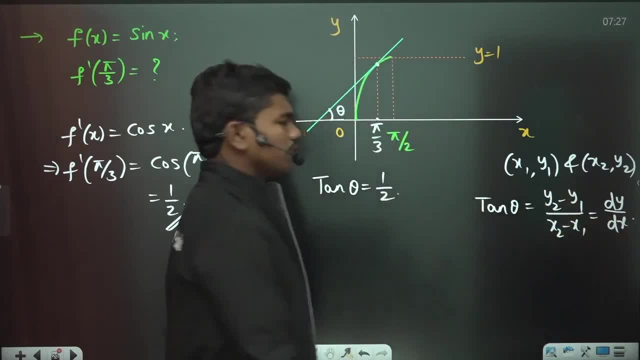 in X. actually, Okay, Change in X and this is change in Y. So all these are basically, you know, very in sync to each other And also you have done this form correct. If I ask you this equation, 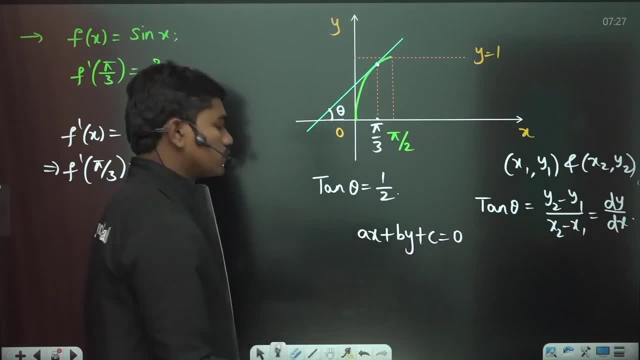 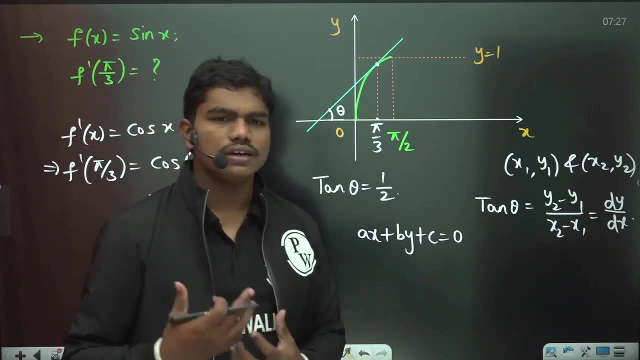 AX plus BY, plus C is equal to 0, which is a linear equation, of course. If I ask you what is the slope of this, you know line, basically it is a straight line. So if I ask you what is the slope of this line, many times you feel some ambiguity, like if it's 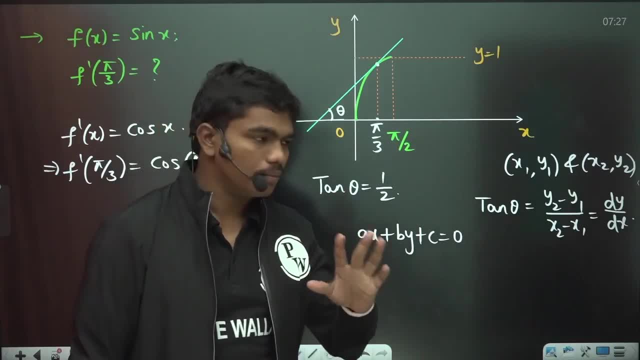 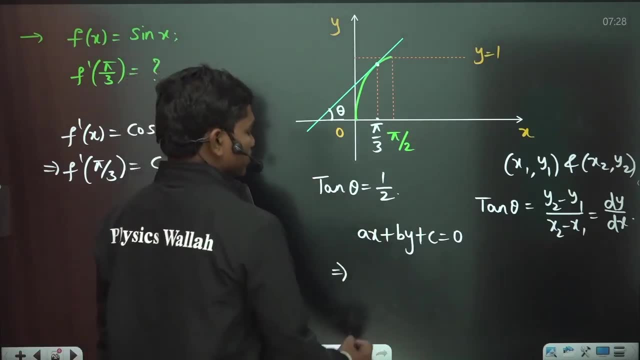 minus A by B or minus B by A. There is always some confusion in your mind, but you can simply tell this. So, as I told you, slope is nothing but derivative. Let us differentiate this function with respect to X. Why we are differentiating with respect to X? Because Y is the dependent. 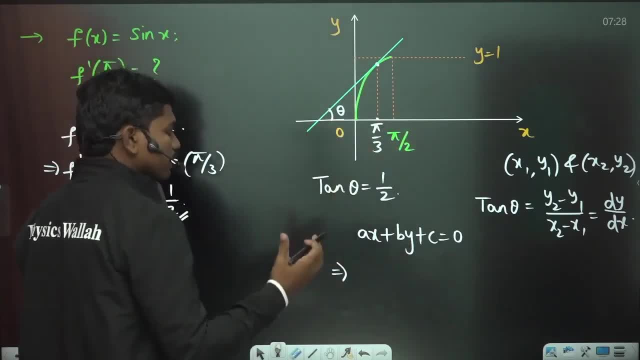 and X is independent. Theta is with respect to X axis, So that's why we need to differentiate with respect to X axis, X, Okay. So if you differentiate this function with respect to X, A into derivative of X, Y is the derivative of X. Okay. So if you differentiate this function, 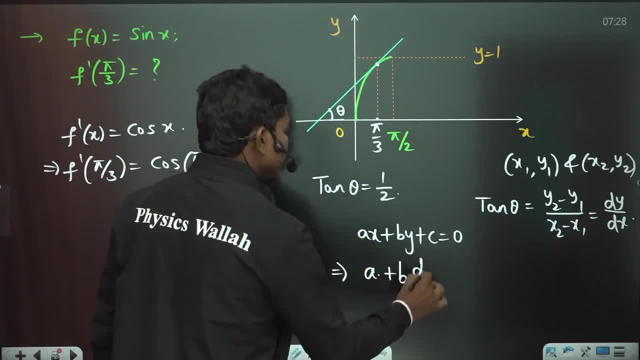 with respect to X. with respect to X is 1 plus B. into DY by DX, Differentiation of a constant is 0.. So is equal to 0. So DY by DX is equal to minus A by B, minus A by B. So this is the. 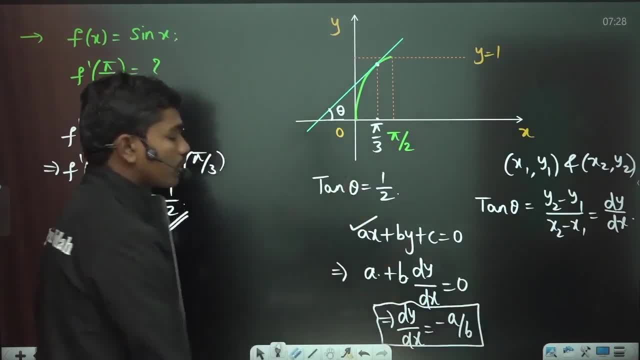 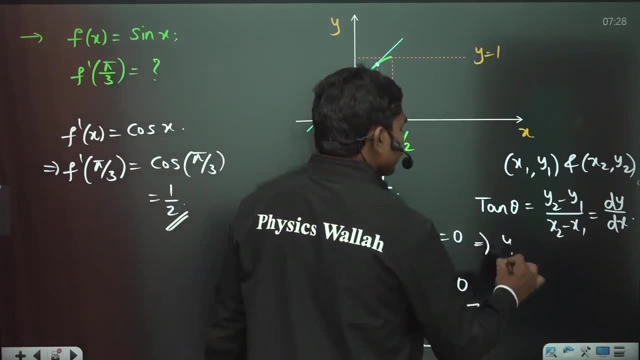 slope of this linear equation, Okay, And also if you can convert this, and of course, without the differentiation. also, you can tell how you can convert this equation into Y equal to MX plus C form. Okay, So then you know this. M is the slope. If you convert, let us see what happens. 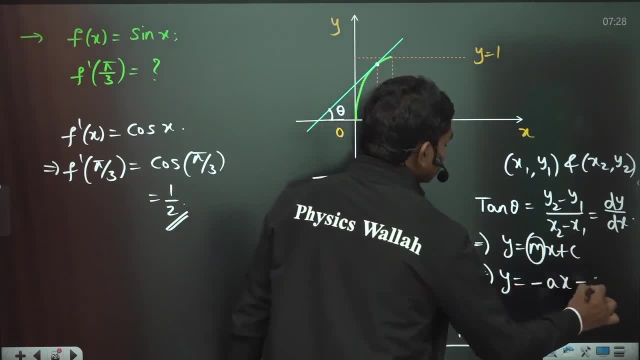 Y is equal to minus AX, minus C by B by B. So Y can be written as minus A by B into X, plus minus C by B. Okay, So you can see. this is the slope minus A by B, which is the same. 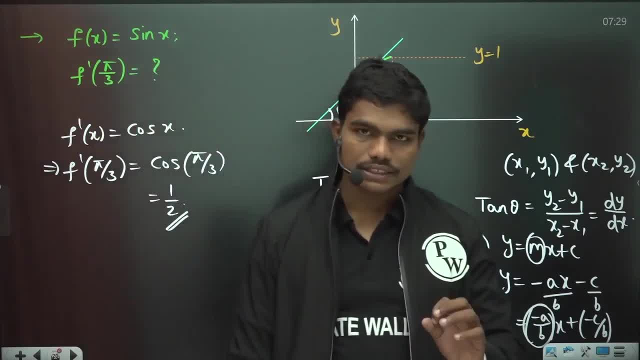 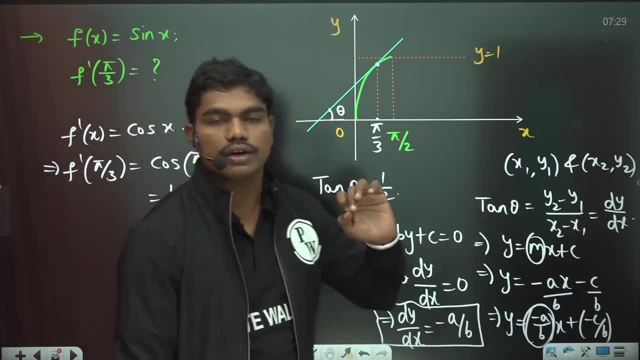 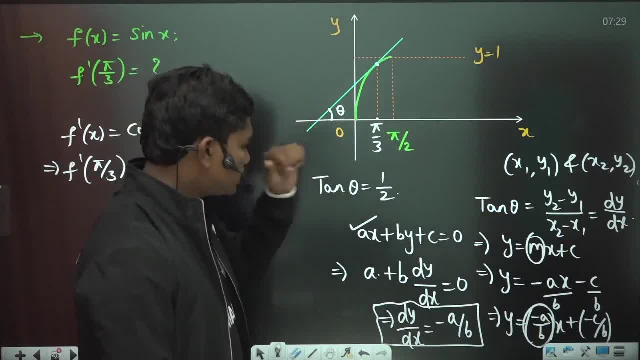 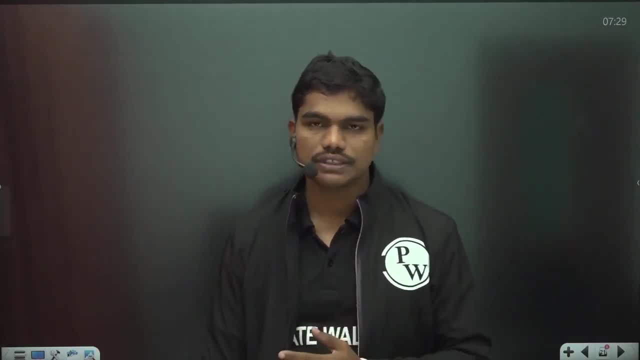 this is how we got the slope. Okay Now, anyhow. so straightaway, let me give you some very important formulas of differentiation. Then we will go for limits once again. Okay, Because why you need differentiation formulas for solving limits is in limits. we have something called. 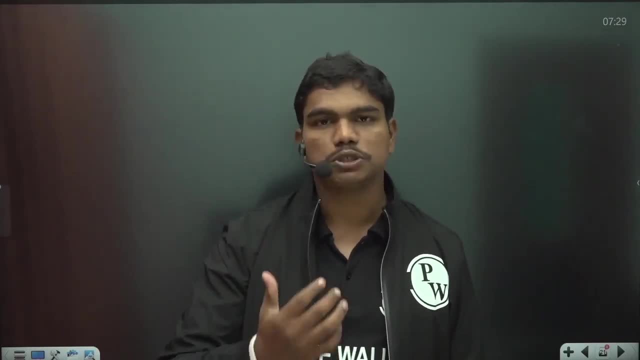 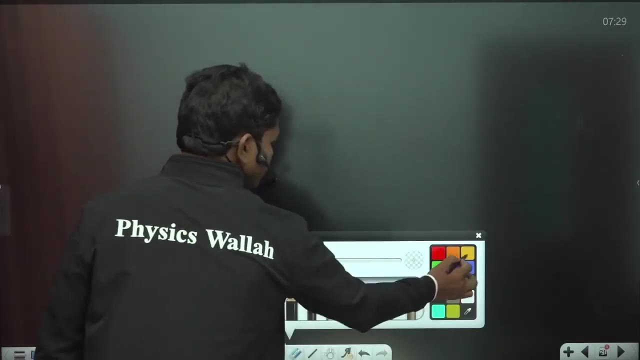 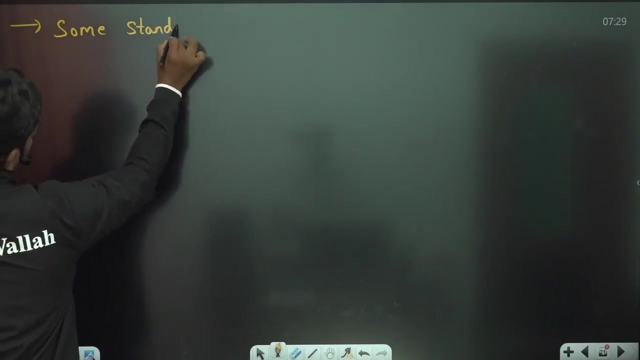 L-hospital. So okay, So we actually need some differentiations of the functions when applying L-hospital, So that is why we will go for some standard differentiations in the beginning. Okay, So some standard derivatives Which many of you generally might know. So, some standard derivatives, Some standard. 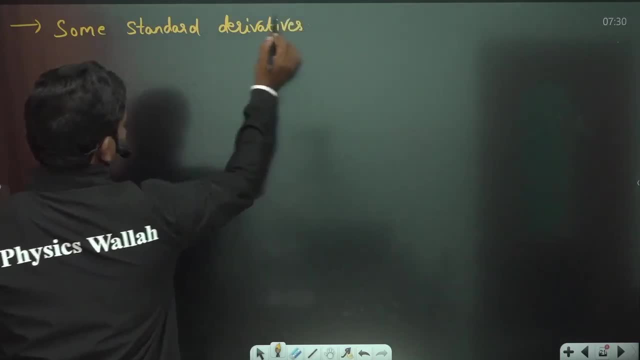 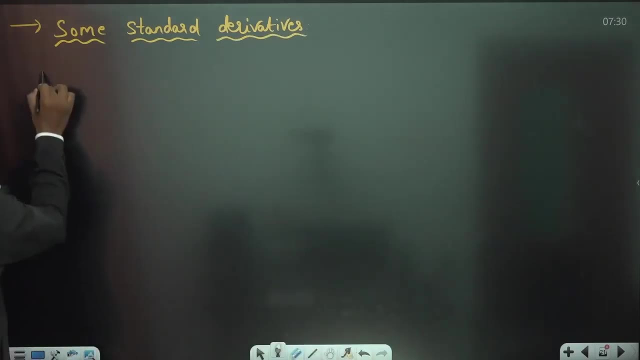 derivatives, Some standard derivatives. Let us see What are these. First, let us start with algebraic function: d by dx of x, power n is equal to n times of x to the power n minus 1.. Okay, So we can substitute whatever the value of n is there. 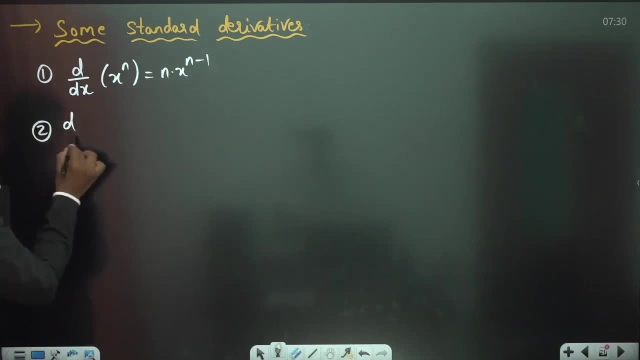 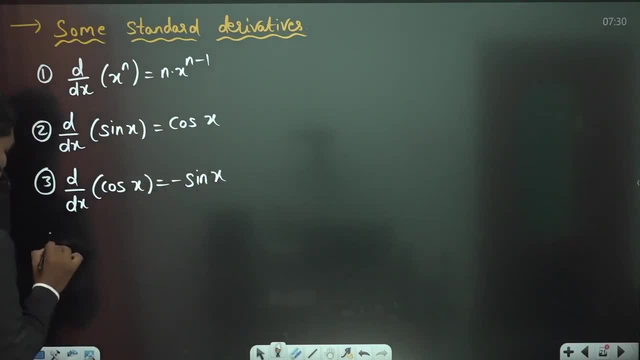 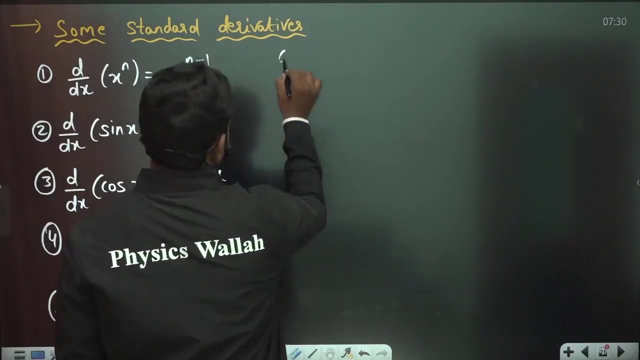 is minus sine x derivative of tan x. Second square x derivative of tan x. Next, d by cot x minus cosecant square x, minus cosecant square x, then 6, d by dx of you know secant. 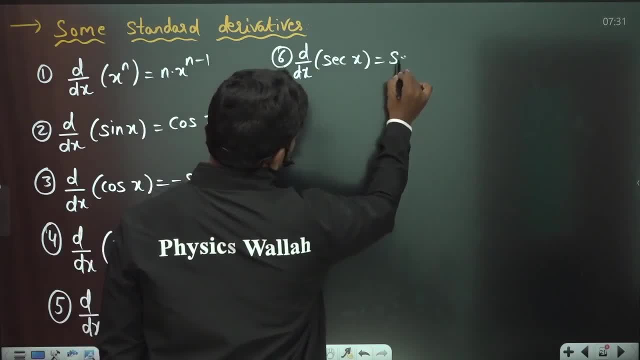 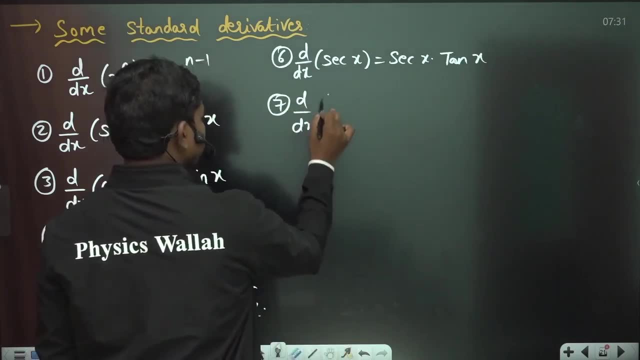 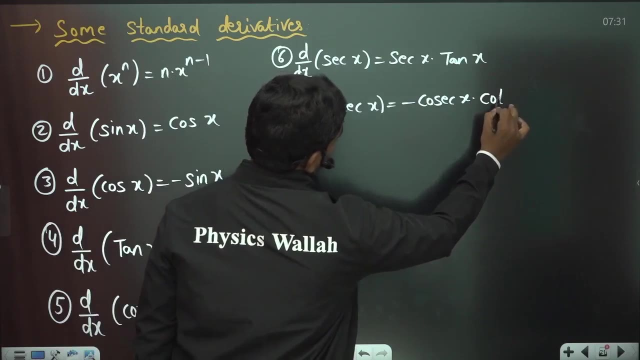 x. you can say secant x, which is secant x, into tan x, then d by dx of cosecant x, cosecant x- this is minus cosecant x- into cortex. okay, so this is what we have. 8, so basically these: 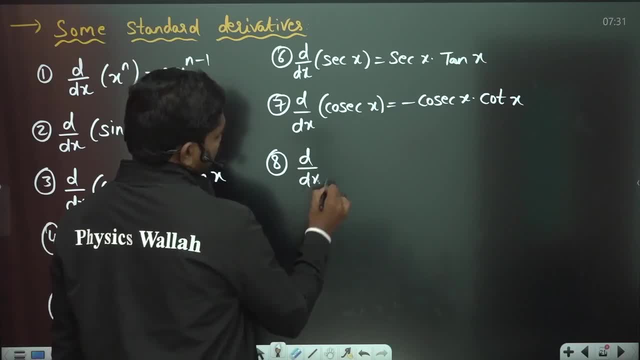 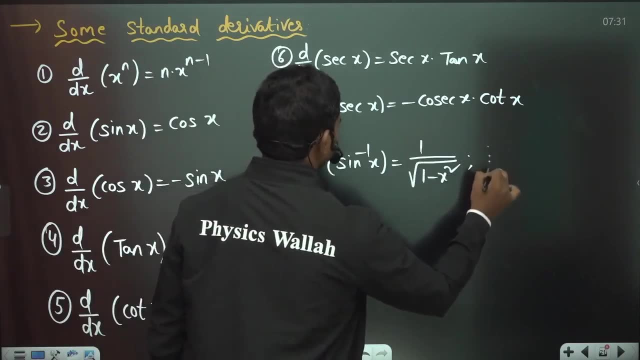 6 trigonometric functions got finished, let us go to inverse trigonometry: d by dx of sine. inverse x is 1 by root of 1 minus x square. and of course you know mod x is less than 1 in this case because if obviously sine cannot take any value between, you know any. 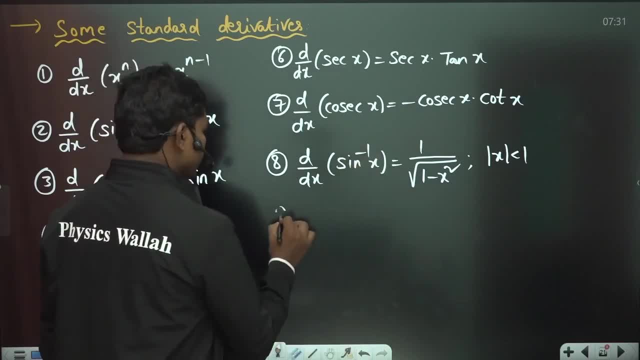 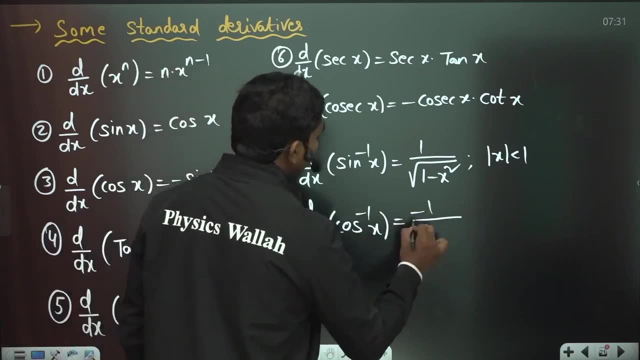 values out of plus and minus 1, so that's why mod x is less than 1, similarly here, d by dx of cos inverse x. this is minus 1 by root of 1 minus x square. similarly here also mod. 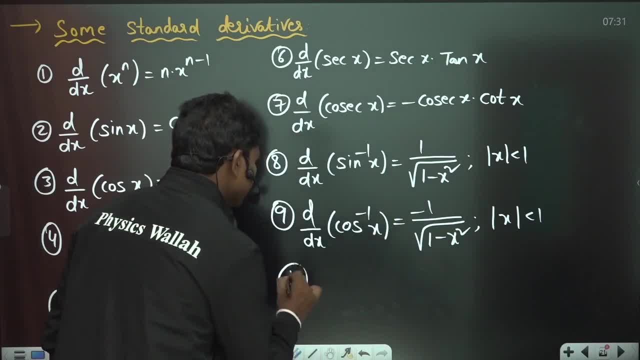 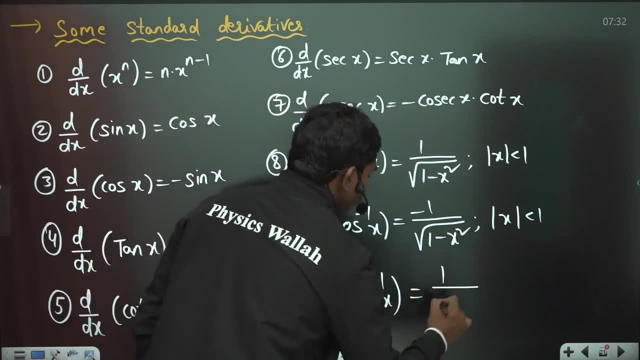 x is less than 1, now similarly 10,. d by dx of tan inverse x, d by dx of tan inverse x. this is 1 by 1 plus x square. and how many formulas? I have given you some 10 formulas. 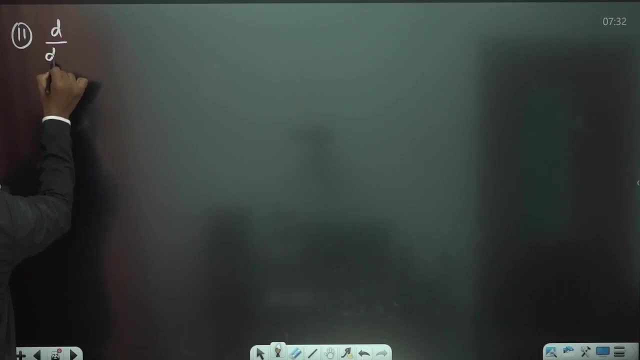 okay, 11,. d by dx of cot inverse x. d by dx of cot inverse x is minus 1 by 1 plus x square. 12,. d by dx of secant inverse x is 1 by mod x into root of x square minus 1, and of course, in this case you know mod. 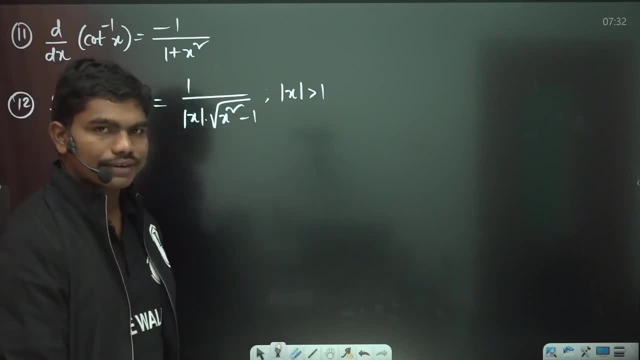 x is greater than 1, because cos always lies between plus and minus 1, so definitely secant will go out of plus or minus 1, always. so 13th d by dx of cosine inverse x divided by mod x into root of x square minus 1, so this is X minus equal to minus 1, and of: cause, if we apply this crossing here independently, of course, in this case, if x and minus 1 do the same, this can be thought of as d by dx of cot inverse. x, number of times, y, x squared of x is less than 2 minus y, and if we apply it, this comes as d dot zm are d by dx of cot inverse. 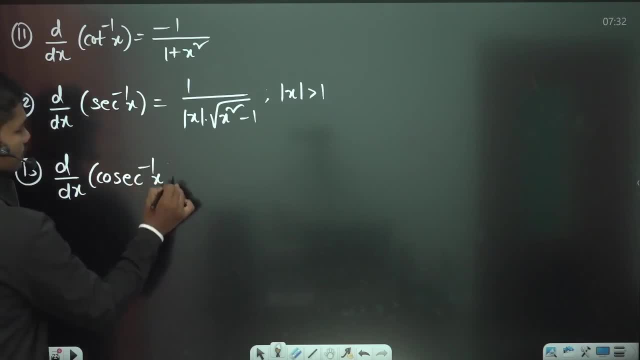 secant inverse x. sometimes generally secant inverse and cosecant inverse are very rarely asked, but still it's good to have them. x square minus 1 mod x greater than 1. okay, so now coming to some exponential functions: d by dx of x power x. if you take this is x power x into 1 plus log x. 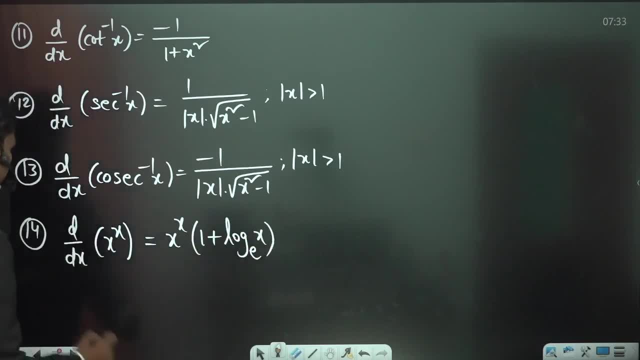 to the base e. okay, so 1 plus log x to the base e. 15th, d by dx of e, a power x, for example. so this is a some constant, so a power x into log a to the base e is what you have then. 16th, 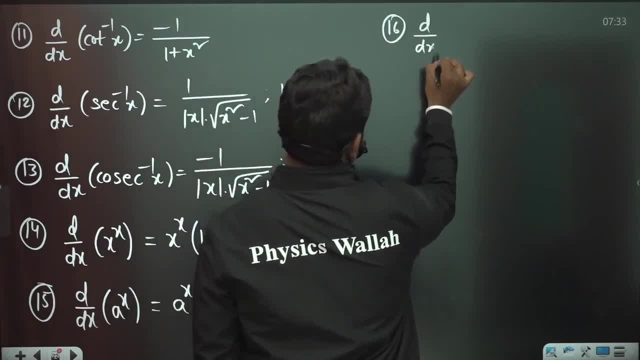 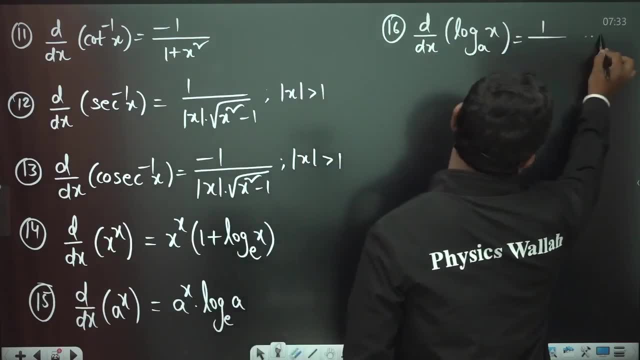 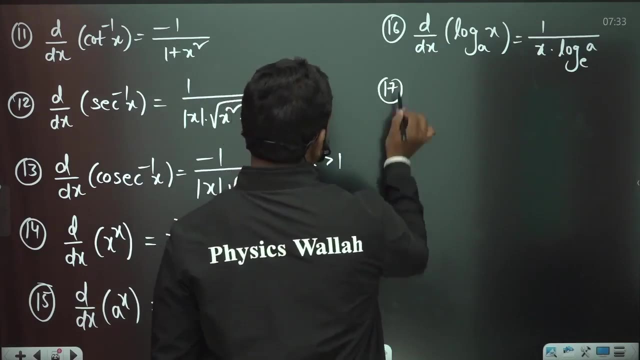 d by dx of log x, log function generally. so log x to the base a, if you take 1 by x, 1 by x times log x to the base e, a to the base e is what you have. okay, so 17th. so definitely, if you keep e power x here, you will get. 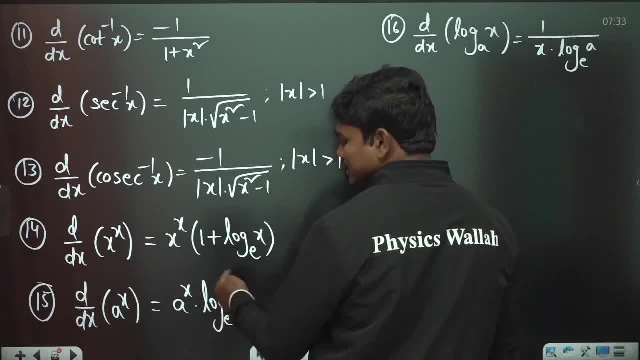 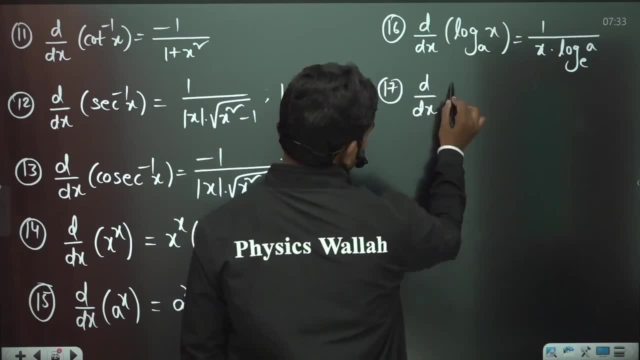 e power x into log e to the base, e, log e to the base, e, log of anything to the same base. if these two are equal, then log value is 1. so that's how differentiation of e power x is e power x and differentiation of, you know, log x to the base e. natural logarithm, if you take this, is 1 by x. 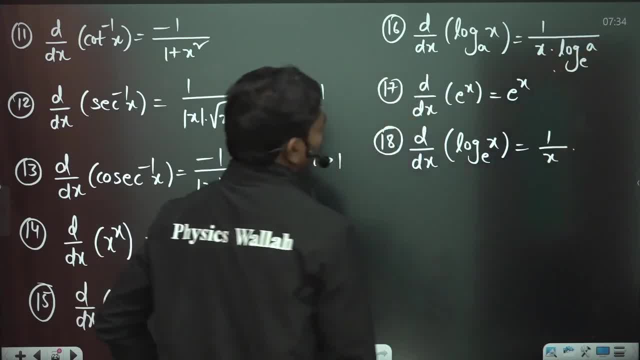 because this log x to the base e, log x to the base e, if you take this, is 1 by x. because this log x to the base e, a to the base e value turns out to be 1 in that case. okay, so generally these are some normal. 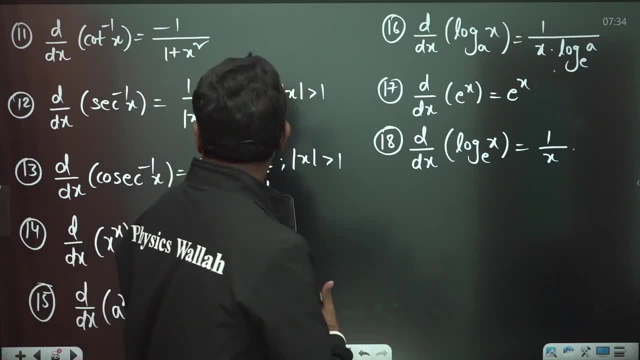 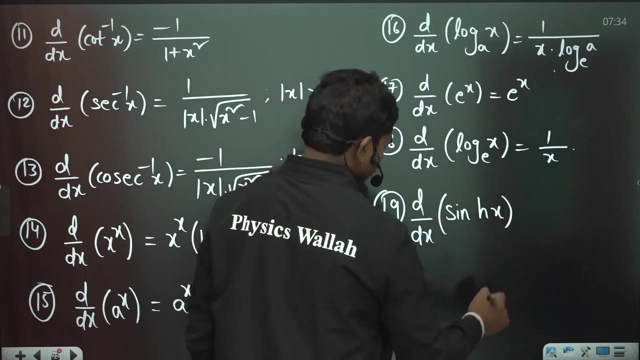 formulas that you will be in need of, for you know this- differentiations derivatives in general in this course: okay, so that's why i have given you so. similarly, if you say hyperbolic functions d by dx of sine hyperbolic x, okay, so this sine hx is nothing but cos hx. okay, so what are these? 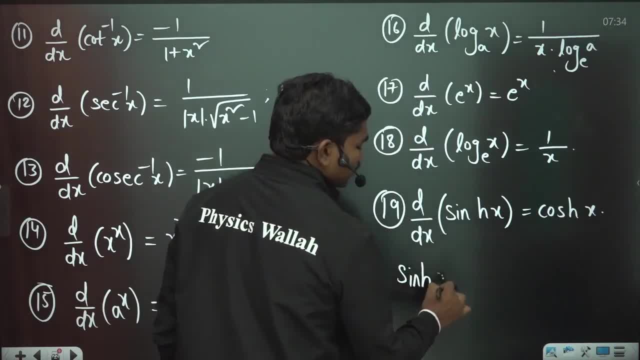 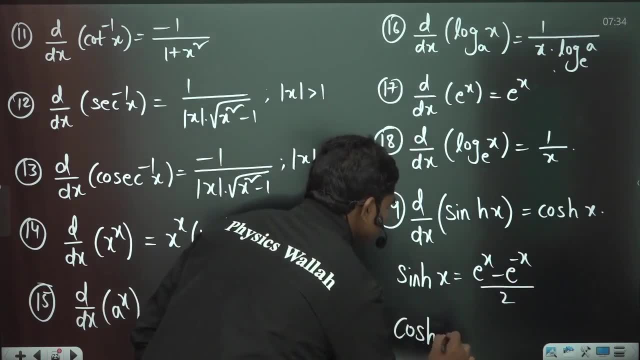 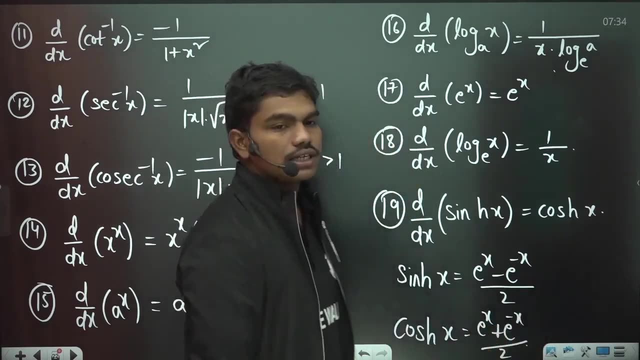 hyperbolic functions. basically i'm just giving you the formulations, but practically they have very big significance: e power x minus e, power minus x by 2 and cos hx is e power x plus e power minus x by 2. okay, so that's how you have the hyperbolic functions defined, actually. okay now. 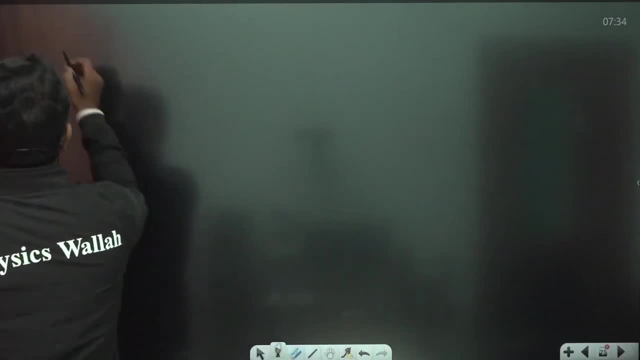 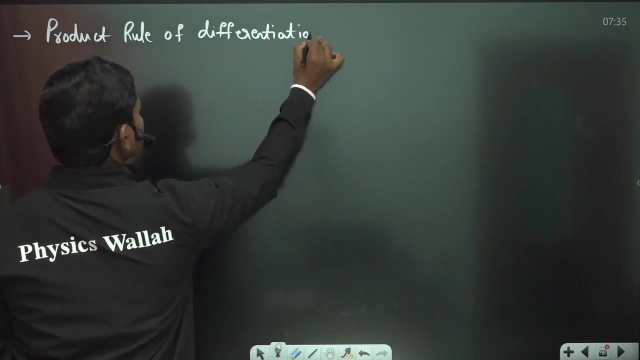 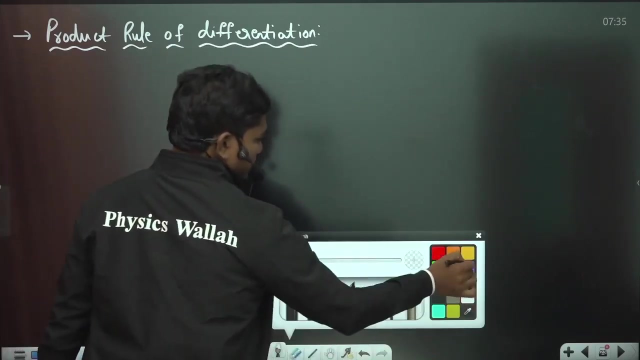 i'd like to give you two, uh, you know, one important tool, which is product tool of differentiation, which is again known to you product tool of differentiation, or sometimes you call this as uvool. okay so, product tool of uvool differentiation, product tool of differentiation, product tool of differentiation. so, basically, if you have two functions, for example, okay so. 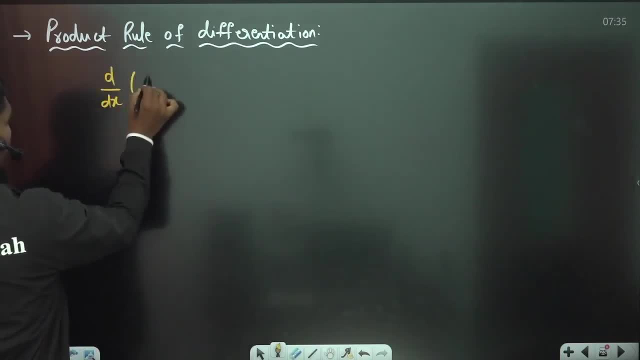 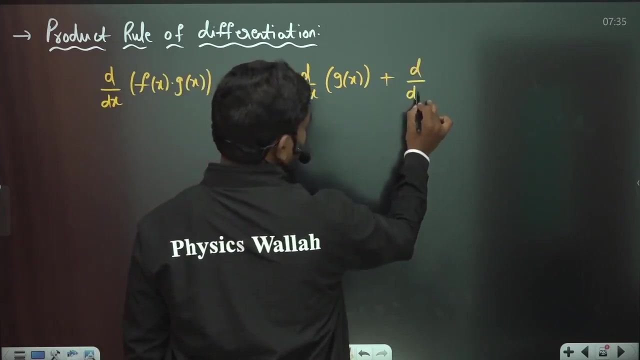 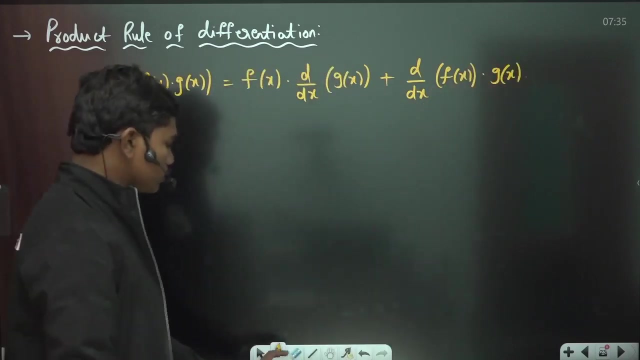 let us write d by dx of f of x into g of x. so this is first function into differentiation of second function, d by dx of g of x, plus differentiation of first function, d by dx of f of x. okay, so this is how we have, and you have the division rule, also quotient tool, so let us write that as well. so, because these are just fundamentals, majority of this chapter you might have found in your plus. 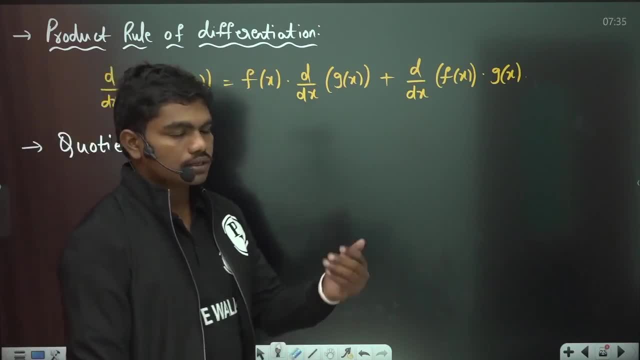 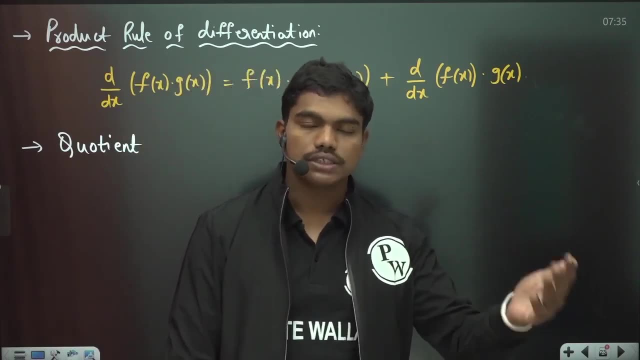 one plus two levels, but of course we will also teach some advanced things. but, uh, once you know some good you know, uh, if you know this chapter in a good way, then definitely this will help you further. further chapters like differential equations, vector calculus, complex calculus, all this you know chapters, okay. so anyhow, let us see quotient tool of differentiation, because that is more especific. for this we will dirty 달�et these and other sections of the hơnertottворke. 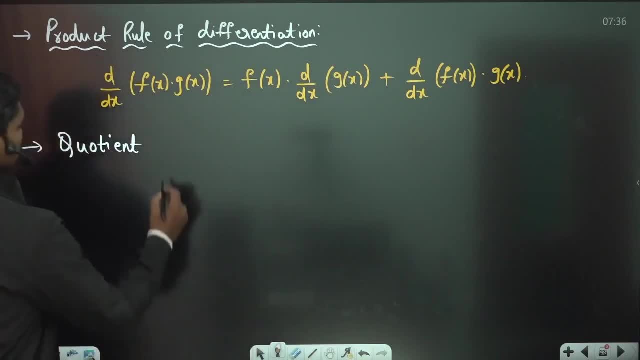 delta calculus, complex calculus, all these you know, uh, chapters. okay, so anyhow, let us see quotient tool of yea or Non2, the P trap entry and other details. pt vector calculus, complex calculus, all these you know our chapters. okay, so anyhow, let So, anyhow, let us see quotient tool of differentiation. quotient tool of differentiation, so quotient. 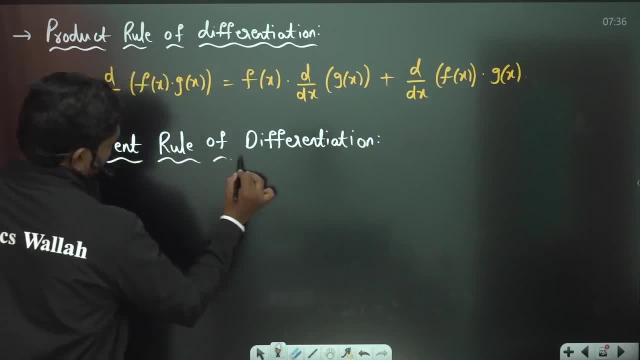 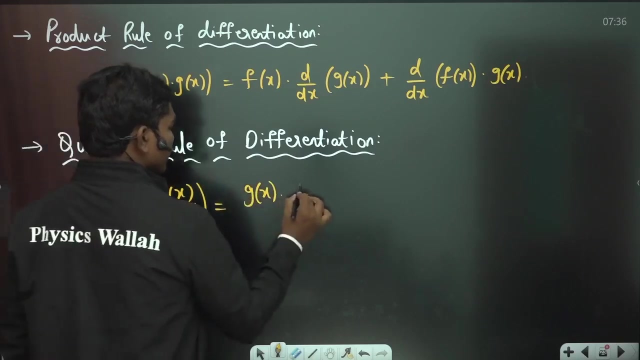 tool of differentiation, quotient tool of differentiation. So if you take the ratio of two functions, d by dx of f of x by g of x, if you take out, then this is: g of x into f, dash of x minus f of x into g, dash of x divided with divided. 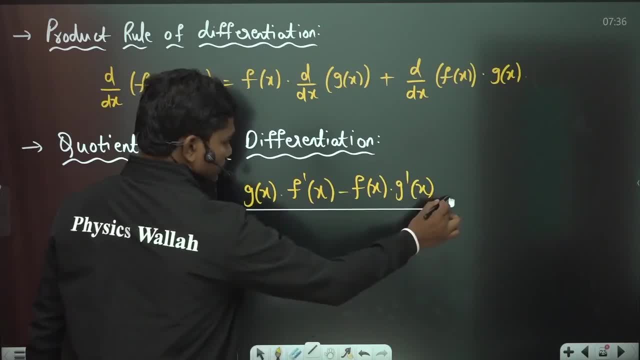 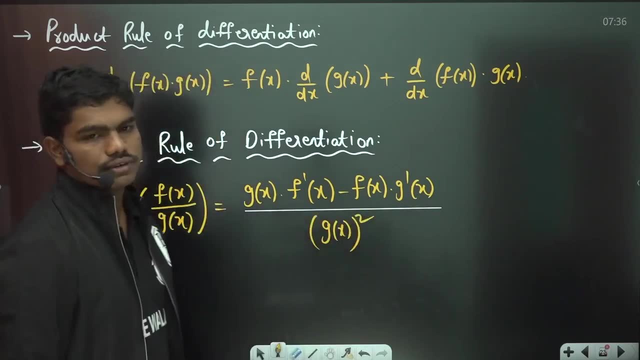 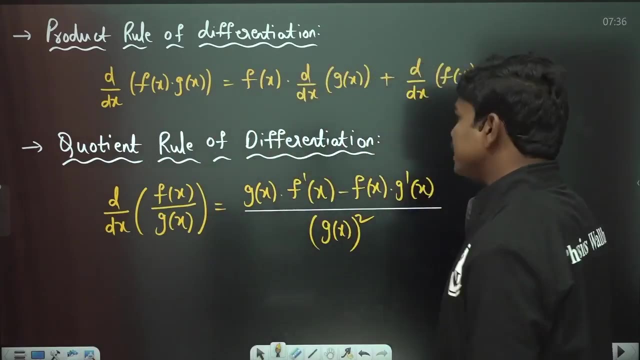 with this, divided with g of x, whole square. okay, because we will be using these expressions after some time, so that is why you know I am giving you this, okay. So quotient tool of differentiation is basically this value. Now let me. 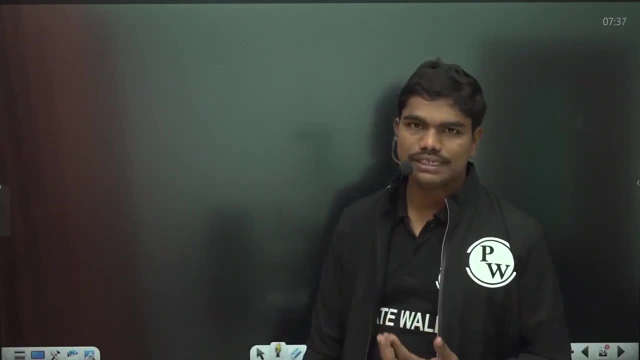 So we have got idea on some differentiations. so let us try to see some limits. okay, because we have just seen the definition of limit, but there are some important, you know points where we will use these derivatives in limits. okay, but before that I would like to give. 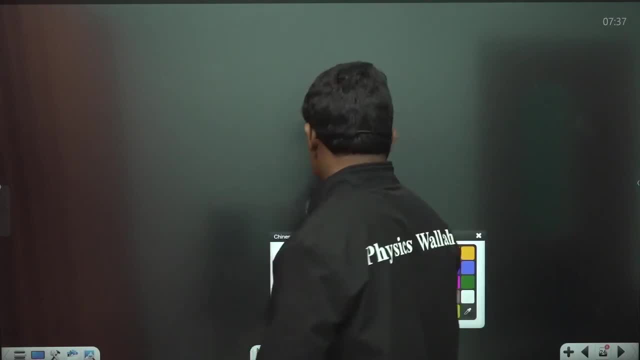 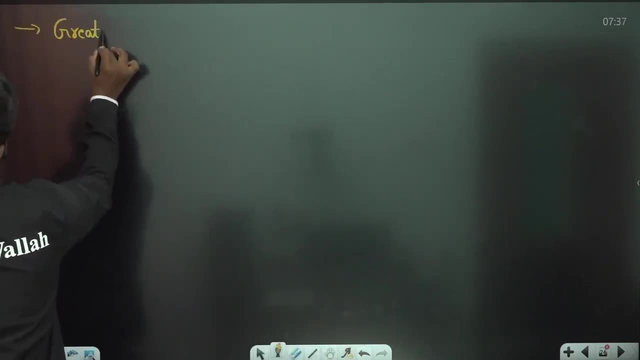 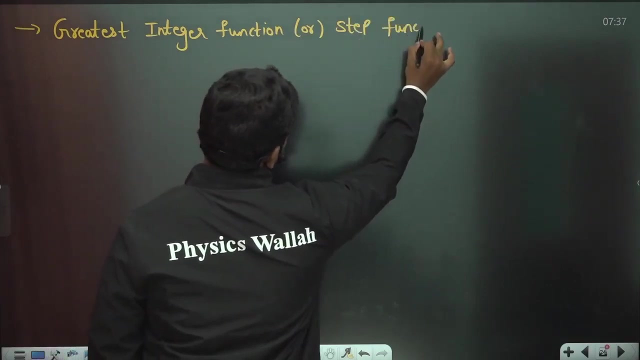 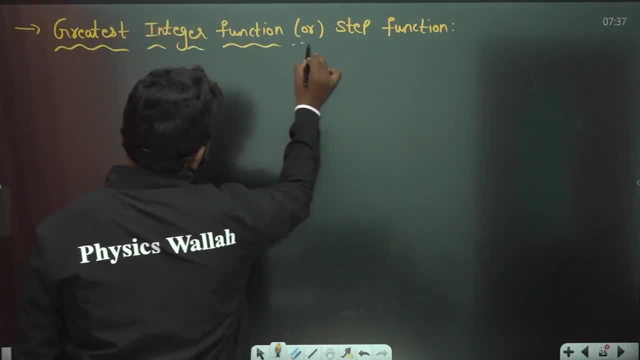 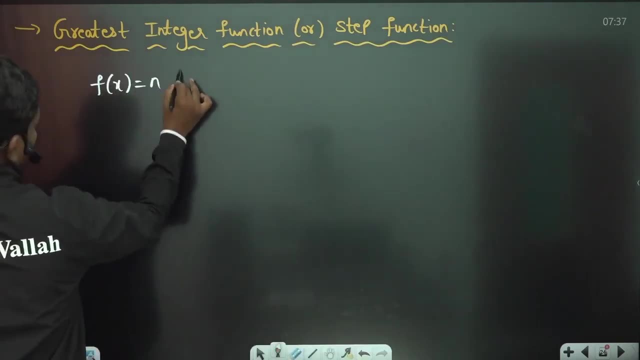 So how this function is defined. Let us see or step function. so how this function is defined. f of x is equal to n for all x, n less than, or equal to x less than n plus 1,. please make a note. 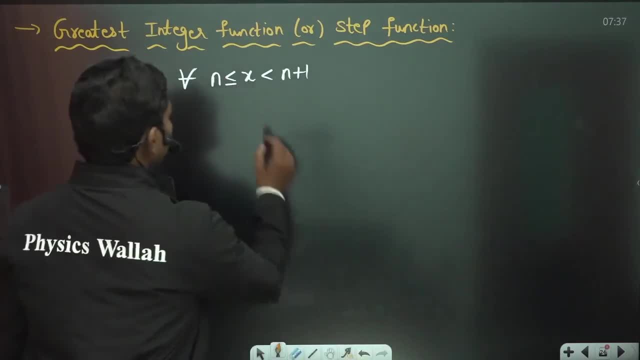 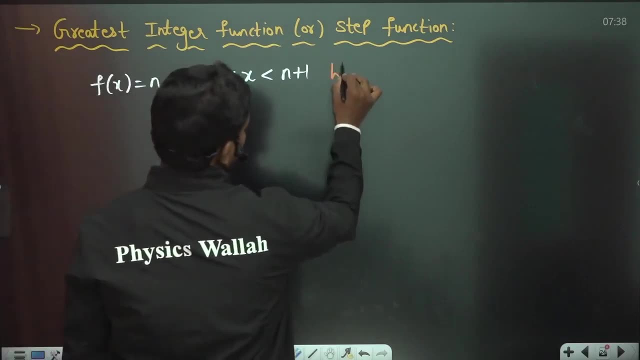 Here. This is the equality sign. okay, If you want, I will highlight this equality with a different color as well. So this equality sign is not here, okay. So where n is some integer, where n belongs to z, n is some integer actually, okay n. 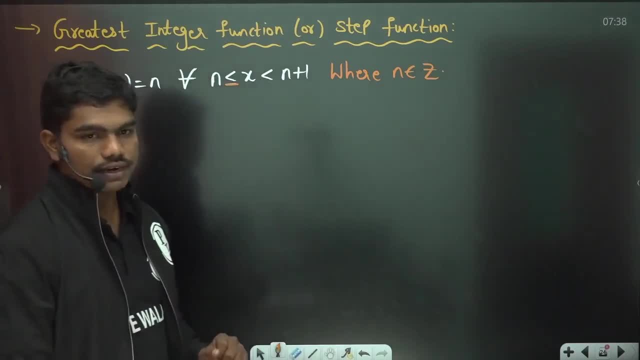 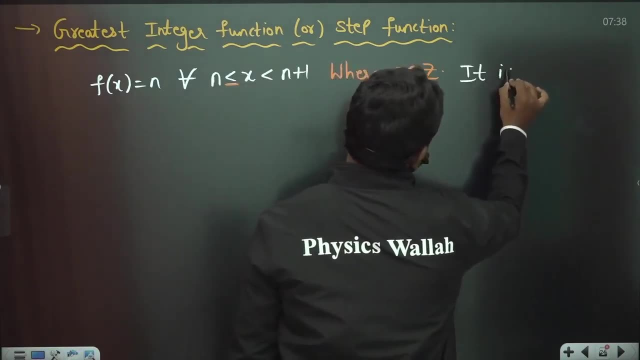 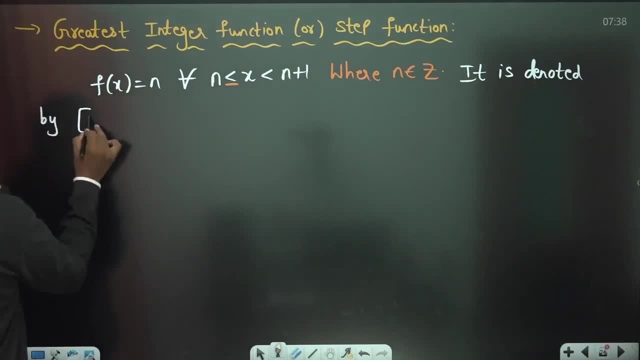 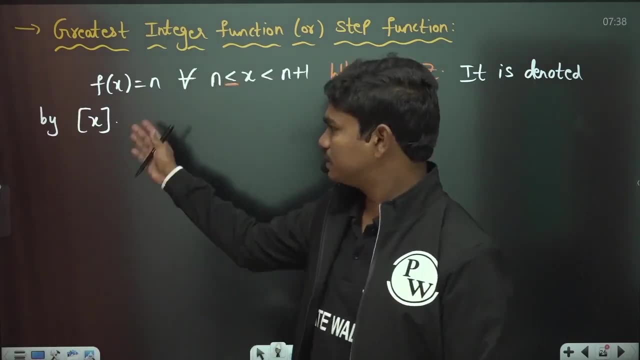 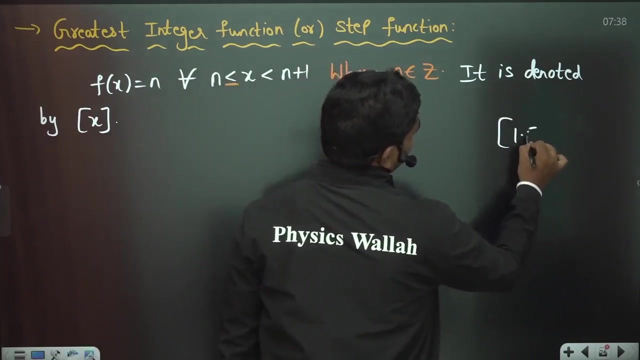 is denoted by Okay, This symbol: square brackets on x. okay, So integer part x is basically defined by this. integer part means basically this: x with the square brackets on both the sides. okay, Now how we actually see this. for example, if I take 1.542, for example, you know this. 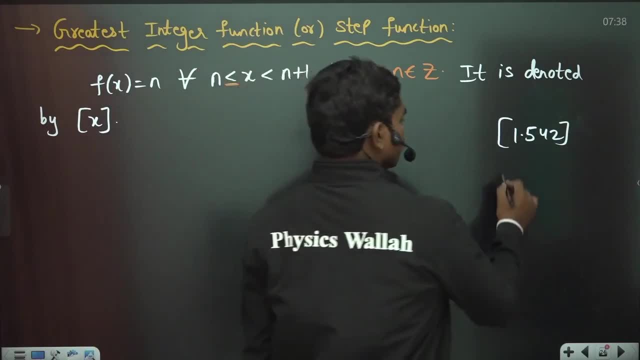 1.542 is in between two integers. What are they? 1 and 2, correct? So 1 less than 1.542 less than 2.. So this is n, this is n plus 1.. So definitely. 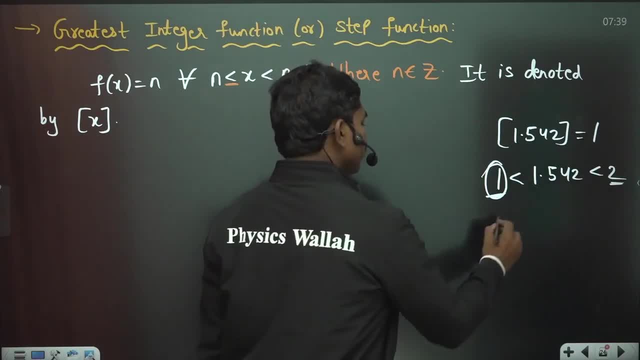 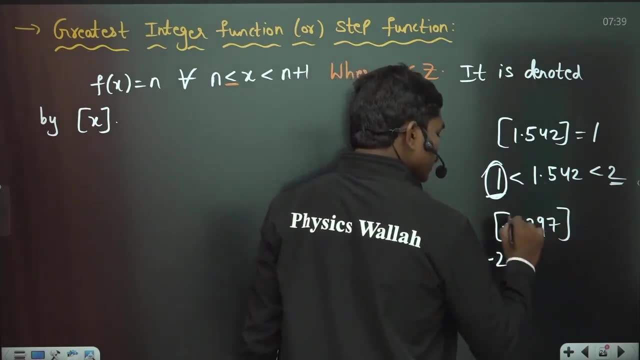 This value is equal to this n value which is here, which is 1.. Similarly, if you take minus 1.297, something like this, then you can see this value is nothing but minus 2, less than or equal to or less minus 2, less than minus 1.297 less. 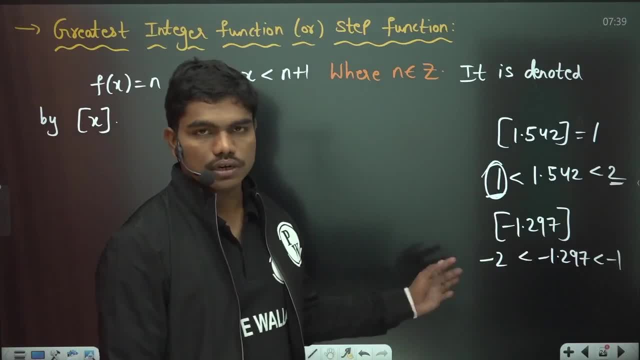 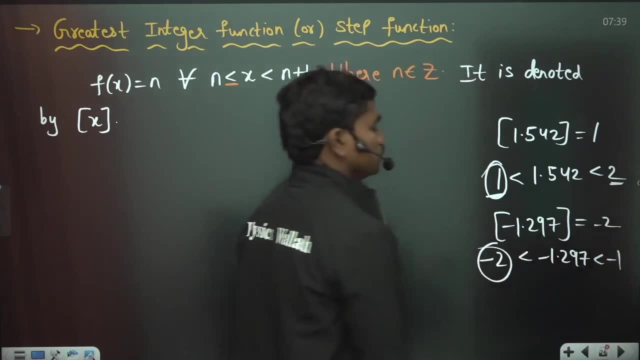 than minus 1.. Okay, Because you see, in negative numbers, as you go towards the left side, the values decreases. So minus 2 is less than this. So this is the integer vertex function. So this is minus 2.. So we need to write this: 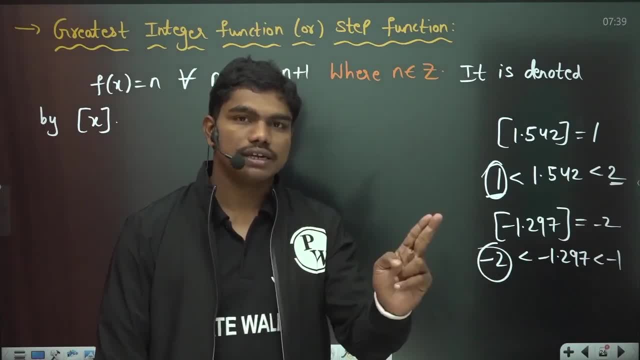 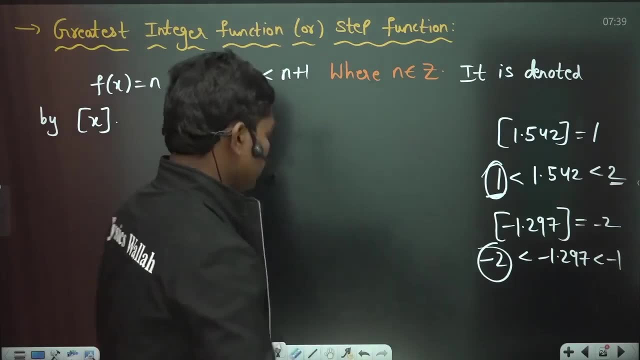 So, basically, whenever you take a real number, Okay, Which is left of that real number is the actual answer? Okay, And if the number itself is integer, then that itself, that itself, is the integer part value, Okay. So if you draw the graph of this function, look how it comes out, I'll tell you. 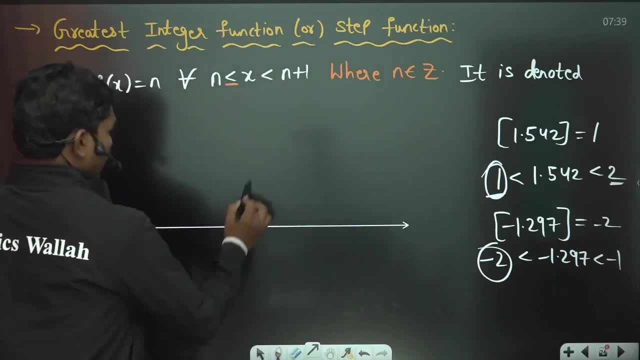 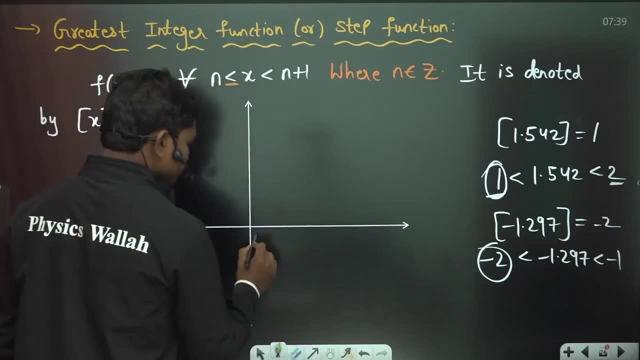 So this is your X axis, for example, and this is your Y axis. Let us say: this is your Y axis, This is your Y axis. So zero X minus X. Why? Why? because zero is equal to minus 1.. 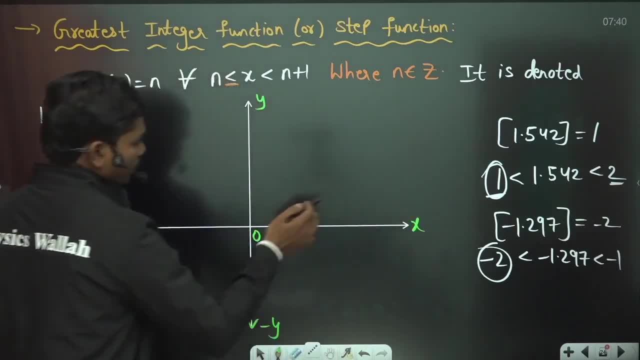 Great. So now, if you check this, let us divide this: X is equal to one, X is equal to two. all these values, Okay. So this is X is equal to one. This is X is equal to two. This is X is equal to two. 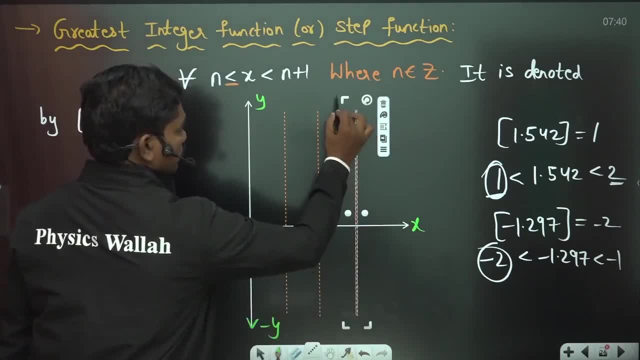 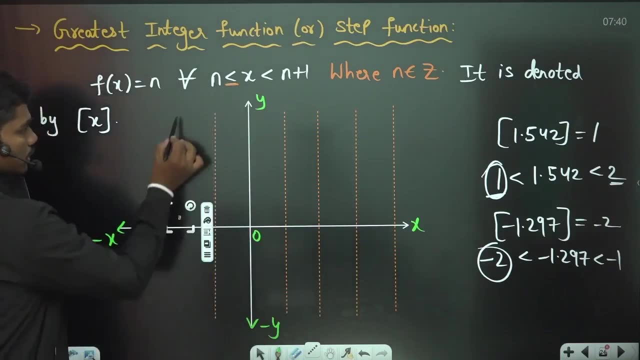 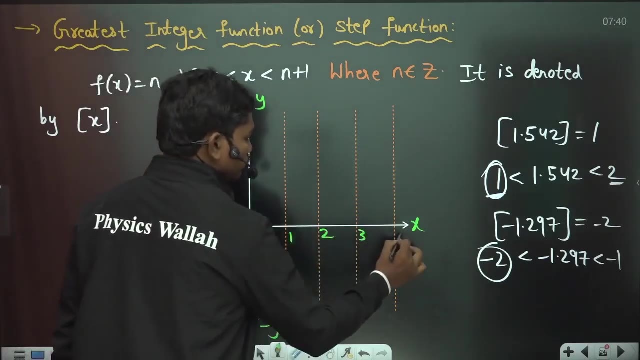 Okay, This is, X is equal to three. Okay, X is equal to three, And you have: X is equal to four, something like this. So X is equal to minus one is like this. Then x is equal to minus 2 is like this: So let us write the values 1, 2, 3, 4, minus 1, minus. 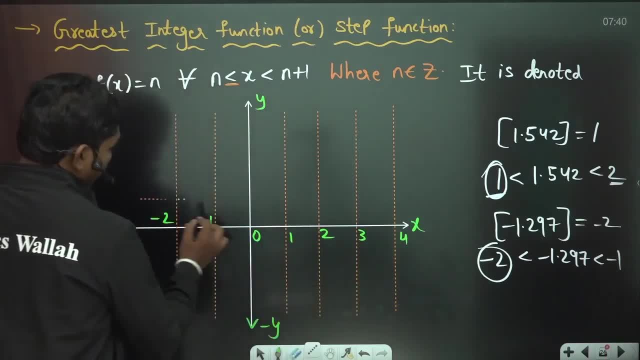 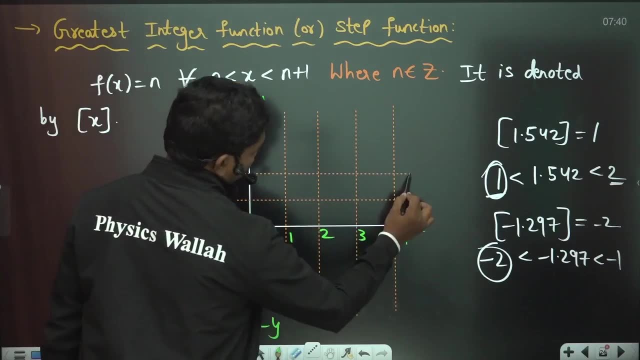 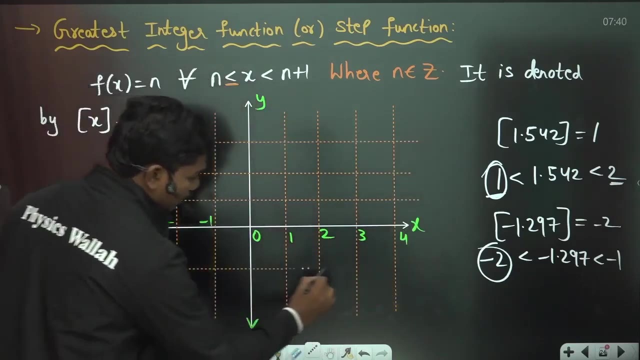 2 like this. Now let us also write: y is equal to 1, y is equal to 1. is this way: y equal to 1, y equal to 2, y is equal to 3,. we have this Similarly: y is equal to minus 1, y. 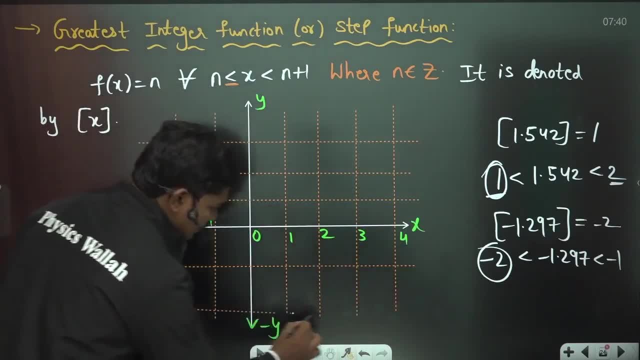 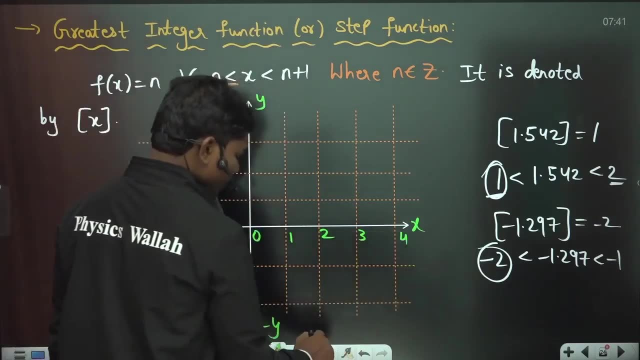 is equal to minus 1, and y is equal to minus 2,. y is equal to minus 2,. okay, y is equal to minus 2.. Now try to understand one thing. try to understand one thing. Let us suppose. 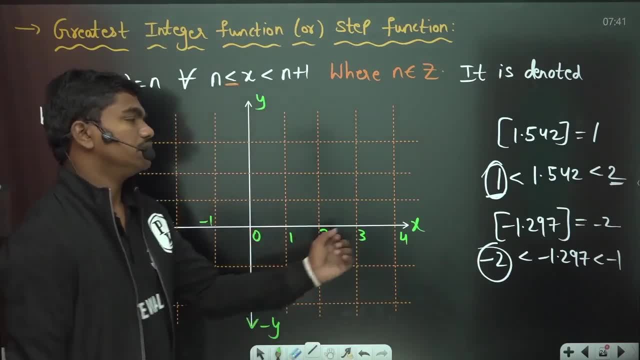 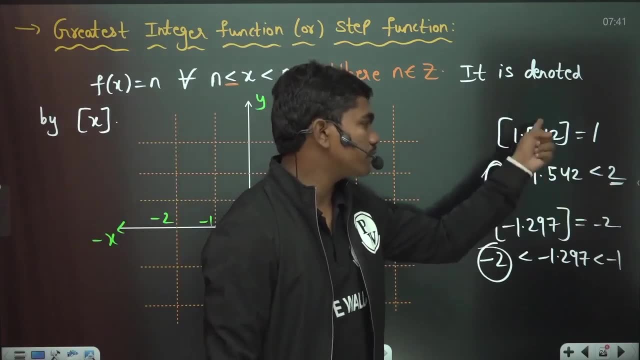 if my x value is lying in between 0 and 1, means if I take any value in between 0 and 1, the answer would be 0, correct. If I take 0 and 1, definitely integer part x value of. 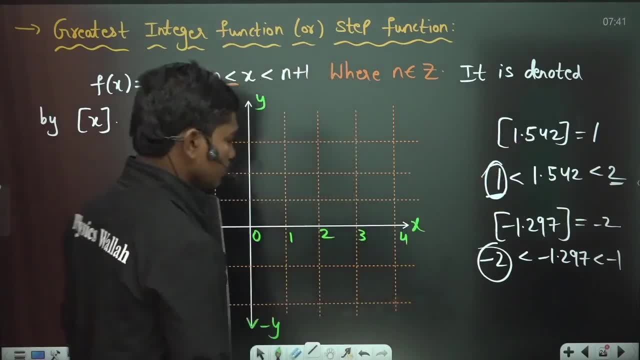 that any value which is in between 0 and 1 is going to be 0, means whenever x is changing from 0 to 1, the integer part x function is going to be 0. So if I take any value in, 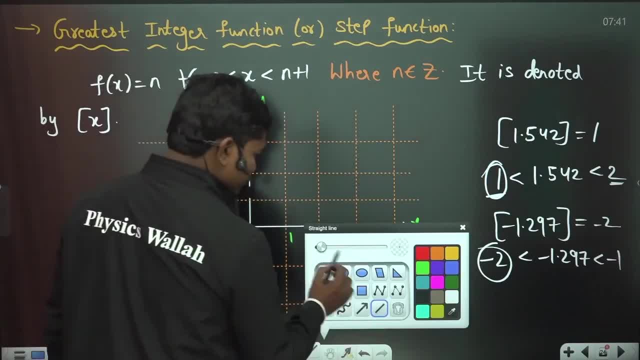 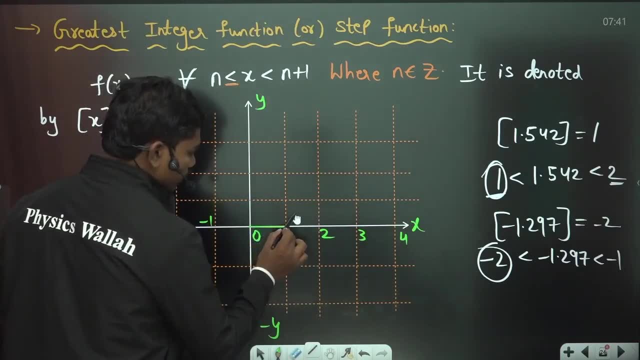 between 0 and 1,. the integer part x function is actually 0,. okay, So let me change the thickness slightly. okay, So now you see this is 0.. Now here you need to maintain one point very carefully: This graph should not touch this. x is equal to 1 line because 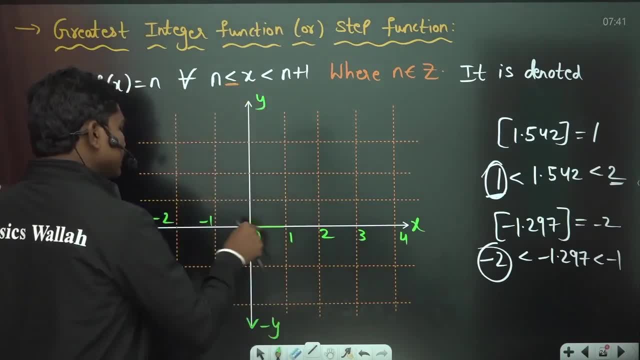 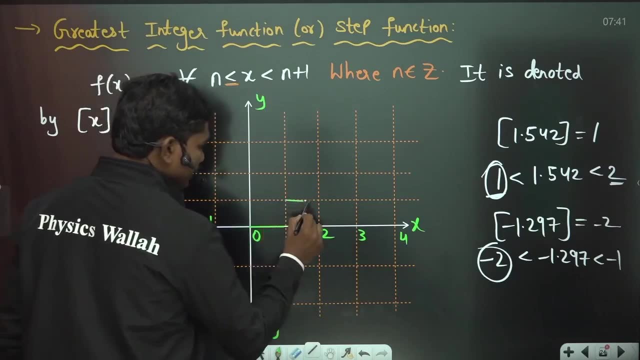 there is no equal design here, okay. So that is why this small green line which I have drawn here should not touch this. x is equal to 1.. Similarly, for any value of x between 1 and 2,, the value of integer part x is 1, actually, okay. Similarly between 2 and 3,. 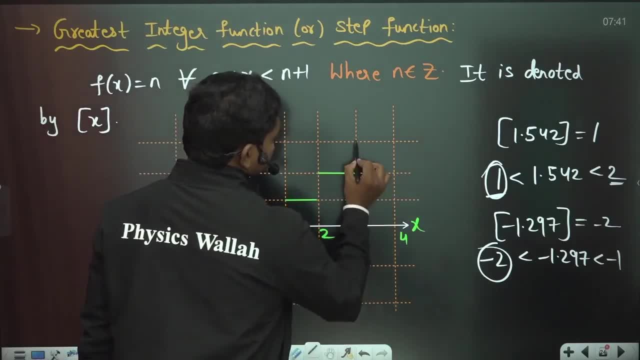 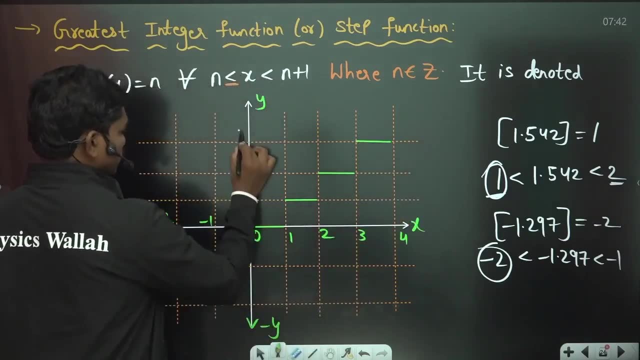 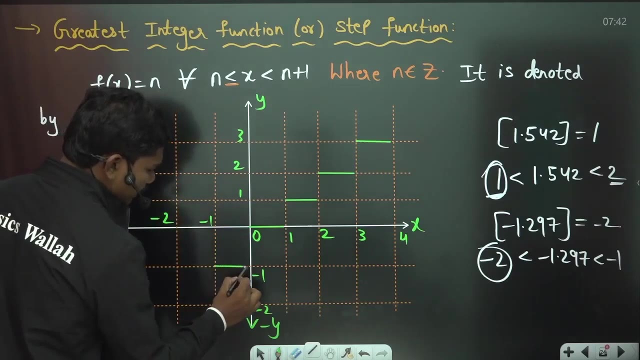 it is 2.. Between 3 and 4, it is 3.. So the green colored ones are the graphs here. okay, So 1, 2, 3, minus 1, minus 2, like this, okay, Similarly, here on the left side, it begins with minus. 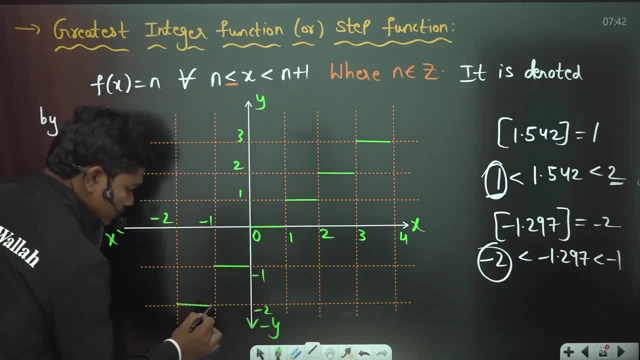 1 and it won't touch 0.. Similarly, here also, this is how the function comes out. okay, So this is the graph of integer part x function, and you can understand one thing: why this is called step function: because if you see, these are like a steps. okay, So that is. 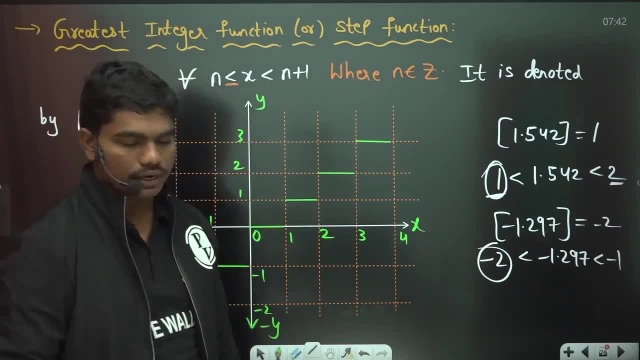 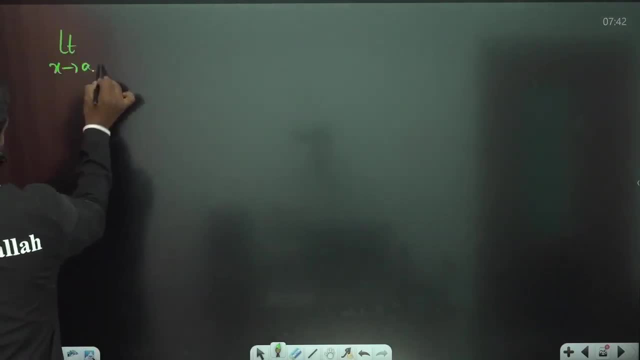 why it is called the step function. and one point, one very important point I'd like to tell you at this point: if I say limit extends to a integer, part x, this value does not exist if a is integer. if a is integer. 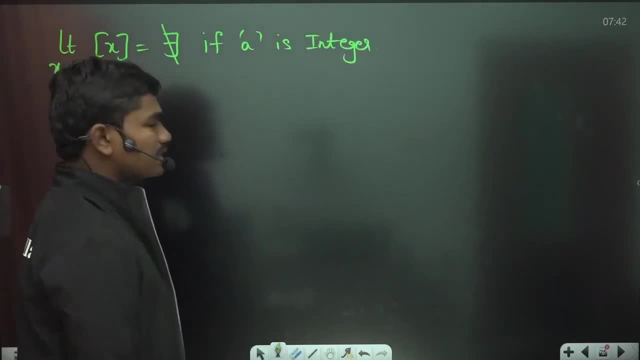 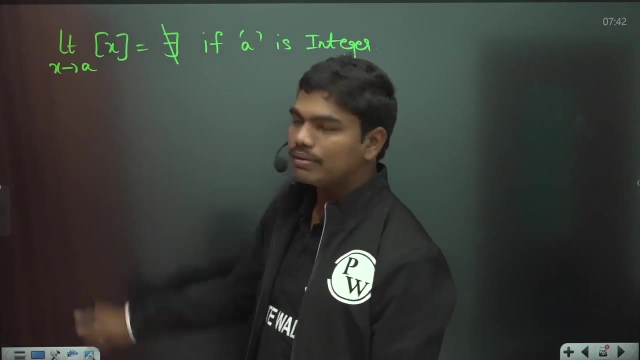 Now let us suppose, if a is not an integer, then definitely this limit will exist. okay, But why? this exactly means, if I keep some integer value here- 2,, 3,, 4, something like that- because you can see, you can see one thing: left limit if you talk about left. 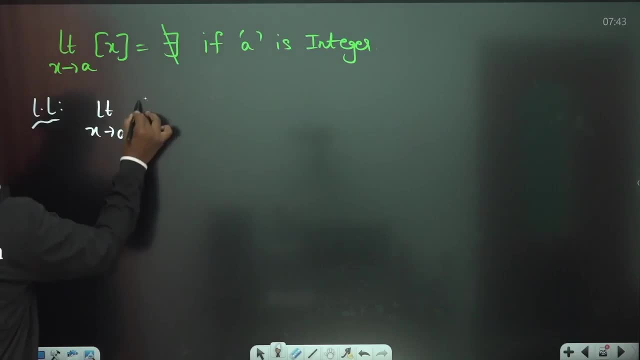 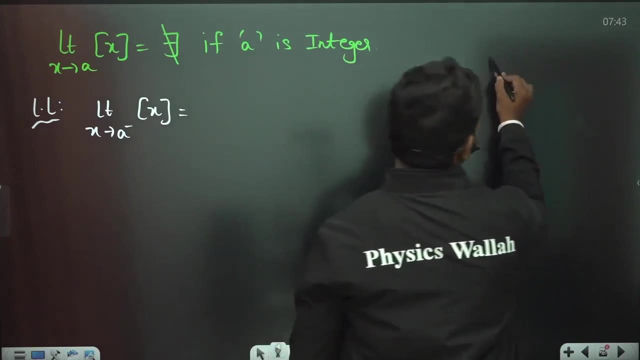 limit limit extends to a minus integer part X. so tell me one thing whenever I'm writing: extends to a minus X is more than a or less, than you look in neighborhood concept. I have told you: if this is your a, then this region, this region is your range of a plus and this region is the range of a minus, correct? 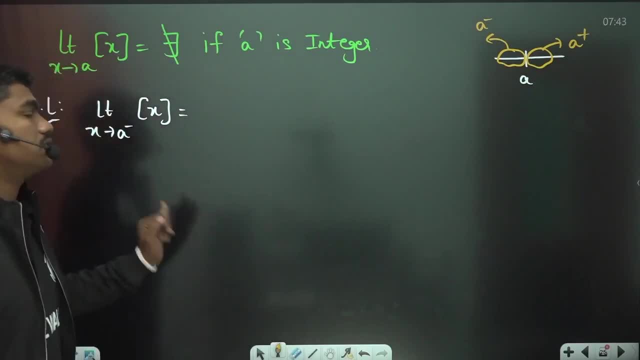 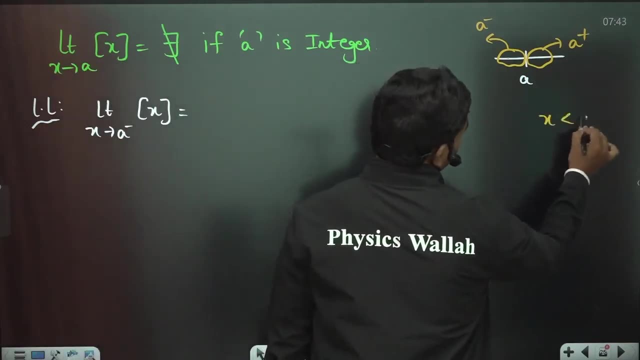 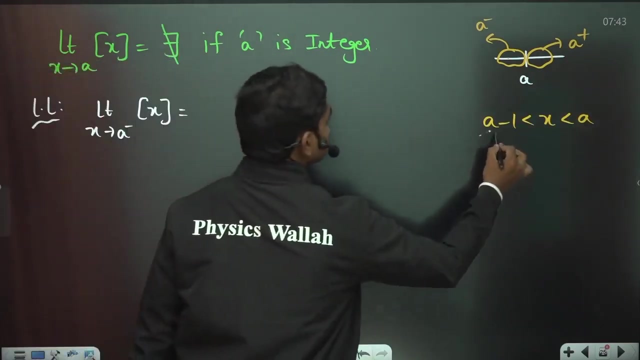 so, if you see, whenever I am talking about extends to a minus means X is somewhere here, which means X is less than a. now, whenever X is less than a, definitely X is less than a, which means a minus 1, something like this, correct. so whenever X is in between a minus 1 and a, then definitely. this is the integer part. 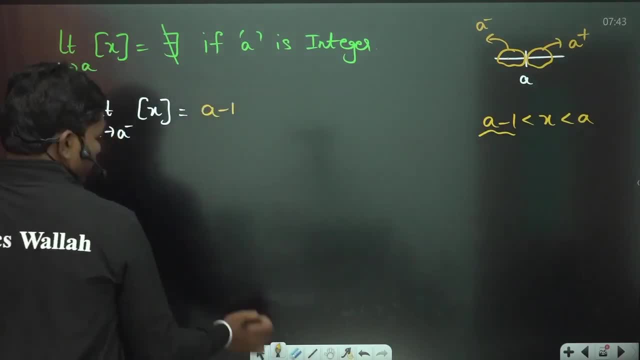 value of X. so this value is going to be a minus 1 and if you calculate the white limit, if you calculate the white limit limit limit, X tends to a plus integer vertex, intro vertex. so this, if you take now, X is in this range. so a is actually less than X, ok, so 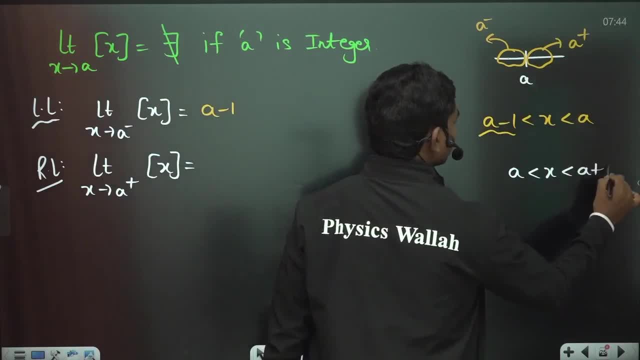 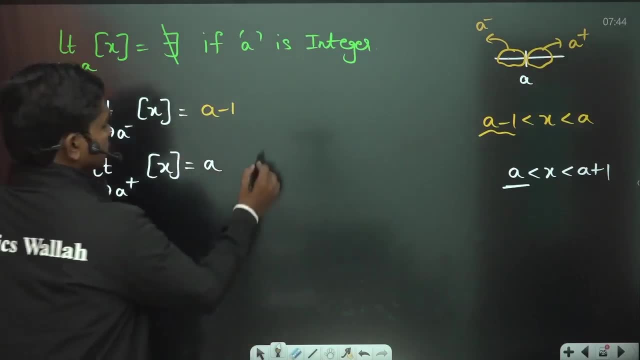 a is actually less than X, which means X is less than a plus 1, so in that case integer vertex value is capital. I mean the small a, and you know these two are not equal. so definitely this implies: limited has not exist, limit does not exist, limit does not exist as such limit does. 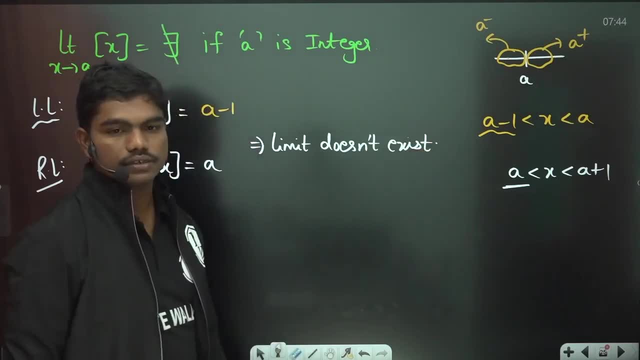 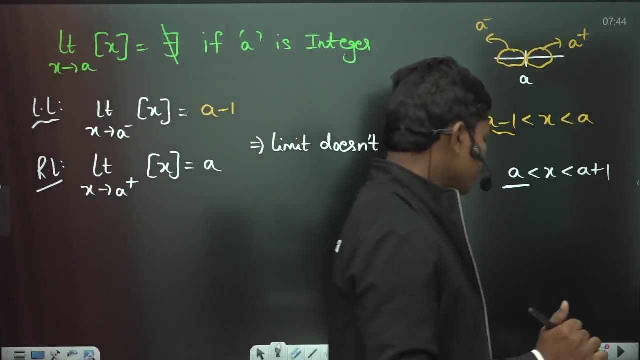 exist actually here. okay. so limit does not exist basically here. okay. so you see, whenever this is a integer, limit does not exist. but let us suppose if a is not an integer, then limit will exist. how look here? let us suppose if I take a point somewhere here, for example, let us suppose if I take a point. 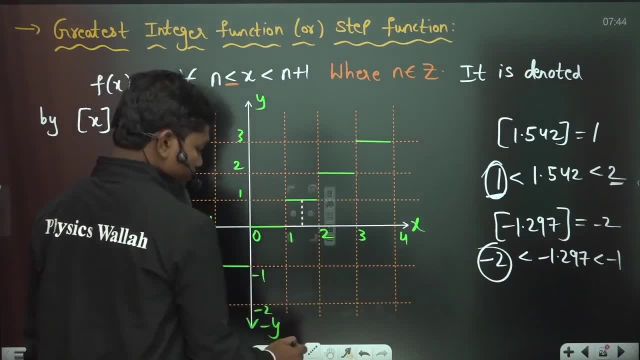 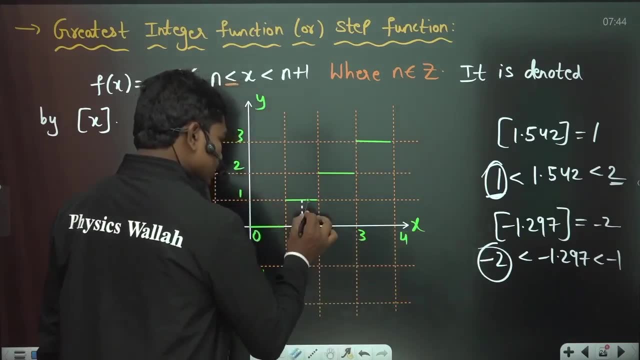 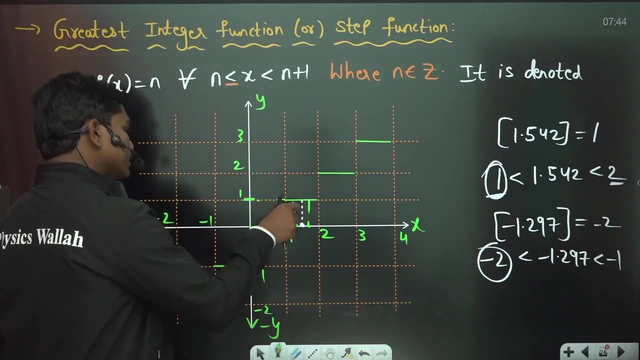 somewhere here, for example. okay, so at this point, at this point, at this point, on the right side and on the left side, in both the cases the function is same, it's one, and also here also, this is one. so that's how, whenever X is in between, 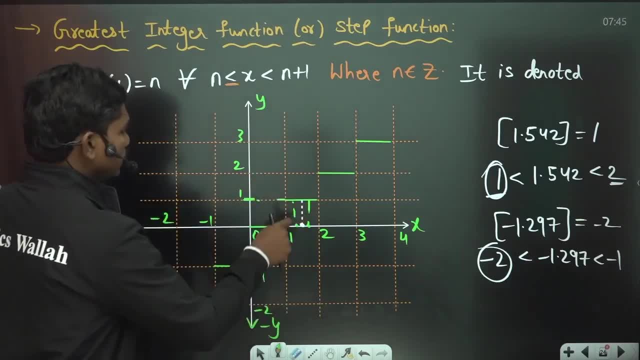 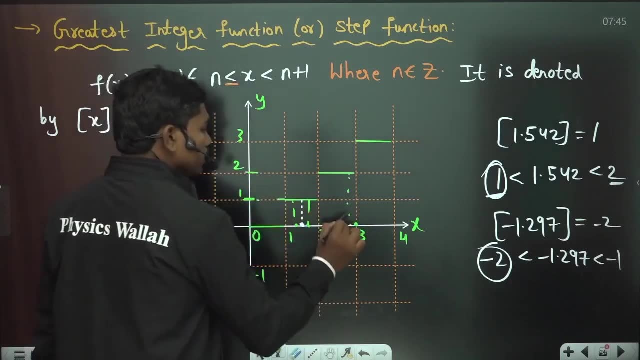 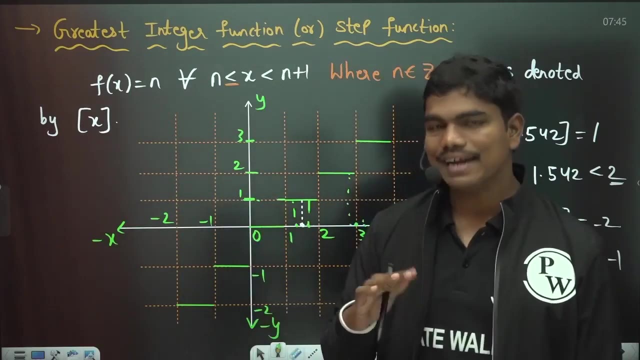 two. you know natural numbers or integers. you can say: this limit will exist. but let us suppose, if I take exactly three, left side, the value is two. you can see this is two. right side, the value is three. okay, so that's why, whenever, exactly when the point is at integer, limit does not exist because right hand, 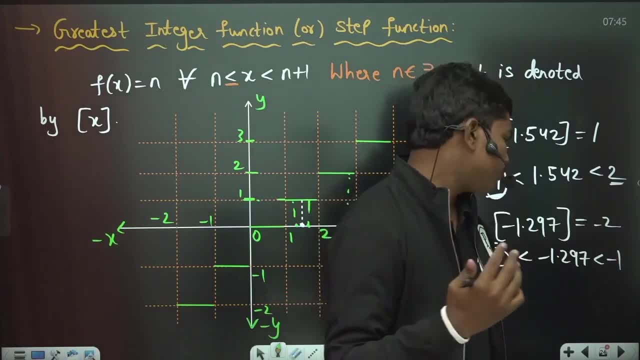 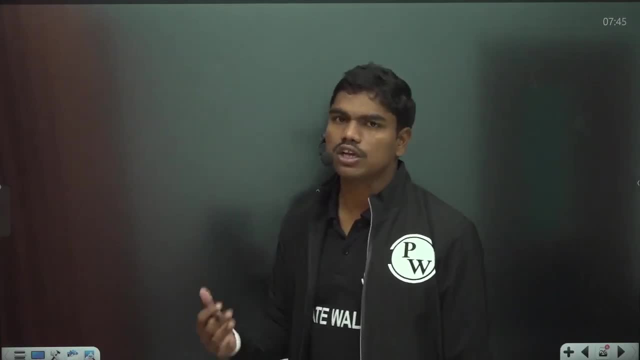 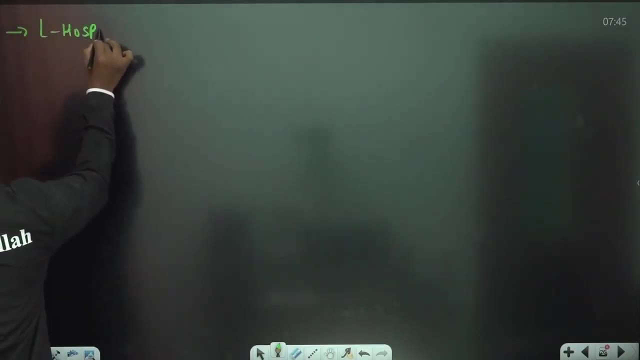 and left hand limits won't be same actually in that case. okay, so with this understanding, we will see some standard. you know limits are. let us see if one thing which is called L hospital, so one very important rule actually okay, so L hospital, whole L hospitals, rule, you can. 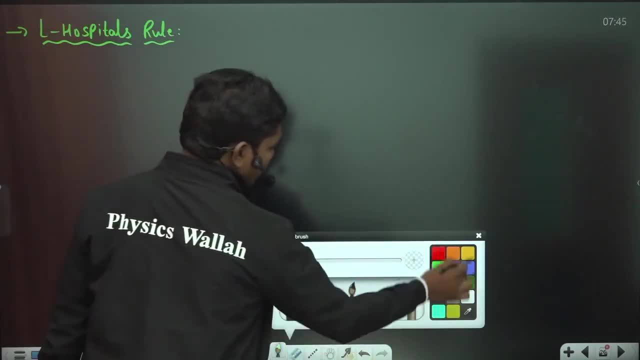 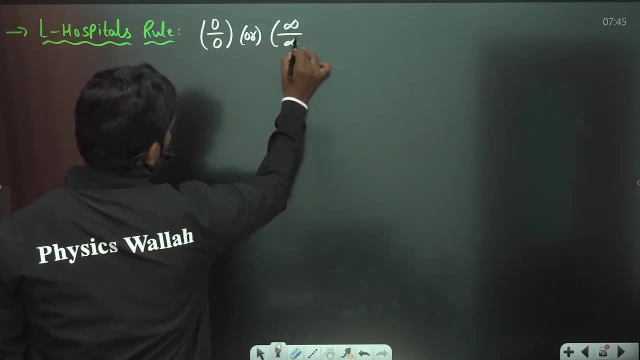 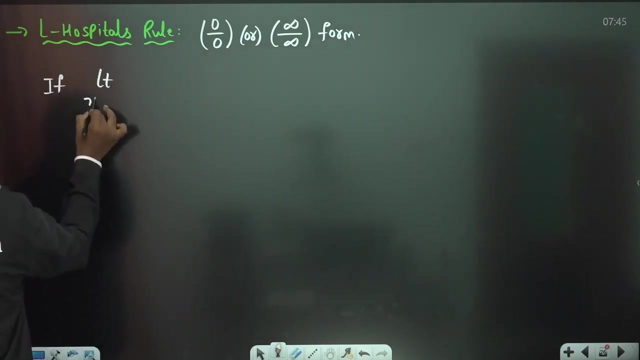 apply this rule only when you have this: 0 by 0 or infinity by infinity forms. okay, this will can be applied only under these two cases: 0 by 0 or infinity by infinity form. so let us see here: if limit X tends to a f of X by g of X, if this value is giving you 0 by 0 or 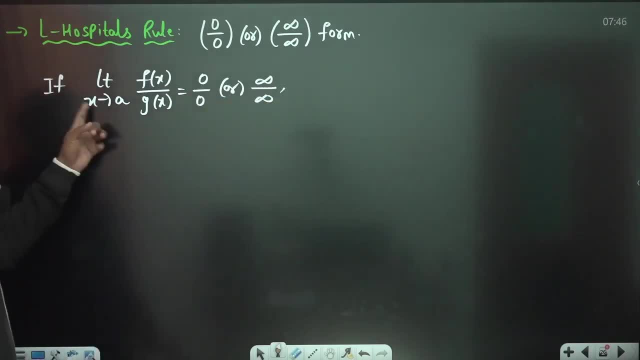 infinity by infinity. so what is the meaning of this? let us suppose when you substitute X is equal to a in this f of X, you are getting 0. similarly, when you're substituting X tends to a, again, this is also getting 0. so you'll get 0 by 0 form. 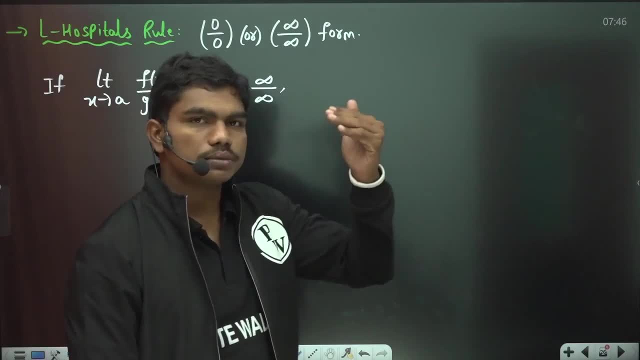 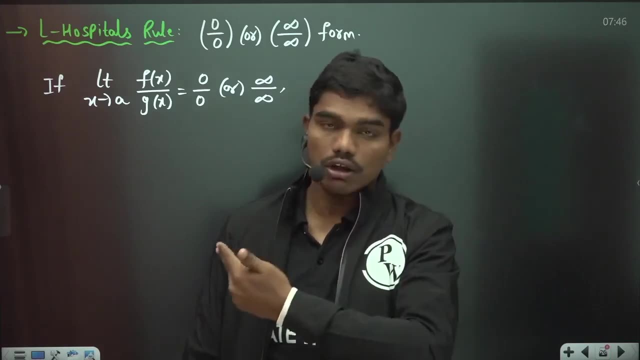 for example, limit X tends to 0 sine X by X. okay, so when you substitute 0 sine X sine 0 is also 0, X is equal to 0 will make denominator also 0. okay, so under such cases, or it can also give you infinity by infinity, for example you: 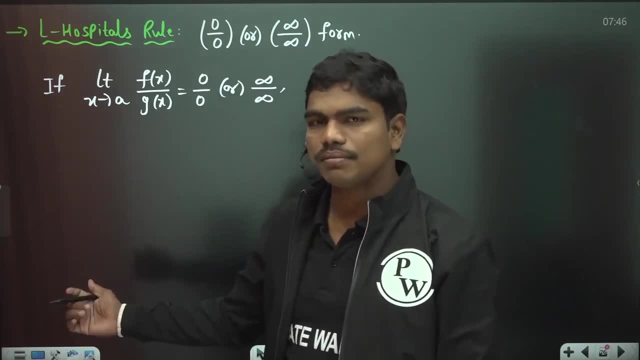 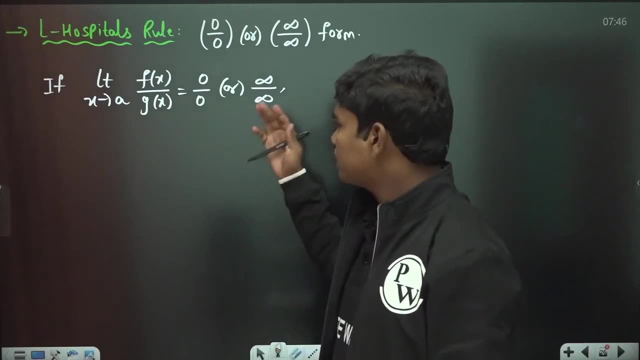 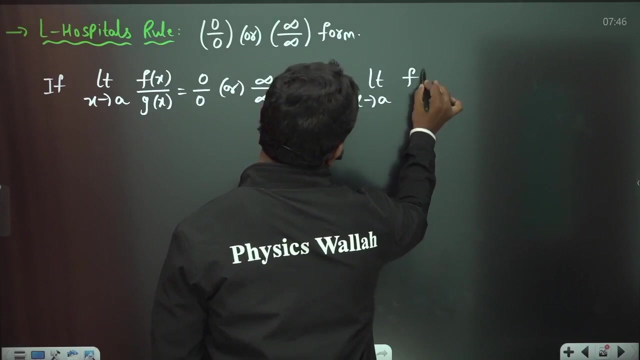 can see log log X divided by some other function, say tan tan- you know some functions as that- it gives infinity by infinity. okay, so if you give some, if this comes out, then limit X tends to a f of X by g of X. this can be written as: 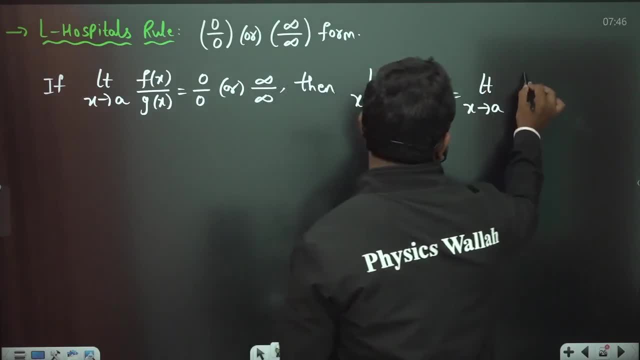 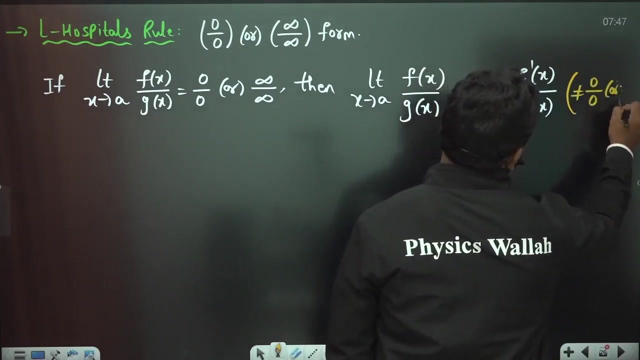 limit X tends to a f dash of X divided by G dash of X. okay, so this value is not equal to 0 by 0 or infinity by infinity, 0 by 0 or infinity by infinity. so let us suppose if that value is also coming to be 0- sometimes it happens you will get if limit X tends to. 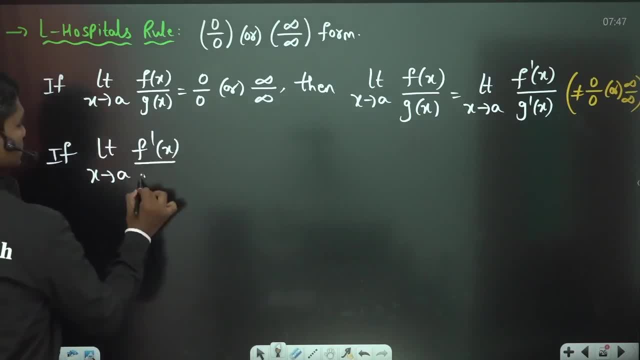 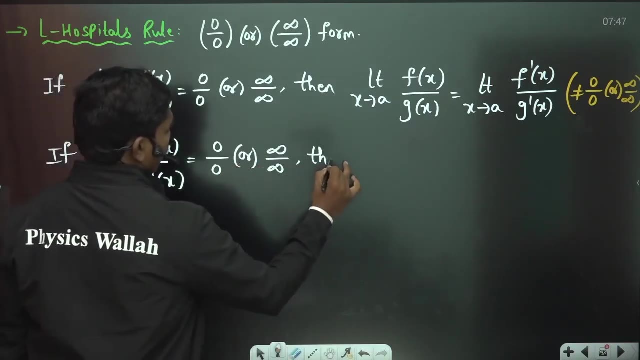 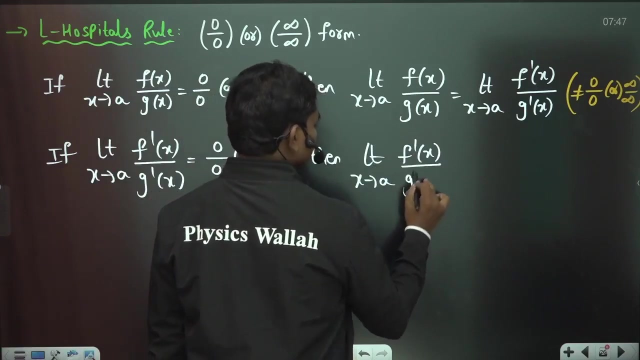 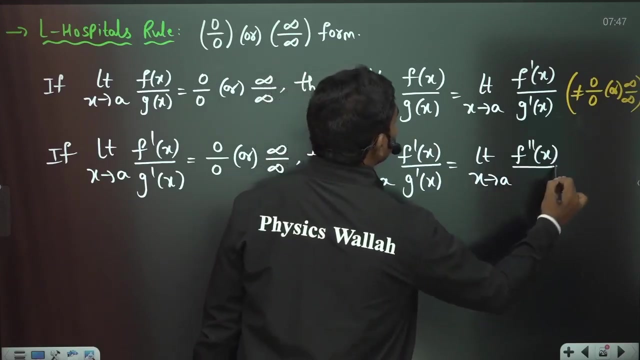 a f dash of X by G dash of X. if this value is same as limit X tends to a means, this is again getting equal to 0 by 0 or infinity by infinity. then limit x tends to a f dash of x by g dash of x. This value can be written as: limit x tends to a f double dash of x divided by g double. 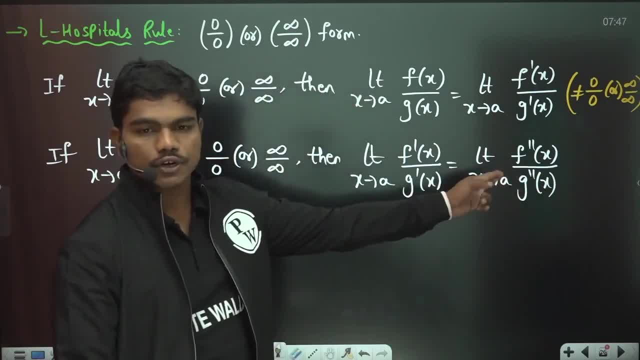 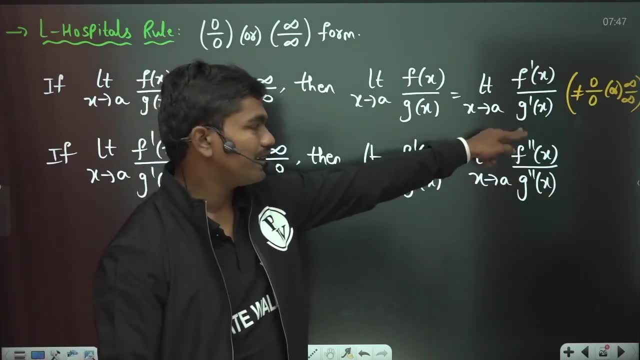 dash of x, And of course this should be again not 0 by 0 or infinity by infinity. If again this is also coming to be 0 by 0 or infinity by infinity, you will go for one more differentiation limit: x tends to a f double dash of x by g double dash of x. So that's why we write, and so on this: 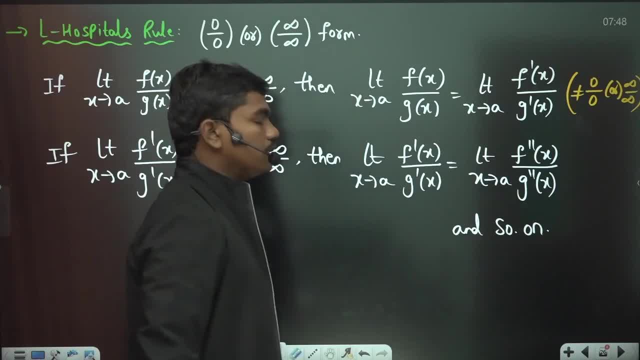 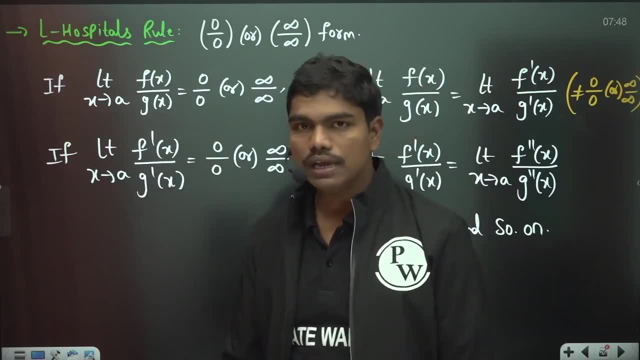 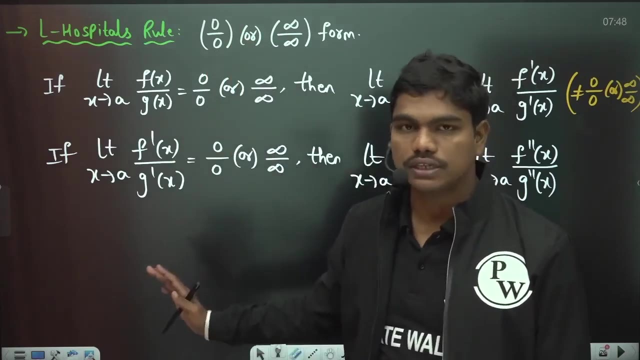 same circuit will follow, and so on, basically. So this is one very important, you know, very powerful, you know actually in calculus, because many times it's quite common we end up with these two ratios. So then we'll break the tie with using this L hospital. So let me give you 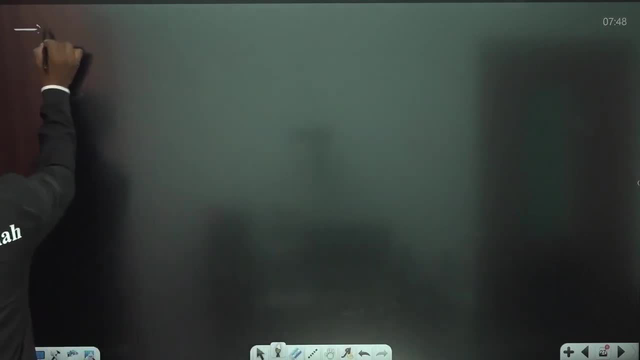 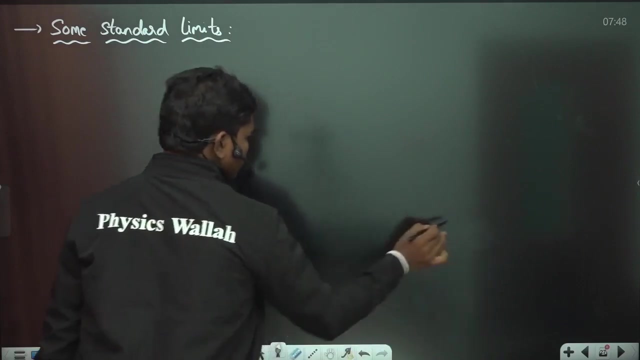 some standard limits, Some standard limits, Some standard limits. Let me give you here, So, some standard limits. Let us see First limit, very friendly limit known to you. limit x tends to a x power m minus a, power m by x minus a. So if you see we are going to get m times of a power m minus one, Okay, 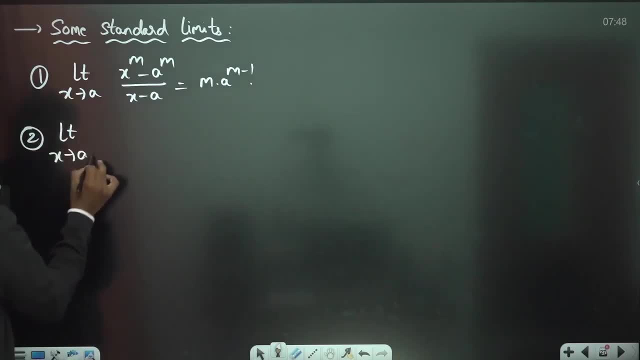 so second limit, x tends to a x power m minus a power m divided by x power n minus a power n. So this value is going to be m by n times of a to the power m minus n. Okay, look, both results you. 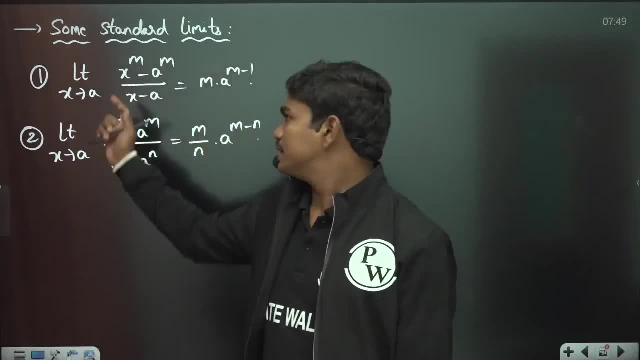 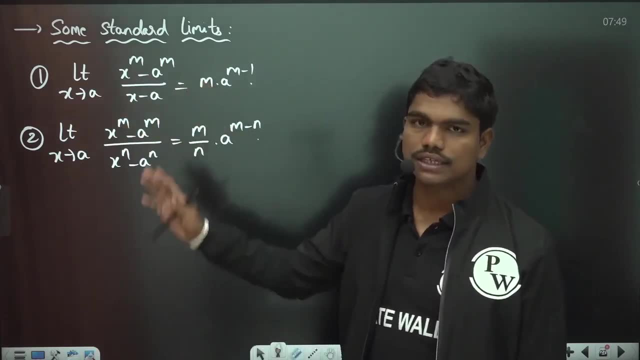 can get using the L hospital. So, because if you substitute x is equal to a, this comes to the form zero by zero And this also comes to the form zero by zero. So if you differentiate one time and if you substitute x is equal to a in the differentiation, you will get these results. 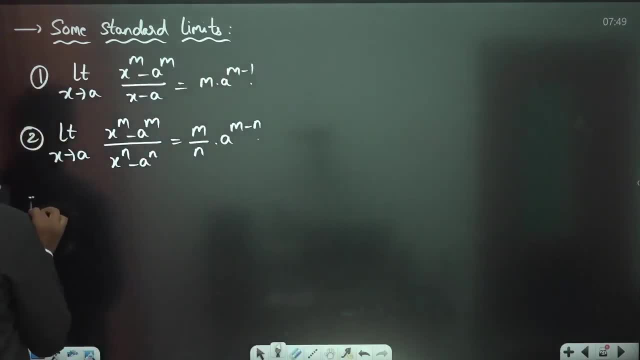 Okay, in both the cases. Okay now. third: limit extends to zero. sine x by x is equal to. limit extends to zero. tan x by x is equal to a. actually, okay, so both these limits will be equal to this value, which is a here. So 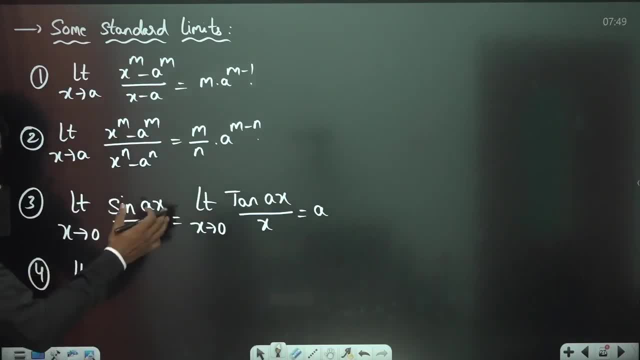 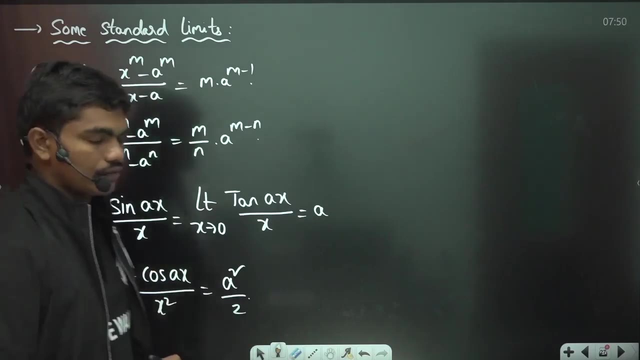 fourth limit extends to zero. again, using L hospital, you can get this. extends to zero. one minus cos x, cos x. let us write cos x by x square, this is equal to a square by two. Okay, so again, L hospital, if you apply, you will get this. a square by two means you can see if you put. 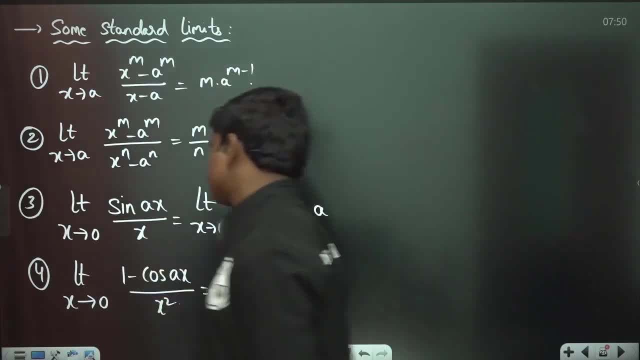 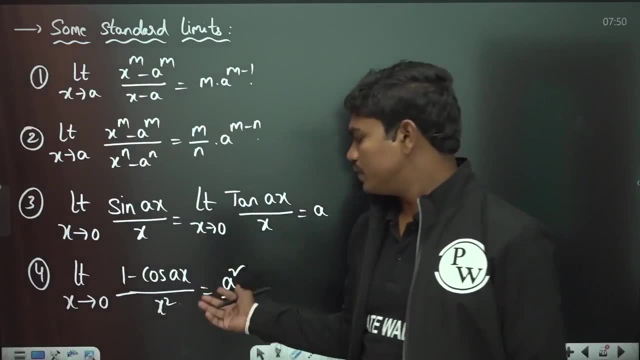 zero, cos zero is one, so one minus one is zero divided by zero. This division is for completely one minus, so you can get zero by zero form. So if you apply L hospital rule, you will get a square by two here, Okay, next. 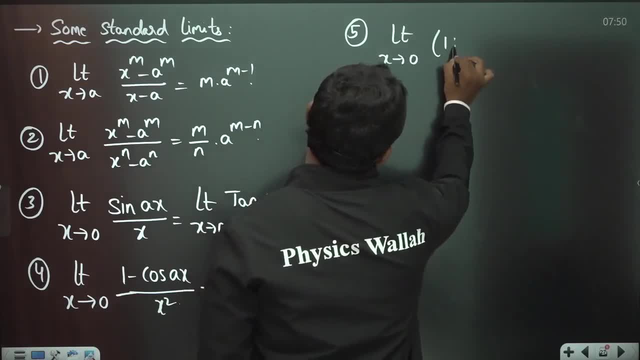 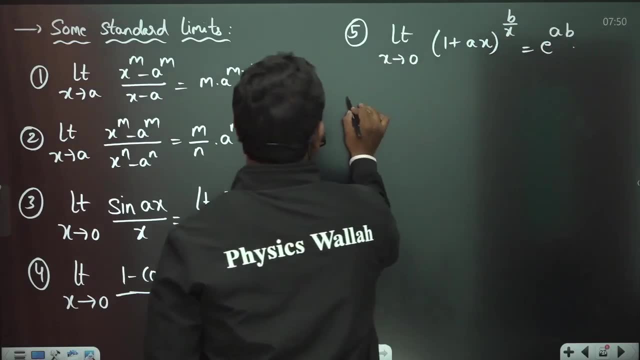 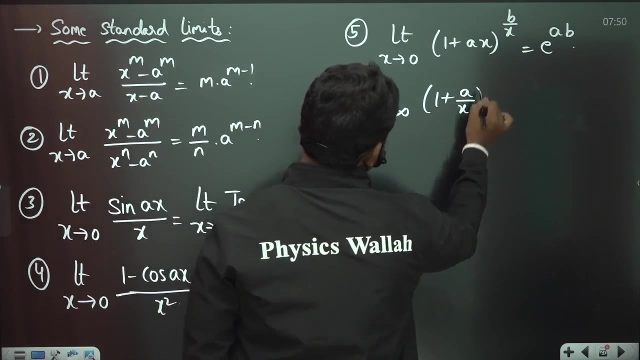 Yeah, a lot of limits. basically, limit extends to zero. one plus a- x. whole power, b by x. this value is going to be e power a b. Similarly, this value limit extends to infinity. one plus a by x- whole power b, x. this value also, it gives you e to the power a b. Okay, so in these two cases, basically, 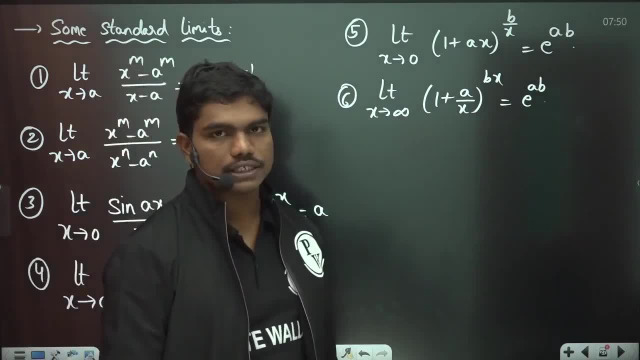 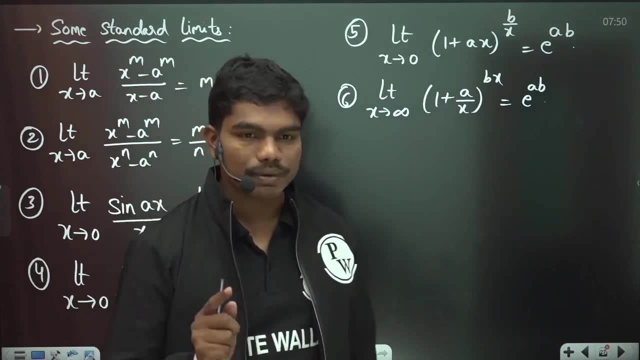 I would like to spend a moment here. In these two cases, actually, if you substitute, x is equal to zero, you will get the form one power infinity. So one power infinity value is not one, Okay, so please keep this in mind. Many people have 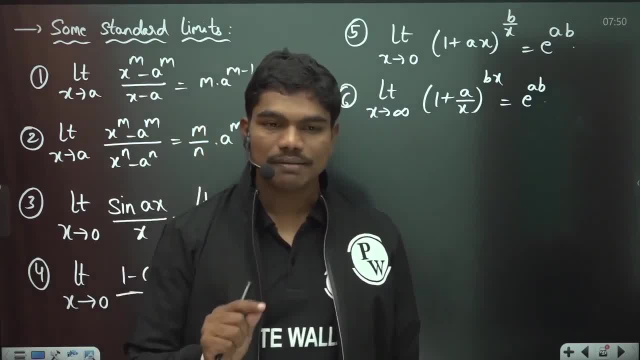 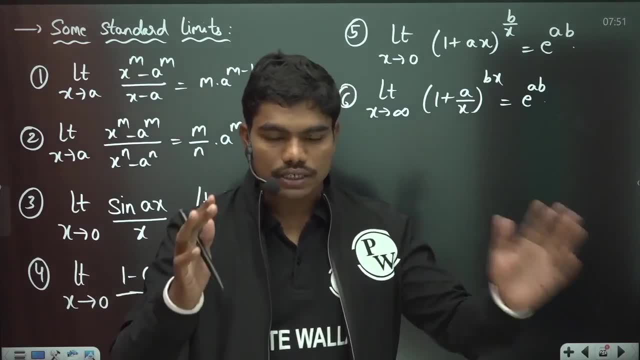 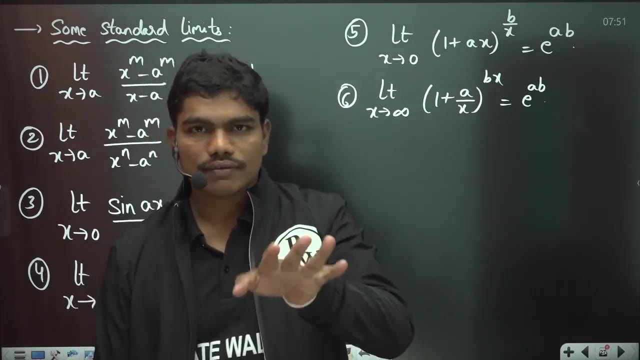 this misconception that one power, infinity, is one. No, because multiplication means if you go to fundamentals, mathematical fundamentals, multiplication is defined only when you can start the multiplication and stop. the multiplication means basically, let us suppose, if I 2.4 into five, into eight, into some numbers, and after that, if I stop, I should locate the ending of the. 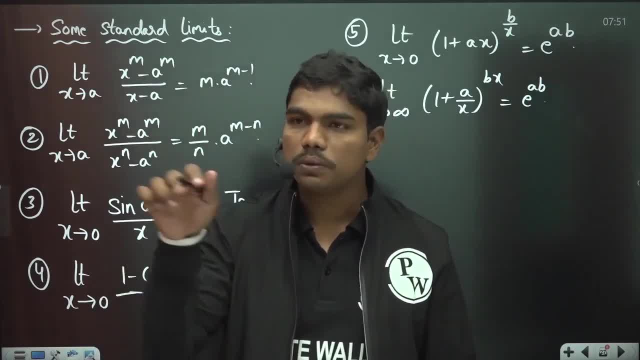 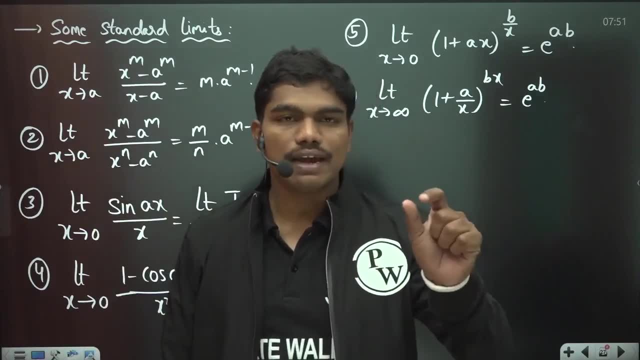 multiplication, Okay, but when I had one point infinity, one into, one into, one into, and I don't know where it stops, okay, infinity is basically a symbol for denoting a large number And I don't know what is the exact value of that large number. So that's why this one power, infinity is. 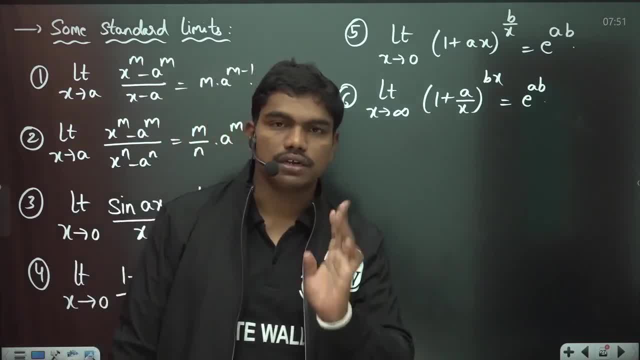 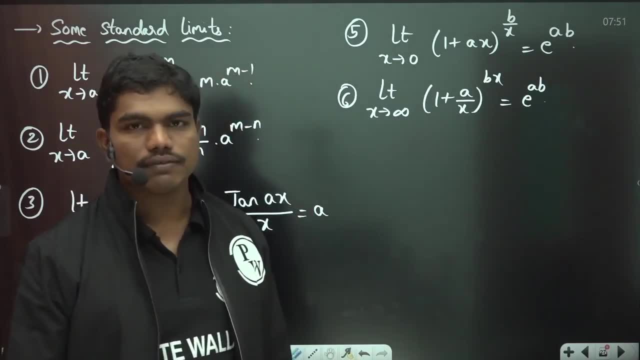 not equal to one because we cannot stop the multiplication Understood. So that's the reason: one point: infinity is not equal to one, it's indeterminate form, basically okay. So whenever you'll get indeterminate forms in powers means one point: infinity, zero power. infinity, one power. 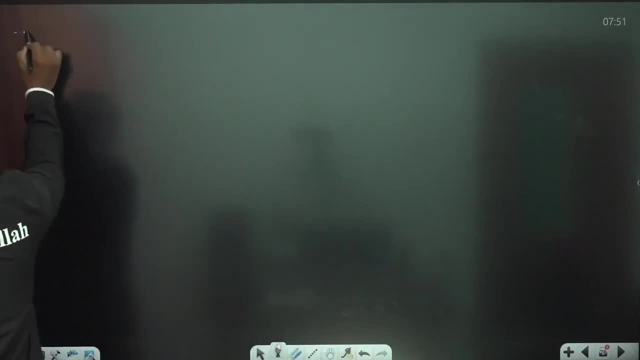 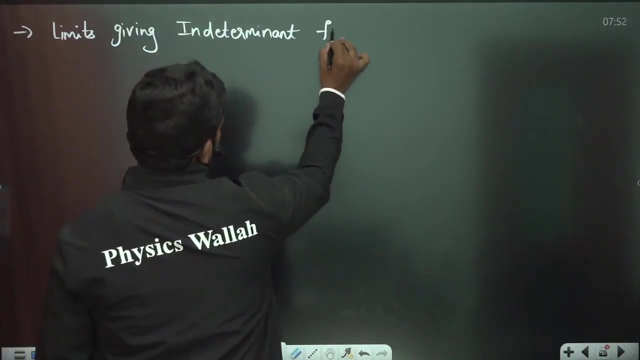 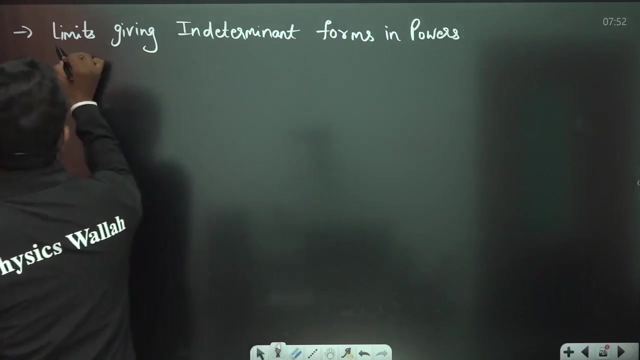 infinity, all these things. So let us see Limits: limits giving indeterminate forms in powers, limits giving indeterminate forms in powers. limits giving indeterminate forms in powers, Let us say, means basically, if you see, you'll get things like one. 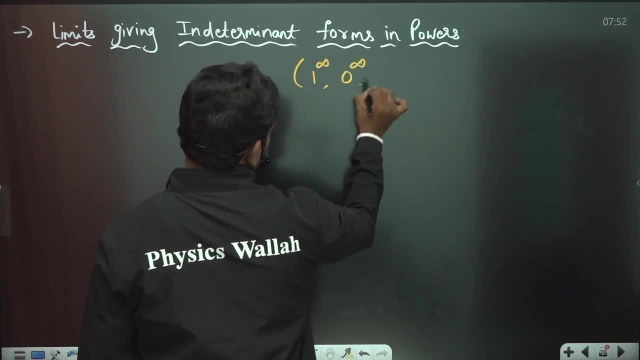 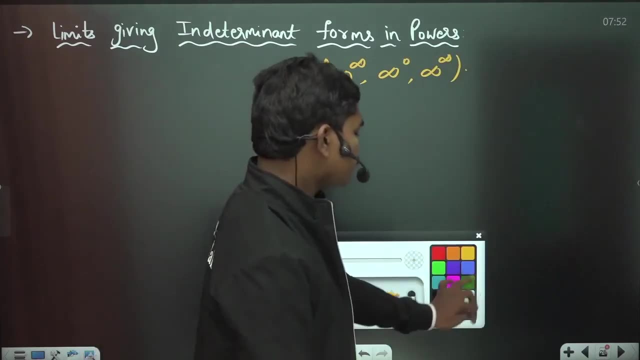 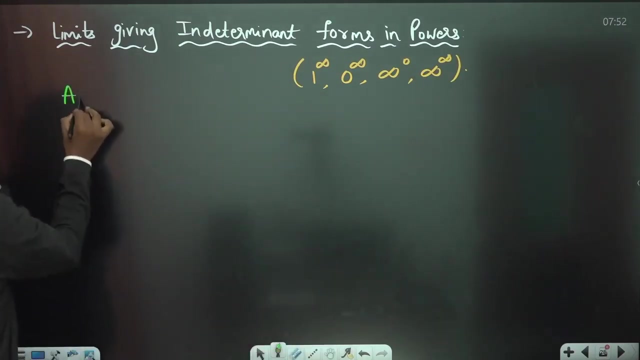 point infinity, zero power, infinity, infinity or zero infinity, point infinity, these kind of things, basically. okay. so whenever you are getting these things, look, there is one standard procedure which is called the 2l procedure. okay, so we'll write: apply 2l procedure, apply 2l procedure. so what is this 2l procedure? 1l stands for log. 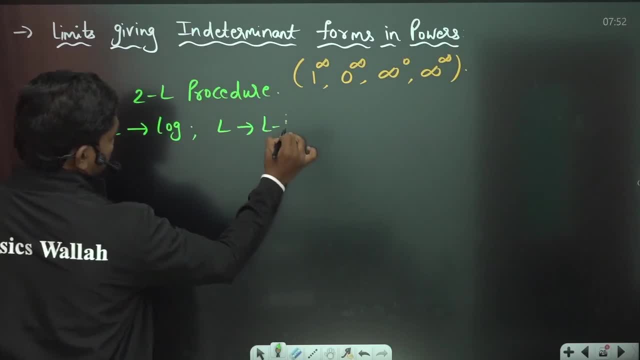 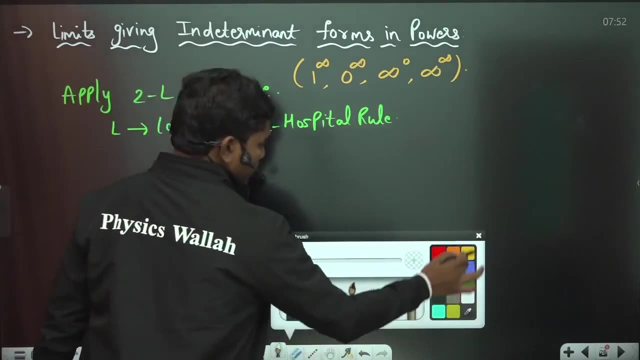 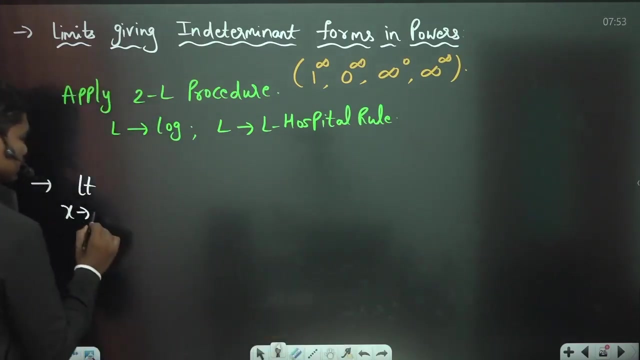 second, l stands for l hospital, l hospital rule. let us see how we are going to do it okay. so let us take this limit, for example. limit x tends to a- sorry, x tends to 0. you can say: x tends to 0, 1 plus ax, whole power, b by x, for example. let us say so obviously this gives you 1 to the. 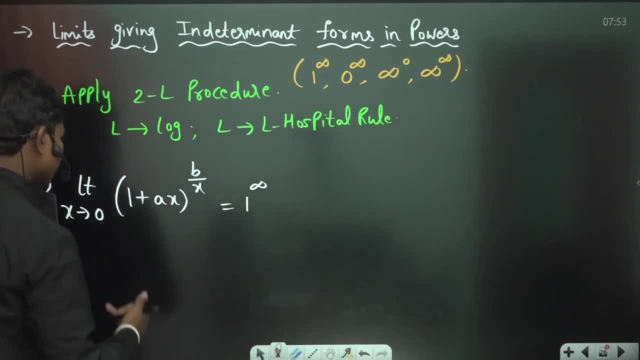 point infinity form a and we have some constants. so whenever this is giving you 1 point infinity form, look, look, this is equal to. now what we assume is: take y is equal to, for example, 1 plus ax, whole power, b by x, so you will take the function as some variable y, then apply log on both sides: the first l, we. 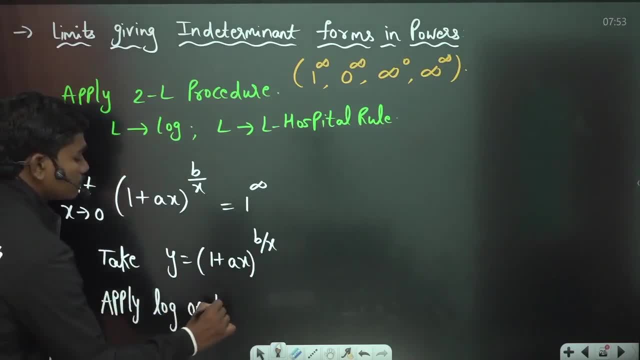 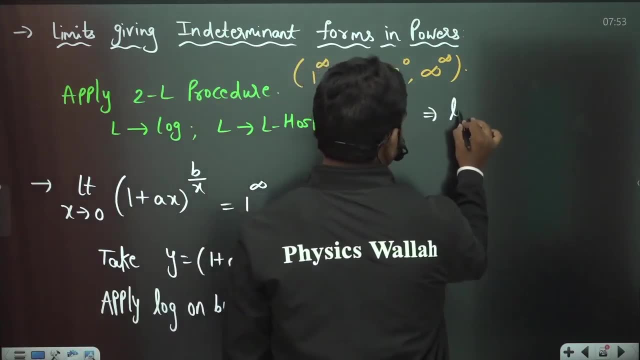 are applying. apply log on both sides. apply log on both sides. so when you apply logarithm on both sides, this gives you something like log y to the base e. this gives you something like log y to the base e. this gives you something like log y to the base e, equal to now. if you apply logarithm to this. equal to now. if you apply logarithm to this: equal to now. if you apply logarithm to this: log of 1 plus x whole power v by x. so this b by x. log of 1 plus x whole power v by x. so this b by x. 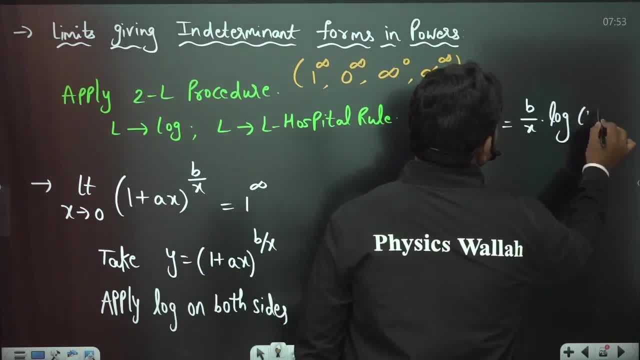 log of 1 plus x whole power v by x. so this b by x can be written separately outside log 1 plus can be written separately outside log 1 plus can be written separately outside log 1 plus ax to the base e. this is what you will get, okay. 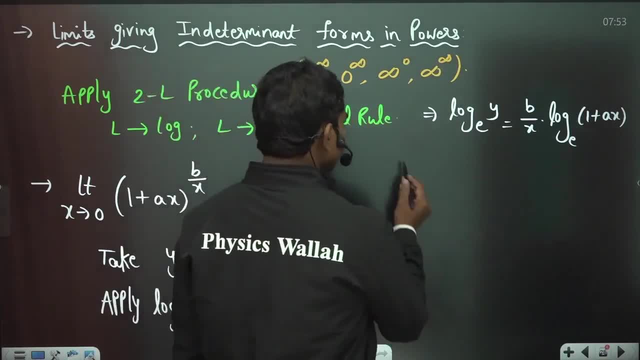 ax to the base e: this is what you will get okay. ax to the base e: this is what you will get okay. so now, if you see if you apply the limit, so now if you see if you apply the limit, so now if you see if you apply the limit, basically on both sides. limit extends to 0. 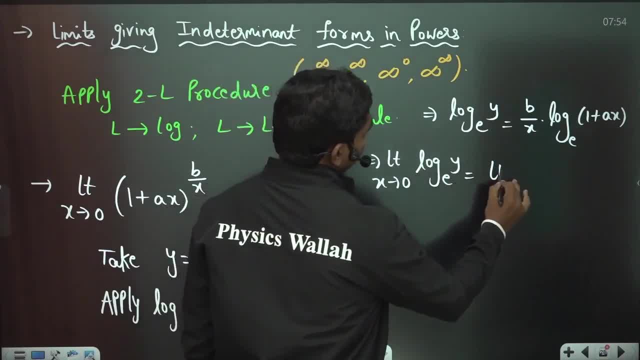 basically on both sides. limit extends to 0, basically on both sides. limit extends to 0. log y to the base e is equal to limit extends to 0. log y to the base e is equal to limit extends to 0. log y to the base e is equal to limit extends to 0. b by x into. 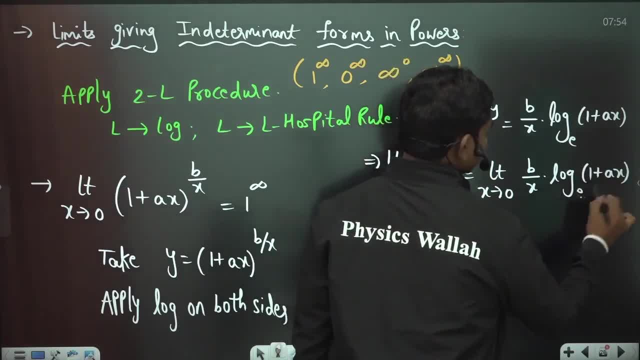 b by x into b by x into log of 1 plus ax to the base e is what log of 1 plus ax to the base e is what log of 1 plus ax to the base e is what you have here. okay, now you can observe. 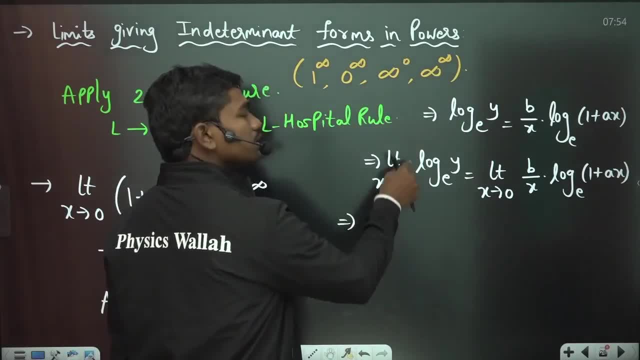 you have here, okay, now you can observe. you have here, okay, now you can observe one thing, one thing, one thing: log and limit. both are transferable- log and limit. both are transferable- log and limit, both are transferable functions. means if you apply log functions, means if you apply log. 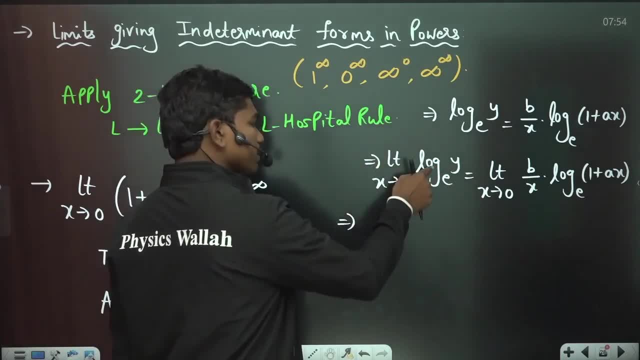 functions means if you apply log to this y and then if you apply limit to this y, and then if you apply limit to this y and then if you apply log, or if you first apply limit and then you, or if you first apply limit and then you. 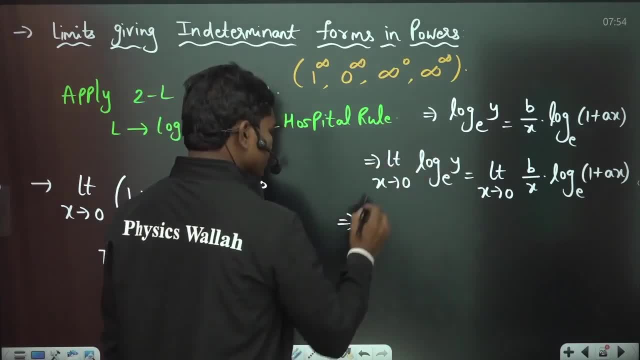 or if you first apply limit and then you take log of that whole value, both remain. take log of that whole value, both remain. take log of that whole value. both remain same. so this expression on the left side: same. so this expression on the left side: same. so this expression on the left side can be written as: 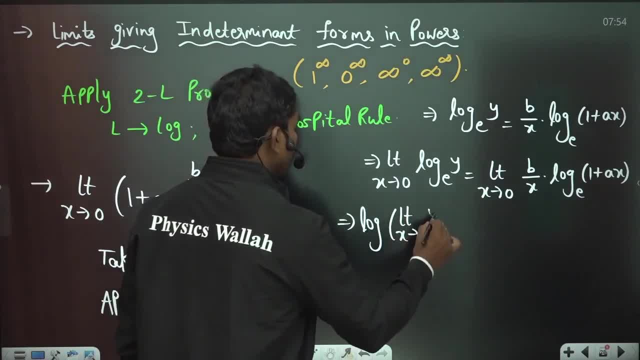 can be written, as can be written as: log limit x tends to 0 y. log limit x tends to 0 y. log limit x tends to 0 y. to the base e. this is what you can write to the base e. this is what you can write. 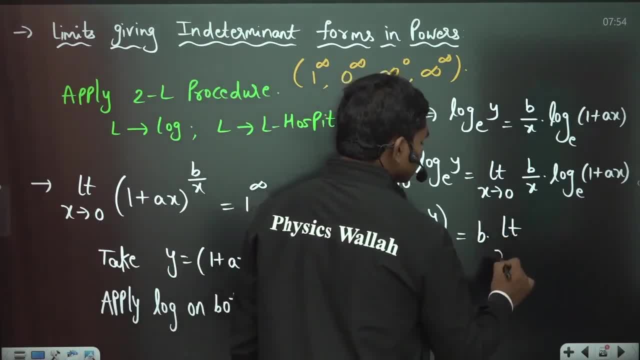 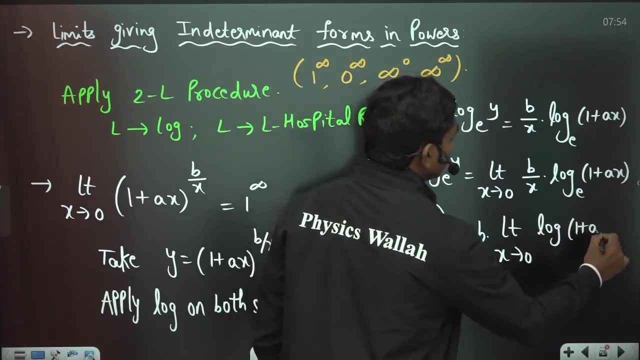 to the base e. this is what you can write here. coming to this b, into what you have here. coming to this b into what you have here. coming to this b into what you have: limit x tends to 0. limit x tends to 0. log of 1 plus ax. 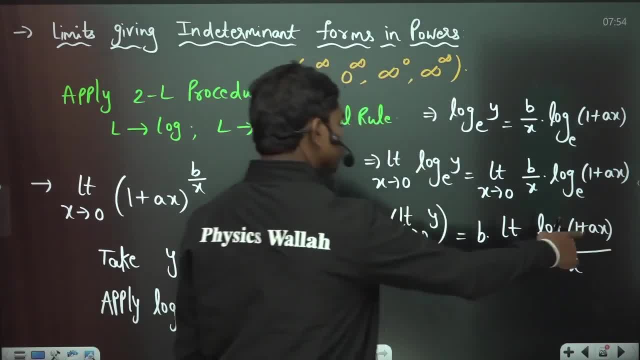 limit x tends to 0: log of 1 plus ax. limit x tends to 0: log of 1 plus ax. to the base e divided by x. now if you to the base e divided by x. now, if you to the base e divided by x. now, if you substitute, x is equal to 0 in this. 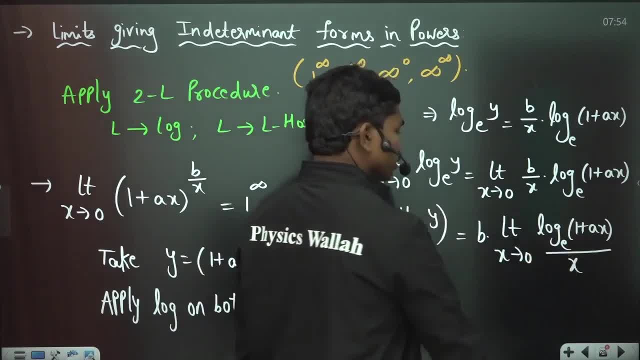 substitute x is equal to 0. in this substitute x is equal to 0. in this equation equation: equation: log 1 is 0. this denominator is also 0. log 1 is 0. this denominator is also 0. log 1 is 0. this denominator is also 0, so that's how you'll get. 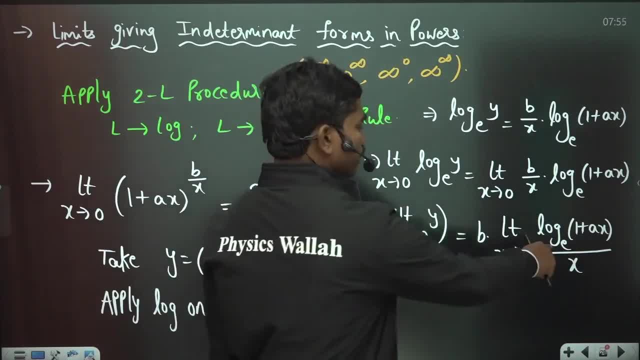 so that's how you'll get. so that's how you'll get 0 by 0 forms. so now you can apply l 0 by 0 forms. so now you can apply l 0 by 0 forms. so now you can apply l hospital to calculate this limit. 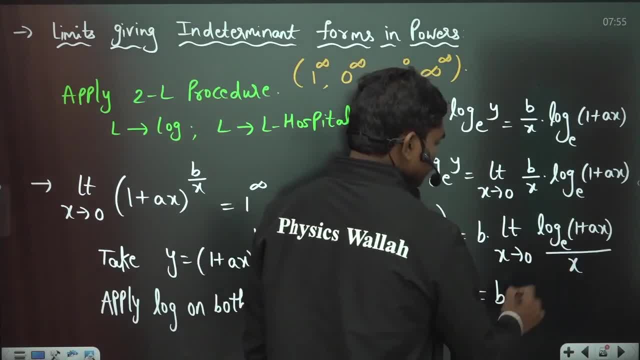 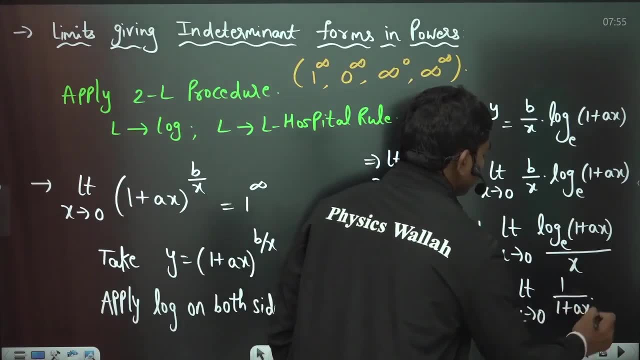 hospital to calculate this limit? hospital to calculate this limit? what? how you can calculate b into if what? how you can calculate b into if what? how you can calculate b into. if differentiation of log is 1 by that, differentiation of log is 1 by that differentiation of log is 1 by that function into the inner differentiation of. 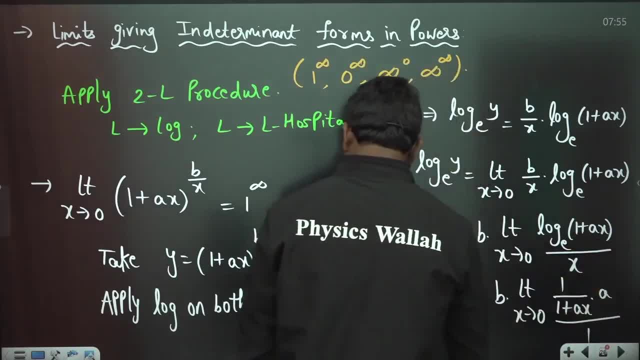 function into the inner differentiation of function, into the inner differentiation of this is a. divided by differentiation of this is a. divided by differentiation of this is a: divided by differentiation of: x is 1, so when you substitute x is equal, x is 1, so when you substitute x is equal. 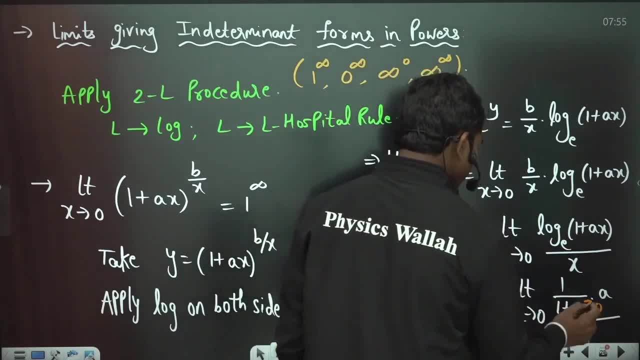 x is 1. so when you substitute x is equal to 0, this value is going to be 0. so you to 0, this value is going to be 0. so you to 0, this value is going to be 0. so you have a, b, a b is what you have, okay, so? 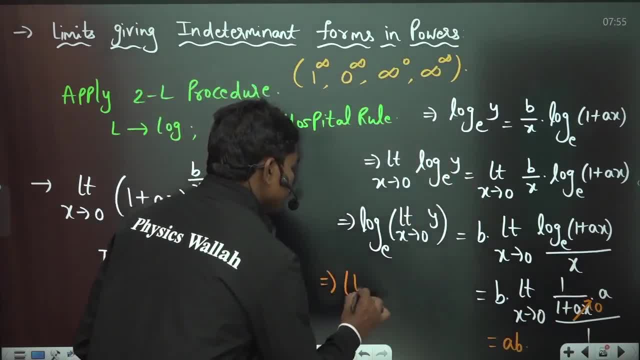 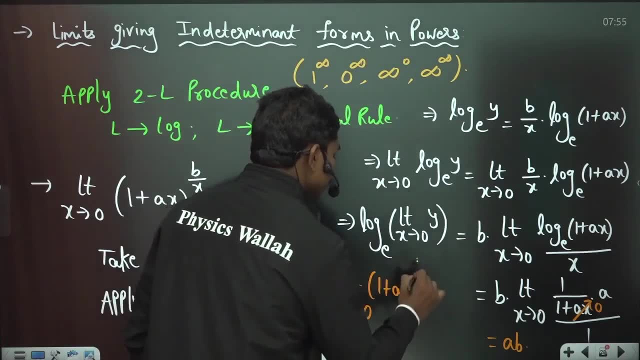 have a b. a b is what you have, okay. so have a b. a b is what you have, okay. so this log value is a b, which means i can. this log value is a b, which means i can. this log value is a b, which means i can give you the power a b. this is how you. 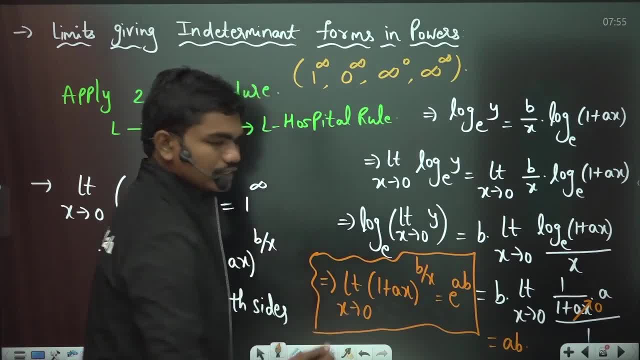 give you the power a- b. this is how you give you the power a- b. this is how you will evaluate the limits. okay, any power will evaluate the limits. okay, any power will evaluate the limits. okay, any power form you will get if you get zero power form you will get if you get zero power. 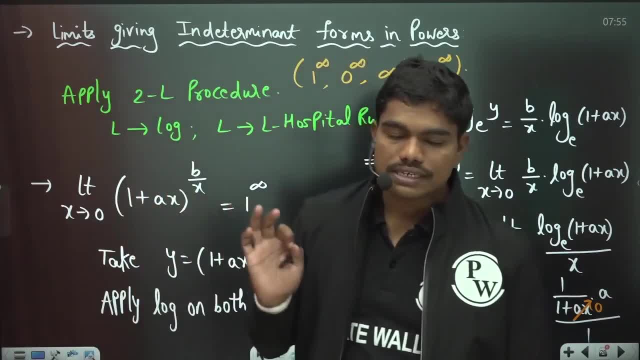 form you will get if you get zero power, zero infinity point, infinity, any power. zero infinity point, infinity, any power, zero infinity point, infinity, any power form. if you, if your indeterminate form form, if you, if your indeterminate form form, if you, if your indeterminate form is in terms of powers, then definitely. is in terms of powers, then definitely is in terms of powers, then definitely this 2l processor is going to help you. this 2l processor is going to help you. this 2l processor is going to help you out so you can play log and then you 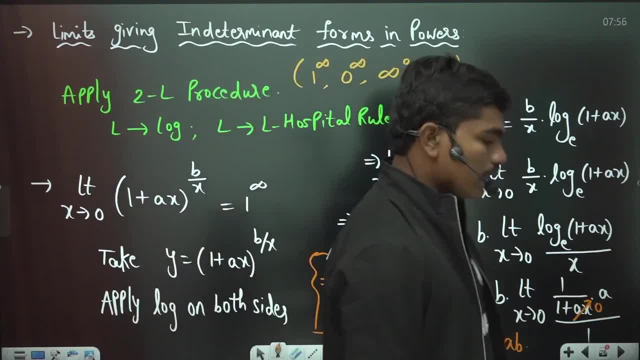 out so you can play log, and then you out so you can play log, and then you apply l hospital, then things get settled. apply l hospital, then things get settled. apply l hospital, then things get settled. okay so, but again i would like to give. okay so, but again i would like to give. 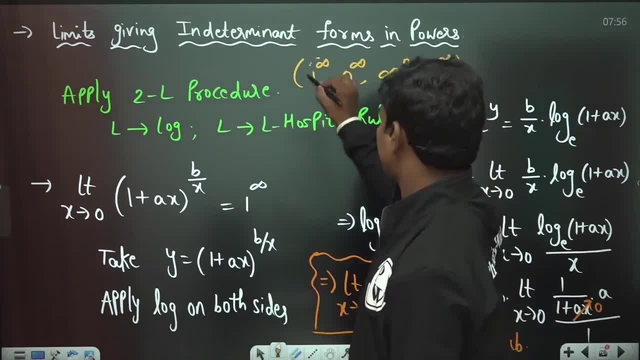 okay so, but again, i would like to give one technique for the first, one technique for the first, one, technique for the first. indeterminate form means this form okay. indeterminate form means this form okay. indeterminate form means this form okay whenever things are in one power. 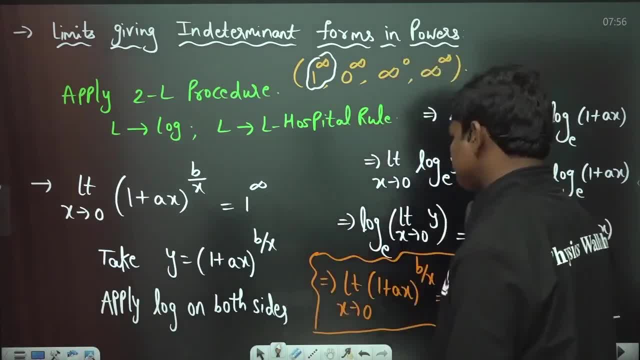 whenever things are in one power. whenever things are in one power, infinity form. i'll give you some infinity form. i'll give you some infinity form. i'll give you some technique, technique, technique. look, what is that technique. if. look what is that technique. if look what is that technique. if, if limit extends to a 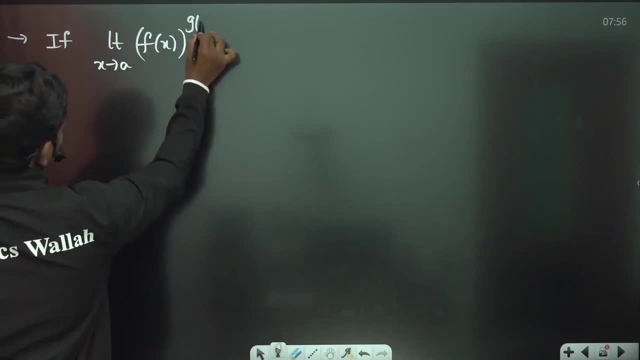 if limit extends to a, if limit extends to a: f of x, power g of x. let us suppose you f of x, power g of x. let us suppose you f of x, power g of x. let us suppose you have power of two functions, have power of two functions. 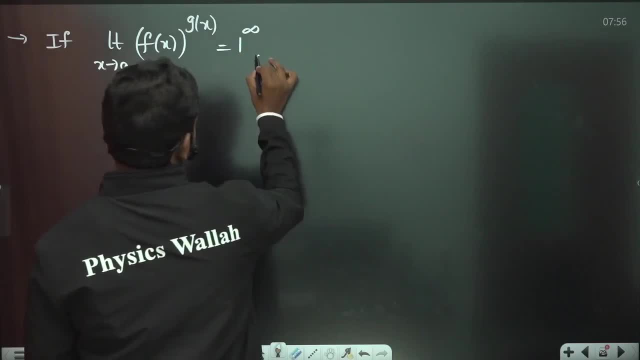 have power of two functions, and this is giving you one point, and this is giving you one point, and this is giving you one point: infinity form, infinity form, infinity form. then, limit extends to a f of x, power g of x. limit extends to a f of x, power g of x. 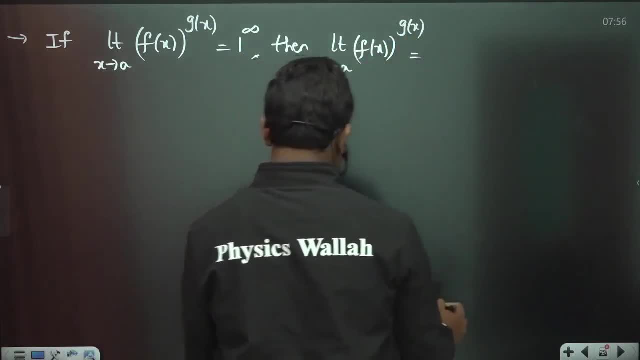 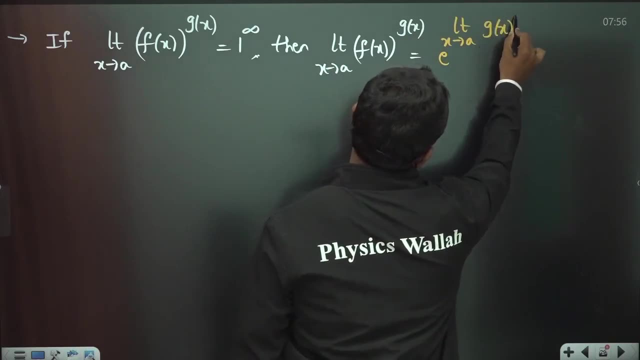 limit extends to a f of x. power g of x. this value is actually equal to. this value is actually equal to. this value is actually equal to e. power limit extends to a e. power limit extends to a e. power limit extends to a g of x. g of x. 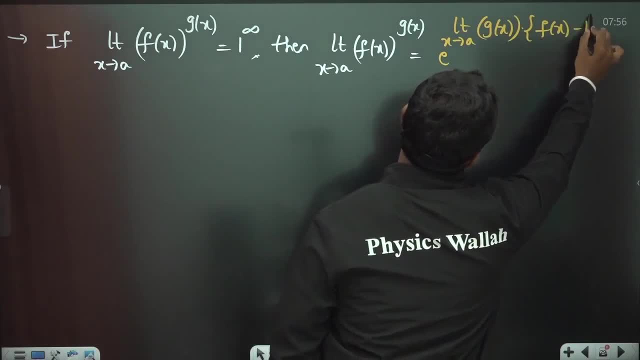 g of x into into into f of x, f of x, f of x. minus one minus one minus one. okay, so this is how you will get this okay. so this is how you will get this. okay, so this is how you will get this okay. of course, i can show you that using: 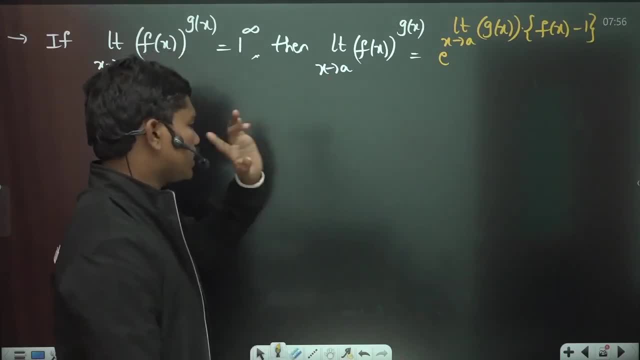 okay, of course i can show you that using. okay, of course i can show you that using the same r2l procedure, but right now i'm the same r2l procedure, but right now i'm the same r2l procedure, but right now i'm not doing the derivation and all i'm 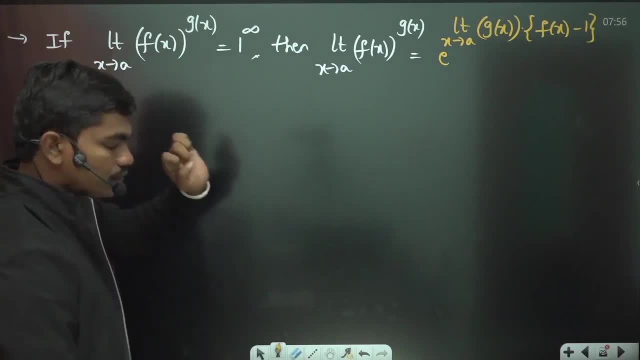 not doing the derivation and all i'm not doing the derivation and all i'm just giving you this formula. okay. so if just giving you this formula, okay, so if just giving you this formula, okay so if, whenever, if there is some power of, whenever, if there is some power of. whenever, if there is some power of functions f of x, power g of x, and if you functions f of x, power g of x, and if you functions f of x, power g of x, and if you are getting this one point infinitive, are getting this one point infinitive. 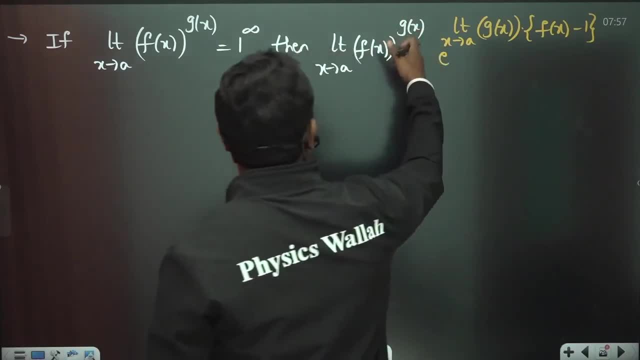 are getting this one point- infinitive form- then definitely this limit extends form. then definitely this limit extends form, then definitely this limit extends to a f of x. power g of x can be to a f of x. power g of x can be to a f of x. power g of x can be calculated using the result. okay, now for 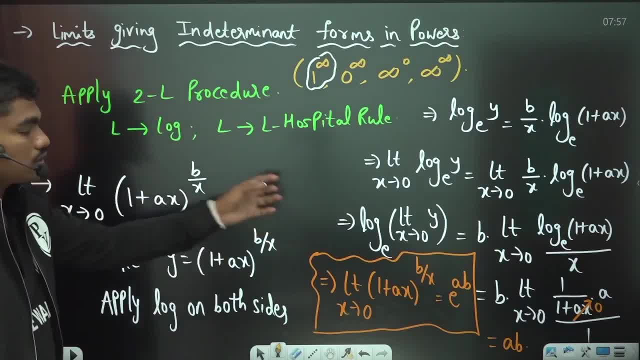 calculated using the result. okay, now for calculated using the result. okay now. for example, if you see this is a one point example, if you see this is a one point example, if you see this is a one point. infinity form: you have applied two else. infinity form: you have applied two else. 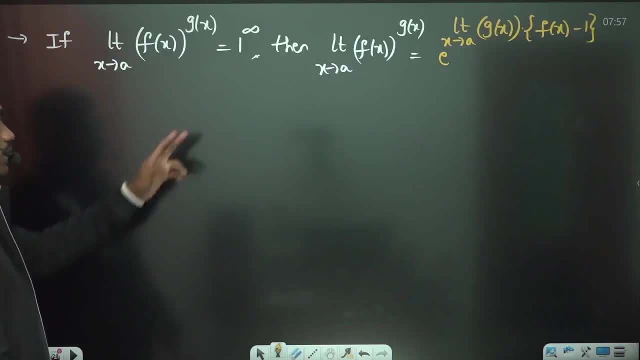 infinity form. you have applied two else, one logarithm and one l hospital to get one logarithm and one l hospital to get one logarithm and one l hospital to get the result. but let us see if you the result. but let us see if you the result, but let us see if you get the same result using this uh technique. 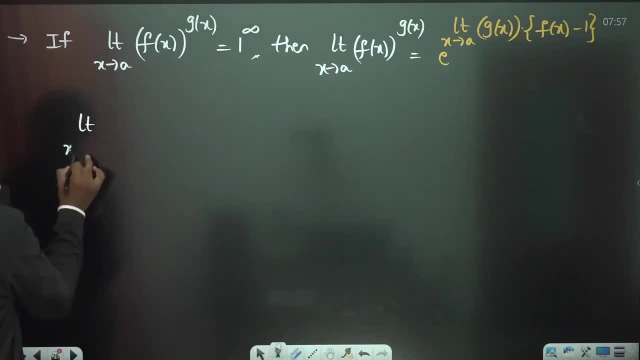 get the same result using this uh technique. get the same result using this uh technique. okay, so, if you see okay, so if you see okay, so if you see limit x tends to 0, limit x tends to 0, limit x tends to 0, 1 plus a x, whole power b by x. this is: 1 plus a x- whole power b by x. this is 1 plus a: x- whole power b by x. this is the limit that you have, okay. so this is the limit that you have, okay. so this is the limit that you have, okay. so this is straight away. giving you one point. 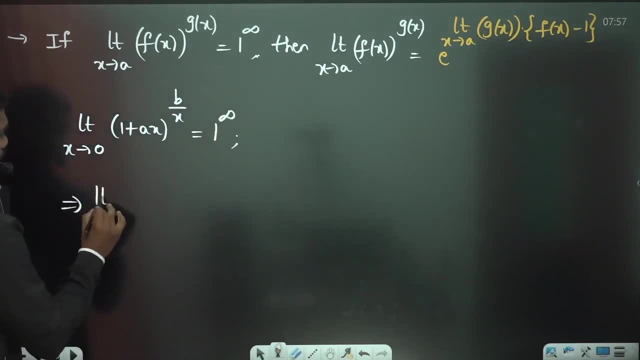 straight away. giving you one point, straight away. giving you one point. infinity substitute. okay, so this implies infinity substitute. okay, so this implies infinity substitute. okay, so this implies limit x tends to 0, limit x tends to 0, limit x tends to 0. 1 plus a x. whole power, b by x. so this: 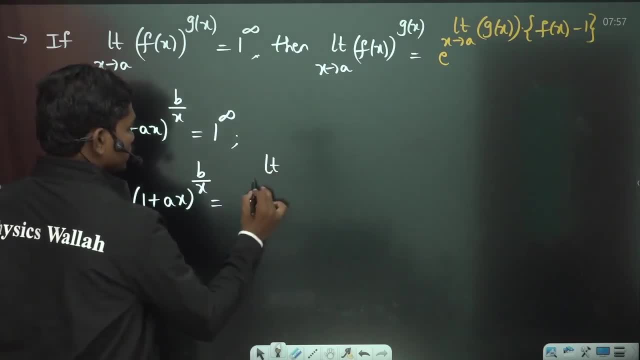 1 plus a x, whole power b by x. so this 1 plus a x, whole power b by x. so this value is equal to e. power limit extends value is equal to e. power limit extends value is equal to e. power limit extends to a. so limit x tends to 0, g of x, which 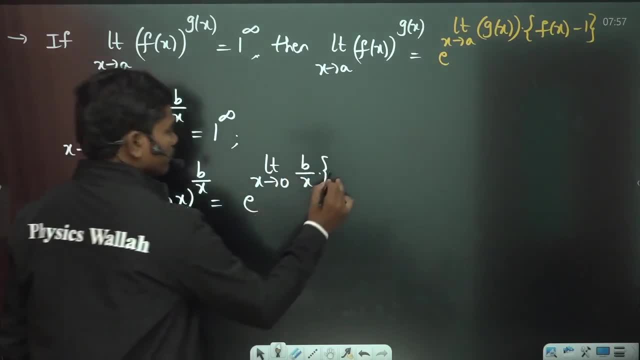 to a, so limit, x tends to 0 g of x, which to a so limit, x tends to 0 g of x, which is b by x into f of x minus 1, so f of x is b by x into f of x minus 1, so f of x. 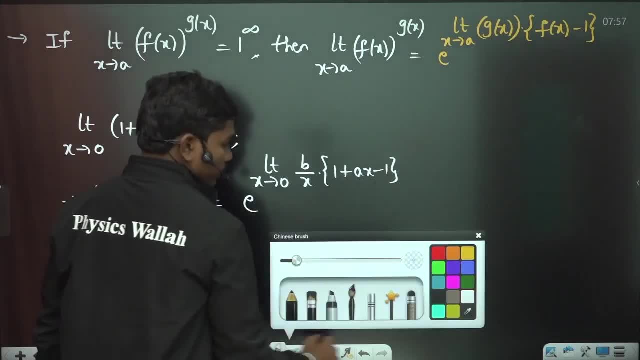 is b by x into f of x minus 1. so f of x is 1 plus a x minus 1. okay. so here, if you is 1 plus a x minus 1, okay. so here, if you is 1 plus a x minus 1, okay. so here, if you can cancel out this one and one, 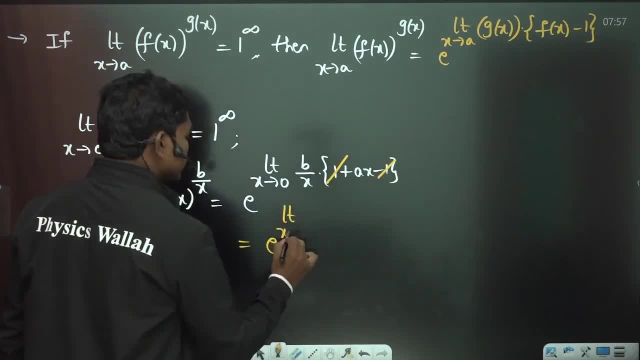 can cancel out this one, and one can cancel out this one and one. this is equal to e power limit extends. this is equal to e power limit extends. this is equal to e power limit extends to 0. b by x into a. x is what you have. 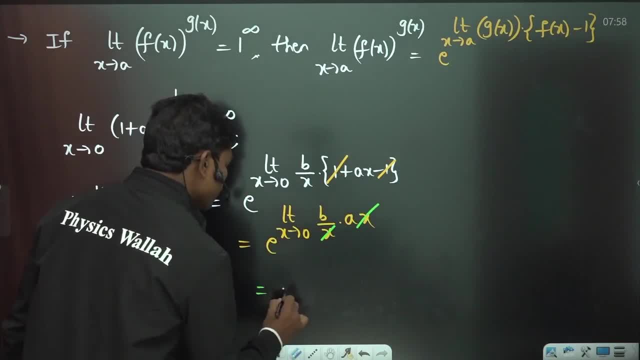 to 0 b by x into a x is what you have. to 0 b by x into a x is what you have. now we can cancel this x and x term here. now we can cancel this x and x term here. now we can cancel this x and x term here. so e power limit extends to 0 a b, no x. 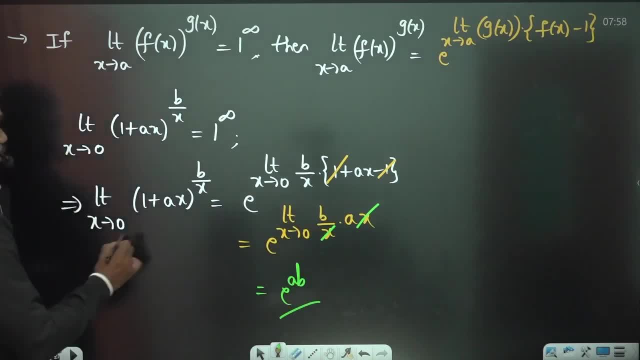 so e power limit extends to 0 a b, no x. so e power limit extends to 0 a b, no x to substitute. so this is directly a b to substitute. so this is directly a b to substitute. so this is directly a- b. that's how you will get the result of. 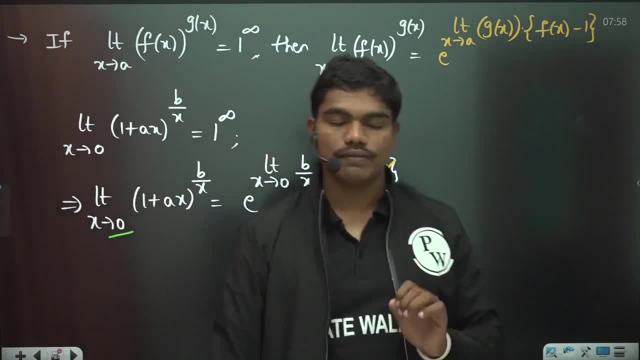 that's how you will get the result of. that's how you will get the result of this limit as e power a b, this limit as e power a- b when you apply this. okay, so this is one. when you apply this. okay, so this is one when you apply this. okay, so this is one way. uh, you know fast track rule in math. 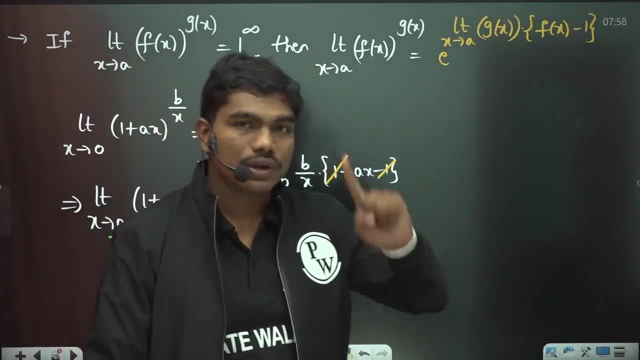 way, uh, you know fast track rule in math. way? uh, you know fast track rule in math: calculus. basically that whenever things calculus, basically that whenever things calculus. basically that whenever things are one power infinity, look, you can are one power infinity, look, you can are one power infinity, look, you can apply this technique only and only when. 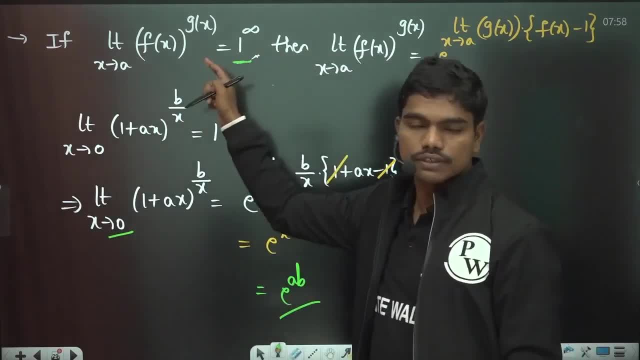 apply this technique only and only when. apply this technique only and only when it is of one power infinity form. okay, it is of one power, infinity form. okay, it is of one power, infinity form. okay. you cannot apply this for zero power. you cannot apply this for zero power. 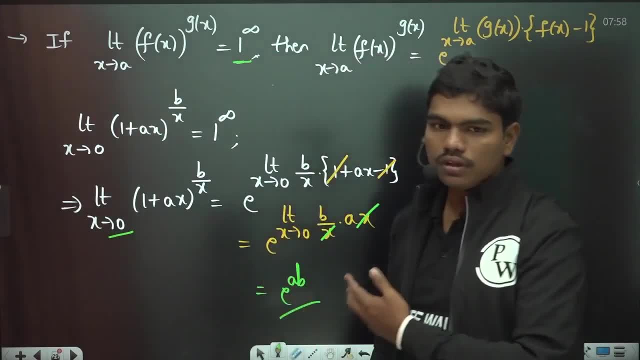 you cannot apply this for zero power. infinity or something like that. okay so, infinity or something like that. okay so, infinity or something like that, okay, so, that's how it's. that's how it's. that's how it's- a very useful result, and also i would 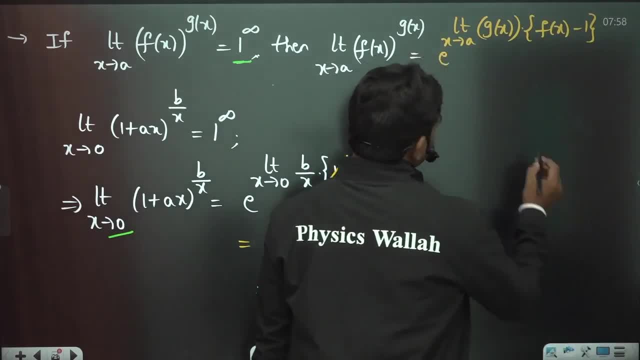 a very useful result and also i would a very useful result and also i would like to give you one more like to give you one more like to give you one more important point: that if important point, that if important point, that if we are getting zero into infinity form, 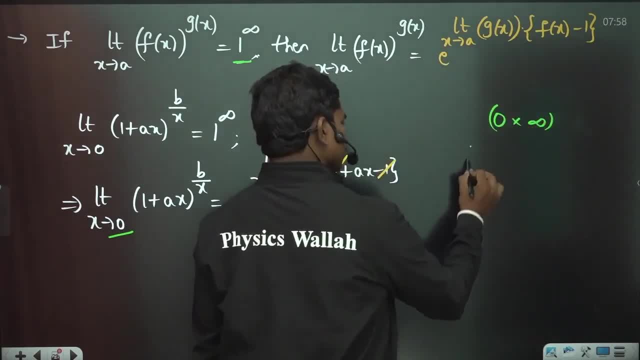 we are getting zero into infinity form. we are getting zero into infinity form anywhere, for example. let us suppose if anywhere, for example. let us suppose if, anywhere, for example. let us suppose if there is two product of two functions, there is two product of two functions. there is two product of two functions, for example. say, limit extends to zero. 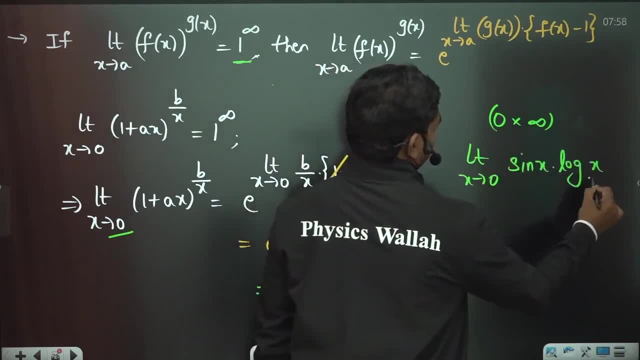 for example, say, limit extends to zero. for example, say, limit extends to zero. sine x into log x. is there? sine x into log x? is there? sine x into log x is there to the base e, for example? okay, so then to the base e, for example. okay, so then. 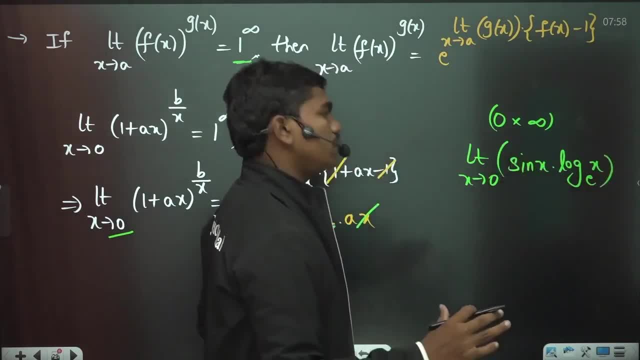 to the base e, for example. okay, so then you will get zero into infinity form. you will get zero into infinity form. you will get zero into infinity form. obviously, then, how you will actually do, obviously then, how you will actually do. obviously then, how you will actually do this. okay, so you will do this as. 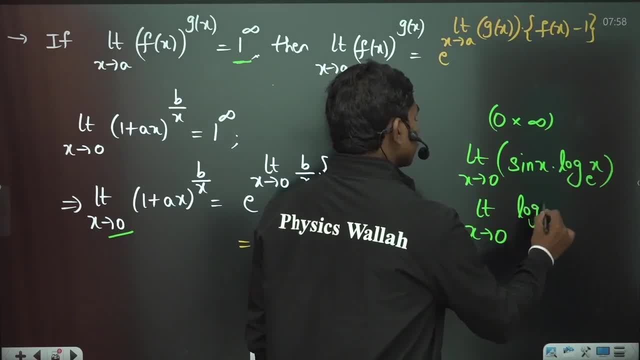 this. okay, so you will do this as this. okay, so you will do this. as this limit extends to zero. this limit extends to zero. this limit extends to zero. log x to the base e divided by one by. log x to the base e divided by one by. log x to the base e divided by one, by sine x, you can write this, okay. or of sine x, you can write this, okay. or of sine x, you can write this, okay. or, of course, you can text. you can write this, course, you can text. you can write this: 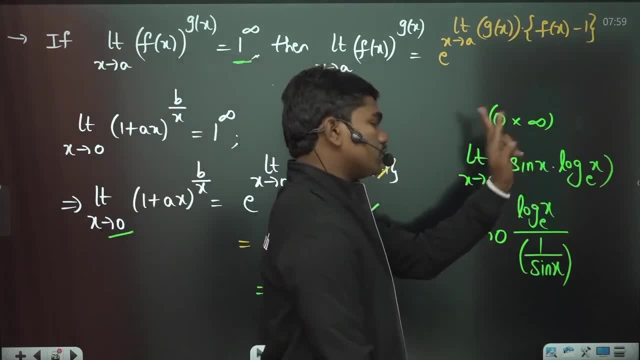 course you can text, you can write this: okay, so when you substitute zero, okay so when you substitute zero, okay, so when you substitute zero, actually, this is of the form zero into, actually, this is of the form zero into, actually, this is of the form zero into infinity. so you don't have any direct 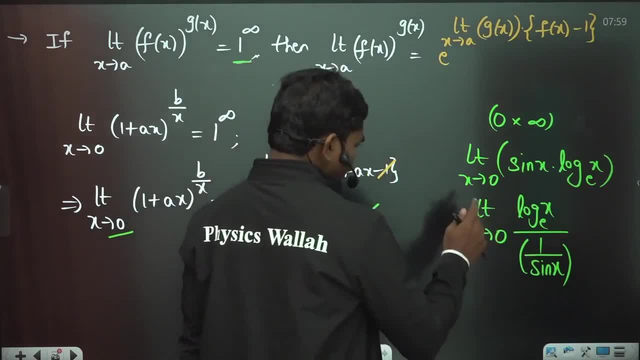 infinity, so you don't have any direct infinity, so you don't have any direct technique. technique, technique. but here you can get this way: limit x, but here you can get this way: limit x, but here you can get this way: limit x tends to zero, tends to zero. 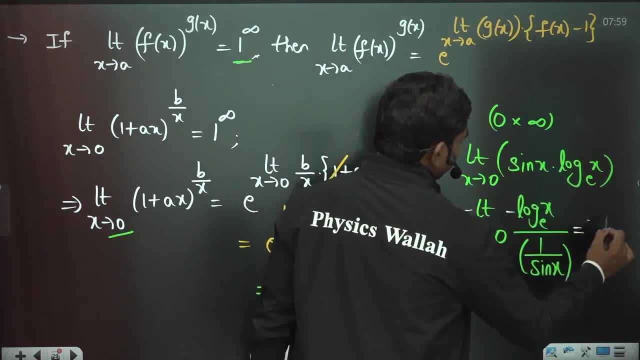 tends to zero. now, this is of the form of course. if you now, this is of the form of course. if you now this is of the form of course. if you adjust a minus sign, this is adjust a minus sign. this is adjust a minus sign. this is minus of infinity by infinity form. okay, 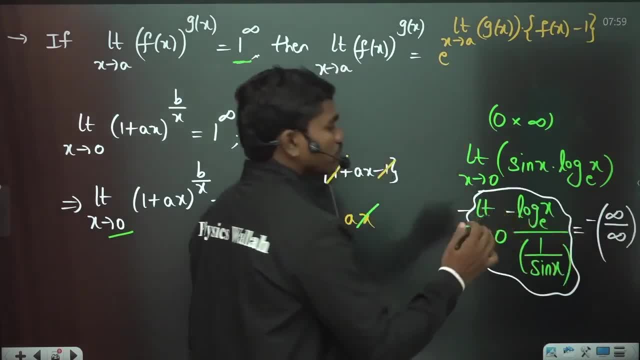 minus of infinity by infinity form. okay. minus of infinity by infinity form, okay. so this limit is now in the form of: so this limit is now in the form of. so this limit is now in the form of infinity by infinity. so now you can. infinity by infinity. so now you can. 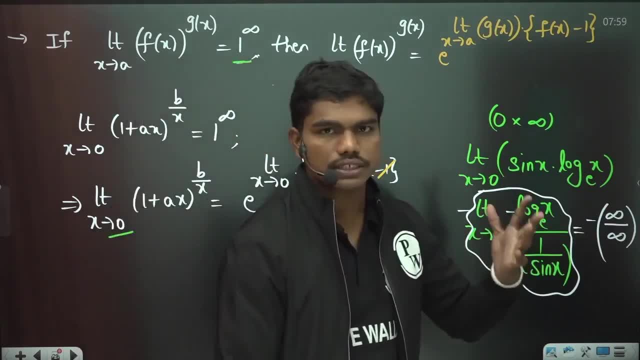 infinity by infinity. so now you can apply l hospital rule by taking log x. apply l hospital rule by taking log x. apply l hospital rule by taking log x, and of course you can text us two. and of course you can text us two. and of course you can text us two functions. you can just differentiate them. 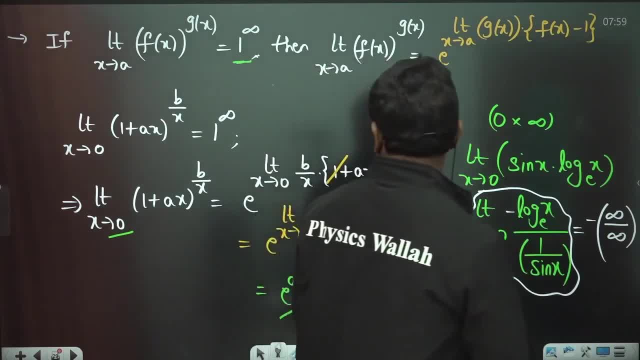 functions, you can just differentiate them. functions, you can just differentiate them and go for the things actually okay, so, and go for the things actually okay, so, and go for the things actually okay, so. that's how this one point form is. that's how this one point form is. 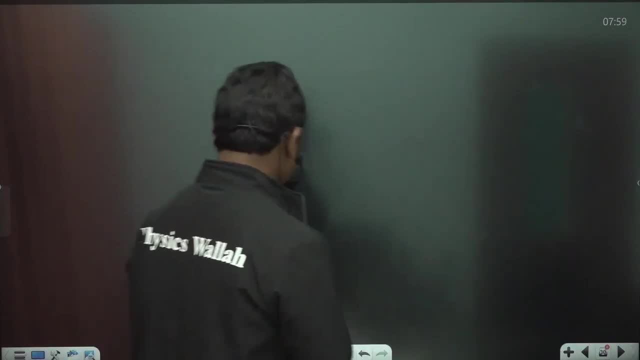 that's how this one point form is actually a bit important for you, okay, actually a bit important for you, okay, actually a bit important for you, okay, and i would like to give you one more, and i would like to give you one more, and i would like to give you one more result. 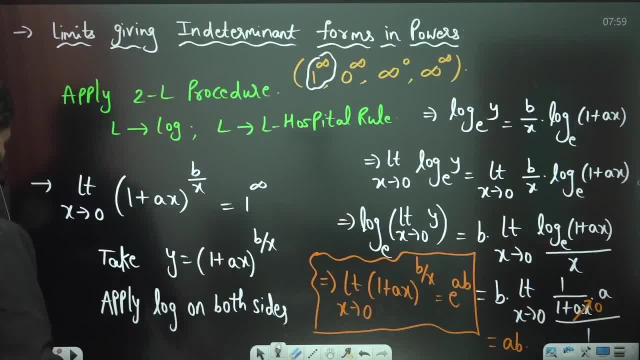 result: result: one more standard limit. that limit is how? one more standard limit. that limit is how. one more standard limit. that limit is how many. we have given you many. we have given you many. we have given you, okay, some number seven. let us say: okay, some number seven. let us say: 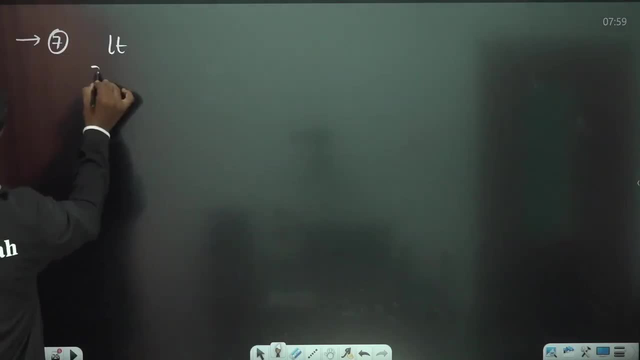 okay, some number seven, let us say seven limit extends to zero one power x. or you can write a power x, one power x, or you can write a power x, one power x, or you can write a power x plus b power x by two plus b power x by two. 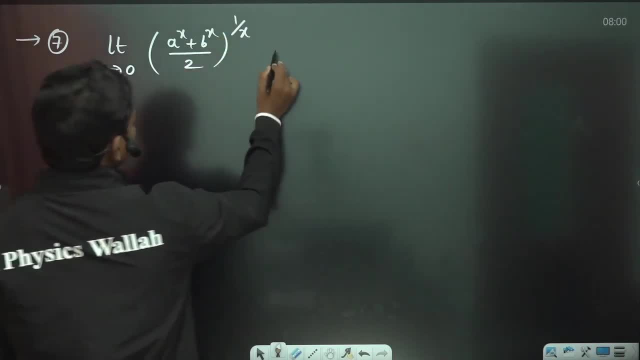 plus b power x by two, whole power, one by x. so again, this is whole power, one by x. so again, this is whole power, one by x. so again, this is of the form: one point, infinity of the form. one point, infinity of the form: one point, infinity. so if you see, the answer is going to be: 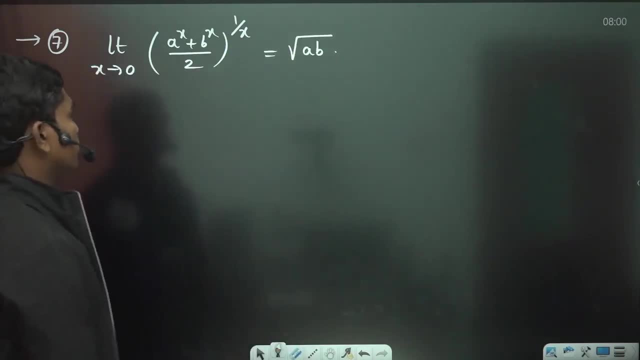 so, if you see the answer is going to be so, if you see the answer is going to be square root of a b, square root of a- b, square root of a b. okay, so you are going to get, uh, square root. okay, so you are going to get, uh, square root. 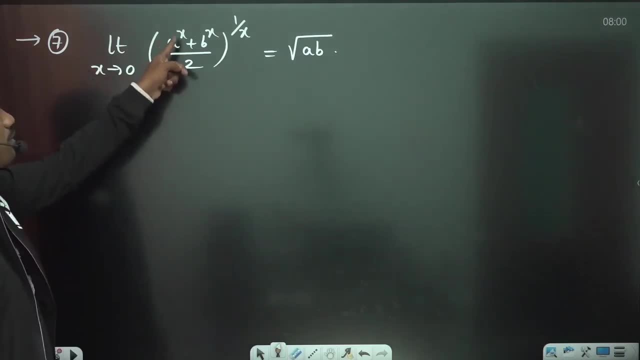 okay, so you are going to get, uh, square root of a, b, basically here, of a, b, basically here, of a, b, basically here, because you can see when you substitute, because you can see when you substitute, because you can see when you substitute: zero, a power, zero is one plus b power. 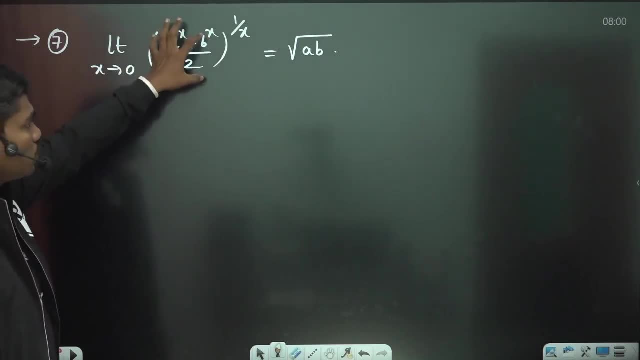 zero a power. zero is one plus b power. zero a power zero is one plus b power. zero is one, so one plus one is two. zero is one, so one plus one is two. zero is one, so one plus one is two. two by two is one. so this total bracket. 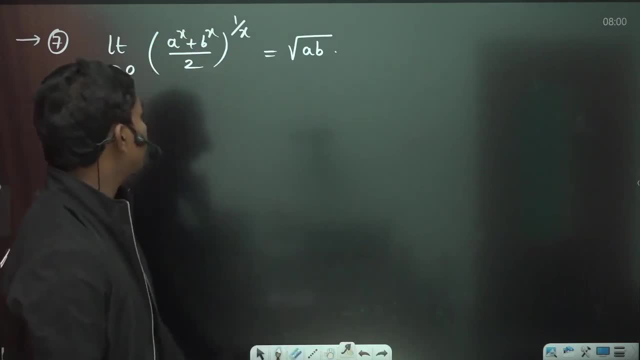 by two is one. so this total bracket by two is one. so this total bracket gives you one, gives you one, gives you one, and this one by x gives you infinity form, and this one by x gives you infinity form, and this one by x gives you infinity form. so, if you see, 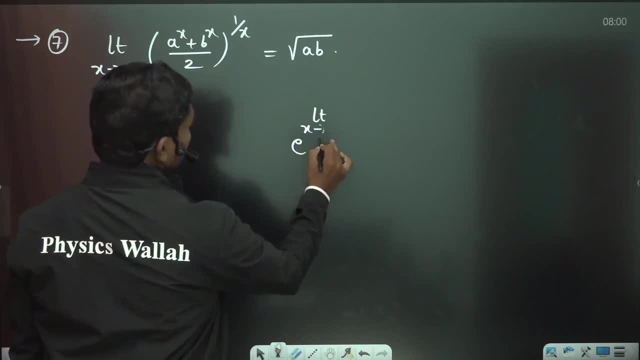 so if you see, so, if you see, if you simplify e power limit extends to a, if you simplify e power limit extends to a, if you simplify e power limit extends to a and all, you will get a square root of a, b and all. you will get a square root of a, b. 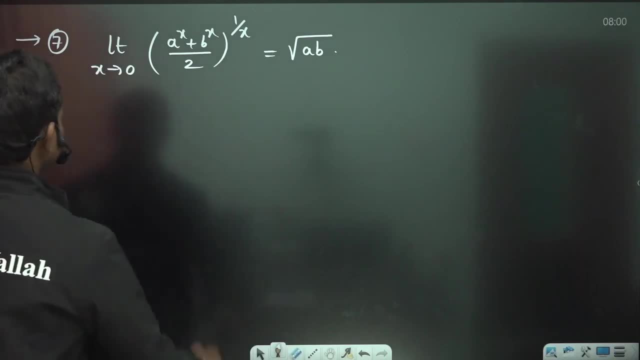 and all. you will get a square root of a- b. basically okay, basically okay, basically okay. so square root of a- b is the correct. so square root of a- b is the correct. so square root of a- b is the correct answer for this. similarly, if you have one, 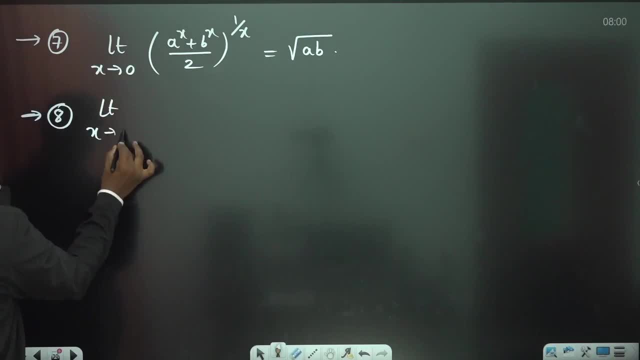 answer for this. similarly, if you have one answer for this, similarly, if you have one more, more, more. for example, limit extends to zero. for example, limit extends to zero. for example, limit extends to zero. a power x plus b power x plus c power x. a power x plus b. power x plus c power x. 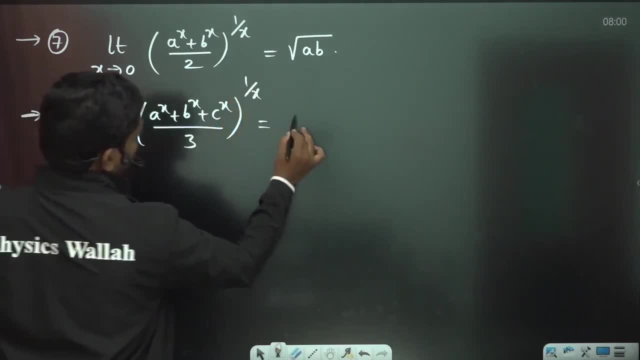 a power x plus b power x plus c power x by 3. whole power 1 by x. so this value is by 3 whole power 1 by x. so this value is by 3 whole power 1 by x. so this value is going to be cube root of. 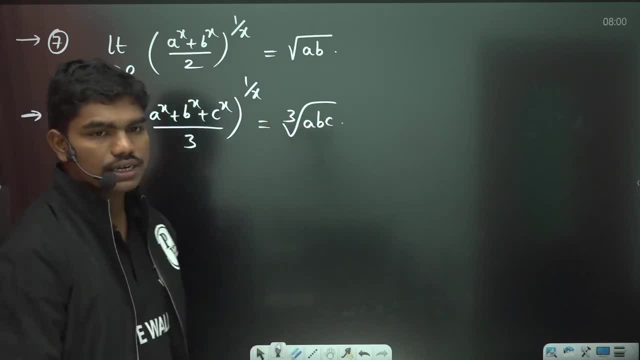 going to be cube root of going to be cube root of abc. this is what you have here. okay, so abc, this is what you have here. okay, so abc, this is what you have here. okay, so these are the limits, some. these are the limits. some. these are the limits some. similarly, if you have one, power x plus. 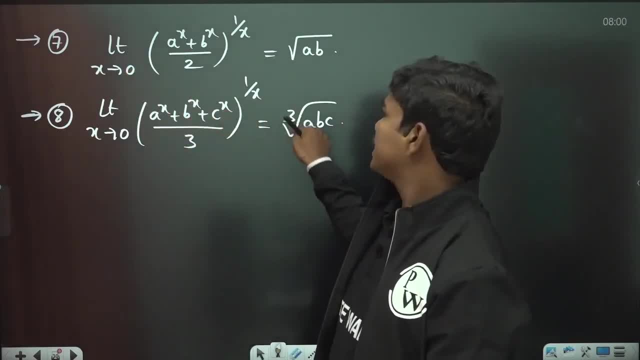 similarly, if you have one power x plus, similarly, if you have one power x plus two power x plus three power x, and so on, two power x plus three power x, and so on, two power x plus three power x, and so on, n power x, then this is n thought of n. 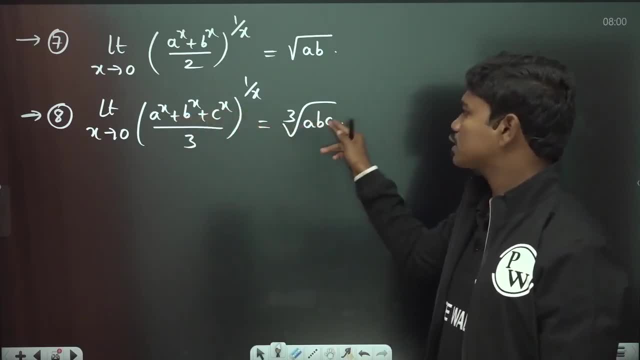 n power x, then this is n thought of n. n power x, then this is n thought of n. factorial basically okay. so because the factorial basically okay. so because the factorial basically okay. so because the n values and product of 1 into 2, into 3, 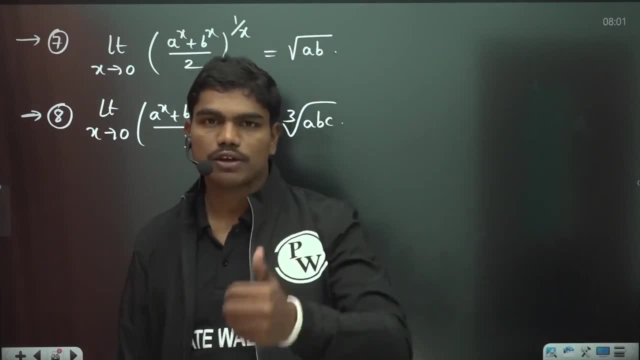 n values and product of 1 into 2 into 3, n values and product of 1 into 2 into 3, and so on, until n gives you n factorial, and so on, until n gives you n factorial, and so on, until n gives you n factorial. so n thought of n factorial is what you. 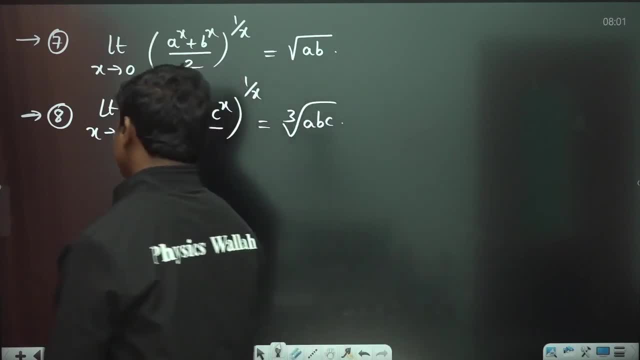 so n thought of n factorial is what you so n thought of n factorial is what you will get in general. okay, now i'll give, will get in general. okay, now i'll give, will get in general. okay, now i'll give you one more, you one more. 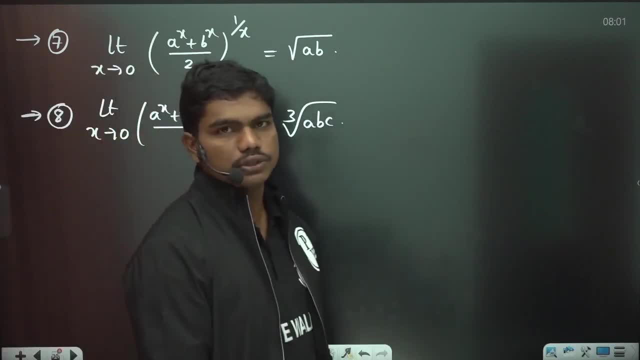 you one more: uh, okay, fine, these limits are generally. uh, okay, fine, these limits are generally. uh, okay, fine, these limits are generally limits that we use in day to day, limits that we use in day to day, limits that we use in day to day. but i would like to give you one special. but i would like to give you one special. but i would like to give you one special kind of limits, because sometimes again kind of limits, because sometimes again kind of limits, because sometimes again, you know you have some gate questions on. you know you have some gate questions on. 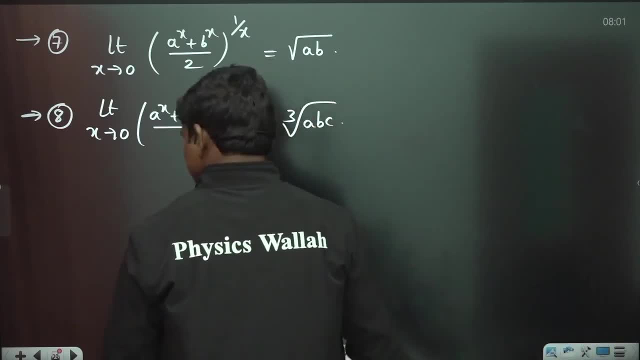 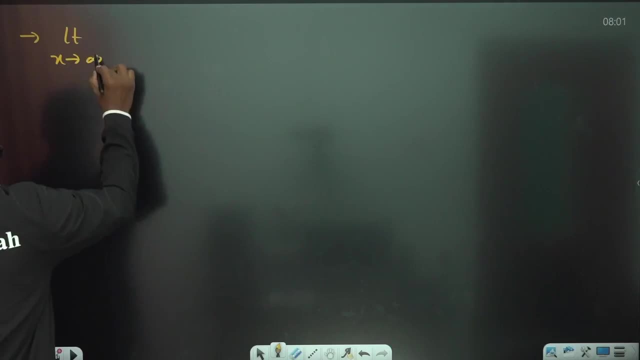 you know you have some gate questions on that. so look, i'll give you that. so look, i'll give you that. so look, i'll give you limit limit. limit extends to a or extends to infinity. you extends to a or extends to infinity. you extends to a or extends to infinity. you can say: limit extends to infinity. 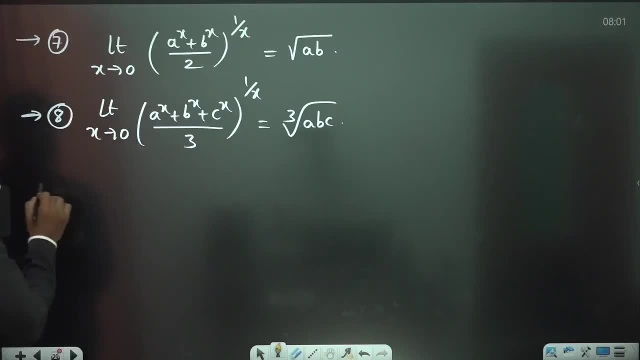 can say limit extends to infinity. can say limit extends to infinity. okay, before this, i would give one limit extends to infinity. okay, before this, i would give one limit extends to infinity. okay, before this, i would give one limit here, here, here, look nine. limit extends to zero. 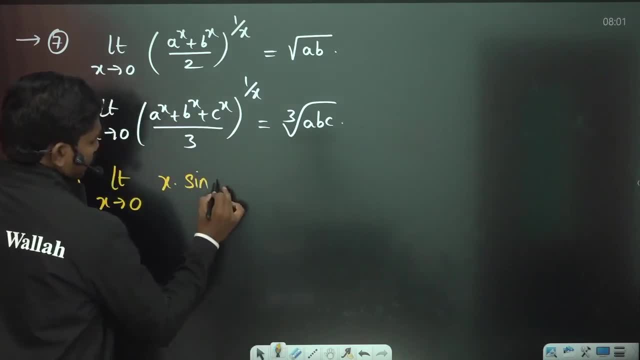 look, nine limit extends to zero. look, nine limit extends to zero. x into sine x. or you can say x into x into sine x, or you can say x into x into sine x, or you can say x into sine x. okay, this is anyhow zero known to. 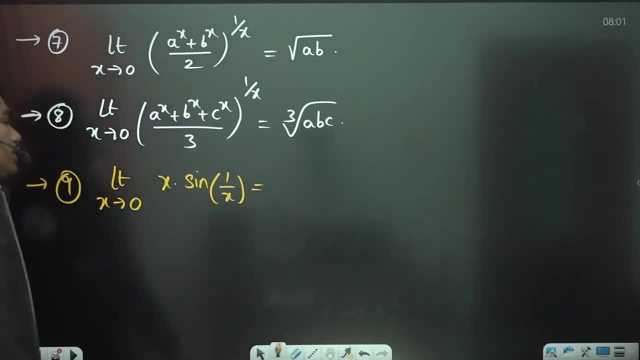 sine x. okay, this is anyhow zero known to sine x. okay, this is anyhow zero known to you. you, you sine 1 by x. let us say okay, so this is x sine 1 by x. let us say okay, so this is x sine 1 by x. let us say okay, so this is x into sine 1 by x, because 1 by x is. 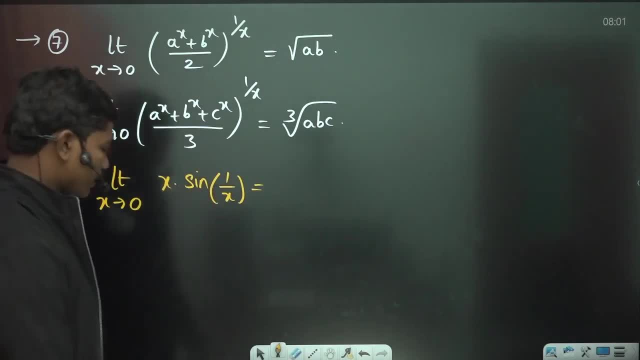 into sine 1 by x. because 1 by x is into sine 1 by x, because 1 by x is infinity. so x into sine 1 by x. okay now, infinity. so x into sine 1 by x. okay now, infinity. so x into sine 1 by x. okay now, when you add x into sine 1 by x. 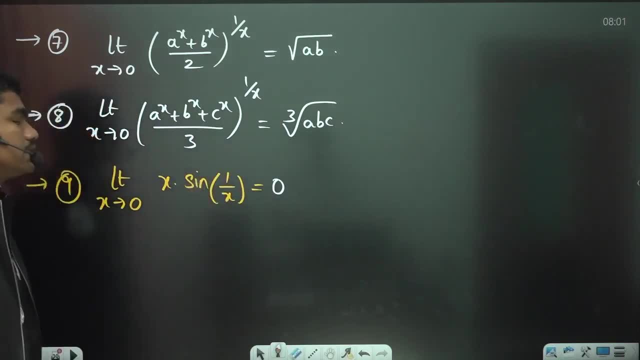 when you add x into sine 1 by x. when you add x into sine 1 by x. look, the answer for this is straight away. look, the answer for this is straight away. look, the answer for this is straight away: zero actually. why it is zero? because 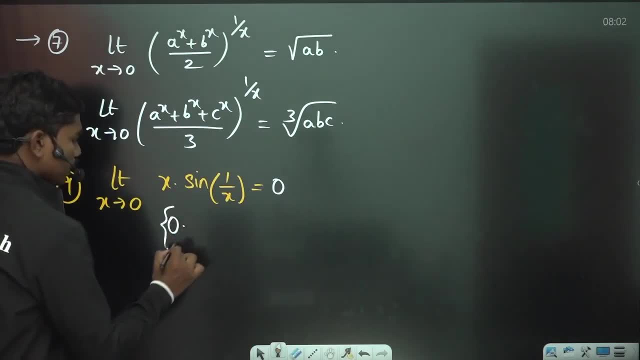 zero actually. why it is zero? because zero actually. why it is zero? because you can see zero into. you can see zero into. you can see zero into some finite value in minus one comma one, some finite value in minus one comma one, some finite value in minus one comma one, correct, whatever might be the value of x. 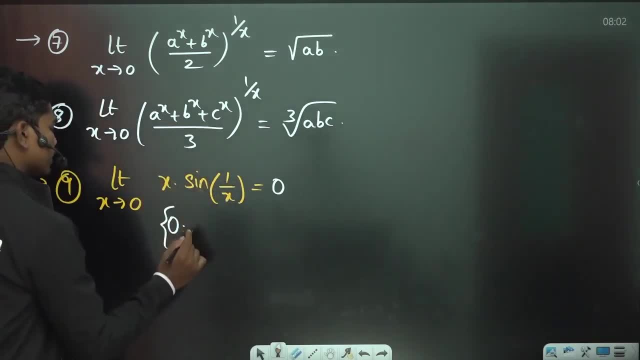 correct whatever might be the value of x. correct whatever might be the value of x. this value is always some finite number. this value is always some finite number. this value is always some finite number which lies in between minus one and one, which lies in between minus one and one. 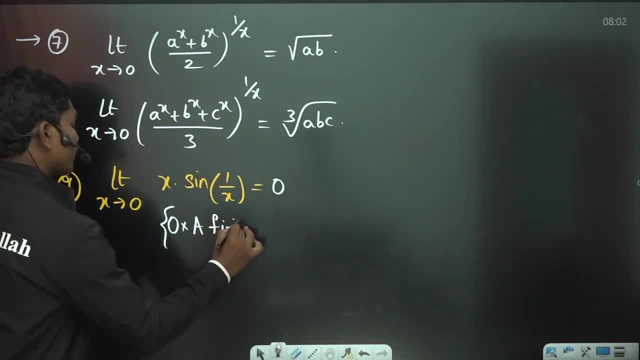 which lies in between minus one and one. so zero into a finite value, so zero into a finite value. so zero into a finite value, a finite value in a finite value, in a finite value, in minus one comma one. so that's why, if you minus one comma one, so that's why, if you 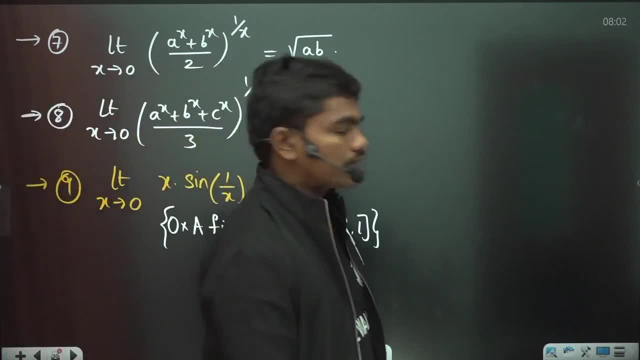 minus one comma one. so that's why, if you see zero into some finite number, will see zero into some finite number. will see zero into some finite number. will always give you zero actually in that. always give you zero actually in that. always give you zero actually in that case. okay. so that's why this limit is. 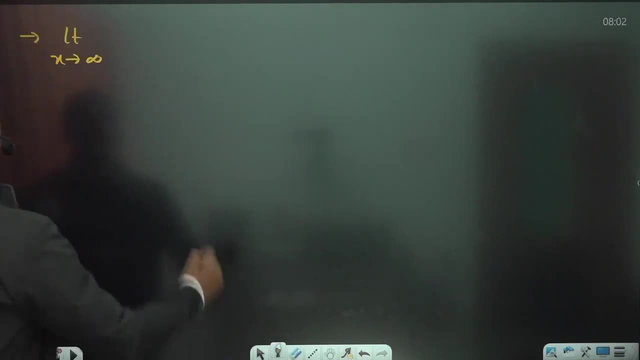 case. okay, so that's why this limit is case. okay, so that's why this limit is basically, basically, basically zero. okay, now, let us come to this zero. okay, now, let us come to this zero. okay, now, let us come to this infinity thing. so limit extends to: 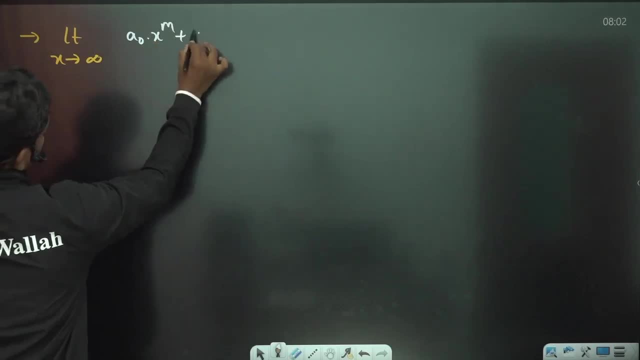 infinity thing, so limit extends to infinity thing, so limit extends to infinity. a naught into x. power m plus a infinity. a naught into x. power m plus a infinity. a naught into x. power m plus a 1 into x. power m minus 1 plus a 2 into x. 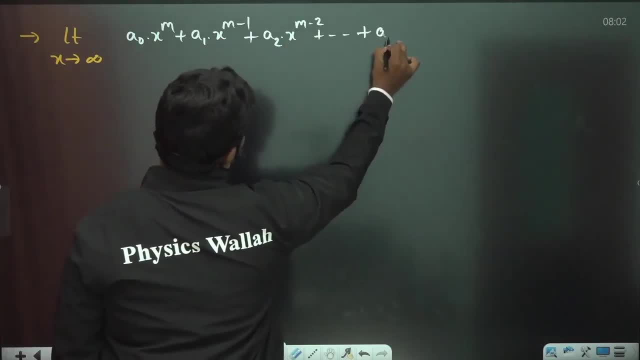 1 into x. power m minus 1 plus a. 2 into x. 1 into x. power m minus 1 plus a 2 into x. power m minus 2, and so on. a m which is power m minus 2, and so on, a m which is. 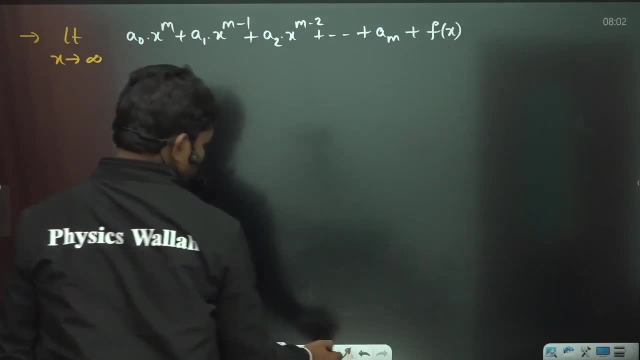 power, m minus 2 and so on, a m, which is some constant plus f of X, some constant plus f of X, some constant plus f of X. divided by this, divided by b naught x power n plus b 1 into x power, b naught x power n plus b: 1 into x power. 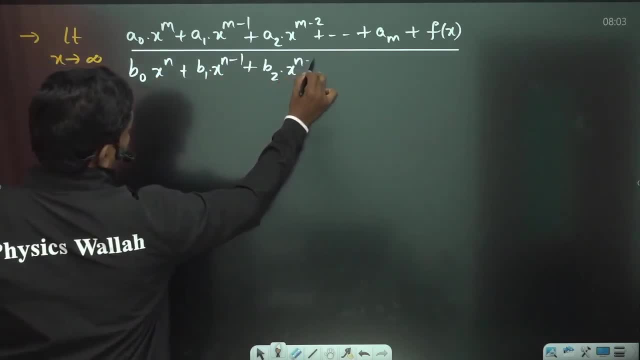 b naught x power n minus 1. b naught x power n plus b 1 into x power n minus 1. b naught x power n plus b 1 into x power n minus 1 plus b 2 times x power n minus 2. 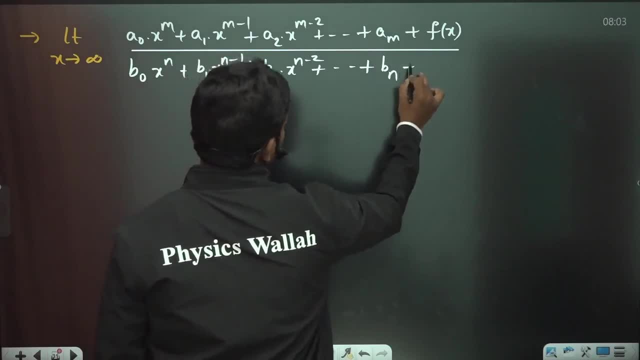 plus b 2 times x power n minus 2 plus b 2 times x power n minus 2 plus, and so on, plus b? n. let us say plus G plus, and so on, plus b? n. let us say plus G plus, and so on, plus b? n. let us say plus G of X. where? 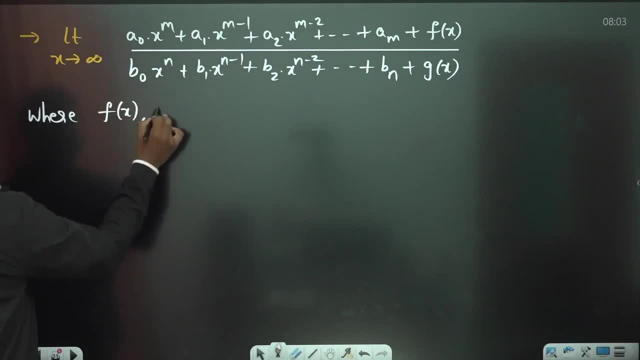 of X. where of X, where F of X comma. G of X are finite valued. F of X comma. G of X are finite valued. F of X comma. G of X are finite valued functions and G of X are finite valued functions and G of X are finite valued. 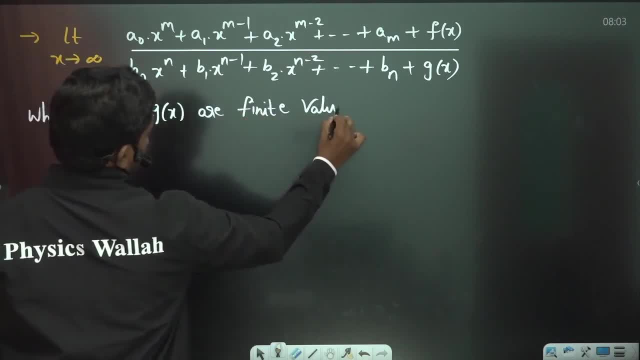 functions and G of X are finite valued functions. finite valued functions, so functions- finite valued functions, so functions- finite valued functions. so what is the meaning of finite valued? what is the meaning of finite valued? what is the meaning of finite valued functions? finite valued functions, functions- finite valued functions. 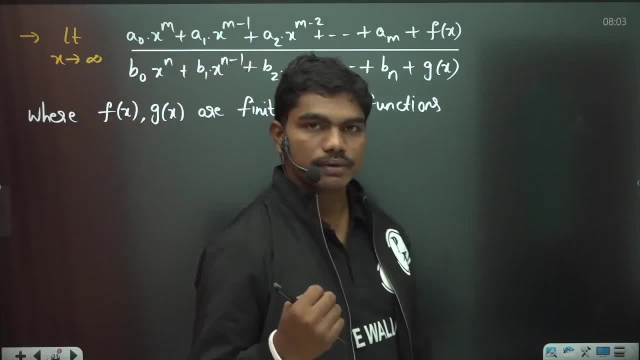 functions, finite valued functions, basically whatever the value is placing, basically, whatever the value is placing, basically whatever the value is placing, whatever the value is substituting place, whatever the value is substituting place, whatever the value is substituting place of X. this F of X and G of X are always. 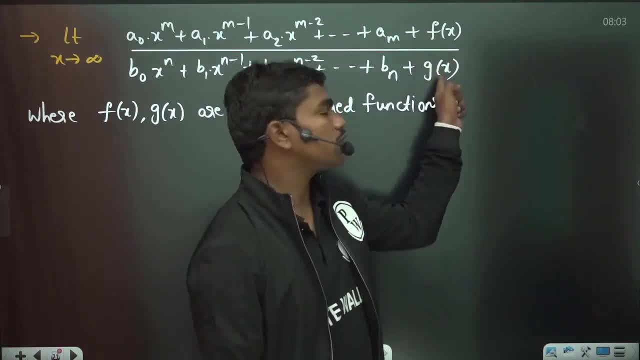 of X, this F of X and G of X are always of X, this F of X and G of X are always some finite numbers. okay, for example, you some finite numbers. okay, for example, you some finite numbers. okay, for example, you have just seen, if I put sine, X and cos, 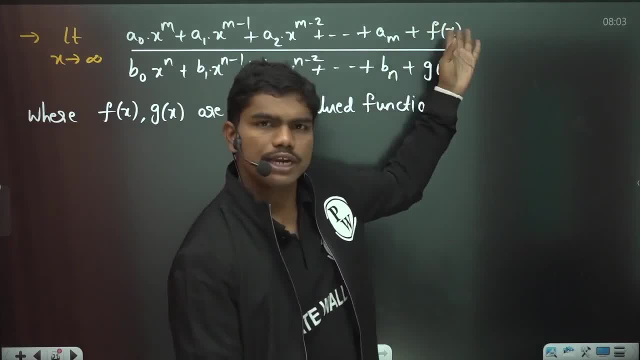 have just seen if I put sine X and cos. have just seen if I put sine X and cos, X here. whatever might be the value of X, X here, whatever might be the value of X, X here, whatever might be the value of X, these two are always finite sine 2x cos. 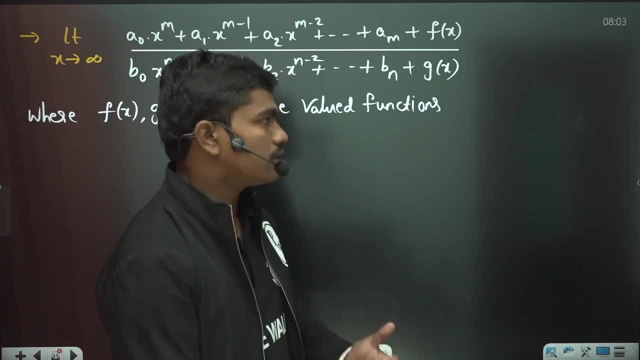 these two are always finite sine 2x cos. these two are always finite sine 2x cos square X. all these values, basically all square X, all these values, basically all square X, all these values, basically, all these are finite. some finite functions. so these are finite, some finite functions, so. 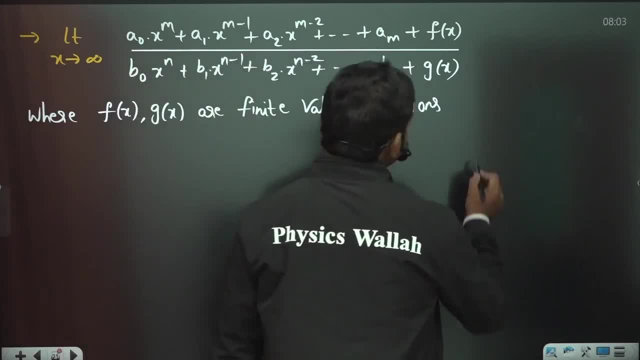 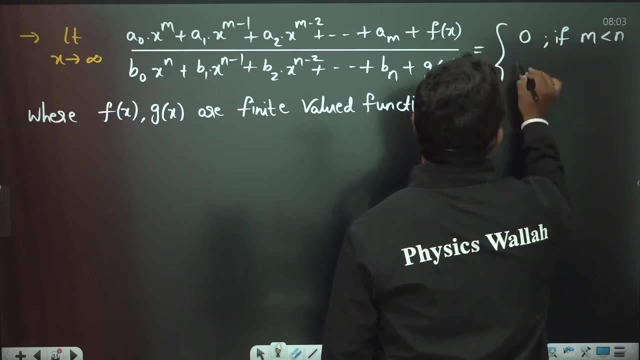 these are finite, some finite functions. so that's why, if you see if these are, that's why, if you see if these are, that's why, if you see if these are finite functions, then this limit is equal finite functions, then this limit is equal finite functions, then this limit is equal to 0. if M less than n, a naught by B naught. 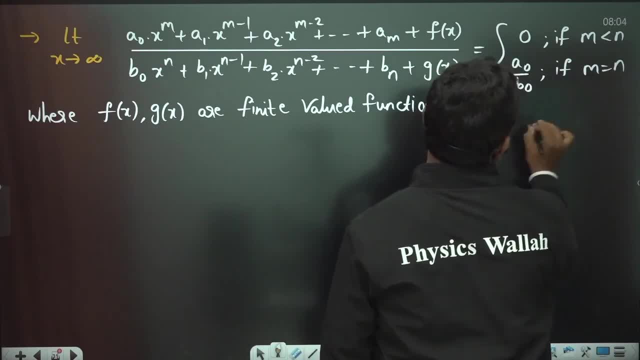 to 0 if M less than n a naught by B naught to 0 if M less than n a naught by B naught. if M is equal to n. infinity. if M is. if M is equal to n. infinity if M is. if M is equal to n infinity. if M is greater than n. okay, so these are very. 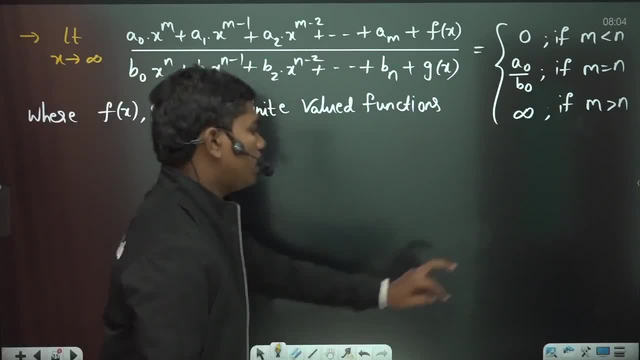 greater than n. okay, so these are very greater than n. okay, so these are very important results. because if you see important results, because if you see important results, because if you see many times in exams, you will encounter many times in exams, you will encounter many times in exams you will encounter questions like this: of course I'm not. 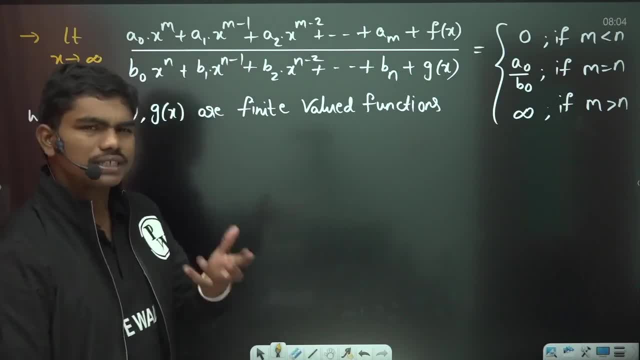 questions like this. of course I'm not questions like this. of course I'm not proving this again. I'm not showing the proving this again. I'm not showing the proving this again. I'm not showing the derivation of this. it's very simple it. derivation of this. it's very simple it. 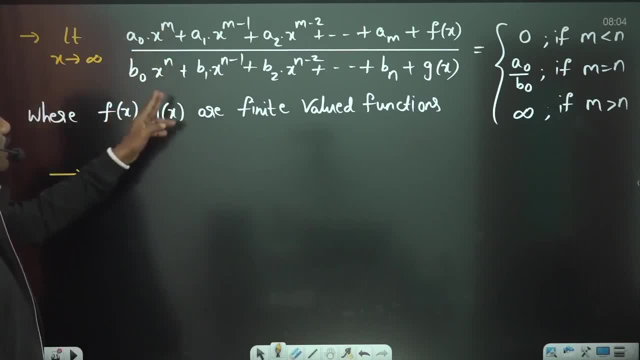 derivation of this. it's very simple. it you need not call this derivation. if you, you need not call this derivation. if you, you need not call this derivation. if you take X power M and X power n here, then take X power M and X power n here, then 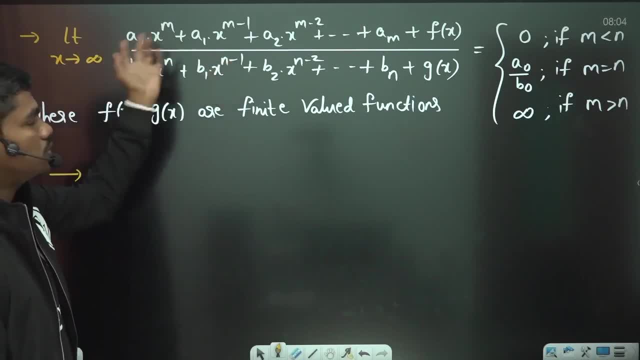 take X power M and X power n here, then if you put X is equal to if X is, if you put X is equal to if X is, if you put X is equal to if X is equal to, if X is equal to if X is equal to n. so in that case, 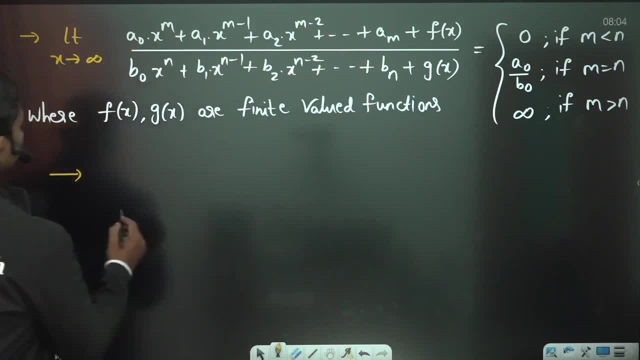 equal to if X is equal to if X is equal to n. so in that case, equal to if X is equal to if X is equal to n. so in that case, if you substitute, and all you will get if you substitute and all you will get, if you substitute and all you will get, this three results actually. okay, why I'm? 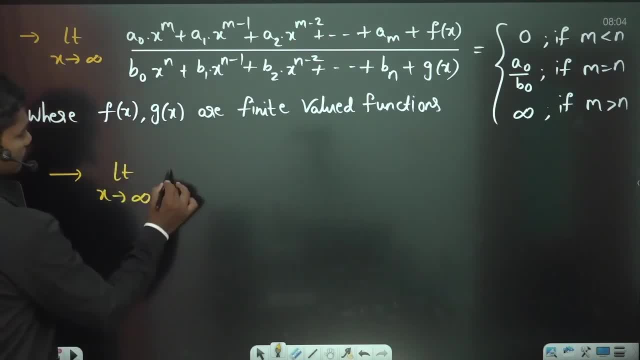 this. three results actually okay. why I'm this? three results actually okay. why I'm telling you this in exams? you will get telling you this in exams. you will get telling you this in exams. you will get questions like this: X tends to infinity. questions like this: X tends to infinity. 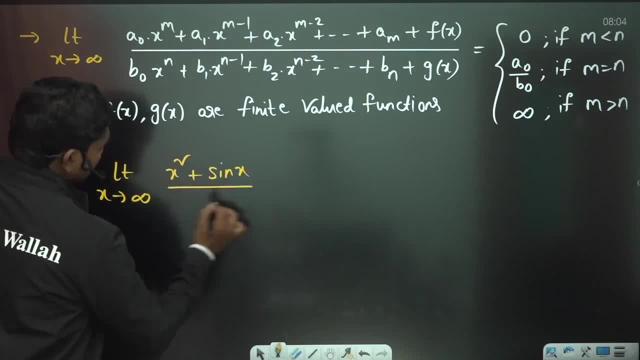 questions like this. X tends to infinity. X square plus sine X by X square plus X square plus sine X by X square plus X square plus sine X by X square plus cos 2x, something like this, they'll give cos 2x. something like this they'll give. 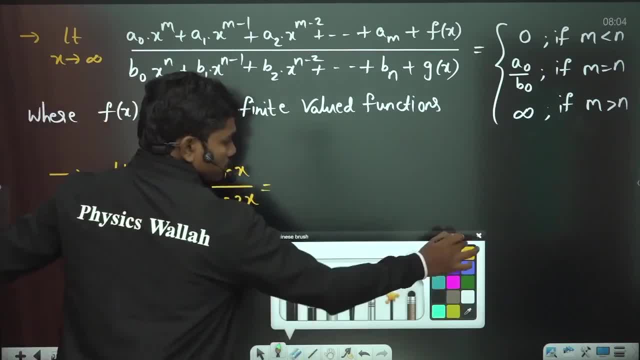 cos 2x, something like this, they'll give you okay. so if you see you, okay, so if you see you okay, so if you see, these two are finite valued functions and these two are finite valued functions, and these two are finite valued functions and here the coefficient is one, here also, 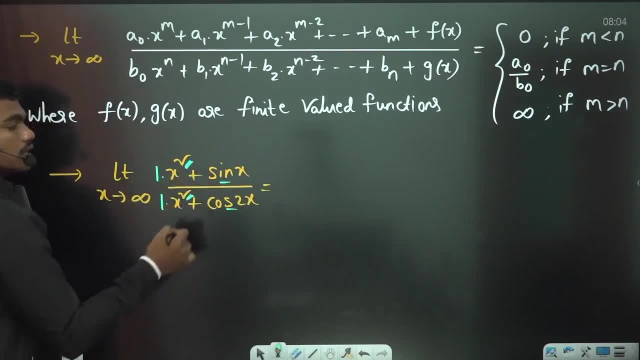 here the coefficient is one, here also. here the coefficient is one. here also the coefficient is one, and this powers the coefficient is one and this powers: the coefficient is one and this powers are same. M is equal to n. so in that case are same. M is equal to n. so in that case, 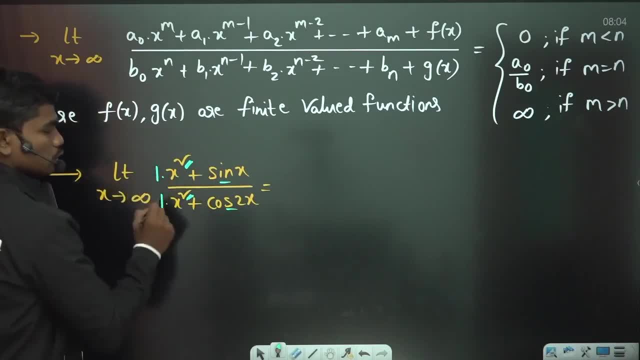 are same. M is equal to n. so in that case, if M is equal to n, the value of this, if M is equal to n, the value of this, if M is equal to n, the value of this. limit is ratio of this coefficients. so limit is ratio of this coefficients. so 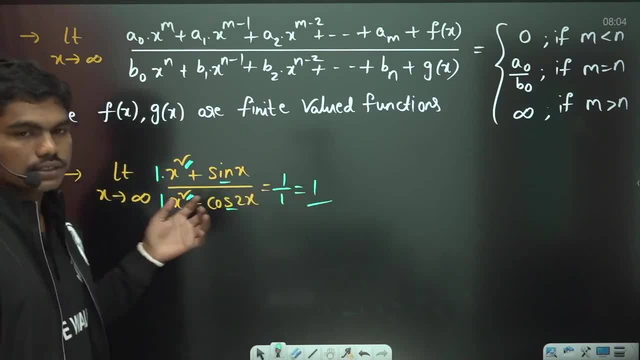 limit is ratio of this coefficients. so 1 by 1, which is 1, that's it finished, okay. 1 by 1, which is 1, that's it finished, okay. 1 by 1, which is 1, that's it finished, okay. so that's how actually this result is. 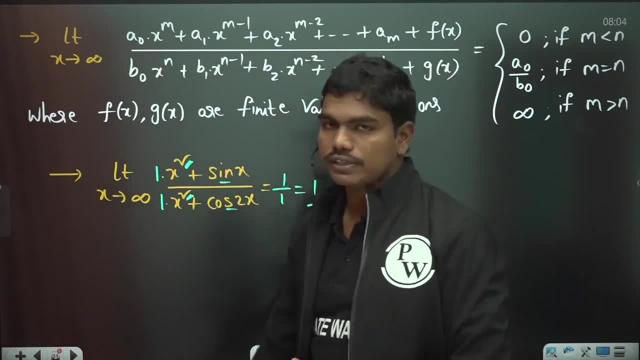 so that's how actually this result is, so that's how actually this result is actually helpful for you. so you know actually helpful for you, so you know actually helpful for you. so you know, basically this is one very good limit, basically this is one very good limit. 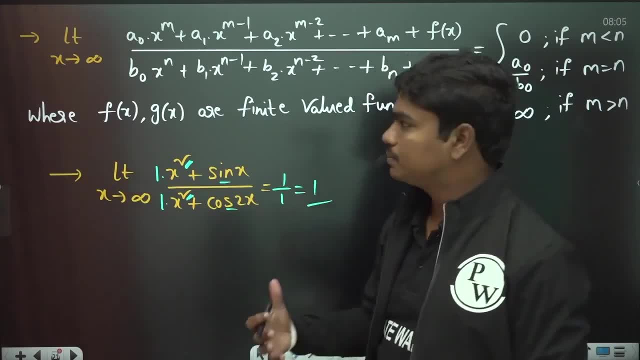 basically, this is one very good limit actually. okay means this limit is actually okay, means this limit is actually okay, means this limit is actually one way you know some powerful actually one way, you know some powerful actually, one way you know some powerful kind of limit, because many questions 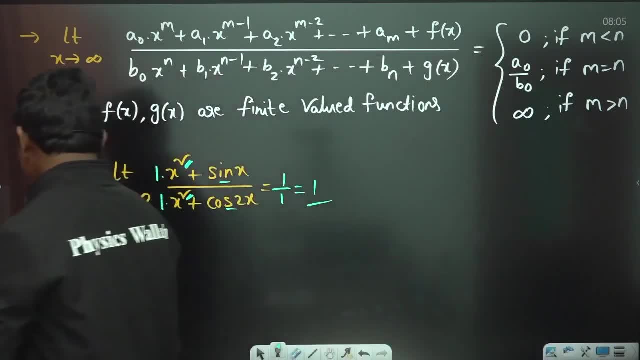 kind of limit because many questions. kind of limit because many questions you will be able to solve directly here. you will be able to solve directly here, you will be able to solve directly here. okay, now, I'll give you one limit here. okay, now I'll give you one limit here. 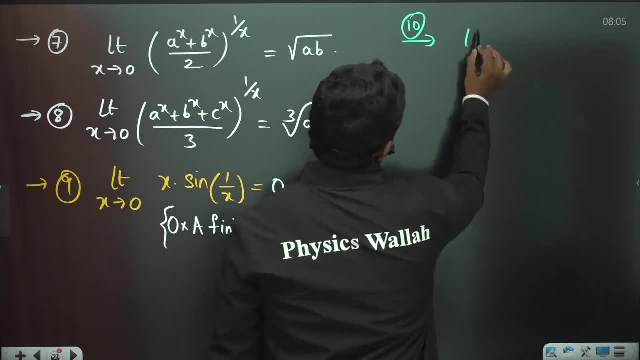 okay, now I'll give you one limit here again, again, again. limit X tends to 0: 1 by X. this value limit X tends to 0: 1 by X. this value limit X tends to 0: 1 by X. this value does not exist. okay, this does not exist. 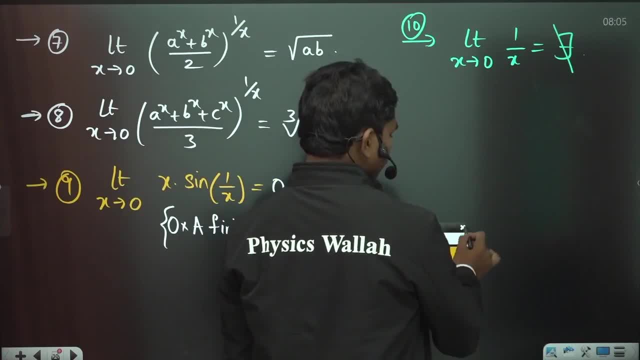 does not exist. okay, this does not exist, does not exist. okay, this does not exist. because you can clearly see if you draw, because you can clearly see if you draw, because you can clearly see if you draw. the graph of that yesterday's class I. the graph of that yesterday's class I. 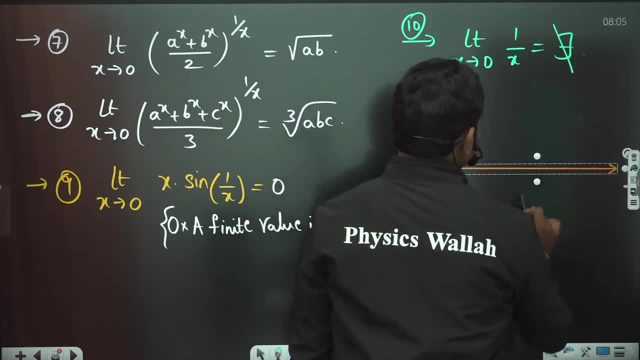 the graph of that yesterday's class. I have given you when sine X by X. I'm have given you when sine X by X. I'm have given you when sine X by X. I'm doing so if you see if this is doing so, if you see if this is. 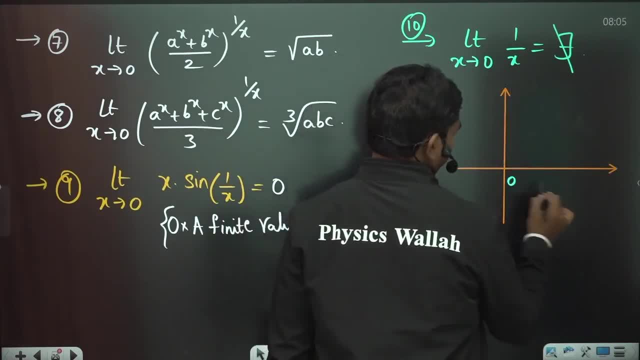 doing so. if you see, if this is something like this 0 X, something like this 0 X, something like this 0 X, let me slightly okay now my point of. let me slightly okay now my point of. let me slightly okay now, my point of interest is only till this point, so this: 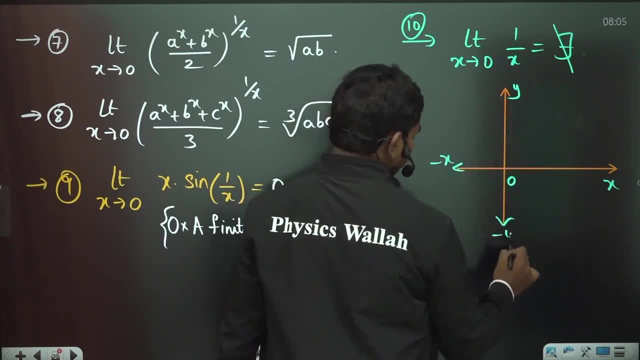 interest is only till this point. so this interest is only till this point. so this is minus X, Y and minus Y, then you know, is minus X, Y and minus Y. then you know, is minus X, Y and minus Y, then you know one thing: if I dollar is equal to 1 by X, 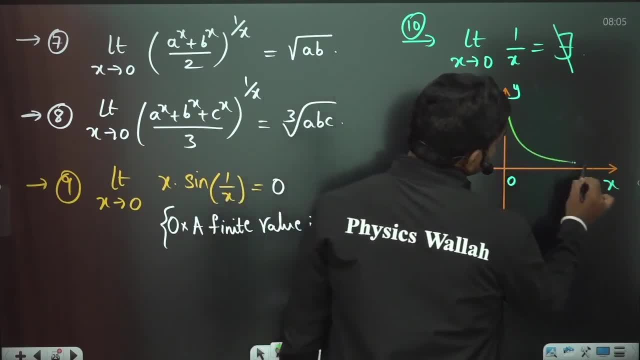 one thing: if I dollar is equal to 1 by X. one thing: if I dollar is equal to 1 by X. graph. it looks like this. here it looks graph. it looks like this. here it looks graph. it looks like this. here it looks like this. and here it looks something. 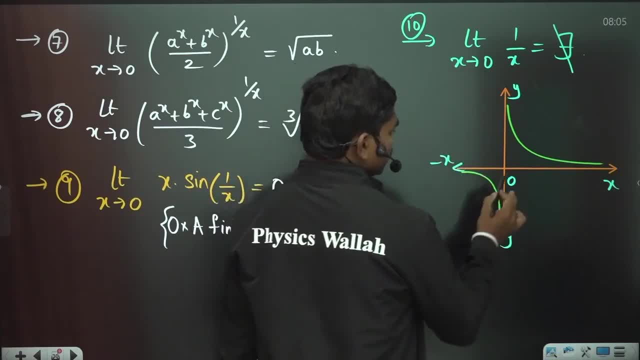 like this. and here it looks something like this, and here it looks something like this cut, so we can see it extends like this cut, so we can see it extends like this cut, so we can see it extends to: 0 plus means basically in this right, to 0 plus means basically in this right. 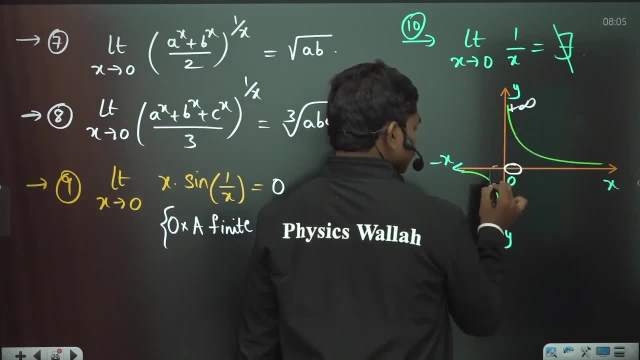 to 0 plus means basically: in this right neighborhood, the value is plus infinity neighborhood, the value is plus infinity neighborhood, the value is plus infinity. in the left neighborhood, the value is in the left neighborhood, the value is in the left neighborhood, the value is minus infinity. that's why left limit and 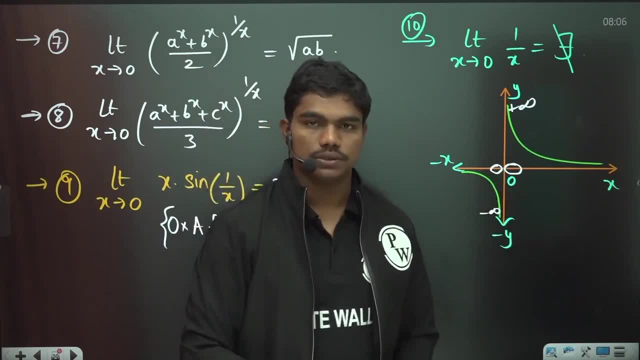 minus infinity. that's why left limit and minus infinity. that's why left limit and right limit. both are not same, so that's right limit. both are not same, so that's right limit. both are not same, so that's why this limit does not exist. okay, so I 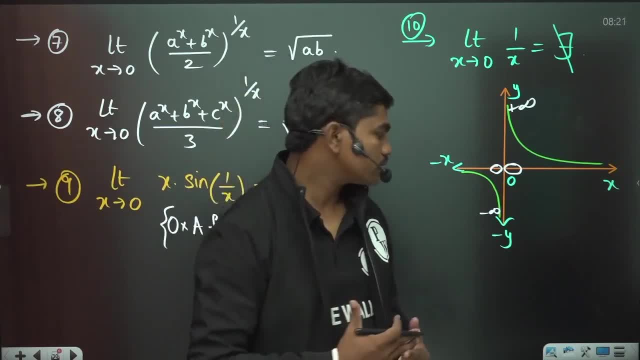 why this limit does not exist, okay, so I. why this limit does not exist, okay, so I will stop the video here. thank you, okay, will stop the video here. thank you, okay, will stop the video here. thank you, okay. so now let us continue after this, so I. 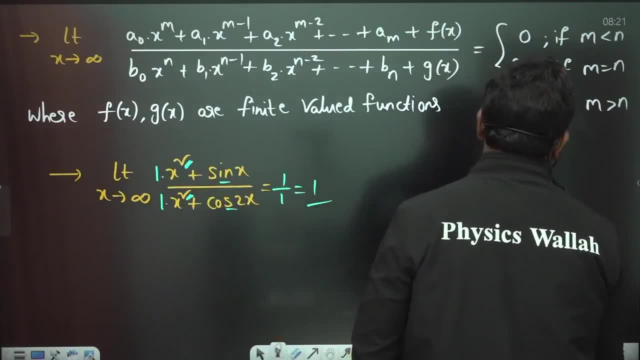 so now let us continue after this. so I so now let us continue after this. so I have given you this results basically, in have given you this results, basically, in have given you this results, basically in the case of limits. okay, now let us move the case of limits. okay, now let us move. 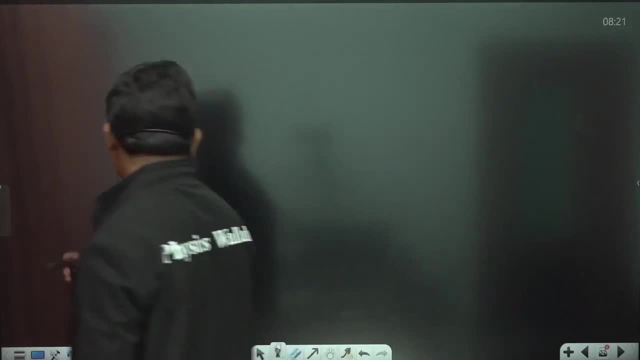 the case of limits. okay, now let us move on to one very important result again, in on to one very important result again, in on to one very important result again. in limits, that if limit extends to a f of x. limits, that if limit extends to a f of x. 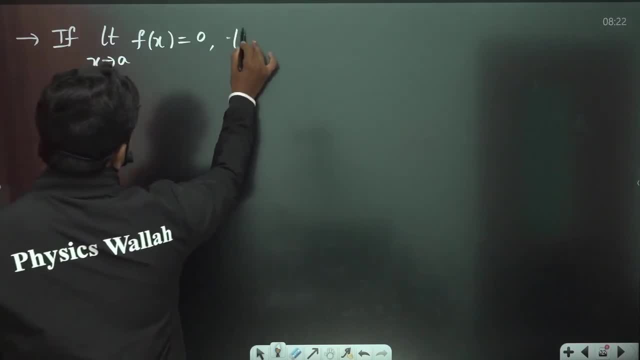 limits, that if limit extends to a f of x is equal to 0, for example, then limit is equal to 0, for example, then limit is equal to 0, for example, then limit extends to a f of X power, f of X. this extends to a f of X power, f of X. this 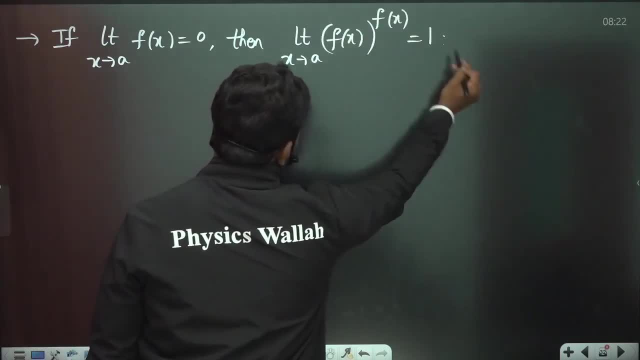 extends to a f of X, this value is equal to 1, actually okay. and of value is equal to 1, actually okay. and of value is equal to 1, actually okay. and of course, please make a note 0, power 0 is course. please make a note 0, power 0 is. 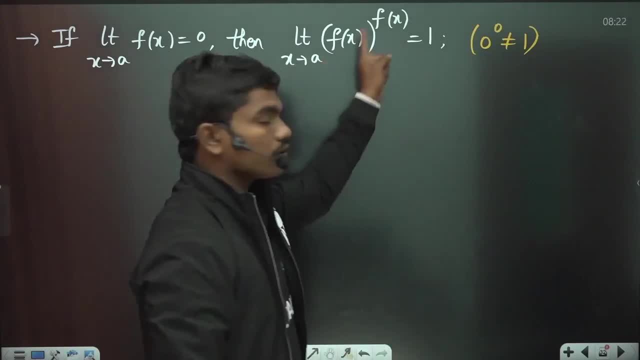 course. please make a note: 0 power 0 is not equal to 1, actually okay. this is one not equal to 1, actually okay. this is one not equal to 1, actually okay. this is one. not because of 0 power 0 is equal to 1. 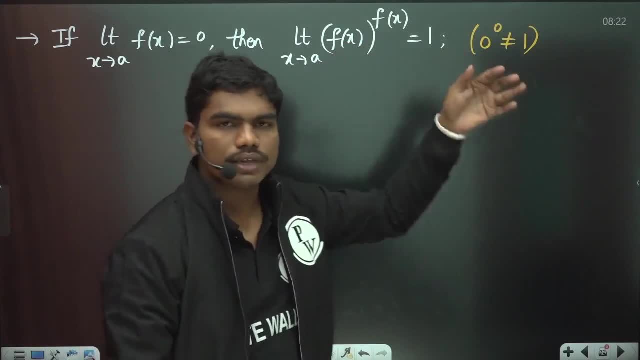 not because of 0 power 0 is equal to 1. not because of 0 power 0 is equal to 1. there is some different logic again you. there is some different logic again you. there is some different logic. again. you get 0 power 0 form. then you need to. 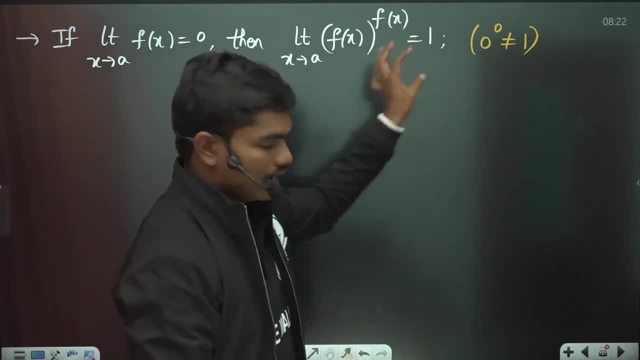 get 0 power- 0 form, then you need to get 0 power- 0 form, then you need to apply to log. I mean to else one log at apply to log. I mean to else one log at apply to log. I mean to else one log at the mud one L Hospital and after final. 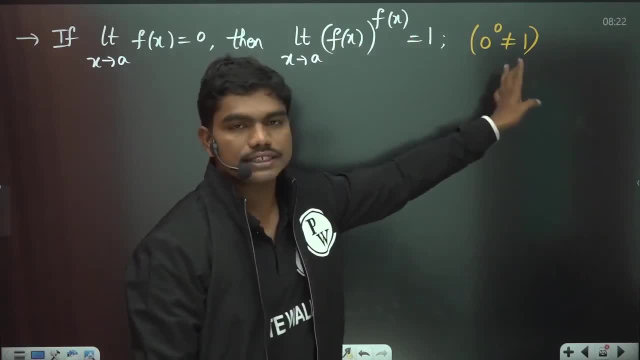 the mud one L Hospital and after final, the mud one L Hospital and after final analysis, you will get one okay, but this analysis, you will get one okay, but this analysis, you will get one okay, but this is not because of the reason that 0, is not because of the reason that 0. 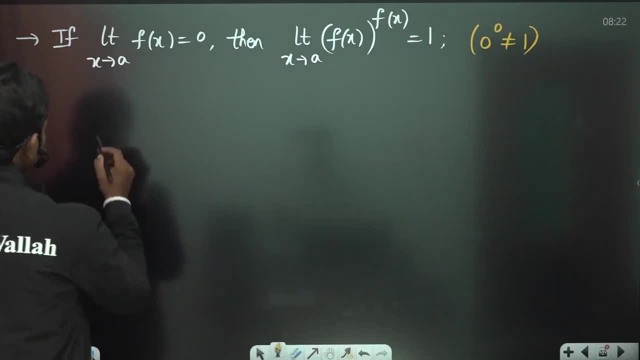 is not because of the reason that 0 power 0 is actually 1- clear now. if you power 0 is actually 1- clear now. if you power 0 is actually 1- clear now. if you write this, for example: I'm not again. write this, for example, I'm not again. 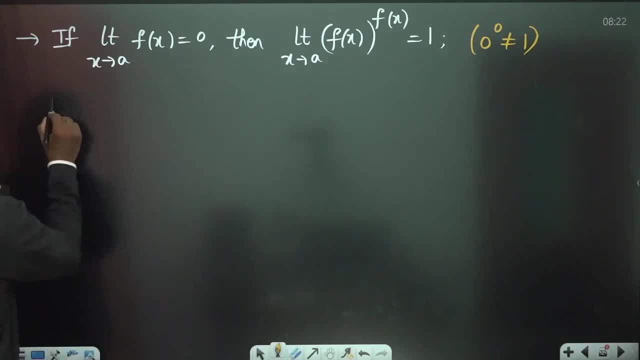 write this: for example, I'm not again showing the proof because it's a short showing the proof, because it's a short showing the proof, because it's a short, single go video. so now, if you see single go video, so now, if you see single go video, so now if you see examples in many times you know you'll. 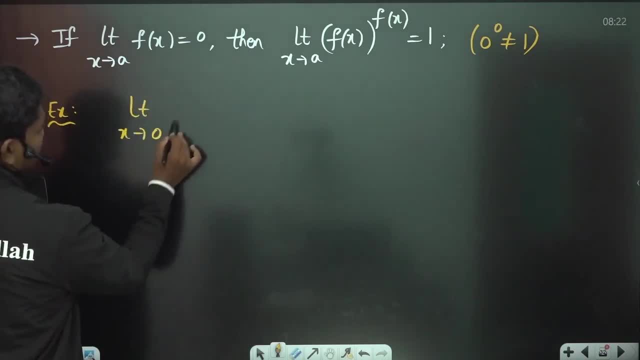 examples in many times you know you'll. examples in many times you know you'll get these questions. limit extends to 0: X. get these questions. limit extends to 0: X. get these questions. limit extends to 0 X. power X: okay, so limit extends to 0 sine. 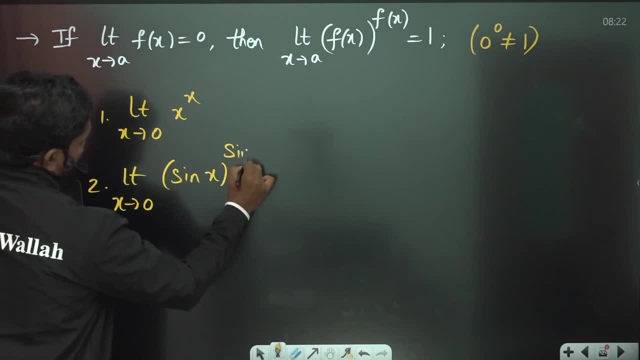 power X. okay, so limit extends to 0 sine power X. okay, so limit extends to 0 sine X. power sine X limit extends to 0 and X. power sine X. limit extends to 0 and X. power sine X. limit extends to 0 and X. power tan X. 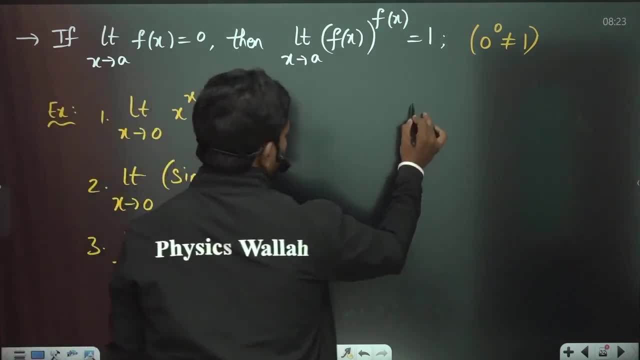 X power tan X X power tan X. tan X power tan X. okay, similarly, you will get tan X power tan X. okay, similarly, you will get tan X power tan X. okay, similarly, you will get limits like this limit extends to pi. limits like this limit extends to pi. 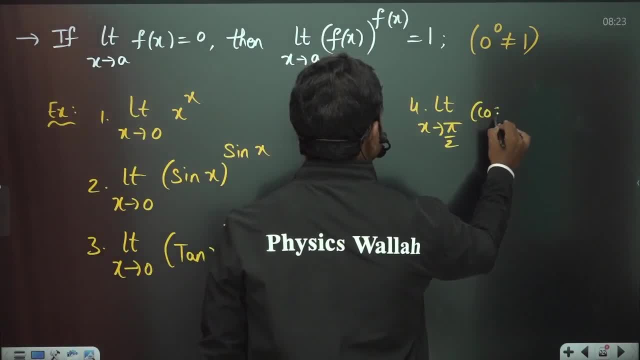 limits like this. limit extends to pi by 2 cos X power cos X. okay, so cos X. by 2 cos X, power cos X. okay, so cos X. by 2 cos X power cos X. okay, so cos X, power cos X. and you can say sometimes: 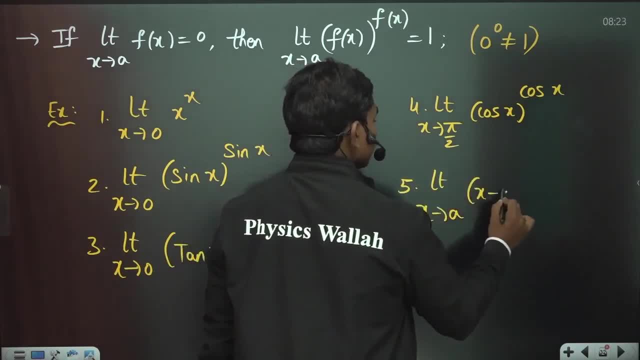 power cos X. and you can say sometimes power cos X. and you can say sometimes they'll give you something like limit. they'll give you something like limit. they'll give you something like limit. extends to a X minus a power X minus a. so extends to a X minus a power X minus a. so 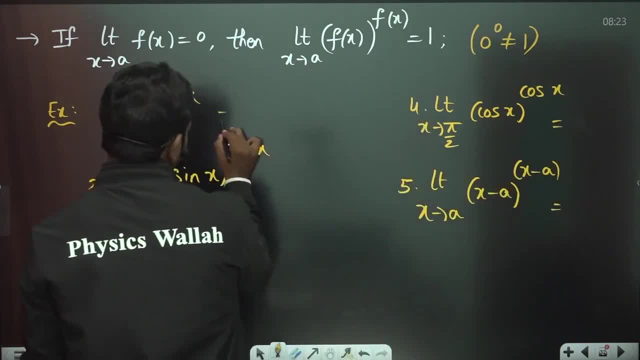 extends to a X minus a power, X minus a. so basically, you will get all these forms. basically, you will get all these forms. basically, you will get all these forms in this: 0 power, 0 forms. okay, so in all, in this: 0 power, 0 forms. okay, so in all. 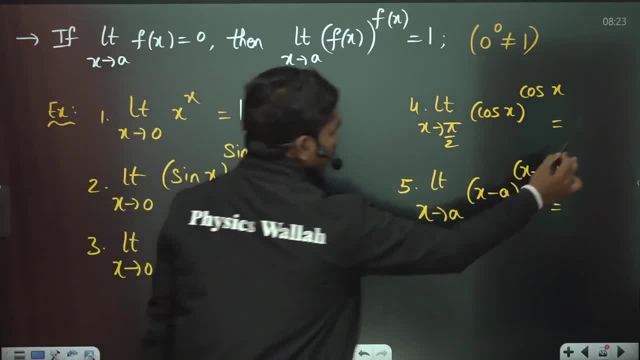 in this 0 power, 0 forms, okay. so in all these cases, this value is basically 1. these cases, this value is basically 1. these cases, this value is basically 1. okay. so 1 and 1 actually okay because. okay. so 1 and 1 actually okay, because. 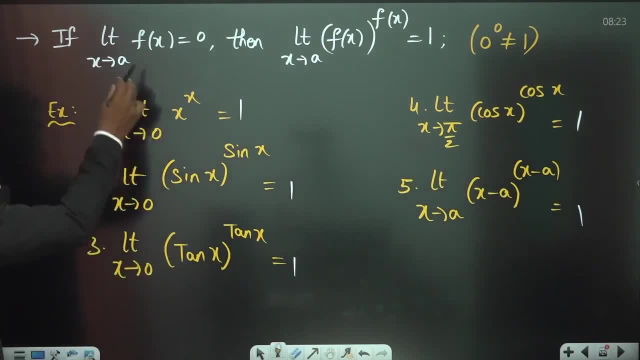 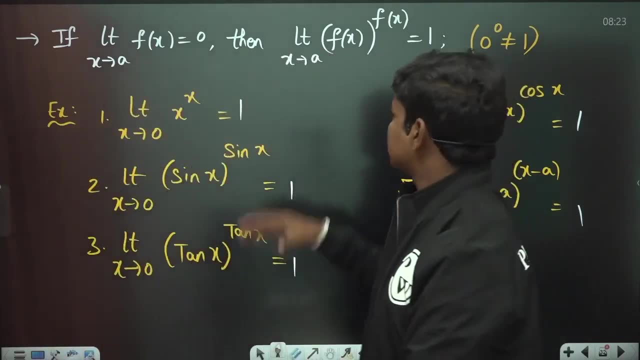 okay, so 1 and 1 actually okay, because this here individually extends to 0 this. this here individually extends to 0 this. this here individually extends to 0. this you know to else procedure. if you apply, you know to else procedure. if you apply, you know to else procedure, if you apply to well procedure, first you take the. 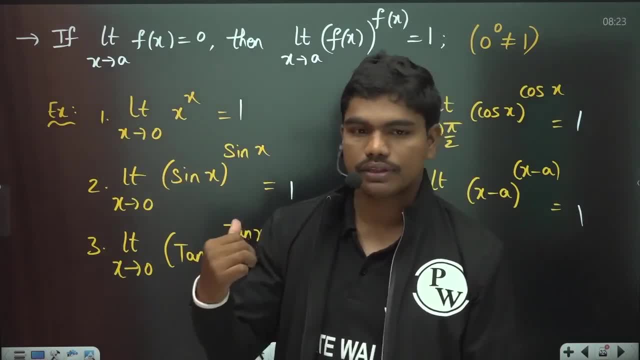 to well procedure. first you take the to well procedure. first you take the logarithm, then you apply the L hospital logarithm, then you apply the L hospital logarithm, then you apply the L hospital. then you will end up with getting one, then you will end up with getting one. 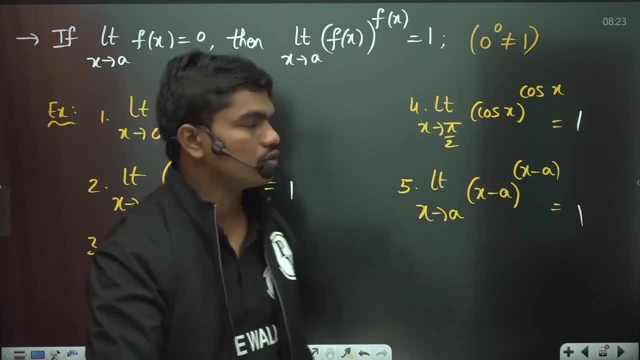 then you will end up with getting one okay, but all these limits since this is okay, but all these limits since this is okay, but all these limits since this is a short single go before the gate, a short single go before the gate, a short single go before the gate examination. I'm giving direct things, not 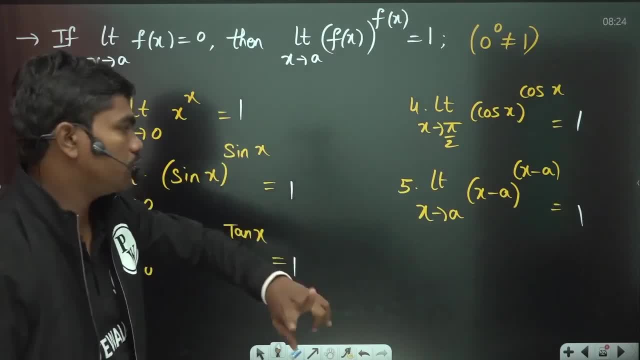 examination. I'm giving direct things, not examination. I'm giving direct things, not division of this. but again, division is division of this. but again, division is division of this. but again, division is very simple to all unit apply to else. very simple to all unit apply to else. 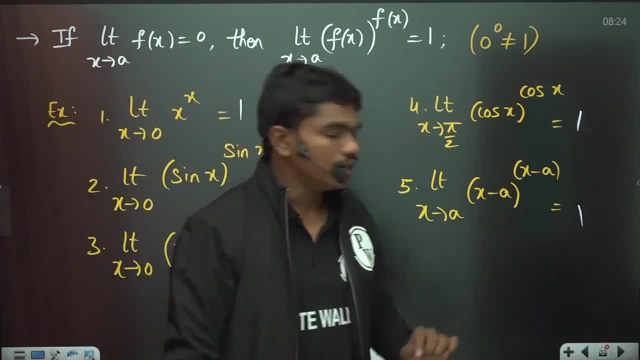 very simple: to all unit apply to else. okay. so in all these cases, the answer: okay. so, in all these cases, the answer: okay. so in all these cases, the answer remains one. okay, now, I'll give you one. remains one. okay, now I'll give you one, remains one. okay, now, I'll give you one. way has a important point or one of the? 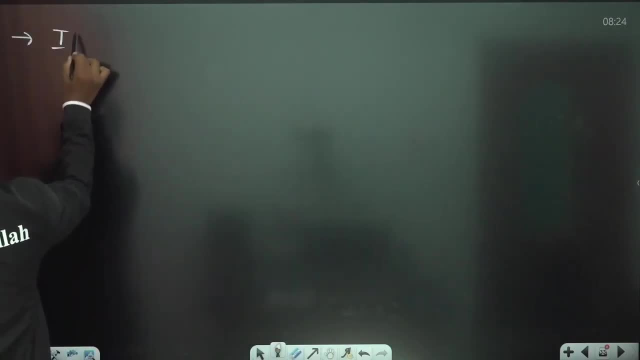 way has a important point, or one of the way has a important point, or one of the very good point. if you see if limit, very good point. if you see if limit, very good point. if you see if limit extends to a f of X, extends to a f of X. 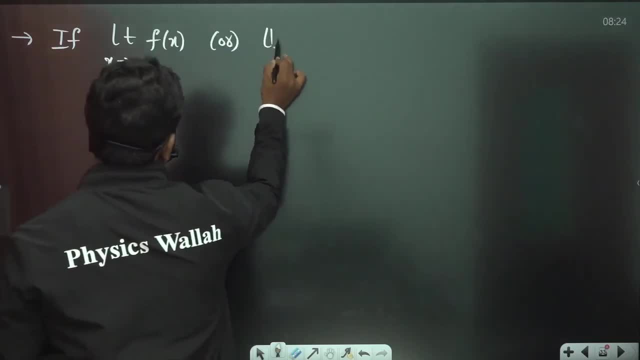 extends to a f of X or limit extends to B or extends to a or limit extends to B or extends to a or limit extends to B or extends to a. G of X does not exist means: let us. G of X. does not exist means, let us. 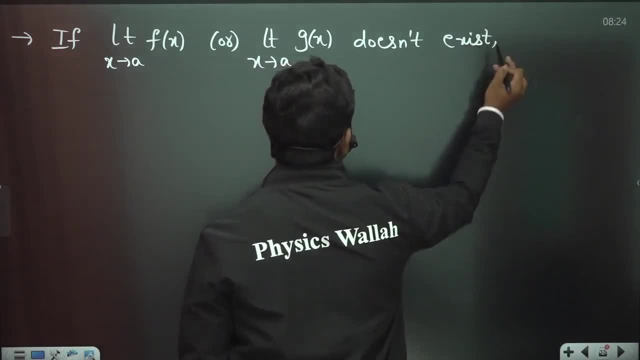 G of X does not exist means: let us suppose if one of these two limits, or suppose if one of these two limits, or suppose if one of these two limits or maybe both sometimes if they do not, maybe both sometimes if they do not, maybe both sometimes if they do not exist still. limit extends to a f of X. 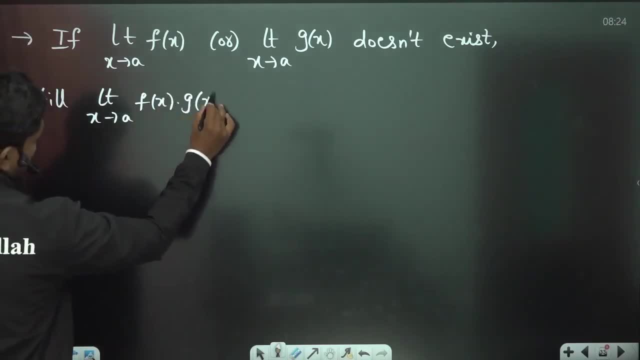 exist still. limit extends to a f of X exist still. limit extends to a f of X into G of X may exist. f of X into G of X into G of X may exist. f of X into G of X into G of X may exist. f of X into G of X may exist. okay, so how you can say this. 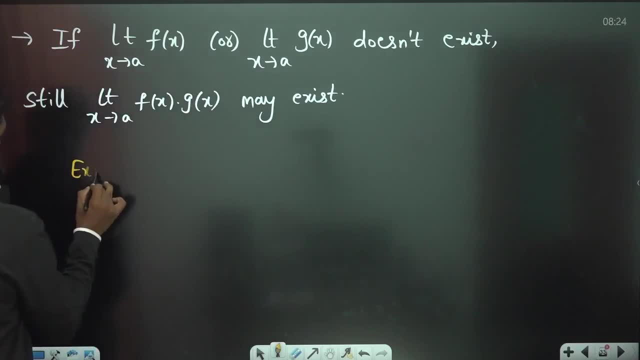 may exist okay. so how you can say this: may exist okay. so how you can say this? because I will give you the help of an, because I will give you the help of an, because I will give you the help of an example. example, you know, limit extends. 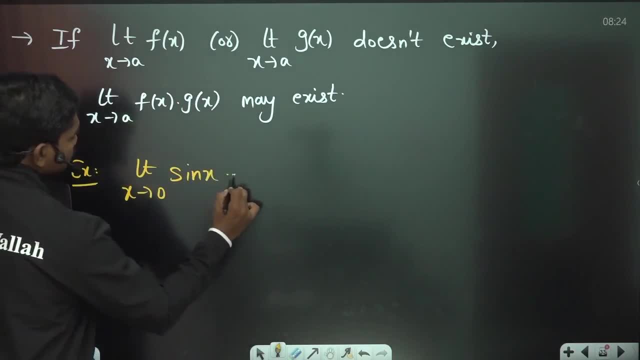 example: you know limit extends to 0 sine X: this is 0. you know this limit to 0 sine X: this is 0. you know this limit to 0 sine X: this is 0. you know this limit extends to 0- 1 by X. this value does not. 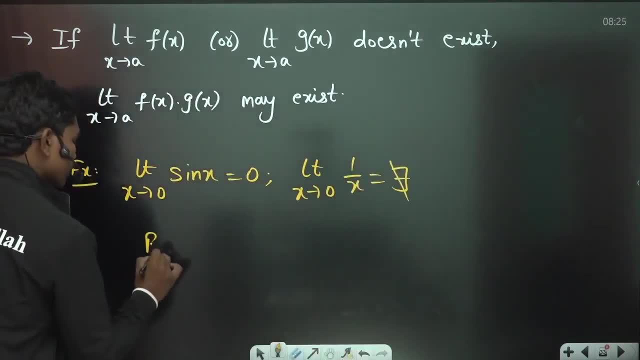 extends to 0, 1 by X. this value does not extends to 0, 1 by X. this value does not exist, that this is does not exist. but if exist, that this is does not exist. but if exist, that this is does not exist. but if you see, limit extends to 0 sine X into 1. 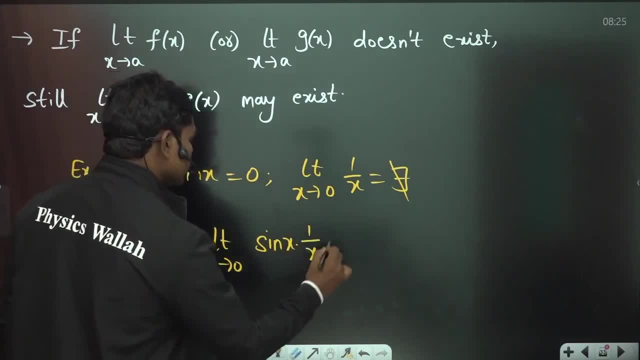 you see limit extends to 0 sine X into 1. you see limit extends to 0 sine X into 1 by X sine X into 1 by X. so this: if you by X sine X into 1 by X, so this: if you by X sine X into 1 by X, so this: if you see, limit extends to 0 sine X by X. so 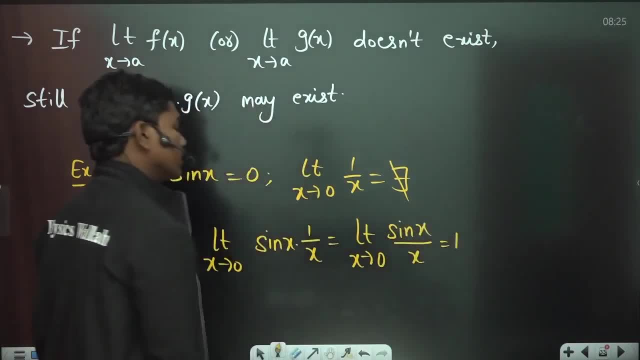 see limit extends to 0 sine X by X. so see limit extends to 0 sine X by X. so sine X by X. so this value is going to be sine X by X. so this value is going to be sine X by X. so this value is going to be 1 actually. so if you see individually one, 1 actually. so if you see individually one: 1 actually. so if you see individually, one of the limits is not existing, but when of the limits is not existing, but when of the limits is not existing, but when you make the product definitely this, you make the product definitely this. 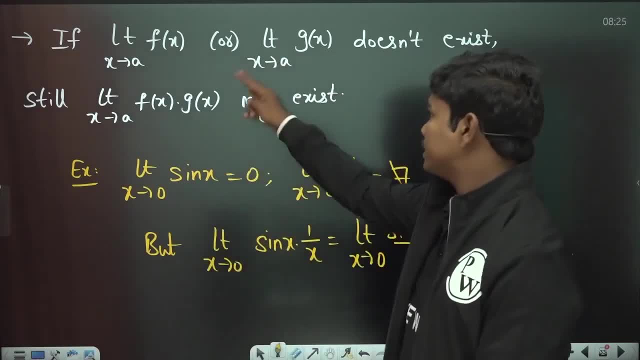 you make the product, definitely this value is finite. so somehow you can see value is finite. so somehow you can see value is finite. so somehow you can see, even sometimes, even if these two limits, even sometimes, even if these two limits, even sometimes, even if these two limits one of these two, or maybe sometimes it. 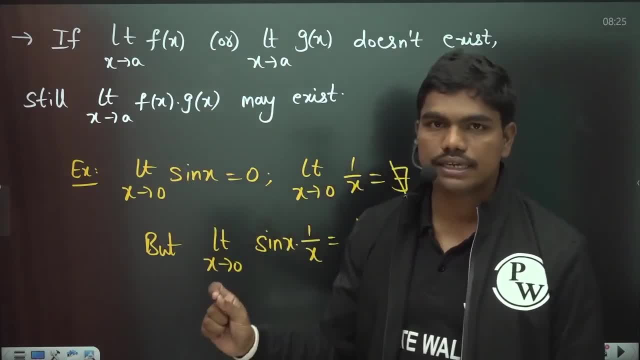 one of these two, or maybe sometimes it one of these two, or maybe sometimes it can happen that both also mean need not. can happen that both also mean need not. can happen that both also mean need not exist, but their multiplication can exist. exist, but their multiplication can exist. 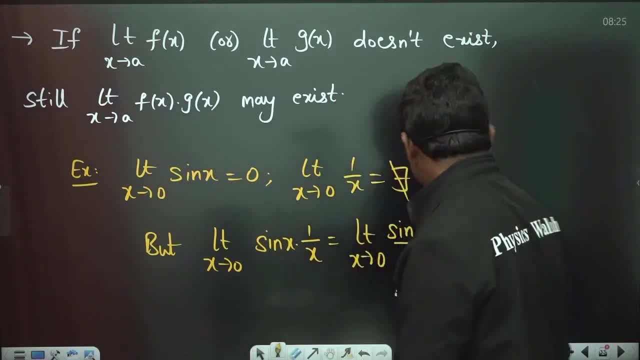 exist, but their multiplication can exist actually okay. so this is one important actually okay. so this is one important actually okay. so this is one important thing actually here, okay now coming to thing, actually here. okay now. coming to thing, actually here. okay now. coming to differentiation, I would like to give 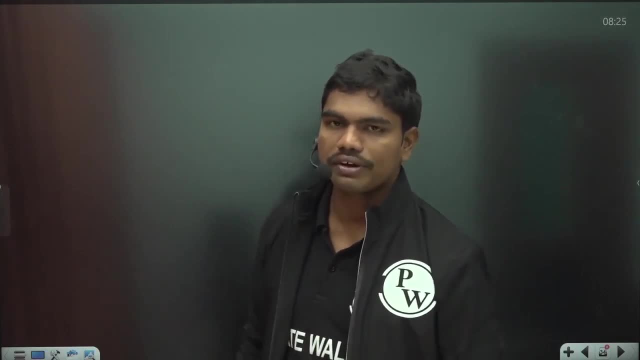 differentiation, I would like to give differentiation. I would like to give only one point, because we have talked only one point, because we have talked only one point, because we have talked already a lot about differentiation, so already a lot about differentiation, so already a lot about differentiation. so now, if you see mod X function this: 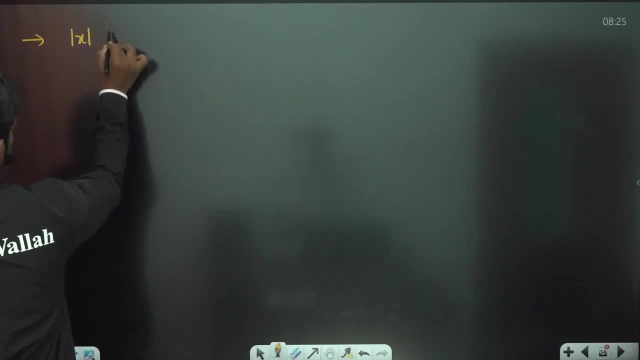 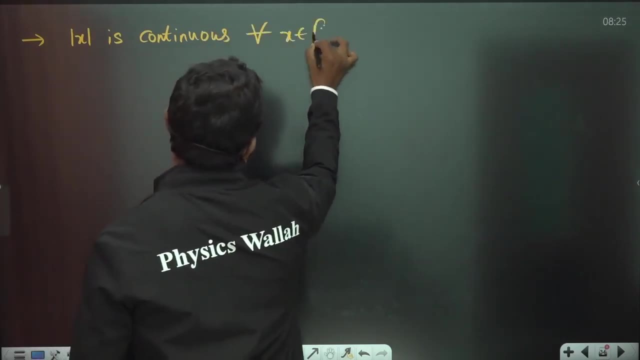 now if you see mod X function this, now if you see mod X function, this function is generally important. so mod X function is generally important. so mod X function is generally important. so mod X is continuous, is continuous for all. X is continuous for all X is continuous for all X belongs to R, but it is not a differentiable, it is. 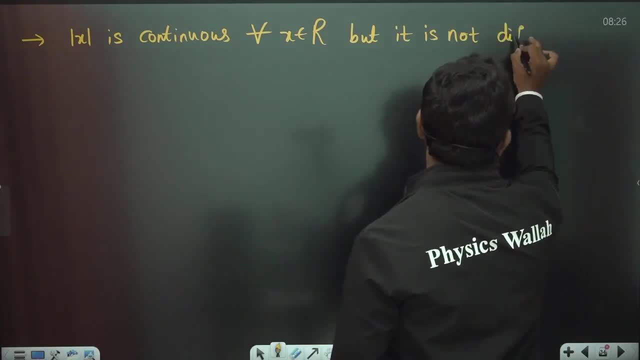 belongs to R, but it is not a differentiable. it is: belongs to R, but it is not a differentiable. it is not differentiable. it is not not differentiable. it is not not differentiable, it is not differentiable. at X is equal to 0, at X is: 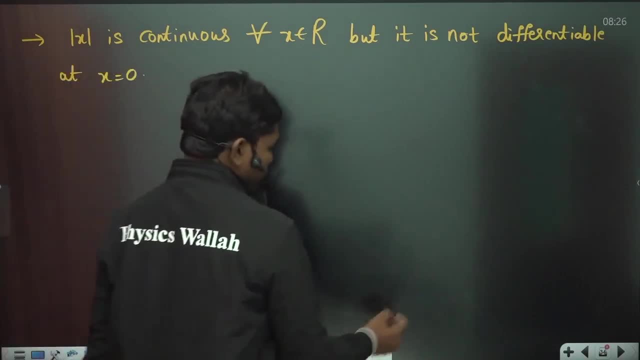 differentiable: at X is equal to 0. at X is differentiable: at X is equal to 0. at X is equal to 0. okay means basically, if you equal to 0. okay means basically, if you equal to 0. okay means basically, if you take this function, mod X. 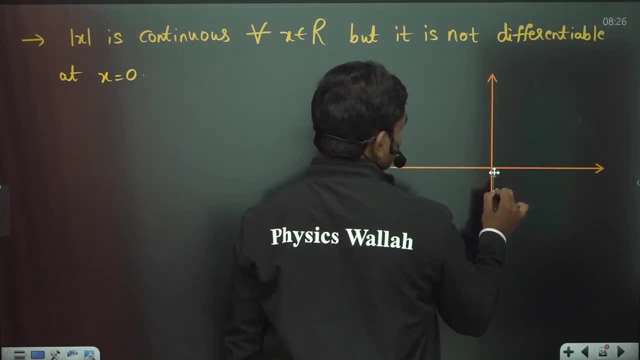 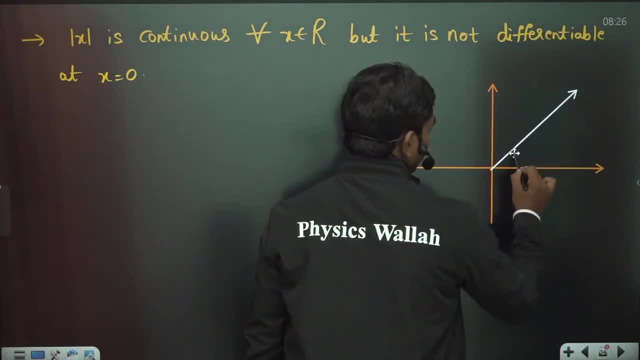 know, we have seen, know, we have seen, know, we have seen. so if you see this is the function, so Y. so if you see this is the function, so Y. so if you see this is the function, so Y is equal to X, Y is equal to minus X. okay, 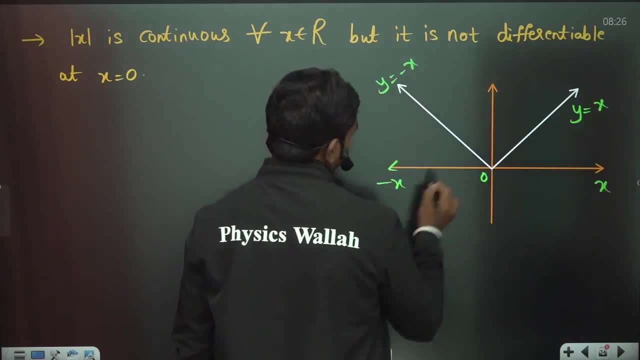 is equal to X. Y is equal to minus X. okay, is equal to X. Y is equal to minus X. okay, 0 X minus X, Y and minus Y. now, if you see 0 X minus X, Y and minus Y. now, if you see 0 X minus X, Y and minus Y. now, if you see carefully, here I am telling you this: 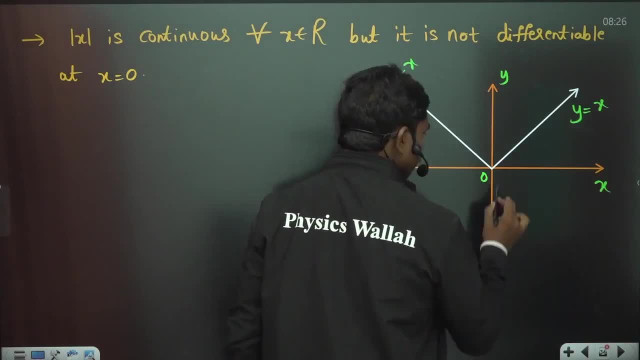 carefully here I am telling you this carefully, here I am telling you this function is not differentiable at. this, function is not differentiable at this, function is not differentiable at this. location X is equal to 0, okay, and location X is equal to 0, okay, and 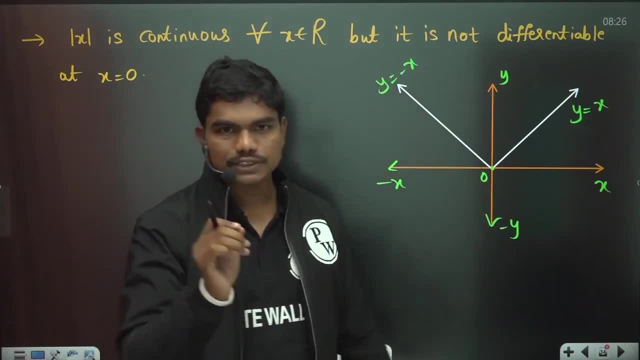 location X is equal to 0. okay, and generally, I will tell you that this, generally, I will tell you that this, generally, I will tell you that this will tell you one thing. any function at will tell you one thing. any function at will tell you one thing: any function at points where it is having sharp edges, points where it is having sharp edges. points where it is having sharp edges. for example, if you see this is a sharp, for example, if you see this is a sharp. for example, if you see this is a sharp edge, right, it's not going smoothly like edge, right, it's not going smoothly like 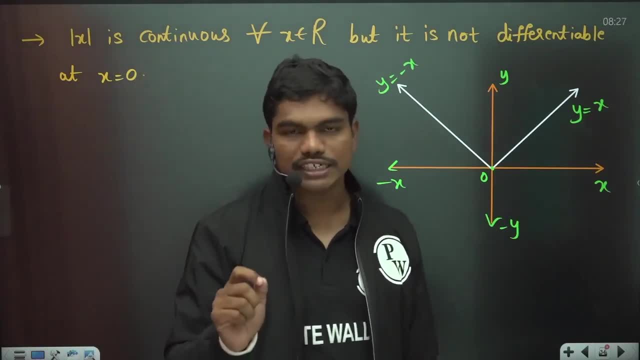 edge. right, it's not going smoothly. like sine X curve, it has a sharp edge, okay. so sine X curve, it has a sharp edge. okay. so sine X curve, it has a sharp edge, okay. so at all the points where there are sharp, at all the points where there are sharp. 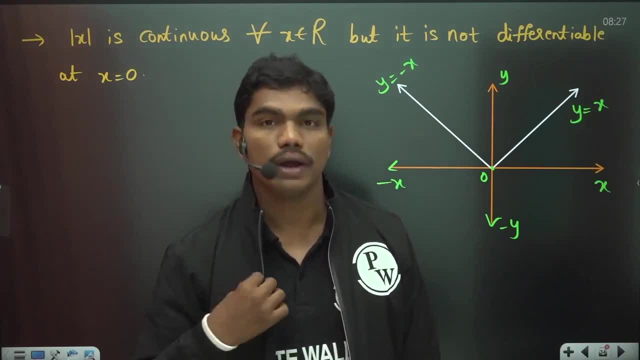 at all the points where there are sharp edges geometrically at those points, edges geometrically at those points, edges geometrically at those points, functions are not differentiable. why I functions are not differentiable. why I functions are not differentiable. why I tell you: look, see here. for example, if I 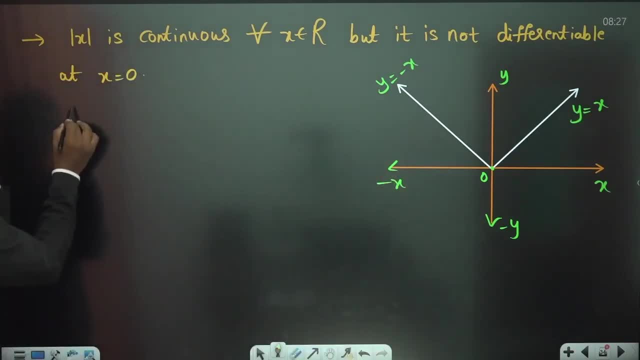 tell you: look see here, for example. if I tell you: look see here, for example, if I want to test the defensibility of this, want to test the defensibility of this, want to test the defensibility of this function. at X is equal to 0, I need to. 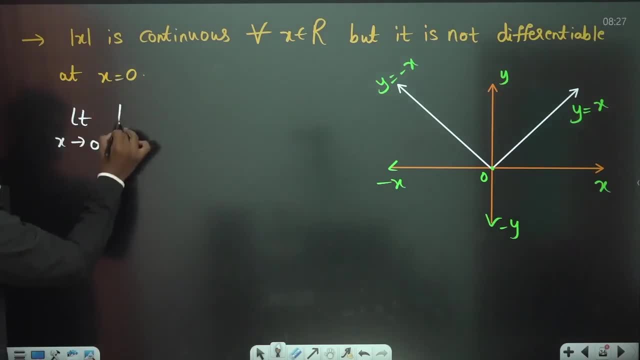 function at X is equal to 0. I need to function at X is equal to 0. I need to check whether this limit limit extends. check whether this limit limit extends. check whether this limit limit extends to 0 f of X minus f of a divided by X. 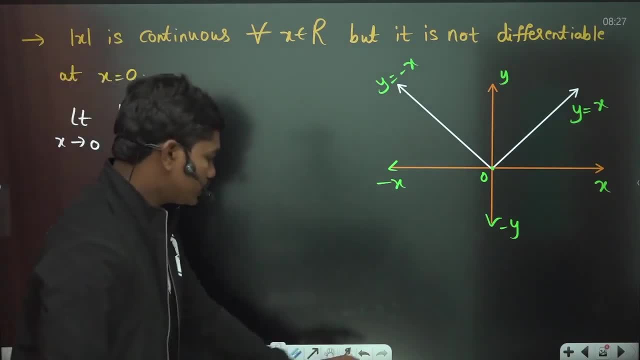 to 0 f of X minus f of a divided by X to 0 f of X minus f of a divided by X minus a. this limit will exist or not. minus a: this limit will exist or not. minus a: this limit will exist or not. correct, because, if you see, this is equal. 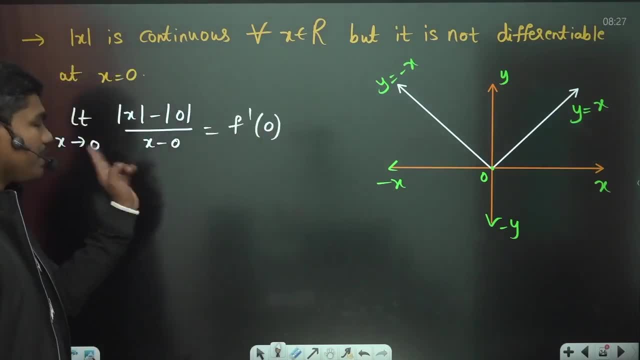 correct because if you see this is equal, correct because if you see this is equal to f dash of 0, actually. so if this limit to f dash of 0, actually so, if this limit to f dash of 0, actually so, if this limit exists, then definitely I will say the. 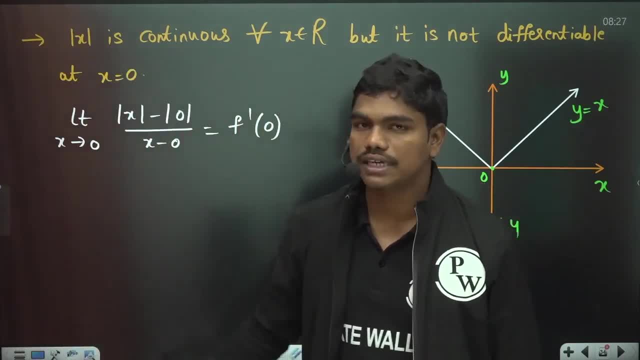 exists, then definitely I will say the exists, then definitely I will say: the mod X is differentiable at X is equal to. mod X is differentiable at X is equal to. mod X is differentiable at X is equal to 0. but this limit does not exist. 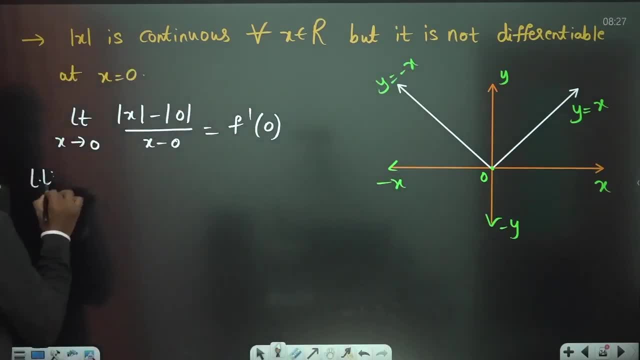 0 but this limit does not exist. 0, but this limit does not exist actually. why you see here? if you calculate the actually, why you see here, if you calculate the actually. why you see here, if you calculate the left limit, if you calculate left limit, if you calculate the left limit limit, X tends to 0 minus. this is. 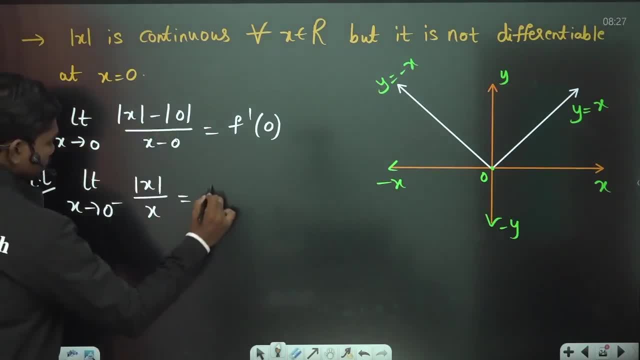 left limit. if you calculate the left limit limit, X tends to 0 minus. this is left limit. if you calculate the left limit, X tends to 0 minus. this is mod X by X. if you simplify mod X, mod X by X. if you simplify mod X by X, so this is equal to limit. X tends to 0. I'm. mod X by X, so this is equal to limit X tends to 0. I'm mod X by X, so this is equal to limit X tends to 0. I'm moving this minus here because I'm moving this minus here, because I'm moving this minus here? because I'm going to modify this function. okay, look. 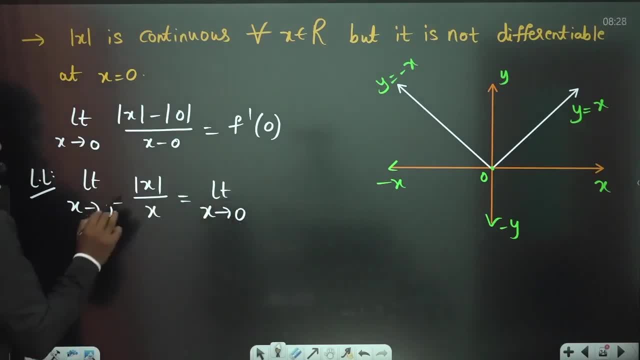 going to modify this function. okay, look, going to modify this function. okay, look, here I have kept a minus. but here I am. here I have kept a minus, but here I am. here I have kept a minus, but here I am not keeping minus. because, according to, not keeping minus because according to, 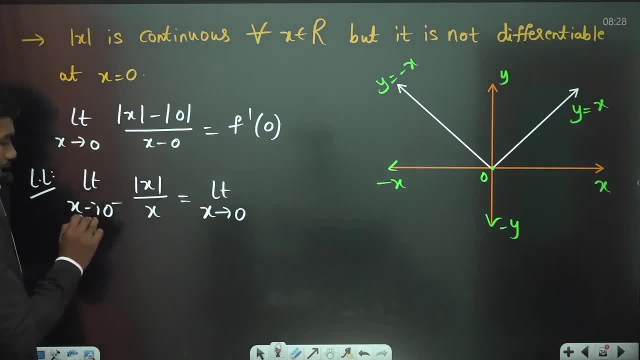 not keeping minus because, according to this minus, I am going to change the this minus, I am going to change the this minus. I am going to change the function here. see here when X is function here. see here when X is function here. see here when X is tending to 0 minus, X is less than 0. 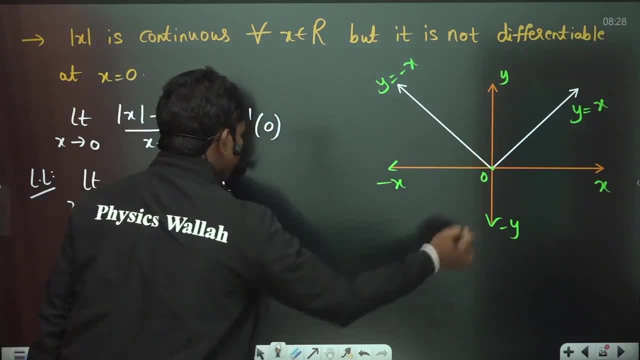 tending to 0 minus X is less than 0. tending to 0 minus X is less than 0: correct. whenever X is less than 0 means correct. whenever X is less than 0 means correct. whenever X is less than 0 means to the left hand side of this y-axis. 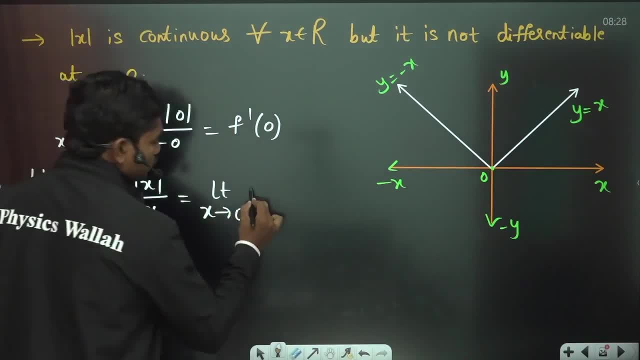 to the left hand side of this y-axis. to the left hand side of this y-axis. whenever X is less than 0, mod X is. whenever X is less than 0, mod X is. whenever X is less than 0, mod X is equal to minus X. okay, so I have. 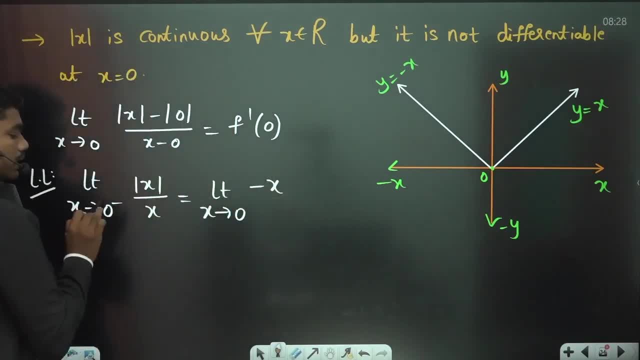 equal to minus X. okay, so I have equal to minus X. okay, so I have converted this mod X function as minus X. converted this mod X function as minus X. converted this mod X function as minus X. because of this minus 0- minus here: okay. because of this minus 0- minus here: okay. 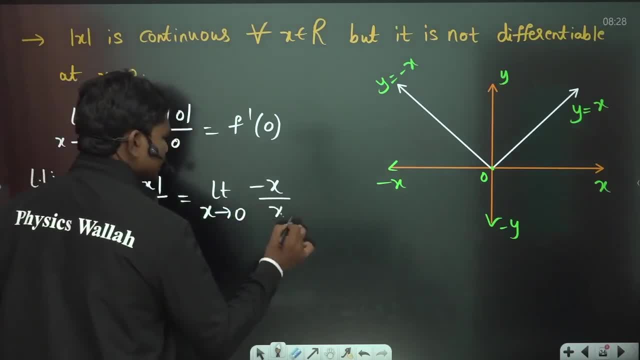 because of this: minus 0 minus here. okay. so no more 0 minus here, only 0 divided. so no more 0 minus here, only 0 divided. so no more 0 minus here, only 0 divided by X, X is X anyhow. so if you see, this is: 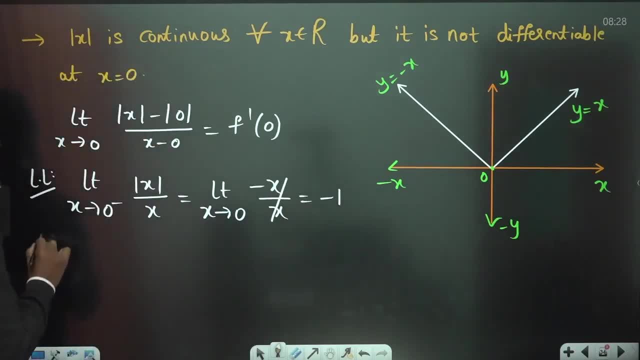 by X, X is X anyhow. so if you see this is by X, X is X anyhow. so if you see this is minus 1, so left side the limit is minus minus 1. so left side the limit is minus minus 1. so left side the limit is minus 1. and if you talk about the right limit, 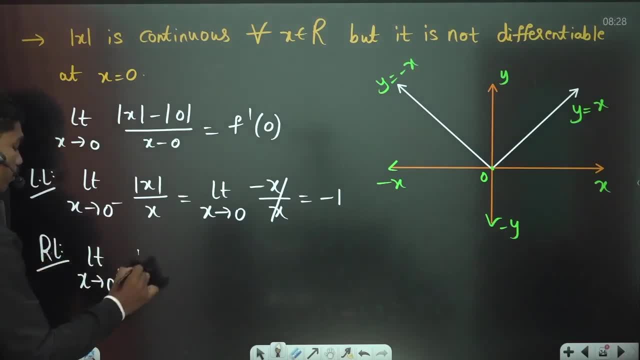 1. and if you talk about the right limit 1. and if you talk about the right limit, limit extends to 0 plus mod X by X. so limit extends to 0 plus mod X by X. so limit extends to 0 plus mod X by X. so this, if you say limit extends to 0, now 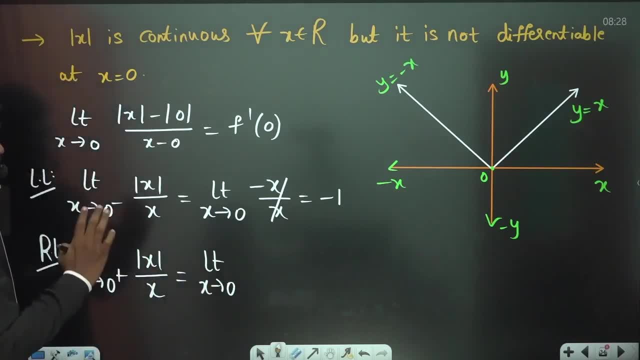 this: if you say limit extends to 0, now this: if you say limit extends to 0, now when this is tending to 0, plus means X. when this is tending to 0, plus means X. when this is tending to 0, plus means X is more than 0. when X is more than 0. 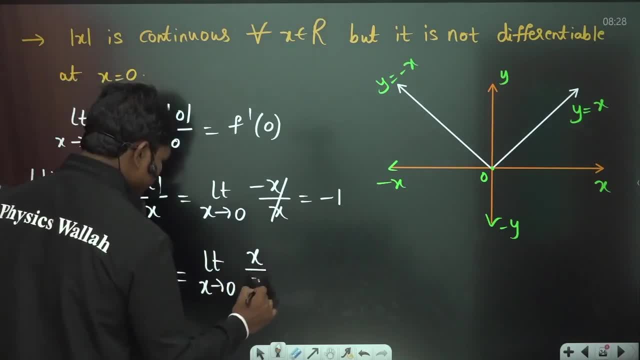 is more than 0, when X is more than 0, is more than 0. when X is more than 0, this mod X value is actually equal to X. this mod X value is actually equal to X. this mod X value is actually equal to X value, and this is how you will get 1 on. 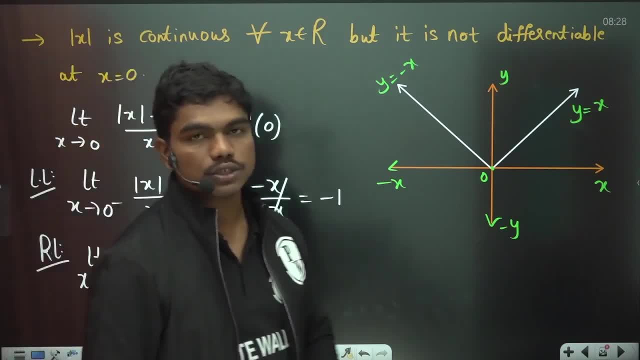 value. and this is how you will get 1 on value. and this is how you will get 1 on this side: okay, so left limit is minus 1. this side: okay, so left limit is minus 1. this side: okay, so left limit is minus 1. the right limit is 1. so basically this. the right limit is 1. so basically this: the right limit is 1. so basically, this limit does not exist, okay. so what's? the limit does not exist, okay. so what's? the limit does not exist, okay. so what's the meaning that physically this limit does? 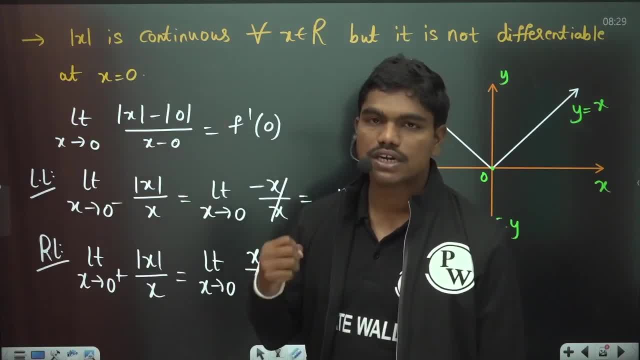 meaning that, physically, this limit does, meaning that, physically, this limit does not exist. this is not existing means: not exist. this is not existing means not exist. this is not existing means. this, this function doesn't have a. this, this function doesn't have a. this, this function doesn't have a differentiation at. X is equal to 0 and. differentiation at X is equal to 0 and differentiation at X is equal to 0. and also, I would like to show you one thing also, I would like to show you one thing also. I would like to show you one thing geometrically here you try to 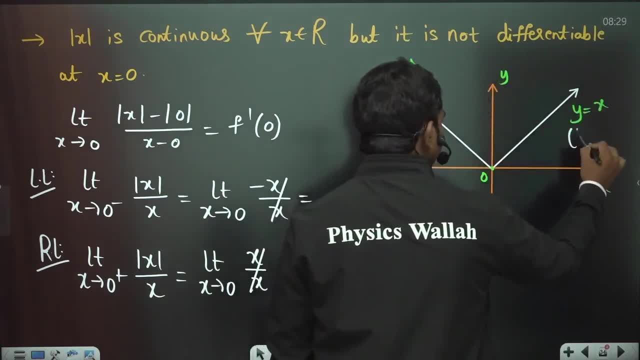 geometrically here you try to. geometrically, here you try to understand this. normally, this is a understand this. normally, this is a understand this. normally this is a straight line passing through horizon, straight line passing through horizon, straight line passing through horizon. so, if you see the equation, this is, Y is. 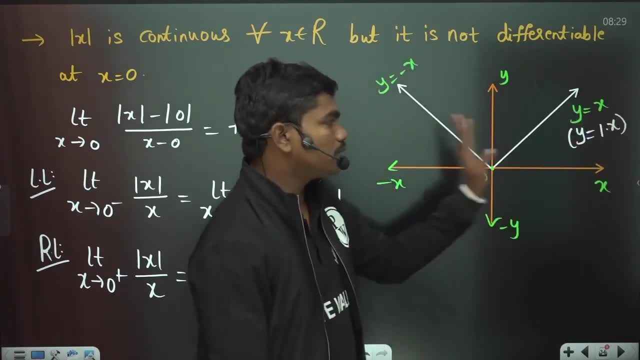 so if you see the equation this is: Y is: so if you see the equation this is: Y is equal to MX form. okay, so Y is equal to equal to MX form. okay, so Y is equal to equal to MX form. okay, so Y is equal to 1 into X, so slope is 1. so basically this: 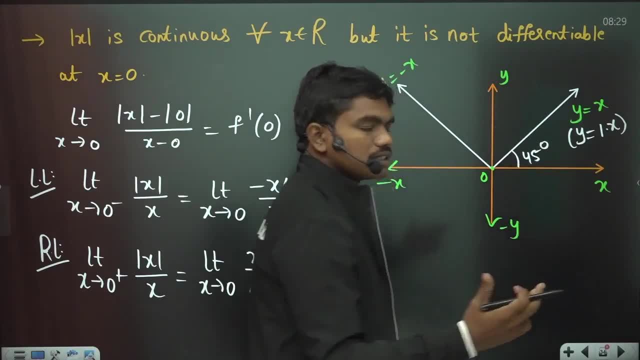 1 into X, so slope is 1. so basically this: 1 into X, so slope is 1. so basically this: angle is 45 degrees. how do you know it? angle is 45 degrees? how do you know it? angle is 45 degrees? how do you know it is 45 degrees? because slope is nothing. 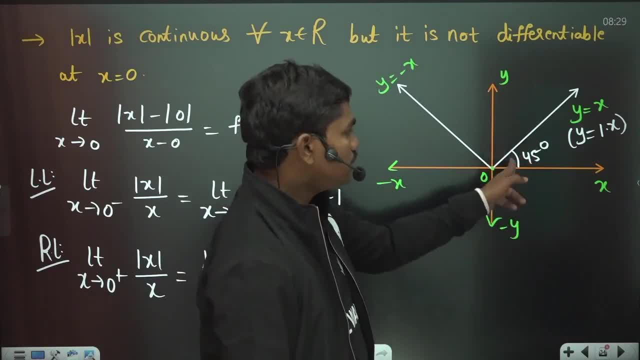 is 45 degrees because slope is nothing. is 45 degrees because slope is nothing but tan theta, so 1 is equal to tan 45, but tan theta, so 1 is equal to tan 45, but tan theta, so 1 is equal to tan 45. that's the reason this angle is 45 and 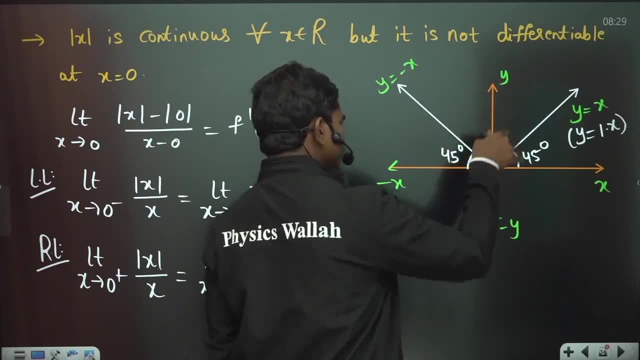 that's the reason this angle is 45. and that's the reason this angle is 45 and, of course, due to symmetry. this angle is, of course, due to symmetry. this angle is, of course, due to symmetry. this angle is also 45 degrees, and these two at 90. 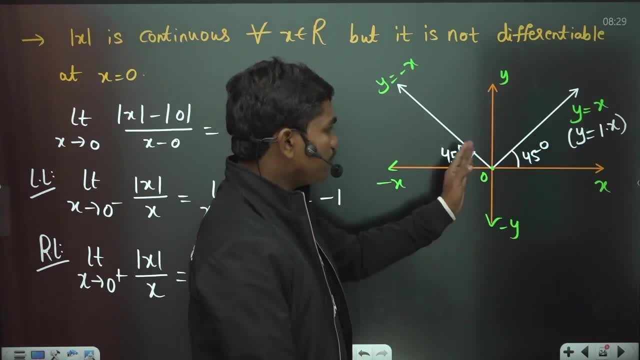 also 45 degrees, and these two at 90, also 45 degrees and these two at 90 degrees to each other. okay now, if you see degrees to each other. okay now if you see degrees to each other. okay now if you see Y is equal to MX means, and this is a. 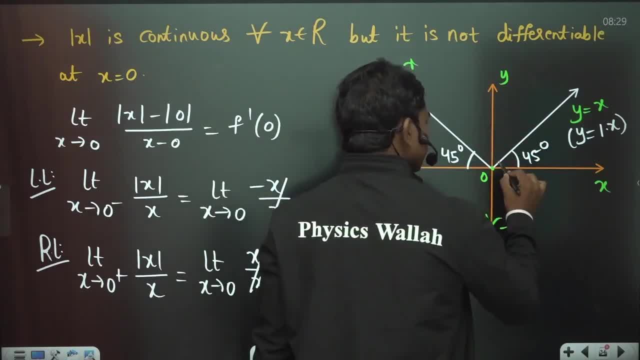 Y is equal to MX means and this is a Y is equal to MX means and this is a straight line slope at every point means straight line slope at every point, means straight line slope at every point means basically this is straight line, so slope. basically this is straight line, so slope. 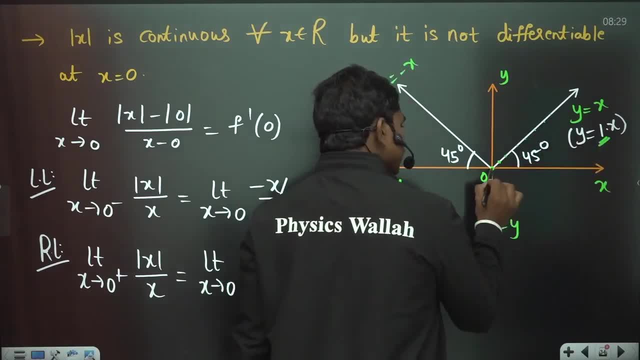 basically this is straight line. so slope at every point is basically one. okay at every point is basically one. okay at every point is basically one. okay means in the right neighborhood also means in the right neighborhood. also means in the right neighborhood also. slope is 1, which means right, different. 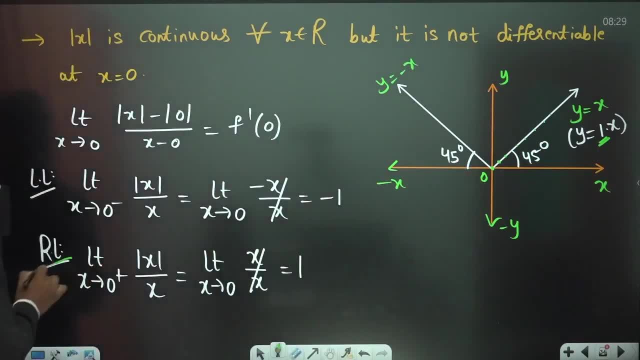 slope is 1, which means right. different slope is 1, which means right. different derivative: a right side derivative is derivative. a right side derivative is derivative. a right side derivative is plus 1. you can see the right limit means plus 1. you can see the right limit means. 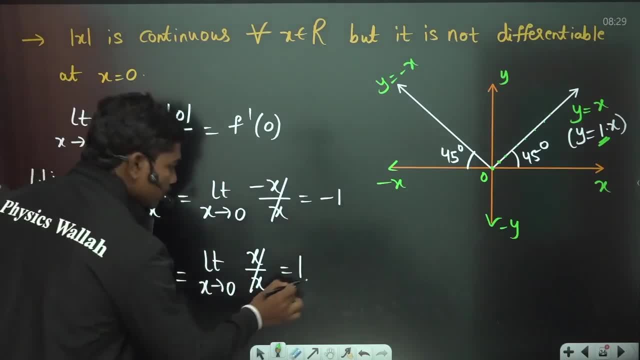 plus 1, you can see the right limit means, basically: if you calculate this, basically, if you calculate this, basically, if you calculate this derivative on the right side, your answer: derivative on the right side, your answer: derivative on the right side- your answer is 1 because geometrically this is equal. 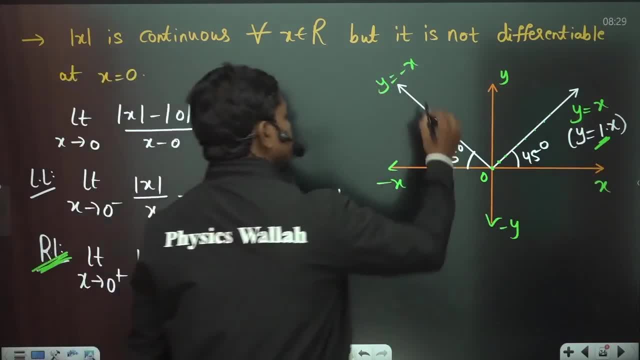 is 1 because geometrically, this is equal is 1 because geometrically, this is equal to Y is equal to MX form. okay, and also to Y is equal to MX form. okay, and also to Y is equal to MX form. okay, and also on the left side. this is the equation. 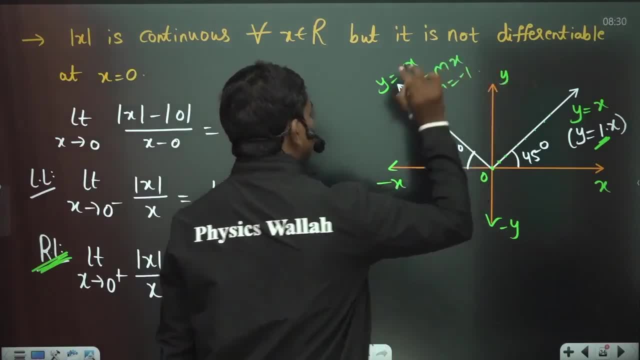 on the left side. this is the equation on the left side. this is the equation with the slope M is equal to minus 1. so with the slope M is equal to minus 1. so with the slope M is equal to minus 1. so that's why, if you calculate the left, 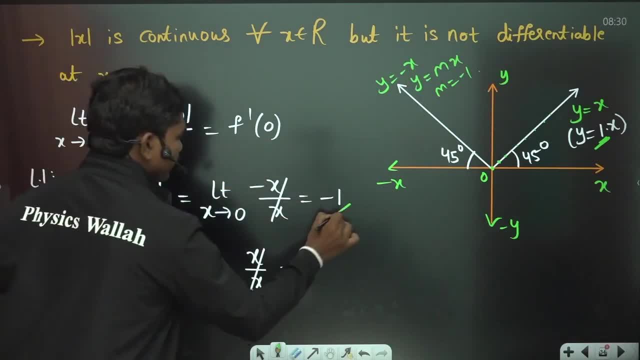 that's why, if you calculate the left, that's why, if you calculate the left hand derivative, you will get minus 1 as hand derivative. you will get minus 1 as hand derivative. you will get minus 1 as the answer which you got here, as minus 1. 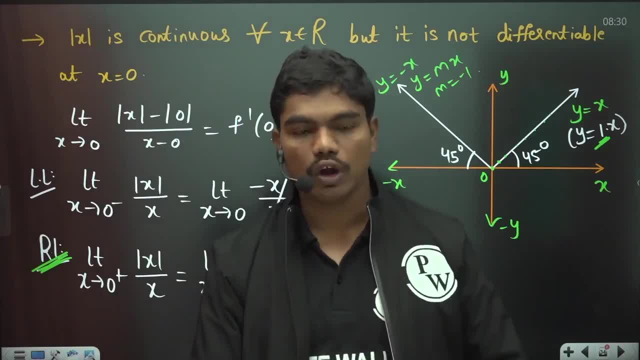 the answer which you got here as minus 1. the answer which you got here as minus 1. okay, so that's how this mod X function. okay, so that's how this mod X function. okay, so that's how this mod X function. is not differentiable at the points X is: 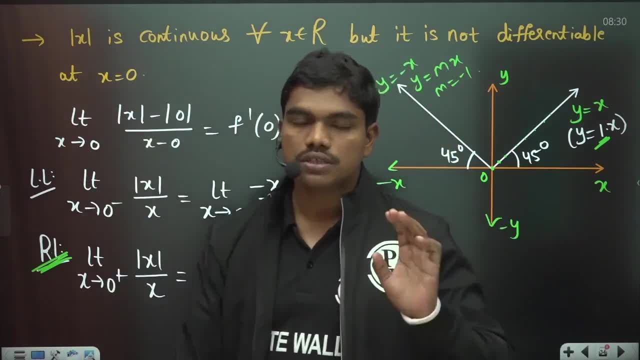 is not differentiable at the points X is is not differentiable at the points X is equal to 0, but of course you cannot see equal to 0, but of course you cannot see equal to 0, but of course you cannot see any breaking in the function. so that's. 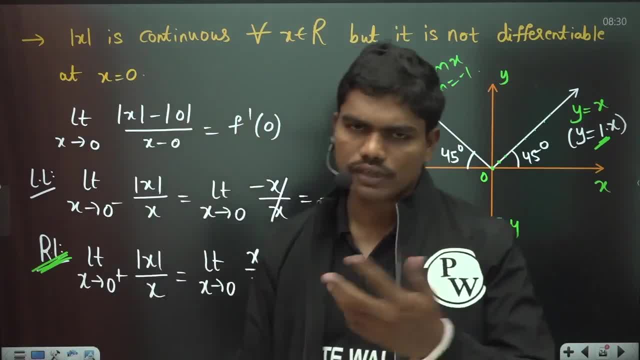 any breaking in the function. so that's any breaking in the function. so that's why mod X is continuous for all X, why mod X is continuous for all X, why mod X is continuous for all X belongs to? are you know, for all X belongs to? are you know, for all X? 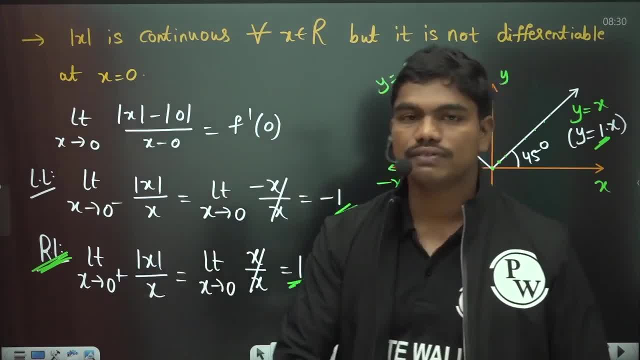 belongs to, are you know for all. X belongs to real numbers. means from minus belongs to real numbers. means from minus belongs to real numbers. means from minus infinity to plus infinity. this mod X infinity to plus infinity. this mod X infinity to plus infinity, this mod X function. do not have any breaking in it. 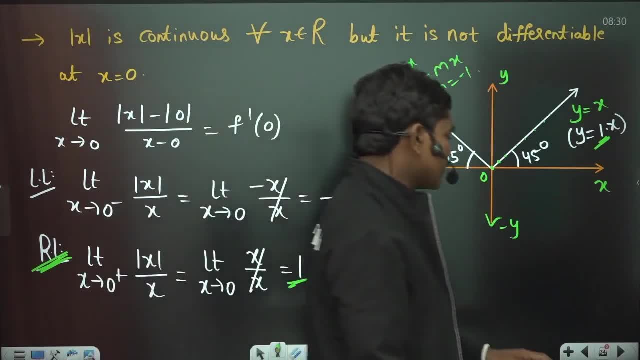 function do not have any breaking in it. function do not have any breaking in it, but obviously it is not differentiable. but obviously it is not differentiable, but obviously it is not differentiable. clear now, let us go for the next part. clear now, let us go for the next part. 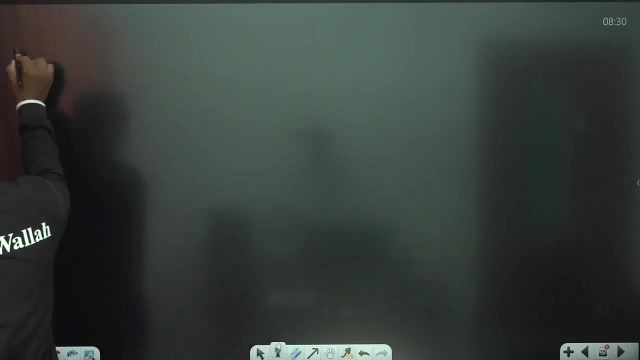 clear. now let us go for the next part. normally I'm giving you one point, which normally I'm giving you one point which normally I'm giving you one point which could help you out: mod f of X and of could help you out: mod f of X and of. 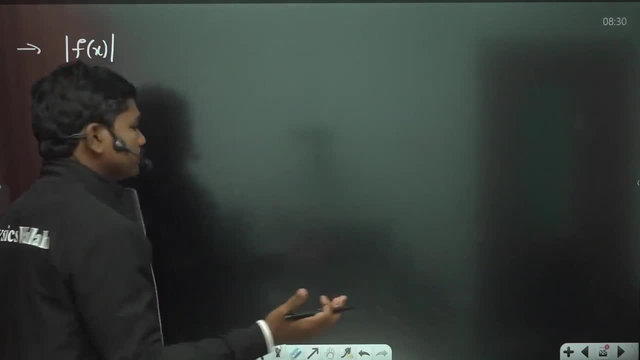 could help you out. mod f of X and of course f of X is polynomial functions. course f of X is polynomial functions. course f of X is polynomial functions. okay, so our trigonometric functions. okay, so our trigonometric functions. okay, so our trigonometric functions. anything it should not have denominator. 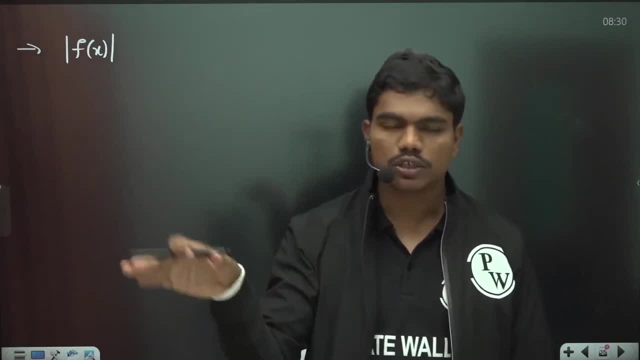 anything. it should not have denominator anything it should not have denominator. basically okay. the discontinuity is not basically okay. the discontinuity is not basically okay. the discontinuity is not because of the denominator, but because because of the denominator, but because because of the denominator but because of the function itself. so mod f of X is: 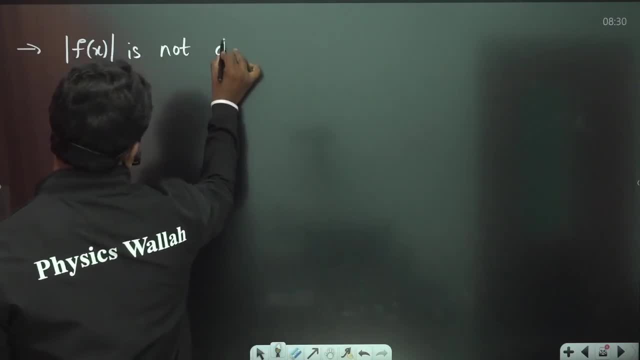 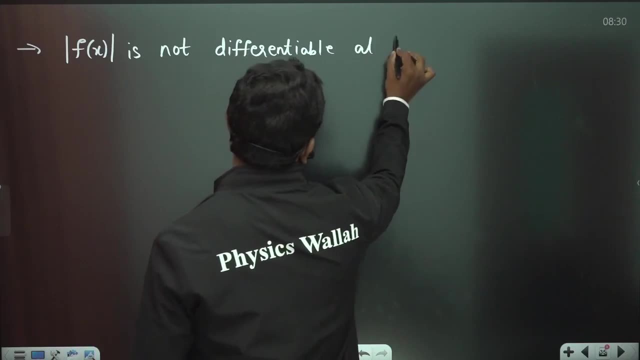 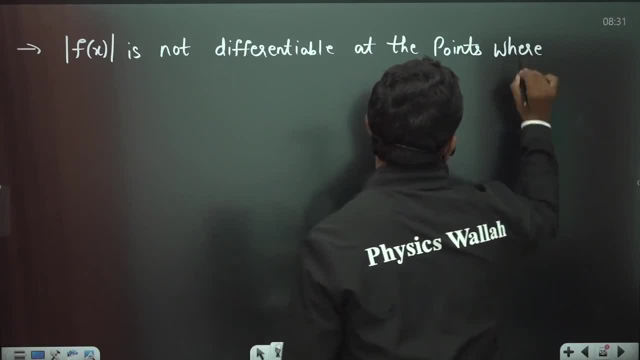 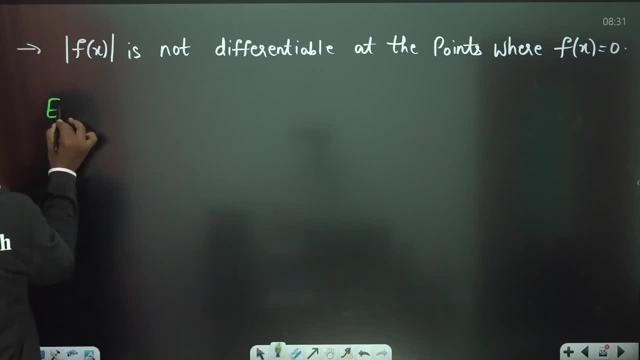 f of X is equal to 0. what's the meaning of this look example. I like to give talk this look example. I like to give talk this look example. I like to give talk about one example here: example: mod X. about one example here: example: mod X. 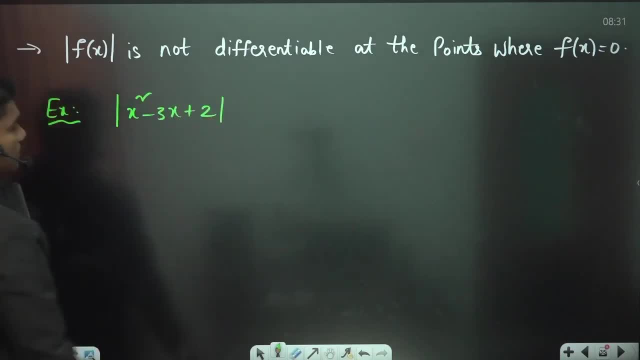 about one example here. example: mod: X- square minus 3x plus 2x. square minus 3x plus 2x. square minus 3x plus 2x. if you take this function, for example, if you take this function, for example. if you take this function, for example, okay, if you take this function, mod. 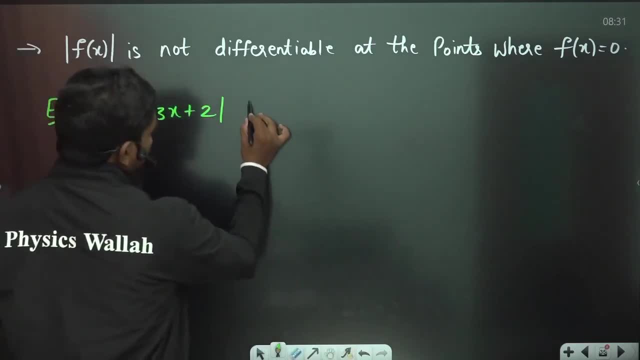 okay, if you take this function mod, okay, if you take this function mod, functions are continuous everywhere, but functions are continuous everywhere, but functions are continuous everywhere, but this function is not differentiable. is this function is not differentiable? is this function is not differentiable? is not a differentiable, is not a. 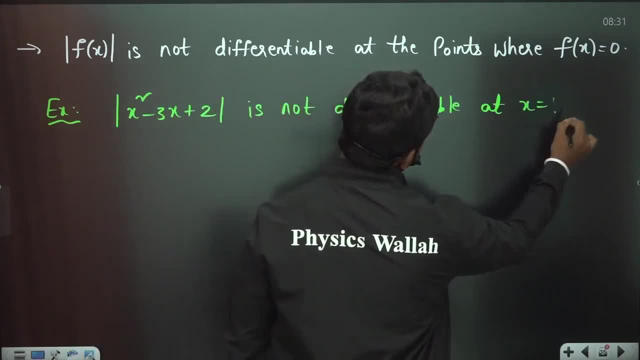 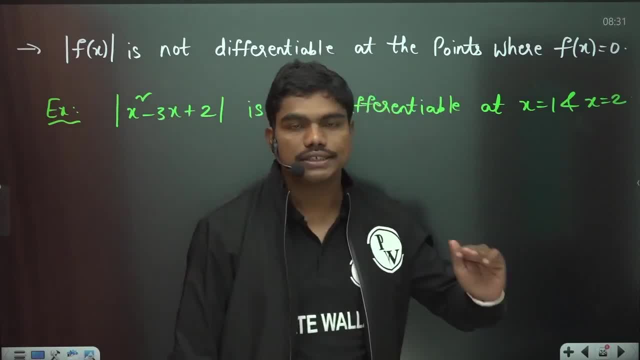 X is equal to 2 because at X is equal to 1 and X is equal to this function, which, and X is equal to this function, which, and X is equal to this function which is inside the modulus becomes 0: okay, so is inside the modulus becomes 0: okay, so. 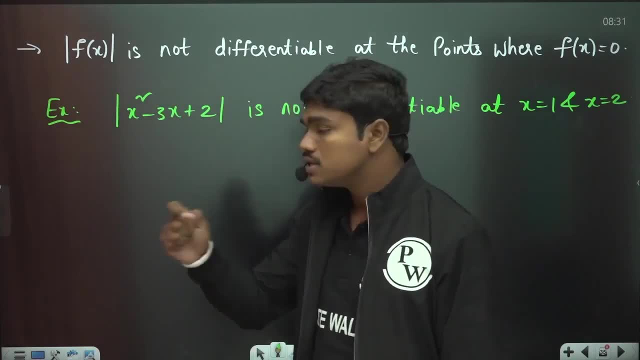 is inside the modulus becomes 0. okay, so whenever you have this function means if. whenever you have this function means if. whenever you have this function means if you identify those points where the you identify those points where the you identify those points where the function inside the modulus is 0 in such 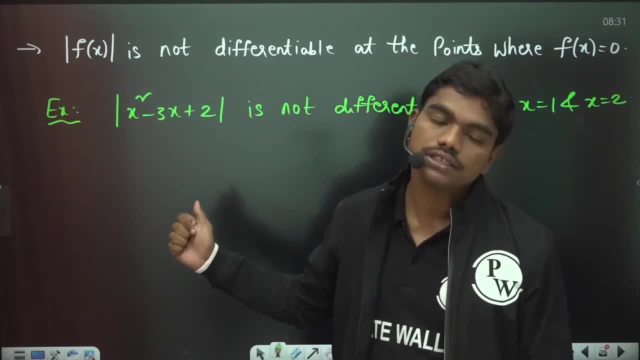 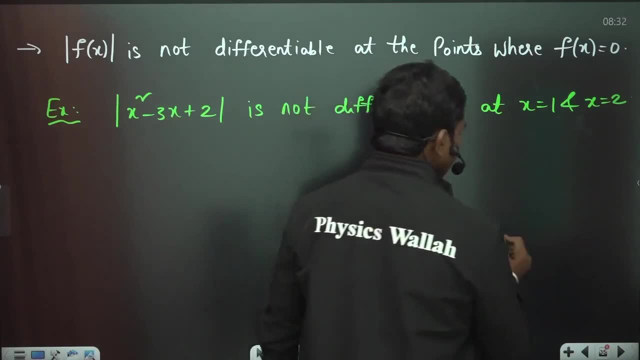 function inside the modulus is 0. in such function, inside the modulus is 0. in such cases, this functions won't be cases. this functions won't be cases, this functions won't be differentiable, clear and at that point differentiable, clear and at that point differentiable, clear, and at that point so 0, X, Y, like this. now what happens is: 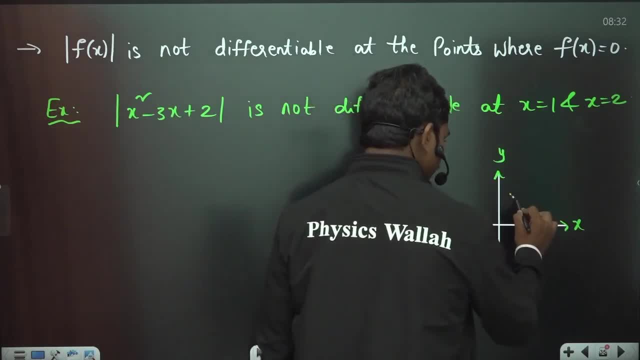 so 0 X Y like this. now what happens is so 0 X Y like this. now what happens is: look, let us suppose you got a sharp pitch. look, let us suppose you got a sharp pitch. look, let us suppose you got a sharp pitch like this: okay, let me draw more clearly. 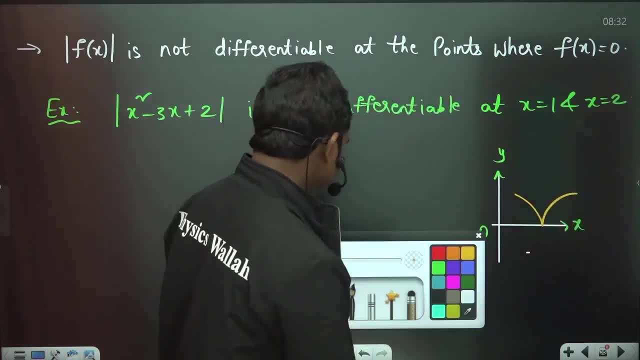 like this: okay, let me draw more clearly. like this: okay, let me draw more clearly. like this: you got a sharp pitch at some. like this: you got a sharp pitch at some. like this: you got a sharp pitch at some location, okay. so, when you got a sharp 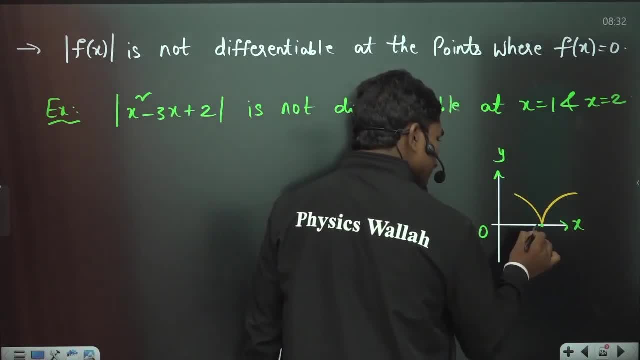 location. okay so when you got a sharp location: okay so when you got a sharp pitch, if this is the point if you take pitch, if this is the point if you take pitch, if this is the point if you take the left side, the tangent to this curve. 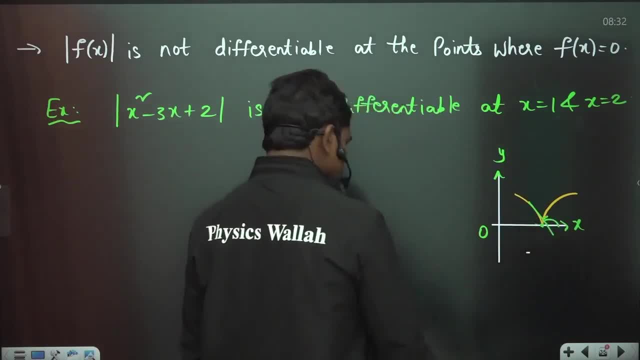 the left side, the tangent to this curve, the left side, the tangent to this curve, will be something like this: okay, so this will be something like this. okay, so, this will be something like this. okay, so this angle will be more than 90. similarly, if angle will be more than 90. similarly, if, 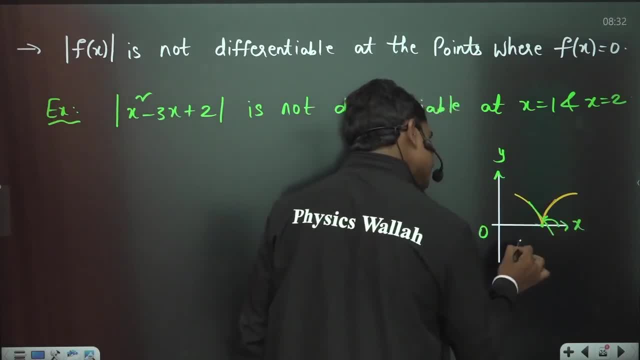 angle will be more than 90. similarly, if you draw a tangent in the right, you draw a tangent in the right, you draw a tangent in the right. neighborhood means somewhere here. if you neighborhood means somewhere here. if you neighborhood means somewhere here. if you take a tangent, this will be. you can see. 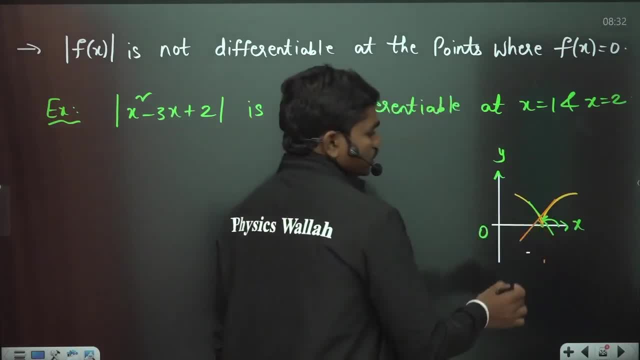 take a tangent, this will be you can see. take a tangent, this will be: you can see: this angle will be less than 90. okay, so this angle will be less than 90. okay, so this angle will be less than 90. okay, so one slope will be negative and another. one slope will be negative and another one slope will be negative and another slope will be positive. like you have seen, slope will be positive. like you have seen, slope will be positive, like you have seen in mod X case, whenever there is a sharp. in mod X case, whenever there is a sharp. 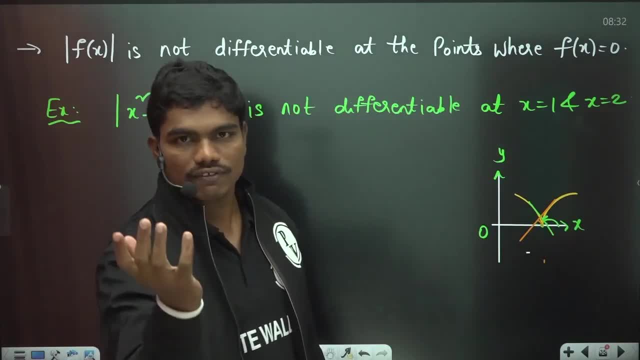 in mod X case, whenever there is a sharp pitch, at this sharp pitch on the right pitch, at this sharp pitch on the right pitch, at this sharp pitch on the right hand side, you will have some positive hand side. you will have some positive hand side. you will have some positive slope on the left hand side you may have. 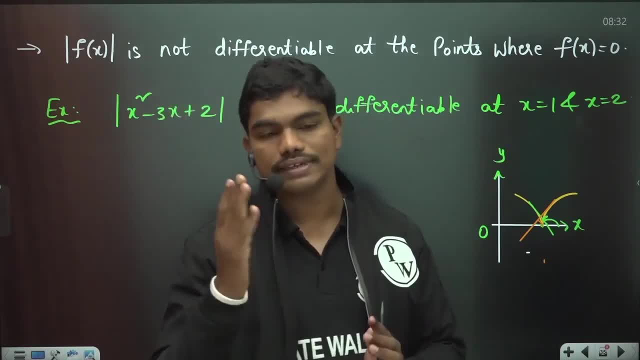 slope. on the left hand side, you may have slope. on the left hand side, you may have some negative slope. that's the reason: some negative slope. that's the reason: some negative slope. that's the reason why these two slopes means a right slope, why these two slopes means a right slope. 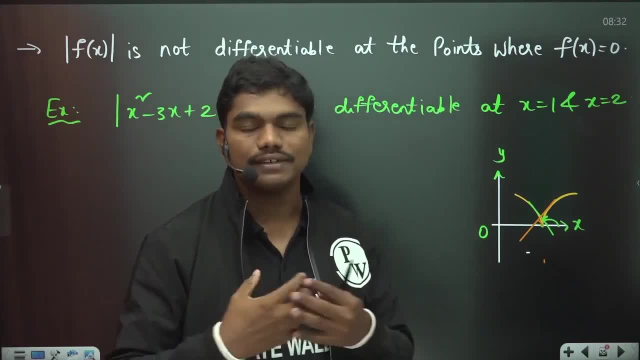 why these two slopes means a right slope and left slope, or you can say right and left slope, or you can say right and left slope, or you can say right derivative and left derivative, these two derivative and left derivative, these two derivative and left slope, won't become equal. generally, whenever you have a 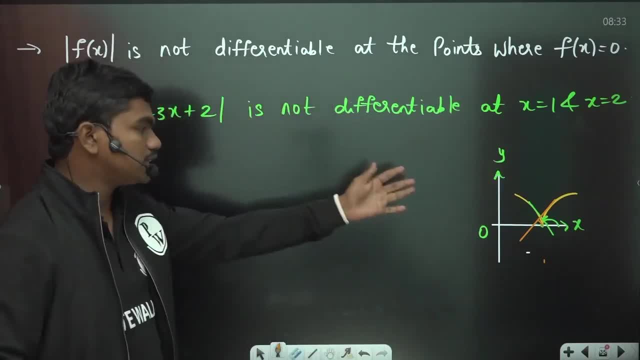 won't become equal generally whenever you have a. won't become equal generally whenever you have a sharp pitch okay. so that's why all sharp pitch okay. so that's why all sharp pitch okay. so that's why all these functions, they generate sharp. these functions, they generate sharp. 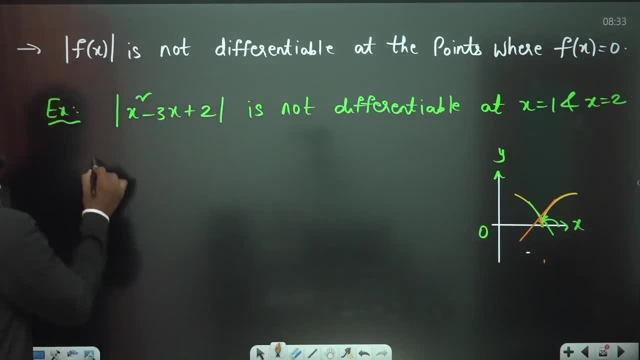 these functions, they generate sharp pages. at. you know these points, now pages at. you know these points, now pages at. you know these points now. similarly, mod sine X is not a. similarly, mod sine X is not a. similarly, mod sine X is not a. differentiable is not differentiable is. 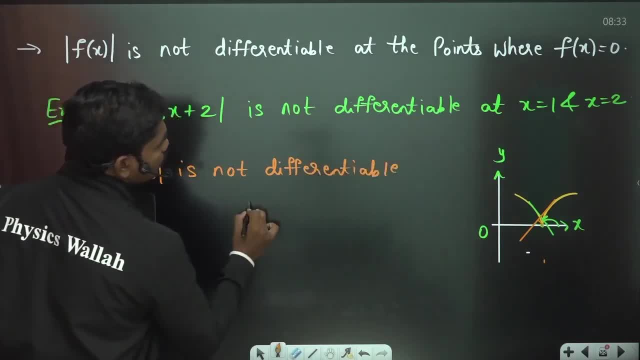 differentiable is not differentiable is differentiable, is not differentiable, is not differentiable. mod sine X is not not differentiable. mod sine X is not not differentiable. mod sine X is not differentiable. at X is equal to 0 plus or. differentiable at X is equal to 0 plus, or. 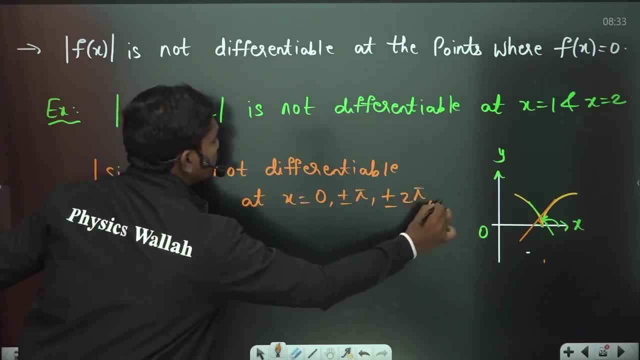 differentiable at X is equal to 0. plus or minus pi, plus or minus 2 pi. all these minus pi, plus or minus 2 pi, all these minus pi, plus or minus 2 pi, all these points, because you see all these points, points, because you see all these points. 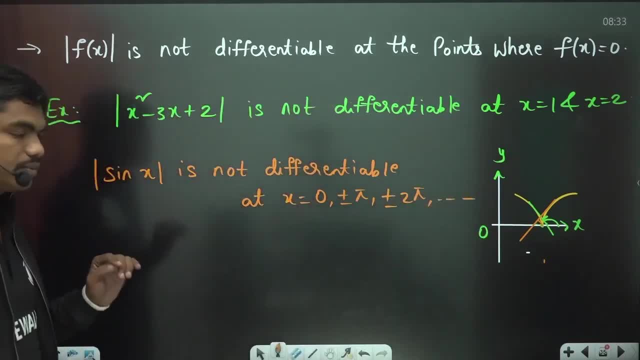 points, because, you see, all these points are the points where this sine X are the points where this sine X are the points where this sine X function is basically equal to 0. okay, so, function is basically equal to 0. okay, so function is basically equal to 0, okay, so, at all these points, these functions are. 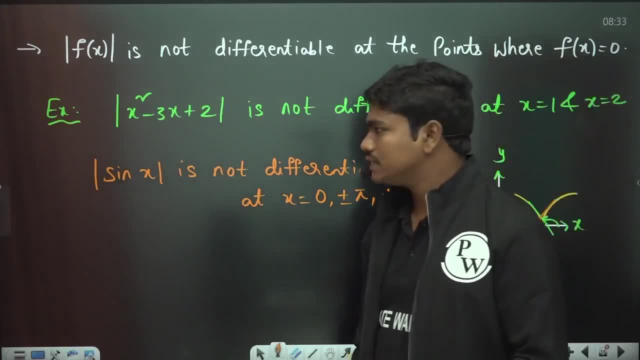 at all these points, these functions are at all these points, these functions are not differentiable clear. so with this we not differentiable clear. so with this we not differentiable clear. so with this we generally finish this differential, generally finish this differential, generally finish this differential calculus. okay, and basically, now we'll see. 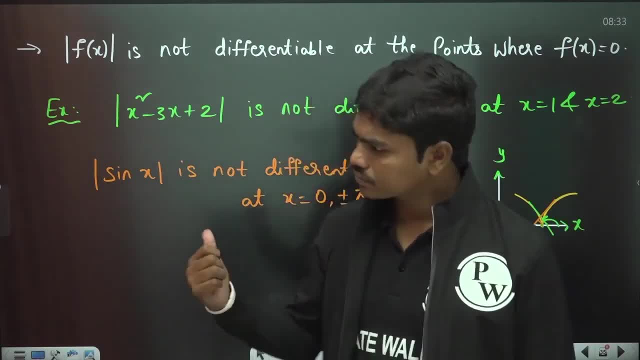 calculus. okay, and basically now we'll see calculus. okay, and basically now we'll see some applications of this differential, some applications of this differential, some applications of this differential calculus. like we'll talk about some calculus. like we'll talk about some calculus. like we'll talk about some applications of differentiable calculus. 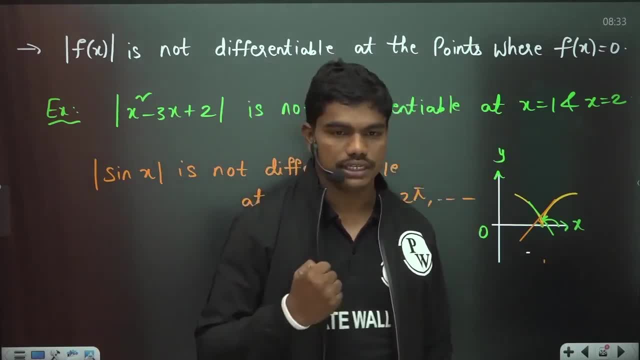 applications of differentiable calculus. applications of differentiable calculus like mean-value theorems. Taylor sees like mean-value theorems. Taylor sees like mean-value theorems. Taylor sees concept of maximum-minimum, all these concept of maximum-minimum, all these concept of maximum-minimum, all these things. okay, so let us quickly start mean. 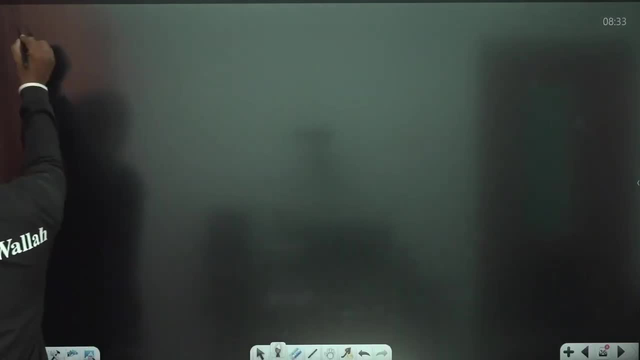 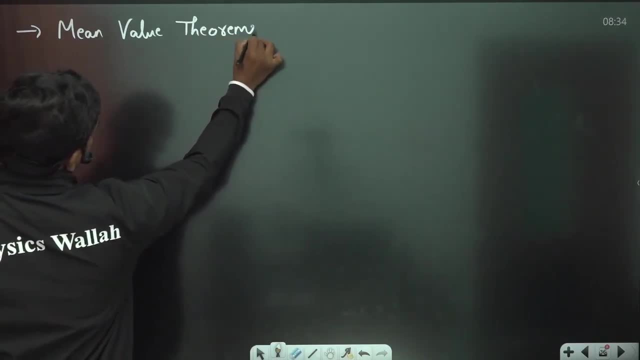 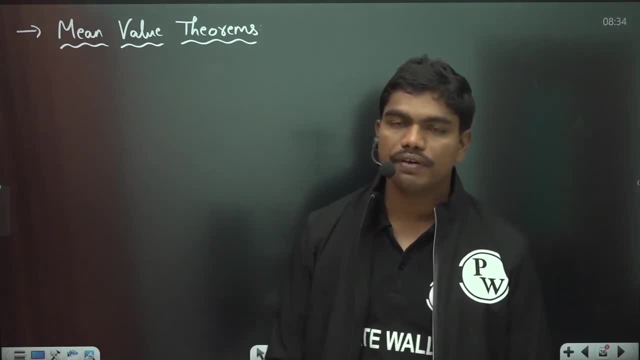 actually very much importance. I'll tell actually very much importance. I'll tell you why and all we. there are many you, why and all we. there are many you, why and all we. there are many concepts where we use this mean value. concepts where we use this mean value. 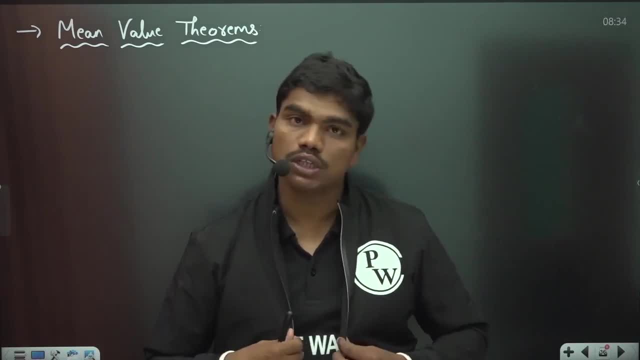 concepts where we use this mean value- theorem, for example. if you see the theorem, for example, if you see the theorem, for example, if you see the concept of maxima and minima is also one concept of maxima and minima is also one concept of maxima and minima is also one of the consequences of this mean value. 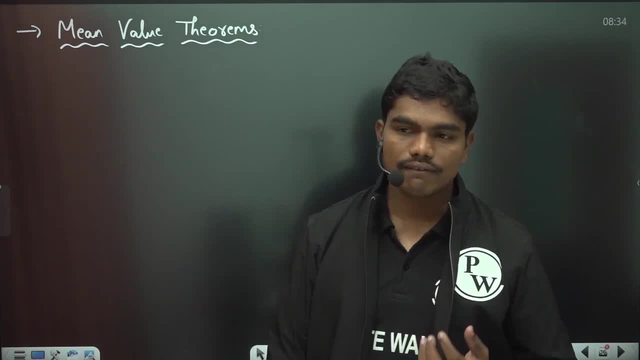 of the consequences of this mean value, of the consequences of this mean value, theorem okay, which is of course the whole theorem. okay, which is of course the whole theorem. okay, which is of course the whole system. we'll see now and we have a lot. system. we'll see now and we have a lot. 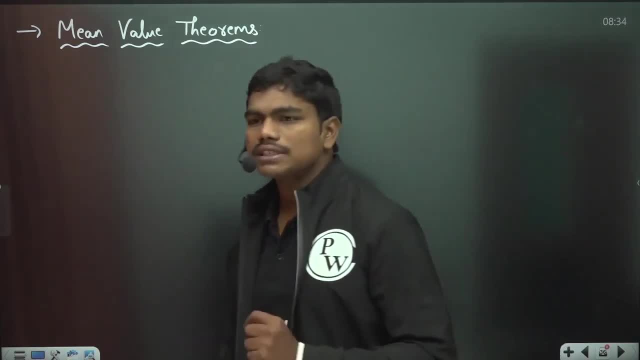 system we'll see now, and we have a lot of lot. many applications of this mean of lot. many applications of this mean of lot. many applications of this mean value theorems. okay, look, let me ask you value theorems. okay, look, let me ask you. 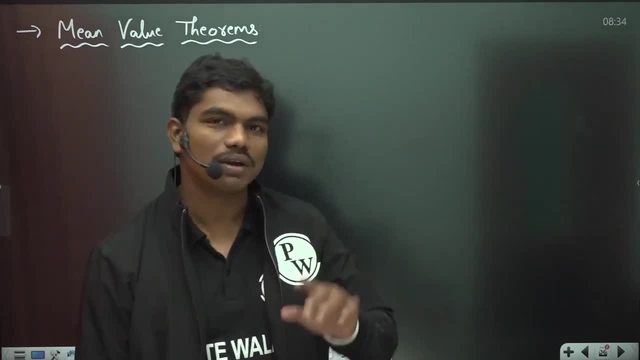 value theorems. okay, look, let me ask you one question. you can pause the video. one question: you can pause the video. one question: you can pause the video. we will see some general example, some we will see some general example, some we will see some general example, some normal example. now let me try to make. 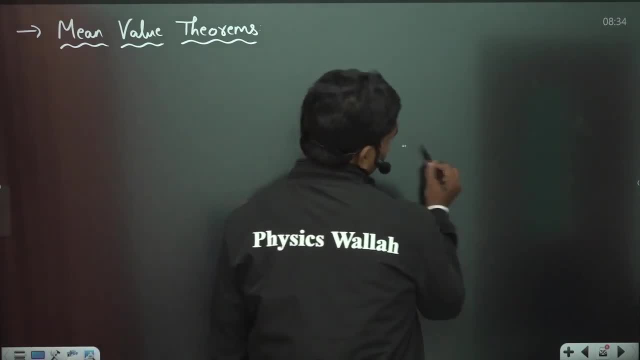 normal example now. let me try to make normal example now. let me try to make you understand this thing. look, let us you understand this thing. look, let us you understand this thing. look, let us suppose there is a straight out. suppose there is a straight out. suppose there is a straight out, straight out on this tight road. let us 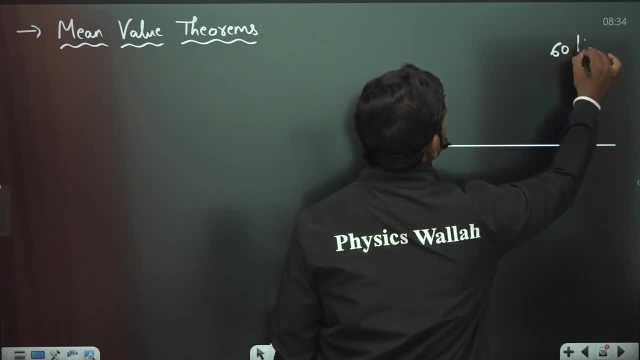 straight out on this tight road. let us straight out on this tight road. let us suppose they have kept some speed limit. suppose they have kept some speed limit. suppose they have kept some speed limit. some 60 kilometers per hour, let us. some 60 kilometers per hour, let us. 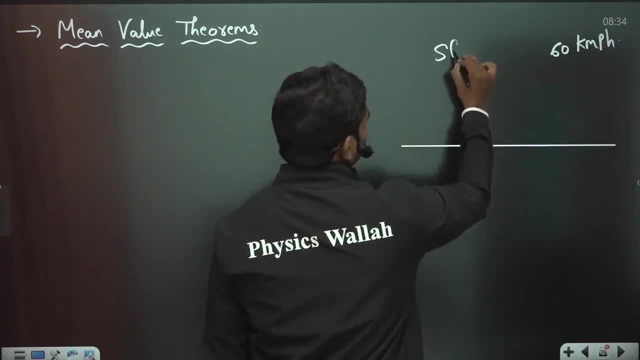 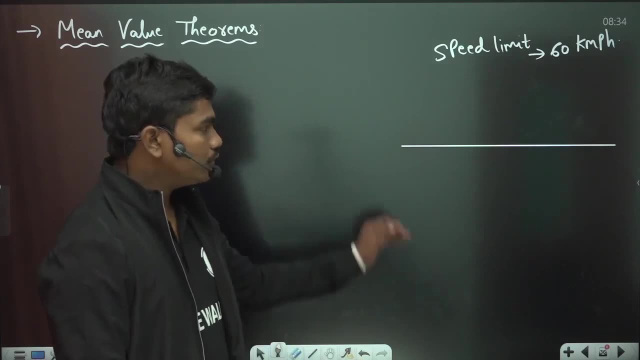 some 60 kilometers per hour, let us suppose okay. so 60 kilometers per hour is suppose okay. so 60 kilometers per hour? is suppose okay. so 60 kilometers per hour is the speed limit, for example, speed limit, the speed limit, for example, speed limit, the speed limit, for example, speed limit. so and they told you, if you cross 60, so, and they told you. if you cross 60, so, and they told you, if you cross 60 kilometers per hour, at any point on the kilometers per hour, at any point on the kilometers per hour, at any point on the sword, you will be charged, you will be. 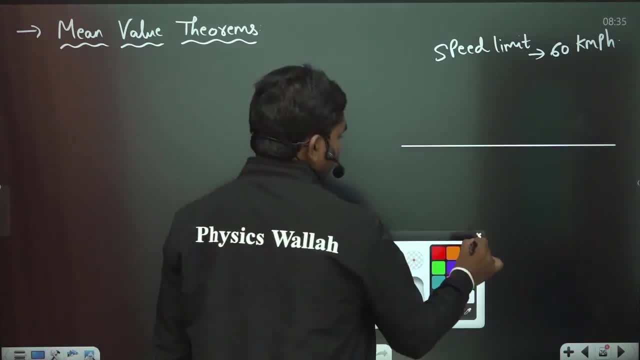 sword. you will be charged, you will be charged, you will be charged, you will be fine, actually. okay now. let us suppose: fine, actually okay now. let us suppose: fine, actually okay now. let us suppose there are speed guns there is one speed. there are speed guns, there is one speed. 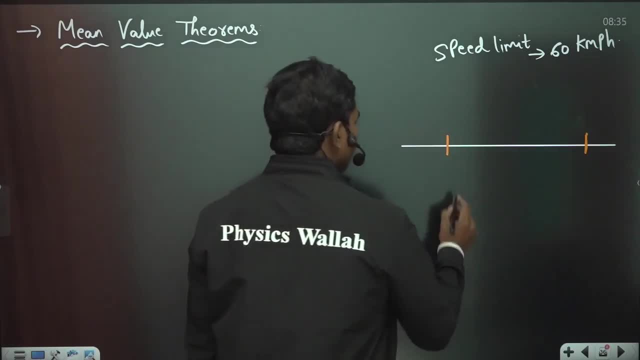 there are speed guns. there is one speed one here and also another speed one here, one here and also another speed one here, one here and also another speed one here. now, let us suppose, if this distance now, let us suppose, if this distance now, let us suppose if this distance between these two is some some two. 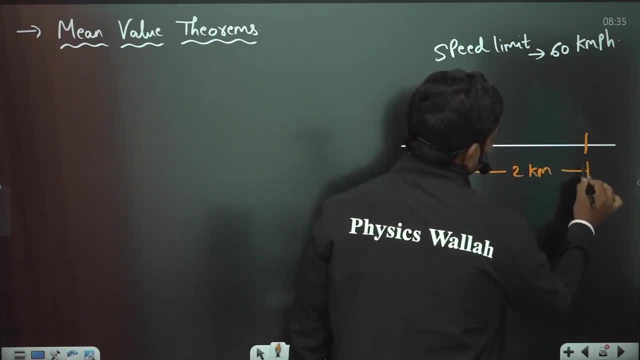 between these two is some some two. between these two is some some two kilometers gap. they have kept for kilometers gap. they have kept for kilometers gap. they have kept, for example, two kilometers gap. they have kept, example, two kilometers gap. they have kept, example, two kilometers gap. they have kept in two kilometer span. they have kept some. 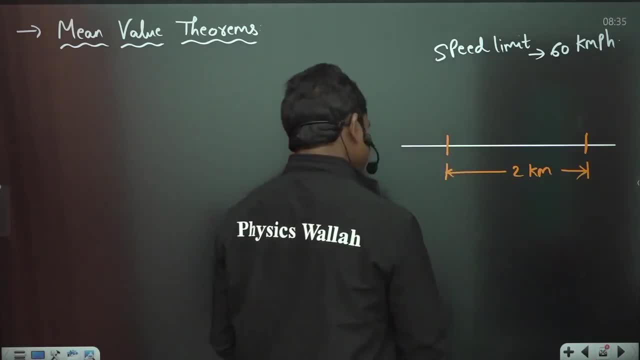 in two kilometer span. they have kept some in two kilometer span. they have kept some two speed guns- okay now. or let us say 20: two speed guns- okay now. or let us say 20: two speed guns- okay now. or let us say 20 kilometers- generally they are placed. 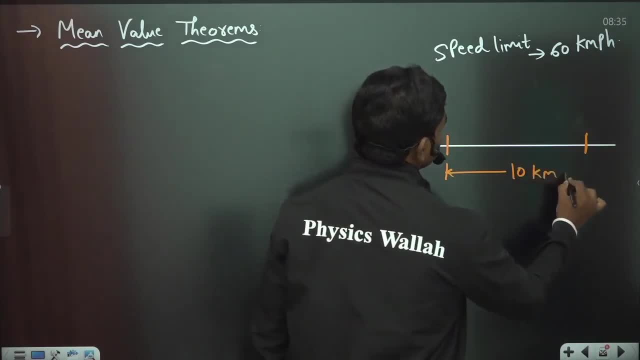 kilometers generally they are placed kilometers generally they are placed some 10 kilometers within the train, so 10, some 10 kilometers within the train, so 10, some 10 kilometers within the train, so 10 kilometers. let us say this is in 10 kilometers. let us say this is in 10. 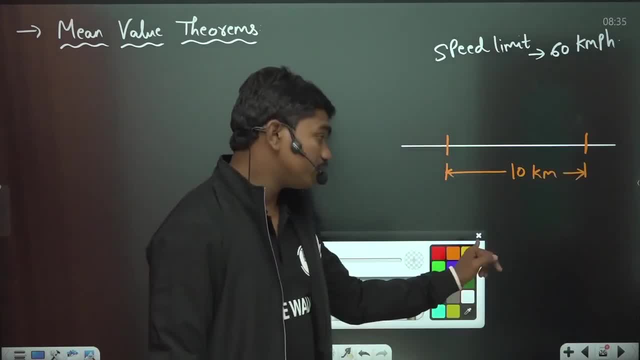 kilometers. let us say this is in 10 kilometers now. whenever you identify that kilometers now, whenever you identify that kilometers, now, whenever you identify that there's a speed gun, what we'll do. there's a speed gun? what we'll do. there's a speed gun, what we'll do. intentionally, we slow down the vehicle. 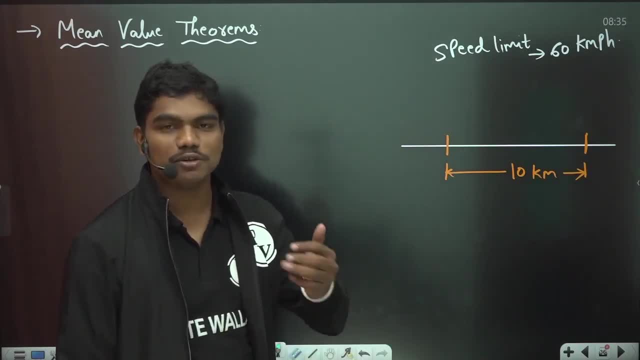 intentionally we slow down the vehicle. intentionally we slow down the vehicle, correct. we apply some brakes and we make correct. we apply some brakes and we make correct. we apply some brakes and we make sure that no fine gets imposed on us, so sure that no fine gets imposed on us. so 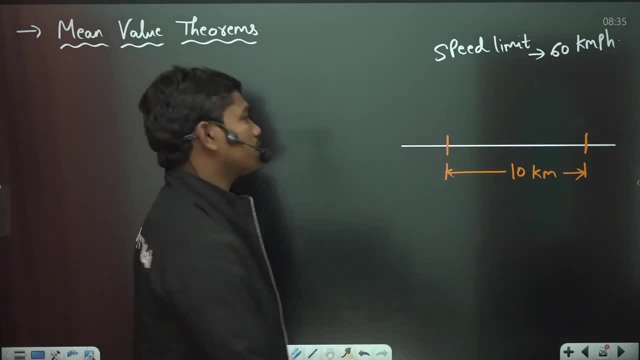 sure that no fine gets imposed on us. so what we do, we will try to you know slow. what we do, we will try to you know slow what we do, we will try to you know slow. down here: okay, so I came very fast. but down here: okay, so I came very fast. but 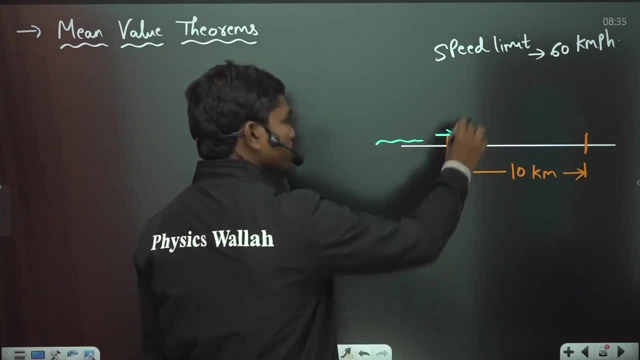 down here okay, so I came very fast, but then I slowed down here very slowly. I'm, then I slowed down here very slowly. I'm, then I slowed down here very slowly. I'm acting so good that people don't acting so good, that people don't acting so good that people don't recognize that I am moving above 60. 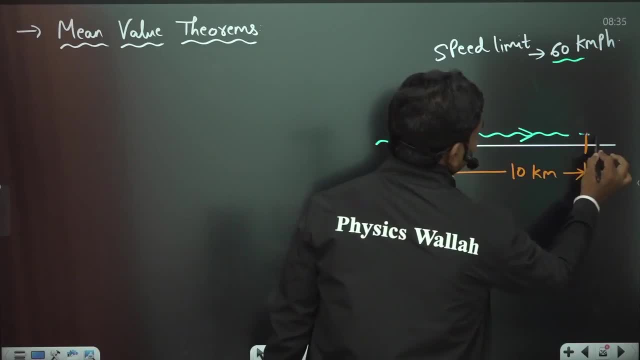 recognize that I am moving above 60. recognize that I am moving above 60, similarly in the main range. I am moving similarly in the main range. I am moving similarly in the main range. I am moving very fast again and at this point again, very fast again and at this point again. 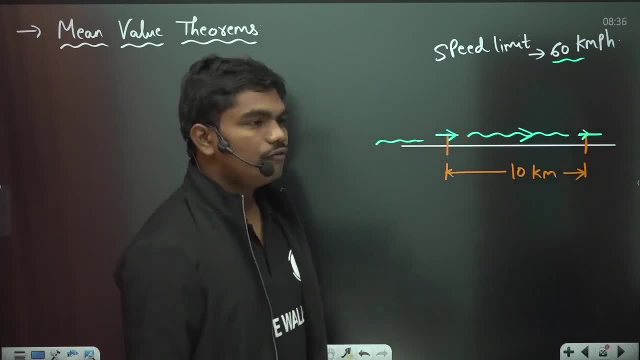 very fast again. and at this point again, I am slowing down to 30 or 40. let us say I am slowing down to 30 or 40. let us say I am slowing down to 30 or 40. let us say now, we assume that since we maintained 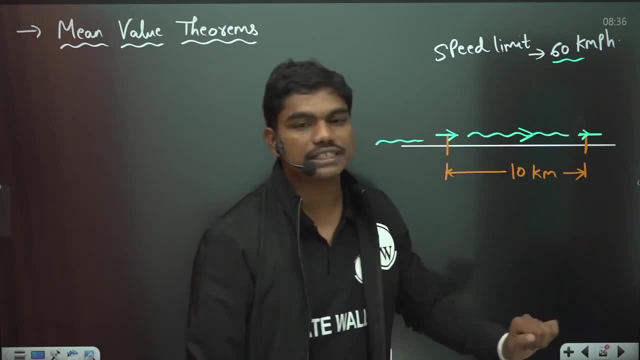 now we assume that since we maintained. now we assume that since we maintained some speed which is below that speed, some speed which is below that speed, some speed which is below that speed limit at these two speed gun locations, limit at these two speed gun locations, limit at these two speed gun locations, there is no fine on us, but actually we 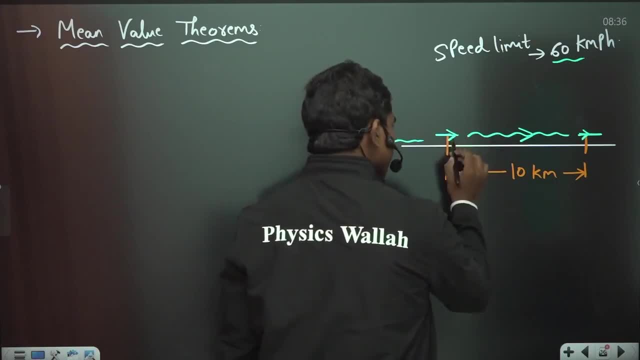 there is no fine on us, but actually we. there is no fine on us, but actually we can still be fine. how come look, let us can still be fine. how come look, let us can still be fine. how come look, let us suppose, if the time taken to cover these 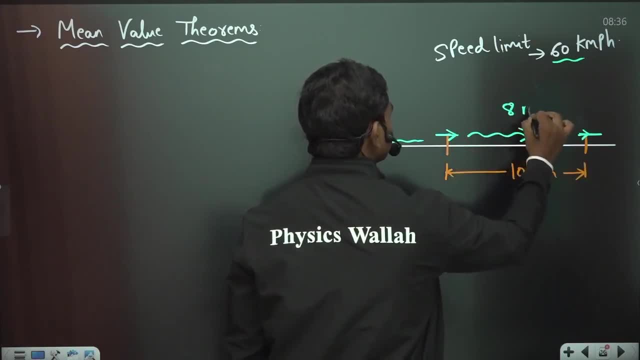 suppose if the time taken to cover these, suppose if the time taken to cover these two points is basically- let us suppose two points- is basically- let us suppose two points- is basically- let us suppose eight minutes, you have covered in eight. eight minutes, you have covered in eight. 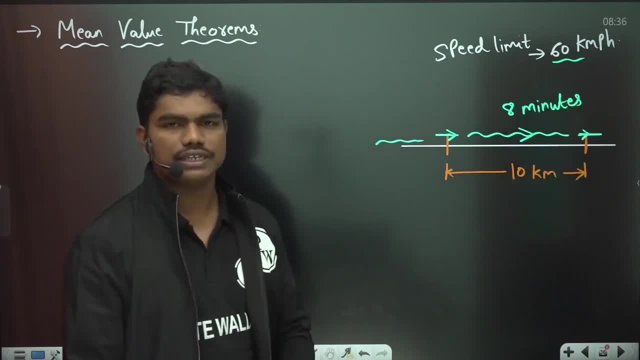 eight minutes. you have covered in eight minutes. you have gone this 10 kilometers minutes. you have gone this 10 kilometers minutes. you have gone this 10 kilometers, which is normal speed. if you direct 70, which is normal speed, if you direct 70, which is normal speed, if you direct 70 or 80, will easily cost 10 kilometers in. 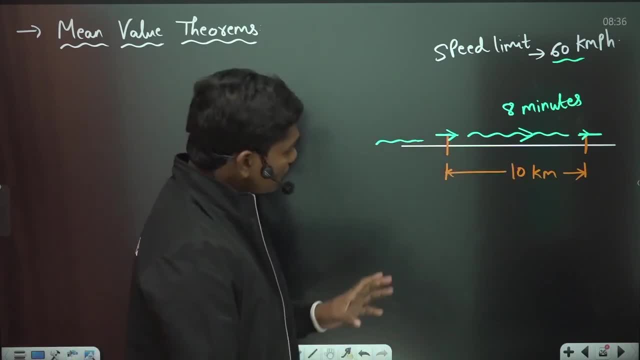 or 80 will easily cost 10 kilometers in, or 80 will easily cost 10 kilometers in eight, eight minutes. okay. so now, if you eight eight minutes, okay, so now, if you eight eight minutes. okay. so now, if you see, if you observe one thing, you can 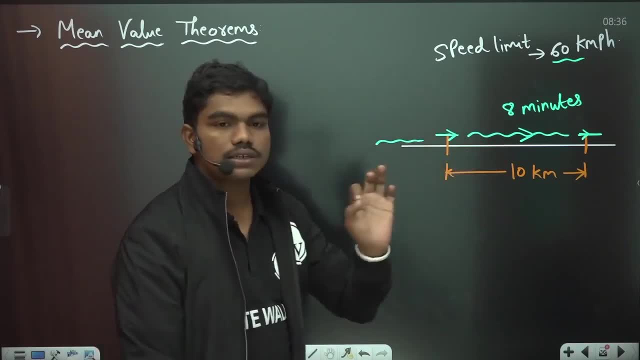 see if you observe one thing. you can see, if you observe one thing, you can cross these two points only in eight. see, if you observe one thing, you can cross these two points only in eight. see, if you observe one thing, you can cross these two points only in eight minutes. only at least at some location, if you. 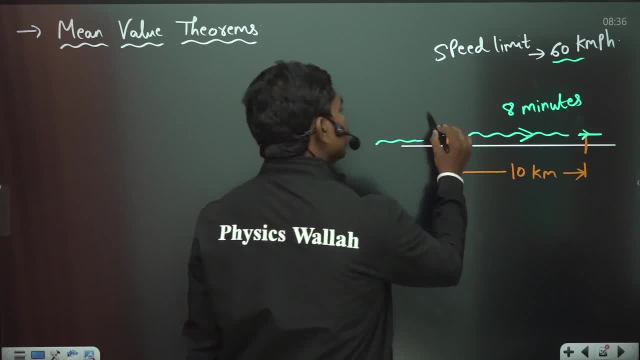 minutes only, at least at some location. if you minutes only, at least at some location. if you have crossed that 60 speed, yes or no. have crossed that 60 speed, yes or no? have crossed that 60 speed, yes or no means definitely here. you maintain that. 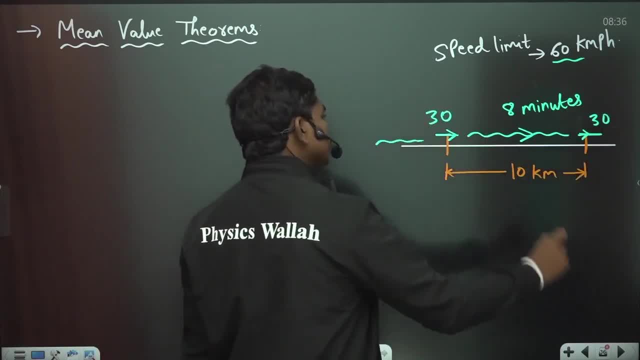 means definitely here. you maintain that means definitely here. you maintain that T. here also you maintain 30 kilometers T. here also you maintain 30 kilometers T. here also you maintain 30 kilometers per hour, but definitely somewhere in per hour, but definitely somewhere in per hour, but definitely somewhere in between. you have definitely crossed this. 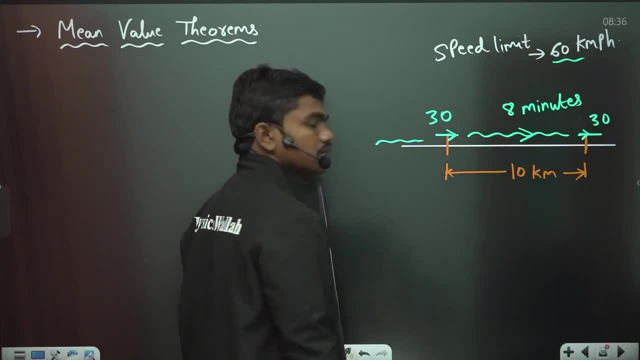 between you have definitely crossed this. between you have definitely crossed this speed. that's the reason why, within eight speed, that's the reason why within eight speed. that's the reason why, within eight minutes, you have cleared this 10 minutes. you have cleared this 10 minutes. you have cleared this 10 kilometers s or no, because if you have, 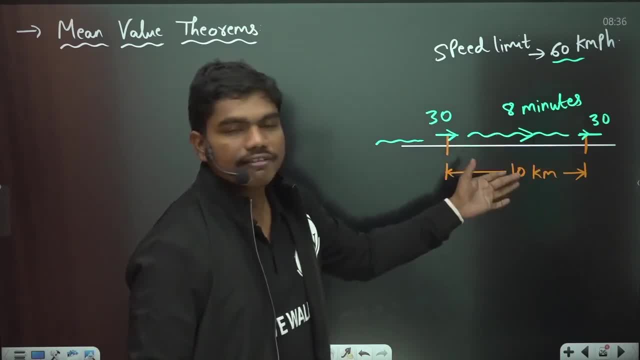 kilometers s or no, because if you have kilometers s or no, because if you have traveled below 60 kilometers per hour, traveled below 60 kilometers per hour, traveled below 60 kilometers per hour continuously, it would have taken you more. continuously it would have taken you more. 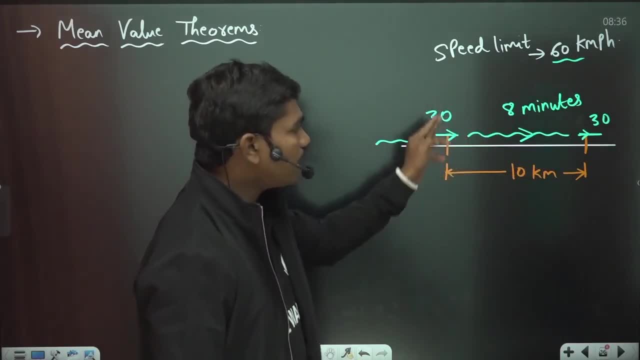 continuously. it would have taken you more than 10 minutes, but this vehicle number than 10 minutes. but this vehicle number than 10 minutes, but this vehicle number is registered here and in less than 8 is registered here and in less than 8 is registered here and in less than 8 minutes this vehicle number is again. 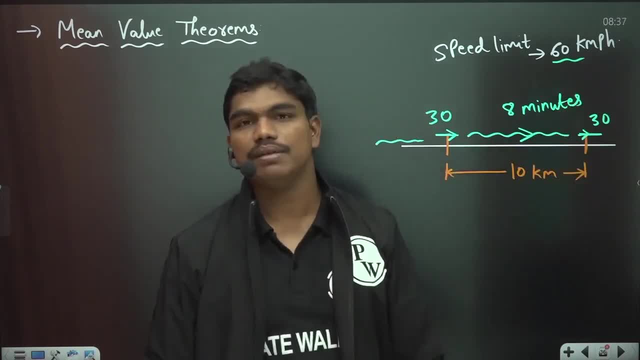 minutes. this vehicle number is again minutes. this vehicle number is again registered here. that means, meanwhile, this registered here. that means, meanwhile, this registered here. that means, meanwhile, this person has crossed the speed limit of 60. person has crossed the speed limit of 60. person has crossed the speed limit of 60. that this can be identified using mean. 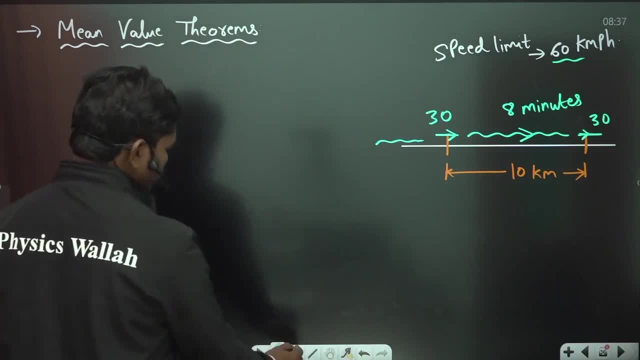 that this can be identified using mean, that this can be identified using mean value theorems- okay, look how I will tell value theorems. okay, look how I will tell value theorems. okay, look how I will tell you now. so first let me give the concept. 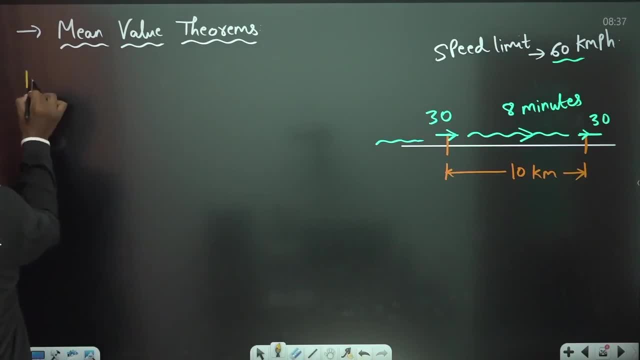 you now. so first let me give the concept you now. so first let me give the concept of this Lagrange's mean value theorem, so of this Lagrange's mean value theorem, so of this Lagrange's mean value theorem, so the first fundamental theorem is. the first fundamental theorem is: 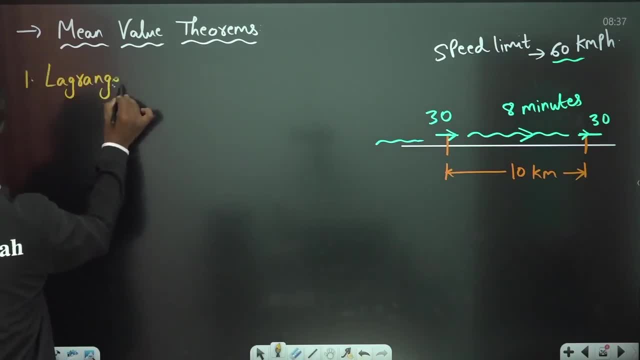 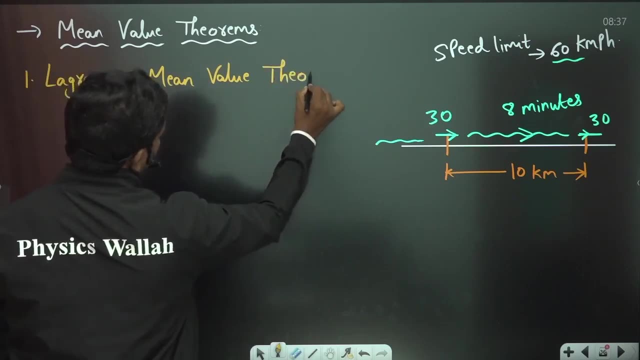 the first fundamental theorem is Lagrange's, Lagrange's, Lagrange's, Lagrange's, Lagrange's, Lagrange's mean value. here Lagrange's mean value, mean value. here Lagrange's mean value, mean value, here Lagrange's mean value theorem. so let's see what is this. 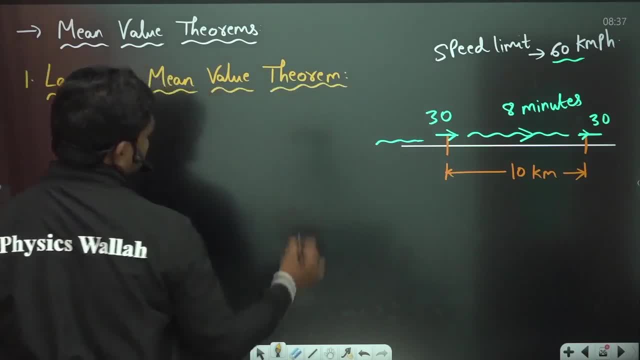 theorem. so let's see what is this theorem. so let's see what is this. Lagrange's mean value theorem. Lagrange's Lagrange's mean value theorem. Lagrange's Lagrange's mean value theorem. Lagrange's mean value theorem if f of X is. 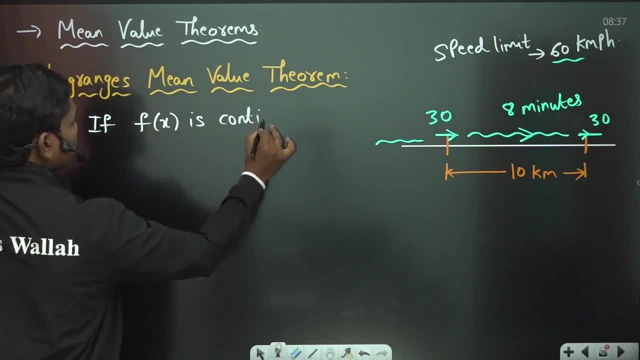 mean value theorem if f of X is mean value theorem. if f of X is continuous. if f of X is continuous on continuous. if f of X is continuous on continuous. if f of X is continuous on closed interval a comma B and it is. closed interval a comma B and it is. 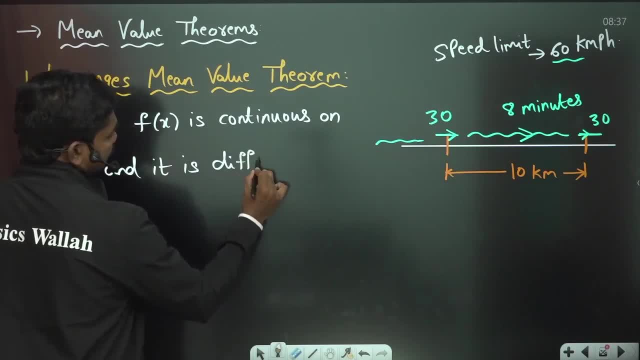 closed interval a comma B, and it is differentiable. it is differentiable and differentiable. it is differentiable and differentiable, it is differentiable and it is differentiable on open interval. it is differentiable on open interval. it is differentiable on open interval a comma B. then there exists a value C. 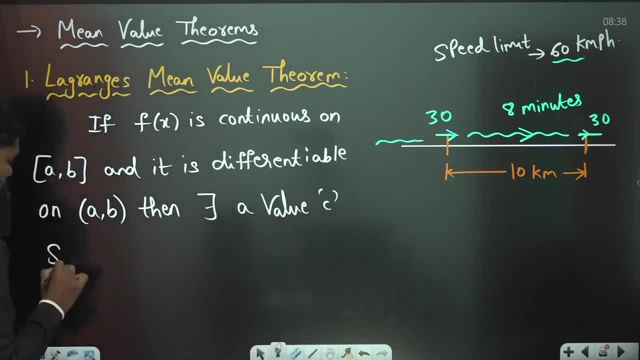 a comma B, then there exists a value C. a comma B, then there exists a value C, then there exists a value C such that such, then there exists a value C such that such, then there exists a value C such that such that X belongs to C. I mean, sorry, X. 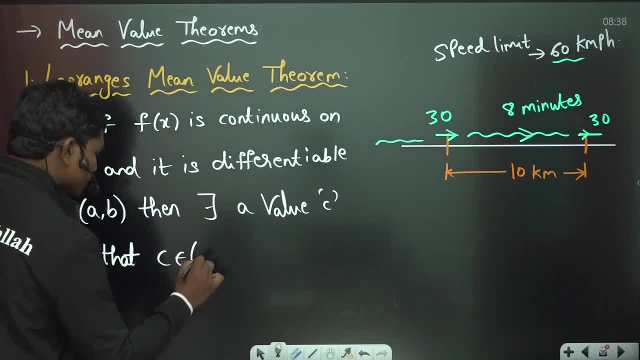 that X belongs to C. I mean sorry X that X belongs to C. I mean sorry X such that C belongs to a comma B and F. such that C belongs to a comma B and F. such that C belongs to a comma B and F. dash of C. 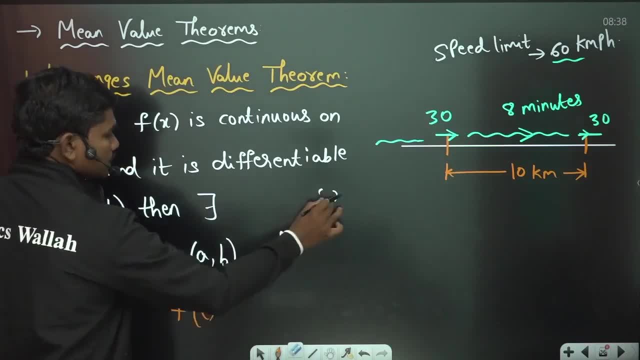 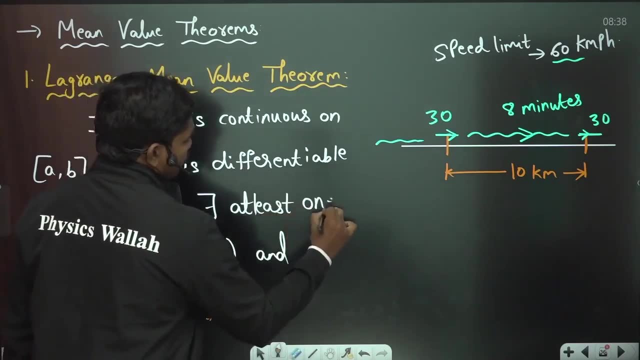 dash of C. dash of C. they exist at least one value it at. they exist at least one value it at. they exist at least one value it at least one value. see, okay, we'll write at least one value. see, okay, we'll write at least one value. see, okay, we'll write at least one value. see, at least one value. 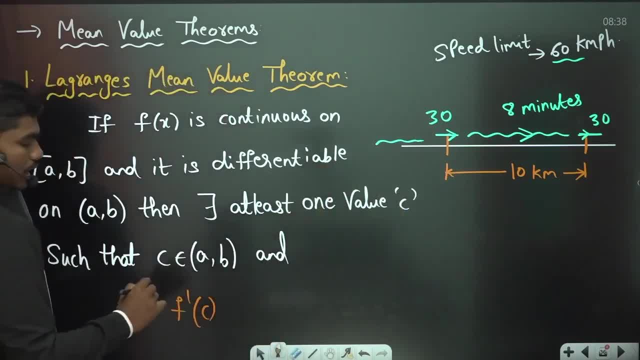 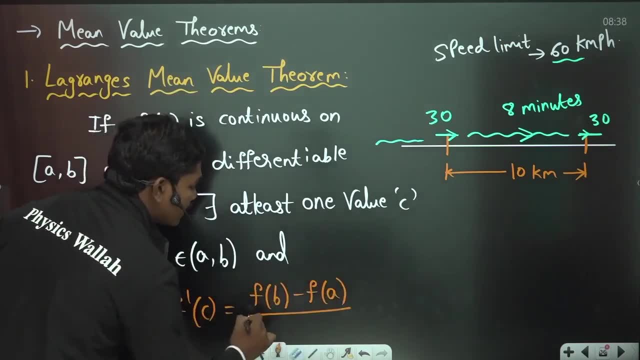 least one value see such that C belongs to a comma B and F dash of C is equal to such that C belongs to a comma B and F dash of C is equal to such that C belongs to a comma B and F dash of C is equal to F of B minus F of a divided by B. 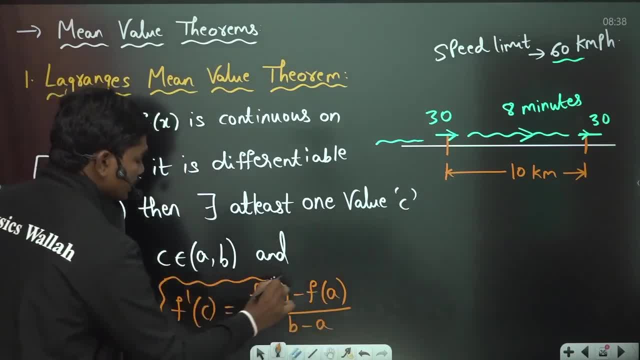 F of B minus F of a divided by B. F of B minus F of a divided by B minus a actually here. okay. so this formula is minus a actually here. okay. so this formula is minus a actually here. okay. so this formula is actually important and we'll. 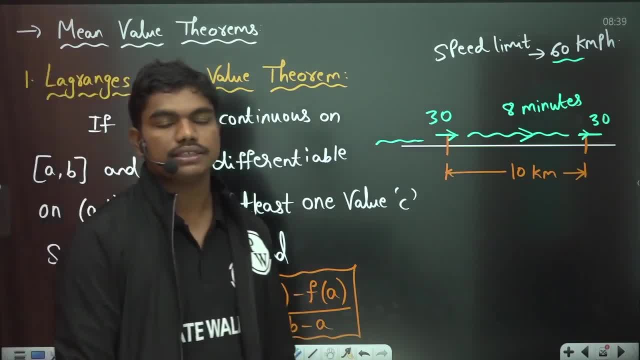 actually important and we'll actually important and we'll see how this formula is coming. what is this F of see how this formula is coming? what is this F of see how this formula is coming? what is this F of B minus F of a by B minus a let? 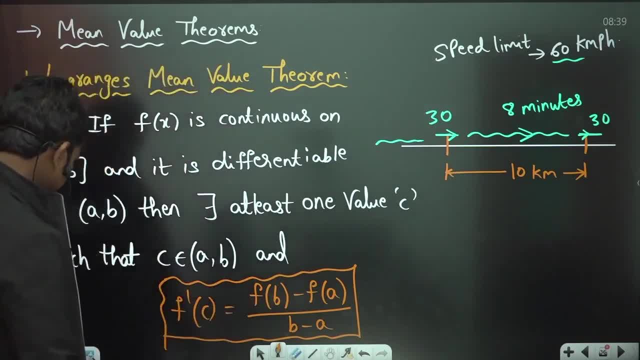 B minus F, of a by B minus a. let B minus F of a by B minus a. let us try to understand this, okay. so what we are us try to understand this, okay. so what we are us try to understand this okay. so what we are trying to do is look F dash of C is. trying to do is look F dash of C is trying to do is look F dash of C is equal to F of a minus F of a by B minus. equal to F of a minus F of a by B minus. equal to F of a minus F of a by B minus a. so what is the meaning of this? 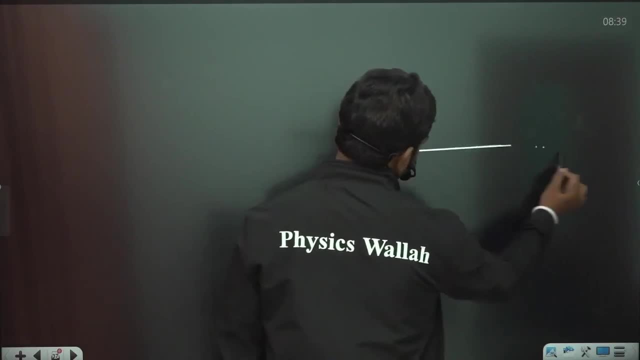 a. so what is the meaning of this? a. so what is the meaning of this? actually look if you take this curve for actually look. if you take this curve for actually look. if you take this curve, for example: this is your x-axis, this is your example, this is your x-axis, this is your 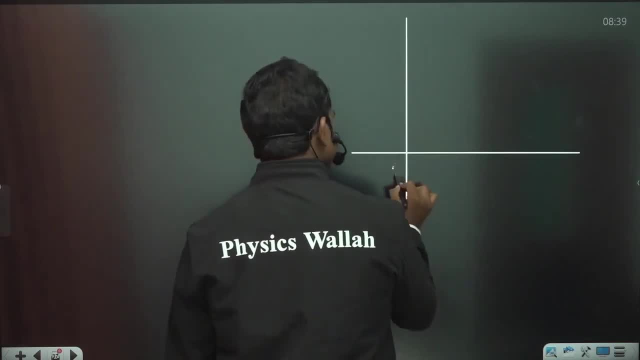 example, this is your x-axis, this is your x-axis, and let us say this is your y-axis x-axis, and let us say this is your y-axis x-axis, and let us say this is your y-axis. for example, so 0 X minus X Y and 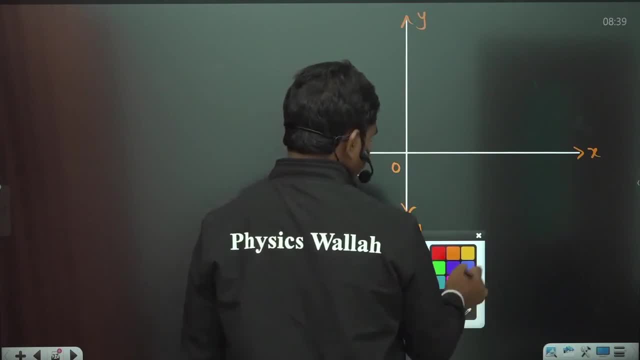 for example, so 0 X minus X Y, and for example, so 0 X minus X Y and minus Y. so let us suppose you have some minus Y. so let us suppose you have some minus Y. so let us suppose you have some curve like this: some curve, some random. 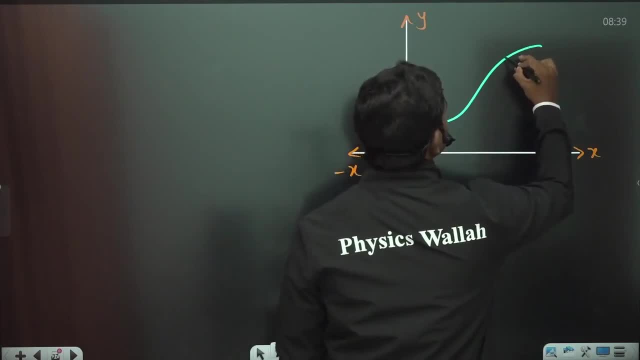 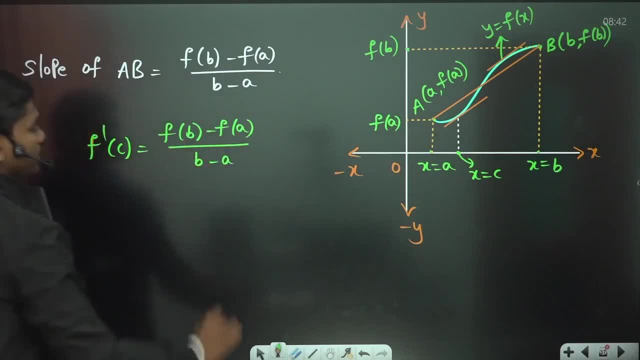 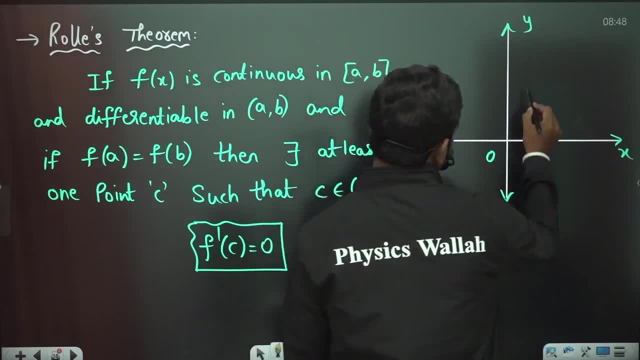 X, for example. so this is: y is equal to F of B minus F of A. Y, for example. so this is y is equal to F of B minus F of A. Okay, Now you see here, let us suppose, if there is some function like this, some function like 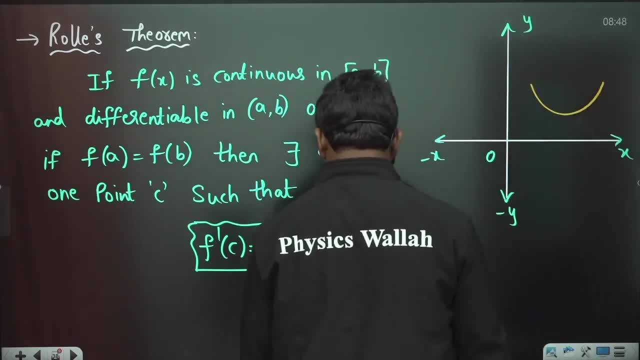 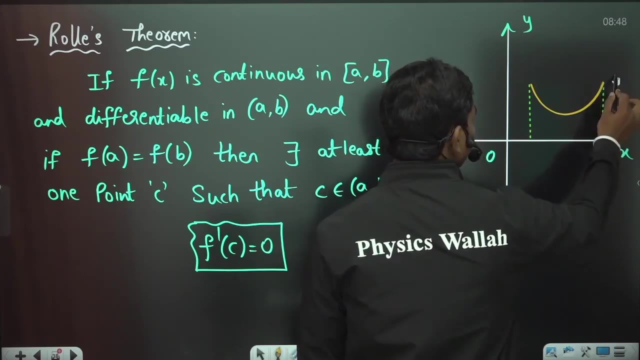 this and function like this, for example. now, in such case, here, if you plot the coordinates: this is X is equal to a. this is X is equal to B. X is equal to B. this is X is equal to B. x is equal to b. Let us say: 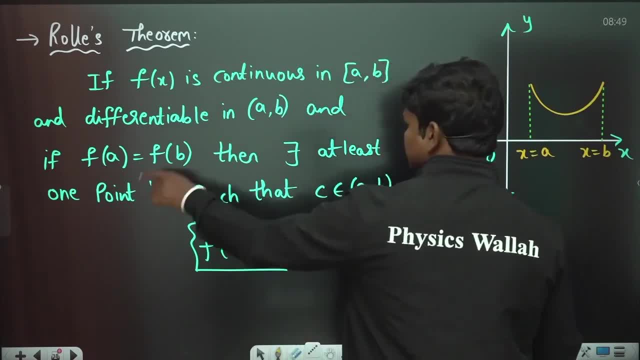 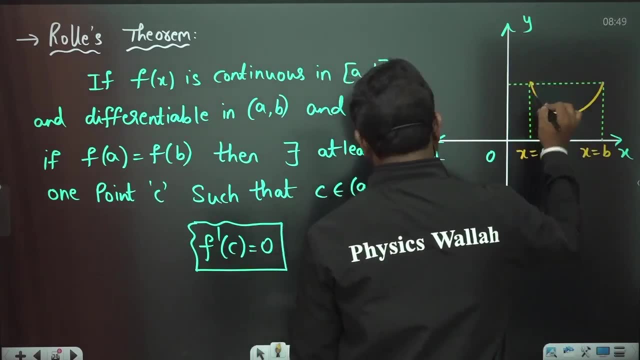 and we know, means we have assumed this assumption- that f of a and f of v both are same, means these two points are on the same horizontal line, correct? so if you see this point means if you write the coordinates of this point, this point has the coordinates a, comma, f of a and this point has 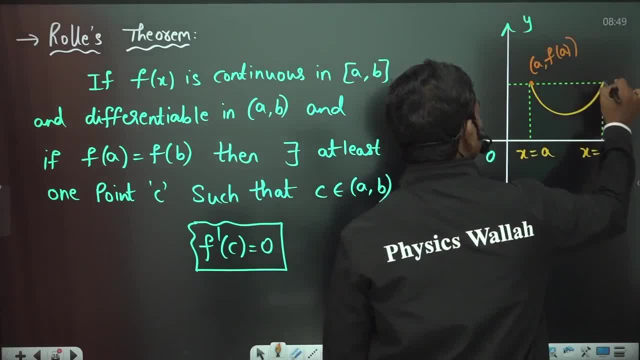 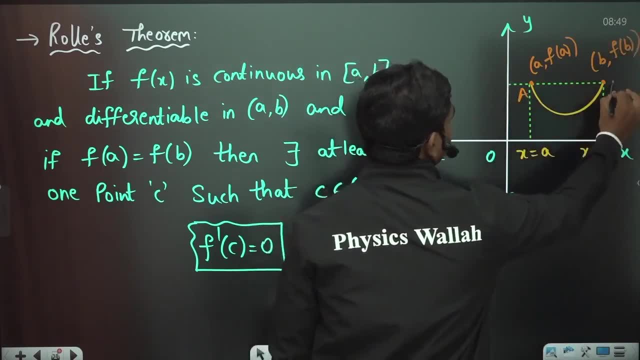 the coordinates b comma f. this point has the coordinates b comma f of b actually here, okay, and you can see capital a, capital b, for example. then, if you see, the slope of this line is zero, correct, because the line connecting these two points is horizontal this time. so whenever the 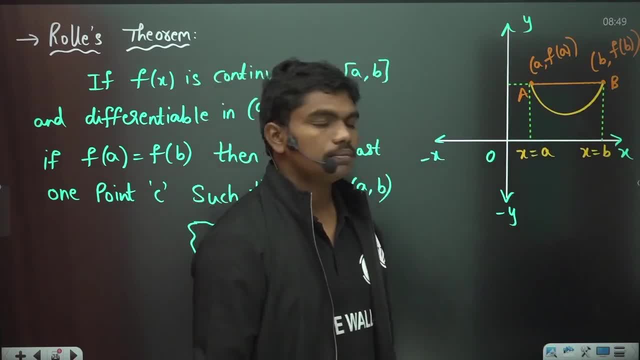 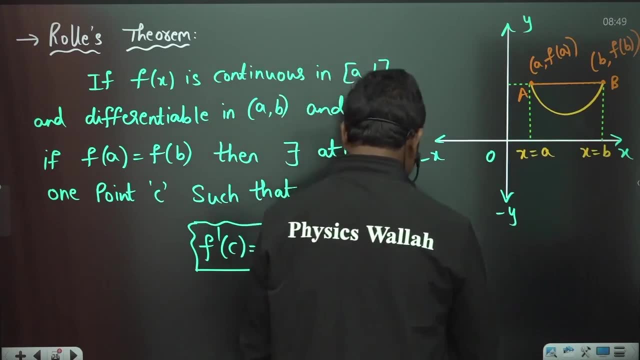 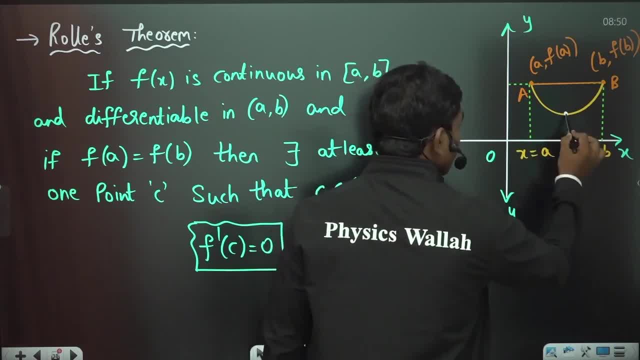 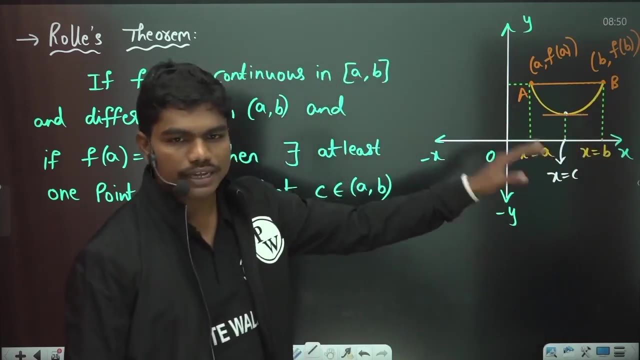 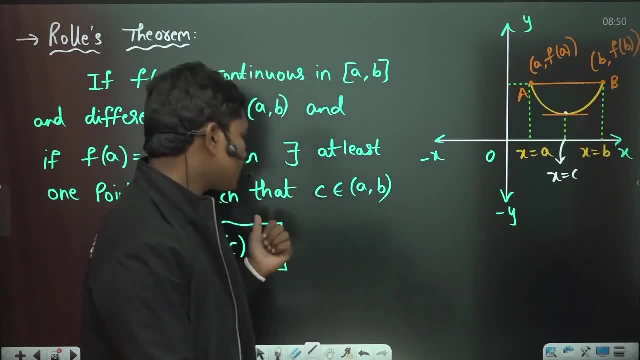 concept of maxima also. okay. so at stationary points, basically the values of x, where this differentiation is zero, are called stationary points, and to identify whether you have a maxima or not, you can say that x is equal to x and x is equal to x and x is equal to x. 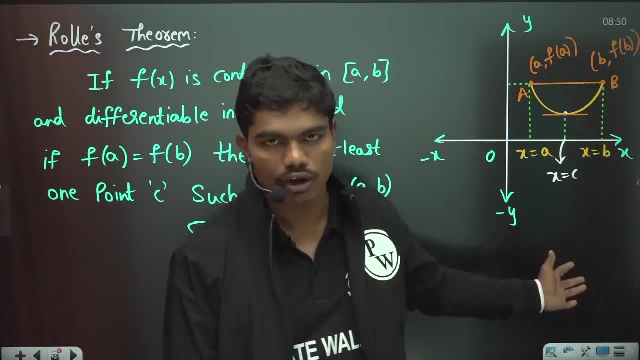 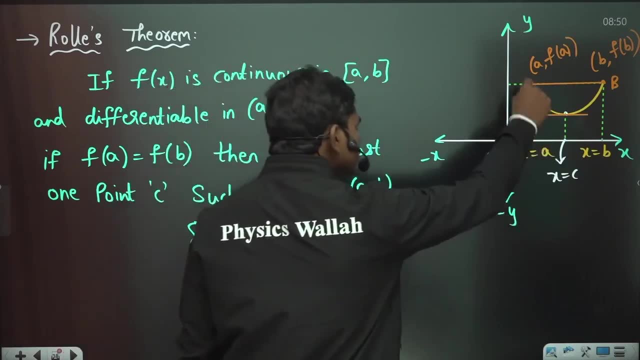 maximum or minimum, you need to go for something called second derivative test. i'll talk about it when i go to concepts of maxima and minima. okay, so right now, my main intention is to tell you that whenever there is some function like this, such that the functional values are same, definitely. 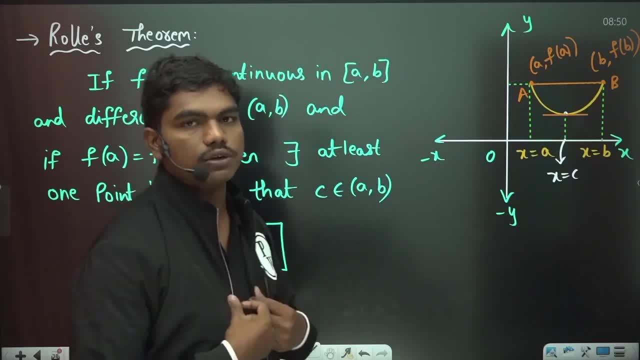 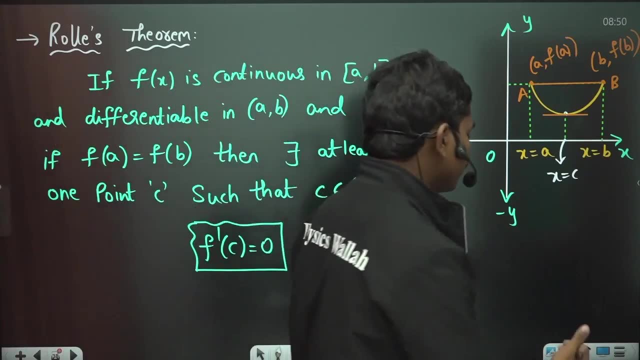 there exists a point where this f dash of c is actually equal to zero clear. so this is basically the foundation for the concept of maxima and minima, of course, okay, so we'll go for that in a moment, but this is the whole theorem. okay, now cauchy's mean value theorem is again something like: 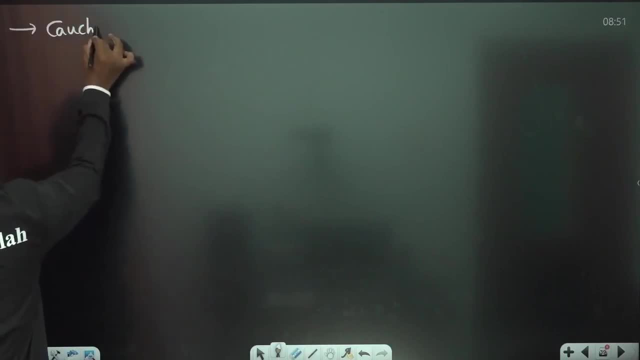 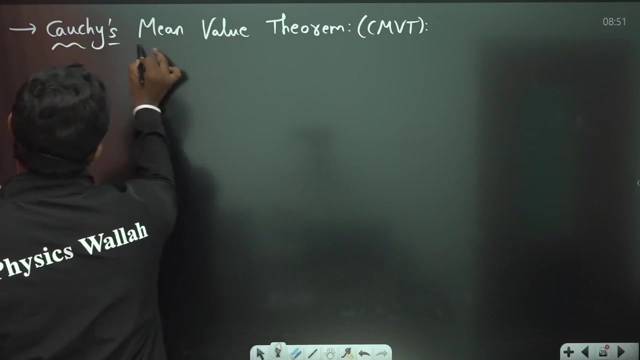 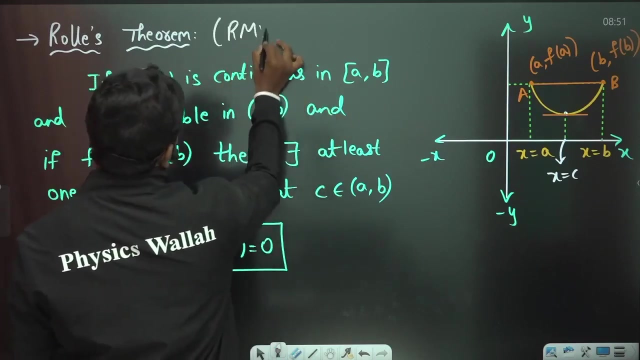 this cauchy's mean value theorem. cauchy's mean value theorem, which is being generally written as CMVT and, ofcourse, if you see this, aVolts mean value theorem. sometimes it is known with the name RMVT, so aVolts mean value theorem and this is cauchy's mean value theorem, so aVolts mean. 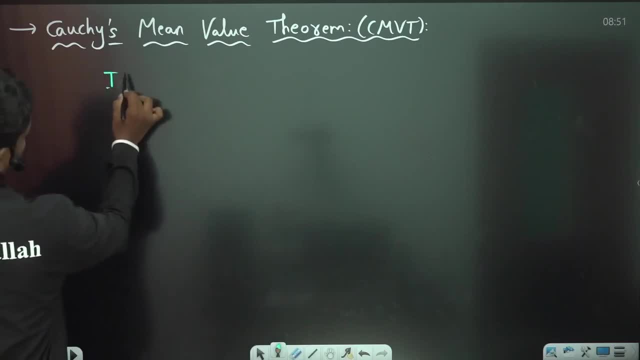 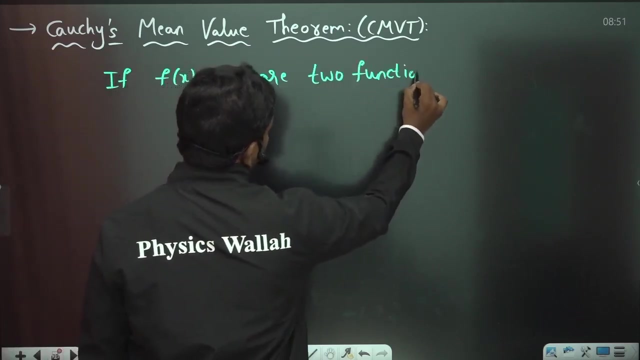 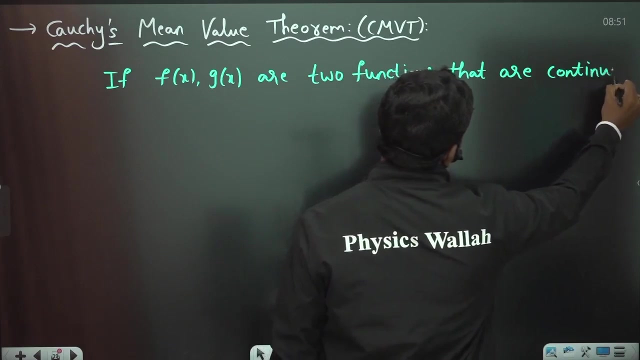 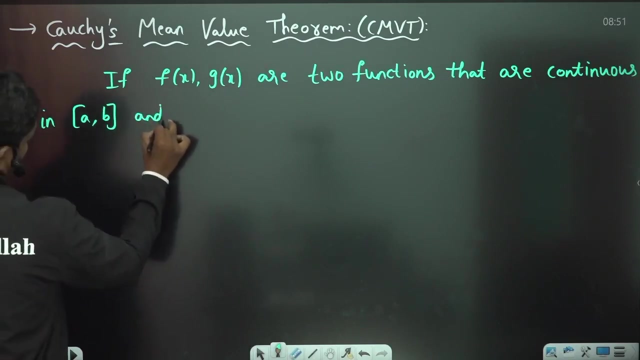 is something like this: If f of x comma g of x, this is nothing but application of Lagrange's to two functions simultaneously. If f of x comma g of x are two functions, are two functions that are continuous, that are continues in a comma b and differentiable in open a comma. 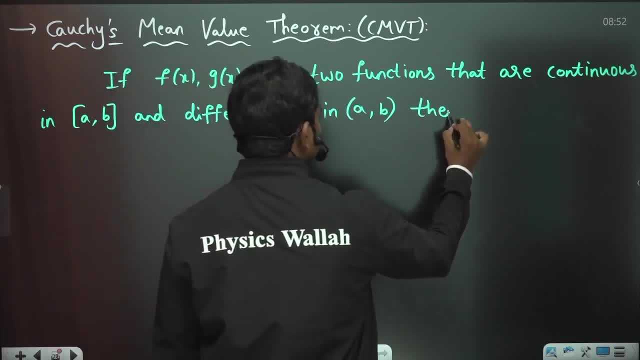 b and differentiable in open a comma b, then there exist at least one point c, which is known to me as δεν and where we have at least one integral x comma b that are continuous and interchangeable in open a comma b, and then they exist at least one point c, If i 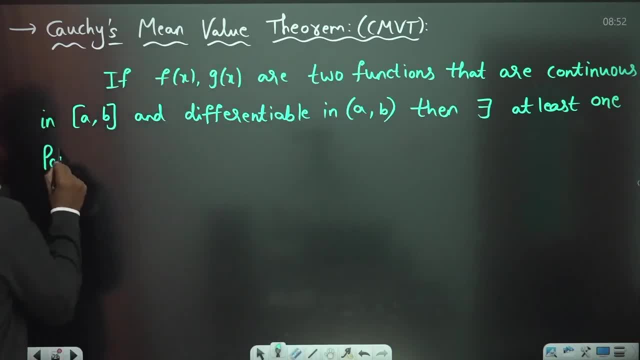 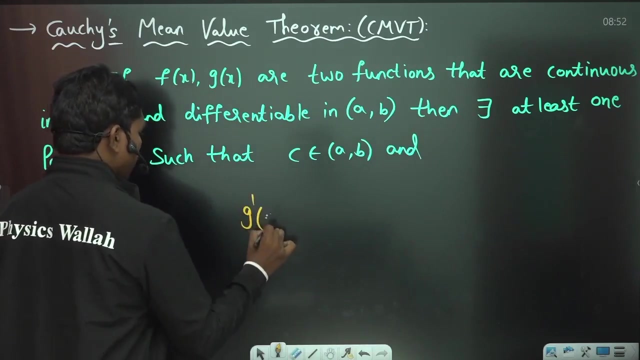 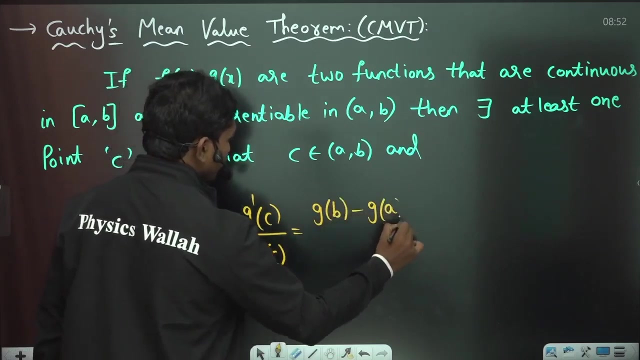 there exists at least one point c, such that c belongs to a comma, b and and g dash of c by f dash of c. this is equal to g of b minus g of a, divided by f of b minus f of a. actually, okay, so this is how we have the result, basically g dash of c by f dash of c. 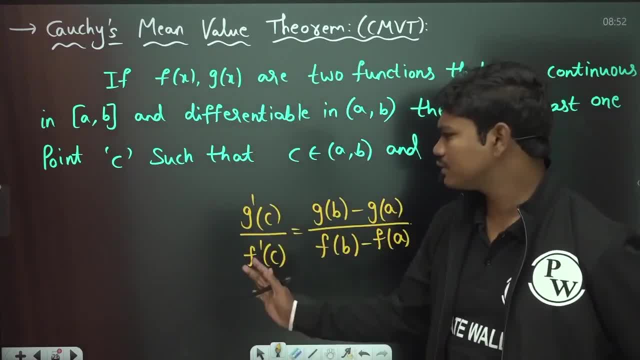 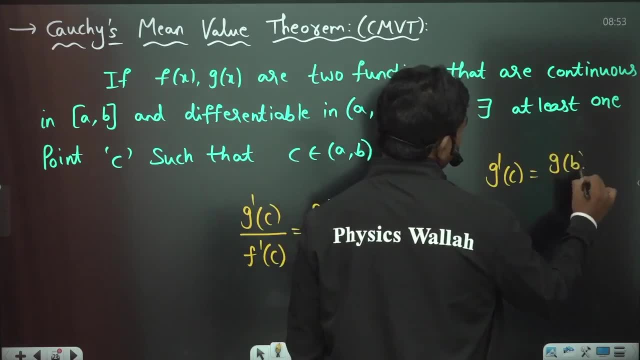 is equal to g of b minus g of a by f of b minus f of a. this is very simple. if you apply lagrangas individually to g of x, you will get this value. g dash of c is equal to g of b minus g of a by. 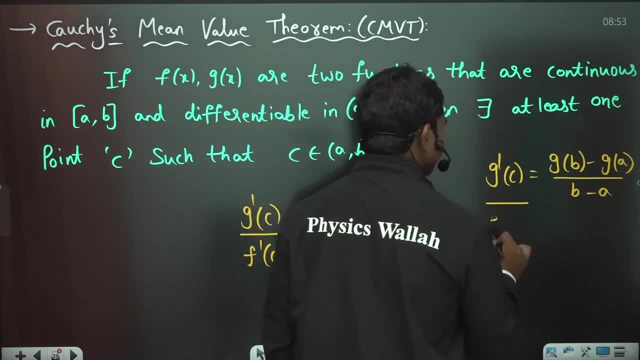 you know b minus a, similarly for f of x. if you apply this, you will get this value f of b minus f of a divided by b minus a. okay, and? and here you will cancel out these two values basically. So that's how you get this result. 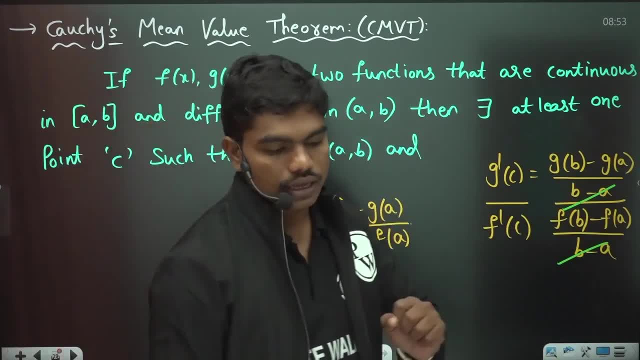 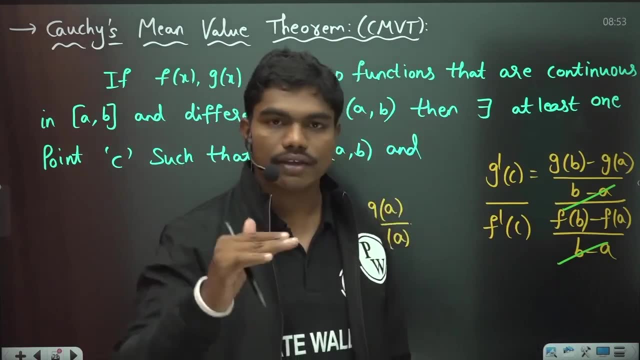 It's basically for cautious minerality, Because many times I'll tell you one thing: It's when you plot a graph, it's not mandatory- that always your horizontal axis takes the value y is equal to x. okay, You can take y is equal to some other function also. 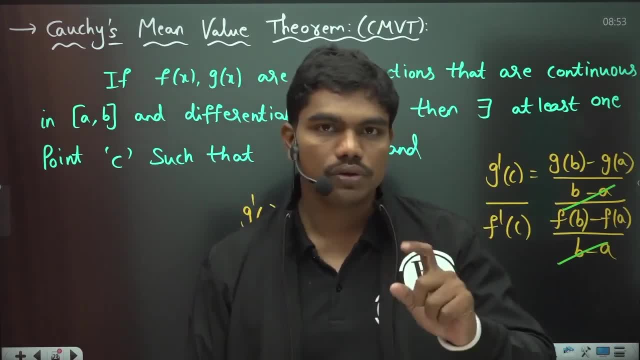 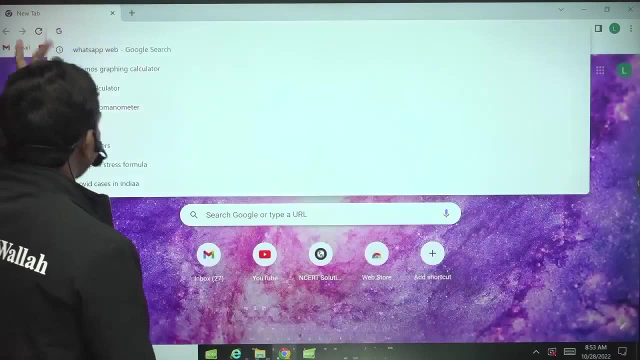 For example, many of you might have drawn this log graphs. Okay, you know, I'll show you. basically, I'll show you with the help of some Google. So so, log x, log graphs, okay, Log graph paper. So, if you see normally, if you see, 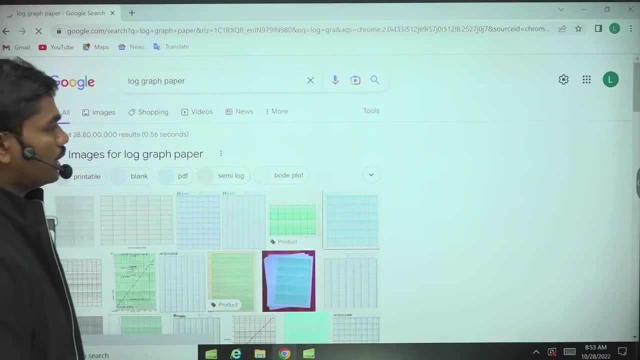 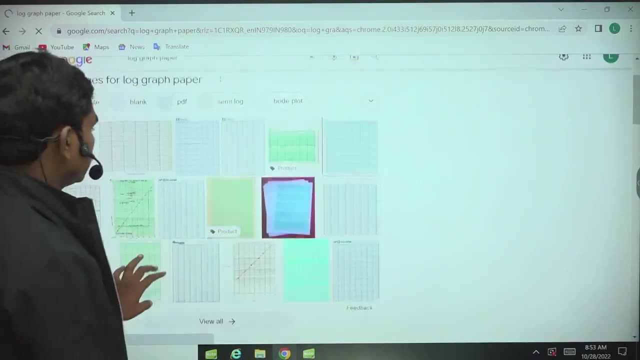 this is how the log graph paper looks like. Okay, here some readings are given, So I'll display this picture better. Okay, I think some internet is slow today, maybe some issue, But right now my intention is to tell you that. 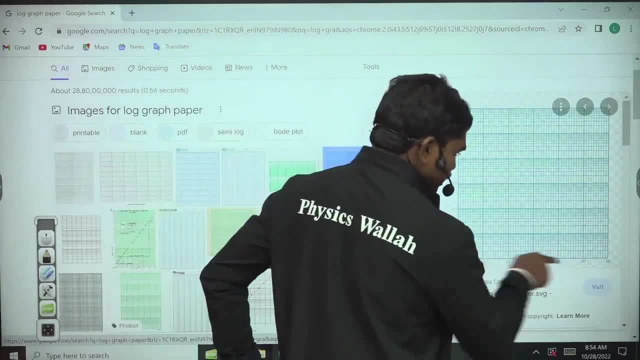 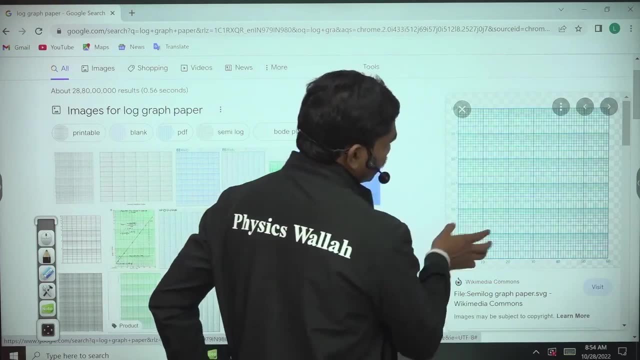 okay, something is opening. So normally when you take this axis, it's need not be x, always okay, It can be some other values also okay. So for example, here you can see, this is 10,. if you take this paper in error's order. 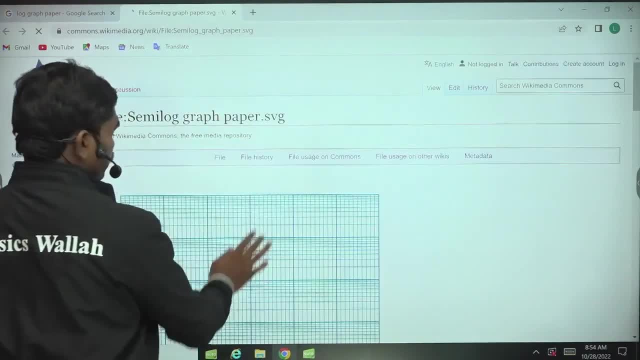 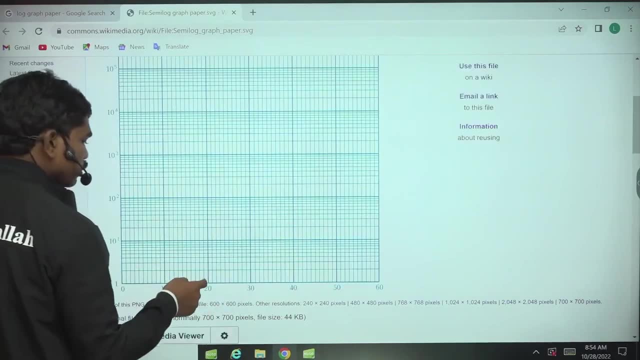 this is 10 power one, 10 power two or this. yeah, here, if you see this y-axis or if you take this x-axis, and it means basically, if you take two axes, the horizontal axis need not be always the x-axis. 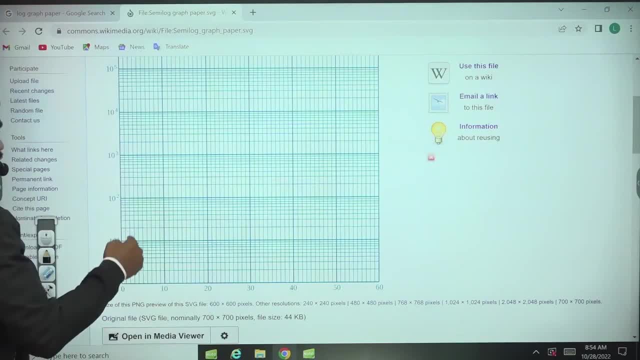 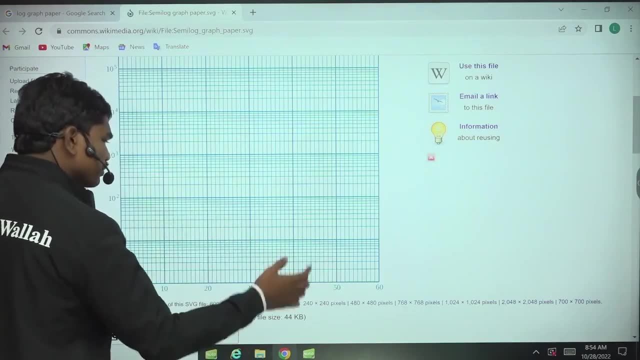 I mean, take the function: y is equal to x. okay, For example in log graph what happened? Here you have the log means the variation is in terms of log. Here you can plot some other parameter, for example voltage or something. 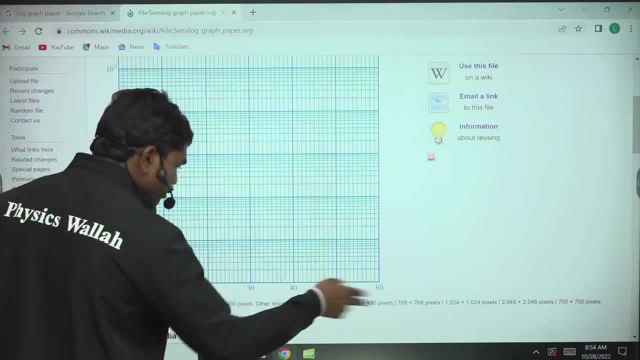 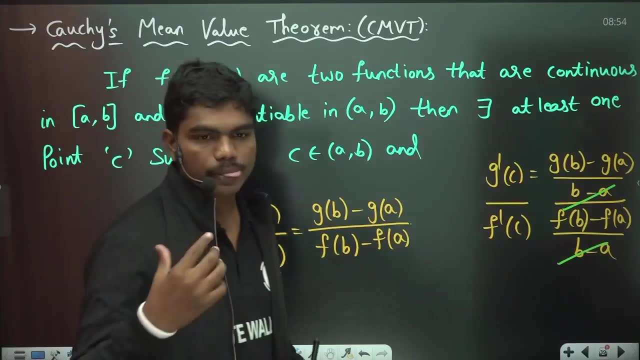 coarseness of grains and all. So, if you see, here you can plot some quantity which is of your interest, and here this scale can be varied according to log. okay, So that's how you need not always plot x and y, f of x. 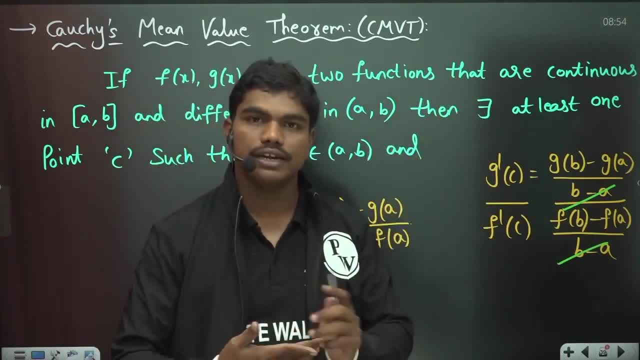 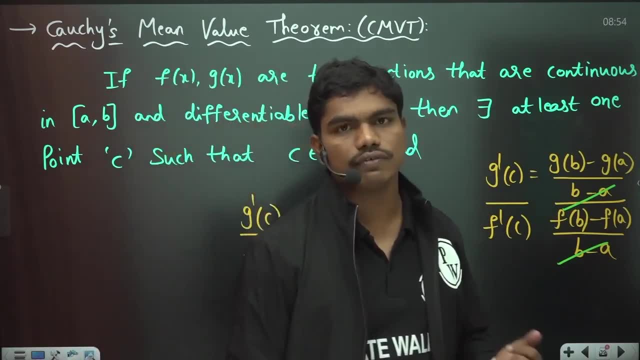 You can plot some f of x and g of x functions simultaneously on a graph in a 2D. okay, So that's how this gorgeous theorem is basically application of this LMVT for two functions. okay. So next let us go for Taylor series. 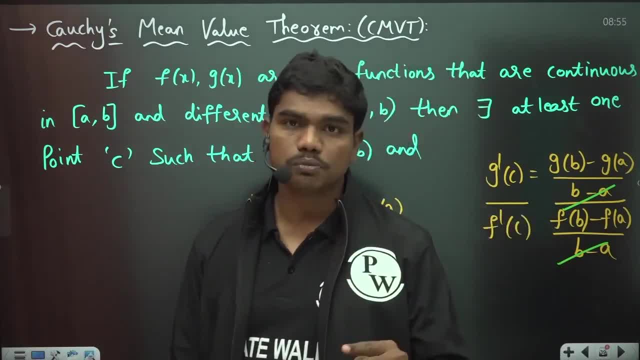 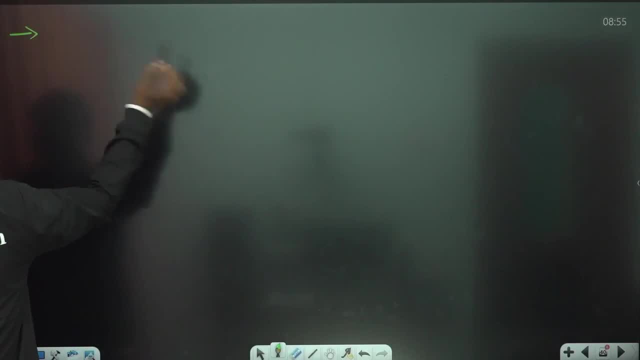 but before going for Taylor series, I would like to give you two very good points actually coming to mean value theorems. What are they? Look, I'll tell you. C. I'll give you one question. You can pause the video and you can solve this. 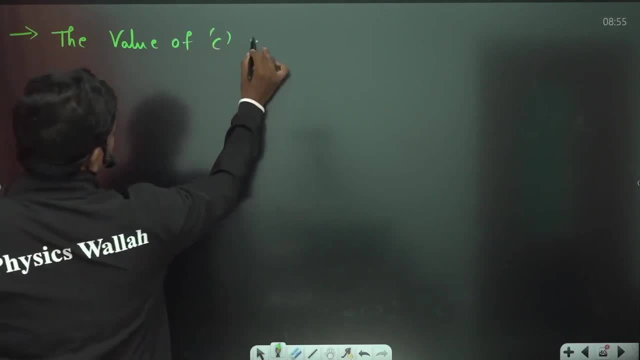 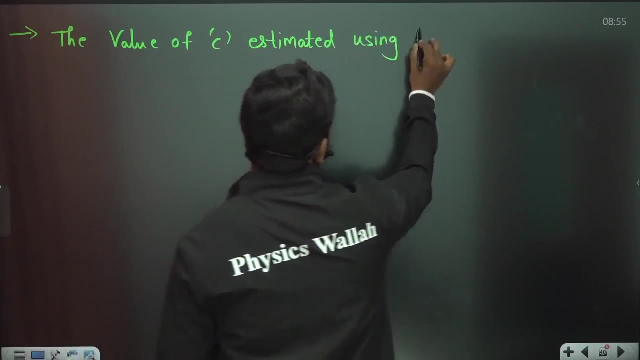 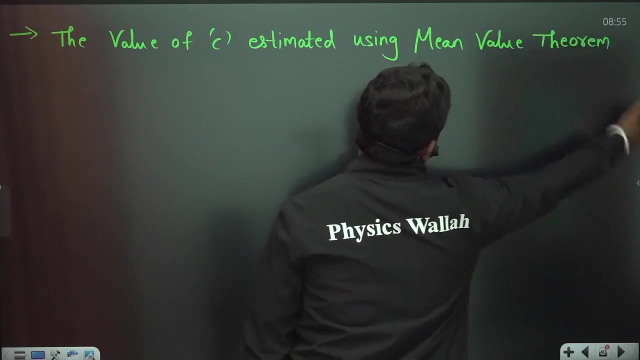 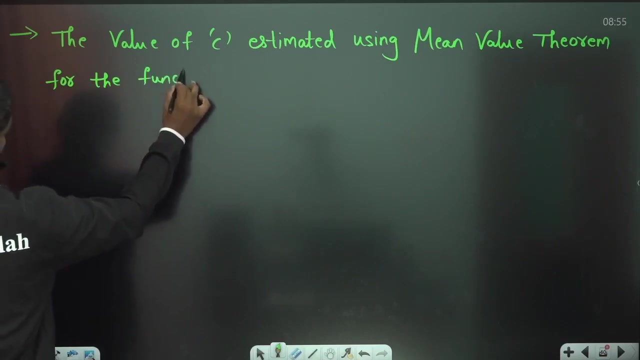 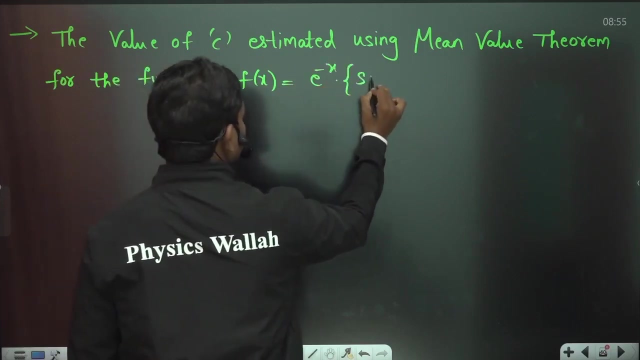 The value of C estimated using mean value theorems. the value of C estimated using mean value theorem for the function. for the function f of x is equal to e power minus x into sin x minus cos x, sin x minus cos x in the interval. 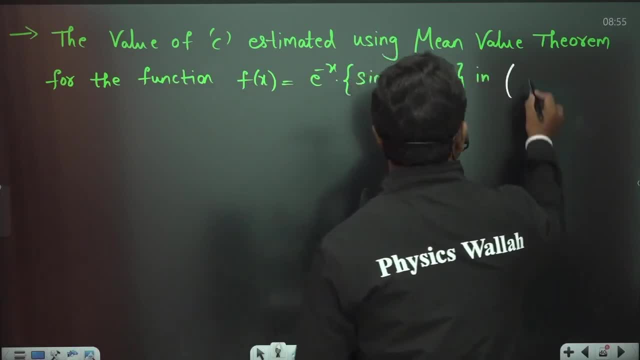 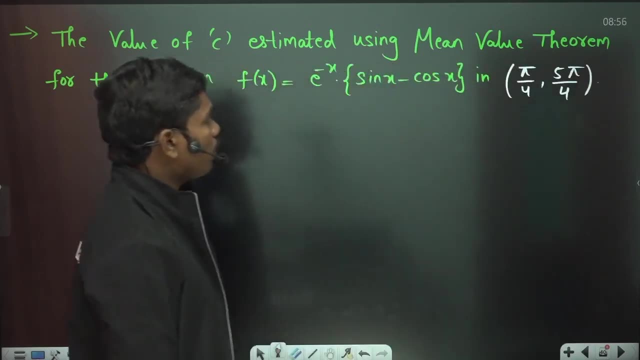 In the interval. say, for example, pi by four, you take pi by four to five: pi by four, you take okay, Five. pi by four, for example, okay. So let us suppose in this interval what is the mean value. 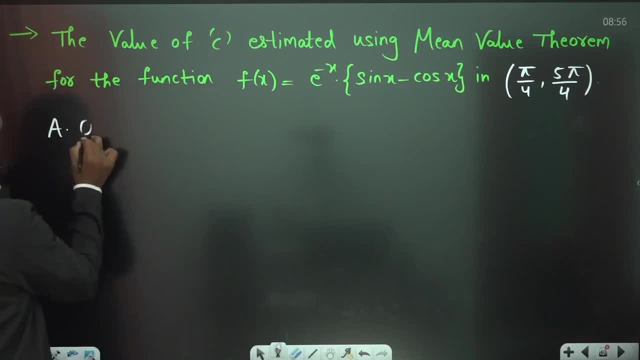 C, calculated using mean value. theorem Options also will give you zero pi by two. pi three pi by two. three pi by two, actually okay. Three pi by two- actually okay. Three pi by two- actually okay. 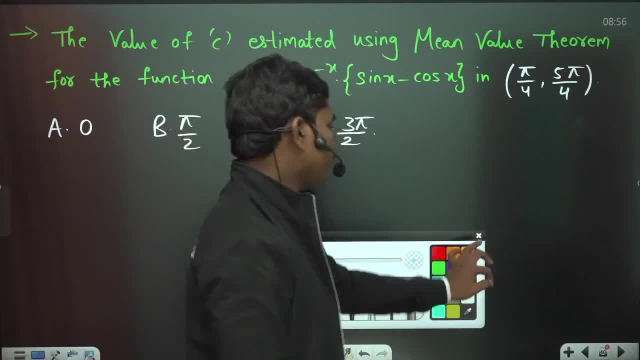 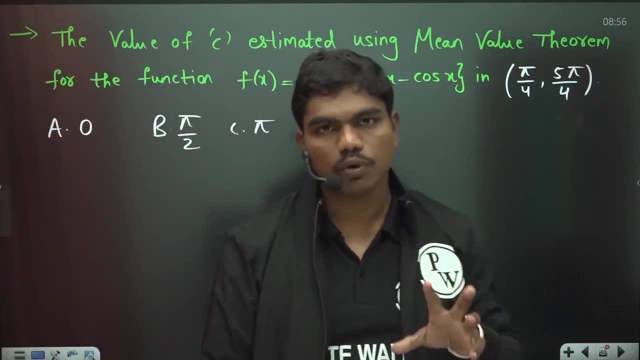 Now, so this is the mean value, So mean value theorem, basically. and they're asking you, what is the value of C? This is one very good question actually. I want to tell you one very cautious point of this mean value theorems with the help of this question. 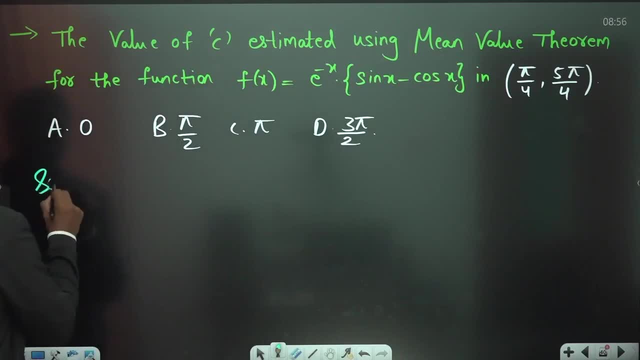 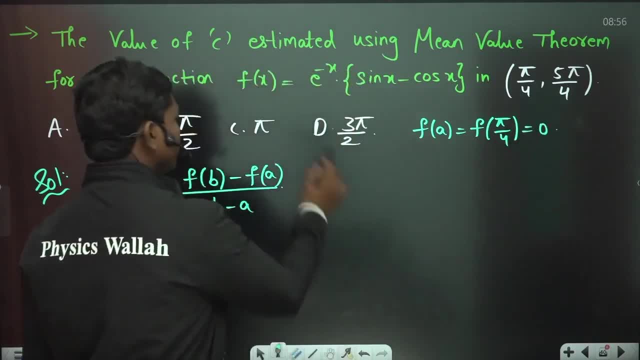 So this value is straightaway zero because of course e power minus pi by four is there, but sine pi by four and cos pi by four are same. So definitely this bracket is going to give you zero. So zero into some value. it is zero. 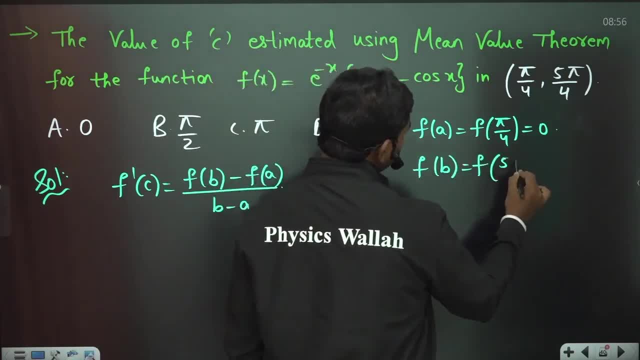 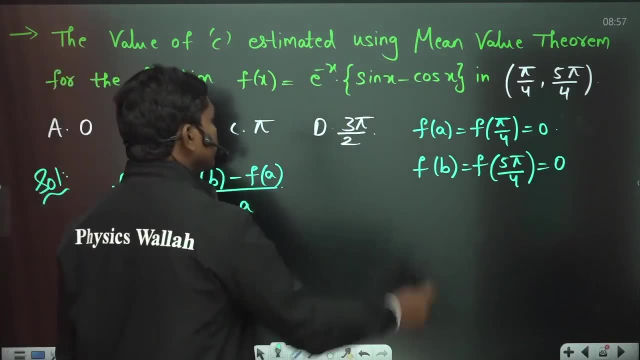 Similarly f of B. if you calculate f of five pi by four, so this value is also going to be zero, because if you check basically again at five pi by four, these two values are same. Both are negatives, of course. 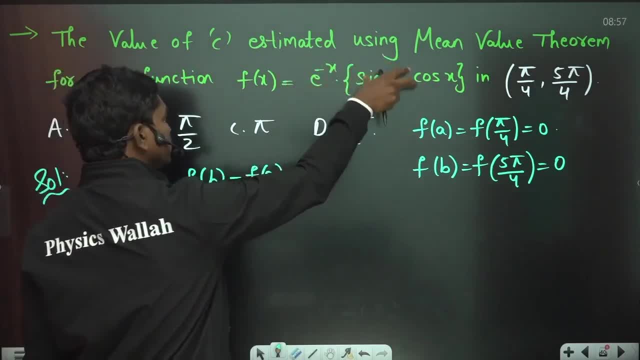 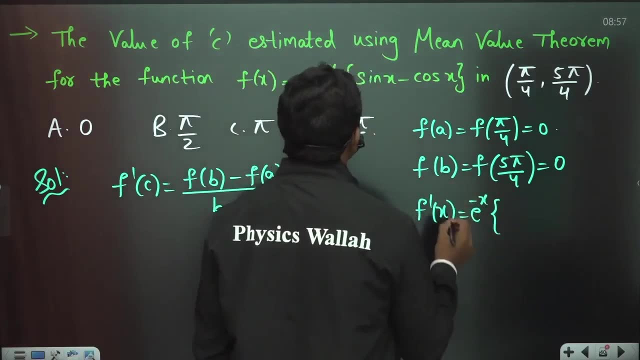 but both these values are same. So e power minus five, pi by four into some quantity is again zero. So what is f dash of x if you calculate first function into derivative of second function? So differentiation of sine x is cos x minus, differentiation of cos x is minus sine x. 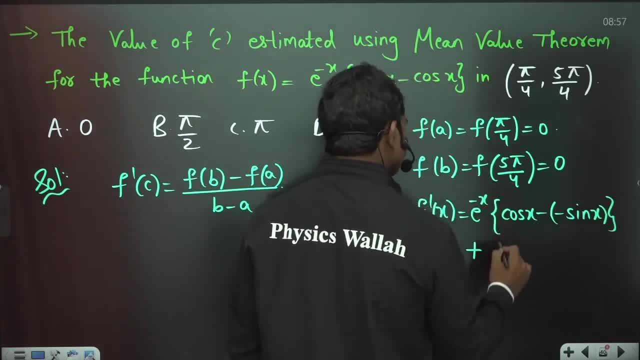 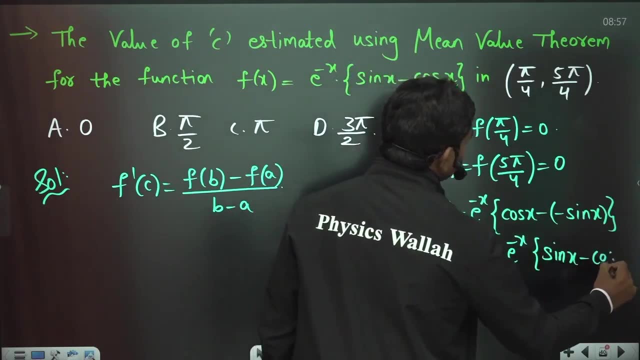 So this is the case plus differentiation of first function, so minus e power minus x, into second function, which is sine x minus cos x. So if you simplify this, if you simplify this, e power minus x, if you take out, then cos x plus sine x. 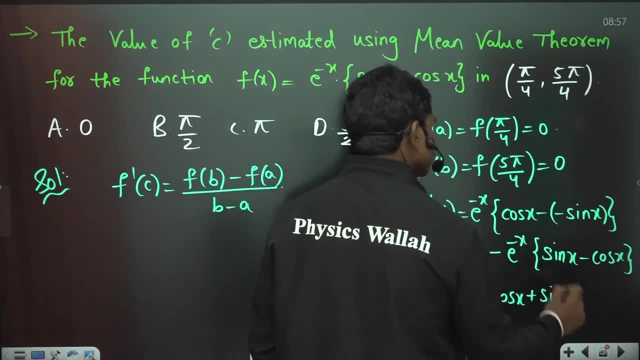 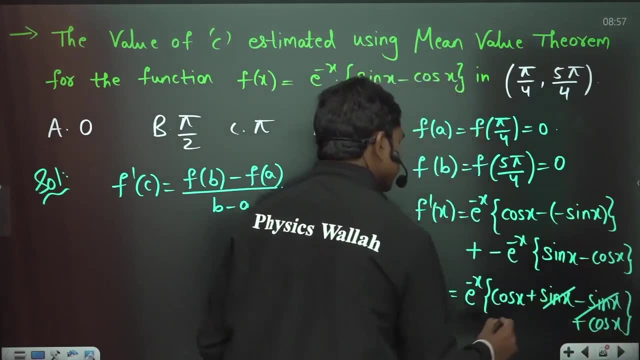 then minus of sine x gives you minus sine x, and minus of minus gives you plus cos x. So this is what you have, this sine x, and sine x gets canceled. So two times of e power minus x into cos x is what you will get here, correct? 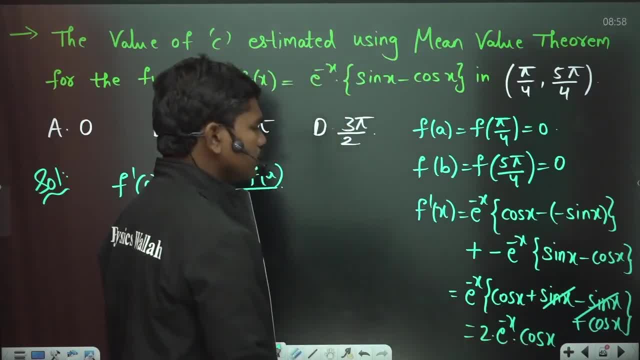 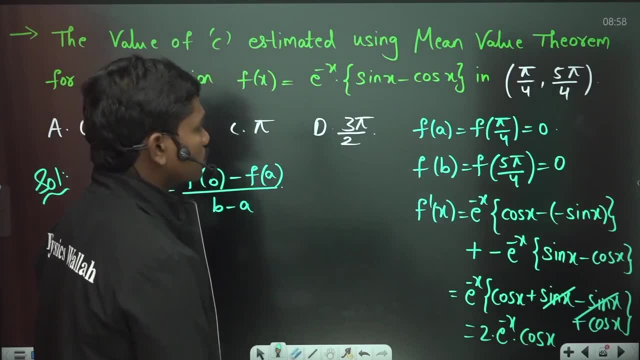 Or did I, you know, do some mistake here? So this is sine x, so e power minus x into e power minus x, into sine x minus cos x. and yeah, I think it is fine, correct, Or else is there some mistake here. 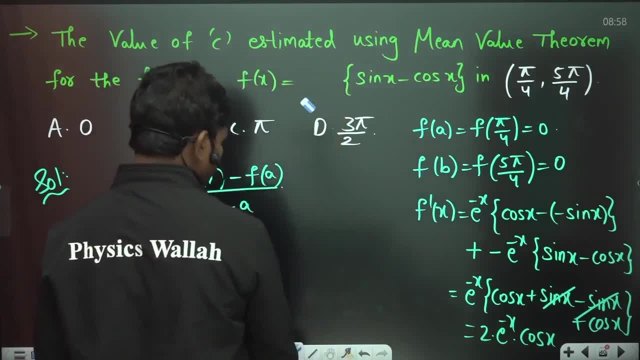 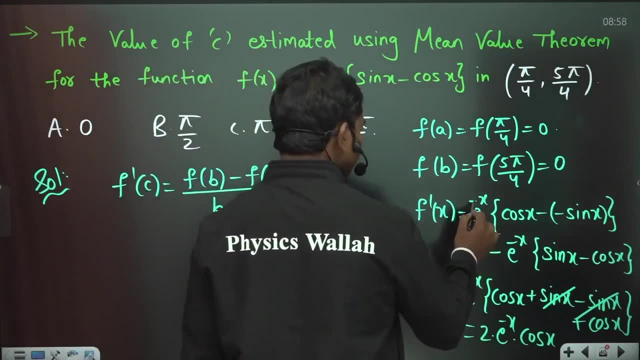 We'll do one thing: we'll take the function as e power x, because I have to show some result here, some important thing: e power x into sine x minus cos x. So this differentiation will be e power x. here also it is e power x. 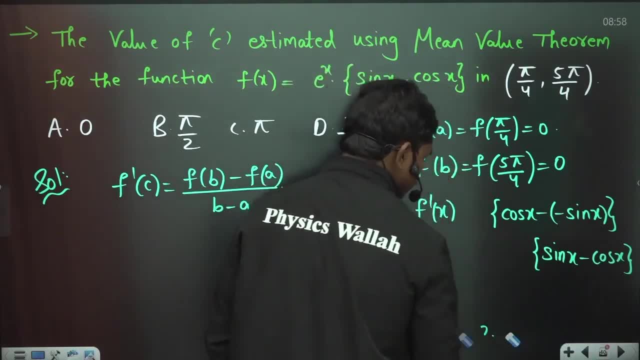 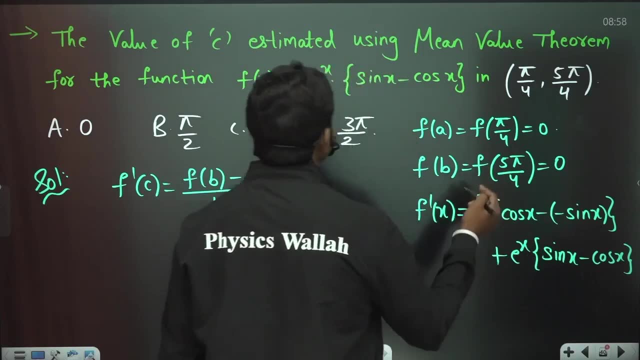 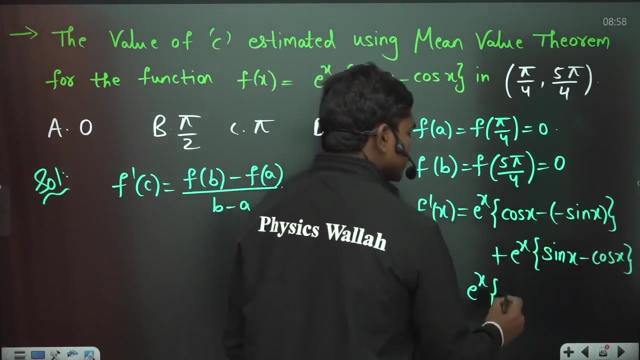 So this result changes slightly. So see, here we'll see e power x plus e power x into sine x minus cos x. So if you take e power x common, you have cos x plus sine x plus sine x minus cos x. then cos x, cos x gets canceled, you have two sine x. okay. 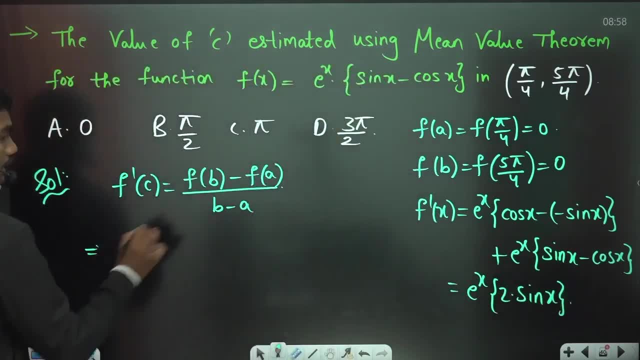 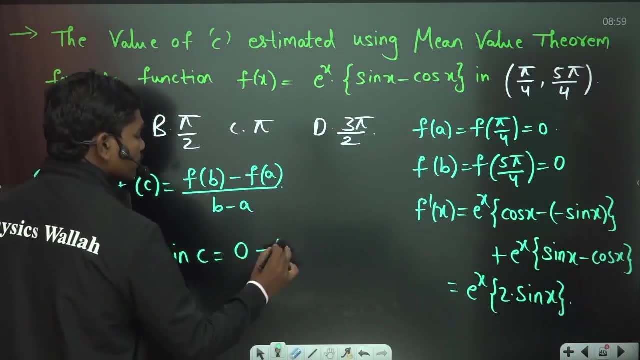 So this is the function. So what is f dash of c? f dash of c is equal to two times of e power, c into sine c is equal to f of b, zero minus f of a, zero by pi, because pi pi by four minus pi by four, anyhow this is zero. 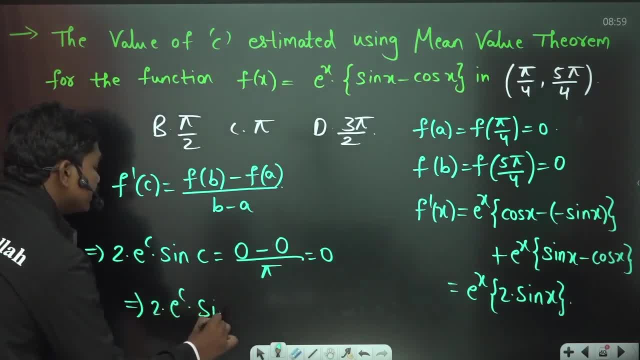 So you know, two times of e power c into sine c is equal to zero. But you know one thing: this e power c cannot be zero for some finite values of c. So c is not infinity, c is some finite value here. 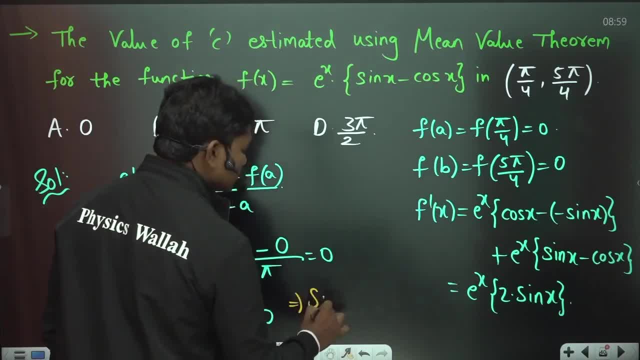 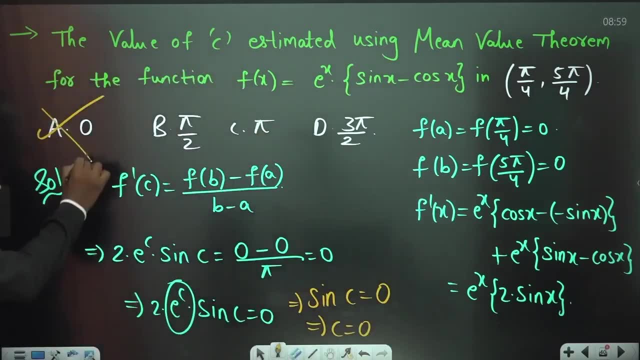 So definitely, you know you have to get this equation: sine c is equal to zero. So as soon as you see this equation, you let c is equal to zero and take the first option. But actually this is wrong, because I told you. 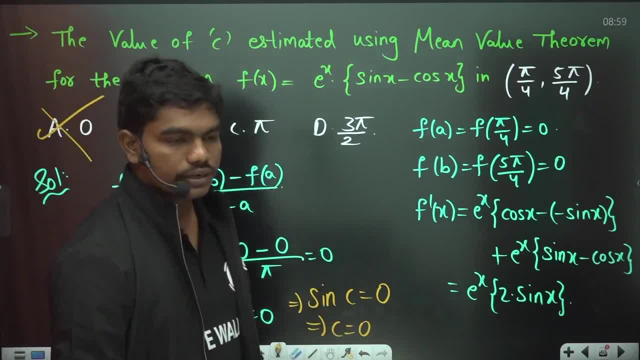 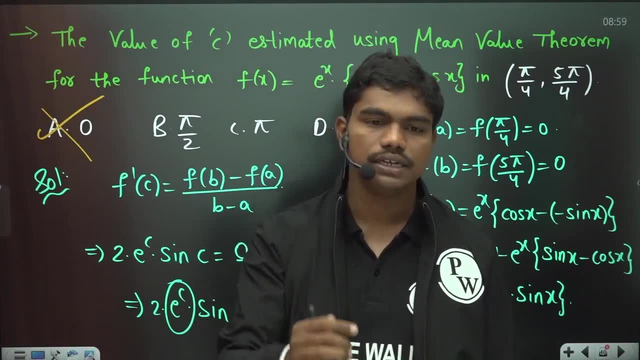 along with the satisfying of this equation, there is one very important criteria: that c should also lie in between a and b, correct? If you generally miss this condition, not only you. you means to me, I'm not personally the one who is watching this- 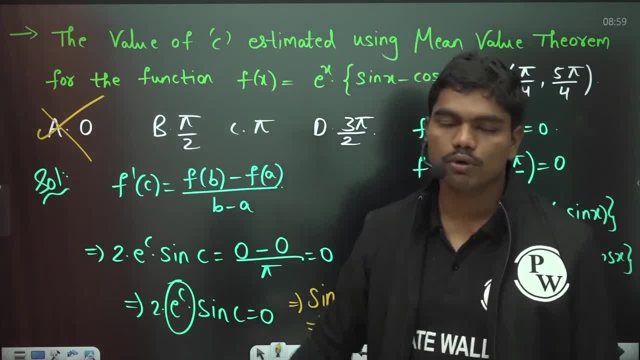 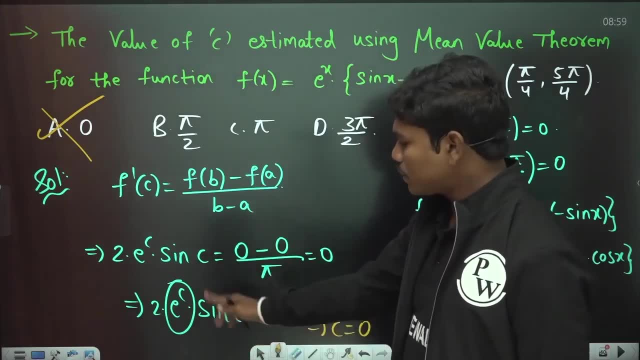 but in general, if you see people miss this, you know a point: that c should lie in between a and b. actually, okay, So that's the reason why, without focusing much on that, they directly equate this: sine c is equal to zero. 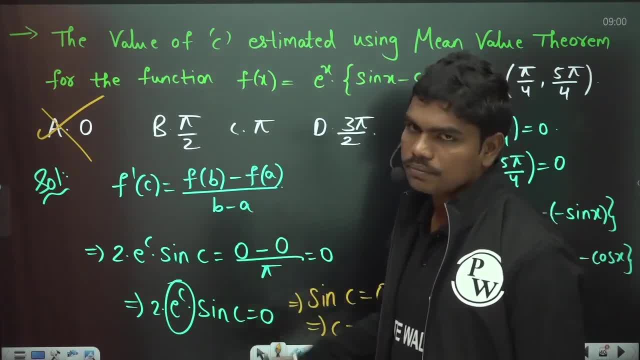 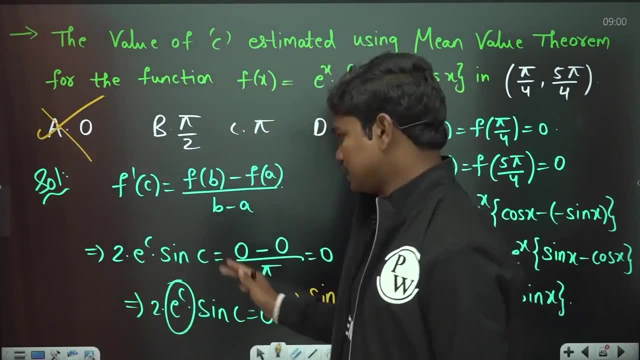 they directly equate: sine: c is equal to zero, and they, you know, basically write this: c is equal to zero, but which is a wrong option. That's why it's given in gate and also in many PSUs. okay, So this is one important point. 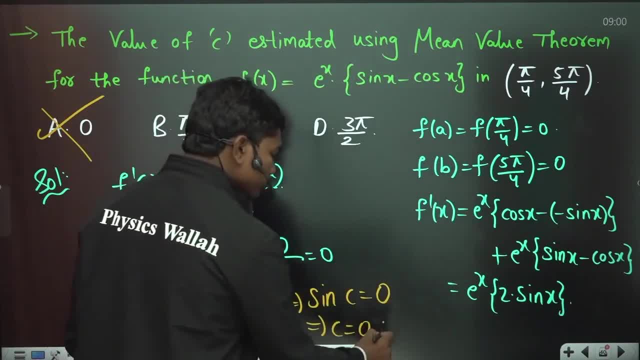 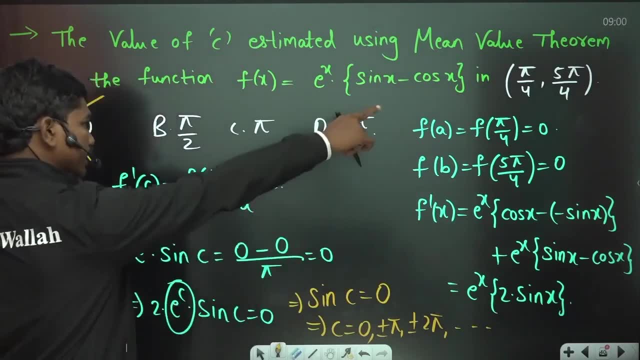 So c, then sine c, equal to zero, plus or minus pi, plus or minus two pi, all these values. But out of all these values, the value which lies in that interval is pi. actually, okay, So pi is the correct answer. 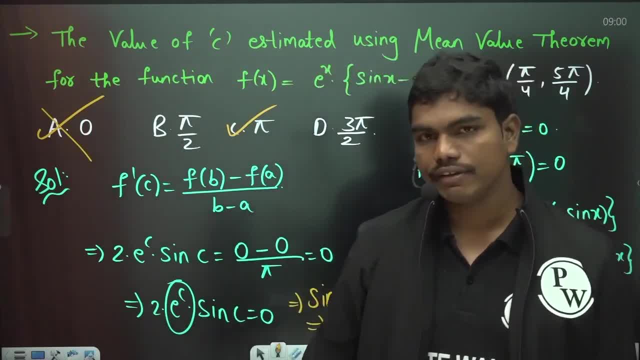 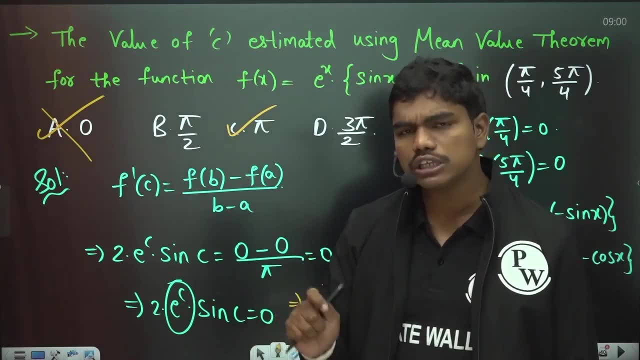 but a is means basically zero is the wrong answer. Why I've given you this example is because you should always keep in mind that, along with satisfying this derivative condition, it should also satisfy that c lies in a comma, b clear. So that's why it's very important, okay. 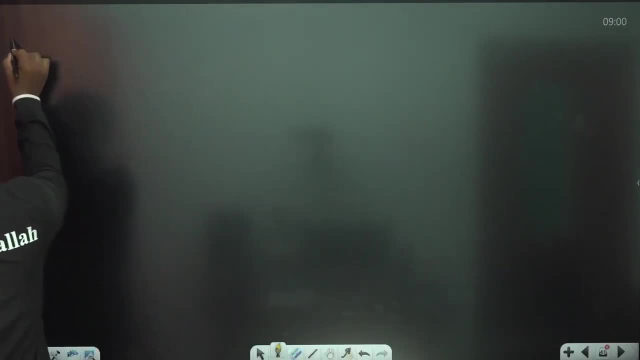 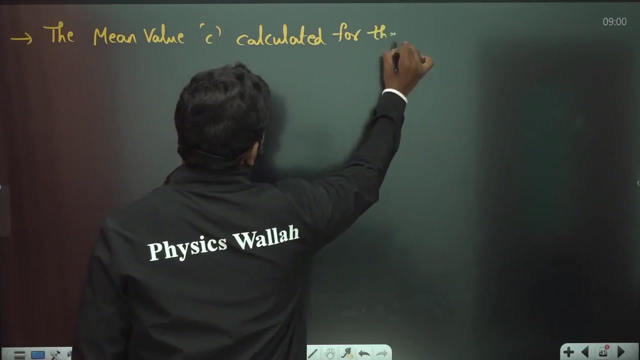 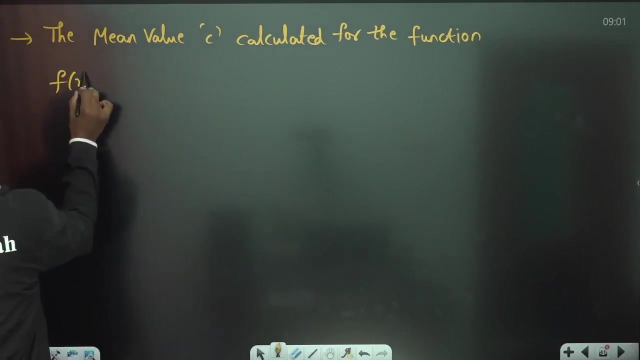 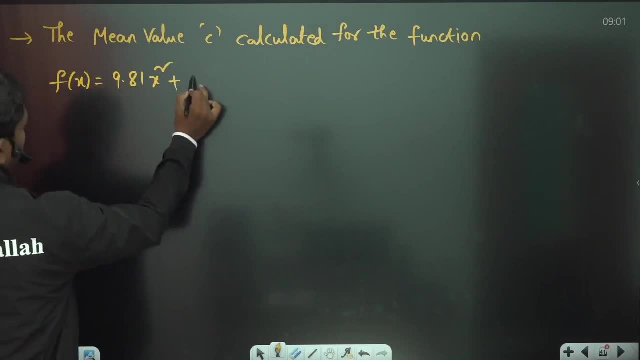 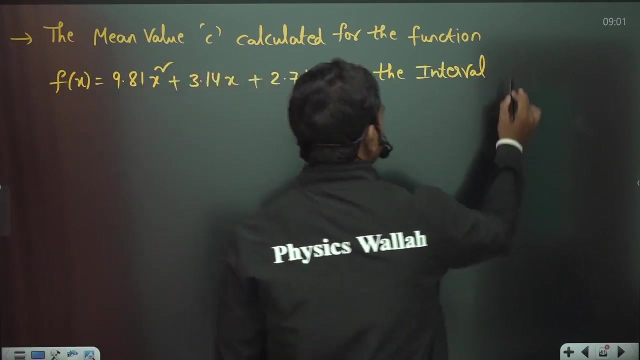 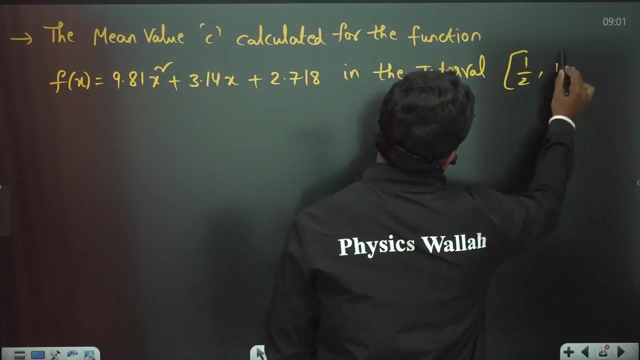 some 9.81 x square, plus some 3.14 x plus some 2.78.. 1, 8, let us say. let us suppose they have given this function in the interval, in the interval, in the interval 1 by 2 comma, in the interval 1 by 2 comma 1, let us say they: 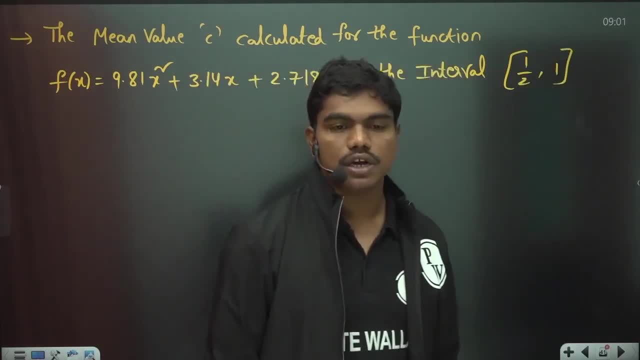 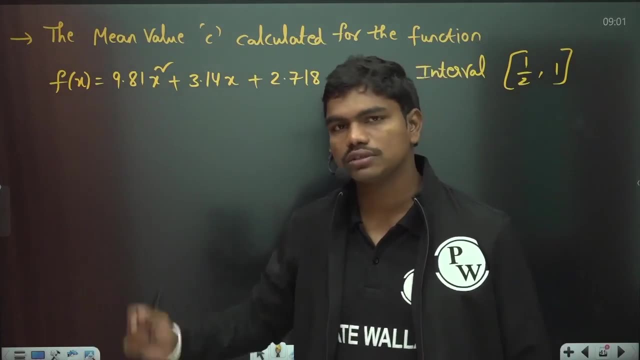 have given you this function then it's obvious you by now you might have understood to calculate c value. it is quite, you know, time taking because the constants are 9.81 and all- and x value also, some fractions are there, okay. so 1 by 2 all these things. so if you calculate the mean value, 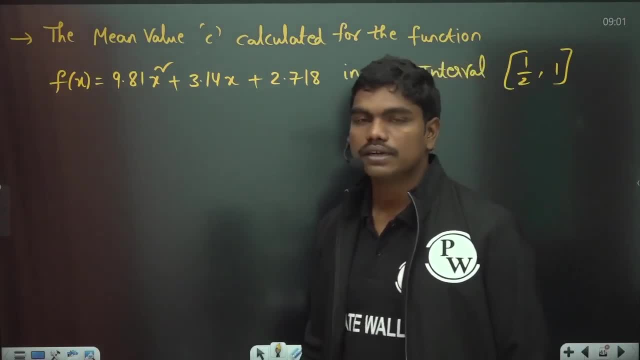 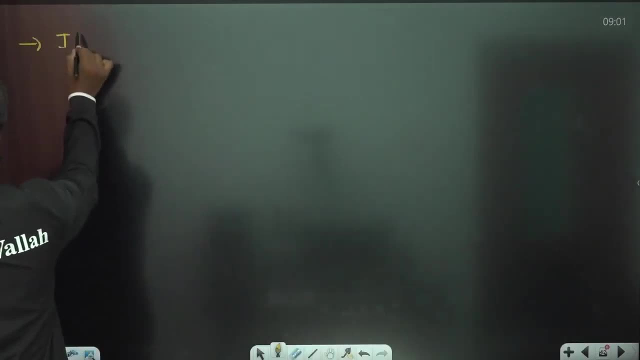 theorem using this normal procedure. you will definitely take some time, but there is a technique for quadratic functions. okay, look what is that technique. i'll tell you. if f of x is a x square plus b, x plus some constant c, for example a x square plus b, x plus c, then the mean value in 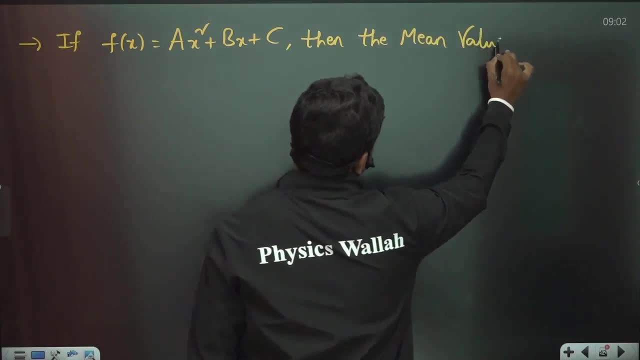 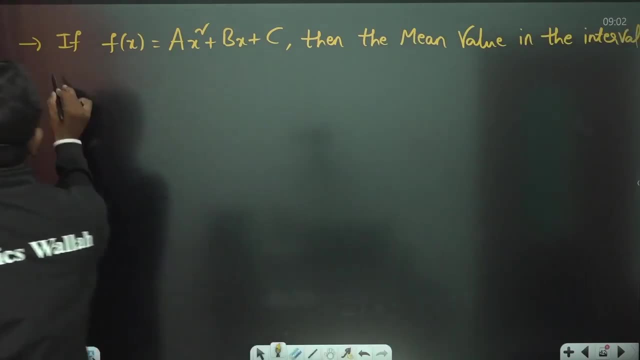 the interval, then the mean value in the interval, then the mean value in the interval. a, comma, b is just a plus b by 2, direct. okay, straight away, it's average of the interval and it doesn't depend upon this. coefficients: capital a, capital by capital c. how this is happening, look, i'll tell you. so as per mean value theorems you can see f. 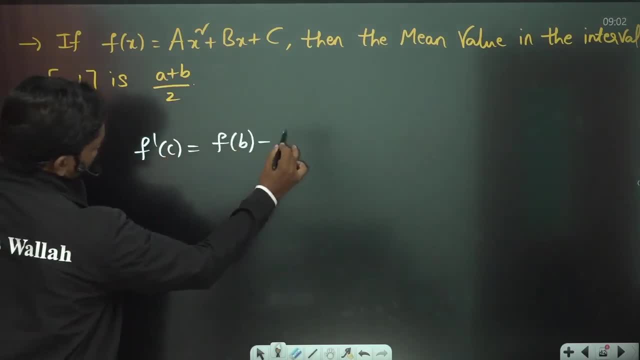 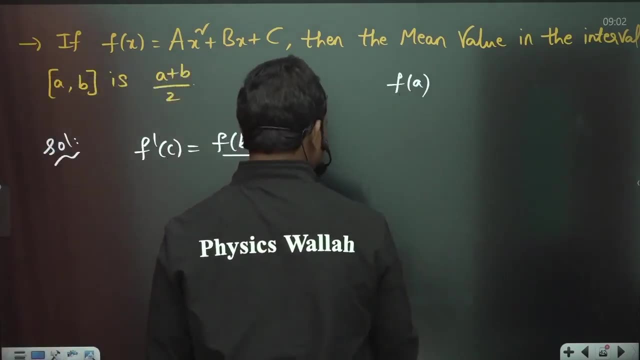 dash of c is equal to f of b minus f of a, divided by b minus a. so what is f of a? f of a is equal to or f of b. let us start with f of b. this is a b square plus capital, b times of b plus c. and what is f? 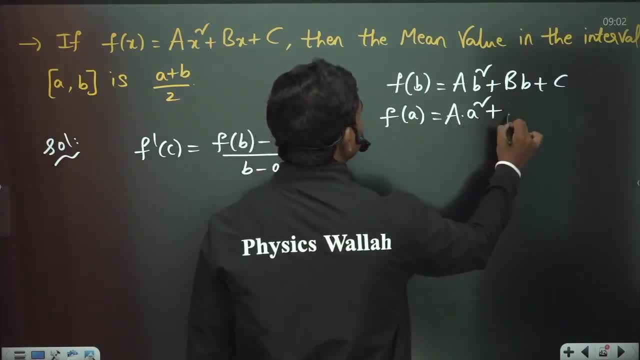 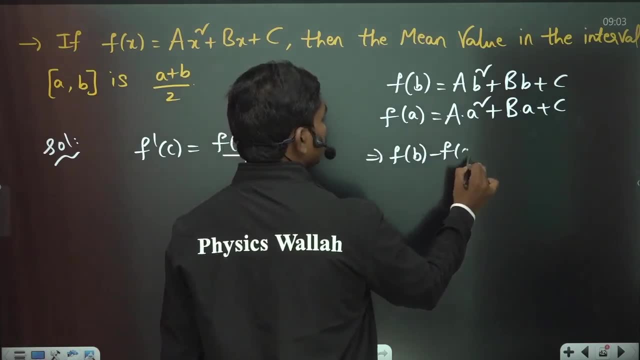 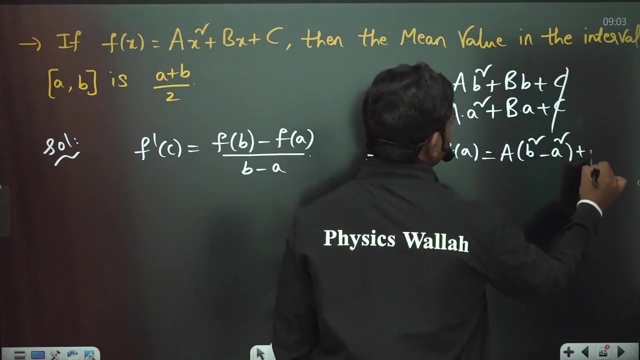 of a capital a into a square plus b, into this small a, glassy. so if you subtract these two things, your fob minus f of a is equal to this. c gets canceled of course. so capital area times of b square minus a. square plus capital b. times of b minus a. okay, so this is what you have. 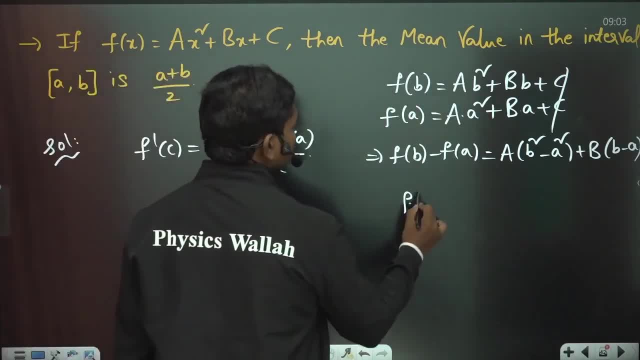 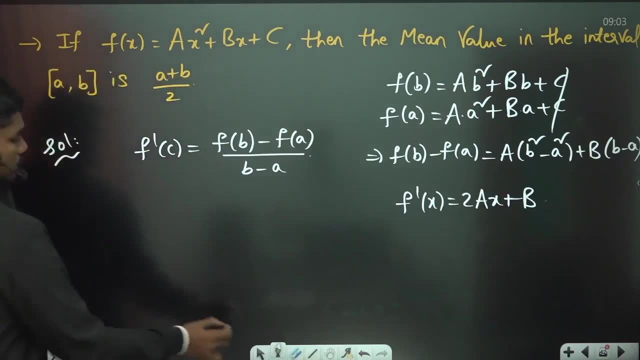 so, divided by b minus a, and what is f dash of x? f dash of x is equal to 2ax plus b. is what you have. okay, now let us substitute. let us call this value zeta, for example, because you'll confuse between the c and capital c. so zeta, for example, so 2 times of capital a, zeta plus b, this is equal to f of b. 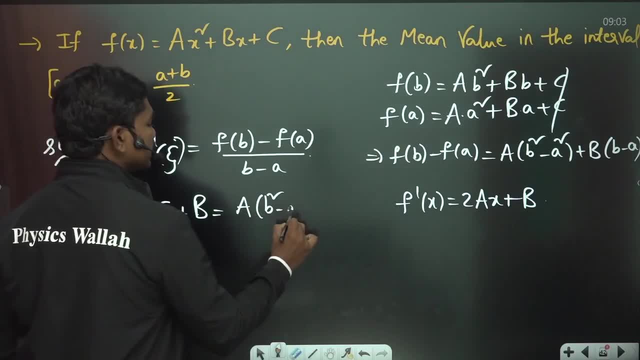 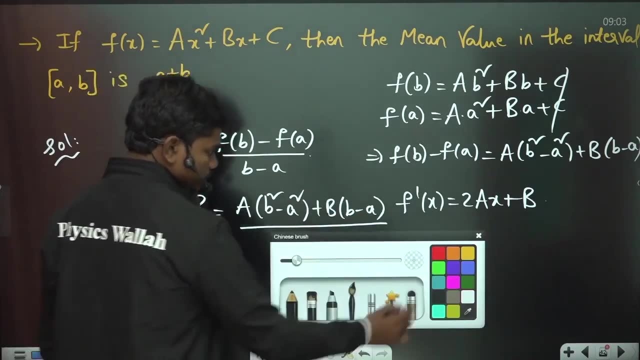 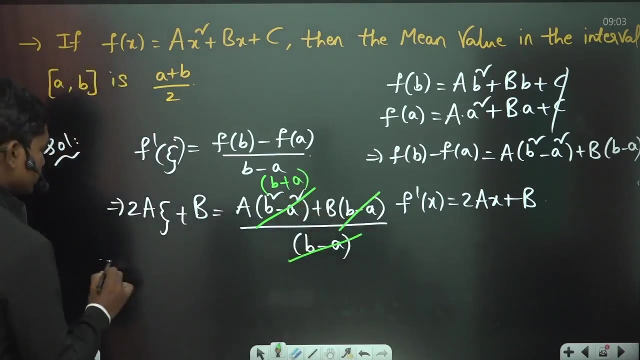 minus f of a, is this value a into b square minus a. square plus b into b minus a, this value divided by b minus a. so you can see this cancels this b plus a times and also it cancels out this term. okay, so that's why, if you see 2a, zeta, where zeta is the mean value plus b, is equal to capital a. 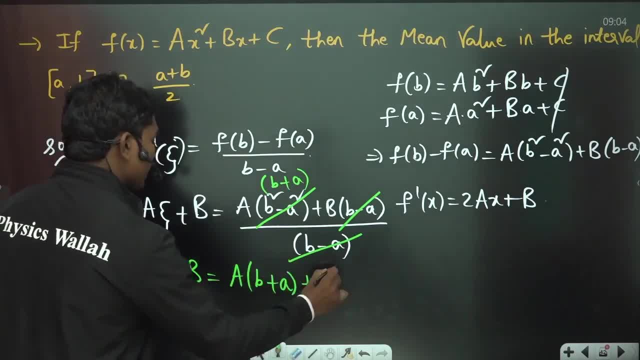 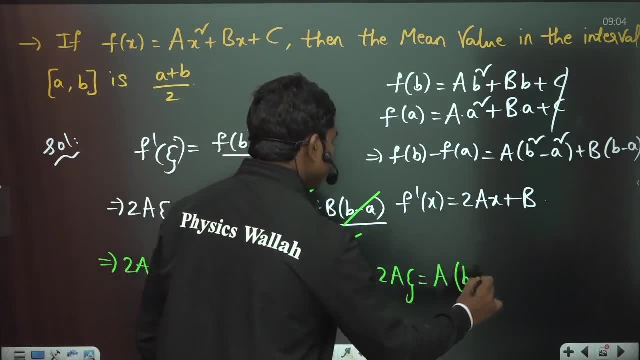 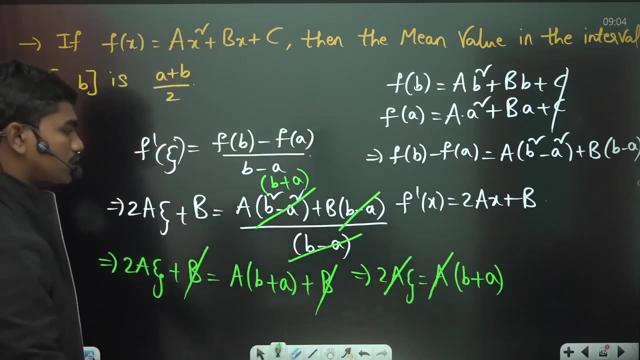 times of b plus a plus capital b. so capital b and capital b gets cancelled. so this implies 2a zeta is equal to a times of b plus a, and i am cancelling this capital a. capital a is not equal to 0, because if capital a is equal to 0, this equation is no more quadratic. okay, so it's just. 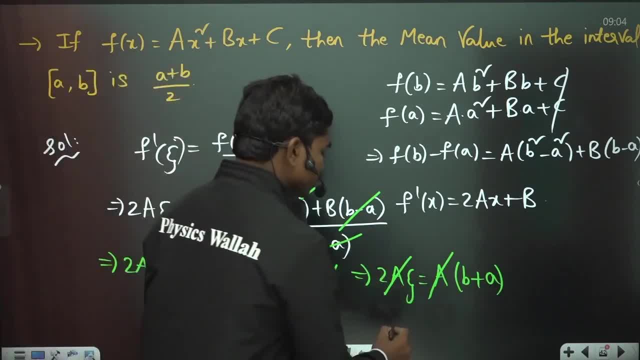 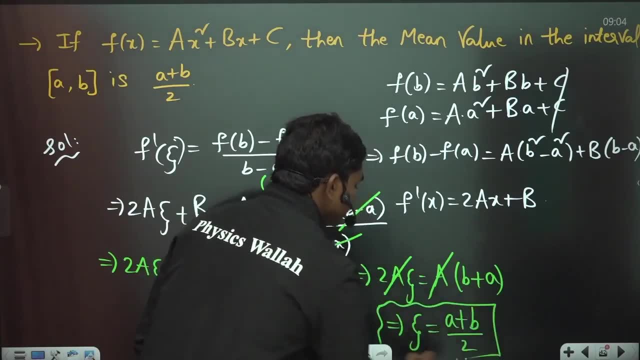 a linear equation. so that's why we are not taking capital a to be z. so, zeta, the mean value is nothing but small a plus small b divided by 2. actually here, okay. so if you see, this mean value is not depending on capital a, capital b, capital c. okay, so it doesn't depend upon the coefficients of the 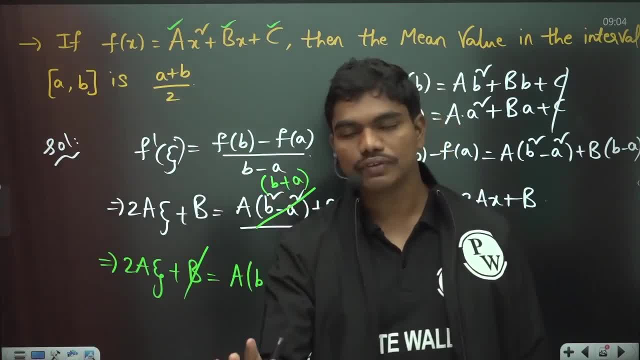 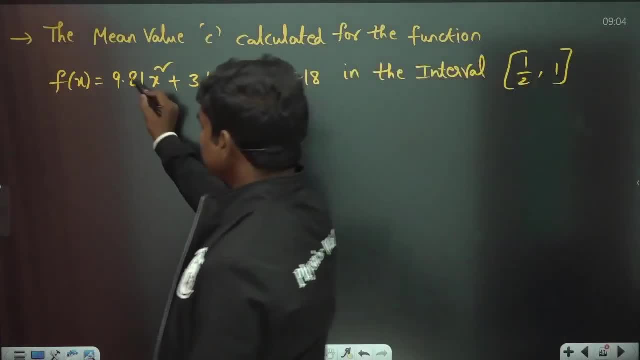 interval values. okay, so once you get the interval values, you just need to take the average of the interval values and that is nothing but the mean value c for this quadratic function. so now, if you come back to this example, intentionally i have given you these coefficients because once or twice, 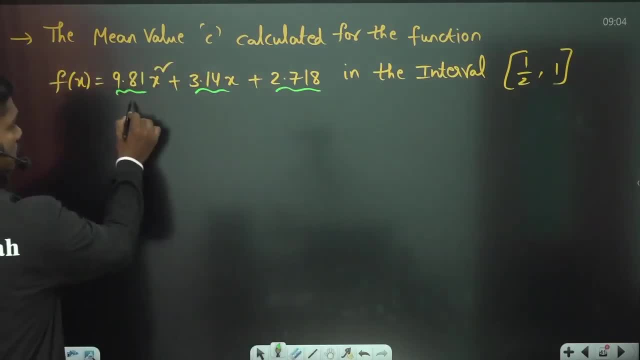 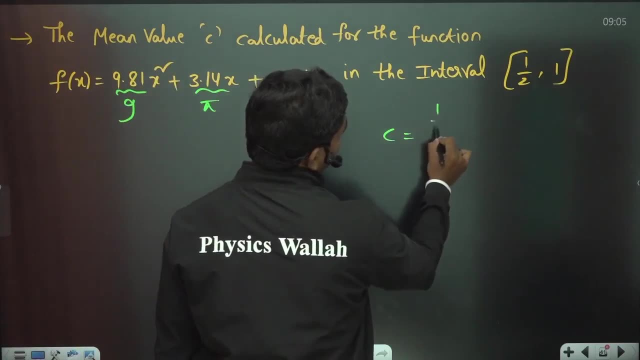 they have done this in examination. so 9.81 is acceleration due to gravity, this is pi, this is e. that's how i framed this question. so basically, if you see, if you calculate mean value directly, this is nothing but 3 by 4. that's it okay. so you need not do the calculations like. 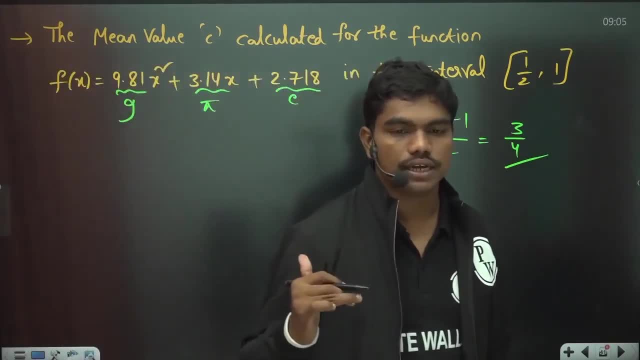 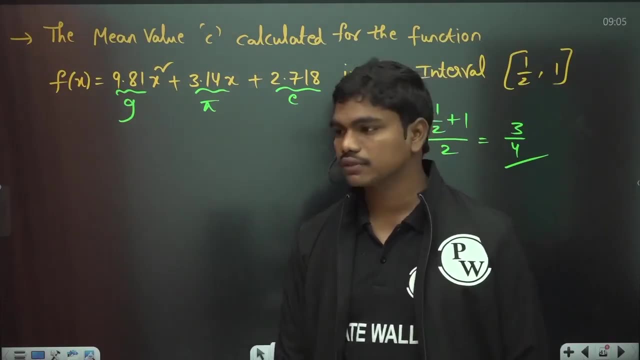 9.81 into 1.2, whole square, nothing. okay, so this is the thing for the quadratic functions. okay, so that's why i have given you, uh, this example. so with this we close. this mean value theorems. and next let us quickly move on to taylor series. okay, so let us see the taylor series, which is one again. 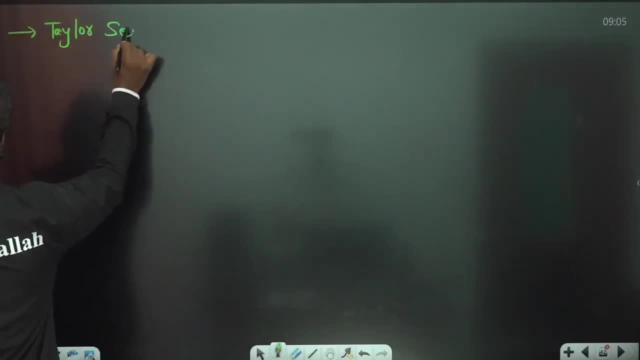 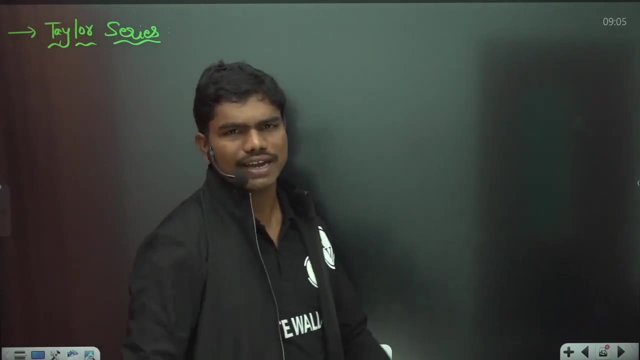 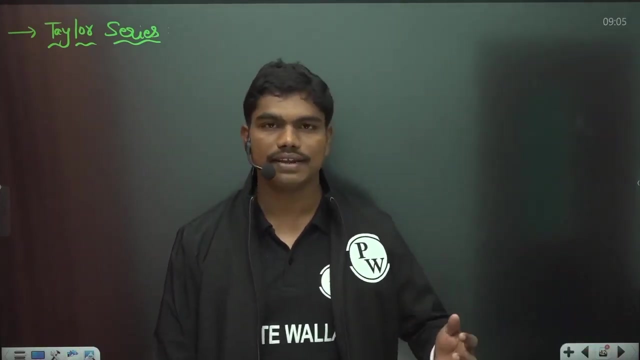 one of the very important- uh, you know- module taylor series. of course, in this video we will do one thing in because this video, calculus, is a vast module. in this video we will cover single variable. we will do some other video means the next video. we will do one multi-variable calculus. 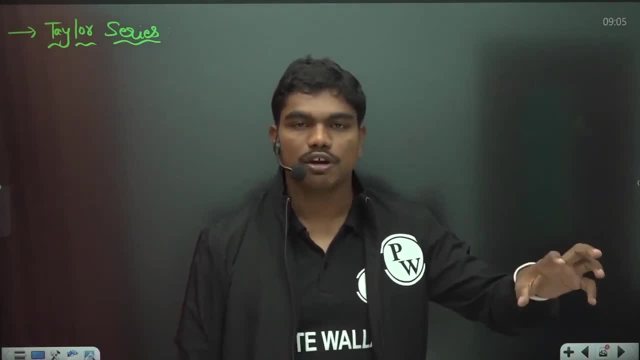 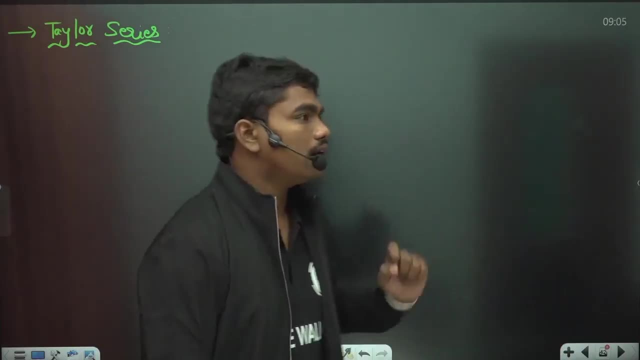 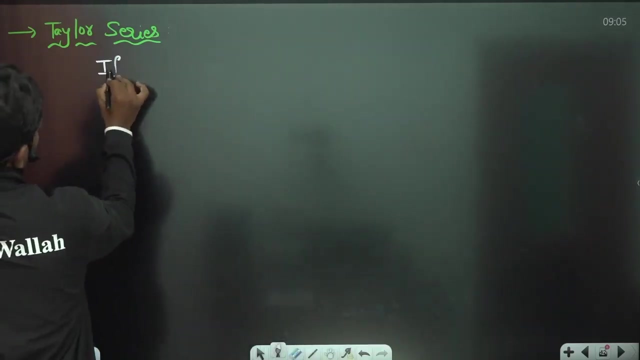 okay, so they will see multiple integrals. uh, you know concept of maximum of two or more variables. we will see there. okay, so in this video let us restrict ourselves to single variable calculus. okay, now let us see here. taylor says: so what is this? taylor says: if a function, if a function f of x. 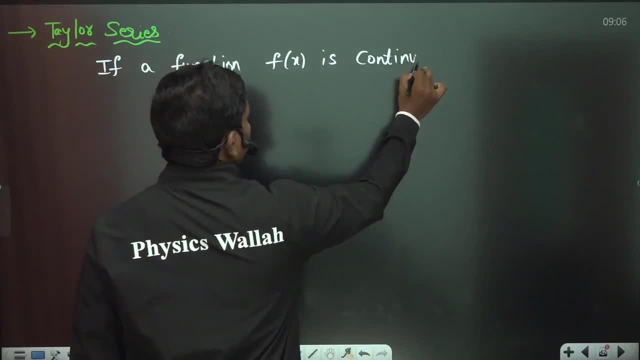 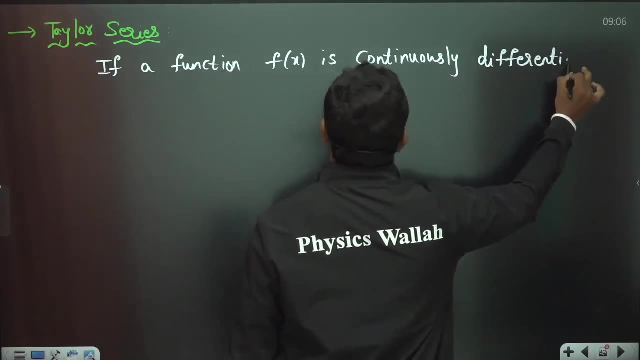 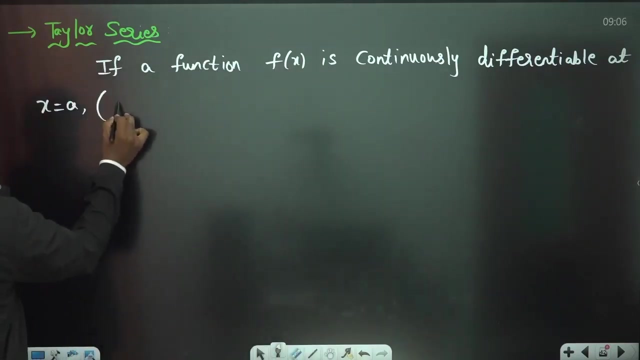 is continuously differentiable is continuously differentiable. differentiable at x is equal to a, at x is equal to a, for example, means: what is the meaning of that? f dash of a, f, double dash of a, f, triple dash of a and so on? all the exist and so on exist then. 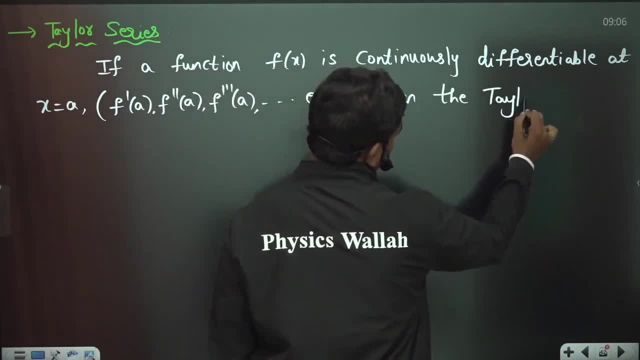 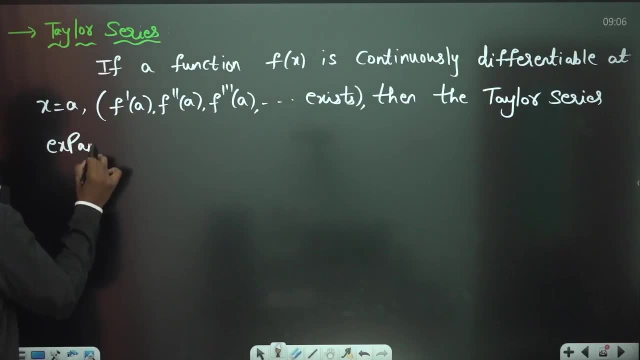 the taylor sees expansion, and then the taylor sees expansion. then the taylor sees expansion of f of x. then the taylor sees expansion of f of x. about x is equal to a. about x is equal to a. is given by: about x is equal to a. is given by this function that f of x is equal to. 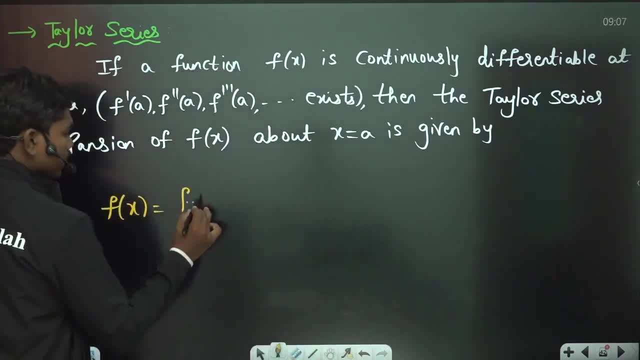 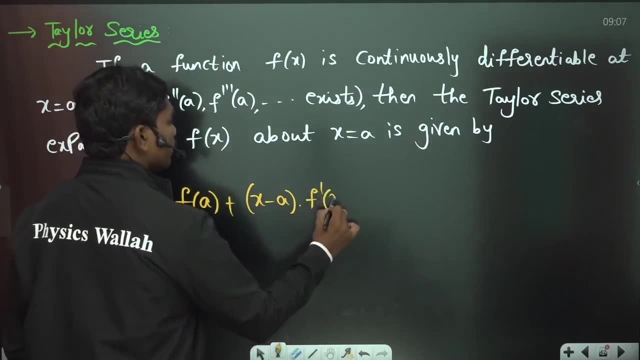 f of x is equal to f of x is equal to f of a plus x minus a. into f of a plus x minus a. into f of a plus x minus a into f. dash of a by one factorial f. dash of a by one factorial f. dash of a by one factorial plus x minus a whole, square into f double dash. 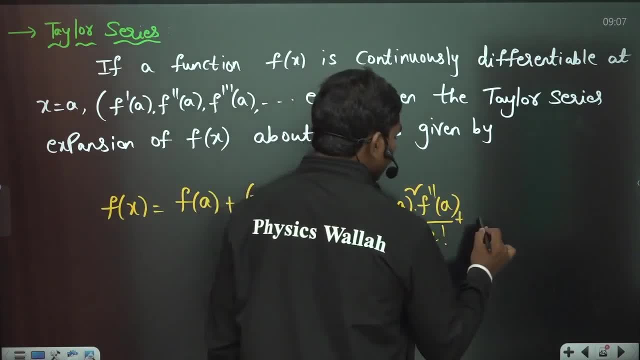 plus x minus a whole square into f. double dash plus x minus a whole square into f. double dash of a by two factorial plus, and so on. of a by two factorial plus, and so on. of a by two factorial plus, and so on. x minus a whole power n into nth derivative. 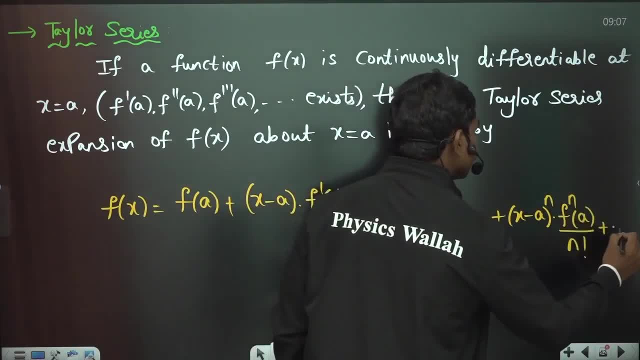 x minus a whole power n into nth derivative. x minus a whole power n into nth derivative of f at a by n factorial plus, and so on. of f at a by n factorial plus, and so on, of f at a by n factorial plus, and so on: infinity, basically. okay, this is a. 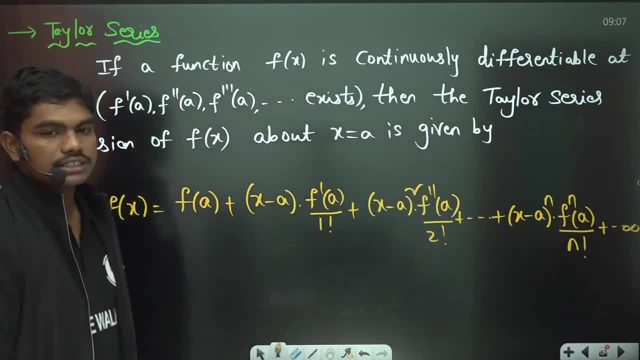 infinity, basically okay, this is a infinity, basically okay. this is a infinitely extending series. so if you see infinitely extending series, so if you see infinitely extending series, so if you see this is how the taylor sees expansion is. this is how the taylor sees expansion is. 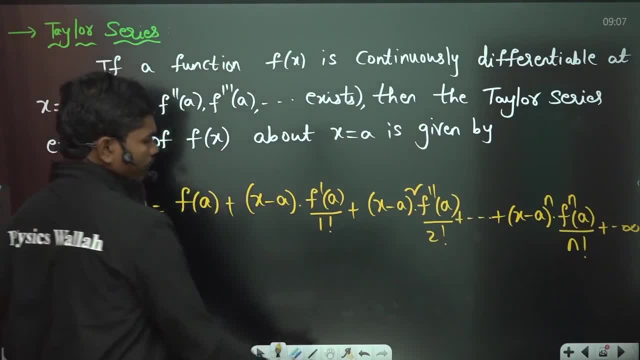 this is how the taylor sees: expansion is given, of course, in single variables, okay. given, of course, in single variables, okay, given of course, in single variables, okay. so now, if you see whenever i'm writing f, so now, if you see whenever i'm writing f, so now, if you see whenever i'm writing f, dash of a, that means, i'm assuming x is. 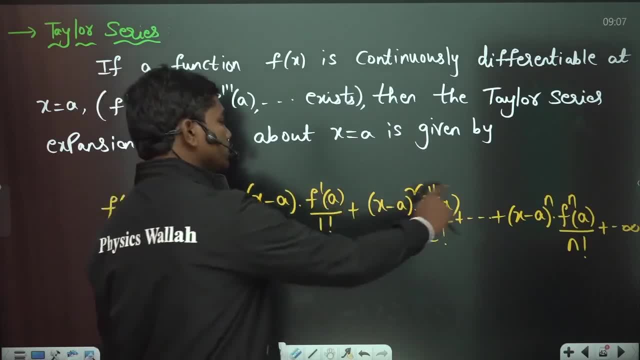 dash of a, that means i'm assuming x is dash of a, that means i'm assuming x is very close to a correct. so whenever x is very close to a correct. so whenever x is very close to a correct. so whenever x is very close to a. this higher, higher order. 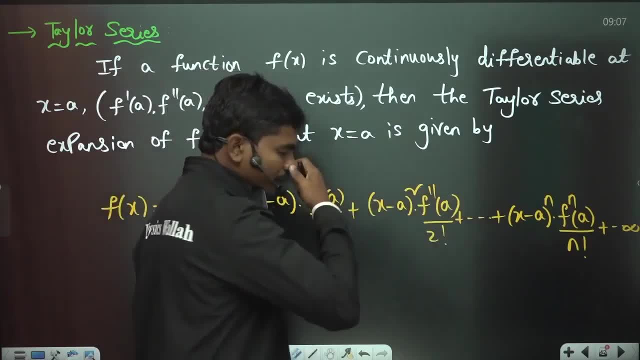 very close to a this higher higher order. very close to a this higher higher order. terms: x minus a whole square. x minus a terms. x minus a whole square. x minus a terms. x minus a whole square. x minus a whole cube. all these terms will be much. 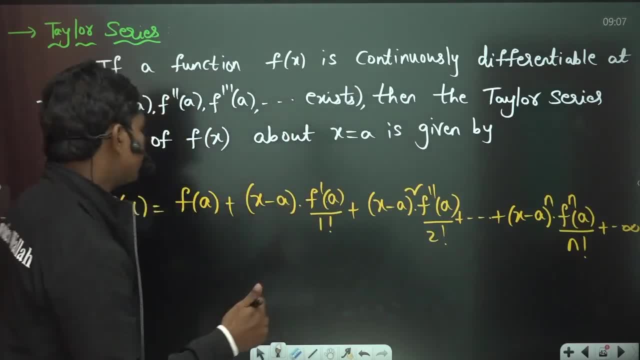 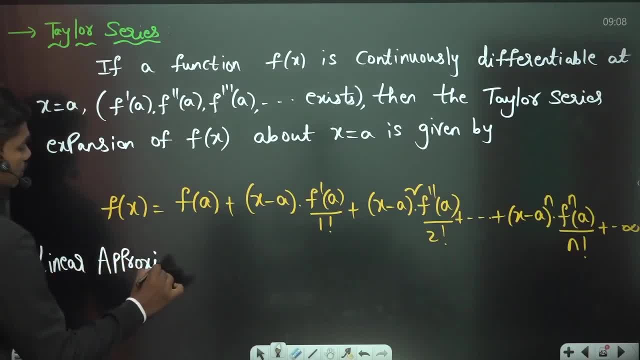 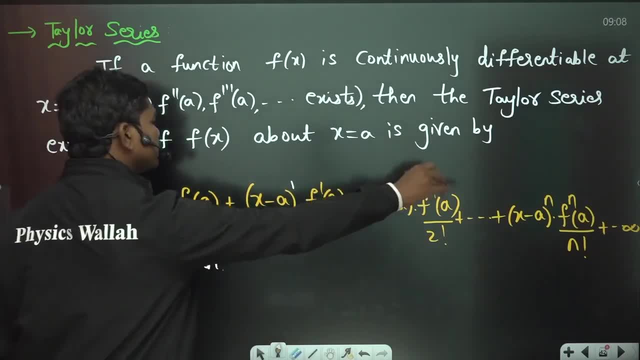 the terms only till the linear degree. the terms only till the linear degree means here the degree is one. means here the degree is one. means here the degree is one. from here they are higher order terms from here they are higher order terms from here they are higher order terms second degree, third degree, and so on. so 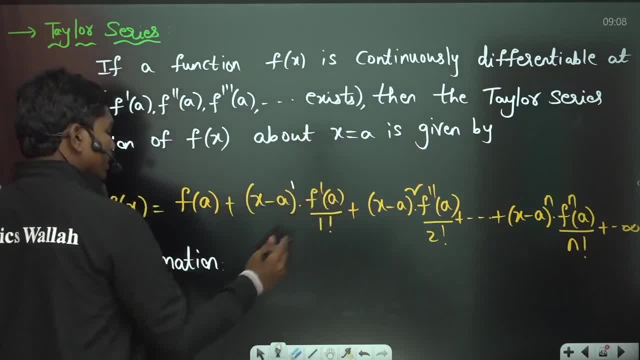 second degree, third degree, and so on. so second degree, third degree, and so on. so, in case of linear approximation, we, in case of linear approximation, we, in case of linear approximation, we consider that lsa is only till this value, consider that lsa is only till this value. 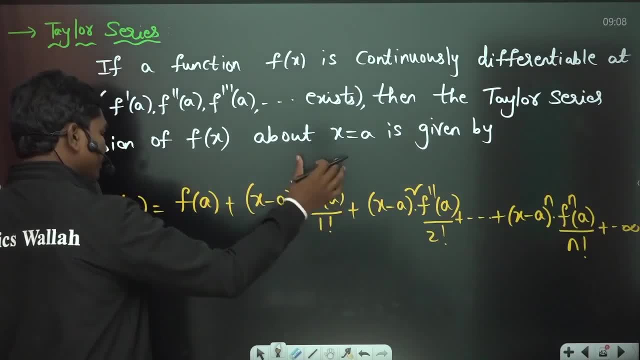 consider that lsa is only till this value so f of. because why? because whenever we so f of? because? why? because whenever we so f of, because why? because whenever we are talking about f dash of a f double are talking about f dash of a f double. 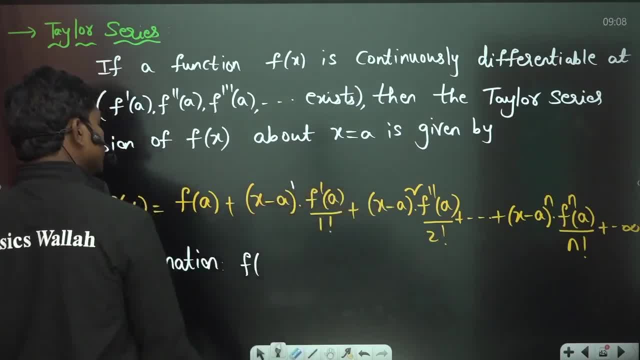 are talking about f dash of a, f double dash of a. all these things we assume dash of a. all these things, we assume dash of a. all these things. we assume that x and a are very close to each other, that x and a are very close to each other. 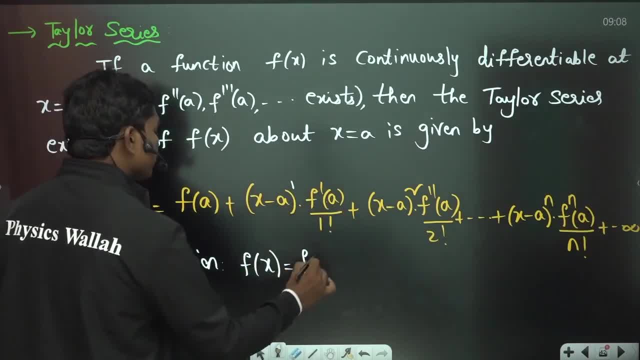 that x and a are very close to each other. so we see f of x is equal to f of a plus. so we see f of x is equal to f of a plus. so we see f of x is equal to f of a plus, x minus a times of f dash of a. 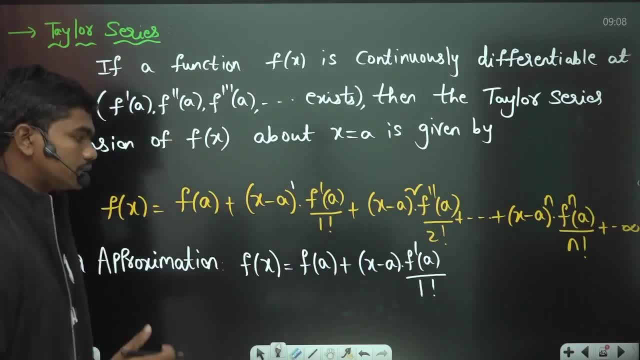 x minus a times of f dash of a. x minus a times of f dash of a by one factorial. okay, this is where we'll by one factorial. okay, this is where we'll by one factorial. okay, this is where we'll end, because this is the linear. 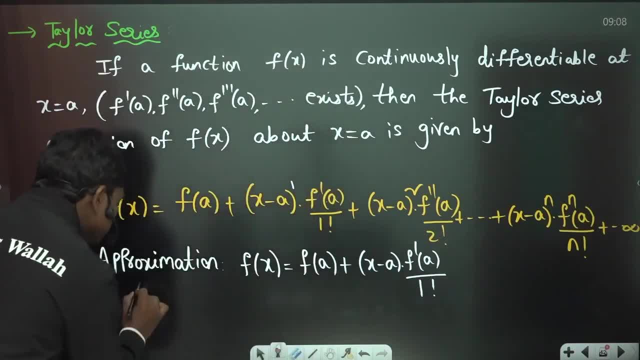 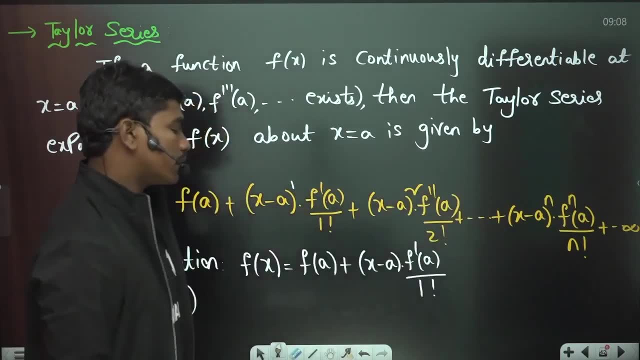 end, because this is the linear end, because this is the linear approximation, approximation, approximation. this linear approximation means approximation, means approximation, means approximation. you will consider till this approximation, you will consider, till this approximation, you will consider till this point, similarly cubic approximation, you point similarly cubic approximation, you. 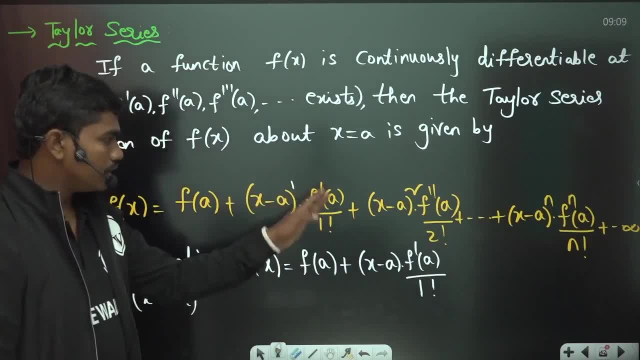 point. similarly, cubic approximation, you will consider till the third derivative, will consider till the third derivative, will consider till the third derivative. okay, but right now, if you see we'll take, okay, but right now, if you see, we'll take, okay, but right now, if you see, we'll take the linear approximation. 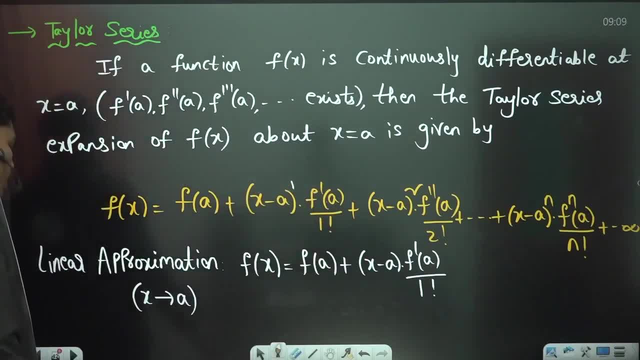 the linear approximation, the linear approximation and the series ends here, okay, and also, and the series ends here, okay, and also, and the series ends here, okay, and also, if you see uh basically one thing, if you see uh basically one thing, if you see uh basically one thing. coefficient of 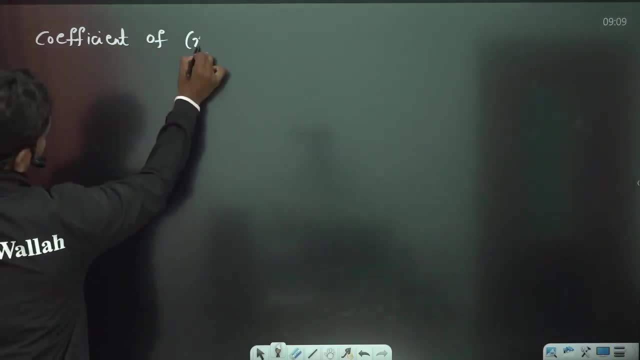 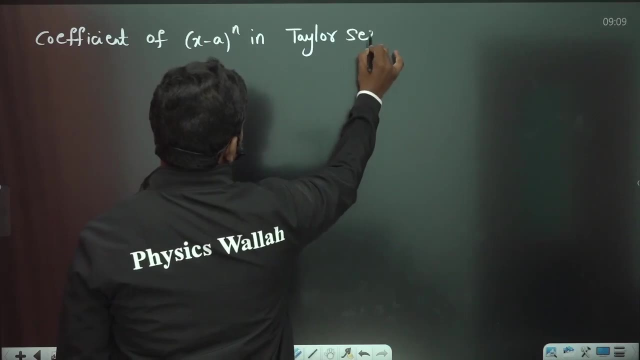 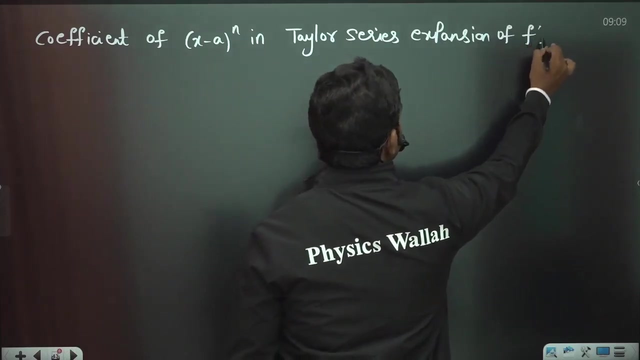 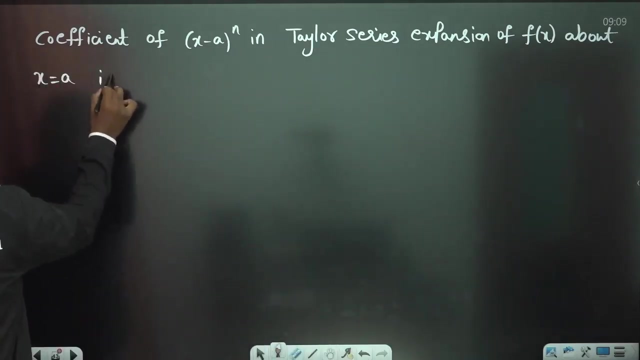 coefficient of x minus a whole power n. x minus a whole power n. x minus a whole power n in in in taylor series. expansion of f of x in taylor series. expansion of f of x. about x is equal to a. about. about x is equal to a is. 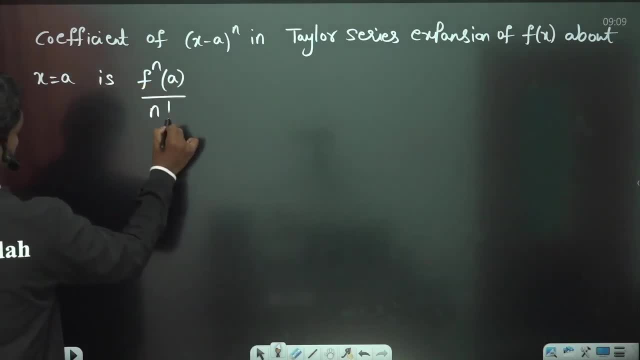 x is equal to a. is x is equal to a. is nth derivative of f at a divided by nth derivative of f at a, divided by nth derivative of f at a divided by n factorial. okay, so this is n factorial. n factorial. okay, so this is n factorial. 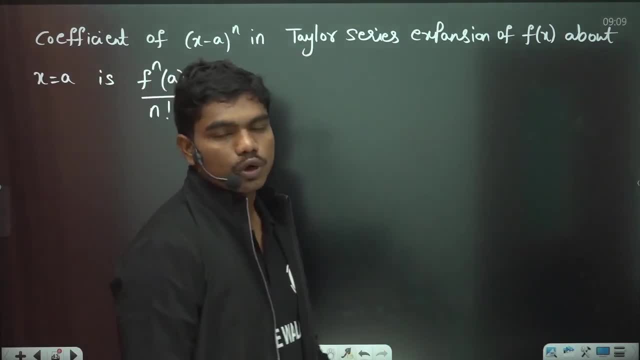 n factorial, okay, so this is n factorial now. let us now. let us now let us see: uh, basically, this is how we'll get see. uh, basically, this is how we'll get see. uh, basically, this is how we'll get the coefficients okay, the coefficients okay, the coefficients okay, and linear approximations aren't all. now, let and linear approximations aren't all now. let and linear approximations aren't all now. let us see some, us see some, us see some. let us generate the taylor series. let us generate the taylor series. let us generate the taylor series. expansions for expansions for. 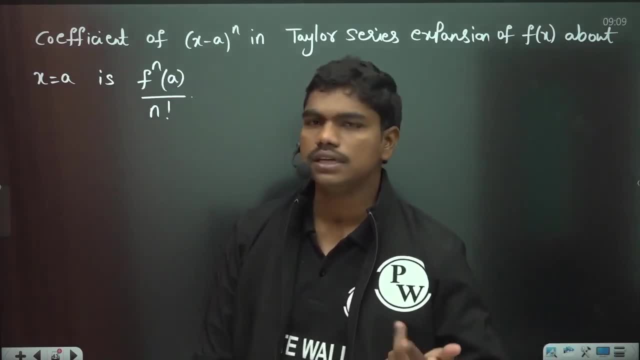 expansions for two, three regular functions: sine x, cos x. two, three regular functions: sine x, cos x. two, three regular functions: sine x, cos x, e power x. let us say these three: e power x. let us say these three, e power x, let us say these three functions, let us generate the. 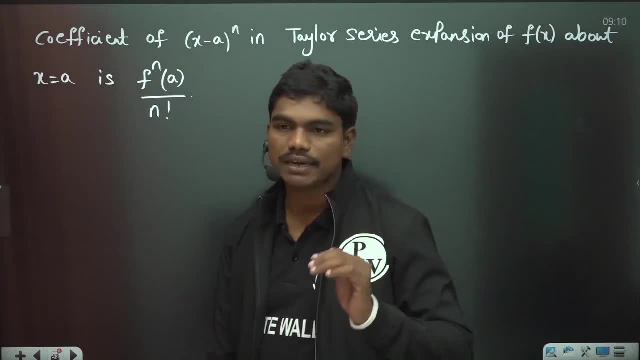 functions. let us generate the functions. let us generate the expansions. okay so, how expansions? okay so, how expansions- okay so how so how these expansions look like. okay so, how these expansions look like. okay so, how these expansions look like: okay so first, so first, so first: f of x is equal to sine x. let us suppose, 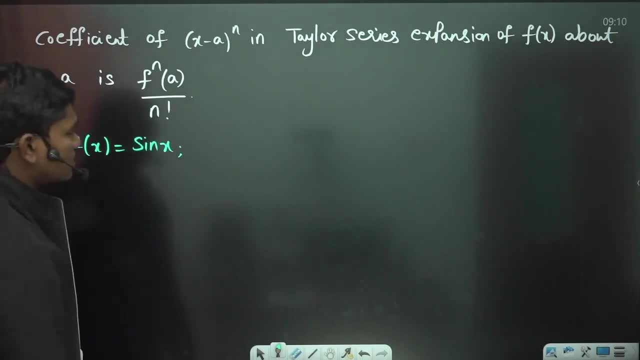 f of x is equal to sine x. let us suppose f of x is equal to sine x. let us suppose you have taken sine x. you have taken sine x, you have taken sine x. so what is the differentiation basically? so what is the differentiation basically? so what is the differentiation basically? look, if you write sine x, if you add this: 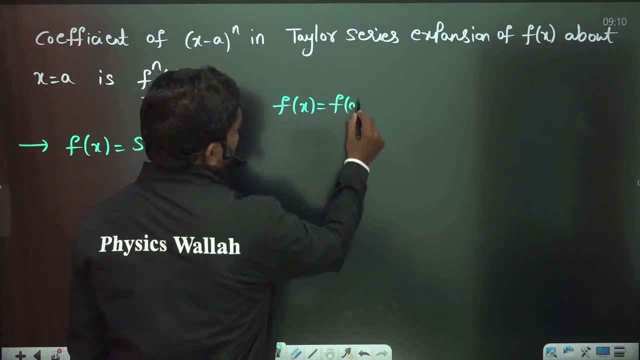 look if you write sine x. if you add this. look if you write sine x. if you add this, expression f of x is equal to f of a expression. f of x is equal to f of a expression. f of x is equal to f of a plus x, minus a into f. dash of. 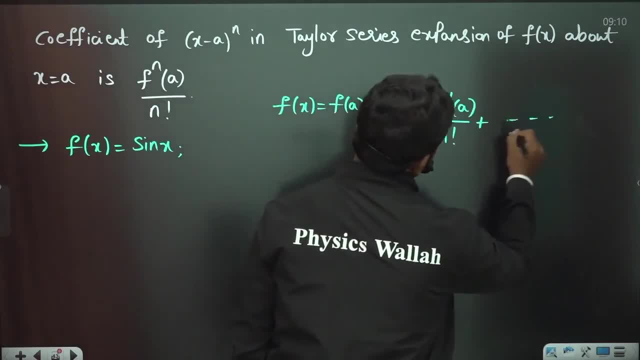 plus x minus a into f. dash of plus x minus a into f. dash of e? a by one factorial plus, and so on. e a by one factorial plus, and so on. e a by one factorial plus, and so on, infinity. let us suppose, if you write the 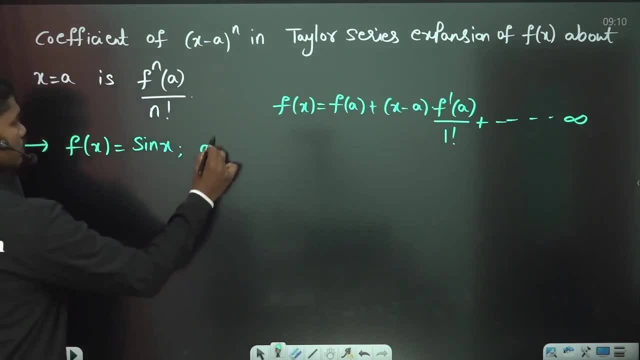 infinity. let us suppose if you write the infinity. let us suppose if you write the infinite electioning series. infinite electioning series, infinite electioning series. so tell me about x is equal to 0. you so tell me about x is equal to 0. you so tell me about x is equal to 0. you are writing about x is equal to 0 means. 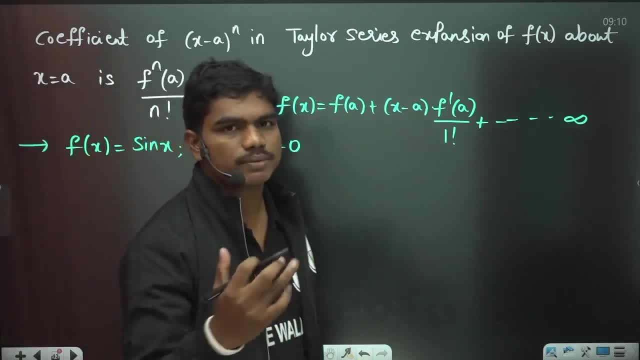 are writing about x is equal to 0 means are writing about x is equal to 0 means in the expansion. you just need x terms in the expansion. you just need x terms in the expansion. you just need x terms. you need not need any term like x minus. 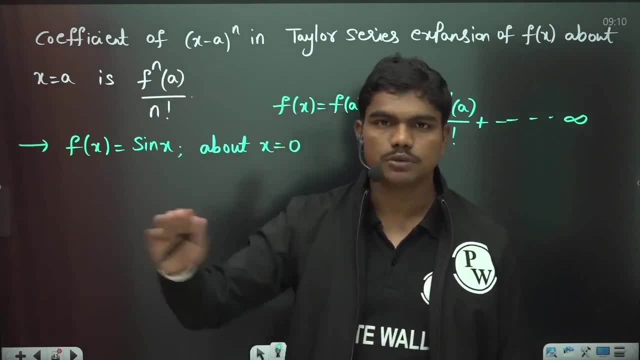 you need not need any term like x minus. you need not need any term like x minus pi by 3 x minus pi by 2- nothing like pi by 3 x minus pi by 2. nothing like pi by 3 x minus pi by 2, nothing like that. you just need the series in terms: 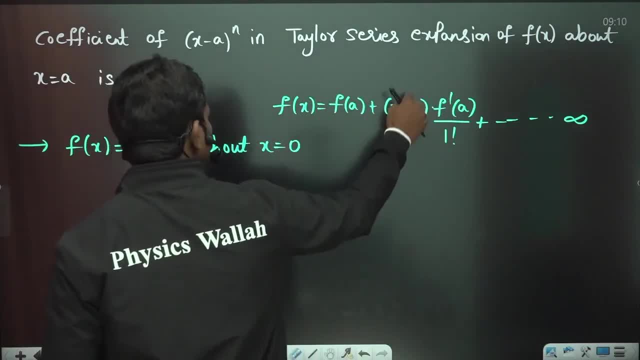 that you just need the series in terms that you just need the series in terms of x. that's it okay. so that means this: a of x, that's it okay. so that means this a of x, that's it okay. so that means this: a value has to be zero, correct if this a. 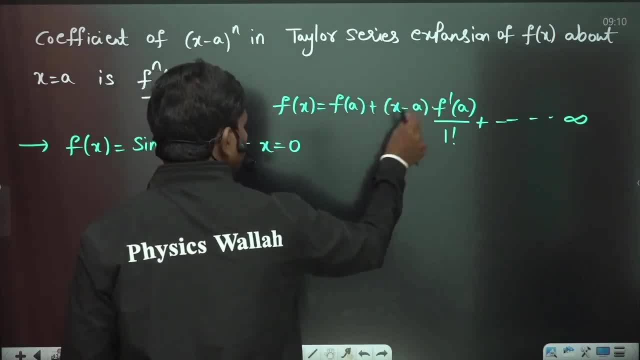 value has to be zero, correct. if this a value has to be zero, correct. if this a value is equal to 0, only in that case value is equal to 0. only in that case value is equal to 0. only in that case you will have x terms, okay, otherwise, 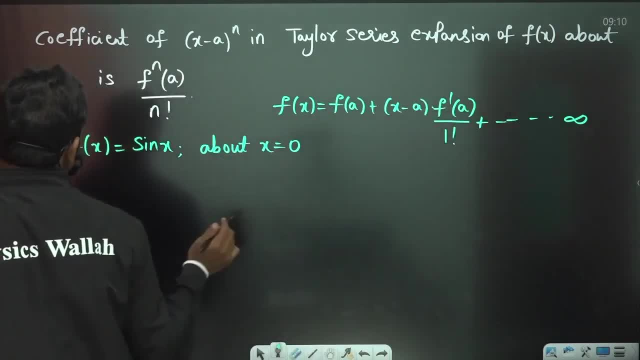 you will have x terms okay. otherwise you will have x terms okay, otherwise you'll have some x minus some constant. you'll have some x minus some constant. you'll have some x minus some constant terms. okay, so we need only x terms now. terms: okay, so we need only x terms now. 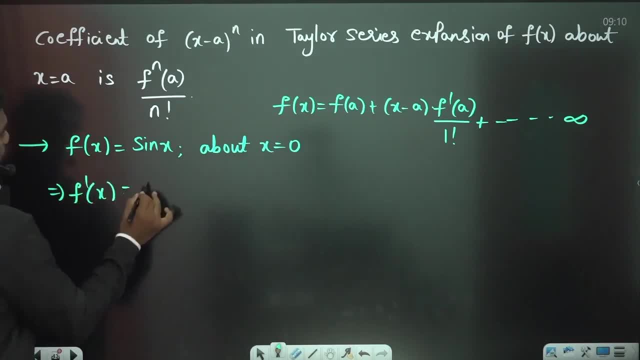 terms. okay, so we need only x terms now see how it's happening. f dash of x is- see how it's happening. f dash of x is: see how it's happening. f dash of x is equal to cos x, equal to cos x, equal to cos x. so this implies f dash of 0 is equal to. 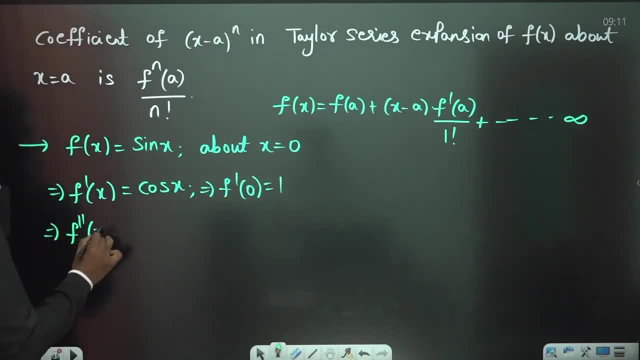 so this implies f dash of 0 is equal to. so this implies f dash of 0 is equal to 1 cos 0 is 1. f double dash of x is equal 1 cos 0 is equal to minus cos x, minus cos x. 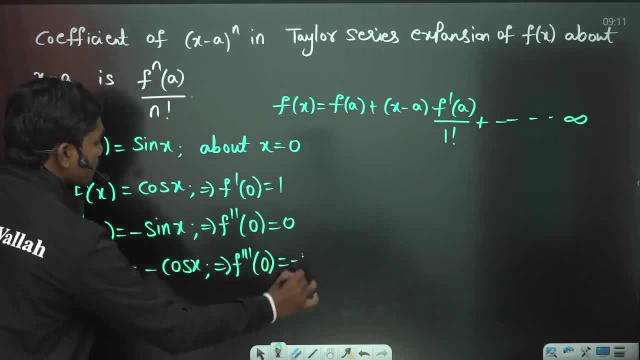 minus cos x. so f double dash of 0 is minus 1, so f double dash of 0 is minus 1, so f double dash of 0 is minus 1. similarly, fourth derivative of x. similarly, fourth derivative of x. similarly, fourth derivative of x, which is minus of differentiation of. 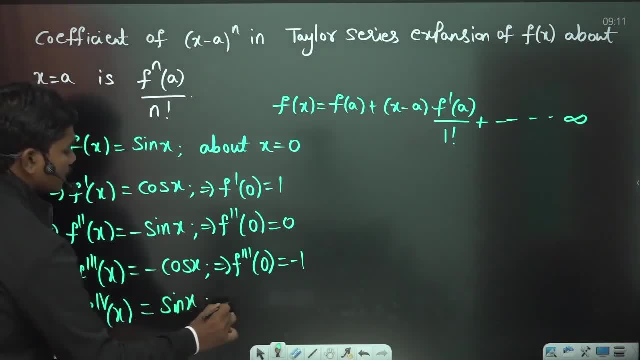 which is minus of differentiation, of which is minus of differentiation of cos x is minus sine x. so total cos x is minus sine x, so total cos x is minus sine x, so total you will have sine x, which means f fourth. you will have sine x, which means f fourth. 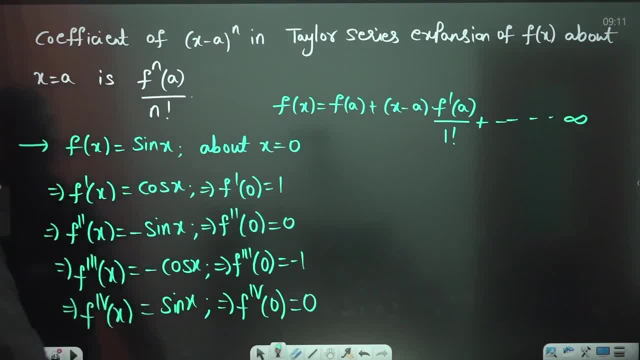 you will have sine x, which means f. fourth derivative of zero. derivative of zero. derivative of zero is again zero, so you can understand. one is again zero, so you can understand. one is again zero, so you can understand one thing, thing, thing. after three derivatives, the fourth. after three derivatives, the fourth. 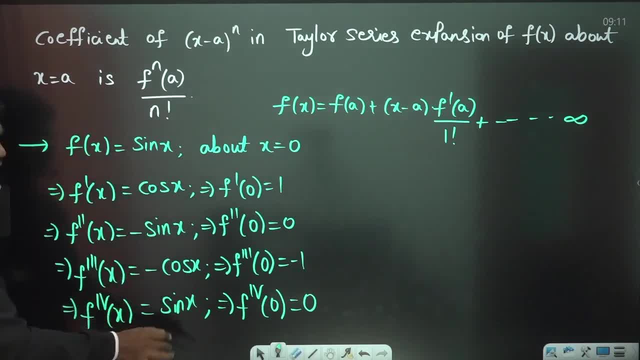 after three derivatives, the fourth derivative is again the function itself. derivative is again the function itself. derivative is again the function itself. now, let us suppose, if you do now, let us suppose, if you do now, let us suppose, if you do differentiation once more, you'll get cos. 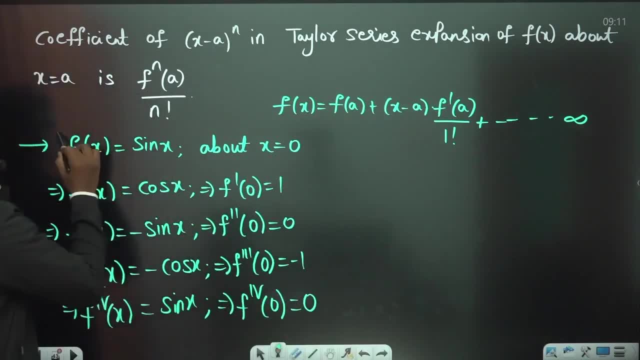 differentiation. once more, you'll get cos differentiation. once more, you'll get cos x, which means this means basically this x, which means this means basically this x, which means this means basically this: sine x, cos x minus sine x minus cos x. sine x, cos x minus sine x minus cos x. 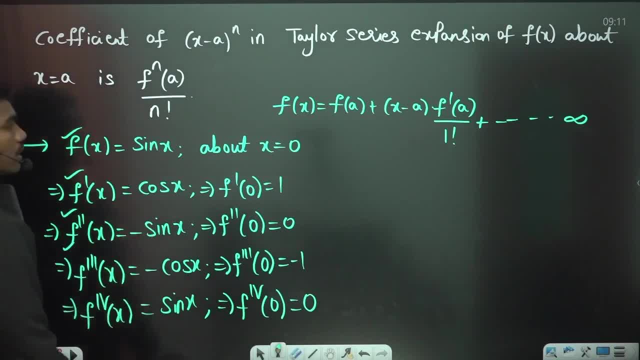 sine x, cos x minus sine x minus cos x. these four terms will be repeating. these four terms will be repeating. these four terms will be repeating actually okay, so that's how. if you see in: actually okay, so that's how. if you see in: actually okay, so that's how. if you see in this is f of X means basically sine X is. 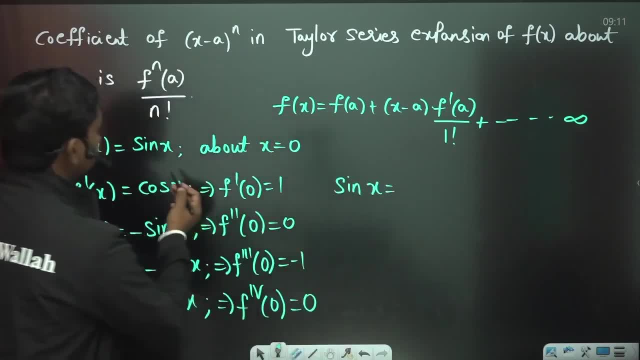 this is f of X means basically sine X is: this is f of X means basically sine X is equal to f of 0, so sine 0 is 0, so f of 0 equal to f of 0, so sine 0 is 0, so f of 0. 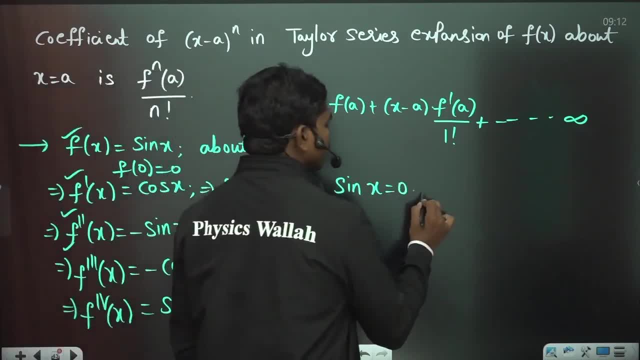 equal to f of 0, so sine 0 is 0, so f of 0. if you write this is 0, so sine 0 plus X. if you write this is 0, so sine 0 plus X. if you write this is 0, so sine 0 plus X minus a, which is X into F. dash of a by 1. 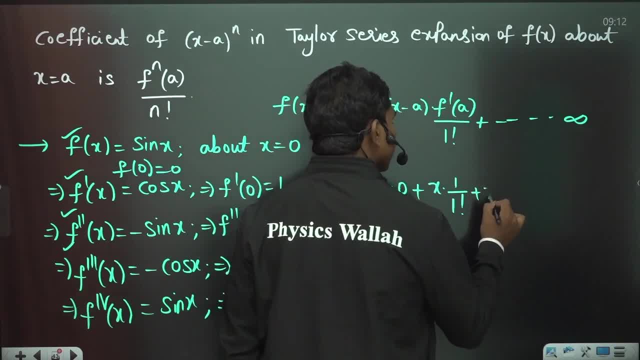 minus a, which is X, into F. dash of a by 1 minus a, which is X, into F. dash of a by 1 factorial, so 1 by 1 factorial plus X. factorial, so 1 by 1 factorial plus X. factorial, so 1 by 1 factorial plus X minus a whole, square into F, double dash. 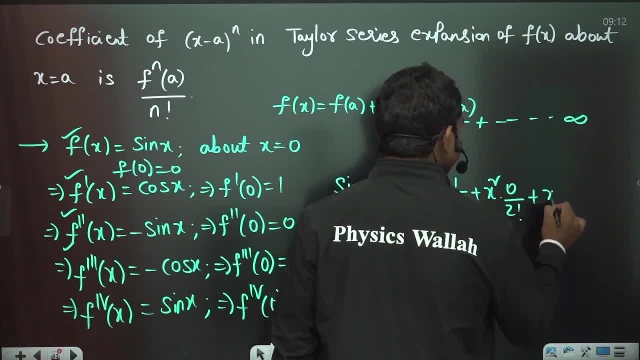 minus a whole square into F double dash: minus a whole square into F. double dash of a 0 by 2 factorial next plus X cube of a 0 by 2 factorial next plus X cube of a 0 by 2 factorial next plus X cube into third derivative, minus 1 by 1. 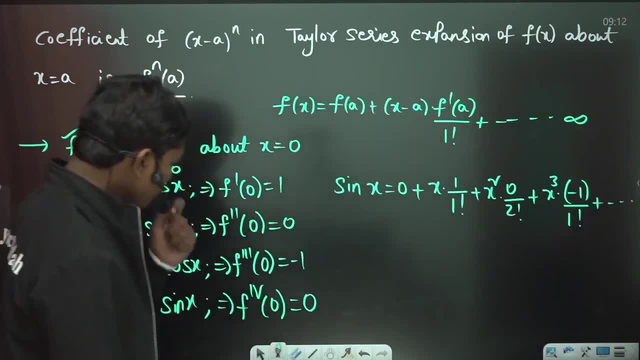 into third derivative minus 1 by 1, into third derivative minus 1 by 1, factorial plus, and so on. this goes on now. factorial plus, and so on. this goes on now. factorial plus, and so on. this goes on. now we can understand one thing, can I say? 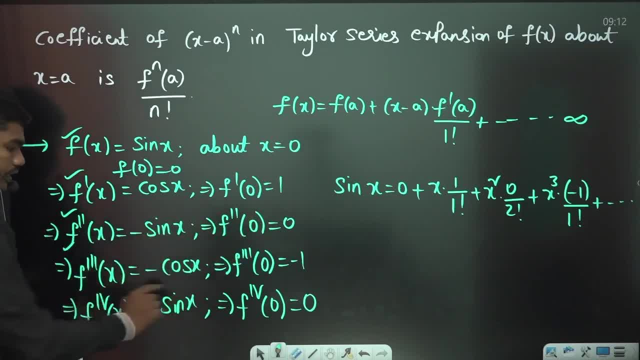 we can understand one thing. can I say we can understand one thing. can I say: all the event derivatives will be 0, all the event derivatives will be 0, all the event derivatives will be 0. second derivative 0. fourth derivative: 0. second derivative 0. fourth derivative 0. 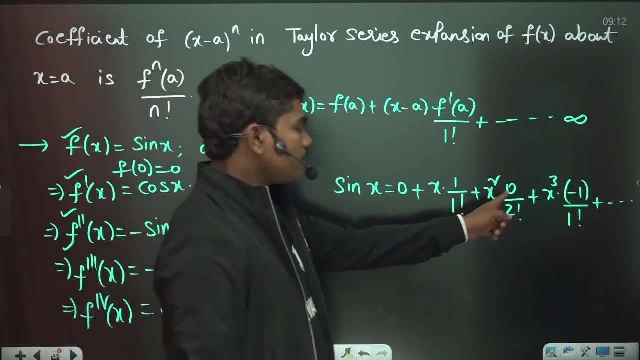 second derivative: 0. fourth derivative: 0. again 6th derivative will be 0, which again 6th derivative will be 0, which again 6th derivative will be 0, which means you can see whenever even means, you can see whenever even means, you can see whenever even derivatives means, if you see the even. 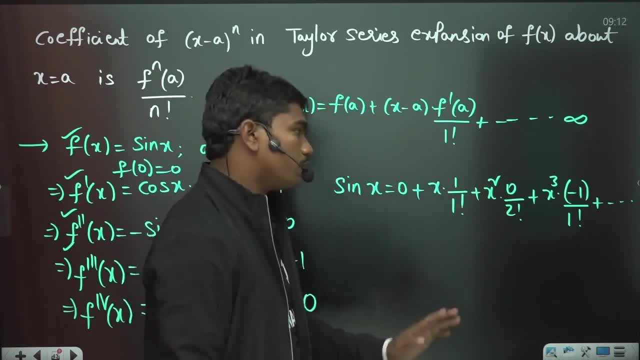 derivatives means if you see the even derivatives, means if you see the even power terms in this Sinex expansion are power terms in this Sinex expansion, are power terms in this Sinex expansion are. you know you cannot see the even power. you know you cannot see the even power. 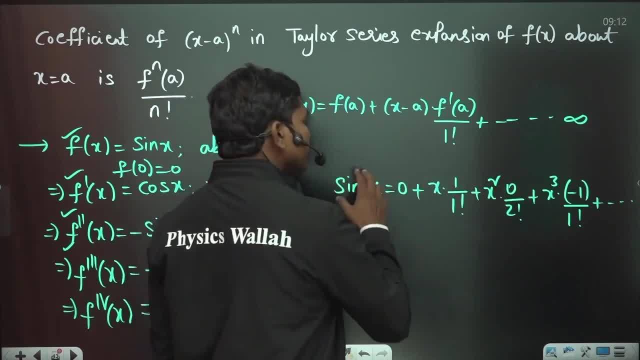 you know, you cannot see the even power terms because the even derivatives of terms, because the even derivatives of terms, because the even derivatives of the function is 0, so in the Taylor series the function is 0, so in the Taylor series the function is 0. so in the Taylor series expansion, you cannot see any terms with 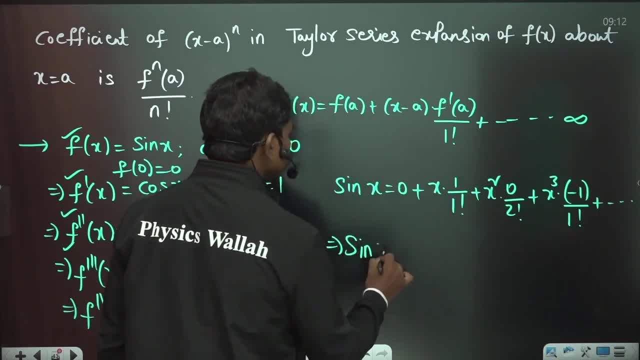 expansion. you cannot see any terms with expansion. you cannot see any terms with even degree. so that's why, if you see even degree, so that's why, if you see even degree, so that's why, if you see your sine, X is equal to X minus X cube by. 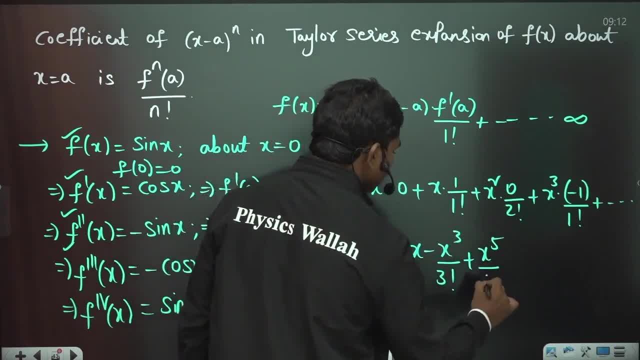 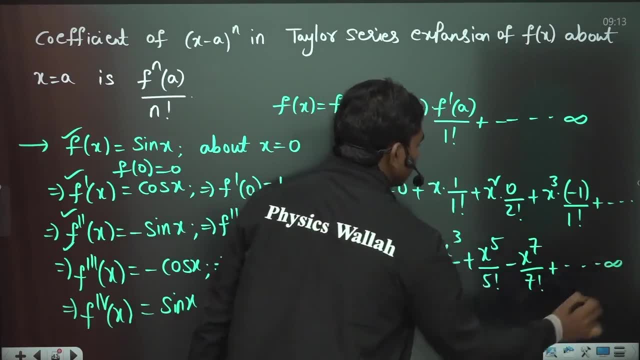 your sine X is equal to X minus X cube by. your sine X is equal to X minus X cube by 3. factorial plus X power, 5 by 5. 3 factorial plus X power, 5 by 5. 3. factorial plus X power, 5 by 5. okay, so this is the expansion of sine X. 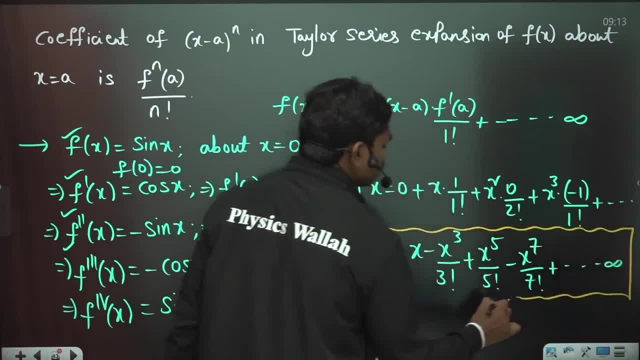 okay, so this is the expansion of sine X. okay, so this is the expansion of sine X. about the function X is equal about the. about the function X is equal about the. about the function X is equal about the point: X is equal to 0. okay, so this is. 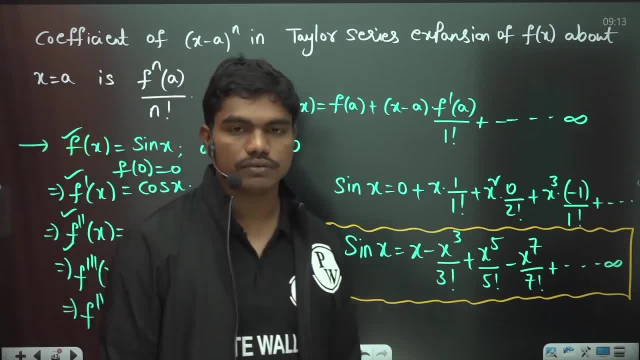 point X is equal to 0. okay, so this is. point X is equal to 0. okay, so this is sine X expansion. now you have written sine X expansion. now you have written sine X expansion. now you have written this point many times for very small, this point many times for very small. 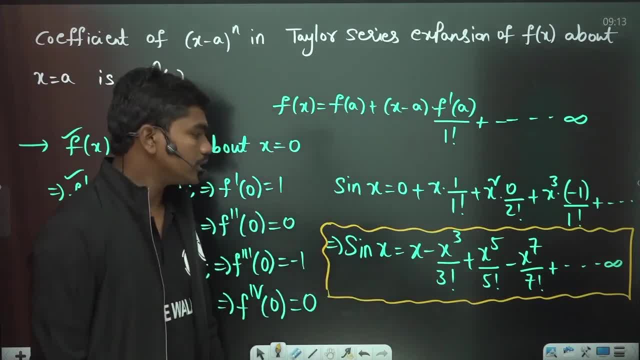 this point many times. for very small values of X sine X is equal to X. how do values of X sine X is equal to X? how do values of X sine X is equal to X? how do you know that? because if you see whenever. you know that because if you see whenever, 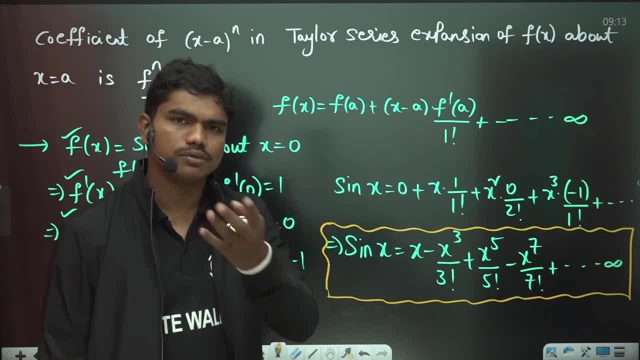 you know that because if you see, whenever X is very small, like for example 0.001 X is very small, like for example 0.001 X is very small, like for example 0.001, 10 power minus 4, you can take like that: 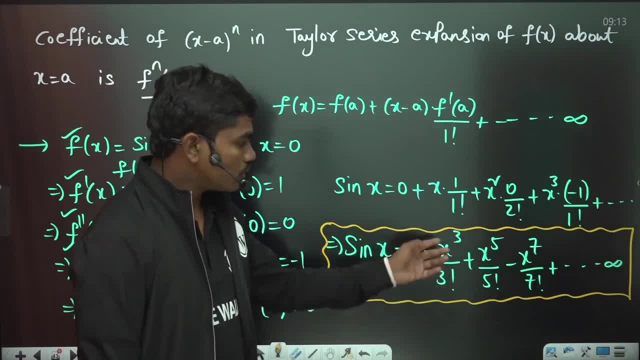 10 power minus 4, you can take like that. 10 power minus 4, you can take like that. so then this X cube value will be much. so then this X cube value will be much. so then this X cube value will be much, much smaller, correct? so X power 5 is. 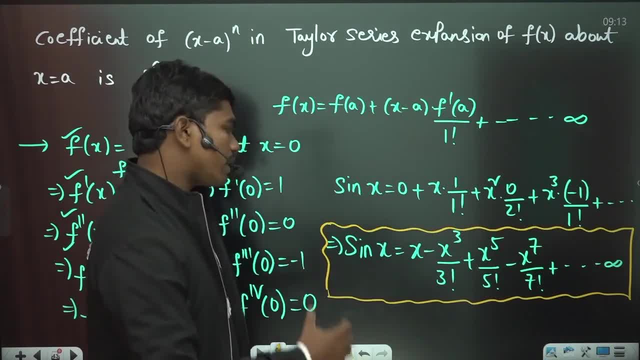 much smaller, correct? so X power 5 is much smaller, correct? so X power 5 is still small. X power 7 is very, very still small. X power 7 is very, very still small. X power 7 is very, very small. so that's why, whenever X is very 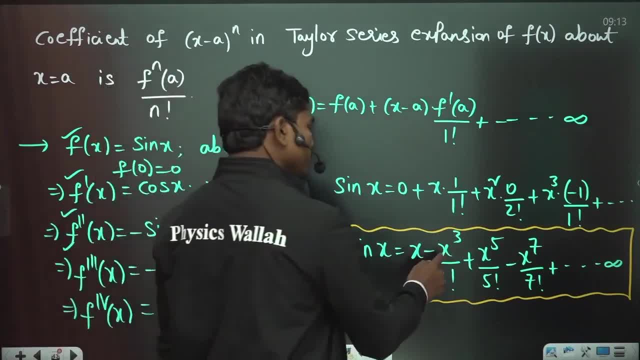 small. so that's why whenever X is very small, so that's why whenever X is very small, for small values of X means X is small. for small values of X means X is small. for small values of X means X is very small. this X cube will be much. 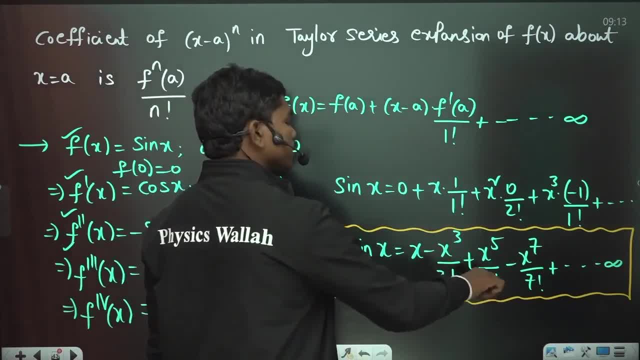 very small. this X cube will be much, very small. this X cube will be much smaller. and 3 factorial is division with smaller, and 3 factorial is division with smaller and 3 factorial is division with 6. 5 factorial is division with 120, 7. 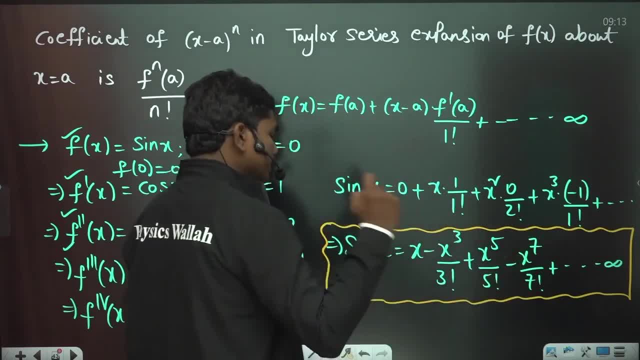 6, 5. factorial is division with 120: 7, 6, 5. factorial is division with 120: 7. factorial: 5 0, 4, 0. so all these terms factorial 5 0, 4, 0, so all these terms factorial 5 0, 4, 0, so all these terms will come very, very small. so that's how. 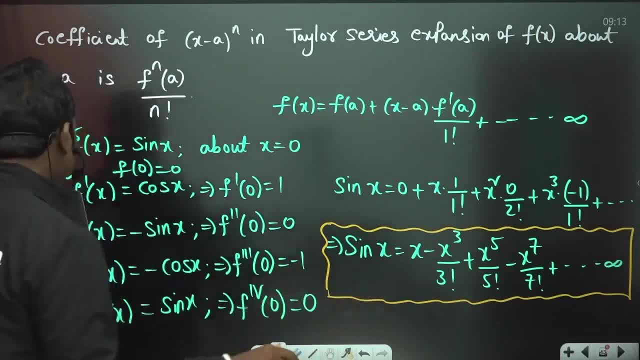 will come very, very small. so that's how will come very, very small. so that's how this sine X value will be almost equal. this sine X value will be almost equal. this sine X value will be almost equal to X. and also I would like to show it: 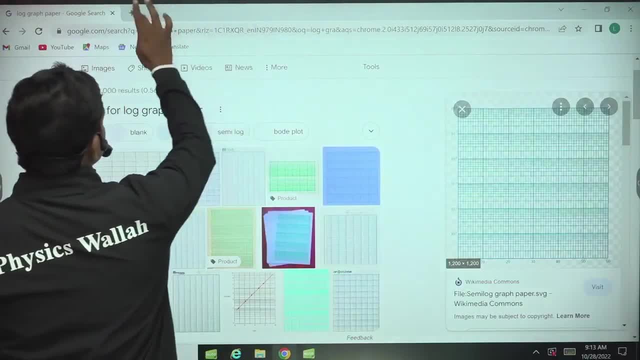 to X and also I would like to show it to X and also I would like to show it graphically, since we have this okay graphically, since we have this okay graphically, since we have this okay, Desmos with us, I will show you this graph. 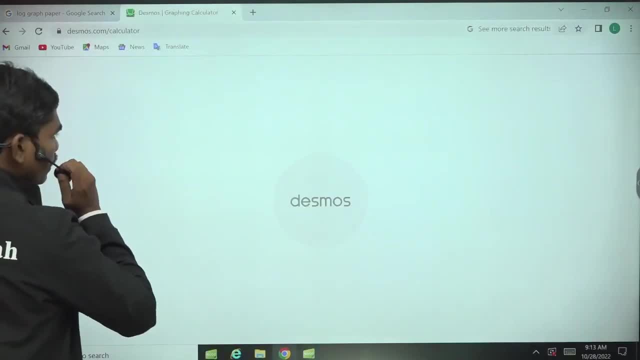 Desmos with us. I will show you this graph. Desmos with us. I will show you this graph. so see here. look will plot sine X. and so see here. look will plot sine X. and so see here. look will plot sine X. and also will plot X. I will show you. 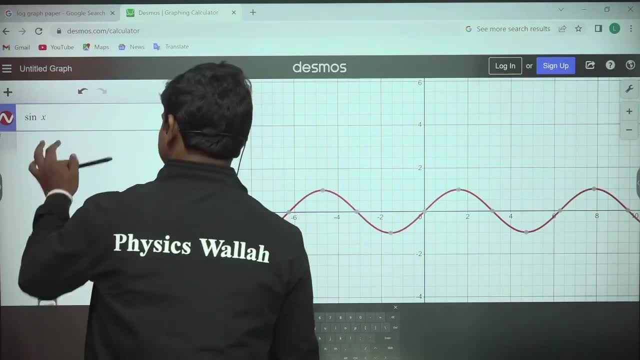 also will plot X. I will show you also will plot X. I will show you something here: so sine X X. so if you see something here, so sine X X. so if you see something here, so sine X X. so if you see, this is the graph of sine X and X. 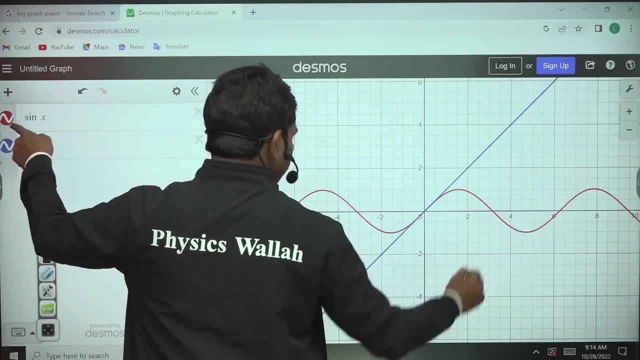 this is the graph of sine X and X. this is the graph of sine X and X, basically the red color one. you see red, basically the red color one. you see red, basically the red color one. you see red symbol is for sine X. so red color one is: 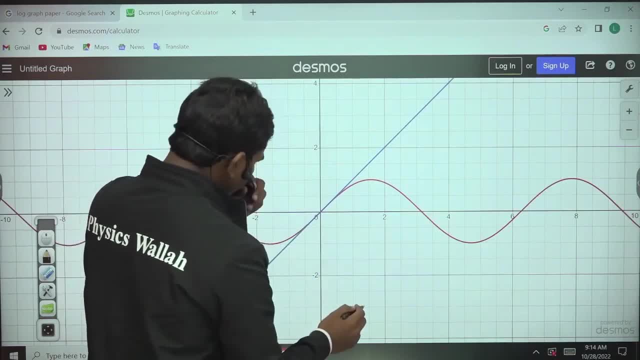 symbol is for sine X, so red color one is symbol is for sine X, so red color one is for sine X. blue is for X. so now, if you for sine X, blue is for X, so now, if you for sine X, blue is for X. so now, if you see this, look, this is x-axis, okay, and 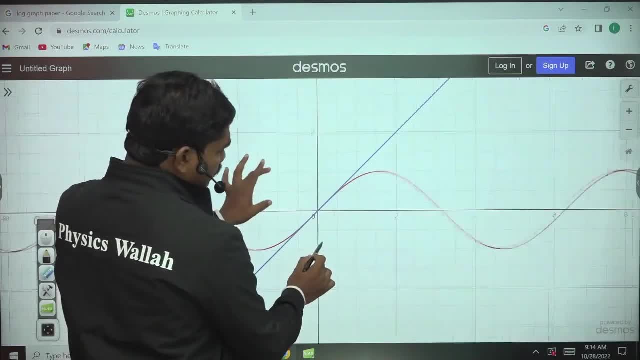 see this: look this is x-axis okay. and see this: look this is x-axis okay. and this is basically some X is equal to 1. this is basically some X is equal to 1. this is basically some X is equal to 1 around. but now, if you see very close to, 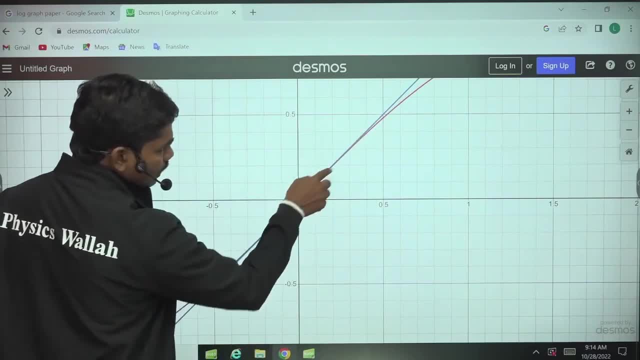 around. but now, if you see very close to around, but now if you see very close to 0, okay, so very close to 0. if you see the 0: okay, so very close to 0. if you see the 0: okay, so very close to 0. if you see the red color curve and blue color curve, red color curve and blue color curve. red color curve and blue color curve. they are almost the same, correct, they. they are almost the same, correct they. they are almost the same, correct. they have overlapped each other and they, you have overlapped each other and they you. 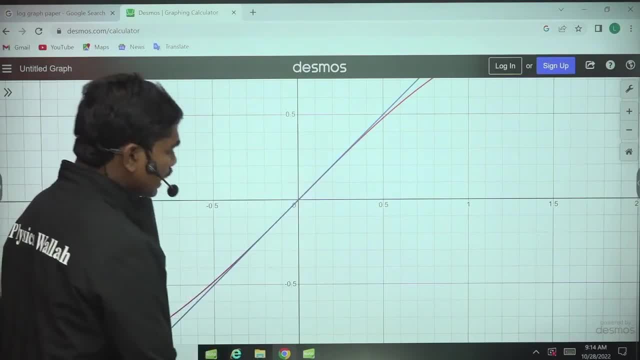 have overlapped each other and they, you can appear. you can observe them as a can appear. you can observe them as a can appear. you can observe them as a single curve actually okay. so that's why single curve actually okay. so that's why single curve actually okay. so that's why. so that's why, if you see, whenever X. 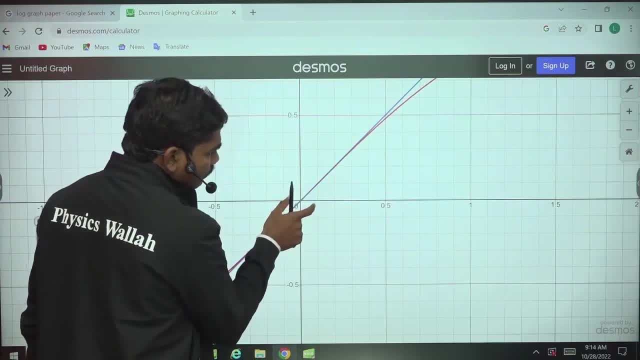 so that's why, if you see whenever X, so that's why, if you see whenever X values are very small, the sine X and X values are very small. the sine X and X values are very small, the sine X and X. you cannot find any variation between 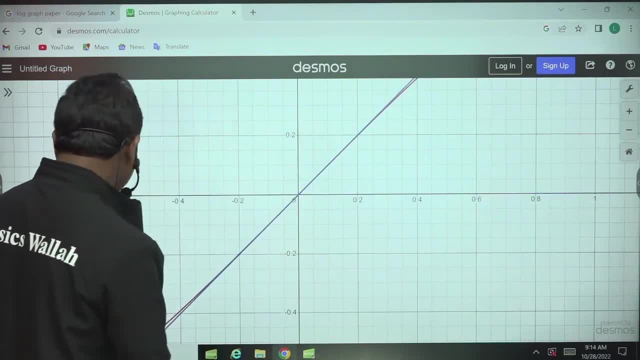 you cannot find any variation between you cannot find any variation between sine X and X. almost okay, they are very sine X and X. almost okay, they are very sine X and X. almost okay, they are very close. so that's how graphically also you close. so that's how graphically also you. 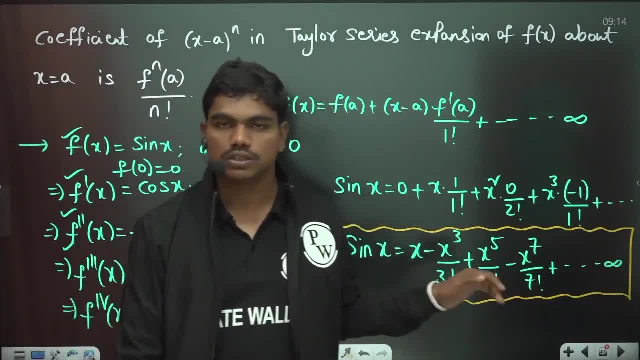 close. so that's how, graphically also, you can see sine X and X are very close. but can see sine X and X are very close. but can see sine X and X are very close. but the logic behind that is because of the. the logic behind that is because of the. 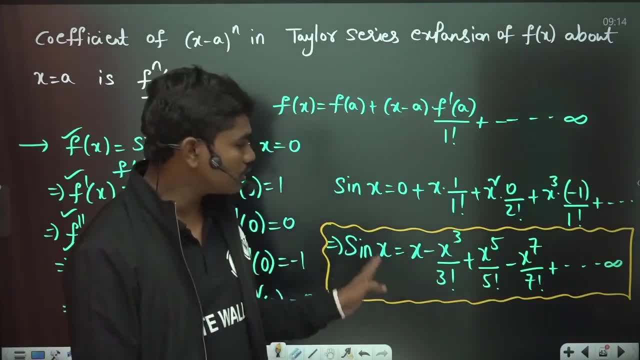 the logic behind that is because of the Taylor says okay. now you know why sine Taylor says okay. now you know why sine Taylor says okay. now you know why sine 0 is 0. if you put X equal to 0 every term, 0 is 0 if you put X equal to 0 every term. 0 is 0. if you put X equal to 0, every term is 0. okay from triangles. of course you is 0. okay from triangles, of course you is 0. okay from triangles, of course you know when theta is very small, so I know when theta is very small, so I. 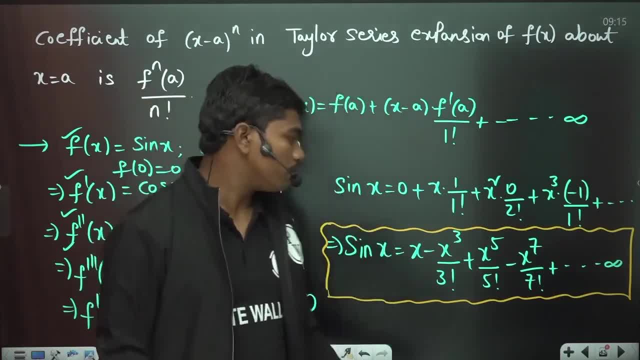 know when theta is very small. so I opposite side length comes very short, so opposite side length comes very short, so opposite side length comes very short. so that's why sine 0 is 0, but again from. that's why sine 0 is 0, but again from. 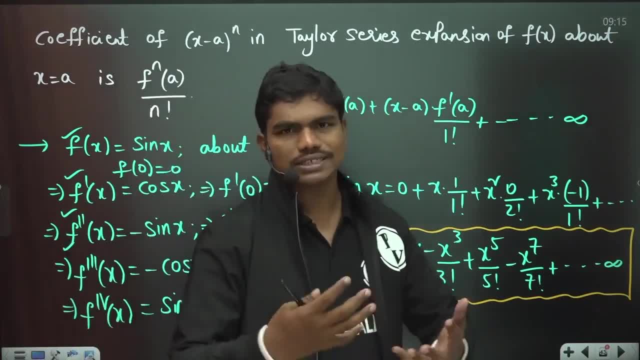 that's why sine 0 is 0. but again, from the Taylor series also. you can observe the Taylor series also. you can observe the Taylor series also. you can observe that sine 0 is 0. so all these are that sine 0 is 0. so all these are. 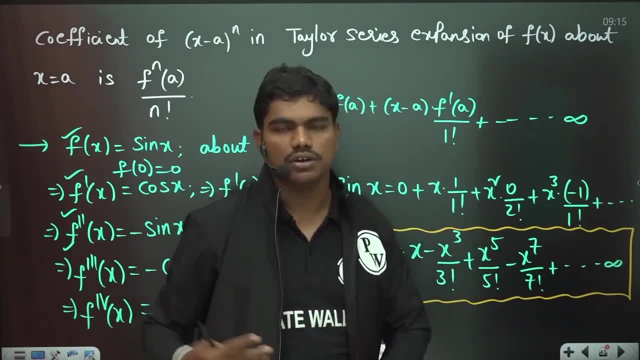 that sine 0 is 0. so all these are basically very good interconnected things, basically very good. interconnected things, basically very good. interconnected things: actually geometry calculus, all the actually geometry calculus, all the actually geometry calculus, all the things. okay. so, similarly, if you generate things, okay. so similarly, if you generate, 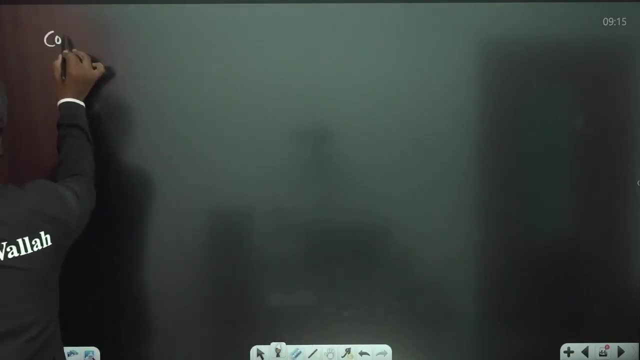 things okay. so, similarly, if you generate: for cos x- cos x 1 minus x square by 2. for cos x: cos x 1 minus x square by 2. for cos x- cos x 1 minus x square by 2 factorial, this is the series you will get. 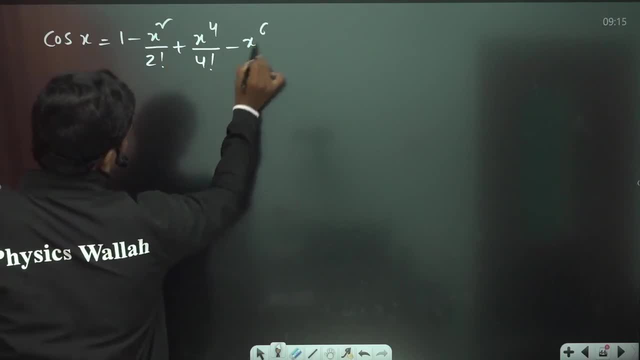 factorial: this is the series you will get. factorial: this is the series you will get if you do the same procedure minus x, if you do the same procedure minus x, if you do the same procedure, minus x, power 6 by 6. factorial plus x: power 8 by. 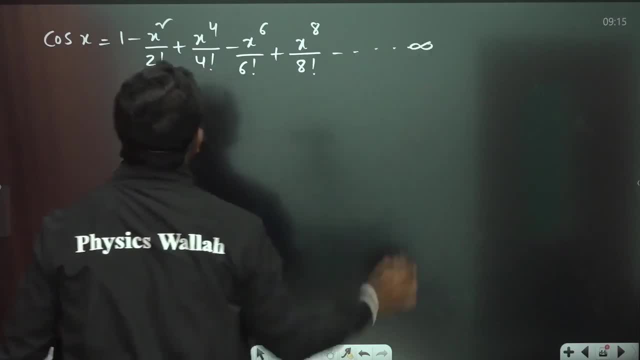 power 6 by 6 factorial plus x power 8 by power 6 by 6 factorial plus x. power 8 by 8 factorial, and so on. infinitely many 8 factorial and so on. infinitely many 8 factorial and so on. infinitely many terms. okay, so now, if you, similarly, if 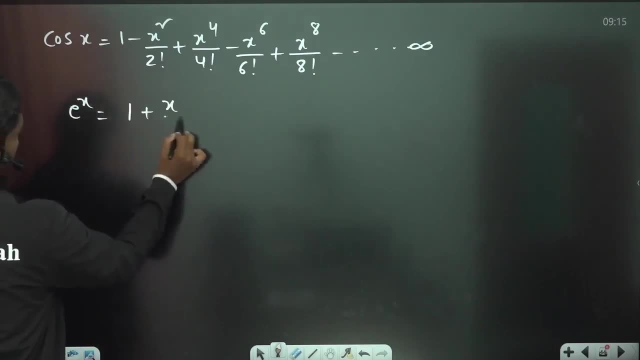 terms okay, so now if you similarly, if terms okay, so now if you, similarly, if you calculate for e power X, you will get you calculate for e power X, you will get you calculate for e power X, you will get 1 plus X by 1 factorial plus X square by: 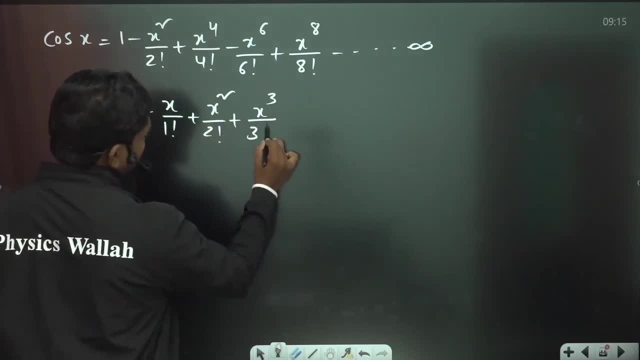 1 plus X by 1 factorial plus X square by 1 plus X by 1 factorial plus X square by 2 factorial plus X cube by 3 factorial by 2 factorial plus X cube by 3 factorial by 2 factorial plus X cube by 3 factorial by 4 factorial and so on. this goes to: 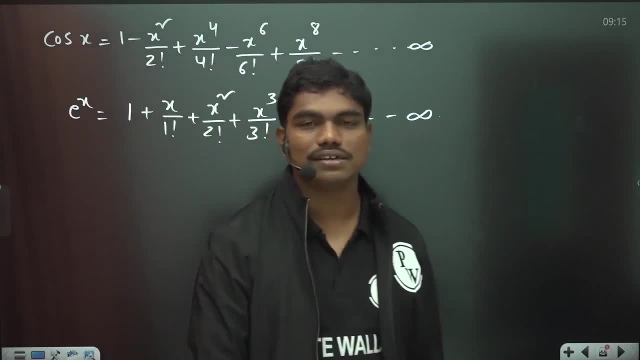 4 factorial, and so on. this goes to 4 factorial, and so on. this goes to infinity now, once in one of the classes. infinity now, once in one of the classes. infinity now, once in one of the classes. students asked me so how, the students asked me so how the. 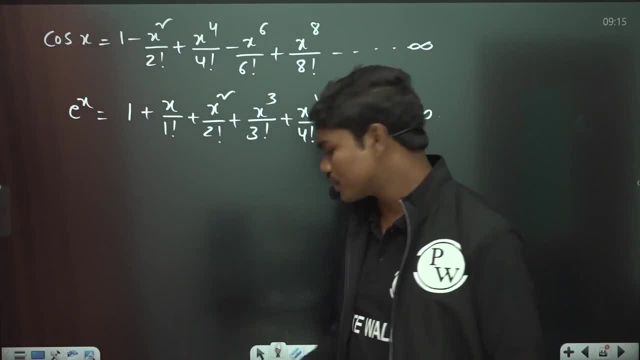 students asked me: so how? the differentiation of e power X is e power X. differentiation of e power X is e power X. differentiation of e power X is e power X. you can just differentiate this, you will. you can just differentiate this, you will. you can just differentiate this, you will get okay. so if you differentiate this, see. 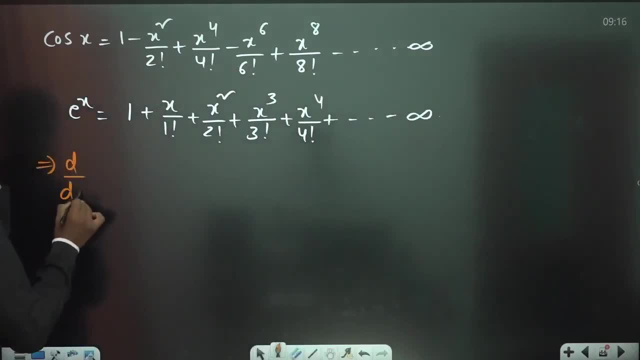 get okay. so if you differentiate this, see, get okay. so if you differentiate this, see what you will get: D by DX of e power X. what you will get D by DX of e power X, what you will get D by DX of e power X is equal to differentiation of 1: 0. it's. 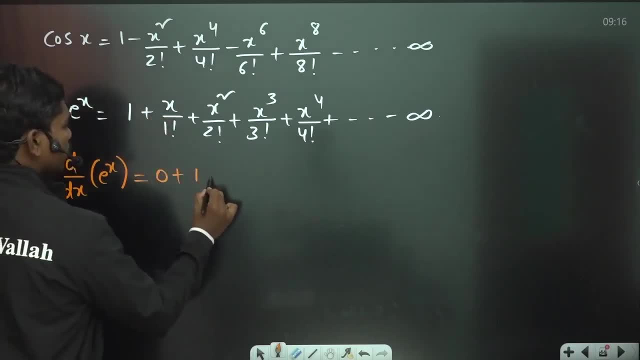 is equal to differentiation of 1: 0. it's is equal to differentiation of 1: 0. it's a constant plus differentiation of X by a constant, plus differentiation of X by a constant, plus differentiation of X by 1 factorial 1 plus differentiation of X. 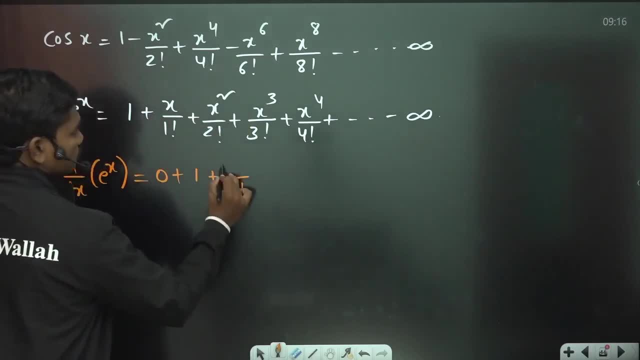 1 factorial 1 plus differentiation of X: 1 factorial 1 plus differentiation of X square by 2 factorial 2 factorial is as square by 2 factorial 2 factorial is as square by 2 factorial 2 factorial is as it is. differentiation of X square is 2x. so. 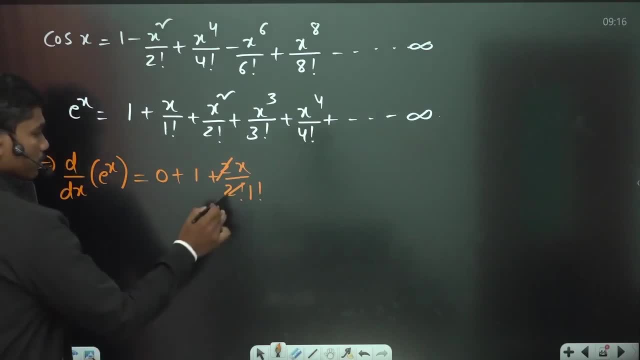 it is: differentiation of X square is 2x. so it is: differentiation of X square is 2x. so 2 can cancel this 2 factorial 1 factorial 2 can cancel this 2 factorial 1 factorial 2 can cancel this 2 factorial 1 factorial times kept because 2 factorial can be. 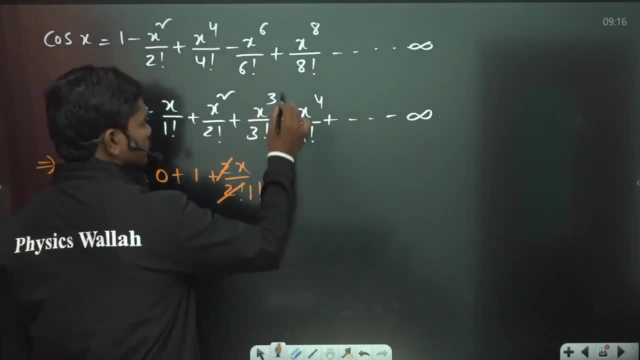 times kept because 2 factorial can be times kept because 2 factorial can be witnessed: 2 into 1 factorial, so 1 witnessed. 2 into 1 factorial, so 1 witnessed. 2 into 1 factorial, so 1 factorial plus differentiation of X cube. 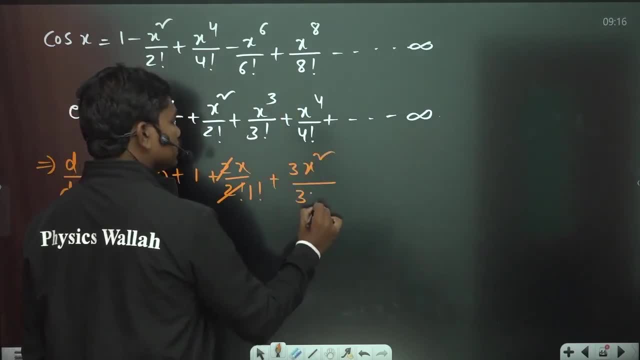 factorial plus differentiation of X cube. factorial plus differentiation of X cube: 3x square divided by 3, factorial is 3. 3x square divided by 3, factorial is 3. 3x square divided by 3, factorial is 3 into 2 factorial, so 3 they gets. 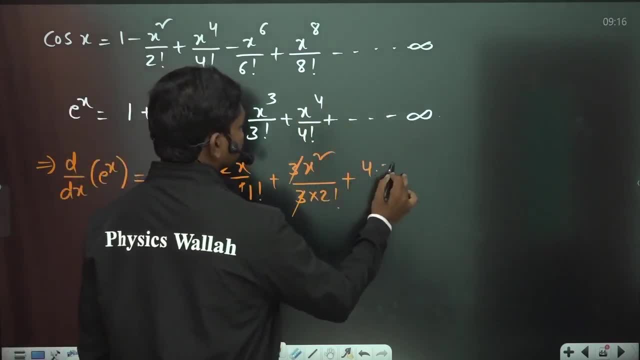 into 2 factorial, so 3: they gets into 2 factorial, so 3: they gets cancelled again. similarly, differentiation of cancelled, again similarly, differentiation of cancelled, again similarly, differentiation of X power 4: 4 into X cube by 4 into 3. X power 4: 4 into X cube by 4 into 3. 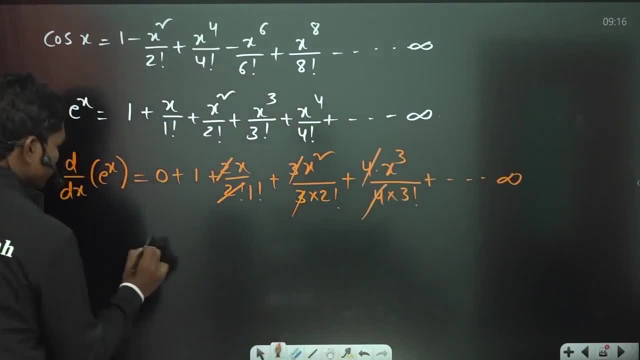 X power, 4, 4 into X cube, by 4 into 3 factorial and so on. this goes on. so you factorial, and so on. this goes on, so you factorial, and so on. this goes on, so you can cancel 4 again. so if you take as a 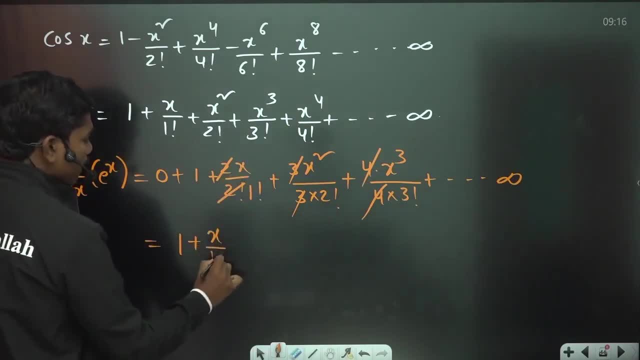 can cancel 4 again. so if you take as a can cancel 4 again. so if you take as a whole, 1 plus X by 1. factorial plus X whole, 1 plus X by 1. factorial plus X whole, 1 plus X by 1. factorial plus X square by 2. factorial plus X cube by 3: 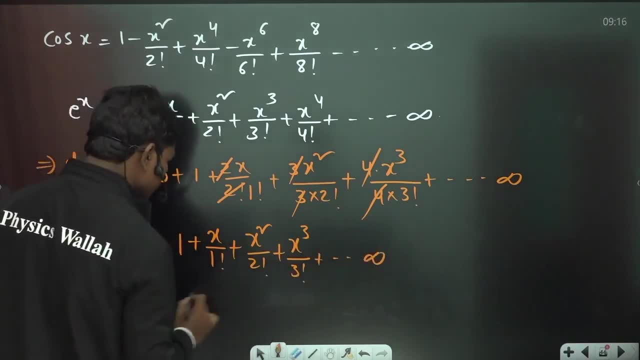 square by 2, factorial, plus X, cube by 3, square by 2, factorial plus X, cube by 3, factorial, and so on. infinity, so, which is factorial, and so on. infinity, so which is factorial, and so on. infinity, so, which is again nothing but e power X, so e power X. 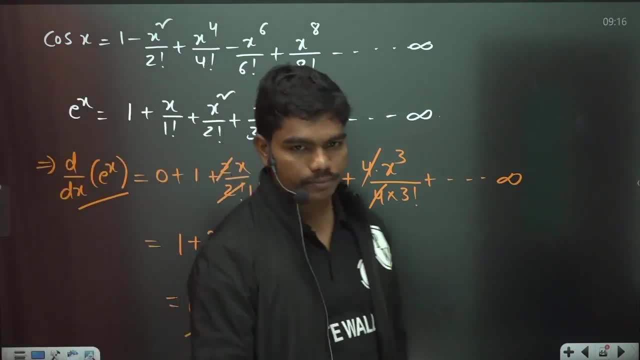 again, nothing but e power X. so e power X, again, nothing but e power X. so e power X is same as its differentiation, okay, and is same as its differentiation, okay, and is same as its differentiation, okay. and now, if you see generally, we have this. now, if you see generally, we have this. now, if you see generally we have this similarly for cos X. if you want to show similarly for cos X, if you want to show similarly for cos X, if you want to show it is minus sine X anything you can. it is minus sine X anything you can. 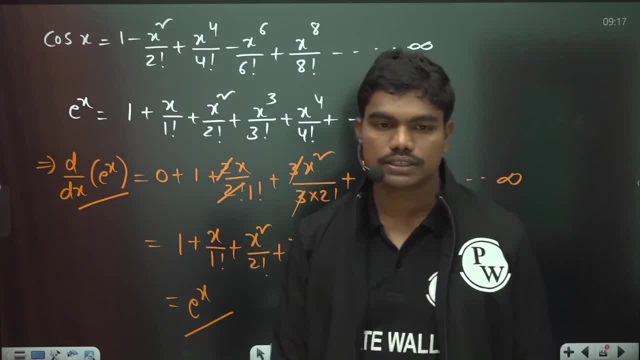 it is minus sine X. anything you can calculate using the Taylor series. calculate using the Taylor series. calculate using the Taylor series. approximations: okay. so that's how Taylor approximations okay. so that's how Taylor approximations. okay. so that's how Taylor series is very useful to you and also. 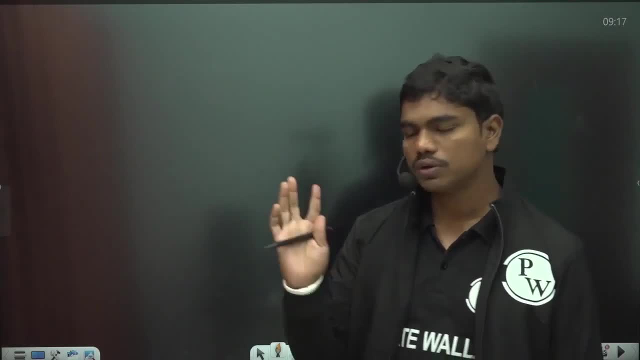 series is very useful to you and also series is very useful to you and also Taylor series. expansion in general means Taylor series. expansion in general means Taylor series. expansion in general means: not at a particular point, if you want to, not at a particular point, if you want to. 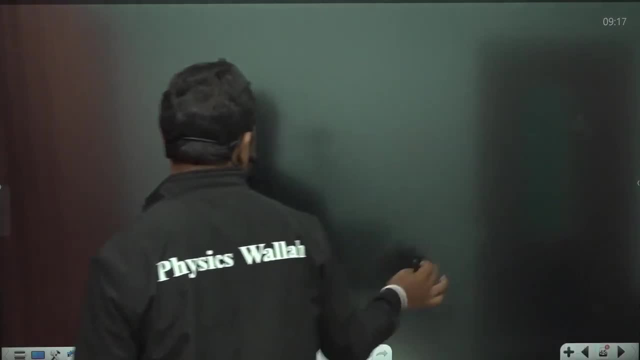 not at a particular point. if you want to calculate at any given point that general, calculate at any given point that general, calculate at any given point that general Taylor series is given by this Taylor series is given by this Taylor series is given by this expression: F of X plus H is equal to F. 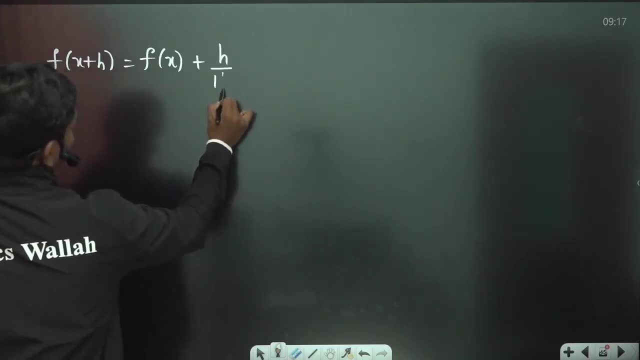 expression F of X plus H is equal to F. expression F of X plus H is equal to F of X plus H. by 1 factorial into F dash of of X plus H. by 1 factorial into F dash of of X plus H. by 1 factorial into F dash of X plus H. square by 2 factorial into F. 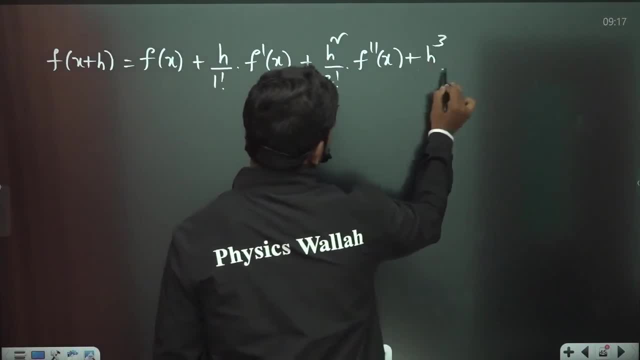 X plus H square by 2 factorial into F. X plus H square by 2 factorial into F. double dash of X H cube by 3, factorial. double dash of X. H cube by 3 factorial. double dash of X H cube by 3 factorial into F. table dash of X and so on. 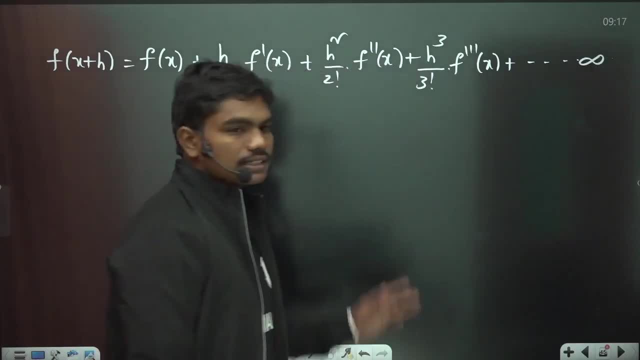 into F table dash of X and so on, into F table dash of X, and so on. basically okay though this goes to. basically okay, though this goes to. basically okay though this goes to infinity. actually so this X, this infinity. actually so this X, this infinity. actually so this X, this expression, and previously at X is equal. 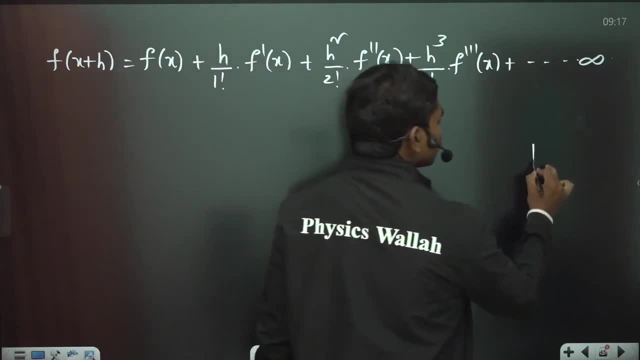 expression and previously at X is equal expression and previously at X is equal to a expression. both are same because to a expression. both are same because to a expression. both are same because, you have seen, H is nothing but X minus. you have seen H is nothing but X minus. 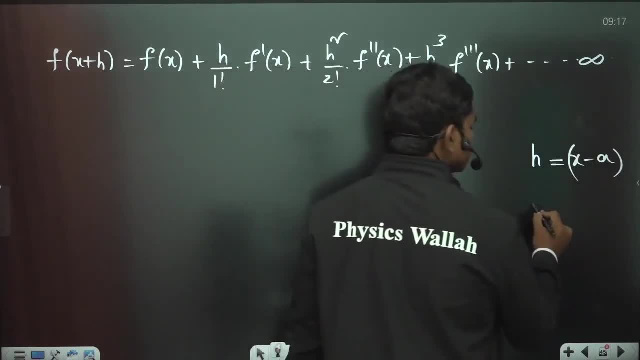 you have seen, H is nothing but X minus a cut. we have seen if you write X minus a cut. we have seen if you write X minus a cut. we have seen: if you write X minus here tends to 0, which means X tends to A, here tends to 0, which means X tends to A. 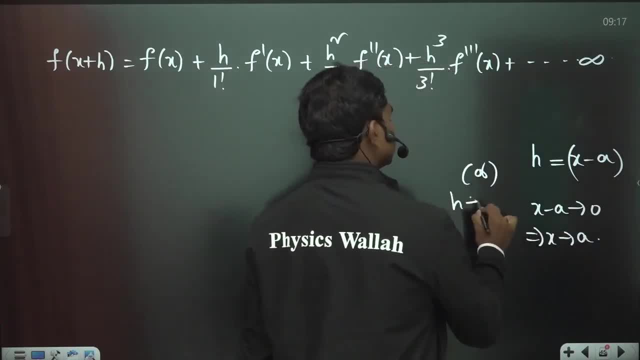 here tends to 0, which means X tends to A, or if you write H tends to 0, both this, or if you write H tends to 0, both this or if you write H tends to 0, both this are actually same that we have seen. 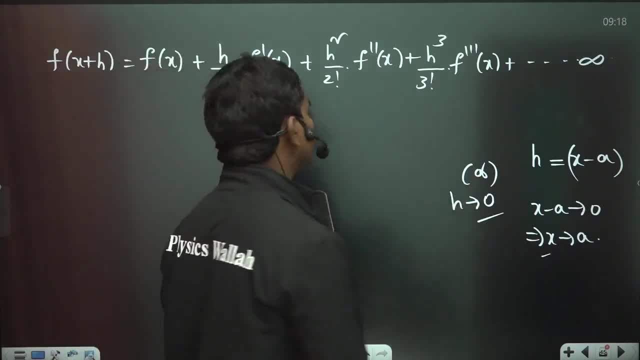 are actually same, that we have seen, are actually same, that we have seen during the first principle of, during the first principle of, during the first principle of differentiation, and all both these are differentiation and all both these are differentiation and all both these are actually identical. so, if you see in 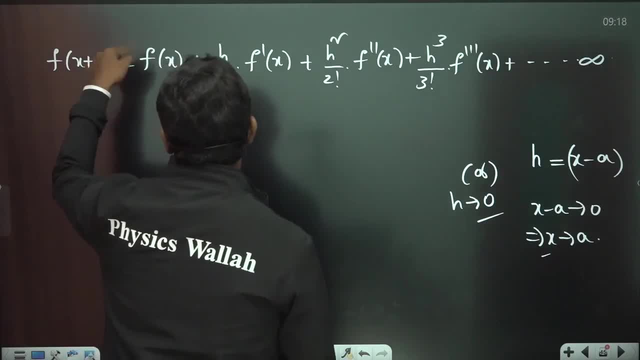 actually identical. so if you see in actually identical. so if you see in place of X plus H, if you keep, since H is place of X plus H, if you keep since H is place of X plus H, if you keep, since H is very small, you can neglect it to 0. so 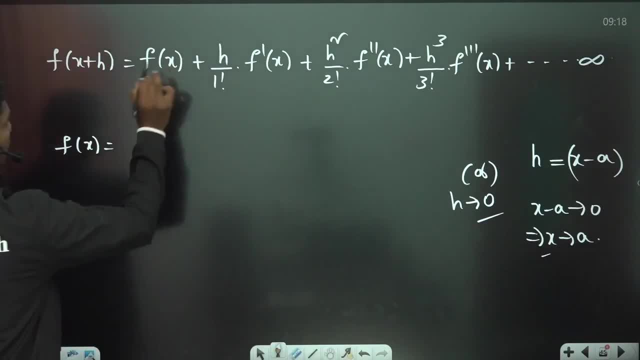 very small. you can neglect it to 0. so very small, you can neglect it to 0. so you like, f of X is equal to this, as X is. you like, f of X is equal to this, as X is. you like, f of X is equal to this, as X is tending to a. you can replace this X with. 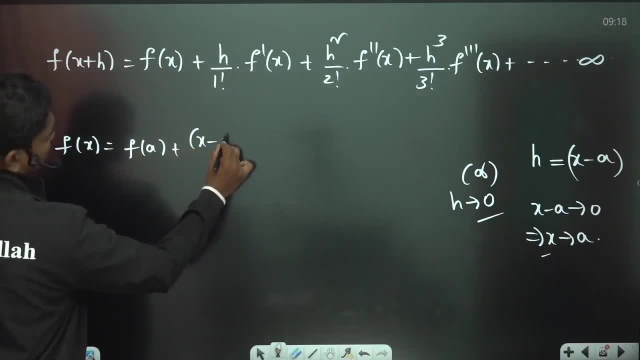 tending to a. you can replace this X with tending to a. you can replace this X with a plus H X minus a by 1 factorial into a plus H X minus a by 1 factorial into a plus H X minus a by 1 factorial into since X, and you are very close to each. 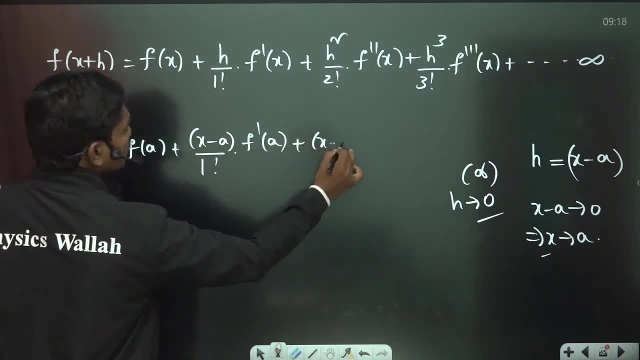 since X, and you are very close to each. since X, and you are very close to each other. you can replace this with F dash of other. you can replace this with F dash of other. you can replace this with F dash of a. all these things, okay, basically X. 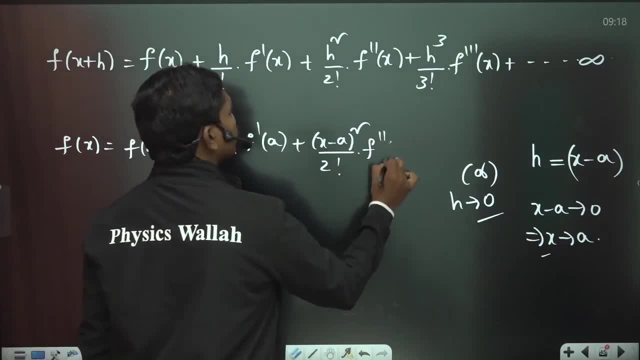 a all these things. okay, basically X a all these things. okay, basically X minus a whole square by 2 factorial into minus a whole square by 2 factorial, into minus a whole square by 2 factorial, into F double dash of a. so all these things, F double dash of a. so all these things. 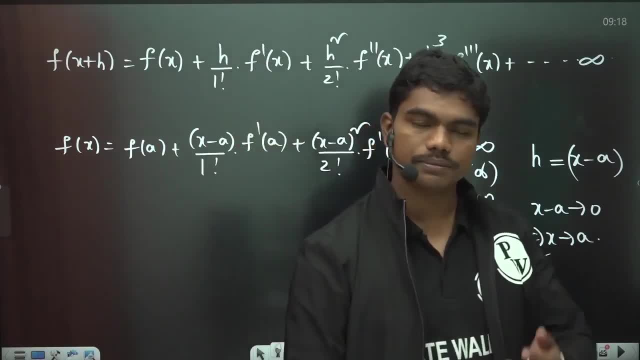 F, double dash of a. so all these things are basically identical again, okay. so are basically identical again, okay. so are basically identical again, okay. so that's how in Taylor says we talk some. that's how in Taylor says we talk some. that's how in Taylor says we talk some good points about the C's and how the 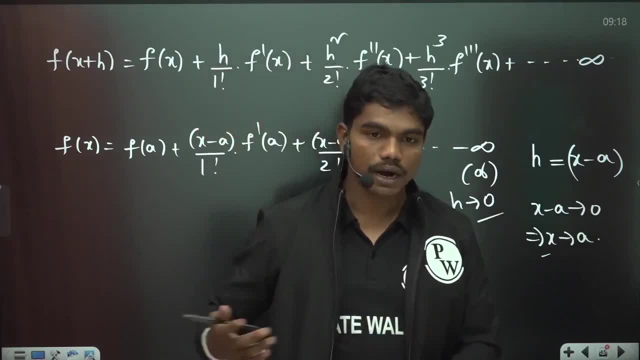 good points about the C's and how the good points about the C's and how the functional values are defined, basically functional values are defined. basically functional values are defined, basically okay, so this is one very important part. okay, so this is one very important part, okay, so this is one very important part of this basic calculus and differential. 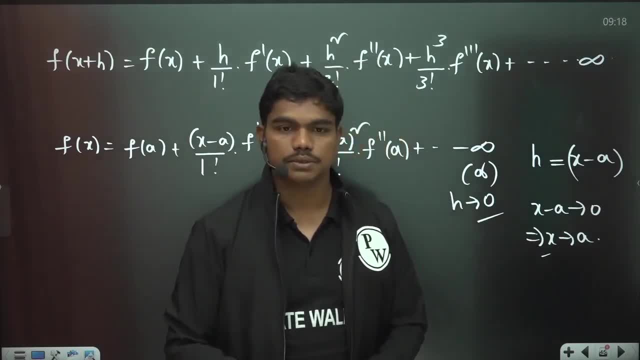 of this basic calculus and differential of this basic calculus and differential calculus actually. so with this we calculus actually. so with this we calculus actually. so with this we conclude this Taylor says part okay. so in conclude this Taylor says part okay. so in conclude this Taylor says part okay. so in Taylor says: if you quickly collect, we. 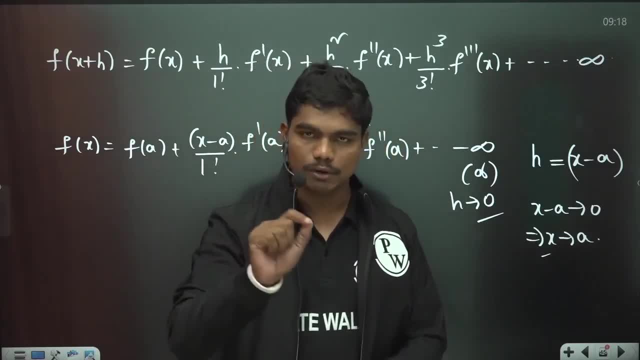 Taylor says: if you quickly collect. we, Taylor says: if you quickly collect. we have talked about what is the generalized, have talked about what is the generalized, have talked about what is the generalized expression of any expansion, about a expression of any expansion, about a expression of any expansion about a particular point a, and also we have 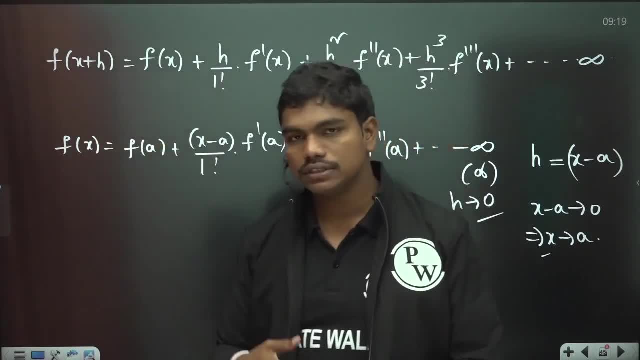 particular point a and also we have particular point a and also we have talked about the most much generalized, talked about the most much generalized, talked about the most much generalized expression. so we have generated what is expression, so we have generated what is expression. so we have generated what is the Taylor says expansion for sine X. then the Taylor says expansion for sine X, then the Taylor says expansion for sine X. then we have seen what are the Taylor C's. we have seen what are the Taylor C's. we have seen what are the Taylor C's, expansions for cos X e, power X, all these 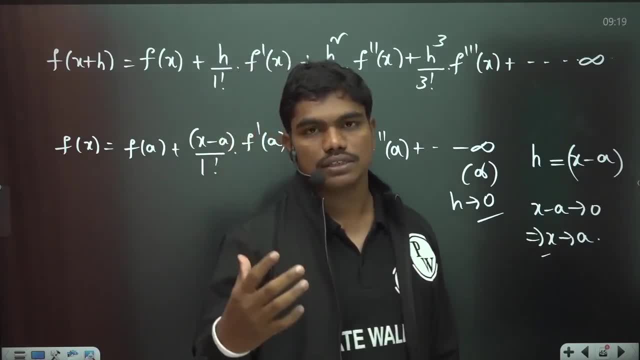 expansions for cos X e power X, all these expansions for cos X e power X, all these things we have understood what is linear things. we have understood what is linear things. we have understood what is linear approximation and what are the approximation and what are the approximation and what are the coefficients of X minus a whole power n. 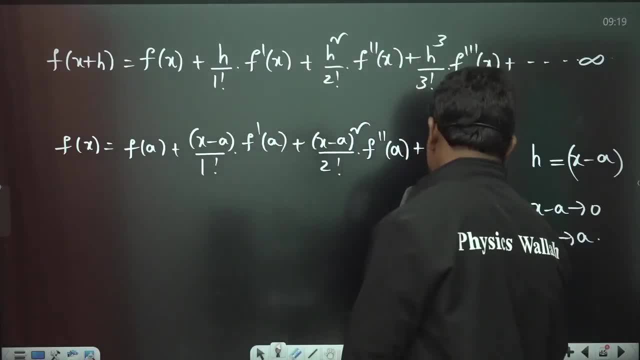 coefficients of X minus a whole power n. coefficients of X minus a whole power n. terms: all these things we have you know terms, all these things we have you know terms, all these things we have you know. observed here: okay, so with this. observed here: okay, so with this. 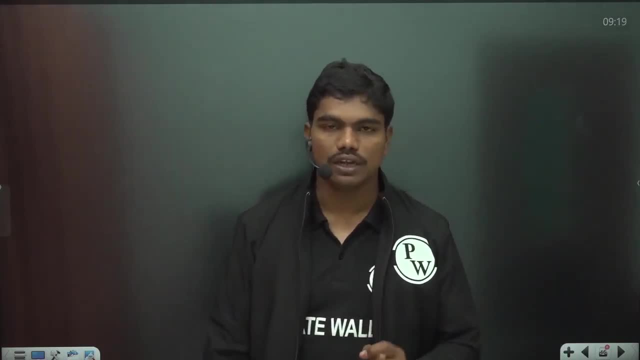 observed here. okay, so, with this understanding, let's move to one last part understanding. let's move to one last part understanding, let's move to one last part of this differential calculus concept, of this differential calculus concept, of this differential calculus concept of maxima and minima. so let us write this: 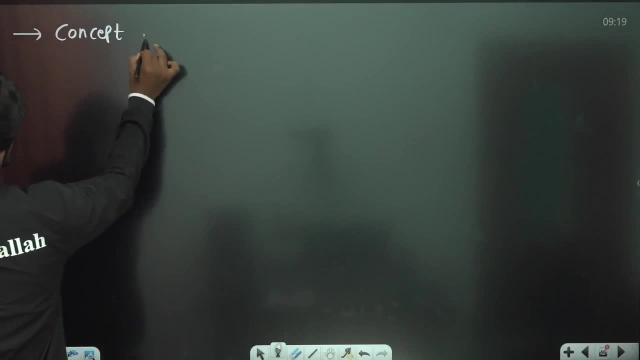 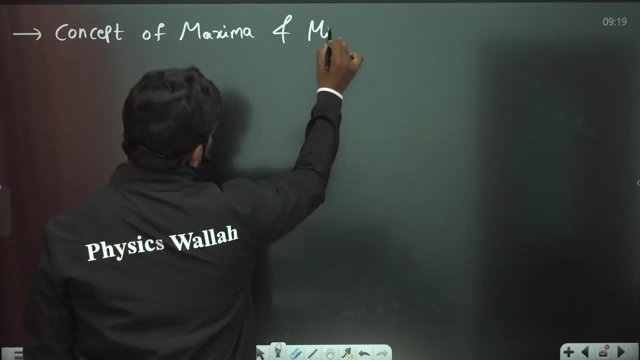 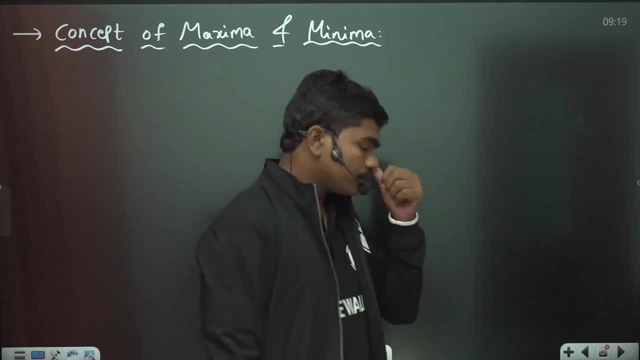 concept of maxima and minima. concept of maxima and minima. concept of maxima and minima. so let us suppose if I concept of maxima and minima. so let us suppose if I concept of maxima and minima. so let us suppose if I give you some function f of X, how will you? 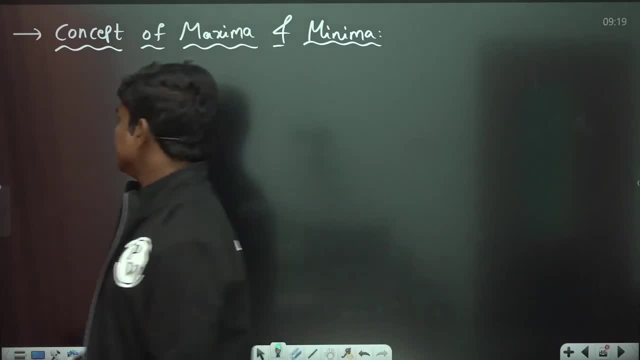 give you some function f of X. how will you give you some function f of X? how will you find the maximum and minimum values? find the maximum and minimum values. find the maximum and minimum values of that. okay, so let us see if f of X is a function, is a. 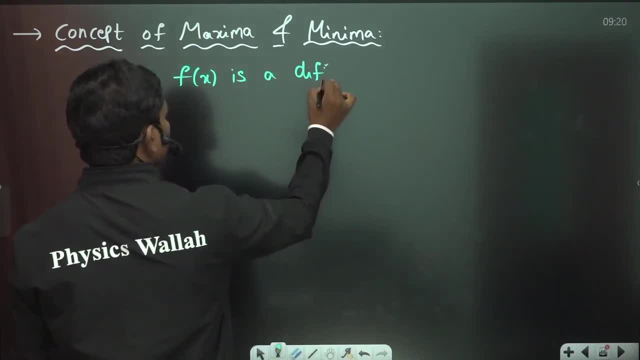 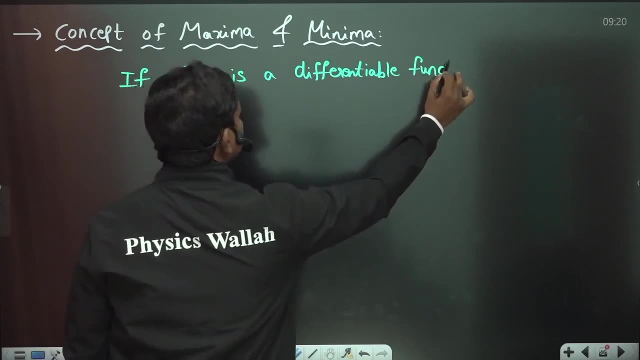 f of X is a function, is a f of X is a function, is a differentiable function, differentiable function. differentiable function is: is: is a differentiable, a differentiable, a differentiable function. if f of X is a differentiable function. if f of X is a differentiable function. 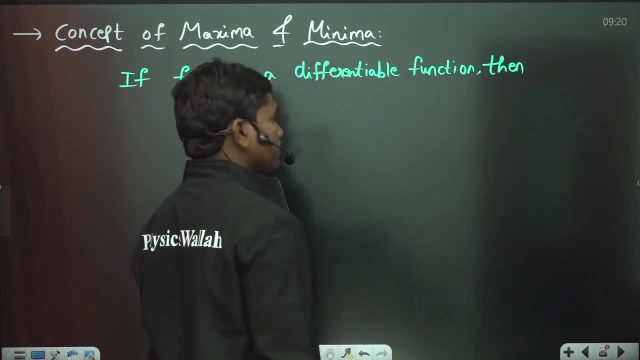 if f of X is a differentiable function, then then then to calculate maxima and minima. I'm giving to calculate maxima and minima. I'm giving to calculate maxima and minima. I'm giving you the working procedure then to you, the working procedure then to: 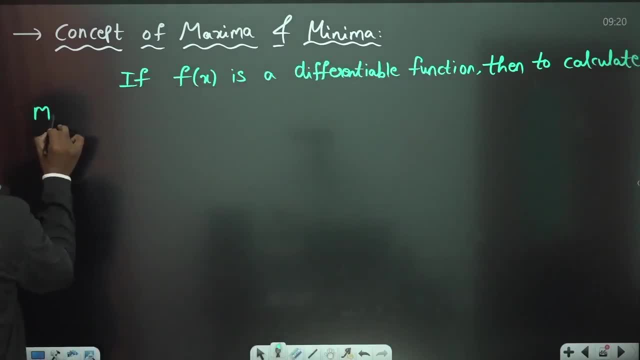 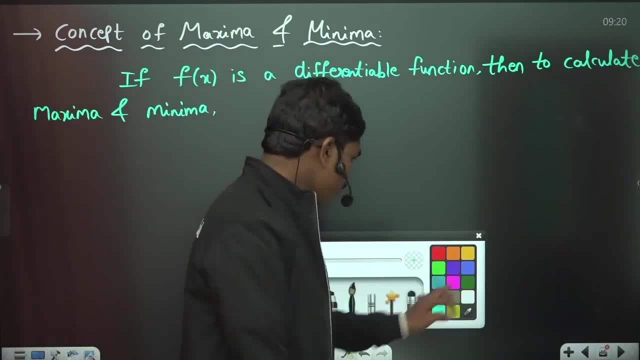 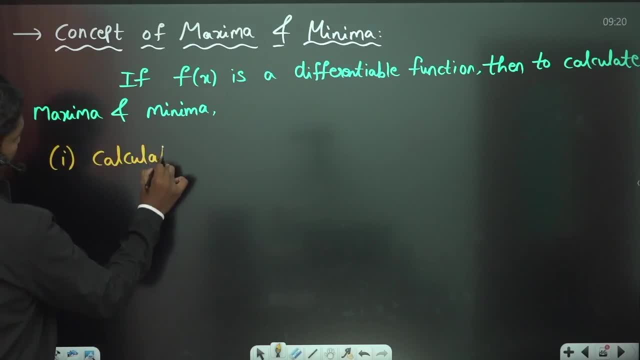 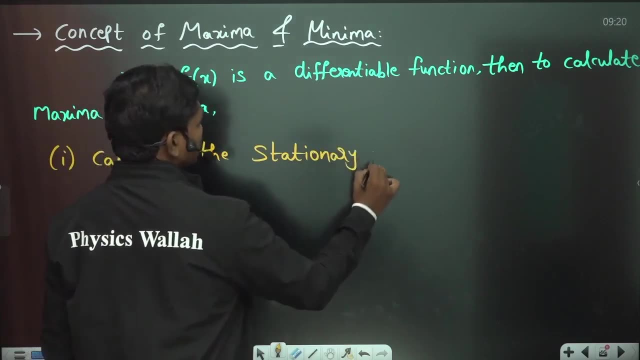 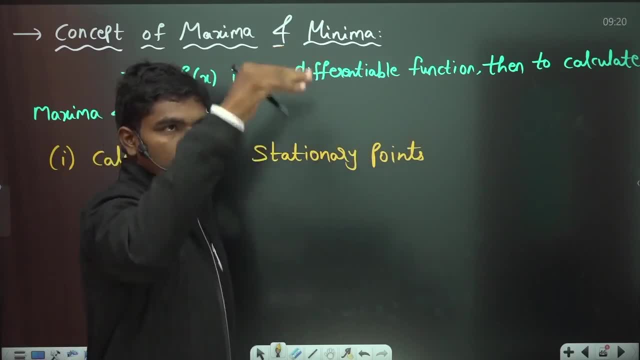 what are stationary points basically? what are stationary points? basically the points where the function stops, like the points where the function stops, like the points where the function stops like it takes a maximum pause and it, it takes a maximum pause and it it takes a maximum pause and it generally decreases for a while. okay, so, 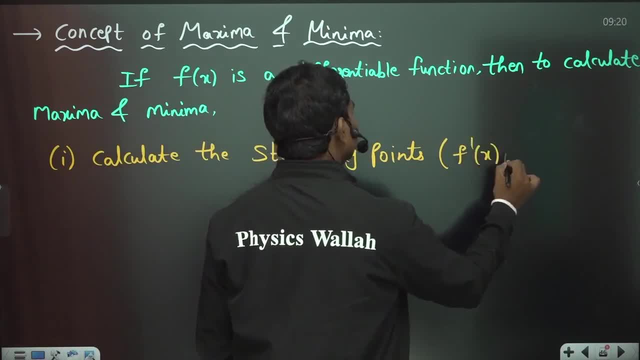 generally decreases for a while. okay. so generally decreases for a while. okay. so stationary points, which means you should stationary points, which means you should stationary points, which means you should calculate these points where f dash of X. calculate these points, where f dash of X calculate these points, where f dash of X is equal to zero. so how many points you? is equal to zero, so how many points you is equal to zero, so how many points you will get? that depends upon the function will get. that depends upon the function will get. that depends upon the function because, for example, let us suppose if I. because, for example, let us suppose if I. 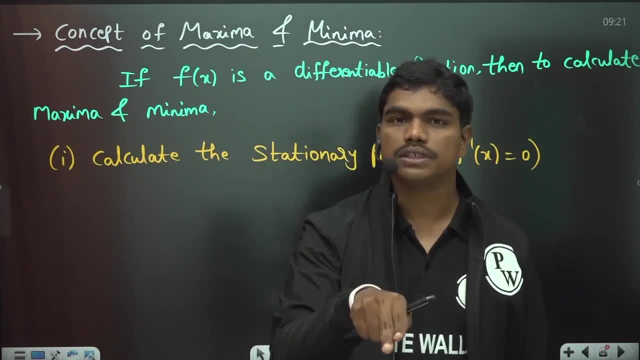 because, for example, let us suppose, if I give you a cubic equation, then when you give you a cubic equation, then when you give you a cubic equation, then when you differentiate it, you will get a differentiate it, you will get a differentiate it, you will get a quadratic equation. correct, when you? quadratic equation correct when you quadratic equation correct. when you create a quadratic equation to zero, you create a quadratic equation to zero. you create a quadratic equation to zero. you will get toots, but let us suppose if we will get toots. but let us suppose if we. 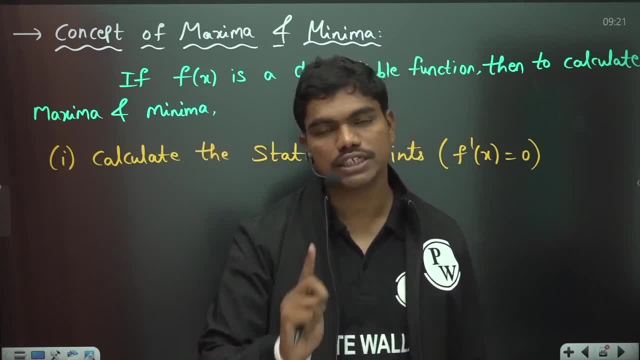 will get toots. but let us suppose: if we give you quadratic equation, and if you give you quadratic equation, and if you give you quadratic equation, and if you differentiate it, you will get linear, differentiate it, you will get linear, differentiate it, you will get linear equation. you have only one stationary. 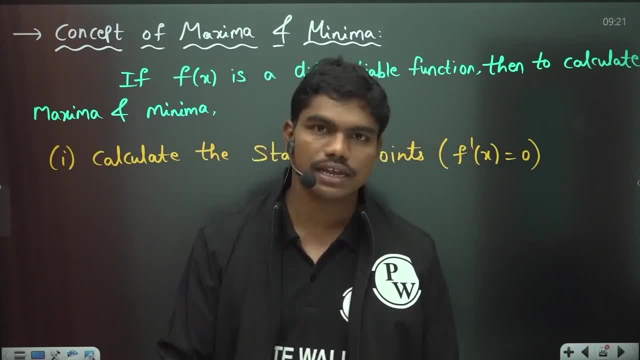 equation. you have only one stationary equation, you have only one stationary point. so number of stationary points: point. so number of stationary points, point. so number of stationary points depend upon the type of function that I depend upon, the type of function that I depend upon, the type of function that I give you. so I'll show you the procedure. 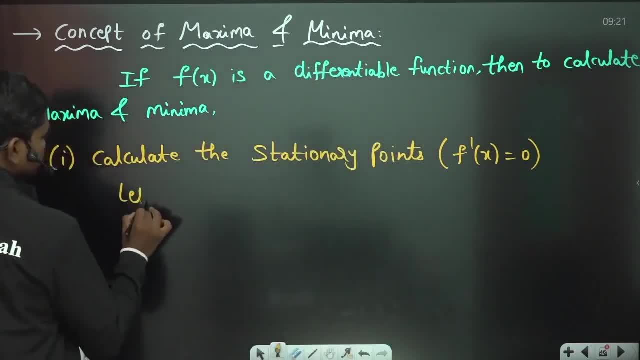 give you, so I'll show you the procedure. give you, so I'll show you the procedure for one stationary point. okay, so, when you for one stationary point, okay. so, when you for one stationary point, okay. so when you have done this, let X naught be a. 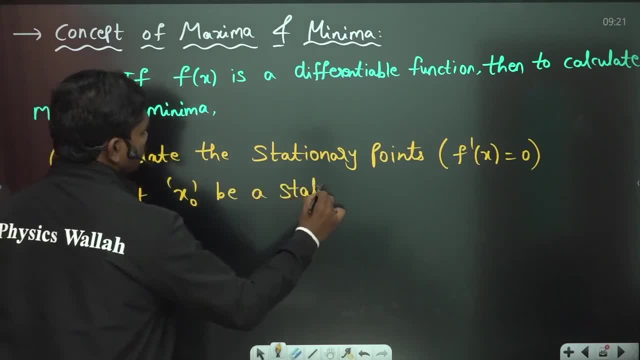 have done this, let X naught be a. have done this. let X naught be a stationary point, for example. okay, let X stationary point, for example. okay, let X stationary point, for example. okay, let X naught be a stationary point if X naught naught be a stationary point. if X naught. 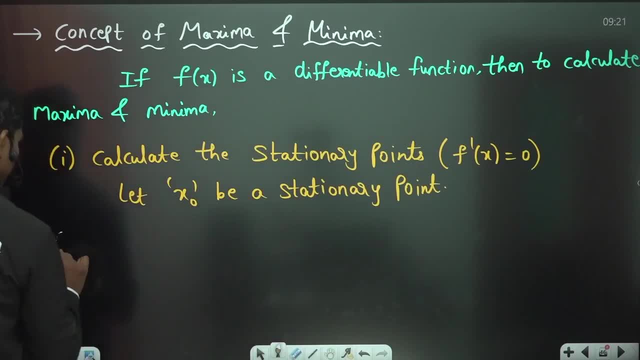 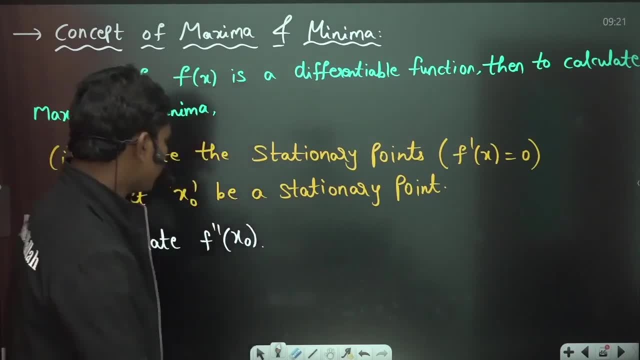 means you need to calculate, means you need to calculate the second derivative value at this, the second derivative value at this, the second derivative value at this stationary point. so once you calculate stationary point, so once you calculate stationary point, so once you calculate this, yay, if F double dash of X naught is: 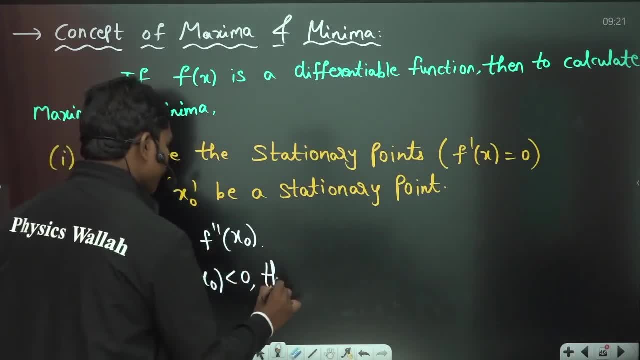 this: yay. if F double dash of X naught, is this: yay. if F double dash of X naught is less than 0, then F of X has less than 0, then F of X has less than 0, then F of X has maximum maximum. 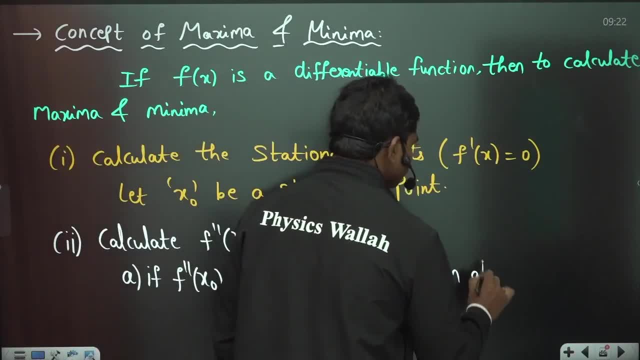 maximum F of X. has maximum at X is equal to F of X. has maximum at X is equal to F of X. has maximum at X is equal to. yay, so X is equal to X, naught and maximum. yay, so X is equal to X, naught and maximum. 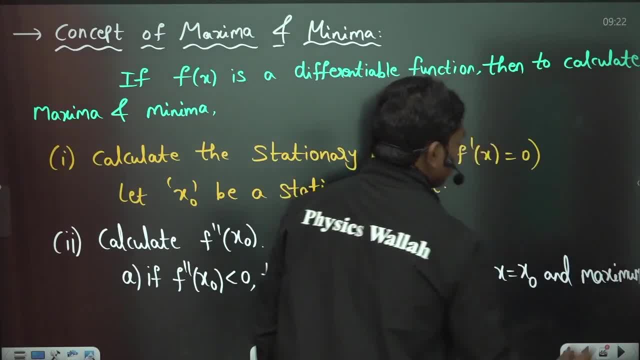 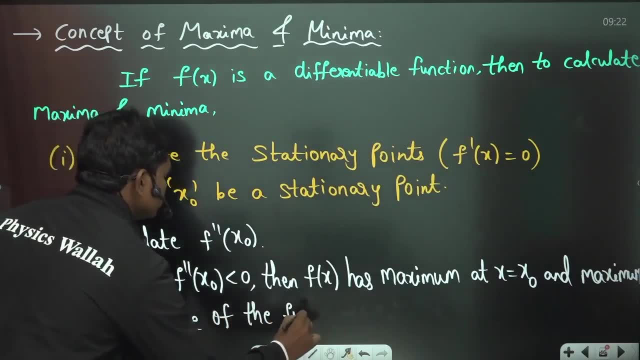 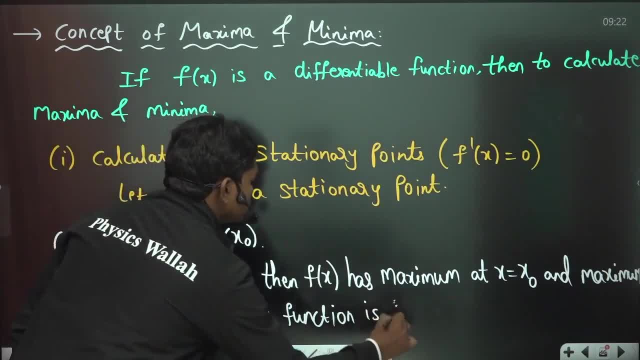 value of the function. maximum value of the function is function is, function is, is F, is F, is F. of X- naught, actually okay now. similarly of X naught, actually okay now. similarly of X- naught, actually okay now. similarly, why this is coming look, I'll, okay, I'll. 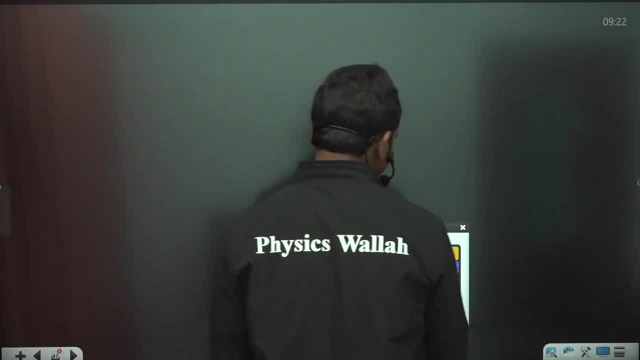 why this is coming. look, I'll, okay, I'll. why this is coming. look, I'll, okay, I'll spend some time and I'll tell you: look, spend some time. and I'll tell you: look, spend some time. and I'll tell you: look, let us suppose you have a function like: 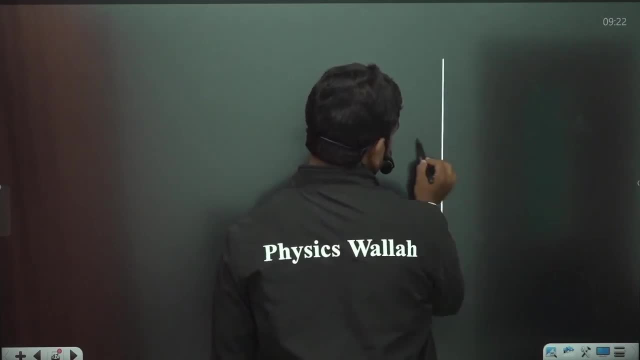 let us suppose you have a function like. let us suppose you have a function like this: okay, so this is some function and I'm okay. so this is some function and I'm okay. so this is some function and I'm intense. this is the graph. actually why? 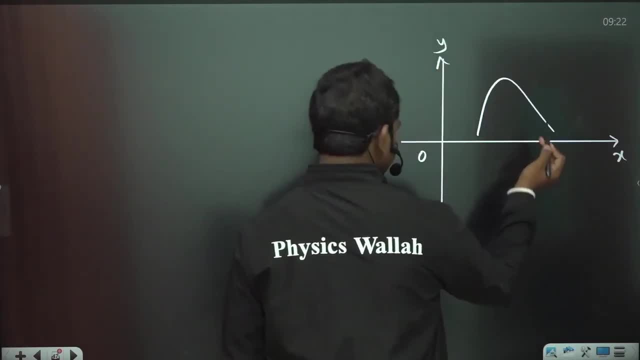 intense? this is the graph actually. why intense? this is the graph actually, why- and let us suppose I have taken some and let us suppose I have taken some and let us suppose I have taken some- function like this intentionally. I am function like this intentionally. I am function like this intentionally. I am taking maximum because I want to show. 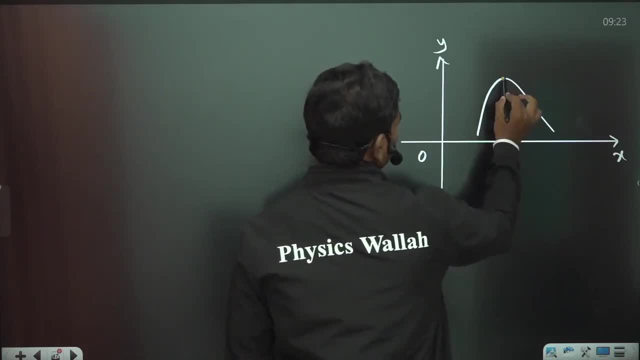 taking maximum, because I want to show taking maximum, because I want to show you the first point. so now this is the you, the first point. so now this is the you, the first point. so now this is the point at which you have a maximum of point, at which you have a maximum of. 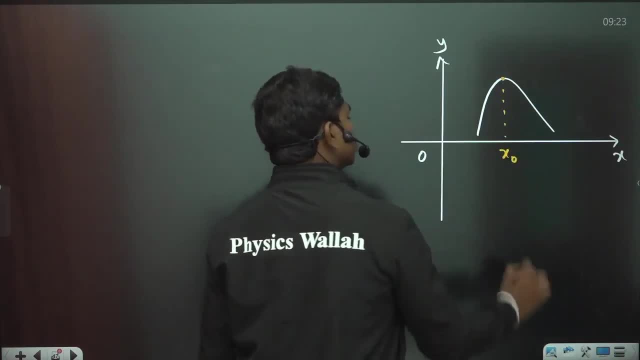 point at which you have a maximum, of course now. why the second derivative? at course now. why the second derivative, at course now. why the second derivative at this point should be negative? that's the this point should be negative. that's the this point should be negative. that's the question correct? of course there's no. 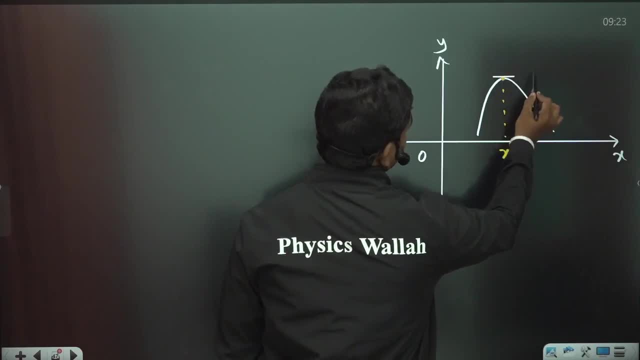 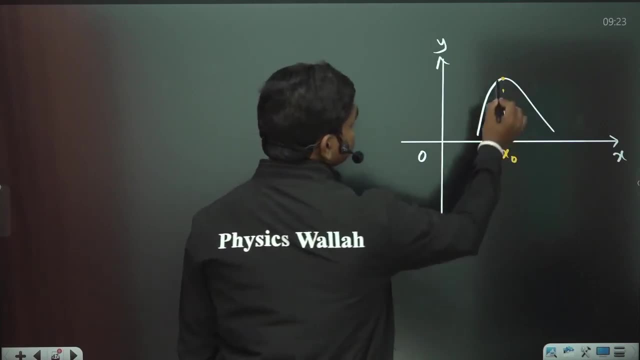 question correct? of course, there's no question, correct? of course there's no point. so you have a zero slope tangent point. so you have a zero slope tangent point. so you have a zero slope tangent. just a minute. you have a zero slope, just a minute. you have a zero slope tangent. that's okay. now why the second? 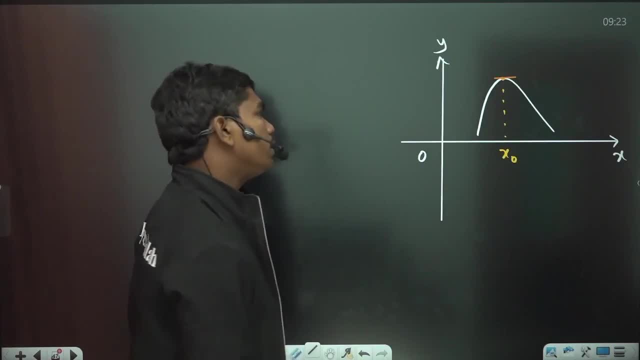 tangent. that's okay. now why the second tangent? that's okay. now why the second derivative has to be negative at this derivative, has to be negative at this derivative, has to be negative at this location. that's the important question. location, that's the important question. location, that's the important question. see secondary derivative if you want to. 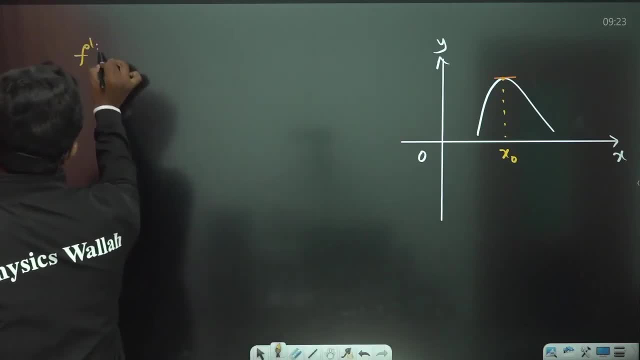 see secondary derivative. if you want to see secondary derivative, if you want to talk about secondary derivative means, if talk about secondary derivative means, if talk about secondary derivative means, if I calculate F double dash of X naught, I calculate F double dash of X naught. I calculate F double dash of X naught, which is differentiation of. 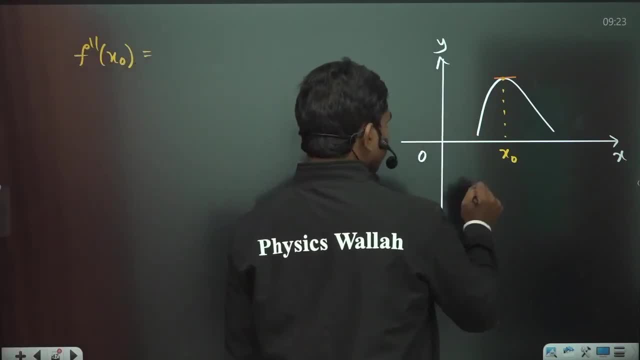 which is differentiation of, which is differentiation of differentiation? can I do it like this differentiation? can I do it like this differentiation? can I do it like this? let us suppose I am taking one point here. let us suppose I am taking one point here. let us suppose I am taking one point here. say X 2 and one more point here: X 1, for. 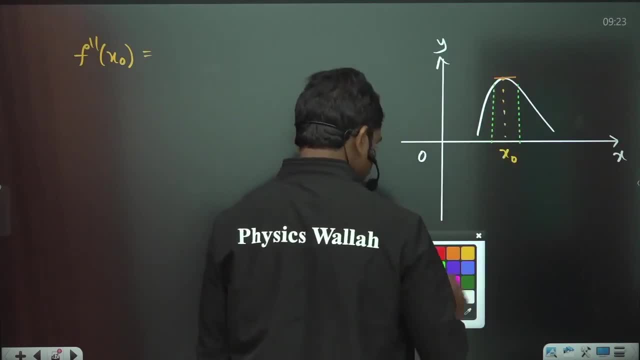 say X 2, and one more point here: X 1 for say X 2, and one more point here: X 1, for example. so this point is example, so this point is example. so this point is X 1 and this point is X 2, for example. so 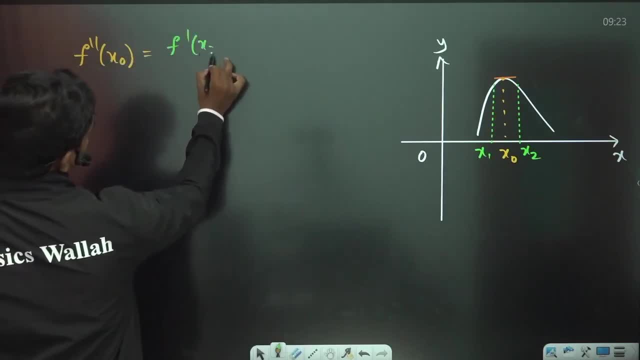 X 1 and this point is X 2, for example. so X 1 and this point is X 2, for example. so can I write this as F dash of X 2 minus? can I write this as F dash of X 2 minus? can I write this as F dash of X 2 minus? F dash of X 1 by X 2 minus X 1? can I write? F dash of X 1 by X 2 minus X 1. can I write: F dash of X, 1 by X 2 minus X 1. can I write it like this? so I can write it like it like this: so I can write it like this: 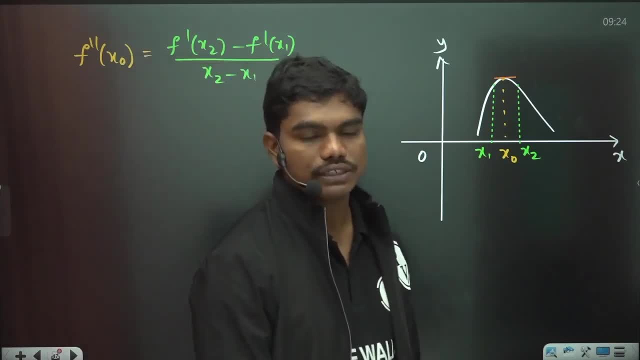 it like this. so I can write it like this, because normally, if there is only because normally, if there is only because normally, if there is only single derivative, you take the functional single derivative, you take the functional single derivative, you take the functional values difference with respect to X, but 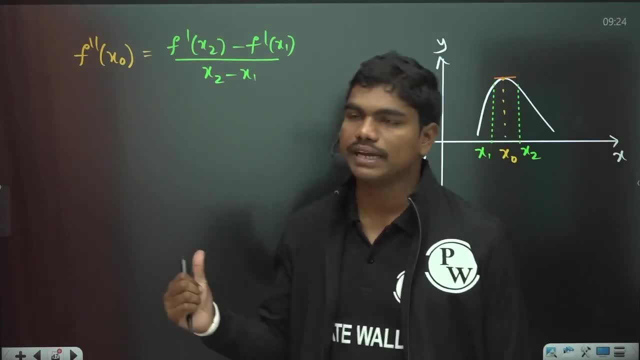 values difference with respect to X, but values difference with respect to X. but if it's second derivative, you take the. if it's second derivative, you take the. if it's second derivative, you take the difference of the derivatives with difference of the derivatives, with difference of the derivatives with respect to X. okay, so now you can observe. 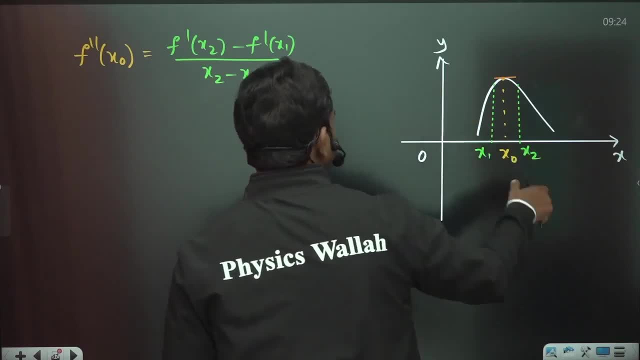 respect to X. okay, so now you can observe respect to X. okay, so now you can observe one thing. let us suppose if I draw a one thing. let us suppose if I draw a one thing. let us suppose if I draw a tangent at this location X 2. 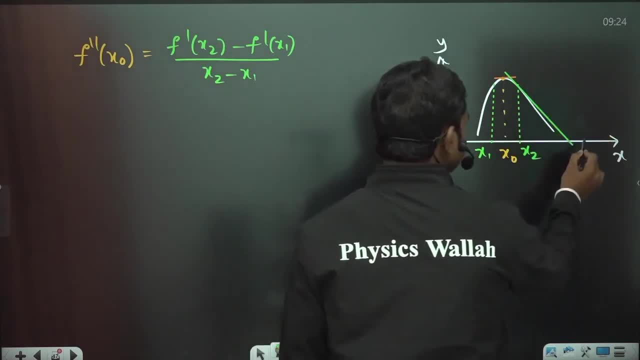 tangent at this location X 2, tangent at this location X 2, then this is how my tangent comes over. then this is how my tangent comes over. and if you see this angle, theta 2- if I, and if you see this angle, theta 2, if I. 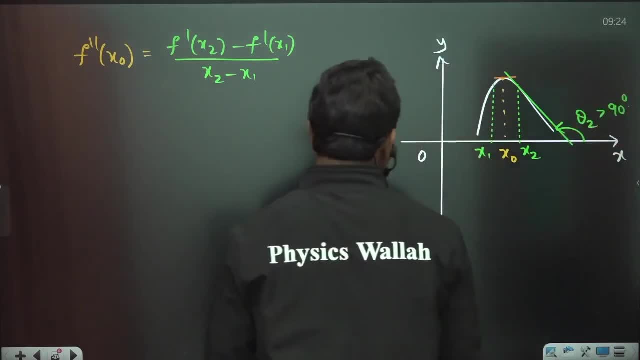 and if you see this angle, theta 2. if I call this is greater than 90. similarly, call this is greater than 90. similarly, call this is greater than 90. similarly, if I die tangent at location 1 for, if I die tangent at location 1 for 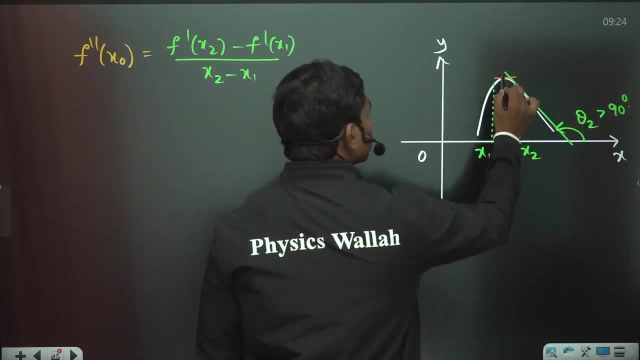 if I die tangent at location 1, for example say at this location, let me example say: at this location. let me example say: at this location, let me change the color so at location 1. if I change the color so at location 1, if I change the color so at location 1, if I die a tangent like this: 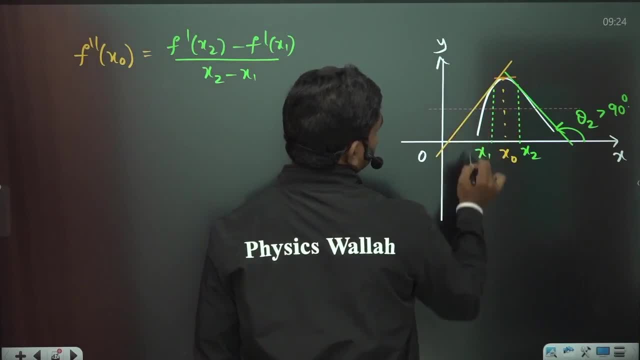 die a tangent like this, die a tangent like this. if I die a tangent like this at this, if I die a tangent like this at this, if I die a tangent like this at this location, then this value is theta 1 location, then this value is theta 1. 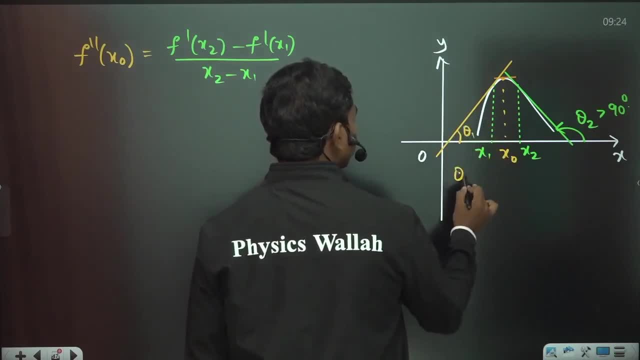 location, then this value is theta 1. this is theta 1- okay, and theta 1 is less. this is theta 1- okay, and theta 1 is less. this is theta 1- okay, and theta 1 is less than 90. now tell me one thing: if theta 1 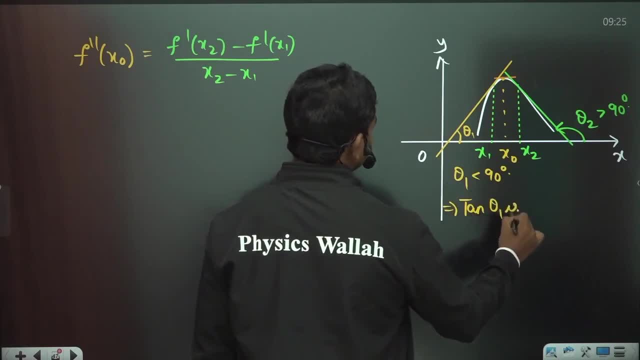 than 90. now tell me one thing. if theta 1 than 90, now tell me one thing. if theta 1 is less than 90 tan theta 1 is positive. is less than 90. tan theta 1 is positive. is less than 90. tan theta 1 is positive, yes or no? and what is tan theta 1? 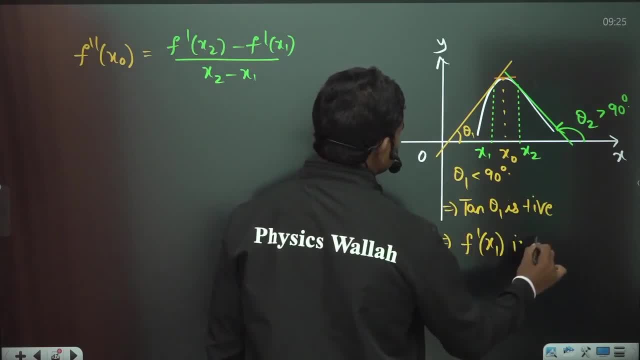 yes or no? and what is tan theta 1? yes or no? and what is tan theta 1? nothing but F? dash of X 1 is positive. nothing but F? dash of X? 1 is positive. nothing but F? dash of X 1 is positive. similarly here, if you consider theta 2, 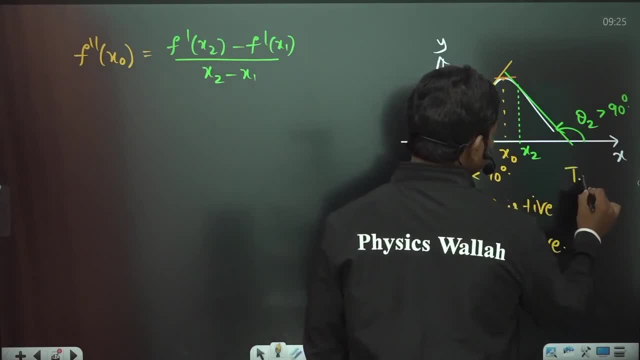 similarly here if you consider theta 2. similarly here, if you consider theta 2 is negative, that means tan theta 2 is 9 is negative. that means tan theta 2 is 9 is negative. that means tan theta 2 is 9 greater than 90, which means tan theta 2. 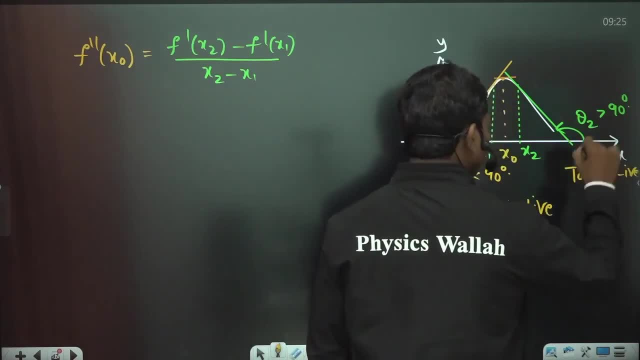 greater than 90, which means tan theta 2, greater than 90, which means tan theta 2, is negative. okay, so this is negative is negative. okay, so this is negative is negative. okay, so this is negative because it falls in second quadrant. so, because it falls in second quadrant. so 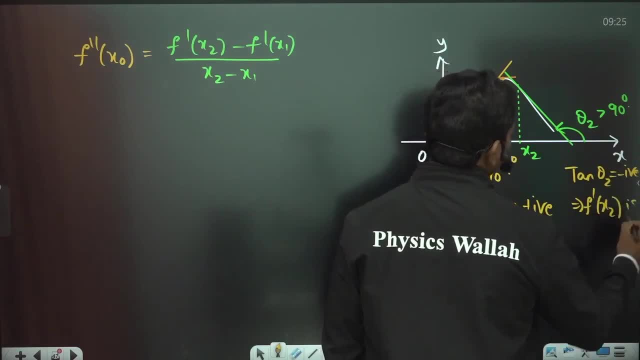 because it falls in second quadrant. so this means F dash of X 2 is negative. I this means F dash of X 2 is negative. I this means F dash of X 2 is negative. I have shown you for this case of maximum. have shown you for this case of maximum. 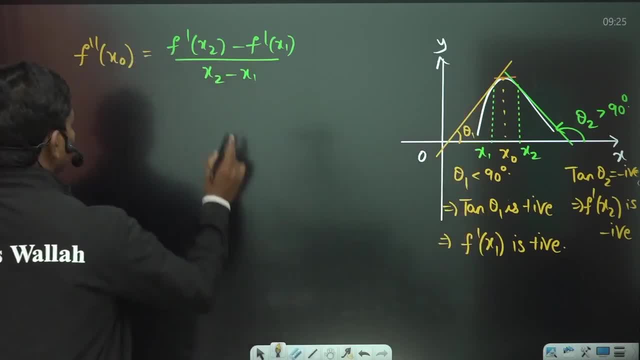 have shown you for this case of maximum: okay, if you have taken the case of: okay, if you have taken the case of: okay, if you have taken the case of minimum results would have been something. minimum results would have been something. minimum results would have been something different. okay, so if you see F dash of 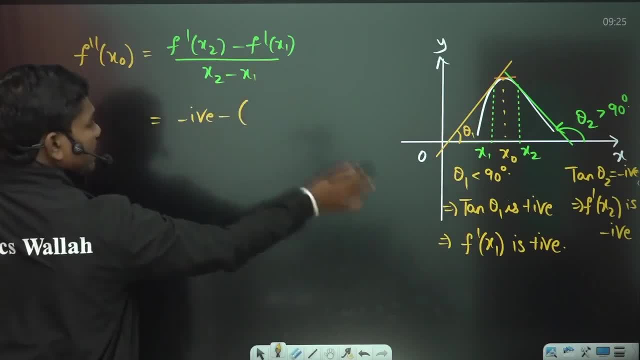 different. okay. so if you see F dash of different, okay. so if you see F dash of X 2 is negative minus F dash of X 1 is X 2 is negative. minus F dash of X 1 is X 2 is negative. minus F dash of X 1 is positive. divided by X 2 minus X 1, this 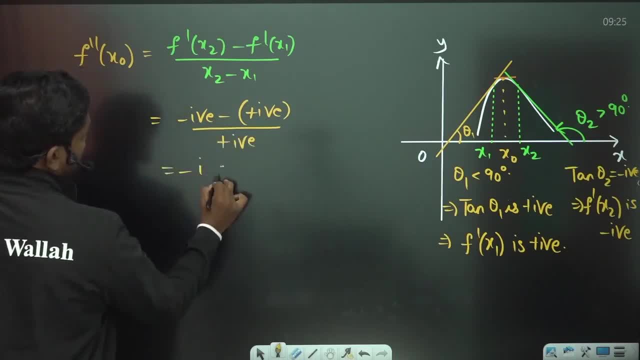 positive divided by X 2 minus X 1, this positive divided by X 2 minus X 1, this is positive. so you see, the total term is is positive. so you see the total term is is positive. so you see, the total term is negative. that's why, whenever you are, 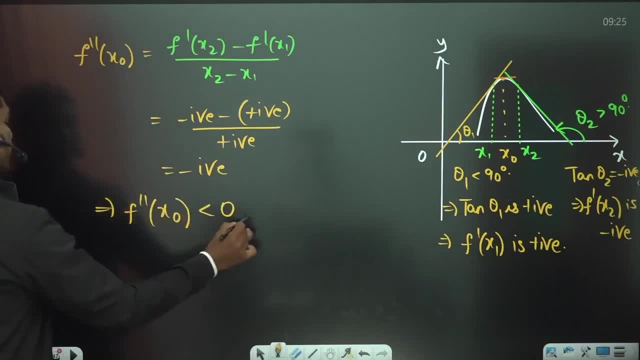 negative. that's why, whenever you are negative, that's why, whenever you are talking about maximum, this second, talking about maximum this second, talking about maximum this second- derivative should be negative clear. so derivative should be negative clear, so derivative should be negative clear. so this is one very important understanding. 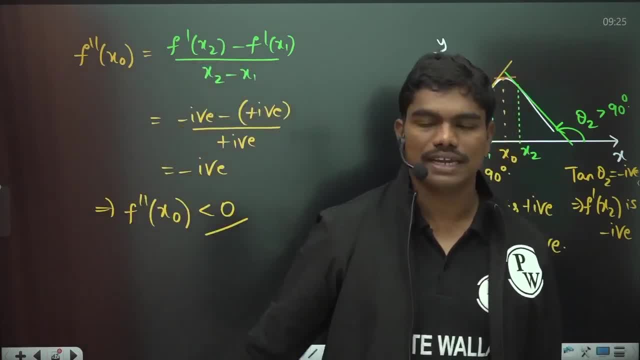 this is one very important understanding. this is one very important understanding and, of course, normally you generally, and of course, normally you generally, and of course, normally you generally don't find this explanation and all in don't find this explanation and all in don't find this explanation and all in books. but this is a very simple. 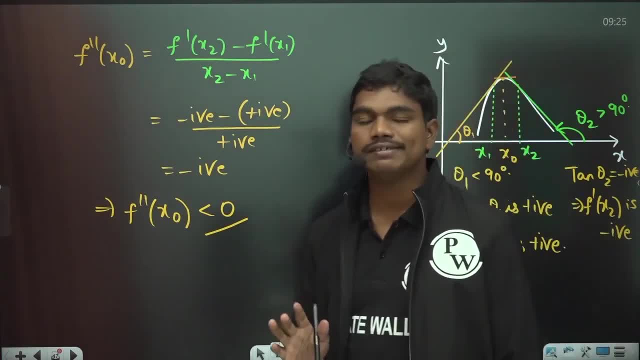 books, but this is a very simple books, but this is a very simple explanation actually that whenever you explanation actually, that whenever you explanation actually that whenever you are talking about maximum, your second are talking about maximum, your second are talking about maximum, your second derivative should be zero. this is the. 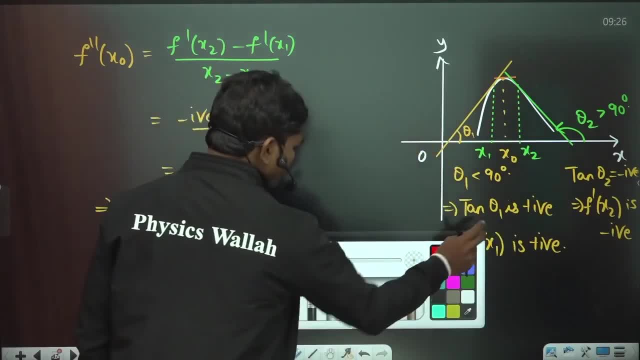 derivative should be zero. this is the derivative should be zero. this is the reason clear now, anyhow. so that's the reason clear now, anyhow. so that's the reason clear now, anyhow. so that's the first point now. second point B if F. first point now. second point B if F. first point. now second point B: if F double dash of X naught now this, I am not double dash of X- naught now this, I am not double dash of X naught now this, I am not going to explain with this diagram, and going to explain with this diagram and 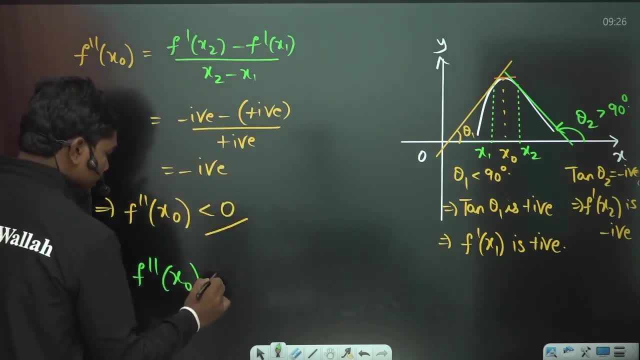 going to explain with this diagram: and all because it's a similar thing. so if F- all because it's a similar thing. so if F, all because it's a similar thing. so if F double dash of X naught is greater than double dash of X naught is greater than. 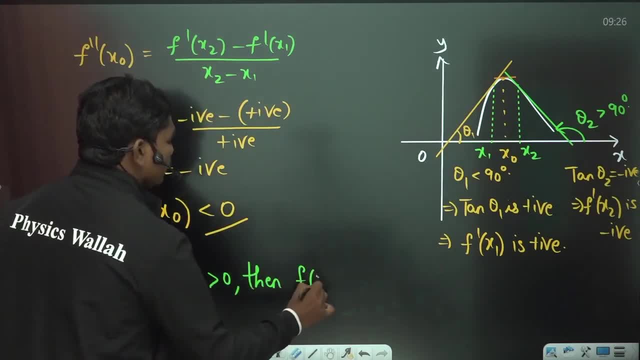 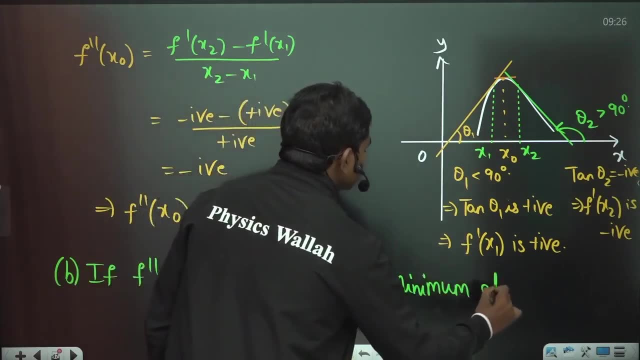 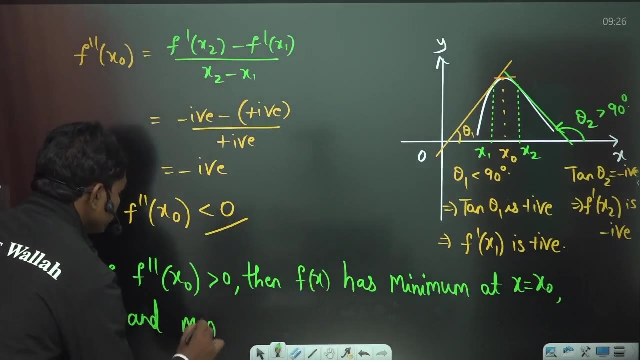 double dash of X: naught is greater than zero, then zero, then zero, then F of X has minimum minimum. minimum at X is equal to X. naught okay at X is at X is equal to X. naught okay at X is at X is equal to X. naught okay at X is equal to X naught. and minimum value is: 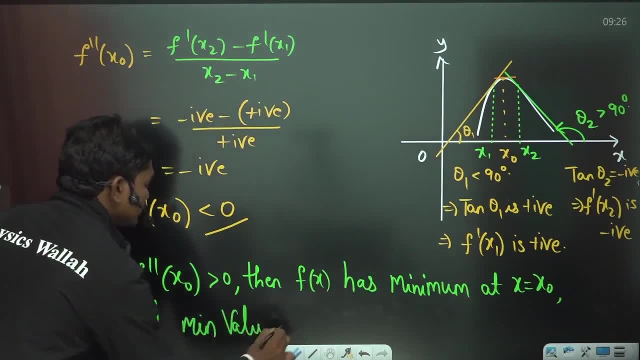 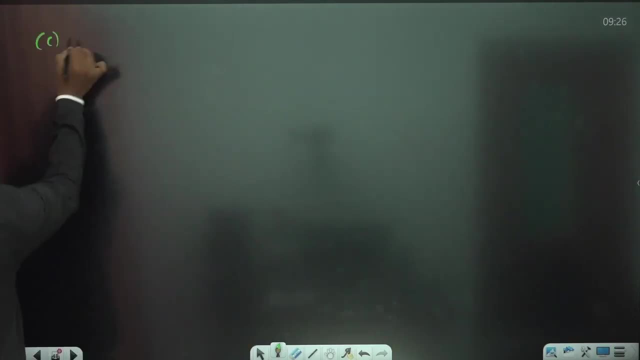 this is F of X naught, clear, so minimum. this is F of X naught, clear, so minimum. value is F of X naught, now last point C. value is F of X naught, now last point C. value is F of X naught, now last point C. if F double dash of X naught is equal, 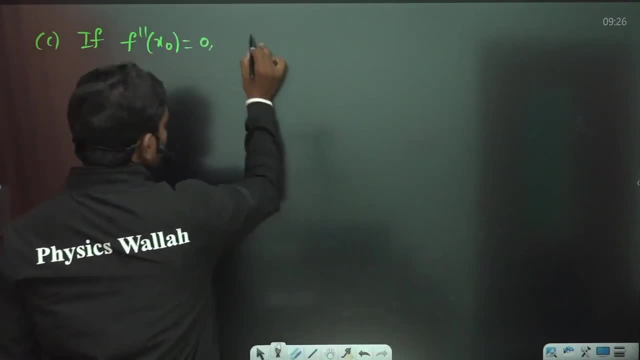 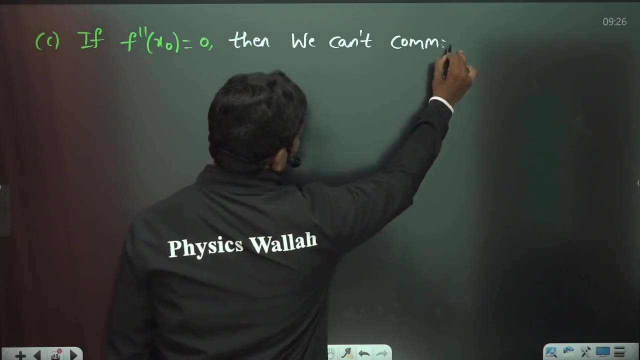 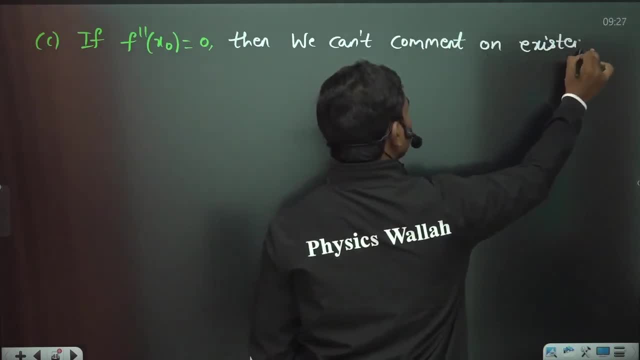 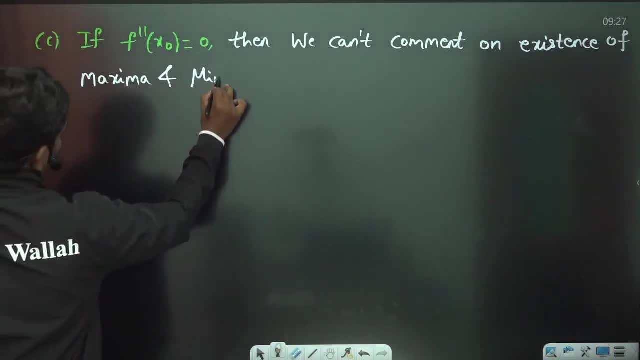 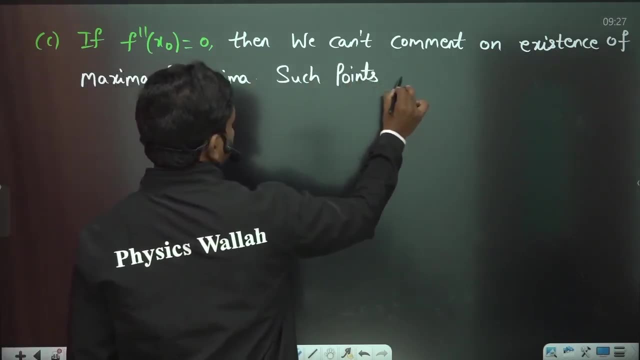 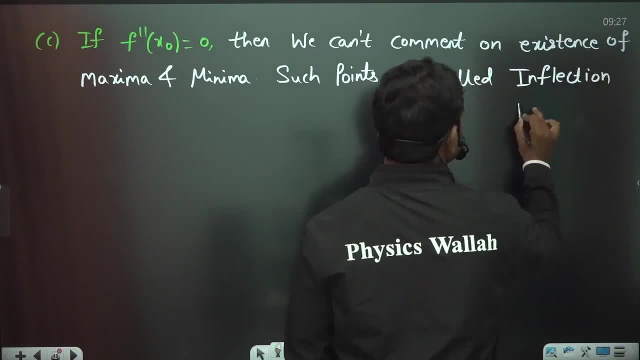 such points are called inflection points, such points are called inflection points, or sometimes they also called critical, or sometimes they also called critical, or sometimes they also called critical points. so inflection points, points, so inflection points, points, so inflection points, inflection points, or they're also called 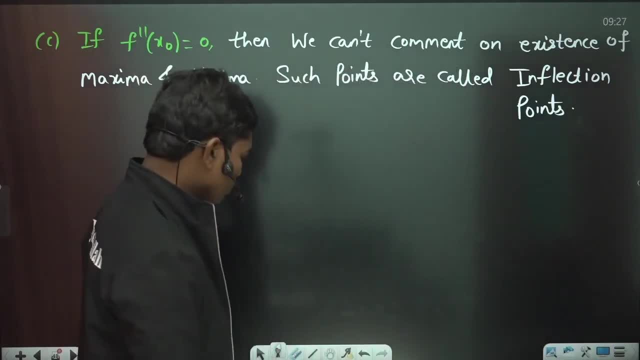 inflection points, or they're also called inflection points, or they're also called points of inflection, or sometimes they're points of inflection, or sometimes they're points of inflection. or sometimes they're also called critical points. also also called critical points. also also called critical points also. look why we can't comment on maxima and 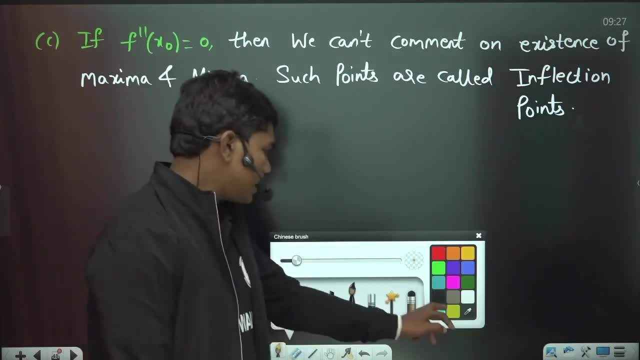 look why we can't comment on maxima. and look why we can't comment on maxima and minima, for example, if you see i'll give minima, for example. if you see i'll give minima, for example, if you see i'll give you two examples so that you'll get. 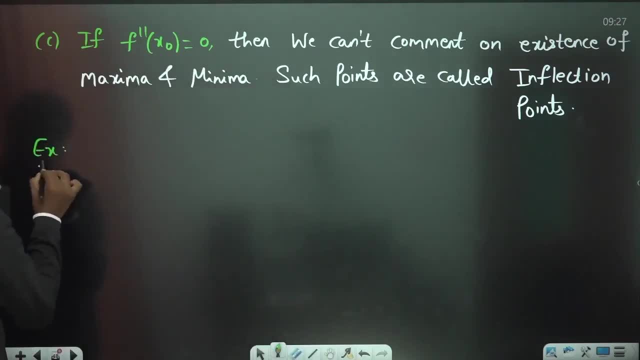 you two examples so that you'll get you two examples, so that you'll get it better. okay, so example x is equal to zero, is a point of x is equal to zero, is a point of x is equal to zero, is a point of inflection, inflection. 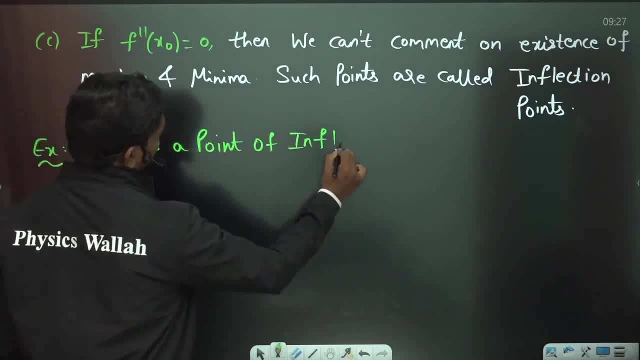 inflection is a point of inflection. x is equal to zero. is a point of x is equal to zero. is a point of x is equal to zero is a point of inflection. for f of x is equal to x cube. inflection for f of x is equal to x cube. 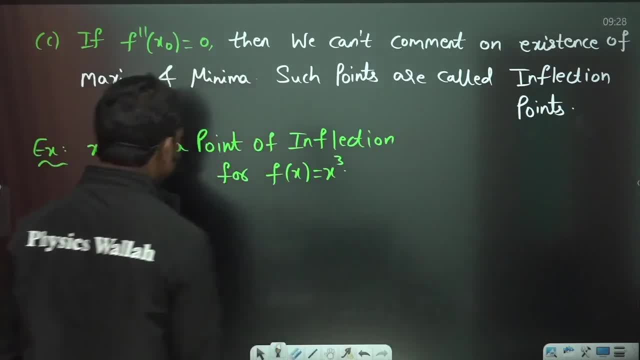 inflection, for f of x is equal to x cube. if you take this, f of x is equal to x. if you take this, f of x is equal to x. if you take this f of x is equal to x cube, then this implies f dash of x is. 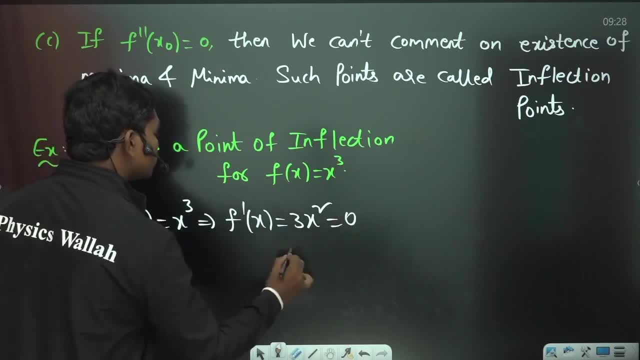 cube, then this implies f dash of x is cube, then this implies f dash of x is equal to t x square. so if you equate it equal to t x square, so if you equate it equal to t x square, so if you equate it to zero, your stationary point is x is. 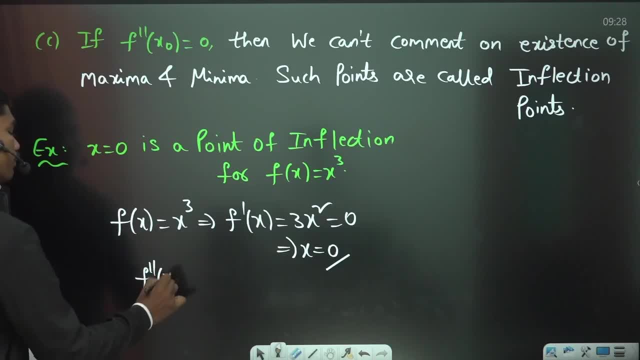 to zero. your stationary point is: x is to zero. your stationary point is: x is equal to zero. now, what about f double equal to zero now? what about f double equal to zero now? what about f double dash of x? naught, f double dash of x is. 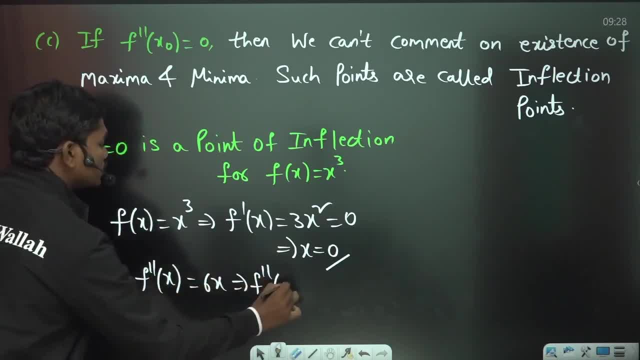 dash of x, naught f. double dash of x is dash of x, naught f. double dash of x is nothing but six x. so this implies f. nothing but six x. so this implies f. nothing but six x. so this implies f. double dash of zero is equal to zero. 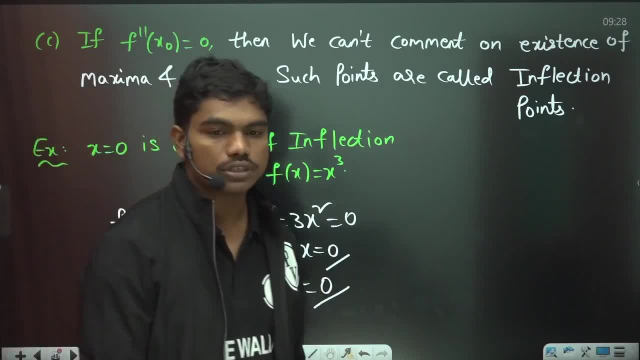 double dash of zero is equal to zero. double dash of zero is equal to zero again. so first derivative and second again. so first derivative and second again. so first derivative and second derivative. at x equal to zero are both derivative. at x equal to zero, are both derivative. at x equal to zero, are both zeros. so here you can't comment on. 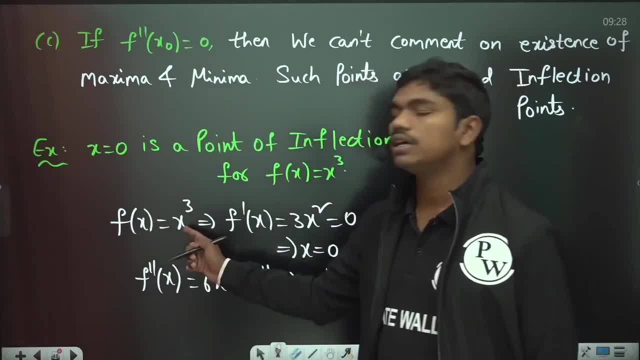 zeros. so here you can't comment on zeros. so here you can't comment on maxima and minima. but actually, if you maxima and minima, but actually if you maxima and minima, but actually, if you see carefully, this function doesn't have. see carefully, this function doesn't have. 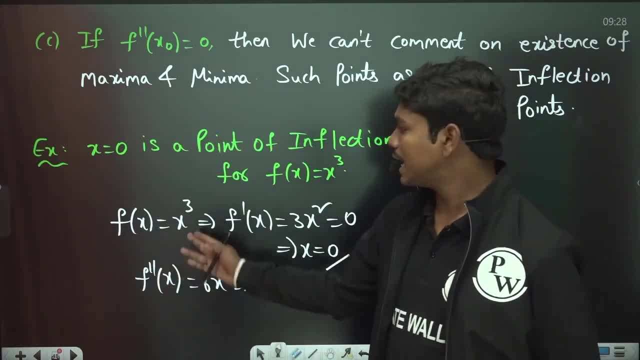 see carefully. this function doesn't have either maxima or minima here at this, either maxima or minima here at this, either maxima or minima here at this point. why? because you see as you keep on point. why? because you see as you keep on. 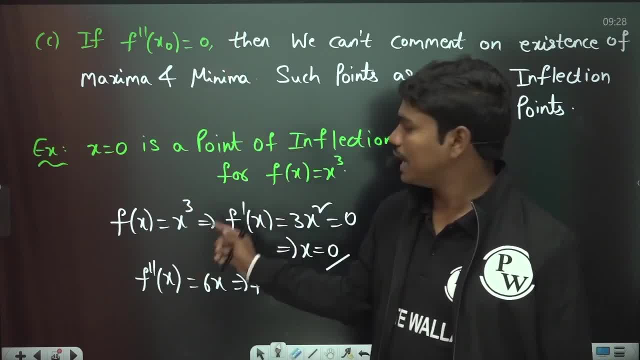 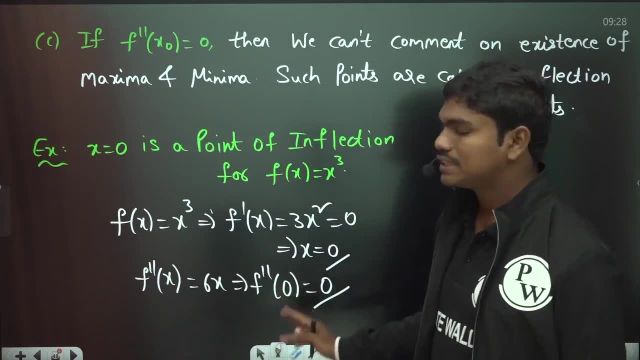 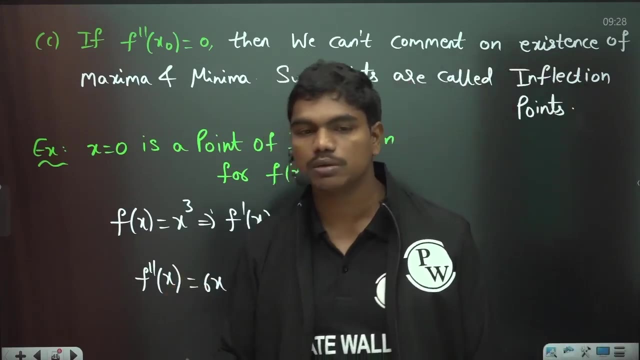 point why? because you see, as you keep on increasing positive value of x, this x, increasing positive value of x, this x, increasing positive value of x, this x derivative test comes into the picture. derivative test comes into the picture. derivative test comes into the picture if the function is having maxima or 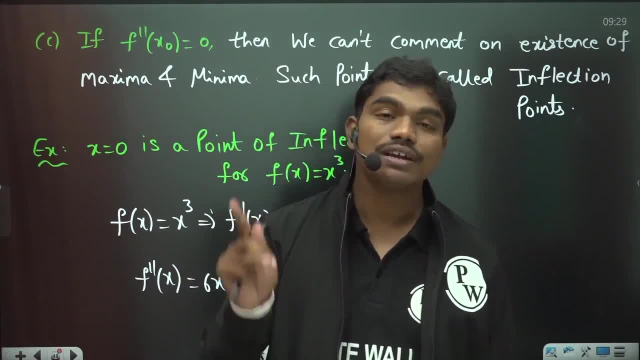 if the function is having maxima, or if the function is having maxima or minimum. definitely yes. differentiation is minimum. definitely yes. differentiation is minimum, definitely yes, differentiation is zero. but if differentiation is zero, the zero. but if differentiation is zero, the zero. but if differentiation is zero, the function need not have maxima or minima. 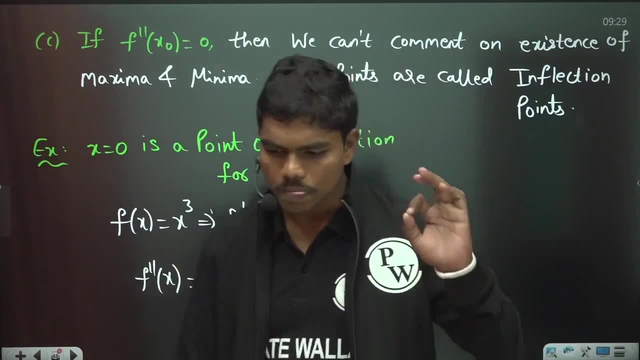 function need not have maxima or minima function need not have maxima or minima. this is the example clear. so these, this is the example clear, so these, this is the example clear, so these points are very much, points are very much, points are very much, you know, very important actually because 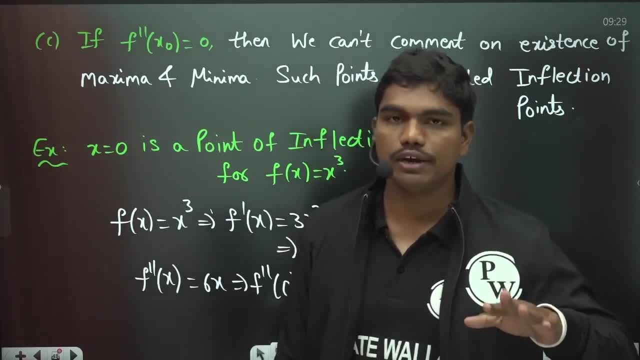 you know very important actually, because you know very important actually, because sometimes they ask you when you, sometimes they ask you when you, sometimes they ask you when you differentiate, definitely did not have a differentiate, definitely did not have a differentiate, definitely did not have a maximum or minimum. this is the example. maximum or minimum. this is the example. maximum or minimum. this is the example. okay, and if you see the graph of y is okay, and if you see the graph of y is okay, and if you see the graph of y is equal to x cube, it looks something like: 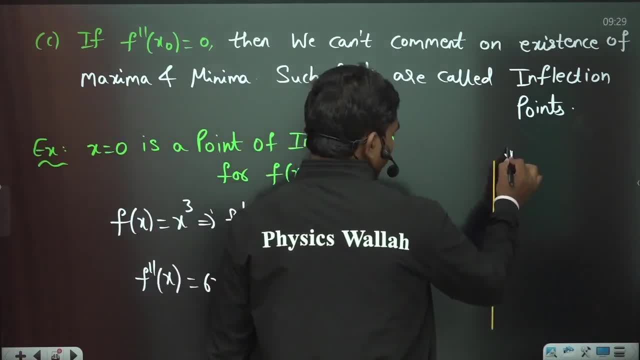 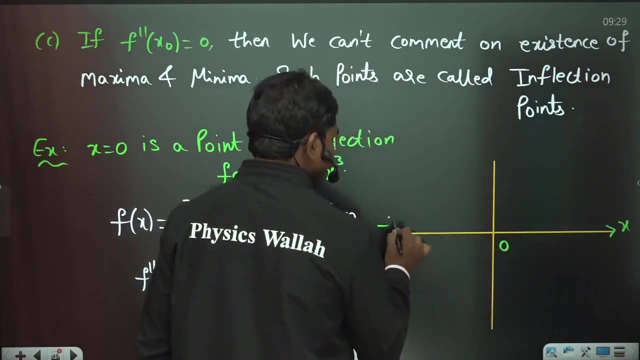 equal to x cube. it looks something like equal to x cube. it looks something like this: so so, so, x, x, x. let us write this the other side, let us write this the other side. let us write this the other side: zero, zero, zero, minus x, minus x. 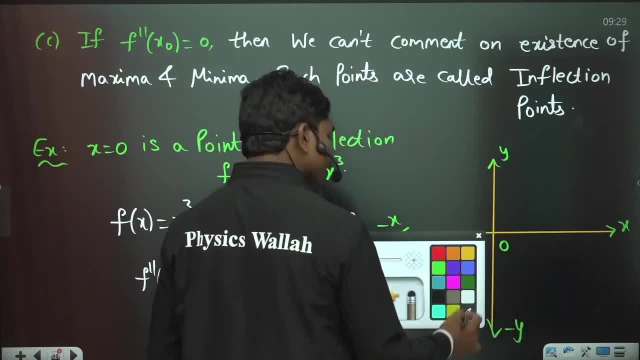 minus x, y minus y, y minus y, y minus y. so if you see the graph, it looks so. if you see the graph, it looks so. if you see the graph, it looks something like this, something like this, something like this. it starts like this, then it gets very. 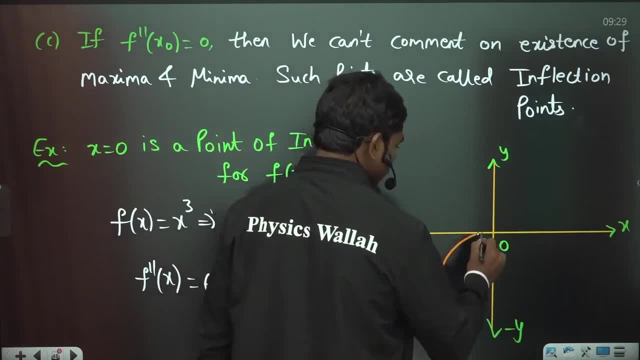 it starts like this, then it gets very. it starts like this, then it gets very flat here, flat here, flat here. it starts like this, then it gets very. it starts like this, then it gets very. it starts like this, then it gets very flat here, almost flat here, almost. 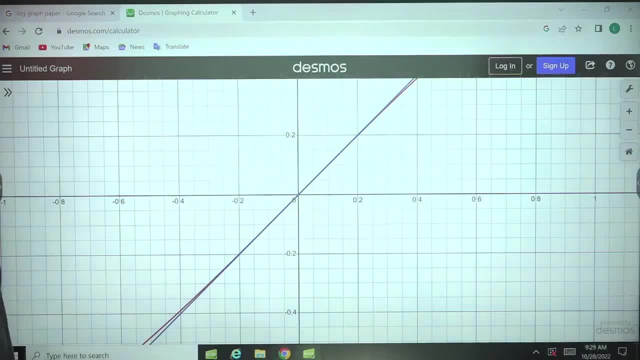 flat here, almost, and then it raises: okay, so anyhow, we have. and then it raises: okay, so anyhow we have. and then it raises: okay, so anyhow, we have this tool. so let me show you more this tool. so let me show you more this tool. so let me show you more clearly. 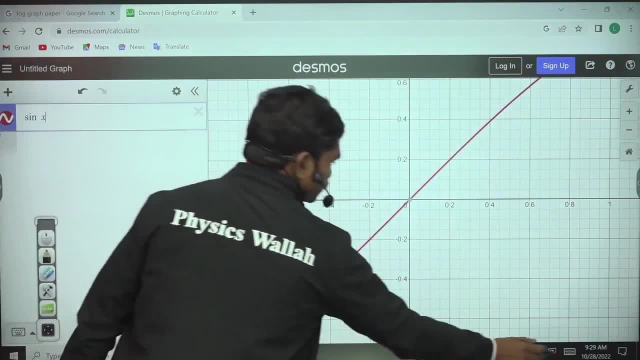 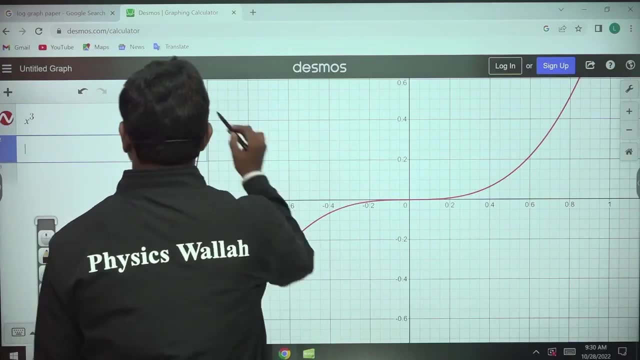 clearly, clearly. so we have this tool. so let me show you. so we have this tool. so let me show you. so we have this tool, so let me show you more clearly. so x, cube, x to the power, x to the power, x to the power three. okay, so if you see, this is x, cube. three okay. so if you see this is x cube, three okay. so if you see this is x cube, increases again. so at this point x is increases again. so at this point x is increases again. so at this point x is equal to zero. you can see, it's not. 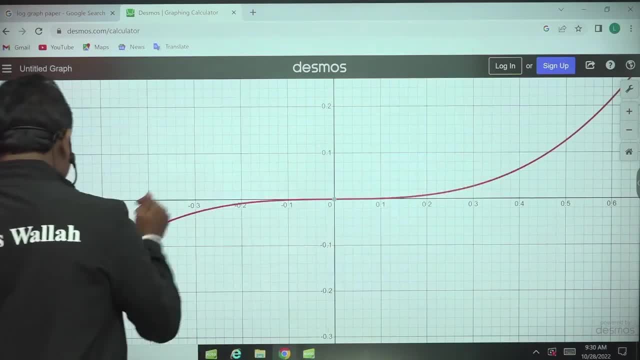 equal to zero. you can see it's not equal to zero. you can see it's not maximum value or minimum value. because maximum value or minimum value, because maximum value or minimum value, because the maximums and also minimums on the, the maximums and also minimums on the. 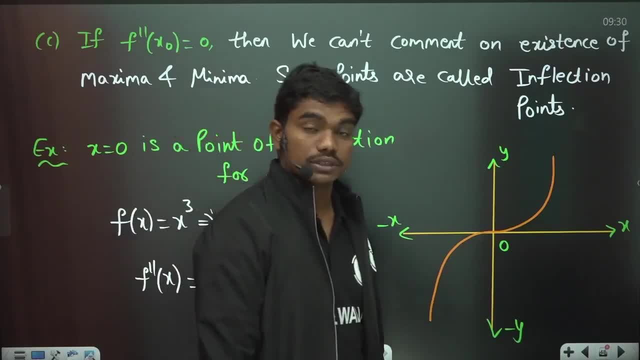 the maximums and also minimums on the left side. okay so, but at x is equal to left side. okay so, but at x is equal to left side. okay so, but at x is equal to zero. the derivative is zero, so this is zero. the derivative is zero, so this is. 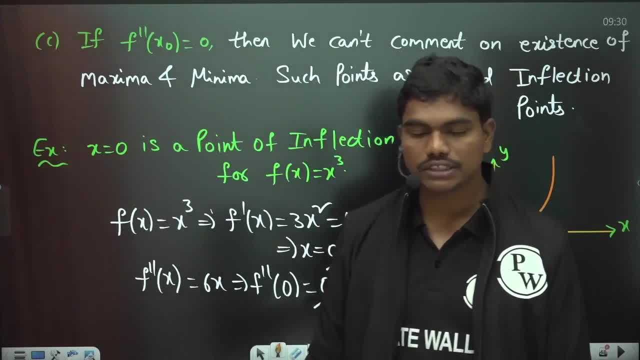 zero, the derivative is zero. so this is one very important point to note, one very important point to note, one very important point to note. actually so, if differentiation is zero, actually so, if differentiation is zero, actually so, if differentiation is zero, the function need not mandatorily have. 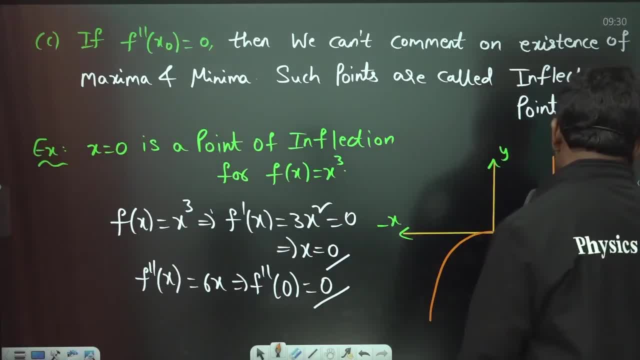 the function need not mandatorily have the function, need not mandatorily have maxima or maxima or maxima or minima- clear now. let us uh minima clear now. let us uh minima clear now. let us uh move to the next example. i'll tell you. move to the next example. i'll tell you. move to the next example. i'll tell you here. you may feel that whenever the here, you may feel that whenever the here, you may feel that whenever the point is point of inflection, point is point of inflection. 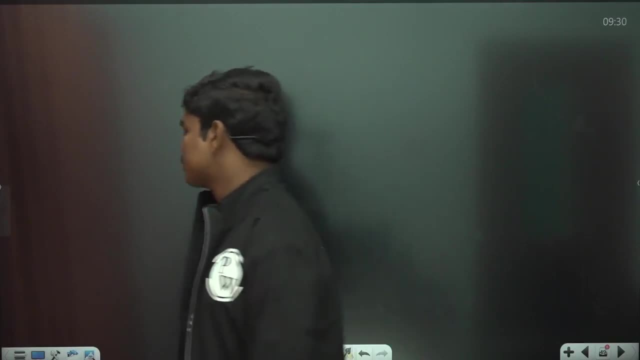 point is point of inflection, then the function may not have maxima, or then the function may not have maxima, or then the function may not have maxima or minima, but minima but minima. but actually the case is something different. actually the case is something different. 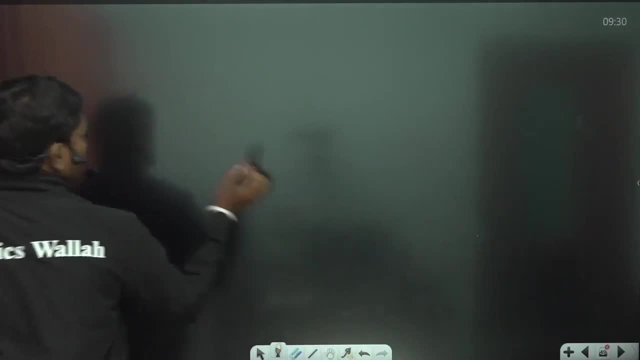 actually the case is something different. look, we can't comment. that's the reason. look, we can't comment. that's the reason. look, we can't comment. that's the reason why. if you see why, if you see why, if you see example x is equal to zero, is a point of. 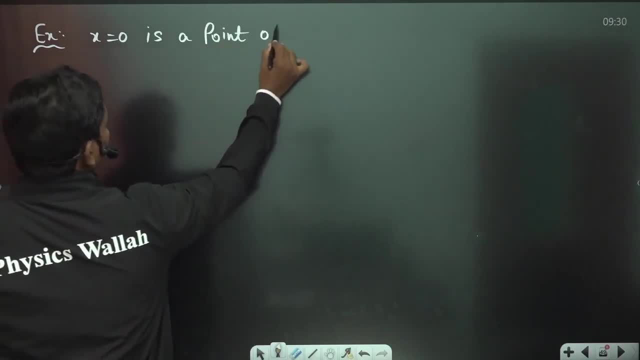 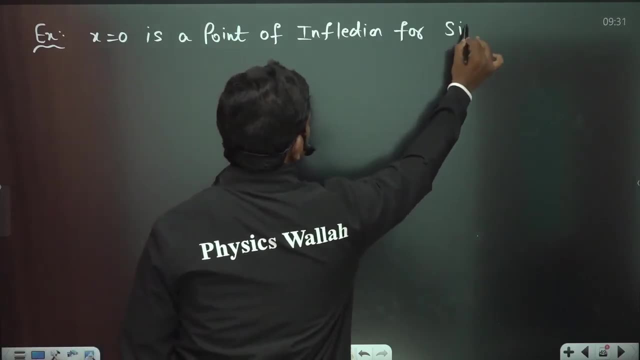 x is equal to zero is a point of x is equal to zero is a point of inflection, inflection, inflection is a point of inflection. for sine x is equal to x, for sine x is equal to x, for sine x is equal to x- i mean sorry- for sine x by x is equal. 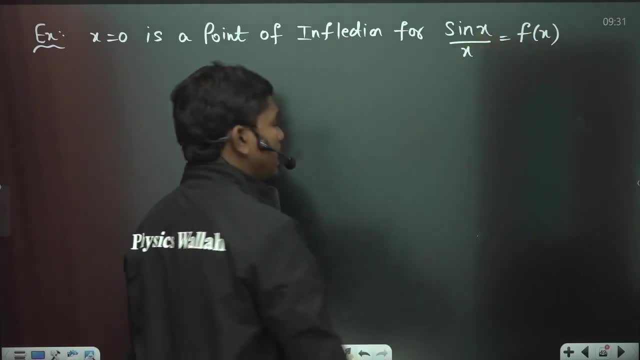 i mean sorry, for sine x by x is equal. i mean sorry, for sine x by x is equal to f of x to f of x to f of x. okay, if you take this function and if you okay, if you take this function and if you okay, if you take this function and if you calculate the differentiation and all, calculate the differentiation and all. calculate the differentiation and all. definitely you will get. x is equal to zero. definitely you will get. x is equal to zero. definitely you will get. x is equal to zero is the point of inflection and x is the point of inflection and x. 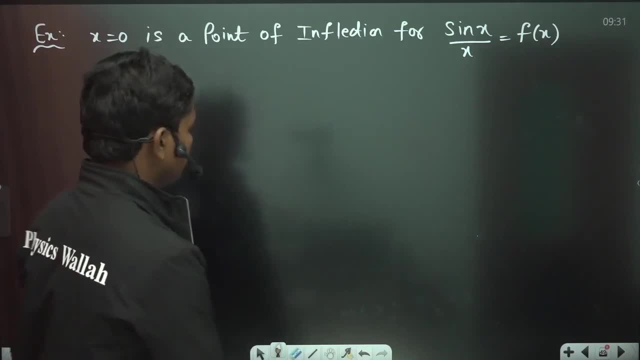 is the point of inflection. and x equal to zero, also satisfies. second equal to zero, also satisfies. second equal to zero, also satisfies. second derivative equal to zero, okay. but if you derivative equal to zero, okay. but if you derivative equal to zero, okay. but if you see, 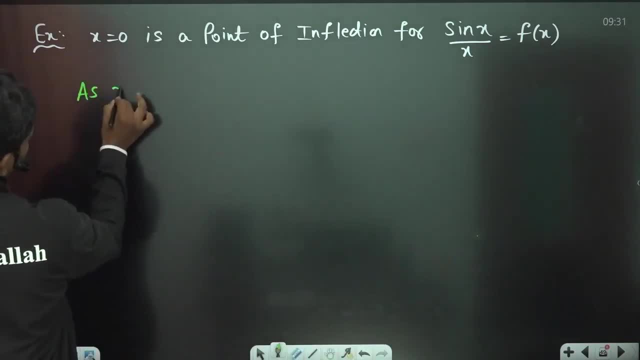 see, see, yet x is equal to zero. uh, you can it. as yet x is equal to zero. uh, you can it. as yet x is equal to zero. uh, you can it. as extends to zero. extends to zero. extends to zero. sine x by x has. sine x by x has. 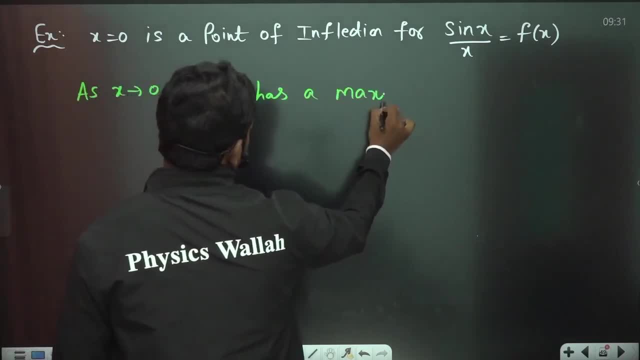 sine x by x has a maximum value of one, correct? we have a maximum value of one. correct, we have a maximum value of one, correct? we have seen, seen, seen, maximum value of maximum value of maximum value of one. actually, okay, look, we have also one. actually, okay, look, we have also. 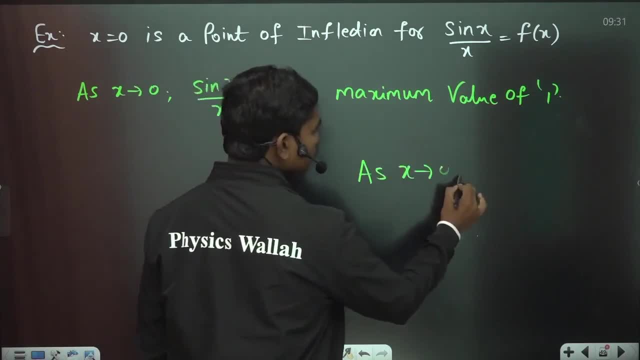 one actually. okay, look, we have also seen that ls is as extends to zero, seen that ls is as extends to zero, seen that ls is as extends to zero. we told sine x, we told sine x, we told sine x will be almost equal to x. this is what. 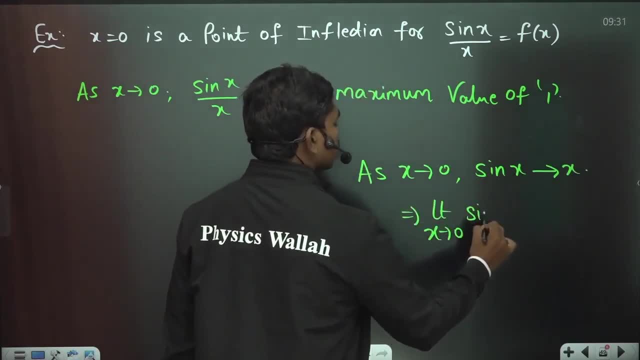 will be almost equal to x. this is what will be almost equal to x. this is what we like as limit extends to zero. we like as limit extends to zero. we like as limit extends to zero. sine x, sine x, sine x by x. if you write, if you divide this x. 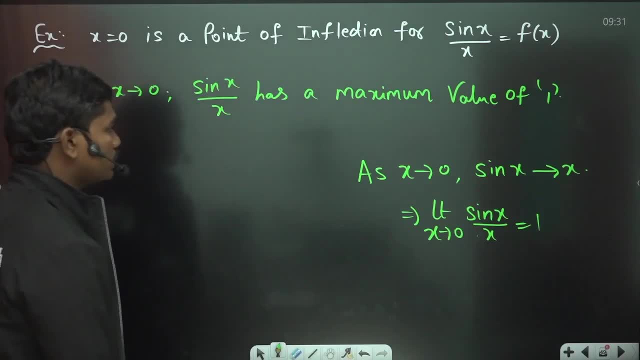 by x. if you write: if you divide this x by x. if you write: if you divide this x here, this tends to one, so this is equal here. this tends to one, so this is equal here. this tends to one, so this is equal to one. this is what we write, so this has. 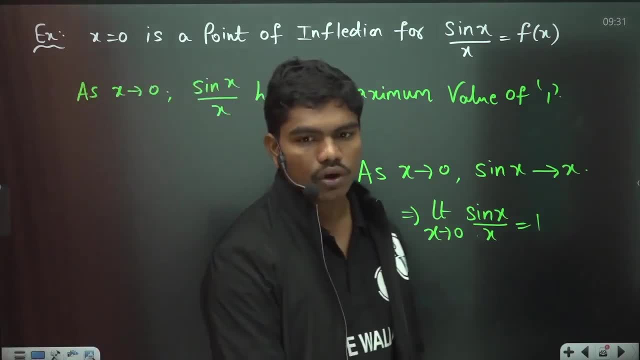 to one. this is what we write, so this has to one. this is what we write, so this has a maximum value of one. so that's why we a maximum value of one. so that's why we a maximum value of one. so that's why we cannot, we can never comment on it is. 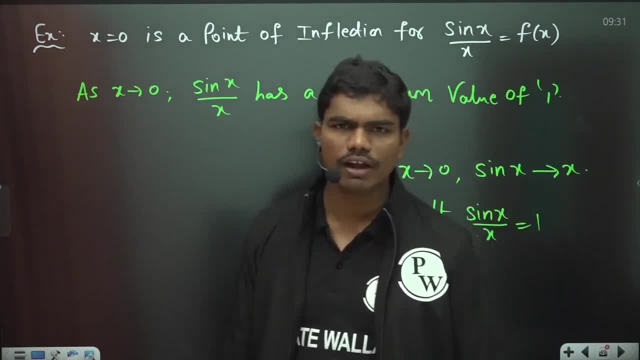 cannot, we can never comment on it. is cannot, we can never comment on it. is maximum or minimum actually, okay it maximum or minimum actually okay. it maximum or minimum actually okay, it depends on the depends on the depends on the function. that, uh, you know we generally function that, uh, you know, we generally. 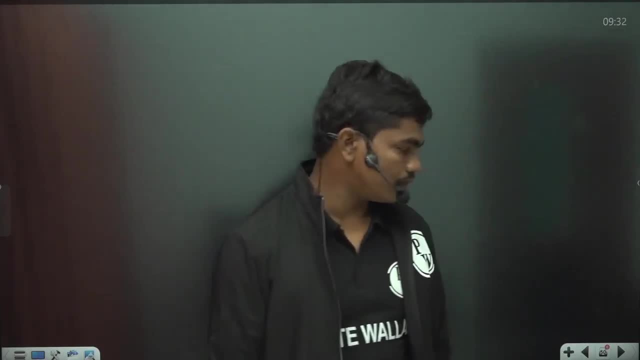 function that, uh, you know, we generally talk about okay. so with this, we talk about okay. so with this, we talk about okay. so with this, we know the procedure how to calculate this, know the procedure how to calculate this, know the procedure how to calculate this concept of maxima and minima. but now i 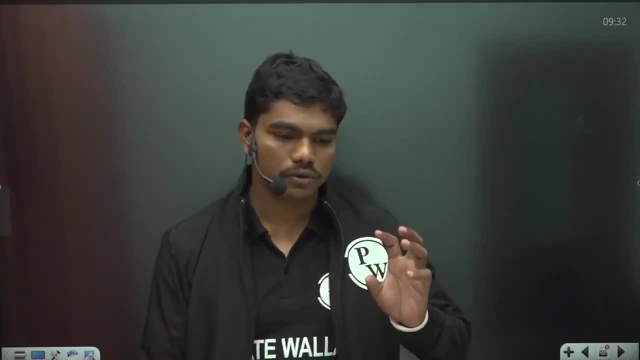 concept of maxima and minima, but now i concept of maxima and minima, but now i would like to give you one important, would like to give you one important, would like to give you one important point uh, one very important, you know uh. point uh one very important, you know uh. 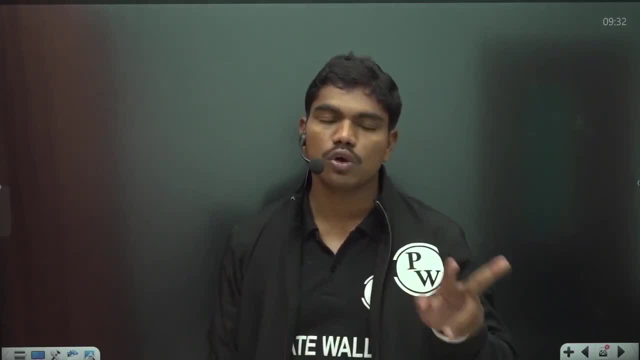 point, uh, one very important, you know, uh, difference between two things, which is difference between two things, which is difference between two things, which is called global maxima, minima, local maxima, called global maxima minima, local maxima, called global maxima minima, local maxima minima. this is some very important point. 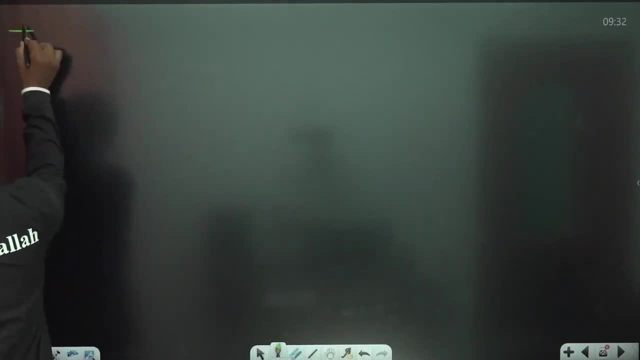 minima. this is some very important point. minima, this is some very important point. actually look what is this global and actually look what is this global and actually look what is this global and local. global maxima or minima global maxima. maxima or minima global maxima. 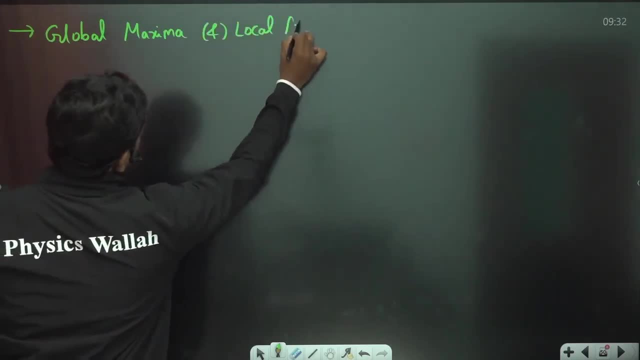 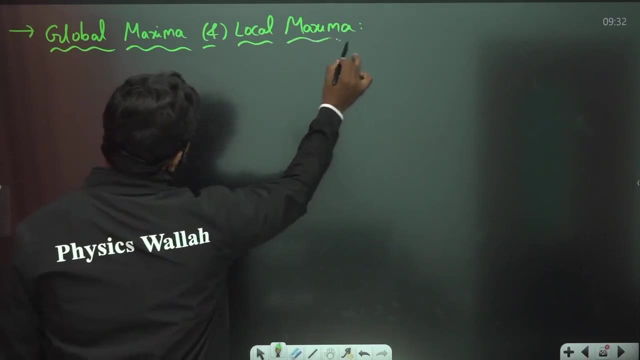 maxima or minima, global maxima and local maxima similarly minima also, and local maxima, similarly minima also, and local maxima similarly minima also. if you write, if you write, if you write global maximum and local maxima. so let us see what is this global maxima? so let us see what is this global maxima. so let us see what is this global maxima and local maxima. look and local maxima. look and local maxima look. let us suppose if you have a function. let us suppose if you have a function. 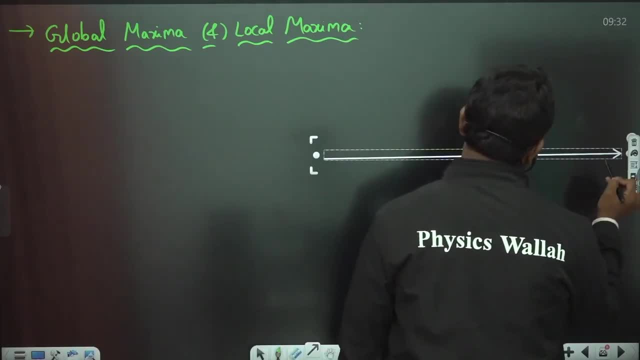 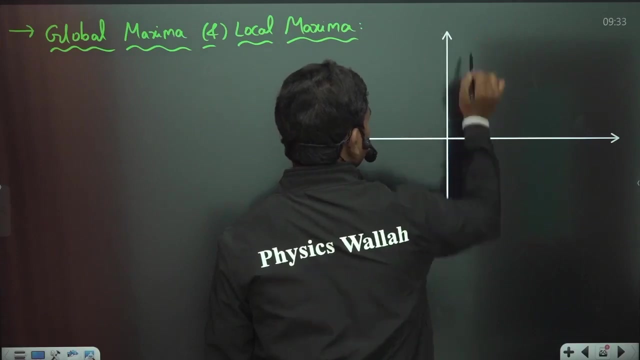 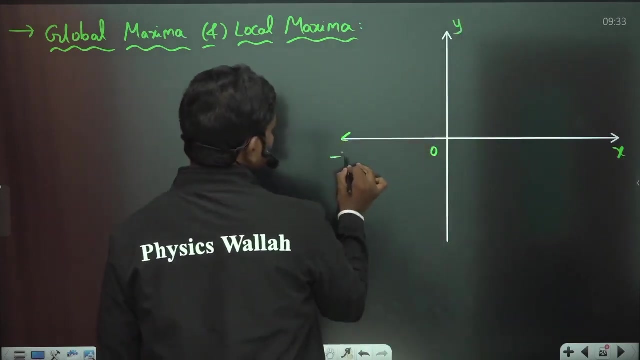 let us suppose, if you have a function like this, like this, like this: okay, so this is horizon. this is x. okay, so this is horizon. this is x. okay, so this is horizon. this is x. this is y. this is minus x. this is y. this is minus x. this is minus y. 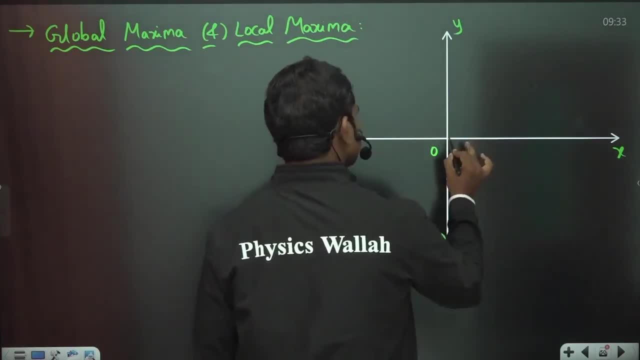 this is y, this is minus x, this is minus y. now you see here, if you plot the graph. now you see here, if you plot the graph. now you see here, if you plot the graph, for example, let us suppose you got some. for example, let us suppose you got some. 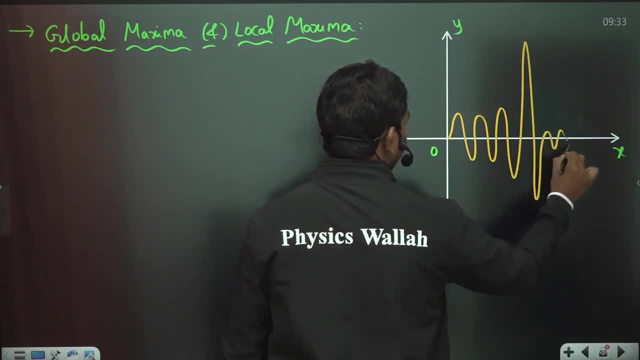 for example, let us suppose you got some random curve like this and the function stopped here, let us, and the function stopped here, let us, and the function stopped here, let us suppose this is the curve. suppose this is the curve. okay, suppose this is the curve. okay, suppose this is the curve. okay, this is. this is the curve, basically here. 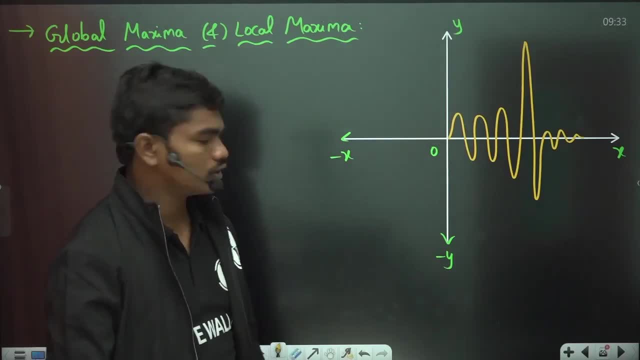 this is, this is the curve, basically here. this is this is the curve, basically here. okay, so let us suppose this is some plot. okay, so let us suppose this is some plot. okay, so let us suppose this is some plot of some function, some sine wave, or of some function some sine wave, or. 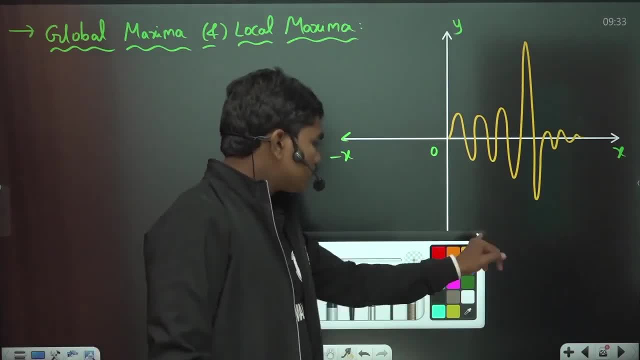 of some function, some sine wave or something. there is some fluctuation, something. there is some fluctuation something. there is some fluctuation meanwhile, now tell me one thing. if i ask: meanwhile, now tell me one thing, if i ask: meanwhile, now tell me one thing, if i ask you, what is the maximum value of this? 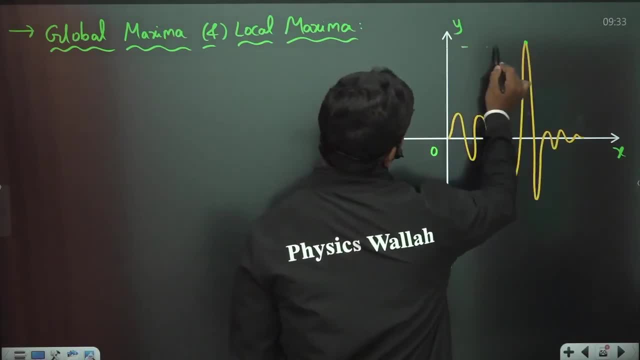 you, what is the maximum value of this you, what is the maximum value of this function? undoubtedly you will say this is function. undoubtedly, you will say this is function. undoubtedly you will say this is the value correct. so, if you see within the value correct. so if you see within, 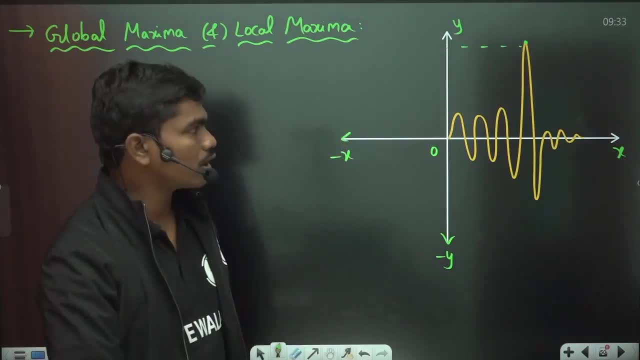 the value correct. so if you see, within, the complete interval means from minus, the complete interval means from minus, the complete interval means from minus. infinity to infinity. let us suppose this infinity to infinity. let us suppose this infinity to infinity. let us suppose this is the only part of the function. now, if 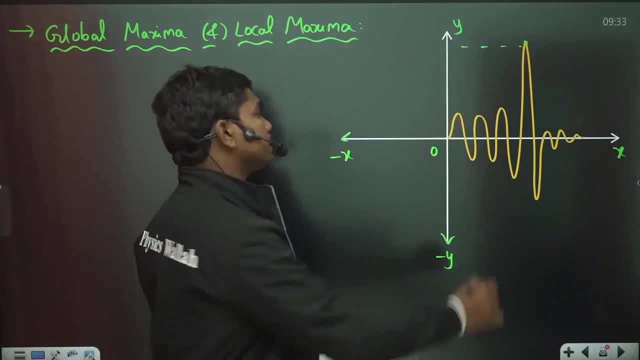 is the only part of the function now. if is the only part of the function now. if you see for the complete real axis, that you see for the complete real axis, that you see for the complete real axis, that value which i'm writing as value which i'm writing as: 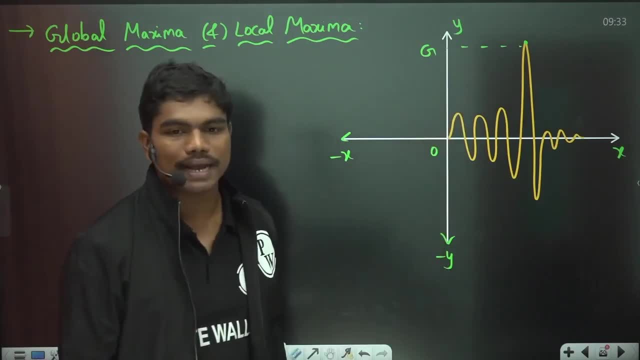 value which i'm writing as g1 for g, for example, this g is the g1 for g, for example, this g is the g1 for g. for example, this g is the maximum value globally, but let us maximum value globally. but let us maximum value globally. but let us suppose, if i give you some interval, that 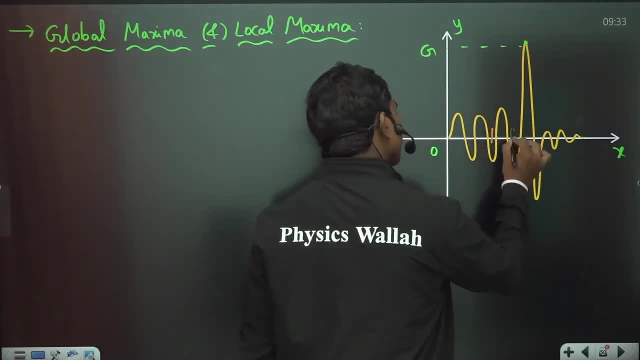 suppose, if i give you some interval, that suppose, if i give you some interval, that i am focusing only on this interval, for i am focusing only on this interval, for i am focusing only on this interval. for example, i am focusing only on this example, i am focusing only on this. 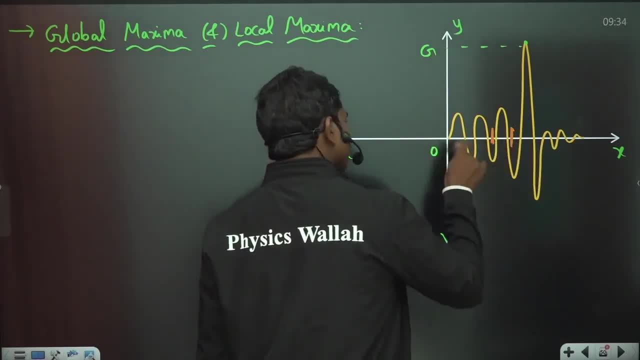 example- i am focusing only on this interval- then if you see if i ask you interval, then if you see if i ask you interval, then if you see if i ask you what is the maximum value of this, what is the maximum value of this, what is the maximum value of this function in this interval, then 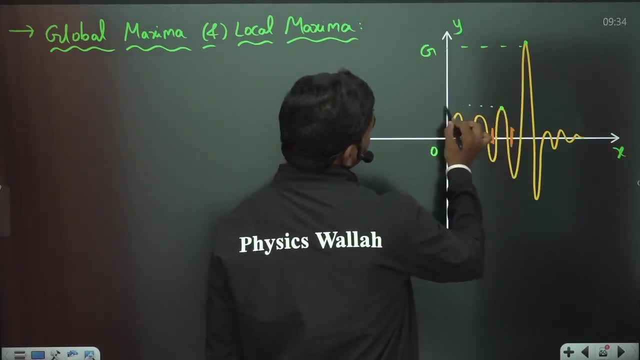 function in this interval, then function in this interval, then definitely you will write. this is the definitely you will write. this is the definitely you will write: this is the maximum value, correct? so this is local maximum value, correct. so this is local maximum value, correct. so this is local maxima within the given interval. so if 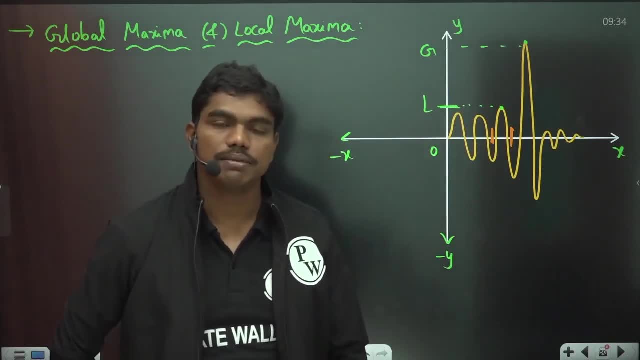 maxima within the given interval. so if maxima within the given interval, so if interval changes, local maximum, can interval changes. local maximum can interval changes. local maximum can change, but global maxima remains same change. but global maxima remains same change. but global maxima remains same for any interval. okay, so that's the 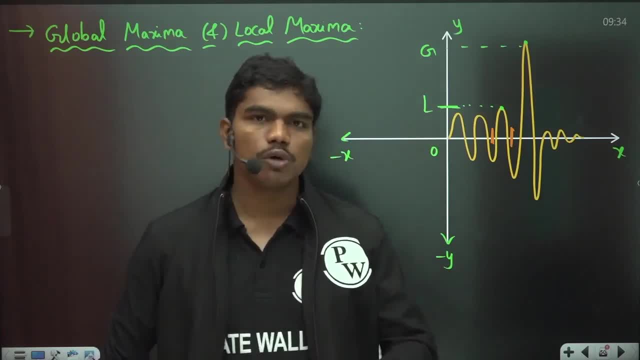 for any interval. okay. so that's the for any interval. okay. so that's the difference between global and local. you difference between global and local, you difference between global and local, you can understand by the words also. global can understand by the words also. global can understand by the words also. global means totally whatever is available, the. 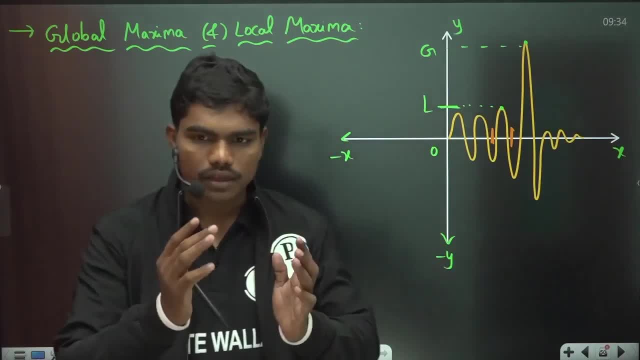 means totally whatever is available. the means totally whatever is available. the complete access. local means some region complete access. local means some region: complete access. local means some region, okay, okay, okay. so some region, if you see this is uh. so some region, if you see this is uh. 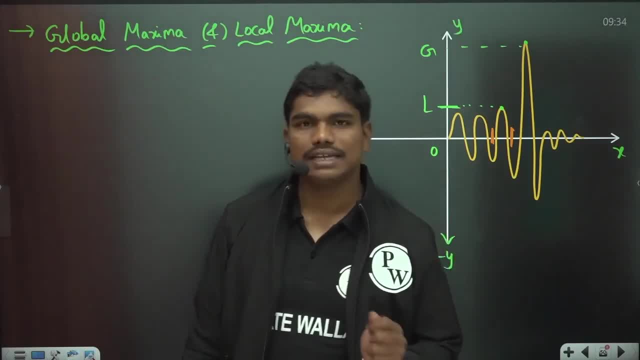 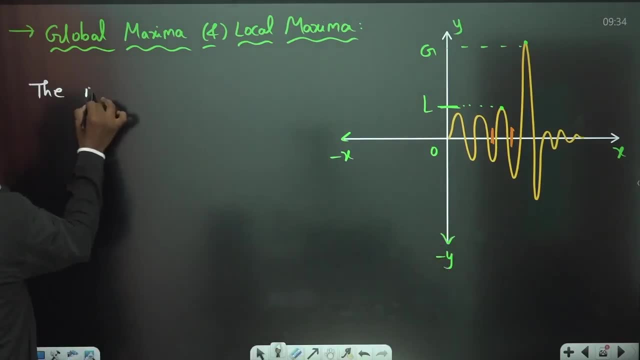 so some region, if you see this is uh, called locally, actually okay. called locally, actually okay. called locally, actually okay. i'll tell you out with the help of an. i'll tell you out with the help of an. i'll tell you out with the help of an example. 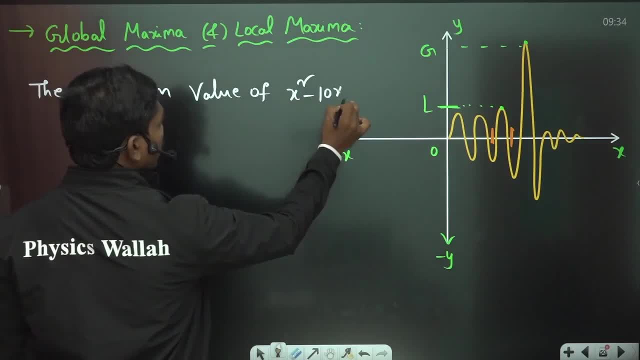 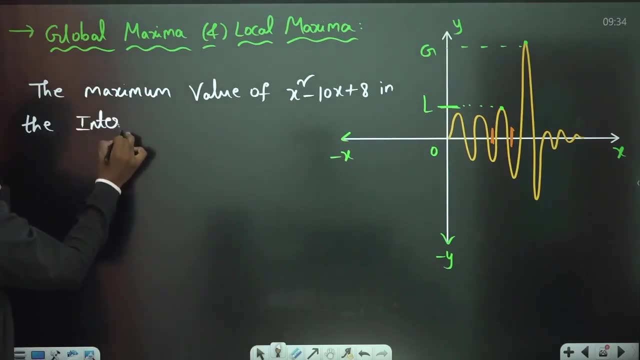 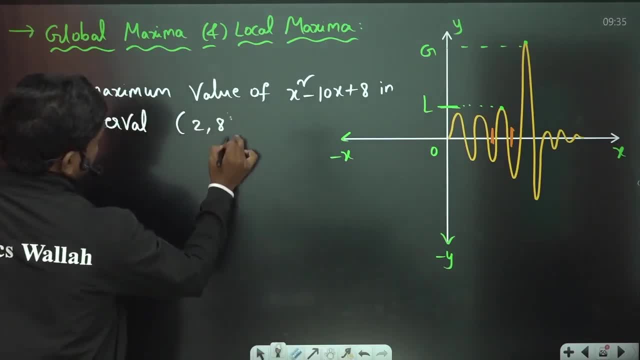 4 comma 6, for example, okay. so what you? 4 comma 6, for example, okay. so what you can say, can say: can say 2 comma 8, let us say: is 2 comma 8. let us say: is 2 comma 8. let us say: is dash. let us suppose, if i ask you this: 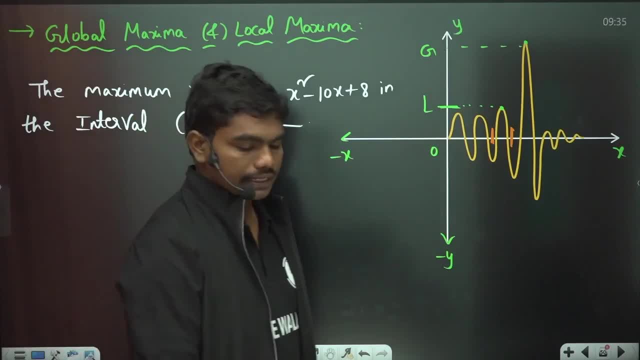 dash. let us suppose if i ask you this dash, let us suppose if i ask you this question, for example: okay, question for example, okay, question for example: okay now if you apply, if you in exam, such now if you apply, if you in exam, such now if you apply, if you in exam. such kind of questions can come. 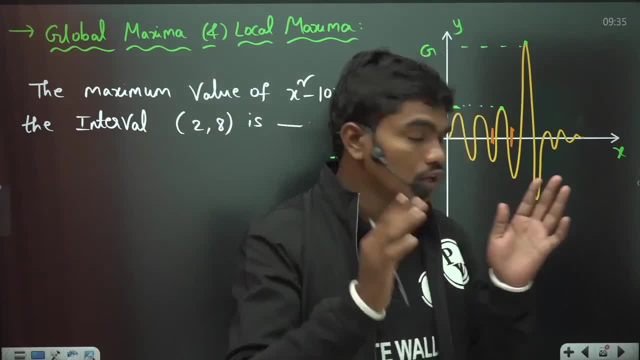 kind of questions can come. kind of questions can come. they'll give you some interval, okay, they'll give you some interval. okay, they'll give you some interval. okay, they'll give you some region they want, they'll give you some region they want, they'll give you some region. they want you to talk on some local. 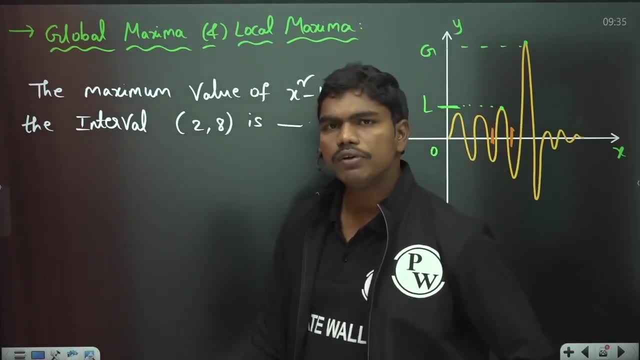 you to talk on some local. you to talk on some local things. so that's why, if you see they'll things, so that's why, if you see they'll things, so that's why, if you see they'll give you one, give you one, give you one region. okay, now how you will do this. 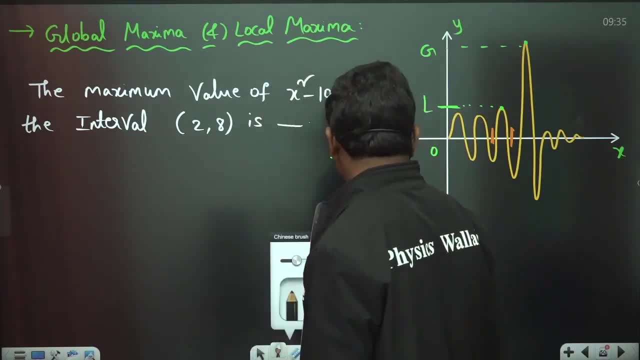 region. okay now how you will do this region. okay now how you will do this. normally, if you start applying the normally, if you start applying the normally, if you start applying the process of local maximum. i mean this process of local maximum, i mean this process of local maximum, i mean this actual global maximum minima. let us see. 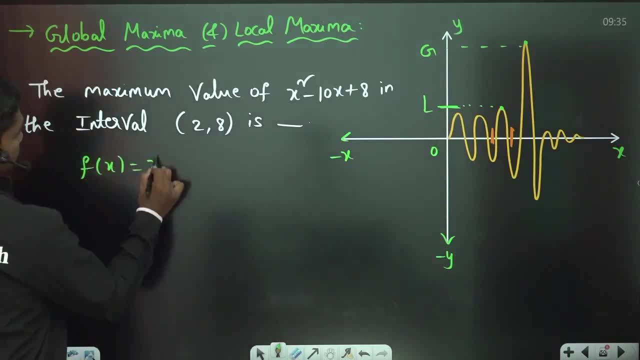 actual global maximum minima. let us see actual global maximum minima. let us see what comes out f of x. what comes out f of x. what comes out f of x is x square minus 10 x plus 8. is x square minus 10 x plus 8. 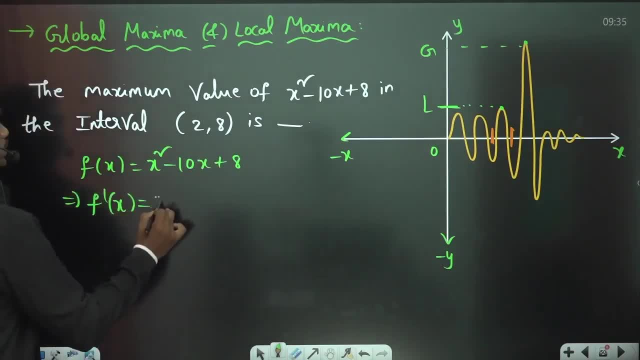 is x square minus 10, x plus 8. so if you calculate f dash of x, so if you calculate f dash of x, so if you calculate f dash of x, this is 2x minus 10. so if you equate, this is 2x minus 10. so if you equate, 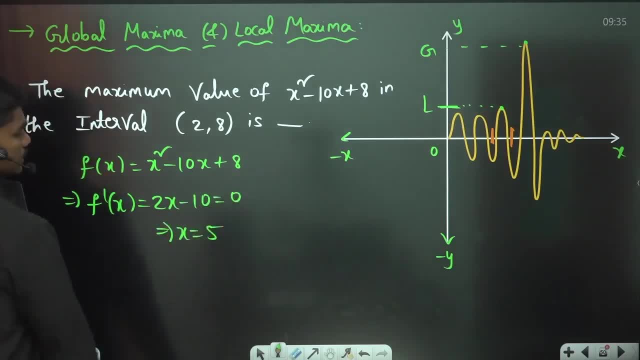 this is 2x minus 10. so if you equate this to 0, x is equal to 5. this to 0, x is equal to 5. this to 0, x is equal to 5, x is equal to 5. so okay, let us change this. x is equal to 5, so okay, let us change this. x is equal to 5, so okay, let us change this question. question, question: let us keep 3 here, for example, 3 comma 8. let us keep 3 here, for example, 3 comma 8. 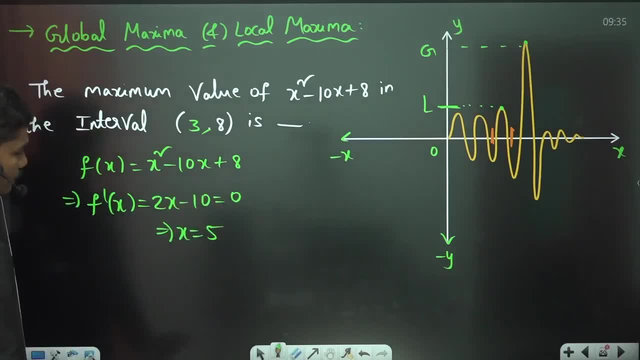 let us keep 3 here, for example 3 comma 8. let us keep okay, so x is equal to 5. so let us keep okay, so x is equal to 5. so let us keep okay, so x is equal to 5. so if x is equal to 5, then what is f? 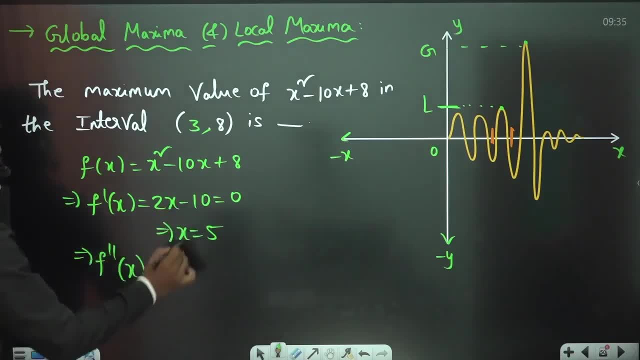 if x is equal to 5, then what is f? if x is equal to 5, then what is f? double dash of x. double dash of x. double dash of x- f. double dash of x is equal to 2, now this. f double dash of x is equal to 2, now this. 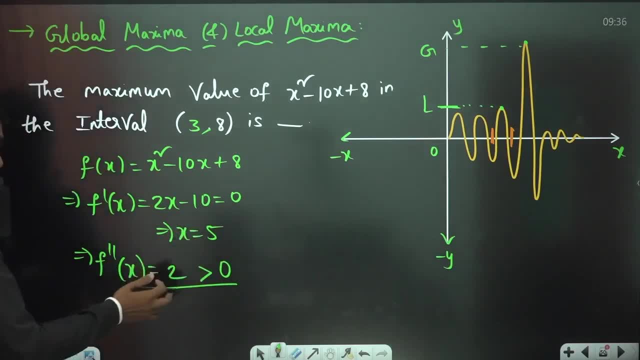 f double dash of x is equal to 2. now, this is greater than zero. now tell me one is greater than zero. now tell me one is greater than zero. now tell me one thing, and you need not substitute any thing, and you need not substitute any thing, and you need not substitute any stationary point. also, this f double. thing and you need not substitute any stationary point. also this f double thing and you need not substitute any stationary point. also this f double dash of x is dash of x is dash of x is always greater than zero now whenever f. always greater than zero now whenever f. 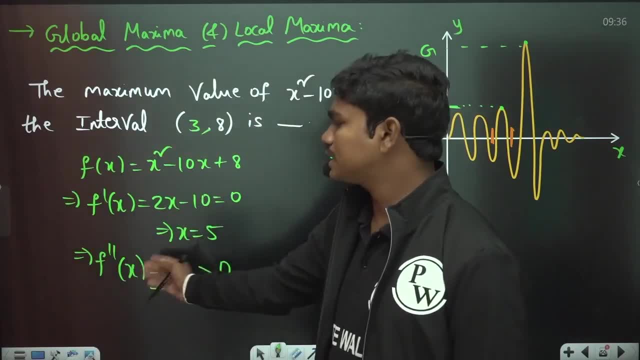 always greater than zero. now, whenever f double dash of x is greater than zero, at double dash of x is greater than zero, at double dash of x is greater than zero. at stationary point also, even if you put x stationary point also, even if you put x stationary point also, even if you put x is equal to 5, you will still get 2. so 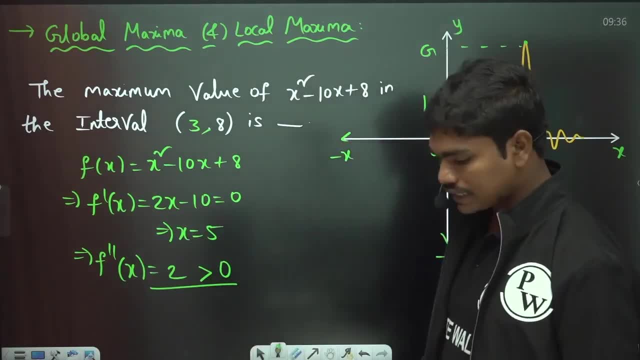 is equal to 5, you will still get 2. so is equal to 5, you will still get 2. so here, if you see this second derivative here, if you see this second derivative here, if you see this second derivative is actually positive now, if second. 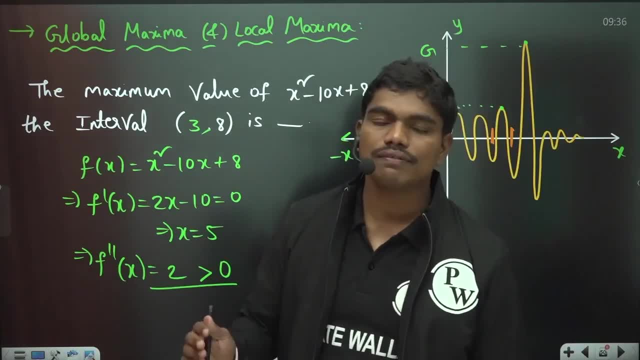 is actually positive now, if second is actually positive now, if second derivative is positive from the concept derivative is positive from the concept derivative is positive from the concept of maxima and minima. you know that the of maxima and minima, you know that the of maxima and minima, you know that the function has a minimum, but in the 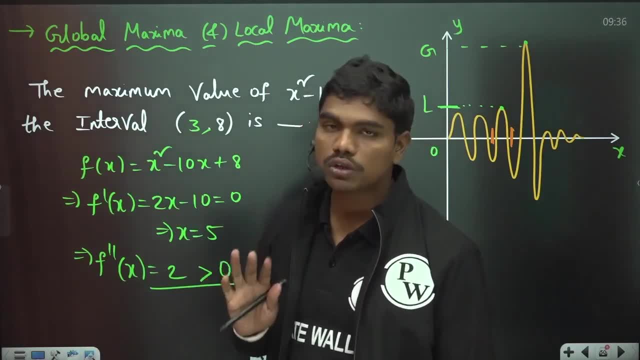 function has a minimum. but in the function has a minimum. but in the question they're asking you maximum question. they're asking you maximum question. they're asking you maximum understood, so here you will get stuck. if understood, so here you will get stuck. if understood, so here you will get stuck. if you don't know the concept of global. 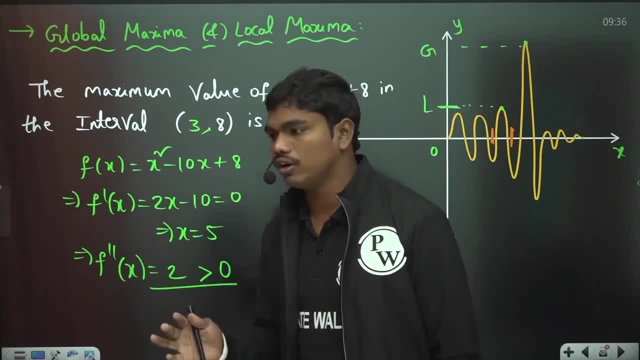 you don't know the concept of global, you don't know the concept of global maxima and local maxima, or similarly maxima and local maxima, or similarly maxima and local maxima, or similarly, global minimum and local minima also, global minimum and local minima also. 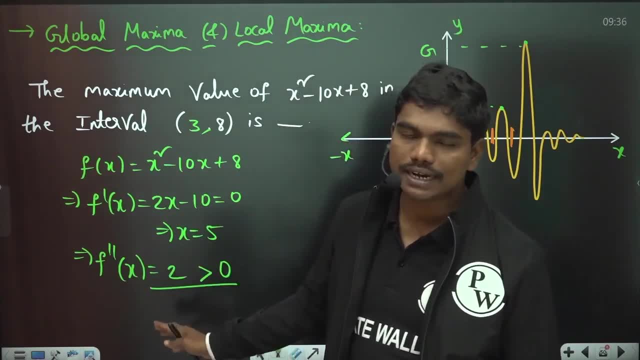 global minimum and local minima also. look, look, look, here you and your, you got ended up with here, you and your, you got ended up with here, you and your. you got ended up with the second derivative being positive, the second derivative being positive, the second derivative being positive. but you know, if second derivative is, 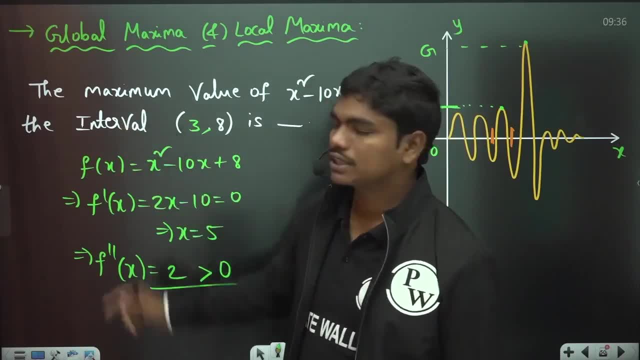 but you know if second derivative is. but you know if second derivative is positive, positive, positive. they uh there, the function has a minimum. they uh there, the function has a minimum. they uh there, the function has a minimum. but they're asking you for the maximum. but they're asking you for the maximum. 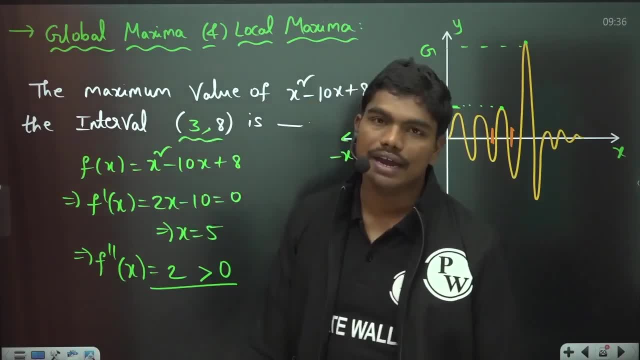 but they're asking you for the maximum value. so that's why they have given you value. so that's why they have given you value, so that's why they have given you this interval 3 comma 8. so what they're? this interval 3 comma 8. so what they're. 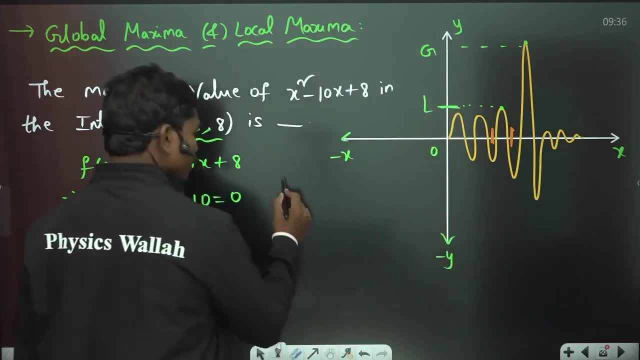 this interval 3 comma 8. so what they're asking you for look whenever they give asking you for look, whenever they give asking you for look, whenever they give you some interval. you need to calculate this function at. you need to calculate this function at. you need to calculate this function at stationary point. so f of 5. so if you 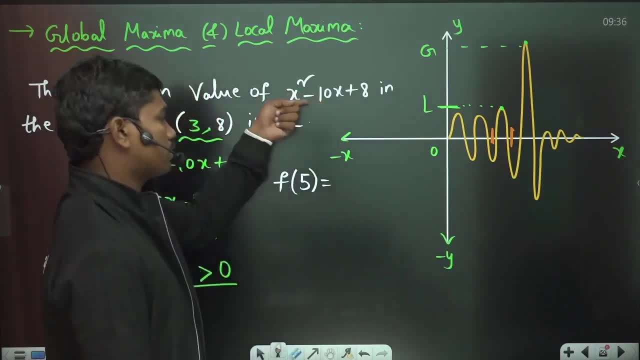 stationary point, so f of 5. so if you stationary point, so f of 5. so if you calculate f of 5, calculate f of 5. calculate f of 5: 25 minus 50. 25 minus 50 is minus 25. 25 minus 50. 25 minus 50 is minus 25. 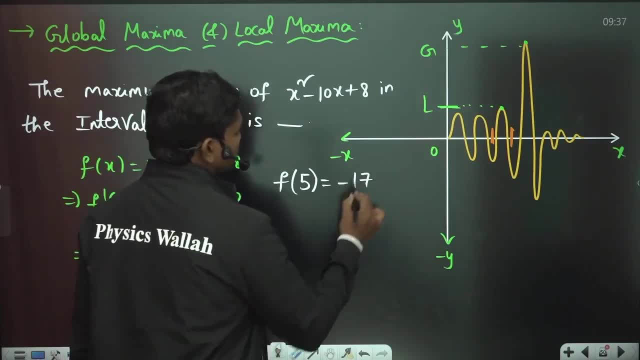 25 minus 50. 25 minus 50 is minus 25 minus 25 plus 8 minus 17, so minus 25 plus 8 minus 17, so minus 25 plus 8 minus 17, so minus 17. next, along with the stationary, 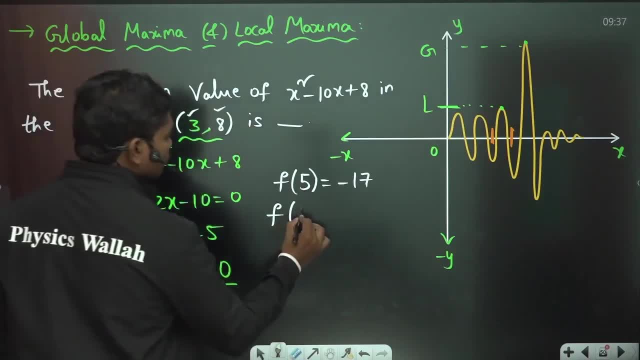 minus 17 next, along with the stationary. minus 17 next, along with the stationary points. you should also calculate these points. you should also calculate these points. you should also calculate these points. okay, so f of 3 if you keep f of points. okay, so f of 3 if you keep f of. 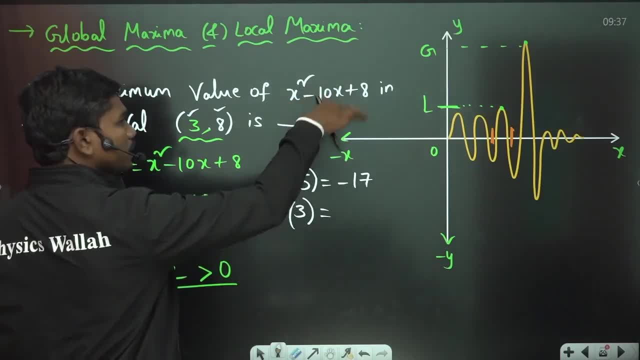 points. okay, so f of 3, if you keep f of 3, 9 minus 30 minus 21 minus 21 plus 8, 3, 9 minus 30 minus 21 minus 21 plus 8, 3, 9 minus 30 minus 21 minus 21 plus 8 minus 13. f of 8. 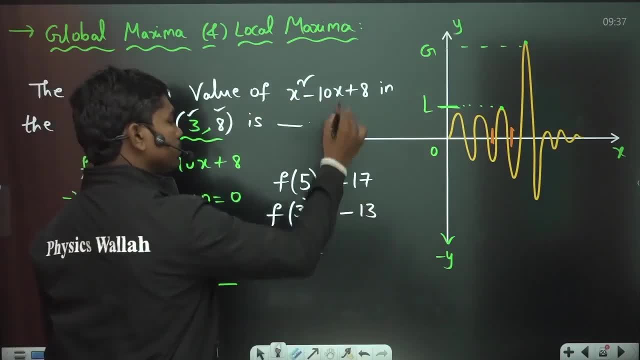 minus 13 f of 8 minus 13 f of 8, 64, 64 minus 80 minus 16 minus 16 plus 64, 64 minus 80 minus 16 minus 16 plus 64 64 minus 80 minus 16 minus 16 plus 8 minus 8. okay, so if you see the maximum, 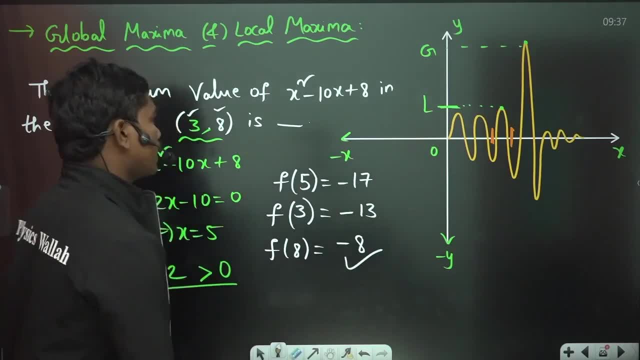 8 minus 8, okay. so if you see the maximum- 8 minus 8, okay. so if you see the maximum value out of these three things is value out of these three things is value out of these three things is basically, basically, basically minus 8. so that's how the answer is. 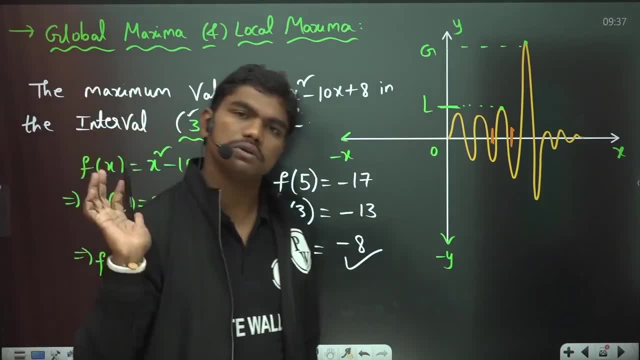 minus 8. so that's how the answer is minus 8. so that's how the answer is minus 8. because it's clearly, even if you minus 8, because it's clearly, even if you minus 8, because it's clearly, even if you read in the form of english, you will. 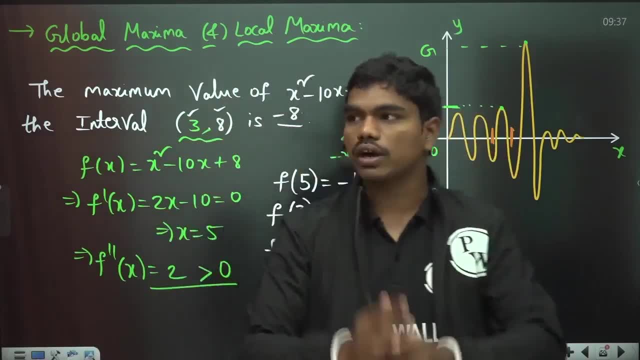 read in the form of english. you will read in the form of english. you will understand this question. understand this question, understand this question. maximum value in this interval is what? maximum value in this interval is what. maximum value in this interval is what? okay, so, if you see this, minus 8 is the. 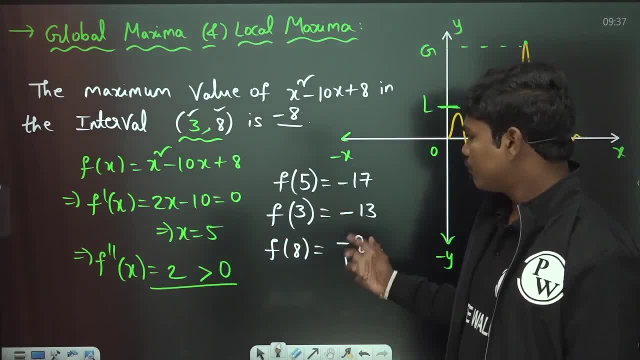 okay. so if you see this minus 8 is the okay, so if you see this minus 8 is the maximum value in this maximum value, in this maximum value in this interval, of course okay. and if you see interval, of course okay. and if you see interval, of course okay. and if you see carefully, 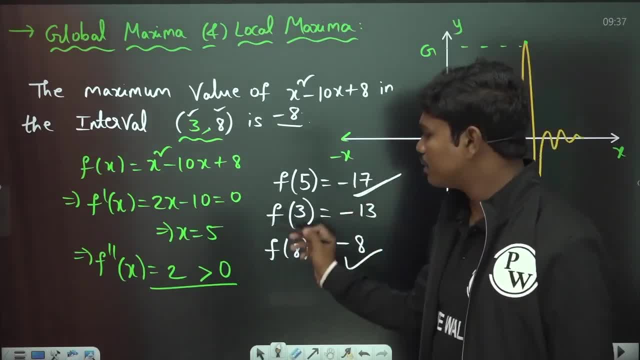 carefully, carefully. out of all these values minimum, is this: out of all these values, minimum is this: out of all these values, minimum is this: which is actually because, which is actually because, which is actually because. this is the point where this function. this is the point where this function. 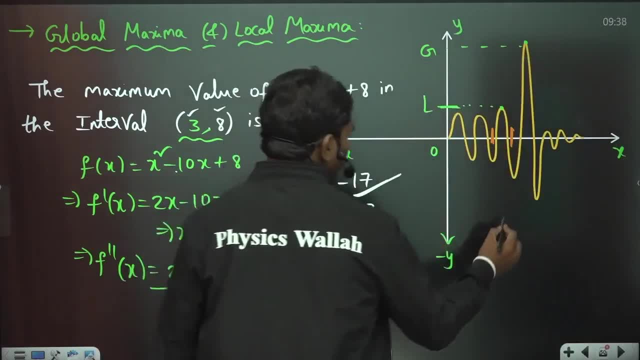 this is the point where this function is higher than minus 17, for example. you is higher than minus 17, for example, you is higher than minus 17. for example, you take 4- f of 4 if you calculate f of 4. take 4- f of 4 if you calculate f of 4. 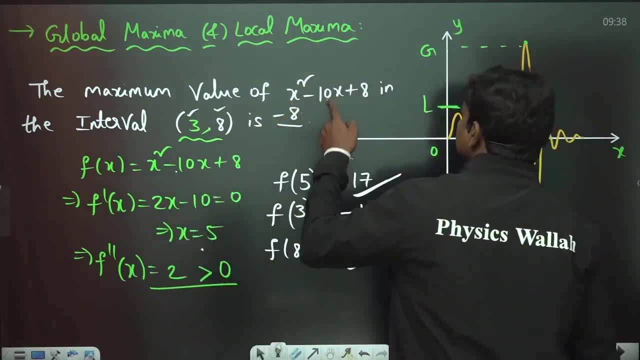 take 4 f of 4. if you calculate f of 4. if you calculate 16 minus 40 minus 24. if you calculate 16 minus 40 minus 24, if you calculate 16 minus 40 minus 24 minus 24 plus 8 minus 16, which is actually. 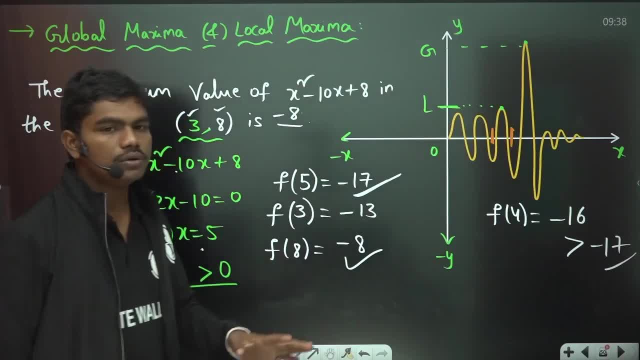 minus 24 plus 8 minus 16, which is actually minus 24 plus 8 minus 16, which is actually greater than minus 17, yes or no? greater than minus 17, yes or no. greater than minus 17, yes or no. so that's why, if you take any value in, 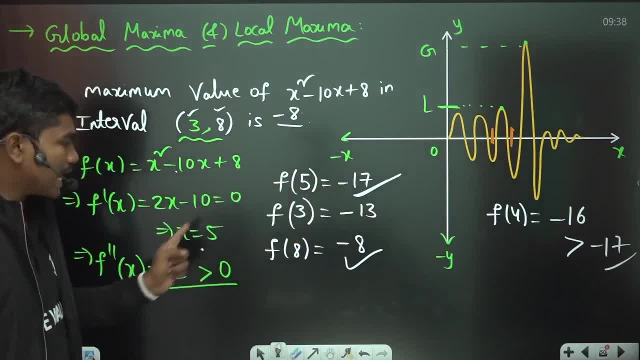 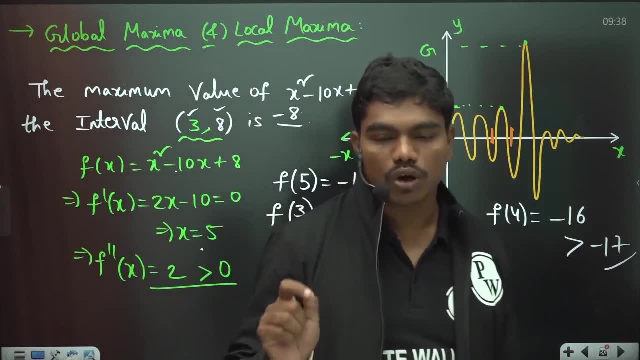 so that's why, if you take any value in, so that's why, if you take any value in this interval, definitely your answer will this interval, definitely your answer, will this interval, definitely your answer will be more than minus 17, because this is be more than minus 17, because this is. 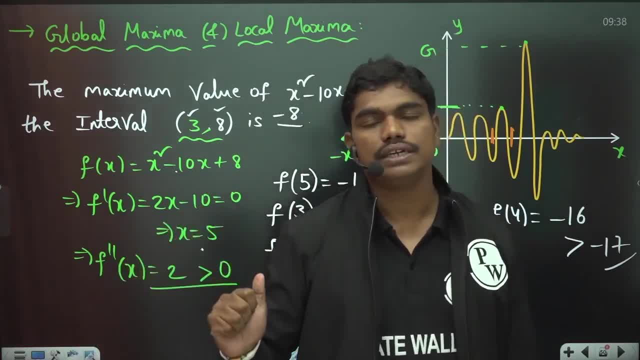 be more than minus 17, because this is only to uh do this and with this, we only to uh do this and with this, we only to uh do this, and with this we finish the concept of maxima and minima, finish the concept of maxima and minima. 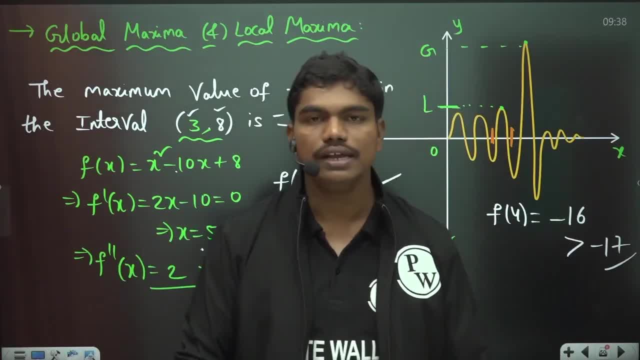 finish the concept of maxima and minima, and of course definitely we'll launch, and of course definitely we'll launch and of course definitely we'll launch one. uh see you soon, hopefully, for one. uh see you soon, hopefully for one. uh see you soon, hopefully for solving some questions on all these. 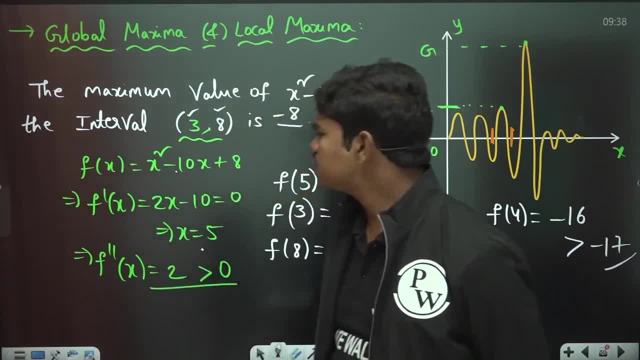 solving some questions on all these, solving some questions on all these things which we are covering in one things, which we are covering in one things, which we are covering in one shot. okay, so shot, okay, so shot, okay. so this is basically some uh, you know the. this is basically some uh, you know the. 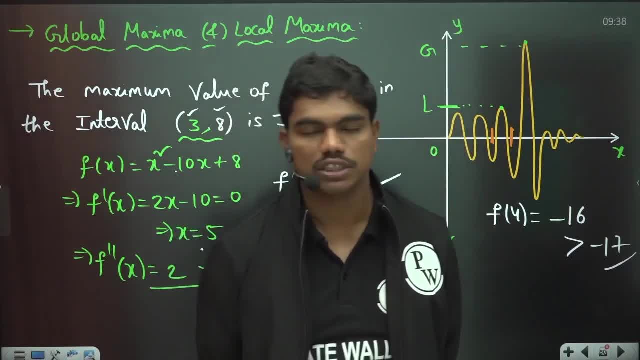 this is basically some, uh, you know the concept of maxima and minima. so with concept of maxima and minima, so with concept of maxima and minima, so with this we conclude a differential calculus. this we conclude a differential calculus. this we conclude a differential calculus. part of single variables. okay, so we'll. 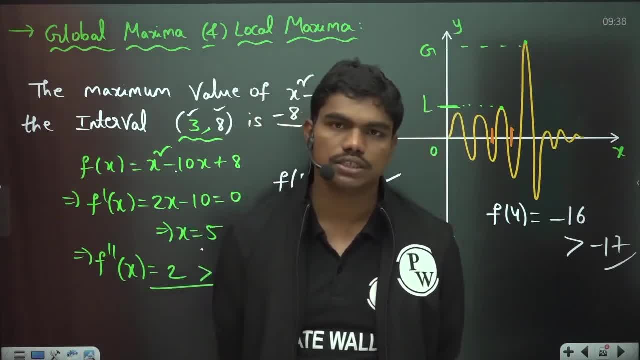 part of single variables. okay, so we'll part of single variables. okay, so we'll do integral calculus also now, and then do integral calculus also now, and then do integral calculus also now, and then we'll close this uh session. basically, we'll close this uh session basically. 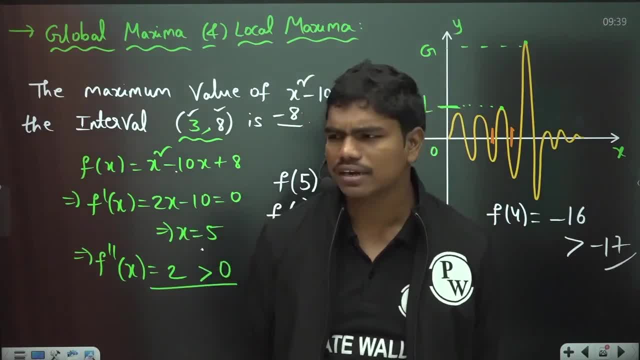 we'll close this uh session basically: okay, so let us go for the integral. okay, so let us go for the integral. okay, so let us go for the integral calculus. uh, because you know calculus is calculus. uh, because you know calculus is calculus. uh, because you know calculus is a vast module you cannot take in a single. 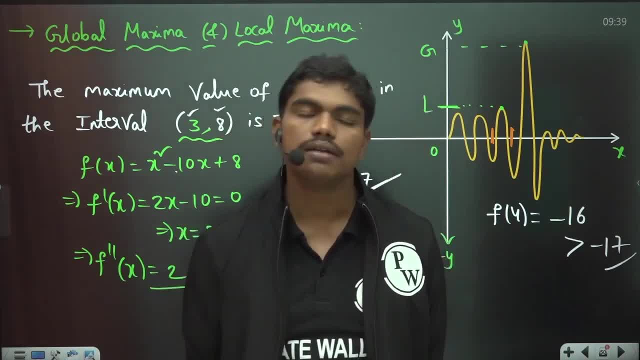 a vast module, you cannot take in a single a vast module, you cannot take in a single video. so we'll split it into two video. so we'll split it into two video. so we'll split it into two single variable: one video and multiple. single variable, one video and multiple. 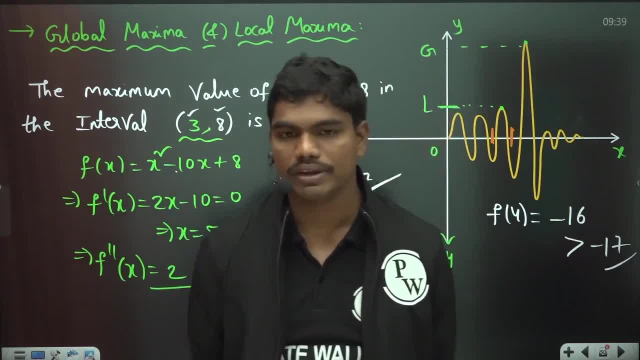 single variable, one video and multiple variables means two, three. all others in variables means two, three. all others in variables means two, three, all others in the next video, maybe okay, so let's the next video, maybe okay, so let's the next video, maybe okay, so let's talk about this. uh, once, quick revision. 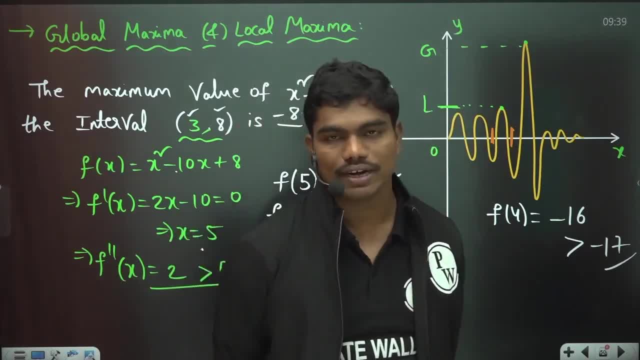 talk about this, uh once quick revision. talk about this, uh once quick revision. we have talked about the concepts of. we have talked about the concepts of. we have talked about the concepts of limit, continuity and differentiability. limit, continuity and differentiability. limit, continuity and differentiability. we have understood what differentiation. 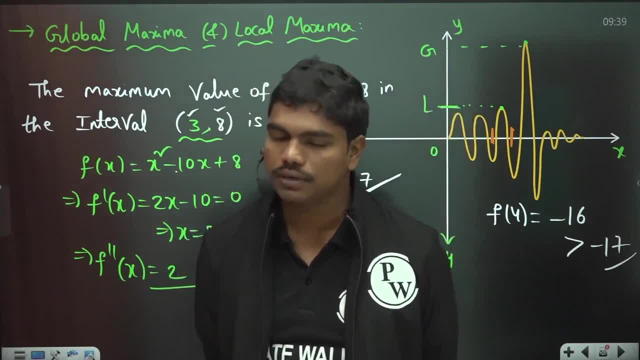 we have understood what differentiation, we have understood what differentiation means geometrically, then we have talked means geometrically, then we have talked means geometrically. then we have talked about some applications of, about some applications of, about some applications of, uh, this differentiation basically, uh, this differentiation basically. 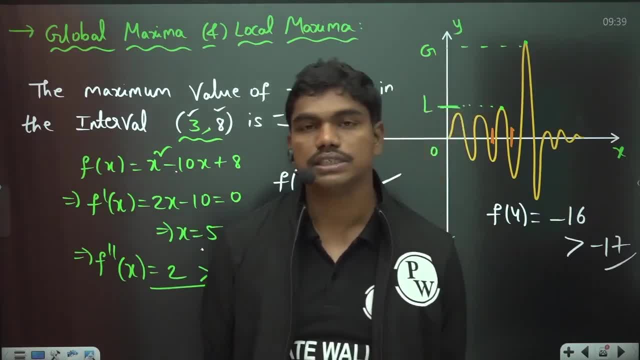 uh, this differentiation basically meanwhile lithium's taylor says, meanwhile lithium's taylor says, meanwhile lithium's taylor says maximum minimum concept. so all these maximum minimum concept, so all these maximum minimum concept, so all these things are very much important and i hope things are very much important and i hope. 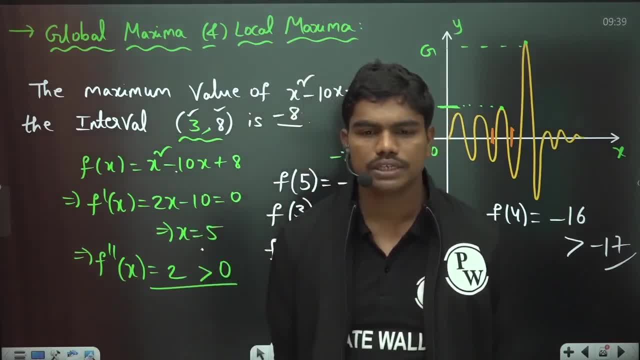 things are very much important and i hope you got some good knowledge also. uh, you got some good knowledge also. uh, you got some good knowledge also. uh, in this first you can say almost some in this first. you can say almost some in this first you can say almost some three years of the session. okay, so let's. 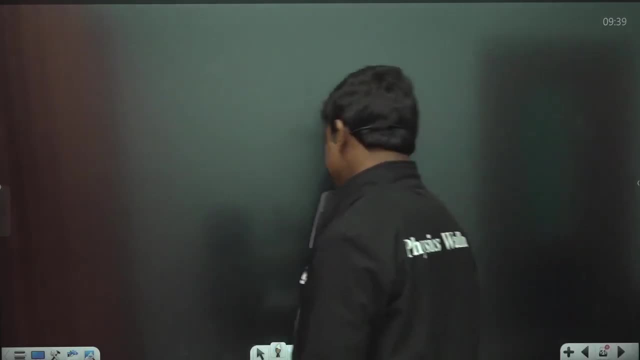 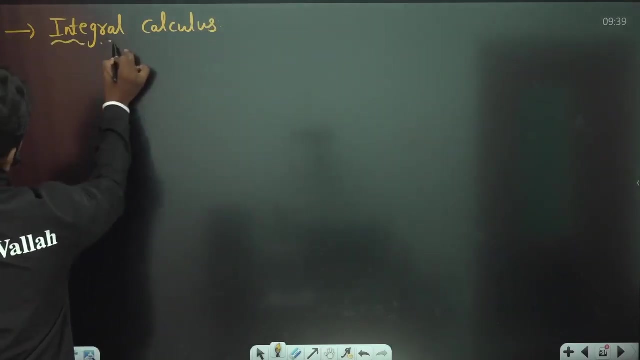 three years of the session. okay, so let's three years of the session. okay, so let's go for the integral calculus, go for the integral calculus, go for the integral calculus. so, integral calculus, integral calculus of single variable, of integral calculus of single variable, of integral calculus of single variable, of course. okay, so integral calculus. 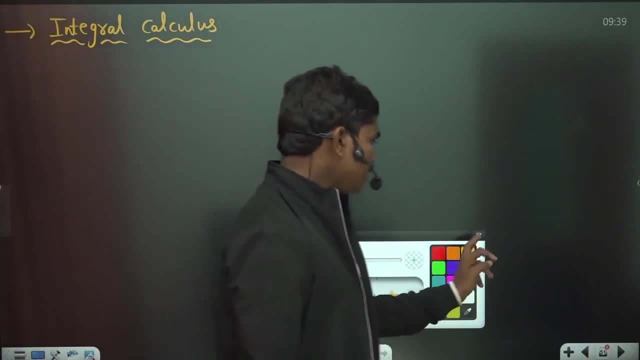 so integral calculus. now generally people so integral calculus. now generally people so integral calculus. now generally people feel integration a bit complex, as feel integration a bit complex, as feel integration a bit complex as compared to differentiation. fact that compared to differentiation, fact that compared to differentiation, fact that we also negate whenever questions comes. 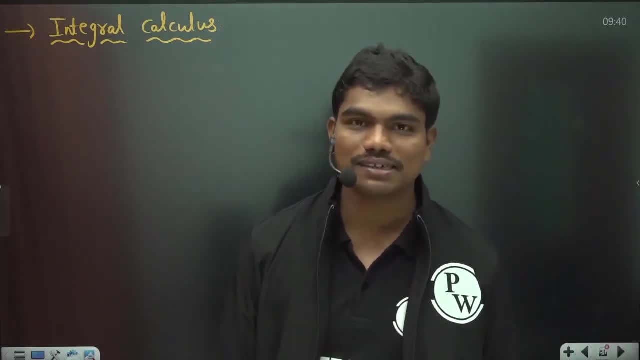 we also negate whenever questions comes. we also negate whenever questions comes from differentiation. we feel very happy from differentiation. we feel very happy from differentiation. we feel very happy that we'll be able to solve. but if that we'll be able to solve, but if that we'll be able to solve, but if questions are coming from integration. 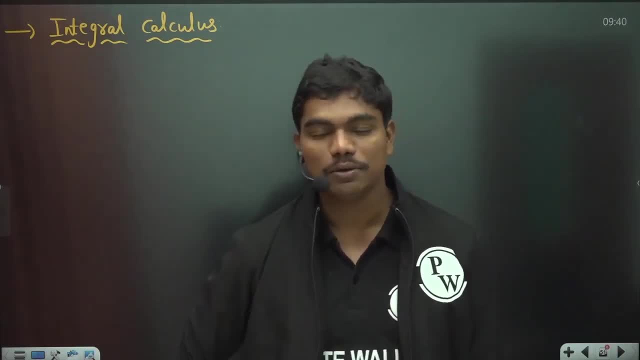 questions are coming from integration. questions are coming from integration. there is some kind of fear, but why this? there is some kind of fear, but why this? there is some kind of fear, but why this fear is existing because I will tell you. fear is existing because I will tell you: 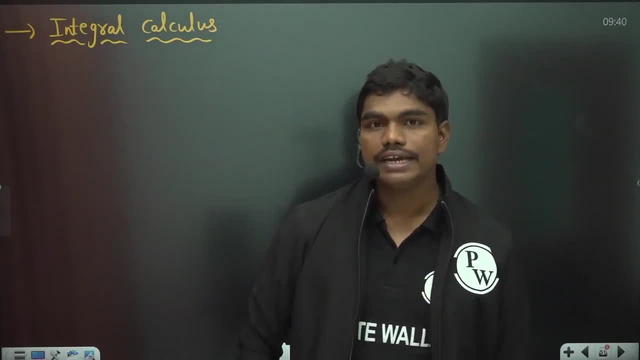 fear is existing because I will tell you, actually integration and differentiation, actually integration and differentiation, actually integration and differentiation, both are easy, but thing is in. both are easy, but thing is in. both are easy, but thing is in differentiation. let us suppose if you differentiation. let us suppose if you. 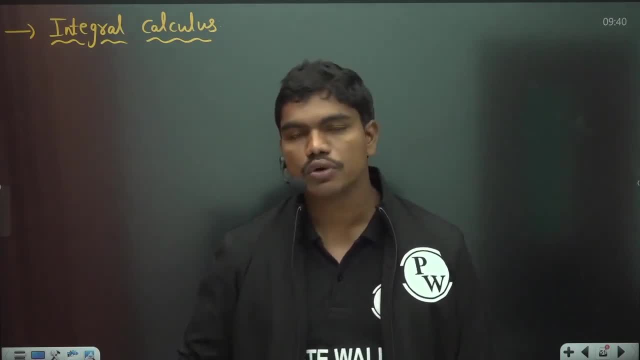 differentiation. let us suppose, if you don't know the derivative of any, don't know the derivative of any, don't know the derivative of any function. for example, if I given you some function. for example, if I given you some function. for example, if I given you some function and you don't know how to. 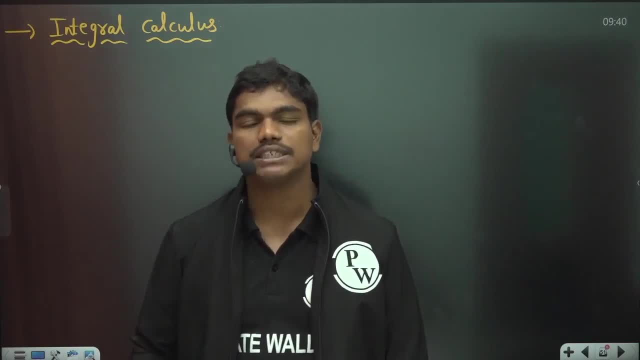 function and you don't know how to function and you don't know how to calculate the derivative. there is some calculate the derivative. there is some calculate the derivative. there is some standard procedure which is called the standard procedure, which is called the standard procedure, which is called the first principle. cut so these first. 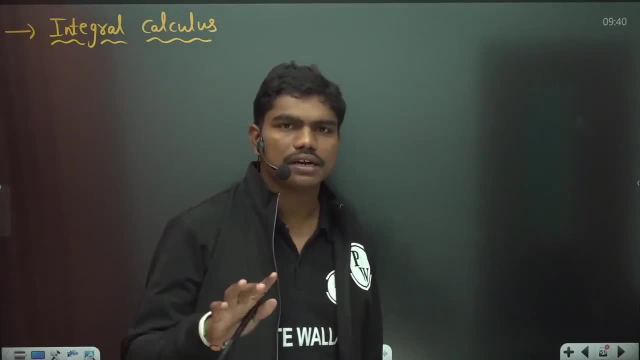 first principle cut. so these first first principle cut. so these first twins flow differentiation. so using first twins flow differentiation, so using first twins flow differentiation, so using first twins flow differentiation, you can twins flow differentiation, you can twins flow differentiation. you can calculate differentiation of any function, calculate differentiation of any function. 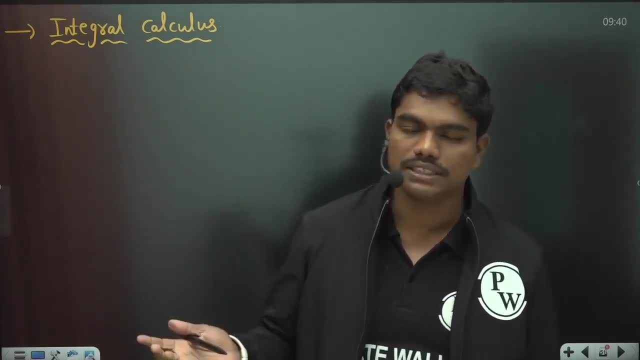 calculate differentiation of any function. but in integration you do not have such. but in integration you do not have such. but in integration you do not have such. you know principles. if I want to write, you know principles. if I want to write, you know principles. if I want to write: integration of sine X is minus, cos X plus. 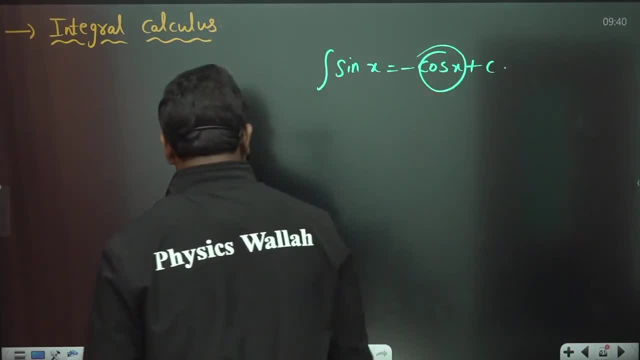 integration of sine X is minus cos X plus integration of sine X is minus cos X plus C. definitely should know differentiation C. definitely should know differentiation C. definitely should know differentiation of cos X is minus sine X. okay, so that's. of cos X is minus sine X. okay, so that's. 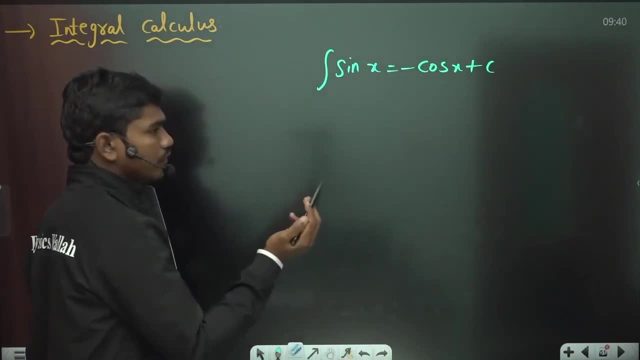 of cos X is minus sine X. okay, so that's why, since people don't remember this, why, since people don't remember this, why, since people don't remember this, David is very often they feel this. David is very often they feel this. David is very often they feel this integration is slightly complicated, but 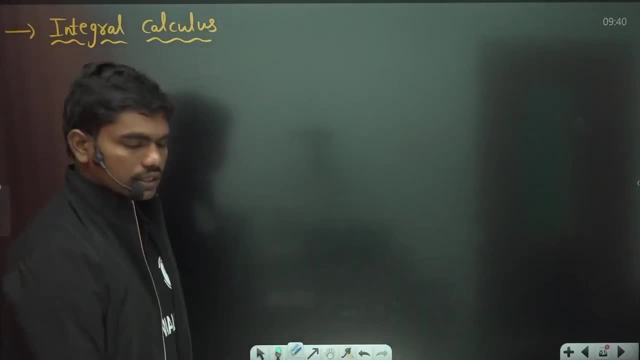 integration is slightly complicated, but integration is slightly complicated. but anyhow, you don't have any such things. anyhow, you don't have any such things. anyhow, you don't have any such things, you can always do the integration also. you can always do the integration also. you can always do the integration also, simply look. so first let us start with. 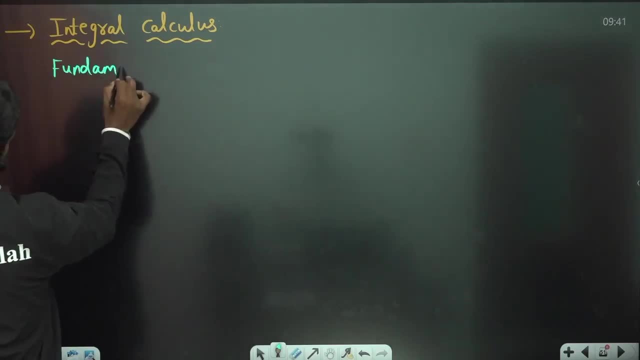 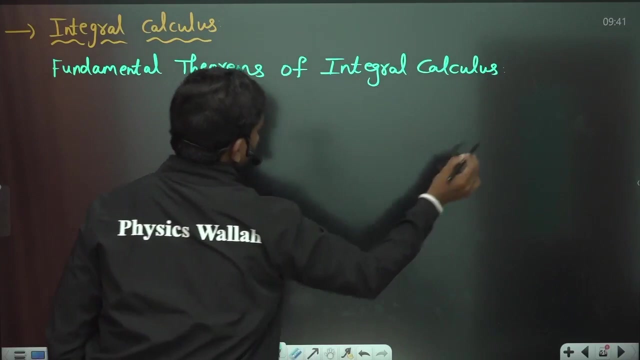 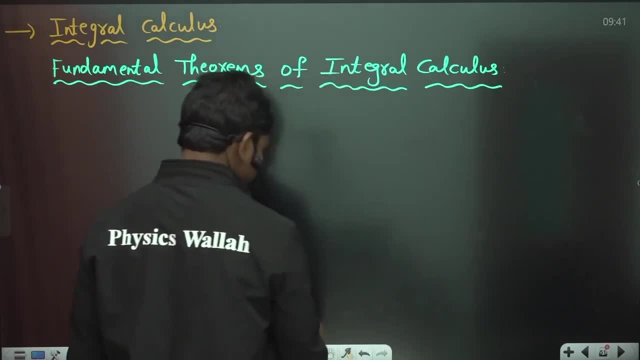 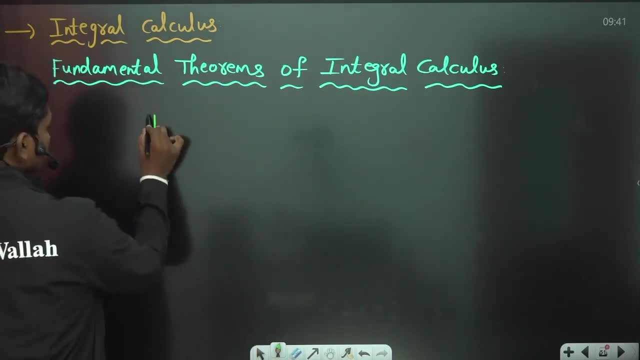 fundamental terms of integral calculus. so first the definition of integration. so first the definition of integration. so first the definition of integration. look if, look if, look. if capital F of X is anti derivative means, capital F of X is anti derivative means, capital F of X is anti derivative means the inverse of derivative. 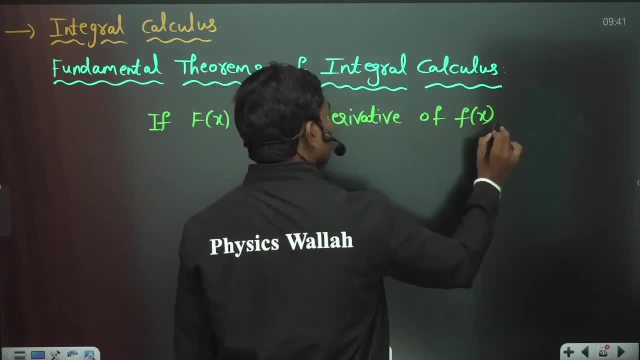 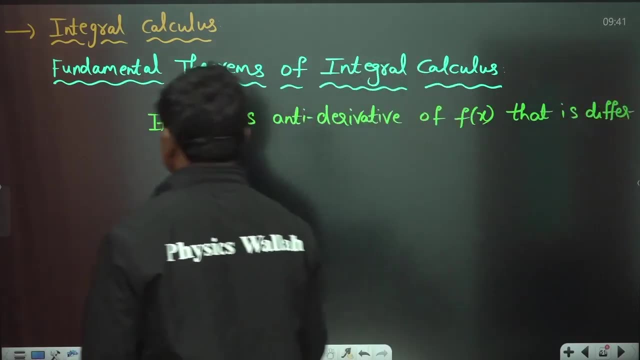 of F of X of F is anti derivative means the inverse of derivative of F of X. of F is anti derivative means the inverse of derivative of F of X. that is continuous. that is differentiable in that is continuous. that is differentiable in that is continuous. that is differentiable in that is differentiable. 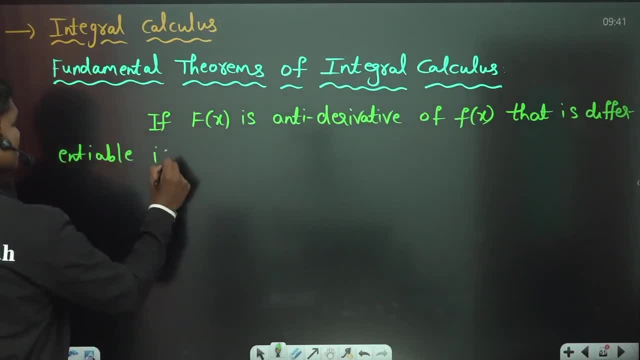 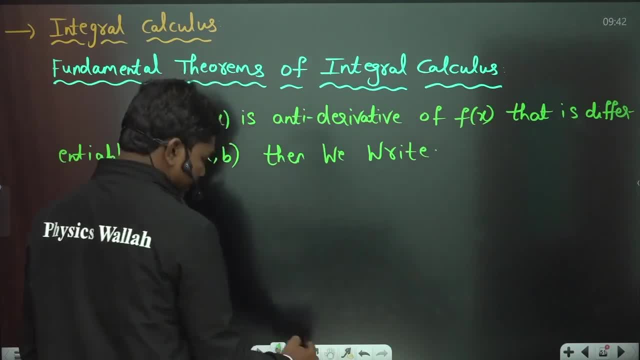 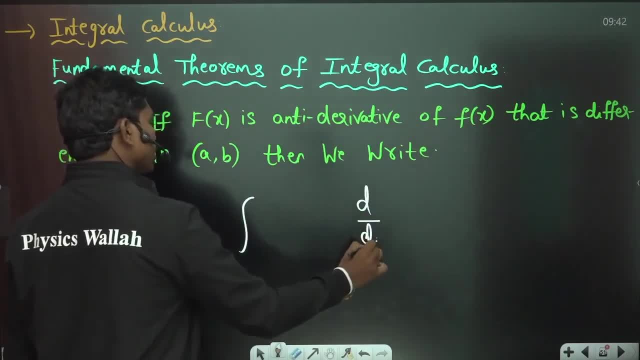 derivative means the inverse of derivative means the inverse of differentiation, differentiation, differentiation- normally. you see D by DX. this is normally. you see D by DX, this is normally. you see D by DX. this is differential operator. so this is inverse differential operator. so this is inverse differential operator. so this is inverse of this operation, so integral. 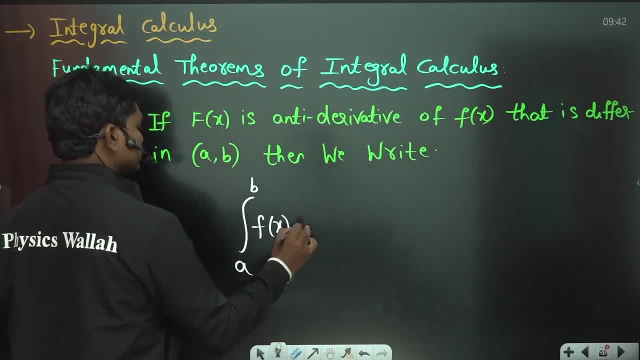 of this operation, so integral, of this operation, so integral. a to B. f of X DX. a to B. f of X DX. a to B: f of X DX is equal to capital F of B, minus is equal to capital F of B, minus is equal to capital F of B minus capital F of a. this is how we define the. 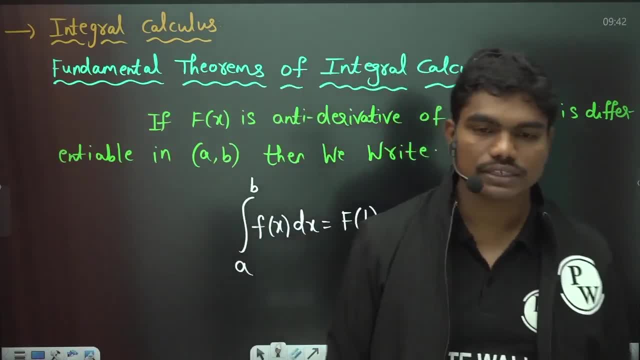 capital F of a. this is how we define the capital F of a. this is how we define the definition of integration. means there, definition of integration means there. definition of integration means there exists some function- capital F of X- such- exists some function- capital F of X, such. 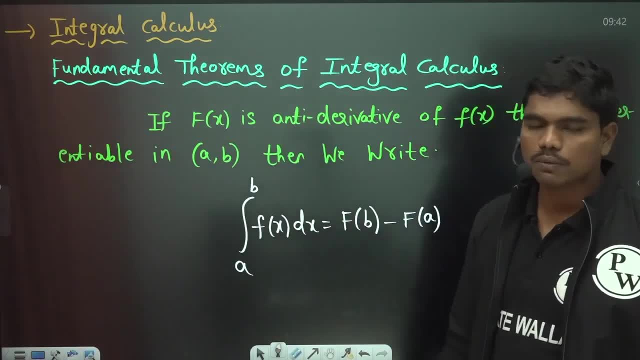 exists some function capital F of X such that this capital F of X is anti, that this capital F of X is anti, that this capital F of X is anti. derivative of this small f of X means derivative of this small f of X means derivative of this small f of X means what's the meaning if you differentiate? what's the meaning if you differentiate? what's the meaning if you differentiate this capital F of X? you again get small this capital F of X. you again get small this capital F of X. you again get small F of X. that's the meaning okay for F of X. that's the meaning okay for. 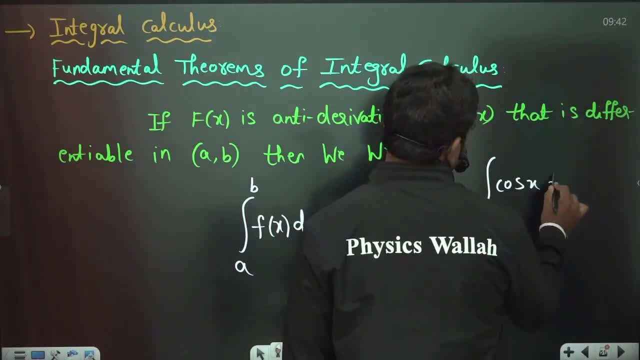 F of X. that's the meaning. okay, for example, if you write integral cos X- DX. example. if you write integral cos X- DX. example, if you write integral cos X- DX, sin X, for example, okay, you'll write this. sin X, for example. okay, you'll write this. 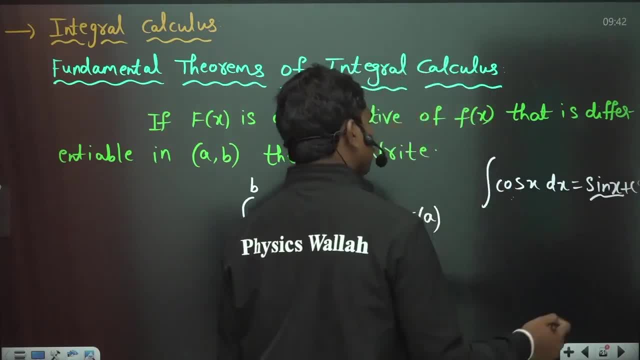 sin X, for example. okay, you'll write this: and here this sin X is called anti, and here this sin X is called anti, and here this sin X is called anti derivative of this cos X. why, if you derivative of this cos X? why, if you derivative of this cos X? why, if you differentiate this function, you will get. differentiate this function, you will get. differentiate this function, you will get this cos X again. okay. so that's the this cos X again. okay. so that's the this cos X again. okay. so that's the meaning basically and of course here it's meaning basically and of course here it's. 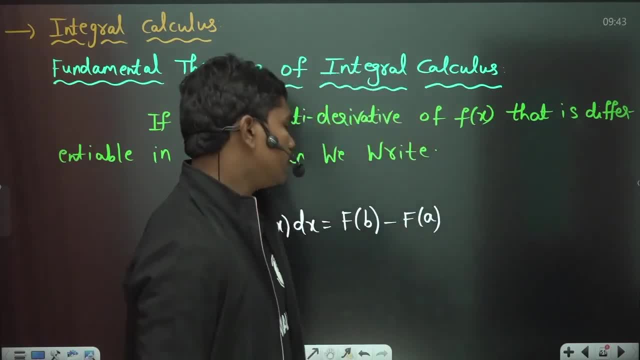 meaning basically and of course, here it's a definite integration. you have a definite integration. you have a definite integration. you have substituted the limits also, that's the substituted. the limits also, that's the substituted. the limits also. that's the only thing. now, if this is the case, then 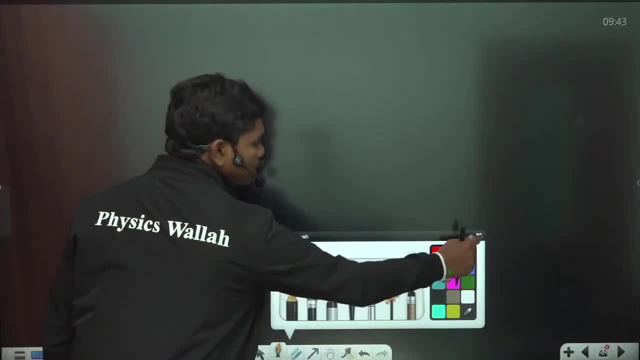 only thing now. if this is the case, then only thing now. if this is the case, then we'll define one very important theorem. we'll define one very important theorem. we'll define one very important theorem, which is called mean value, theorem of, which is called mean value theorem of. 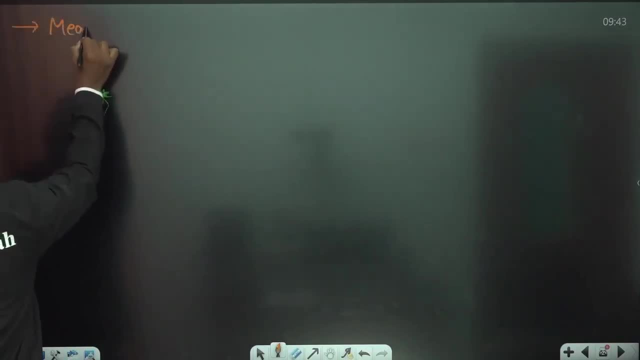 which is called mean value theorem of integration. so mean value theorem of integration. so mean value theorem of integration. so mean value theorem of integration. integration mean value theorem of integration. mean value theorem of integration. mean value theorem of integral calculus, integral calculus. integral calculus mean value theorem of integral calculus. 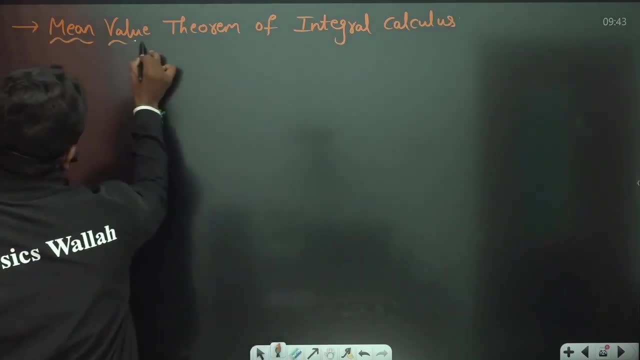 mean value, theorem of integral calculus. mean value, theorem of integral calculus. let us see mean value, theorem of integral. let us see mean value, theorem of integral. let us see mean value, theorem of integral calculus. mean value, theorem of integral calculus. mean value, theorem of integral calculus. look what is this. mean value, theorem of. 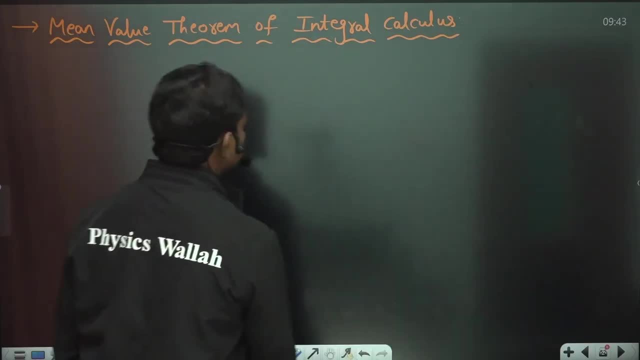 look what is this mean value. theorem of. look what is this mean value. theorem of integral calculus. I'll write the equation, integral calculus. I'll write the equation integral calculus. I'll write the equation then again, then again, I'll explain it geometrically: what's? I'll explain it geometrically, what's. 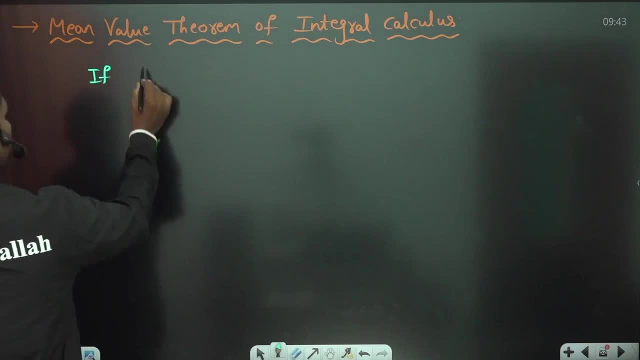 I'll explain it geometrically. what's happening? okay, so, if happening okay, so, if happening okay, so if f of x, f of x, f of x is continuous, is continuous, is continuous on a comma b, on a comma b, on a comma b, continuous on a comma b. and. 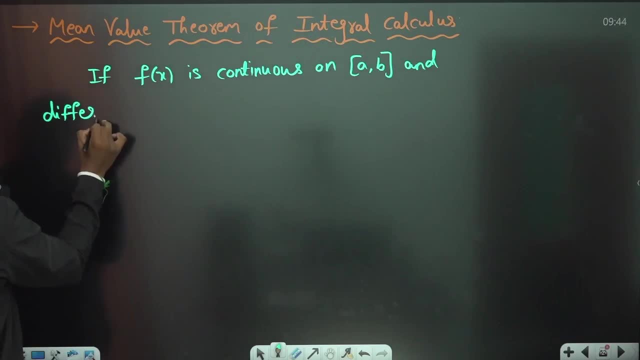 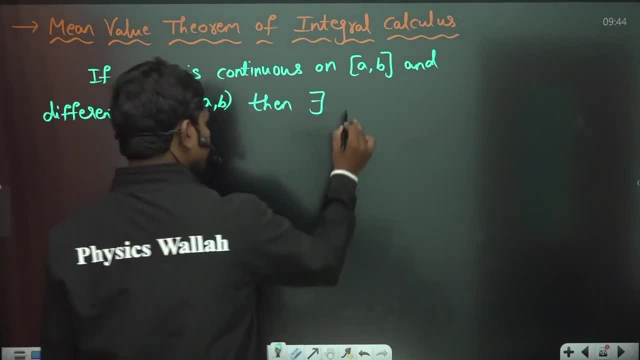 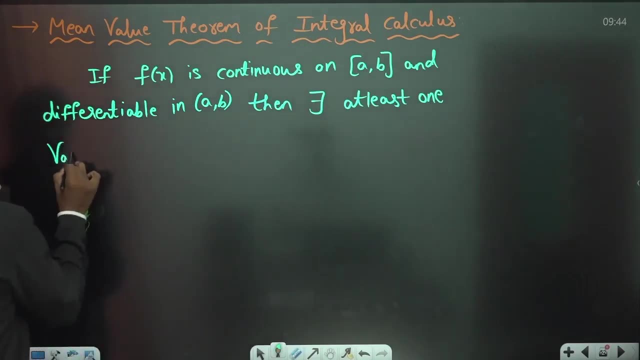 open interval a comma b. open interval a comma b. then, then, then, there exists, there exists, there exists at least one value C, at least one, at least one value C, at least one, at least one value C, at least one value C such that, such that value C, such that, such that. 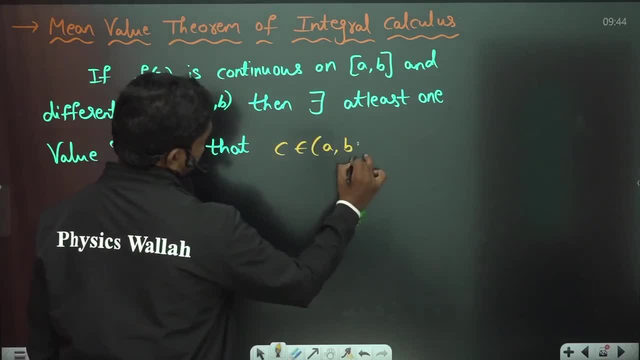 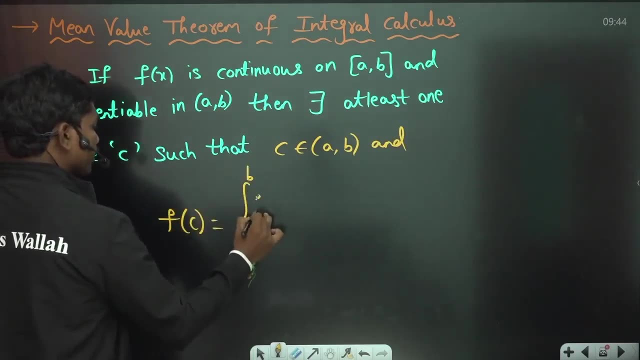 value C such that such that C belongs to a comma B and f of C. C belongs to a comma B and f of C C belongs to a comma B and f of C is equal to integral a to B. f of X DX is equal to integral a to B. f of X DX. 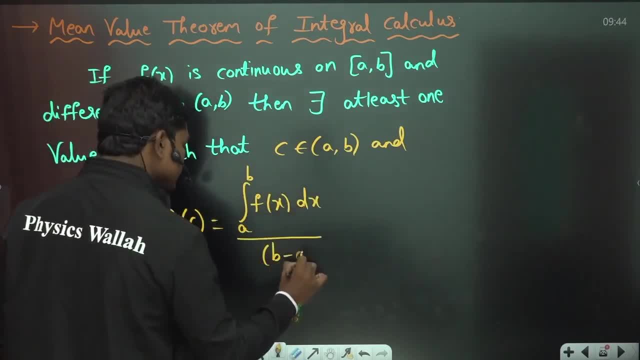 is equal to integral a to B, f of X, DX, divided by B minus. divided by B minus. divided by B minus a. this is called mean value term of a. this is called mean value term of a. this is called mean value term of integration, like how in differential. 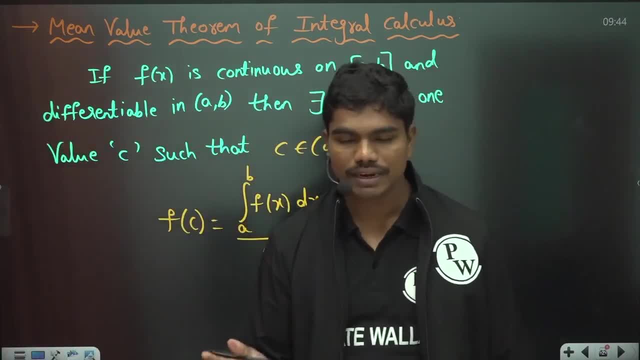 integration, like how in differential integration, like how in differential calculus. we have: f dash of C is equal to calculus. we have: f dash of C is equal to calculus. we have f dash of C is equal to f of V minus f of a, by B minus a. now, f of V minus f of a by B minus a. now, f of V minus f of a by B minus a. now, this is something similar to that. this is something similar to that. this is something similar to that integral here to be f of X, DX divided by. 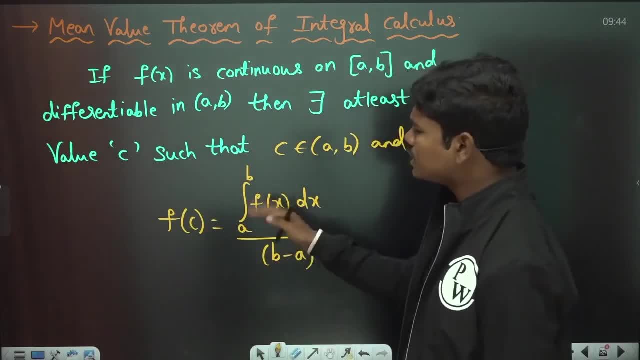 integral- here to be f of X- DX divided by integral, here to be f of X- DX divided by B minus a. now let us see what is the B minus a. now, let us see what is the B minus a. now, let us see what is the meaning of this. okay, now to know this. meaning of this. okay, now to know this meaning of this. okay, now to know this. you should know what is the meaning of. you should know what is the meaning of. you should know what is the meaning of this integral, here to be f of X? DX of this integral, here to be f of X? DX of. 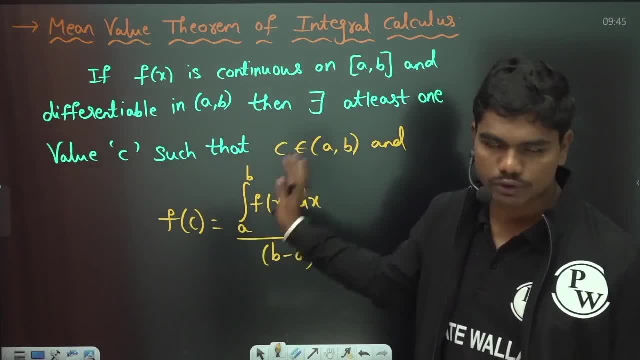 this integral here to be f of X, DX. of course we are. it will take simple case, course we are. it will take simple case, course we are. it will take simple case that f of X is positive to explain you, that f of X is positive to explain you. 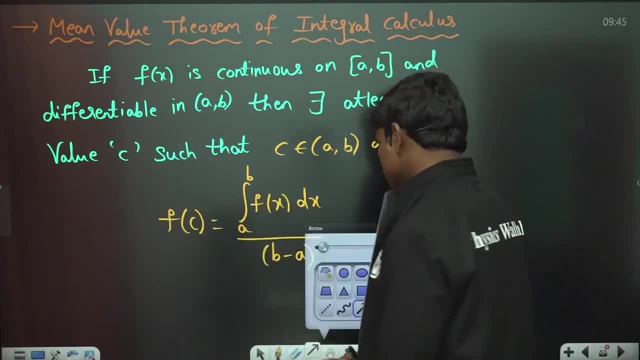 that f of X is positive. to explain you geometrically. but this holds good for geometrically, but this holds good for geometrically, but this holds good for any equation. okay, so let us see this. let us any equation. okay, so let us see this. let us any equation. okay, so let us see this. let us suppose this is your x-axis and this: 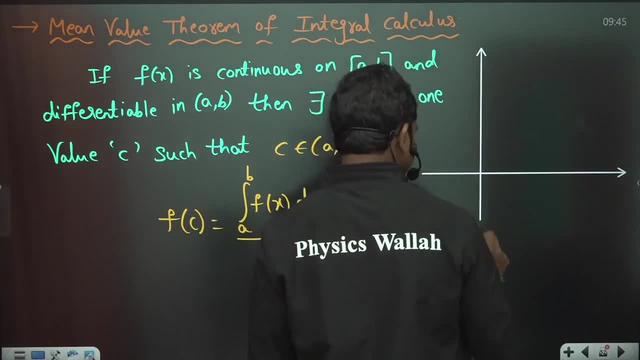 suppose this is your x-axis and this: suppose this is your x-axis and this is your y-axis, for example. so this is 0 X. Y is your y-axis, for example. so this is 0 X. Y is your y-axis, for example. so this is 0 X. Y is equal to f of X. now, if this is y is, is equal to f of X. now, if this is y, is is equal to f of X. now, if this is, y is equal to f of X. now, let us suppose you equal to f of X. now, let us suppose you equal to f of X. now, let us suppose you have some function like this, some random. 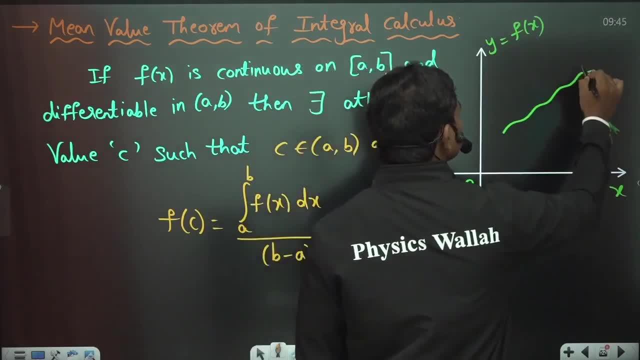 have some function like this, some random. have some function like this, some random. function y is equal to f of X. okay, so function y is equal to f of X. okay, so function y is equal to f of X. okay, so this is: y is equal to f of X. 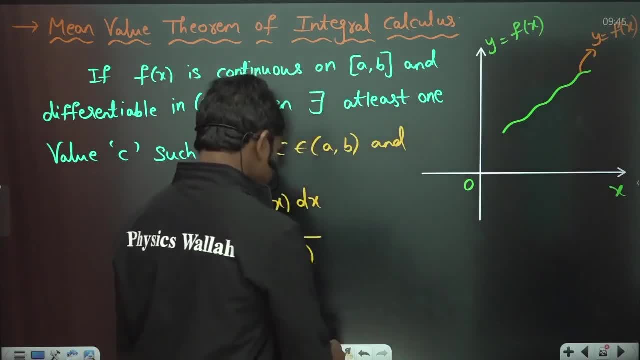 this is: y is equal to f of X. this is: y is equal to f of X. y is equal to f of X. now let us assume this: y is equal to f of X. now let us assume this: y is equal to f of X. now let us assume this point is: X is equal to a. 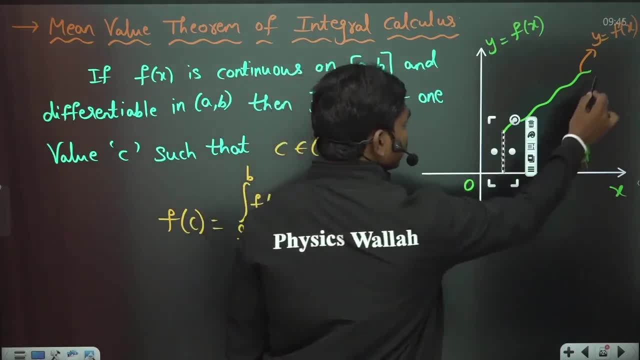 point is X is equal to a. point is X is equal to a. this point is X is equal to a and this- this point is X is equal to a and this- this point is X is equal to a and this point is X is equal to be, for example. so: 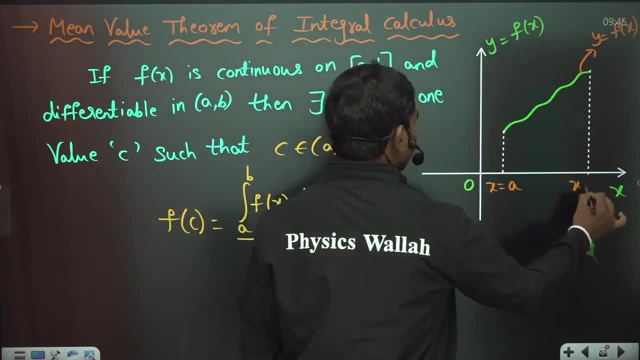 point is: X is equal to be, for example: so point is: X is equal to be, for example: so X is equal to a. X is equal to be: now X is equal to a. X is equal to be: now X is equal to a. X is equal to be now integral a to be f of X, DX will. 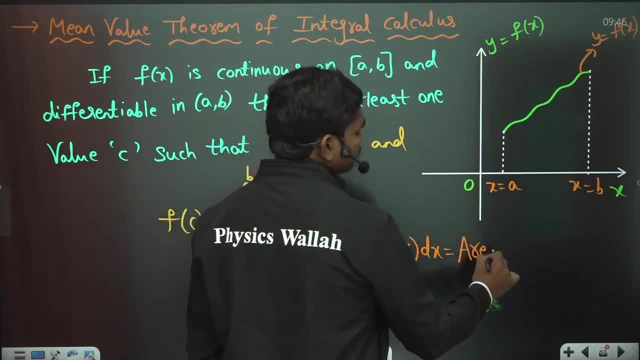 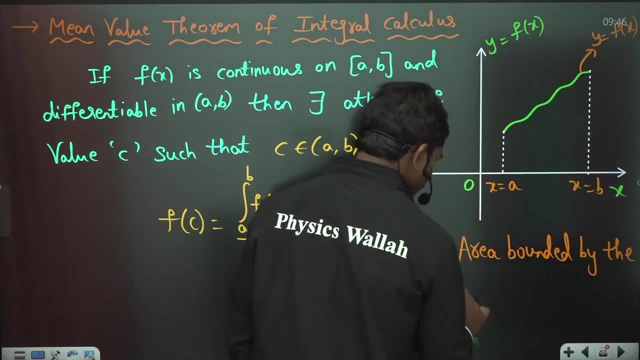 integral a to be f of X DX. will integral a to be f of X DX will actually give you area bounded by area. actually give you area bounded by area. actually give you area bounded by area bounded by the curves, area bounded by the bounded by the curves, area bounded by the. 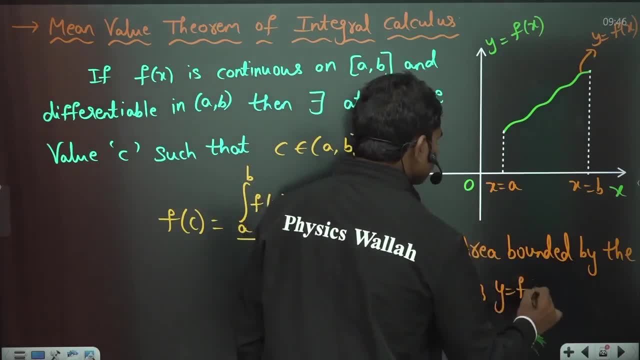 bounded by the curves. area bounded by the curves: y is equal to f of X. y is equal. curves: y is equal to f of X. y is equal. curves: y is equal to f of X. y is equal to 0 means basically: x axis, X is equal. 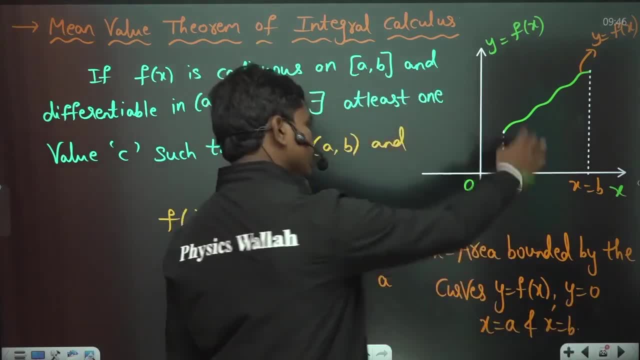 to 0 means basically: x axis X is equal to 0 means basically: x axis X is equal to a and X is equal to B. so this means to a and X is equal to B. so this means to a and X is equal to B. so this means basically, if you keep the shading, 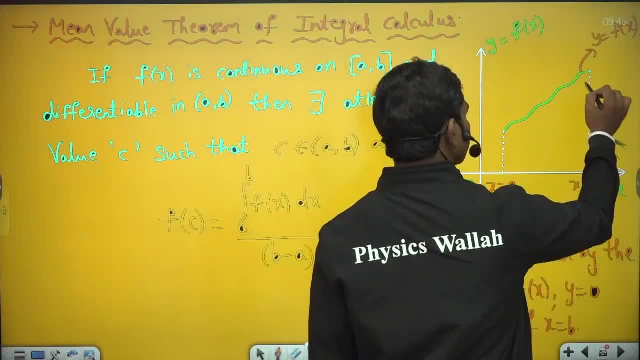 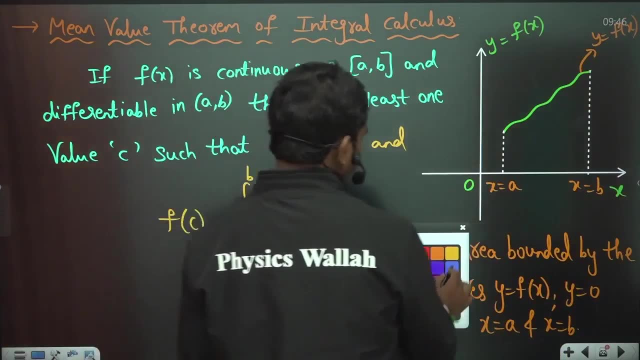 basically, if you keep the shading, basically, if you keep the shading, look the area looks like this. look the area looks like this. look the area looks like this: Oh, something happened just a minute. Oh, something happened just a minute. Oh, something happened just a minute. okay, fine, sorry. so, if you see the 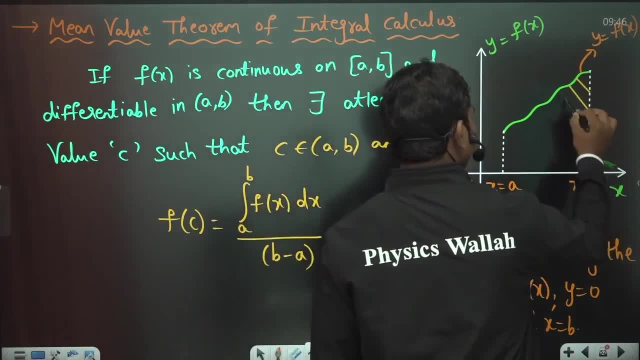 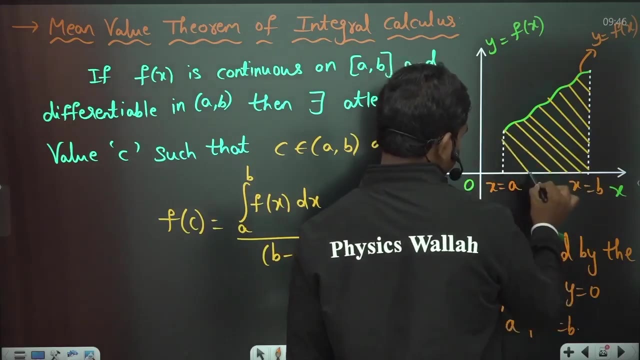 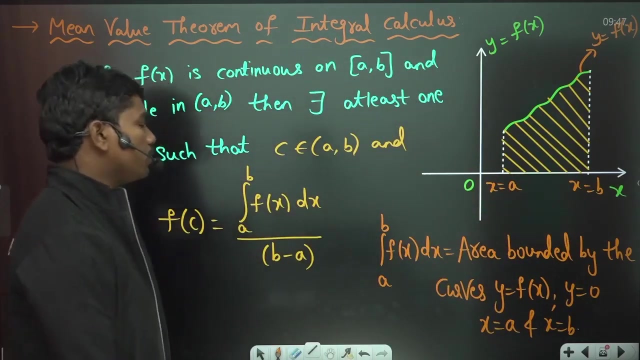 okay, fine, sorry so if you see the. okay, fine, sorry so if you see the shading, this is the area basically. this is the area basically now. this is the area, now what they are now. this is the area, now what they are now. this is the area, now what they are telling you. there exists at least one. 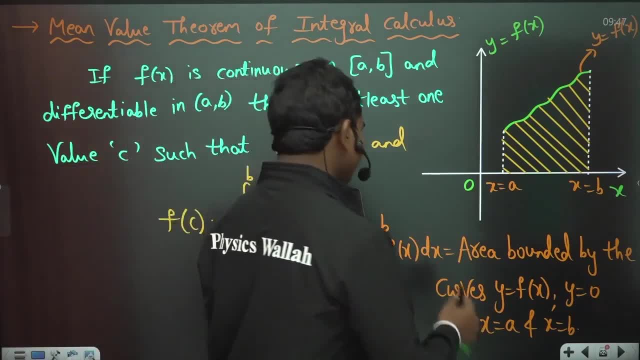 telling you there exists at least one, telling you there exists at least one point C, such that f of C into B minus a point C, such that f of C into B minus a point C, such that f of C into B minus a means, basically, f of C is equal to this. 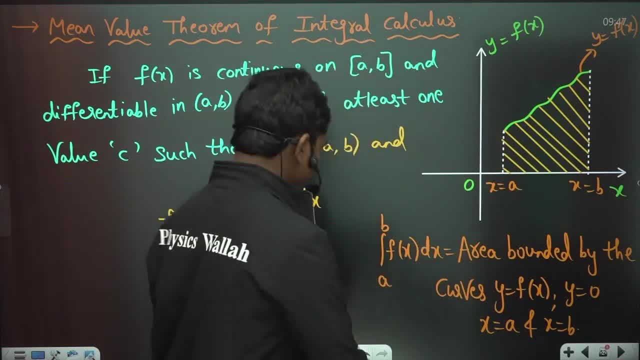 means basically, f of C is equal to. this means basically, f of C is equal to this: integral a to B. f of X- DX divided by B- integral a to B. f of X- DX divided by B. integral a to B. f of X- DX divided by B minus a. now let us see what's happening. 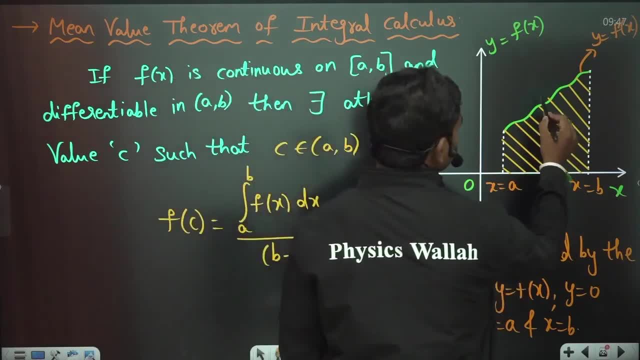 minus a now let us see what's happening. minus a now let us see what's happening here. let us suppose, if you take at least here, let us suppose if you take at least here, let us suppose, if you take at least one point, there exists at least one. 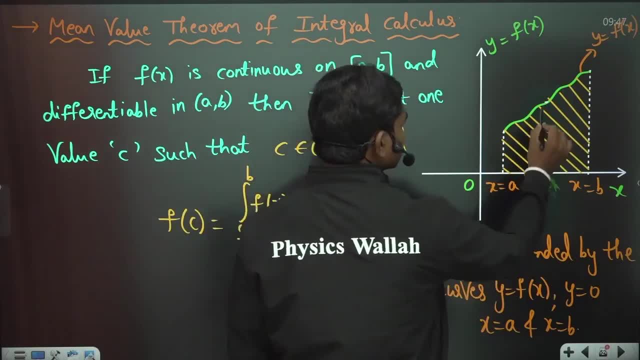 one point. there exists at least one one point. there exists at least one point such that: look, let us suppose if I point such that. look, let us suppose if I point such that. look, let us suppose if I take a horizontal line, if this is X is, take a horizontal line if this is X is. 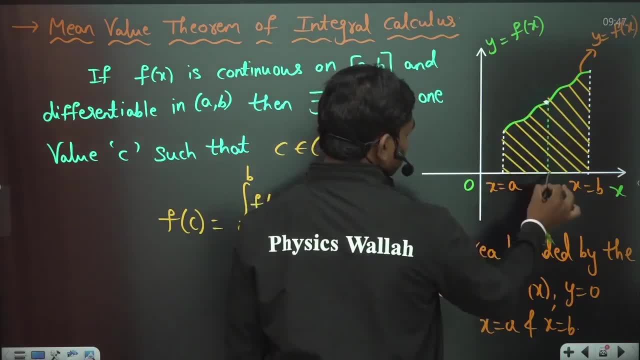 take a horizontal line. if this is X is equal to C, let us suppose if this is X is equal to C, let us suppose if this is X is equal to C, let us suppose if this is X is equal to C, equal to C, equal to C. this point here is: X is equal to C. now, 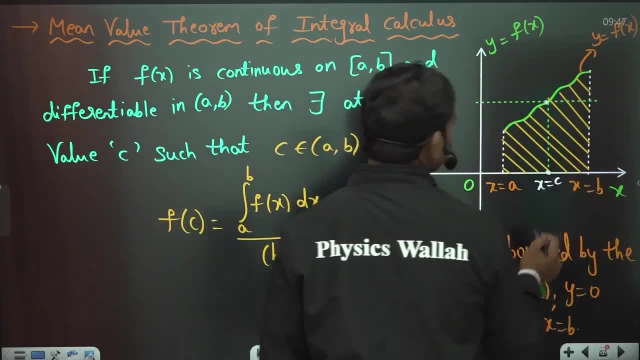 this point here is: X is equal to C. now this point here is: X is equal to C. now, f of C will be a straight line like this. f of C will be a straight line like this. f of C will be a straight line like this is on. so this: if you see something like 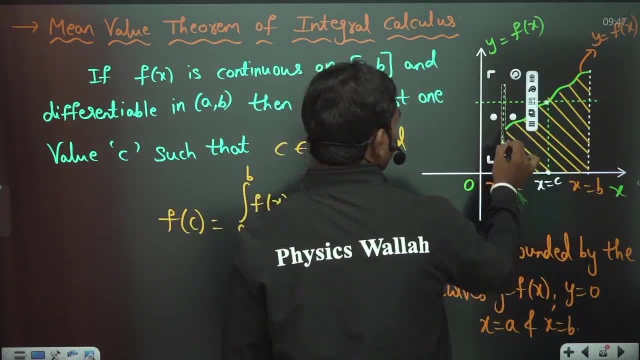 is on, so this: if you see something like is on, so this: if you see something like this: this is X is equal to a. this is X is equal to a. this is X is equal to a. this is X is equal to B. now let us suppose. 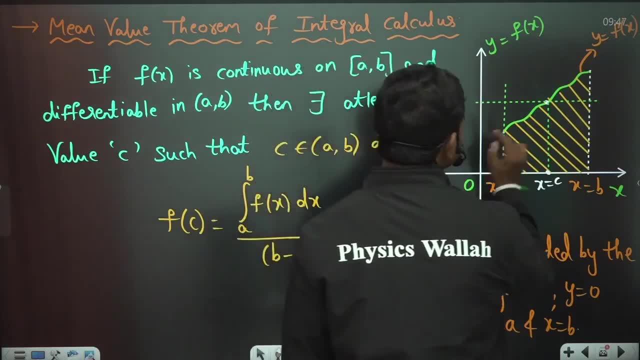 this is X is equal to B. now, let us suppose this is X is equal to B. now, let us suppose, if you take this segment, if you, if you take this segment, if you take this segment, f of C, for example, like f of C, for example, like: 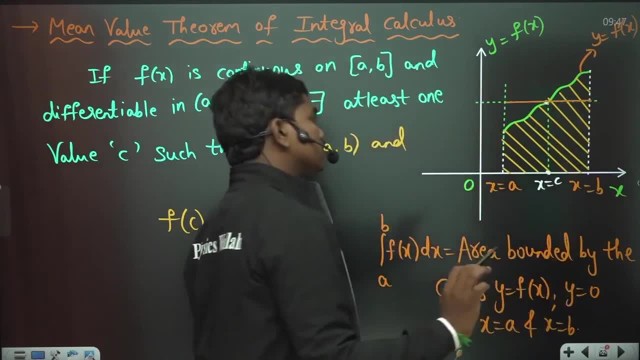 f of C, for example, like this: okay, so something like this now their this: okay, so something like this now their this: okay, so something like this: now their intention is to tell you that there intention is to tell you that there intention is to tell you that there exists at least one point C such that exists at least one point C, such that exists at least one point C, such that, of course, depending on the function, of course, depending on the function, of course, depending on the function, there can be many also, but at least at. there can be many also, but at least at. 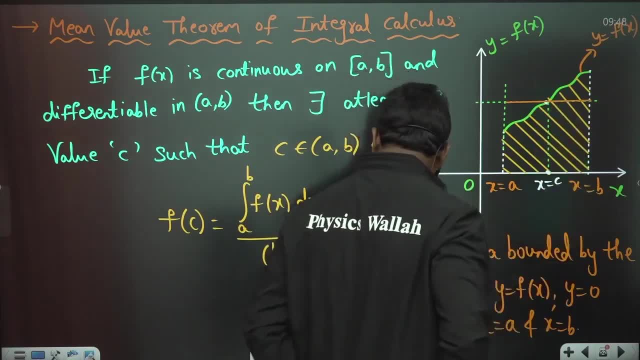 there can be many also, but at least at one location look. let us suppose, if you one location look. let us suppose, if you one location look. let us suppose, if you form this rectangle, for example, if you form this rectangle, for example, if you form this rectangle, for example, if you form this rectangle. okay, so let us. 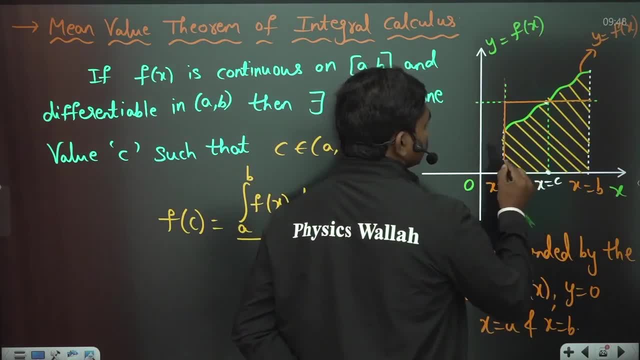 form this rectangle. okay, so let us form this rectangle. okay, so let us suppose you are forming this. suppose you are forming this. suppose you are forming this rectangle, like this rectangle, like this rectangle, like this: if you form the rectangle, so this is X. if you form the rectangle, so this is X. 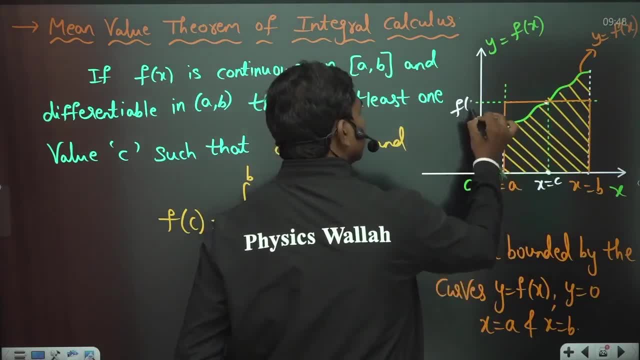 if you form the rectangle, so this is: X is equal to C. so definitely this value of is equal to C. so definitely this value of is equal to C. so definitely this value of Y is nothing but F of C. you know this. Y is nothing but F of C. you know this. 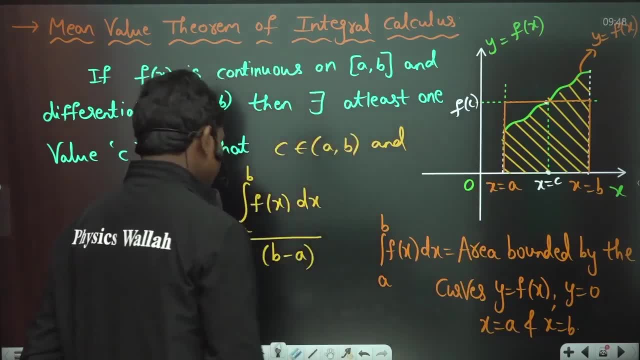 Y is nothing but F of C. you know this okay. so if you take the area of, okay, so if you take the area of, okay, so if you take the area of rectangle, area of rectangle is equal to F. rectangle area of rectangle is equal to F. rectangle area of rectangle is equal to F of C into B minus a, as on correct F of. 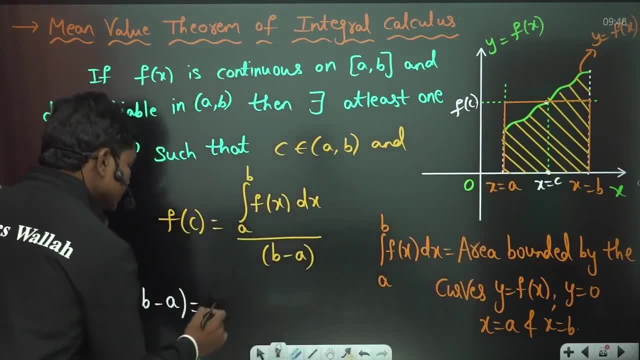 of C into B minus a, as on correct F of of C into B minus a, as on correct F of C is basically the height and B minus a is C is basically the height, and B minus a is C is basically the height and B minus a is with it, so this is equal to integral. 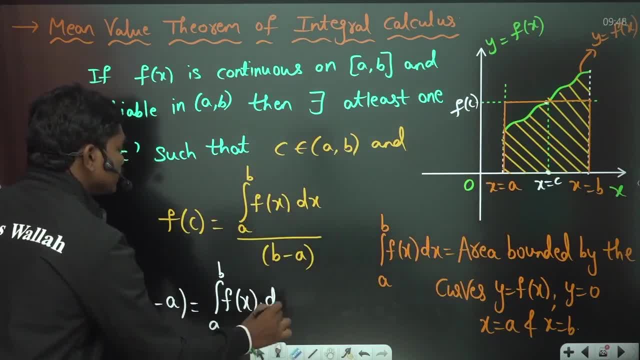 with it. so this is equal to integral with it. so this is equal to integral da to be F of X DX s on, because if you da to be F of X DX s on, because if you da to be F of X DX s on, because, if you see, definitely, if you keep on moving, 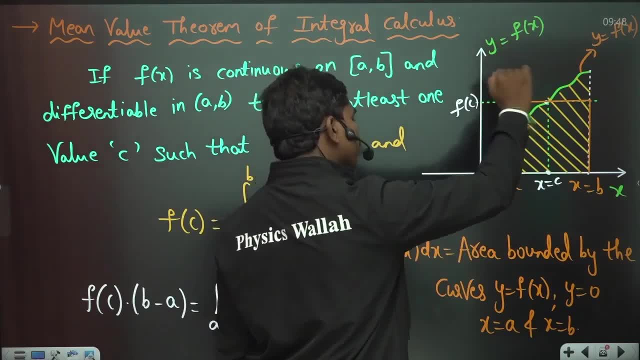 see, definitely, if you keep on moving, see, definitely, if you keep on moving this line up and down, at least at one, this line up and down, at least at one, this line up and down, at least at one point, there comes some location where point. there comes some location where 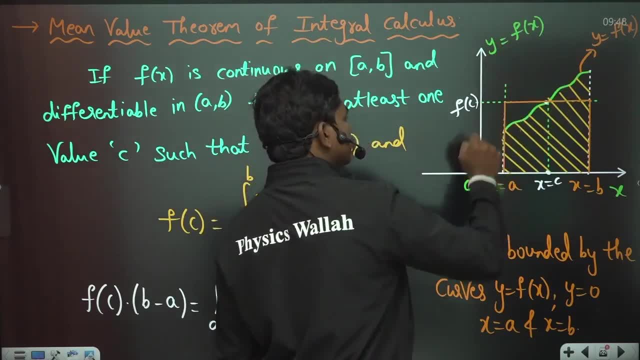 point, there comes some location where this area which you are losing here is this area which you are losing here, is this area which you are losing here is actually compensated. here s on here actually compensated. here s on here actually compensated. here s on here. there's a blank and here it is shaded. 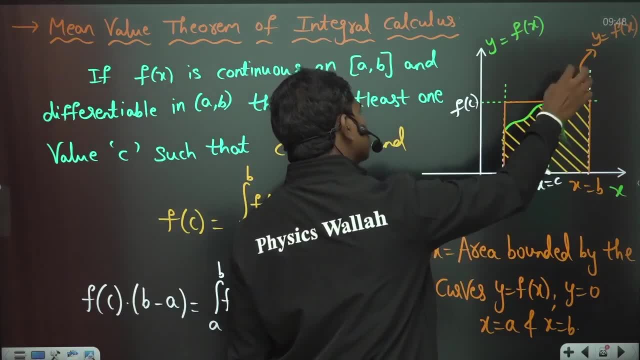 there's a blank and here it is shaded. there's a blank and here it is shaded. when you are taking the area of, when you are taking the area of, when you are taking the area of a tangle, you are losing this area. so this a tangle. you are losing this area. so this: 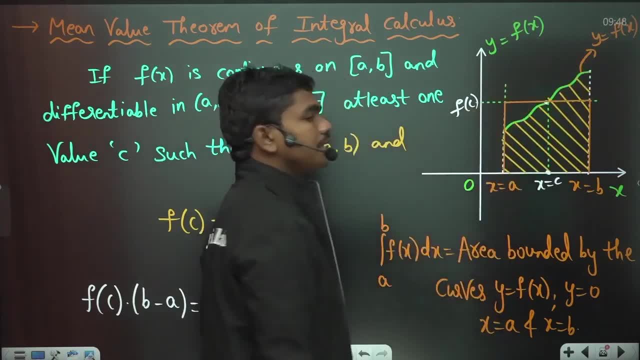 a tangle. you are losing this area, so this lost area can be compensated in this lost area can be compensated in this lost area can be compensated in this gap here. so they exist at least one such gap here. so they exist at least one such gap here. so they exist at least one such point, such that these two gets. 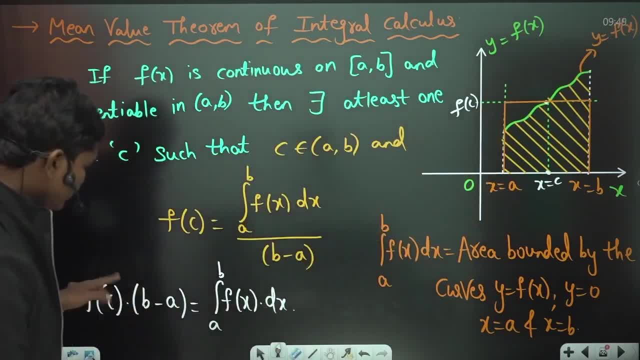 point such that these two gets point, such that these two gets compensated each other. so that's how you compensated each other. so that's how you compensated each other. so that's how you have this area of that tangle is same. have this area of that tangle is same. have. this area of that tangle is same as shaded area part. and if you bring as shaded area part and if you bring as shaded area part and if you bring this B minus C to the right hand side, this B minus C to the right hand side, 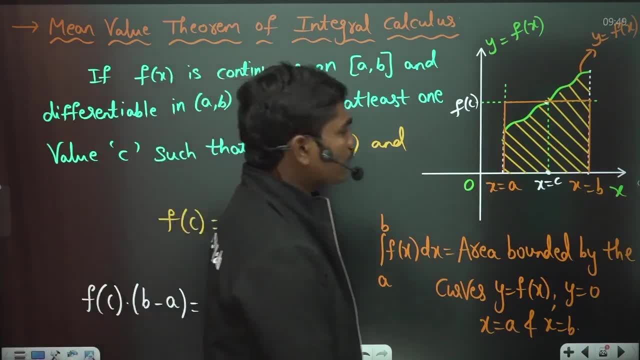 this: B minus C to the right hand side. this is the equation that is with you. this is the equation that is with you. this is the equation that is with you. okay, so it's a simple geometrical. okay, so it's a simple geometrical. okay, so it's a simple geometrical understanding, but again, it's a very 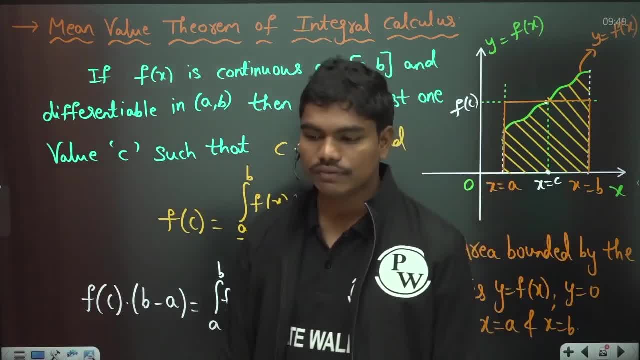 understanding, but again, it's a very understanding, but again it's a very powerful theorem. why because mechanical powerful theorem. why because mechanical powerful theorem? why because mechanical students might know this actually, when students might know this actually, when students might know this actually when you do something called a Rankine cycle. you do something called a Rankine cycle. you do something called a Rankine cycle in wrapper power cycles. when you plot in wrapper power cycles, when you plot in wrapper power cycles, when you plot the TS diagram, basically, if you see in the TS diagram, basically if you see in: 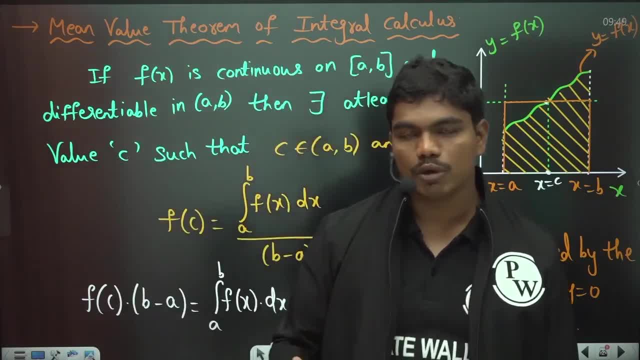 the TS diagram. basically, if you see in boiler it's a constant pressure heat, boiler it's a constant pressure heat, boiler it's a constant pressure heat addition. okay. so in case of boiler it's addition. okay. so in case of boiler it's addition, okay. so in case of boiler, it's constant pressure heat addition. so in 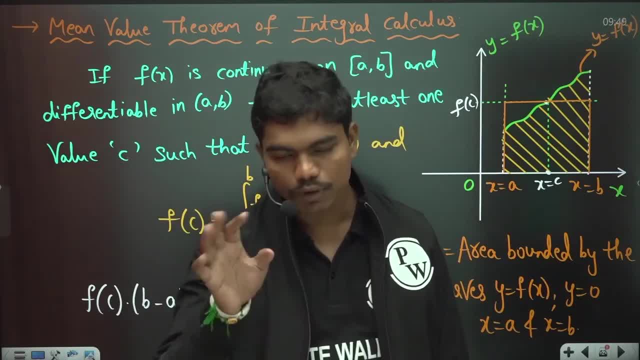 constant pressure heat addition. so in constant pressure heat addition. so in case of constant pressure heat addition, case of constant pressure heat addition, case of constant pressure heat addition. your temperature is not constant, correct. your temperature is not constant. correct, your temperature is not constant. correct, as you keep on adding heat, your. 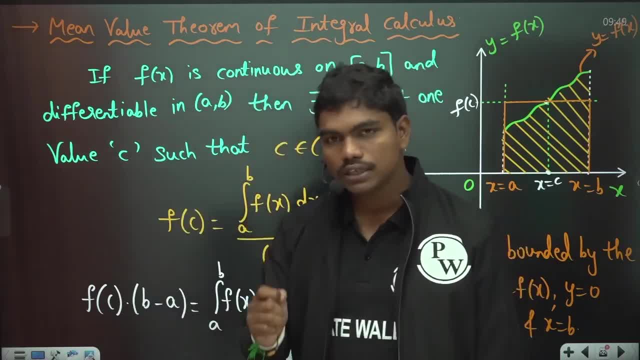 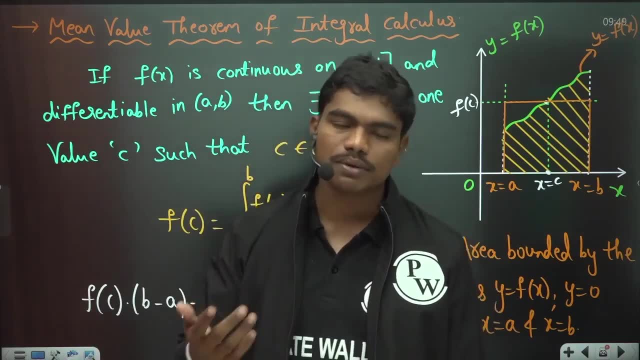 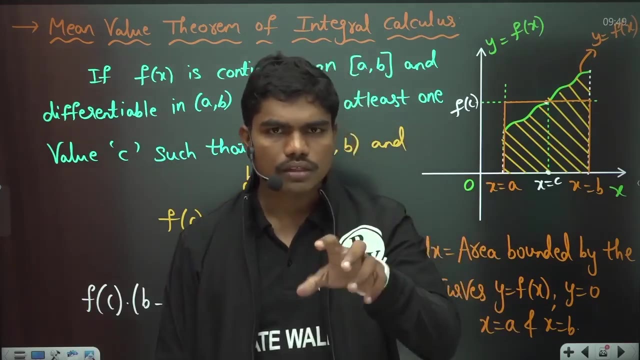 as you keep on adding heat, your, as you keep on adding heat, your temperature keeps on increasing, so in temperature keeps on increasing, so in temperature keeps on increasing. so, in such case, what happens? since, if you such case, what happens since, if you such case, what happens since, if you? so I am talking some mechanical things, but 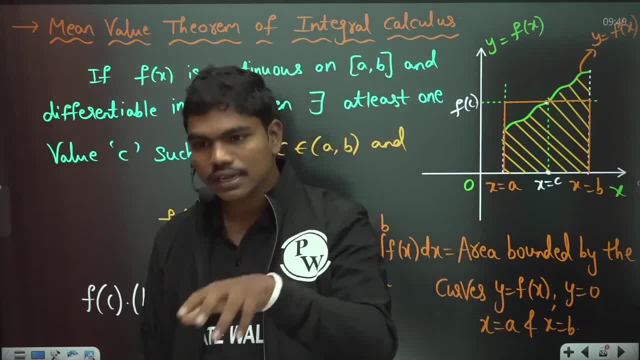 so I am talking some mechanical things. but so I am talking some mechanical things, but yeah, so if some of you are there, you, yeah. so if some of you are there, you yeah. so if some of you are there, you can connect to it. so, if you see, this mean. 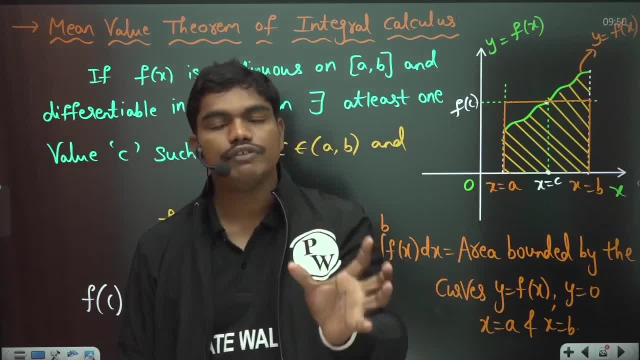 can connect to it. so if you see this mean can connect to it. so if you see this mean, temperature of heat addition is that temperature of heat addition is that temperature of heat addition is that temperature at which, if you supply, the temperature at which, if you supply the 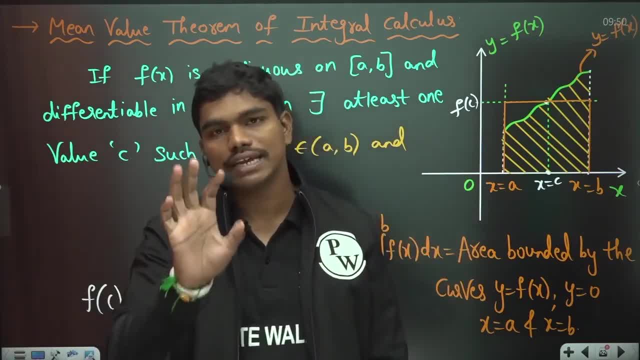 temperature at which, if you supply the same amount of heat at that temperature, same amount of heat at that temperature, same amount of heat at that temperature, your efficiency of the cycle I mean same. your efficiency of the cycle: I mean same. your efficiency of the cycle I mean same. work output: I mean same. okay, so that. 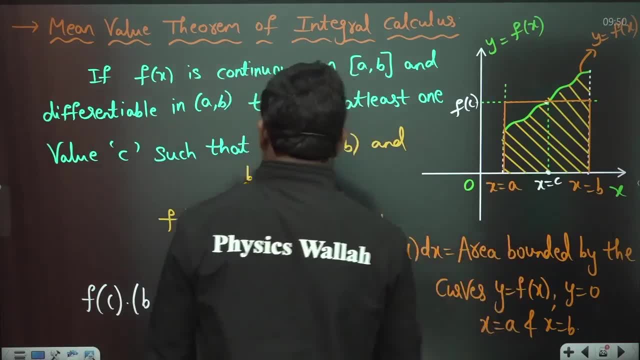 work output. I mean same. okay, so that work output. I mean same. okay, so that mean. temperature of heat addition is mean. temperature of heat addition is mean. temperature of heat addition is actually calculated using this equation, actually calculated using this equation, actually calculated using this equation. T mean is equal to the heat supplied by. 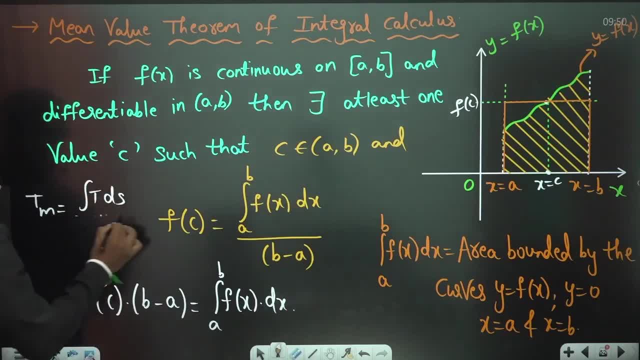 T mean is equal to the heat supplied by T mean is equal to the heat supplied by change in entropy at that place. so TDS change in entropy at that place. so TDS change in entropy at that place. so TDS, integral TDS gives you the heat. 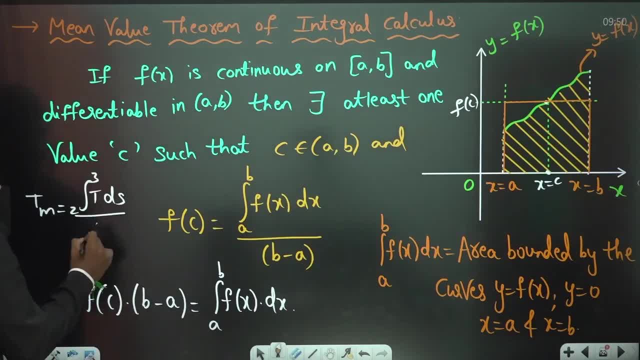 integral TDS gives you the heat. integral TDS gives you the heat interaction between state 2 to 3 boiler interaction, between state 2 to 3 boiler interaction between state 2 to 3 boiler states and Delta S, which means s2, s3. 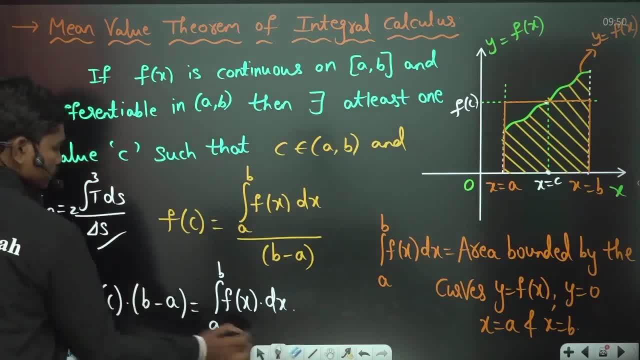 states and Delta S, which means s2, s3 states and Delta S, which means s2, s3 minus s2. so this equation is something minus s2. so this equation is something minus s2. so this equation is something similar to this. okay, so both these are. 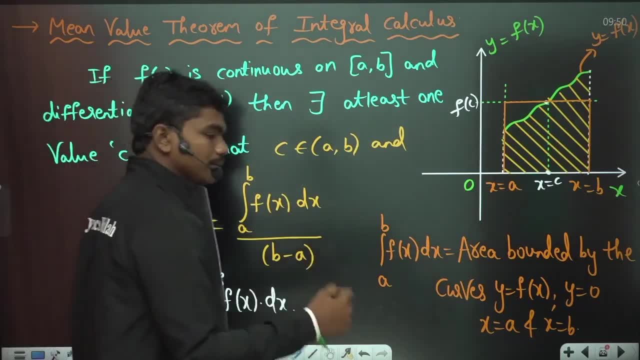 similar to this. okay, so both these are similar to this. okay, so both these are same. actually so mean. temperature of same. actually so mean temperature of same. actually so mean temperature of heat addition is actually calculated. heat addition is actually calculated. heat addition is actually calculated using this mean value. theorem of. 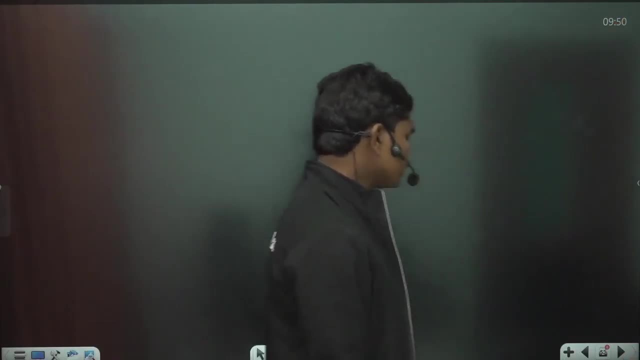 using this mean value theorem of using this mean value theorem of integration. okay, so now let us go for integration. okay, so now let us go for integration. okay, so now let us go for some other part: Newton Leibniz, rule one. some other part: Newton Leibniz, rule one. 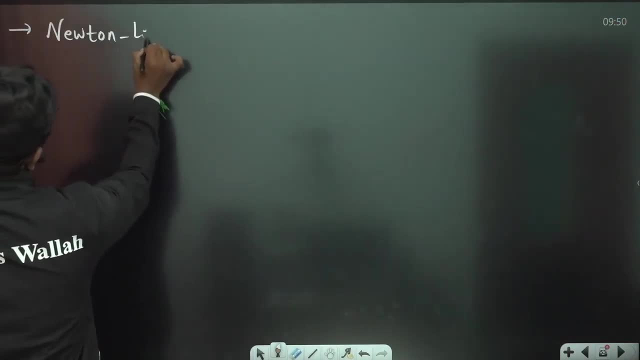 some other part. Newton, Leibniz rule- one very important tool again. so Newton, very important tool again. so Newton, very important tool again. so Newton, Leibniz rule actually okay, so let us see Leibniz rule actually okay, so let us see Leibniz rule actually okay. so let us see what is this Newton's Leibniz rule? okay, so 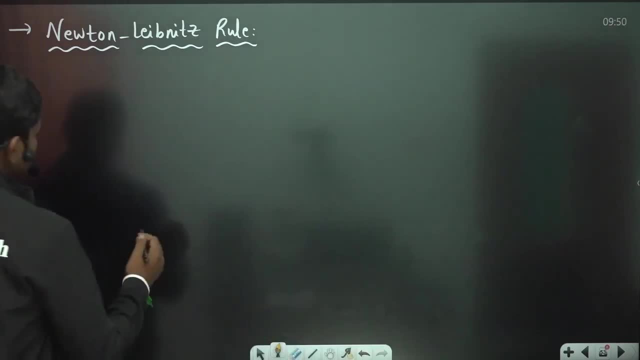 what is this Newton's Leibniz rule? okay, so what is this Newton's Leibniz rule? okay, so let us see this Newton's Leibniz rule. let us see this Newton's Leibniz rule. let us see this Newton's Leibniz rule. this is basically differentiation of. 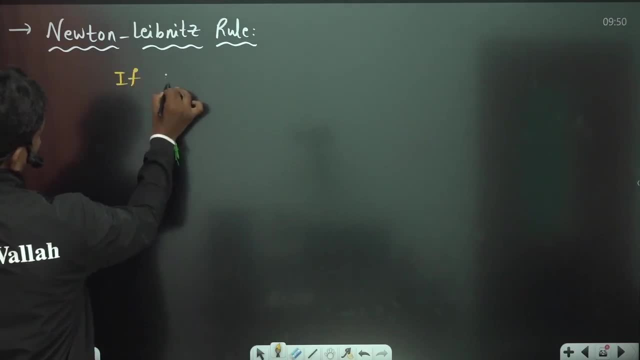 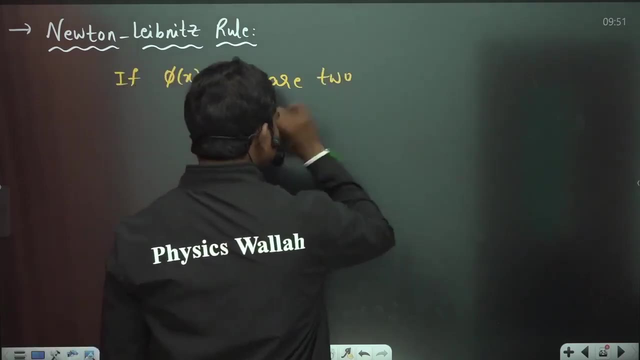 this is basically differentiation of, this is basically differentiation of integration. okay. so, if integration, okay, so, if integration okay. so if Phi of X comma psi of X are true, Phi of X comma psi of X are true, Phi of X comma psi of X are true, differentiable functions. 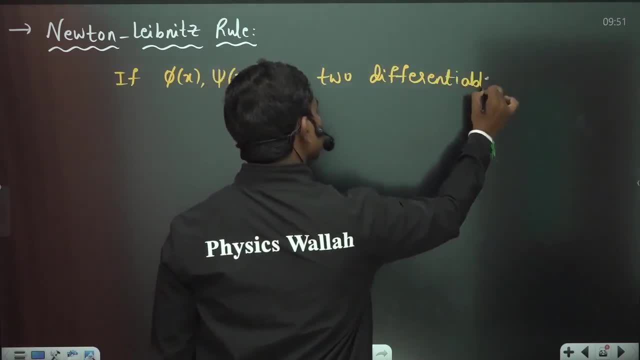 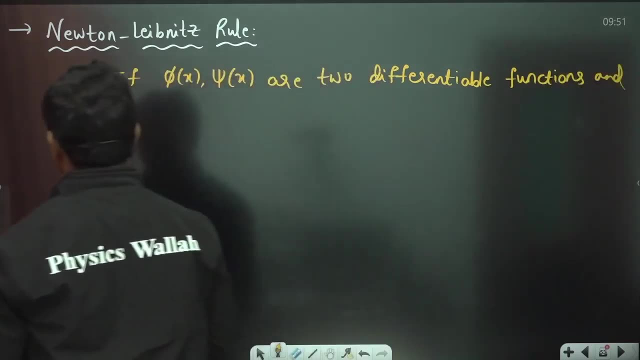 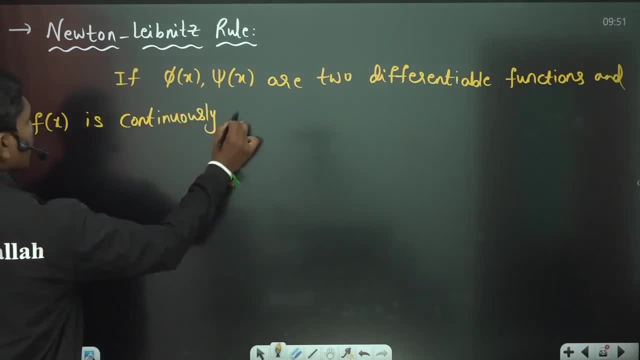 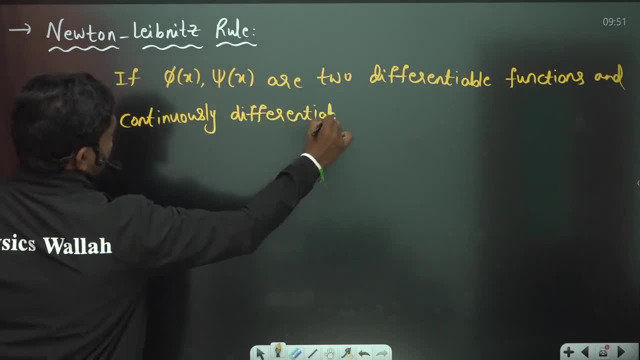 what's the meaning of that? you can integrate this f of X very easily. integrate this f of X very easily. integrate this f of X very easily. differentiable then. then then d by dx of differentiable, then then d by dx of differentiable, then then d by dx of d by dx of integral Phi of X to Psi of X. 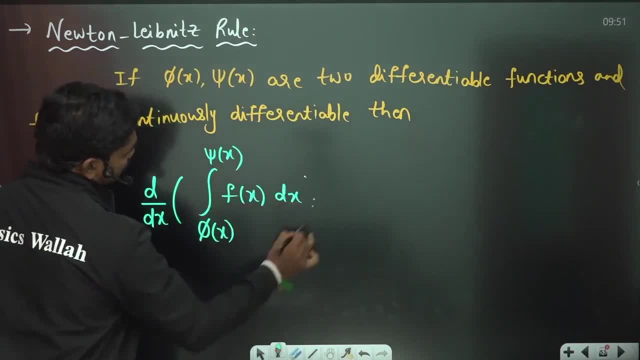 d by dx of integral Phi of X to Psi of X. d by dx of integral Phi of X to Psi of X. f of X dx means basically you have f of X. dx means basically you have f of X. dx means basically, you have variable limits and you are differentiating. 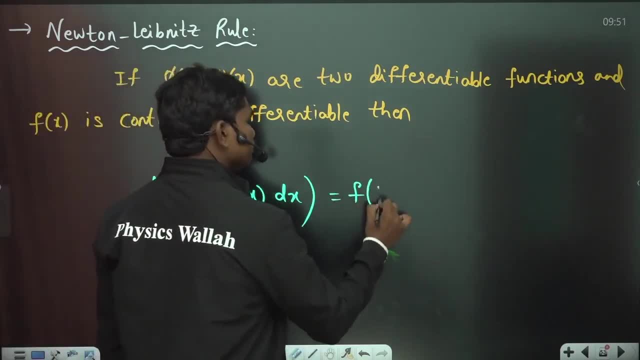 variable limits and you are differentiating variable limits and you are differentiating this. okay, so this is actually equal to this. okay, so this is actually equal to this. okay, so this is actually equal to f of Psi of X means you see you might have. f of Psi of X means you see you might have. 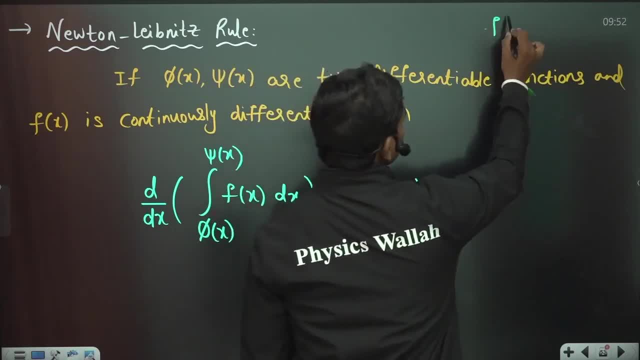 f of Psi of X means. you see, you might have studied about composite functions. cut studied about composite functions. cut. studied about composite functions. cut means, for example, if I say f of X is means, for example, if I say f of X is means, for example, if I say f of X is equal to X, square G of X is equal to sine. 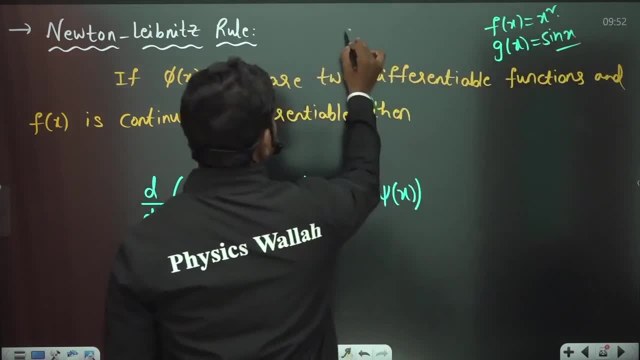 equal to X. square G of X is equal to sine, equal to sine X, for example. then if I write G of f of X, X, for example, then if I write G of f of X, X, for example, then if I write G of f of X, for example, let us suppose: if I write: 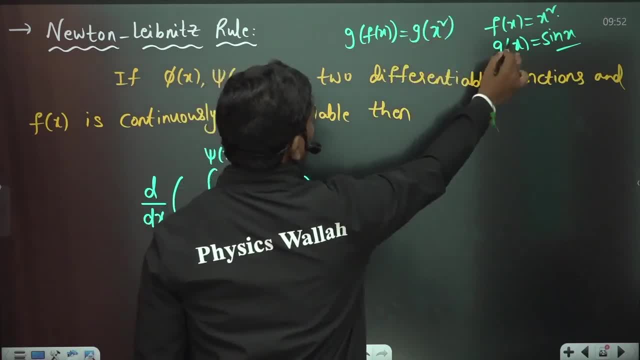 for example. let us suppose if I write, for example, let us suppose if I write like this, then what happens? this is G of like this, then what happens? this is G of like this, then what happens? this is G of X square, so G of X is sine X, so G of X. X square. so G of X is sine X. so G of X X square. so G of X is sine X. so G of X is square sine X square. this is how you is square sine X square. this is how you is square sine X square. this is how you work out the composite functions. 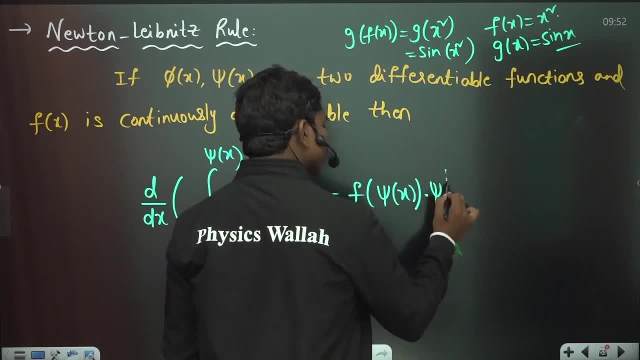 work out the composite functions. work out the composite functions actually so. f of Psi of X into Psi dash actually so. f of Psi of X into Psi dash actually so. f of Psi of X into Psi, dash of X minus F of Phi of X into Phi dash. 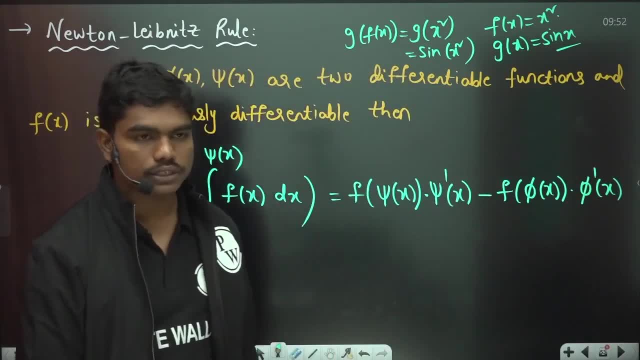 of X minus F of Phi of X into Phi dash of X, minus F of Phi of X into Phi dash of X. okay, so this is called Newton's of X. okay, so this is called Newton's of X. okay, so this is called Newton's Leibniz rule, and you know, this is very. Leibniz rule and you know this is very Leibniz rule and you know this is very important rule actually, because many important rule actually, because many important rule actually, because many times, especially if you are writing XC times, especially if you are writing XC- 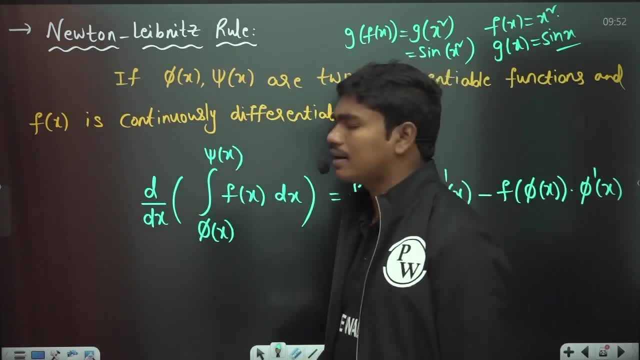 times, especially if you are writing XC and all. there are many questions on this and all. there are many questions on this and all. there are many questions on this. Newton's Leibniz rule- okay so. and if you Newton's Leibniz rule, okay so. and if you? Newton's Leibniz rule, okay. so, and if you notice Newton's Leibniz rule, some nice notice, Newton's Leibniz rule, some nice notice, Newton's Leibniz rule, some nice questions in integration can be solved. questions in integration can be solved. 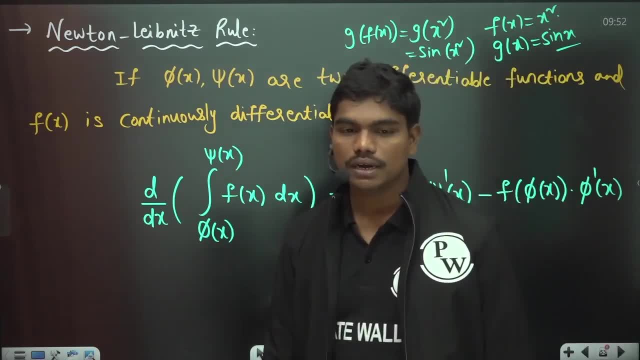 questions in integration can be solved easily. okay, we'll see when we solve the easily. okay, we'll see when we solve the easily. okay, we'll see when we solve the P? Y Q C's or something. okay, I'm P? Y Q C's or something. okay, I'm. 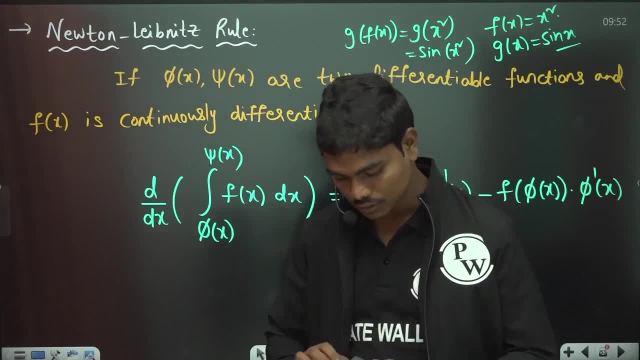 P, Y, Q, C's or something. okay, I'm continuously checking, because I'm continuously checking, because I'm continuously checking, because I'm doubting my battery is going off, or what, doubting my battery is going off, or what doubting my battery is going off, or what. okay, so yeah, we have enough battery. good. 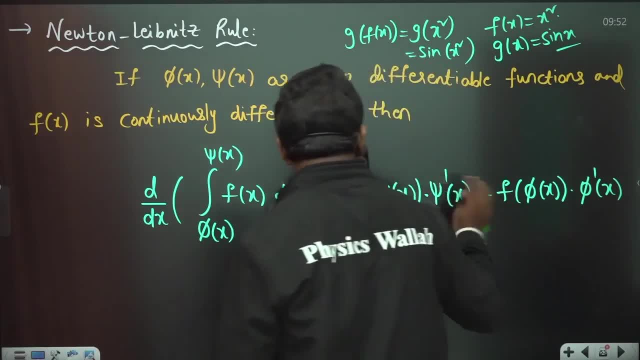 okay. so yeah, we have enough battery, good. okay. so yeah, we have enough battery, good. so D by DX of this thing is basically so. D by DX of this thing is basically so. D by DX of this thing is basically equal to this variation now. so, basically equal to this variation now. so basically. 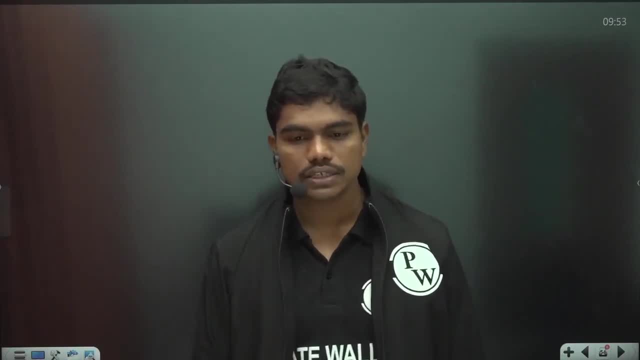 equal to this variation now. so, basically, these are some fundamental theorems, and these are some fundamental theorems, and these are some fundamental theorems and rules of this integral calculus now one. rules of this integral calculus now one. rules of this integral calculus now one. you know, I will give you some standard. 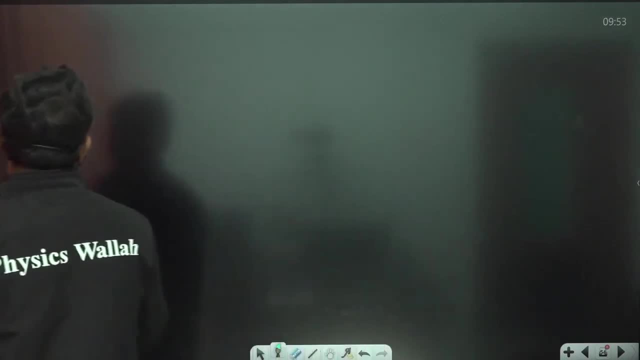 you know I will give you some standard. you know I will give you some standard, integral, standard integrals which could integral standard integrals, which could integral standard integrals which could be helpful to you. so some standard be helpful to you, so some standard be helpful to you. so some standard integrals. 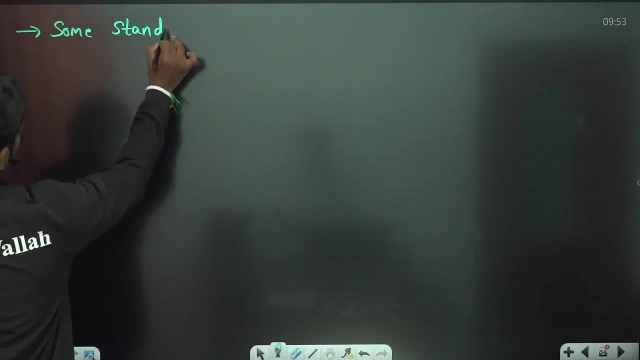 integrals, integrals, some standard integrals, some standard integrals. okay, like how? some standard integrals. okay, like how, some standard integrals. okay, like how. we have given you some standard derivatives. we have given you some standard derivatives. we have given you some standard derivatives. let us now work the reverse of. 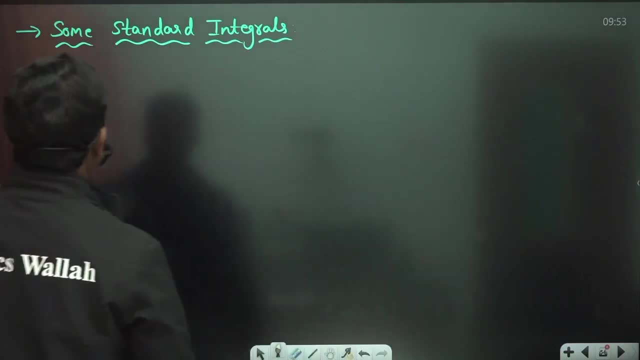 let us now work the reverse of, let us now work the reverse of that. so some standard integrals, okay, so that. so some standard integrals, okay, so that. so some standard integrals, okay. so first first integral X, power n DX, this first, first integral X, power n DX, this. 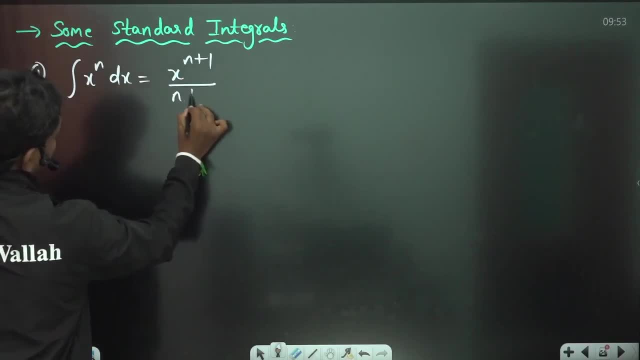 first, first integral: X, power n, DX. this is equal to X to the power n plus 1, is equal to X to the power n plus 1, is equal to X to the power n plus 1, divided by n plus 1 plus some arbitrary. divided by n plus 1 plus some arbitrary. 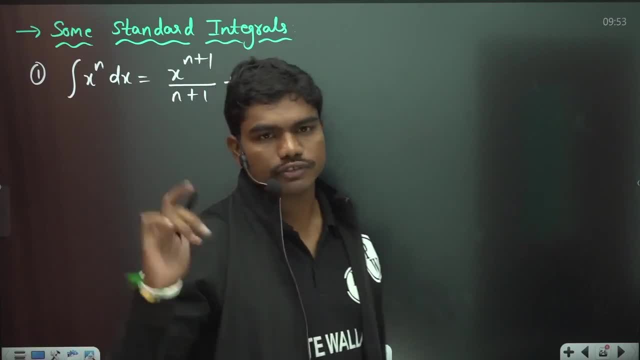 divided by n plus 1 plus some arbitrary constant C is some arbitrary constant constant C is some arbitrary constant constant C is some arbitrary constant means. what are the value you put in means? what are the value you put in means? what are the value you put in glass of C? still, this equation holds. 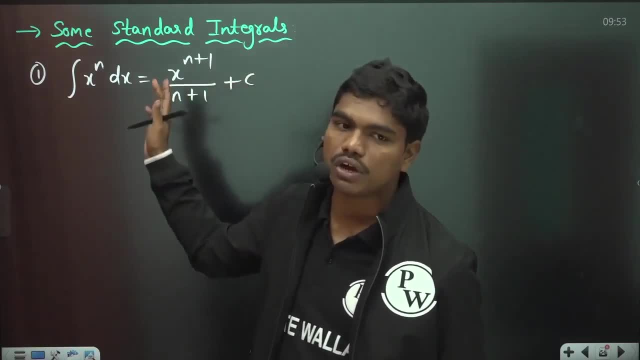 glass of C. still this equation holds. glass of C, still this equation holds: good, okay, if you differentiate the good. okay, if you differentiate the good, okay, if you differentiate the right-hand side, by taking any value of right-hand side, by taking any value of right-hand side, by taking any value of the constant, you will get X power n. 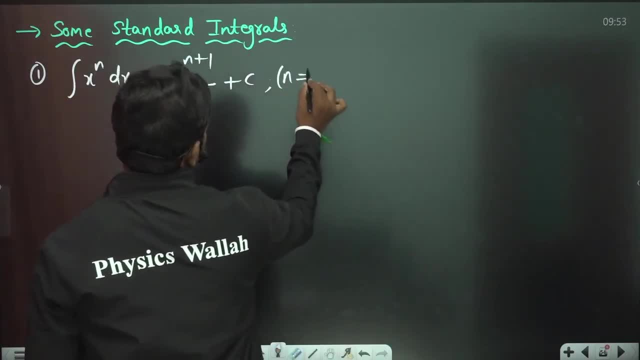 the constant, you will get X power. n. the constant, you will get X power n. that's the meaning okay, and this is that's the meaning okay, and this is that's the meaning okay, and this is valid when n is not equal to minus 1 of. 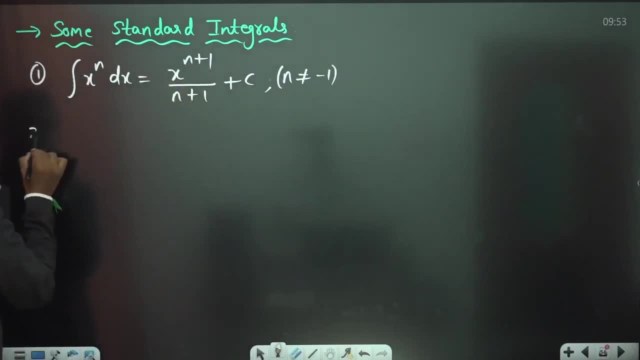 valid when n is not equal to minus 1 of. valid when n is not equal to minus 1, of course okay. if n equal to minus 1, course okay. if n equal to minus 1, course okay. if n equal to minus 1 division with 0, not different, okay. so. 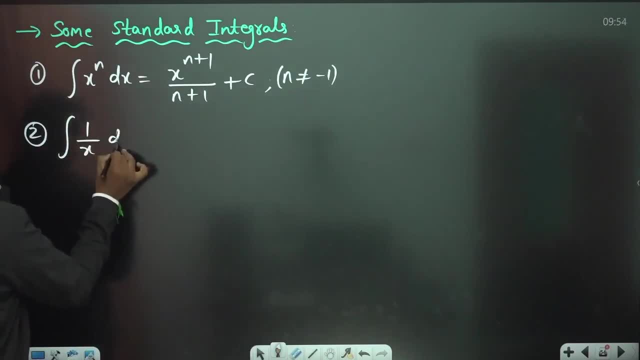 division with 0, not different. okay. so division with 0, not different. okay. so what is the case with n is equal to. what is the case with n is equal to. what is the case with n is equal to minus 1 means 1 by X, DX. this is log mod. 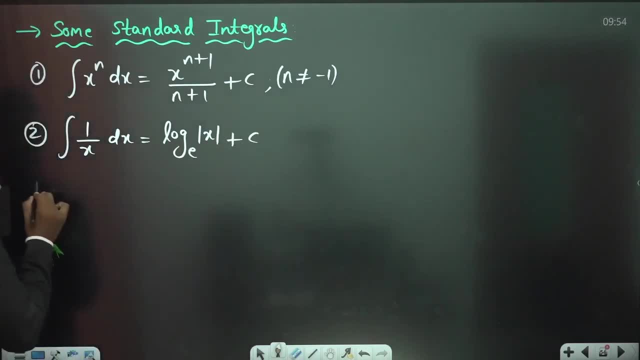 minus 1 means 1 by X DX. this is log mod. minus 1 means 1 by X DX. this is log mod. X to the base e, plus constant- okay. next X to the base e- plus constant. okay. next X to the base e, plus constant, okay. next 3. sine X. integration of sine X DX is: 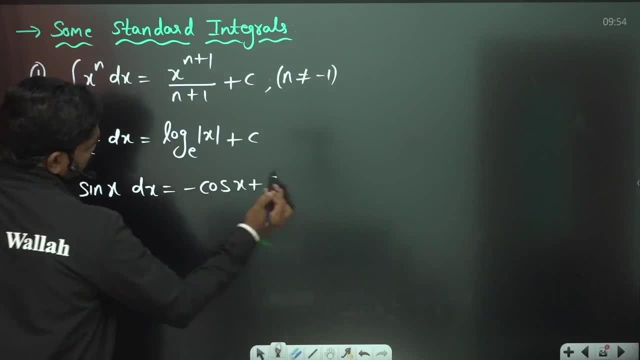 3 sine X integration of sine X DX is 3 sine X integration of sine X DX is again: minus cos X, plus constant. again minus cos X, plus constant. again minus cos X, plus constant. similarly, integral cos X DX is equal to. similarly, integral cos X DX is equal to. 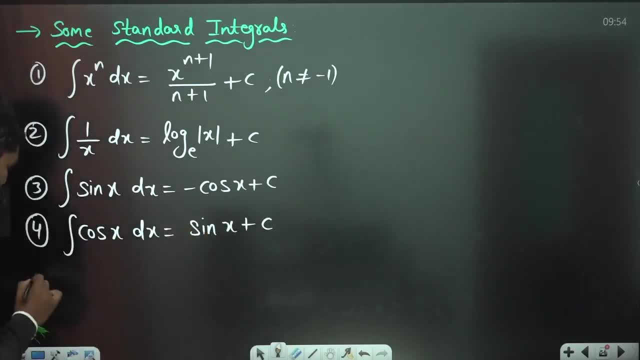 similarly, integral cos X DX is equal to sine X plus constant. sine X plus constant: 5. integral secant square X: 5. integral secant square X: 5. integral secant square X is equal to, is equal to, is equal to tan x plus C, because you know tan x. 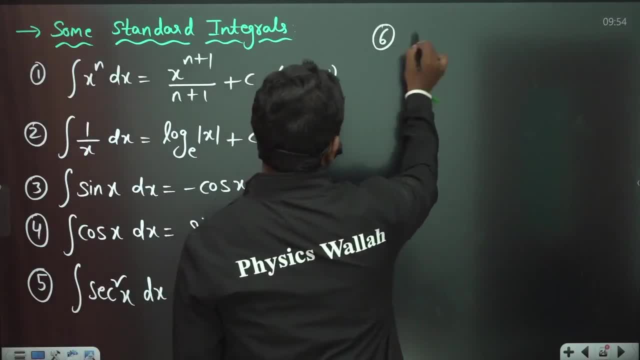 tan x plus C because you know tan x, tan x plus C because you know tan x. differentiation is secant square X, so differentiation is secant square X, so differentiation is secant square X. so, anyhow, let us write integral tan X. and anyhow, let us write integral tan X. and. 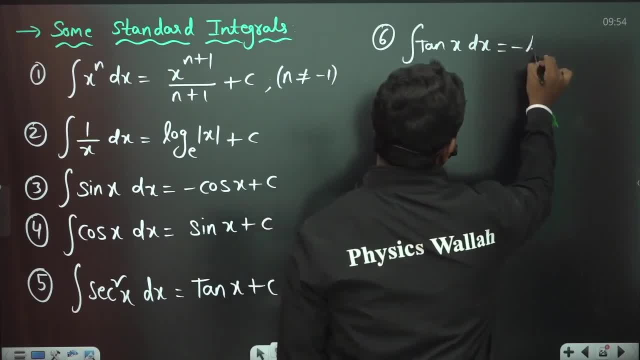 anyhow, let us write integral tan X and DX is equal to minus log mod. you know DX is equal to minus log mod. you know DX is equal to minus log mod. you know. integral tan X by the integral tan X- DX. integral tan X by the integral tan X- DX. 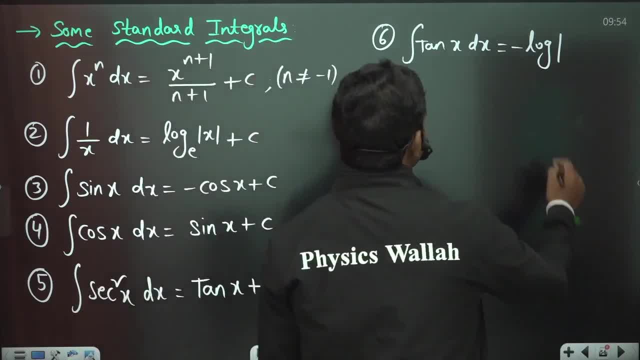 integral tan X by the integral tan X. DX is minus log mod, secant X: okay, so minus is minus log mod. secant X: okay, so minus is minus log mod. secant X: okay, so minus log mod. cos X actually connect minus log log mod. cos X actually connect minus log. 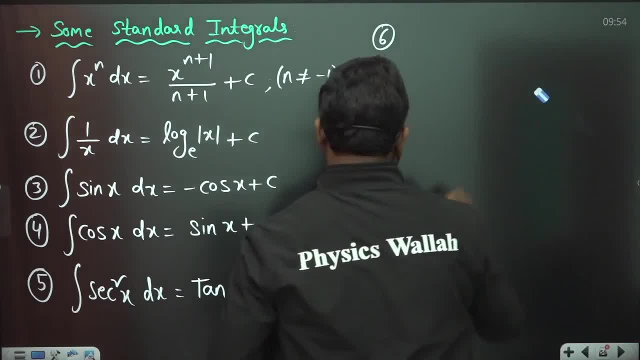 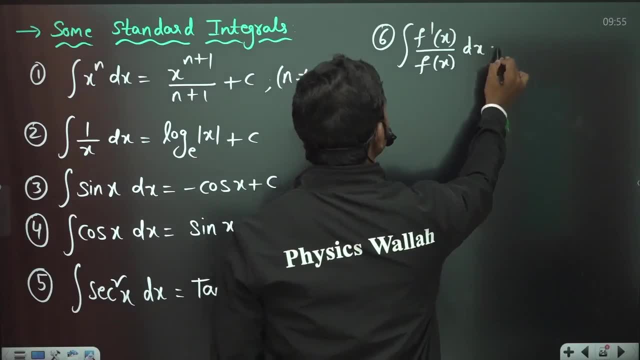 log mod. cos X actually connect minus log mod. anyhow, let us see before going for mod. anyhow, let us see before going for mod. anyhow, let us see before going for tan X. let us write one result: integral F, tan X. let us write one result: integral F, tan X. let us write one result: integral F: dash of X by F of X, DX is equal to log. 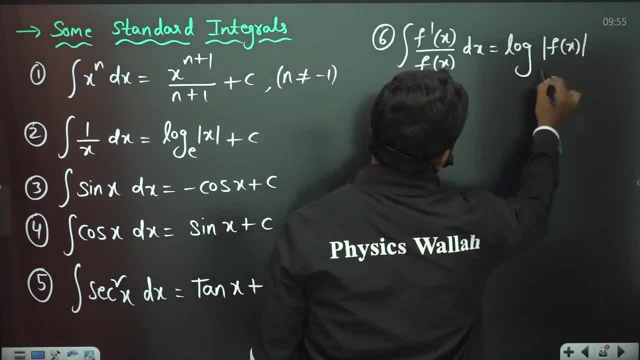 dash of X by F of X- DX is equal to log dash of X by F of X- DX is equal to log mod F of X to the base e, plus constant. mod F of X to the base e, plus constant. mod F of X to the base e, plus constant. okay, why this is the case? because if you 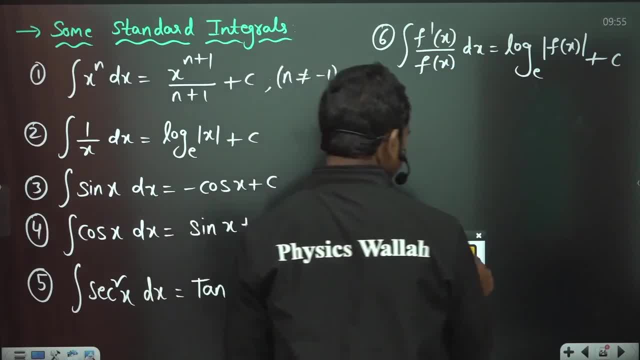 okay. why this is the case? because, if you okay. why this is the case? because if you differentiate this, you can get this 1 by differentiate this. you can get this 1 by differentiate this. you can get this 1 by mod F of X to the base e, if you write. 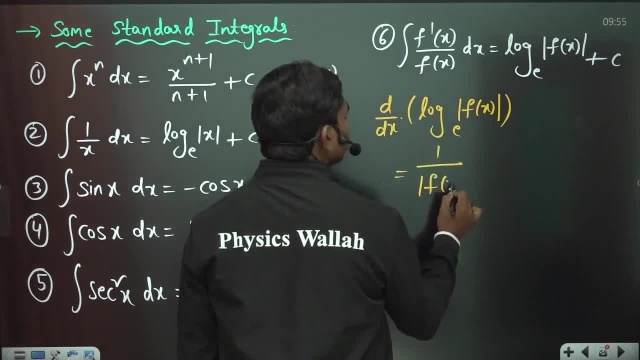 mod F of X to the base e. if you write mod F of X to the base e, if you write this, this is 1 by mod F of X into this. this is 1 by mod F of X. into this: this is 1 by mod F of X. into differentiation of mod F of X is mod F of. 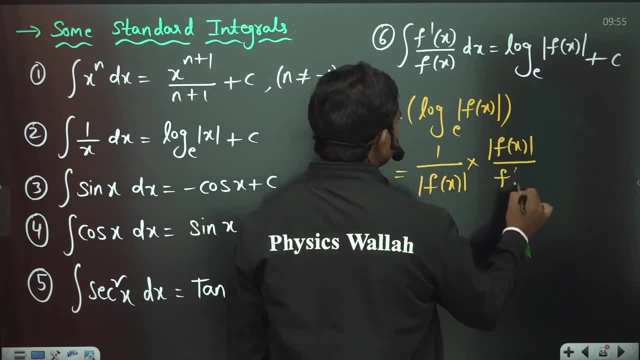 differentiation of mod F of X is mod F of. differentiation of mod F of X is mod F of X by F of X. derivative of mod X is mod X. X by F of X. derivative of mod X is mod X. X by F of X. derivative of mod X is mod X by X. so that's how this is mod F of X by: 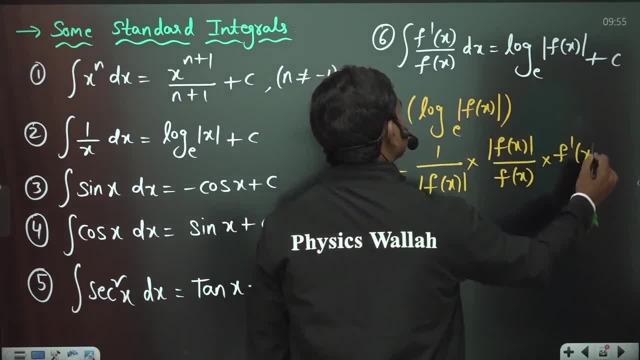 by X. so that's how this is: mod F of X by by X. so that's how this is: mod F of X by F of X into the inner derivative of F of F of X into the inner derivative of F, of F of X into the inner derivative of F of X into the inner derivative of F of X is F dash of X. so 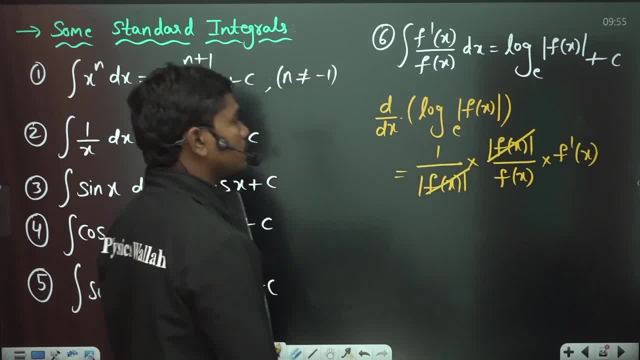 is F dash of X, so is F dash of X. so these two terms gets cancelled out. so you, these two terms gets cancelled out. so you, these two terms gets cancelled out. so you have F dash of X by F of X. that's how. have F dash of X by F of X. that's how. 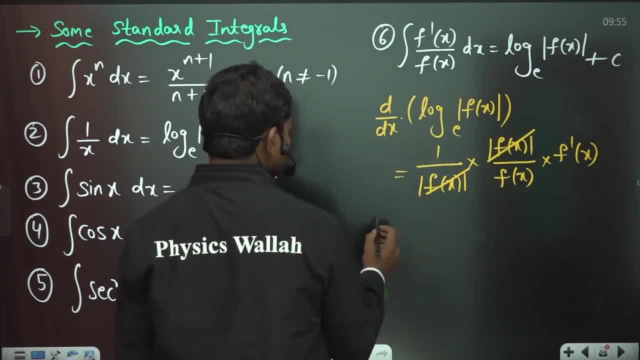 have F dash of X by F of X. that's how this integration is not basically now. if this integration is not basically now, if this integration is not basically now, if you write for tan x integral, tan x dx this, you write for tan x integral, tan x dx this. 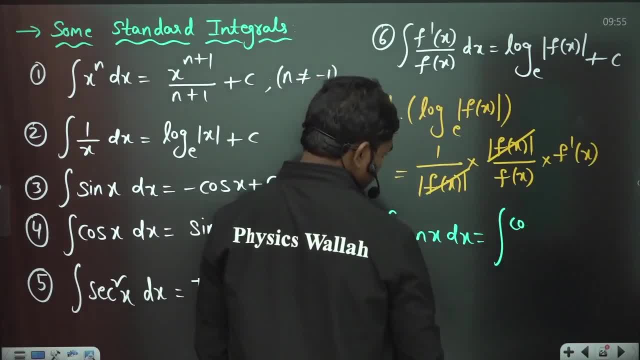 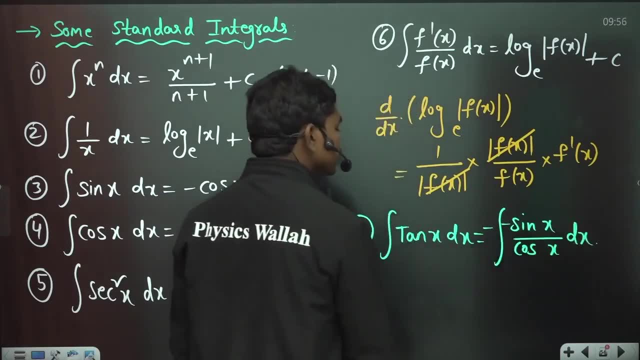 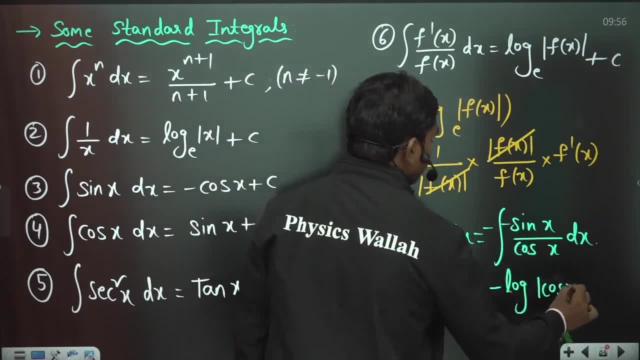 nothing but derivative of cos X. so this, nothing but derivative of cos X. so this is minus log mod. cos X to the base e is minus log mod. cos X to the base e is minus log mod. cos X to the base e: plus constant. okay, so if you say right, 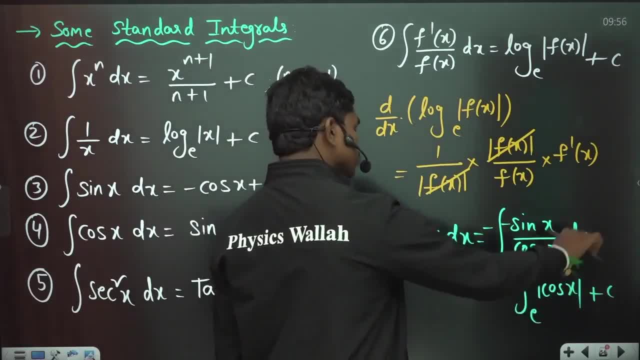 plus constant, okay. so if you say right plus constant, okay. so if you say right, if you take a minus, if you take this, if you take a minus, if you take this, if you take a minus, if you take this minus n to the power 1 here, cos X. 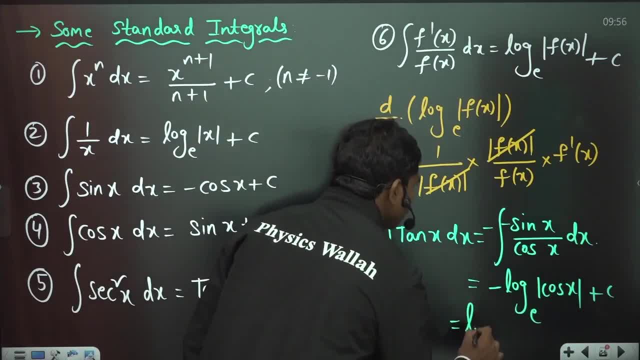 minus n to the power 1 here cos X. minus n to the power 1 here cos X inverse. so 1 by cos X is nothing but inverse. so 1 by cos X is nothing but inverse. so 1 by cos X is nothing but secant X. so this can be written as log. 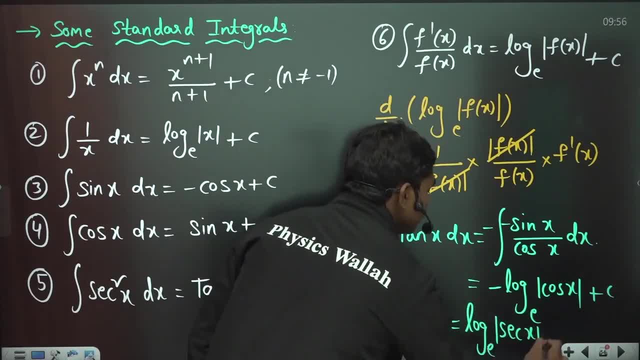 secant X. so this can be written as log secant X. so this can be written as log mod secant X to the base e plus mod secant X to the base e plus mod secant X to the base e plus constant. anyhow, okay, so that's also same. 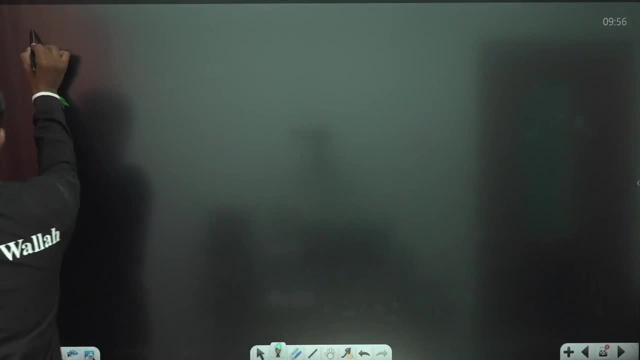 constant, anyhow okay, so that's also same constant, anyhow okay, so that's also same case. now let us see eighth one: integral cortex DX. so this time you integral cortex DX. so this time you integral cortex DX. so this time, you know, this is cos X by sine X DX, which is: 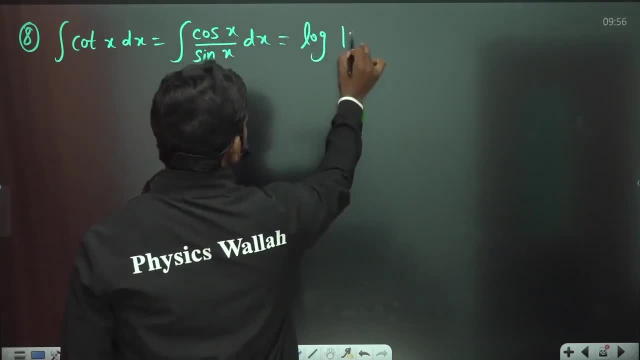 know this is cos X by sine X DX, which is know this is cos X by sine X DX, which is: differentiation of sine is directly cos. differentiation of sine is directly cos. differentiation of sine is directly cos. so log mod sine X to the base e plus. so log mod sine X to the base e plus. 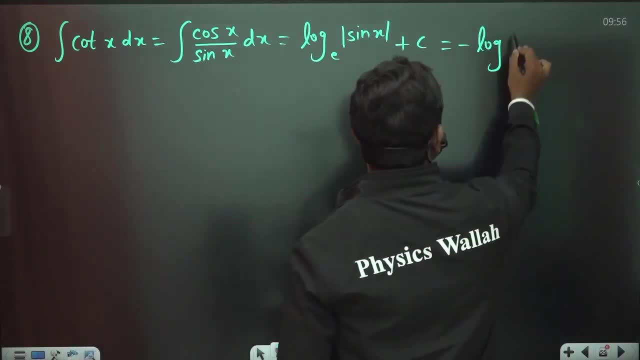 so log mod sine X to the base e plus constant. if you want to play with a constant, if you want to play with a constant, if you want to play with a minus, you can write minus log mod minus. you can write minus log mod minus. you can write minus log mod cosecant X to the base e plus constant. 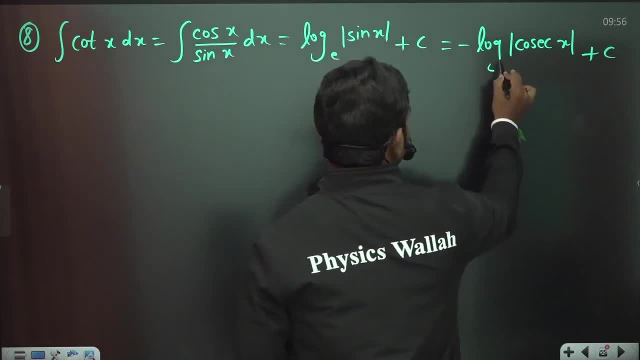 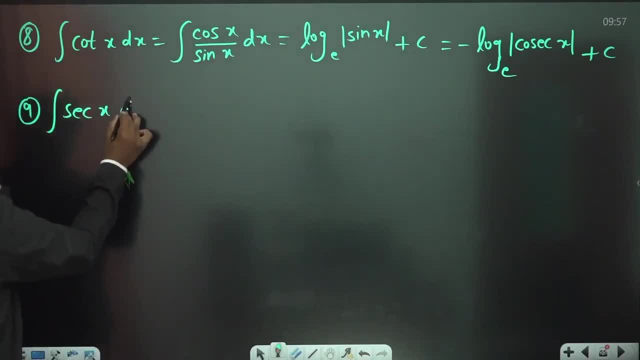 constant. similarly, if you write first constant. similarly, if you write first secant X, integral secant X, DX, so this secant X, integral secant X DX. so this secant X, integral secant X DX. so this is log mod. log mod secant X plus tan X. 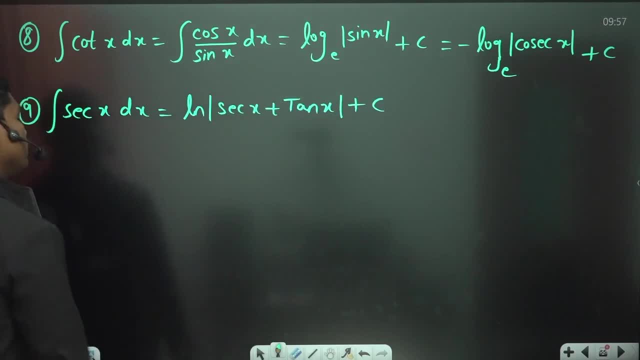 is log mod: log mod secant X plus tan X is log mod: log mod secant X plus tan X. to the base e, plus constant of course, e. to the base e, plus constant, of course, e. to the base e, plus constant of course, e. I have a 10 natural logarithm, so 10th. 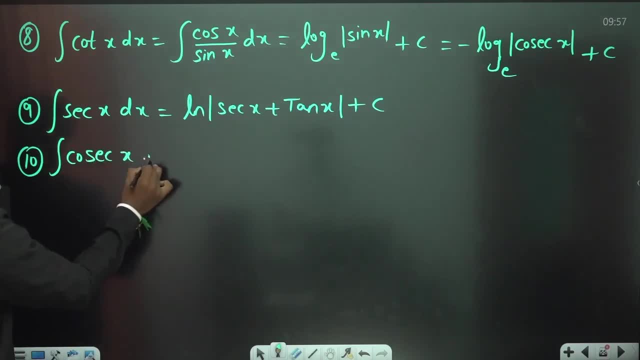 I have a 10 natural logarithm, so 10th. I have a 10 natural logarithm, so 10th. integral cosecant X. integral cosecant X- DX. this is equal to integral cosecant X- DX. this is equal to integral cosecant X- DX. this is equal to minus log. okay, log mod. 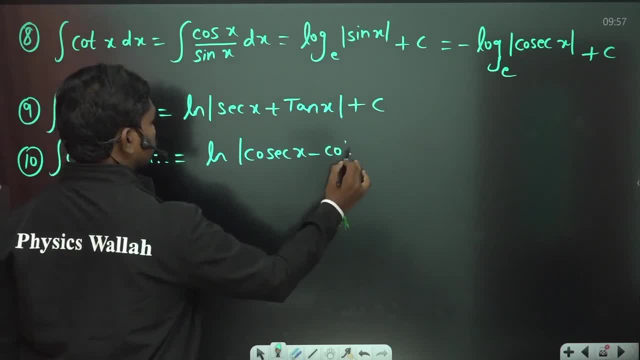 minus log: okay, log mod. minus log: okay, log mod. because he can text minus cortex, because he can text minus cortex, because he can text minus cortex plus, see actually here. okay, will there be plus. see actually here. okay, will there be plus. see actually here. okay, will there be minus n here? let us check. let us check. 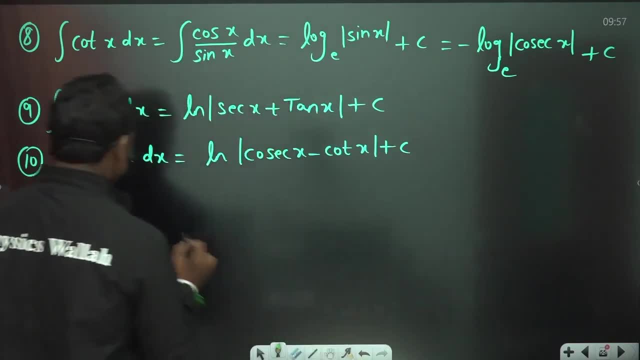 minus n here, let us check. let us check minus n here, let us check. let us check here. so integral cosecant X if you take here, so integral cosecant X if you take here. so integral cosecant X if you take integral cosecant X if you take here DX. so what we can. 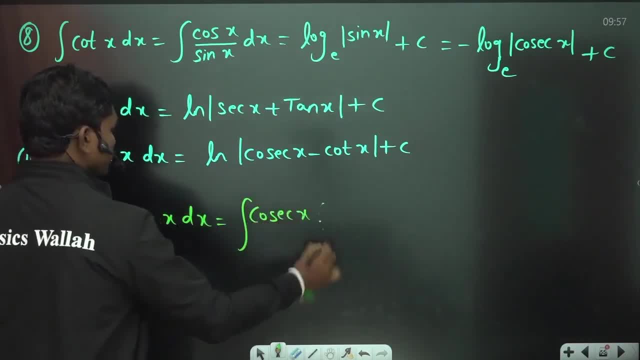 integral cosecant X. if you take here DX, so what we can. integral cosecant X. if you take here DX, so what we can do. we can rationalize with this. so do we can rationalize with this. so do we can rationalize with this. so cosecant X times, cosecant X minus cortex. 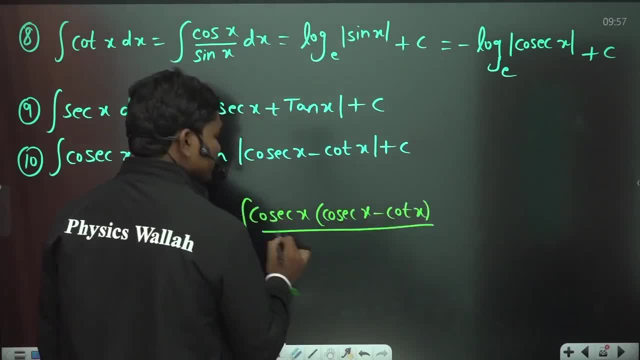 cosecant X times cosecant X minus cortex. cosecant X times cosecant X minus cortex. by cosecant X minus cortex. if you write by cosecant X minus cortex. if you write by cosecant X minus cortex, DX okay. so if by cosecant X minus cortex, DX okay. so if 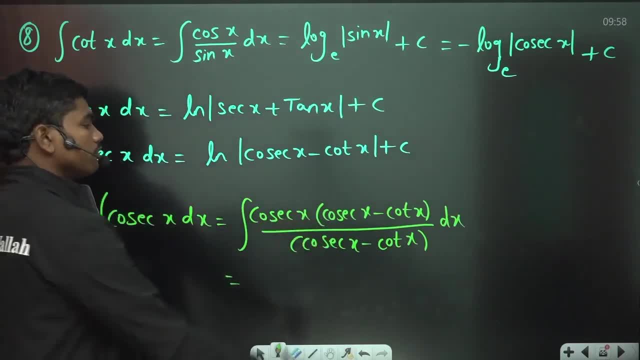 by cosecant X minus cortex DX. okay, so if you see this is cosecant square X, so you see this is cosecant square X. so you see this is cosecant square X. so cosecant square X is differentiation of. cosecant square X is differentiation of. 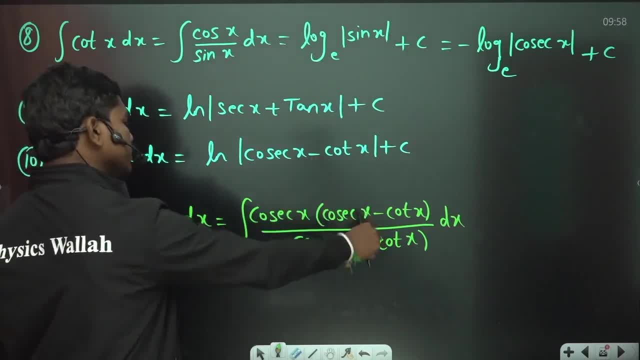 cosecant square. X is differentiation of minus cortex, because cortex is minus minus cortex, because cortex is minus minus cortex, because cortex is minus cosecant square. so if you have cosecant cosecant square, so if you have cosecant cosecant square, so if you have cosecant square, so this is minus cortex. and 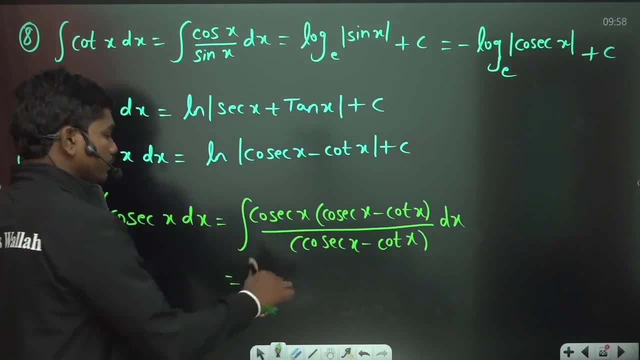 square, so this is minus cortex. and square, so this is minus cortex. and cosecant X is minus cosecant X- cortex. cosecant X is minus cosecant X- cortex. cosecant X is minus cosecant X- cortex. okay, so that's how it's finished, so log. 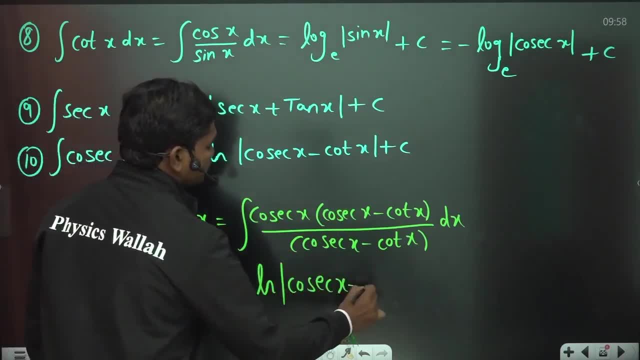 okay, so that's how it's finished. so log: okay, so that's how it's finished. so log. mod cosecant X minus cortex: no minus sign. mod cosecant X minus cortex: no minus sign. mod cosecant X minus cortex: no minus sign. cortex plus constant: that's how we have. 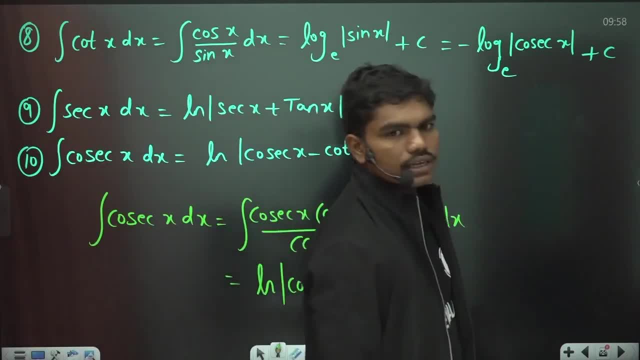 cortex plus constant. that's how we have cortex plus constant. that's how we have this formulas okay. and if you write for this formulas, okay, and if you write for this formulas, okay and if you write for some more like sine inverse and all I'll- some more like sine inverse and all I'll. 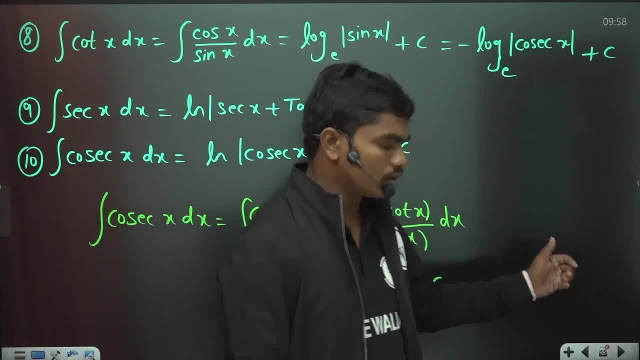 some more like sine inverse, and all I'll tell you after one principle, actually tell you after one principle, actually tell you after one principle, actually, which is called Eilat principle and all which is called Eilat principle and all which is called Eilat principle, and all I'll tell you how to write for inverse. 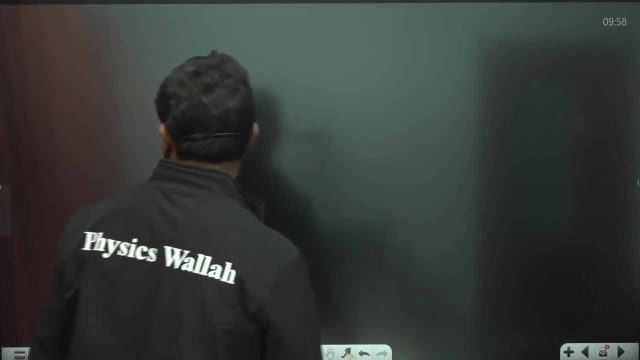 I'll tell you how to write for inverse. I'll tell you how to write for inverse functions right now. we will put inverse functions right now. we will put inverse functions right now. we will put inverse functions on hold now. let us see 11th. functions on hold now. let us see 11th. 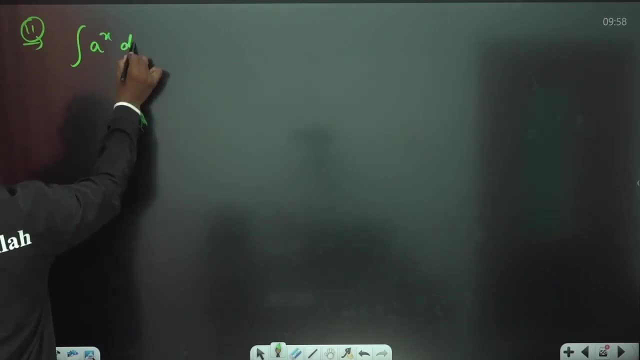 functions on hold. now let us see 11th integral a power X DX. this is a power X integral a power X DX. this is a power X integral a power X DX. this is a power X. by log a to the base e plus constant. by log a to the base e plus constant. 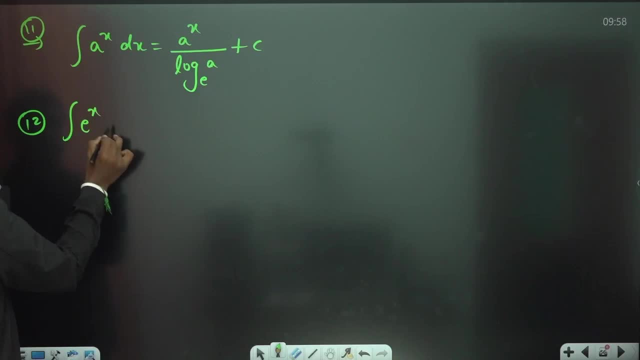 by log a to the base e plus constant. okay, and 12th integral e power X. so you okay. and 12th integral e power X, so you okay. and 12th integral e power X. so you know, if you put a is equal to e. this. 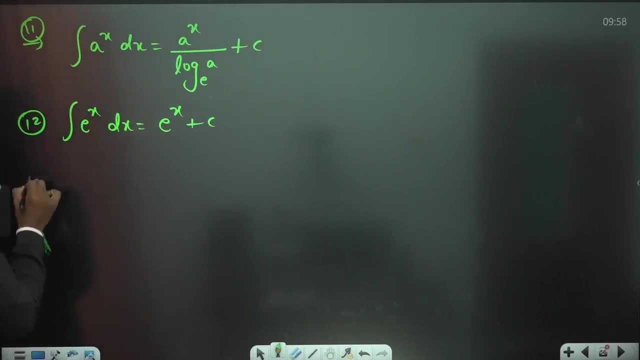 know if you put a is equal to e. this know: if you put a is equal to e, this denominator turns 1, so e power X plus denominator turns 1, so e power X plus denominator turns 1, so e power X plus constant. okay, so 13th integration log X. 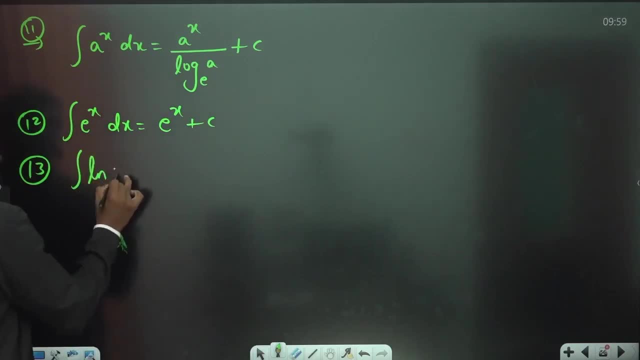 constant. okay. so 13th integration: log X: constant. okay. so 13th integration: log X: also again, I'll okay. fine integration, also again, I'll okay. fine integration, also again I'll okay. fine integration log X: I can give you, it's a small one. log X: I can give you, it's a small one. 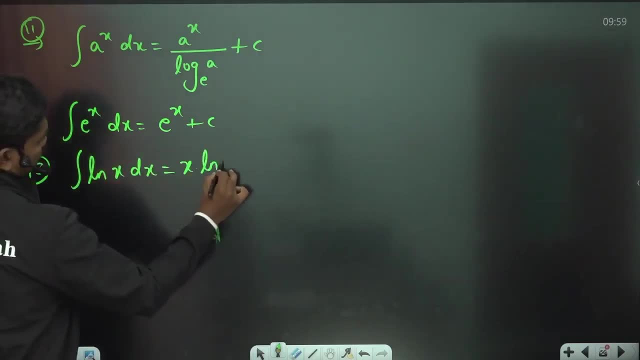 log X. I can give you. it's a small one. log X- DX is X into log X minus X less. log X DX is X into log X minus X less. log X DX is X into log X minus X less constant. okay, so basically X times of. 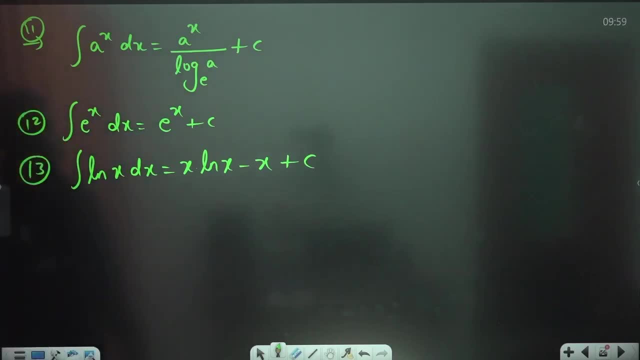 constant. okay, so basically X times of constant. okay, so basically X times of log X minus 1 is what you will have. log X minus 1 is what you will have. log X minus 1 is what you will have generally. okay, so X into log X minus X. so 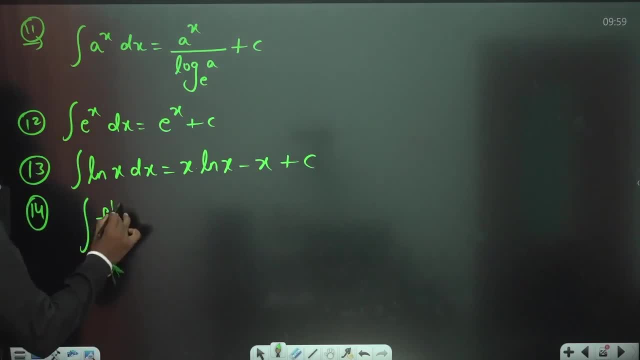 generally okay. so X into log X minus X. so generally okay. so X into log X minus X. so 14th integral F dash of X by root F of 14th integral F. dash of X by root F of 14th integral F. dash of X by root F of X is equal to 2 times of root F of X. 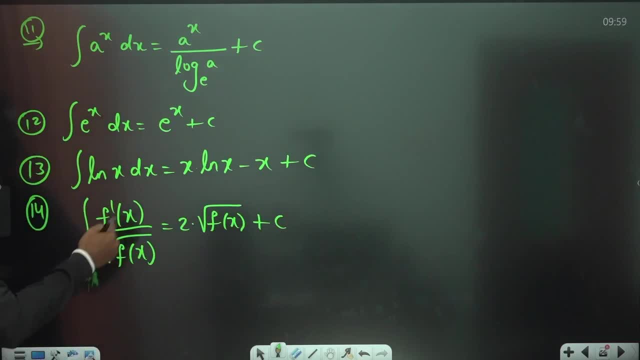 X is equal to 2 times of root F of X. X is equal to 2 times of root F of X, plus constant. so sometimes if you have plus constant, so sometimes if you have plus constant, so sometimes if you have sine X by root, cos X or cos X by root, 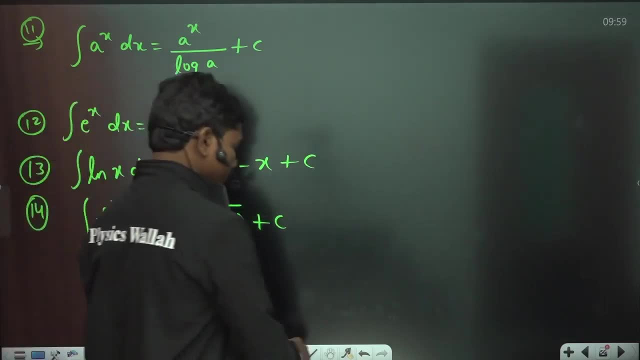 sine X by root, cos X or cos X by root, sine X by root, cos X or cos X by root, sine X, such kind of things you can play sine X. such kind of things you can play sine X. such kind of things you can play with this. okay, so 14th, so 15th, so inverse. 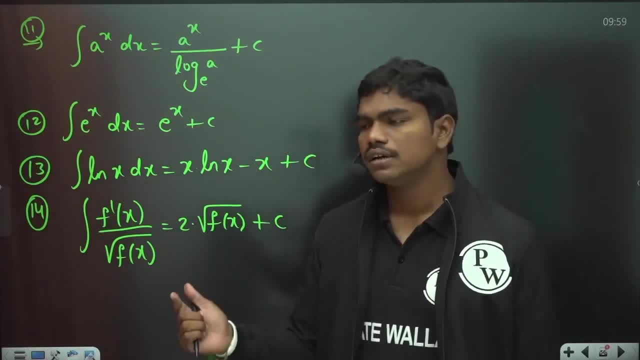 with this. okay, so 14th, so 15th. so inverse with this: okay, so 14th, so 15th. so inverse of algebraic functions is done. logarithmic of algebraic functions is done. logarithmic of algebraic functions is done. logarithmic we have seen, then exponential we have. 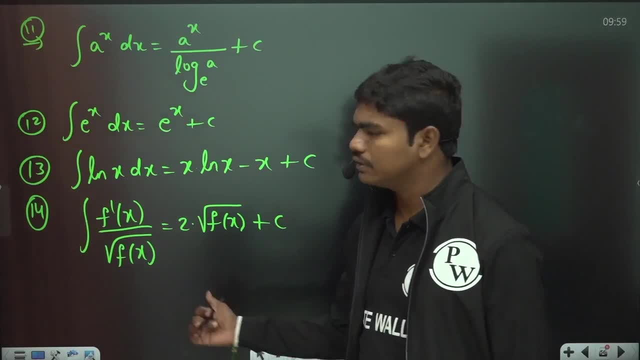 we have seen then exponential, we have. we have seen then exponential. we have seen technometrics, we have seen so seen technometrics. we have seen so seen technometrics. we have seen so inverse inverse functions. we will see inverse inverse functions. we will see inverse inverse functions. we will see later. okay, so basically these are the 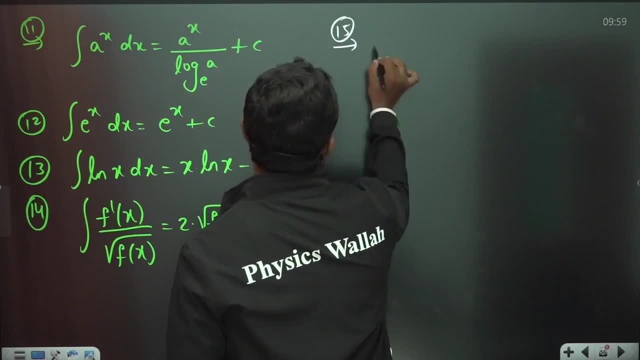 later, okay, so basically these are the later, okay. so basically these are the functions and I would like to give one functions and I would like to give one functions and I would like to give one more also: 15th integral F of X into F functions and I would like to give one more also 15th integral F of X into F. 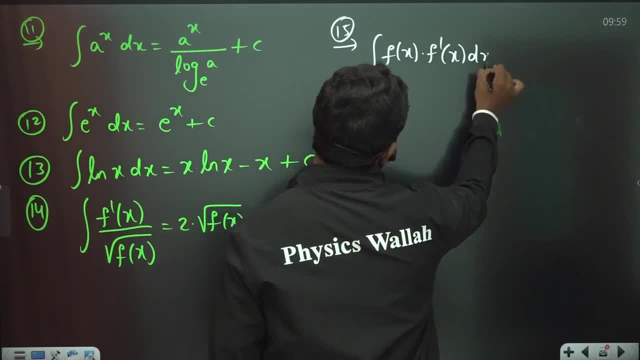 functions. and I would like to give one more also, 15th integral: F of X into F dash of X. so sometimes you have sine X dash of X. so sometimes you have sine X dash of X. so sometimes you have sine X into cos X, this kind of things. so the 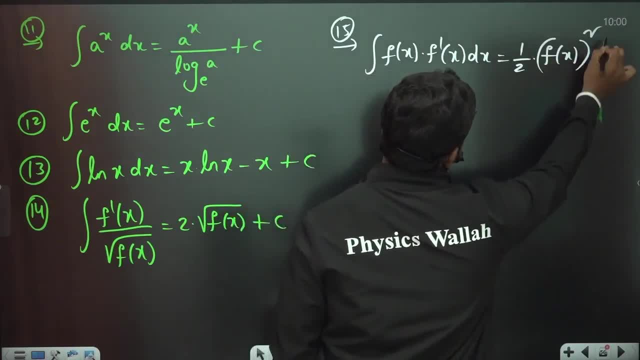 into cos X this kind of things. so the into cos X this kind of things. so the answer is half into F of X whole square. answer is half into F of X whole square. answer is half into F of X whole square, less constant. why? because if you 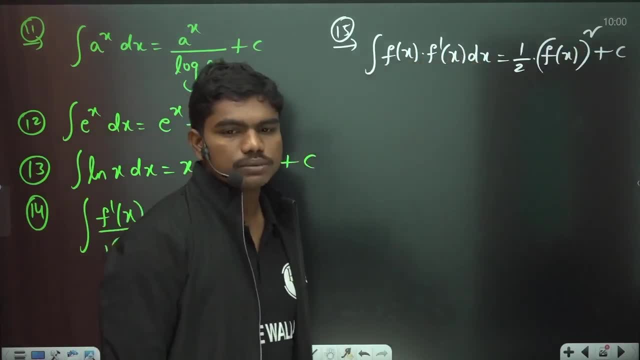 less constant. why? because, if you less constant, why? because if you differentiate this, you will get the same. differentiate this, you will get the same. differentiate this, you will get the same thing again. okay, so, normally, you need thing again. okay, so normally, you need thing again. okay, so, normally, you need not remember this. formulas in a single. 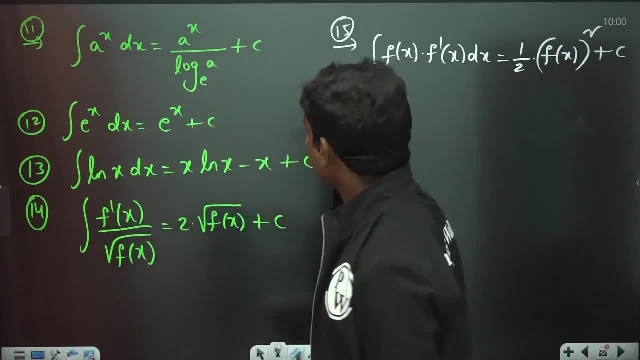 not remember this. formulas in a single, not remember this formulas in a single go. but as you keep on using them, you go. but as you keep on using them, you go. but as you keep on using them, you will get familiar with them. okay, so, now will get familiar with them. okay, so now. 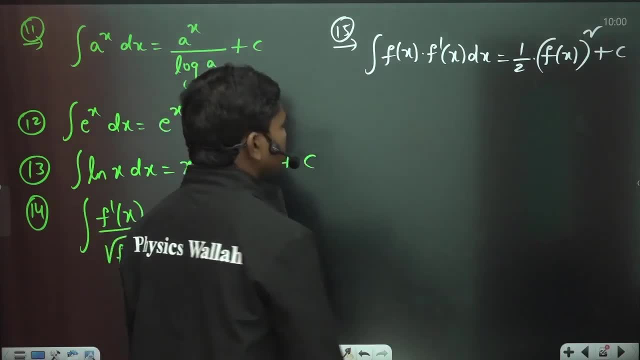 will get familiar with them. okay, so now, this is 15th and 16. so basically, yeah, this is 15th and 16. so basically, yeah, this is 15th and 16. so basically, yeah, these are the more or less the general. these are the more or less the general. 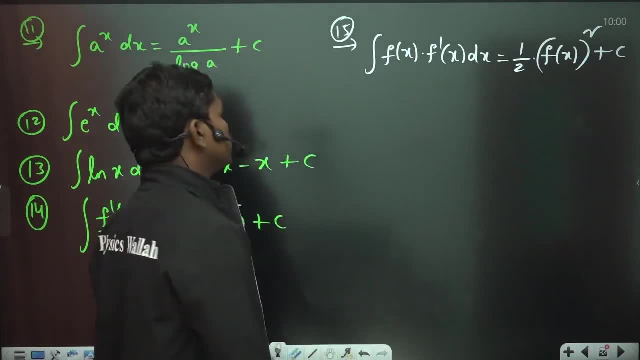 these are the more or less the general formulas that we have. okay now. if you do formulas that we have, okay now. if you do formulas that we have, okay now. if you do, for some things, some algebraic functions for some things, some algebraic functions for some things, some algebraic functions which I'm not okay, fine, let us talk about. 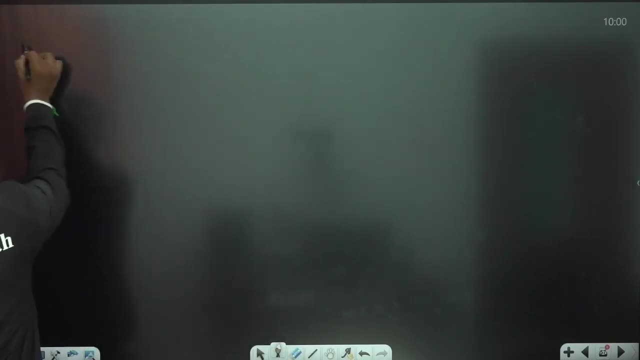 which I'm not okay, fine, let us talk about which I'm not okay. fine, let us talk about that later, okay, or now itself, but okay. that later, okay. or now itself, but okay. that later, okay. or now itself, but okay, fine. so let us see integral root of. 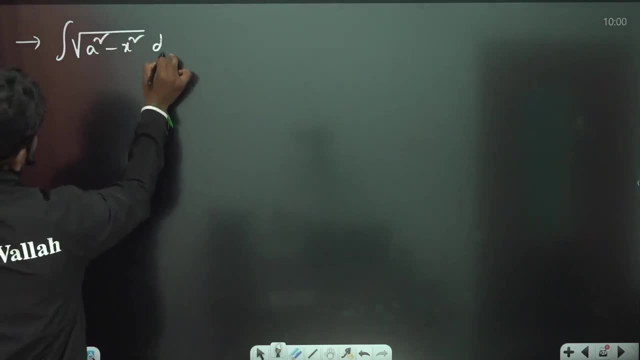 fine. so let us see integral root of fine. so let us see integral root of a square minus x square DX. so this is one a square minus x square DX. so this is one a square minus x square DX. so this is one very, very important integral actually. 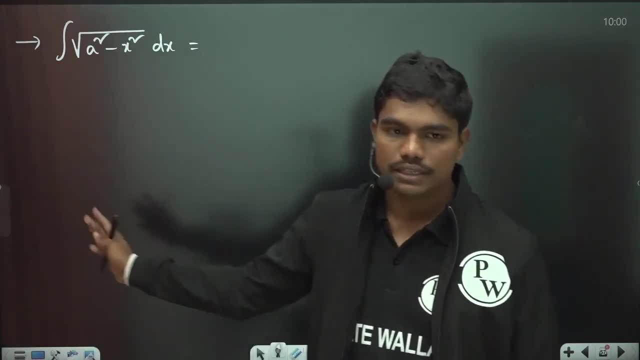 very, very important integral actually, very, very important integral actually, because we calculate the area of ellipse, because we calculate the area of ellipse, because we calculate the area of ellipse, all these things using this integration, all these things using this integration, all these things using this integration, okay, so, anyhow. so right now I am giving 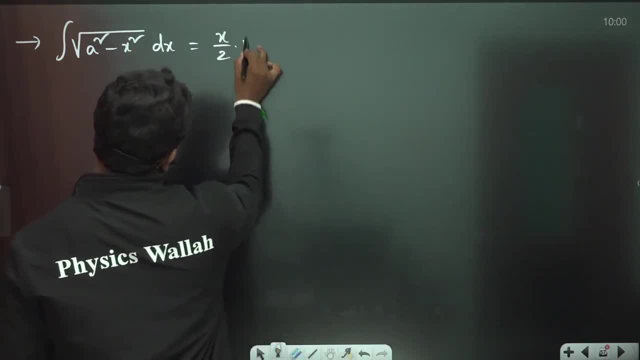 okay, so anyhow. so right now I am giving. okay, so anyhow. so right now I am giving you: the formula is x by 2 into root of a you. the formula is x by 2 into root of a you. the formula is x by 2 into root of a square minus x square plus a square by 2. 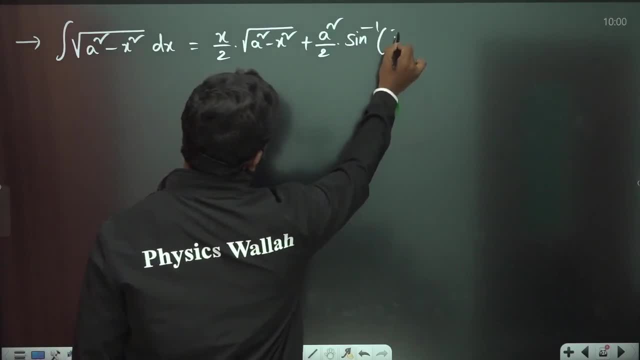 square minus x square plus a square by 2. square minus x square plus a square by 2 into sine inverse of X by a plus into sine inverse of X by a plus into sine inverse of X by a plus constant. okay, it's not a very complicated. constant. okay, it's not a very complicated constant. okay, it's not a very complicated integral. it's actually very easy if you integral. it's actually very easy if you integral. it's actually very easy if you take X is equal to a sine theta or a. take X is equal to a sine theta or a. 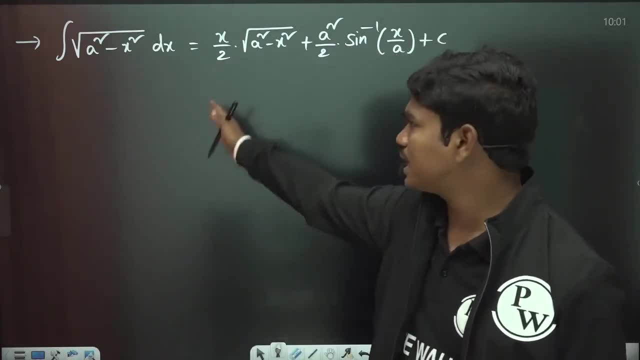 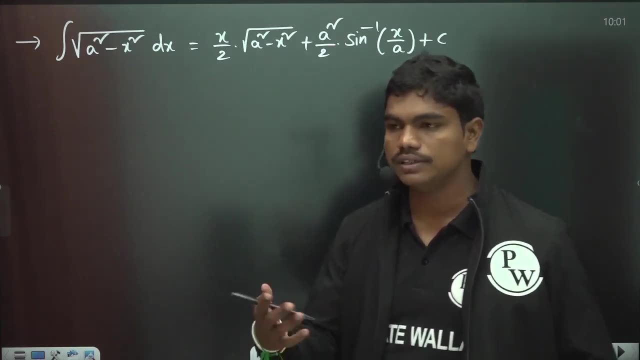 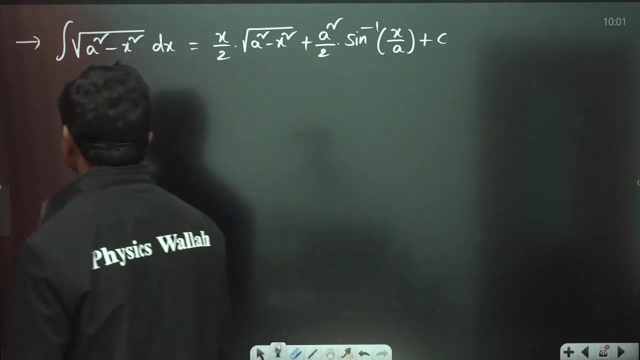 take X is equal to a sine theta or a cos theta. and if you do substitutions and cos theta, and if you do substitutions and cos theta, and if you do substitutions and calculate the things, you will get that. calculate the things, you will get that. calculate the things, you will get that. perfectly okay. now, if you talk about 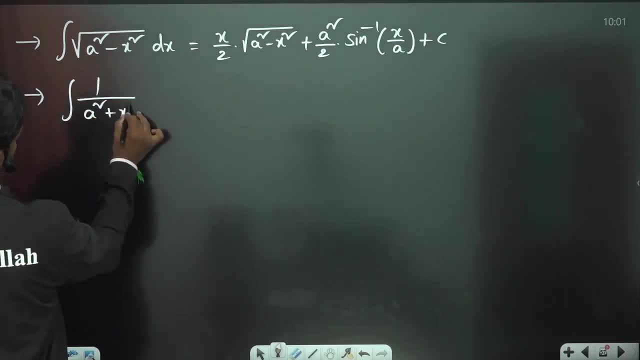 perfectly okay now if you talk about: perfectly okay now if you talk about: integral 1 by a square plus X square DX. integral 1 by a square plus X square DX. integral 1 by a square plus X square DX, this is 1 by a times of tan inverse X by. 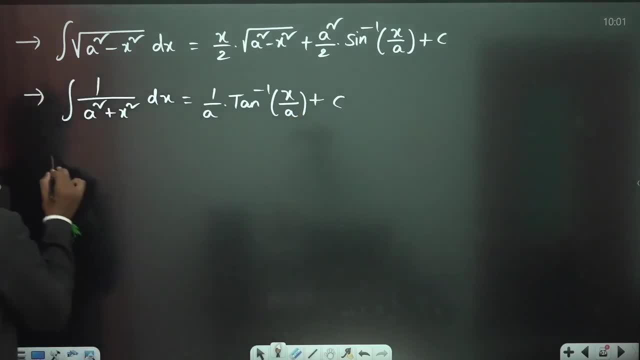 this is 1 by a times of tan inverse X. by: this is 1 by a times of tan inverse X by a plus constant. okay, so next integral 1 a plus constant. okay, so next integral 1 a plus constant. okay, so next integral 1 by root of X square minus a square DX. so 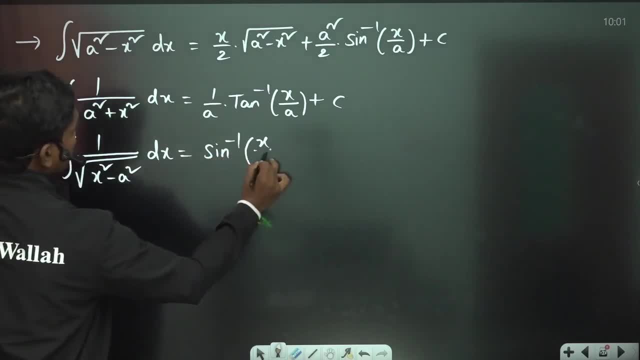 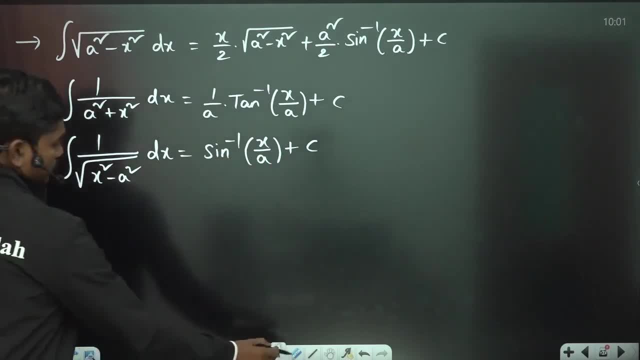 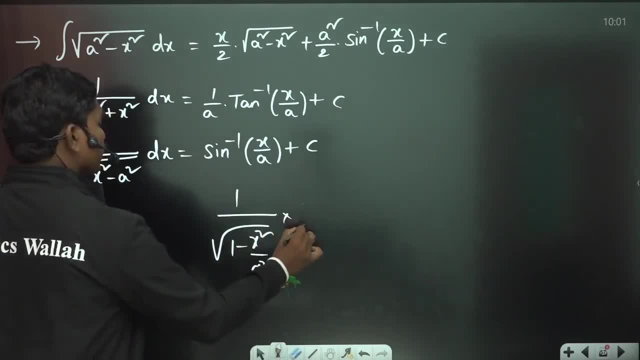 you differentiate this 1 by 1 by root of. you differentiate this 1 by 1 by root of 1, minus this time, into 1. by a so root of 1, minus this time into 1. by a so root of 1 minus this time into 1. by a so root of a square minus X square. yes, so basically. 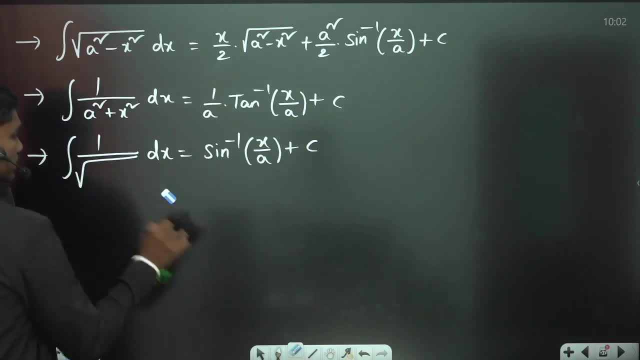 a square minus X square. yes, so basically a square minus X square. yes, so basically, if you see signs we have altered here, so if you see signs we have altered here, so if you see signs we have altered here, so this is a square minus X square, this is a square minus X square. 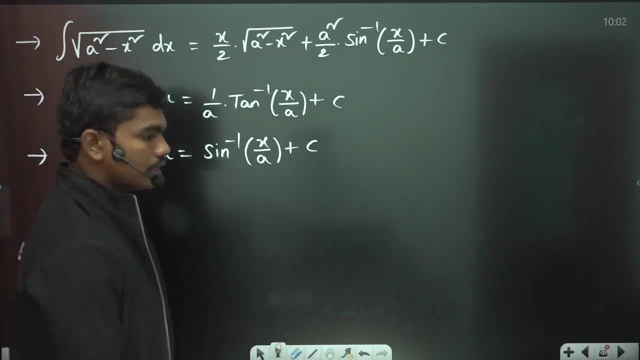 this is a square minus X square. if there is minus 1, then it's cos inverse. if there is minus 1, then it's cos inverse. if there is minus 1, then it's cos inverse. actually okay, so. integral root of 1 by. actually okay, so integral root of 1 by. 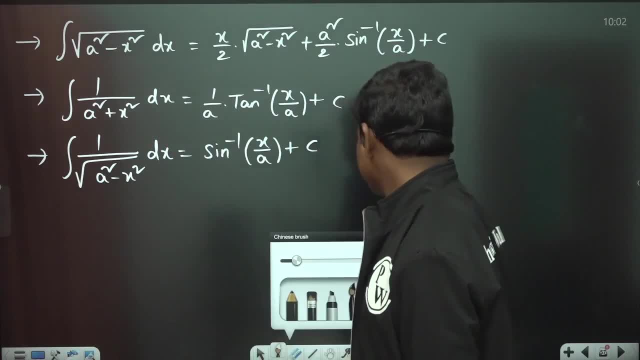 actually okay. so integral root of 1 by root of a square minus X square, all root of a square minus X square. all root of a square minus X square, all these things, it's you know you can these things. it's you know you can these things. it's you know you can calculate them. but here, this is the some. 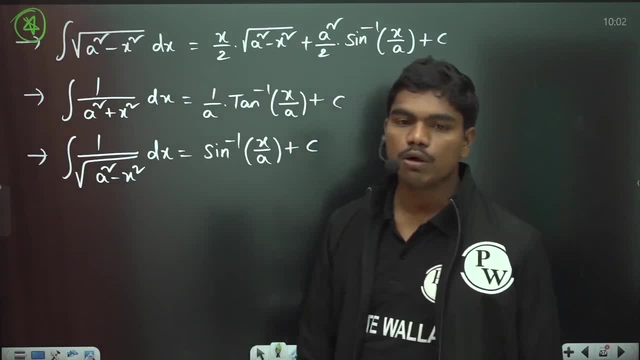 calculate them, but here this is the some calculate them. but here this is the some important result that comes out here. okay, important result that comes out here. okay, important result that comes out here. okay, now, how to integrate two functions. now how to integrate two functions. now how to integrate two functions product of two functions, if you have. 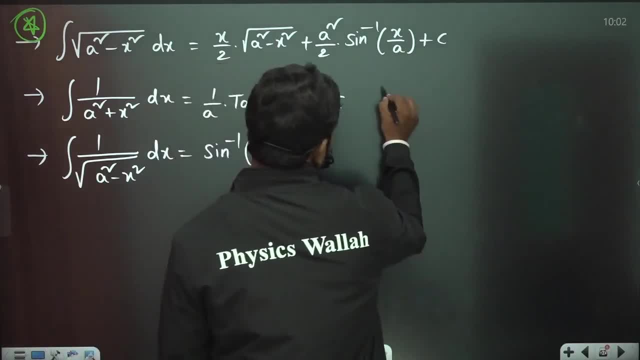 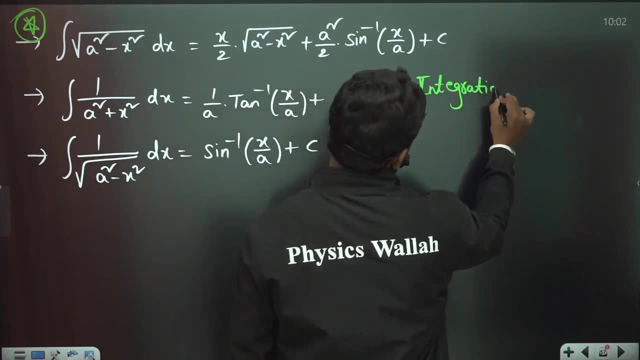 product of two functions. if you have product of two functions, if you have product of two functions, how to integrate product of two functions? how to integrate product of two functions, how to integrate them? okay, so, let us see them. okay, so, let us see them okay. so let us see integration by parts, integration by: 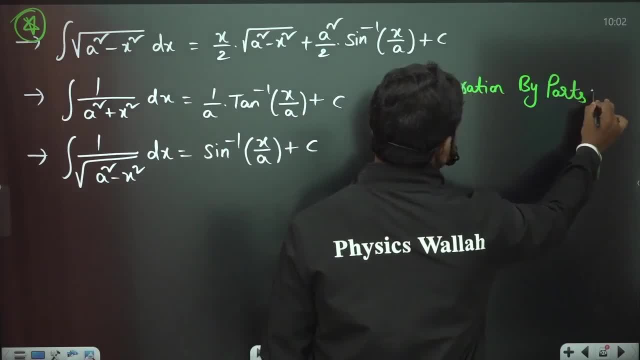 integration by parts, integration by integration by parts, integration by parts. so if you have two functions, how to parts? so if you have two functions, how to parts, so if you have two functions, how to integrate them actually? so let us see, integrate them actually. so let us see. 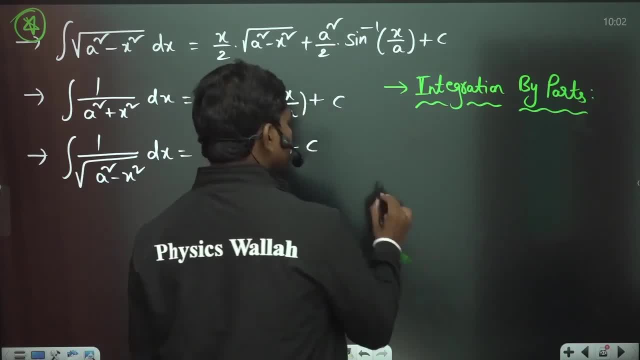 integrate them actually. so let us see here: if you have this two parts for here, if you have this two parts for here, if you have this two parts, for example, means if you have this integral example, means if you have this integral example, means if you have this integral integral F of X. 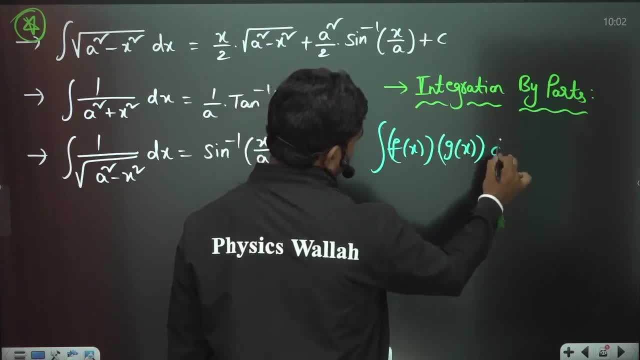 integral F of X, integral F of X into G of X, into G of X, into G of X, DX, DX, DX, DX. so so, if you have this function, how you will, if you have this function, how you will, if you have this function, how you will integrate? this is actually equal to F of 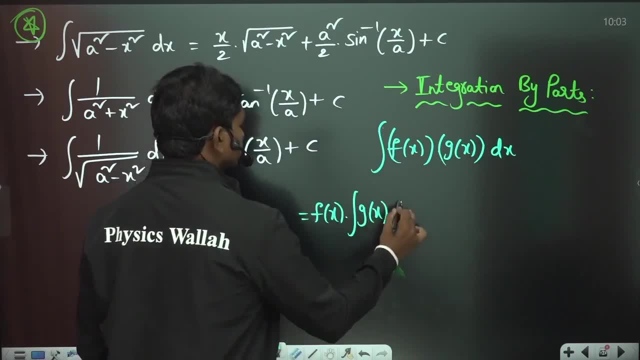 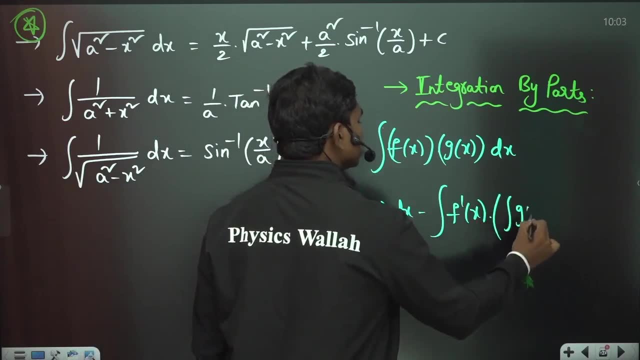 integrate. this is actually equal to F of integrate. this is actually equal to F of X into integral G of X DX minus integral X into integral G of X DX minus integral X into integral G of X DX minus integral F. dash of X into integral G of X DX to. 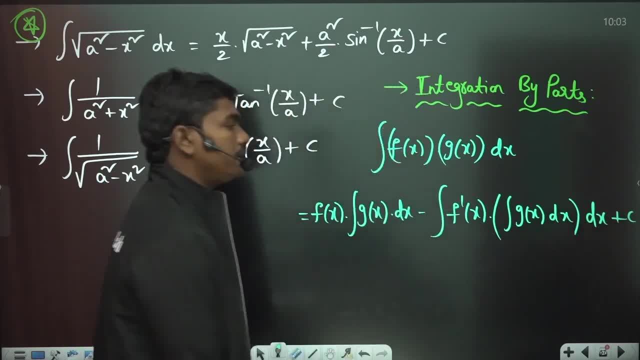 F dash of X into integral G of X. DX to F dash of X into integral G of X. DX to this whole DX plus some constant. okay, so this whole DX plus some constant. okay, so this whole DX plus some constant. okay, so this is how you integrate the product of 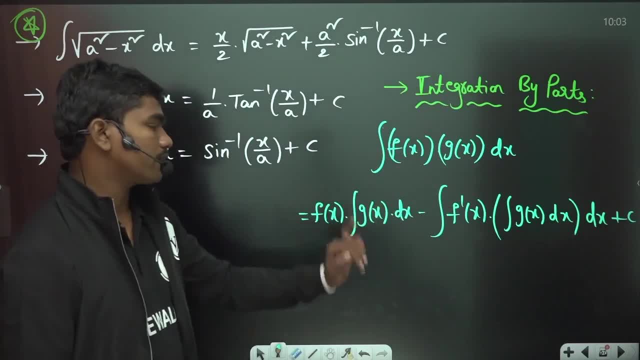 this is how you integrate the product of. this is how you integrate the product of two functions, actually okay so first two functions, actually okay so, first two functions actually okay. so: first function into integration of second function, into integration of second function, into integration of second function, minus integral of. 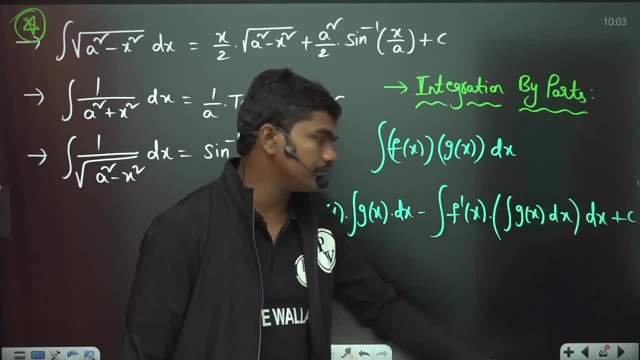 function minus integral of function minus integral, of differentiation of this first function, differentiation of this first function, differentiation of this first function into the second integral, DX plus, into the second integral DX plus, into the second integral DX plus constant. okay now, when you apply this constant. okay now, when you apply this. 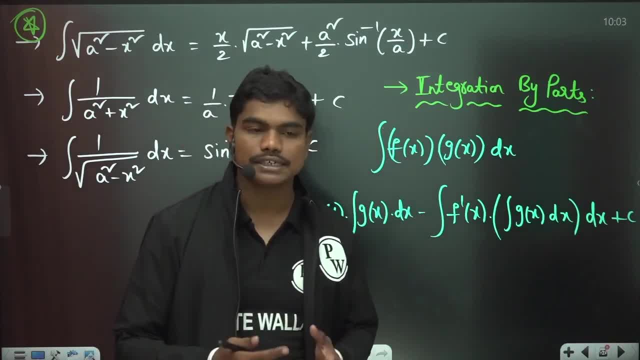 constant. okay now, when you apply this integration by parts, you can, of course, integration by parts. you can, of course, integration by parts. you can, of course, you can multiply. you can keep the. you can multiply, you can keep the, you can multiply, you can keep the product. in any way, you will get the. 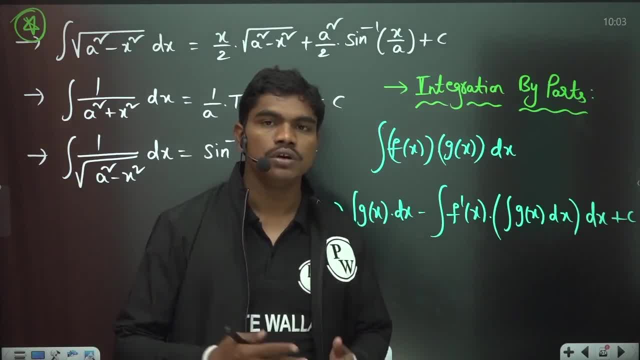 product in any way, you will get the product. in any way you will get the answer. but generally this one principle answer, but generally this one principle answer, but generally this one principle which if you follow you will get in a, which if you follow you will get in a. 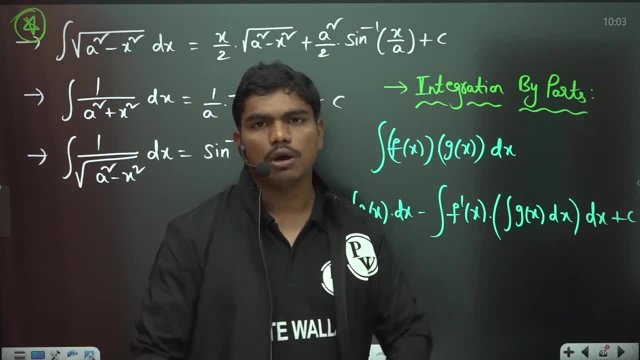 which, if you follow you, will get in a sequence in a systemized way, otherwise sequence in a systemized way, otherwise sequence in a systemized way, otherwise what happens? sometimes calculations go. what happens sometimes calculations go. what happens sometimes? calculations go out of range means they go very big. 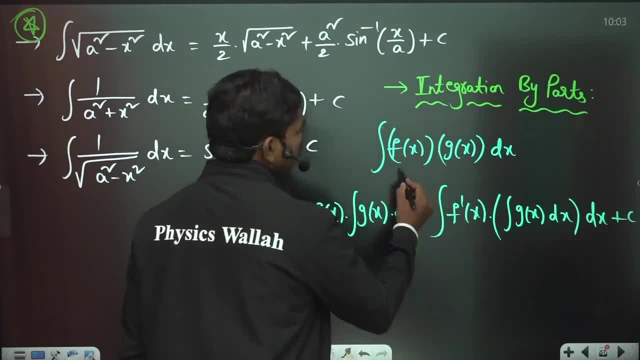 out of range means they go very big. out of range means they go very big actually, okay. so when you are deciding, actually, okay, so when you are deciding, actually okay. so when you are deciding, the product, actually this product of the. the product actually this product of the. 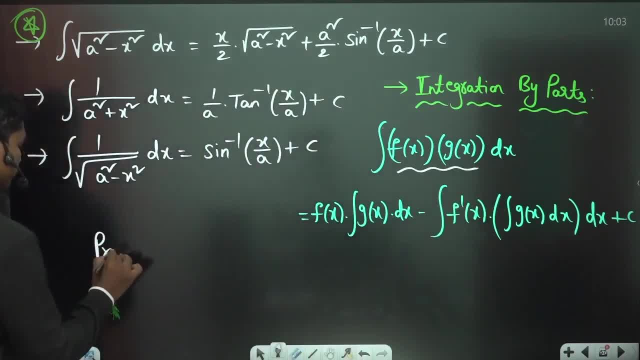 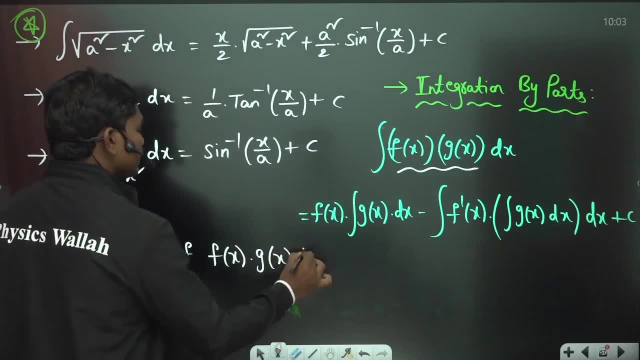 the product. actually, this product of the functions, product of f of X into G of X functions, product of f of X into G of X functions, product of f of X into G of X, product of f of X into G of X is denoted. product of f of X into G of X is denoted. 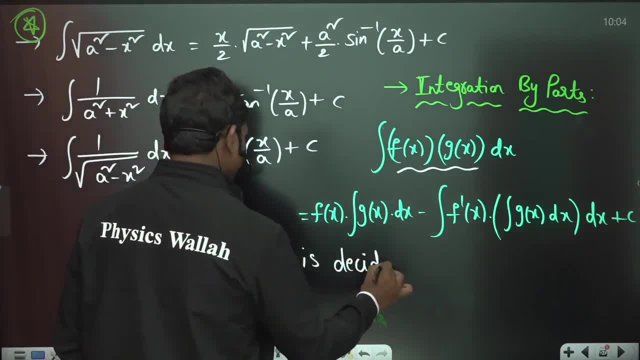 product of f of X into G of X is denoted by or is decided by by: or is decided by by. or is decided by: is decided by: I late order. this is there's one order is decided by: I late order. this is there's one order. 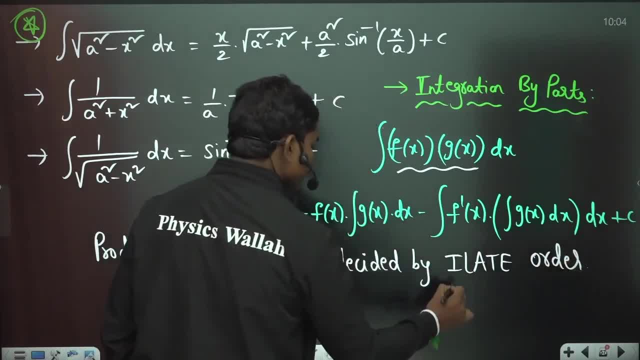 is decided by I late order. this is: there's one order which is called this I late, and what does which is called this I late and what does which is called this I late, and what does this? I let me I for inverse functions. this, I let me I for inverse functions. 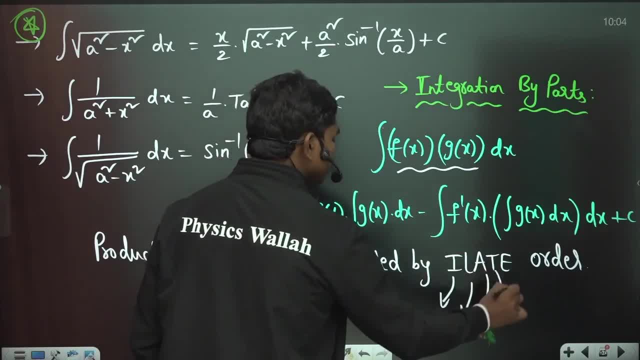 this. I let me: I for inverse functions, alpha logarithmic functions. a for alpha logarithmic functions, a for alpha logarithmic functions, a for algebraic T for technometric. and if a algebraic T for technometric and if a algebraic T for technometric and if a exponential functions, okay, so I'll give. 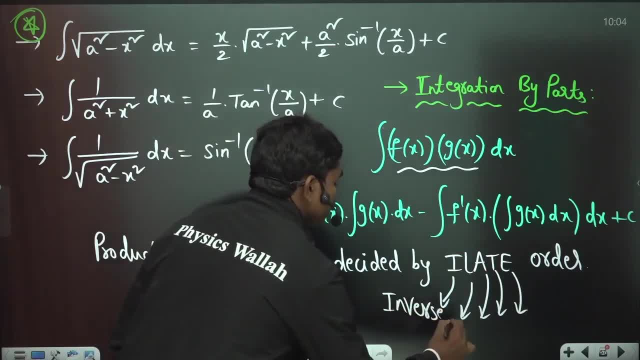 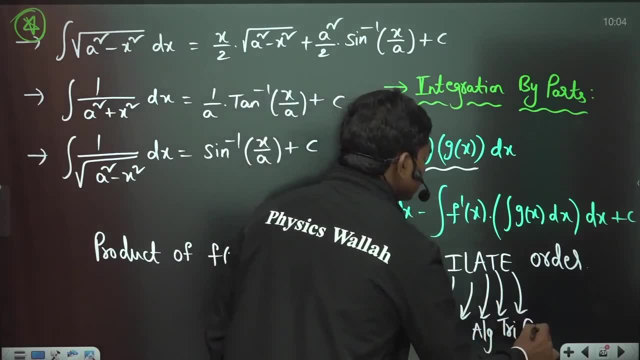 exponential functions. okay, so I'll give exponential functions. okay, so I'll give a quick note inverse. a quick note inverse, a quick note inverse. then log, then algebraic means all these, then log, then algebraic means all these, then log, then algebraic means all these functions, technometric and exponential. 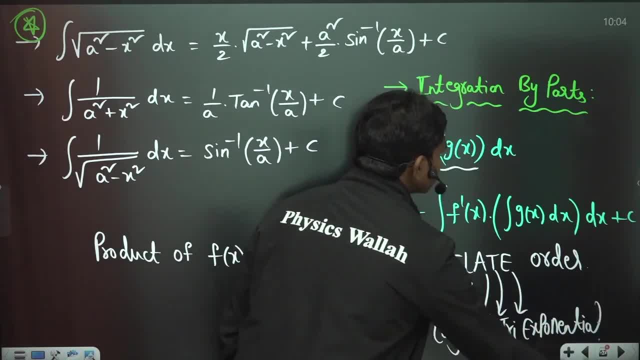 functions, functions, technometric and exponential functions. functions, technometric and exponential functions like this, functions like this, functions like this, exponential functions. okay, so we have this exponential functions. okay, so we have this exponential functions. okay, so we have this. many things like this, so integration. many things like this, so integration. 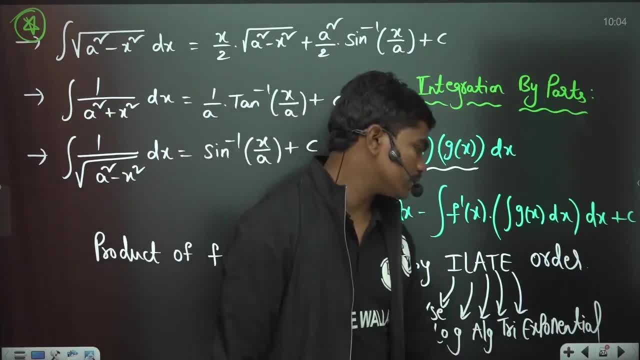 many things like this. so integration by parts is what we generally do, and of by parts is what we generally do, and of by parts is what we generally do. and, of course, using this. let us suppose if I course using this. let us suppose if I course using this. let us suppose if I want to, I, because I want to give you one. 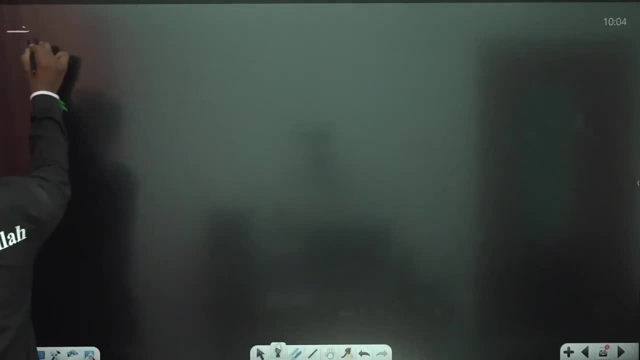 want to I because I want to give you one, want to I because I want to give you one technique also here. okay, so see, let us technique also here. okay, so see, let us technique also here. okay, so see, let us suppose, if I calculate integral X cube: 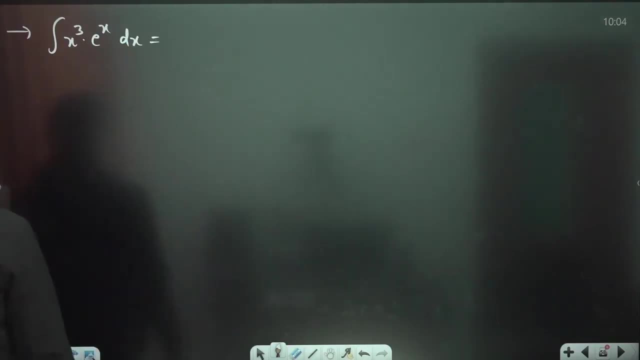 suppose, if I calculate integral X cube. suppose if I calculate integral X cube into: e power X DX- simple case okay. X into e power X DX- simple case okay. X into e power X DX- simple case: okay. X cube into e power X DX, for example: okay. cube into. e power X DX, for example: okay. 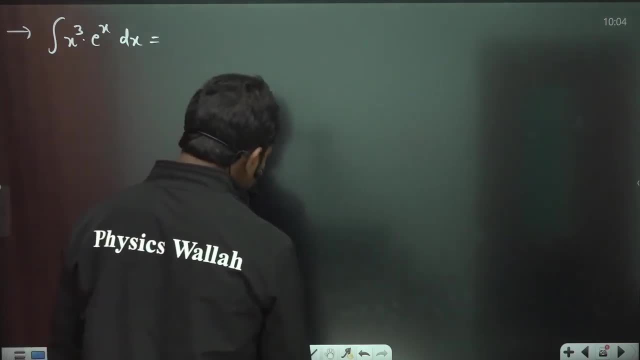 cube into e, power, X, DX, for example. okay, now let us see what or how it happens now. let us see what or how it happens. now, let us see what or how it happens. okay, so, first function into integration. okay, so, first function into integration. okay, so first function into integration of. second function, minus integral of: 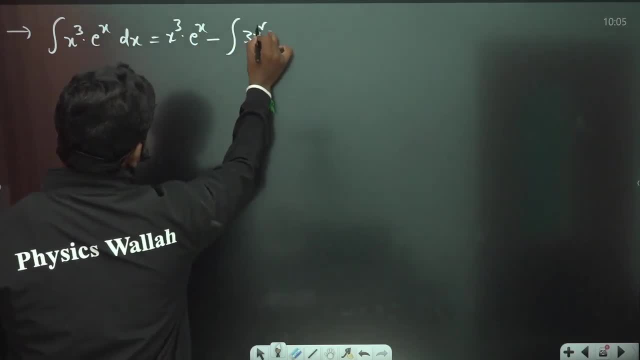 of second function minus integral of of second function minus integral of differentiation of this first function. 3. differentiation of this first function. 3. differentiation of this first function. 3, X square into integration of second X square into integration of second X square into integration of second function, which is again e power X, DX. so 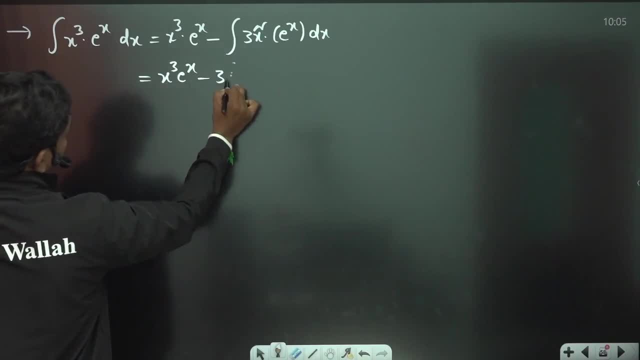 function which is again e power X DX. so function which is again e power X DX. so X cube into e power X minus 3 times off. X cube into e power X minus 3 times off. X cube into e power X minus 3 times off. now integral X square into e power X. so. 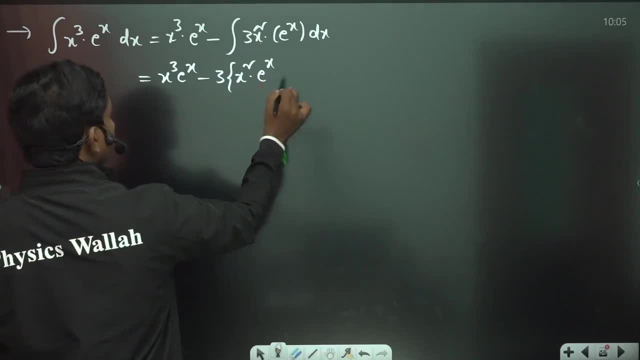 now integral X square into e power X. so now integral X square into e power X. so again first function into integration of again first function, into integration of again first function, into integration of second function minus integral derivative, second function minus integral derivative, second function minus integral derivative of this first function, which is 2x, into 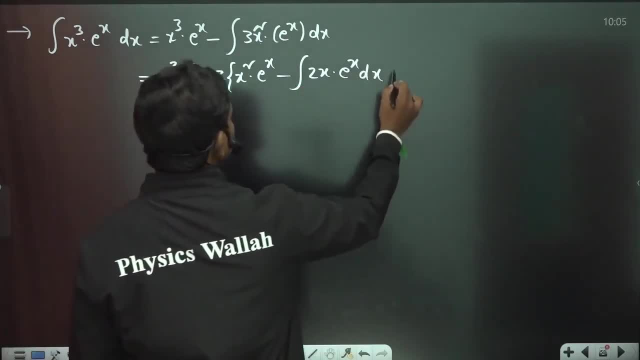 of this first function, which is 2x into, of this first function, which is 2x into integration of that, so plus so, integration of that, so plus so, integration of that, so, plus. so. basically, this is what you have, okay, so, basically this is what you have, okay, so, 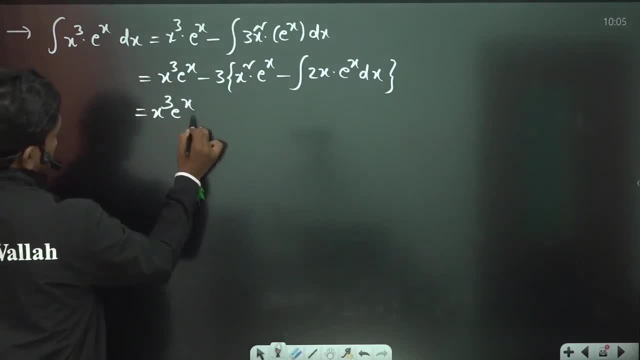 basically, this is what you have, okay. so if you simplify this X cube e power X, if you simplify this X cube e power X, if you simplify this X cube e power X minus 3 X square e power X, so minus of minus 3 X square e power X, so minus of. 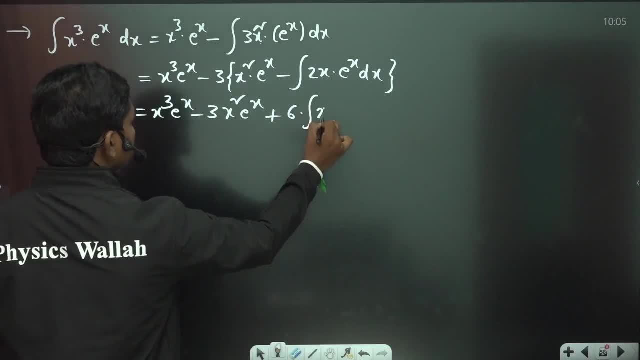 minus 3 X square e power X. so minus of minus plus and 2. if you pull out 6 times minus plus and 2, if you pull out 6 times minus plus and 2, if you pull out 6 times of integral X into e power X, DX is what? 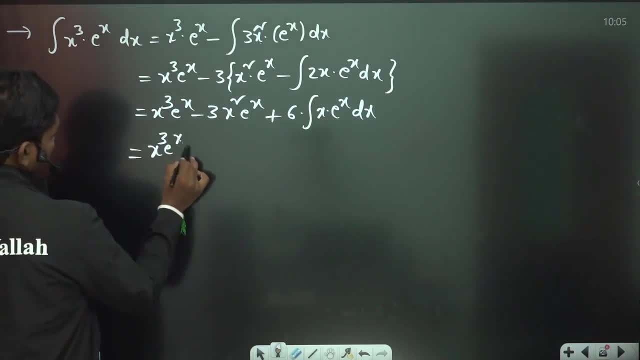 of integral X into e power X DX is what of integral X into e power X DX? is what you have, so X cube e power X minus 3 X. you have. so X cube e power X minus 3 X. you have so X cube e power X minus 3 X square, e power X plus 6 into this. 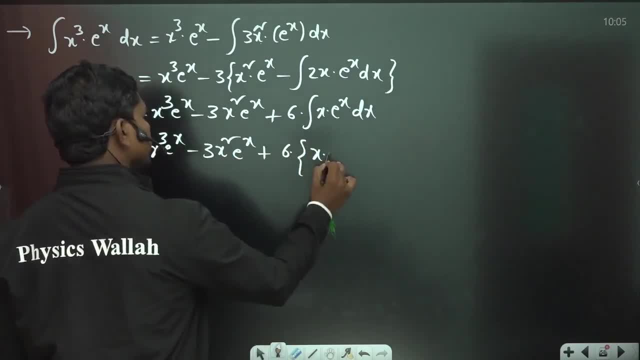 square e power X plus 6 into this square e power X plus 6 into this integration. if you simplify this first integration, if you simplify this first integration, if you simplify this first function into integration of second function, into integration of second function, into integration of second function, is this minus integral? 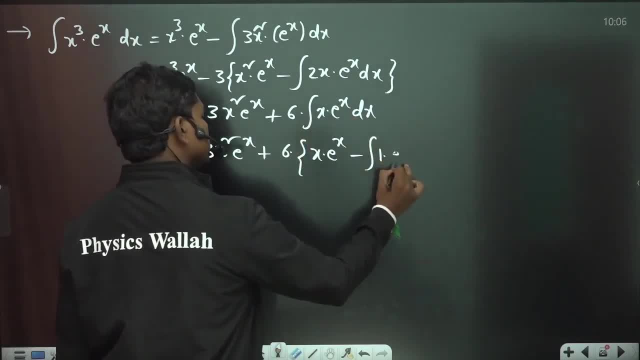 function. is this minus integral function? is this minus integral? differentiation of this first function is differentiation of this first function is differentiation of this first function is: one integration of e power X is e power. one integration of e power X is e power. one integration of e power X is e power, X DX. this is what you have. so if you 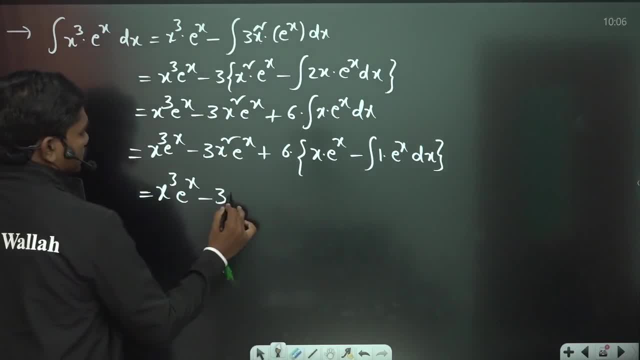 X DX, this is what you have. so if you X DX, this is what you have. so if you write the final result, you have X cube e write the final result: you have X cube e write the final result: you have X cube e power X minus 3 X square e power X plus. 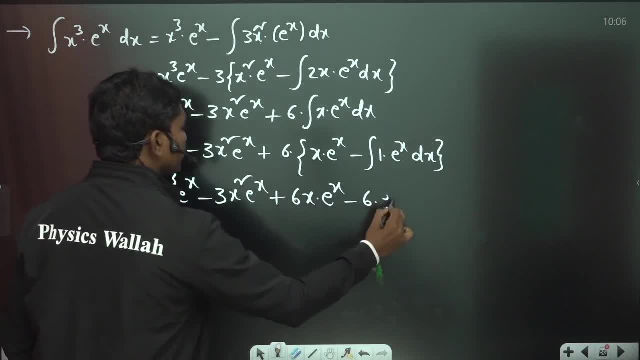 power X minus 3 X square e power X plus power X minus 3 X square. e power X plus 6 X. e power X minus 6 times of e power X 6 X e power X minus 6 times of e power X 6 X e power X minus 6 X plus constant. now, if you are deleting the 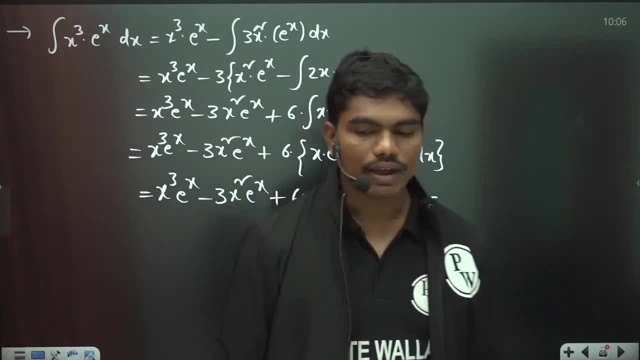 constant, now if you are deleting the constant, now if you are deleting the integration. so this is how you apply integration. so this is how you apply integration. so this is how you apply by parts, now in by parting why I have taken. by parts, now in by parting why I have taken. 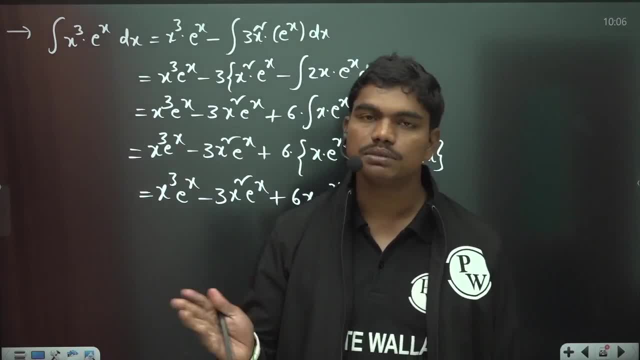 by parts, now in by parting, why I have taken the first function as X cube. because the first function as X cube? because the first function as X cube? because if you follow the islet order, a comes. if you follow the islet order, a comes. if you follow the islet order, a comes before. e correct. so algebra functions. 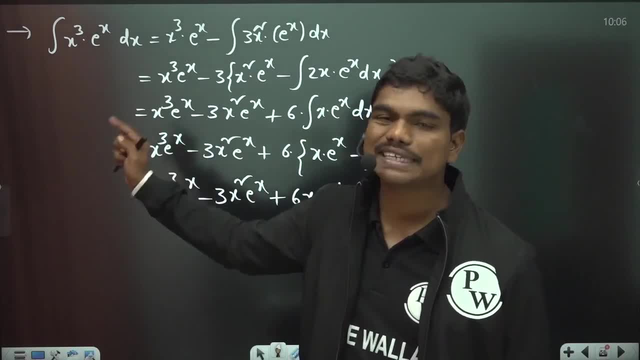 before. e correct. so algebra functions before. e correct. so algebra functions must be taken before exponential functions must be taken before exponential functions must be taken before exponential functions. so that's why I have taken X cube. so that's why I have taken X cube, so that's why I have taken X cube here. okay, so X cube is taken as the first. here. okay, so X cube is taken as the first here. okay, so X cube is taken as the first function and I have done the integration function and I have done the integration function and I have done the integration. but if okay, I have got some four five. but if okay, I have got some four five. 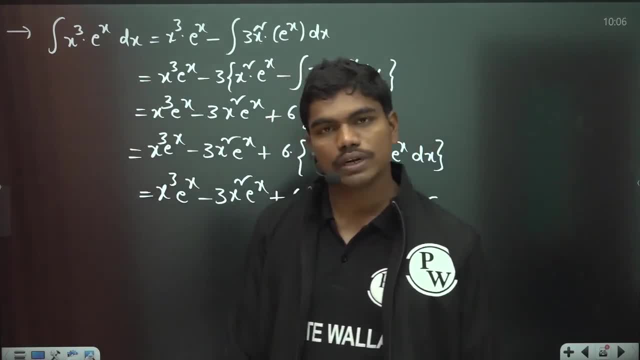 but if okay, I have got some four, five steps and you know I have got the answer steps and you know I have got the answer steps and you know I have got the answer. but if you see there is one technique in, but if you see there is one technique in, 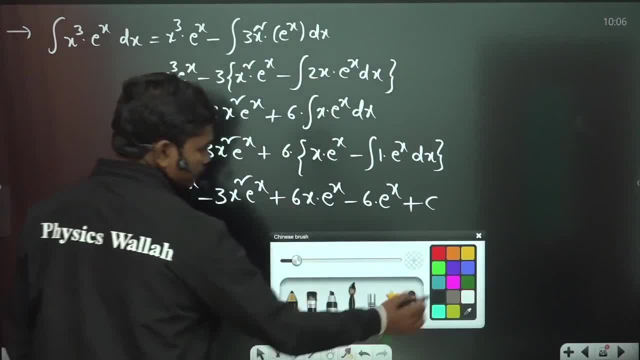 but if you see, there is one technique in integrations, that integral UV, let us integrations that integral UV, let us integrations that integral UV. let us suppose if we have a lot of two. suppose if we have a lot of two. suppose if we have a lot of two functions, integral u into V, let us. 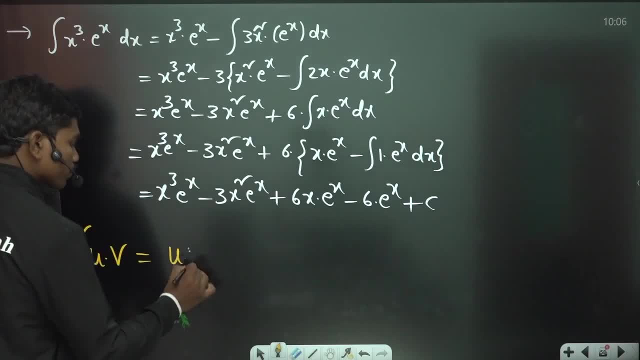 functions integral u into V. let us functions integral u into V. let us suppose: if we have this, we get this as u suppose. if we have this, we get this as u suppose. if we have this, we get this as u into V. 1 V 1 is integration first. 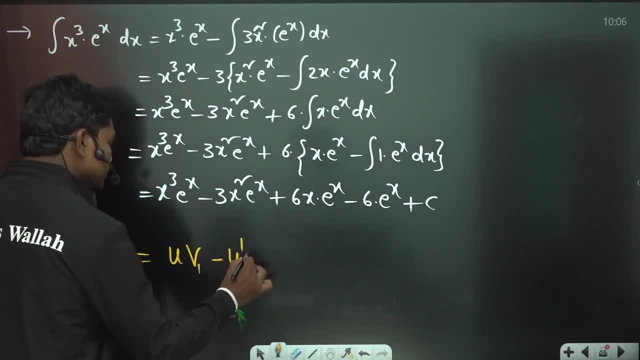 into V 1. V 1 is integration first into V 1. V 1 is integration first. integral of V okay, minus u. dash into V 2, integral of V okay, minus u. dash into V 2. integral of V okay, minus u. dash into V 2, plus u. double dash into V 3, minus u. 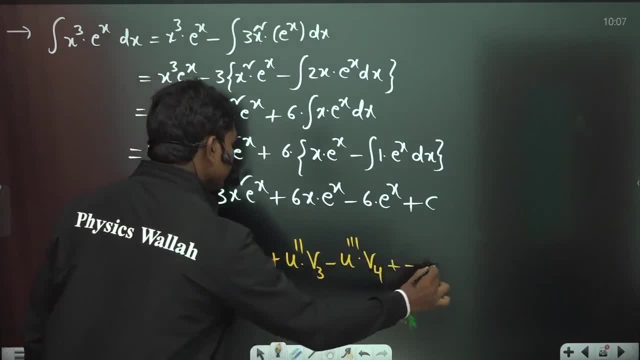 plus u double dash into V 3 minus u plus u double dash into V 3 minus u table dash into V 4 plus, and so on. like table dash into V 4 plus and so on. like table dash into V 4 plus and so on, like this. okay, this goes on. actually, now what? 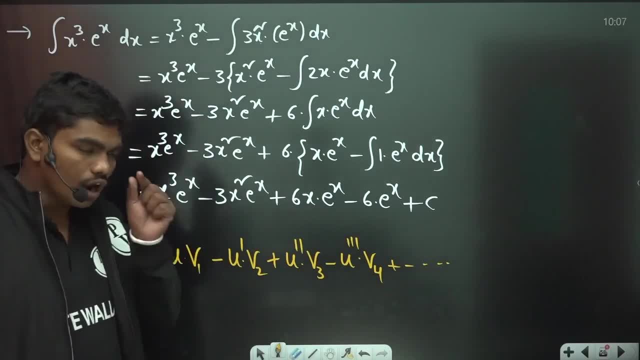 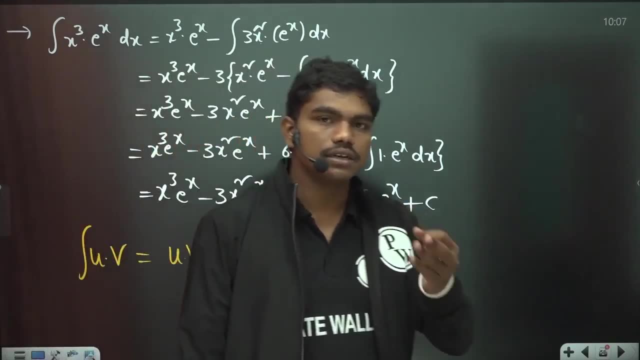 this okay, this goes on actually. now what happens whenever this u first function is algebraic function of some finite degree, then what happens? after certain terms, the differentiation term becomes zero. for example, if you differentiate a third degree function four times, then what happens? differentiation is zero. for that, correct. 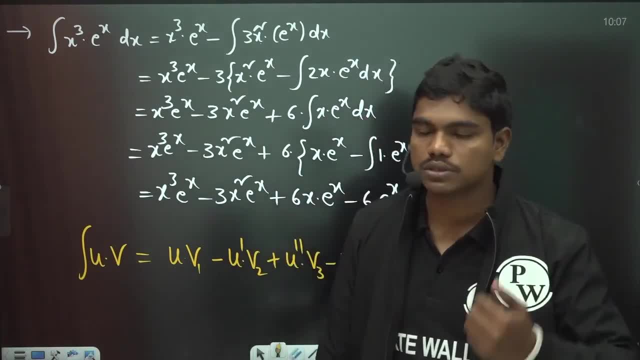 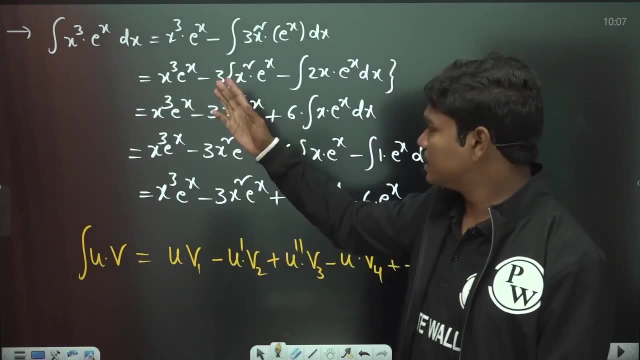 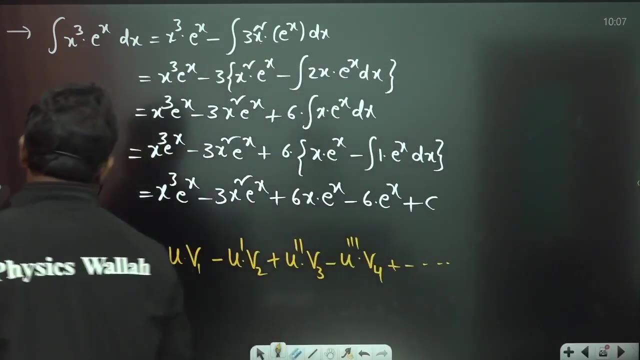 similarly, if you differentiate a quadratic function three times, then derivative becomes zero. so whenever one of the functions is actually algebraic function having certain finite power, then definitely this differentiation will come to zero after some time. so you can simplify the result easily. for example, in this case, if you see integral x cube into e power, x, dx. so if you 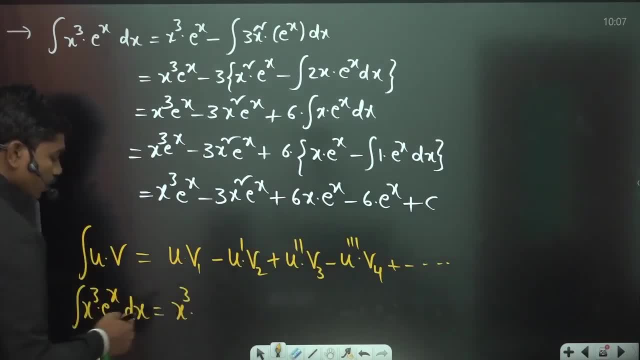 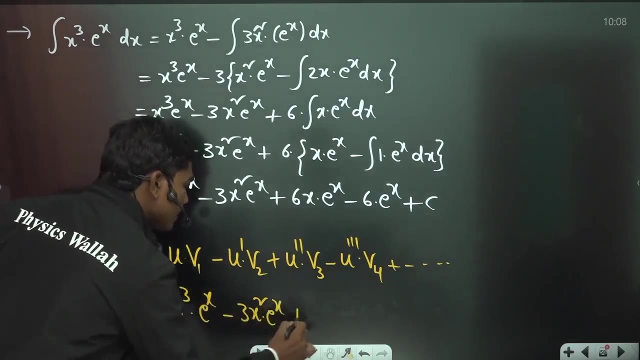 take first function x cube into what is integration of this. e power x. e power x, okay, minus- derivative of this x cube. 3x square into what is the integration of this function. e power x function again. e power x plus derivative, second derivative of this function. so this 3x square is the first. 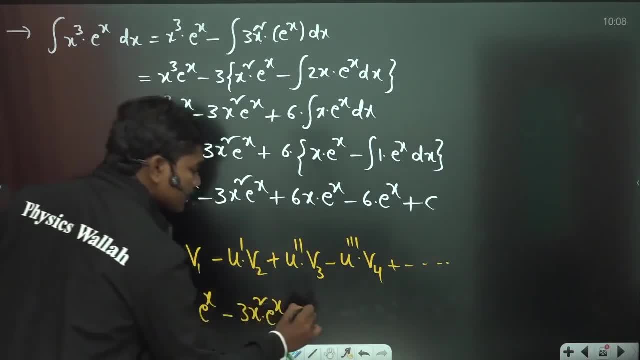 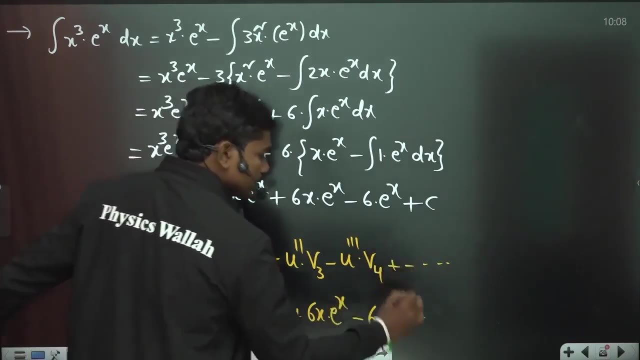 derivative way too. so what is the differentiation of this 3x square 6x into integration of this e power x, again e power x, minus differentiation of this 6x, 6 into integration of this e power x, e power x plus differentiation of this 6: 0. that's it from here. it is finished. so we learned off to a. 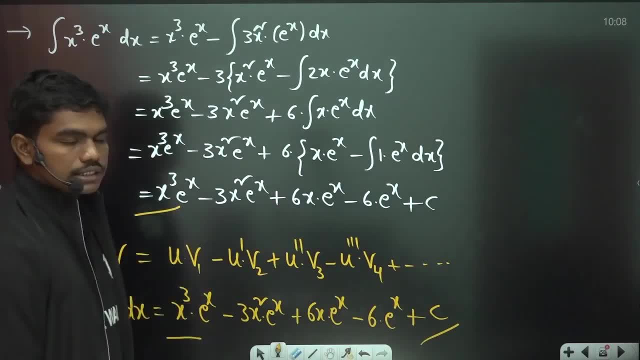 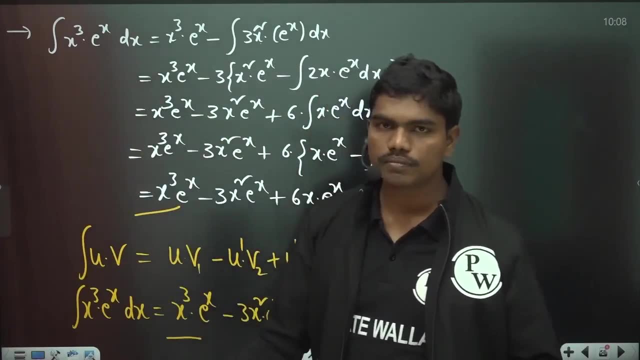 constant and if you see this result and this result, both are same. actually okay. but this technique is generally helpful only when one of the functions is algebra. or you can say: first function is algebraic function with some finite degree. actually okay, let us suppose, if in place. 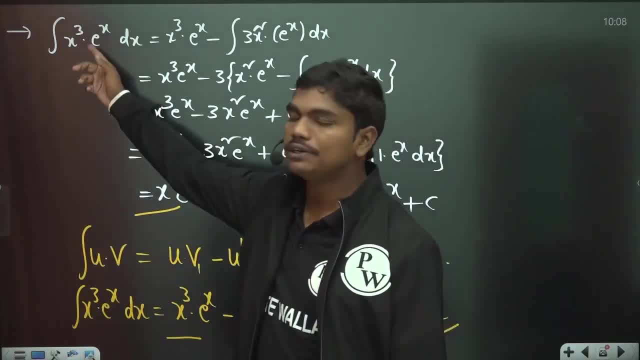 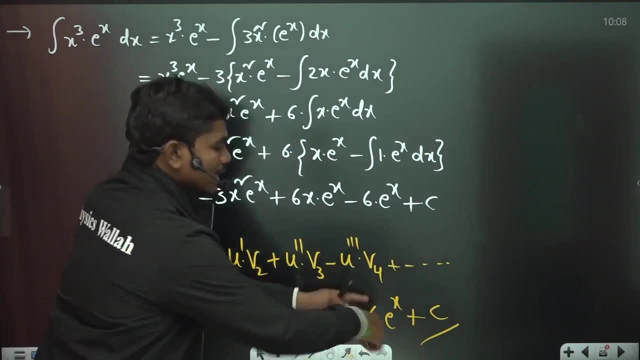 of x cube. if i have some sine x or cos x, for example sine x into e power x or cos x into e power x, is there then what happens? sine x, cos x minus sine x, minus cos x, again sine x. this loop keep on repeating. i'll never come to a conclusion. okay, i'll never can get my saves. but when one of 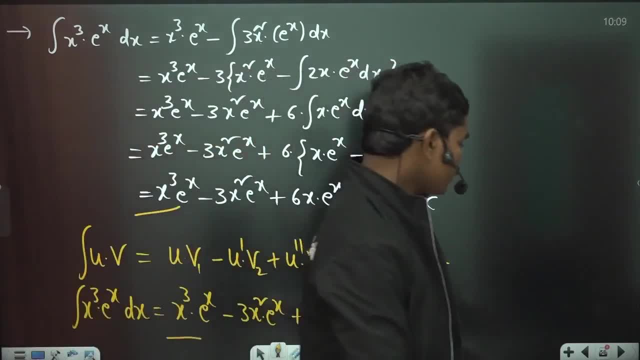 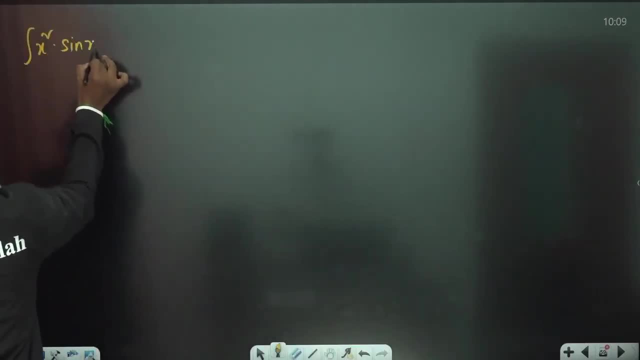 the functions is algebraic. you can definitely go for this technique, actually clear next. so, similarly, if you write this function x, square into sine x, if you write this sine x, dx, so first function, into integration of sine x, integration of sine x is minus cos x. that integration of sine x is minus cos x. okay now. 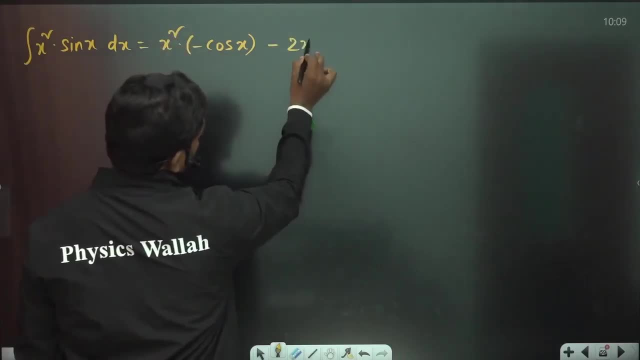 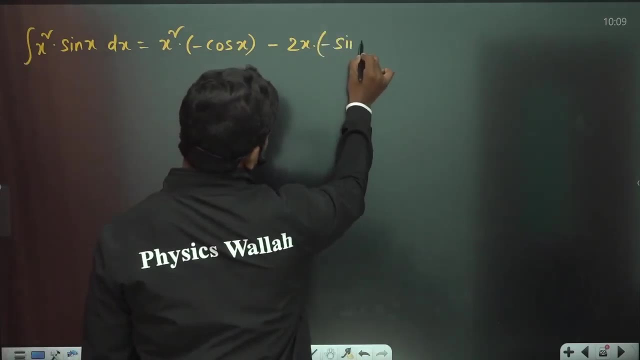 minus derivative of x square 2x into integration of minus cos x. what is the integration of minus cos x? minus sine x, so minus sine x, because if you differentiate minus sine x, then you'll get minus cos x plus differentiation of 2x- 2. 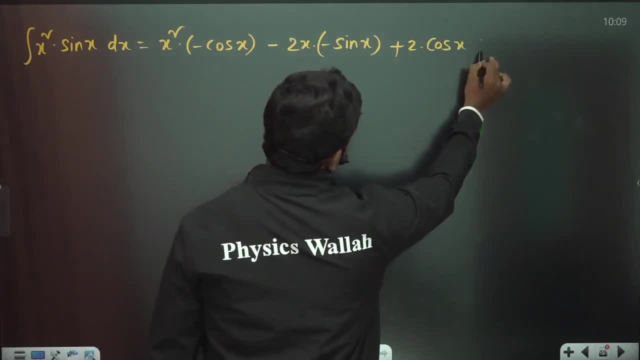 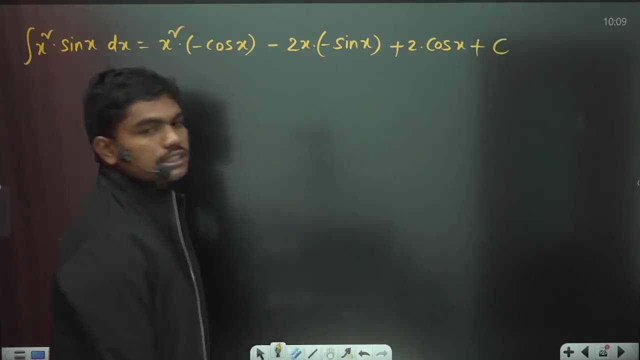 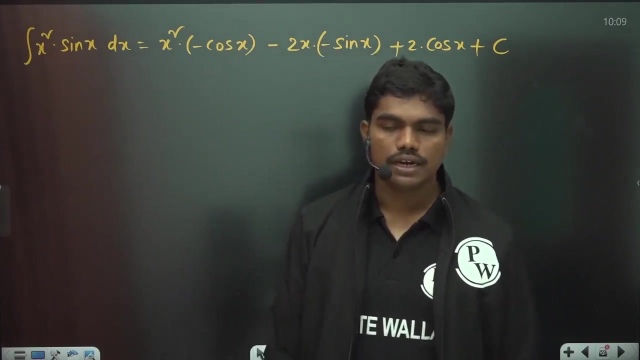 into integration of minus sine x, cos x plus differentiate, sorry, minus differentiation of 2: 0. so we'll write some arbitrary constant here that c is got ended up. so this is how you actually do the uv integration, depending upon the things like this. okay now, so with this we 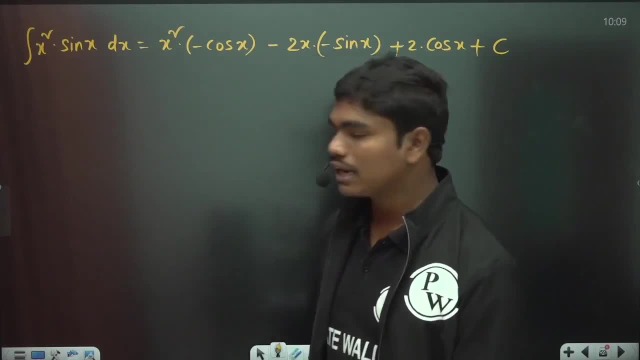 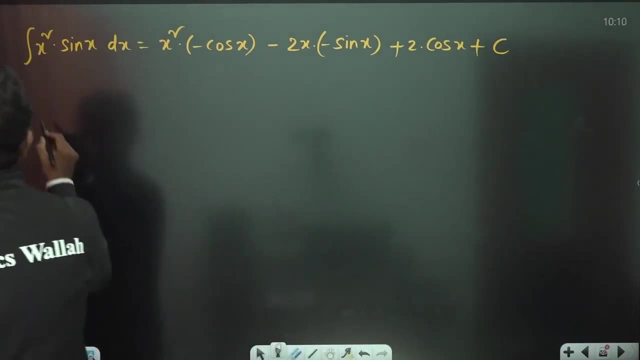 generally. uh, you know, close this. uh, okay, before closing, i would like to give one, one result, which is for sine inverse x, because i promised you that i'll give, so see here: integral sine inverse x- dx. integral sine inverse x- dx. so what we'll do? integral sine inverse x into 1 dx, let us add. 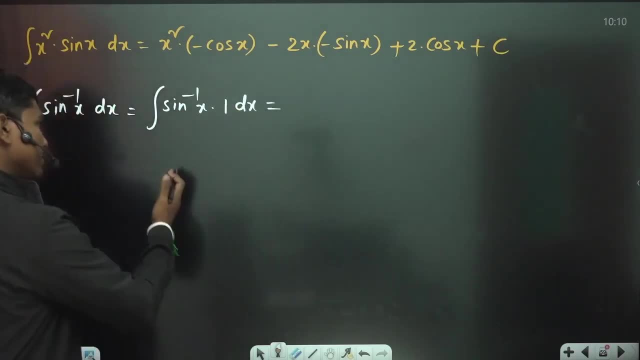 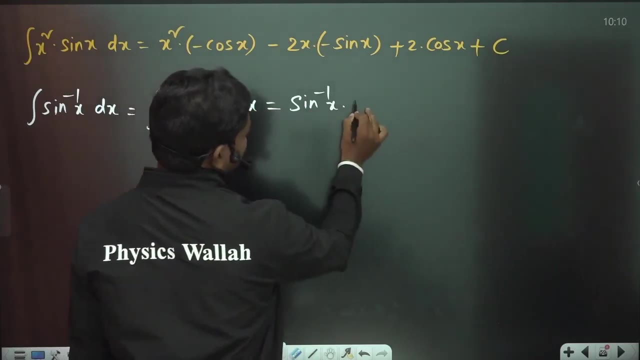 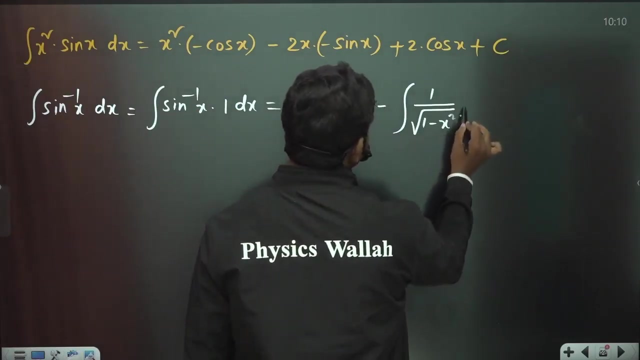 this. okay. so this is again sine inverse x. so eilat principle inverse: this is already in the first place. so integration of this is sine inverse x into integration of this. one is x minus integral derivative of sine inverse x: 1 by root of 1 minus x square into integration of this. 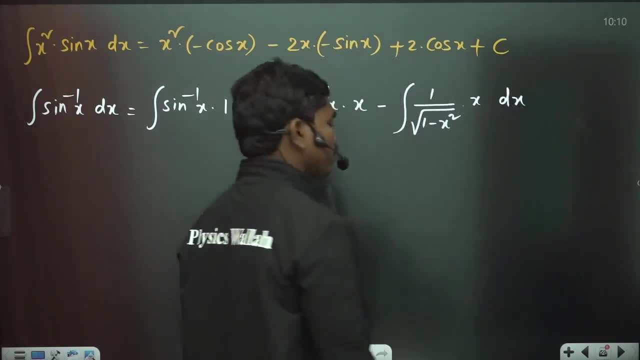 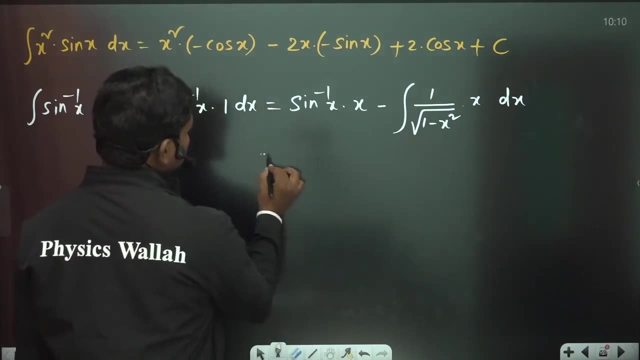 one is x, dx. okay, so this is what you have. basically, you applied this by parts, integration by parts, okay. so if you calculate this, then this integration is equal to x into sine inverse x. next, if you see the differentiation of 1 minus x square, this is minus 2x. so what we can do, 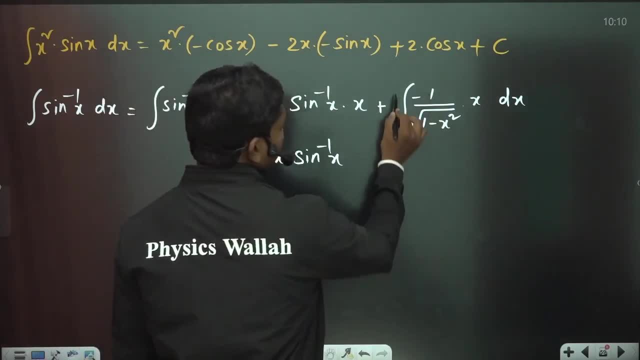 we'll multiply a minus inside and outside. we'll write 1 by 2 and a 2 here. okay, if you multiply, then you can see x into sine inverse, x plus half into this. one is x, dx. okay, so this is what you have. basically, you applied this by parts integration. 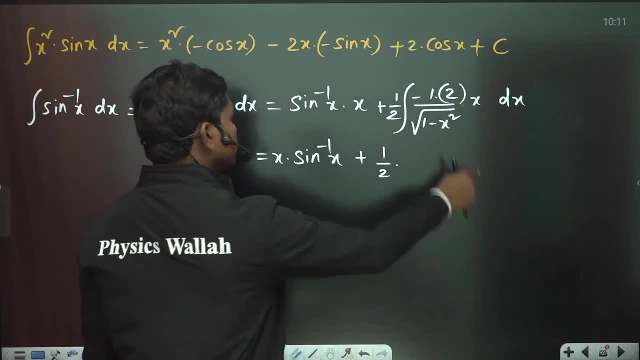 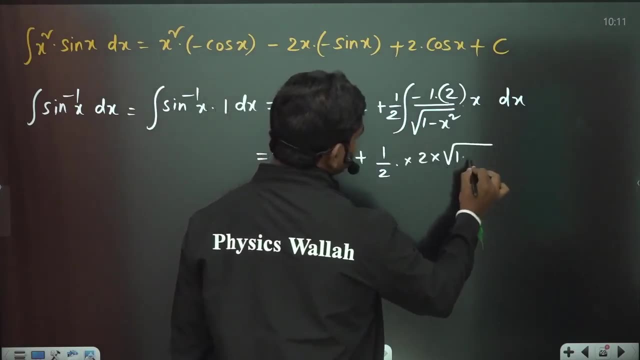 this is integration of minus 2x by root of 1 minus x square. so if 1 minus x square is your function, this minus 2x is like f dash of x. so this is 2 times of root, f of x. so 2: 2 gets cancelled. 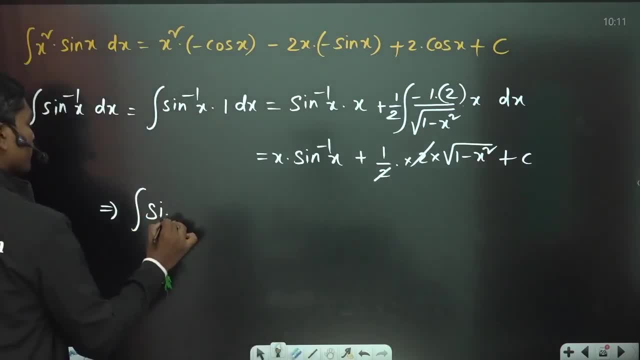 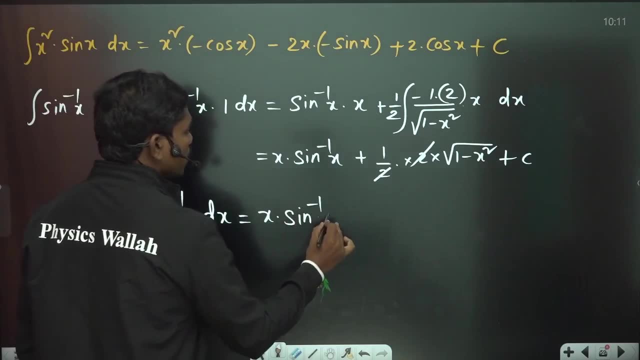 so basically, integral sine inverse x dx, integral sine inverse x- dx is equal to x into sine inverse x plus root of 1 minus x, square plus constant. okay, so this is how you can calculate integration of sine inverse x. similarly, log also, you can take log as one function and one as second function. and 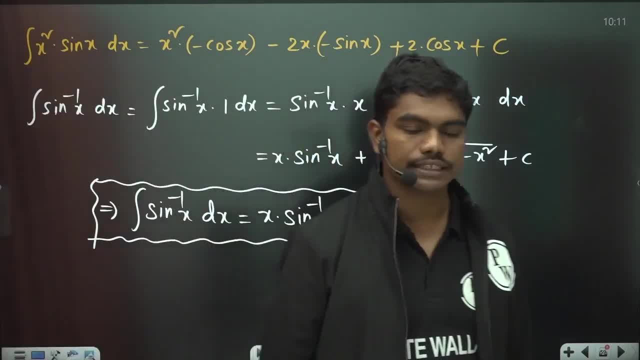 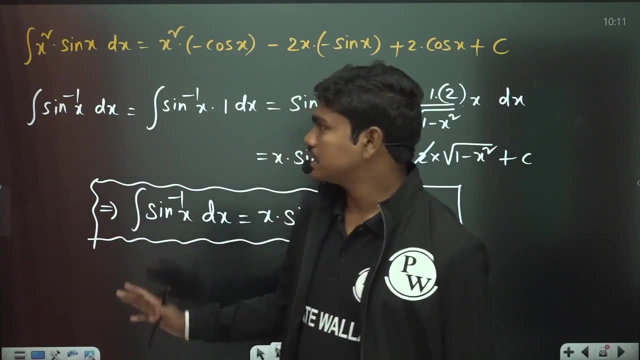 you can do the integration in by parts, okay, then you'll get x into log, x minus x, okay. so all these things are very, you know, simple things. so this is what you have with, uh, this, uh, you say, uh, indefinite integrals. okay, so now let us see some properties of definite integration. okay, so properties of 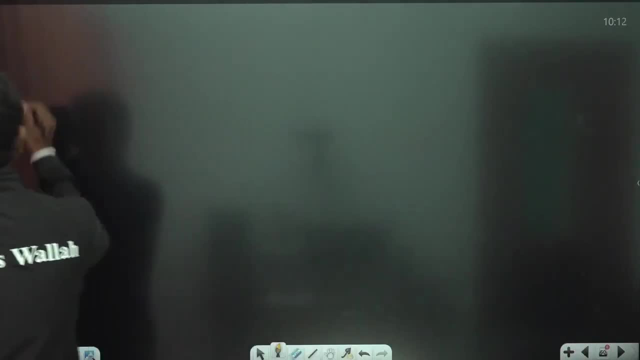 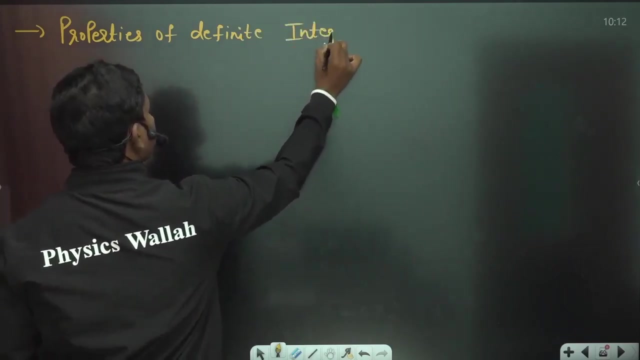 definite integration, which is one important part actually. so see, properties of definite integration means basically summing up properties of definite integrals, properties of definite integrals. okay, so see here properties of definite integrals. so first property, you know, integral a to b, f of x, dx, this is equal to minus. 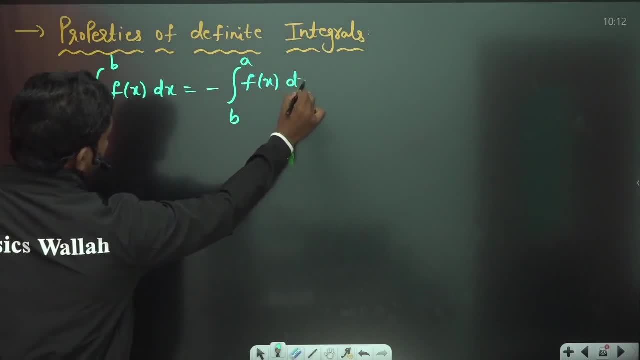 integral b to a, f of x, dx. why? because we have defined this integration as capital f of b minus capital of a, if you remember correct. so let us suppose if i change the integrations then that becomes capital f of a minus capital of b. there is some minus sign difference between these two. 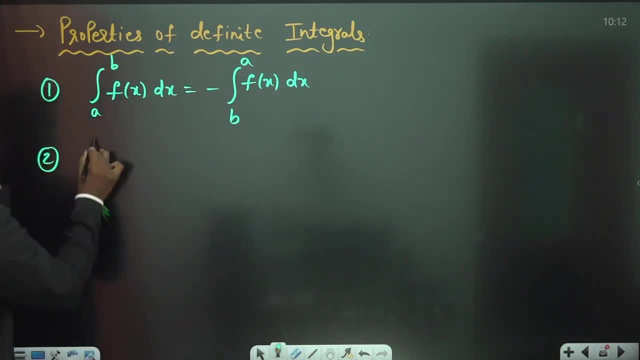 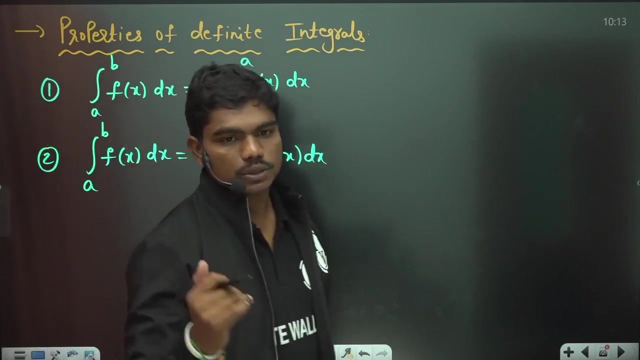 so that's why a minus sign is kept here. second, integral a to b f of x- dx is equal to integral a to b f of a plus b minus x dx. of course, in all these examples i am assuming f of x is differentiable at a waypoint. okay, so that's why i'm taking directly. so if f of x is, 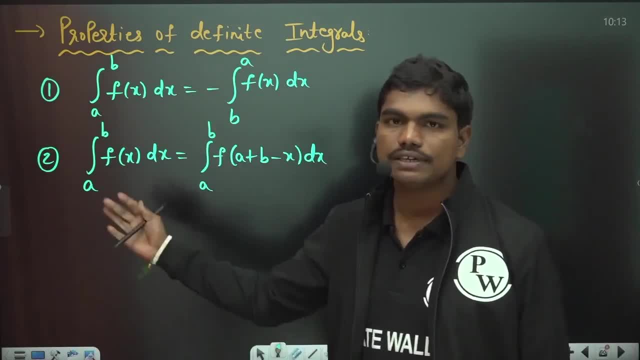 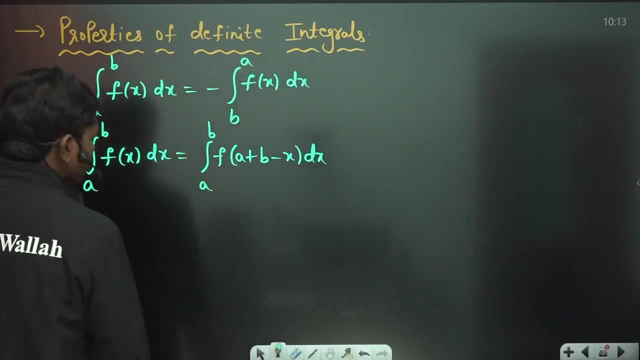 differentiable, only then i can write this, because if it's not differentiable, then derivative doesn't exist. you cannot integrate them, basically, okay. so this is how we can write. okay, and how this is coming. it's very simple. if you see some one, two steps, you can write: look, let us take this integral. 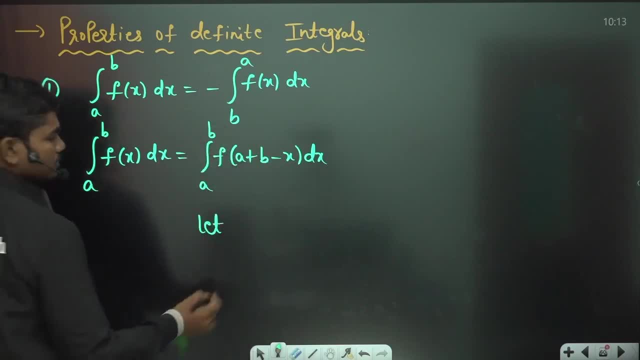 okay, so let, because some of you might be interested how this comes. so let: a plus b minus x is equal to t. then what happens if you differentiate this? differentiation of a: 0 plus, differentiation of b: 0 minus dx is equal to dt. so dx can be replaced with minus dt. what about lower limit, lower limit? 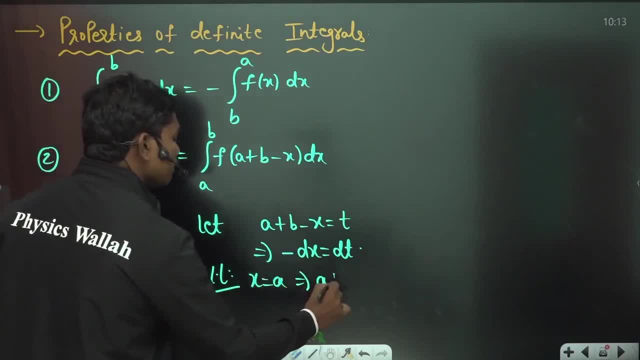 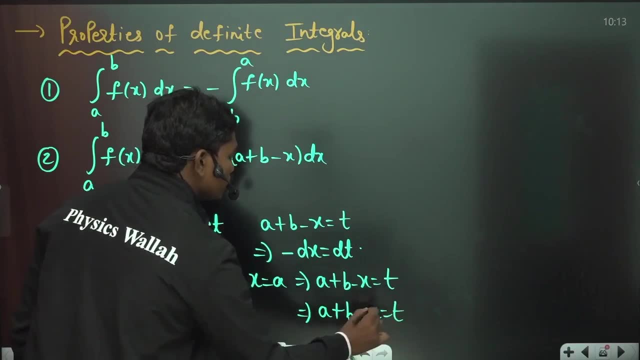 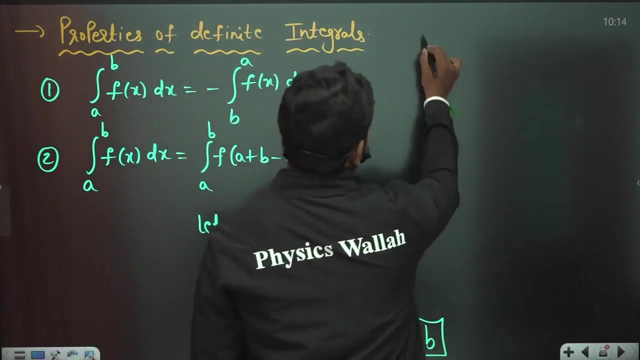 x is equal to a right. so this implies a plus b minus x is equal to t. so if you replace, x is equal to a. a plus b minus a is equal to t. so a, a gets cancelled. so t is equal to b. t is equal to b. next upper limit: if you calculate upper limit, what comes here, a plus b minus x- is: 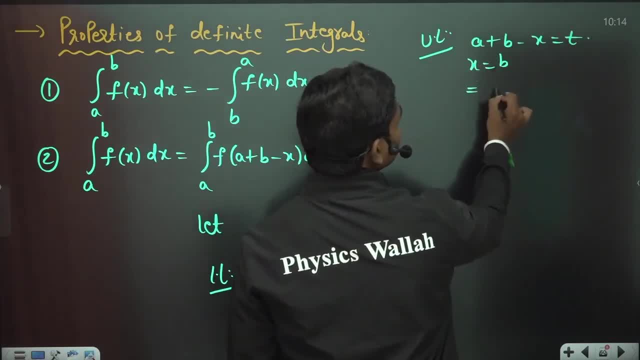 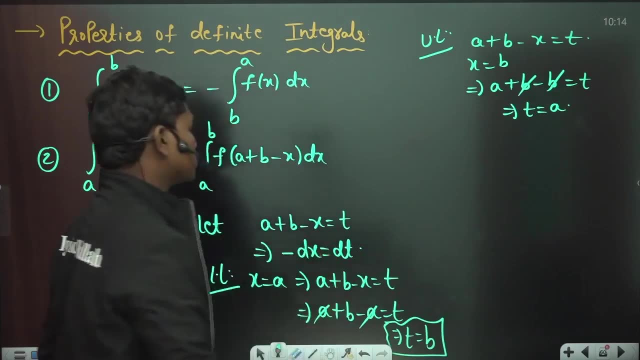 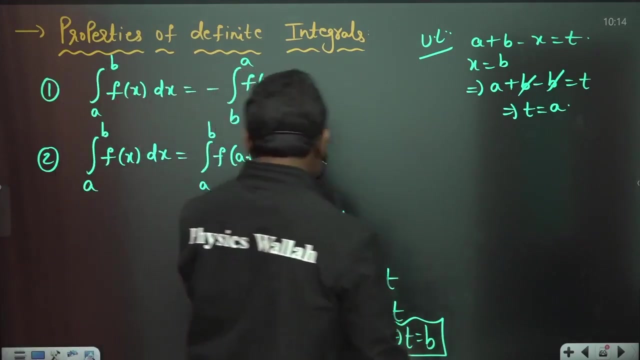 equal to t and in case of upper limit in terms of x, x is equal to b. so this implies a plus b minus b is equal to t, so t is equal to a. so by making the substitution a plus b minus x is equal to t. u dx is minus dt, lower limit is b, upper limit is a. so if you substitute all these four things in 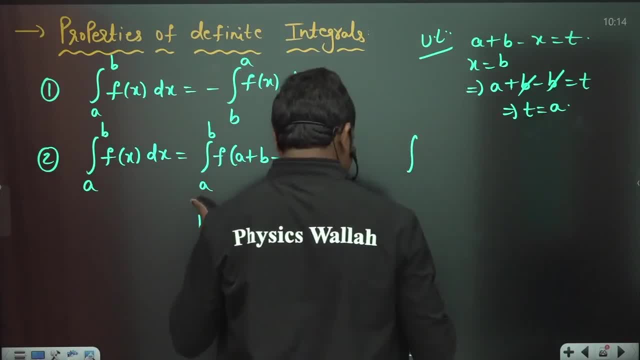 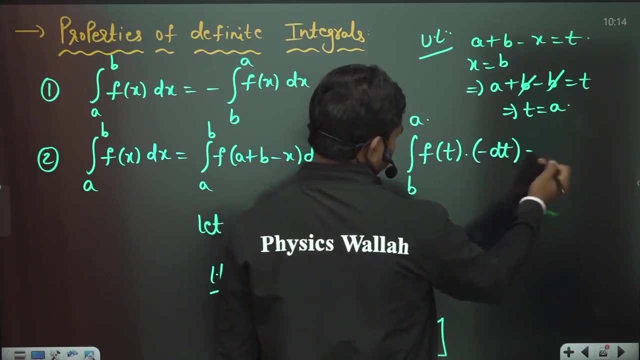 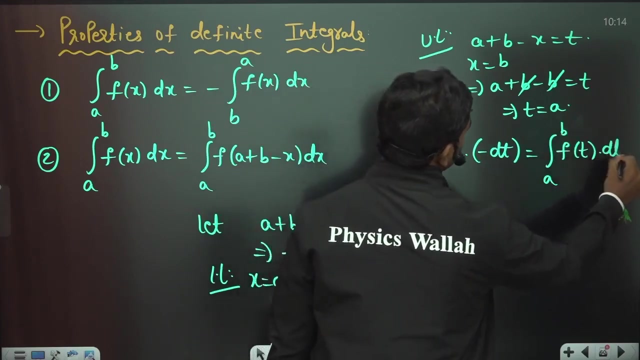 this integration integral lower limit became cap small b 2 a, f of t into dx is nothing but minus dt a sign. if you change this limits, this becomes integral a to b, f of t, dt. okay, so this is how you have the things. so this is same as integral a to b, f of x, dx. whatever could be the variable. 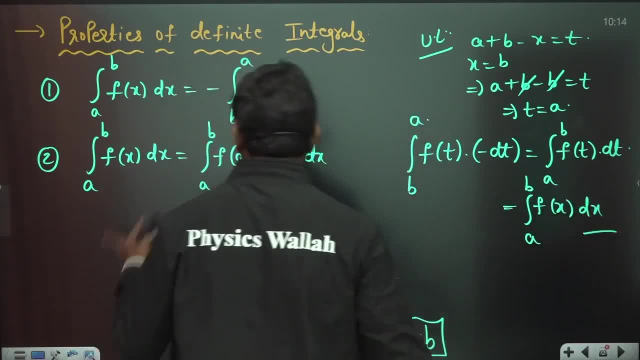 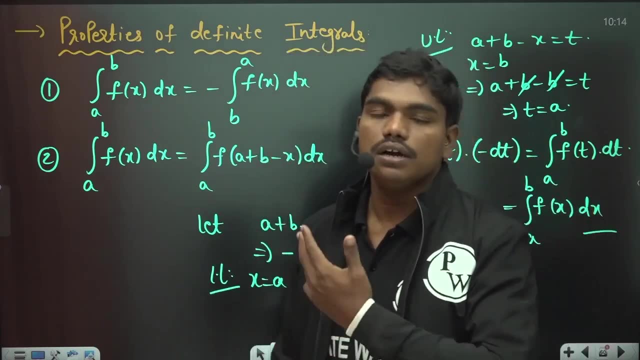 the result remains same. so that's how these two integrals are actually the same value and this is actually one very important, you know property of definite integration. you will be able to solve some good you know integrals using these things. okay, so integral a to b, f of x, dx, all these. 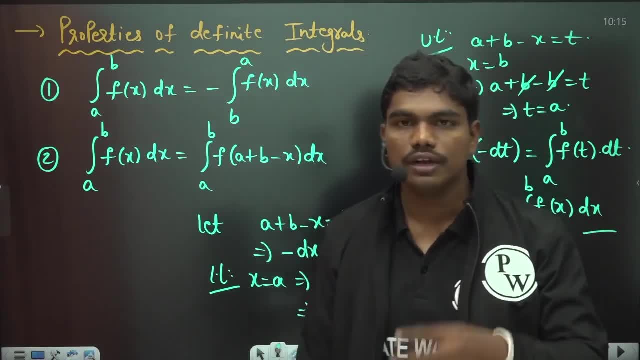 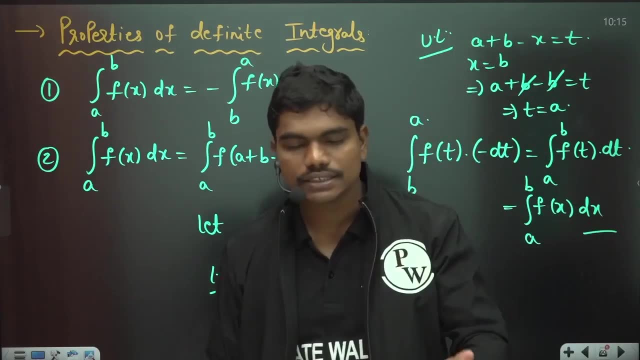 things okay. so right now i'm not looking into the problems. this is a quick go of some revision for the theory. so that's why you are seeing a lot of theory, but later, when it comes to practice, definitely, uh, in practices i will bring the practices also. so very soon and definitely. 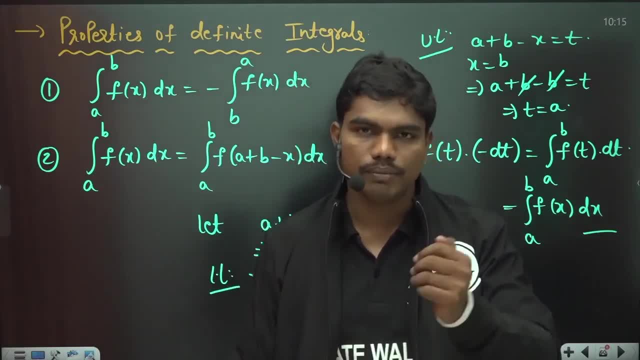 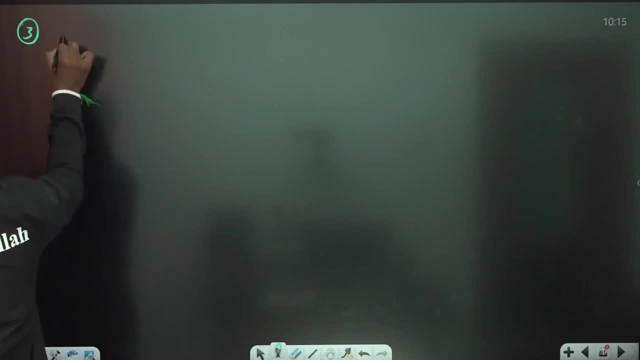 we will try to solve some good questions in mathematics, okay, and that will make you more confident, even okay. so let us look at these properties quickly. third, if c is a point, c is a point, c is a point in a comma b, such that f of x is not a differentiable. 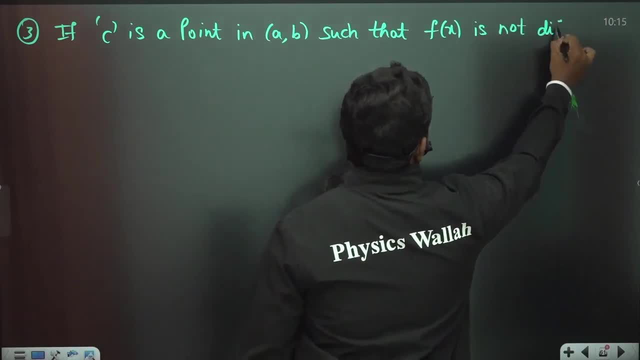 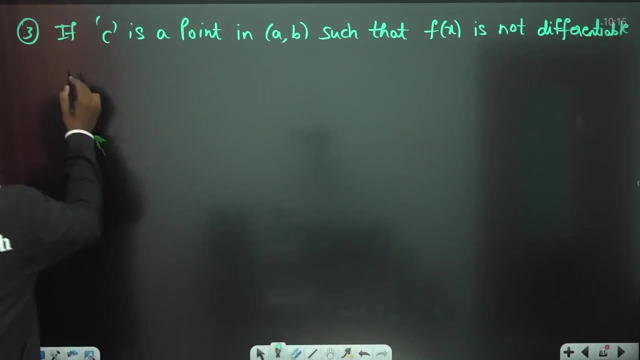 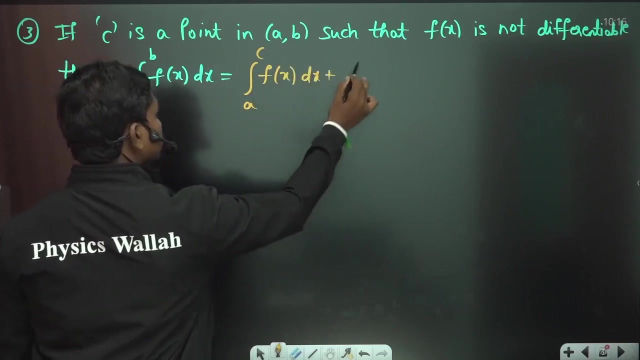 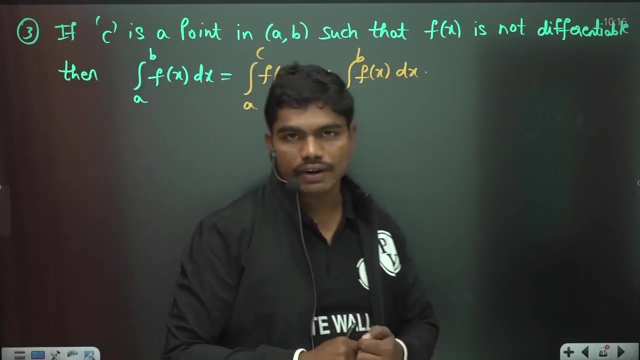 f of x is not differentiable, then integral a to b f of x dx. this is equal to integral a to c, integral a to b f of x dx, plus integral c to b f of x dx. okay, so basically you need to split the integration at that point whenever they are not differentiable. okay means let us suppose for. 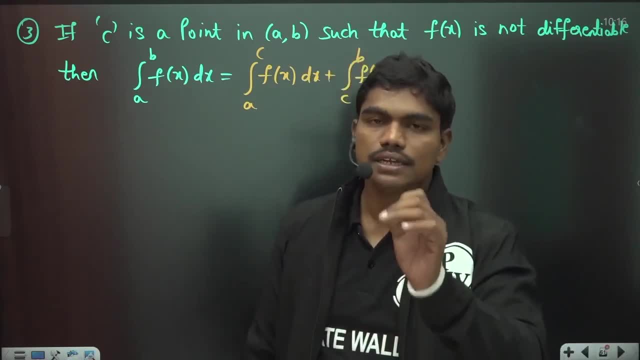 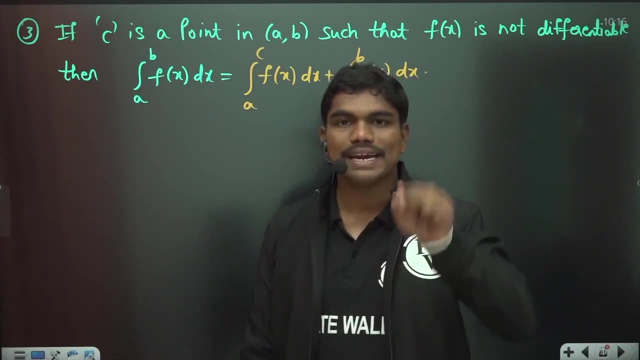 example, if i'm talking about integral minus two to two, mod x, dx- then you need to split the integration at zero, because definitely mod x is not differentiable at x equal to zero. so you need to split that into two: integrals minus two to zero and zero to two. okay, so that's how you need to do. 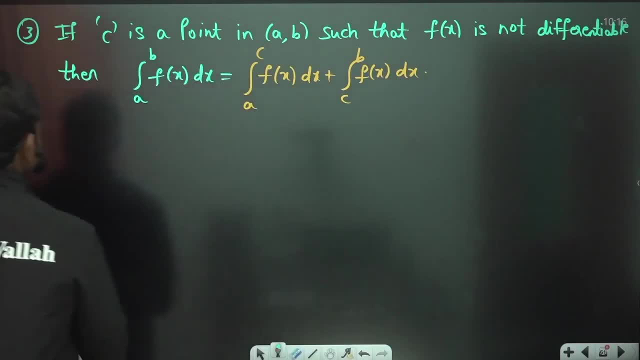 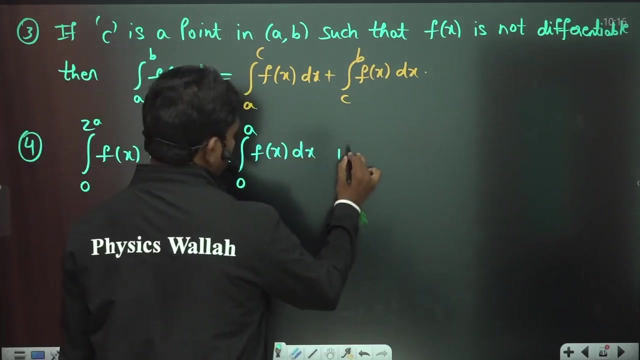 the things. then, fourth, fourth, fifth, you want triangle: f of x, x, x, z x is equal to if- okay, let us avoid this- integral zero to 2 a. f of x dx is equal to 2 times integral 0 to a f of x dx. if f of 2 a. 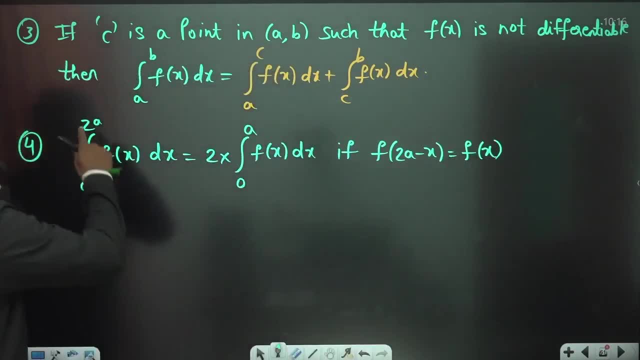 minus x is equal to f of x. okay, so sometimes they give you functions like sin and all and they keep vu 8, pi things like this year. so it is just as Hard to find something that also works in". if this can be split in this form two times of integral 0 to a f of x, dx actually, okay. so 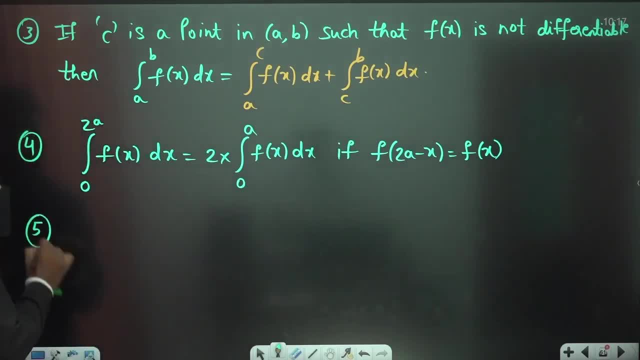 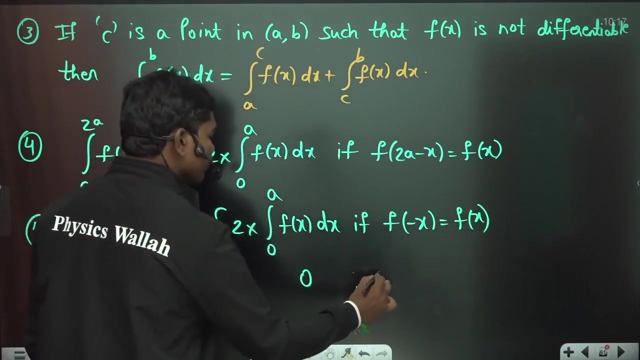 if you can write this now, fifth: integral minus a to a f of x dx is equal to two times of integral 0 to a f of x dx. if f of minus x is equal to f of x, means if this is even function. similarly, this is 0. if f of minus x is equal to minus f of x, means if this is odd function. then this is is. 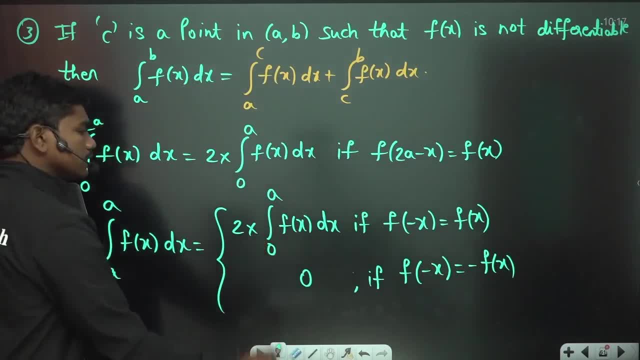 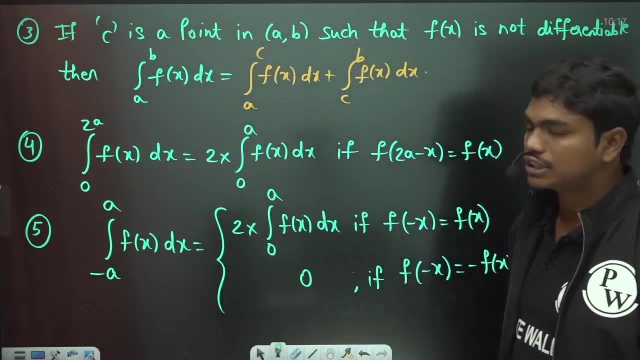 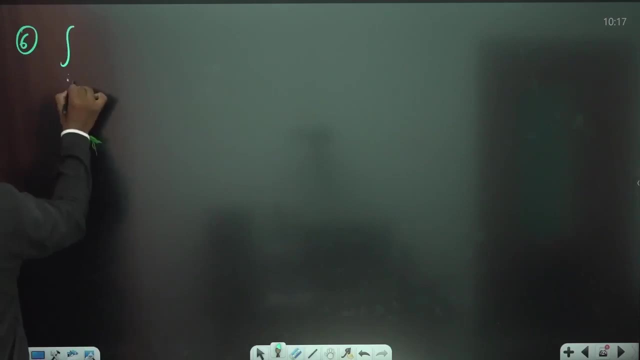 basically 0 directly. okay, so this result is also again useful at many places. whenever you have some even functions, then this minus a to a can be written as two times of this integration actually here. okay, so that's again one important thing. next we'll go for one more property: integral 0 to pi. 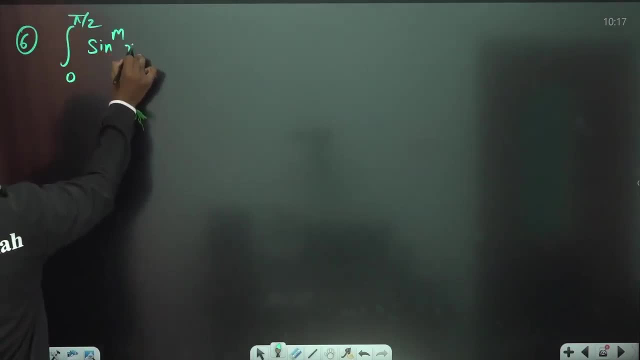 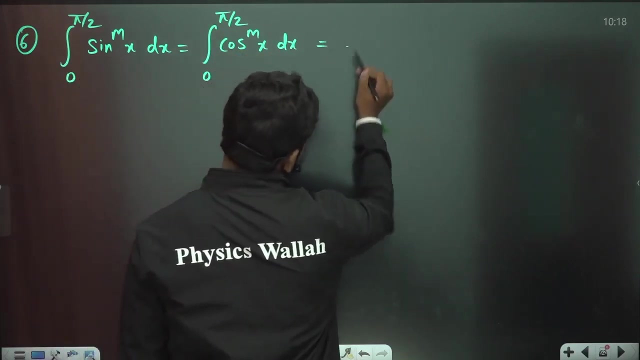 by 2 sine power mx dx, this is 0 to a f of x dx. this result is same as integral 0 to pi by 2 cos power mx dx. okay, so cos power mx dx and this is equal to. basically, if you see, if you write this equation, m m minus 1 into m minus 2 into m minus, 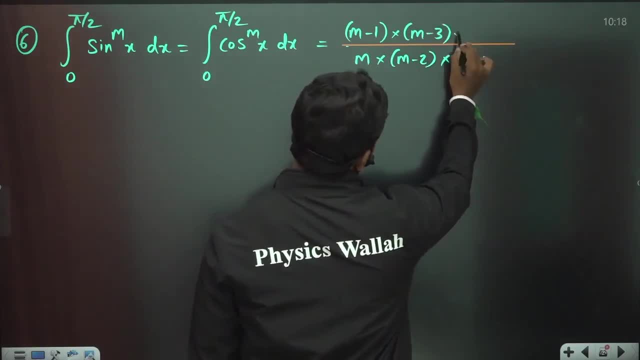 3 into, and so on. this goes on and finally you will end with either 2 by 3 or 1 by 2, depending upon m is even or odd. okay, so if m is even, you will end up the series with 1 by 2. if m is odd, you will come by 2 by 3. 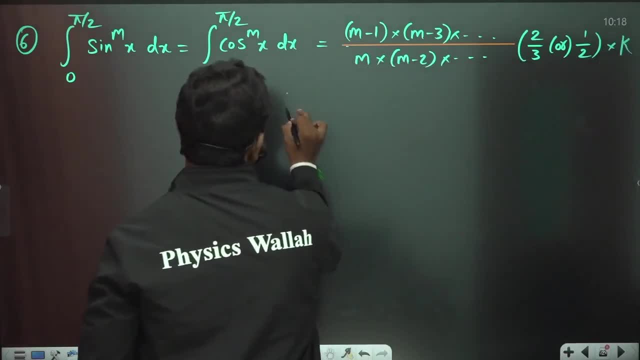 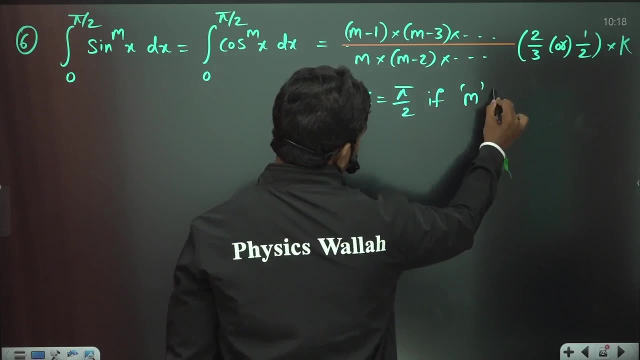 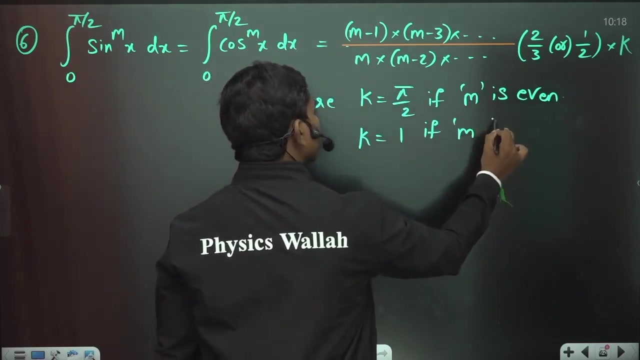 into k. so what is the value of k where? k equal to pi by 2 if m is even, k equal to pi by 2 if m is even and k equal to 1 if m is odd. why this is coming at all we will see when we go for this. 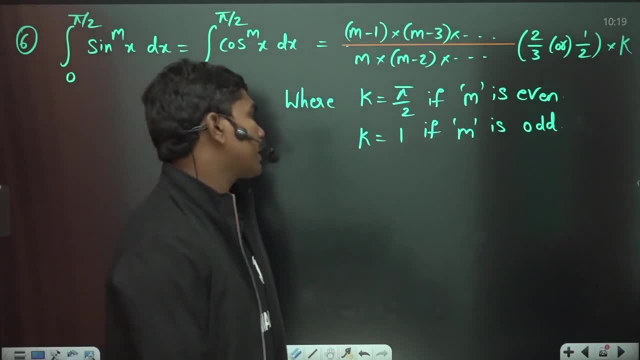 gamma function, all these things. okay, so k equal to pi by 2 if m is even and k equal to 1 if m is odd, and it depends upon this m being even or odd. okay, so one last property i would like to give you here, which is a bit important. so integral 0 to pi by 2, sine power mx. 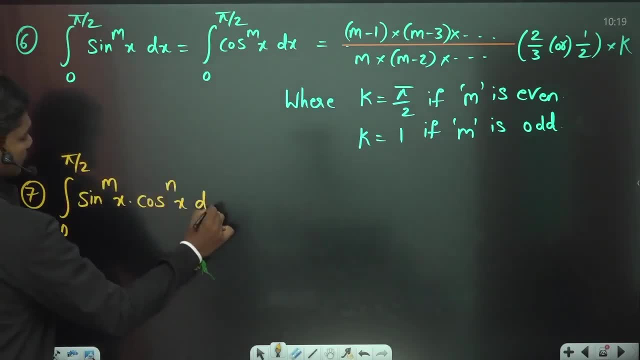 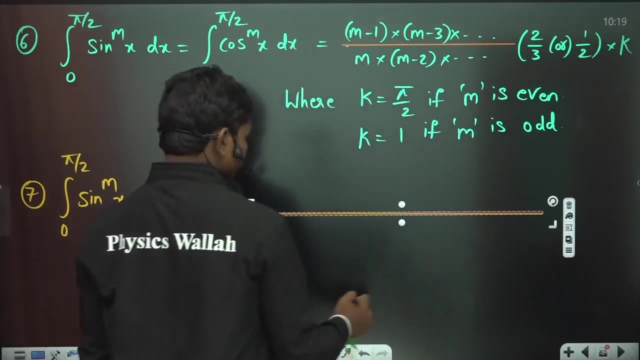 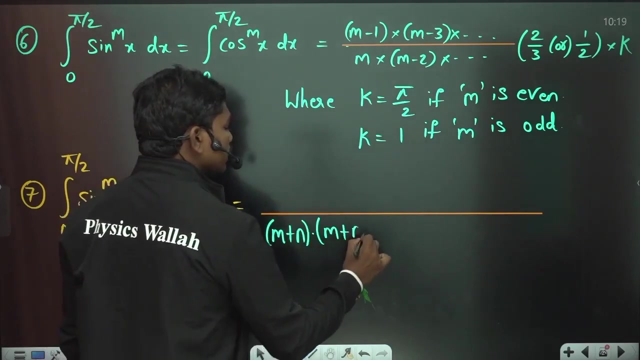 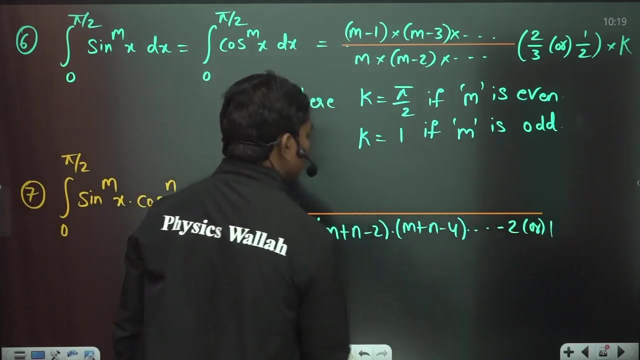 so into cos, power, nx, dx. so this is equal to. if you see, we will have this result. so see here carefully. this is m plus n into, m plus n minus 2 into, m plus n minus 4 into, and so on 2 or 1. now this: 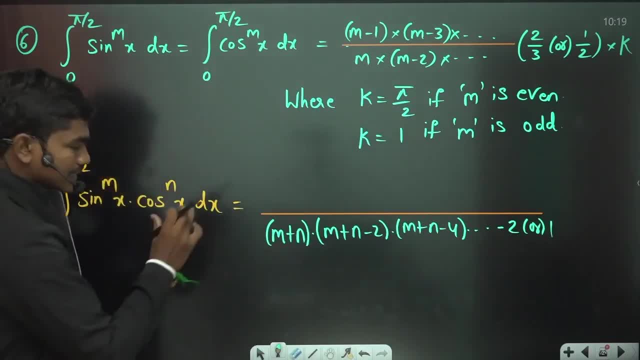 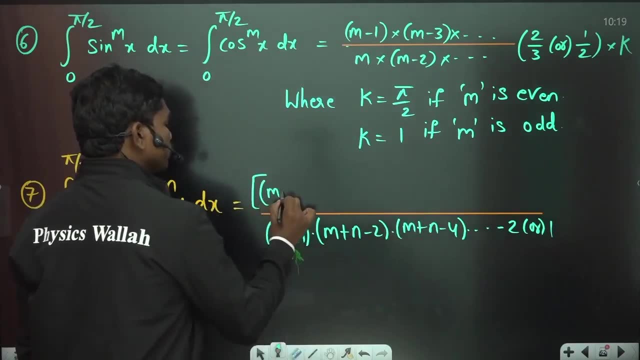 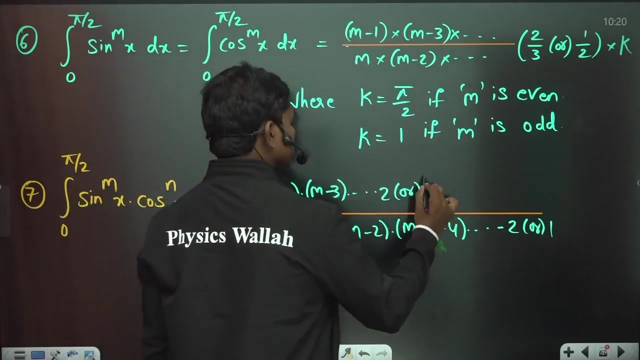 is in the denominator means basically, once you know this m and n values, then you can write m plus 1, then every, all alternative number till 1 or 2, depending upon the things. now, here m minus 1 into, m minus 3 into, and so on 2 or 1. again here into n minus 1, n minus 3, and so on 2 or 1. 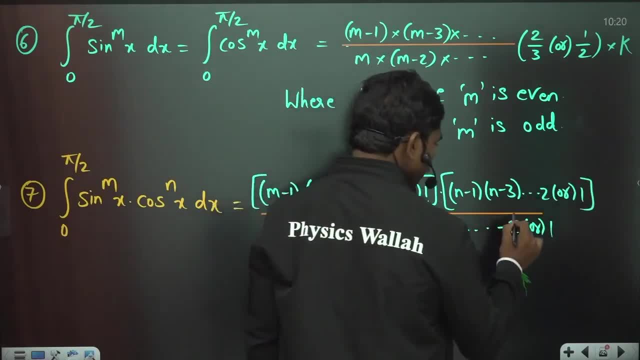 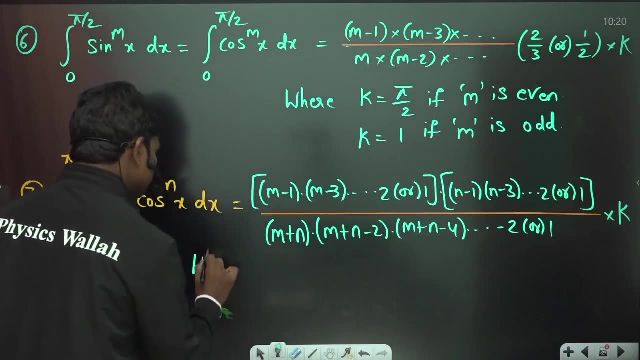 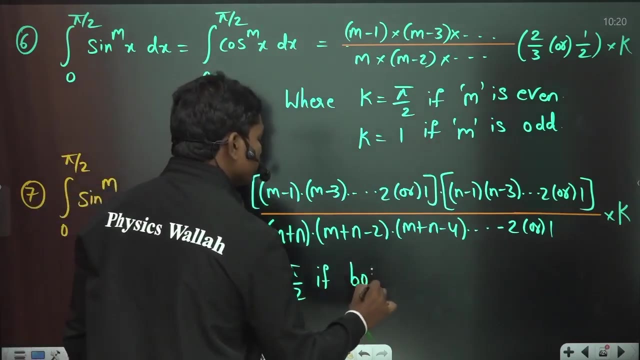 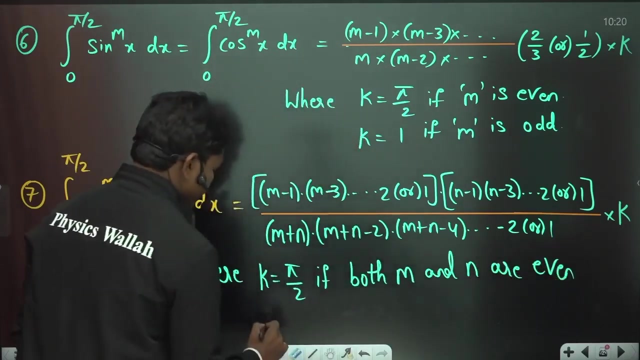 this whole value into k, into k. so where k is, where k is equal to pi by 2, if both m and n are even, if both m and n are even, similarly, if you see k is equal to 1, otherwise what is the meaning of otherwise? if m is even, n is odd, or if m is odd and 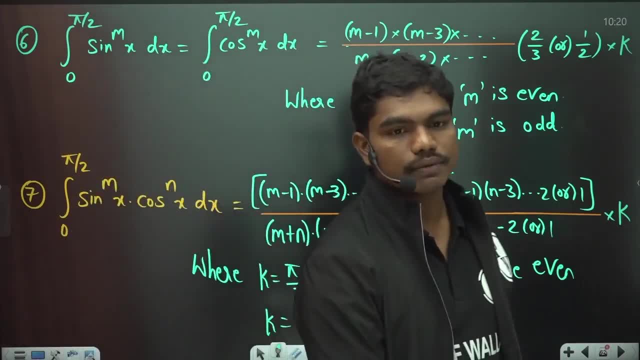 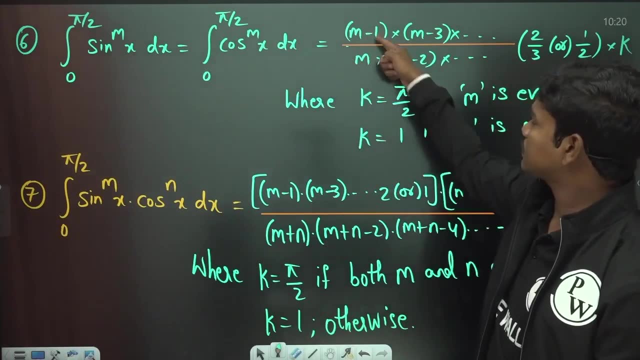 n is even or if both are odd. in those cases your k value is equal to 1. okay, but this is. these are very simple things to remember here. if you see m will, if there is m, you will start with m. then m minus 1, m is odd and n is even. so that means if you see k is equal to 1 or if you see k is equal to, 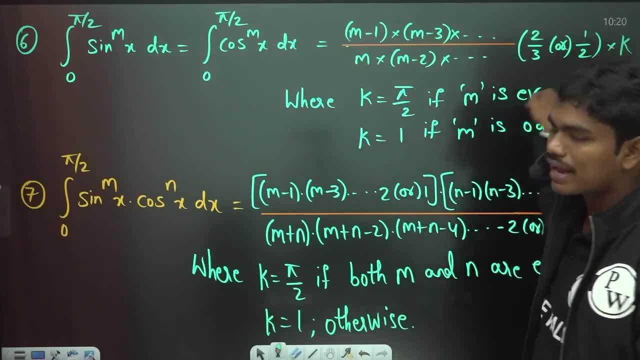 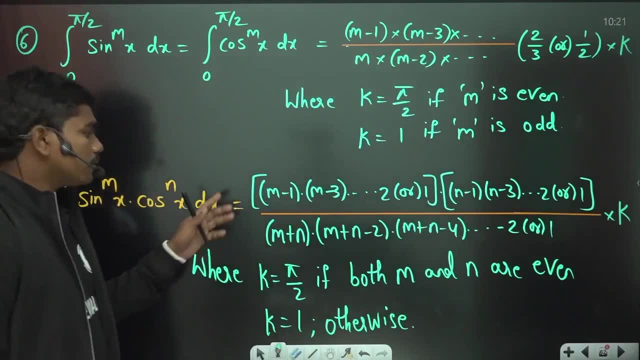 minus 2, m minus 3, this multiplication, you keep on going and, depending upon m being even or odd, you'll substitute pi by 2 or 1 respectively. similarly in this case also, if you see, if you identify what is m and n, then these values. writing this expression is also very, uh, you know, simple. 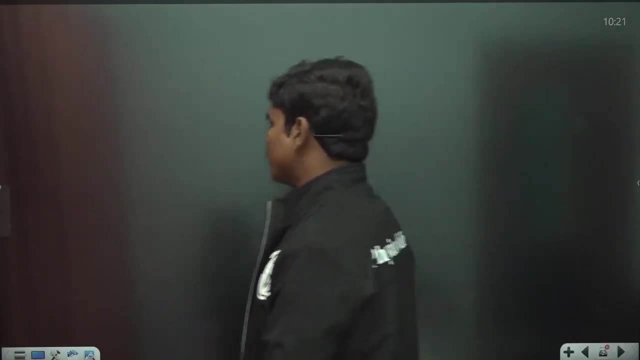 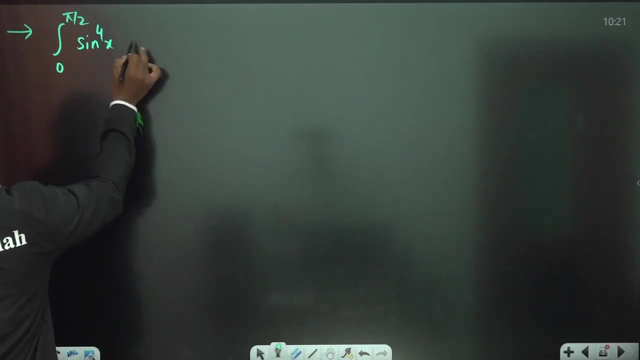 actually. okay, i'll give you one example, which is some common thing. so if you see, uh, for example, i'll give you one simple thing: 0 to pi by 2, sine square, x, dx, for example. okay, sine square is very simple, so let us take sine power 4x, okay, sine power 4x, dx, for example, okay, 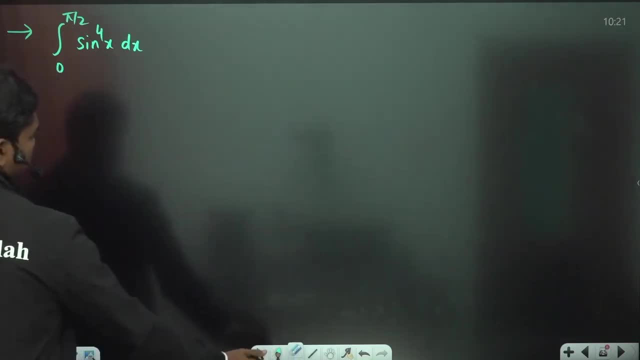 so sine power 4x. okay, uh, sine square will take simply- let us keep the thing simple, that's not my complicated sine square- x, dx, for example. so this can be recognized. if you want to integrate this, you know, 0 to pi by 2, 1 minus cos x, cos 2x divided by 2 dx. okay, so this is what you will get. 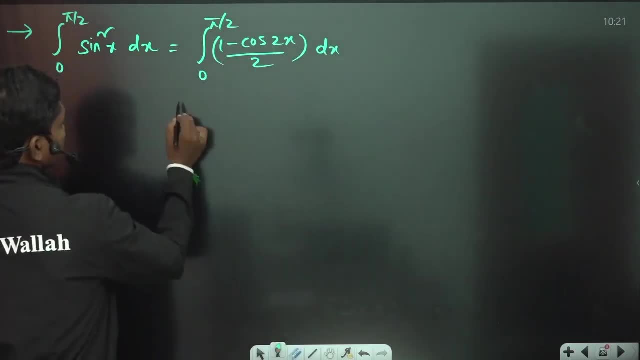 so 1 minus cos 2x is basically uh sine square x. so if you integrate this, 1 by 2 times of integration of 1 is x minus integration of cos 2x is sine 2x divided by 2. so within the limits 0 to pi by 2. so if you simplify this result 1 by 2 times of. 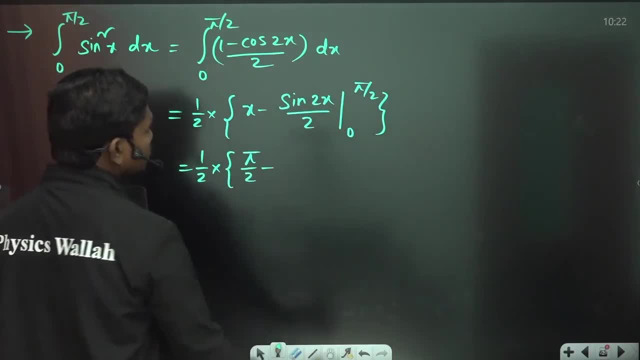 when you substitute x, pi by 2 minus when you substitute x is equal to pi by 2. here this is sine pi 0. so when you substitute 0, both are 0s, so this is pi by 4. this is the result which you. 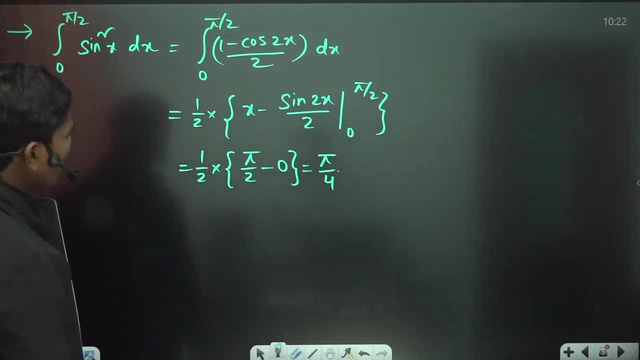 have, which is pi by 4 actually here. okay, so so the mass of the integration into x is basically 1 minus cos 2x. so integration of x is 1 by 2 plus a cos 2x. in fact that is 1 by 2, which is a sine 2x. so we are talking about 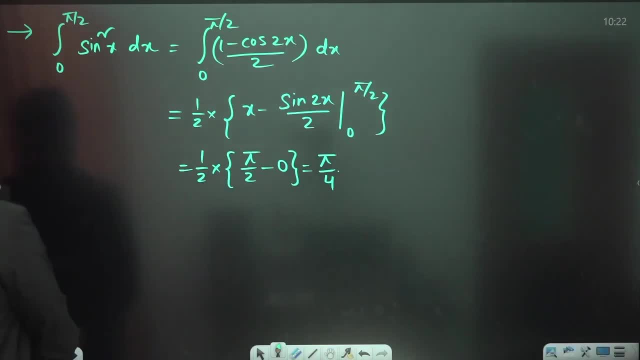 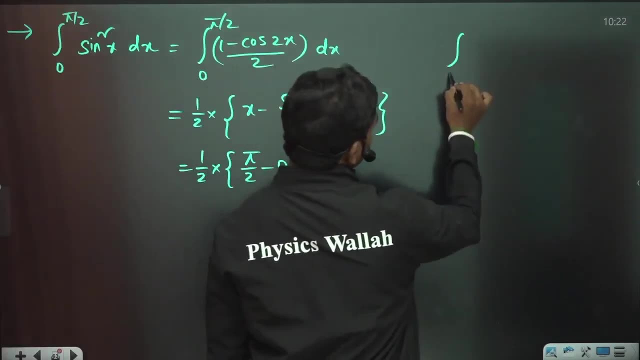 half into 1 minus cos 2x. so integration of cos 2x is sin 2x and it is 2, fine, so if you substitute from 0 to pi by 2, you have this pi by 4. good, now if you see, if you calculate. 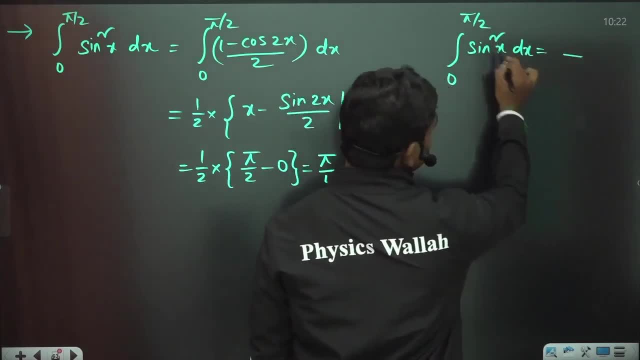 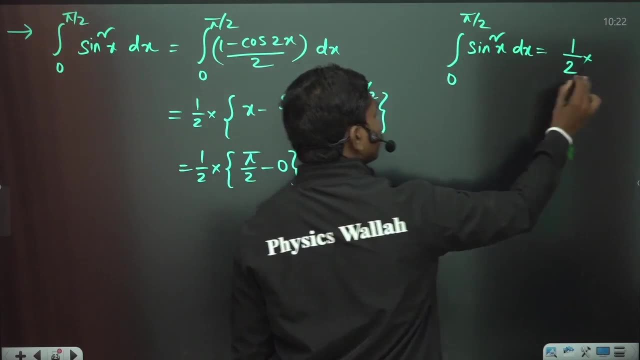 this result using. Look, you have two here, So M is two, So obviously one. that's it. No more numbers is into K, So here n is even. so K value is pi by 2.. That's it. So this is pi by 4 directly. 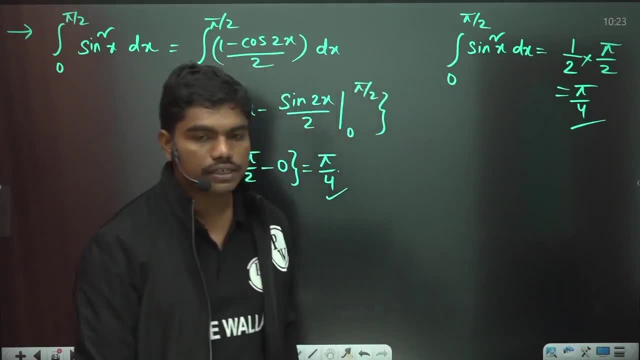 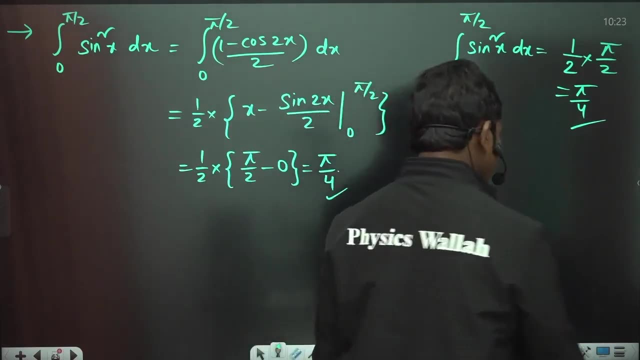 So this is pi by 4 and this result is also pi by 4, actually clear. So that's how you can apply This rule for calculating some powers of sine and cos combinations. Okay, and also I'd like to give one more example here. 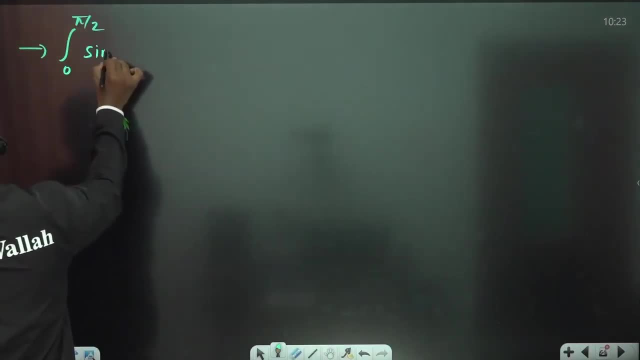 Integral 0 to pi by 2 sine square X Into cos square X DX. So let us suppose you have this integration, for example. okay, Now, if you have this integration, how will you Proceed? basically, you can write: there are multiple ways of doing this, actually, okay. 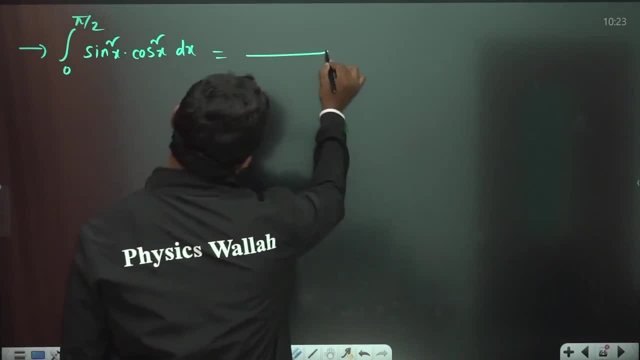 But if you simply apply this rule, you can see this: M plus n, M plus n is 4.. So 2, that's it, into 0.. You cannot write: this is 2, So M minus 1 is 1, that's it. See also: M minus 1 is 1. now both are even so. K value is pi by 2. 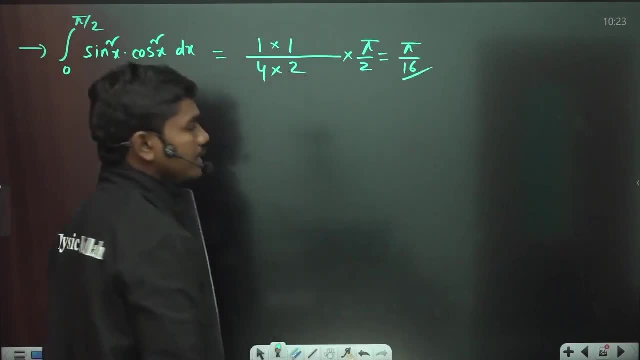 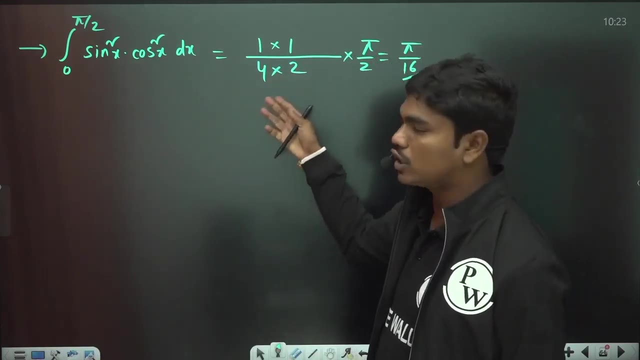 So if you see, If you simplify, pi by 16 is the correct answer for that integral, Okay, So pi by 16 is what you will get if you solve that integration clear. So M plus n value, then after 2, 2 difference means basically very alternate numbers unit right, since M is 1. 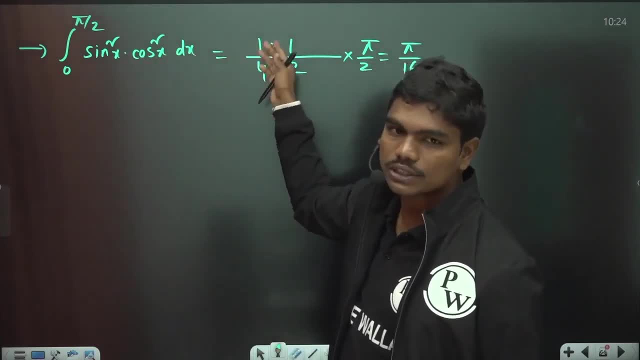 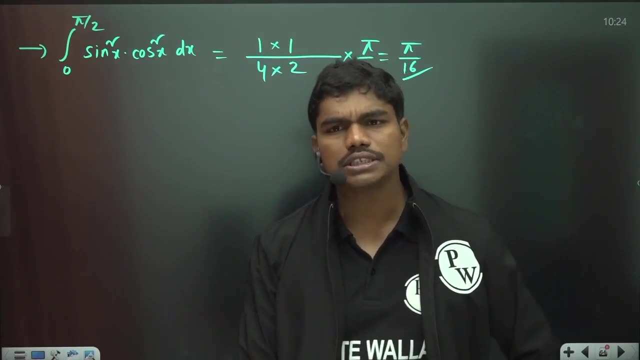 Sorry, Ms, 2 a minus 1 is 1 and you don't have any series to continue. So one is the cases for both this and you have that cases. Okay, now why this Integration is very much important for you. Okay, integration means basically adding up, summing up, and you have lot of applications. 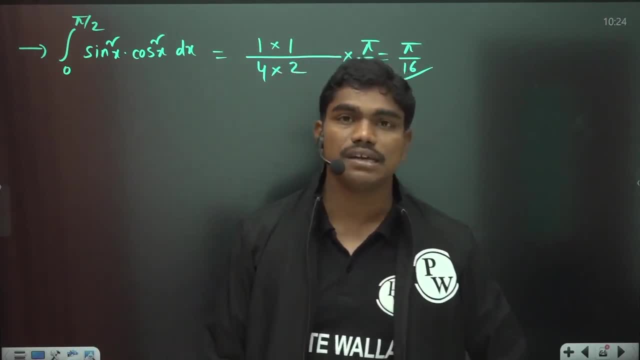 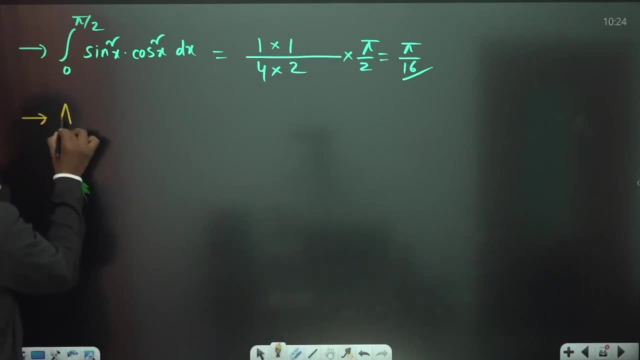 I buy example. if you see geometry applications, you can find the area between the curves. okay, so how we will find the area between the curves, see here. so let us write: area between curves, area between the curves, area between the curves. so how you'll calculate this area between the curves, basically, 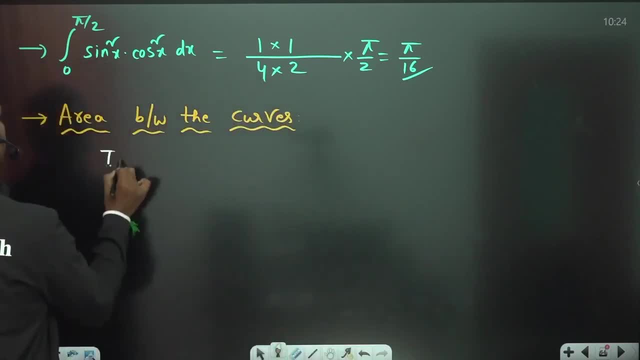 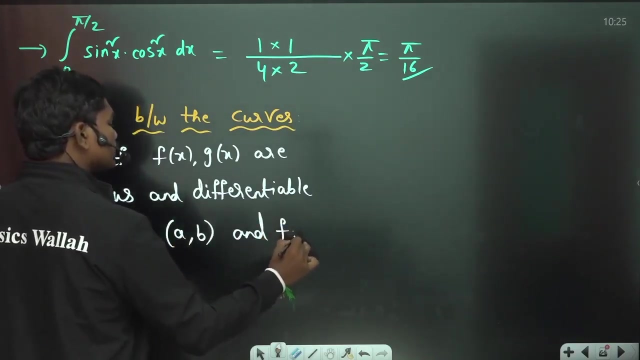 in a very normal way, that if f of x comma g of x are continuous and differentiable functions, continuous and differentiable functions, continuous and differentiable functions in a comma b, and let f of x greater than f of g of x, for example say, let us suppose if f of x is greater than g of x, so in that case, if f of x is greater than g of x, 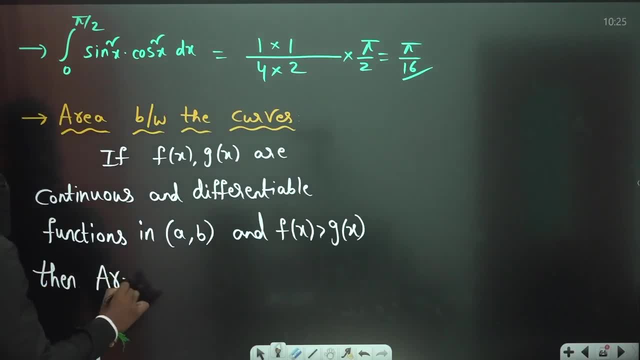 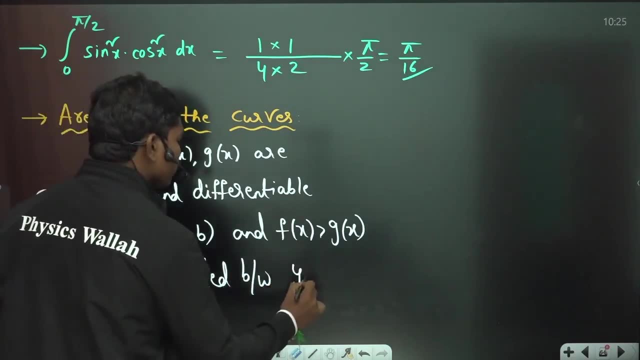 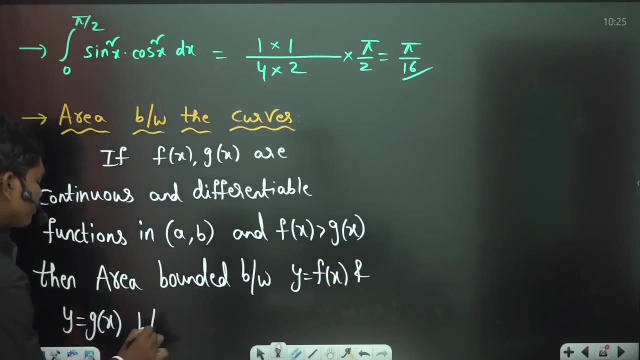 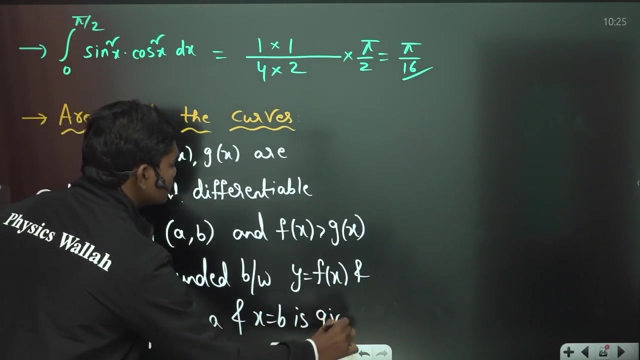 then, the area bounded between, area bounded between y equal to f of x and y equal to g of x and y is equal to g of x, between x is equal to a and x is equal to b, is given by these two areas. this is given by this result: a is equal to integral a to b. 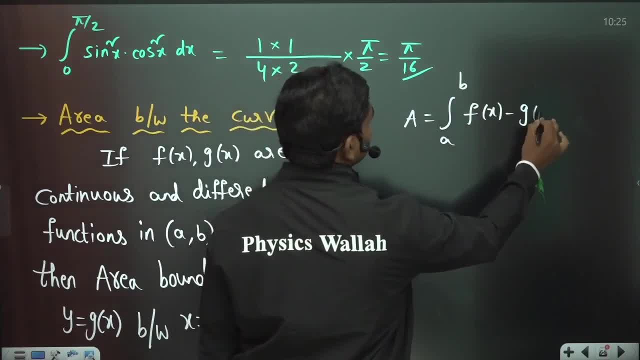 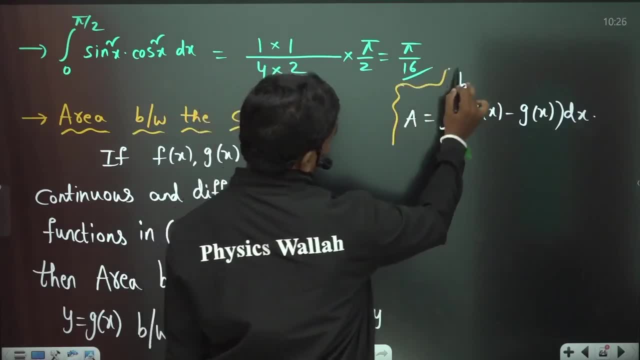 since f of x is more, you can write f of x minus g of x, dx. so this is the integration. so if f of x and g of x are given to you, then this f of x minus g of x will be some function of x and you can integrate that and how you will do this basically like this: 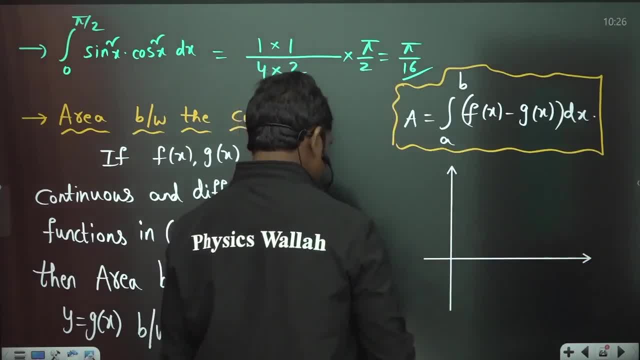 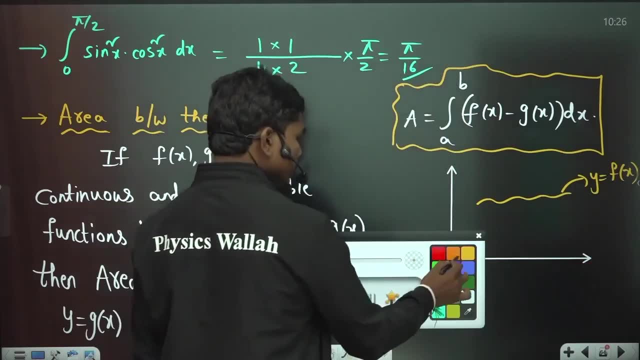 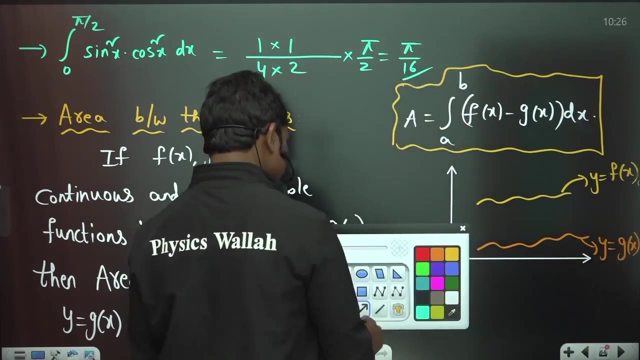 look, if you have some functions like this, then let us suppose this is: y is equal to f of x, y is equal to f of x. okay, and if you see, let us suppose this is y is equal to g of x, y is equal to g of x. okay, now, if you take this area, x is equal to a. 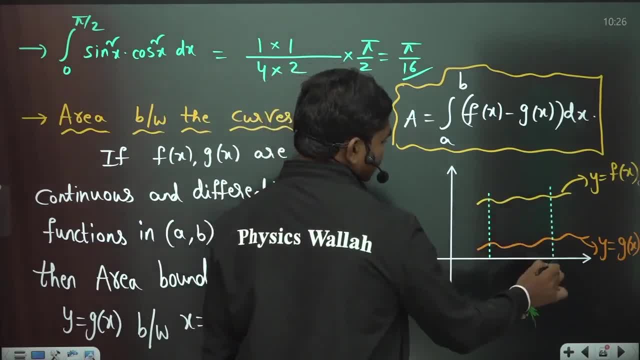 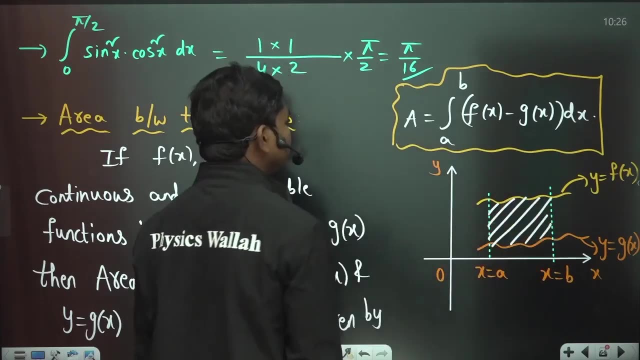 this is: x is equal to a, and let us suppose this is: x is equal to b, x is equal to a, x is equal to b. this is x axis, or is in y. now the a here is at this shaded part. so how do you know? this area is given by this equation because 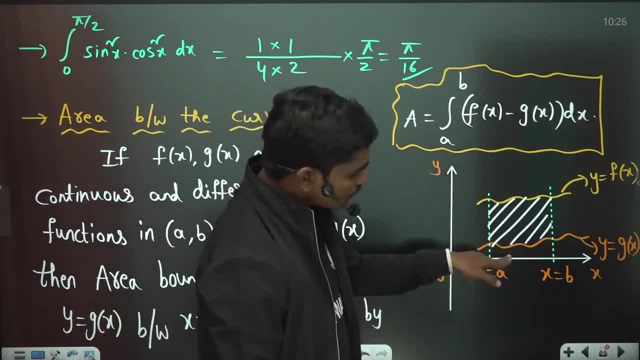 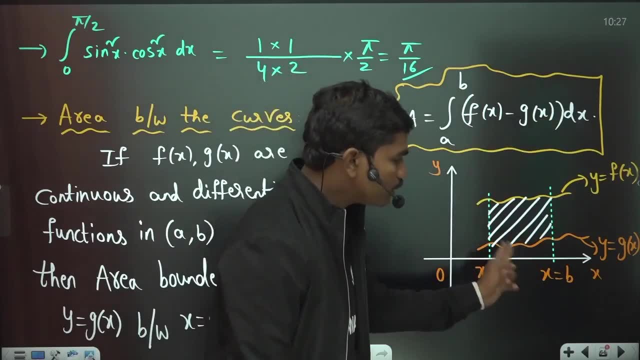 if you calculate integral here to be f of x, dx, you will get the total area, which is even below this orange curve, correct. and if you calculate integral here to be g of x, dx, you will get this area below the orange curve. so if you take the difference to get this area, this total area minus. 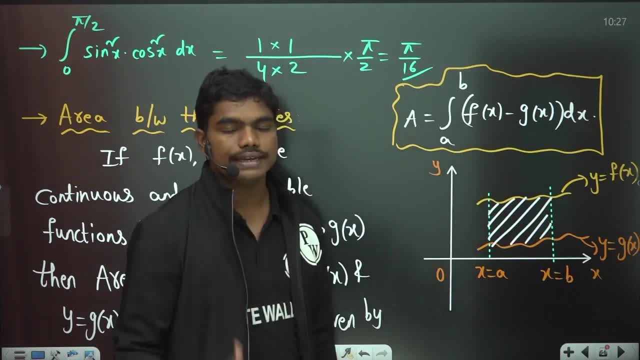 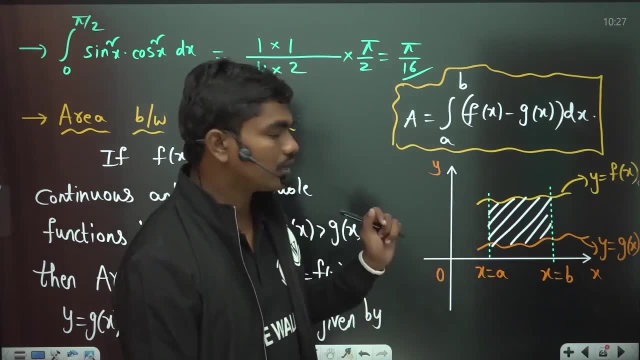 this area which is below the orange will actually give you the area which is bounded. so that is actually f of x minus g of x. but one very important question here is this: f of x should be definitely more than this g of x function okay, otherwise your result goes wrong actually. so your f of x. 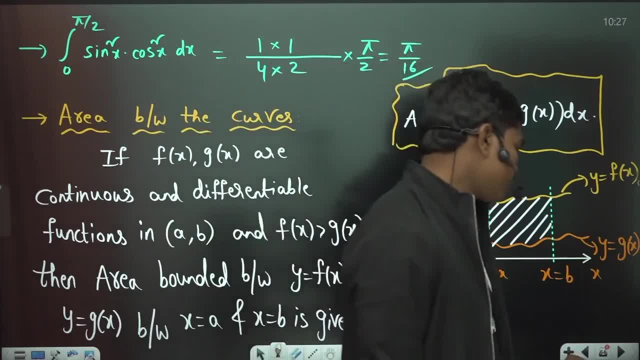 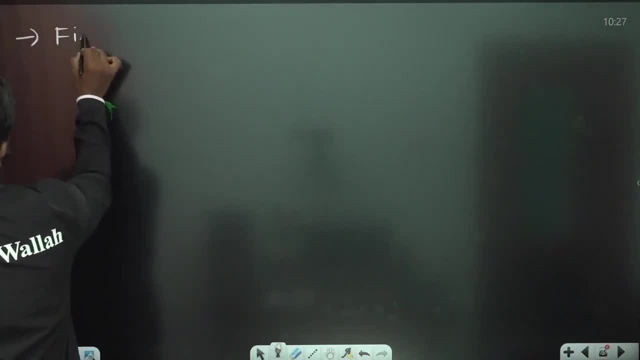 function should be definitely more than your g of x function. okay, so this is one very important thing. because, why this is important? i will give you the help of an example. if you, if i ask you to calculate, find the area between, find the area between the curves. 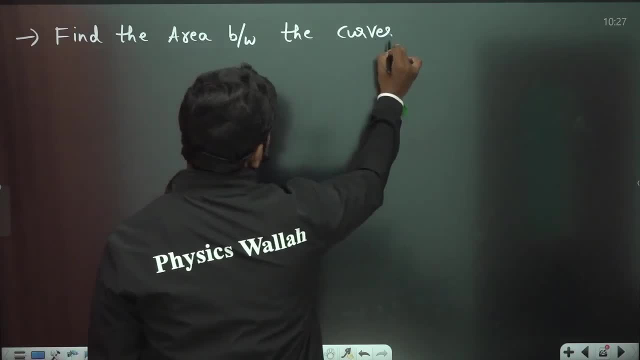 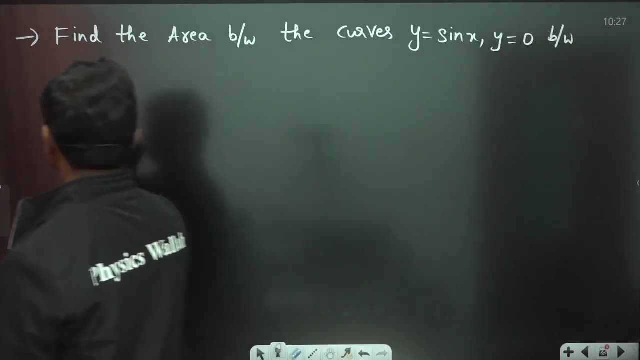 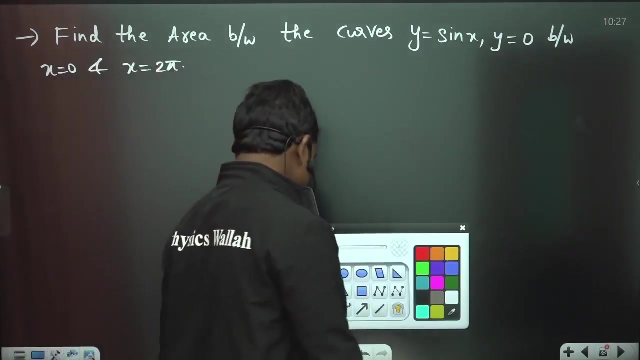 the curves, y is equal to sine x, y equal to 0, between x equal to 0 and x is equal to 2 pi. let us suppose if i write this, okay, let us suppose if i write this, then if you plot these curves means basically, if i give you this: uh, sine x minus 0, you generally feel that sine x is. 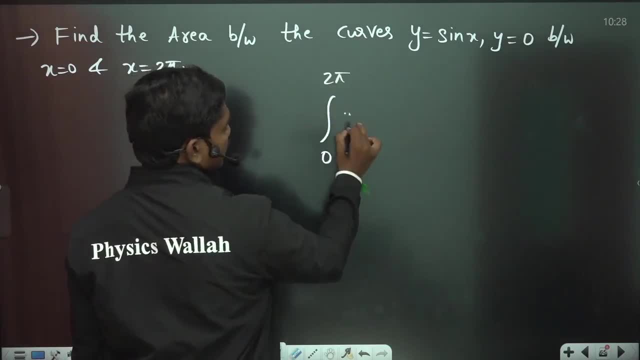 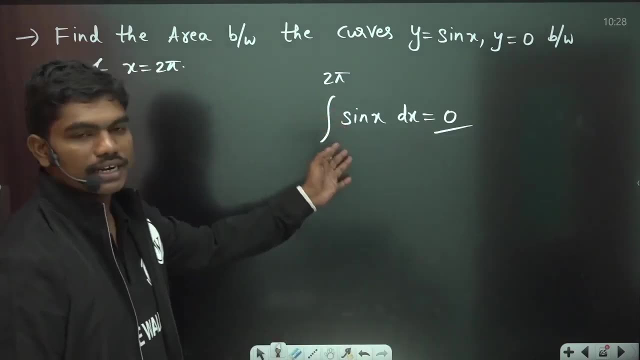 more. so if you do this integration 0 to 2 pi, sine x minus 0, which means sine x dx, you will end up with 0. okay, this answer is 0 because the integration is minus cos x, cos 2 pi and cos 0. both are same. so 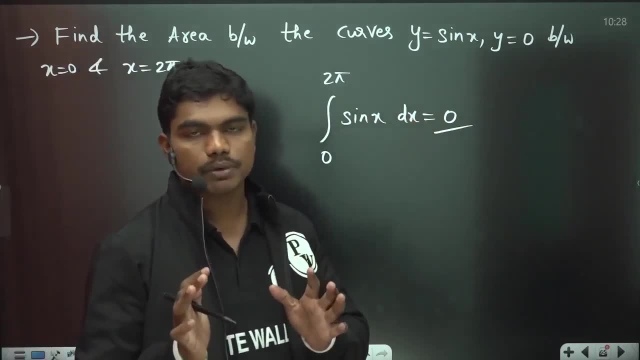 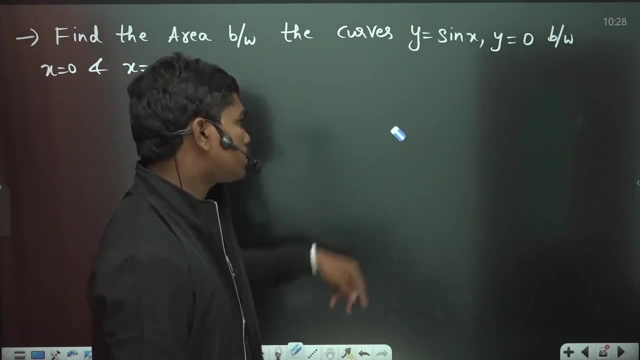 the answer is 0, but actually speaking, there is some area which is bounded between sine x and 0. actually, that you will come to know if you draw the graphs. that's the reason why i've given you graphs in the beginning, so let us try to draw now. so if you see, if you try to draw the graph, 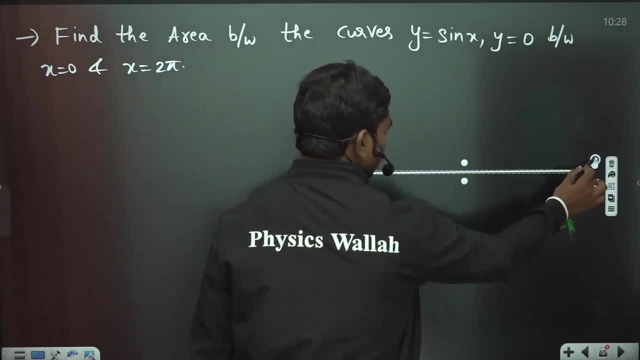 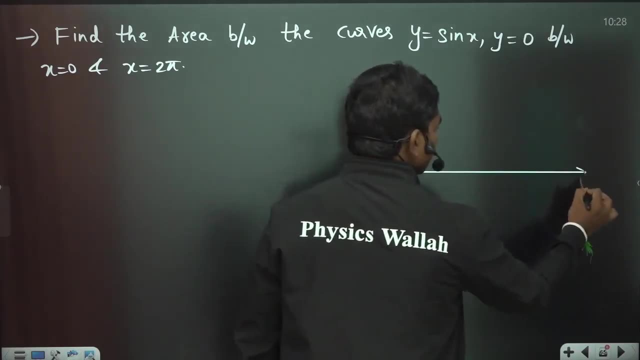 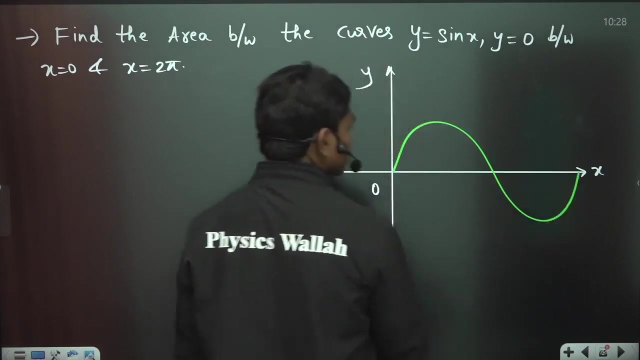 this is, you know, x axis, this is x axis. then this is your y axis: horizon x, y, so sine x. so if you take the graph of sine x, like this something, for example: and let us suppose this value is 2, pi and this value is pi, now the area bounded is actually this complete area. this complete area, correct, is the area. 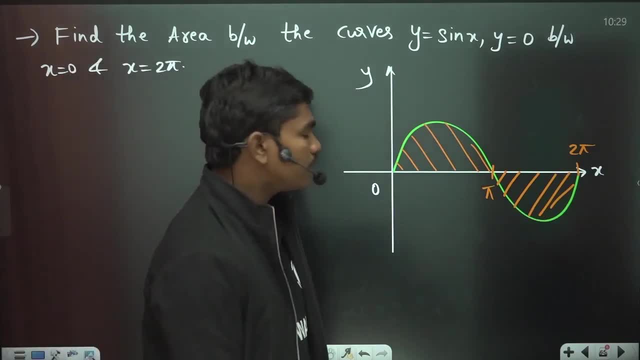 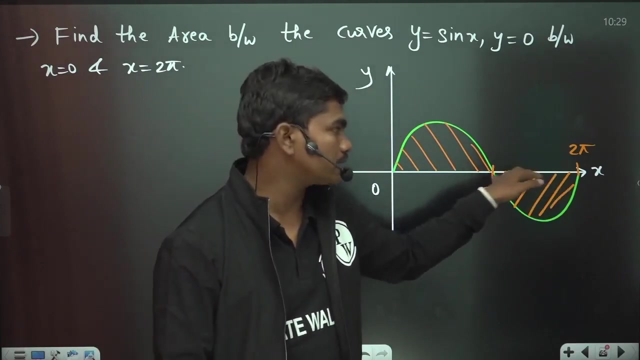 but why you are getting zero answer? because you have completed one mistake: that from 0 to pi, sine x is on the top and x axis is on the bottom. so sine x minus 0 is good, but sorry, excuse me so, but from pi to 2 pi, if you see sine x is on the bottom and x equal to, i mean this y axis, sorry, y equal to. 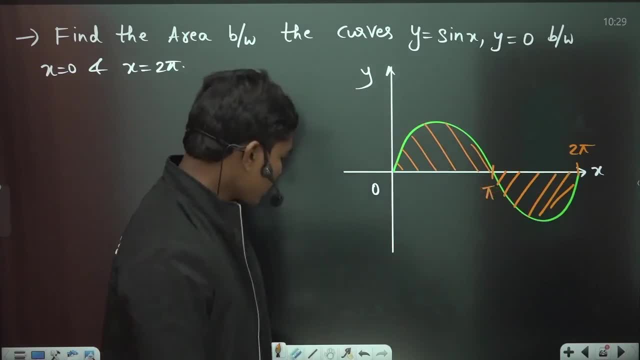 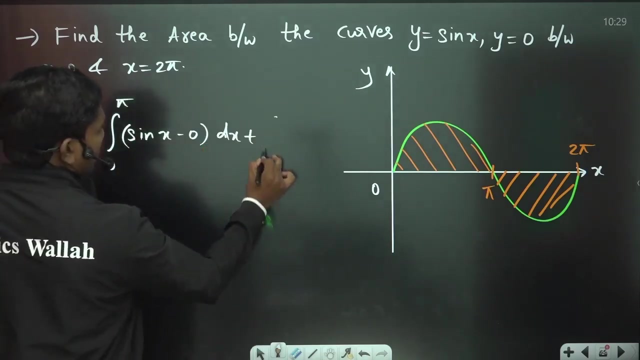 0 means basically this x axis is on the top. so if you want to calculate this area, i told you first f of x should be always above g of x. so if you want this area you should do integral 0 to pi, sine x minus 0, because sine x is on the top, plus pi to 2 pi. you know, 0 minus sine x because 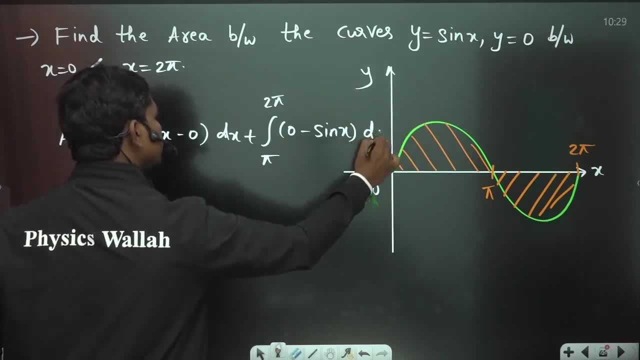 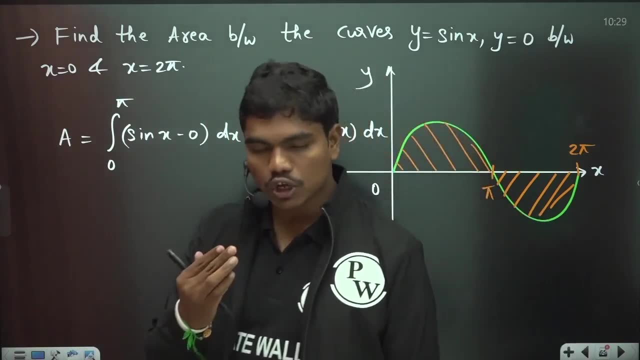 x equal to means x axis is on the top. so that's why this is the integration you need to do, because after x is equal to pi or x equal to pi, the curves are intersecting and the curve which is on the top till then is going bottom okay. so that's why you need to split the curves at any point where they. 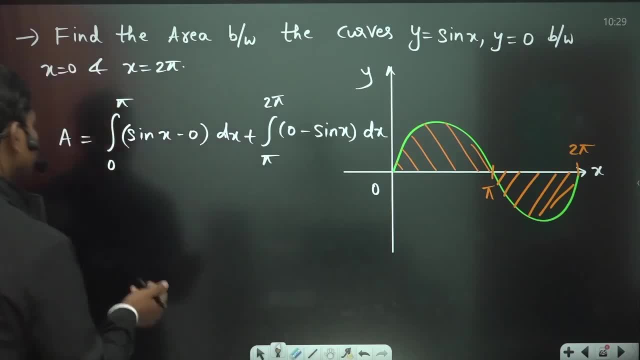 actually cut each other. you need to check carefully and you need to do this integration. so if you do this integration now, minus cos x 0 to pi plus integration of minus sine x is cos x from pi to 2 pi. so if you substitute minus cos pi is minus 1, minus cos 0 is 1 plus cos 2 pi is 1 minus cos pi. 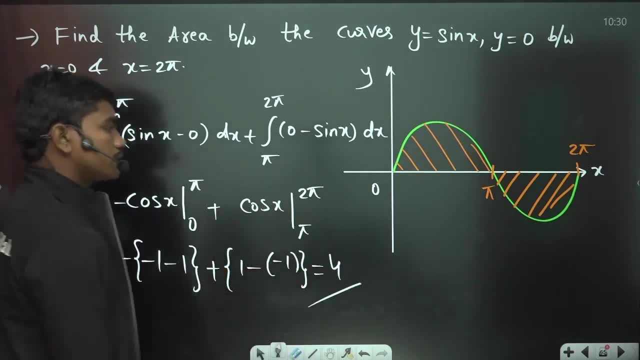 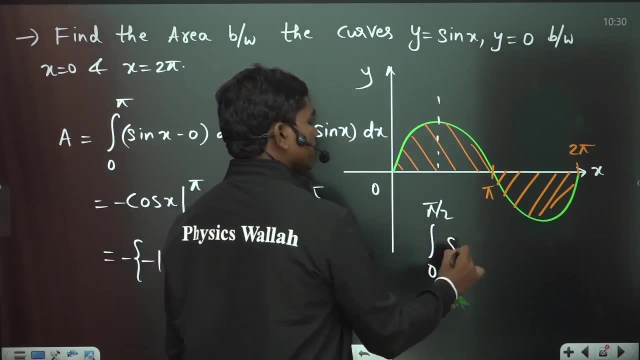 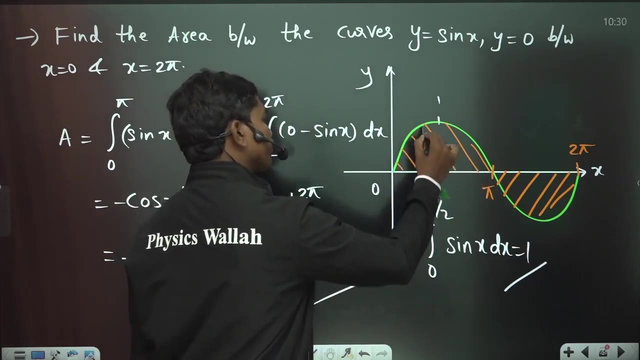 is minus 1, so total value is 4, actually, okay. so basically, you have seen, if you take only till this part integral 0 to pi by 2 sine x, this value is actually 1, okay, so that's why this total area is 4 times of this part. so that's why 4 times of 1 is 4, is what you. 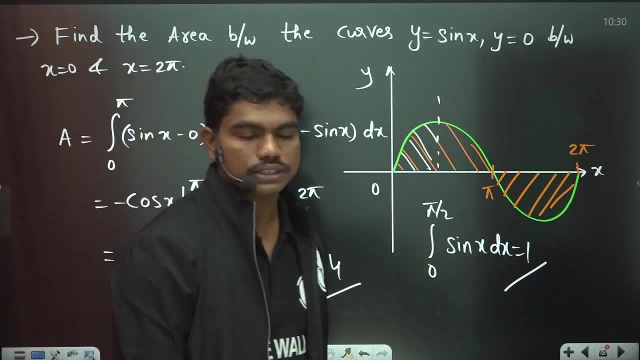 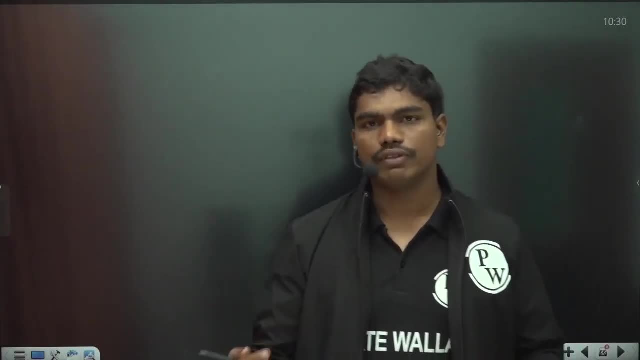 will get actually here. okay, so this is how you get this equation. similarly, if you are calculating length of a curve, let us suppose if you have some length of the curve, if you have a curve which is of some not proper geometry, okay, let us suppose if i give you a line segment and if i ask you what is. 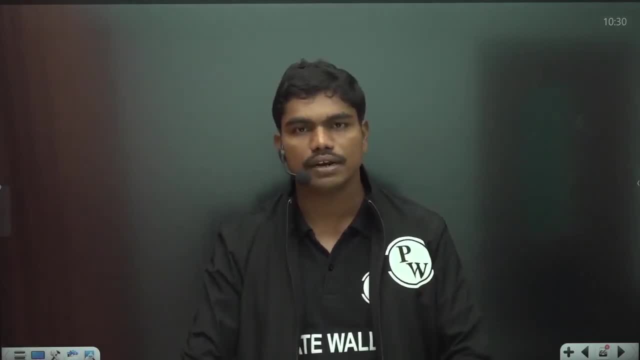 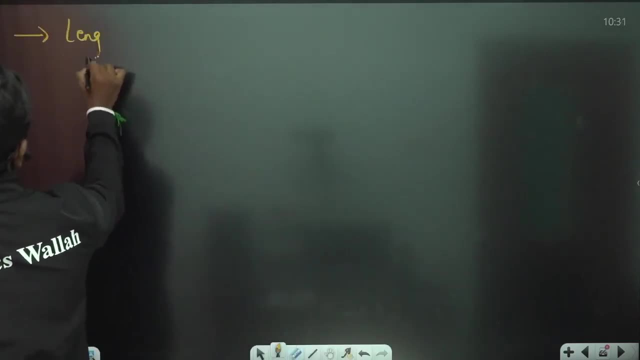 the length. you can easily tell me like. you will put a scale and you will tell me: okay. so but let us suppose if i give you some random curve like this length of a curve, if you see, let us suppose if i give you some random curve like this, 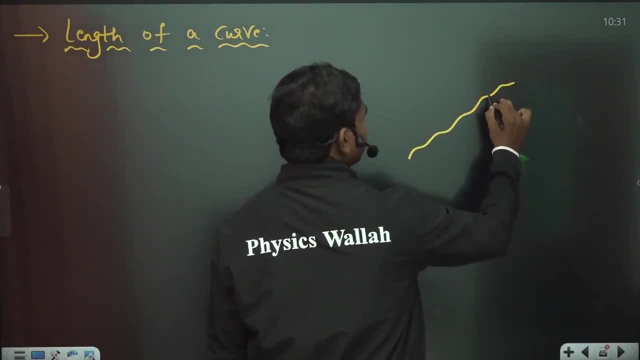 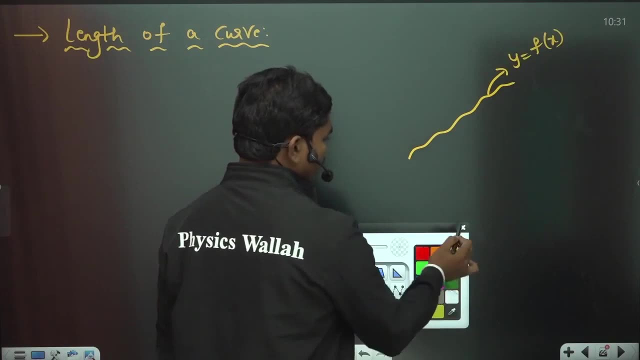 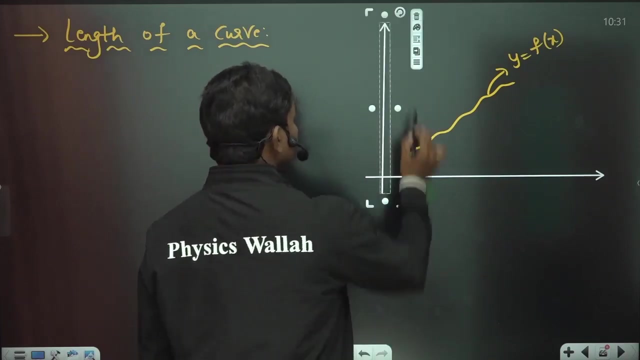 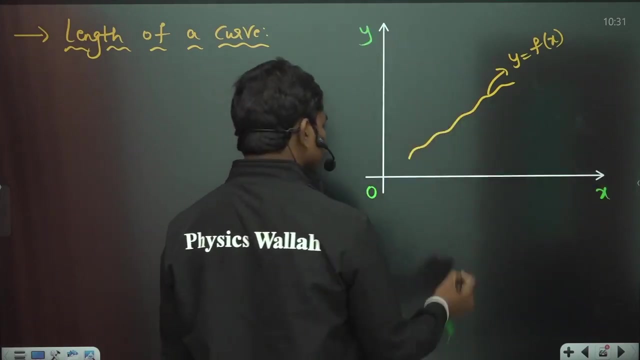 no, this is straight line. so some random curve: y is equal to f of x. so what is the length of this curve from to? let us suppose if i establish a coordinate system, so if you see, i have established some coordinate system. so this is horizon x, y. so let us suppose this is: x is equal to a. 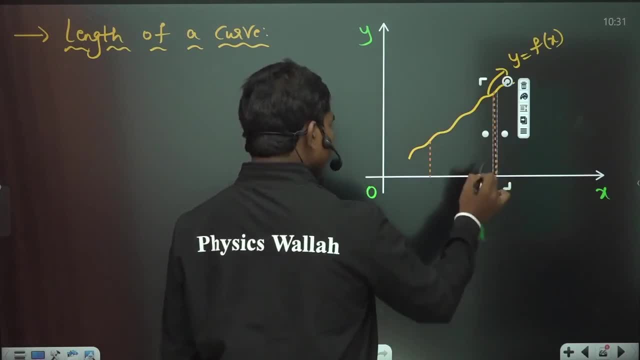 this is x is equal to a and this is x is equal to b. now my a. so this is x is equal to a and this is x is equal to b. now my job is to calculate the length of the curve from this point to this point. let us say okay, mathematically, of course, physically, if you. 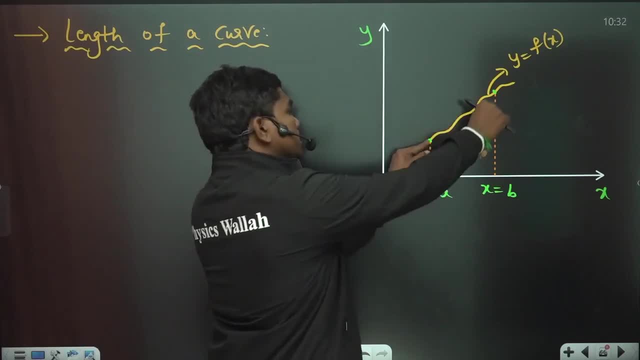 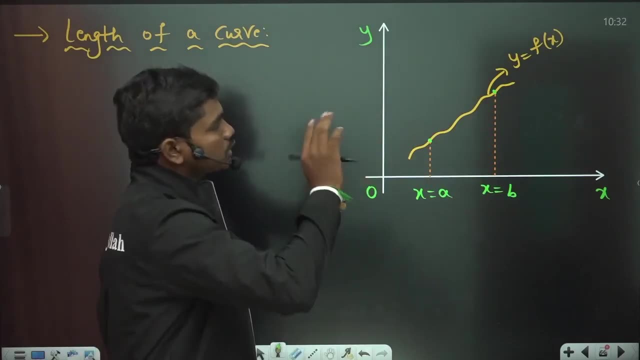 want to measure. how do you measure? you take a third, keep the third along this curve, then take the third, make it straight, put it on a scale. you will get the length. okay, but mathematically, how do you calculate this? look, and the equation of the curve is given, but it's not a very regular 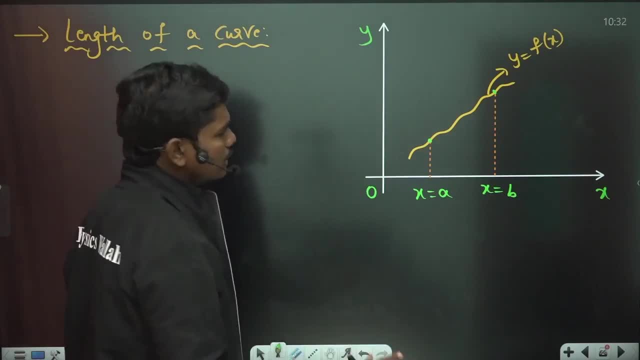 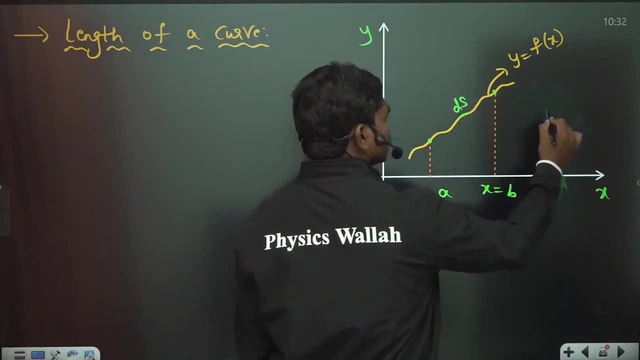 geometry. so in such cases, how you do, how you do is like this way: so look, what we'll do is we'll take some small length ds, okay, so we'll take some small length ds and this small length ds, which is like this, you project it onto this coordinate system. so this is dy and this is dx. so whenever ds is very 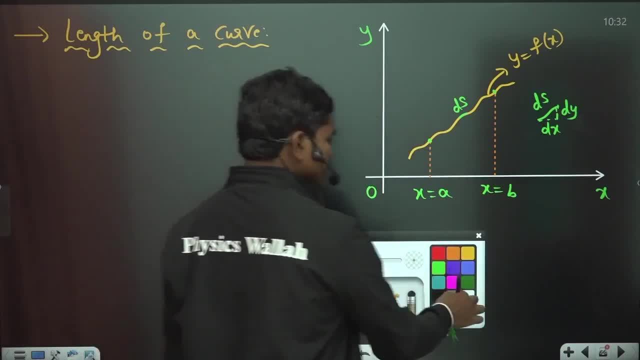 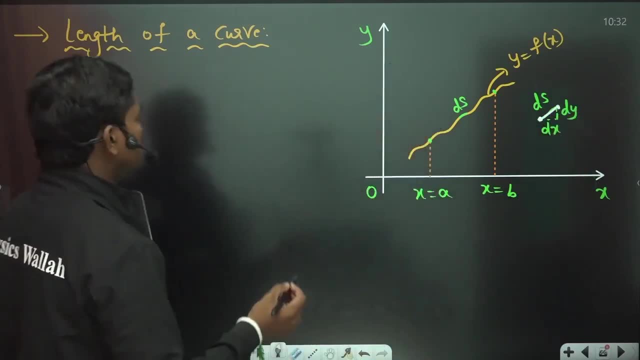 small, you can make sure you can assume that this curve is actually straight line. okay, when these points are very close, you can. you can see the line and the curve almost they look same. so ds square will be equal to dx whole square plus dy whole square. pythagoras them, if you apply pythagoras. 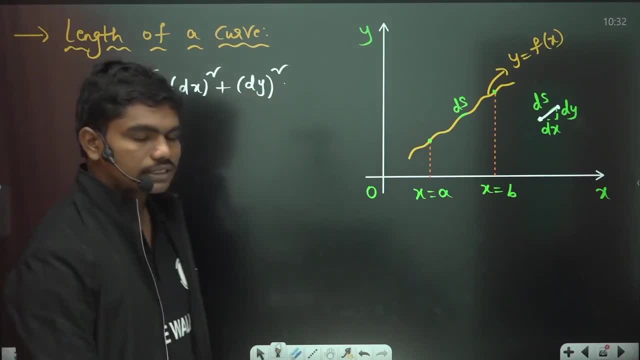 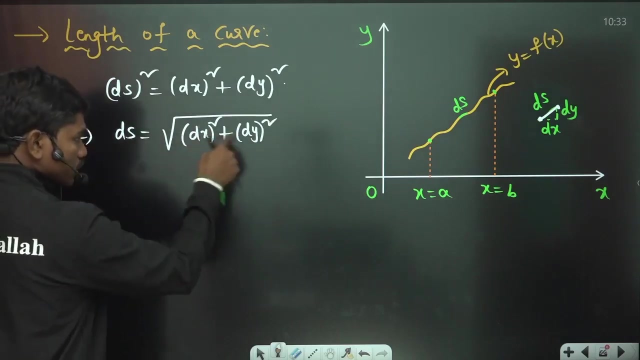 them for the right angle triangle, you will get this: ds whole square is equal to dx square plus square. okay, now, if you see, ds is equal to square root of dx whole square plus dy whole square. so here, if you take this dx whole square out, you will get the result like this: ds is equal to root. 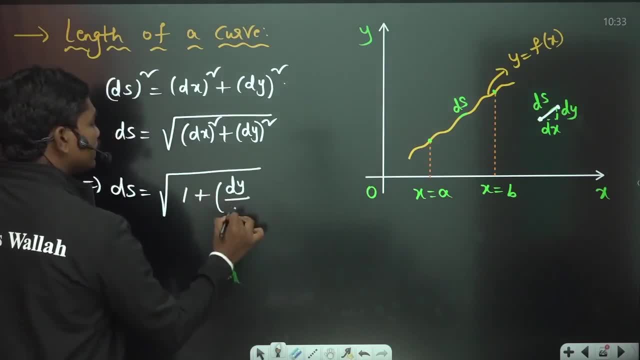 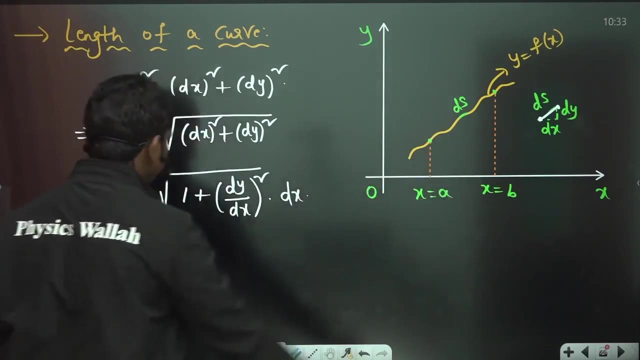 of 1 plus dy by dx, whole square into dx. actually like this, okay. so root of 1 plus dy by dx, whole square dx. so this is the length of the small element. so if you want the total length, here dx is the integrating variable, so you need to integrate from a to b, say. therefore total length. 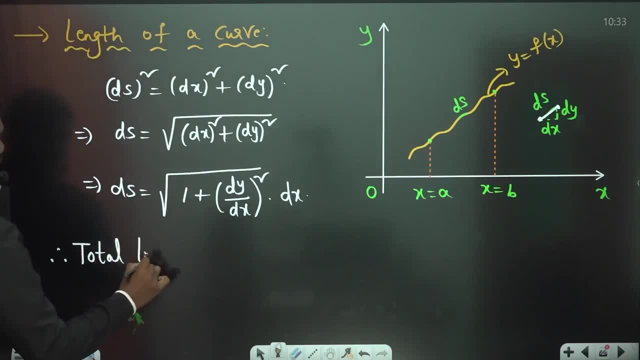 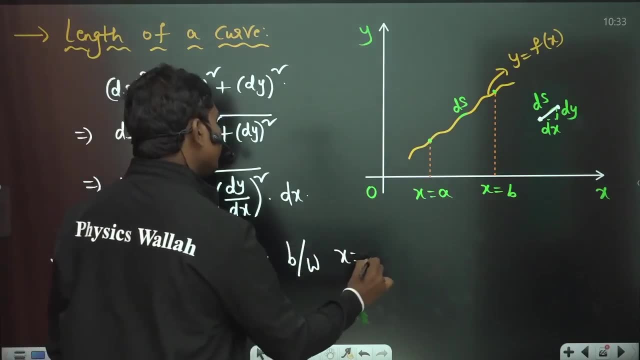 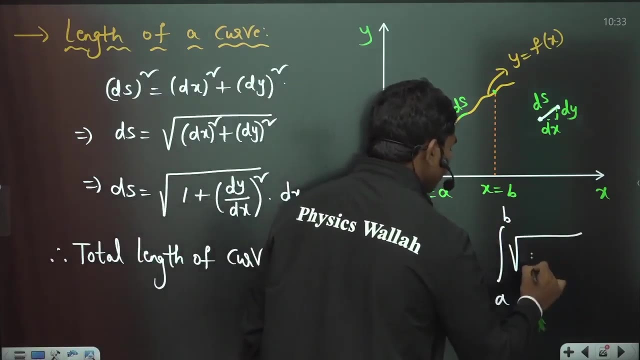 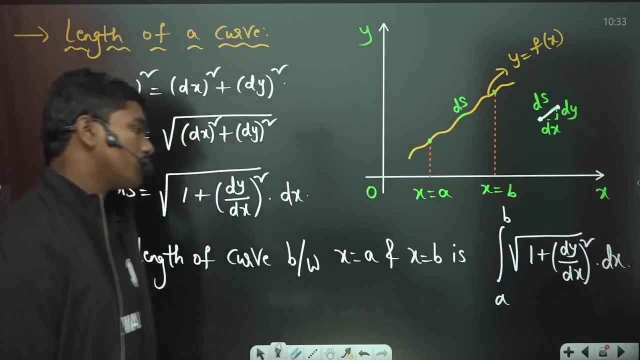 of the curve, total length of curve. total length of curve between x is equal to a and x is equal to b. is integral a to b. root of 1 plus dy by dx, whole square into dx. okay, so this is what you'll have: root of 1 plus dy by dx, whole square. 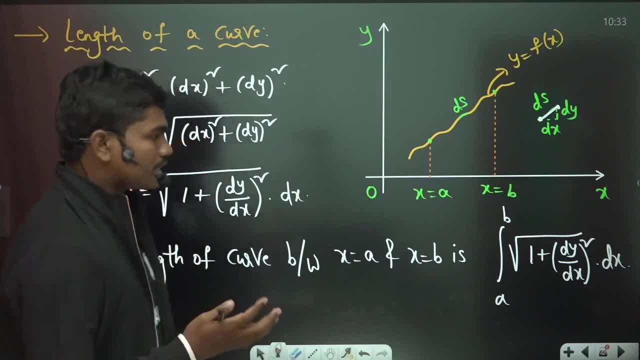 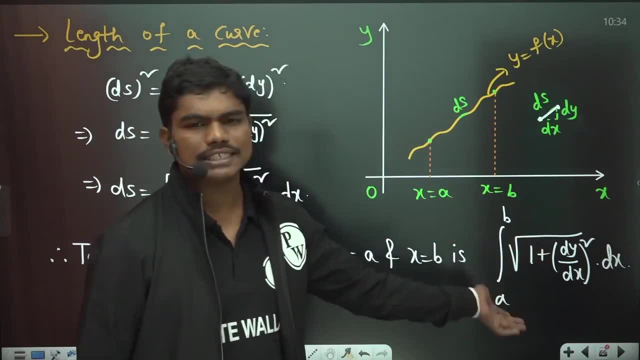 into dx. so it's a simple Pythagorean theorem: some two, three steps. if you apply, you will get that okay. so, and once, if they give you the variation of y with respect to x, you will get dy by dx. so you can solve this integral. okay, to get the length of the curve actually okay. now let us see. 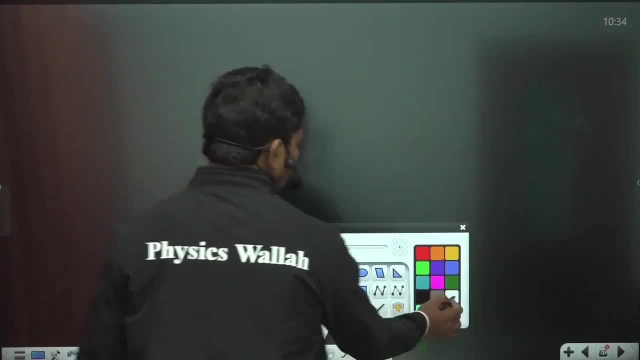 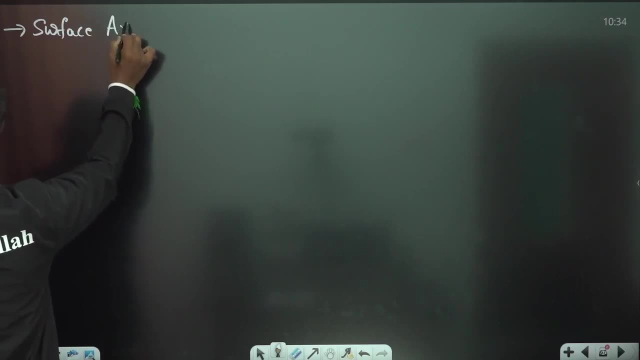 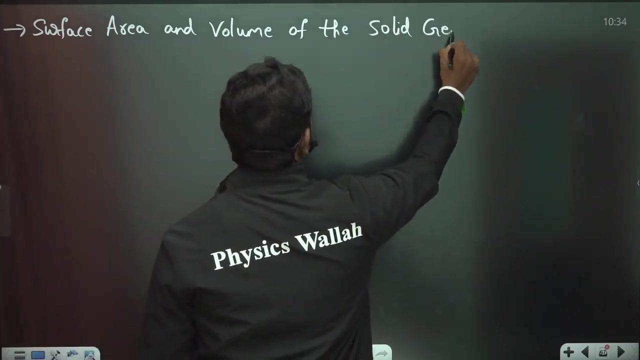 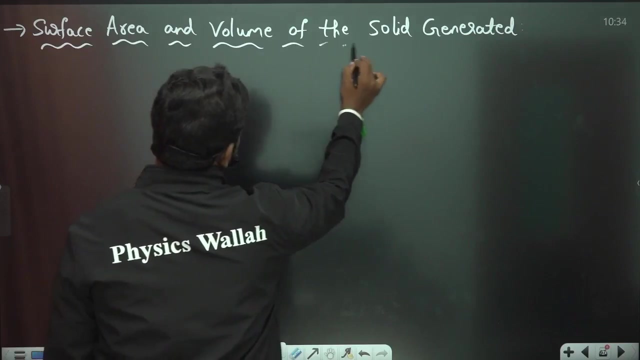 let us try to understand one thing: areas, or you can say surface areas, and the volumes of the solids generated. surface areas, surface area and volume of the solid generated. you can again calculate this using some simple integration techniques: surface area and volume of the solid generated. look where you will get a solid. look, let us 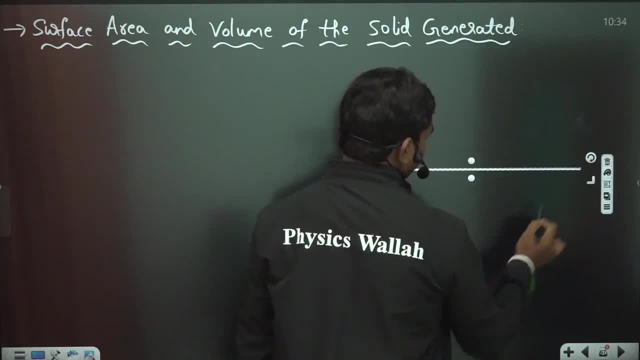 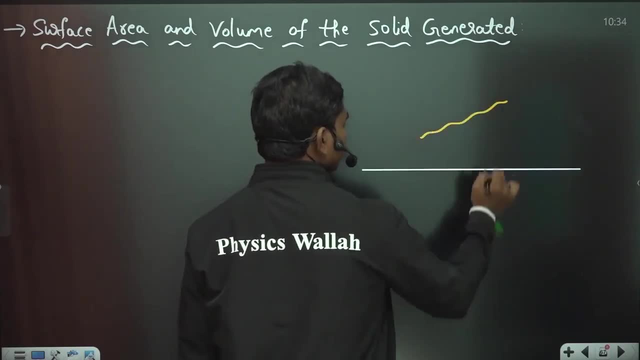 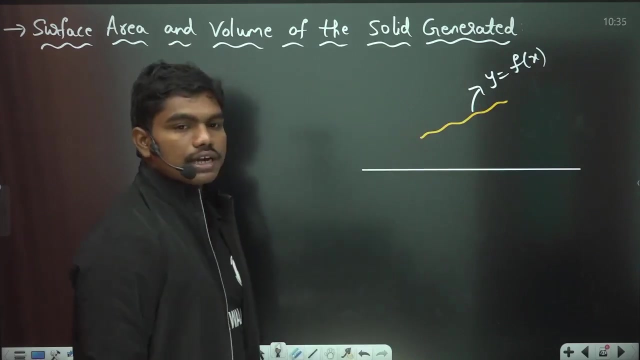 suppose if you draw a line, for example. now let us suppose you have some random curve, for example some random curve, Y is equal to f of x. this curve equation is: y is equal to F- X. now let us suppose if you are evolving this curve about this axis, then definitely you'll get the solid. 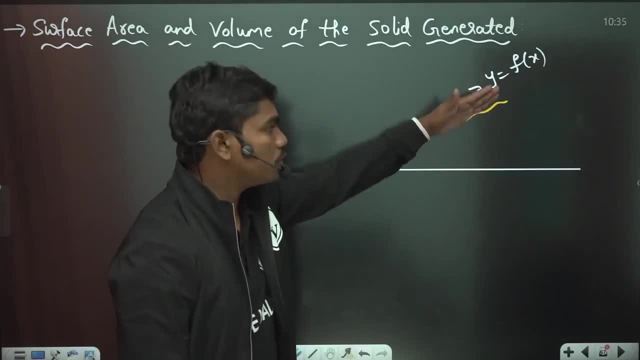 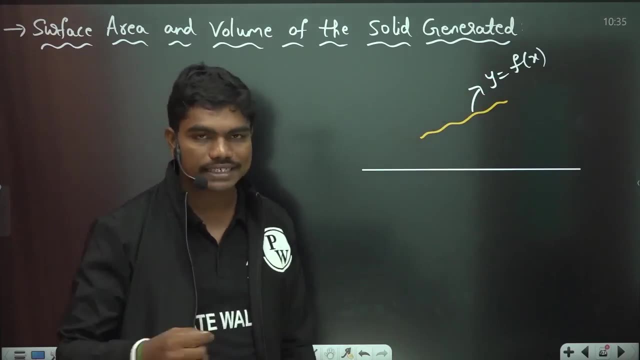 depending on this curve, you will get some solid. if it's a straight line, you will get some first team of a cone. if it's a horizontal line, you will get a cylinder. depending on this curve, you will get some different solid. now, once that's all it gets generated, the solid will have certain volume and also the solid will have certain surface area. so how is that going to work? 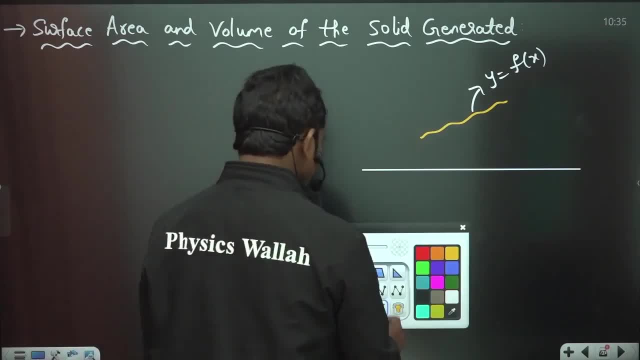 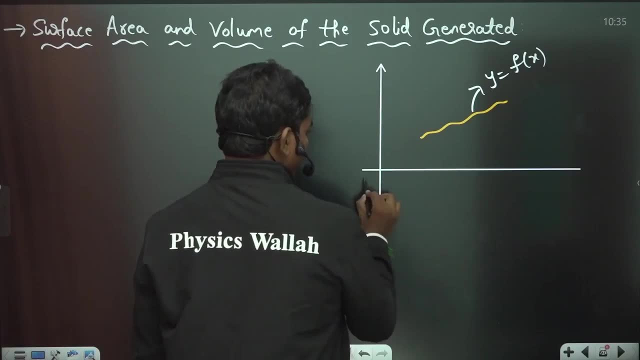 by the way, you don't have to Dollبيhuss, pero sorry, sorry, you areates me. help your solid find any minute this 이거. the identity will have certain volume and also the solid will have certain surface area layer. So how do we calculate that? look So again, if you assume this as your y axis, 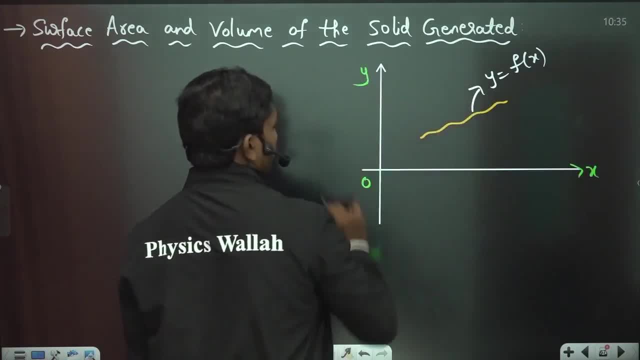 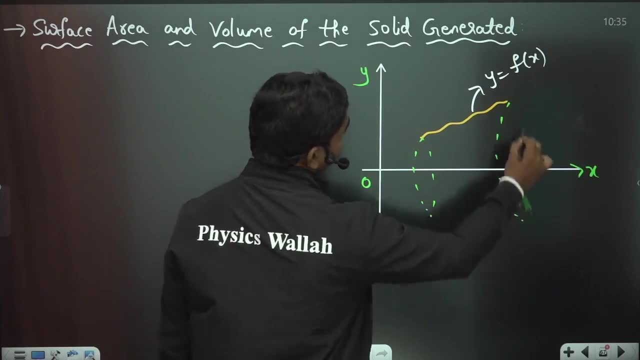 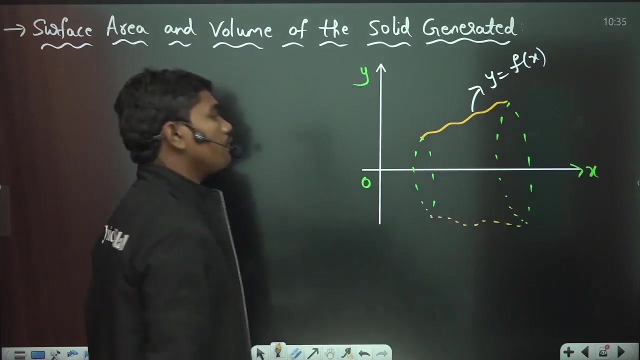 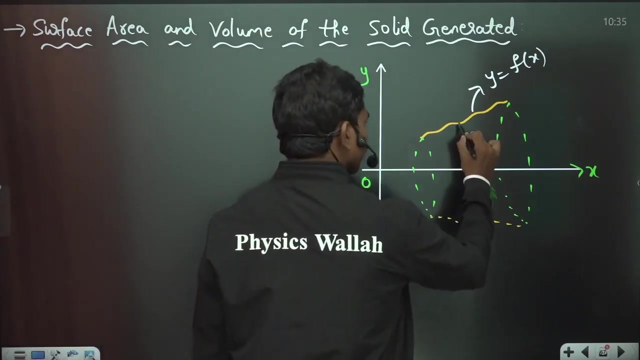 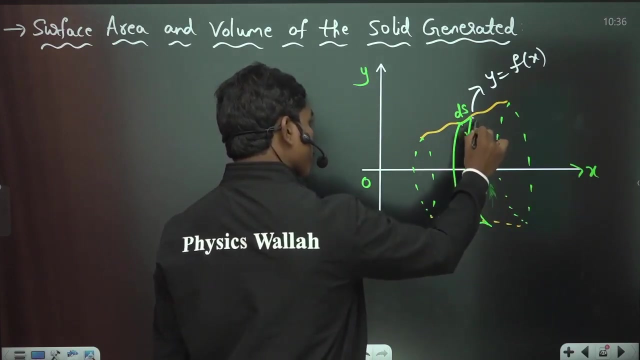 or isn't x, y? Now, if you evolve this, it comes out something like this: So this is how you'll get a solid cut. Now, what is the surface area of this solid Look? let us suppose, if you take a small section ds, small length ds here, then definitely. 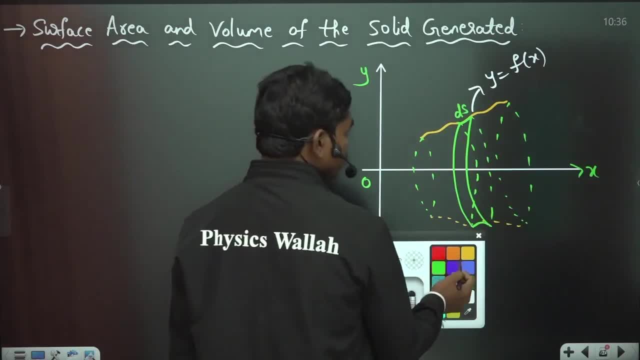 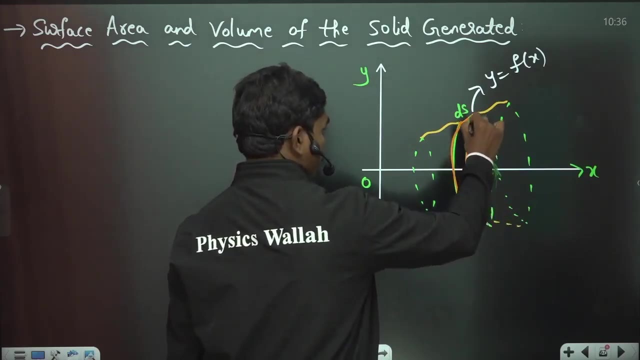 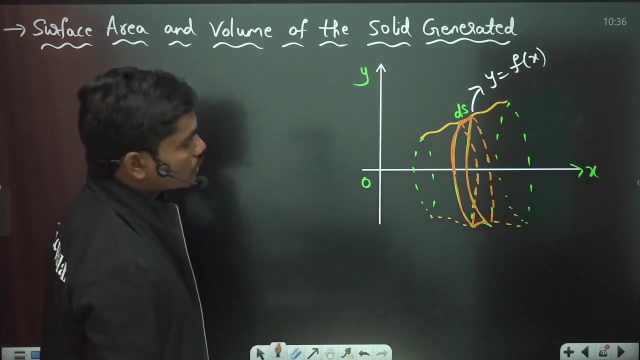 if you see, this is how we have the curve cut. I'm highlighting this with some different color So you can see. So this is small disk that you will get by evolving the small element of length, ds. Now, if you want the surface area, then you can see. surface area is basically this. 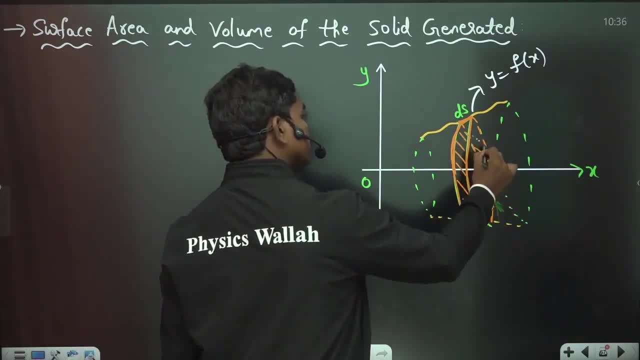 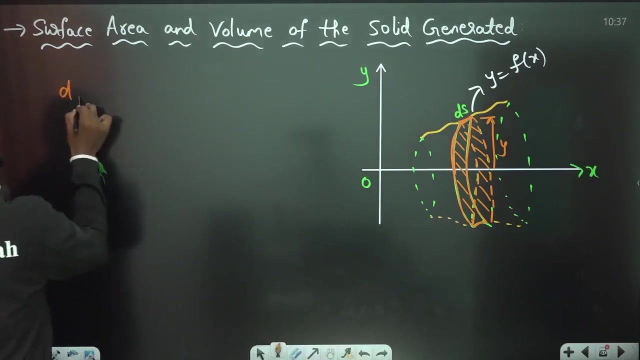 So, And this is the surface area of the small disk. So what could we do? surface area. Let us suppose at this location the height from this base is y, So surface area of that ds is equal to a surface area dA. 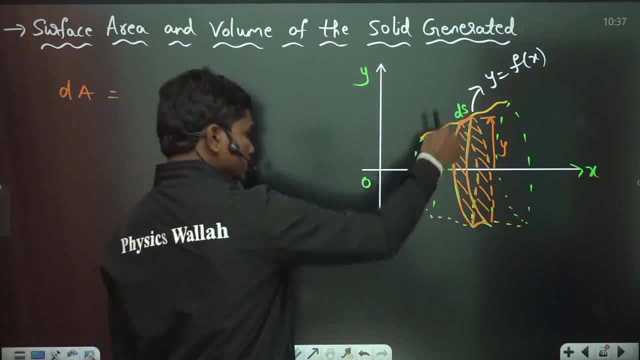 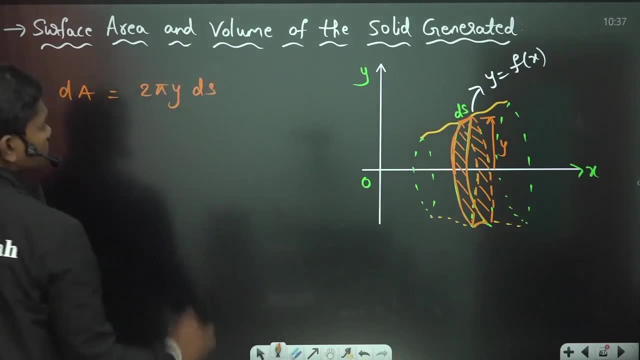 Basically a small surface area is equal to this circumference. into this thickness ds gives cat Ok. So 2 pi y into dsCK, so 2 pi y into ds gives the surface area right because It's the same surface area as ds dry. So you 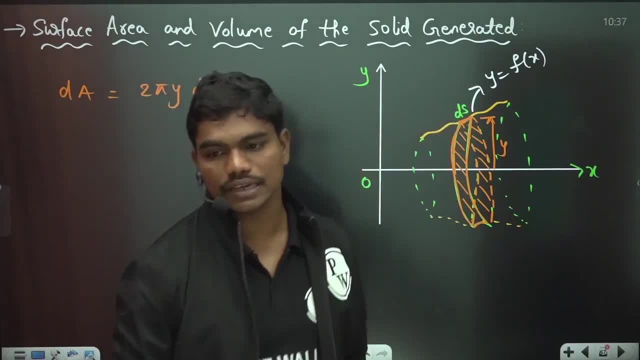 can achieve a range of ds here in 30 seconds. right, correct, Alright, it's almost the right. It's like a disc, for example. okay, So if you take, for example, this is like a small disc that is coming here. 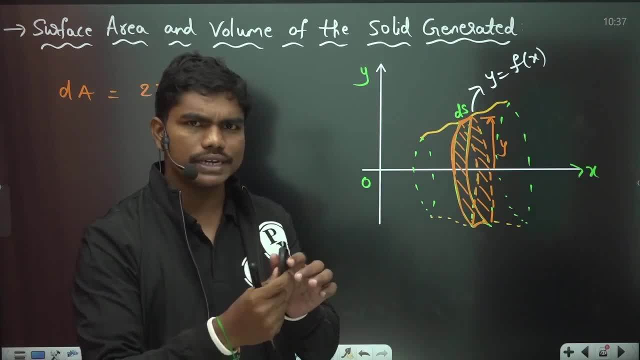 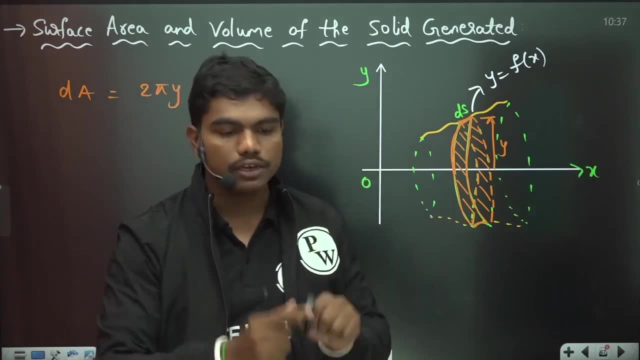 So, basically, if you want the surface area of this small disc, you need to multiply. this circumference means, basically, this perimeter. you need to multiply with this thickness ds, Then you'll get the surface area of this disc. okay, So this is how you'll get the surface area of this disc. 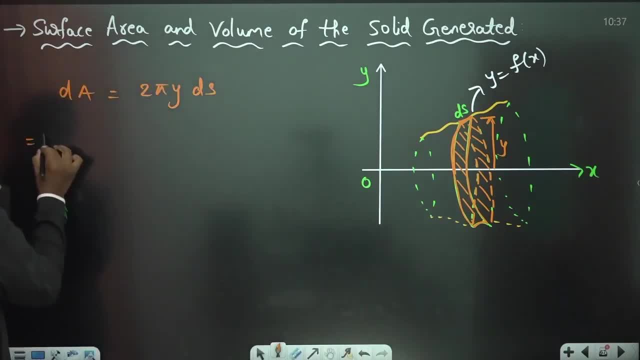 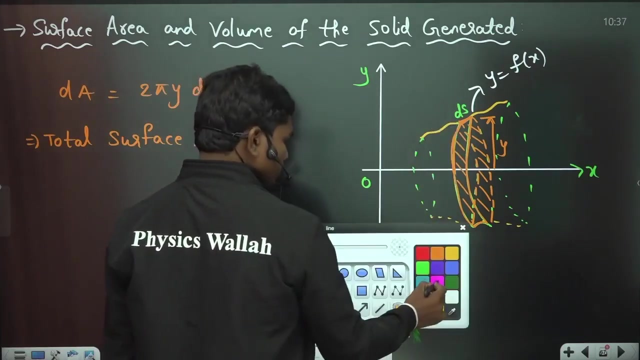 So two pi y into ds. So this implies total surface area. total surface area is equal to between: x is equal to a to x equal to b. If you take, let us suppose, if this coordinate you have taken, if this coordinate you have taken, x is equal to a. 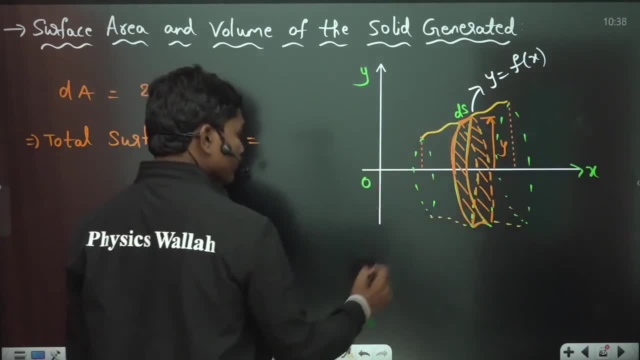 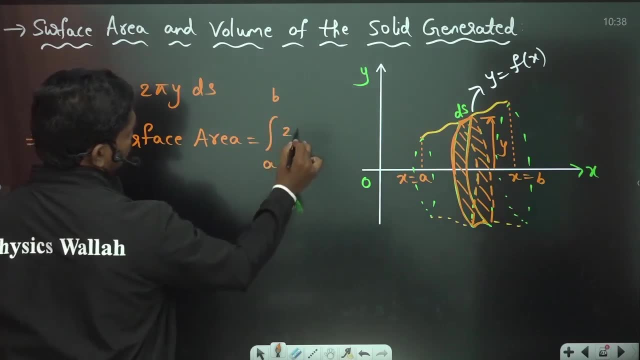 and if this coordinate you have taken, x is equal to b means basically the curve in between x is equal to a and x is equal to b, then this integration is integral: a to b, two pi, y, ds. okay, So this implies: 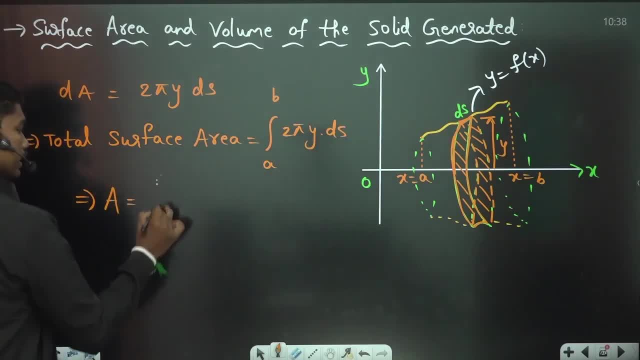 total surface area. a is equal to integral, a to b. two pi y into ds And ds is nothing but out of one plus dy by dx. whole square into dx. okay, So this is how you will get the surface area of any solid. 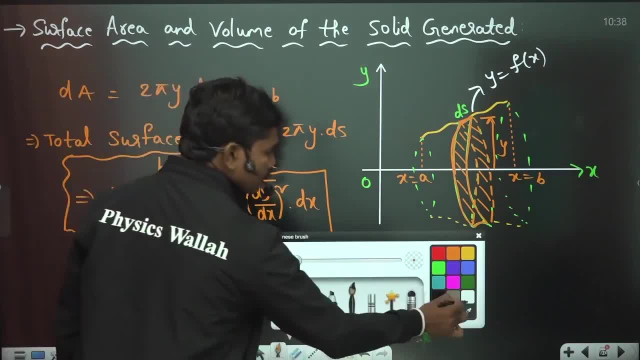 Surface area of any solid. okay, Now what about the volume? The same diagram. if you see volume, small elemental volume, dv is equal to: from this diagram if you want to calculate, dv is equal to: from this diagram if you want to calculate. 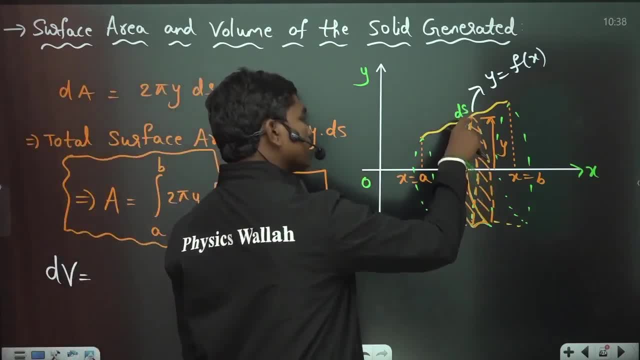 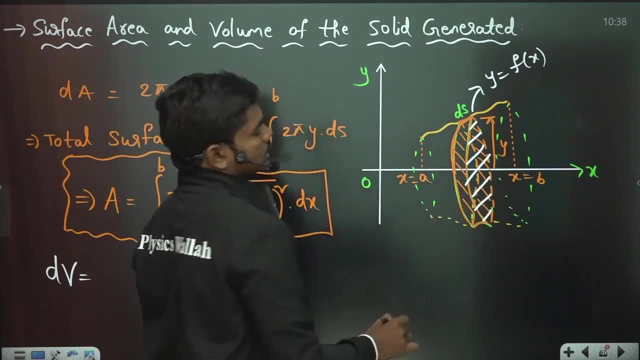 dv is equal to. from this diagram, if you want to calculate the volume of the disc instead of perimeter, you need to calculate the cross-sectional area, okay, So basically, in that case, this is the cross-sectional area of the disc. 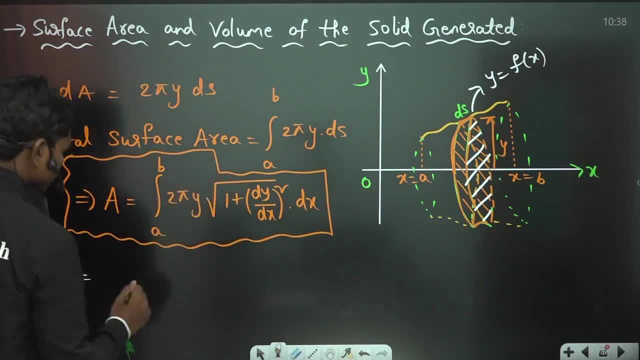 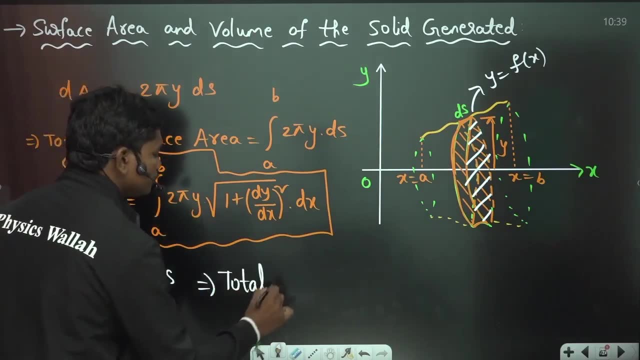 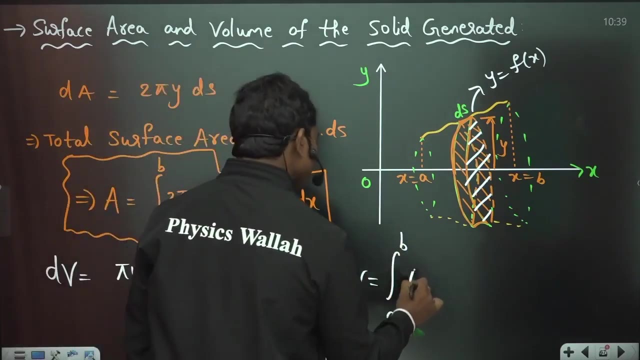 that cross-sectional area has to be multiplied with the thickness. So what is the cross-sectional area Circle? pi y square into ds, So this implies total volume v. total volume v is equal to integral a to b pi y square. So pi times of y square ds. 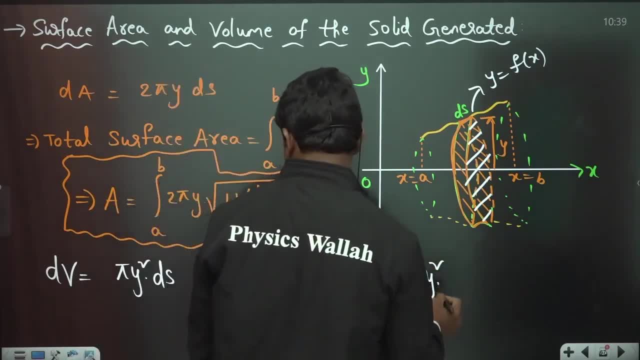 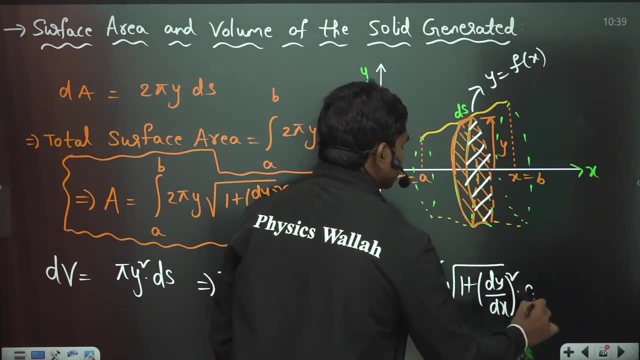 So pi times of y square into ds basically here. okay, So ds is out of one plus dy by dx, whole square into dx And generally, sometimes what you do, this dy by dx values will be very small When the curves are very flat. 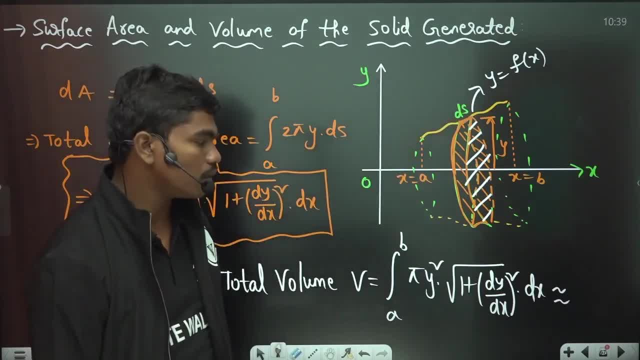 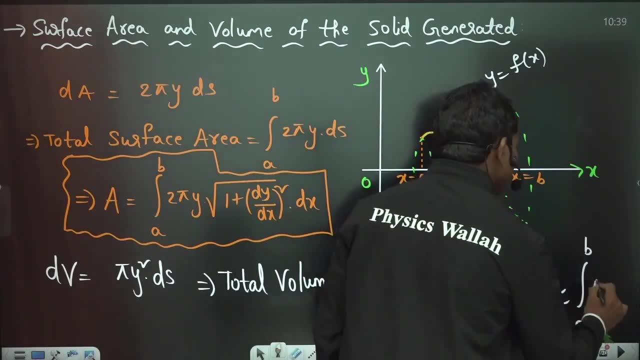 or with very little inclination, this dy by dx will be very small. So dy by dx, whole square will be much smaller. So in such cases you approximate this as integral a to b, pi, y, square, dx. okay, So this is what you have for the, okay. 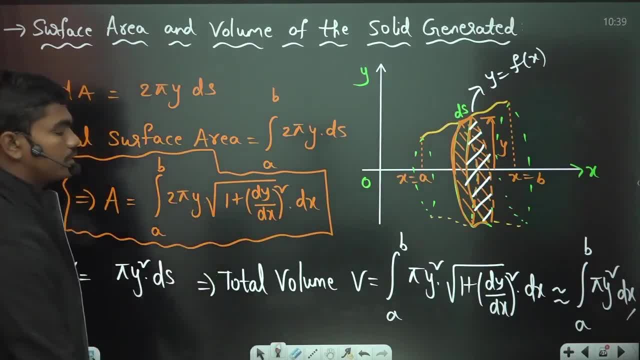 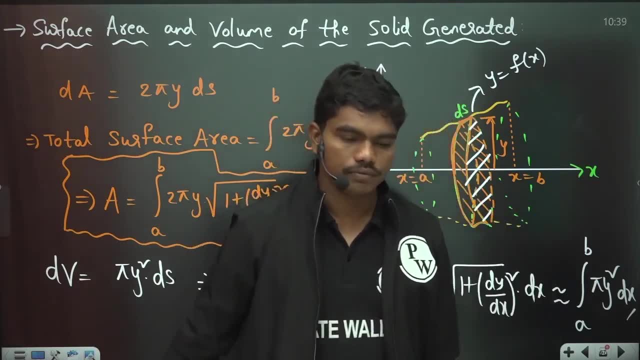 For the expression into the absolute volume And this is the expression to calculate the surface areas. okay, So this is how you calculate surface areas of solids and also you know volumes of the solids- actually clear. Now we have one last part. 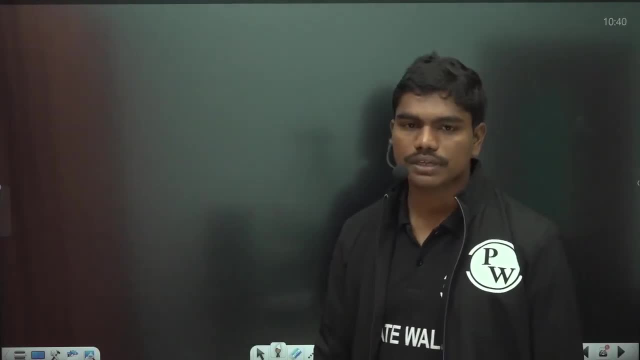 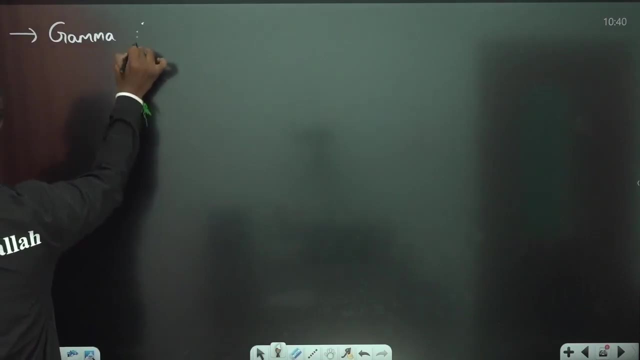 which is the gamma functions and the beta functions, Of course, something which is important at this level. So, if you see gamma functions basically Gamma function, So this gamma function basically. So this gamma function basically Gamma function, basically. 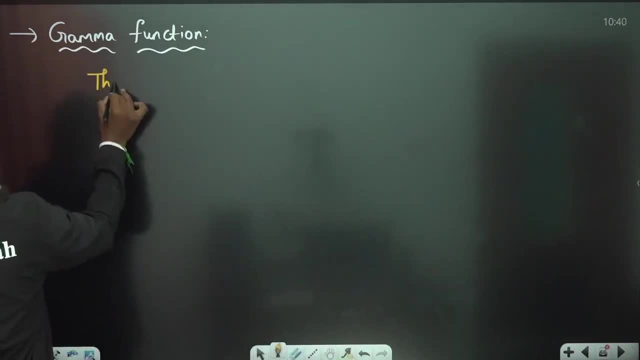 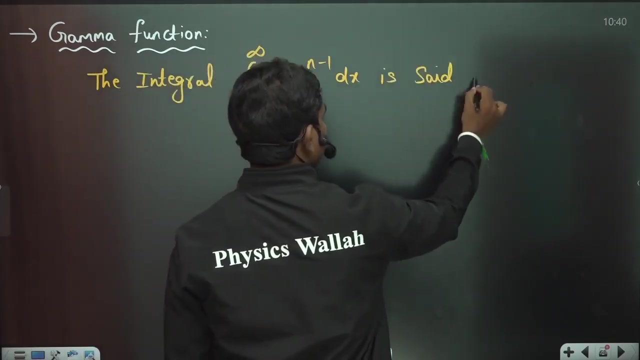 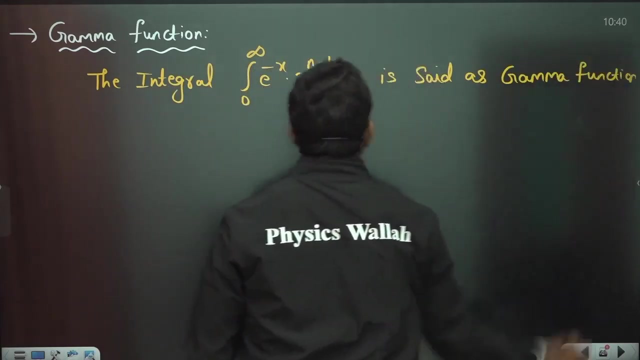 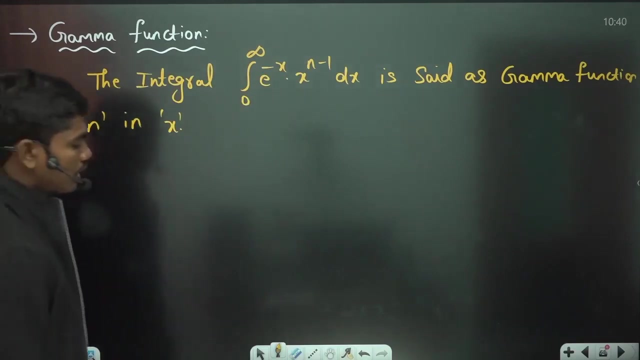 If you see this gamma function, So the integral, the integral Integral, zero to infinity, e power minus x into x power, n minus one, dx, is set as gamma function of n, Gamma function of n, gamma function of n in x in terms of x, actually. okay, so that's why it's called gamma function of n. it is denoted by: 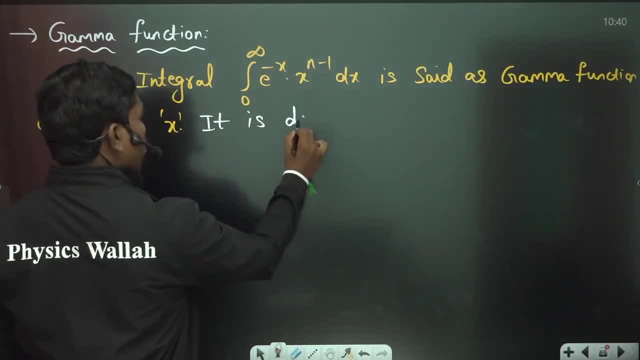 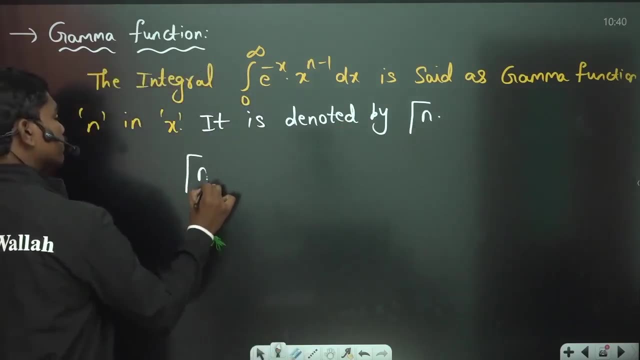 it is denoted by. it is denoted by gamma n. okay, so gamma n is equal to integral 0 to infinity e power minus x, into x to the power n minus 1 dx. okay, and if you see a few properties of this gamma function, properties of gamma function. 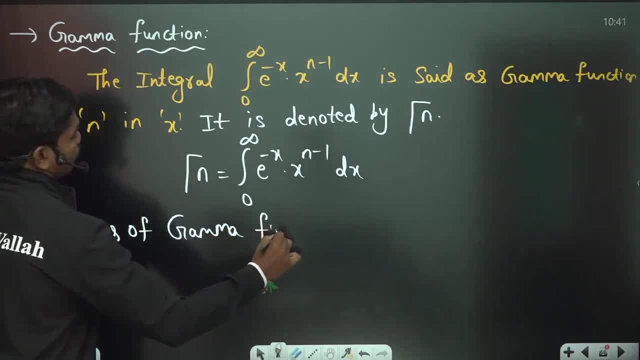 properties of gamma function. then if you say this: properties of gamma function first, if, of course, if n is integer, gamma of n plus 1 is nothing but n factorial. and of course you know factorials are defined only for positive integers. so definitely you can see gamma if n is. 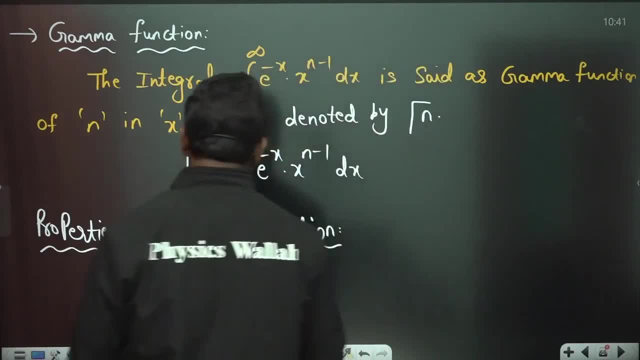 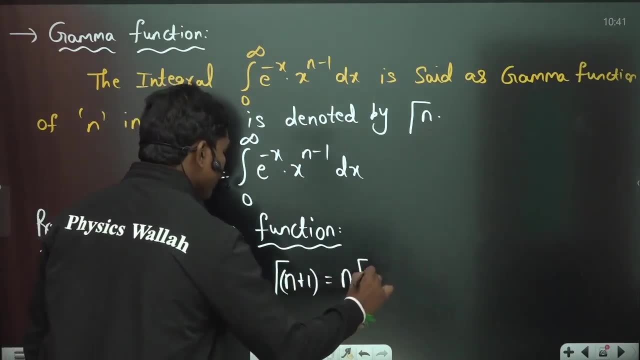 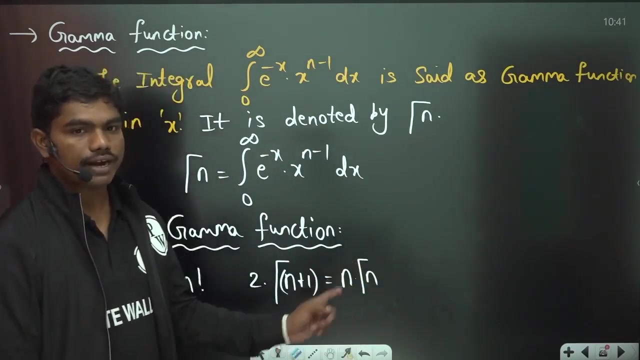 a positive integer. gamma of n plus one is equal to integral 0 to infinity, e power minus x minus n factorial and you can write this gamma of n plus 1 as n times of gamma n. actually okay. so basically n factorial can be written as n into n minus 1 factorial and that n minus 1 factorial. 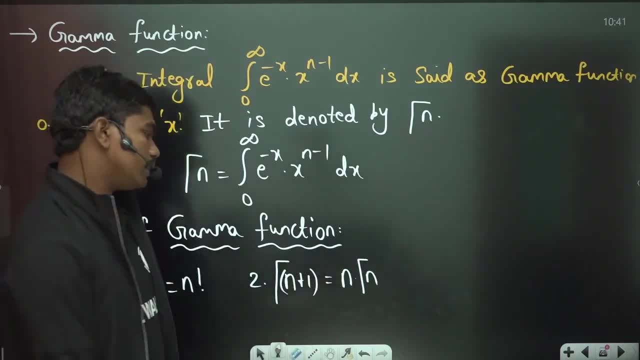 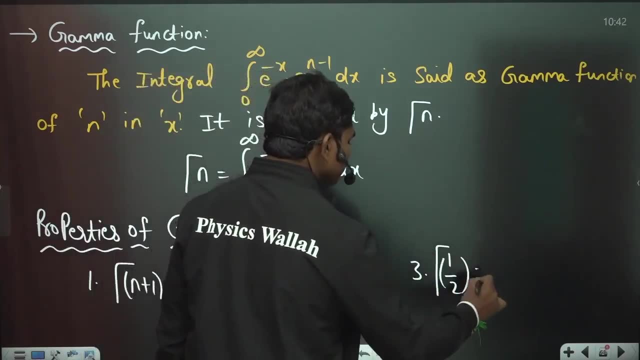 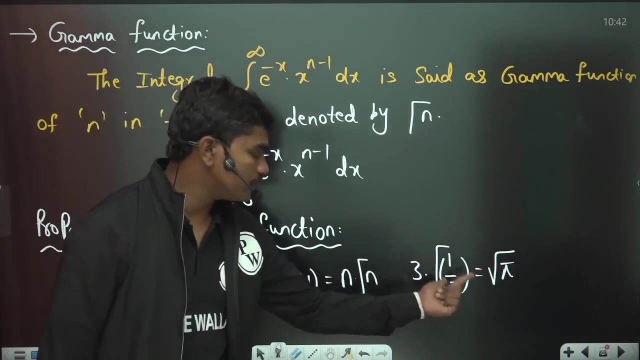 can be written as gamma n. actually okay. so gamma of n plus 1 is equal to n times of gamma n. third important property, which of course it's very not simple to prove, but you can take the result: gamma of 1 by 2 is equal to square root of pi. actually, okay. so this. it is very small to see, but actually. 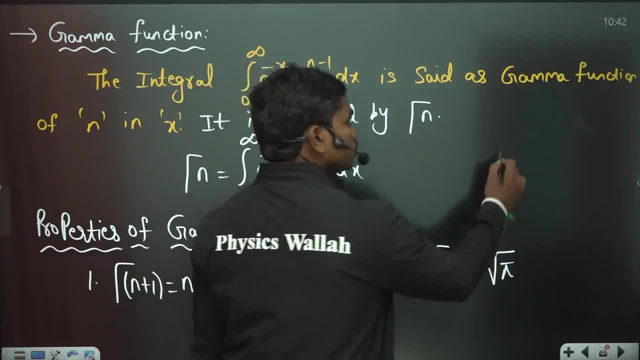 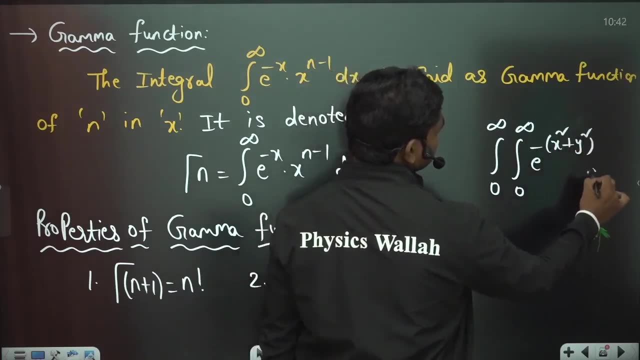 if you want to calculate this, if i want to show you this result, i should consider this thing: integral: 0 to infinity. 0 to infinity. e power minus x square plus y square, dx, dy. this is the integration which i need to do to tell you, or to prove you that, how gamma of 1 by 2 is equal to. 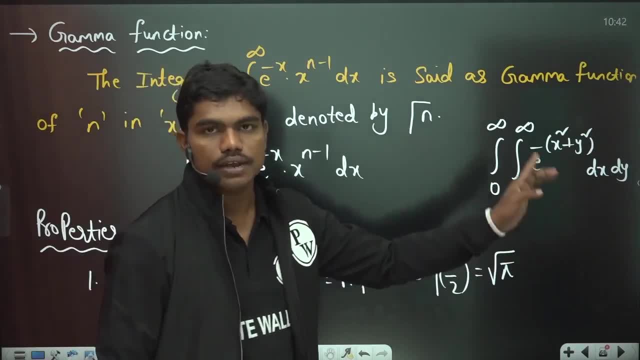 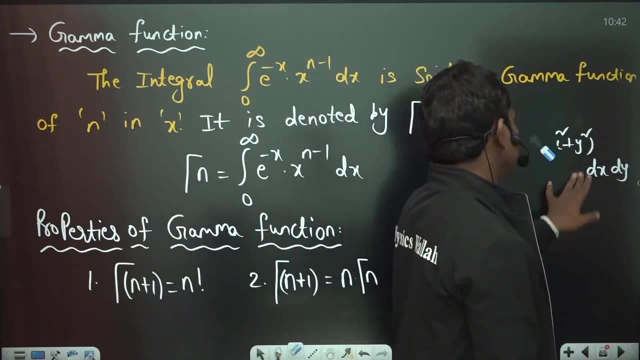 root pi that is a multiple integral and that do not very simple integral. so that's why we'll see that in the next lecture, that when we talk about multi variable calculations, okay, so anyhow, right now this is not the importance, but and also fourth property that i 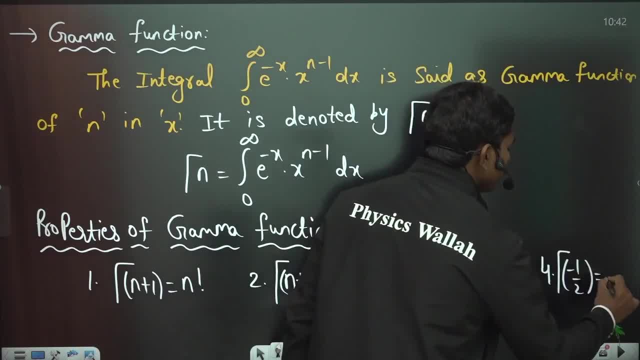 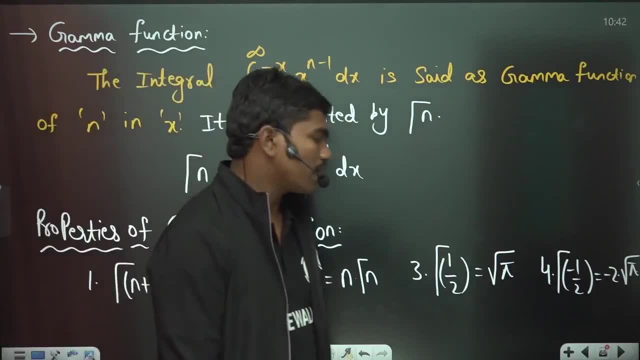 would like to give you: gamma of minus 1 by 2 is equal to minus 2 times of square root pi. okay, so all these are four properties are very important properties for this gamma function. so gamma of minus 1 by 2 is minus 2 times of square root of pi. if you can assume this, i can show that very 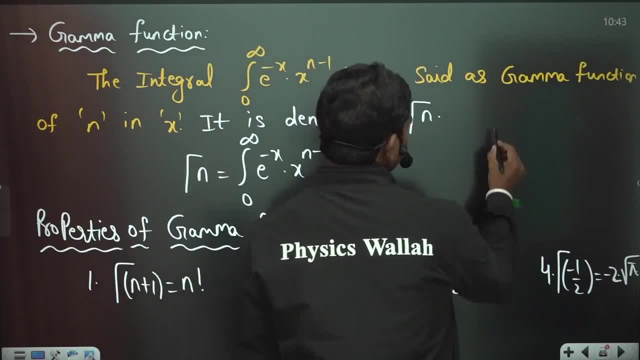 easily because if you see, gamma of n plus 1 is n into n plus 1 is equal to n times of square root of pi. so if you put n is equal to minus 1 by 2, minus 1 by 2 plus 1, 1 by 2 is equal to minus 1 by 2. 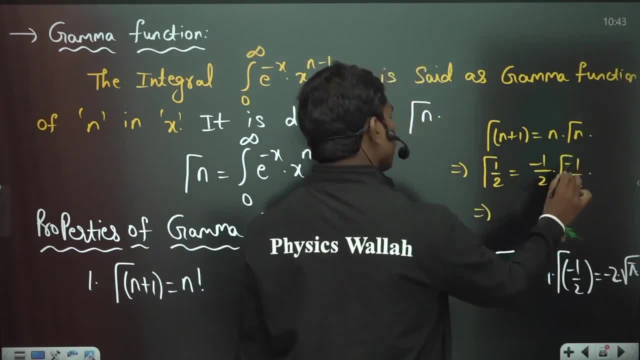 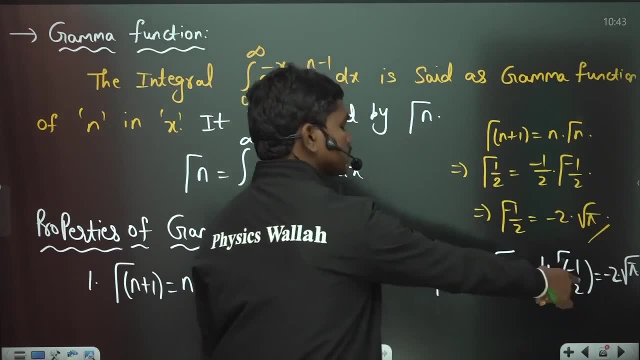 into gamma of minus 1 by 2. so this implies gamma of minus 1 by 2 is equal to minus 2 times. gamma of 1 by 2 is root pi. that's how i can show you this result very easily, if you can accept this. 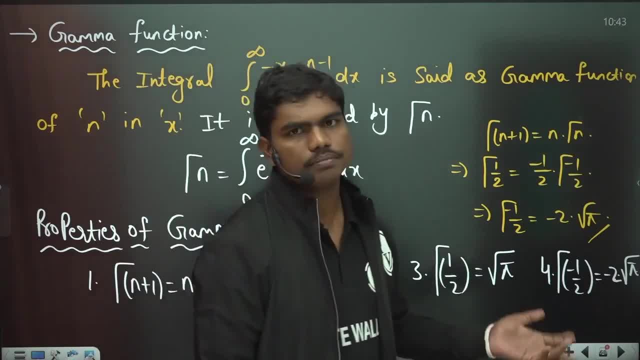 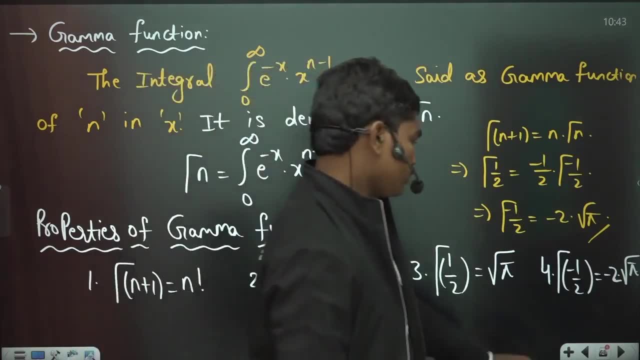 okay, so these are the general- uh, you know, for general important properties of gamma function. so sometimes they give you values like this and they'll ask you for the answer. so i'm going to ask you, okay. so look, they i'll give example of one gamma value. so let us suppose, if they ask you, 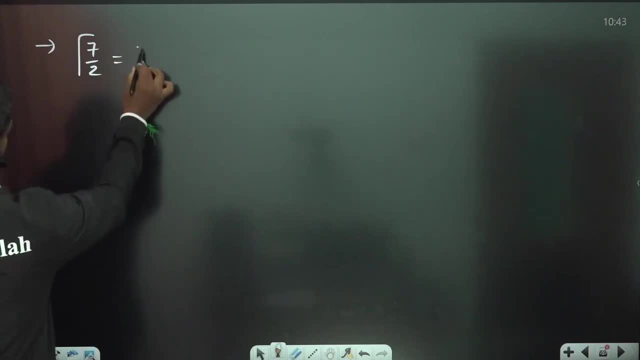 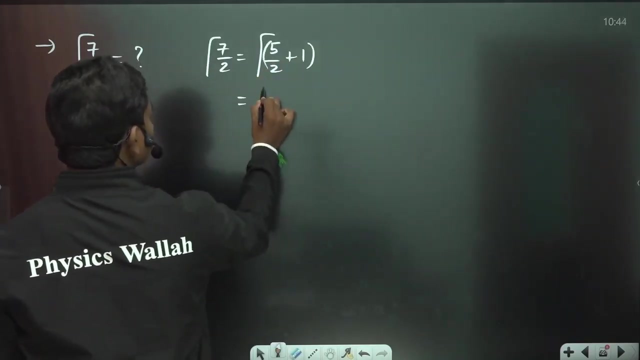 what is gamma of 7 by 2, for example? anyhow, if there are integers, you will solve. but let us suppose if they give you gamma of 7 by 2, for example, how to go for this? okay, so gamma of 7 by 2 is equal to gamma of 5 by 2 plus 1. you can write this: so this is n plus 1, so n into gamma n. 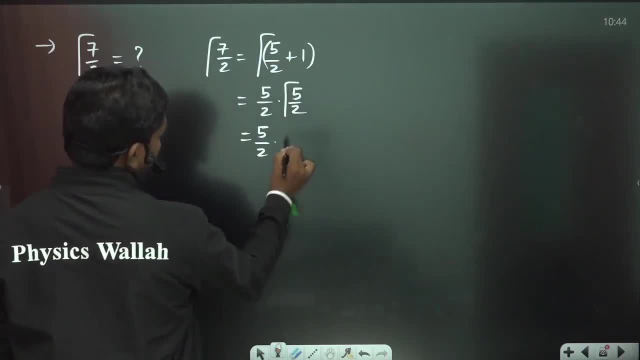 so this can written as: 5 by 2 into gamma of 3 by 2 plus 1, so this is 5 by 2 into 3 by 2 times gamma 3 by 2, so this is equal to 5 by 2 times of 3 by 2 into gamma of 1 by 2 plus 1. so this can be written as 5 by 2 times 3 by 2. 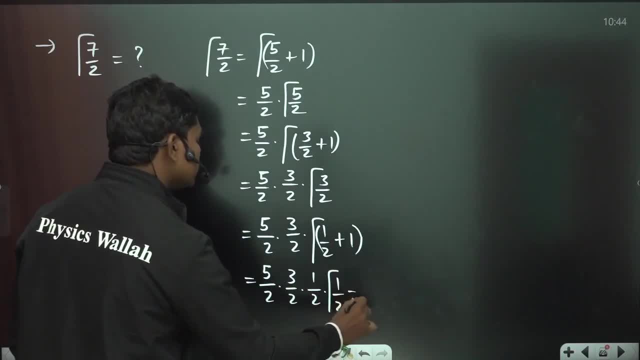 into 1 by 2 times gamma 1 by 2. so this is this: gamma 1 by 2 is square root of pi. so 15 by 8, 15 by 8, into square root of pi. this is how you calculate gamma of 7 by 2 value with this succession. okay, and one last thing before we close this. 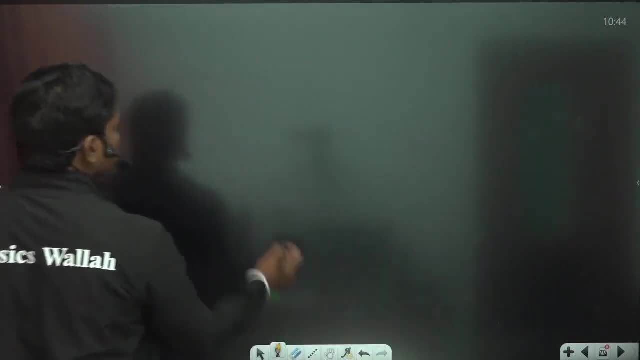 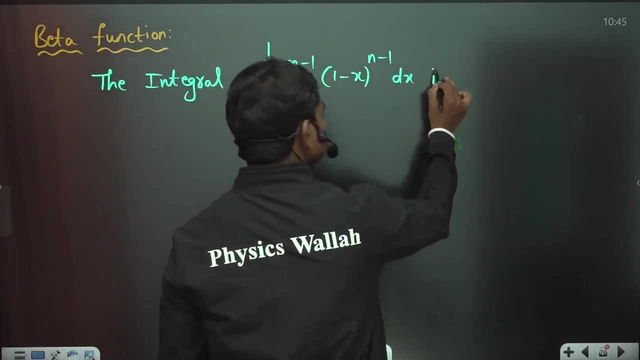 lecture is beta functions. okay, so this beta functions is also again such an important thing. so beta function, beta function, actually beta function. so if you see, the integral beta function means basically beta function is also integral. the integral integral 0 to 1, X power m minus 1 into 1 minus X, whole power n minus 1, DX is said to be beta. 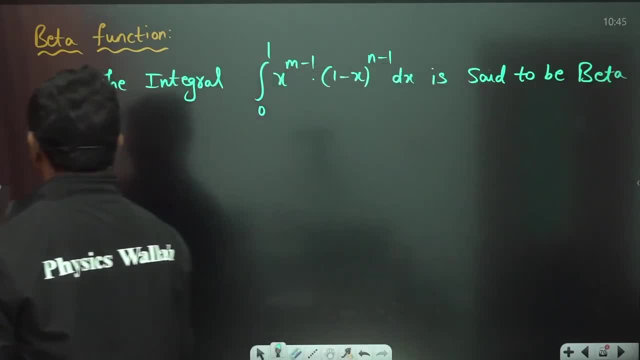 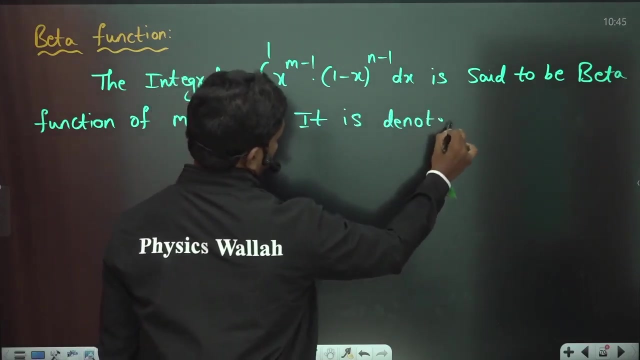 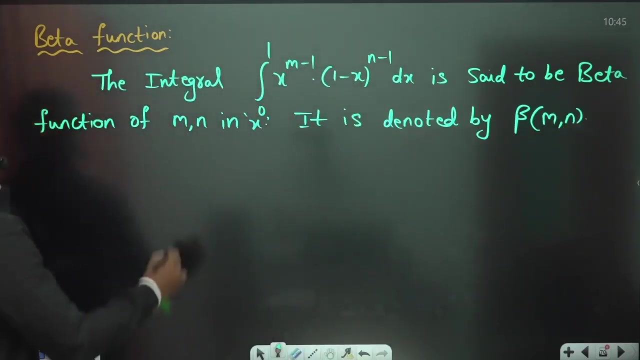 function, beta function of m comma n in X. actually, okay, and it is denoted by. it is denoted by. it is is denoted by beta of m comma n. okay, so it is denoted by beta of m comma n, and beta of m comma n is equal to gamma times m into gamma times n divided by gamma of m plus n. actually here, okay, 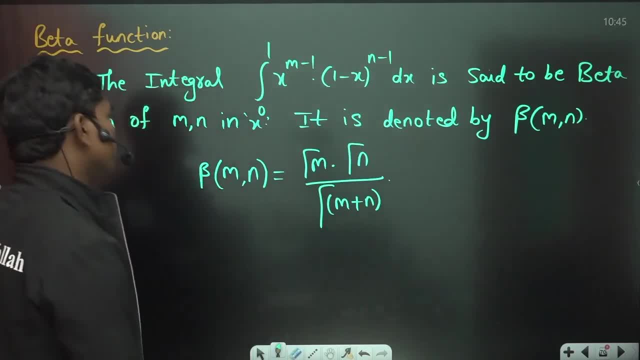 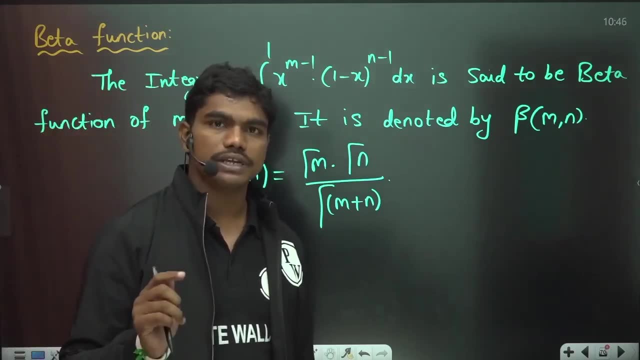 so this is how the beta functions are calculated, basically. so whenever i give you certain integrals- integral 0 to 1 x power 5 into 1 minus x whole power 6, dx, when you assume 1 minus x is equal to t, again x gets converted to 1 plus t whole power 5. then you know things are not very easy, but using 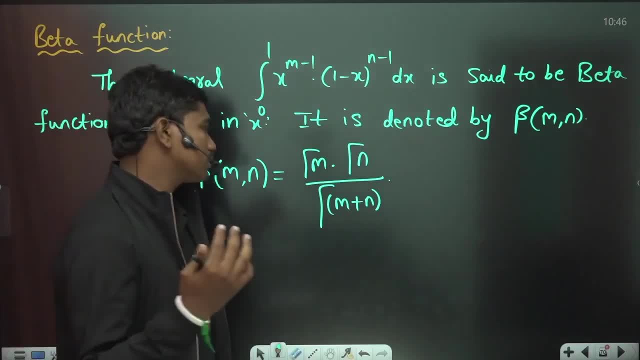 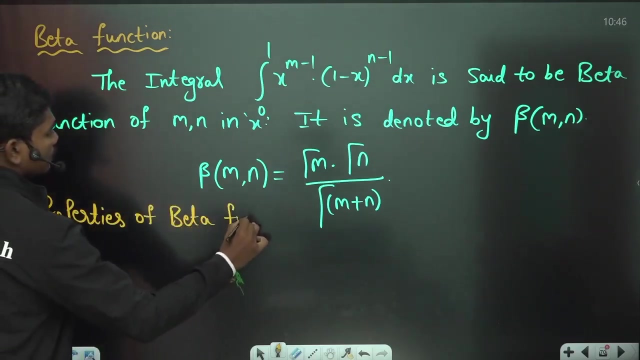 this gamma function. you can easily sort out the things, okay, so this is about the gamma, the beta function, and this beta function has also got some properties, that properties of beta function. so if you take this properties of beta function, so properties of beta function- if you take v, you will get like this first function. 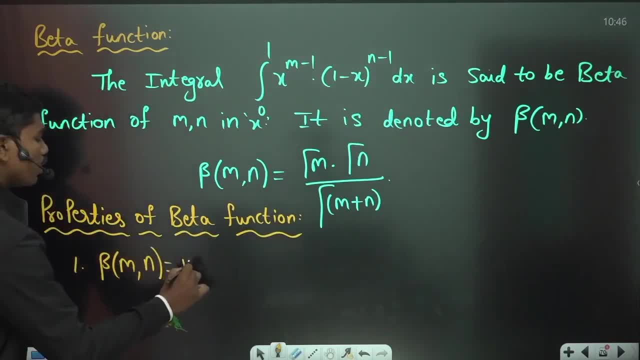 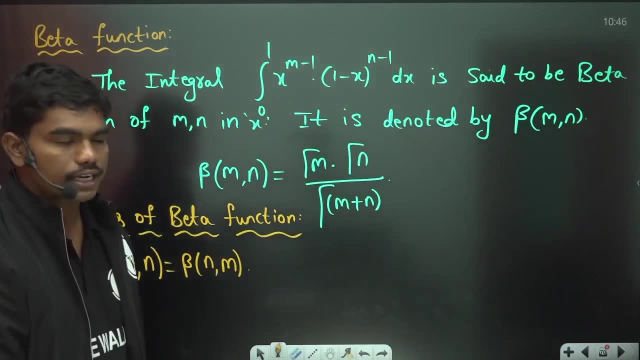 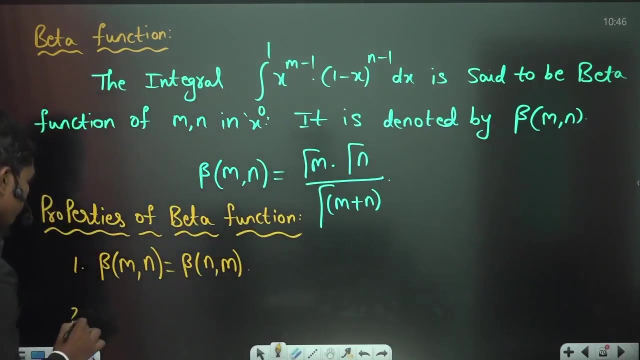 beta of m comma n is same as beta of n comma m. okay, so means basically, if you replace this m and n values, still the result remains the same. you can check it out by putting 1 minus x is equal to t and changing the limits of integration. you will again get same beta of m comma n. okay, and second property: 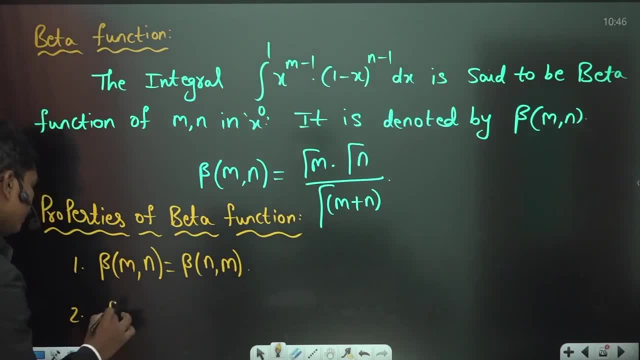 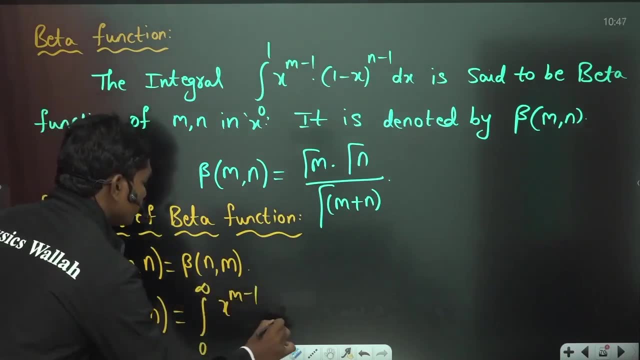 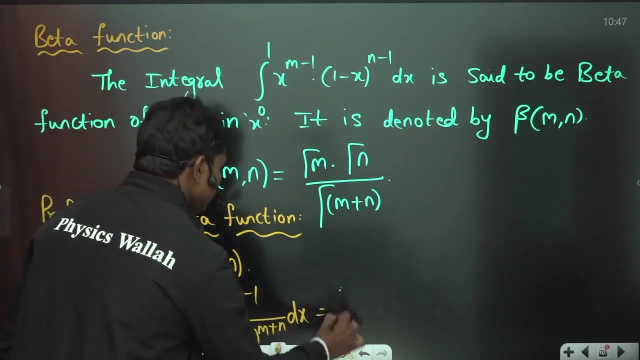 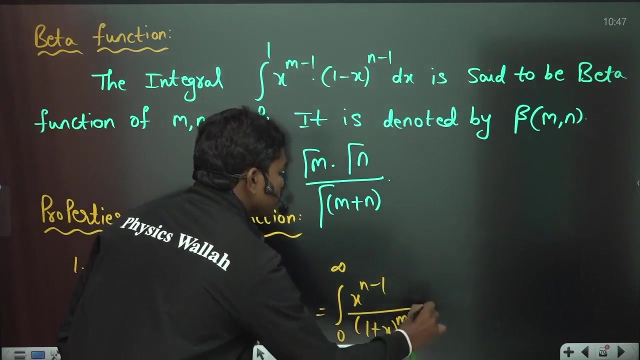 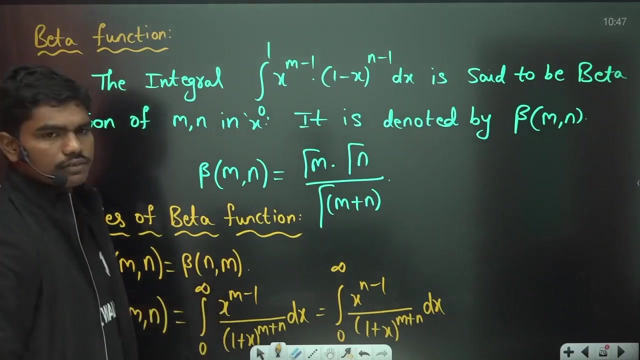 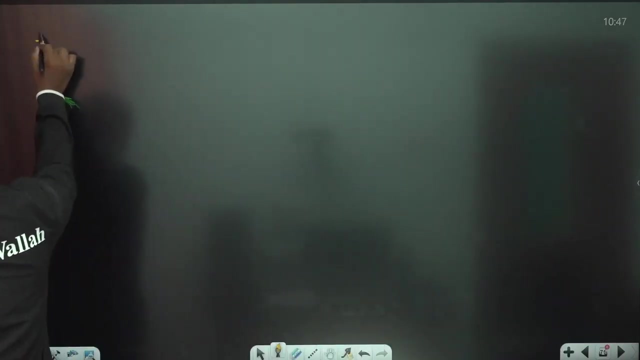 is beta of m, comma n can be written as integral 0 to infinity x power m minus 1 divided by 1 plus x whole power m plus n? dx, which is, of course, same as integral 0 to infinity x power n minus 1 divided by 1 plus x whole power m plus n? dx. okay, so these are again some very good properties that could, by putting x is equal to 1 plus x is equal to t and all these substitutions, you can generate those results, okay. and one last property that i would like to give here is integral 0 to pi by 2 sine power m plus n dx, which is, of course, same as integral 0 to infinity x power n minus 1 divided by 1 plus x whole power m plus n dx. okay, so these are again some very good properties that could, by putting x is equal to 1 plus x is equal to t and all these substitutions, you can generate those results, okay. and one last property that i would like to give here is integral 0 to pi by 2 sine power m plus n? dx, which is, of course, same as integral 0 to infinity x power n minus 1 divided by 1 plus x whole power m plus n dx. okay, so these are again some very good properties that could, by putting x is equal to 1 plus. 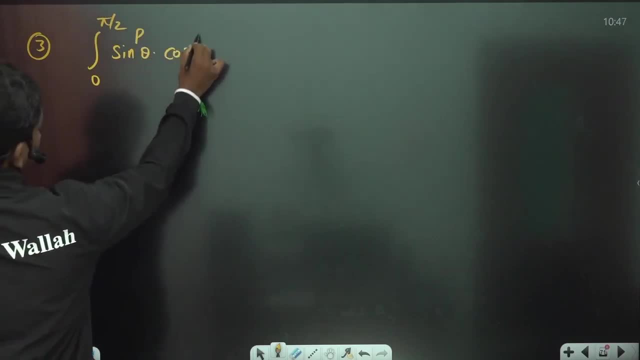 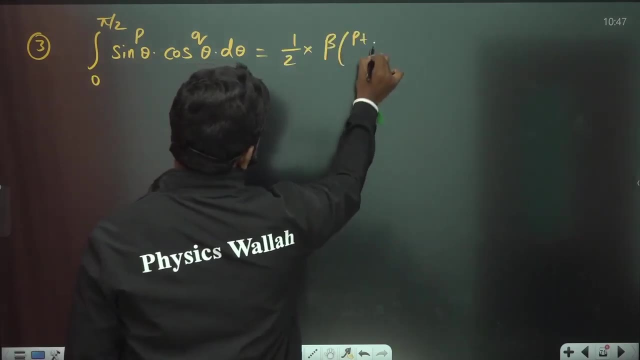 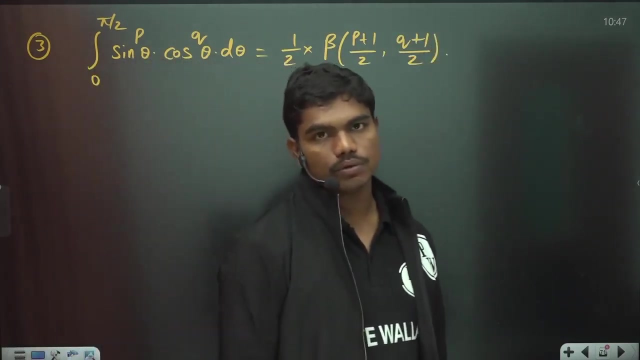 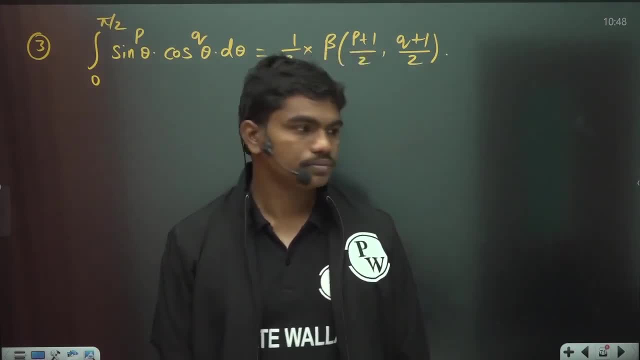 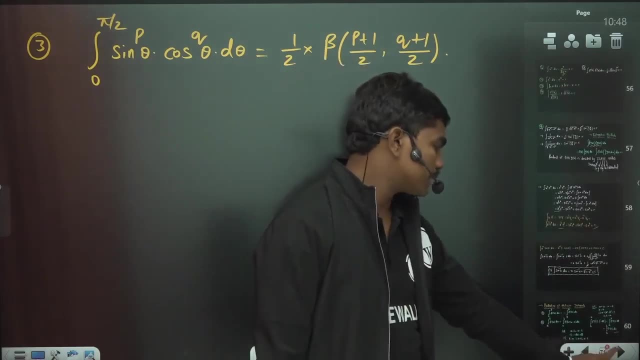 you will be able to solve the integrals slightly easier. okay, so with this, almost some 71 pages of notes. i think we got some hectic notes, but yeah, basically these are some good properties of this: definite integrals and all these things. okay, so with this we conclude this video on basic calculus. 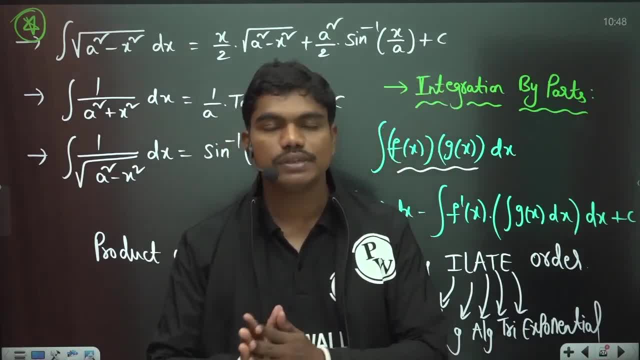 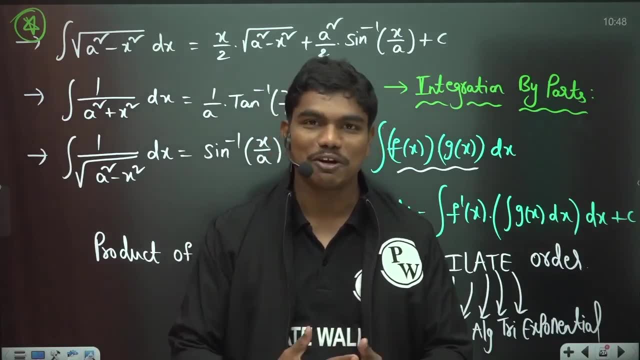 of single variable, okay, and basic calculus of multi variables we'll look in the next video because calculus is a very vast, you know, subject which cannot be, uh, to be honest, we cannot deal in one single video or like that, so we'll split that. so in this video we talked about single.